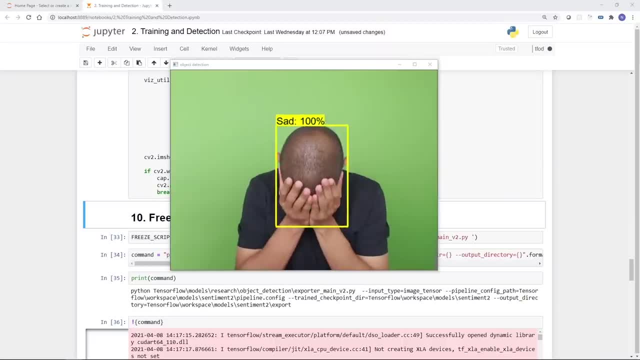 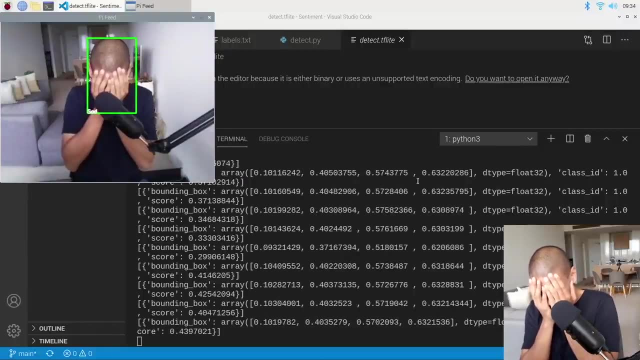 and tense flow object detection. Now again, this could be used in a whole different range of use cases. to say, for example, you want to detect a person's face, or if you want it to do sign language detection or face mask detection, you want to do face mask detection, you want to do. 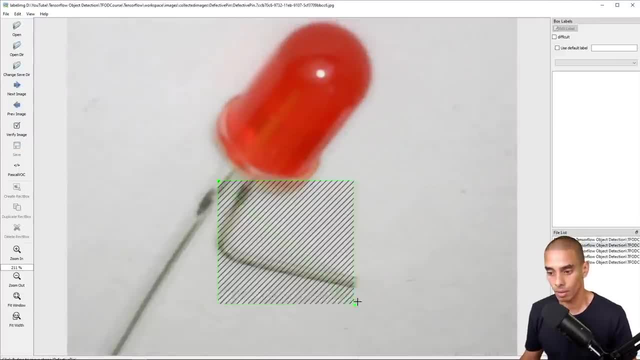 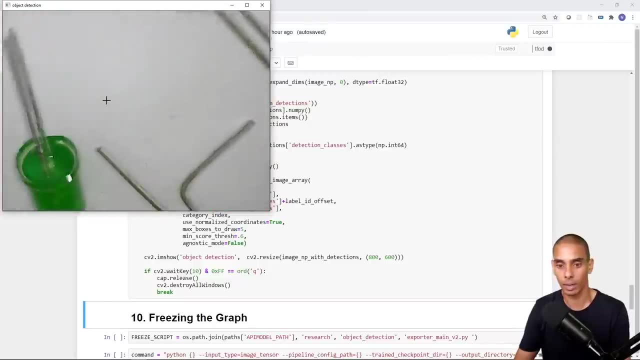 face mask detection. This is the exact same code that you can use. Now. the nice thing about this as well is that we'll go through all of the setup. All of the installation will show training. We'll also show exporting, which is a really big part of being able to build object detection models. 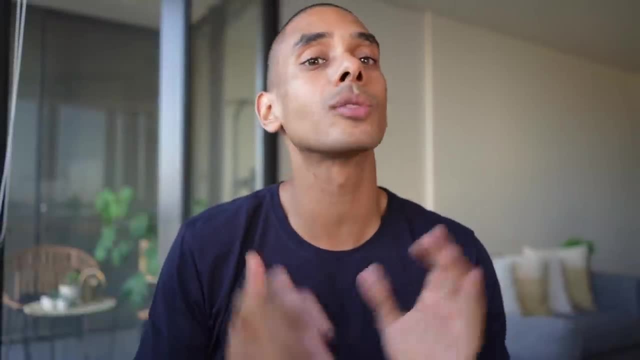 So we'll be able to export this to the tense flow JS format as well as TF light. So if you wanted to run it as part of a web app, or if you wanted to even use it on a Raspberry Pi, you could. 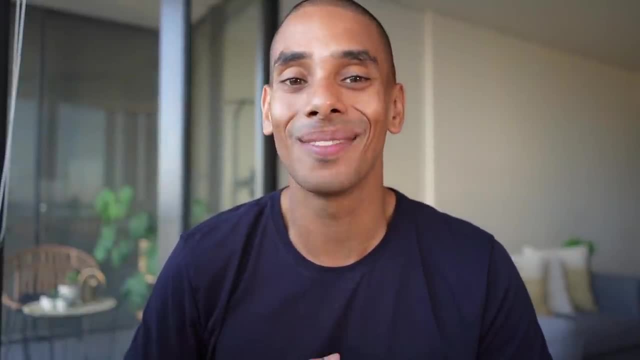 and we might just do that in one of our projects towards the end of the tutorial. So, without further ado, let's get started. So let's get started. So let's get started. So let's get started Without further ado. ready to do it, Let's get to it. 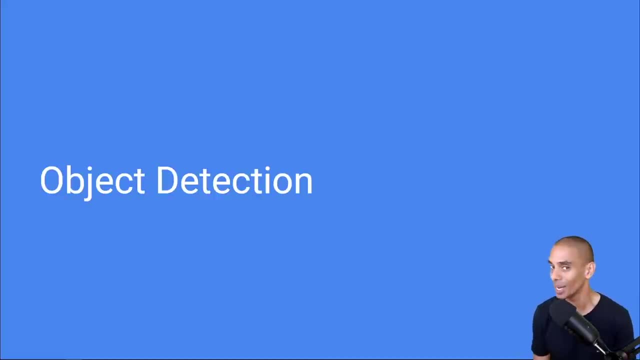 Alrighty, what's happening, guys? welcome to the object detection course. Now, this course is intended to take you from being a complete beginner when it comes to object detection all the way to being fully proficient and acting as a practitioner. Now, again, we're going to take 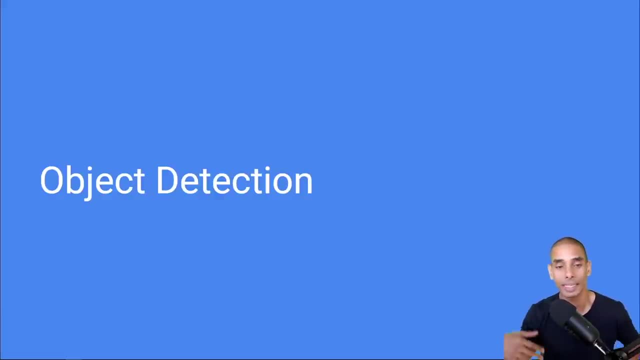 this step by step, so you'll be able to walk through at your own pace and be able to learn and leverage the technologies. So let's take a look as to what our actual game plan is for this. Now, there's going to be a bunch of stuff that we're going to go through, So, ideally, this course is: 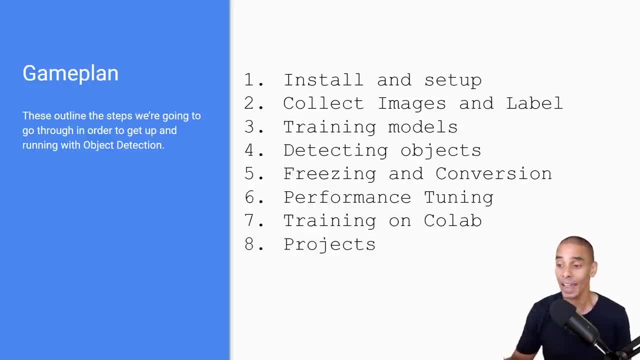 going to be fully comprehensive, So you're going to need every or you're going to have everything that you need to be able to get up and running. So there's eight key parts that we're actually going to go through, And each of these key parts are pretty important when it comes to building. 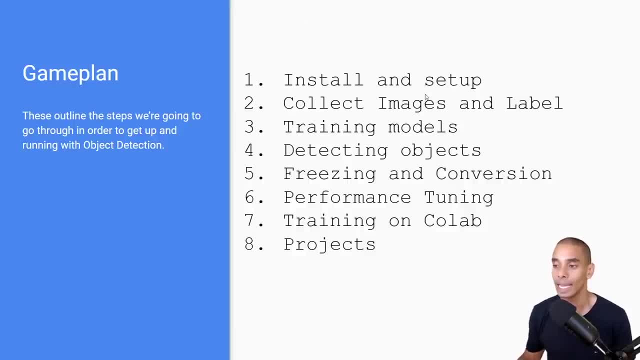 object detection models. So, first up, what we're going to do is we're going to install and set up everything that we need to be able to perform object detection on our local machine or PC. Now, in this case, we're going to be using the TensorFlow object detection. 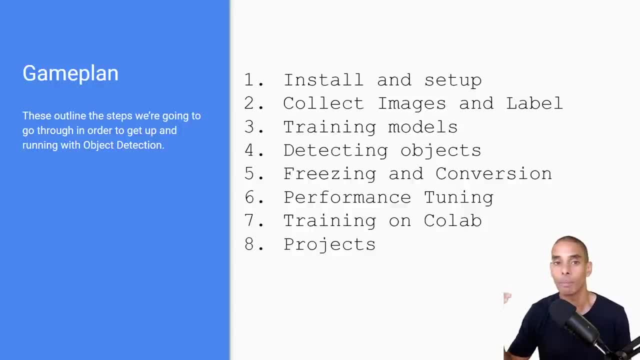 API, And we're going to be doing that mainly using Python. Now, the reason that we're using the TensorFlow object detection API is that it has a whole bunch of additional capabilities that make it a whole heap easier to be able to build object detection models. So if you've ever 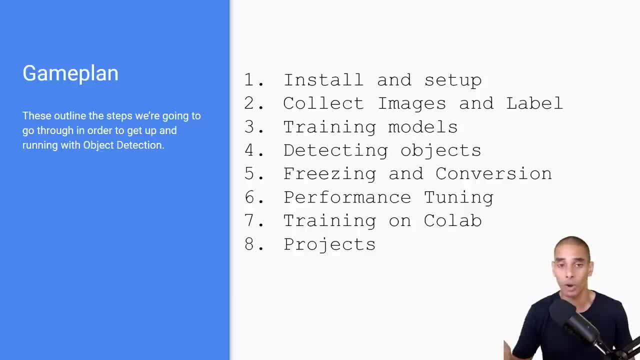 looked at a real time object detection architecture or model before. there is a bunch of stuff that you actually need to build in order to actually get one of these up and running. There's pre processing steps, there's post processing steps, there's visualization utilities. 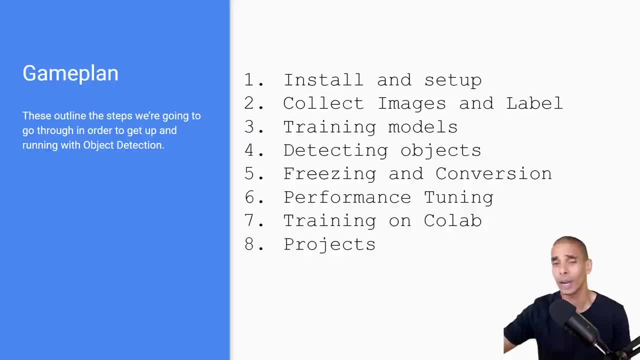 and again, if you're not familiar with any of these terms, don't fret, we're actually going to take a step by step and walk through each of those components. Just know that building this from scratch takes a lot of effort, So using TensorFlow object detection speeds this up a whole. 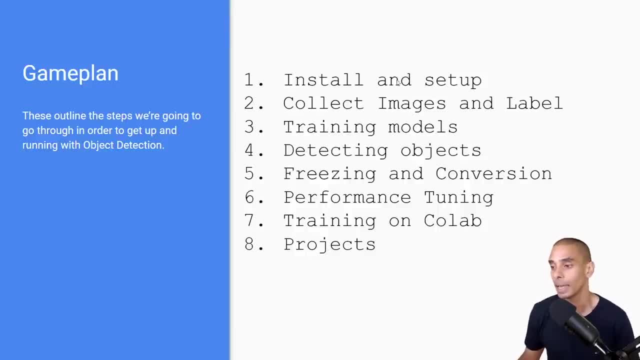 heap. So what we're going to do is we're going to install and set up the TensorFlow object detection API. Then what we're going to do is we're going to collect images and label them. So, in order to do that, we're going to be leveraging our webcam. So we'll leverage our webcam to be able to do a. 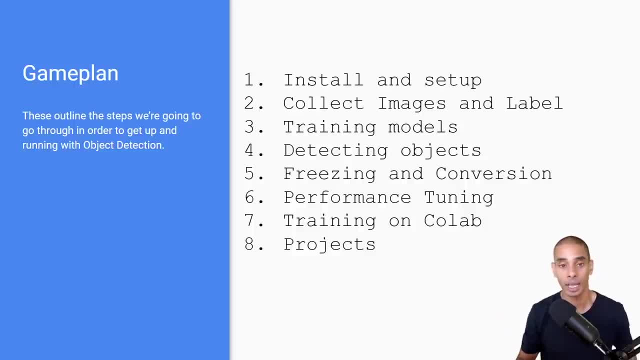 whole bunch of images to be able to label our objects. Now you're probably thinking, Nick, what the hell is labeling? Well, ideally, what you want to do when you're building an object detection model is you want to be able to label or identify the objects that you want to try to. 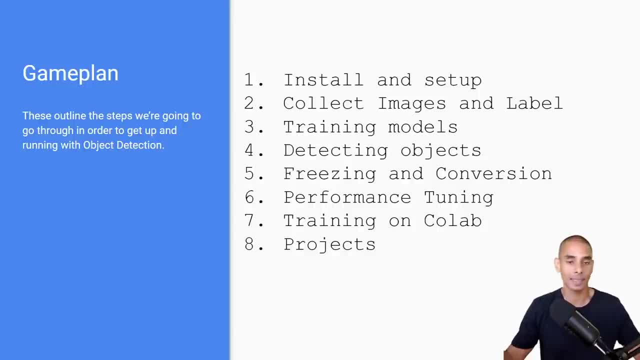 detect. Let's say, for example, we were building a face detection model. Well, I might use my webcam to take photos of myself and then draw a label around my face, So that what I'll then do is I'll take that trained image or that image which has been labeled and I'll leave it there, And then I'll. 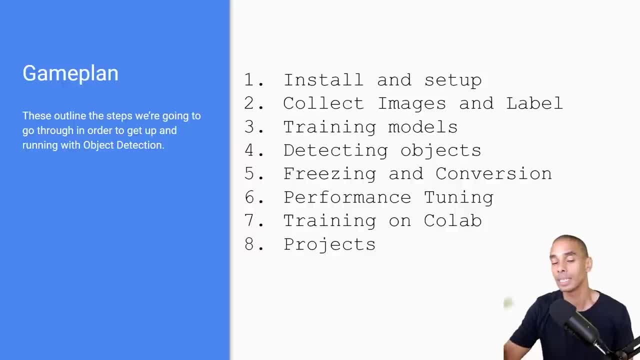 leverage that in my trained object detection model to be able to detect that in the future. That brings us to our next step: training the model. So again, we're going to be using the TensorFlow object detection API And we're going to be passing through both our images. 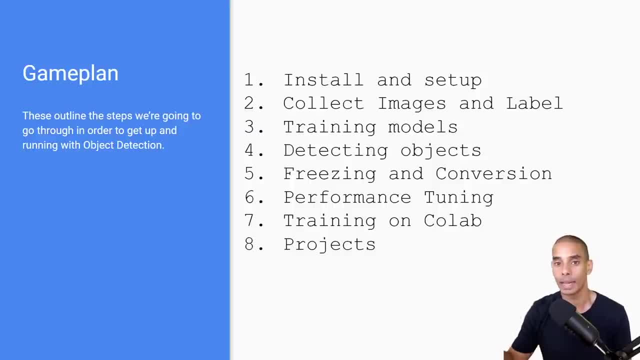 and our labels or annotations to be able to train this model. Now there's a whole bunch of different types of models that you can actually leverage there, And there's a bunch available through the TensorFlow object detection API, So we're going to be using a mobile 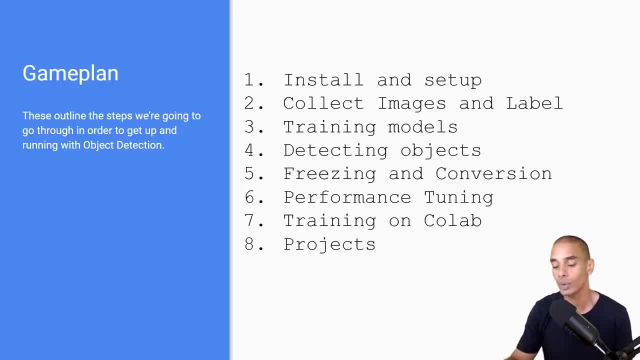 net architecture, But again, I'll talk about that a little bit more once we get to it. So we're going to be training that model initially and we'll be able to leverage that throughout the process. Now, if you're not sure what training is, so when it comes to traditional programming, 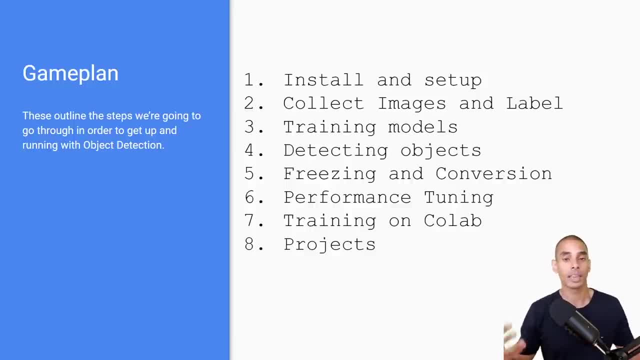 you typically have data plus rules. So think of your data as the feed that you're effectively getting and then you pass it through some rules or some logic to be able to get answers or an outcome right. So say, for example, you get somebody sets a color variable, for example. 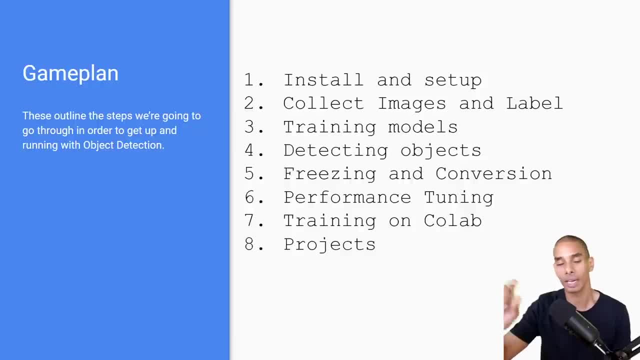 So the color is red. you might then take that variable and go: if the color is red, then do x, if the color is not red, then do y, So that if statement, think of those as those rules And effectively what you're doing in that action is your intended consequence. Now, 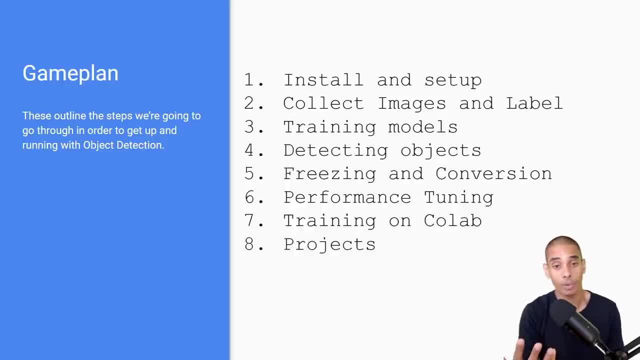 when we actually train a deep learning model or object detection model in this case, we're not actually specifying those rules explicitly upfront. This is the beauty of machine learning and deep learning. So, rather than defining those rules and defining what to look for in the data, we're actually going to do it the other way around, And this is normal when it comes. 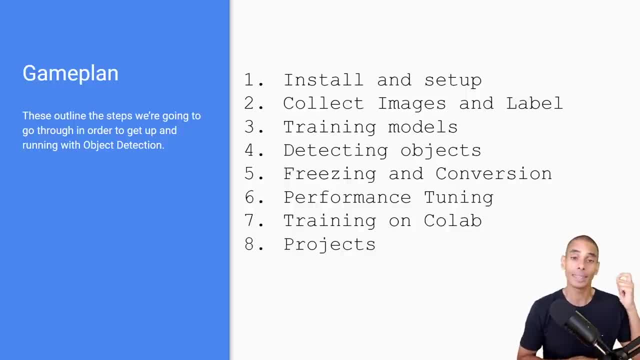 to machine learning, We're going to give it data plus answers. So our data is our image and our answers are our labels or annotations. And we're going to train our object detection model to learn the rules to be able to detect faces. So machine learning sort of flips traditional programming on. 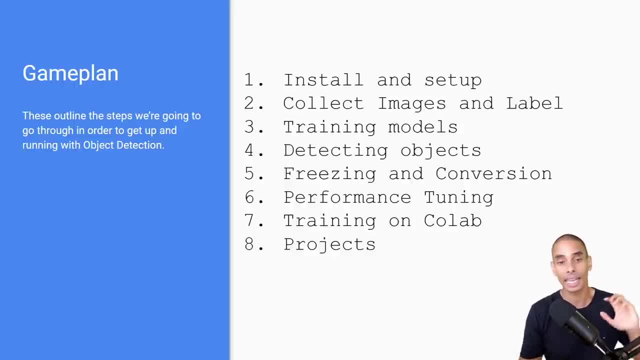 its head. So, rather than starting off with data and rules and getting answers, we're starting off with data and answers to get rules. So it's a slightly different paradigm, but it ideally gives you a really cool output. So, once we've trained our model, what we're then going to do is we're 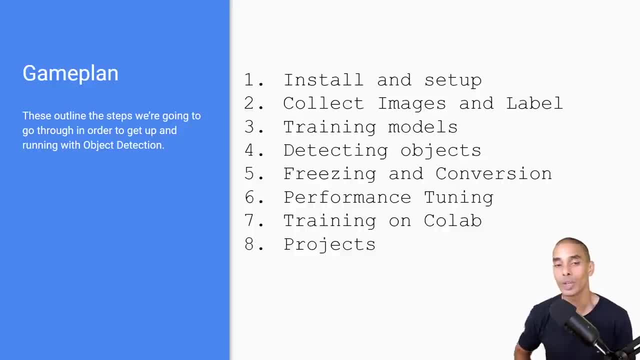 then going to start detecting some objects. Now we're going to do this in two different ways. So we're actually going to detect an object using an image. So say, for example, you had an image and you wanted to be able to detect different objects in that image. we're going to be able to do that. 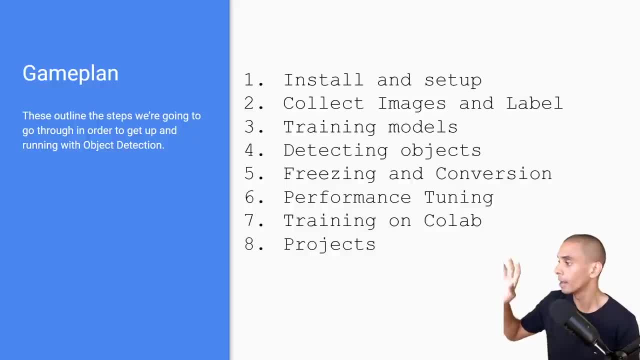 So this is normally known as static detection. So you're going to be grabbing a particular object from over there or over there, and being able to grab that image, pass it through to our model and detect an object, But then we're going to be able to do that in a different way, So we're going to 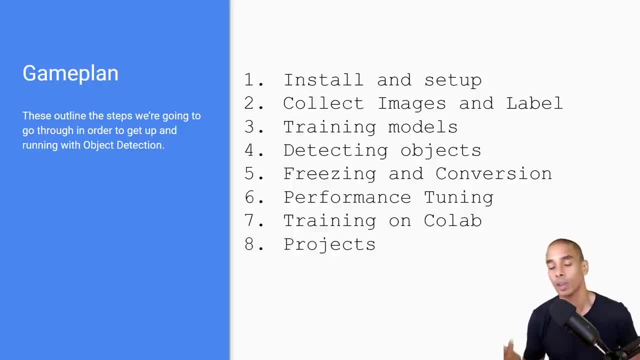 be able to do that in a different way. So we're going to be able to do that in a different way. So, then, where I think the real good bit is is being able to detect objects in real time, So we'll be able to take our webcam, face it towards a particular frame or a particular thing. 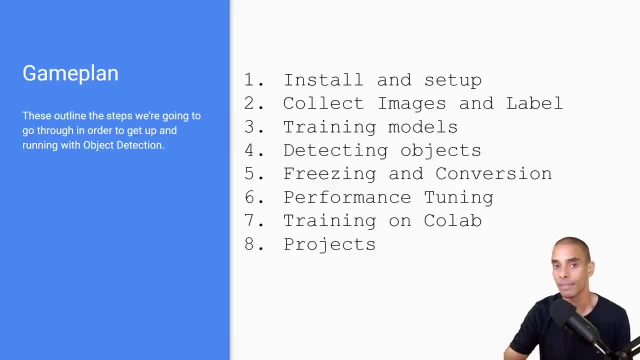 and we'll actually be able to detect objects using a real time feed. Now, the beauty of this, and particularly the beauty of the model that we picked in step three, which is a mobile net model, is that it's going to be super fast, So we'll be able to detect objects in real time when we've 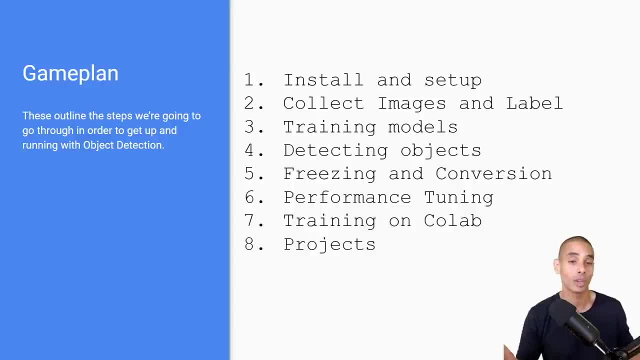 got a computer or a GPU powered machine and we'll be able to detect those objects in real time. So we can do a lot with that because it is fast. Now normally there's a trade off between speed and accuracy, But again we'll talk about that in performance tuning, Alright, so in detecting, 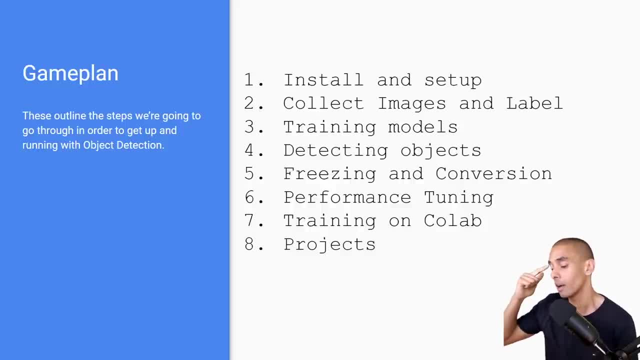 objects. we're going to detect stuff with an image And we're also going to detect stuff using a real time video feed. Then what we're going to do is we're going to learn how to freeze and convert our model. So, whenever you're building models, ideally what you want to be able to do- 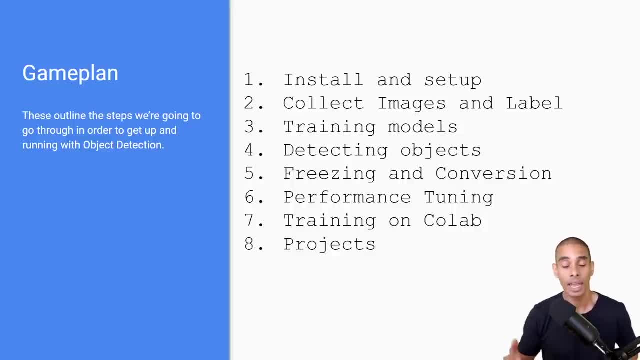 is: save down that model and maybe give it to somebody else. So if you're part of a software engineering team and you're the data scientist, what you might want to do is you might want to export your train detection model, pass it through to your software development engineers or your 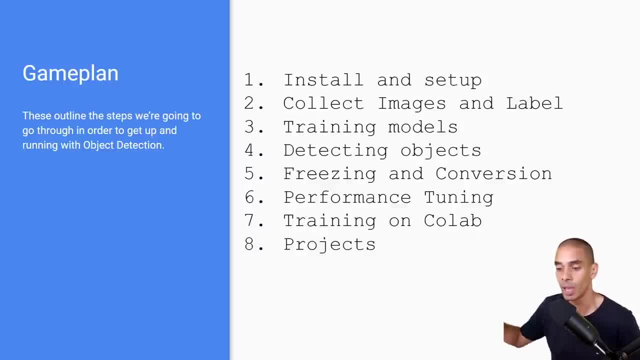 machine learning engineers to then be able to go and deploy that model. This is where freezing and conversion comes into play. Now again, with TensorFlow object detection, you're able to freeze down your model. think of freezing as saving it, And then, if you wanted to, you can. 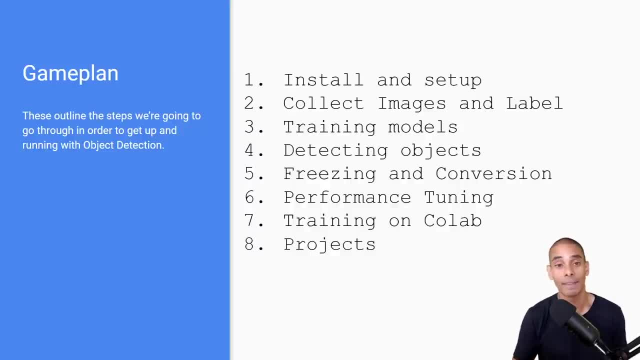 convert it into different formats, And this course we're going to cover how to convert it into a TensorFlowjs format, And we're also going to cover how to convert it to TF Lite. So those tend to be the two most popular formats that people leverage when using the TensorFlow object detection API. we're going to 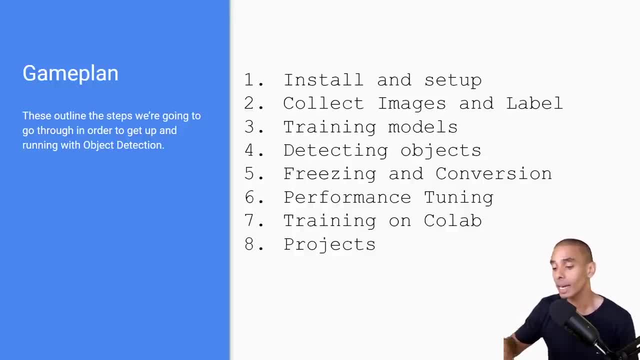 cover them both Now. I normally get a lot of questions on this, So performance tuning. So we're now up to step six. So we're going to be covering install, collecting images and labeling, training, detecting, freezing and conversion. Step six is a lot of the time where people come undone, So being 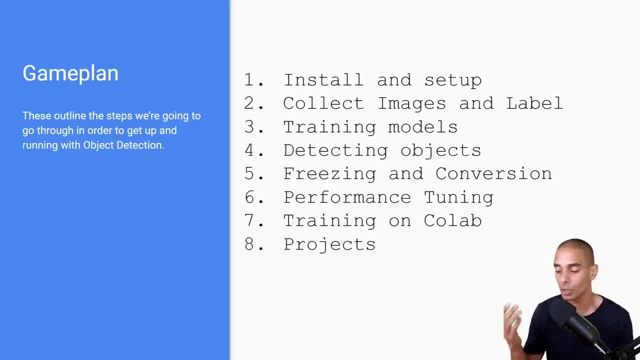 able to performance tune. your model is so, so important. For example, you use your webcam, you go to detect some stuff and it sucks. It's really, really crappy And it's not actually detecting the objects that you want it to detect. Well, what are the? 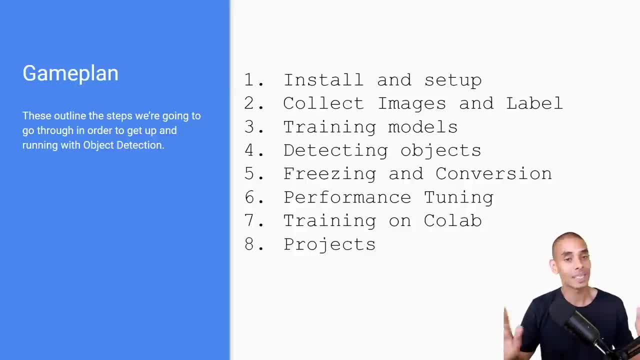 steps that you actually go through to be able to improve the performance of that model, to then be able to accurately and effectively detect those objects. So we're going to cover what to do when things go wrong and how to actually performance tune your models and improve that performance. so 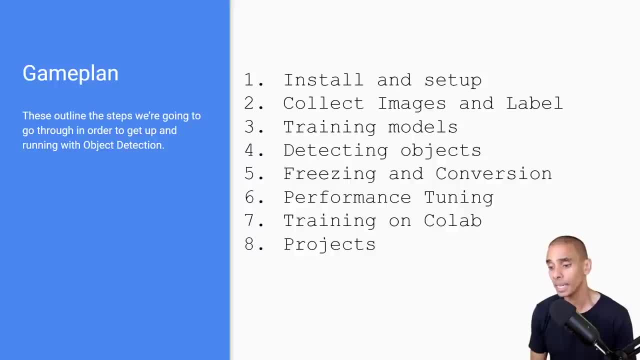 that you can get back on track. All right, so that's step six. Then what we're going to do is we're going to learn how to train on code, So we're going to run a code lab and a cloud instance. Now, the beauty of this, and everything that I cover in this course, is that all of the code and the full walkthrough, as well as a guide, is going to be available on GitHub. So if you go to the GitHub repositories that I'll show you later, you'll actually see that there's a written guide in terms of how to do this as well. So I've written a really big readme and a step by step walkthrough to actually get this up and running, as well as a couple of extra bonuses to make this a little bit easier on you. Now, in step eight, this is going to be a little bit easier on you, So I'm going to go ahead and go ahead and do a little bit of a test run. So, as you can see, I've already done the test run. So I've already done the test run. So I'm going to go ahead and do a test run and actually get a little bit more of a 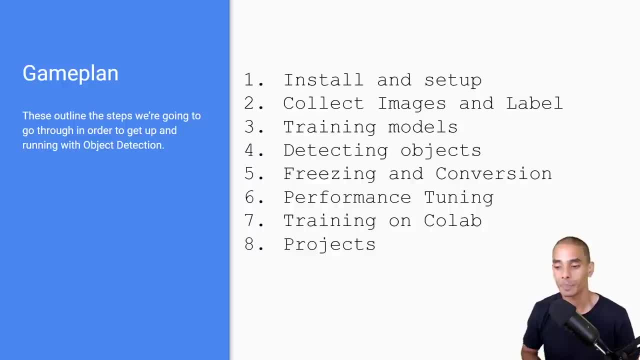 read me- and a step-by-step walkthrough to actually get this up and running, as well as a couple of extra bonuses to make this a little bit easier on you. Now, in step eight, this is where it all comes together, So we're going to be doing three different projects now And again. these are: 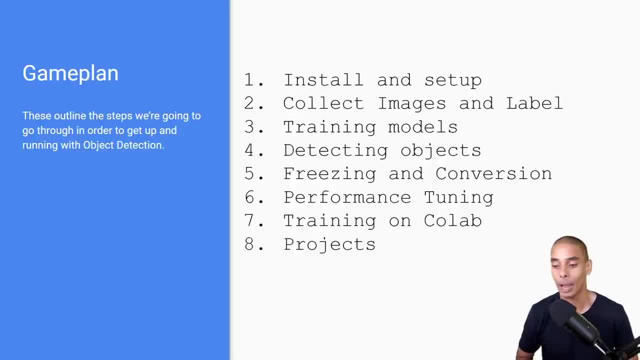 projects that I've really wanted to do for quite some time, and we're going to be doing them in real time, So the first project is actually going to be one that I've always wanted to do. We're actually going to be using this microscope, which is a USB microscope, to be able to detect defects in 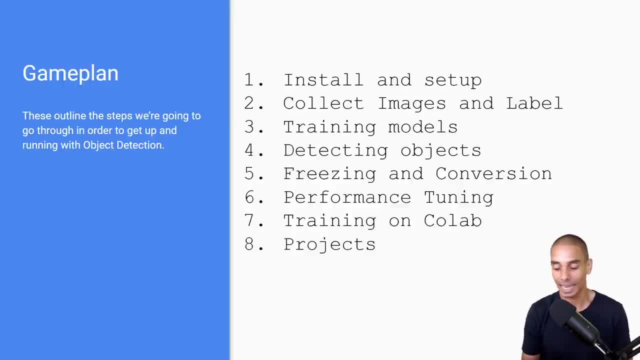 particular or small pieces. So in this case I've got a couple of LEDs here that I pulled out of my Raspberry Pi kit. So in this case it's really really small. Let's see if we can see that. You can see that right there. So it's a really small LED and you can see that this one there's. 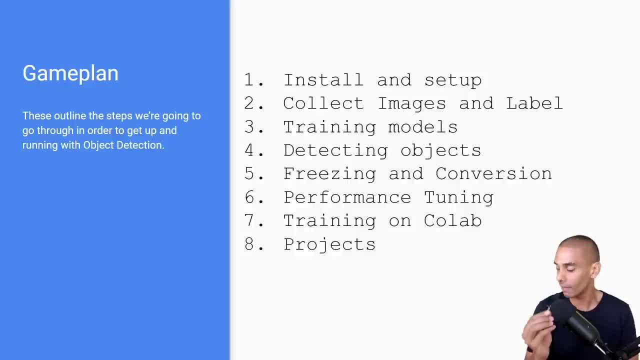 no issues with it, right. But then this one: I've obviously got a bent pin, So if I bring that a little bit closer, you'll see that this particular pin is bent right. We're actually going to train an object detection model to leverage this microscope. 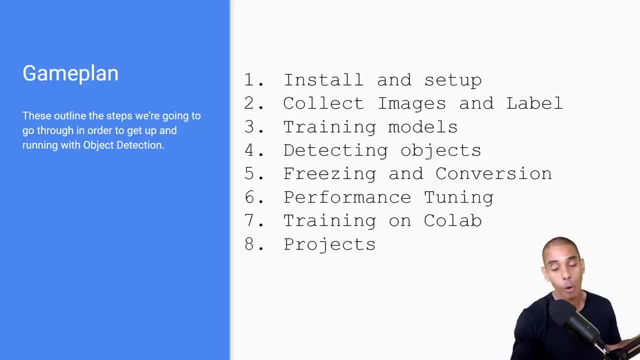 To be able to detect those bent pins. Now, this has a whole wide range of use cases. to say, for example, you had a PCB, so a printed circle board, and you want it to be able to detect defects in that. Say, for example, you want it to be able to look at a Petri dish and be able to detect 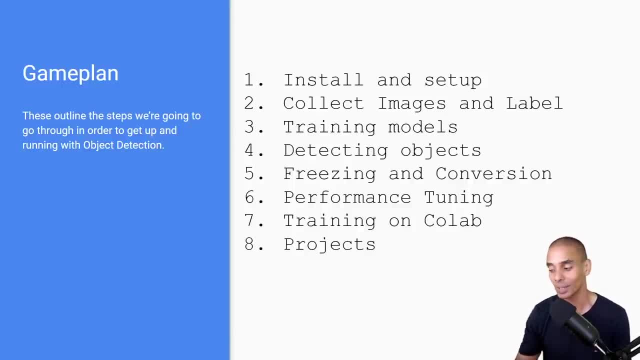 different things within a particular microscope slide to do that as well. So that'll be project number one. Project number two is going to be able to detect directions. So we're going to train a model to be able to detect our hand pointing up, left, right and down, And then we're going to 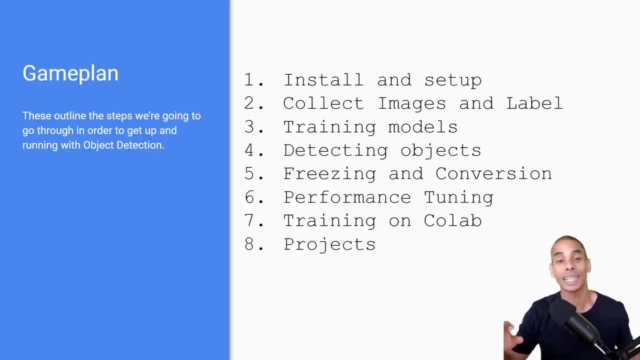 take that model, convert it to TensorFlowjs and actually integrate it into a web app. So say, for example, you want it to build up on that and build a real time game and pass through detections using your hand or using object detection. you'd be able to do that. And then our third and final project. 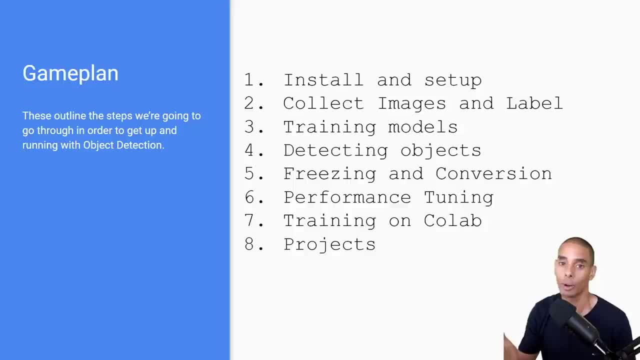 is actually going to be Raspberry Pi object detection. So again, this one tends to be really, really popular. I have seen a bit of a performance drop off when you do pass it to Raspberry Pi, but we'll take a look at that. So we're going to be. I did say we're going to be doing a little bit of a. 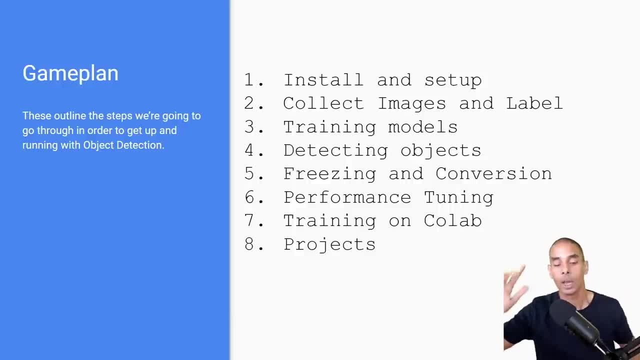 test, So ideally, trying to be able to detect sentiment from our face using our Raspberry Pi. So, again, I'm going to show you how to do all that, Alrighty, so there's eight steps. we're going to go through it all And again, take this step by step. So, ideally, what I'd recommend is go through each. 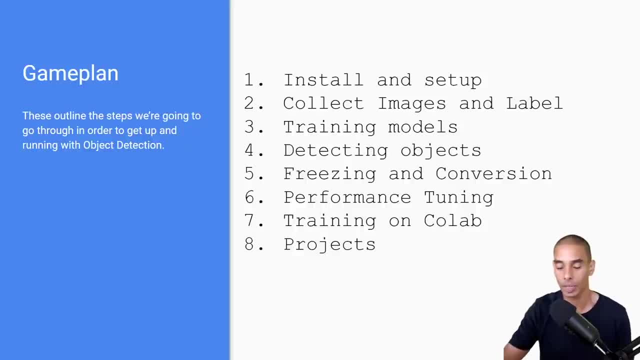 part. take a break, review what you've actually gone and done, make sure it's all working before going on to the next step. Take lots of notes And again, if you've got any questions, hit me up in the comments below and join the Discord server. That's probably my best tip as well, So I'm going. 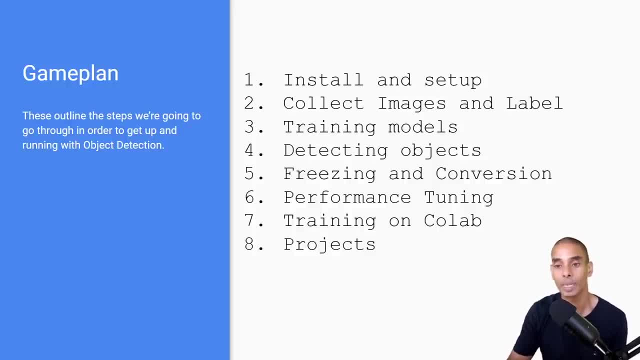 to include a link inside of the description, as well as in the pinned comment, to be able to join the Discord server. So, again, a lot of the people following the tutorials that I put out on YouTube are on that Discord server, as well as yours truly, So you'll be able to jump on in there and get. 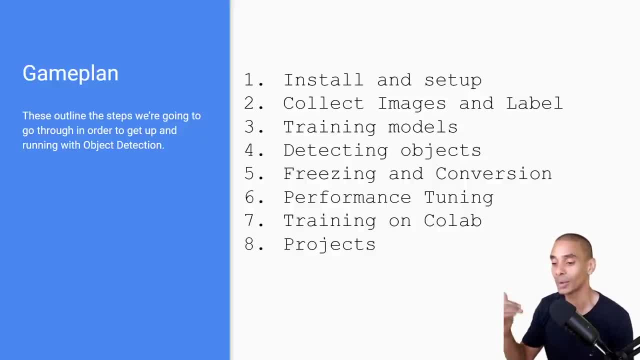 some help if you need it. But I also show you how to sort of debug and walk through this tutorial. So that's our game plan, those eight steps. Now, without further ado, let's kick things off and let's step into step one: install and set up. Alrighty, install and set up. 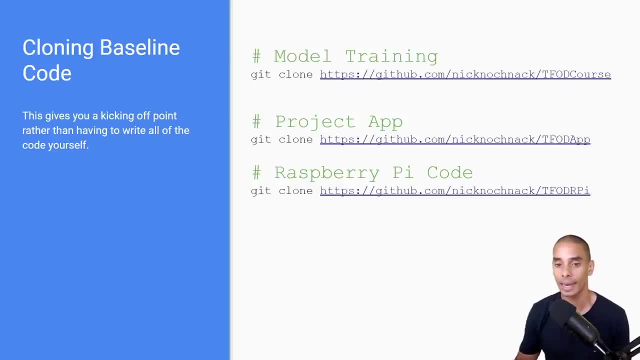 So the first thing that I'm going to sort of show you is where to get the code for these tutorials. So in this case, I've got three sets of code. One is more important than the others, but I'll show you each of those. So I've gone and written three different, or I've gone and built three different sets. 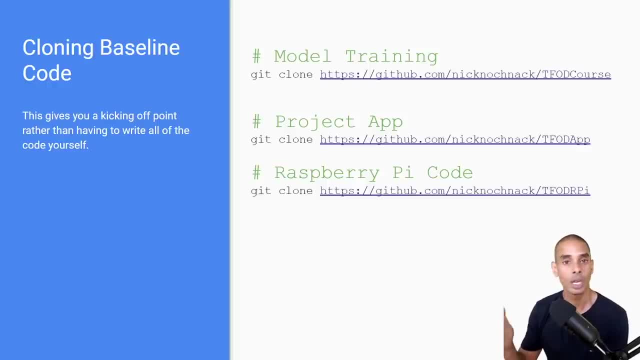 of GitHub repositories that you're going to be able to pick up and leverage to get up and running with object detection a whole heap faster. And if you've done any of my previous object detection tutorials- let's say, for example, the Face Mask Detector or the Sign Language Detector- what I've actually 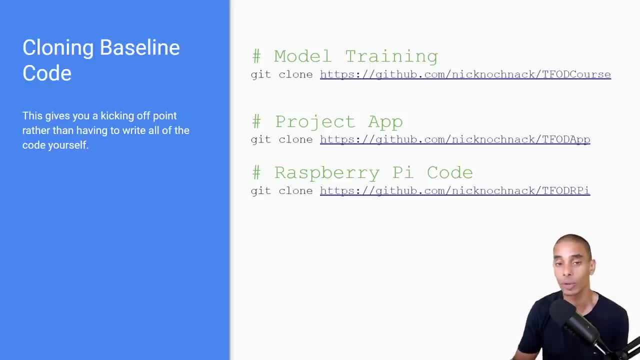 done is I've actually improved that code base So I've actually made this flexible enough to work on a Windows machine, a Linux machine, work on Colab, a whole bunch of different environments, So it actually detects what environment you're trying to use and runs the appropriate code, sorts out the file paths, so on. 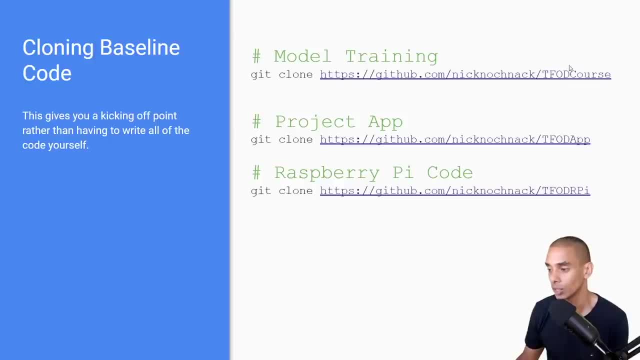 So there's three different sets of code. So there's the TensorFlow Object Detection course code. There's the TensorFlow Object Detection app. So whenever I say TFOD, that's just TensorFlow Object Detection. Then there's the TensorFlow Object Detection Raspberry Pi code. So you're going to get three different. 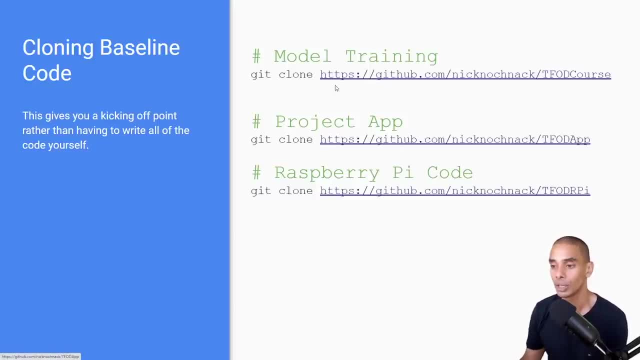 sets of code. Now, in order to get to these, you just need to go to https colon. forward slash. forward slash githubcom, forward slash knickknock nap. forward slash tfod course, forward slash tfod app and forward slash tfod rpi. So if we actually take 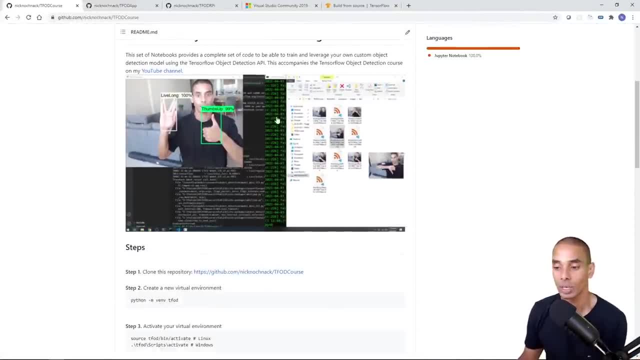 a look at those. So this is the course code And again you can see that we've actually got our baseline image. So here you can see that we're detecting live long and thumbs up. Now again, I'm actually. we're actually going to build this course, We're actually going to build this object detection model first up, So it's going to be a. 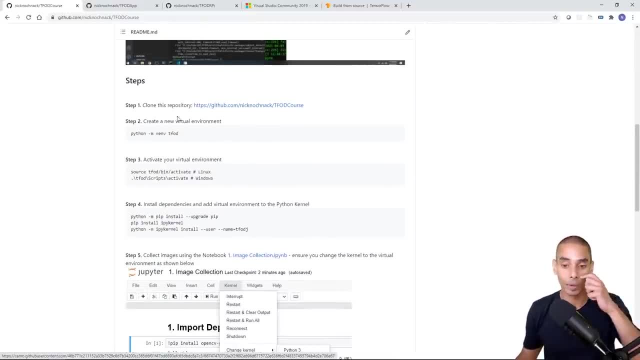 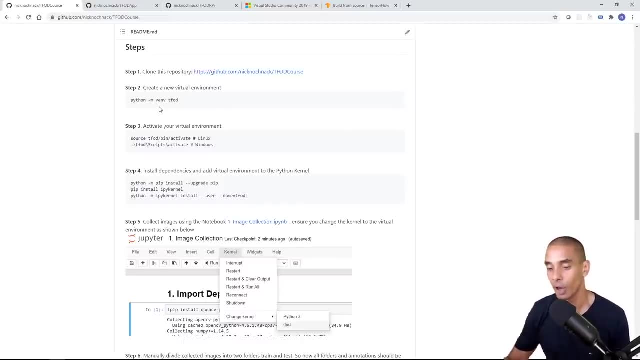 gesture based model. And the nice thing about each of these repositories is I've actually written steps, or written steps, rather than made a video tutorial on top of this, so that, if you prefer just walking through a step by step guide, you can just walk through each one of these to be able. 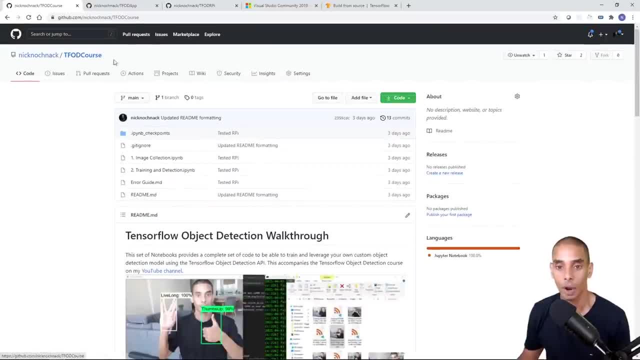 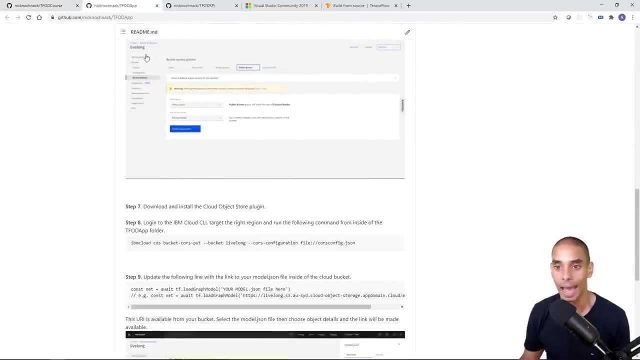 to build up these models as well, And I've done this for the TensorFlow Object Detection course code, which is the main training code. I've also done it for the app code, So it shows you how to deploy the app, And I've also done it for the Raspberry Pi code, So it shows you what you need to install. 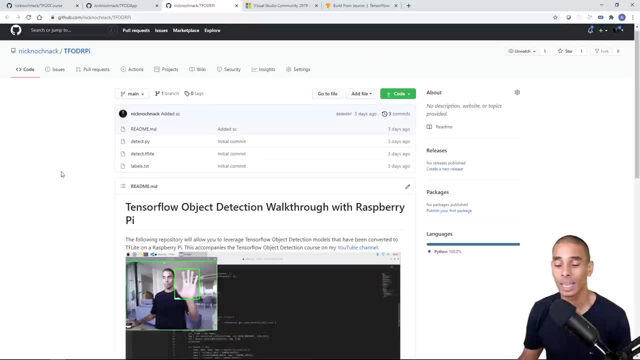 what you need to clone to be able to get this up and running. So, again, all of this code is going to be made available. So if you check the links in the description below, you'll be able to pick all this up. You'll be able to leverage it to. 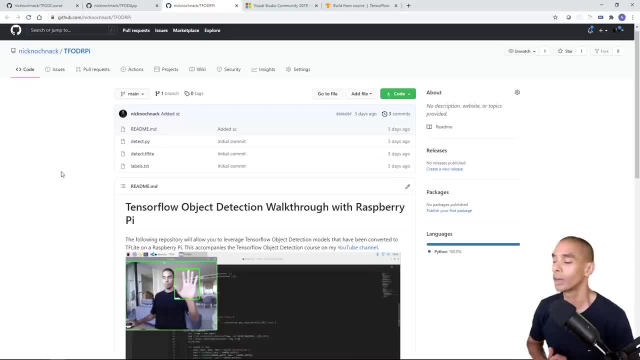 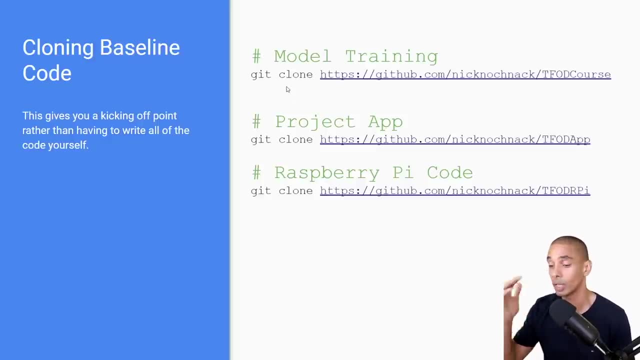 your heart's content and be able to build a whole bunch of different object detection models. So those are the three sets of code that we're going to be able to leverage. So you'll see once we kick off or once we actually start. the first step that we're actually going to go through is clone this code And 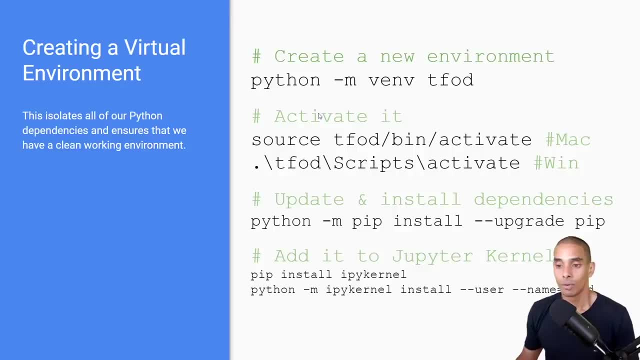 again, we'll just be using git clone to be able to do that. Now, the next thing that we're going to be doing is we're going to be creating a virtual environment. So, again, I'm going to explain a little bit of the code before we actually go ahead and do it. but I don't want to spend too much time on slides, So 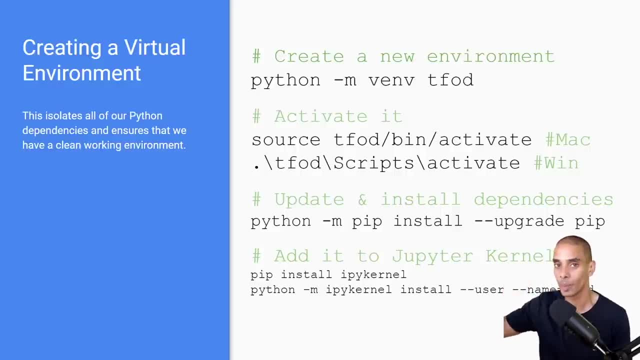 think of a virtual environment as a separate room in your house. So it's like creating a separate room in your house. Now, the reason that we're actually using a virtual environment is that it isolates all of the different Python and all of the different libraries. 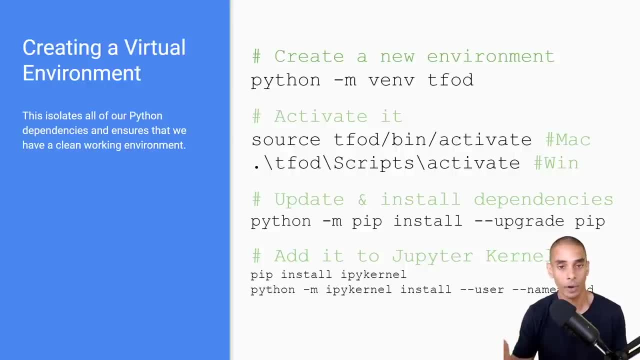 dependencies and different things that you're actually going to need for your TensorFlow object detection model. Now this makes sure that it doesn't conflict with all of the different libraries and dependencies that you've already got installed inside of your Python or Jupyter environment. So 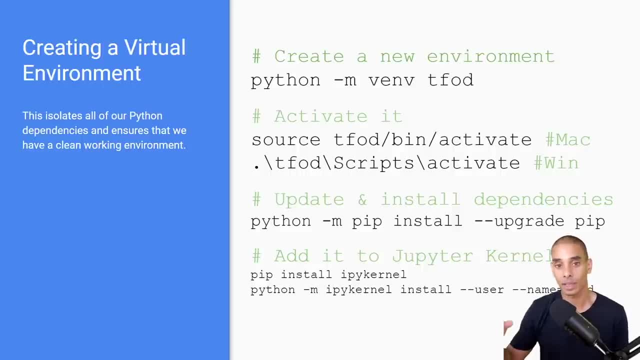 what we're going to do is we're going to create a new virtual environment- So think of it as creating a new room in your house- And we're going to install all of our object detection stuff inside of there So it doesn't mess around. 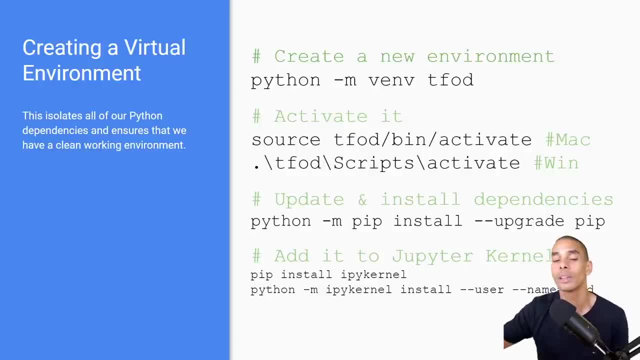 with any of the other things, And it ensures that you get all of the main dependencies that you need and you don't get any dependency conflicts. Now, in order to do that, we're going to be using a library called venv, So this allows us to create a new Python environment And, again, 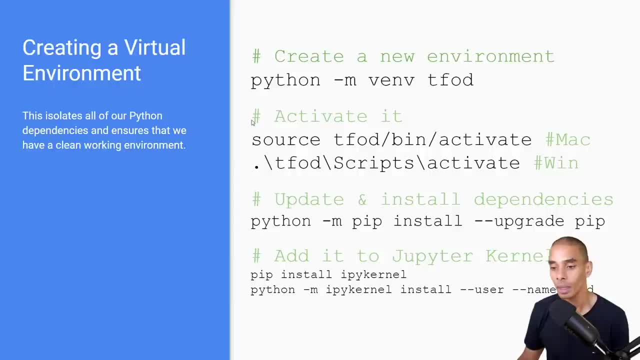 we can name it whatever I want or whatever you want. Then what we're going to do is we're going to activate it. I'll talk a little bit about that later. We'll upgrade our pip dependency, So this makes sure that we have the latest resolvers and all of the good stuff that we need. 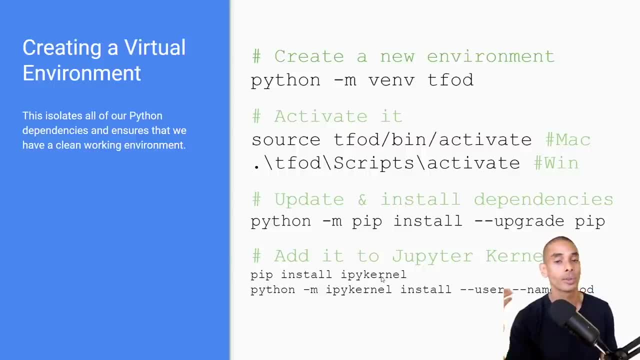 And then we're going to be installing ipyekernel. So ipyekernel is a really important dependency because it allows you to associate your virtual environment with your Jupyter notebooks. So ideally so we're going to be working inside of Jupyter notebooks. Now we won't cover installing that. 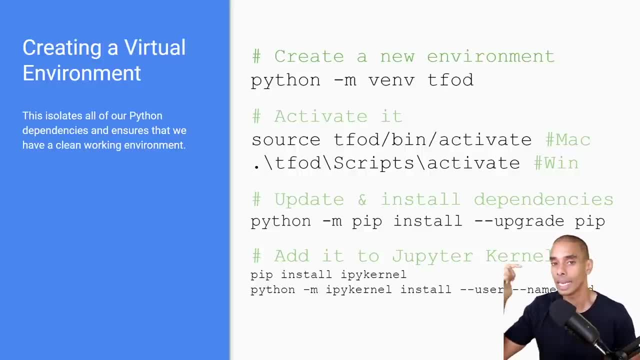 But again, if you want to see how to install that from scratch, I'll link to the other installation video where we do the Anaconda install and the Jupyter notebook install. But more often than not, if you've done any data science or object detection tutorials before, you'll have Jupyter notebooks installed. So this is going. 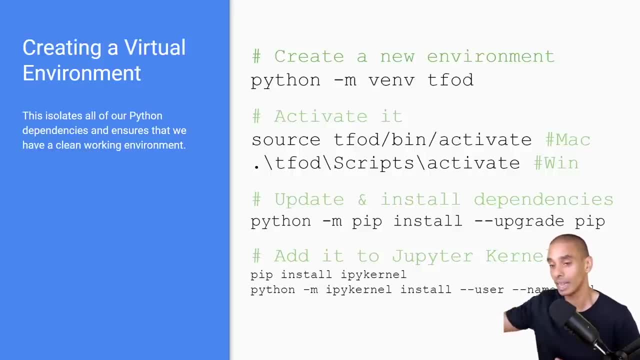 to cover all the stuff that you need to go from Jupyter notebooks a little bit further and be able to build your object detection models- All right, creating a virtual environment. So think of it as a separate room inside of your house where you're going to install all of your object detection stuff, so that 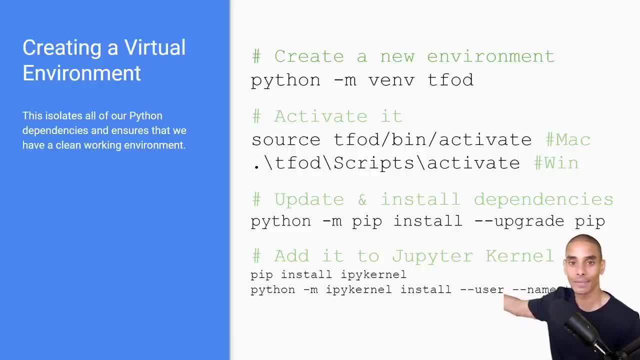 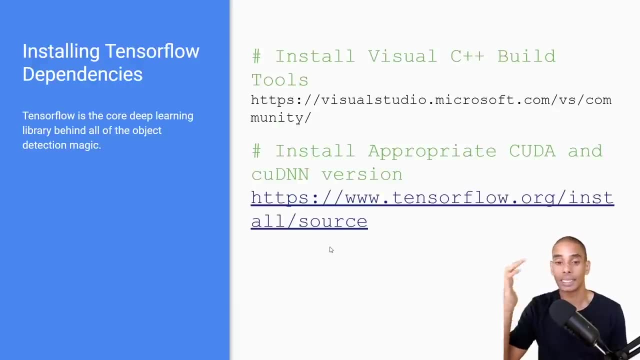 it doesn't screw up everything else. It's also like locking yourself in a room and getting stuff done, Keeping everything in one place. Now there's a bunch of dependencies that you need to install whenever you're working with TensorFlow. Now the first and foremost one is going to 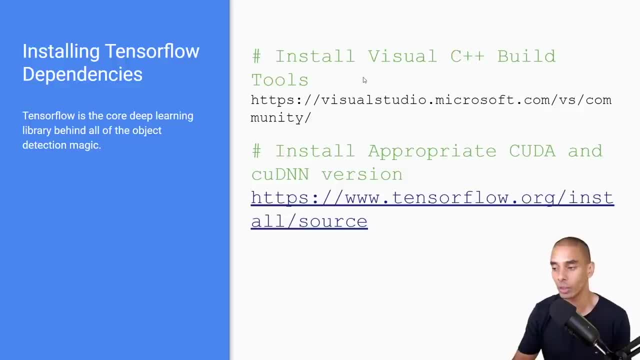 be the Visual C++ build tools. I'll show you where to install that. So it's really a just download and install. nothing too special there. So TensorFlow needs Visual C++ build tools in order to run. That's pretty straightforward. Now, again, I'll link to the other install tutorial. 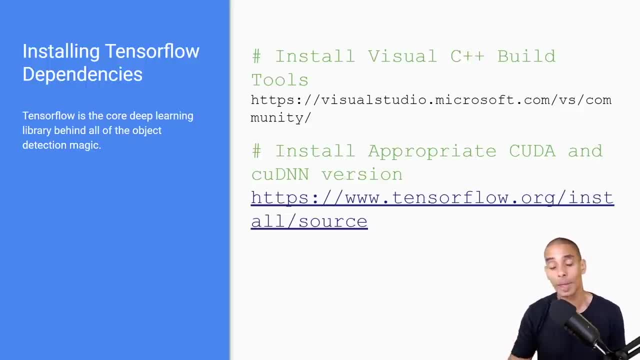 where you can pick that up. So that one's pretty straightforward. Where most people tend to get hung up is installing these two though: CUDA and CUDNN. So CUDA and CUDNN give you GPU based acceleration when training your TensorFlow object detection model. 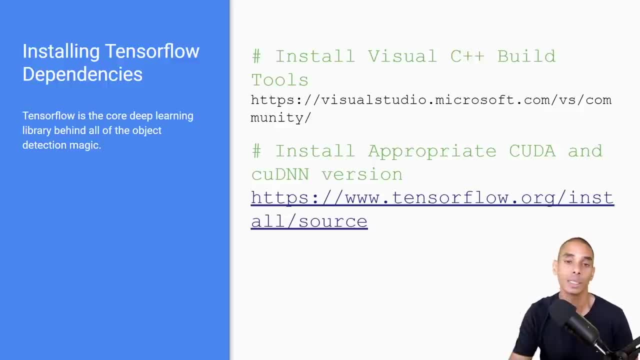 So the reason that you use a GPU is that it is exponentially faster to train an object detection model using a GPU versus just using your raw CPU and your raw memory. Now, if you don't have a GPU, don't worry about it. You can still go through this tutorial. 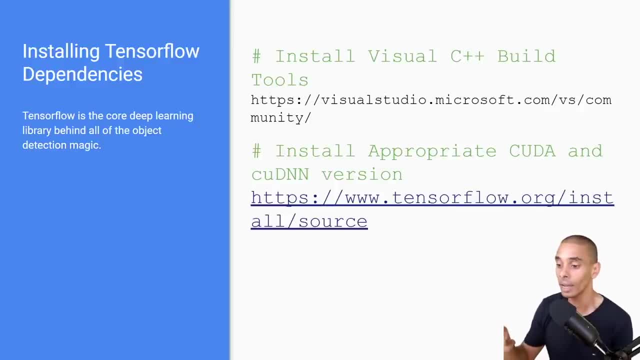 It'll just take a little bit longer to train your model. Now, if you do have a GPU and you've gone through an object detection tutorial before and it wasn't actually activating or it wasn't actually being utilized, I'll show you how to check that Then- what it might have actually been, particularly if you're using 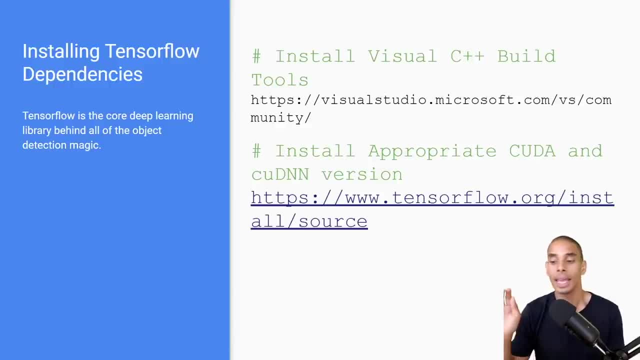 TensorFlow is that you might not have had the right CUDA and CUDNN installations available, But I'll show you how to actually see whether or not, or how to actually find an appropriate combination. Now, the reason that I'm talking about this is because there's consistently going to be new versions of TensorFlow coming. 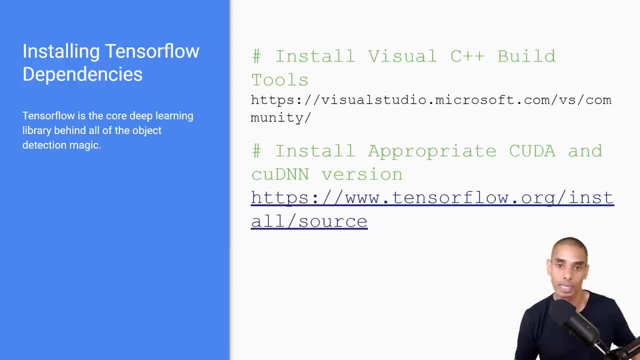 out. So you might need to update your CUDA version or update your CUDNN version in order to be responsive to that actual change. So I'll show you where to do both of those, or how to detect both of those, And let's actually take a look at that. So, in terms of Visual Studio, 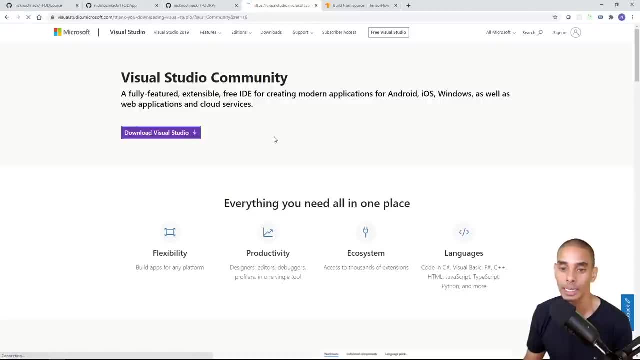 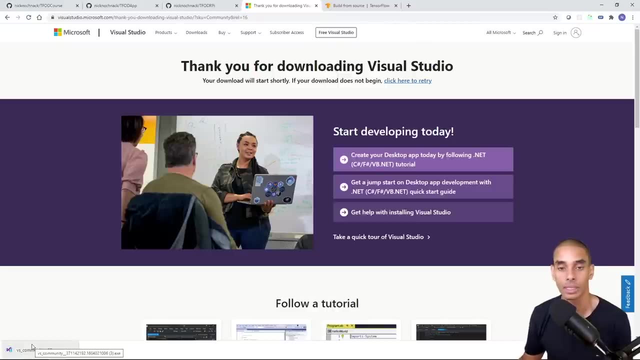 so what you just need to do is go to Visual Studio Community, download Visual Studio. So this is going to download everything that you need And then, ideally, what you want to do is just run this in and install. So this is going to install the C++ build tools. And again, if you want a full walkthrough, 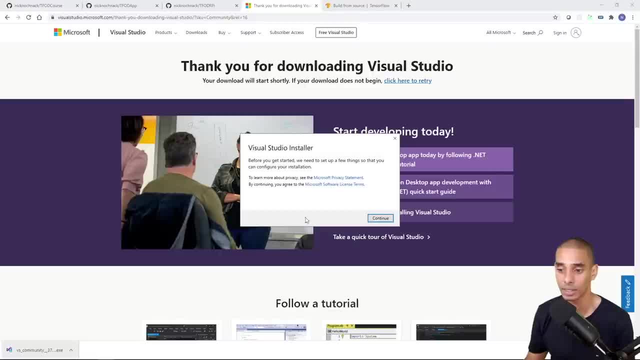 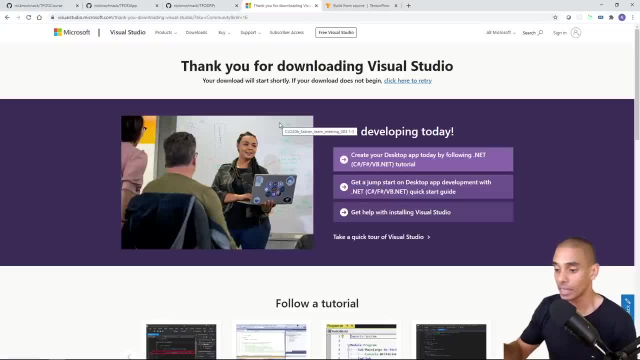 so really it's just a matter of downloading this and installing that, So it doesn't need a whole bunch of stuff. So I'm going to cancel that because I've already got it installed. So you just need to download that, install that and that's going to give you your C++ build tools. But again, if you want to see a full, 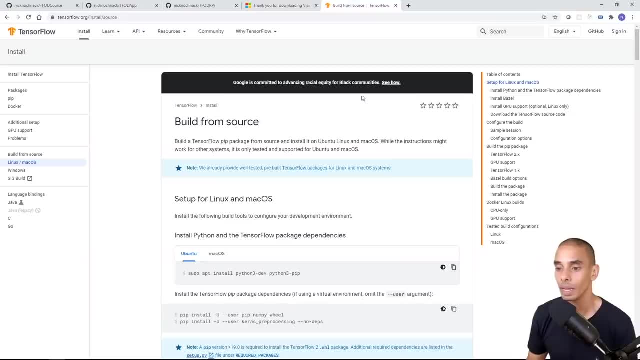 walkthrough on how to install that. I'll include a link to that as well. Now, the next thing, which is more important, is CUDA and CUDNN. So this only applies if you've got a GPU and you want to use GPU accelerated training. Now, I'm not going to do this first up, because 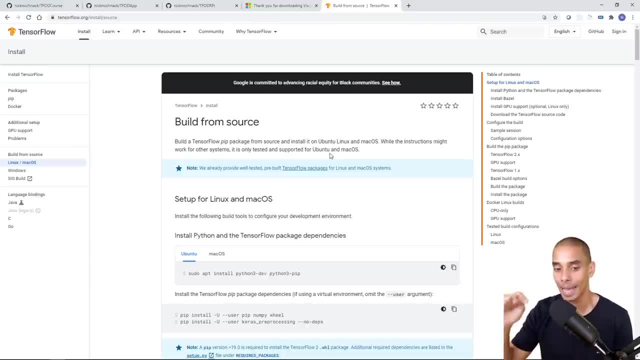 I'm going to show you how to check your TensorFlow versions and then map to the appropriate CUDA and CUDNN libraries. Now, the reason that I say this is if you actually go to this link, so tensefloworg forward slash install. forward slash source, also this one. 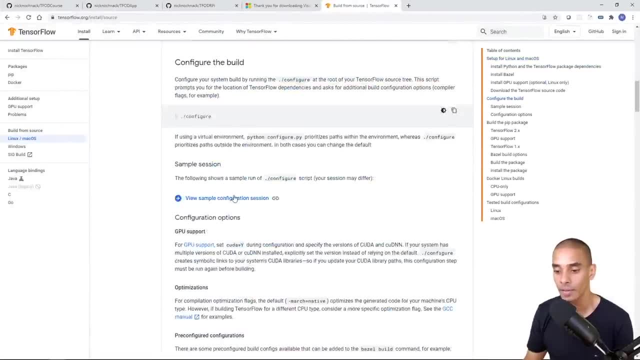 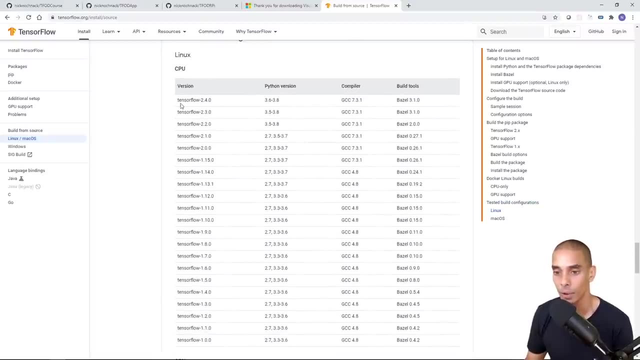 down here. But again, links will be available in the description. If you actually scroll all the way to the bottom, it actually gives you the appropriate versions of TensorFlow and CUDA and CUDNN to use In this case. this is just CPU, So again. 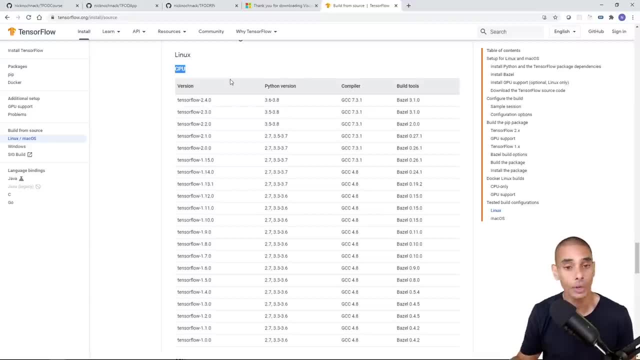 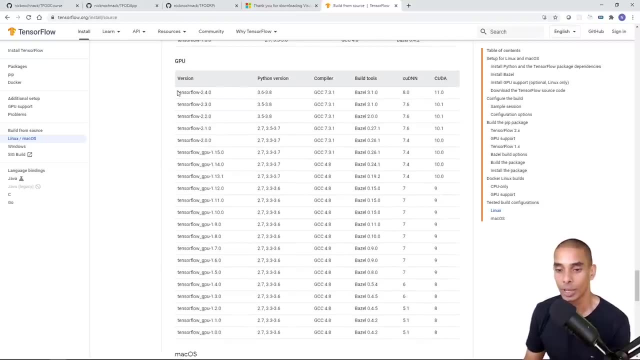 you can run this full object detection tutorial on your computer even if you don't have a GPU. It'll work fine. It'll just be a little bit slow. But, more importantly, these are the GPU combinations. So here, if you're using TensorFlow 2.4.0, you need to be using Python version 3.6. 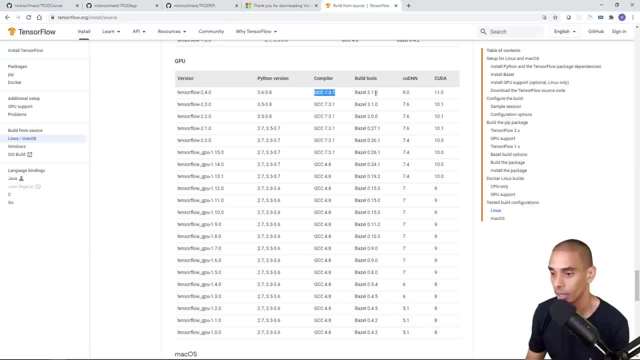 to 3.8.. You need to have the GCC compiler 7.3.1, Bazel 3.1.0, and, more importantly, CUDA and CUDNN. So here we've got so many different versions of TensorFlow. 2.4.0 runs with CUDA 8 and CUDA. 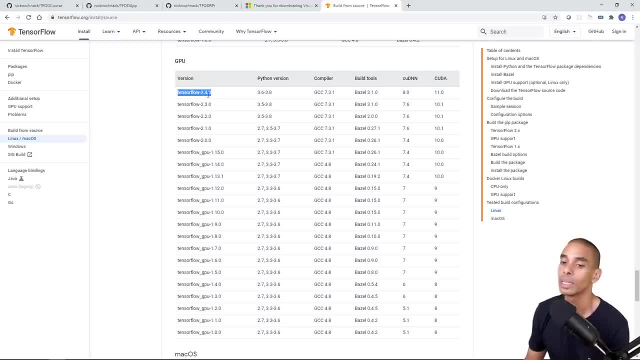 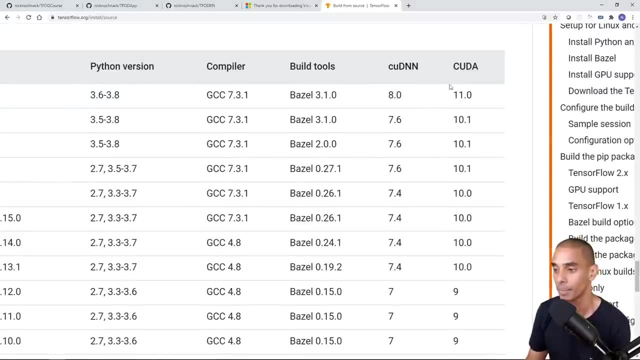 or CUDNN 8 and CUDA 11.. So you need to make sure- this is so important- You need to make sure that the TensorFlow version matches these two CUDA and CUDNN versions up here. So if they don't match, it'll still run, It just won't leverage. 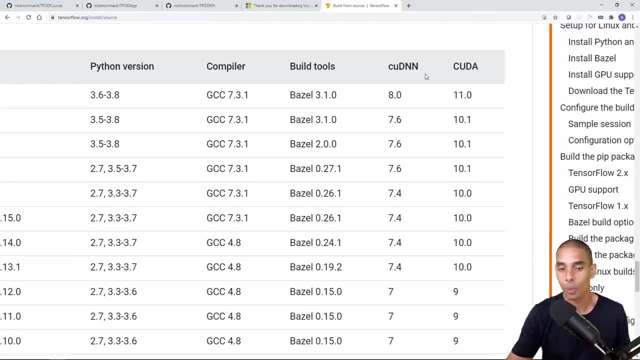 your GPU, And you'll probably be sitting there thinking, hey, I've got a GPU. Why isn't this training faster? More often than not, it's because of that, And I'll actually show you how to check your TensorFlow version and how to get the. 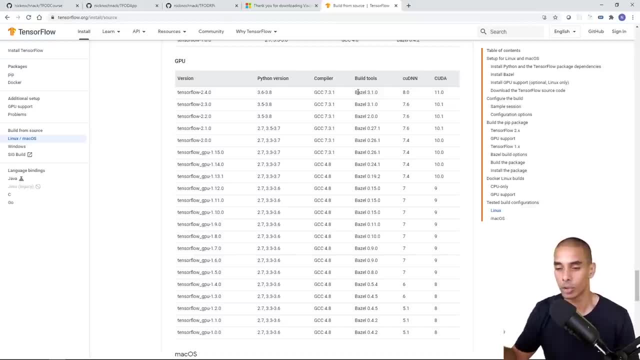 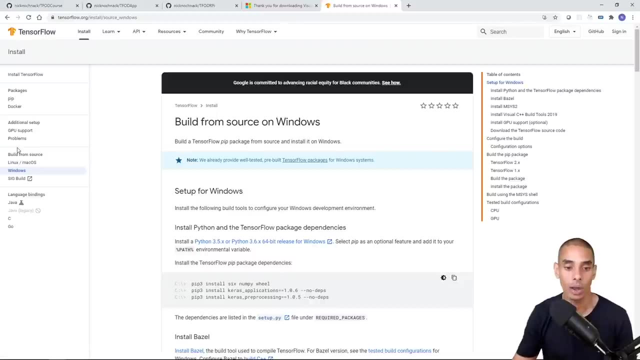 appropriate CUDA and CUDNN versions once we've gone through the initial steps of our install. So this is the Linux-Mask OS combo If you go to the Windows one over the left hand side here. So in this case the install or the link is: 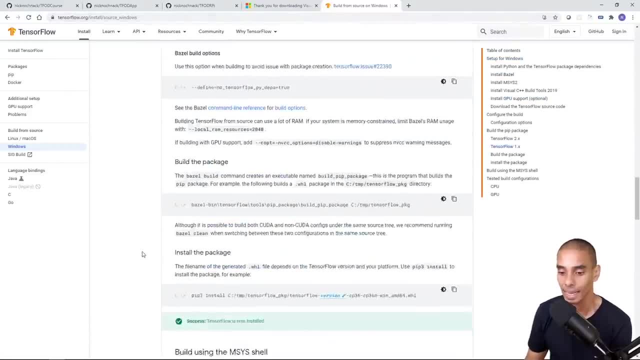 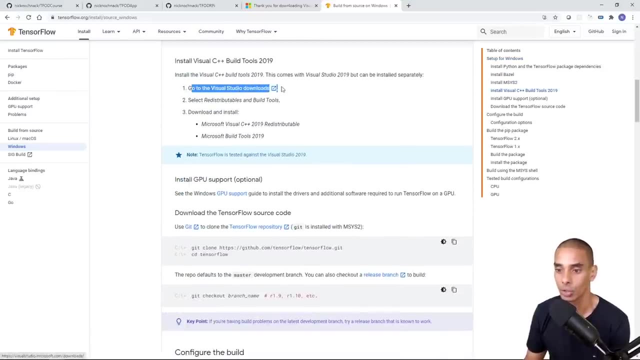 forward slash. install forward slash source underscore Windows. Again same style of thing. And again it talks about the Visual C++ build tools over here. So again it just tells you: go to Visual Studio, hit Visual Studio downloads, select redistributable download and. 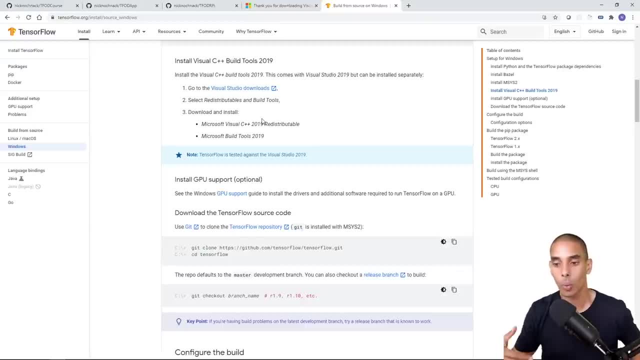 install, And the reason that I'm sort of going through this is I'm sort of showing you where the information that I'm teaching you is coming from. So this gives you an idea as to where to go to get help. But again, you can always hit me up in the comments. 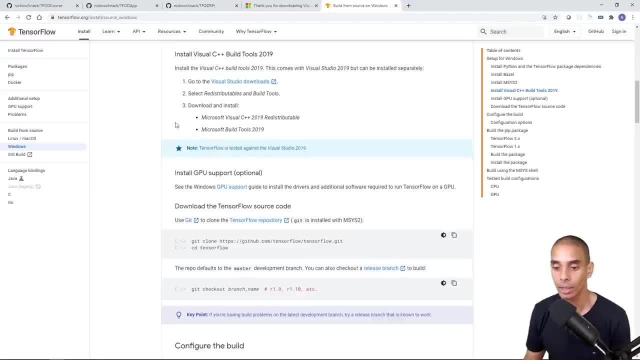 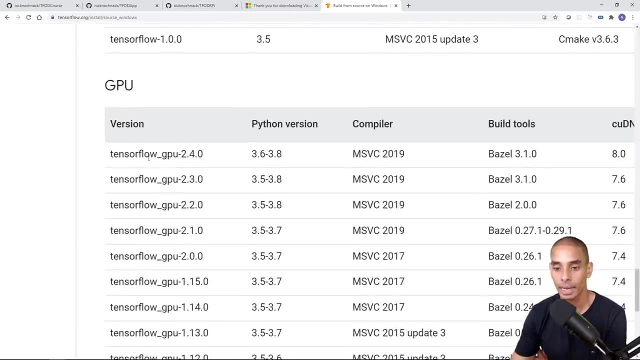 So again, you've got to install Visual C++ build tools through the downloads. Now, if you go down further towards the bottom, these are the combos for Windows. Again, if you're using TensorFlow or if you're using TensorFlow GPU, you need to be using. 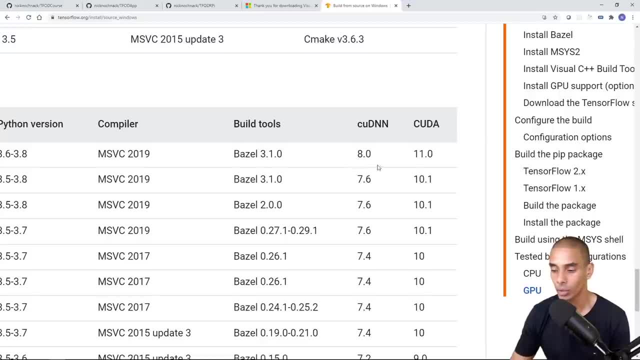 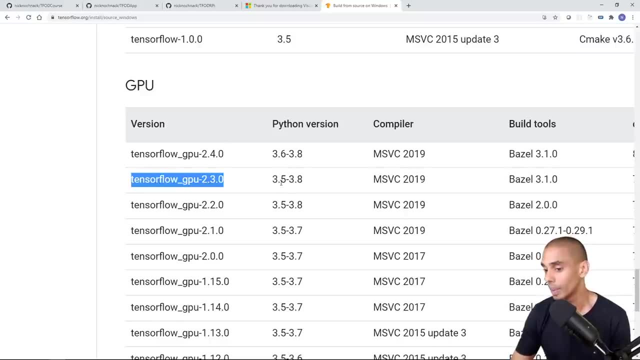 TensorFlow GPU 2.4.0 and CUDA 8 and 11.. If you're using TensorFlow GPU 2.3.1,, for example, then it's going to fall into this category. So you need to be using Python 3.5 to 3.8.. You need to use the Microsoft. 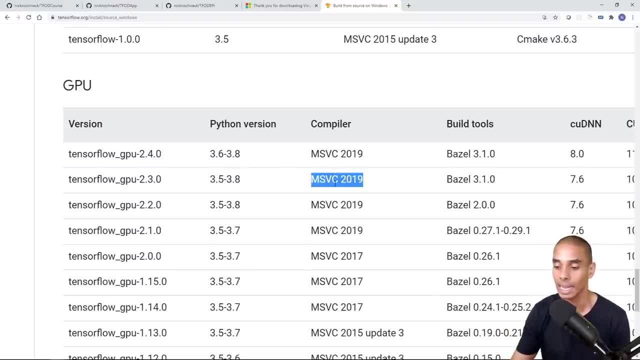 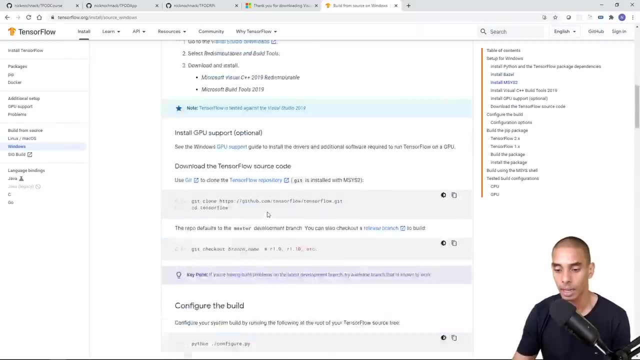 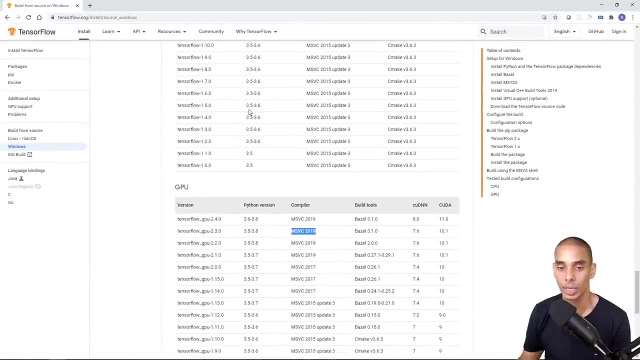 Visual C++ build tools to 2019.. So this is just talking about that compiler that we had Right up here. So it sounds complicated, but really it's just talking about that Visual or this thing that we were just downloading. So that's fine, So you can use that. Oh, we've moved that. 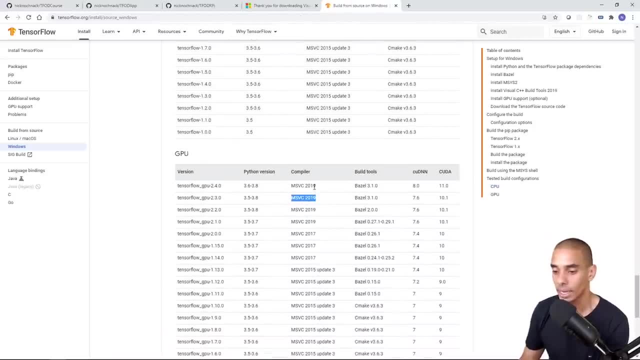 So Microsoft Visual Studio 2019 and you need Bazel, But again, that's normally pre-installed and you need. So, in this case, if you're using 2.3.0, you need CUDA, CUDA 7.6 and 10.1.. So again, there's really. 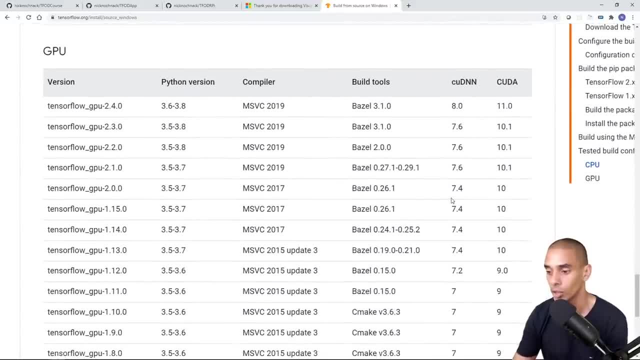 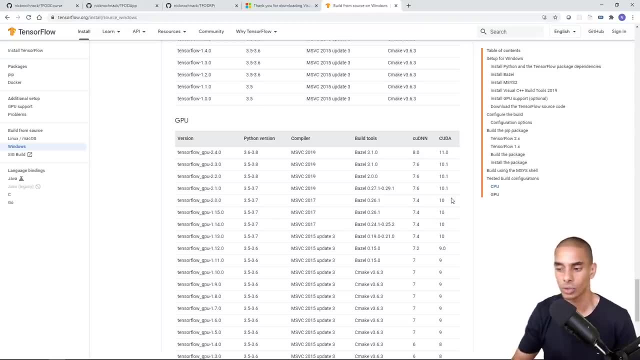 specific combinations that you need to be using if you want to be training on your GPU Cool, All right. So that talks a little bit about that, but we'll actually come back to that GPU install a little bit later. So I'll actually show you how to check your TensorFlow version. 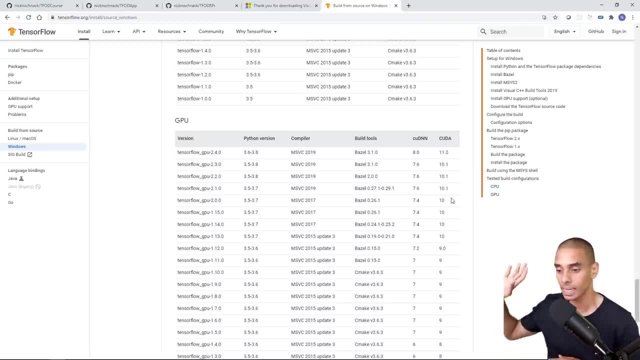 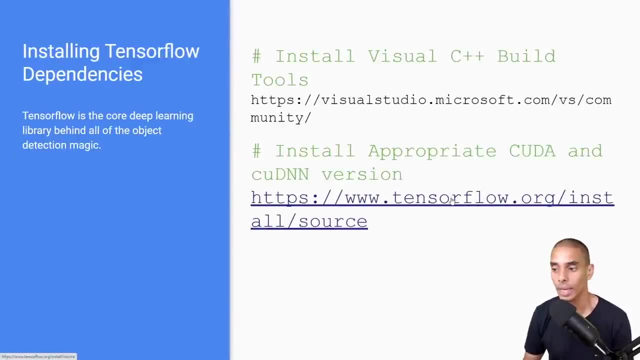 Make sure that you've got the right version in your virtual environment. Think about it as the other room inside of your house, and then find the matching CUDA and CUDNN versions. Okay, Now, all of that might seem pretty complicated, So you're probably thinking: all right, Nick, what? 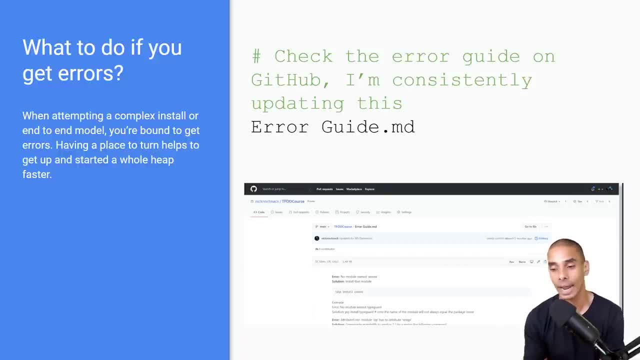 the hell am I going to do if I get errors? Because undoubtedly you will get errors as part of this. It's always being updated, There's always changes. There's a couple of things. So the first thing that I'd recommend is: if you're getting errors, by all means do mention it in the comments below, But if you're 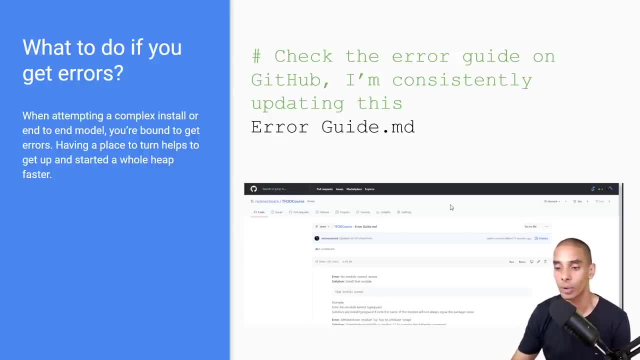 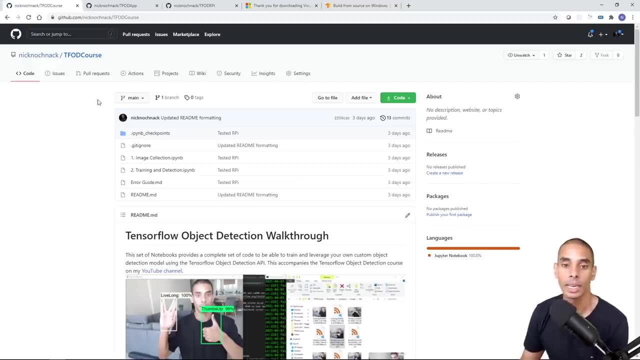 getting errors during the installation steps or while you're actually running the notebook. I've actually put together an error guide. So if you go through to the TensorFlow Object Detection Course GitHub repository, which is available at githubcom, forward slash, nicknocknack, forward slash, tfod course, And again this link is going to be available in the 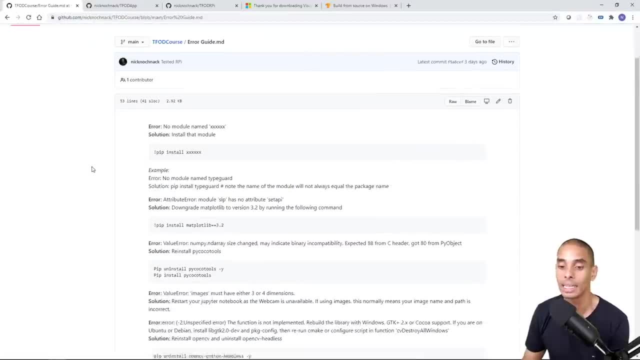 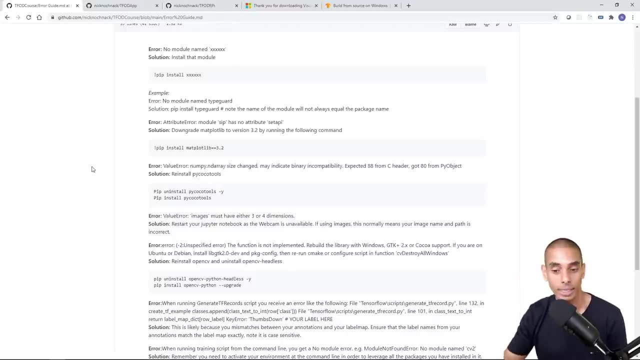 description below. I've actually put together this error guide and this is based on all the errors, all the questions that I saw people were asking me as part of the other object detection tutorials that I've got, So you can see here that say, for example, you: 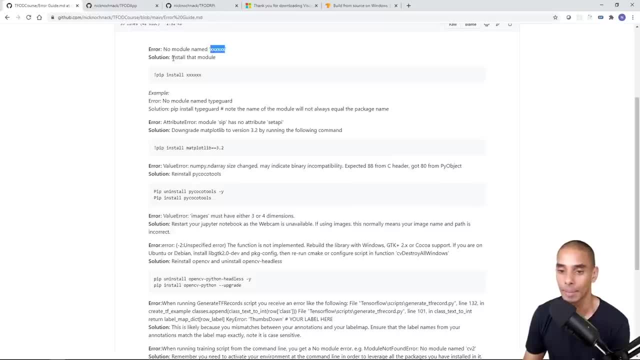 get an error which says: no module named. whatever that module name is, Well, more often than not, the solution to that is to go on ahead and install that module. So say, for example- I've actually got an example here- So if there's no module named typeguard, well, what you want to do is then go and 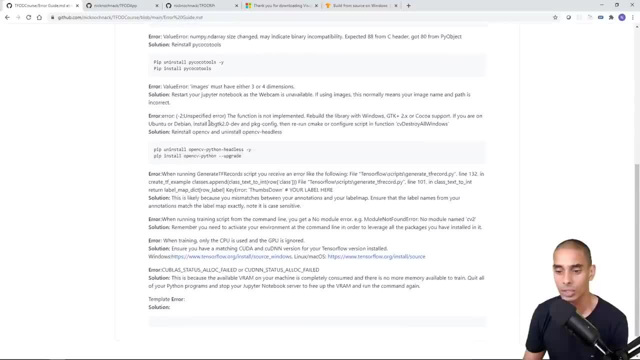 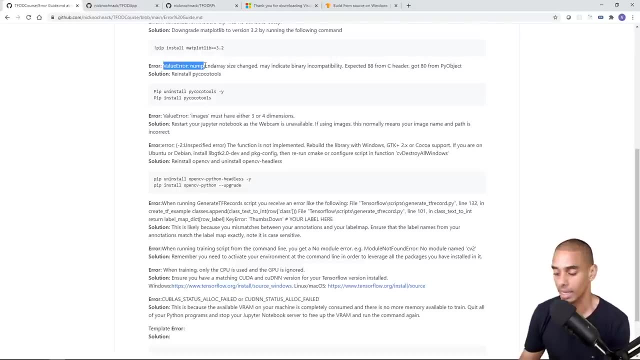 install typeguard using pip install. Another one that's really, really common is the PyCoco tools one. So in this case, say, for example, you get a this error here, So let's zoom in on that so you can see it. So value error numpy nd array size change. 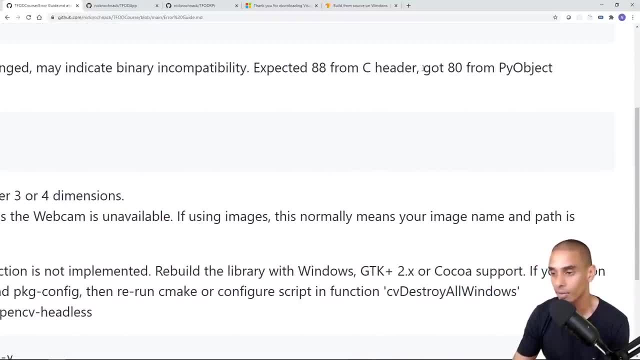 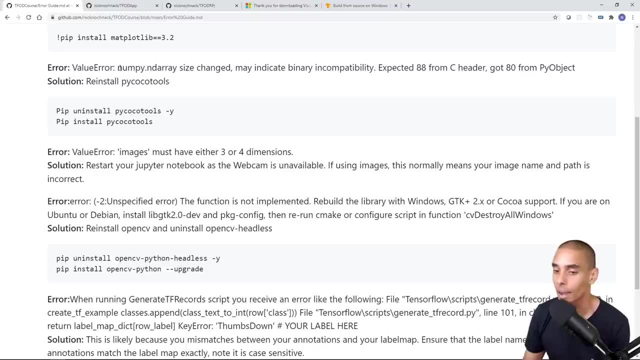 may indicate binary incompatibility. expected 88 from C header, got 80 from object. Sometimes these errors aren't very descriptive So you probably think, oh well, that's a numpy error, But actually it's a PyCoco tools error. Now again all of these errors. 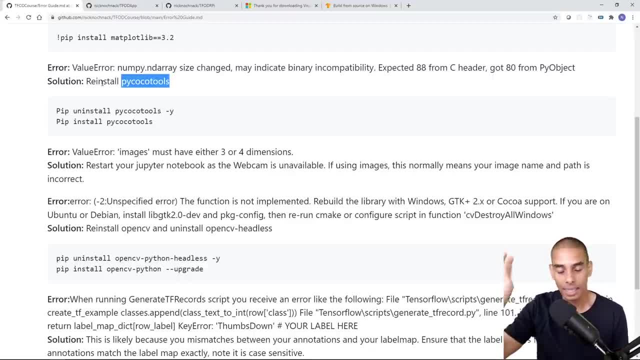 and all of this error guide is going to be available inside of the GitHub repository, And my goal is to ideally be consistently updating this. So if there's new errors that pop up or if there's new things that pop up that need a solution, I'm going to be consistently posting it. 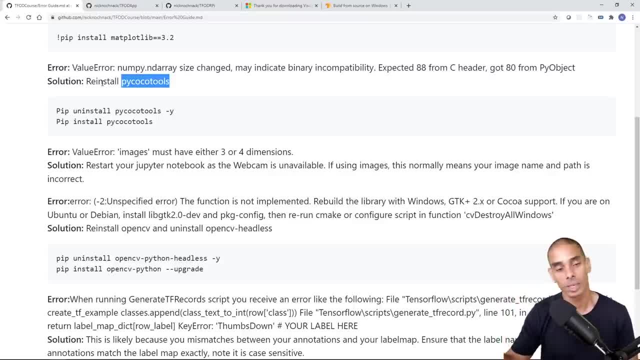 in here. So I'll be cloning it, updating the error guide so that you've consistently got another place to turn. But again, the other place that you can turn if you need support is to jump onto the Discord server. Again, I'll include a link in the description below. There's a bunch of people that are already on there that are 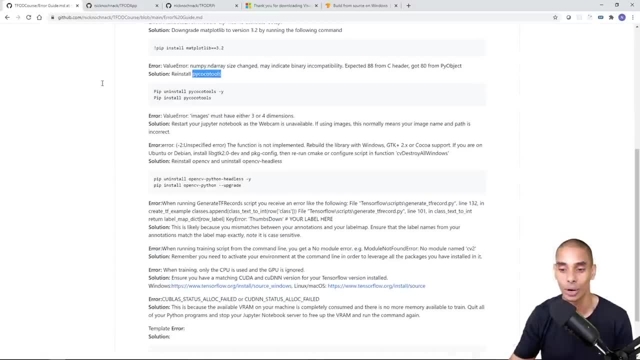 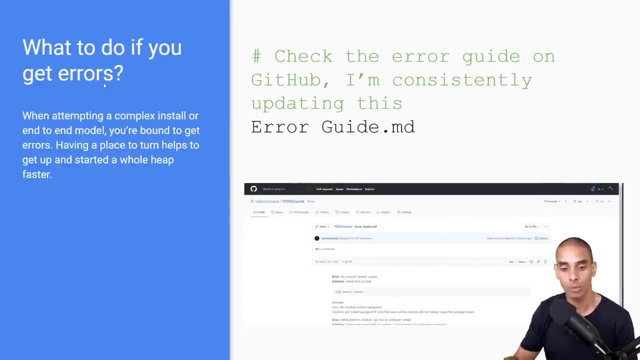 awesome. They're providing help to anybody that's actually going through these tutorials. Okay, so that is the next thing that I sort of wanted to show you. So that's the error guide and where to get help if you get stuck. Okay, so, 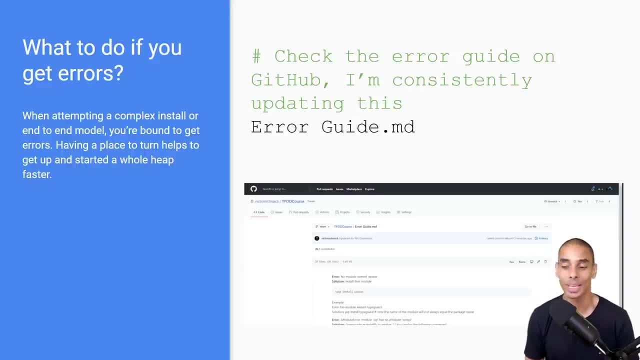 that's a lot of slides. Now we want to do is: or now what we want to do is actually get started with this thing and start building up our object detection model. So the first thing that we're going to do is, as I was saying, we're going 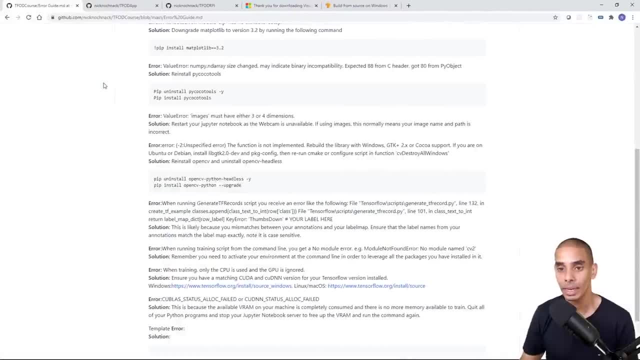 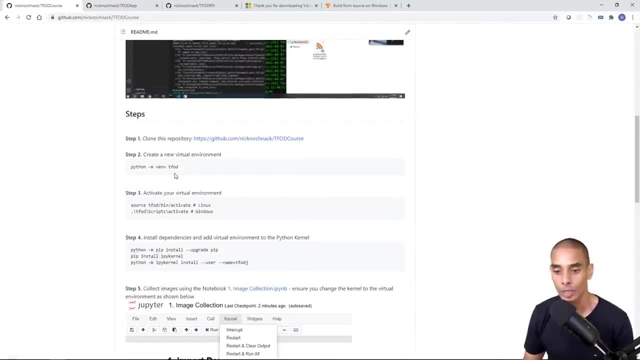 to start up by creating a virtual environment. Now, in this case, I've actually got the steps to create the virtual environment inside of the TensorFlow object detection course code, which you can see down here. Now the first step that we're ideally want to do is we want to: 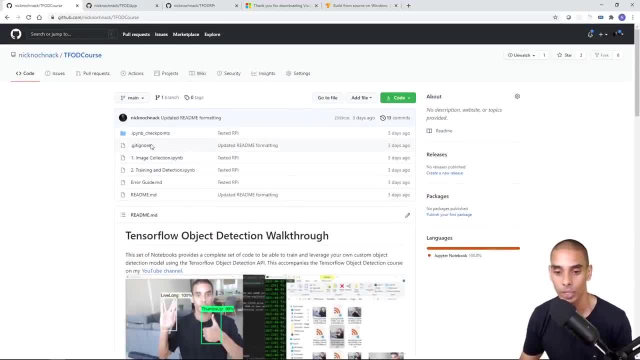 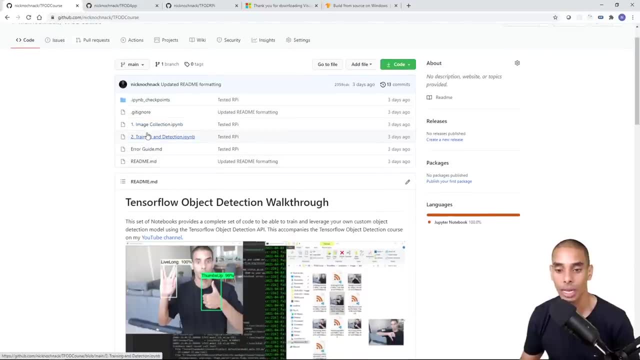 clone this TensorFlow object detection course repository which contains our checkpoints, which we can get rid of that. I don't know why I included that. It includes our gitignore file, our image collection notebook, training- Let's zoom in a training and detection notebook. 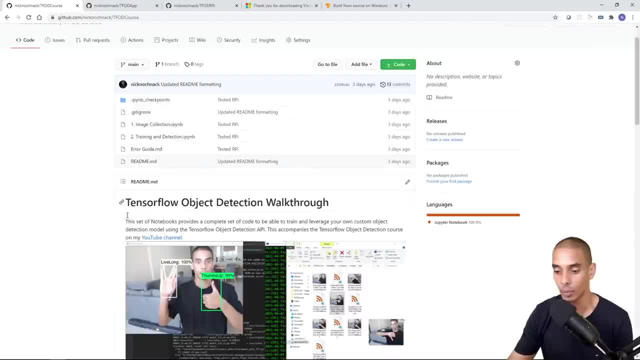 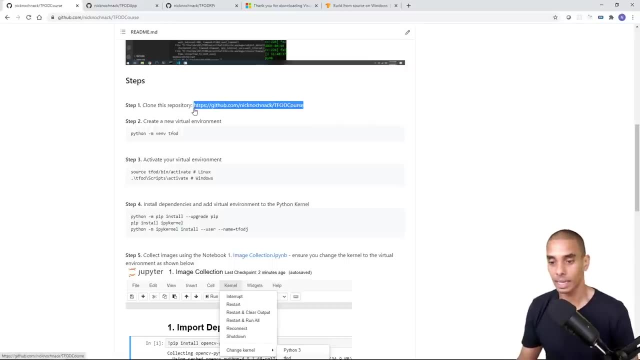 error guide which I just showed, as well as this readme, which gives you all of the steps that you need to go through. So let's go on ahead and clone this repository. So I'm just going to copy this link and go to a new command prompt. So in this case, I've got a new command. 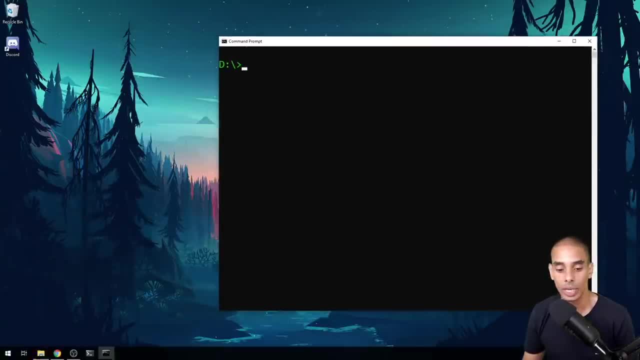 prompt because I'm on Windows. If you're on a Mac or a Linux machine, you'd just be opening up a terminal And I'm going to do this side by side so you can see what we're doing. So I'm going to create a new folder inside. 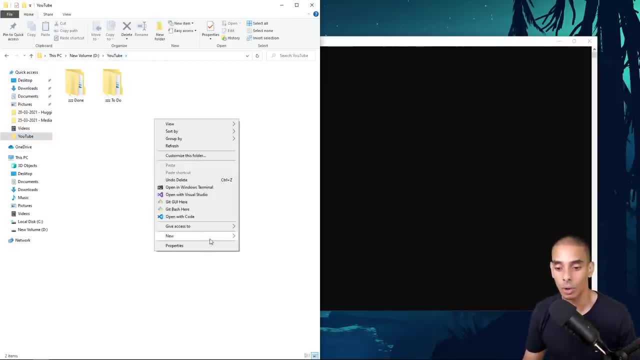 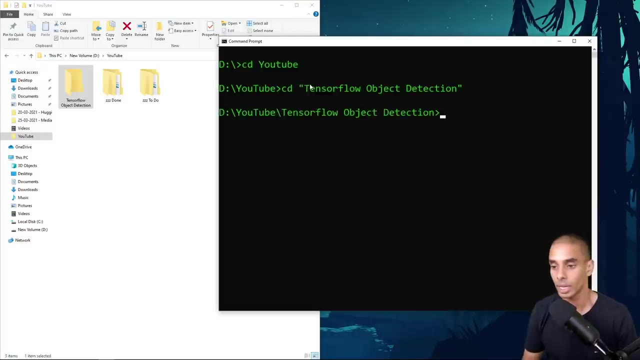 of my D drive and inside of my YouTube folder And I'm just going to call it. let's call it TensorFlow object detection, Cool. And then what we're going to do is go into that folder. So I'll go into CD, YouTube CD- TensorFlow object detection, And then 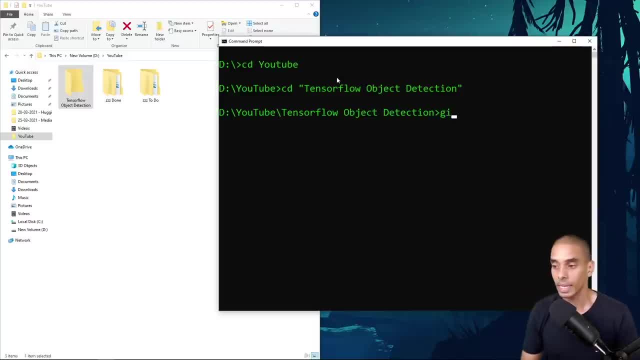 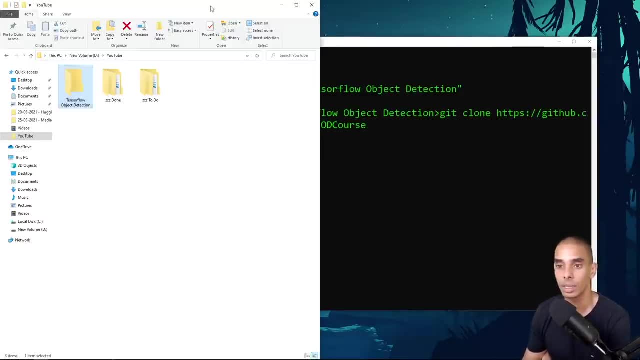 what we're going to do is clone that repository, as I was saying. So we'll type in git clone and then that link. So again, all of those links are going to be available inside of the description below. Let's just make this a little bit easier to see what we're doing. All right, So we've written git. 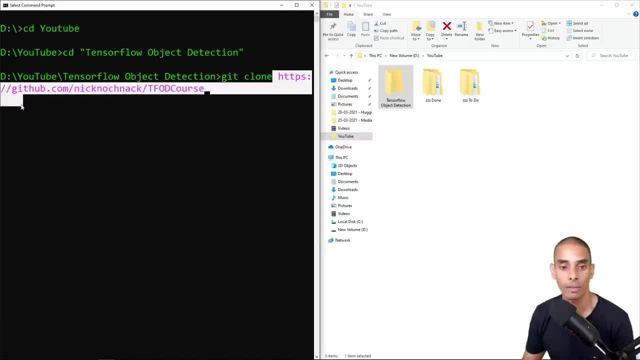 clone and then https colon forward slash, forward slash githubcom, forward slash nick knock, knock, forward slash tfod course. So this is going to give us all of that stuff that you saw inside of GitHub, Right? So it's going to give us the notebooks and a bunch of other. 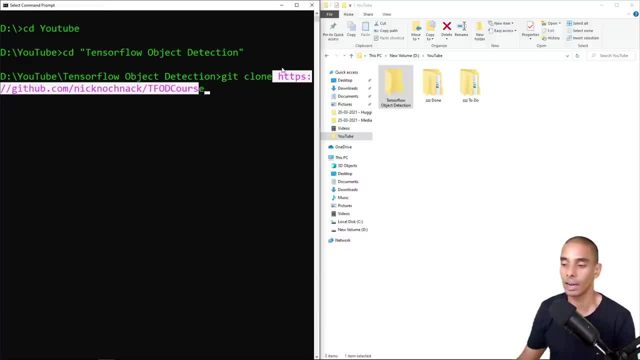 stuff And it's actually going to clone, create a new folder inside of this TensorFlow object detection repository or inside of our TensorFlow object detection folder that we've already got inside of our file explorer. So if we go on ahead and run that, that 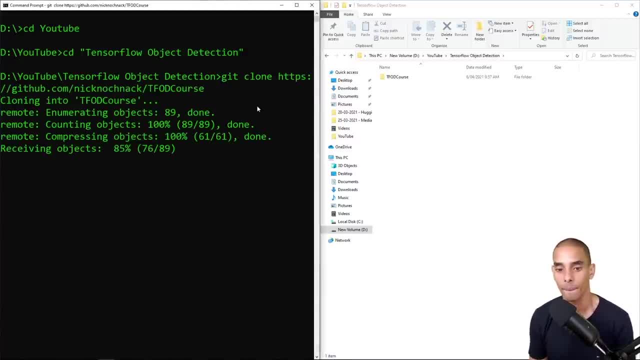 should clone down. You can see it's cloning. We're receiving objects. So again, the speed at which this clones is going to be dependent on your internet. Mine over here sucks, So you can see I'm getting 2.39 megabytes. 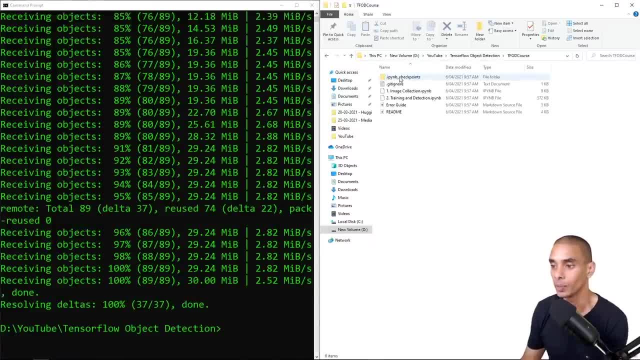 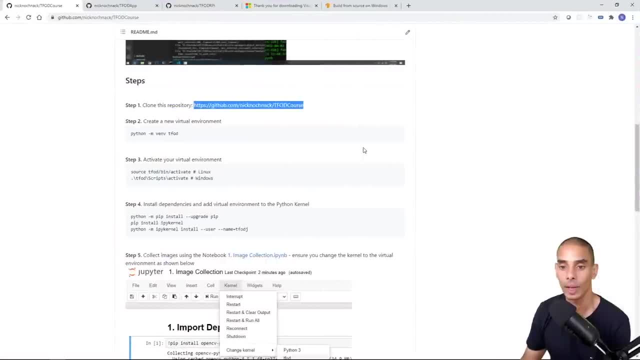 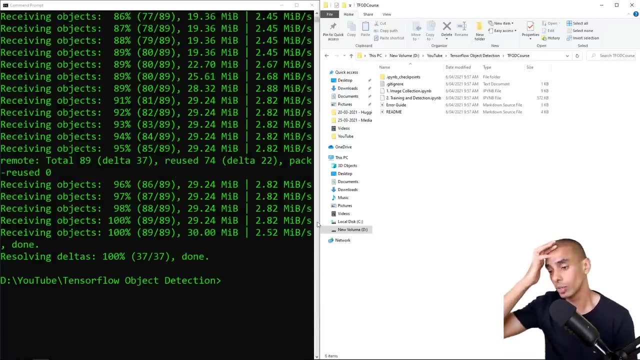 per second In this case. that's now done. All right, cool. So we've now got our repository clone. So, again, everything that you saw over here is now over here locally. So what we now want to do is start creating our environment. So in order to do that, as I was saying, we're going to use that. 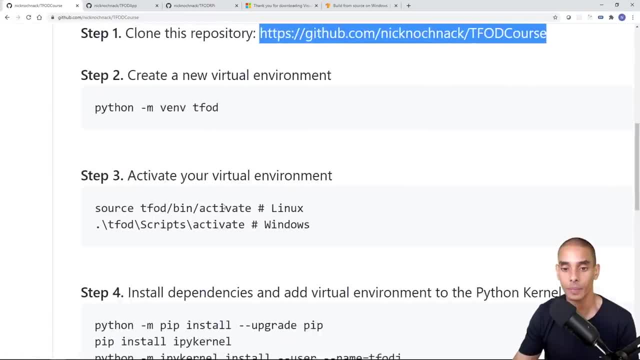 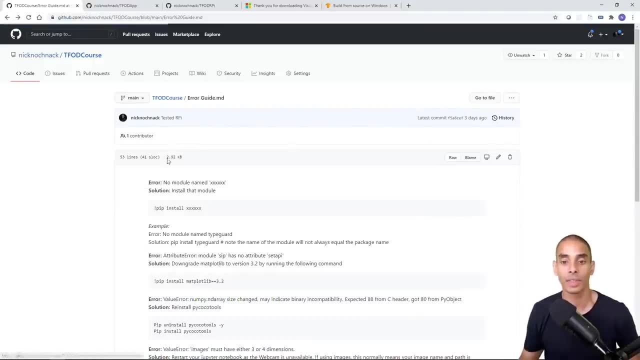 venv package which we had over here. So we're effectively going to go through steps two and three now. So we're going to create our virtual environment and then we're going to activate it. So think of activating it, as actually we've actually stepped out of that. Think of activating. 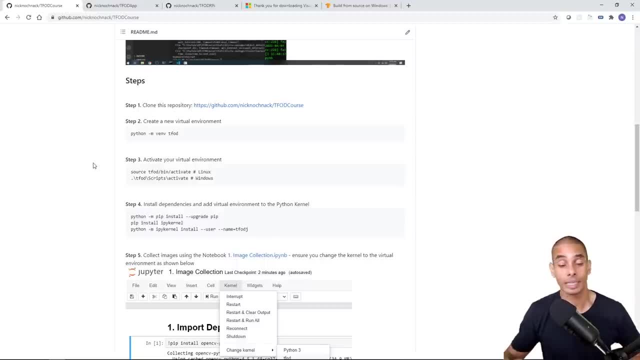 it as actually stepping into that room. So I said, creating a virtual environment is like creating a new room in your house. Well, activating it is actually like stepping into that room. So you're now inside of that environment where you're going to isolate your libraries. So we're first up going to create a new. 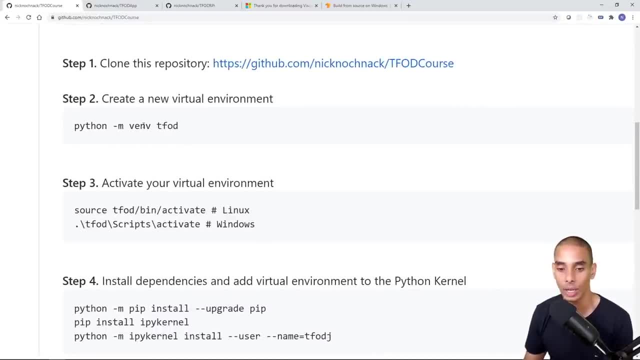 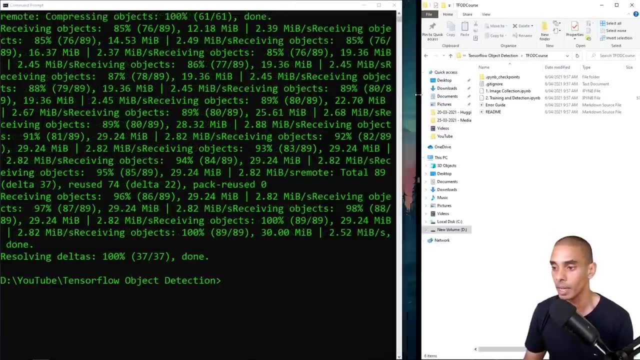 environment, and we can do that using this command here. So python dash m venv tfod. Now the tfod. I'm just going to make this a little bit bigger. The tfod at the end of that is actually the name of the environment that we're going to be. 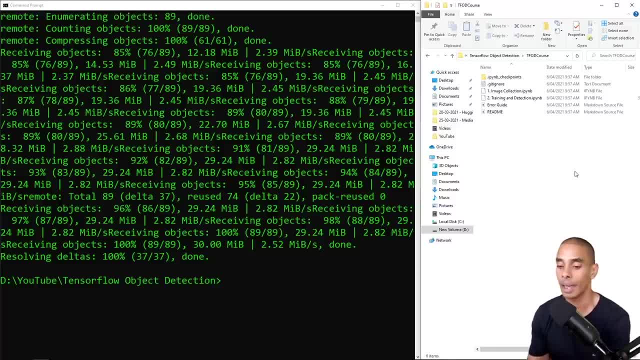 creating. So if you wanted to name it something differently, you could. If you wanted to name it my special environment, you could. You can name it whatever you want. So in this case, I'm just going to clear this using CLS, If you're. 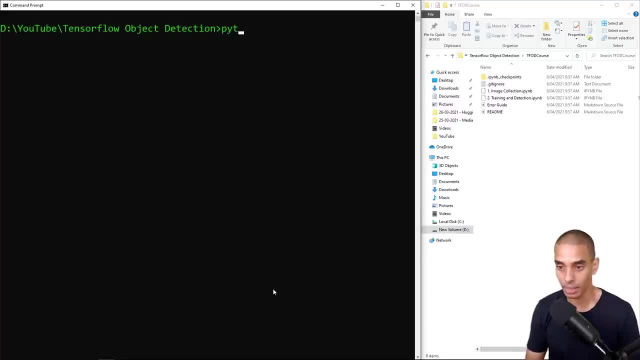 on a Mac. it's going to be clear and we're going to do that. So python dash m, venv tfod. So what I've actually written here is: we're using Python, We're passing the m flag and then we're going to be using venv. 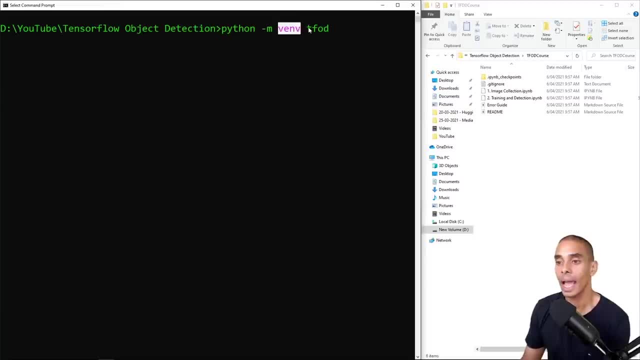 which is the dependency that we're using, And then we're going to be creating a new environment called tfod, So our virtual environment. think of it as our new room is going to be called tfod. So if I hit enter, 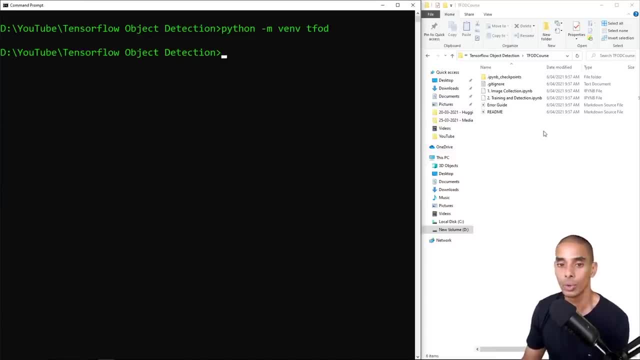 what you should see is that we're now creating a new. we should have done it inside of there. Let's delete that. All right, that's my error. Again, there's going to be errors. stuff breaks. This is sort of what I want: to show you The realities of actually doing this. So we're going to delete this here. We're actually going to do it. 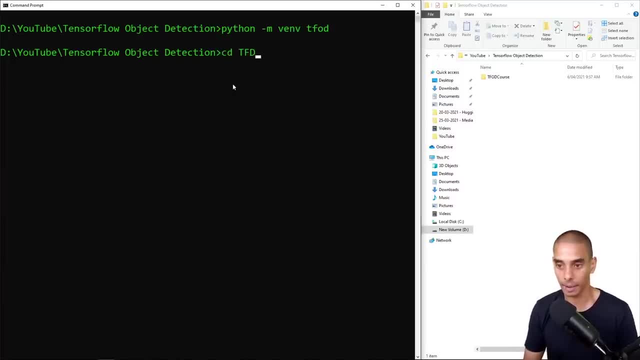 inside of this tfod course folder. So we're going to cd into that And we're actually going to repeat that command here. So you saw that when I created it initially it created it outside of there. So we're going to go into this folder now and create it in here. So let's do it again. 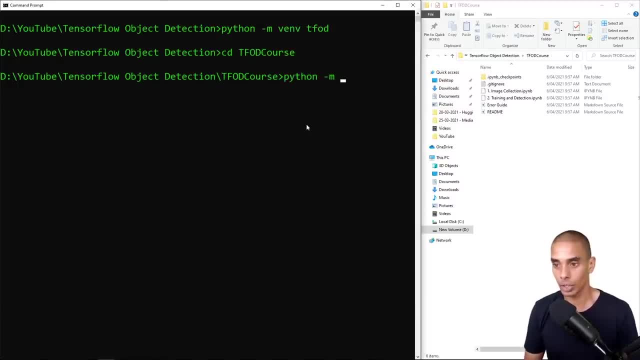 So we'll type in python dash m venv tfod. So now it should create in here. And the reason that I do this is I just like keeping everything isolated. So the main training code, I like having it in one section. The app code, I like having it in a separate section, And then the raspberry pi code I like keeping. 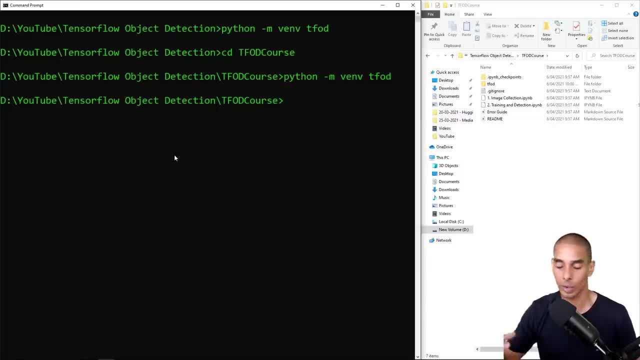 that separate as well. Again, you can play around with this. You can have your environment elsewhere if you wanted to. I just keep them isolated so that I can see what is what. Okay, so you can now see that we've now got our TensorFlow object detection repository created. So if I make this a little bit, 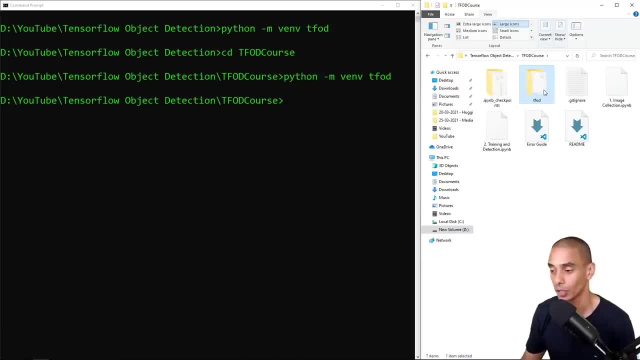 bigger. this folder over here is our TensorFlow object detection virtual environment. So if we open this up, there's a bunch of stuff in here. So in this case it's going to vary depending on whether or not you're doing this on a Mac or whether or not you're doing it on a Windows machine. If you're doing this, 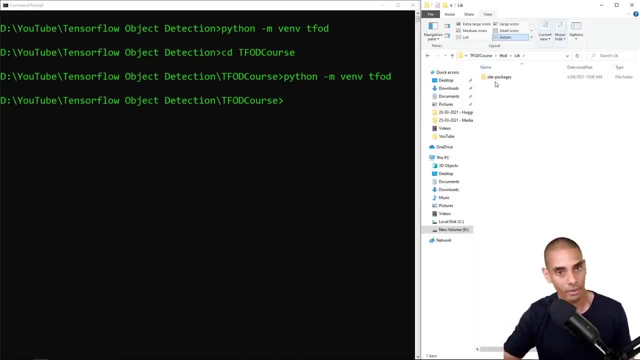 on Colab or on a cloud instance. you don't need to create a virtual environment. So those are set up so that they all run on their own individual pods. So you don't need to go on ahead and do this. But if you're doing it locally- which I suggest you do, because that allows you to do real time detection- 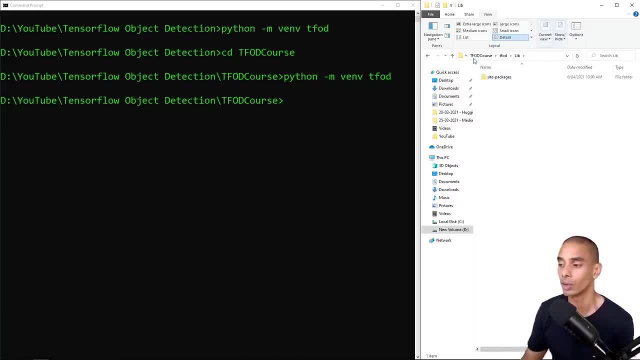 More on that later. Go on ahead and create a virtual environment. So the main thing that I tend to look for is inside of the for windows. If I go into list lib site packages you can see that we've got a bunch of different libraries available. 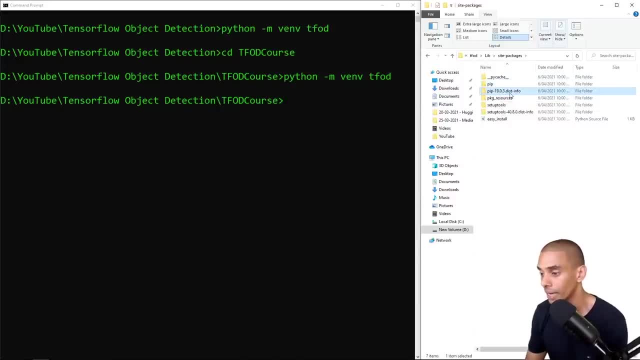 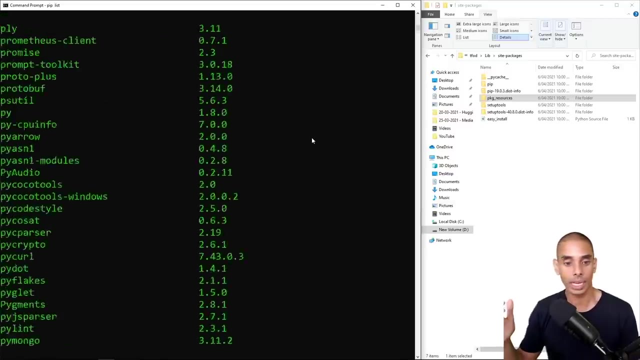 there. So we've got pip, pip dash 19.03. that got this dash info bunch of different packages. right Now, a really important thing is right. So if I type in pip list, which normally shows me the different Python packages that I've got available, you're going to see a ton here right? So I've got a. 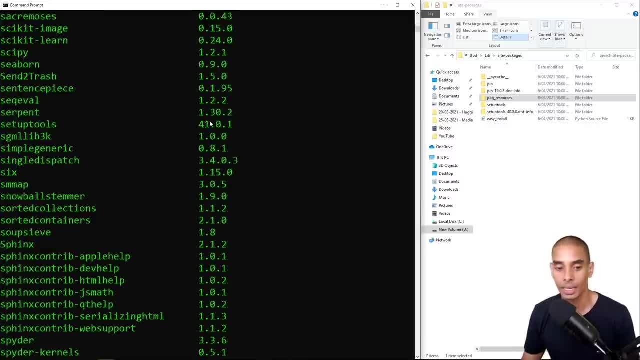 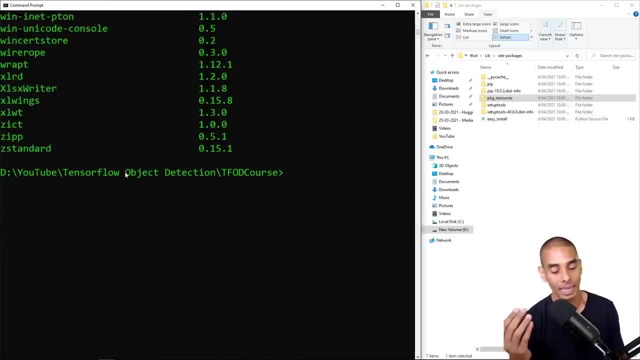 whole heap of different libraries available right now. Now, the reason that you're seeing all of these here, but only a couple here, is because I actually haven't activated my environment yet. Now this happens so often. You need to make sure that you activate your environment in order. 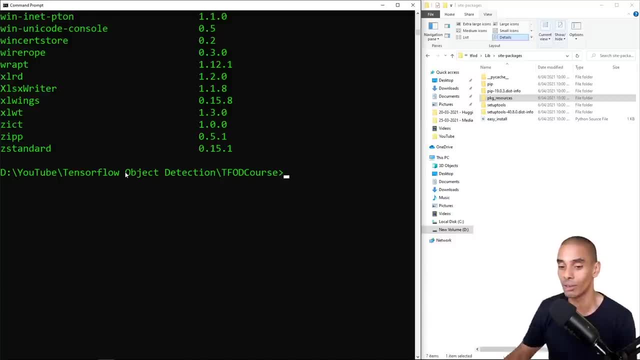 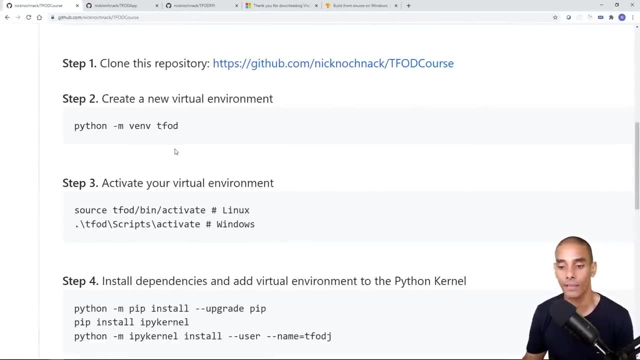 to see, or in order to see your isolated packages that you've actually got in sort. So what we're going to do now is actually activate our environment. Now the command that you use is going to differ depending on whether or not you're running on Linux or a Mac. So if it's on a Linux, what? 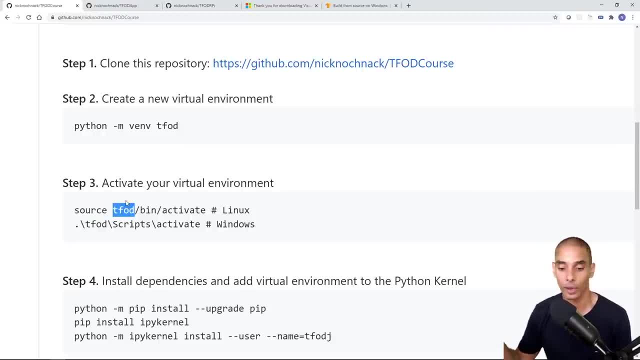 you're going to do is run source TFOD or whatever. the name of your virtual environment is forward slash bin, forward slash activate, to be able to activate your environment. Now, if you're on Windows, I don't know why they made this different, but it is different. It's dot backward slash. 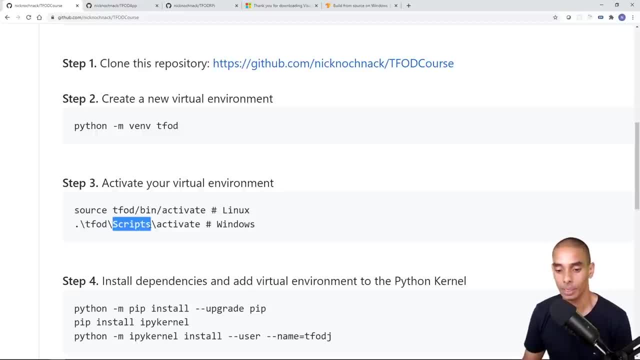 TFOD again, or the name of your environment. backward slash scripts. backward slash activate. So in this case I'm on a Windows machine, So we're going to be using the second command here, So we are going to effectively be going. So, if I go back into our main folder, 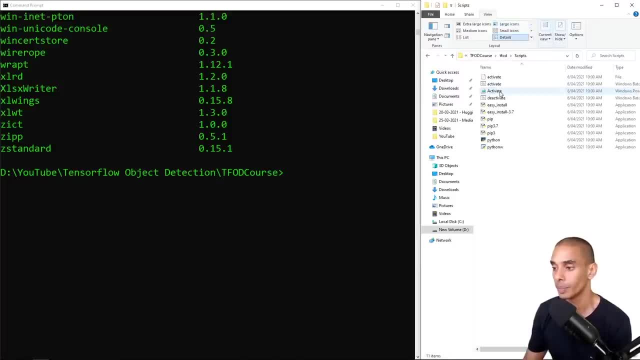 we'll go into TFOD, We'll go into scripts and we're going to be running activate, which you can see over there. So there's an activate file and an activate batch file. So let's go on ahead and run that. So we're going to backward slash TFOD, backward slash scripts. 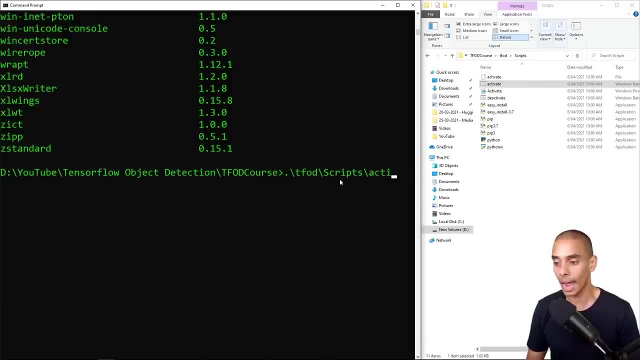 backward slash, activate And watch what happens once. I actually run this right. So right now we don't actually have we don't, we're not actually inside of our virtual environment. If I run this, you now see that we've got this little thing over here. So this: 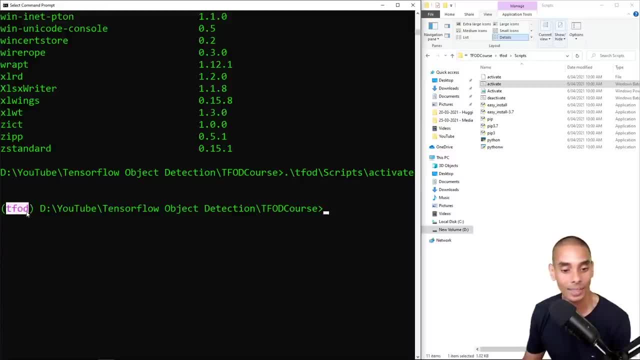 tells us what virtual environment we're actually in. So we're now inside of our TensorFlow object Detection virtual environment. So again, we've now stepped into our new room. Now, if I type in pip list, you'll see that it's way shorter right. So this actually represents. 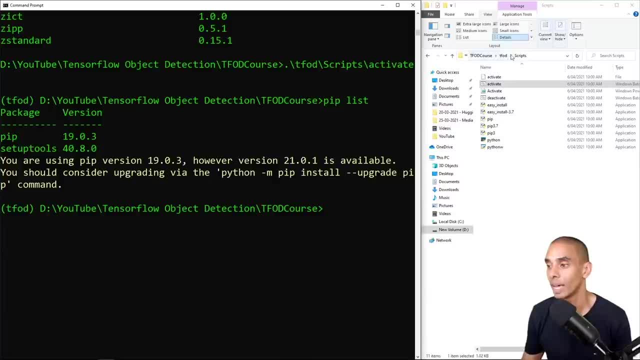 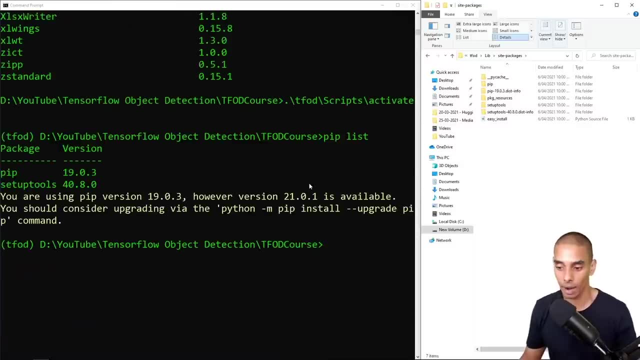 the actual sets of libraries that we actually had available inside of there. So remember, all of these packages are here. We don't have all of these over here Now. if you wanted to deactivate the environment later on, all you need to do is type in deactivate. This is going to. 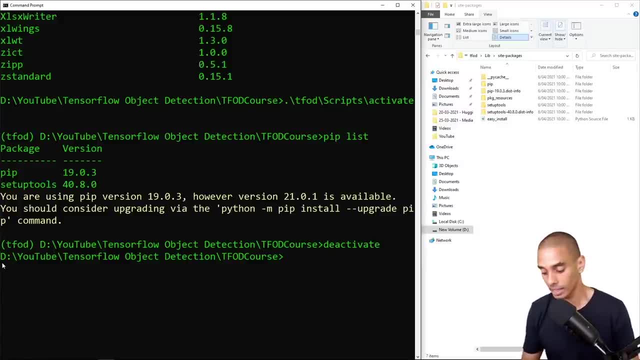 step out of it, right, So you can see that the TFOD is now gone. In this case, we actually want to activate it, So let's do that. TFOD scripts activate. So we're now back in. So you can see that we're now there. All right, we're going to clear this, clean it. 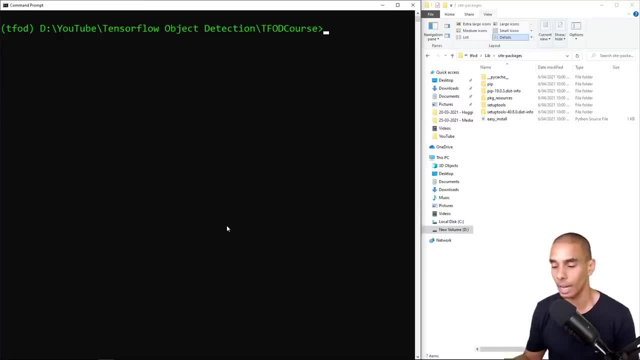 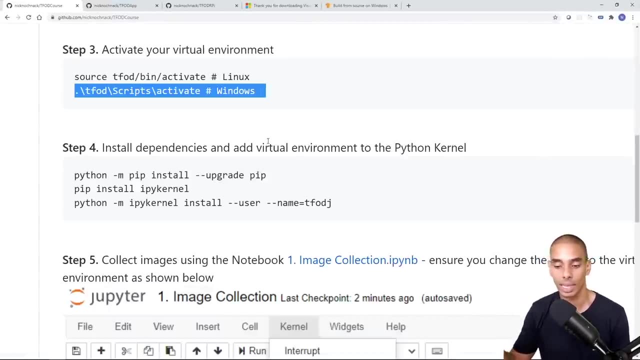 up. The next thing that we need to do is install a couple of key dependencies. So the first one is we want to upgrade pip. So this is going to make sure that we update using the latest resolvers and that we've got the latest pip package, And in order to do that, we just need to run this command here. So 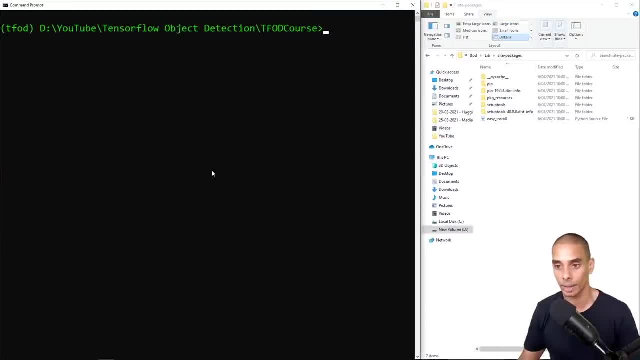 python-m: pip install- dash dash, upgrade pip. So let's do that. We're going to type in python one: dash m- What was it again? pip install- dash, dash, upgrade pip. pip install- dash dash, upgrade pip. So this is going to upgrade our pip installer. 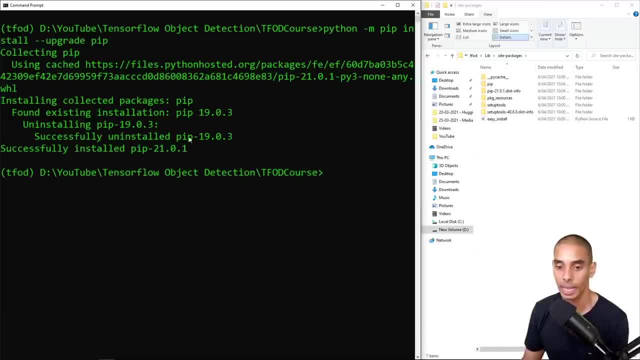 And you can see it's uninstalled 19.0.3 and it's installed 21.0.1.. And the thing that you'll notice is that as you're updating these packages, you can see them updated inside of our site packages folder as well. 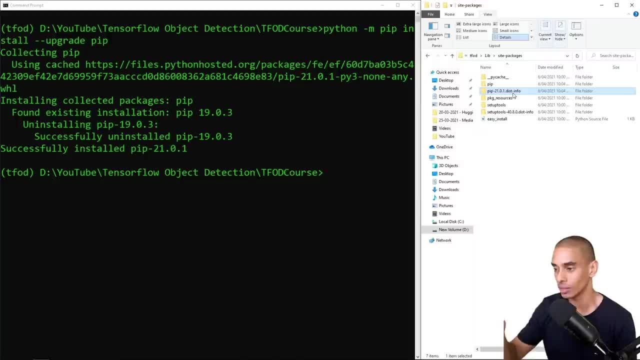 Now, this just makes your life a whole heap easier, because you can actually see what's being installed in real time. Now, when it comes to actually installing TensorFlow, you'll actually see that this is really useful, because sometimes you need to run through the install multiple times to make sure they're installed. But I've actually also got a verification. 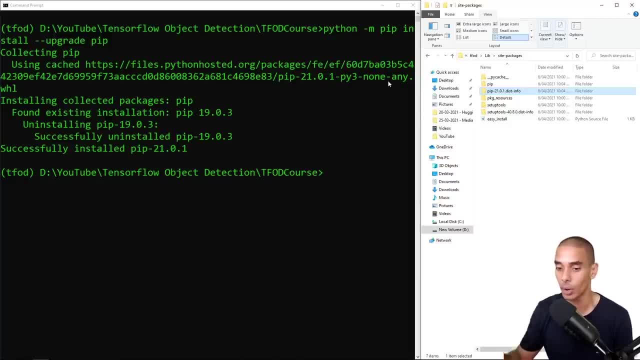 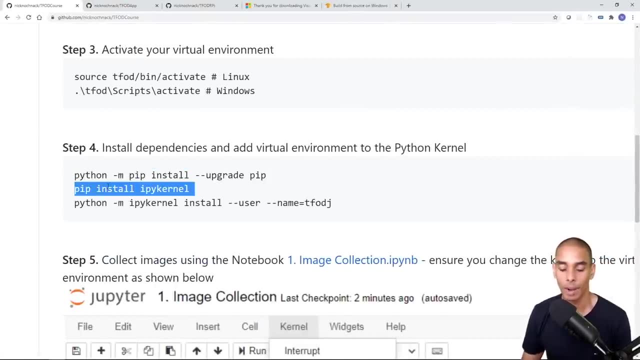 script as well, to make sure that we've got all the right packages to be able to go on ahead. Okay, so we've now gone and upgraded pip, So the next thing that we want to do is install ipyekernel. So ipyekernel allows us to associate our virtual environment with our Jupyter Notebook. 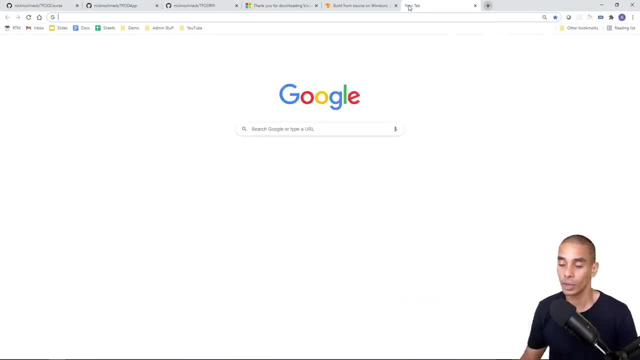 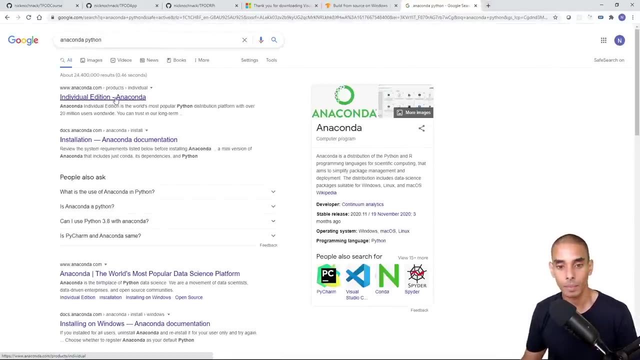 So we're going to be mainly working with Jupyter Notebooks. If you're installing Jupyter Notebooks for the first time, I'd highly recommend go to Anaconda Python So you can actually install Anaconda and this is going to give us, or give you, a bunch of Jupyter Notebooks. 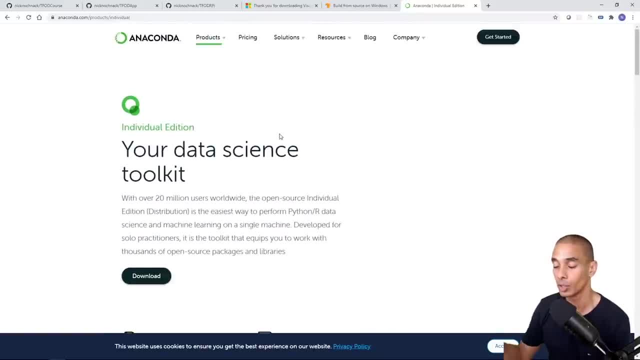 Jupyter Labs to be able to get this up and running. If you don't have Jupyter Notebooks installed already, I'd highly recommend just running through this Reasonably straightforward to get up and installed. I've got a video on installing that separately that I can link to you as well. 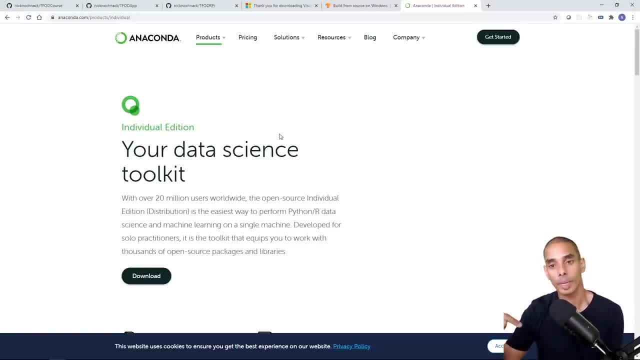 So let me know in the comments below if you want that. Also, let me know in the comments below if you like this sort of format- me sort of just walking through and giving you an idea as to how to actually go through this. I'm always welcome for feedback. If there's anything you do like or you don't like, by all means do let me know. 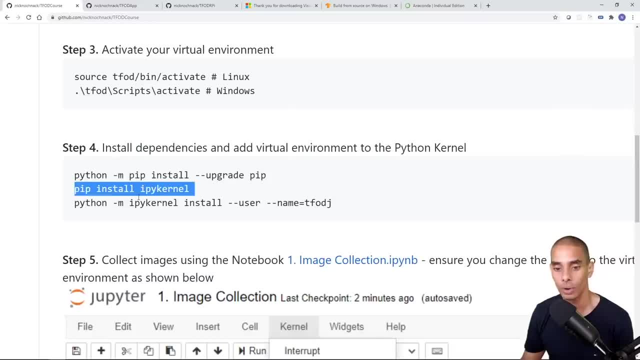 Okay, so where are we up to now? So we were installing ipyekernel, So let's do that. So again, ipyekernel allows us to associate our virtual environment to our Jupyter Notebook. So first up, we need to install it, And then the second line here is actually going to allow us to associate. 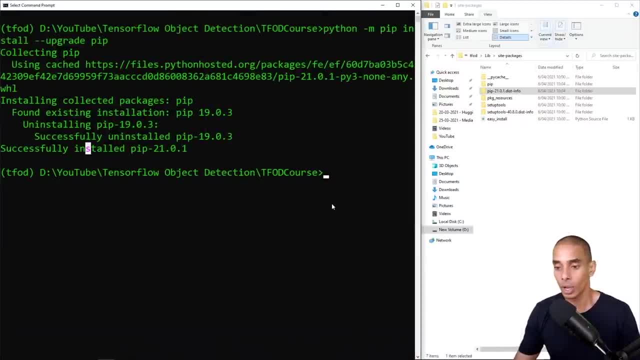 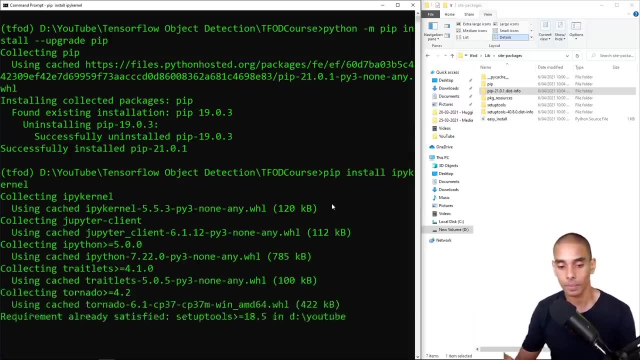 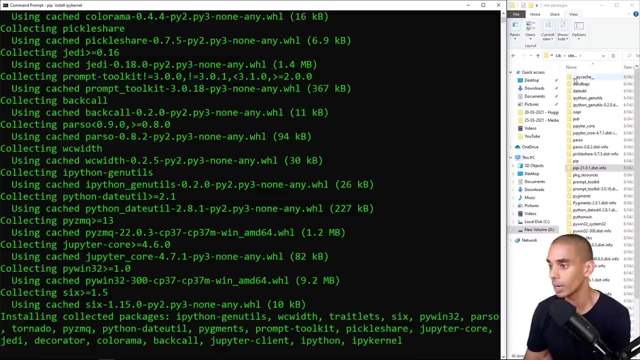 a little bit of a typo there, That's fine. So let's go on ahead and install ipyekernel. So, pip, install ipyekernel. Let's make this a little bit bigger, And again you can see that we're installing libraries over here. 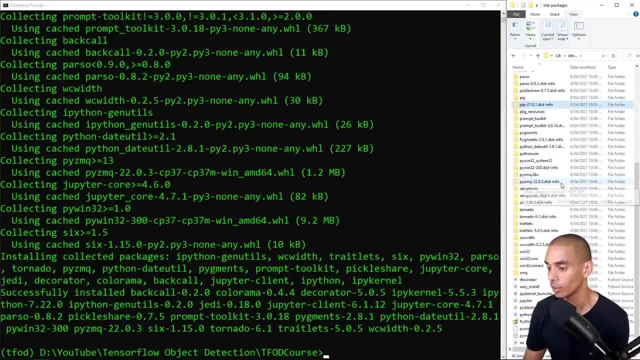 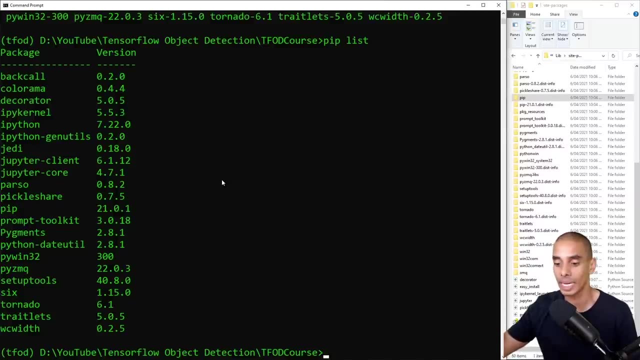 We can hide our navigation pane so you can see that these are all being installed now, right Now. if we type in pip list again, you can see that we've now got additional packages. Now the next thing that we want to do is actually install a virtual environment into Jupyter. 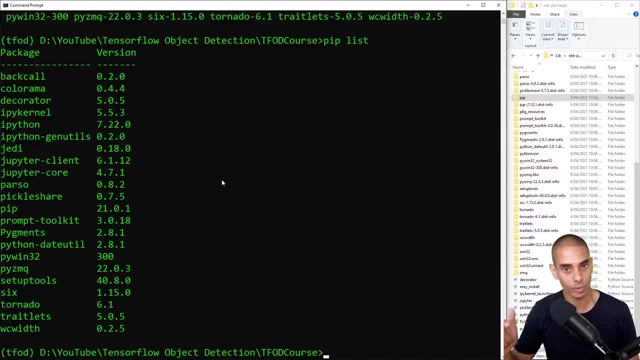 So this is often where people come unstuck when using virtual environments with Jupyter for data science workloads. You need to install it into your Jupyter kernel notebook, So this is going to give you the ability to see that virtual environment associated to your notebooks. 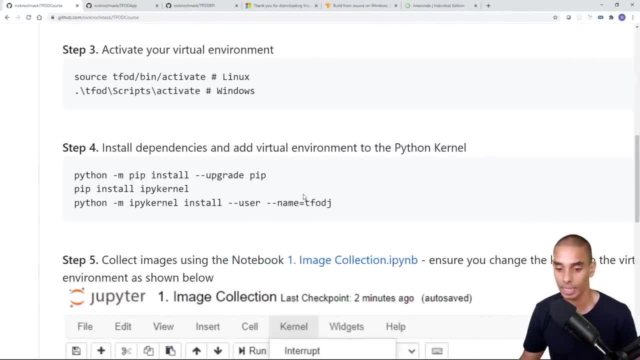 So in order to do that, we're going to be running this command So python-m- ipyekernel. install dash dash, user dash dash. name tf equals tfod, So let's go on ahead and run that So ipyekernel. 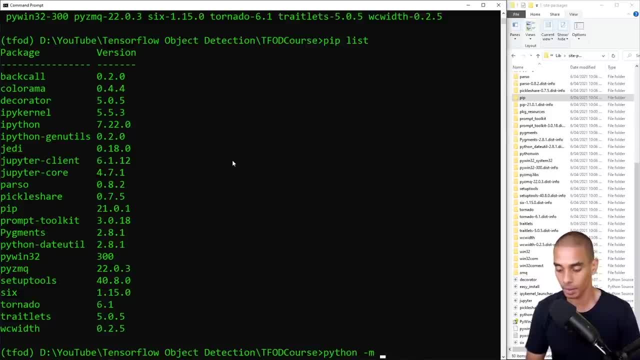 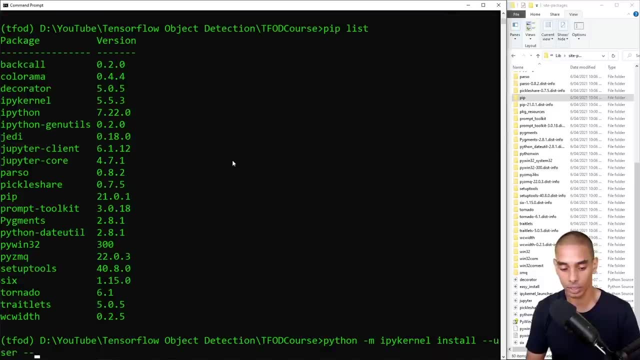 So python-m, what was it again? I already forgot- ipyekernel install dash dash user. dash dash name equals tfod. That should be right. So actually, let's clear this, so we can actually see it a little bit better. 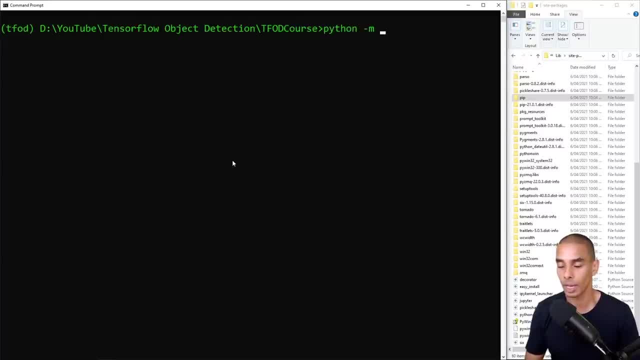 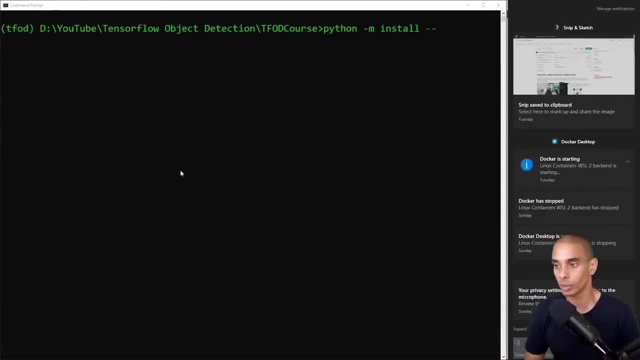 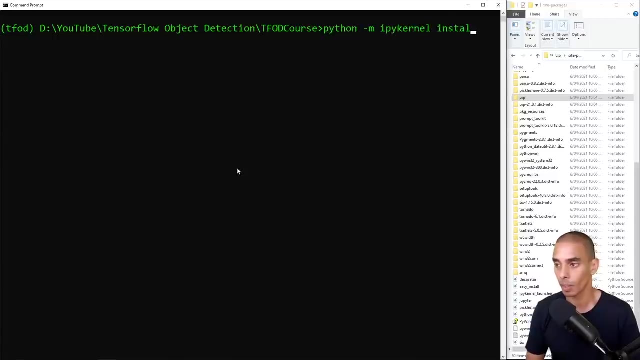 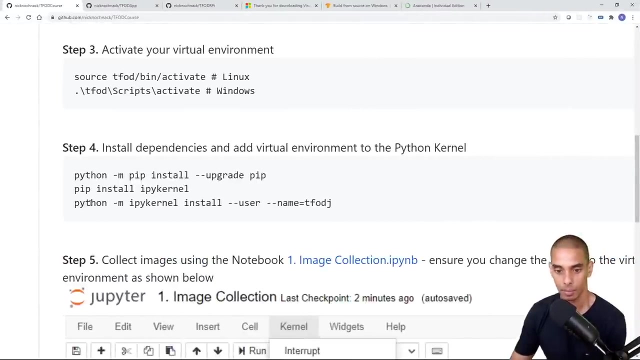 So what was it So? python-m install. python-m ipyekernel install. Not bad. python-m ipyekernel install. python-m ipyekernel install. python-m ipyekernel install. Okay, let's check that. python-m ipyekernel install. dash dash user. dash dash name: tfod. 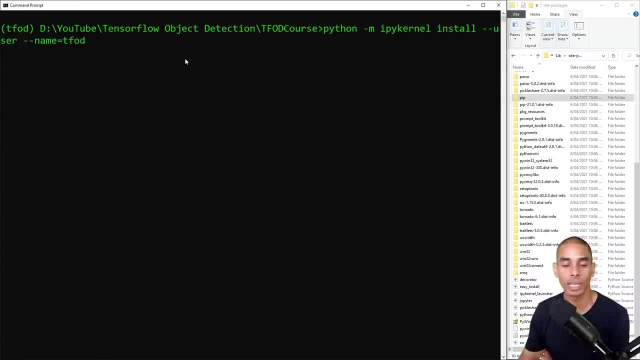 Yeah, it's all good. Now I wanted to call this out. So this last bit here is effectively telling the ipyekernel package what the name of your virtual environment is. So if you change the name of your virtual environment, you need to make sure that you change this name here. 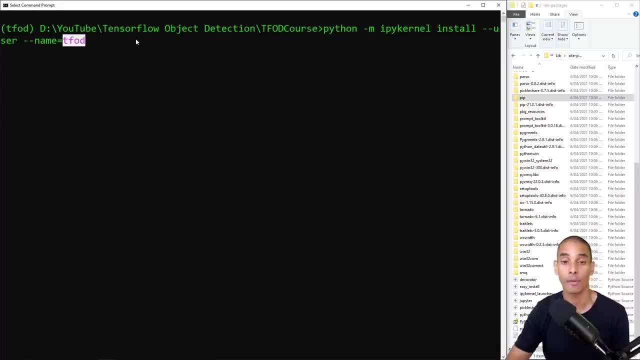 So say, for example, when I created my virtual environment, I wrote python-m venv- my special environment. When I go to install that virtual environment into my Jupyter notebooks, I need to change that name here, So in that case it would be my special virtual environment. 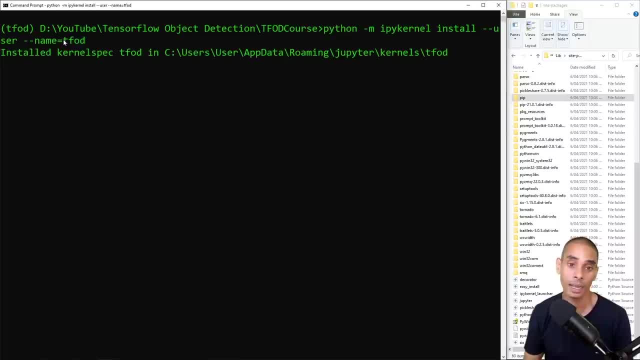 whatever you called it. So in this case, if I hit run, that's going to now install it, So you can see installed kernel, spec tfod and blah, blah, blah, blah. So now we've actually got that particular virtual environment. 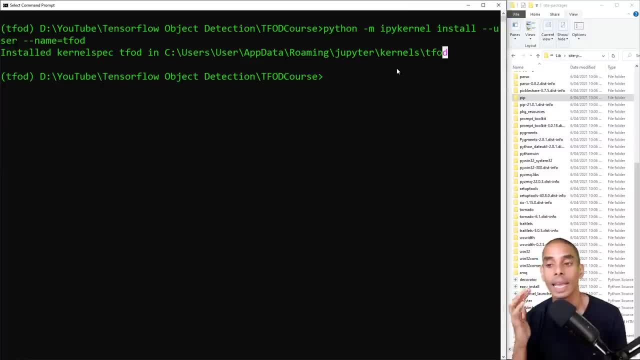 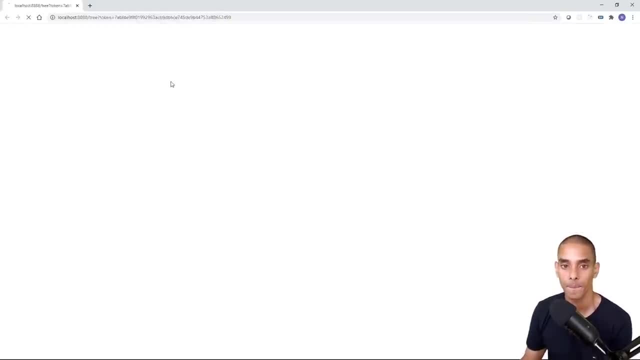 available inside of our Jupyter notebook. Now, an easy way to validate that is just start up Jupyter notebooks And if you create a new dummy notebook, even if you just hit new, so you'll see that we actually have tfod available there. 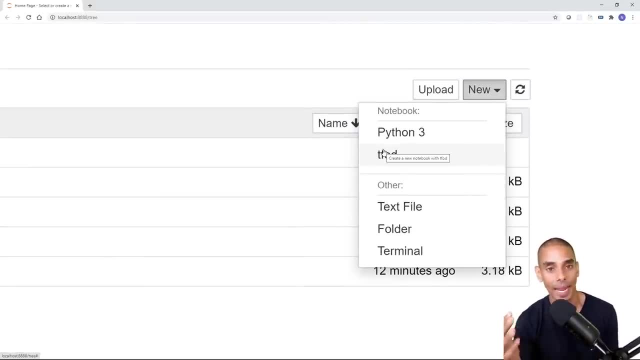 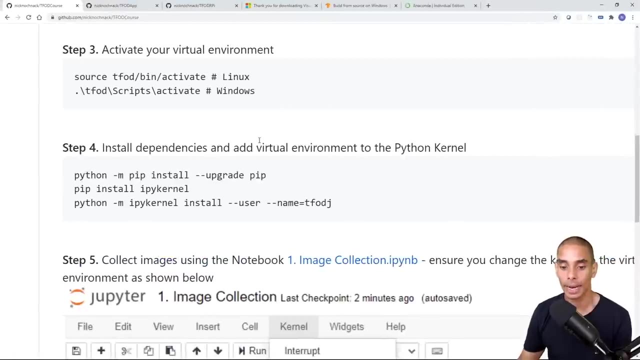 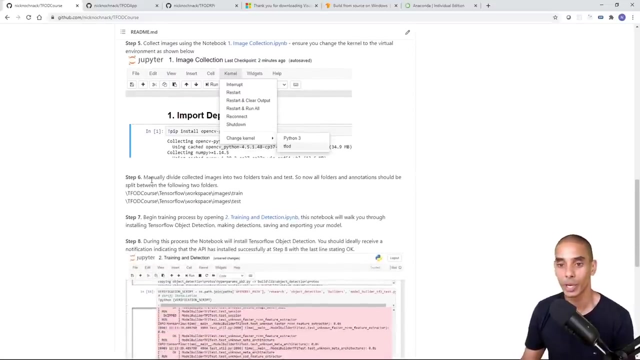 So that is our virtual environment now made available. So now we can actually leverage that virtual environment when we work with our notebooks. Cool, All right. So that brings us to step numero five. I don't know how to say five in Spanish, unfortunately, but step five. 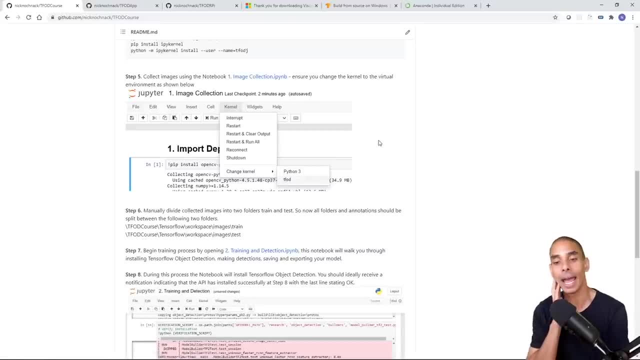 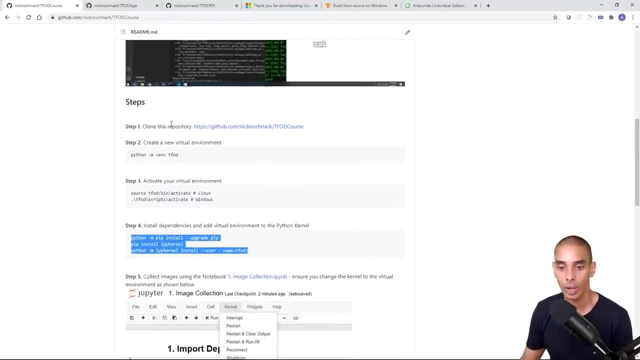 All right. So we're now up to here, where we're actually going to go on ahead and collect our images, All right. So up until now we've sort of done quite a fair bit. So we've gone through and set up our virtual environment. 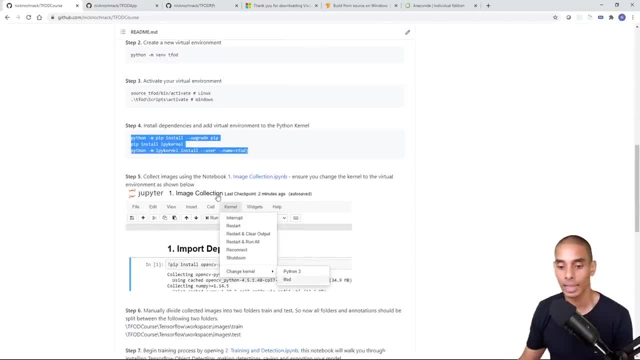 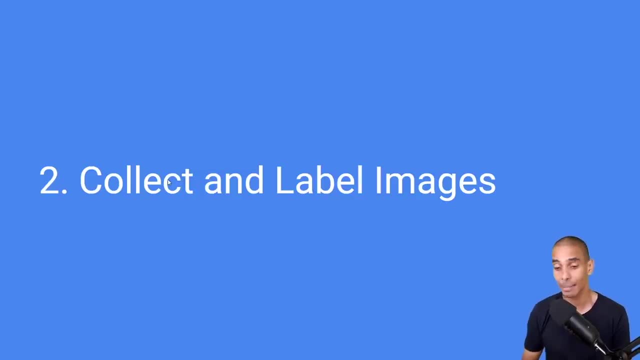 And that's our baseline setup now installed. Now the next thing that we're going to be doing is, as I was saying, collecting our images. So let's go back And we're now going to collect and label our images. So part two is collecting and labeling our images. 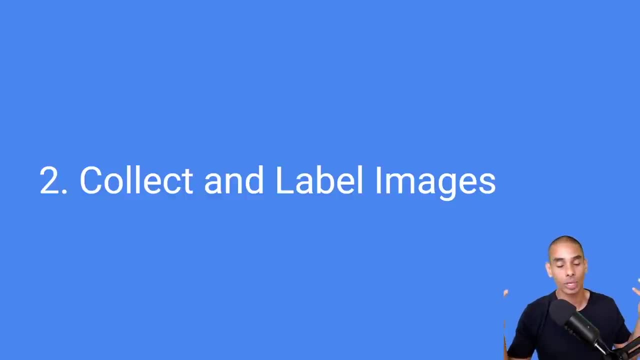 So remember, cast your mind back. What I was saying is, when we actually go and leverage deep learning models, we're going to be passing through data, aka images and answers, Aka our labels, to be able to train our object detection model. 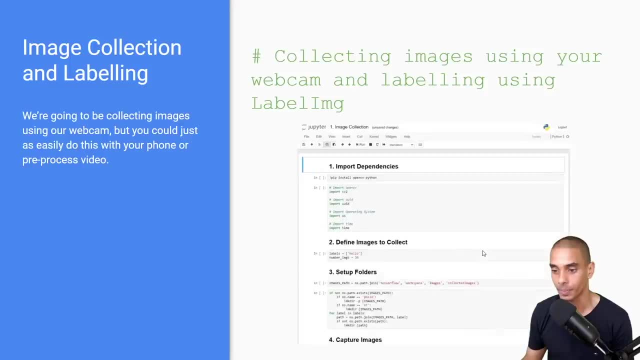 So collecting and labeling good images is really, really important. Now, in this case, to be able to collect and label our images, we're going to be leveraging this Jupyter notebook that you've got here, which is one dot image collection. 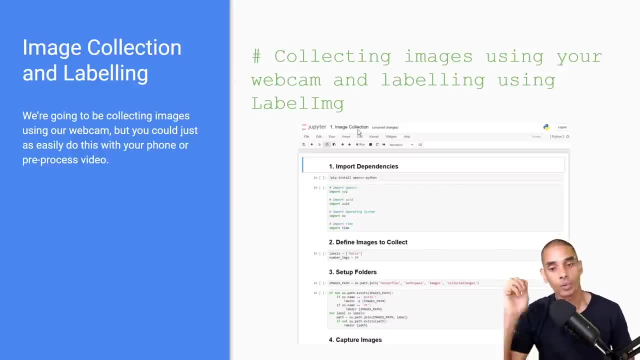 And we're going to be using a webcam. Really important thing to know is if you're doing this on your machine. you need to be able to have access to your webcam in order to be able to actually collect images using your webcam. Now, when it comes to labeling, 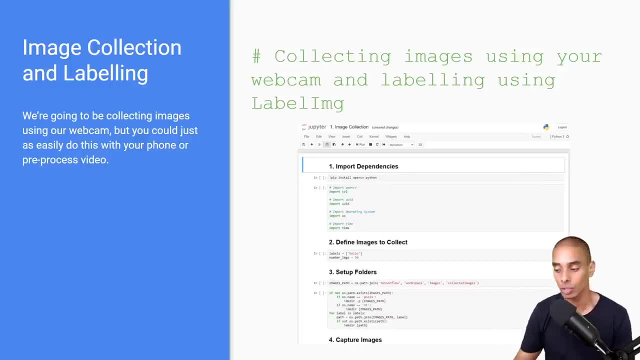 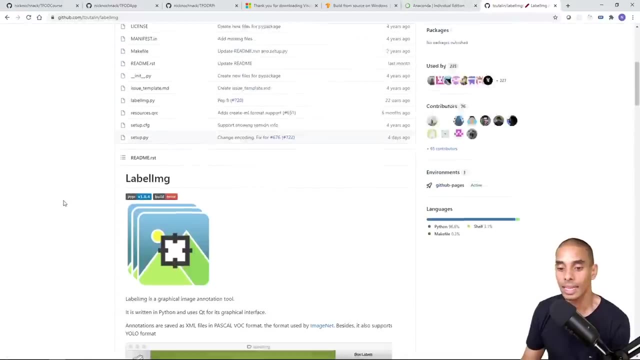 we're going to be using a library called label image, So if I actually go back, I can show you what that looks like. So label image, And this allows you to label different images within an image. So in this case, it's really really simple. 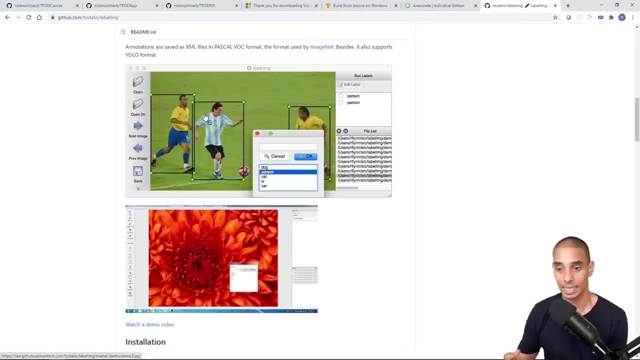 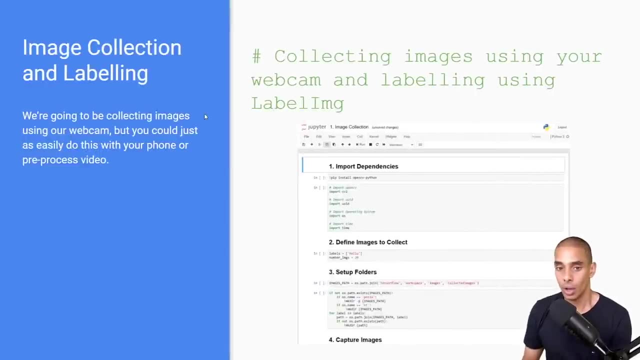 And it's really sort of fit for purpose- Nothing crazy that actually is involved in actually doing this. So we're going to be using that as well And I'll sort of walk you through setting that up. Okay, Now in terms of best practices. 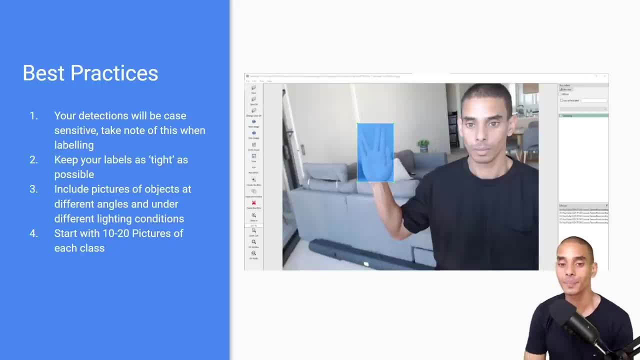 there are a couple of things to note. So when you're labeling, keep in mind the case that you're actually passing through your images. So you want to make sure that the names that you pass through when you're actually labeling them are the specific case. 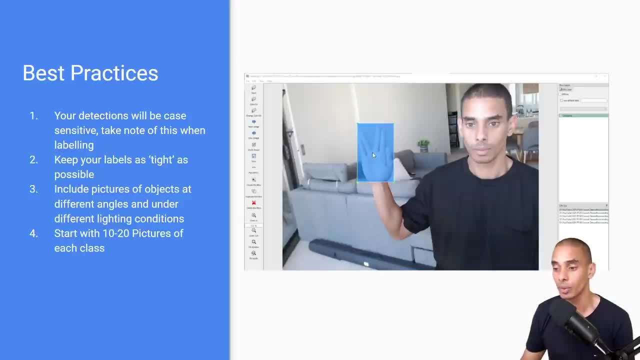 that you want to render. So in this case, if I name this completely lowercase- live long. when I go to actually train my model, the label that I pass through needs to be live long as well. So, again, I'll talk about that a little bit later. 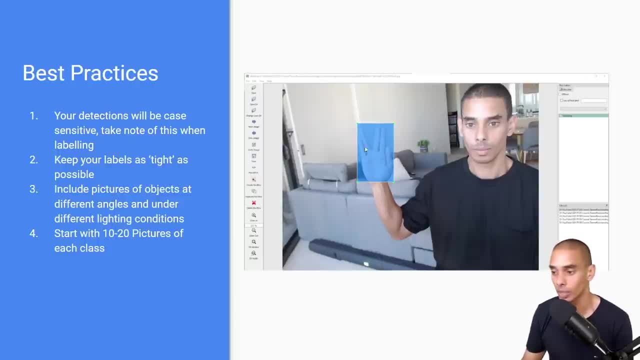 Keep your labels as tight as possible, So don't be going. So in this case, I was labeling the live long sign. Don't create a big square around it, right? So you want to keep these labels as tight as possible in order to make sure that your model is able to detect. 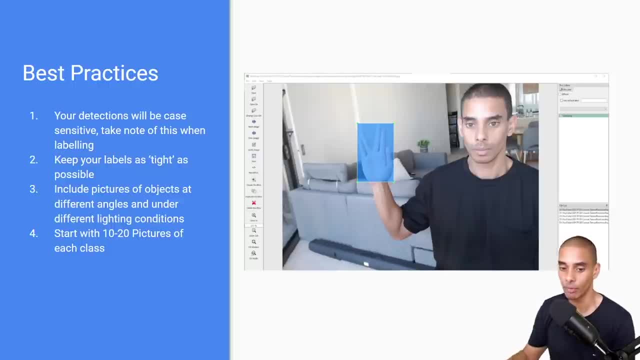 specifically that object right- This helps a lot when boosting performance- And then include pictures of objects at different angles and under different lighting conditions. So what I tend to do is I'll actually like so if I'm doing gesture recognition, for example. 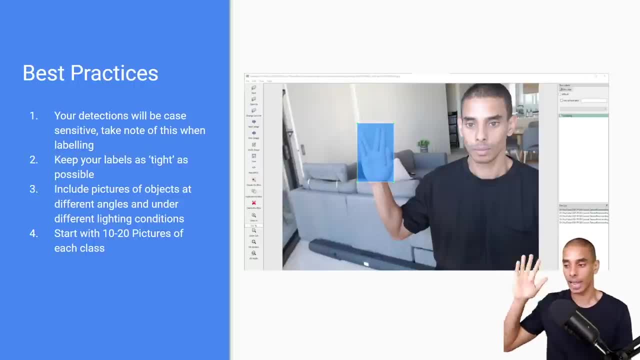 let's get my hand in the photo, So I'll actually move my hand around. I'll look at different angles, at different lighting positions, so that my model learns to generalize better. So, ideally, what you want your model to do is perform well. 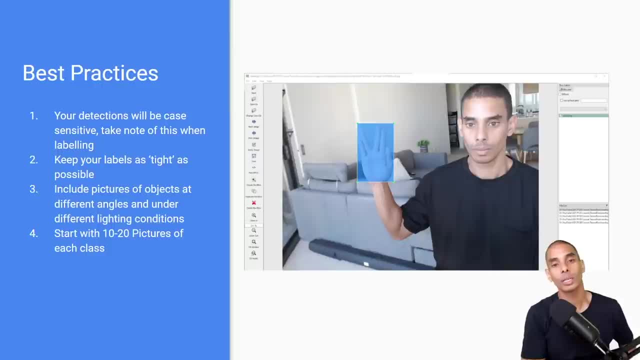 not only on your training data, but also in the real world. This is what is known as your model being generalized right? So it works well in general. Now, in order to get a model that performs that well, you want to give it a whole bunch of different types of instances. 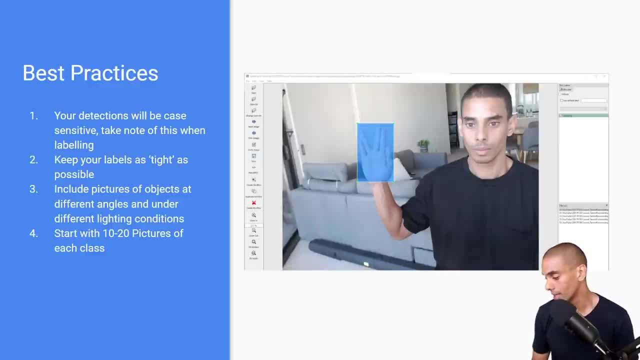 of the object that you're trying to detect. So say, for example, I was trying to detect pictures of my phone. right, If I took a photo of my phone, let's disable that. So if I took a photo of my phone, just like this in the real world, 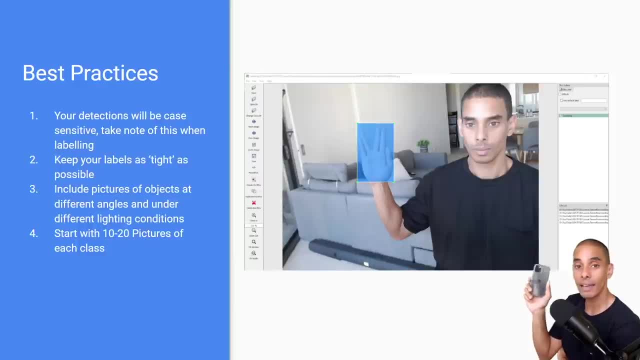 if I then went and flipped my phone, if it had never seen images of a phone that looks like this right with the different cameras, it'd be really difficult for it to detect that right. So ideally you want a whole bunch of different angles. 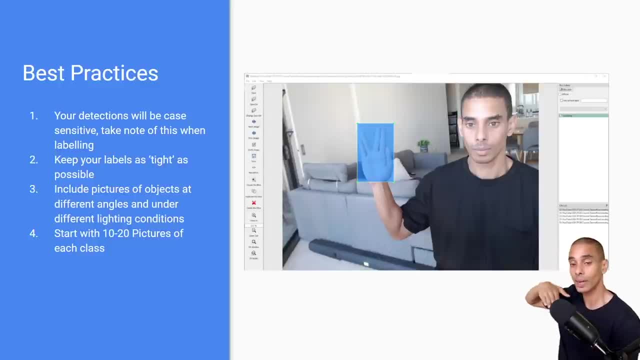 So if you're detecting fish, for example, you'd want to take pictures of the fish front on side, on the other side and the back top, bottom, So your model has a chance to be able to see different angles for that particular object. 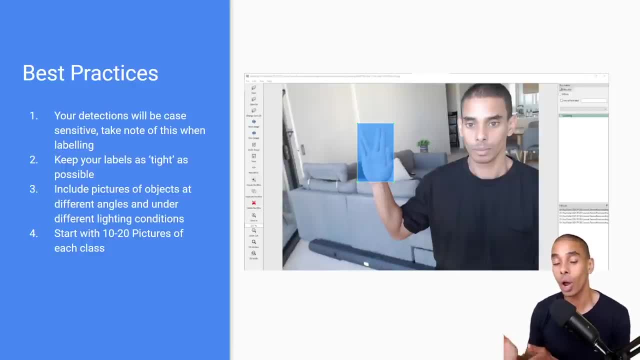 Because if it doesn't, it's going to be really hard for it to know that that particular object is what it is. Another best practice is to start off with 10 to 20 pictures of each class. Now I'm going to start off with way less than that. 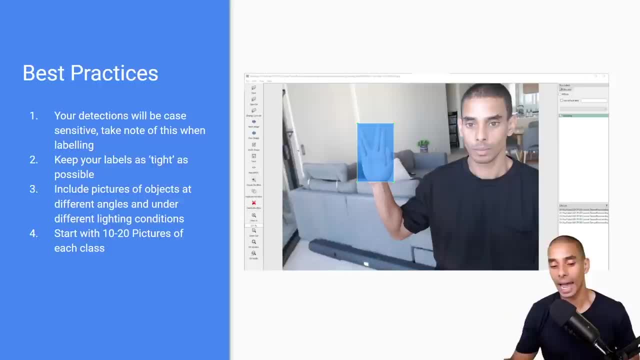 because I'm going to show you what to do if you get sucky performance, and how to add additional pictures, how to retrain. So we're going to start off with less. I think we're going to do five initially. Then we're going to rebuild and then redo this model. 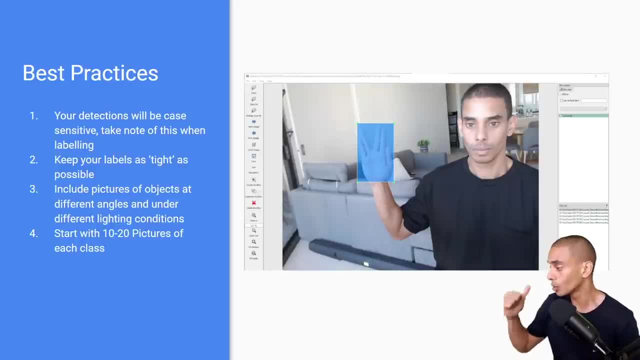 So ideally we should get better performance later on, And we'll also do it with the green screen and without the green screen. So again, we're going to give it a chance to better generalize. So if we've got a green screen in the background, as I do right here- 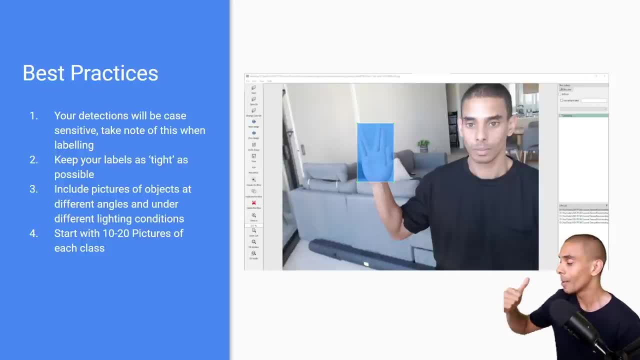 which you probably can't see right now because I've got chroma key on. But if I had the green screen up- and I only give it images where I've got a green screen available- what would happen if I took the green screen down? 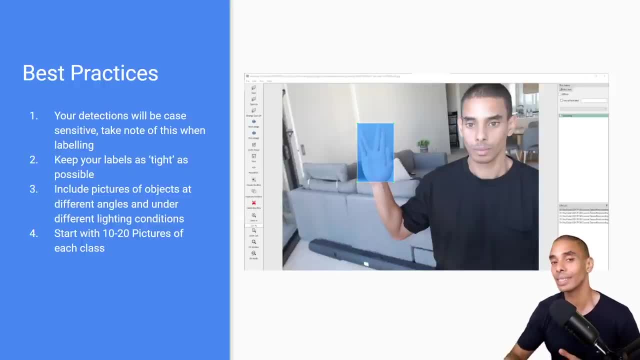 Maybe it might not actually perform that well because it has never seen images of my hand without a green screen behind it. So ideally, you want to give your image, or you want to give your model the best chance possible to actually go on ahead and detect objects. 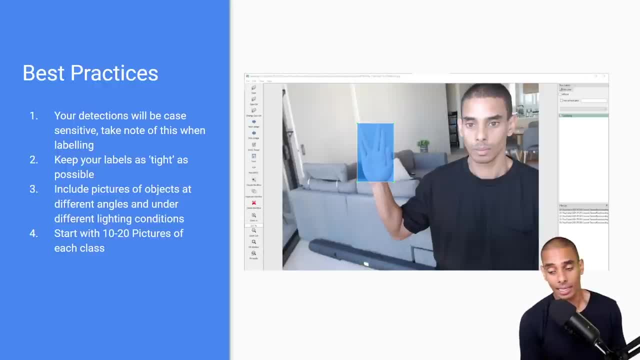 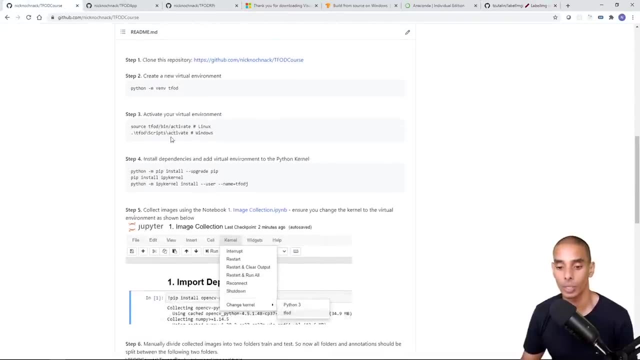 Okay, so, on that note, let's go on, Go on ahead and start collecting images and labeling images. So, in order to do this, we're going to be using one of the Jupyter Notebooks that we cloned down, which is this one here. 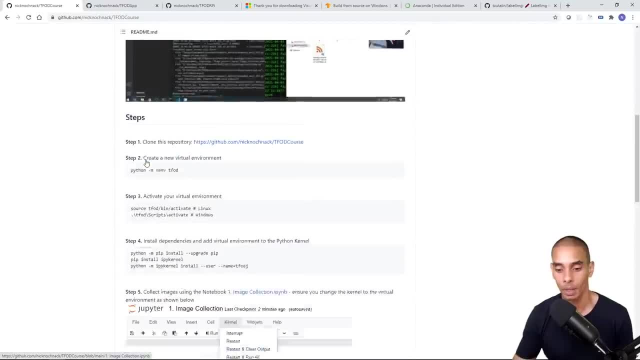 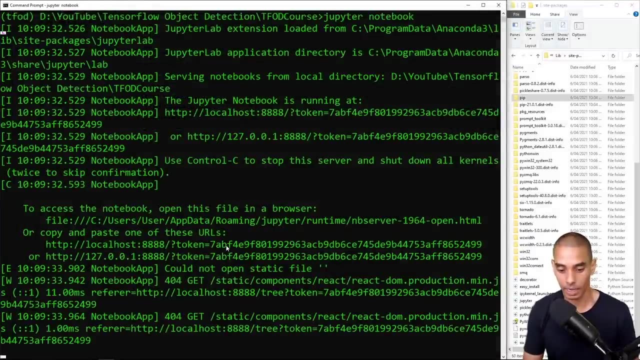 So imagecollectionipynb. So this is step five. So we're now up to here, All right. So remember we started off at Jupyter Notebook. So again, I'll cancel this so you can see it. So let's clear it. 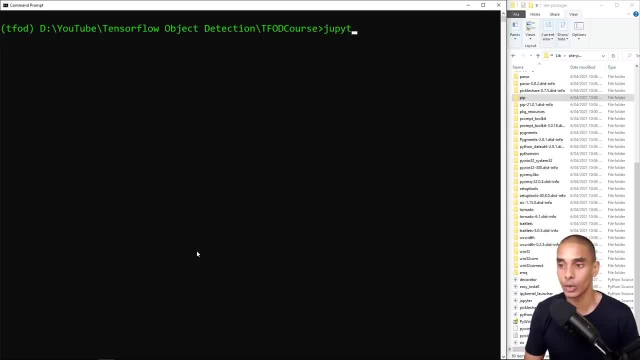 So, in order to do this, I'm just going to start our Jupyter Notebook. So by typing d-a-u-p-y, d-a-u-p-y-t-e-r notebook. So this is going to start up our Jupyter Notebook server that we're able to use. 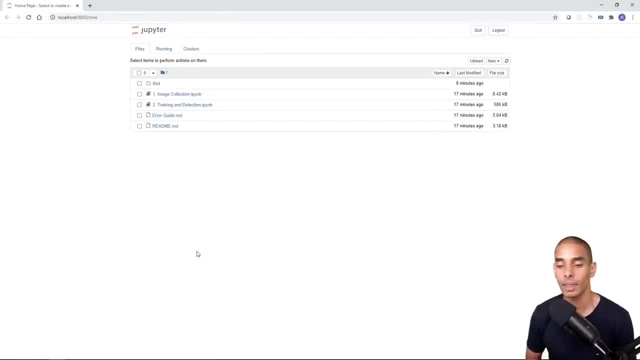 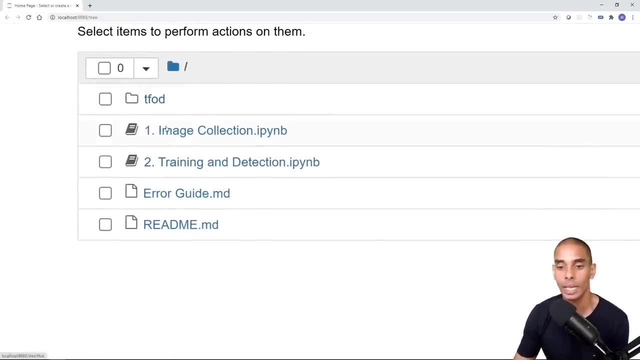 So if we hit enter now, that is now started And you can see inside of here we've got a bunch of stuff. So we've got our virtual environment. so tfod, We've got that image collection notebook, so oneimagespacecollectionipynb. 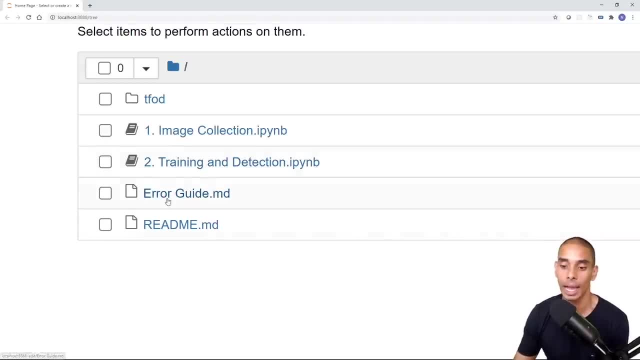 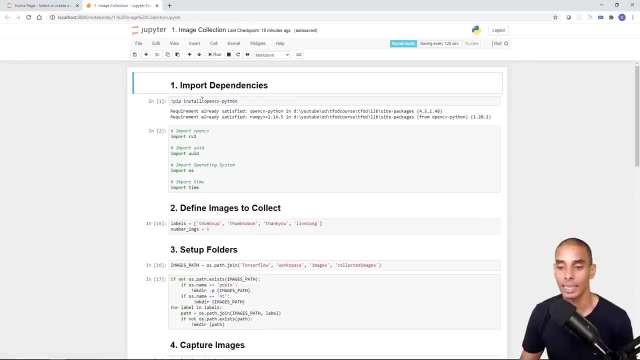 We've got our training and detection notebook, which we'll talk about more later, Our error guide and our readme. So we are going to start off with our image collection component, All right. so if we select that, that's going to open up our notebook. 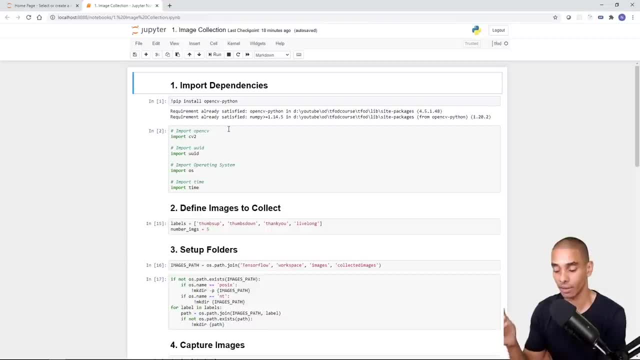 And then we're just going to step through this particular file. So what we're going to do is we're going to step through it, So I'm going to hold shift and enter on my keyboard. This is going to allow me to step through each one of these cells. 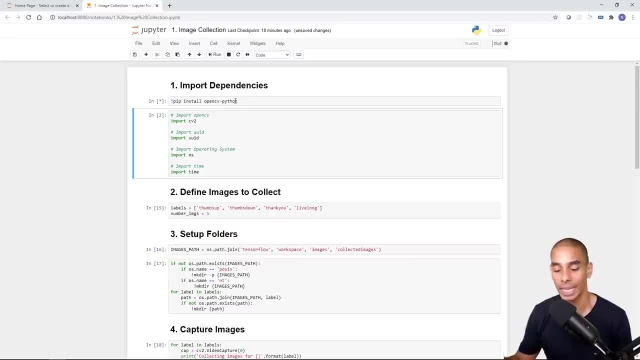 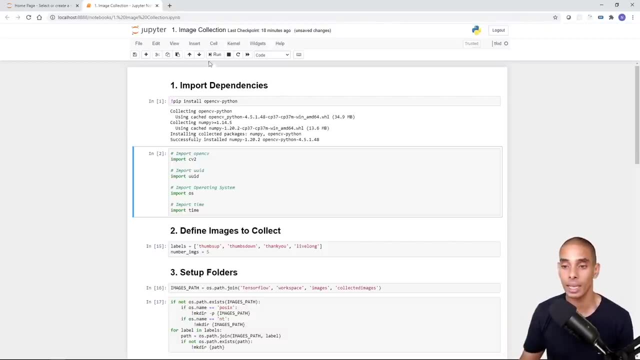 So shift, enter, And this first line here is going to install OpenCV. So this is a new dependency that we've actually got available Now. a key thing to note is that, when you're running this, what I want you to check is either over here in the top left-hand corner: 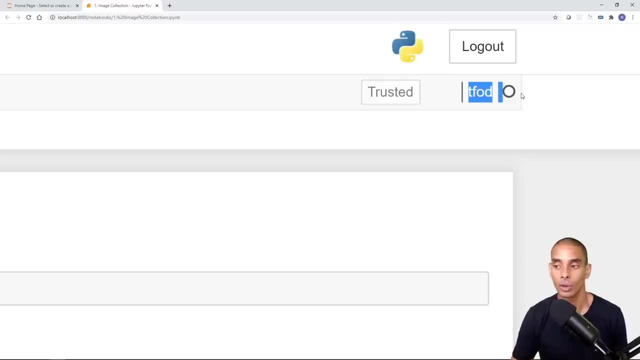 the name of your kernel that you're using is the same as your virtual environment. So if it's not the same, that means that you're not currently working inside of your virtual environment, So you're not leveraging that pre-isolated environment that you went and created. 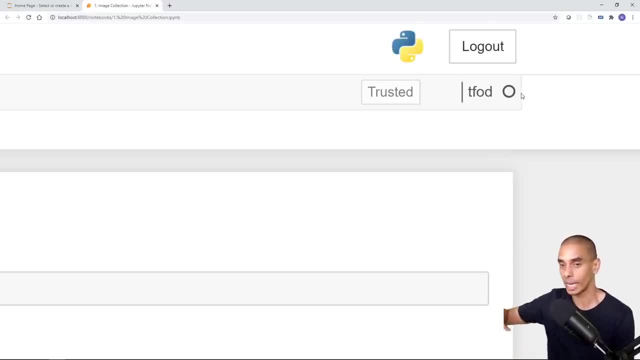 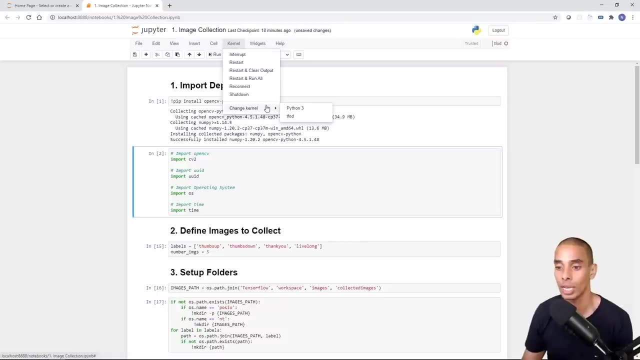 And all of the stuff that you're going to be installing is on your local machine inside of your baseline virtual environment, So that will mean that it's not as controlled as possible. Another way to check that is, if you hit kernel, change kernel. 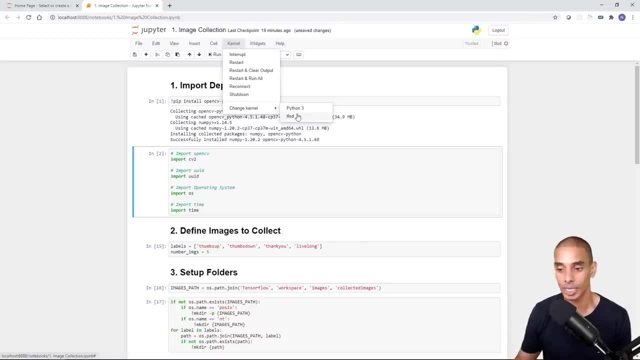 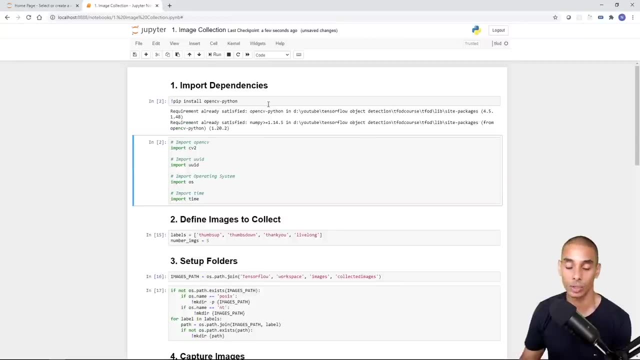 just make sure you've got the right one selected. So in this case, just to be safe, so I can hit TFOD again, And in this case I'm already inside of that. So now when I go in, install pip, install OpenCV. 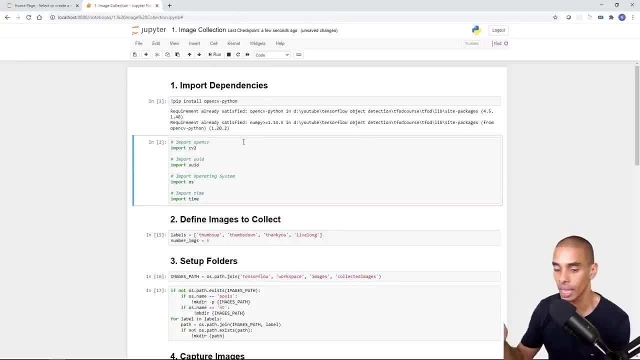 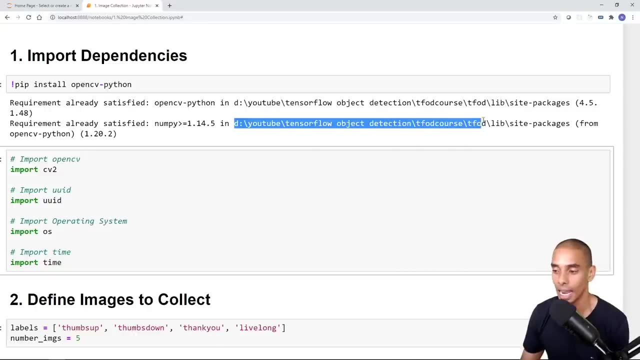 I'm 100% sure that I'm actually installing inside of my virtual environment And again, you can tell this based on the install command right. So here you can see that it's actually installing inside of this TFOD lib site, packages, library. 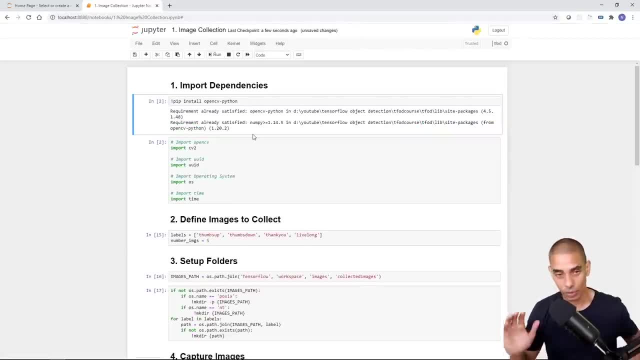 So again, installing in the right place, Really really cool. So if you're getting errors where you're installing a library and then you got to use it and you're like it's not picking up, sometimes it can be that. So say, for example, you install it on your command line. 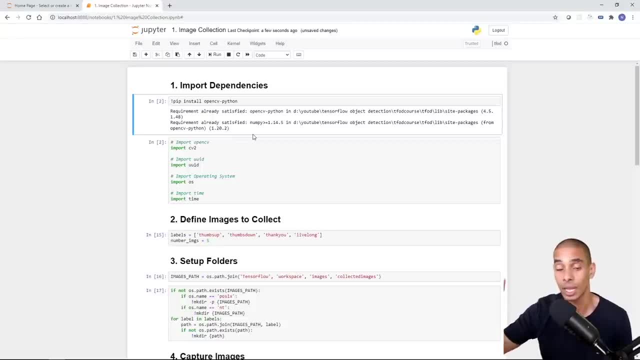 and you don't have your virtual environment activated. Well then, it's going to be installing, not inside your virtual environment. So when you do use it inside your Jupyter notebook, it won't be picking it up. Key thing to note: make sure this little bit over here is your virtual environment. 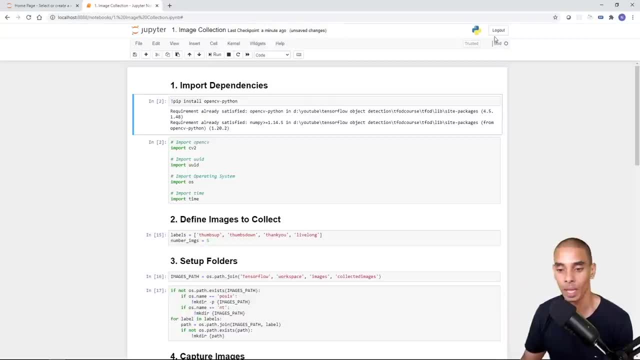 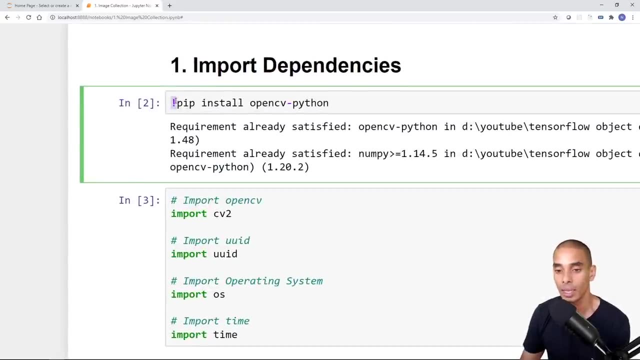 so that you are 100% sure that you're actually using it. So again, we're going to step through. So this next cell, so this first up cell is: let's zoom in on that. So exclamation mark: pip install OpenCV-Python. 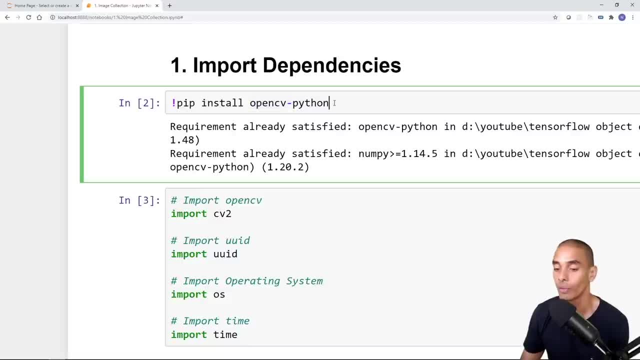 So this is installing OpenCV into your virtual environment. OpenCV just stands for Open Computer Vision, So it's a really really popular computer vision library, Really really good for working with the images or video. In this case, we're going to use it to access our webcam and collect a bunch of images. 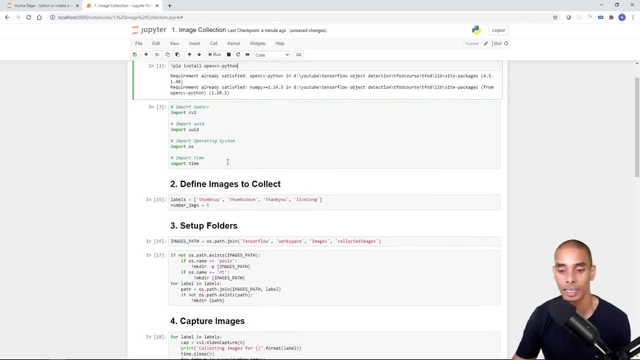 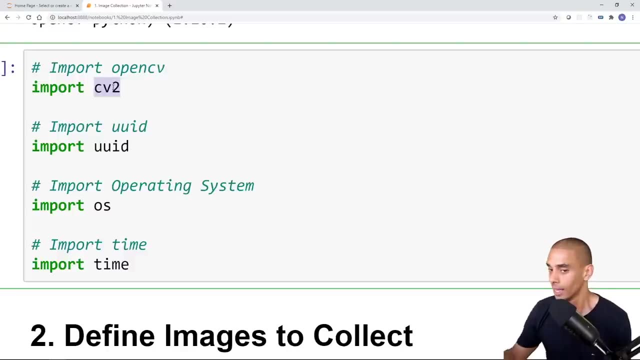 Then the next cell is actually importing some dependencies. So you can see here that we have a lot of dependencies. We are now importing OpenCV. So import CV2 actually imports OpenCV- Slightly different naming convention, This is pretty normal. We're then importing UUID. 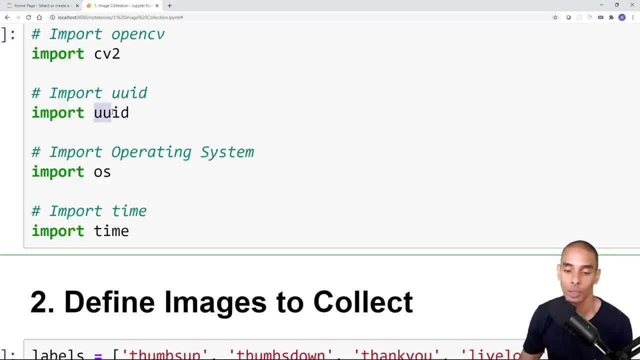 So this is now giving us our unique identifier, So this will allow us to name our images uniquely, so we don't have overlaps. We're then importing OS, which gives us our operating system. This is really good when you're working with file paths. 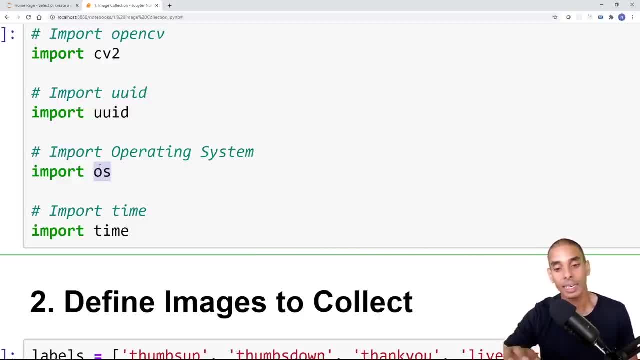 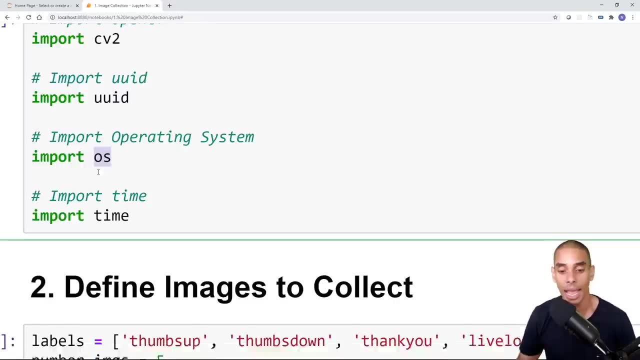 I've used OS a lot in both of these notebooks, particularly to ensure that we have file paths that are compliant with both Linux, Mac and Windows, so that you can sort of step around those. And we're also importing time. So we're going to use this when we actually collect our images. 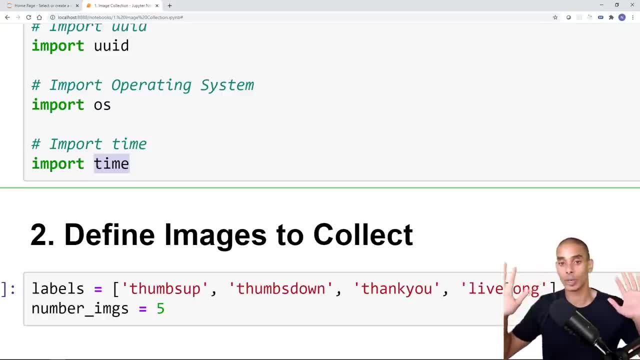 to take a two-second break between each image that we collect, So this will give us time to move to our different angles. So remember really, really important to have images at different angles to help our model generalize. Okay, Then we're going to define the different images to collect. 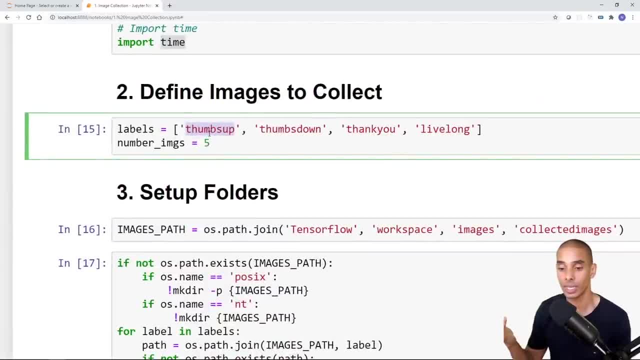 So in this case, we're going to collect four different objects. So in this case, this is going to be a multi-class object detection model, So we're going to be able to detect thumbs up, thumbs down. thank you, which is a sign language, pose and then live long. 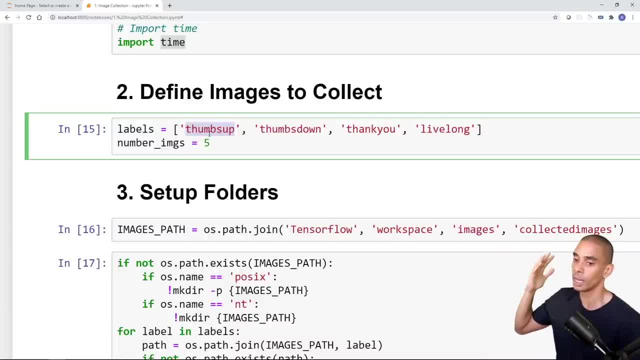 So we're going to give it a bunch of different types of images or a bunch of different types of objects to detect. So in this case, what we've actually got here is an array, so, which is labels equals square brackets, and then we've just got a bunch of different strings. 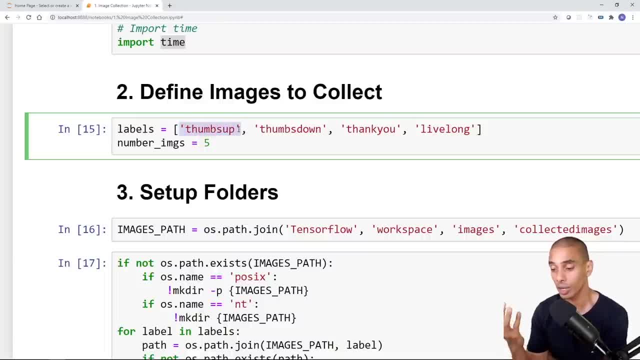 So if you wanted to have different objects to detect or different types of objects, this is where you change those labels. So in this case, here we've got thumbs up, thumbs down, thank you and live long. Now again, you could change this to your heart's content. 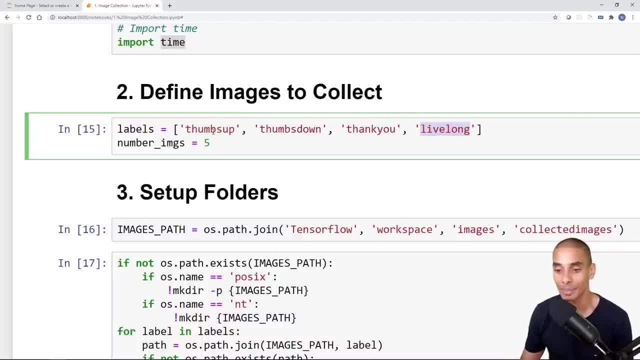 Just make sure that whatever the label is named here is actually it's not so important here, It's important later on When you actually go to label. make sure that you pay attention to the case. In our projects we're actually going to change this up. 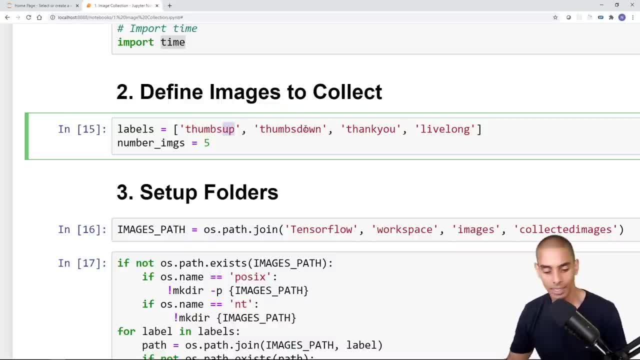 So, rather than doing thumbs up, thumbs down, live long, say, for example, with our little LEDs, we'd be doing bent and not bent, for example, In this case, we're pretty happy so we can run that cell. 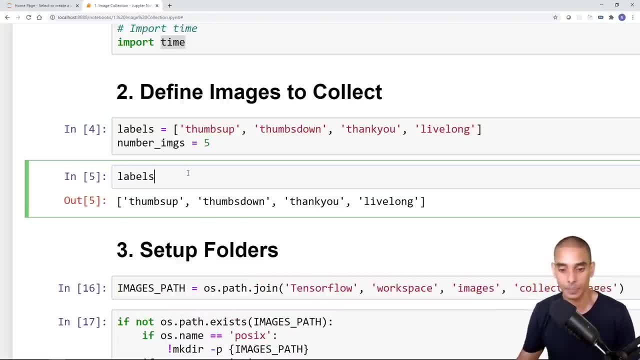 And if we actually take a look at our labels, this is just a list. So if we actually type in type, you can see it's just a standard list. There's nothing super fancy going on there. It's just a place that we can hold our different labels. in this case, 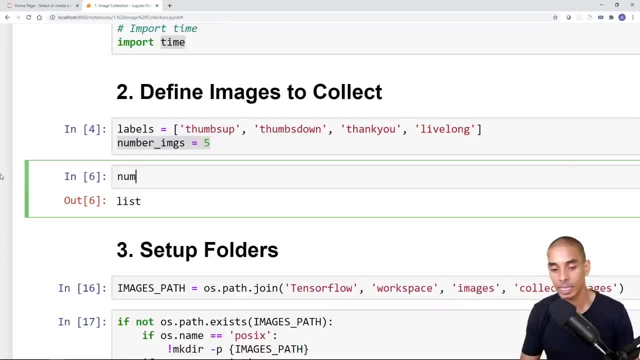 And we've also got this line here- number of images. So this just represents how many images we are going to collect per class. So we're going to collect five images of thumbs up, five images of thumbs down, five images of. thank you. 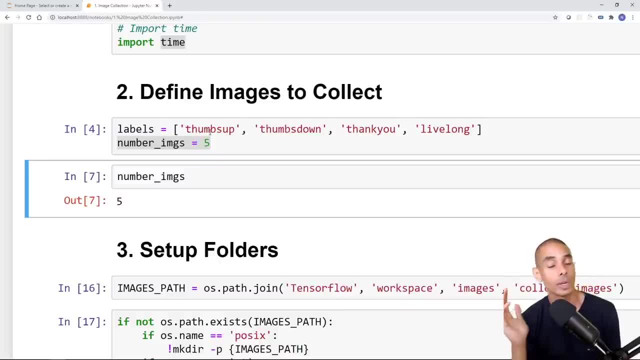 and five images of live long. Now remember what I said During the best practices: ideally, you want to have 10 to 20 of these images just when you're getting started right, So I'll talk about this in performance training as well. 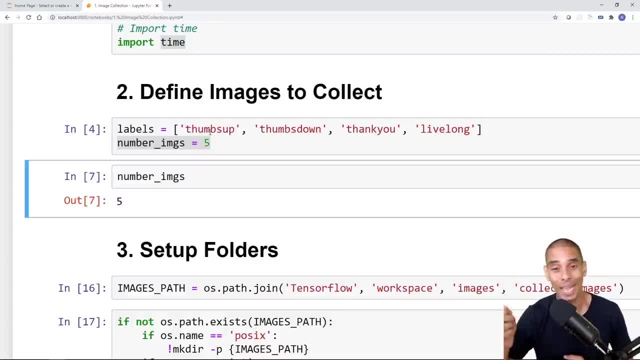 When you want to scale this up and produce a model which is way, way better, you want to use way more images than that, But to prototype and to get up and running, 10 to 20 images is ideal. I'm doing five on purpose here. 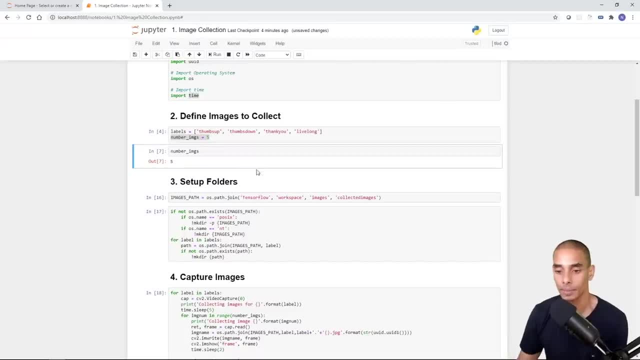 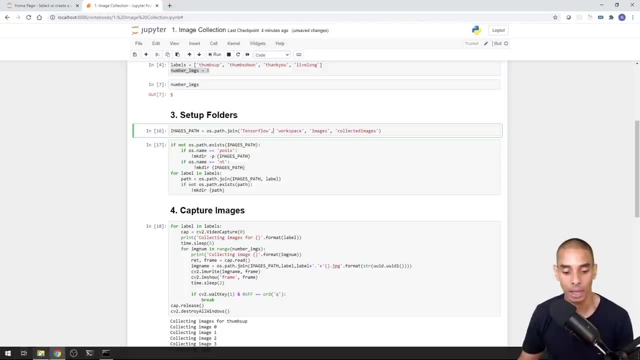 because we're going to performance tune later on. Okay, Then the next thing that we're going to be doing is setting up our folders. So right now, we don't actually have anything created inside of our folder directory, right? So let's just add our navigation pane again. 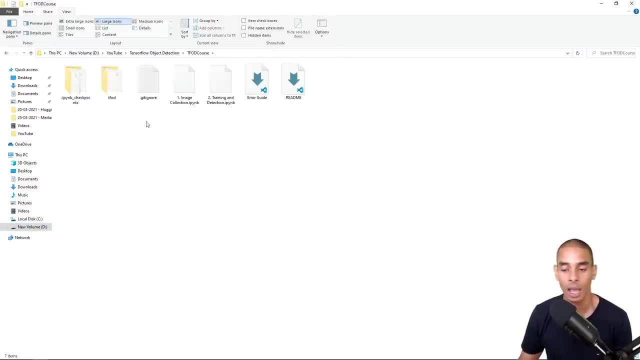 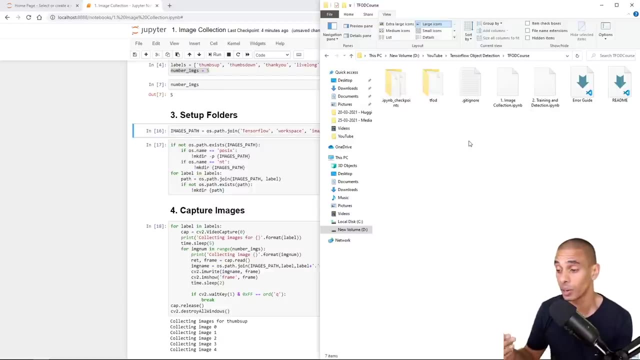 So if I go into our TensorFlow object detection repository, I don't have any folders here, But I'm actually going to set up a little folder directory that's actually going to be serviced really, really well when it comes to training and doing all of our other stuff. 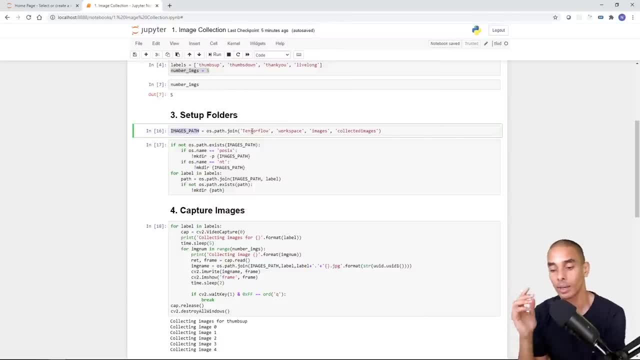 So this particular line here is just setting up our images path. So what we're doing is we're now going to create a new path which is going to be called TensorFlow, And then inside of that we'll create a folder called workspace. 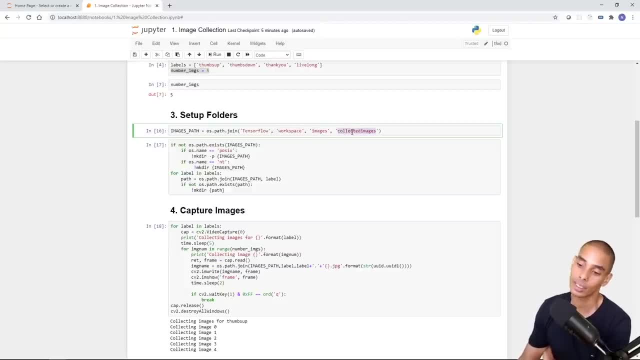 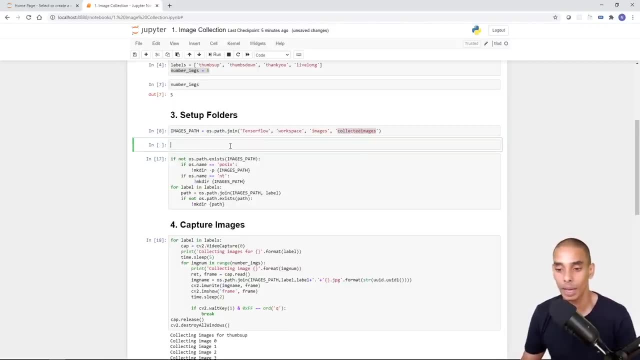 folder inside of that called images and a folder inside of that called collected images Probably doesn't make sense right now. Let me show you. So. if I hit shift enter, it's going to set up our images path right. So for Windows you're going to get a double backslash. 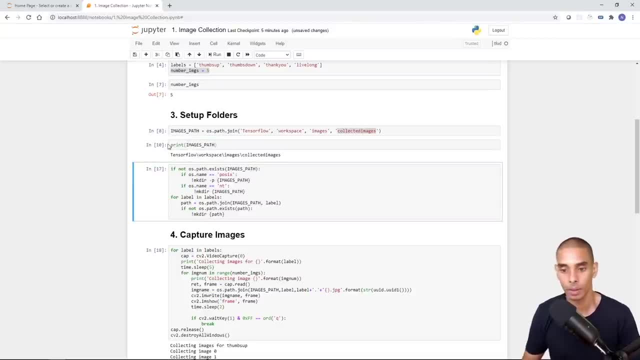 if you print this out right, You can see that what it's actually doing is just navigating to TensorFlow workspace images- collected images. If you wanted a different file path, you could change this, But just bear in mind that the rest of the tutorial 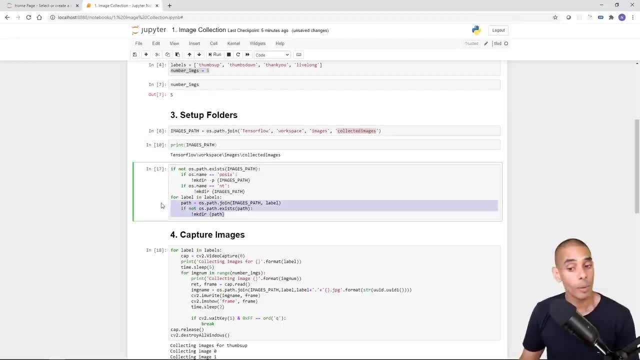 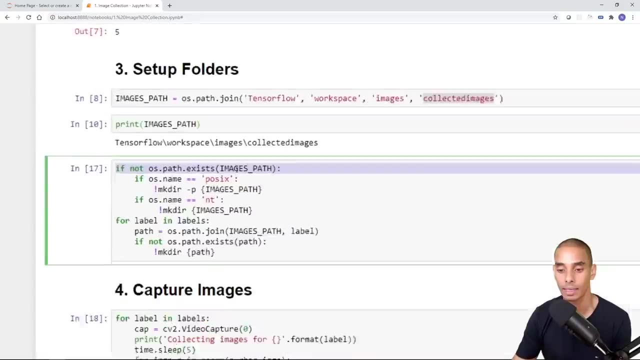 is going to follow that file path, And then what we're going to do is create those file paths. So, first up, what this line is doing is checking whether or not the path exists. Then it's checking what type of operating system is being used. 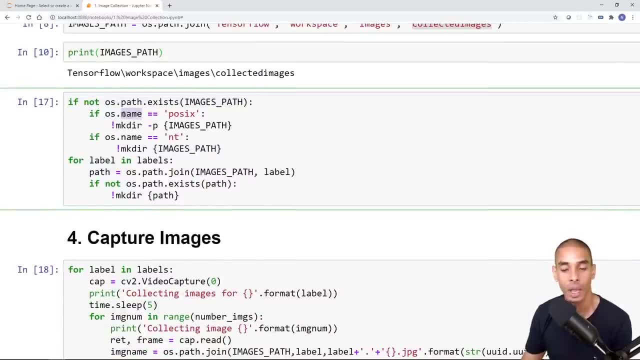 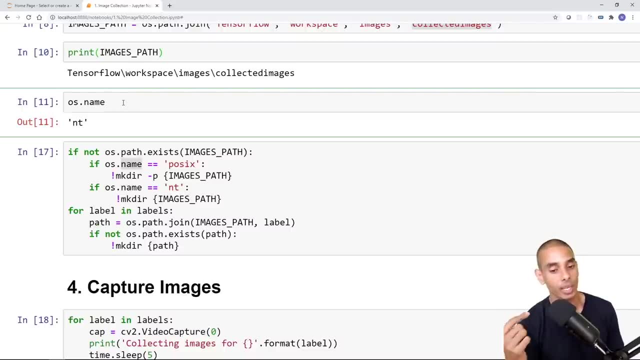 So in this case osname actually checks what type of operating system is being used. So if I actually type that out, so osname, because I'm on a Windows machine, it's going to read out NT. You'll see later on when I do this on a Colab instance. 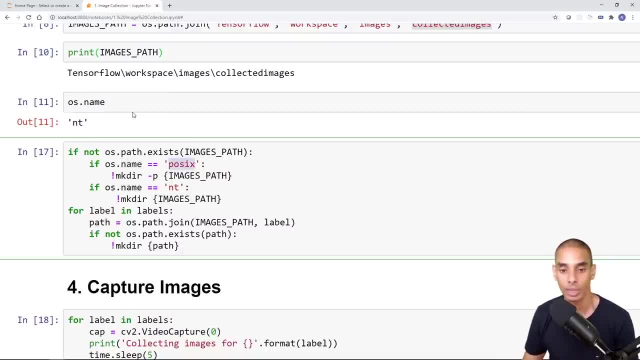 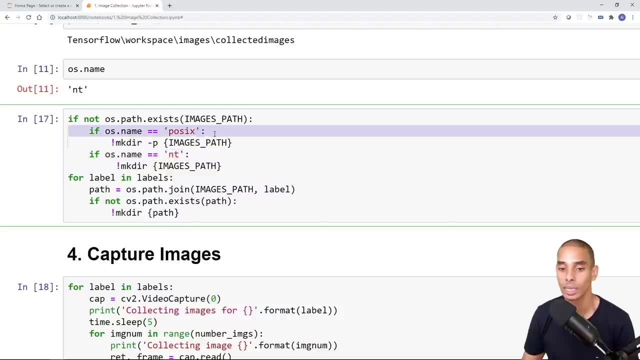 because that's a Linux machine. it's actually going to say POSIX. So this gives you the ability to work out to run on both of those operating systems. So in this case, NT is going to be Windows, POSIX is going to be Linux. 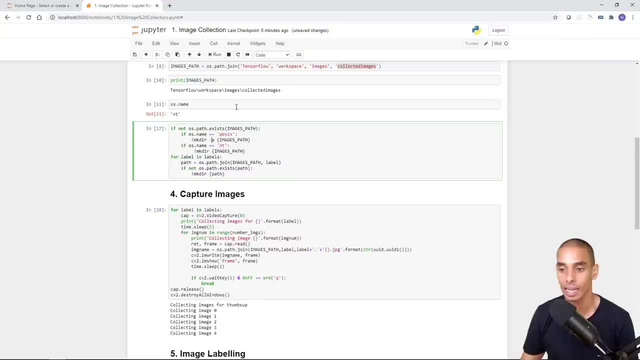 Now that's all good. What we're going to do is run this cell, and this is actually going to create this folder directory, Or this folder path. So if I hit Shift Enter, you can see that that's run successfully. Now, if we go back, 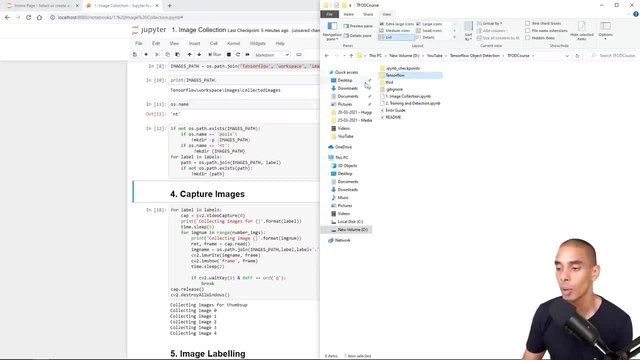 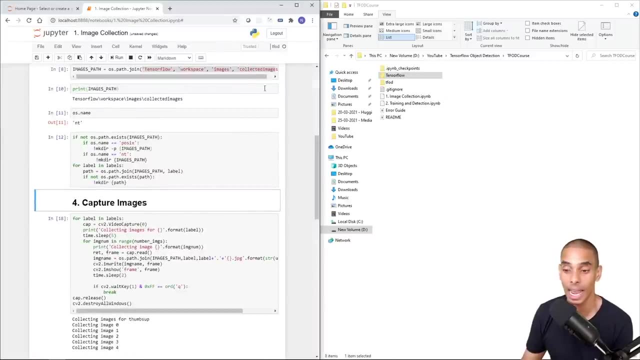 you can see. let's just make this a list so it's easier to see. We've now gone and created a new folder called TensorFlow, So that's now available there, And if I step in, what you'll actually see is that it's actually creating the whole file path. 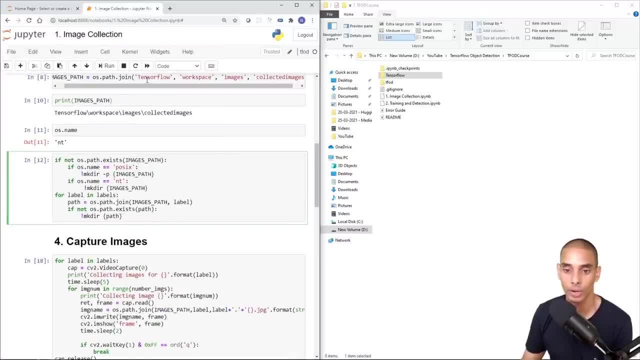 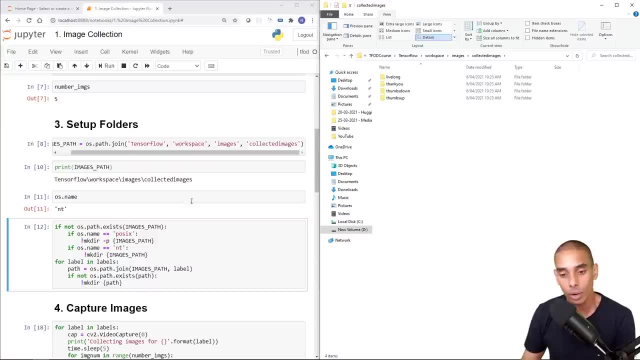 So TensorFlow workspace. I should zoom in on this. by default, it's going to create TensorFlow workspace images, collected images. So TensorFlow workspace images, collected images. Now, what it also does at the same time is it creates a new folder for class. 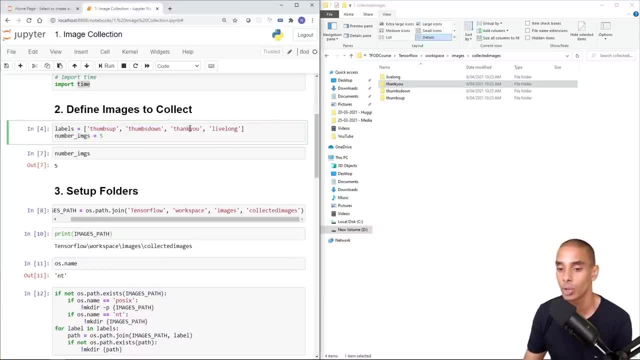 So it'll create a new one for thumbs up, new one for thumbs down, new one for thank you and a new one for live long. If you change this, add different objects, add different labels, then it's going to create those folders as well. 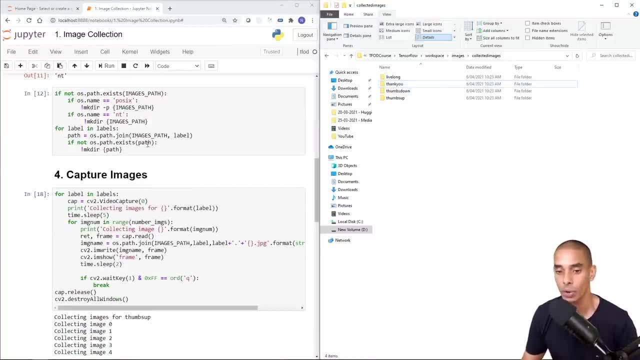 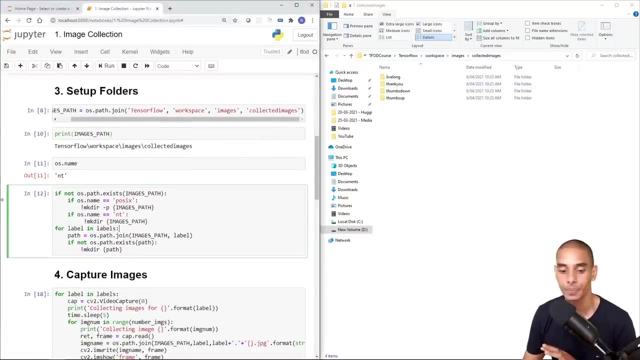 when you run this particular cell here. So if you don't have these folders created, make sure that you've got your labels defined correctly and make sure that you run this cell. it'll create those folders for you. Now, the next thing that we're actually going to do: 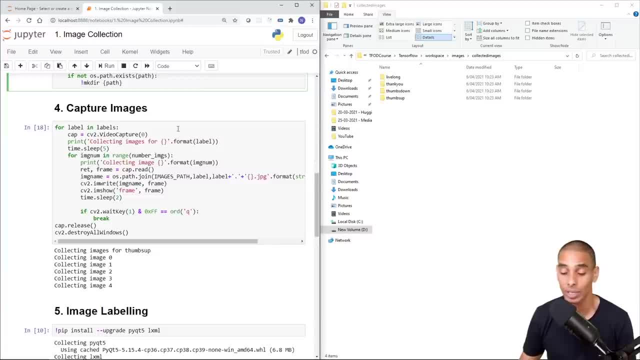 is actually capture our images. So this cell over here is actually going to do all of this for us. So it's going to loop through all of our labels. It's then going to connect to our webcam. Now, this line is really, really important here. 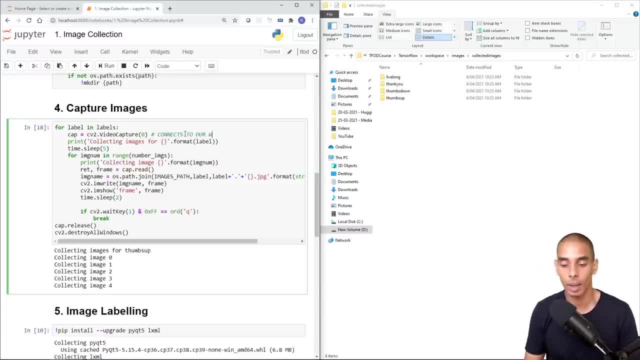 So this line connects to our webcam or capture device. So right now we're just doing it using our webcam, right? But later on, when we go to do object detection using our microscope, I'm actually going to need to change this device number to be able to detect. 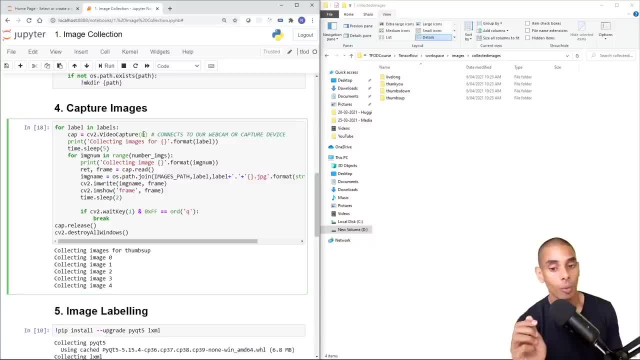 that particular microscope. Now, what might happen is this number that you see here, so right now I've got zero in there. If you're working on a different machine- which undoubtedly you will be, this number or this video capture device is going might vary, right? 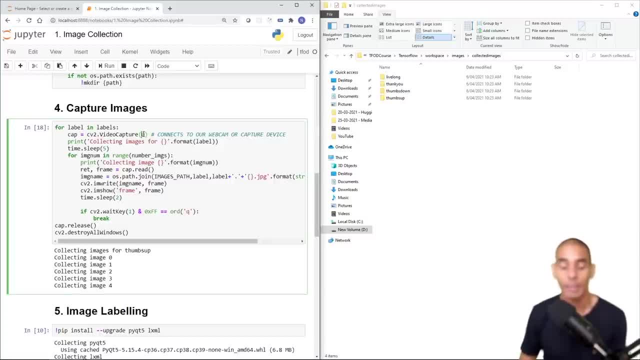 So on my Mac, so on my other Mac machine. the number that I need to pass through into here in order to be able to connect to my webcam is number two. Now, if you get errors, which undoubtedly it might happen. So if I actually go back into our error guide, 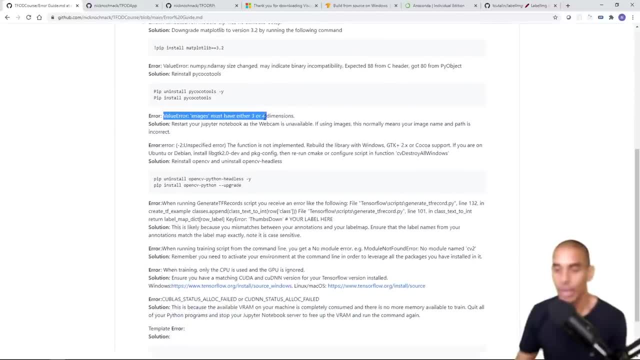 So if you get an error that looks like this, so value error images must have three or four dimensions. More often than not that is because your webcam. you haven't got that webcam number correct. So if you see a gray box pop up, 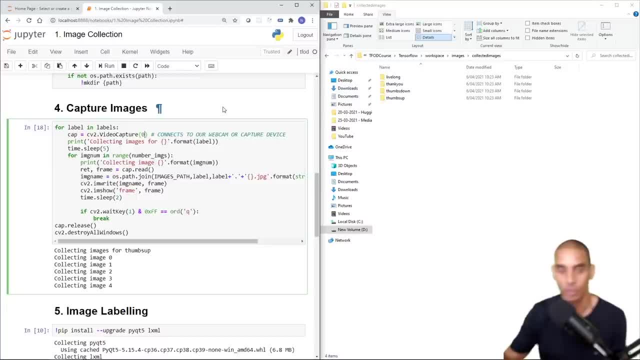 and you're not getting any images back again. it could be that as well. So sometimes you might need to either change that number or restart your notebook to be able to connect to your specific webcam. Now, in this case, I believe video capture device one is correct. 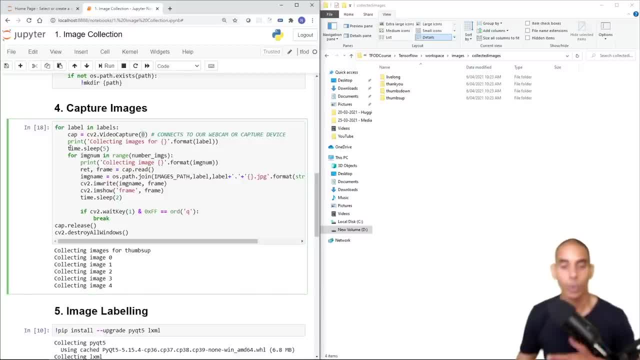 So we should be good to go. So what's going to happen here is we're going to first up print out which label that we're collecting images for. So it's going to print out collecting images for, and then the label that it's looping through. 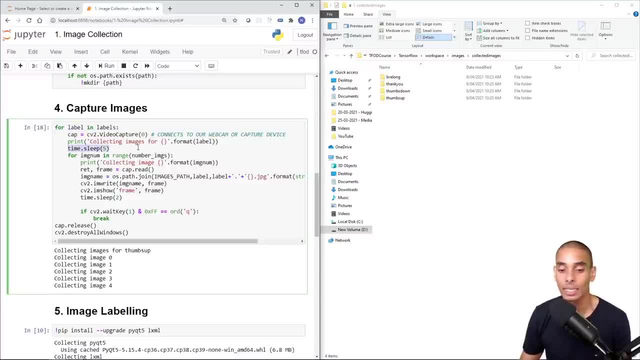 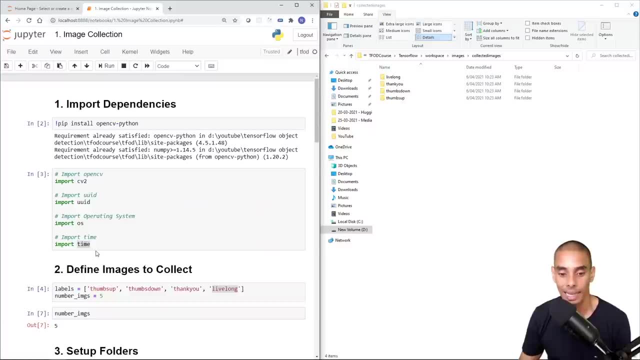 because, remember, it's going to loop through our labels up here. It's then going to give us a break for five seconds to enable us to get into position. So it's going to sleep for five seconds And this is where that sleep library, down here. 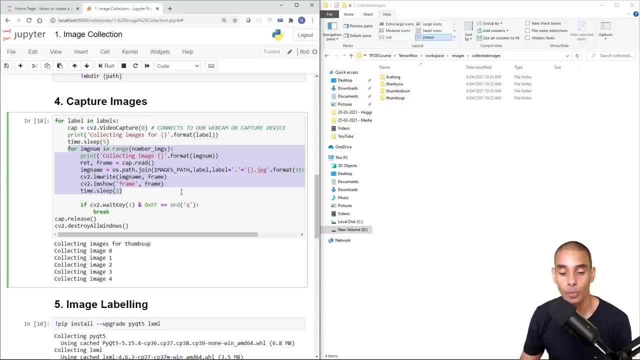 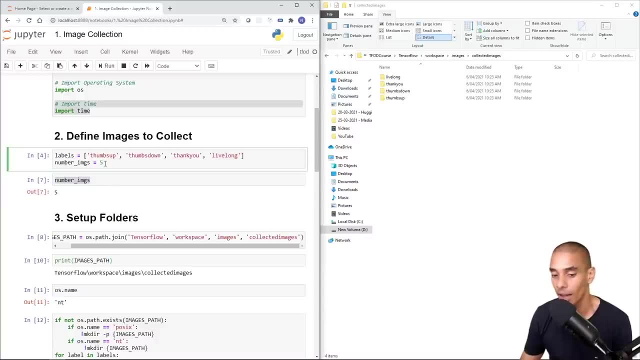 is coming in handy And then it's going to loop through the number of images that we want to collect. So remember, we're going to collect five images in this case, If we change this number up here from five to 10 or 15 or whatever. 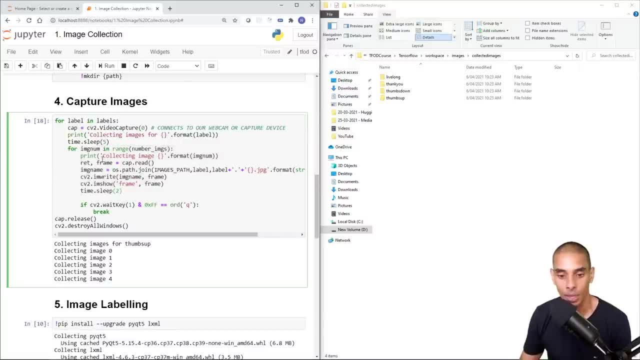 it's going to change the number of images that we actually collect, So it'll then print out collecting image for a specific label. It'll then capture the frame using our webcam And then what it's going to do. this is really important. 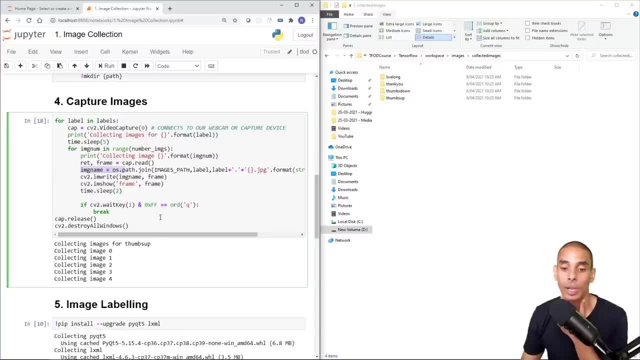 So it's going to create a new image and it's going to place that inside of the frame, Inside of this particular folder path, So it's going to place it inside of images path, which is: let's actually print this out, so you'll see it. 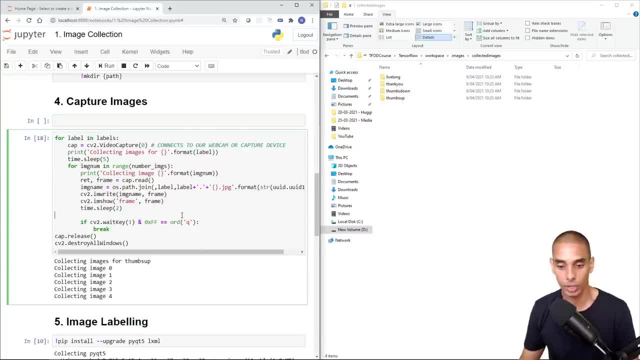 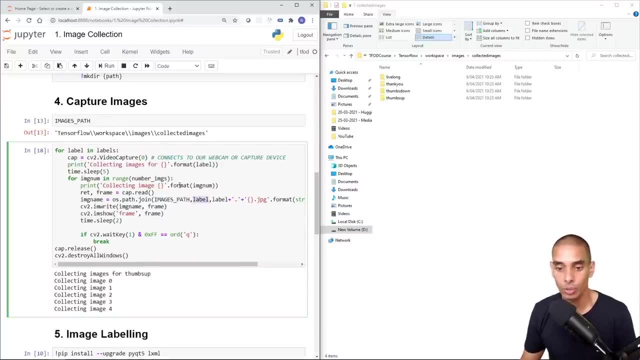 It's not going to work if I don't have an image, So it's going to put it inside. I'll change that now. It's going to paste it inside of images path And then label. So in this case say, for example: 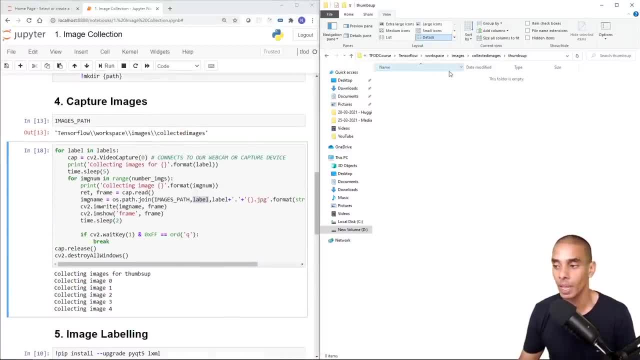 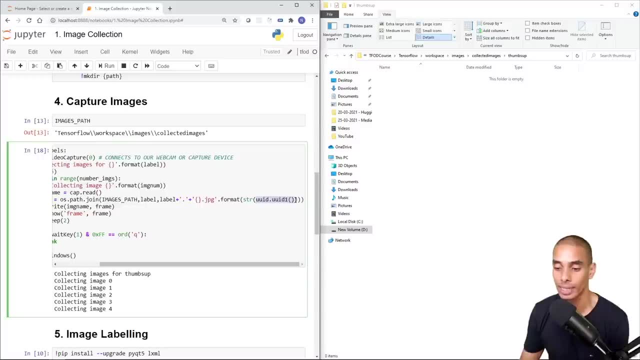 we are up to thumbs up. It'd put it inside of thumbs up, which is over here, And then it'll name the actual file label, dot, and then a random number. So it's going to create this unique identifier dot, jpg. So all of our files will be jpeg. 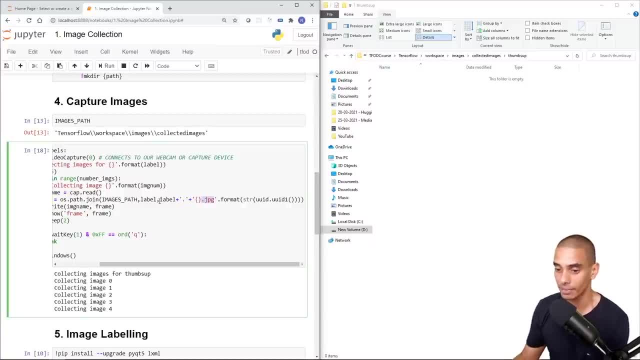 They'll be named the specific label plus the unique identifier, and they'll all be inside of their respective label folders. So we're going to need to move these around a little bit later, but that's fine for now. Then it's going to use the cv2.imwrite command. 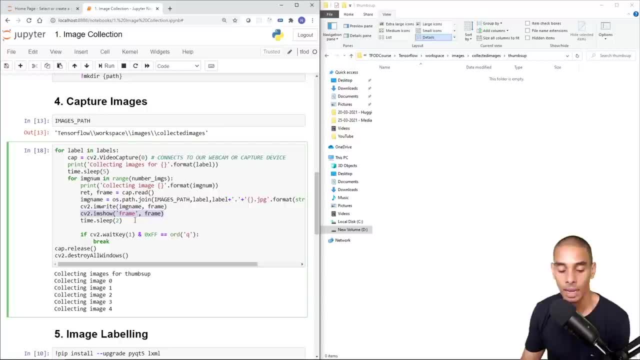 to be able to write that down into file and it'll actually show it to a screen. It'll then take a two second break again, And if at any point we need to escape out of it, we can hit the Q key on our keyboard. 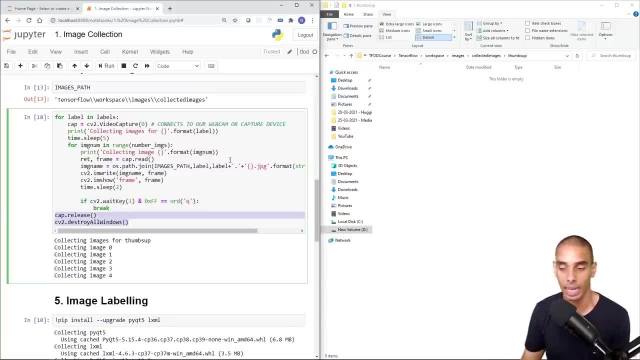 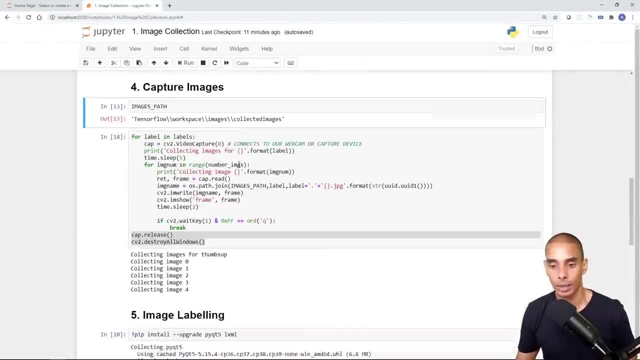 to be able to get out of that. It'll then close everything down. If I zoom out of that now, let's go on ahead and run this. Are we zoomed in? No, we're not zoomed in. All right, cool. 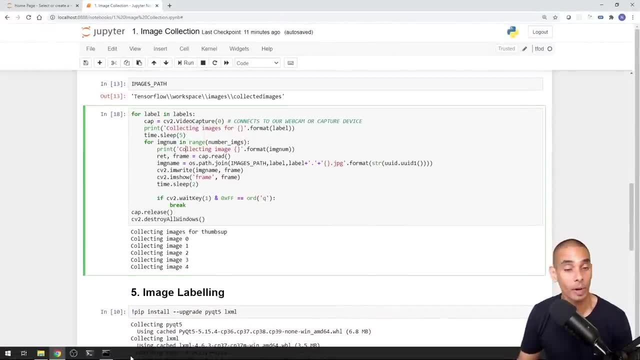 So if we run this ideally, what you should see is a little pop up at the bottom of your screen which indicates that it's now connected to OpenCV and it's actually rendering. So you've got remember. you've got five seconds to get into position. 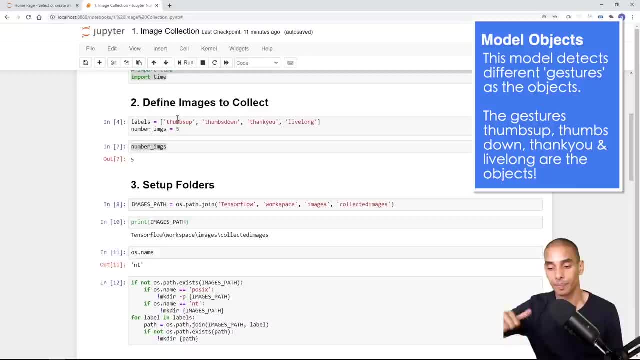 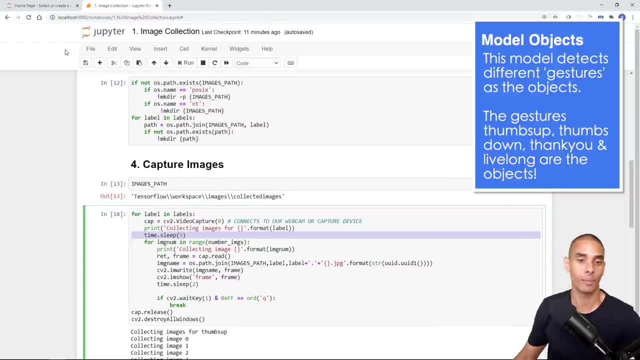 So in this case, the part that we're going to go down is thumbs up, thumbs down, thank you, and then live long. So again, I'm going to make sure so we might do this once. see where our webcams position. 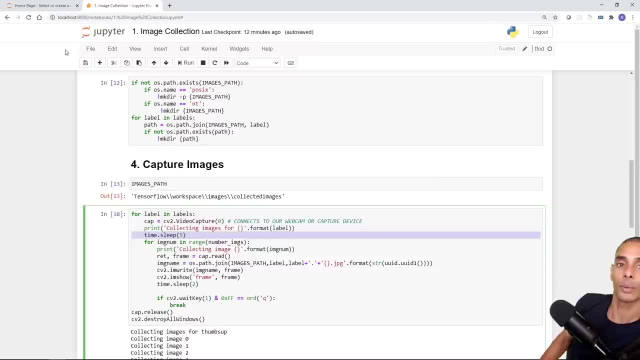 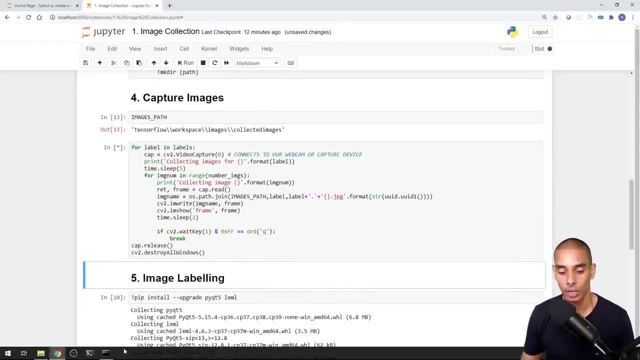 and we might need to fix that up. So I'm just looking at where mine is now. It should be okay. Let's give it a crack, All right. So I'm just going to run that cell Again: shift, enter. Should see a little pop up down the bottom. 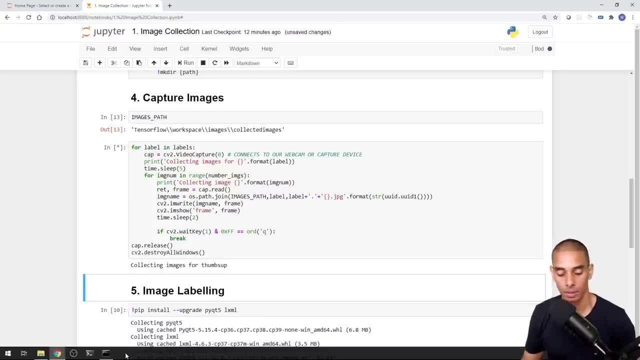 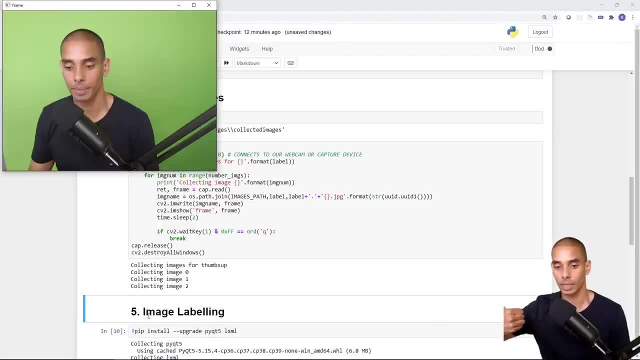 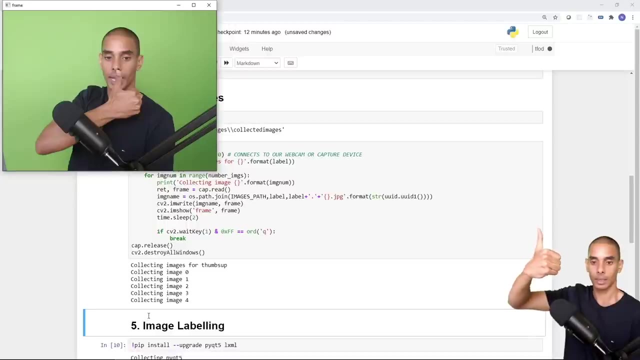 It looks like it's okay for now. Let's see if that's popped up now And again. first position is going to be thumbs up. It's very dark. Let's get back into the center. Not the best images of thumbs up. 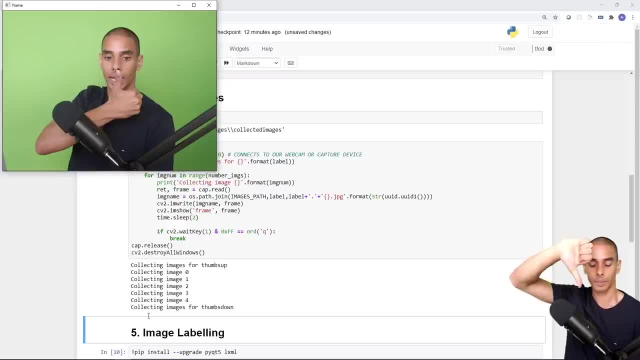 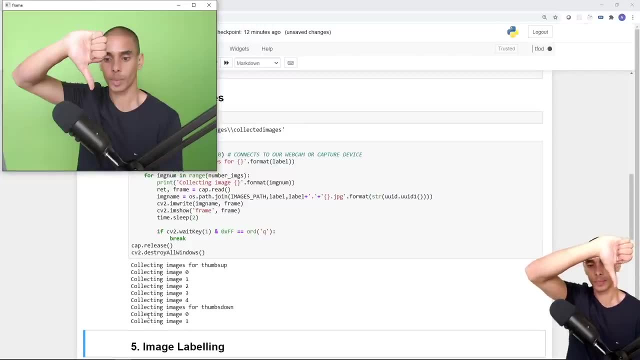 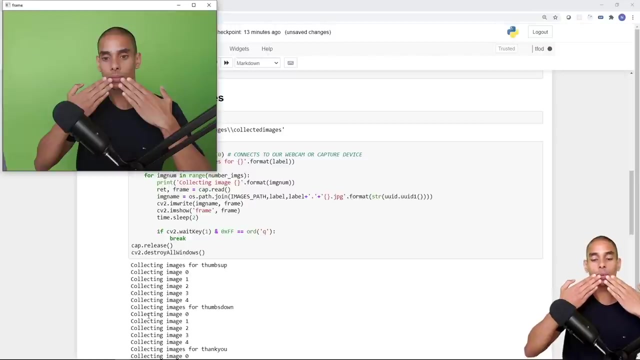 We'll try it anyway and see what it looks like. Thumbs down, And the next one should be thank you, I believe. Let me switch to this position. So again, you get a little bit of a break between each of these images. 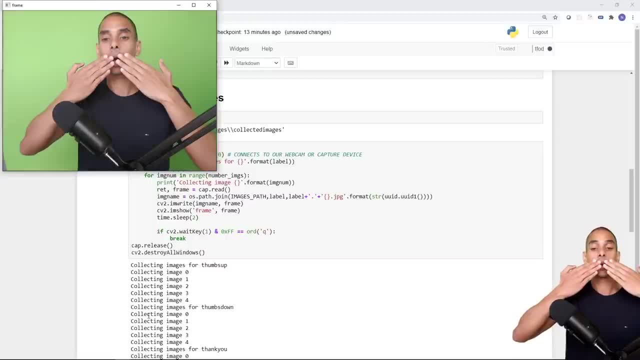 So you've got time to move around, right, If you want to increase the break, you can just change that number. And again, I'm trying to get into slightly different positions each time, And then the last one: it should be: live long. 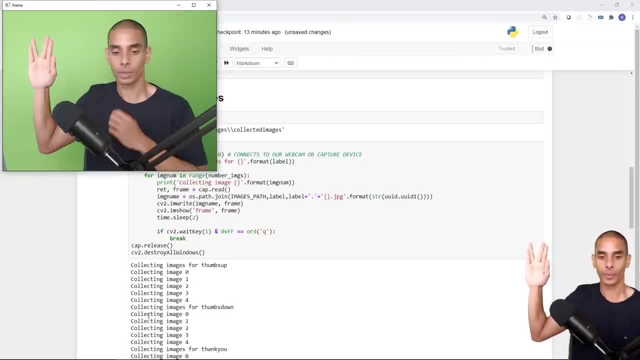 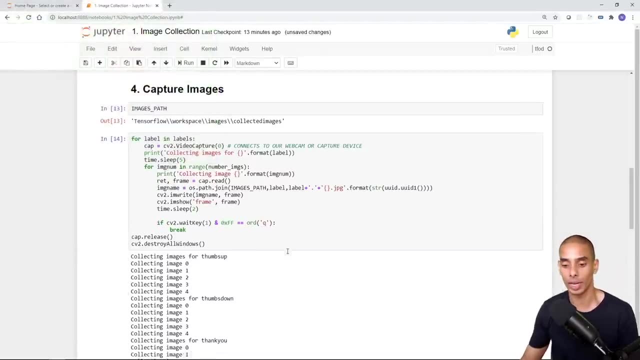 All right, Looks good, So let's keep this running. All right, We're still there, So we'll take a quick look at the screen. Remember, right now we've only got our green screen in the images as well, So we might choose to drop the green screen. 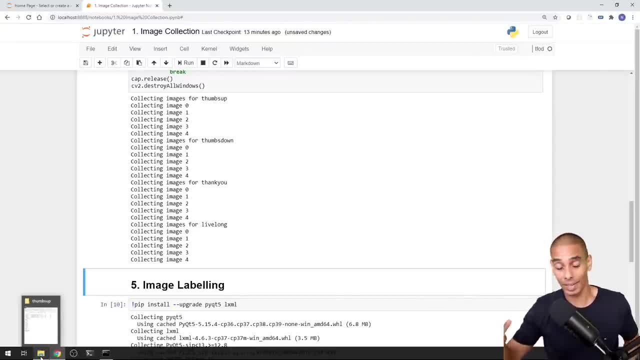 and create new detections later on If we get really, really poor performance. we'll test this out Again. this meant to be a live example, So you can see what some of the challenges that you might face and how to solve those. 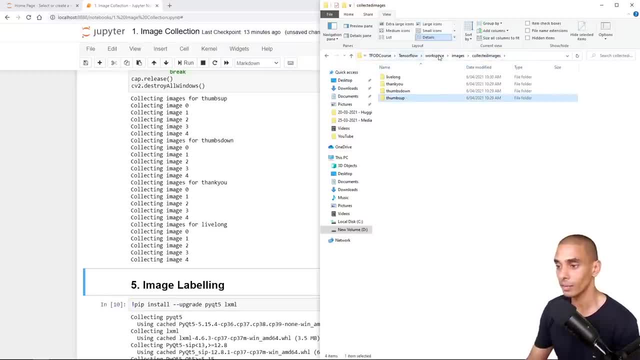 All right, Cool. So it looks like we've now got a bunch of images. So, again, if we go into tense flow, workspace images, collected images, images, so our live long positions looking fine and the way that i'm sort of judging these, the 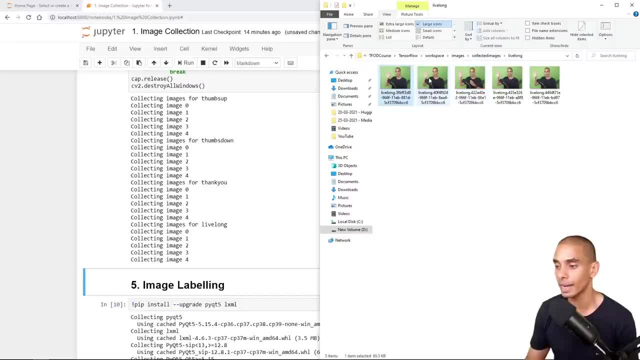 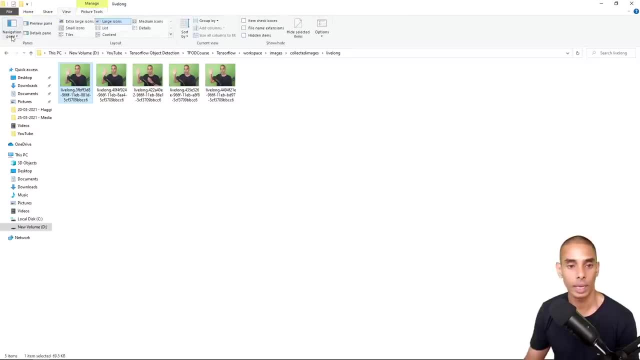 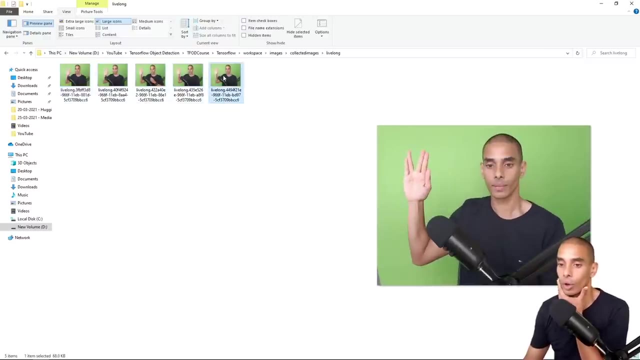 only thing i'm a little bit concerned about with these images is that right now they're all in the same format, so let's just enable preview. how do we do this again? preview pane. yeah, so right now they're all sort of in the same position, right? so this is not good practice. 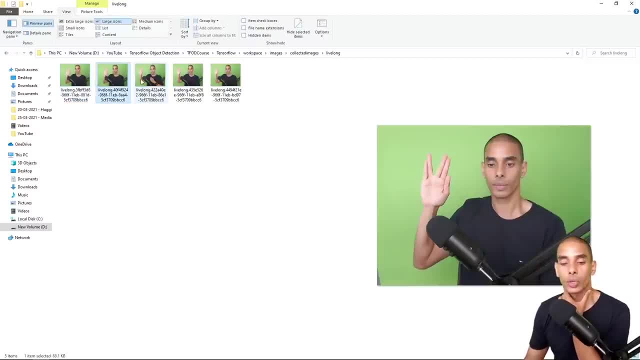 when it comes to building a generalized model. so what we might choose to do later on is move into different positions and, ideally, drop the green screen, add more images, train this up again. so in this case, that's our baseline right. so and again, when you're prototyping, a key thing: 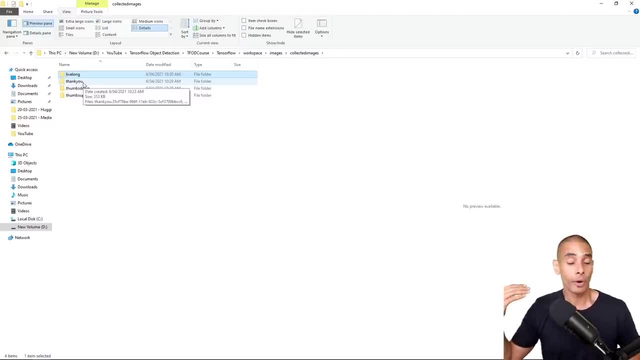 in any data science project i preaches all the time: prototype as fast as possible, because then you're going to work out whether or not what you're trying to do is feasible and whether or not it's possible. so say, for example, you're trying to detect i don't know. say, for example: 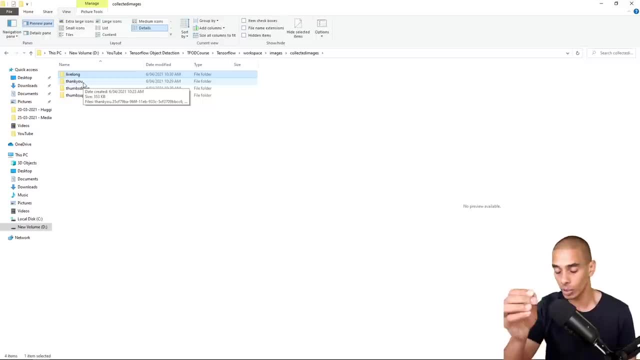 you were trying to detect bent uh leds and you're just doing it with a web cam. well, you're going to need a really really hyper accurate model, or one that's able to see really really fine grain detail, to be able to do this. so if you were to prototype, really really 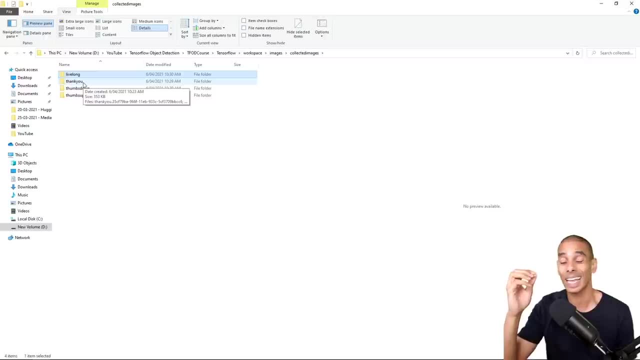 quickly with a mobile net model model and just a webcam, you might see that you get absolutely sucky performance. now, if you do this fast, at least you get to the end output to realize that, hey, maybe we need to try a different technique. maybe we need a different sensor aka microscope. 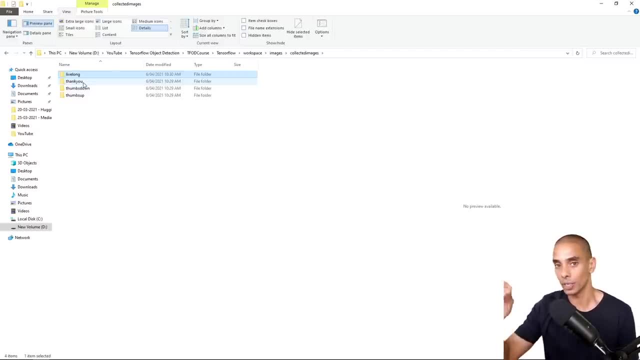 by doing this quickly and prototyping quickly, you're able to see and establish a baseline for which you can go on then and try to improve performance. in this case, we're going to give it a crack and see what it looks like. so we've got our live long images. let's check. thank you these. 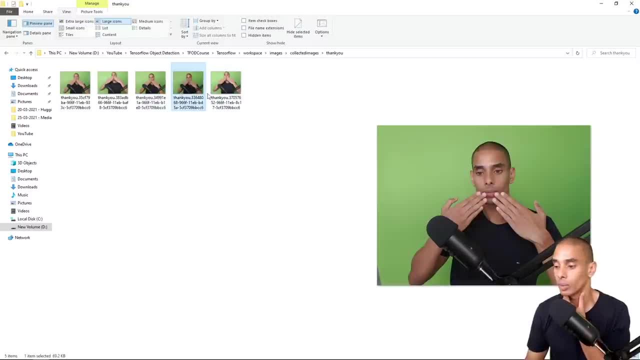 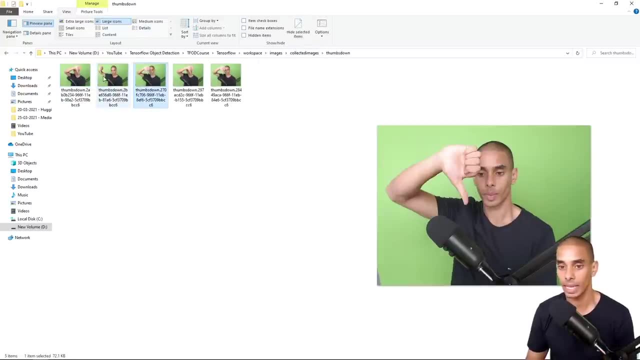 ones look a little bit better again, obstructed by the microphone. a little bit, we'll see how that performs. it's looking good. thumbs down, that looks all right again, so you can see that right. so i'm giving my model a better chance to generalize by having a thumb position there and a thumb position. 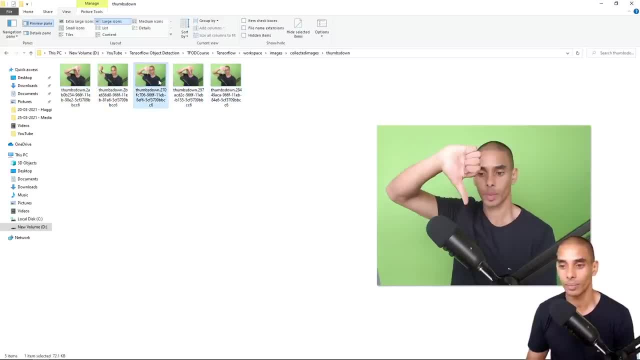 there that's looking better. and again few different ones, again reasonably close together. now another idea here, right, is to do it with different hands. so in this case i've just done it with this hand, but i could have chosen to do it with this hand, right, you're going to give me a better chance to generalize that way. 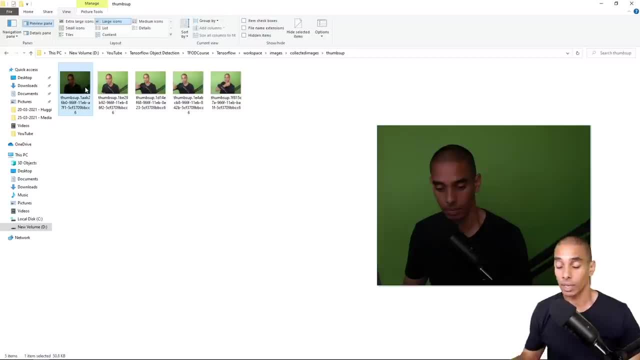 and thumbs up. that image is crap, so we're actually going to get rid. so this is another thing to know, right, so that sometimes you might need to delete images. so in this case, this one's really dark and it doesn't even contain an image of a thumbs up. so if you don't have the object included within, 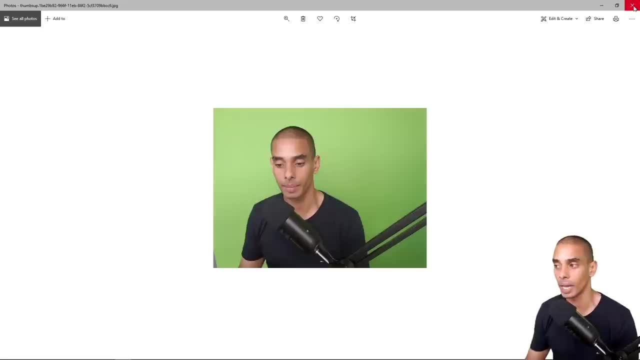 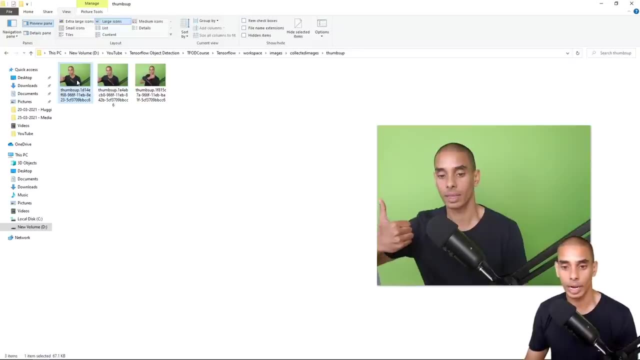 the image. it's not going to be used for training as part of the tense flow object detection, api, so we can actually just delete this image and delete this one, because it kind of sucks and i've got a feeling that after we train this model, our thumbs up detection. 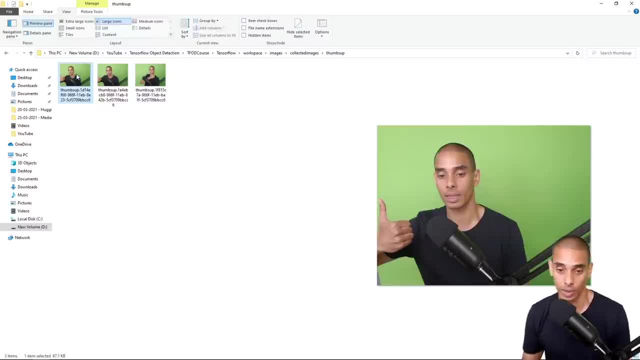 is not going to be good, but let's give it a crack and see what it looks like. we can always performance tune later on. so keep in mind, our thumb is really, really close to the edge. this one, it's half cut off. this one it's in front of our face. so again, we don't have a good run of. 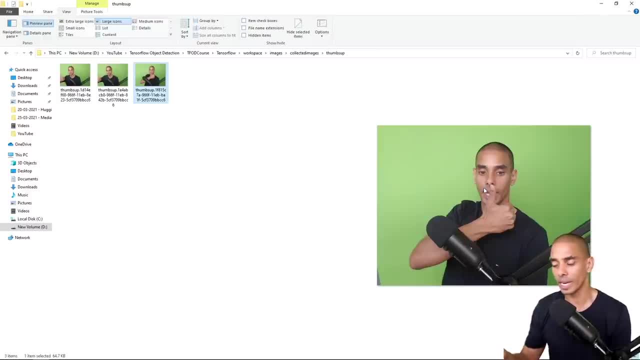 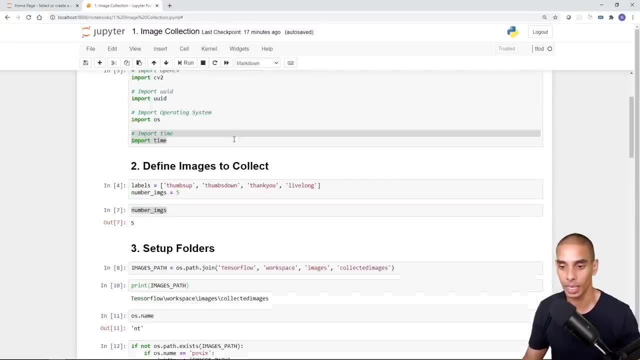 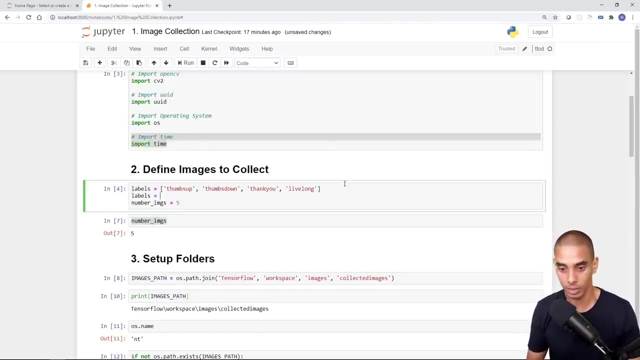 example, images there. so if we wanted to, we could actually just add more images in now, right? so rather than collecting images all the way again for all of these labels, what i'll do is i'll just delete um or we'll add in a new array, because i've got a feeling that those thumb images really aren't that good, and 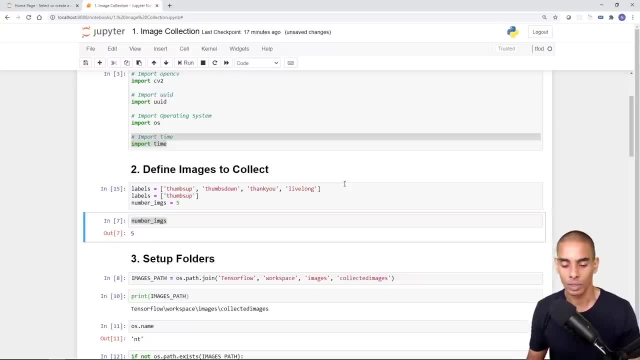 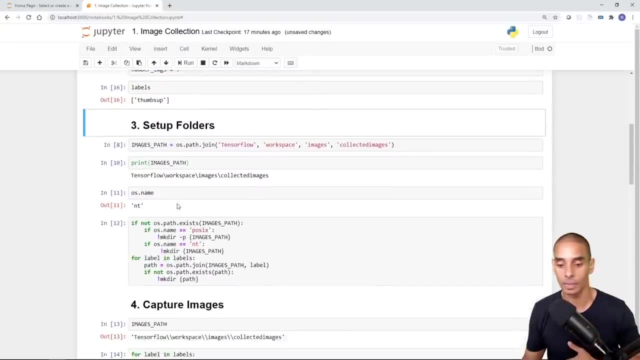 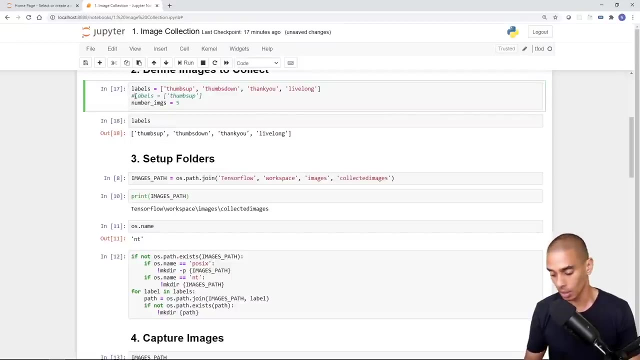 we'll just call it thumbs. what was it up? i think it was thumbs up. so now, if we take a look at our labels, so now we should be able to collect more images for thumbs up. so let's go on ahead. so i've got a new one, so i'm going to go back to the old one and add in a new variable. so if we wanted to, 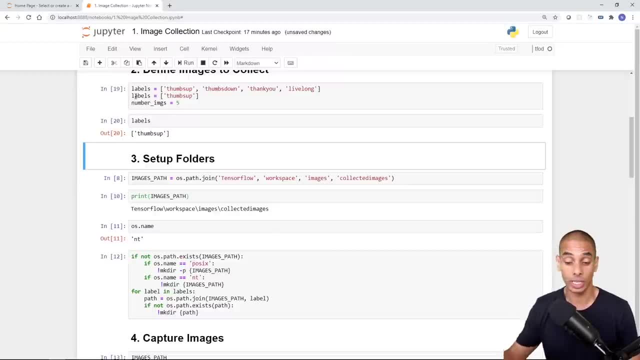 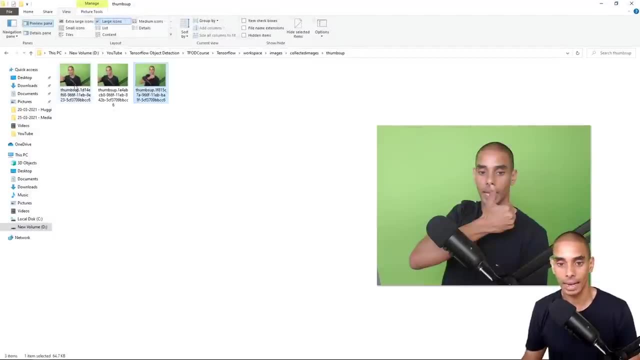 go back to our normal labels. we could do that as well. now again, this is pretty common, so you might need to add or capture additional images or capture less images. in this case, i'm just going to capture a couple more images of thumbs up, because we've only got three and all three of 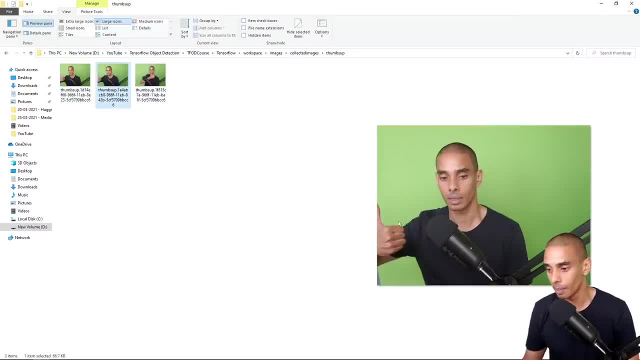 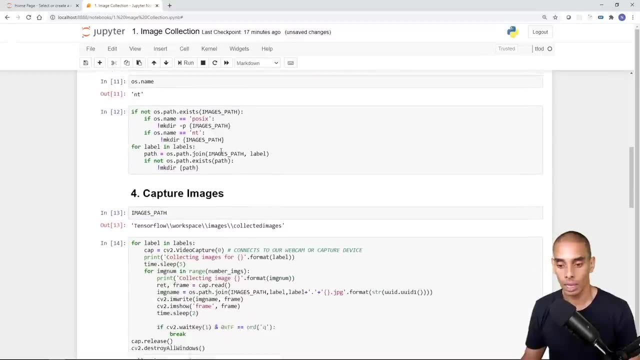 them kind of suck so and right, so like they're only like half detection, so this one barely even counts. you can only just see your thumb there. so ideally we want to get a number of good images, so let's do this now. so what i'm going to do is i'm going to run this cell again and see how we go. 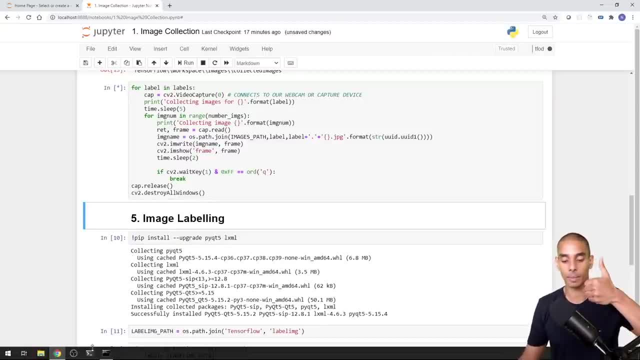 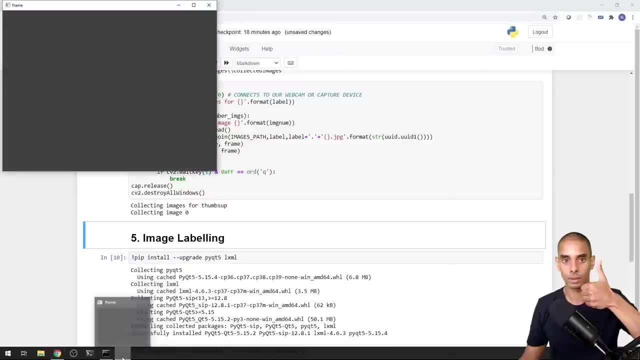 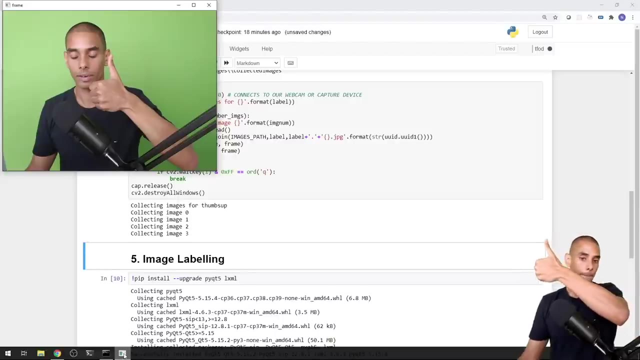 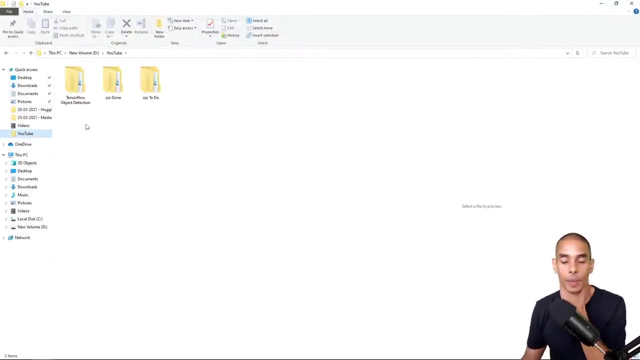 so if i run that ideally- so we're going to be trying to collect thumbs up- you should see a little pop-up again. all right, we've got our frame. it's looking better. all right, that looks a little bit better now. so again, we go back into our 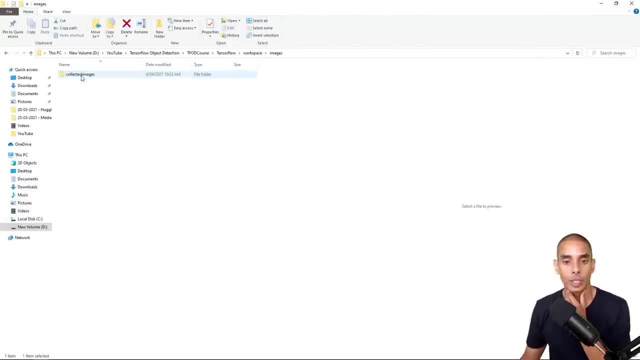 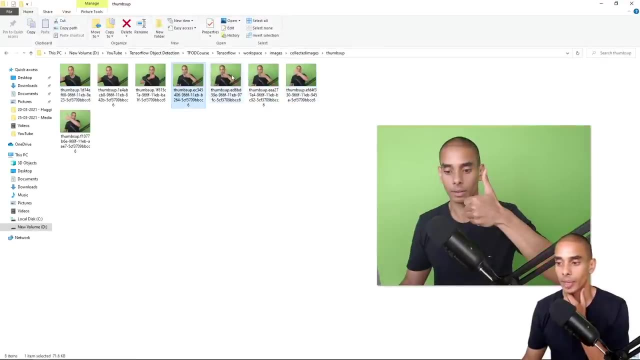 folder, tens of flow, workspace images, collected images and thumbs up. so now we've got way more right. so if we take a look at our latest ones again, we've got a bunch of different piece. eyes are closed there, great um. so again got a bunch of different images we're giving it. 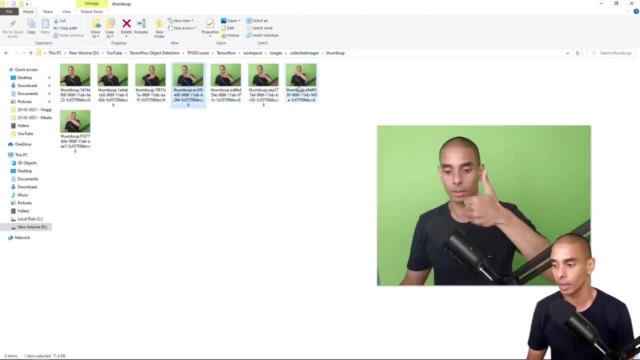 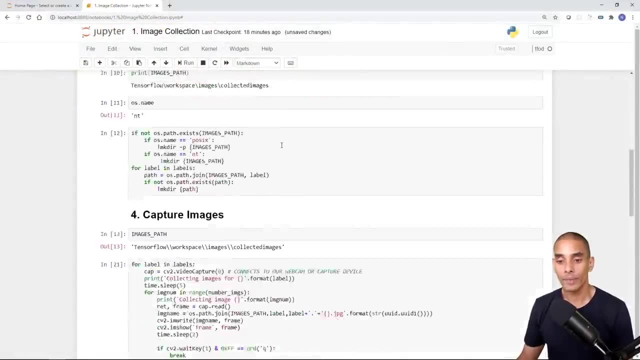 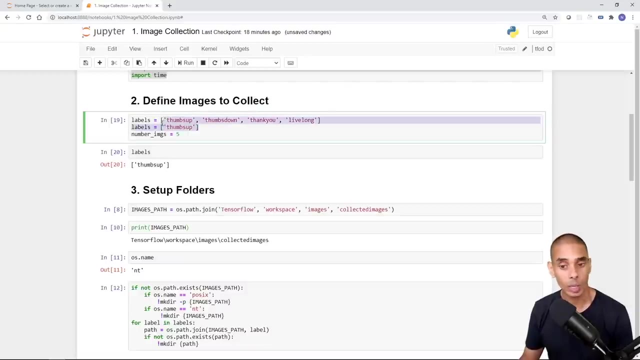 a better chance to journalize, and now we've got images for both hands as well, right, all right, so let's do that and see how we go. all right, so we've now gone through installing and importing our dependencies for image collection, defining the labels that we want to collect as well as how to collect additional. 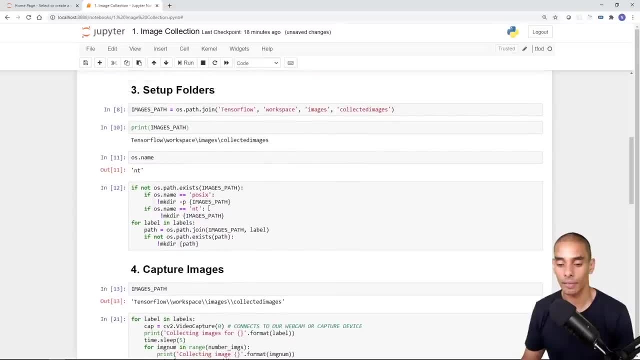 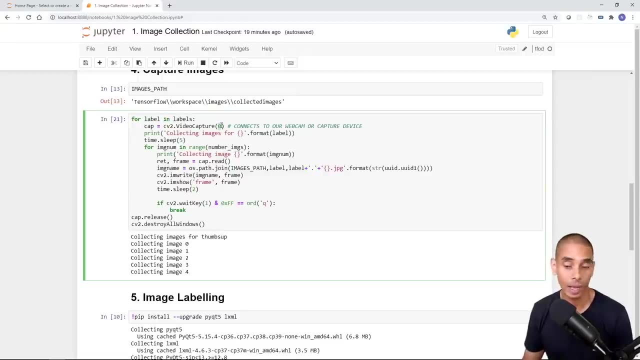 images for a particular class, and we've also gone and set up our folders and captured our images. now again, keep in mind when you are doing this bit, you might need to change this number depending on your webcam capture device number. so it's fine to change it. if you have to change it, by all means do. 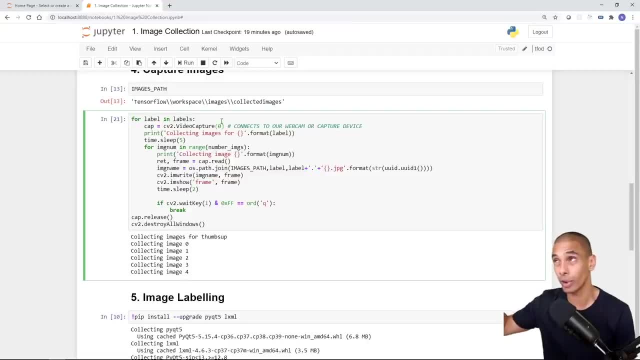 make sure that it works for you. sometimes i try zero, one, two, three and some particular some. actually some devices have virtual video capture devices, so you need to take those into account as well. just again, you might need to try five, six, seven, eight, nine. just make sure that you try a. 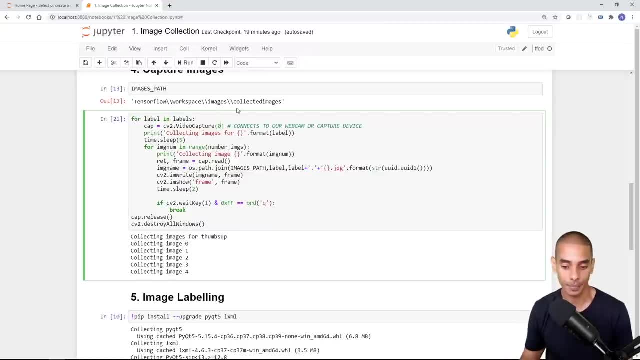 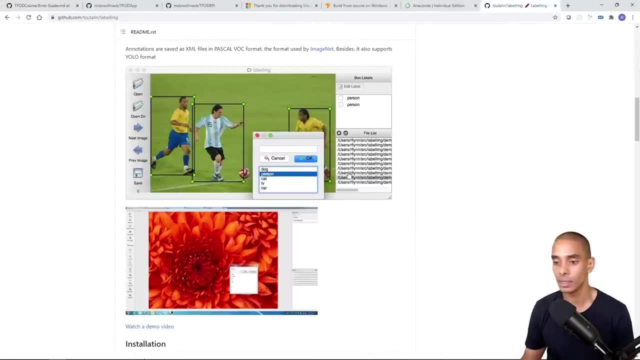 bunch of them. ideally, you should see that pop up appear exactly as i showed. now we're going to get to our labeling. so, as i was saying, we're going to be using label image for this. so this particular package here now. if you want to take a look at this package, you can go to githubcom. forward slash. 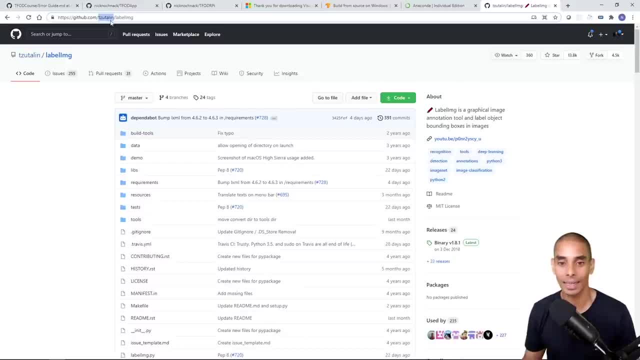 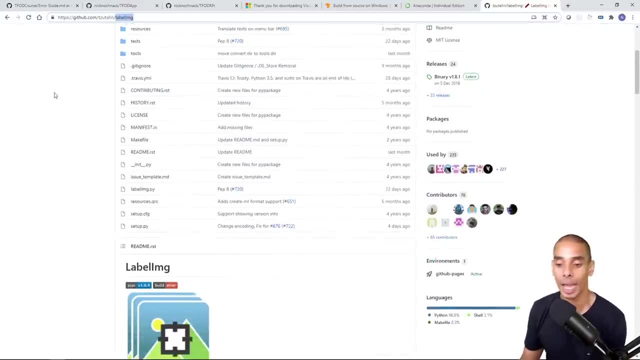 i don't know how to pronounce that t-z-u-t-a-l-i-n. zootap. sorry if i butchered that name. massive respect to you. it's an awesome package, all right. so we're going to be using label image to be able to go and label our images. now, when i talk about labeling, 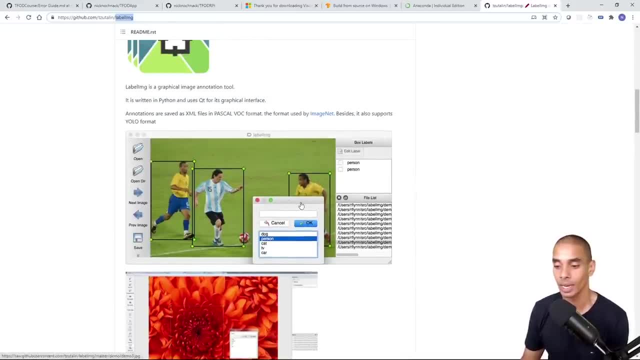 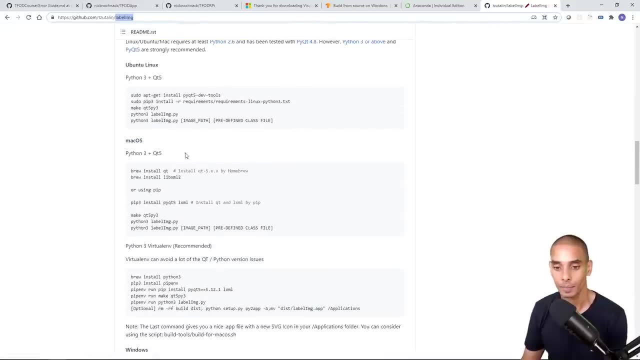 really we're just drawing boxes around the stuff that we're trying to detect. now. also, another thing to keep in mind is you can label multiple objects in one image as well. so another thing to to keep up your hand now down the bottom here there's a whole bunch of installation steps that you can. 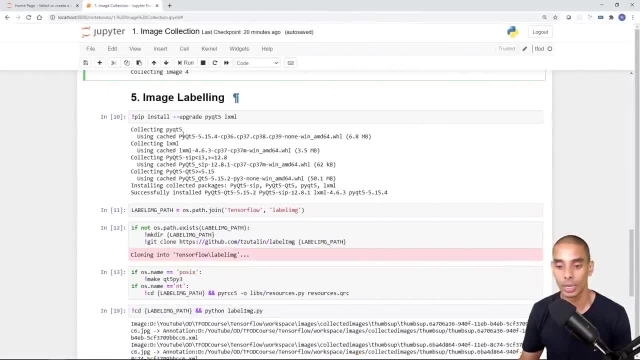 actually go through. now. what i've actually done is i've actually included this within the jupyter notebook. so rather than having to step out, install, do all of that stuff, we can actually just install it using our notebook. so, first up, what we're going to install is pi, qt5 and lxml. so 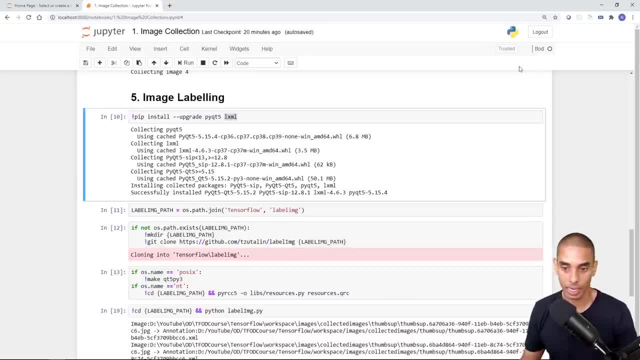 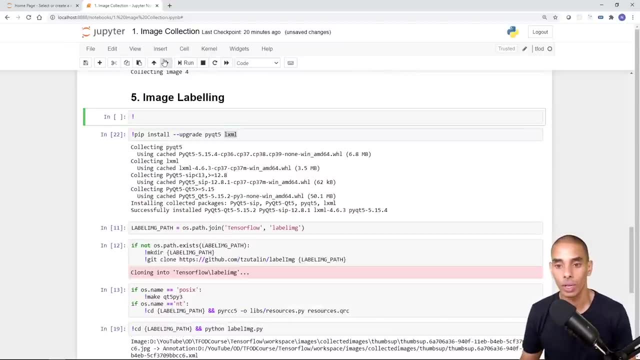 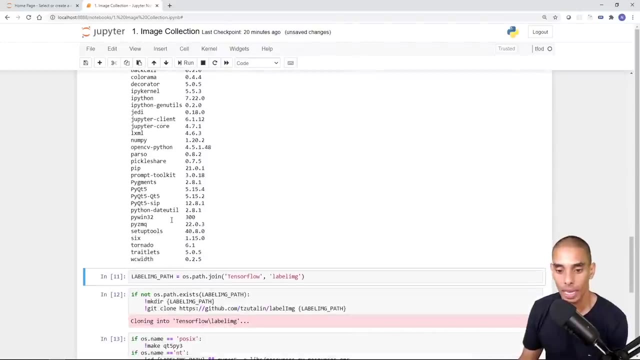 if we run that now, remember we're inside of our virtual environment. so if we actually take a look at what we've got in here now- pip list, now let's actually run the cell first. cool, so that's now installed. and if we run pip list, you can see that we now have a whole bunch. 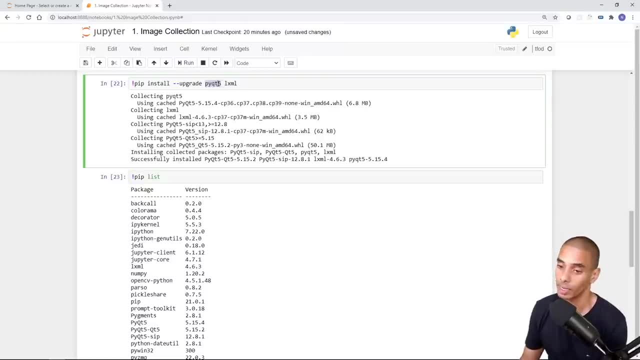 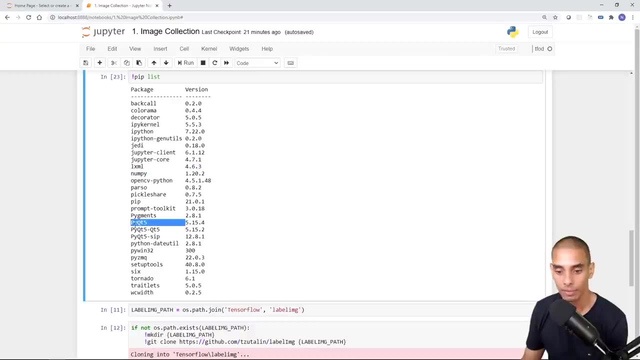 of other stuff installed and if i we look at the two libraries or dependencies that we just wanted to install, so pi qt5 and lxml. we now have lxml, which is there, and pi qt5, as well as all of its other dependencies, so we're good there right now. the next thing that we want to do is create a. 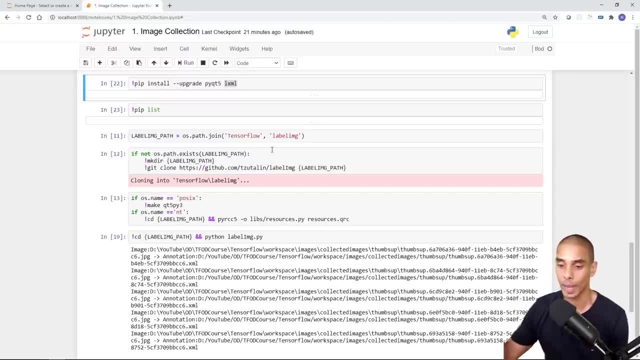 little home for our label image file or label image package to be saved. so what we're actually going to do is create a new folder called tense flow and then label image, so it'll be inside of our tense flow folder, and then a new folder called label image, so it's effectively going to be able to. 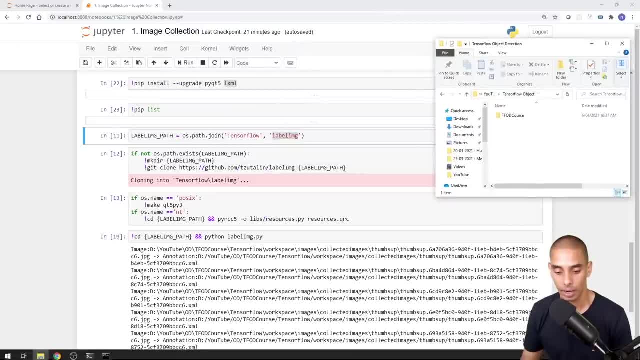 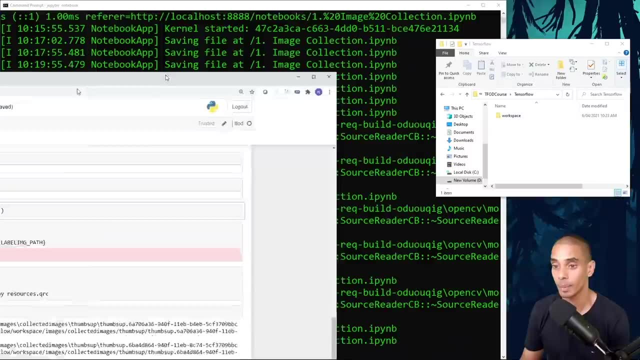 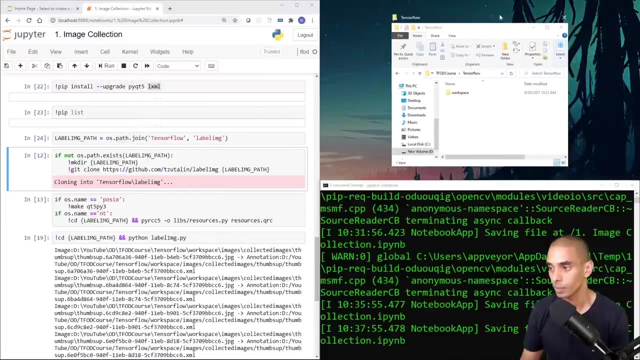 to be. let's keep this open. i don't know why i keep closing that. um. so tfod course, tense flow. so we're going to create a new directory here called label image, and that's going to be where it gets stored. so if i run this cell, minimize this and then if we now go ahead and create this, what we're 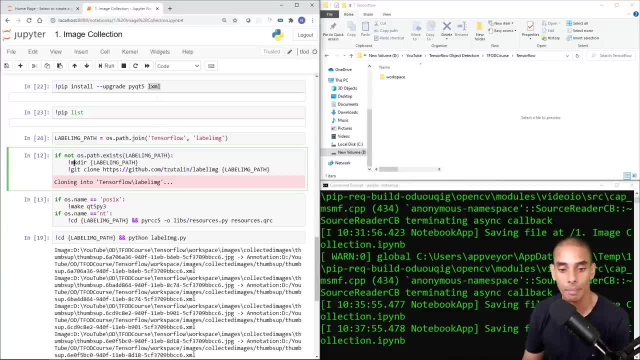 effectively going to be doing is, first up, creating a new directory using make dir or that make dir command there. so first up, we're actually going to be creating a new directory called label image. so here we're going to check whether or not that file path exists. So if it does already exist, as in it's 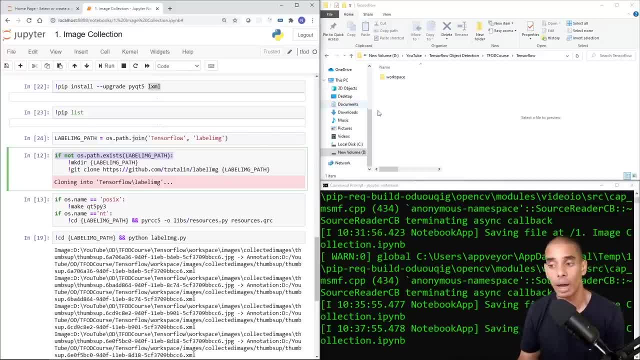 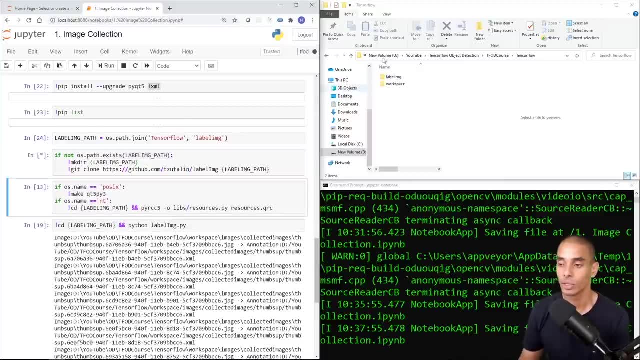 is installed, then it's not going to do anything. So if you get any errors, what you might want to do is actually just delete the label image folder and run this cell again- Now, in this case we haven't run it, so we can run that. So it'll create a new directory called label image, which you can. 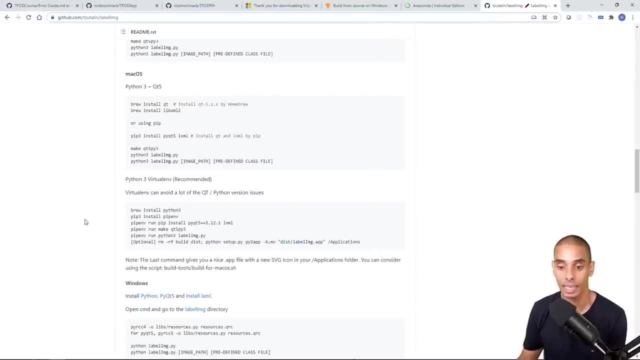 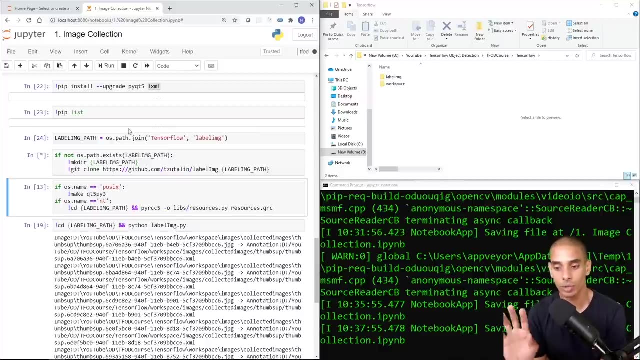 see there, And then it's actually going to go in ahead and clone this thing that I was actually showing you. So this GitHub repository, it's going to clone that. So whenever I'm running these commands through a Jupyter notebook, it tends to be not a little bit slow, but you don't actually. 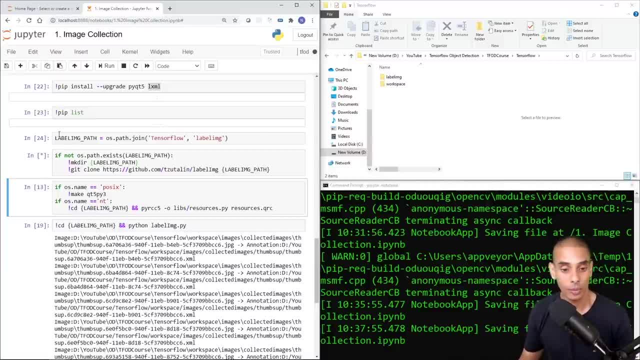 see the progress. So right now it is running. So we've got our little star over there so you can see it. So it is running. You're just not going to see it if you're running on a Windows machine. but it is cloning. So if we open that it doesn't look like there's anything there yet. Let's wait. 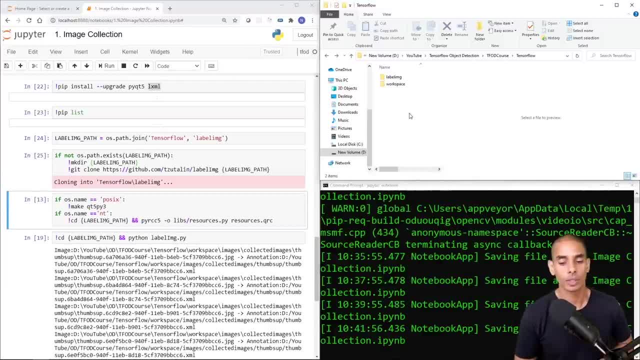 for that to clone, All right. So that is our label image package now cloned. So if we actually open that up, you can see that we've now got. We've got that cloned into that folder. So we've got tfod tenseflow label image and inside of that 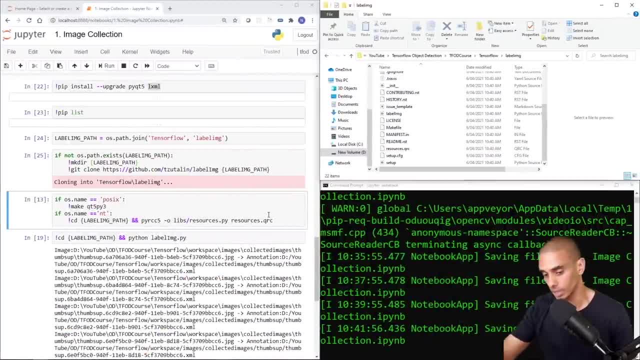 we've got effectively all of this stuff cloned into our local repository. Now the next thing that we need to do is actually go on ahead and install label image. So I believe that might be a typo there, So let's just copy that over here. Okay, And then what we're going to be doing. 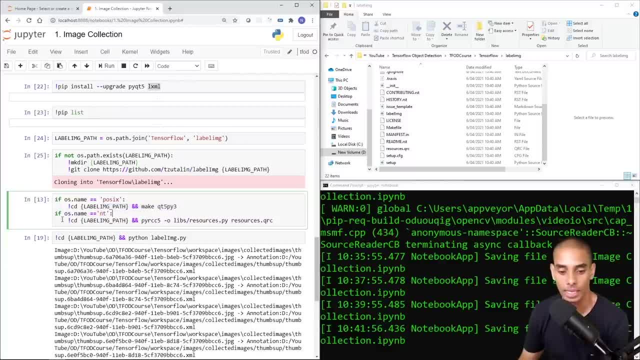 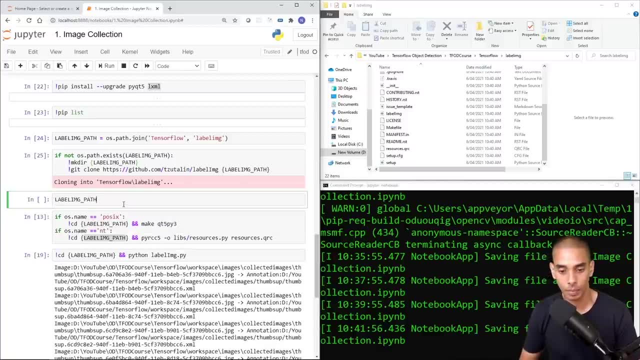 so again we're running on a Windows machine, So we're going to be executing this path down here. So we're going to cd into that label image folder. So if I actually show you that label image, So again we're going to be going into this folder. So tenseflow label image, Then we're going to be 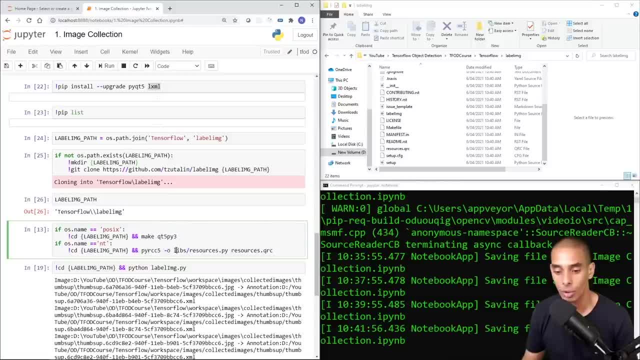 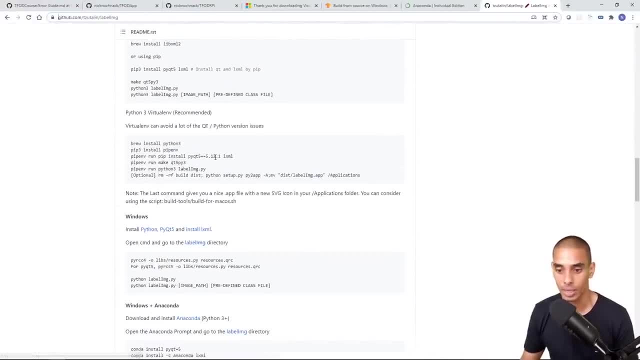 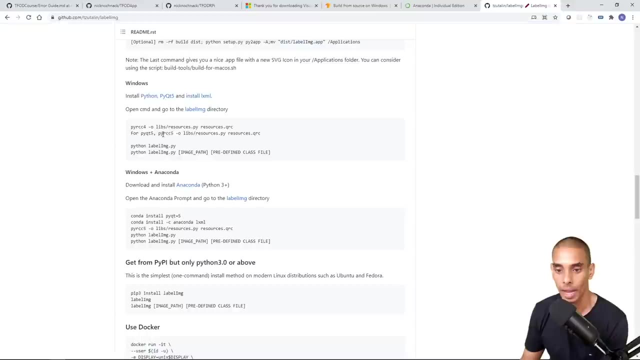 running this command here. So pyrcc5-o libs forward slash: resourcespy- resourcesqrc. This is effectively the installation steps that are recommended from the main package. So if I actually go down here, So for Windows we're going to be doing this. So pyrcc5-o libs forward slash. 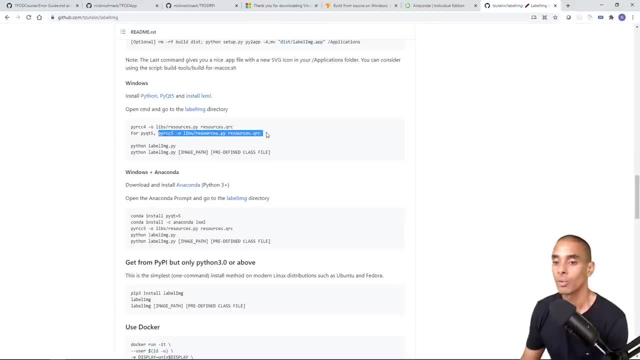 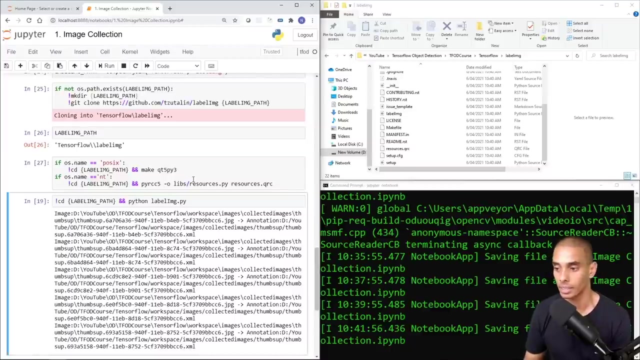 resourcespy, resourcesqrc- And then we'll open it up So effectively. we're just running through the same installation steps that you would get from the actual repository itself. So if I go on ahead and run, this now should ideally run successfully. So it doesn't look like we've. 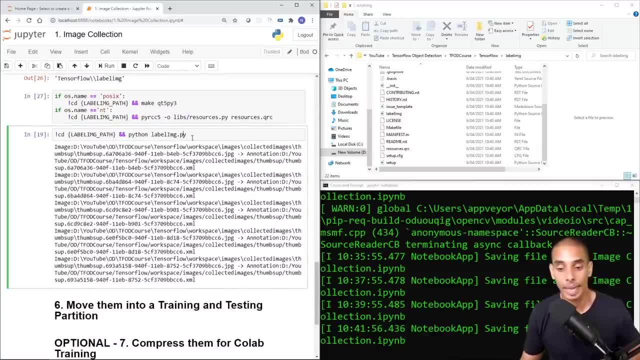 got any errors there And then if we go on ahead and run this command, what should actually happen now is that it'll actually open up the label image package, So the actual application will actually open up. So if I actually hit shift enter, you can see label. 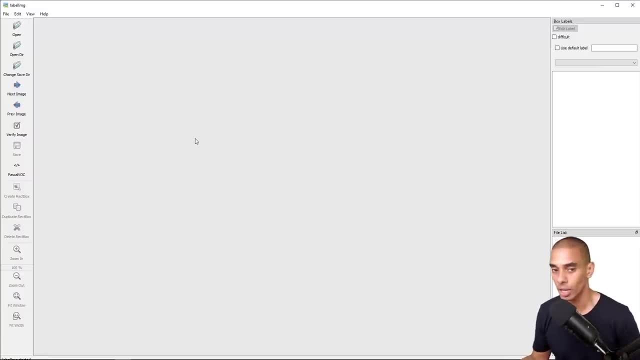 images opening up. So we've now gone and installed it from scratch and actually opened up the label image package. Now the fun bit comes: actually going on ahead and labeling our images. So what I'm going to do is I'm going to over this left hand side here. you can see that this button 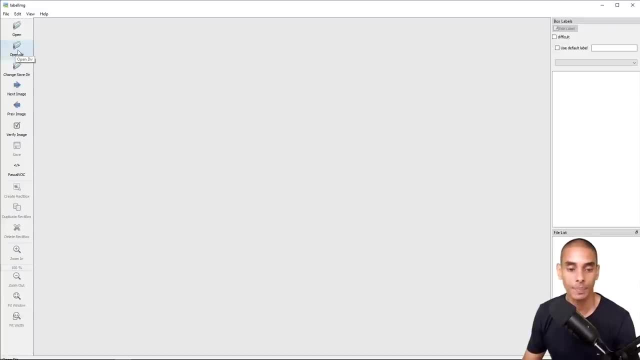 called open deer. I'm going to wave my cursor around it so you can see it. So I'm going to hit open directory, we'll open deer, And then I'm going to navigate to my folder. So I'm going to go to YouTube. TensorFlow object detection. TensorFlow object detection. 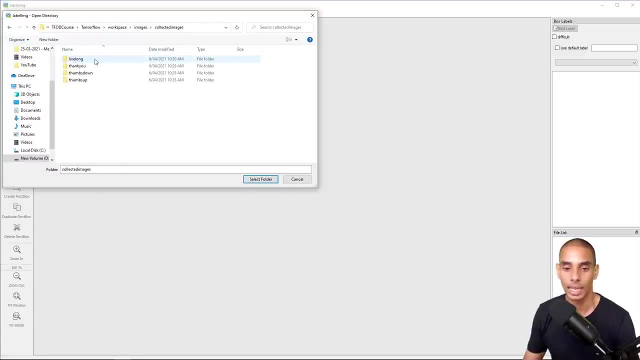 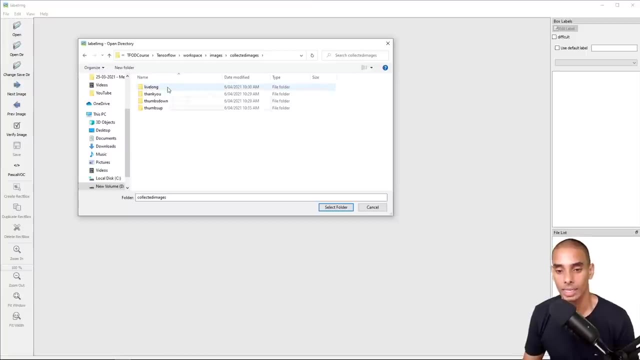 course, TensorFlow, workspace images, collected images, And remember we've got a repository or a folder for each one of our different classes. So in this case, here, what I'm going to do is step into live long first hit select folder And sometimes it won't actually open that folder. 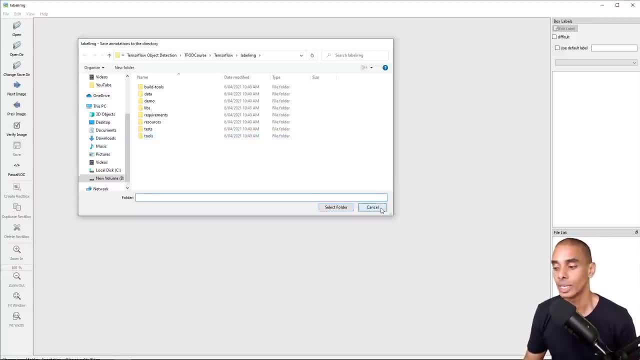 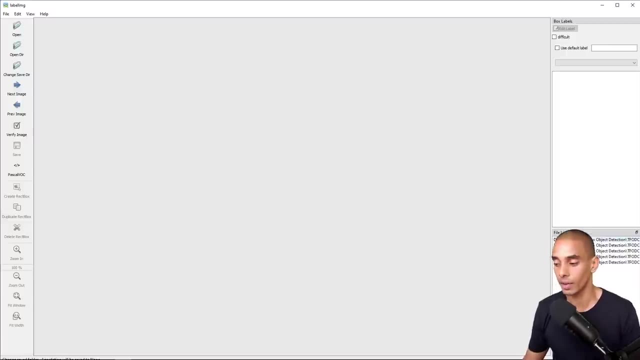 it'll just ask you to select that folder again. what you need to do is just hit cancel. But as long as you've got the files down here, it means that you're able to label them. So I'm going to start out by labeling my first image. So if I double click onto that, that opens up our image. 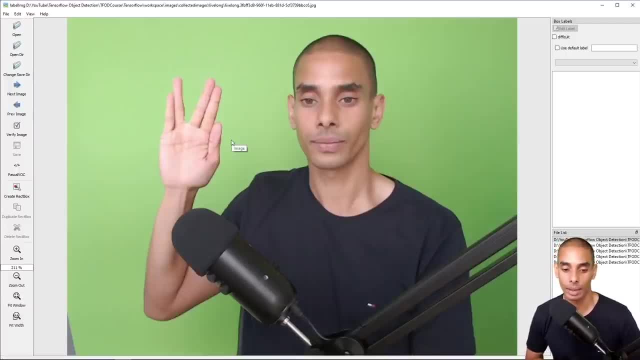 Now just a couple of quick tips So what you can do in order to label this image. so there's a shortcut, right? So all you need to do is hit W And this is going to open up a little labeling thing over here. So you can see we've got our cursor To label an image. what you then want. 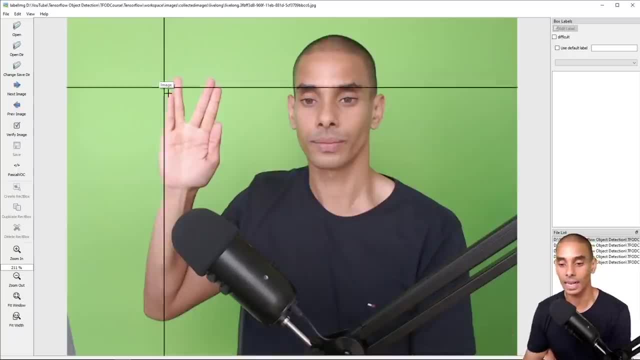 to do is just select the first point that you want to label and then drag down and create the object. Now, what I tend to do is, I find, tend to find the bottom most points. In this case I'm going right to the top of my finger and right to the edge of. 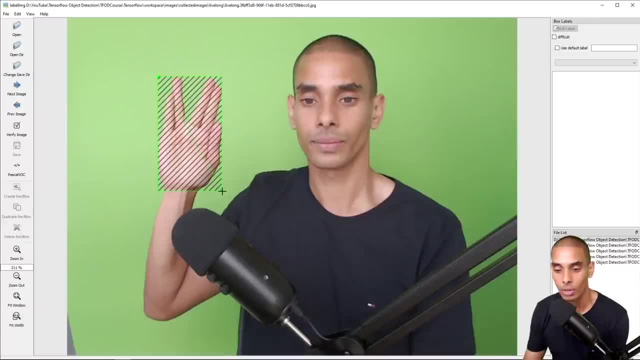 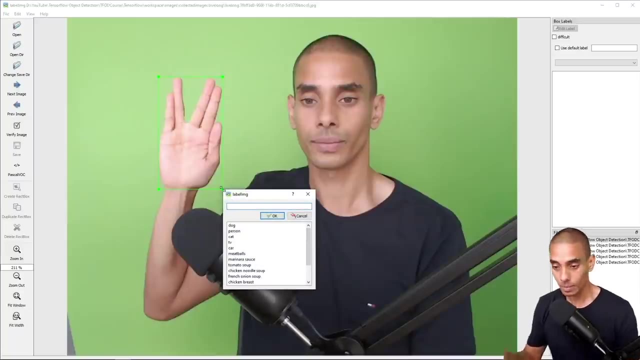 my hand, then what I'll do is I'll drag it so that I only encapsulate the components of my hand that I want. So you can see I'm going just to the edge of my- what is that? pointer finger? and to the edge of my wrist. So I'm going to be as tight as possible with my detection or my label, And then 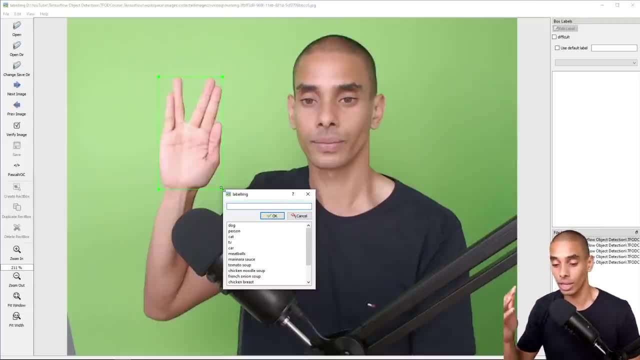 to remember when I kept on hopping on about make sure that your label detections are tight. So make sure that you pay attention to what you actually name these labels, because when we go to train you're going to need to make sure that the names of the labels in your annotations, which is 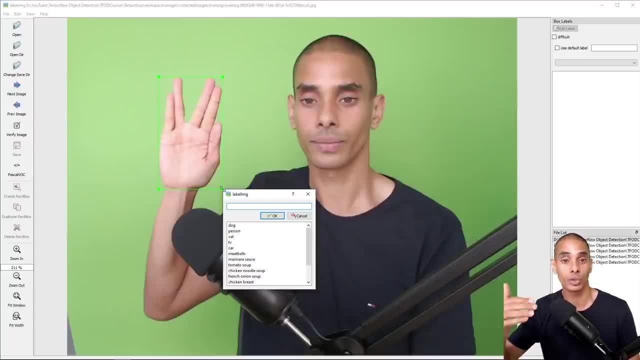 what we're doing right now match the actual labels that you pass through to your model that you're training. So in this case I'm going to label it live long and I'm going to have a capital L and a capital capital alpha live and a capital alpha long. Now when I go to set up my labels later on, 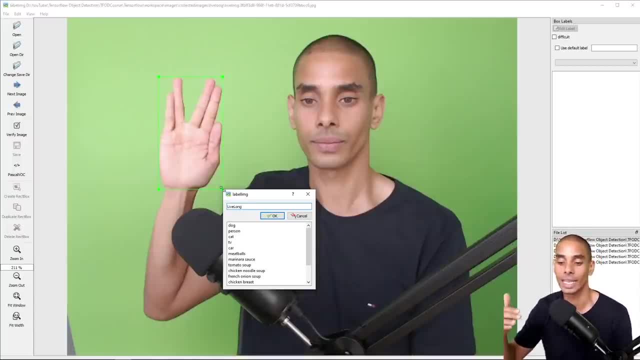 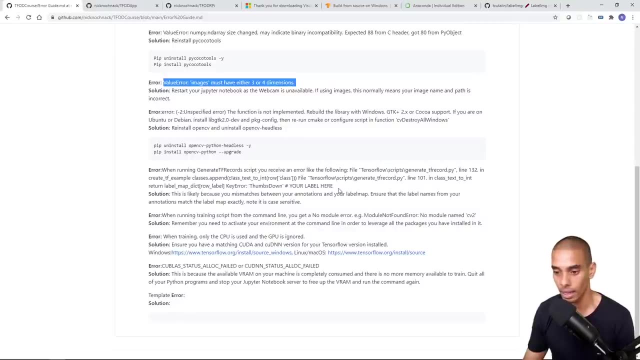 in my training step, I'm going to make sure I've got the exact same thing. If you don't, you're going to get an error right And that error is going to look like this. So in this case- here you can see- it's when running generate TF. 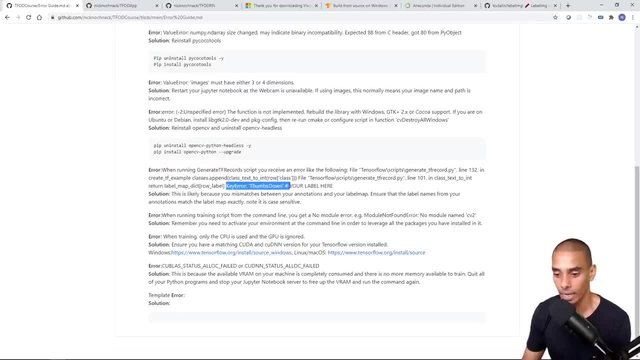 record script: blah, blah, blah, blah, blah. And then it's: you're going to get this key error here, But I'm actually going to show you what that looks like when we go to do it. So in this case, 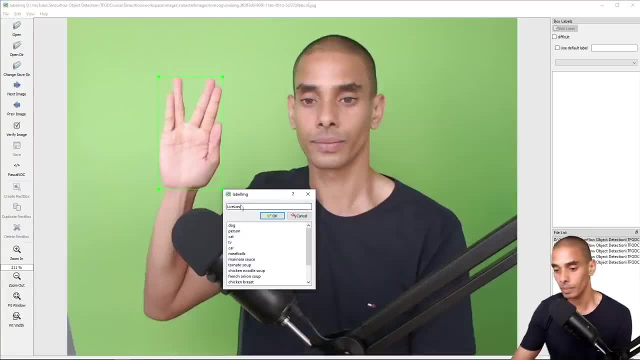 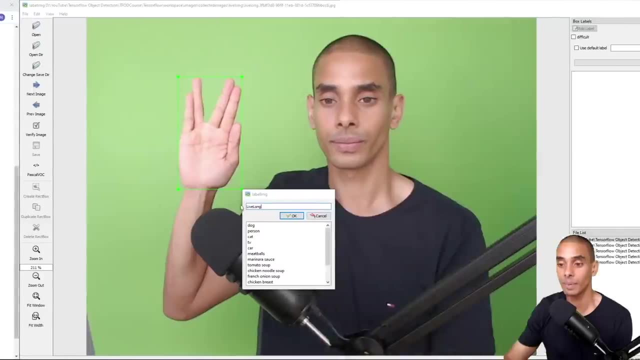 keep in mind. I've labeled it capital. live capital long. If I go and screw up when I go to train, it's fine, you can fix it, it's not hard, But you are going to get an error In this case. pay a lot of attention to the capitalization and the case of your labels. 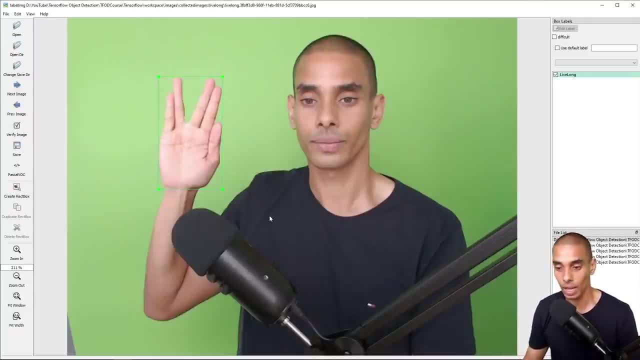 So I'm going to label it live long, hit OK and then hit Ctrl S to save it. and save: That's my first image labeled. So we're going to go through and do the rest So I can select my next image. And again, we're going to keep them tight. I can do that And say I screw up. 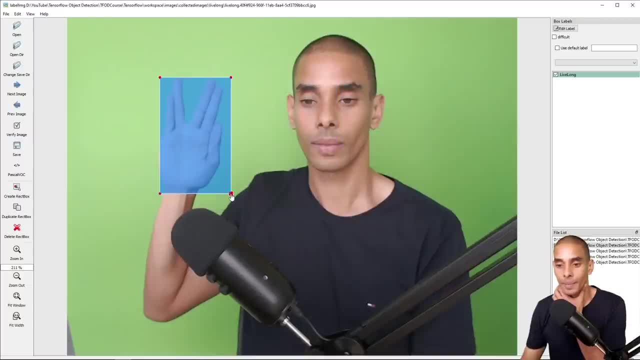 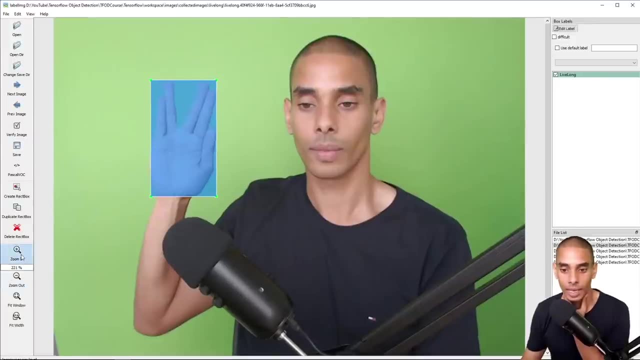 right and do that. I can still go in, drag this back and tighten up my detection, So I can do that, Make it a bit tighter, And you can see that there's a little bit of my image over here that I haven't actually captured, So if I zoom in, 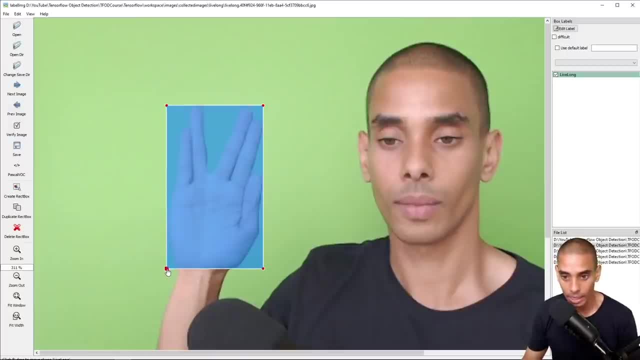 you can see over there that I'm not capturing that, So we might pull that in Now. maybe I'm being a little bit pedantic now, But that is my OCD kicking in And it is best practice, right? So you want to make sure that you get this as accurate as possible, So we're going to save. 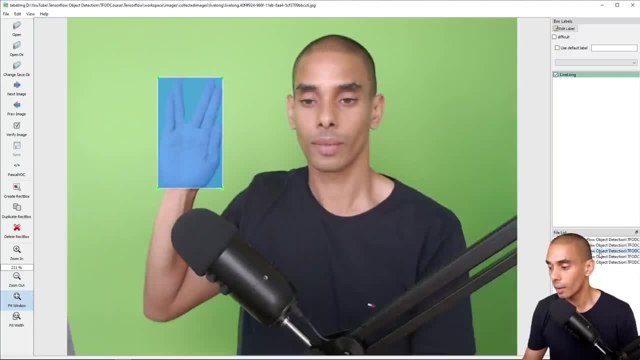 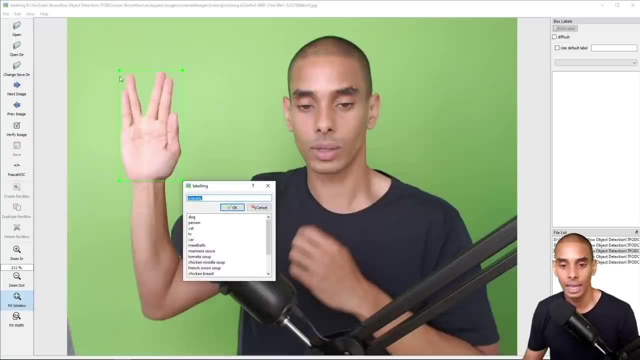 this. That's annotation two done. Now we're going to go to our next image And again do the same thing. So we're just going to do this for all of our images. Now, the beauty of what we're doing right now right- is that we can do this for whatever type of object that we wanted. 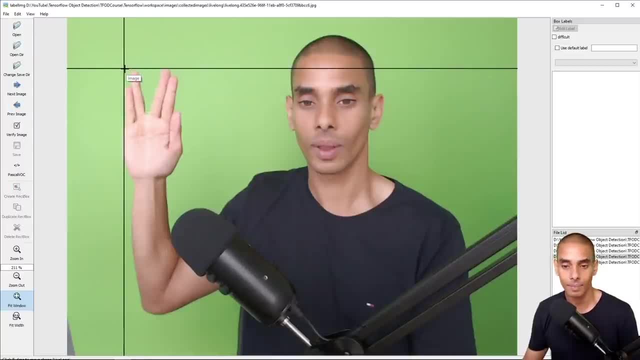 to say, for example, we wanted to do I don't know- And I saw a really, really cool video the other day of someone that used this to classify which way waves were breaking. I thought that that was pretty awesome. You could do it for a whole range of different applications, Obviously, 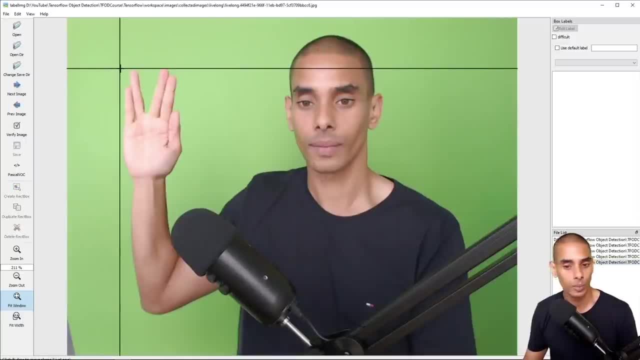 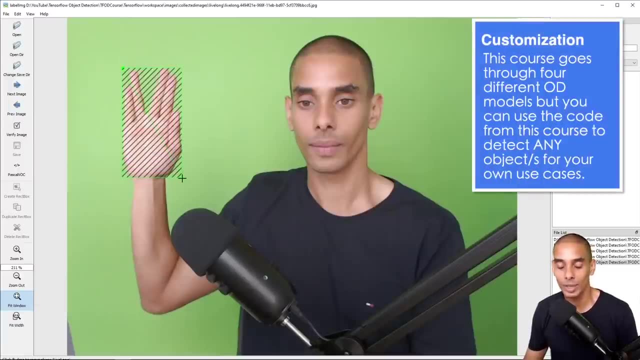 we did sign language. that was a great use case, super practical and super altruistic And there's like a whole heap of capabilities, Like there's people out there that need this technology. So if you've got the capability to do it and you're watching this course, by all means find something. 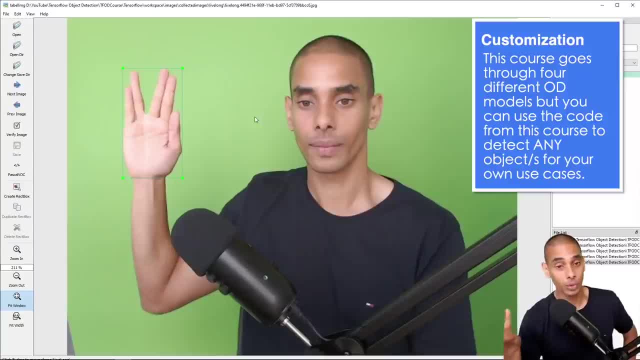 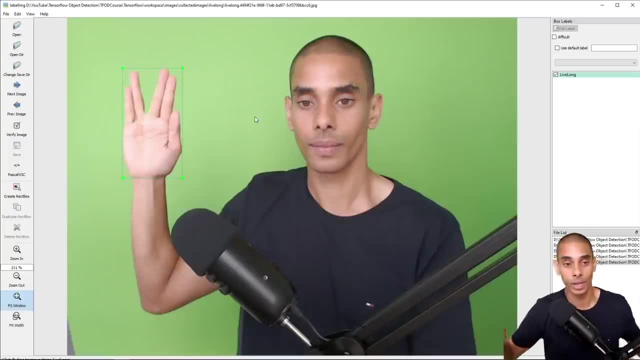 and give it a crack. So I'm obviously going to give you some examples when we actually go to do our projects. But again, if you get, come up with a good idea, this exact same process that we're going through: define your labels, collect your images, label them and then we'll get through. 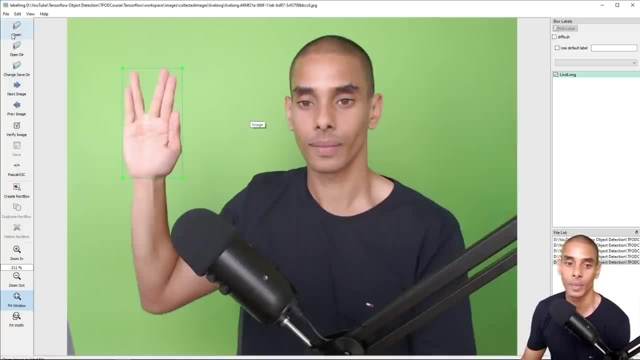 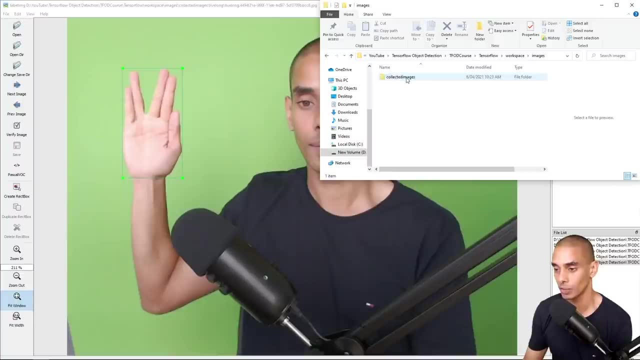 to the training later on, But you sort of get the idea That's what we're going through. Okay, so we're now going to label these images. Now, one thing that I want you to check as you're doing this is if you go into the images folder- and in this case we've done live long right. 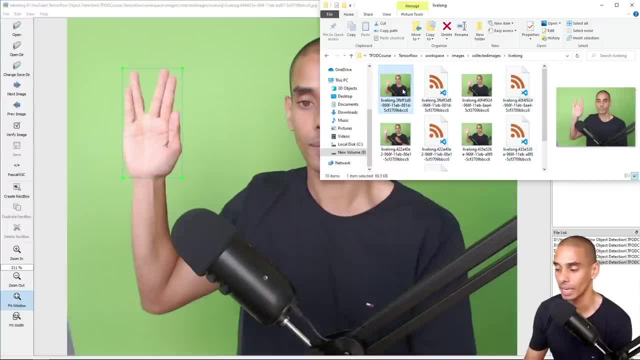 We have these annotations available, right? So in this case- I'm looking at this image here- I should have a matching annotation and it's going to have the exact same name as your image file, but rather the extension is going to be XML. So if I actually take a look, let's go details. 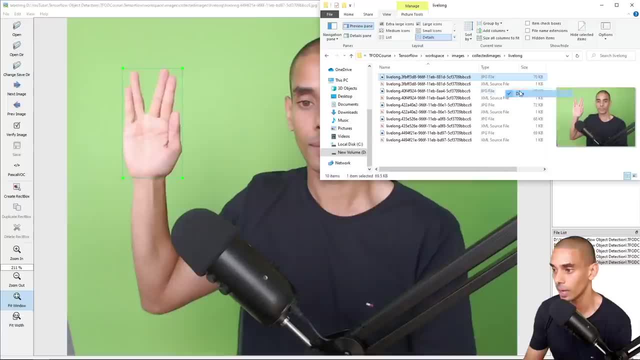 So in this case, I've got the image, let's do. we need date, we don't need date. So I've got my image over here, which is named whatever that is, dot jpeg file, and then I've got the annotation. 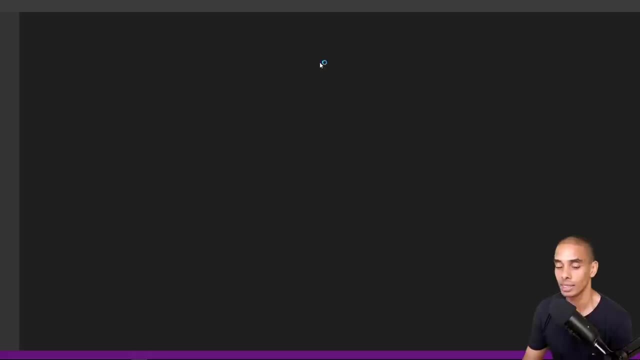 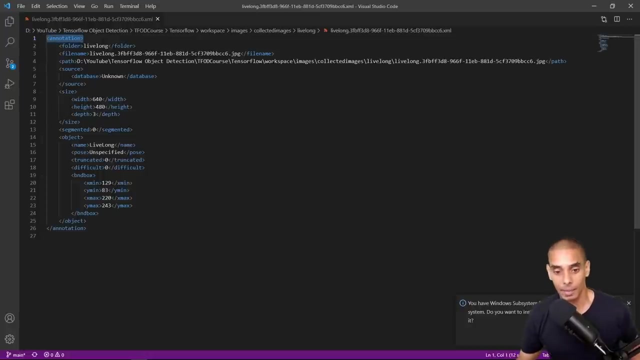 which matches that image. So if I open up this annotation, let's take a look at what's actually included in here. So inside of my annotation I've got obviously the fact that it's an XML file. So it starts off with annotation, then tells me what folder I'm in, what my file name is, the path to that file name. 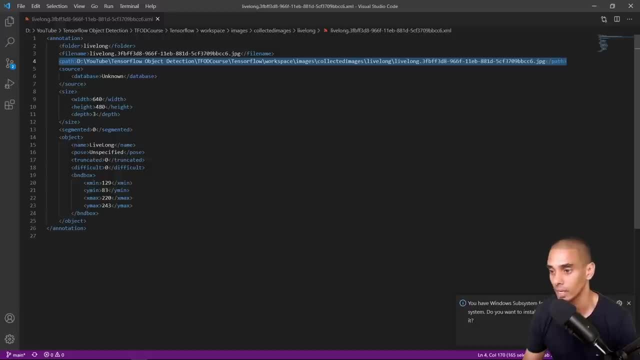 Now, this doesn't matter so much when it actually comes to training, because we're going to move these around the source And again, the database doesn't matter. here. The size is quite important, because this defines how big our image is. So in this case we've got width, height. 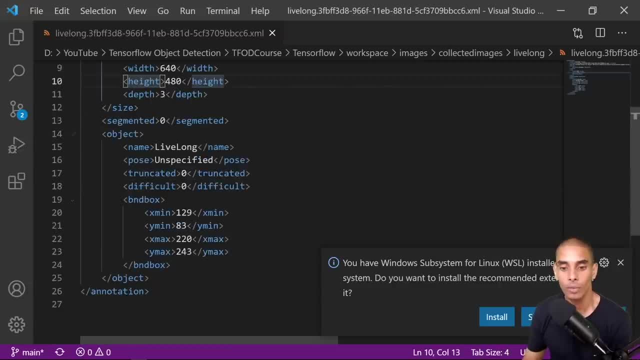 let's make this big A bit bigger. you can see a bit better. We've got width, height and depth. So in this case it's a color image, So it's going to have R, G and B whether or not it's segmented. So we're not. 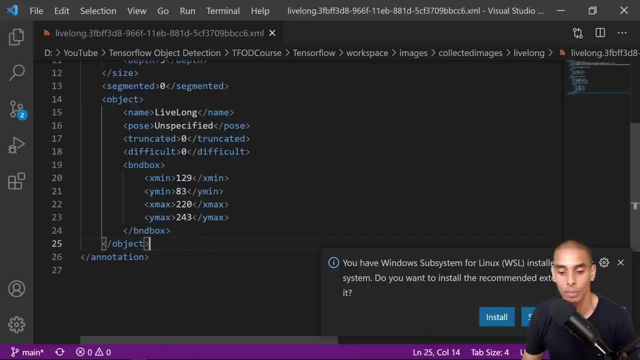 segmenting at the moment, And then- this is the bit that's really important. So you might have multiple objects in an image, in which case this will be repeated multiple times. So here we've got the name of our object, And again we've got it: capital live, capital long. So if you screw up, 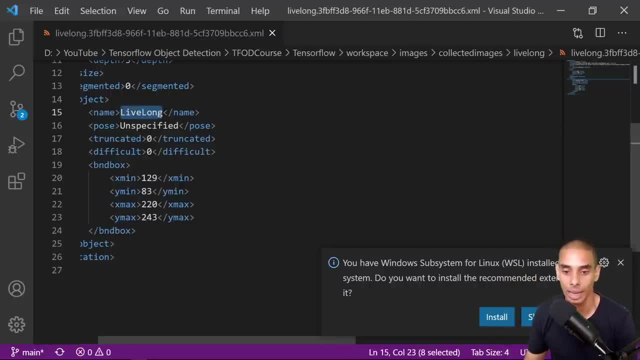 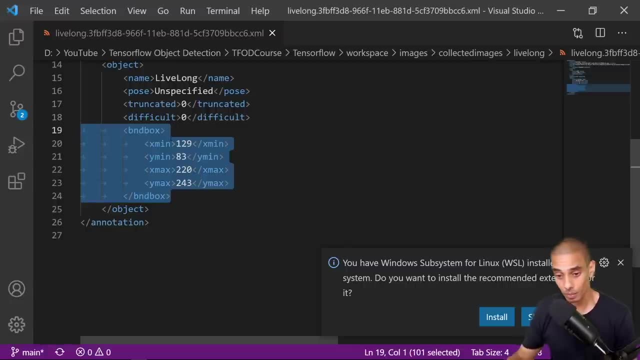 and you want it to the names to be different. you could just come in and change these names as well. We've got pose: we're not using that. truncated and difficult, we're not using that. And then we've got the bounding box. So again we've got the different coordinates. So we've got the minimum x. 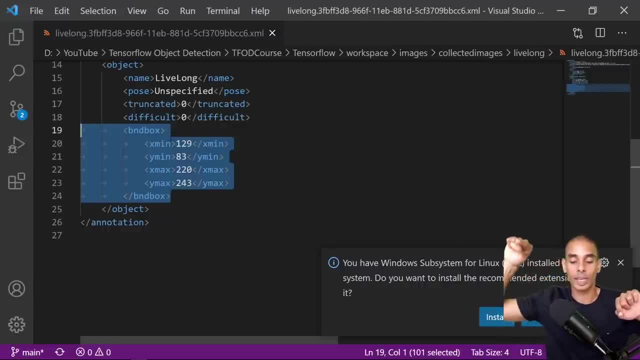 value and the minimum y value. So, effectively, we're just giving it two points, And we're giving it a point here and a point here, And the square that represents that box is going to be our bounding box. So that's really what it comes down to when it comes to labeling. So we're 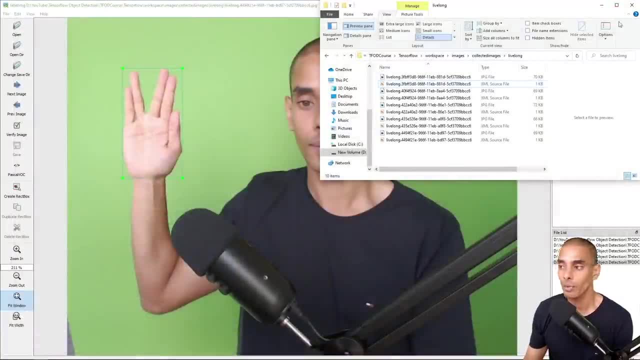 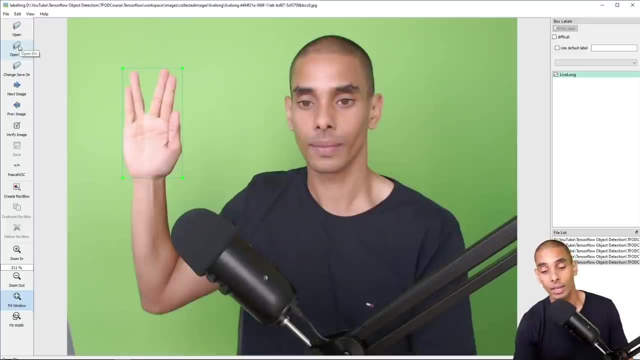 effectively creating these XML files. Okay, but right now we've only done our one class. So if we just wanted to detect live long, that's perfectly fine. You can go on ahead and jump off to training. If you only had one object to do, you can do that. In this case, keep in mind, we had live long. 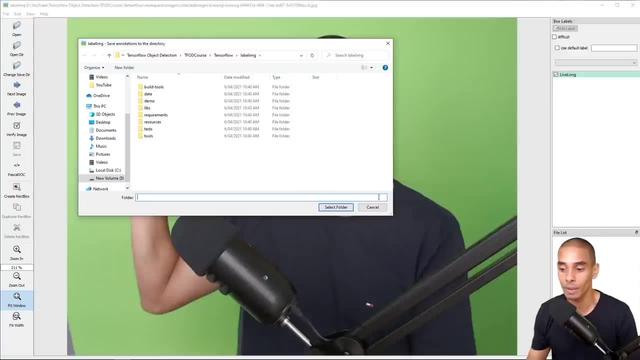 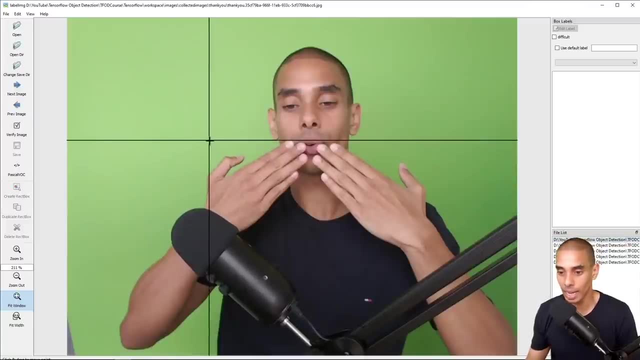 we had thank you. So if we go and do that now, so I'm going to step into that folder and then hit select folder. sometimes you got to hit cancel and then open up our image. So again we're going to do the same thing Now. again I'm a little concerned that we've got the mic there, But that's. 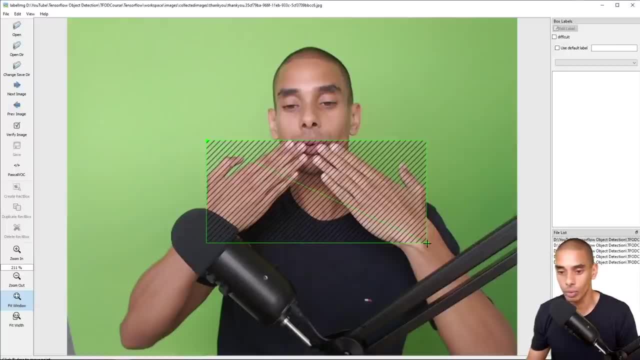 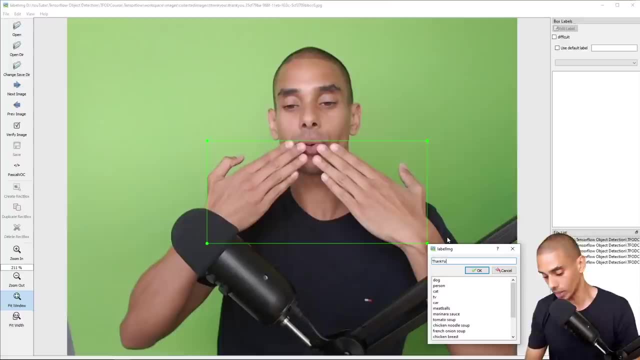 fine, Let's give it a crack. So in this case I'm going to label to my knuckles and again to my face. So this one is going to be called Thank you. Oh, almost had a type of that dangerous. So. 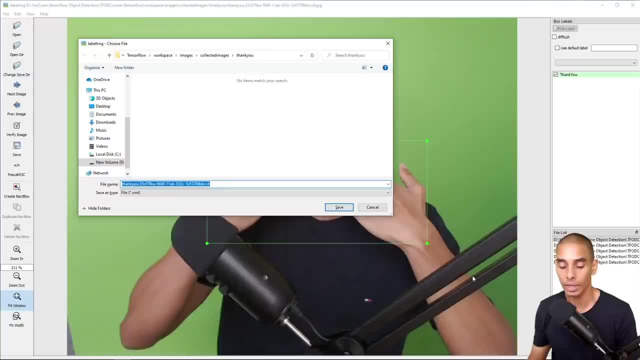 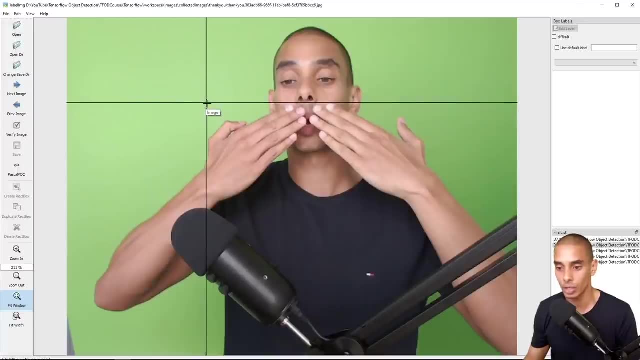 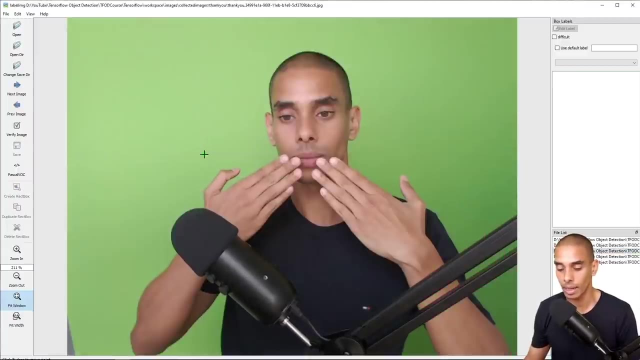 capital T and capital Y, hit OK, Then again Ctrl S to save and we'll go to our next one, Again, different angle. So this should ideally give us a better chance at generalizing, And let's save that. save, Go to our next image. And again Mike, there we'll see what that does Again. 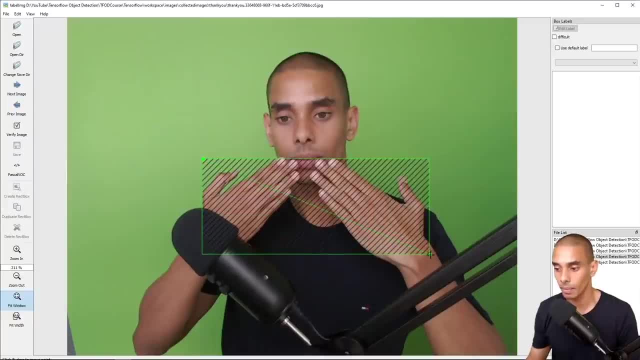 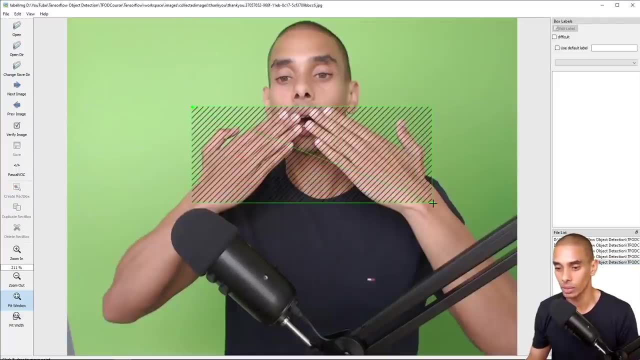 we're just going to keep going through. So we're going to do the next one, Save, Next one. And again, looks like I've only got two angles. they're sort of up and down. So one idea there and I've screwed up my detection. So I'm just going to hit OK, And then I'm going. 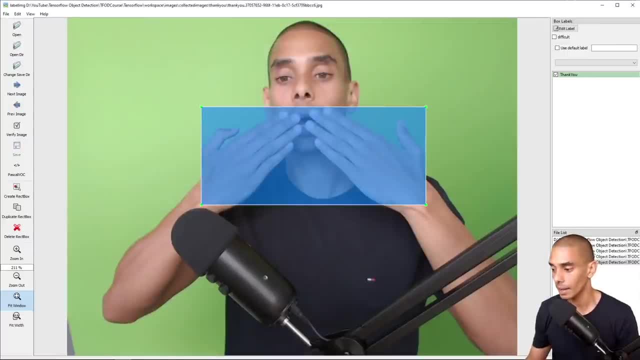 to tie it in that up, Save, Cool, So we can double check just by clicking through all of them. In this case, I can see all of my detections are saved and they're good. I've got a couple of images here, But I believe what will happen actually I'll show you in the 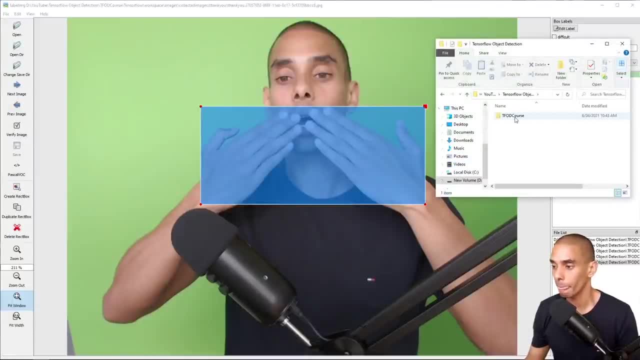 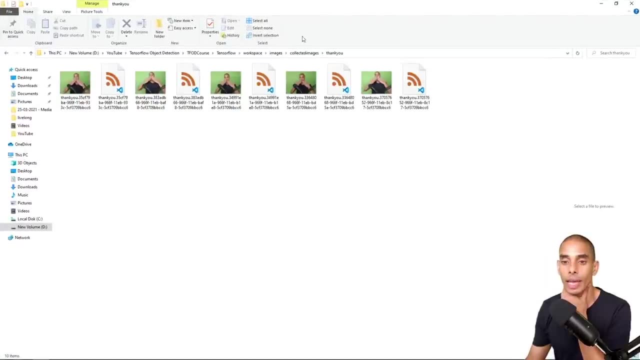 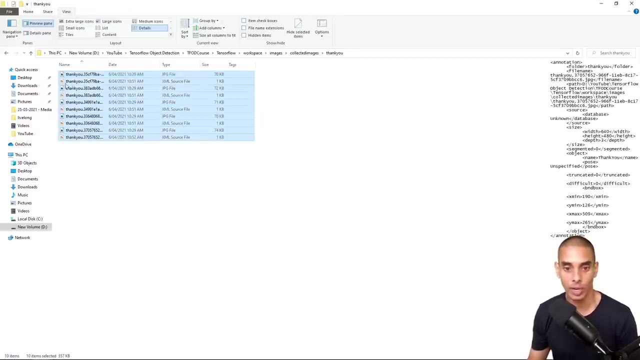 next one. So in this case we should be fine. So if we go and check out images again, Thank you. So again, remember, we've got all of our images and we've got their associated annotation files. So ideally we should have a round number, So it should be even so we've got. 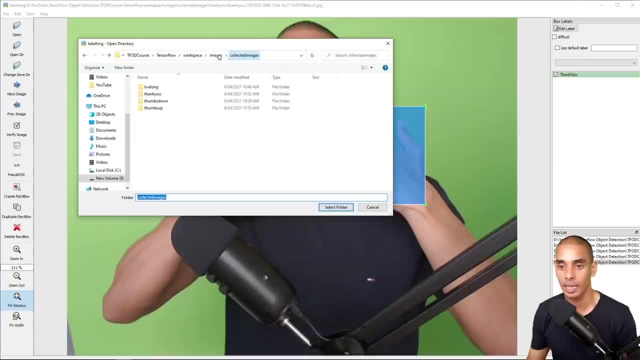 10 images or five images, and we've got five annotations, So we're good. Then I want to show you what happens if we forget to save. So let's do thumbs down now. So double click Right. So I'm going to label thumbs down. 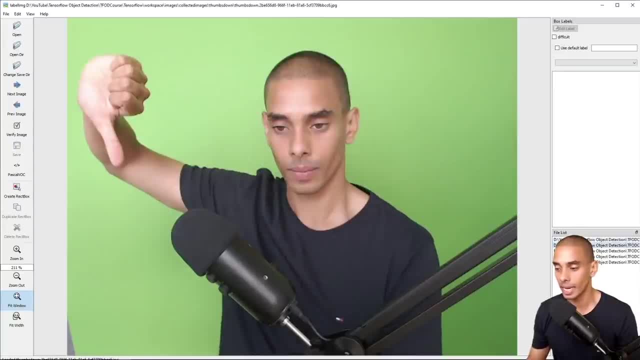 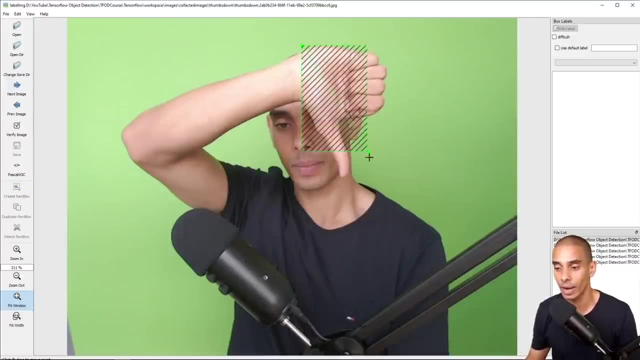 Hit okay. If I then go and double click into my next one, when I come back to that image, my annotation isn't going to be saved. So you've got to keep in mind that you need to save it right So you won't actually have that file created. 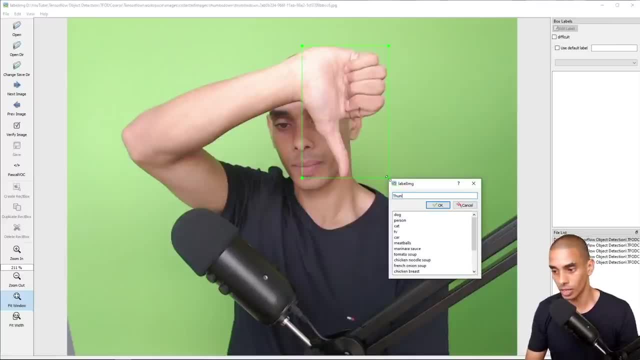 Again, I'm going to just do thumbs down, Change my label name. So it's going to be thumbs down, Save. Now, if I step into my next image and come back, I'm going to have that annotation saved. So we'll do our next one. 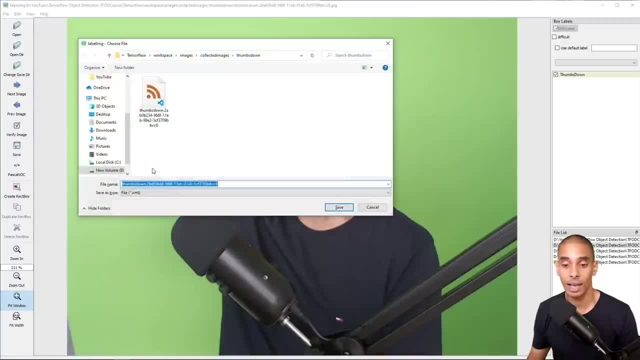 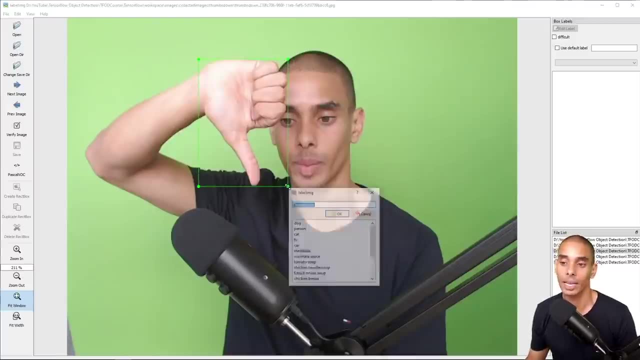 So sometimes you might notice you forget one. If you're doing a ton of these again, you might, you might. sometimes it happens You forget to save. Now a lot of some people have asked about how would we scale this up? 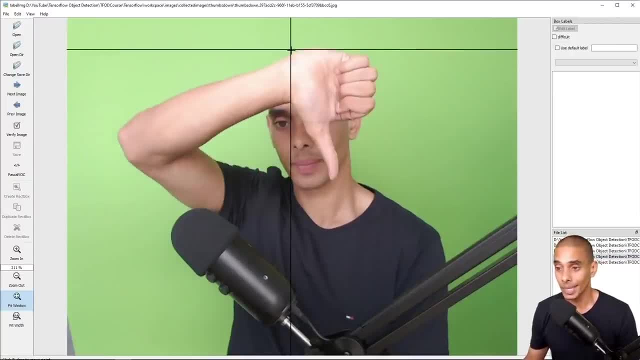 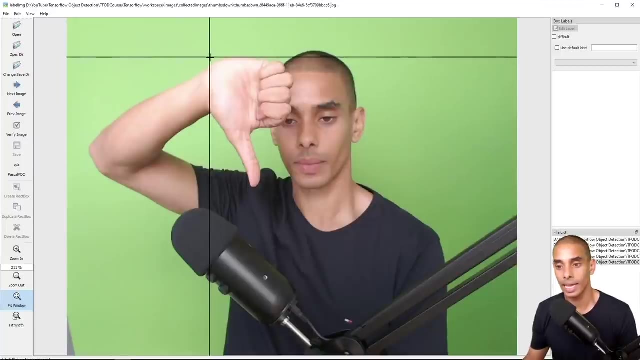 So say, we've got thousands of images. There's normally two ways that I recommend. So you can either outsource this- mechanical Turk is one way to go- Or if you go to like Upwork or Freelancer, that's another way. The other way is that there are newer tools these days that actually use a technique called. 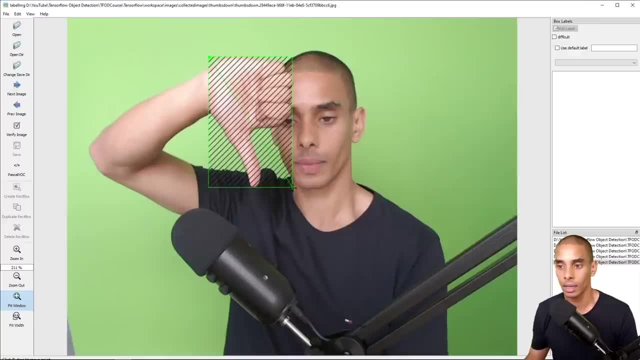 auto labeling. So they'll actually train a lightweight object detection model to be able to detect the different objects within the images. So it's pretty cool, right? And then what it'll do? it'll ask you to label, say, for example, 10 or 20 or 15 images. 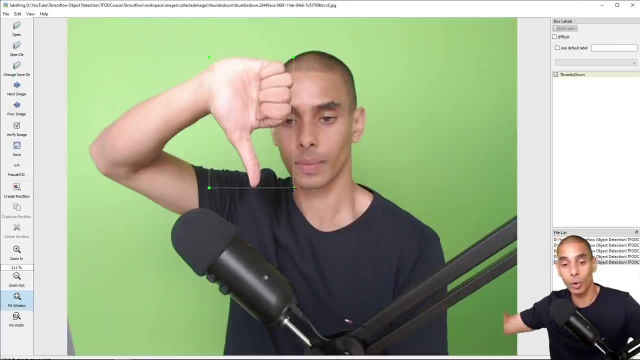 And then you can run that auto labeling And it'll go and auto label all of the other images based on the lightweight model that's already trained. Now again, those are pretty sophisticated, but if you'd like to see a video on that, 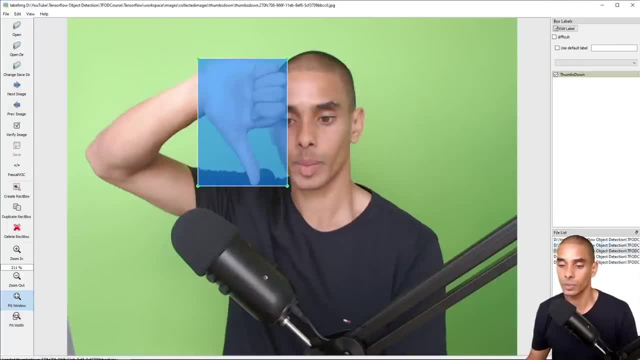 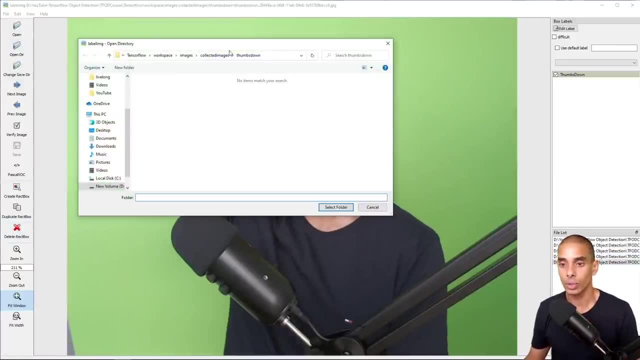 by all means, do let me know. I'll see if I can spin something up. In this case we're just going to use label image. So again, you can see all of our images looking fine there, No issues? Okay, let's do our next directory now. 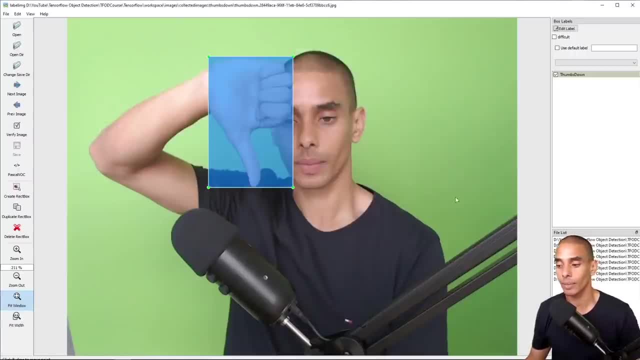 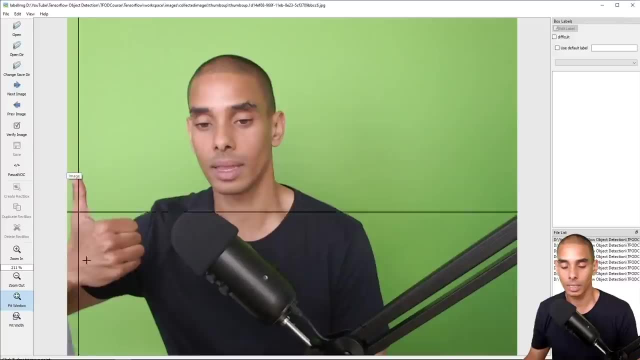 So we've done thumbs down, Now we want to do thumbs up, And this was the one that we remember we had a lot of images for, So we went and collected more, So we are now doing thumbs Down. Let's just- I can't remember if I labeled that correctly. now, 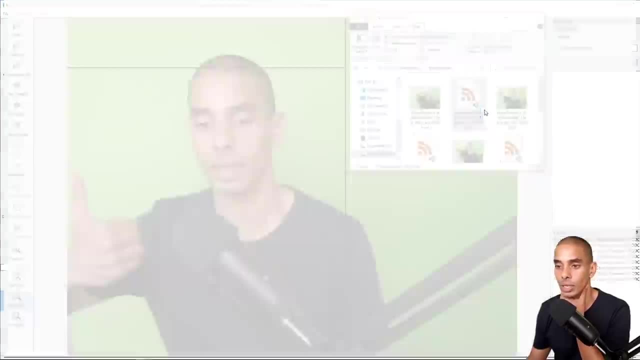 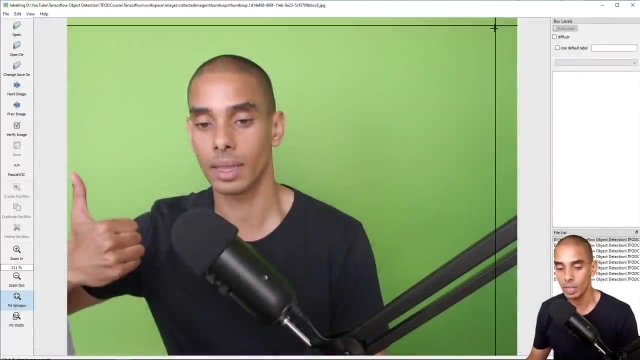 So the other one: we did label thumbs down. right. So if we open up our annotation, Yep, thumbs down, Okay. so we're good. And thumbs down with capitals, Perfect, All right. So now we're going to do thumbs up. 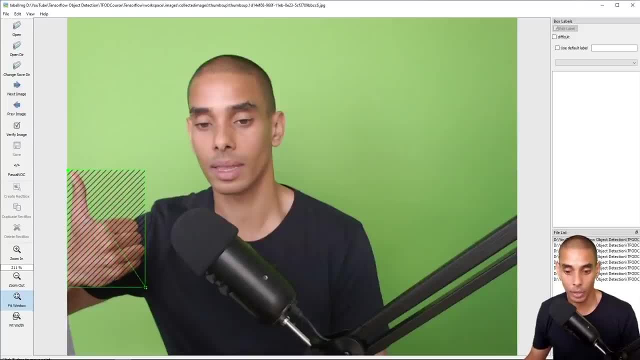 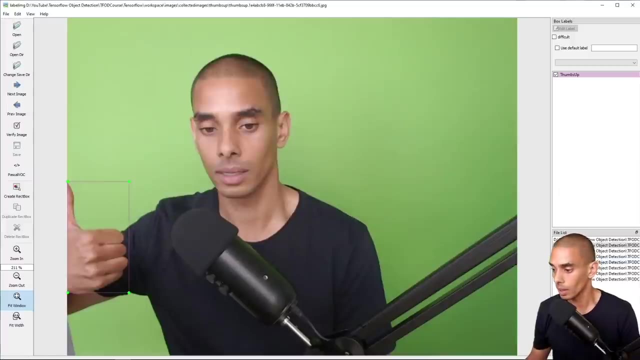 So let's label it. And same thing. hit W to get that shortcut and open it up. This is going to be thumbs up. Save Next image. This is a partial, so that's fine, Let's do it anyway. Again, I'm just going to keep going through. 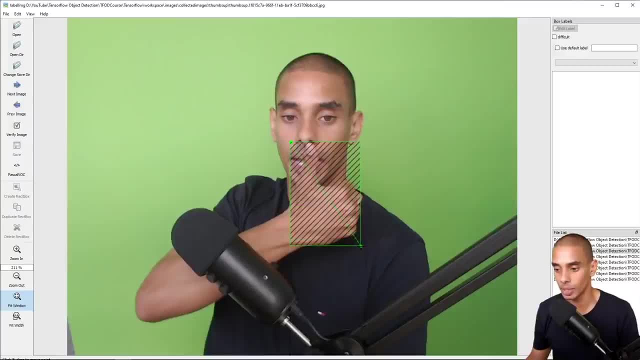 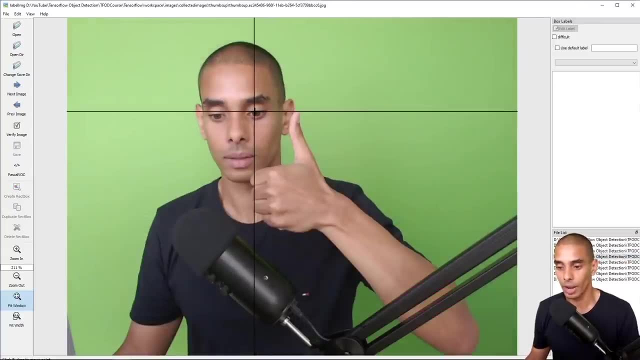 So again, this can get a little tedious when you've got a ton of images But just sort of walk through. Normally I'll grab a coffee and I'll just grind through and label these objects And again prototype. So don't start out by labeling thousands of images. 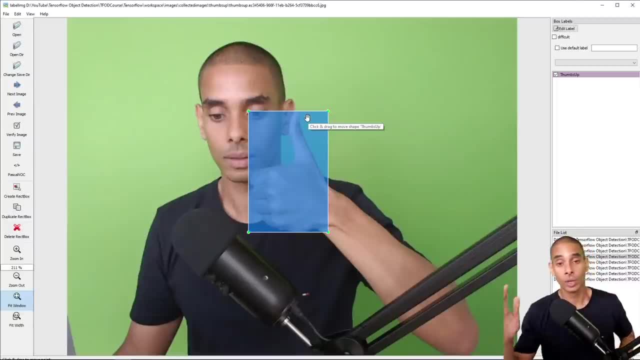 because it might not be the right technique. So what I'd always recommend is do 10,, 20,, 5. If you really want to keep it super fast, prototype, train and then evaluate right. So don't commit to building a huge object detection model before. 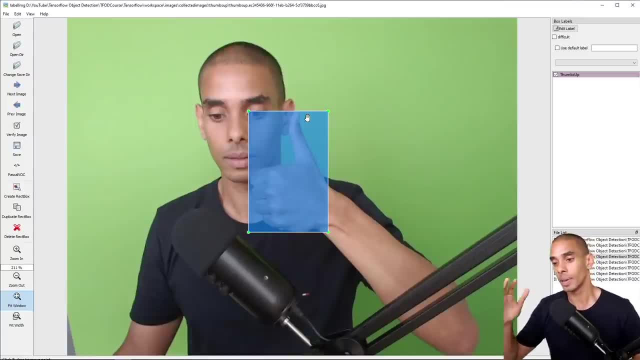 Don't commit to building the whole thing with thousands of images, because you want to make sure that you are going down the right technique, You're getting the right levels of data, You're getting you're using the right types of sensors to be able to do this. 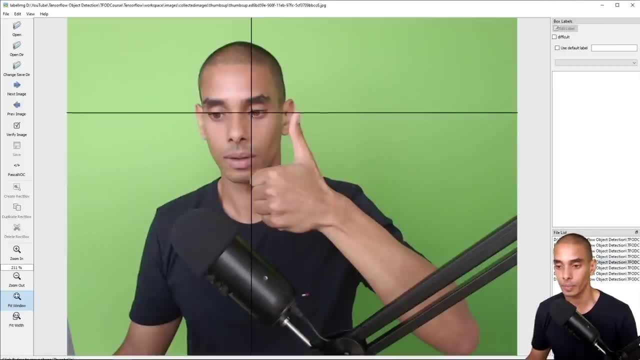 So, prototype, first, going to make you a lot more efficient. Going to keep doing our thumbs up And again going to adjust our label- this time because I screwed up So that looks a bit better- Save, And then we're going to do that. 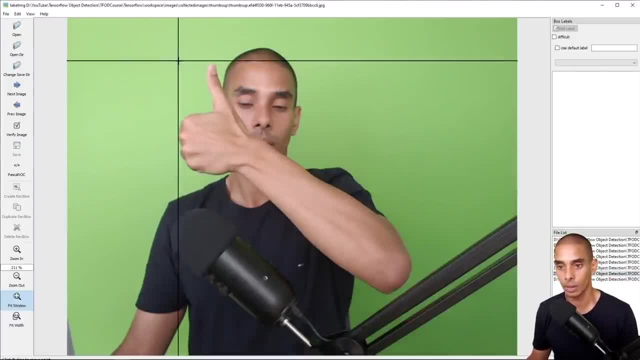 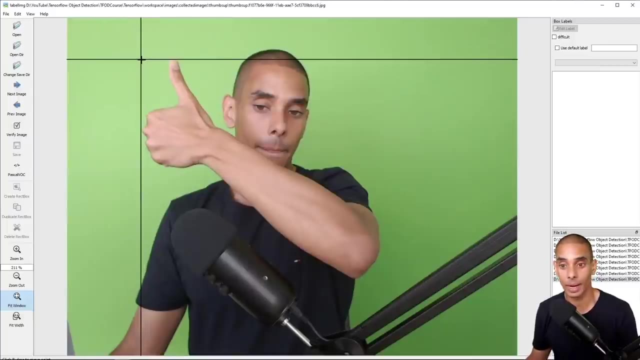 Thumbs up save And you can see- so I did that. thumbs up might perform a little bit better now, because we've now got images at a bunch of different angles. Let's tighten that one up and save it again. But keep in mind we've only got a green screen in the background at the moment. 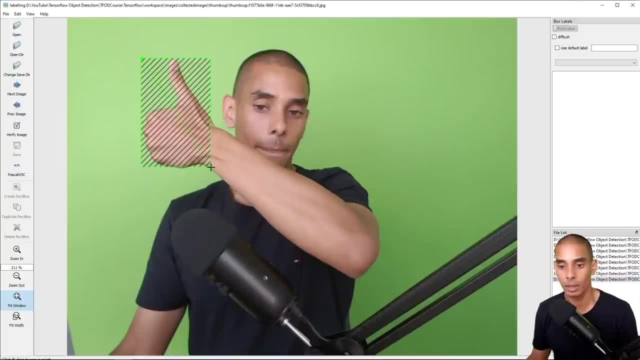 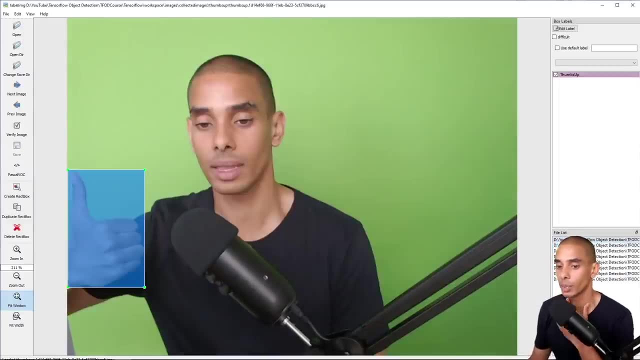 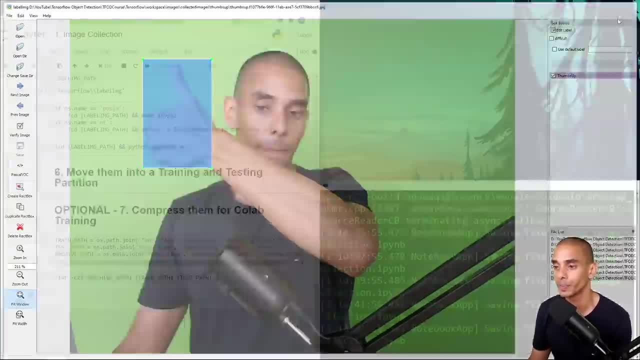 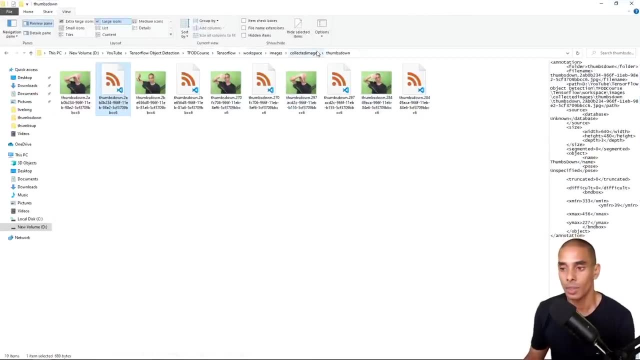 All right, cool. So that looks all good. So we've now labeled all of our images And if we check that, let's bring them back. So thumbs down now has all of our annotations. So if we're going to live long, we're good there. 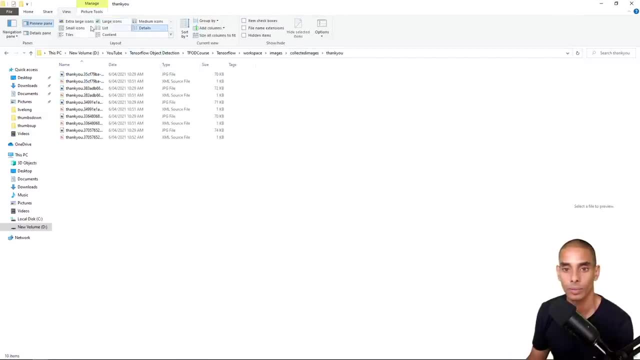 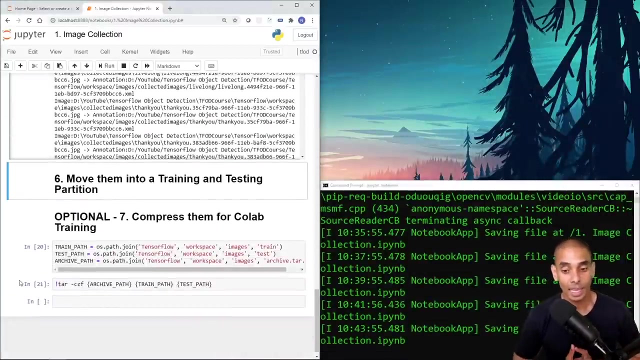 Thank you, We are good there. Thumbs down- we're good there. Thumbs up- we're good there as well. Okay, cool, So we've now gone and completed all of our labeling. Now the next thing which you really need to do is we're now going to split this up. 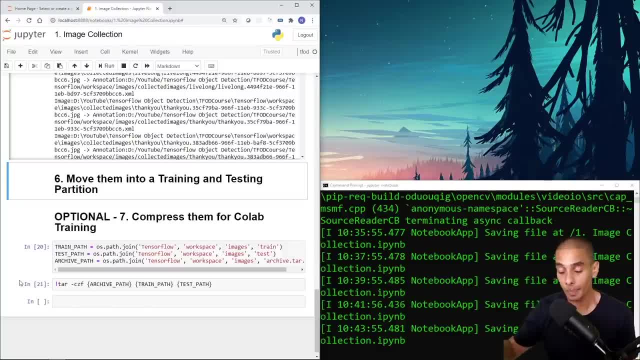 into a training and testing partition. So when we get to our training step, we're going to train our images or train our model on a portion of images, and then we're going to separate part of it out, or we're going to use the other part of our images to actually test how it is. 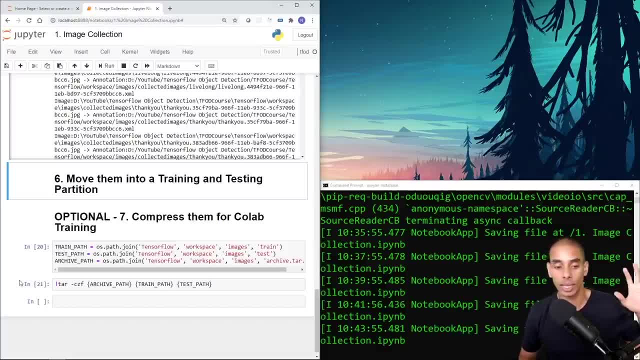 So the reason that we split this up is we want to train it on a segment of images that we're going to use for training, And then we want to test it on a set of images that it's never seen before. Look, the images might be similar. 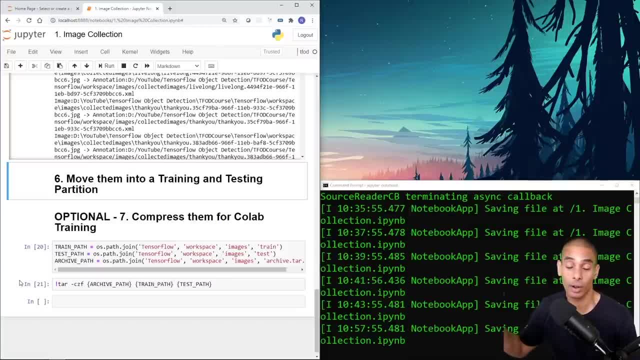 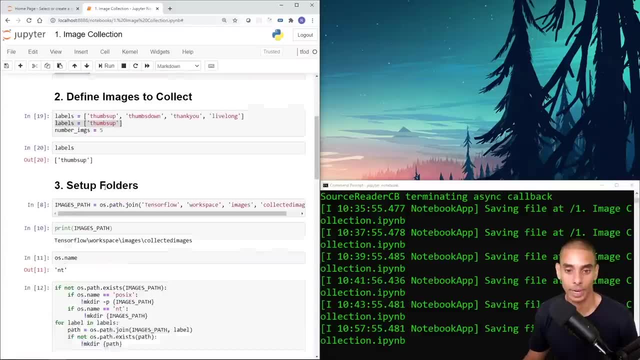 We want to give it a chance to try it out and see what performance looks like on images that it hasn't explicitly seen before. So to do that, so you can see, we've got step six here. So we've now done. let's quickly recap. 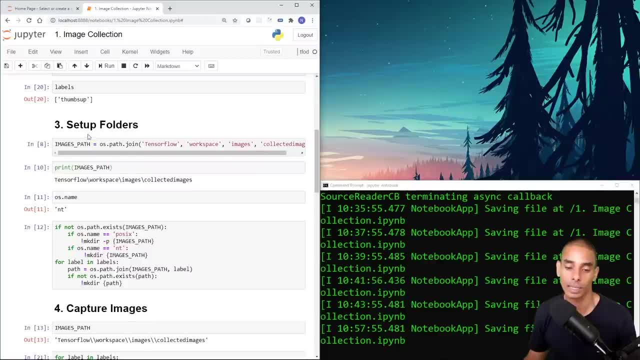 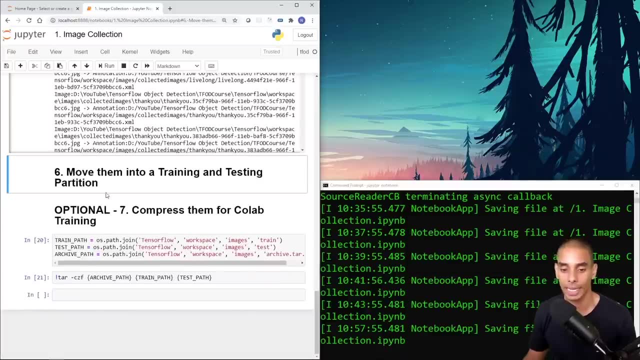 So we've imported our dependencies, We've defined our images To collect, we've set up our folders, We've captured our images and we've labeled. So we've done quite a fair bit. Now what we need to do is move them into a training and testing partition, which is step six. 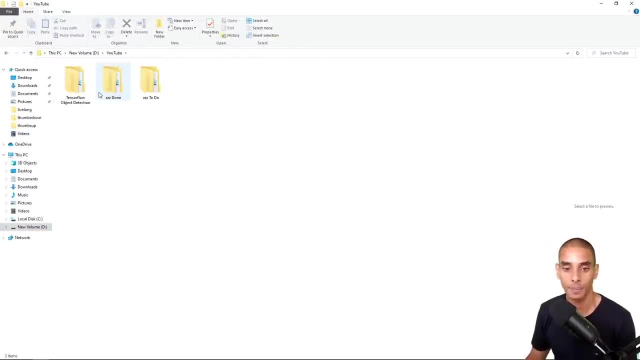 So what I'm going to do is I'm going to go back into that folder, So inside of our images folder, So I'm going to hold there and I'm going to create two new folders now. So I'm going to call one called train. 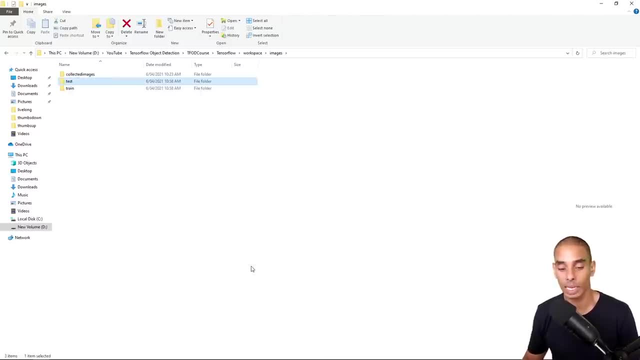 And I'm going to call one called test. Now, the names of these folders is really, really important because inside of the training script it's actually going to be looking for these training and testing folders, or the test and train folder explicitly. So you need to make sure that you create these folders and you need to make sure that you have images and the associated annotation in it. 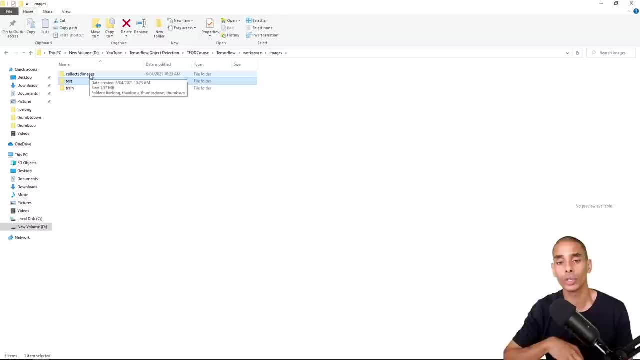 So what I'm going to do now is I'm going to take a random portion of our images from each class. So we're going to take some from live long, some from thank you, some from thumbs down, some from thumbs up, And we're going to put it into that training folder. 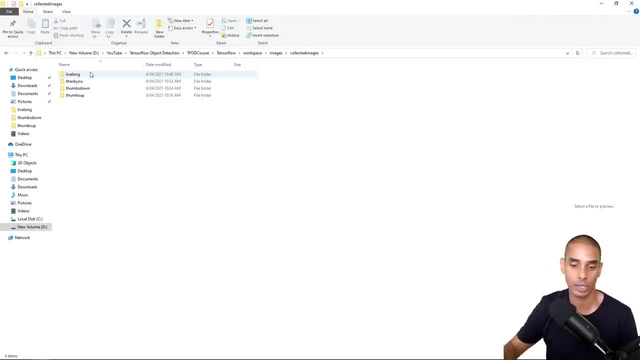 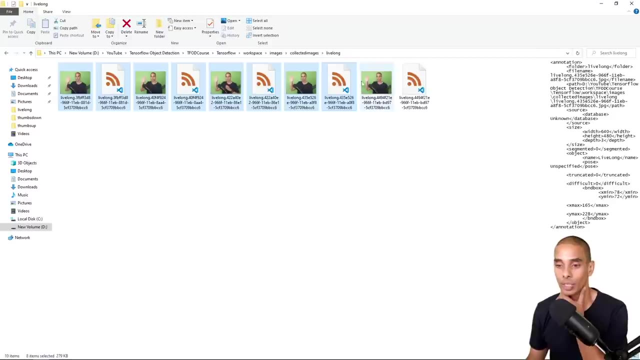 So these are the going to be the images that we use to train our object detection model. So if I step into live long, I'm going to get everything, including the annotation, So maybe we'll leave one image for testing. So what we're going to have effectively one, two, three, four images and one, two, three, four annotations. 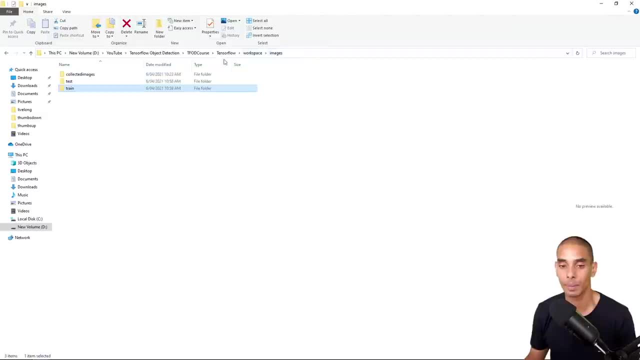 So I'm going to cut that, Paste it into the training folder and I'm going to do this for each class. So we're going to go into, thank you. So one, two, three, four, five, six, seven, eight. 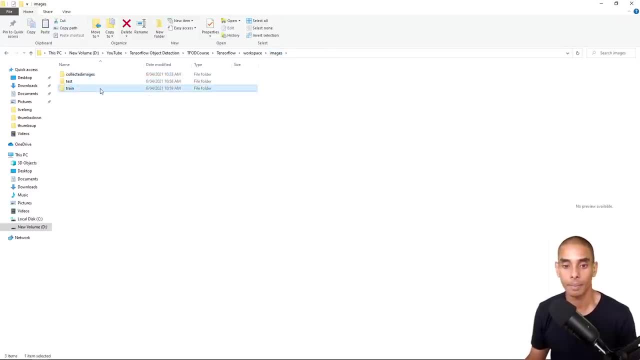 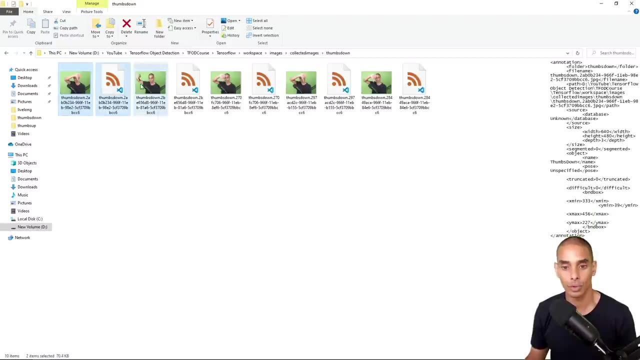 So again, four images, four annotations. Again, paste it into the training folder. Now we're going to do it for thumbs down. And again, one, two, three, four, five, six, seven, eight. Got to grab that one. 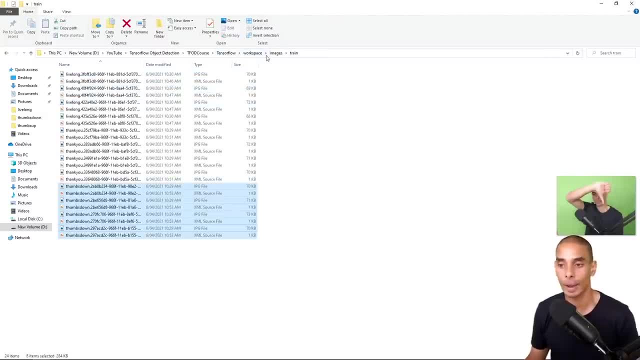 Going to go back in, And the reason why I'm being so explicit in making sure that we grab the annotation and the image is if you skip out and you don't have the annotation, or if you skip out and you don't have the image, it's going to screw up when you go to do the training step. 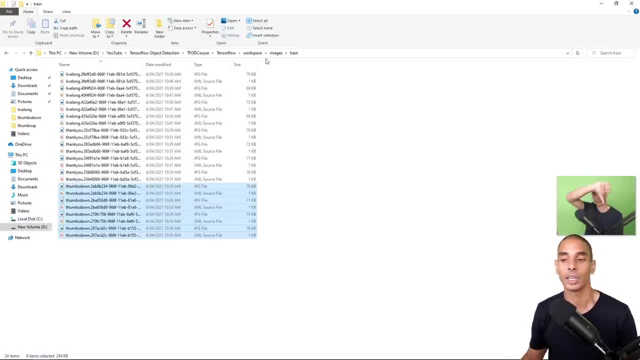 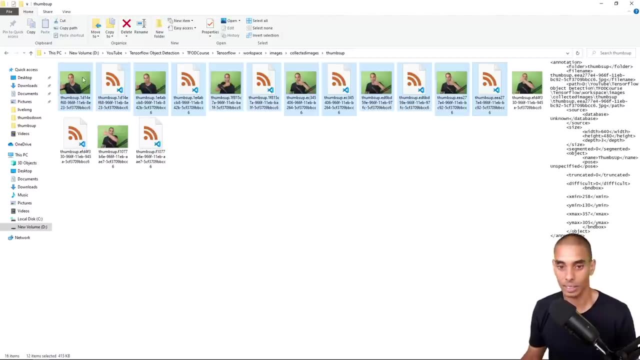 So you need to make sure that you grab both the image and both the annotation- Really really important, And we're going to do the last part. So I'm going to grab. let's leave two images for testing there. So I'm going to grab one, two, three, four, five, six, seven, eight, nine, 10,, 11,, 12.. 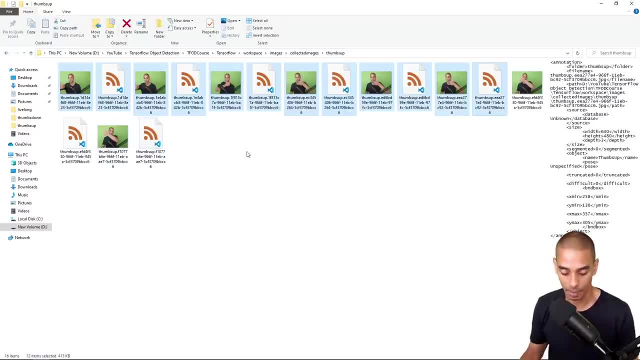 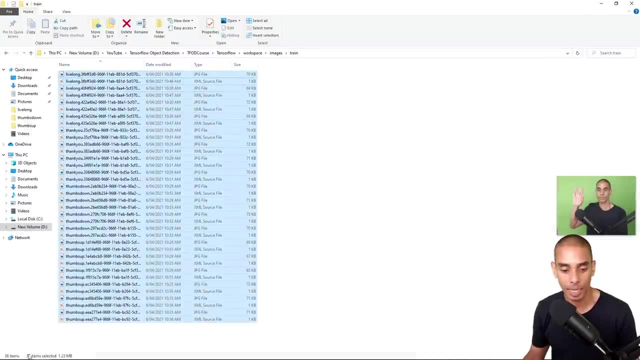 All right. So we'll leave two images and two annotations for thumbs up, because, remember, we add more images there, All right, And then we're going to paste those into our training folder. So now we should have an even number. So we've got 36, a little bit small down there, but we've got 36 images. 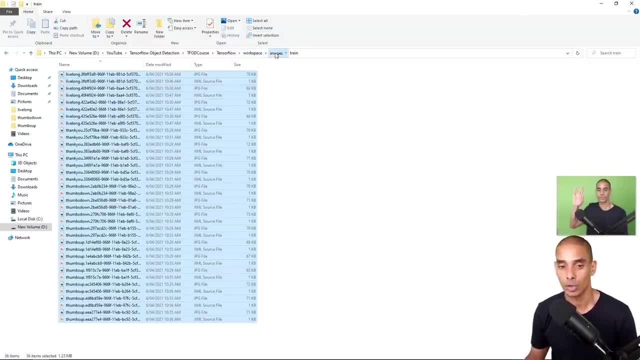 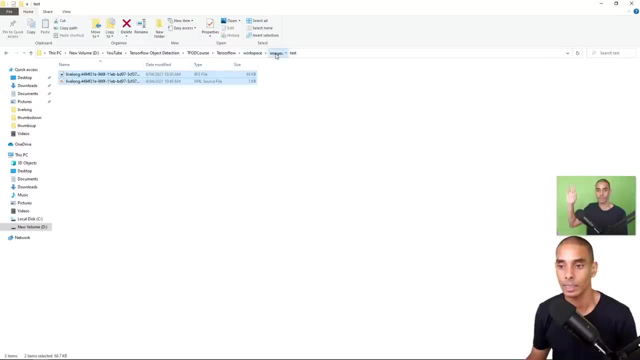 So we've got the images and the annotation, So we're good for our training. Now we need to do the same thing for our testing. So we're just going to grab the rest, Paste it into our test. Thank you, And again, you could automate this. 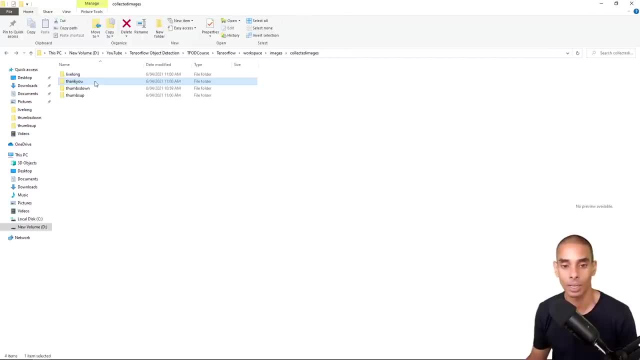 You could write a little bit of Python script to randomly select your folders. If you do get around to it, let me know. I'd love to see the code, Paste it into test, But I found that just doing it manually isn't too bad. 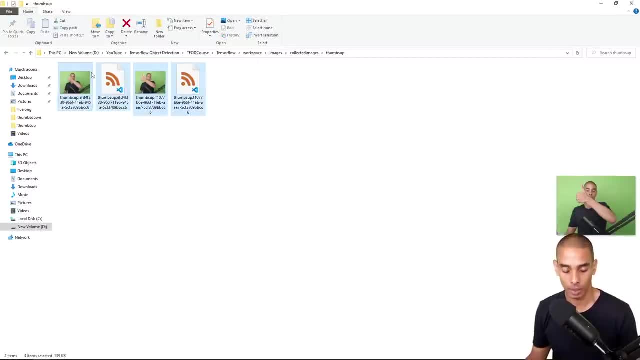 Particularly. if you only got a small segment of images, I'm going to grab out Thumbs down, thumbs up, then paste that into test, right? So ideally, what you should end up with is an even number of images both inside of your test folder and inside of your train folder. 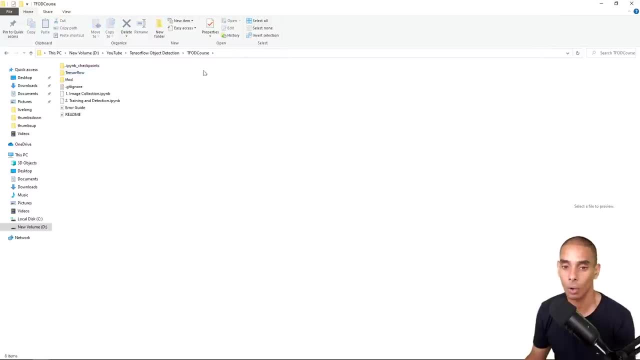 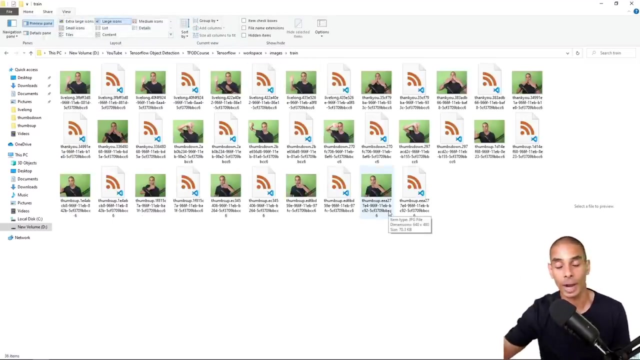 So if we take a look at our full file path, inside of our tfod course folder, we should have tensorflow workspace, images, test and test has images and annotations, and train and again train has images and annotations. So these images and annotations are going to be used to actually train our model. 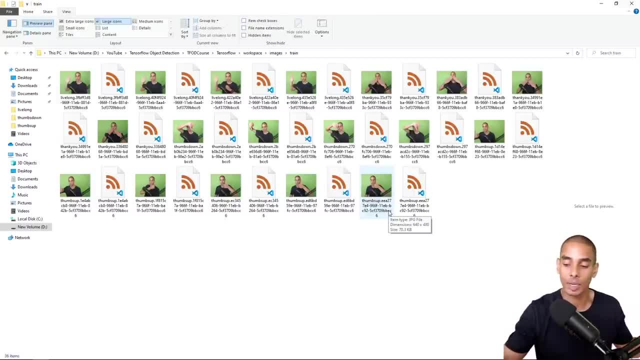 We're going to do this technique. I'll use the technique which converts these images and annotations to something called a tensorflow record, And again I've got scripts to help you do that. So we're going to convert those and then use that, those tensorflow records, to be able to actually train our model. 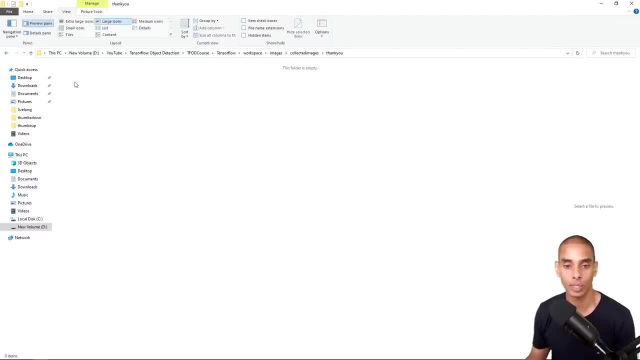 Now, if we go back into our images folder, we can also just delete these folders as well now, because we don't need these. There's nothing in them, So inside of collected images, we can actually just delete that now. So again, all of our images and annotations are inside of test and train. 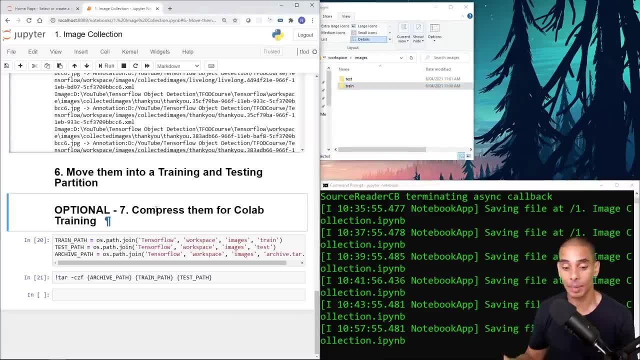 So we're good to go now. inside of that image collection notebook I've also got the code to compress these images to be able to push them up into Colab. But again, we're going to do that when we get to our Colab training. 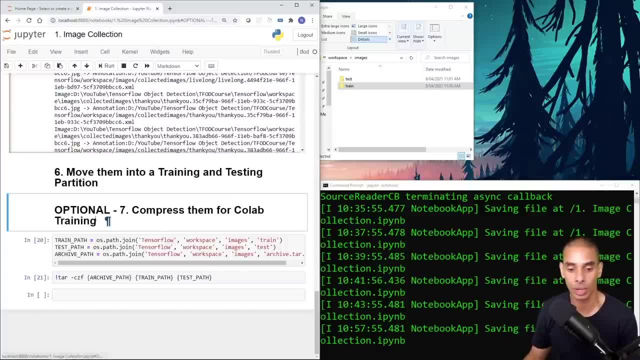 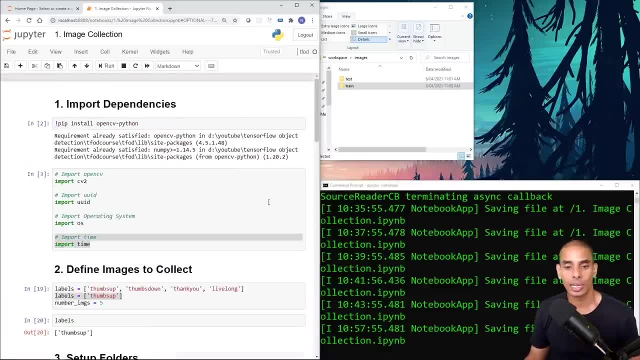 So, again, hold on to that. for now You don't need to run these last two cells, which is everything under step 7, which says optional: Cool, All right. So that's image collection and labeling done. So I've gone and collected our images, captured our images, labeled them using label image and we've now gone. 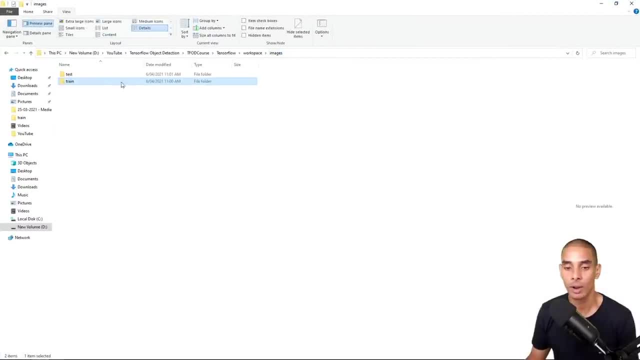 And split them up into our training and testing partition. So again, remember, last step was really, really important. You need to have a training and a testing folder because this is what our training script is going to be looking for. So we've also adhered to some of those best practices. 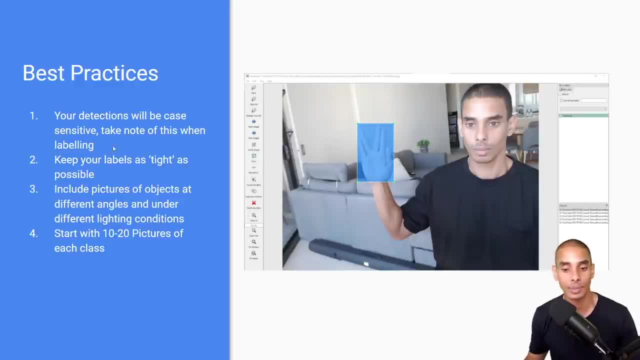 So we were case sensitive, We made sure we got our cases right, We kept our labels tight and right now we've only done five images of each class, except for thumbs up. So again, we might choose to add more later on. So we're good there. 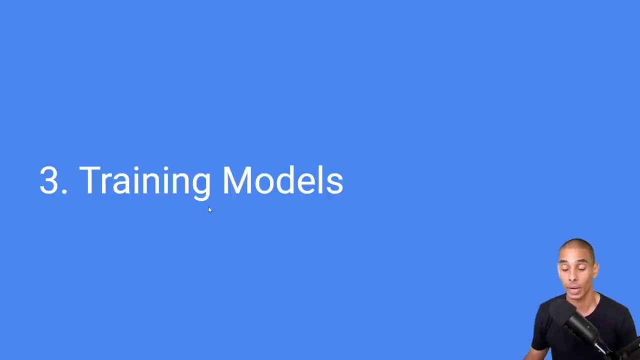 This brings us to step three: training our models. So in part three, we're actually going to start training our models. So we're specifically going to be using a model called a mobile net, which is a specific deep learning architecture, But you could use a bunch of different types of models, and we might actually do that in the performance shooting section as well. 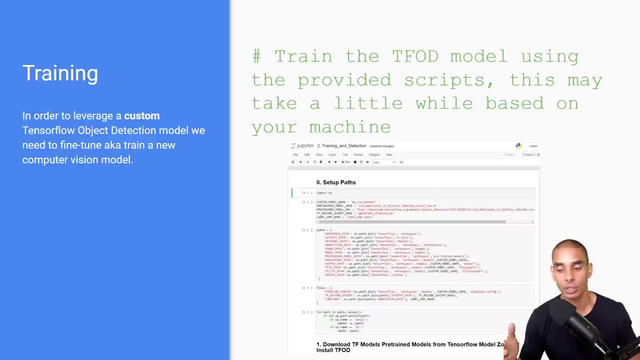 So when it comes to training a model using tensile object detection, So there's a bunch of steps that you need to go through and a bunch of dependencies that you're going to be needing now. namely, because we are using TensorFlow object detection, One of the core dependencies is going to be tensile flow. 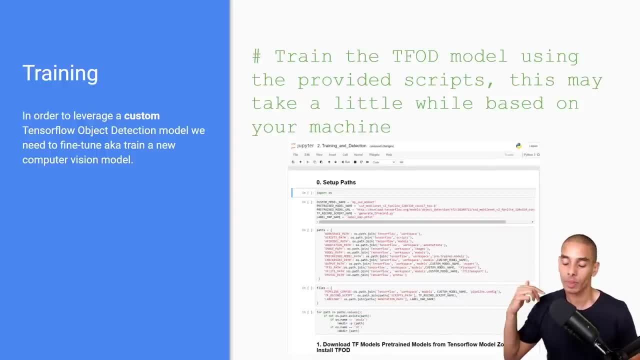 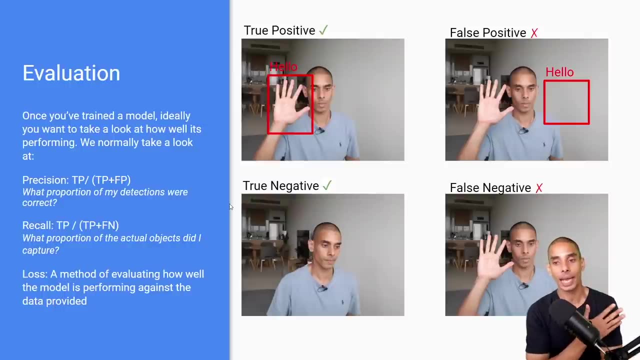 So we're actually going to go through, install all of our dependencies, set up our folder structures and actually start training this model Now. as part of this, we're also going to be evaluating our model Now. I might come back to this a little bit later, but I wanted to talk about how to evaluate your models. 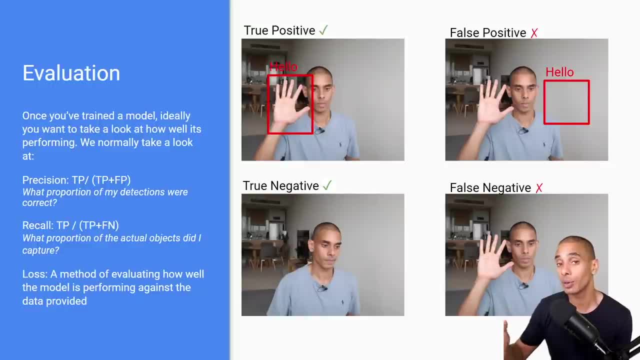 Now the nice thing about TensorFlow object detection is that you're able to calculate these evaluation metrics after you've actually gone and trained your model. Now, specifically, when you run your evaluation, you're going to get two key things. So you'll get precision, and normally you'll get a metric called MAP, which stands for mean average precision. 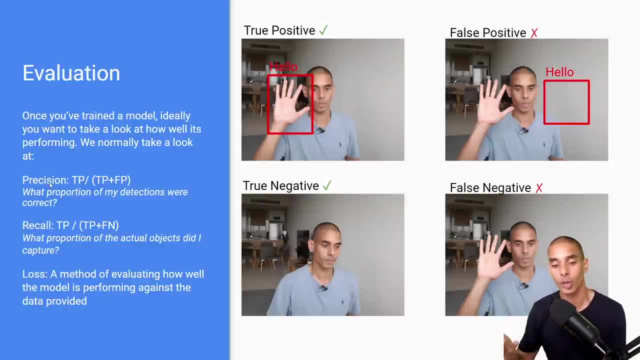 And this basically tries to calculate what proportion of your detections were correct. right? So what it's actually doing is it's calculating the true positive. No, So how it's actually calculated is it's the number of true positive detections divided by the true positives and false positives. 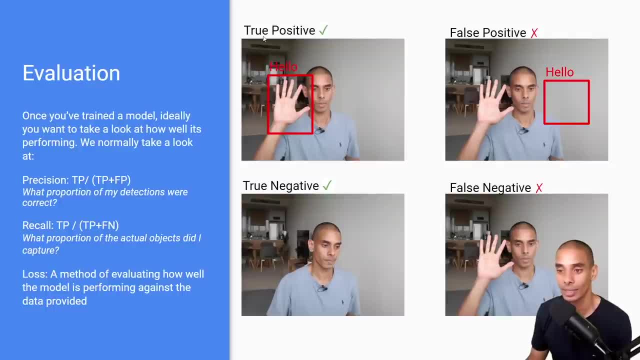 So effectively. it's the number of detections That it got right. So in this case, here you can see, I've got this little Matrix. So this is a true positive detection. So you can see, this is the sign for hello, right. 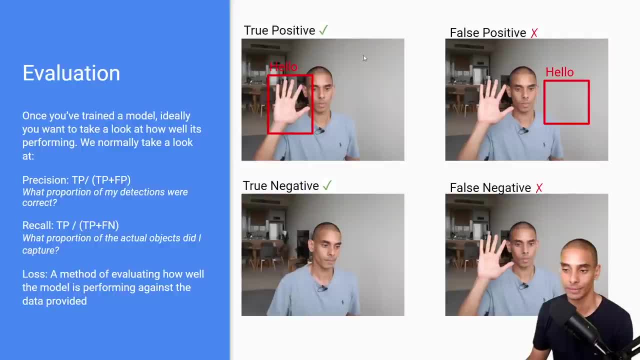 And it's accurately detected the sign Hello. So it's a true positive. Now, on the other case, you might have a false positive. So it's gone and detected a label here which says hello, but it doesn't. that's not actually correct, because it doesn't actually have that label there or it doesn't actually have that object there. 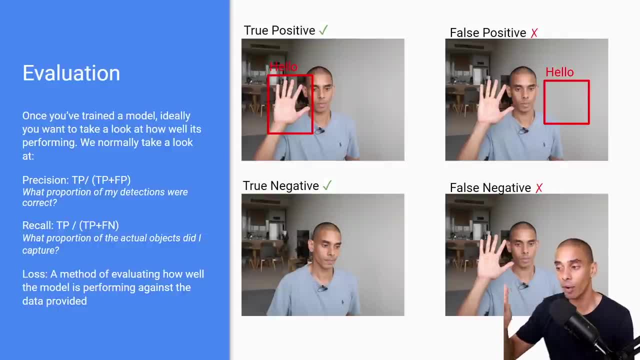 So even though it's gone and made a positive detection, it's a false positive Because It's not actually correct. You've also got a true negative, which in this case there's no object, So there's no hello in there. 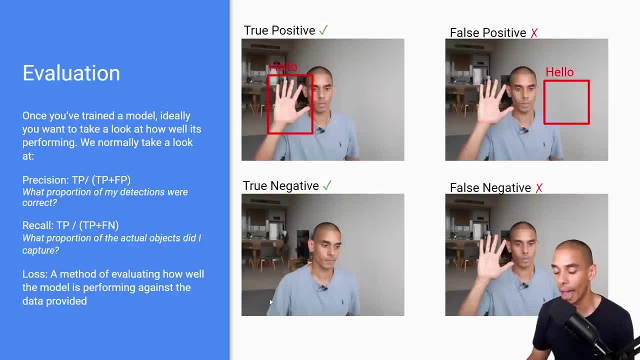 So say, for example, this is just a hello model, So there's no actual hello object in there. In that case it's actually a true negative. In this case we've got a false negative. So there is a hello object in there, but it hasn't detected that as hello. 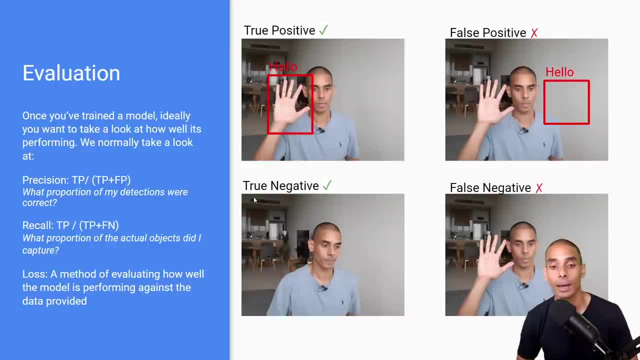 So it's falsely rejected it, right? So what you're actually going to get when you calculate your evaluation metrics are precision and recall, which are calculated off The Number of true positive, false positive, true negative and false negative detections. So in this case, your precision metric is going to be true positive, which are the number of detections that have actually detected the correct object, divided by the number of true positives and the false positive. 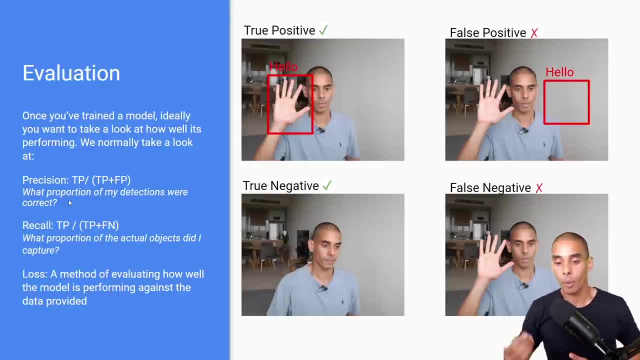 So effectively. what that's giving you in layman's terms is what proportion of my detections were actually correct. right, So this is correct. This is bad. So ideally, you want this precision number to be as high as possible. A higher precision number is a better precision number. 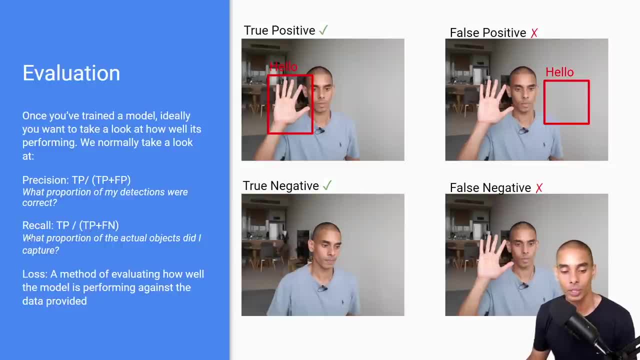 Likewise, A higher recall number is also a better number. So your recall is calculated as the number of true positives divided by the true positives and the false negatives. right, So this is basically capturing. what proportion of my actual objects did I capture? So in this case, you can see that we might have captured this, but we didn't capture this. 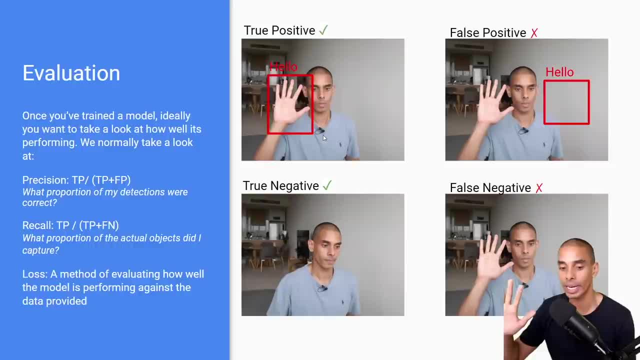 So really is trying to measure hate for the objects that were in the screen. What proportion of those did we actually get? So when we calculate our evaluation metrics later on, you'll actually be able to see these. You'll also see loss, talked about a little bit. 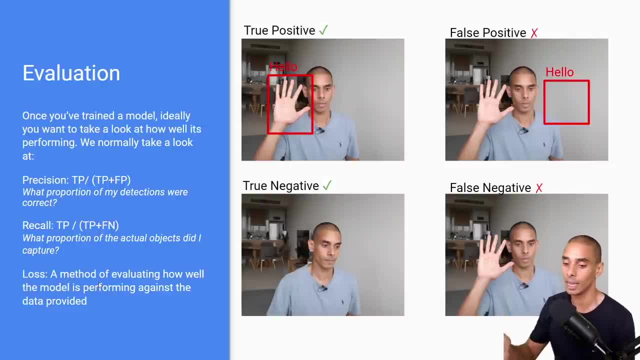 So it's a method of evaluating how well the model is performing against the data provided. Ideally, you want loss to be as low as possible, recall to be as high as possible and precision to be as high as possible, But again, we'll talk about this when we get to that step. 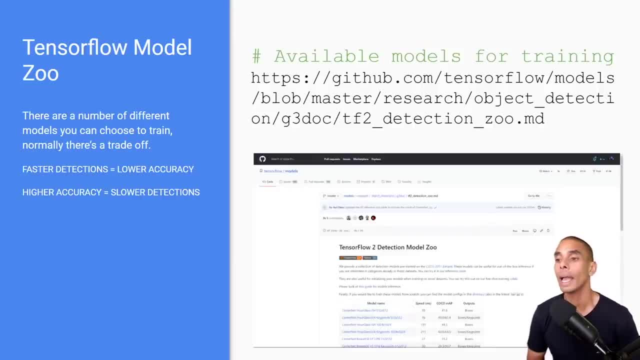 All right. So TensorFlow, model zoo, So there's a whole heap of different type of model that you can actually go on ahead and train. right Now, what you normally have to do is balance a trade-off, So you'll balance faster detection. 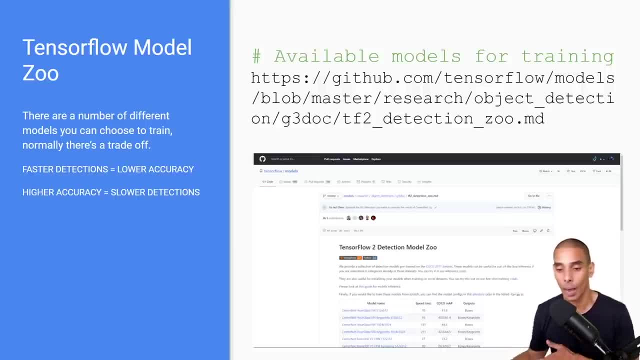 So ideally, being able to detect stuff Really really quickly, versus lower accuracy. So the ones that tend to be faster tend to be less accurate, Not all the time, but most of the time. the ones that are highly accurate tend to be slower, right. 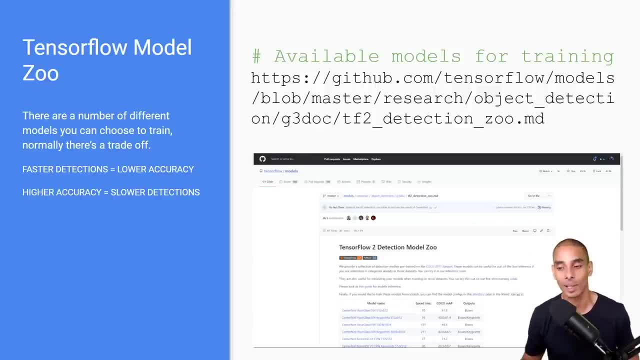 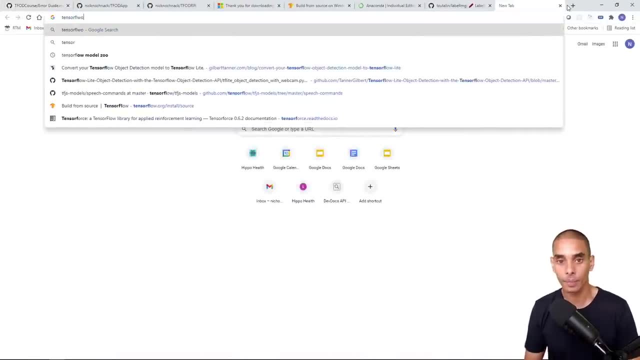 So if you have more sophisticated models, bigger architectures, it's going to take slower to actually make that detection. So, if I actually show you right, So if you actually go to Google and type in TensorFlow model zoo and make sure you type in TF2, which stands for TensorFlow 2.. 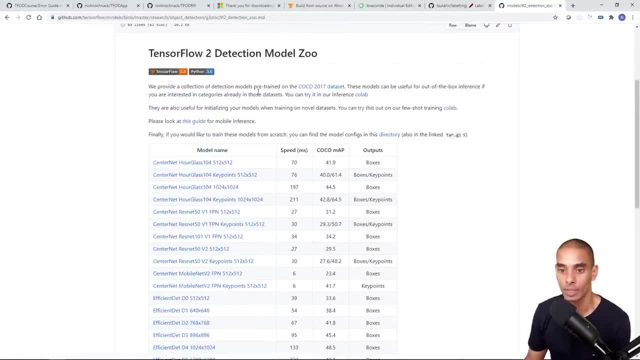 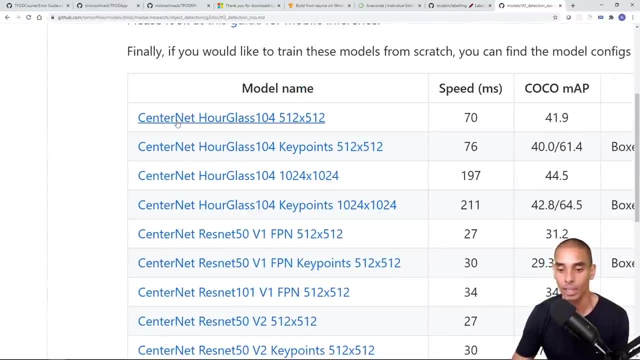 There's a heap of them, Different types of models, right. So these models are just different model names and different model architectures. So if I zoom in here, you'll see that we've got a model called center net. We've got another model called efficient det. 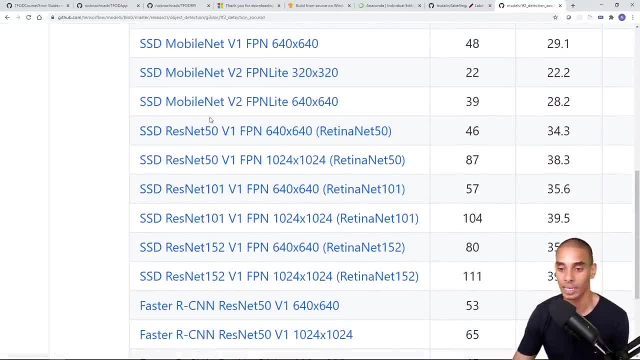 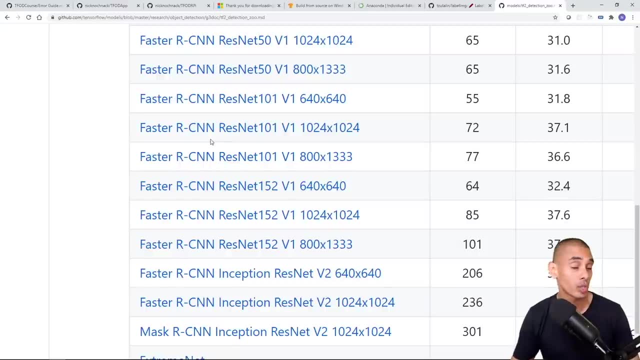 We've got an SSC mobile net, which stands for single-shot detector mobile net, single-shot detector resonant. So each of these just represent different neural network architectures which are used for object detection. Now you don't need to go into great amounts of detail as to how these are. 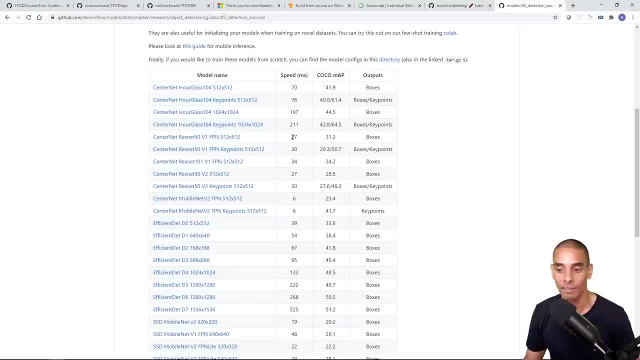 Actually built up. What you do need to know as a practitioner, However, is that using different models is going to result in different levels of accuracy as well as different levels of speed. So say, for example, I wanted to use so let's actually take a look at the model that we're going to be using. 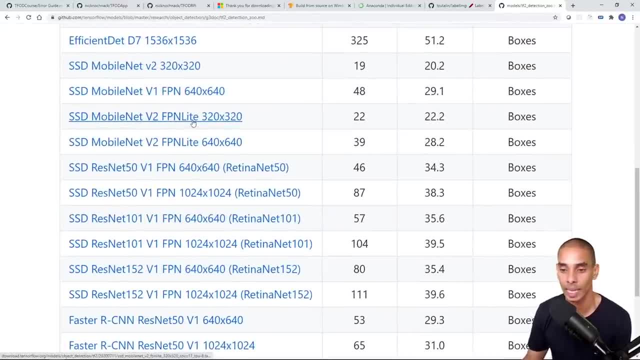 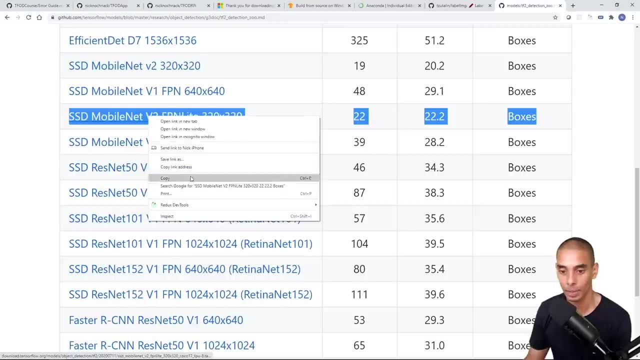 So we're actually using this one here. So SSD mobile net v2.. FPM light, 320 by 320.. So this is the model that we're actually going to be using and if you actually take a look at that link there, So if I copy this link address: 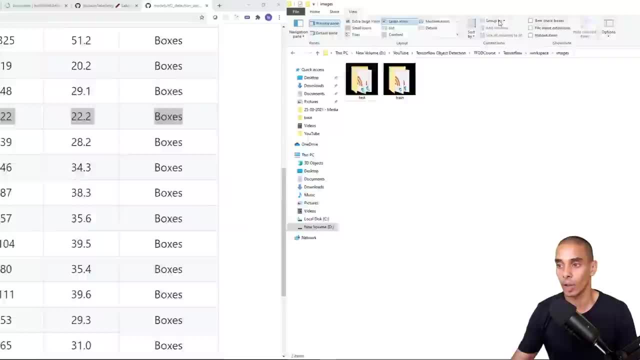 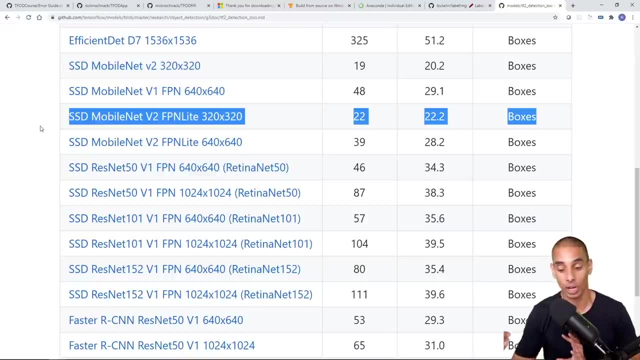 Let's actually open up the notebook. Actually, we'll come back to that. So the link for this is actually going to be the link that we're actually using in our notebook, and I'll show you that in a sec. Now this model has a. let's take a look here. 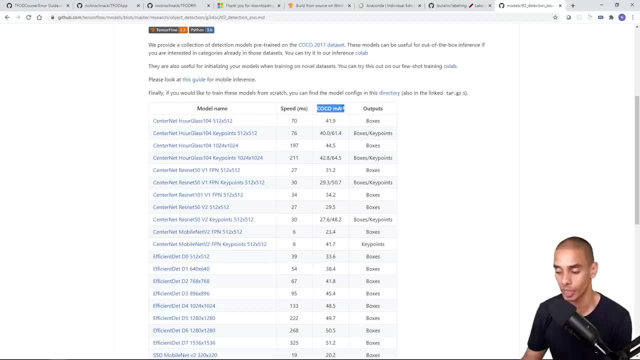 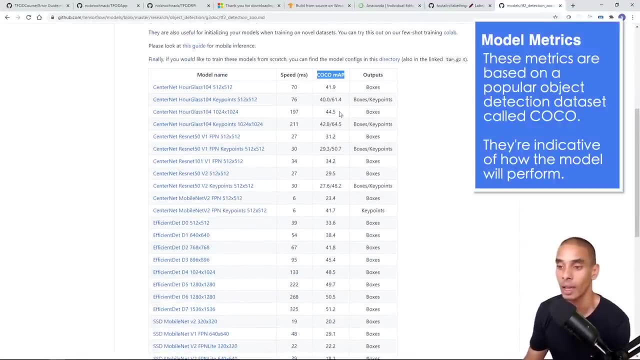 So we've got two components. So we've got speed and we've got our mean average precision. Remember, we talked about precision here. in this case We've got the average precision which is represented over here on the cocoa data set. So this is just a standard data set. 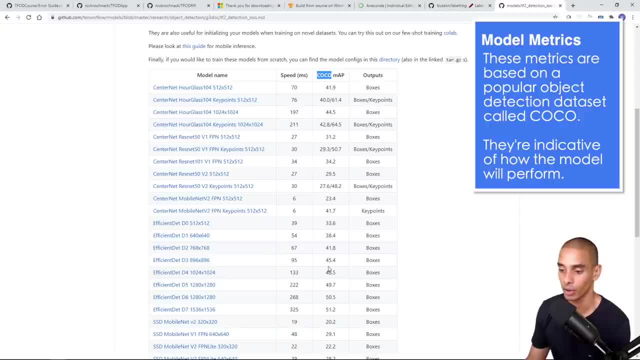 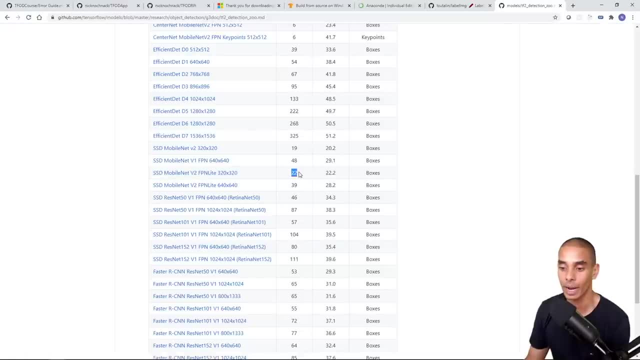 So just think of these two columns as how fast the model is and how accurate the model is likely to be. So in this case we've got a bit of a balanced model right. So our SSD mobile net is going to run each frame in 22 milliseconds. 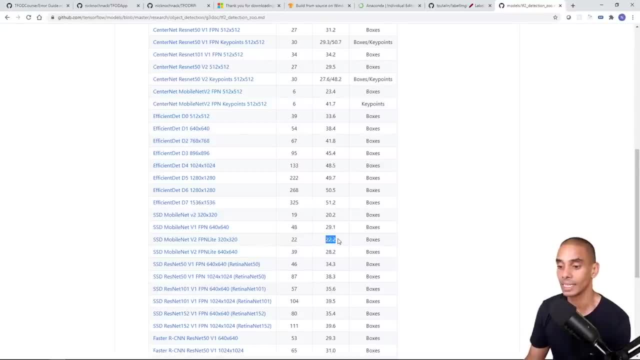 So ideally, you want this number to be the lower the better, and it's going to have a mean average precision of 22.2.. So again, it's reasonably balanced. now Remember when I said so you're going to have a bit of a trade-off here. 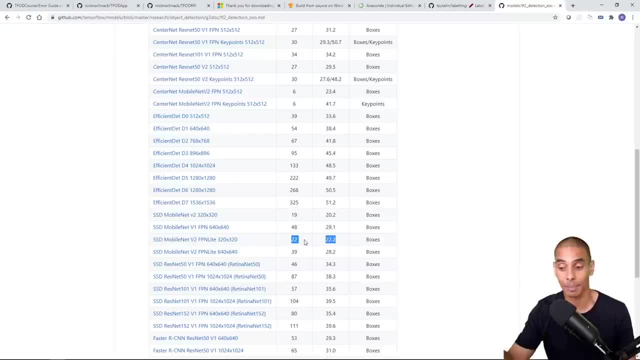 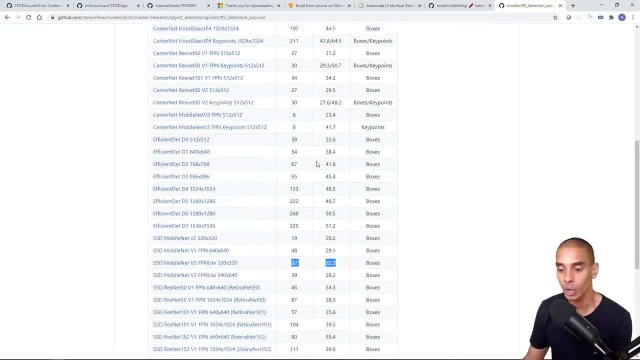 So in this case- And so Certain architectures can be fast and can be highly accurate as well- So just keep that in mind as well, So you might get a model that's really really quick but also really really accurate. So we could use this one here. 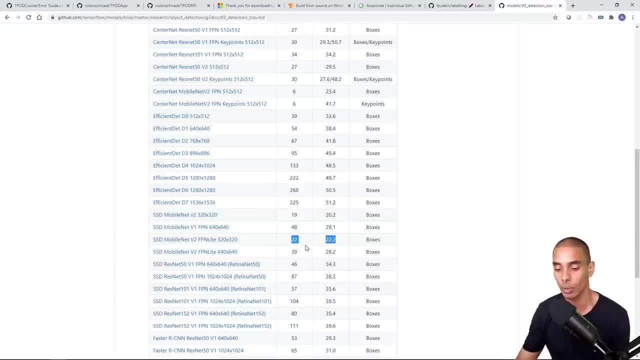 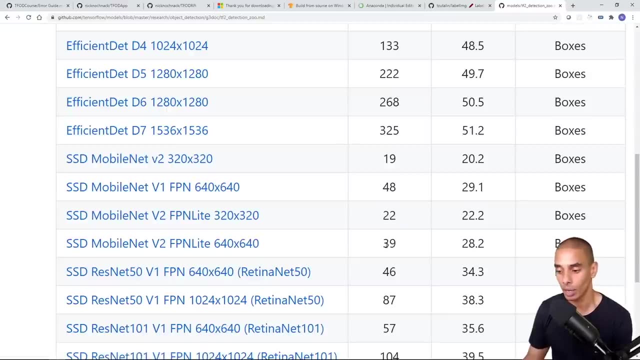 But say, for example, we wanted to get a model which is more accurate later on. Well, we might choose to go to this one. So SSD mobile net v2 FPM light, 640 by 640.. So it is going to be slower. 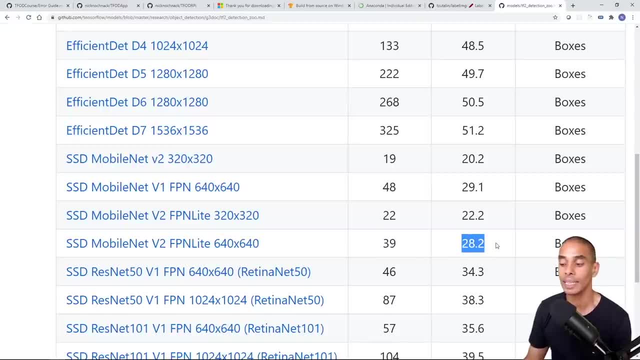 So it's going to take 39 milliseconds per frame. You can see here that our mean average precision is 28.2.. So again there's a trade-off, So you might choose to use a. so I guess you can sort of make a decision here. 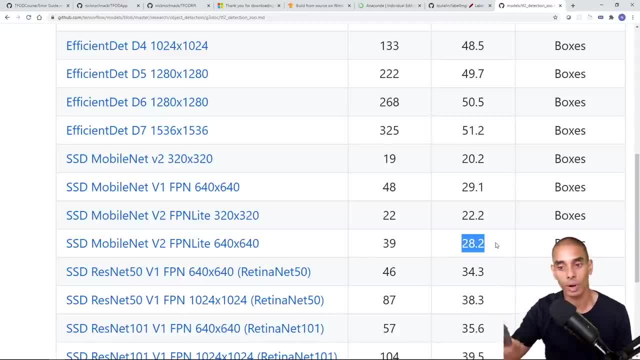 So if you need a model that's going to be deployed on a phone or on a raspberry pie, you ideally want to optimize for speed right, Because in a raspberry pie isn't going without any acceleration, isn't going to be that perform or isn't going to be able to perform that fast anyway. 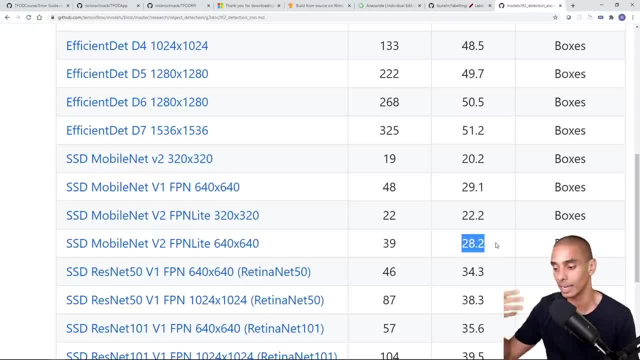 So you want to choose the model which is already really, really lightweight and it's going to be able to run. So in this case, this is why I tend to use this model a lot, unless I have a specific use case where I need a really, really accurate model. 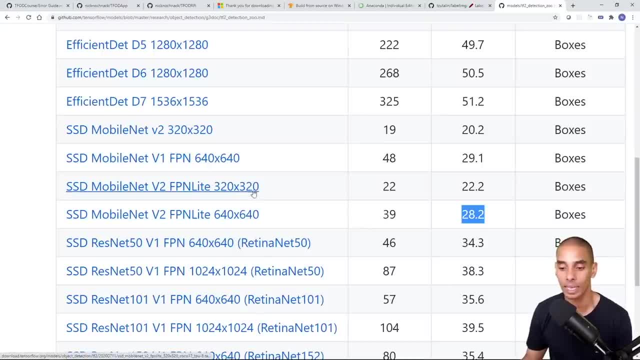 Now again, a core difference between this model and this model is that this model is actually going to compress our image from 640 by 480, which we had from our webcam- to 320 by 320 when we actually pass it through. You don't actually need to do anything as part of this. 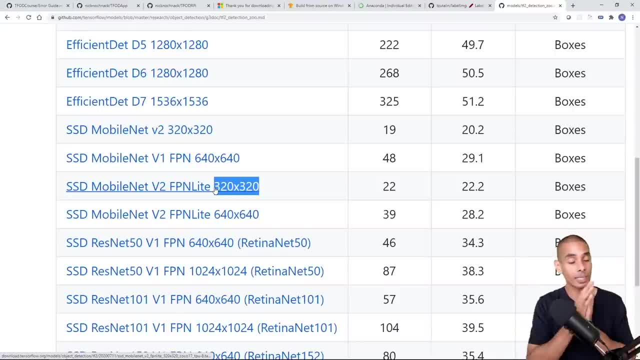 It's actually going to use a technique called pre-processing to compress that down to 320 by 320 and then in post-processing It's going to take the detections that it found and convert it back to your original resolution. So it'll actually do that for you. 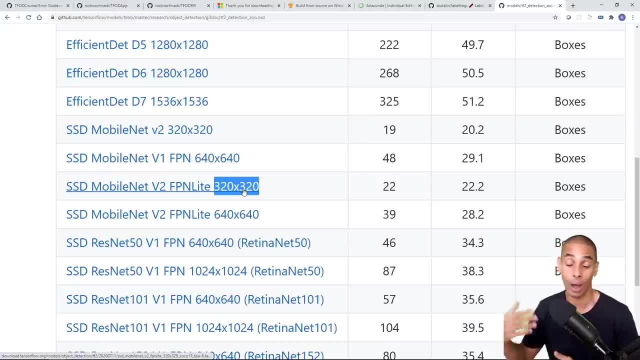 And this is one of the advantages of the tens-flow object detection model, or API. You don't have to do that pre-processing and post-processing, which can be a pain sometimes. Another cool thing about it is it does a technique, or uses a bunch of techniques, called image. 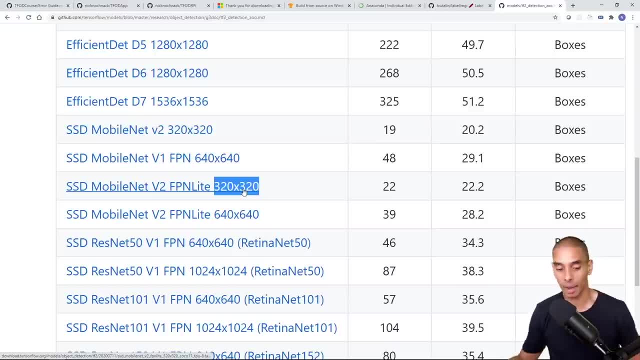 augmentation. So it might darken your image, it might shift it, it might flip it and it will do the same for the detection. So it does all of that for you. Certain models will have different levels of data augmentation or image augmentation, But just keep in mind the reason that you do those is to ideally get a better performing model. 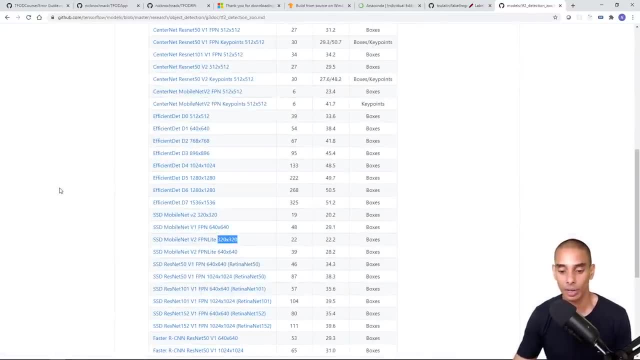 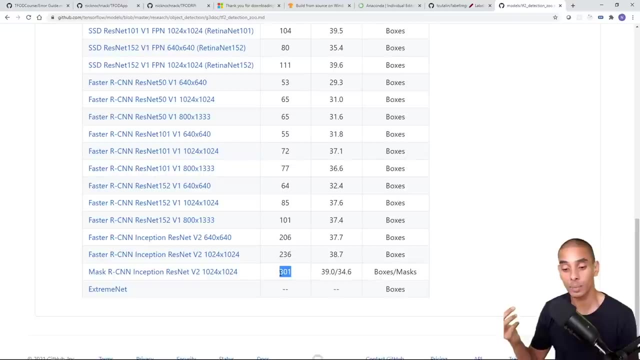 So ideally a more accurate model. Now again, you can use a bunch of different types of models. There's one really really slow one down here which again runs in 301 milliseconds, But the reason that this particular model takes a lot longer is because this actually gives you a bunch of 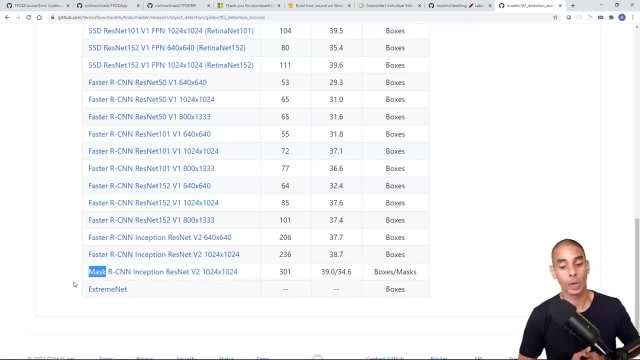 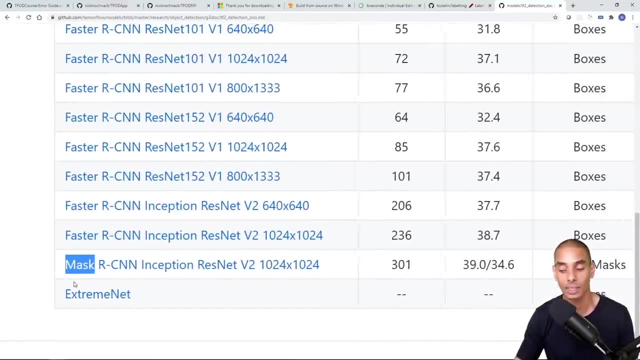 additional stuff as well. So this actually uses a mask, which, in this case, this, this course- covers object detection. The mask model which you can see down here actually does something called image segmentation as well. So rather than just detecting a box around my face, 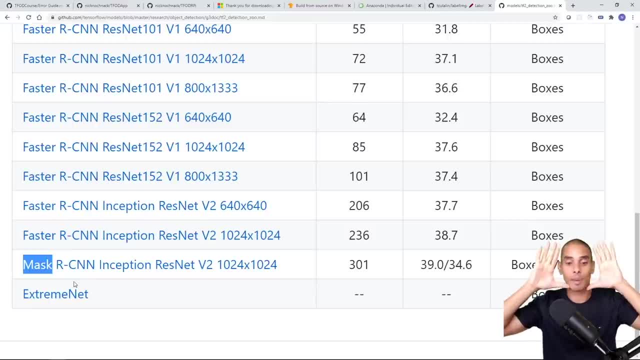 It can actually trace Face around my face and detect the specific shape of my face, Not just a box. Now again, because it is a lot more sophisticated, It's going to take a lot longer to run, So in this case, 301 milliseconds. 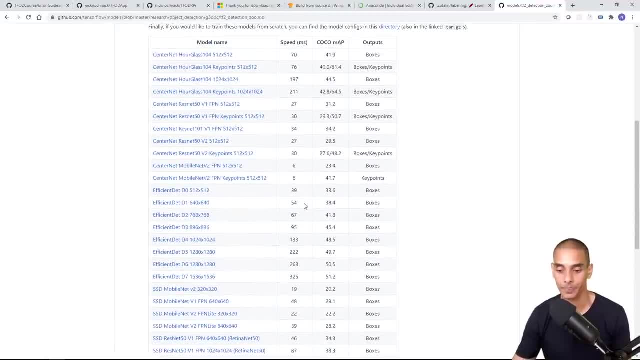 So again, you got a bit of a trade-off here as to which model you choose to use. Now we're going to be using this one over here. So SSD mobile net V2, FPM light 320 by 320.. 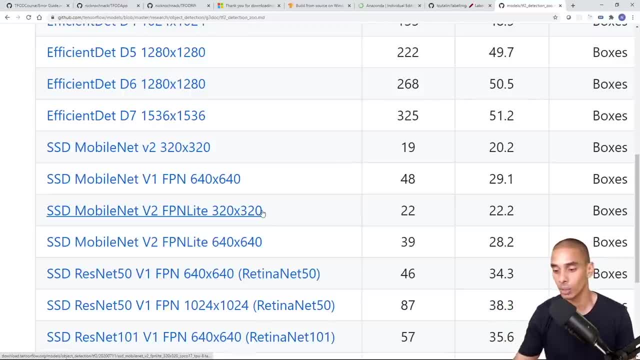 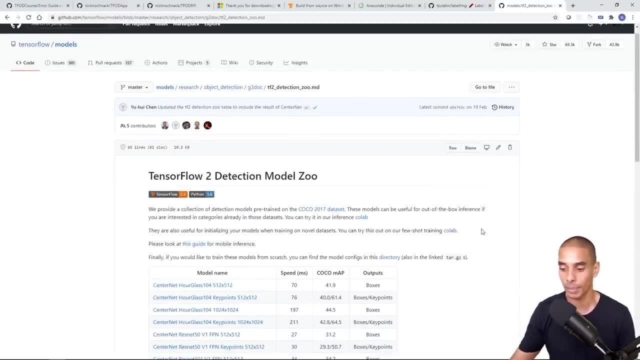 But again, in performance tuning we might choose to use a different model and see what that looks like. So that is TensorFlow Model Zoo. So whenever somebody asks you about TensorFlow Model Zoo, This is normally what they're talking about. Okay, so that is that. 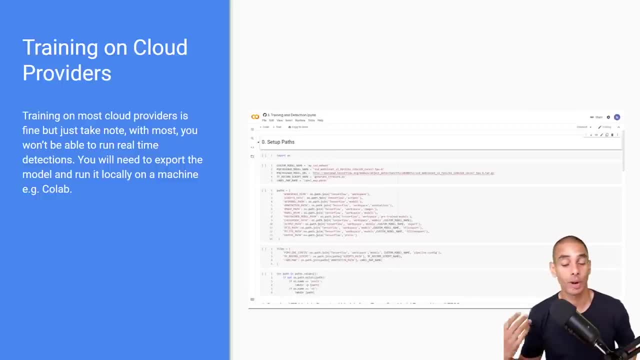 Now, sometimes you might not want to train locally on your machine. You rather use a cloud instance. to say, for example: you're not at home, You can't access your desktop. You might want to train something on Colab? Well, you can do that. 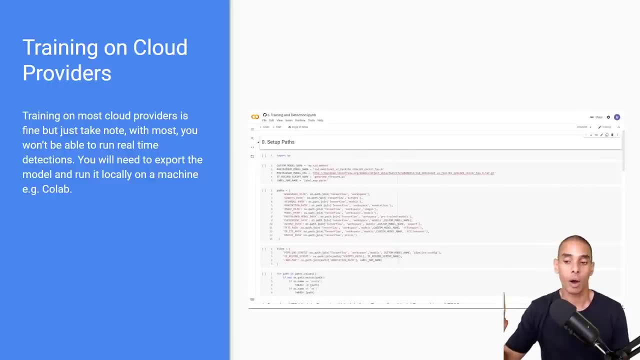 But a key thing to note is that when you train on a cloud instance, sometimes it can be difficult to connect to different devices. To say, for example, you wanted to connect to your microscope or connect to your webcam. Sometimes that can be a little bit tricky. 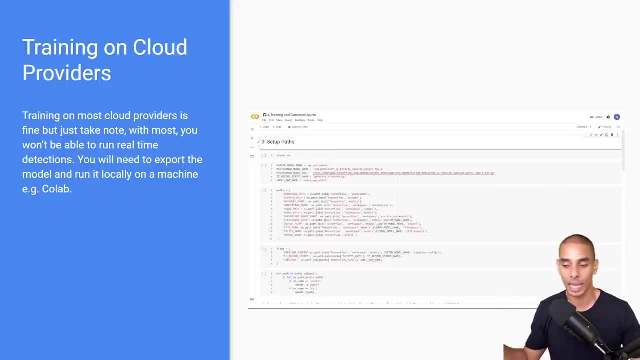 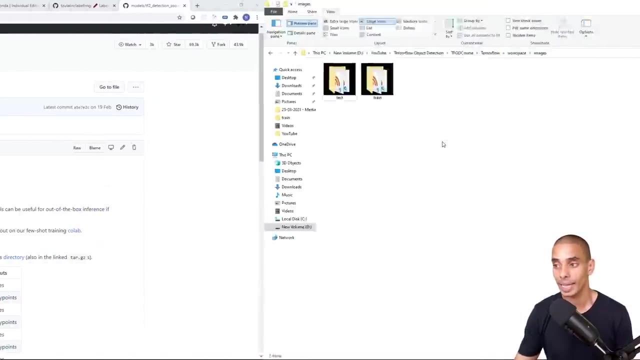 So that's just one thing to keep in mind, But again we'll cover that a little bit later on, when we get to that cloud section. So on that note, it's time to kick off our training. So again we're going to jump back into our Jupyter notebook, which we had over here. 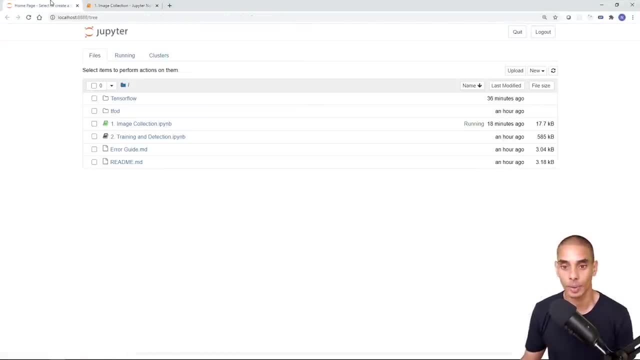 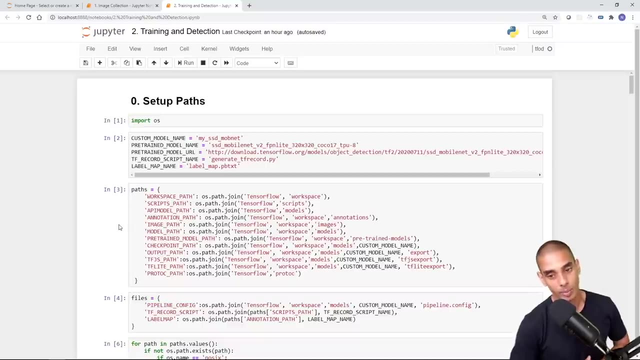 And before we were operating inside of our image collection notebook, But this time we are now going to open up our training and detection notebook. So there's a bunch of stuff that we're going to be going through this, but we're going to go step by step. 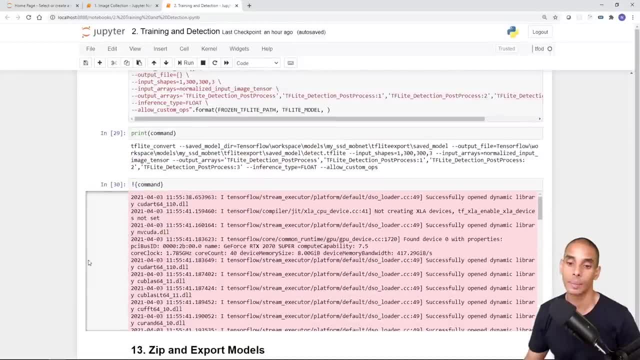 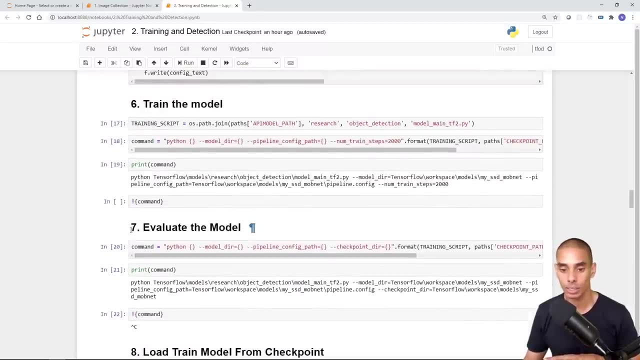 So all up, There are 13 steps altogether in this notebook, but we are going to go for our training section At least. we are going to go up to step seven. So evaluate our model, So we're going to effectively go through all of these steps. 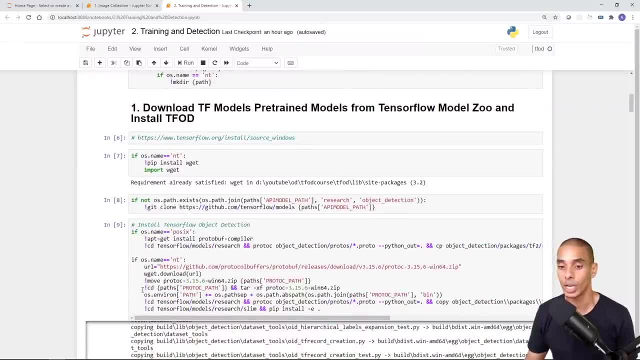 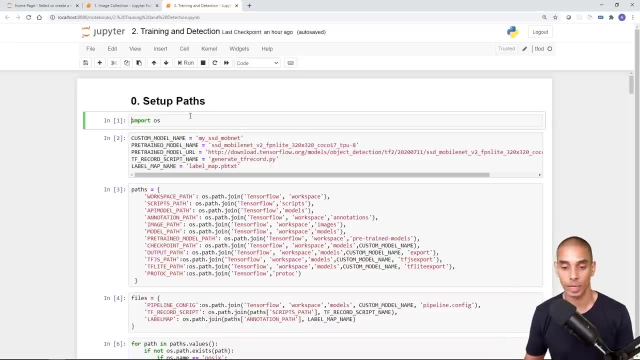 So by the end of this we should have a trained object detection model that we can then begin to use in our detection section. So again, we're just going to step into our first cell and we're going to run it. So in this case we're importing operating system as well. 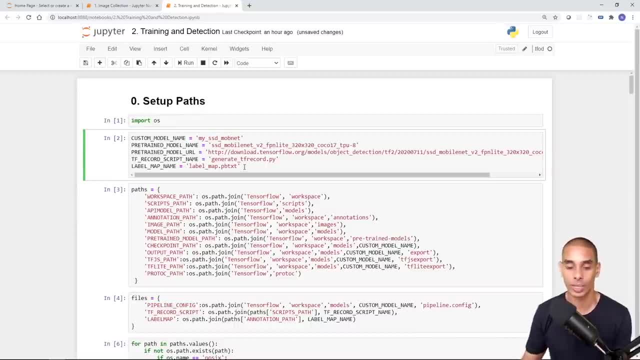 And then we're actually going to set up our pre-trained model Variables. So in this case we're defining what we want our custom model folder to be. So again, when we go to our performance tuning model, we might change this. 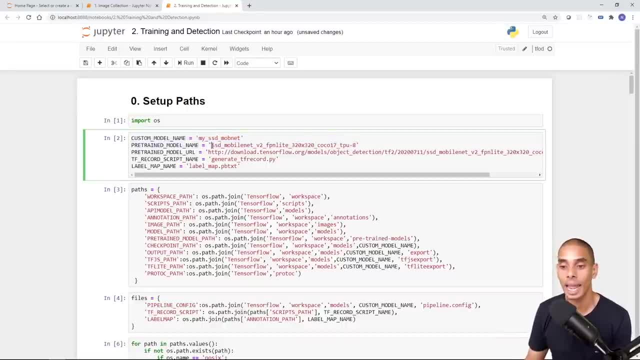 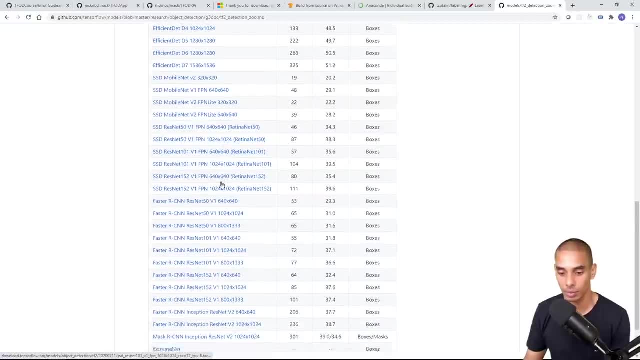 We're setting up the name of our pre-trained model, So this is going to be the name of the file that we download from our TensorFlow model zoo, which is over here. So when we actually download this, where is it? Let me find it again. 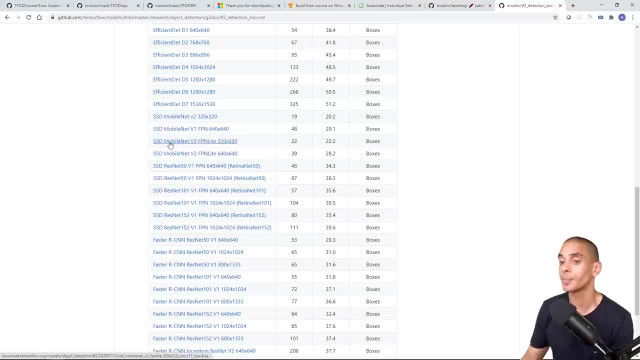 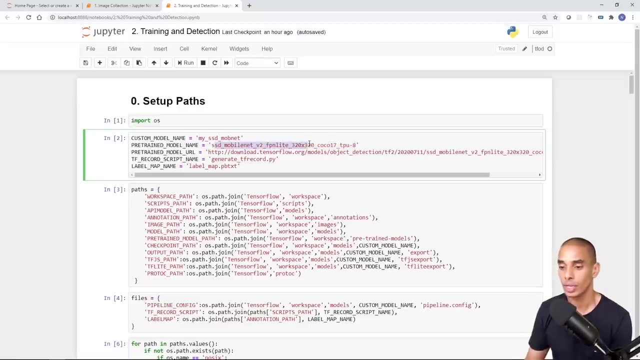 So this particular file here? If so, when we actually download it from here, what you'll actually see is the file that we get back is called SSD underscore mobile net underscore V2.. PM light 320 by 320, Coco, 17 TPU, dash 8.. 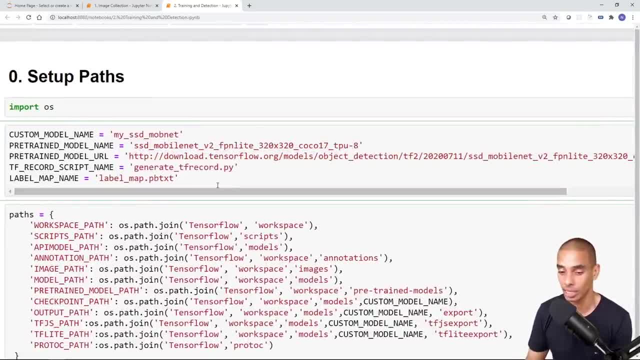 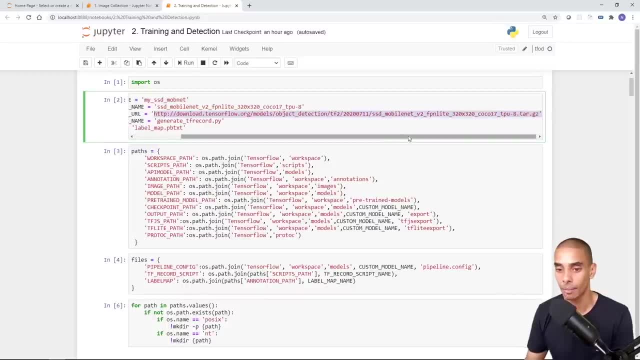 So again, this is something that I've just sort of pre-configured. So, again, if you wanted to customize this, you could as well. And then what I've also got in here is the pre-trained model URL. So I was saying before that we've got our model URL. 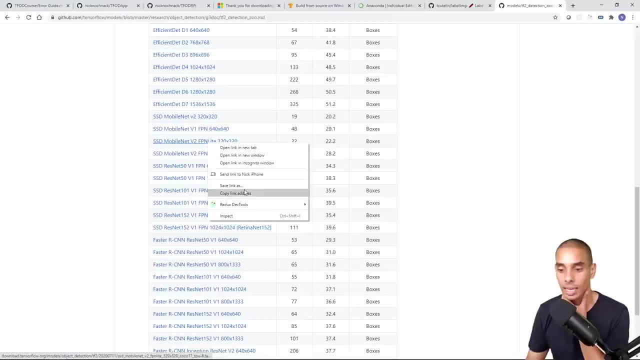 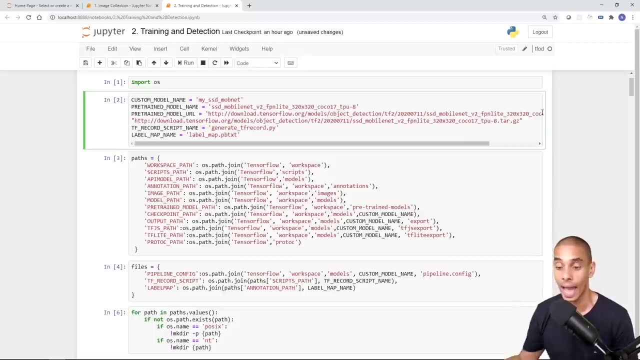 Now, where I got this from is if I right click on this and copy this link address, what you'll actually see. So I'm going into a lot more detail in this than I normally do And I sort of wanted to show you how I build these up. 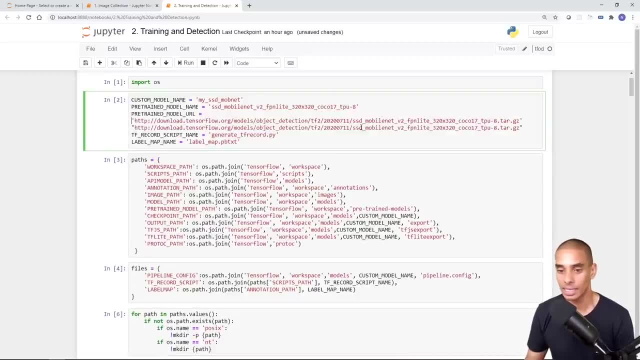 So this link that we've got Here is the same right, So you can see that that's the exact same link. So what we're effectively doing is we're going to be downloading that model from the TensorFlow model zoom and using it in here. 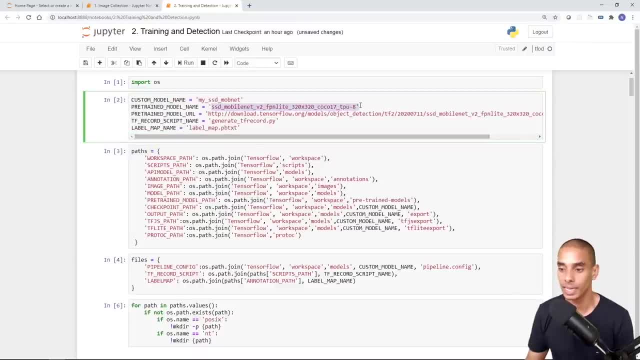 Right, So we've got the name of the file. So if we wanted to replace this, we just need to make sure that we get the name of the new file right. So in this case, we can see that it's going to be SSD underscore mobile net underscore V2.. 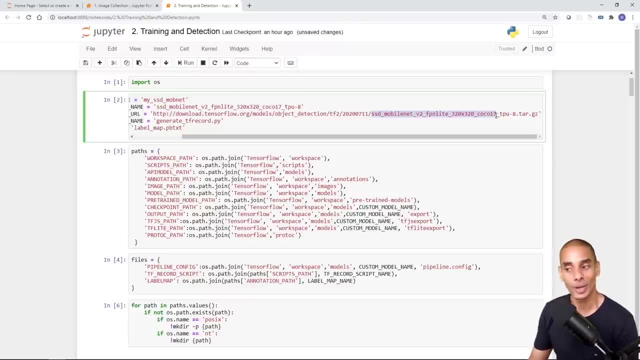 FPM light 320 by 320.. Underscore: Coco 17. underscore: TPU: dash: 8 dot tar, dot GZ. So again, if we got a different one, We could change this pre-trained model name, or we'd need to change this pre-trained model name and this pre-trained model URL. 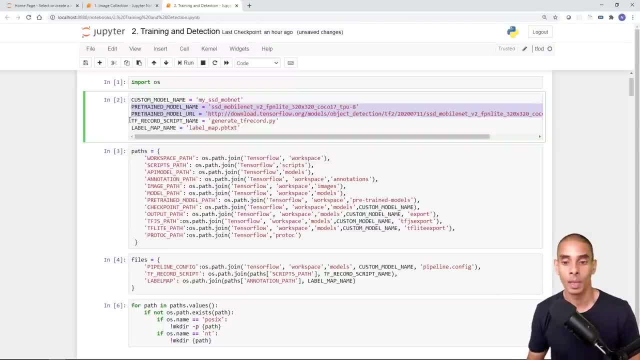 But you don't need to stress about this, for now You can just leave it. It's going to work. And then we're setting up a few different variables. So we're setting up at generate TF record script, which will come to later, in our label map name, which again will come to later. 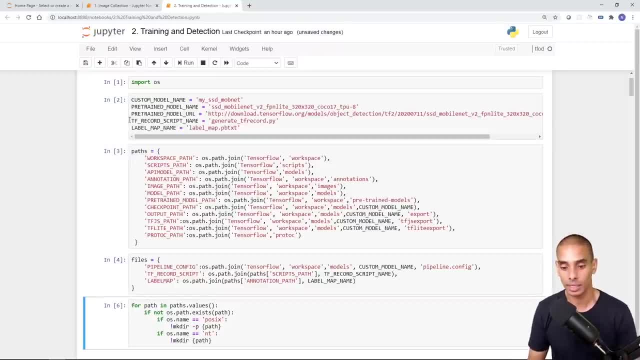 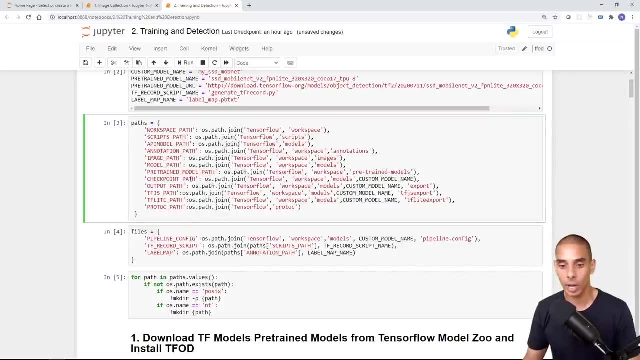 So I'm actually going to run through this cell, this cell, this cell and this cell, And what you'll actually notice now is that we've actually got a couple of things. So this over here is going to create Our different paths. 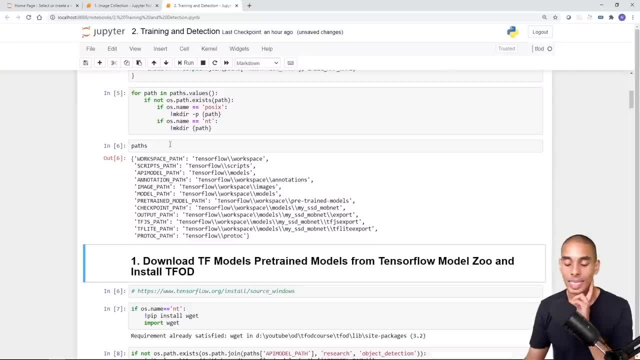 So if I actually type in paths, So this just makes it a whole heap easier to work with all of the stuff that we've got available within our working directory So we're able to refer to each one of these reasonably easily. So say, for example, we wanted to get where our model is going to be. 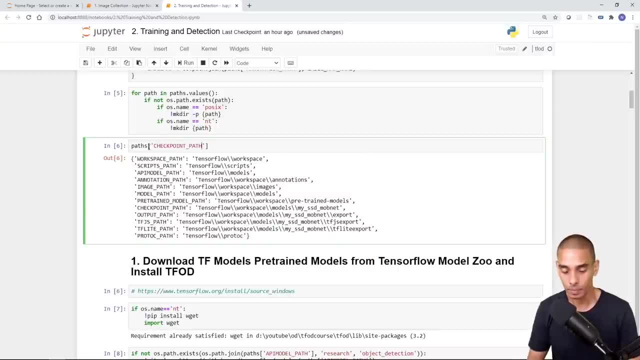 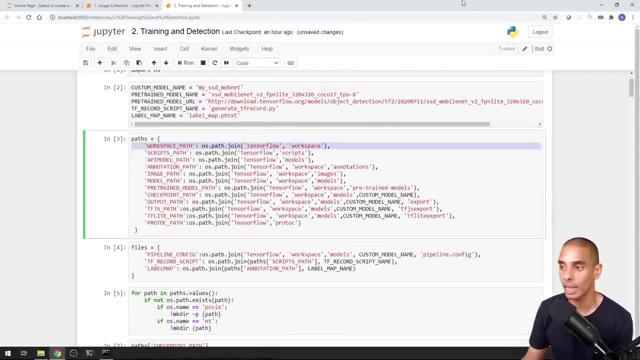 We could just type in paths, checkpoint, path- And you can see that we're now going to have that folder there. Now let me explain each one of these parts. Our workspace is going to be our high-level workspace, So let's. 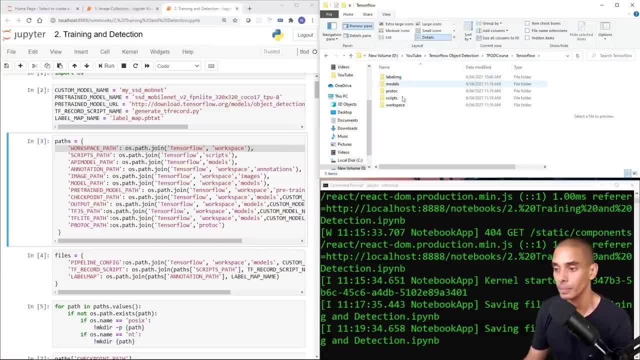 Open this up. So our workspace is going to be this, and inside of our workspace We're going to have our annotations, which is where we're going to create our TF record files. more on that later. Images was already there from when we collected our images. 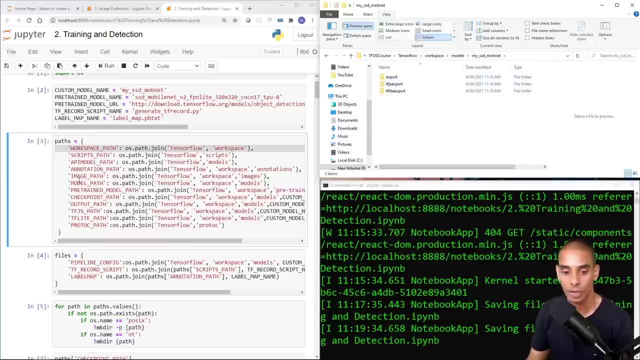 We also have our models folder and our my SSD mob net folder, which represents these two lines over. Let's find it. So we've got our models folder, which is this, and our, which is our model path, And we've also got 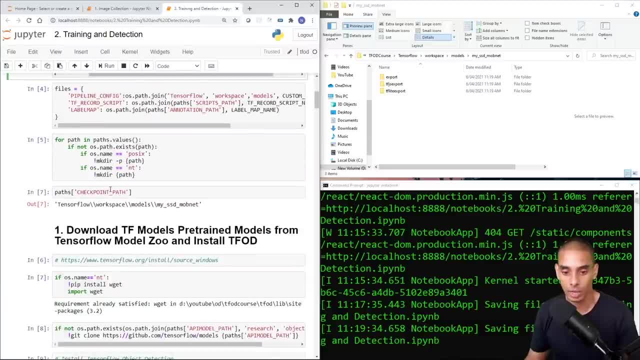 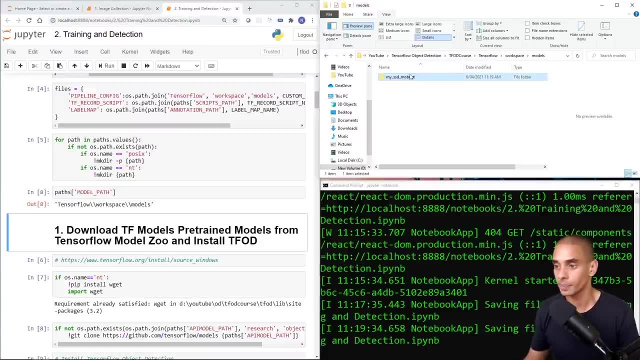 Checkpoint path, which is this as well. So if you actually take a look at checkpoint path or if we type in model path first up, That is this folder here. So TensorFlow workspace models, we type in checkpoint path. That is this folder here. 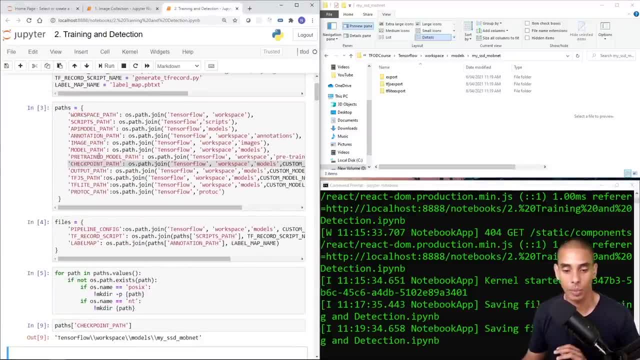 But again, you don't need to mess around with this. I'm sort of just giving you a bit of an explainer as to what each one of these are. So each one of these represents a different file path that we've got available there. 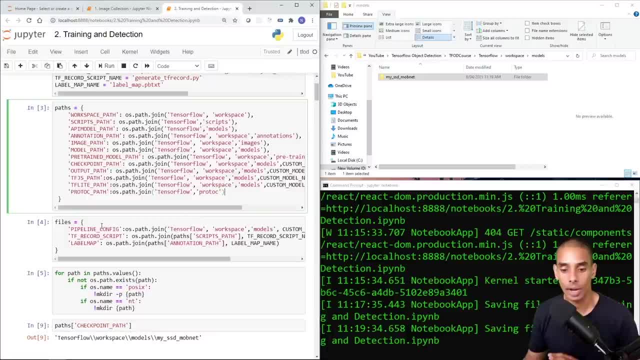 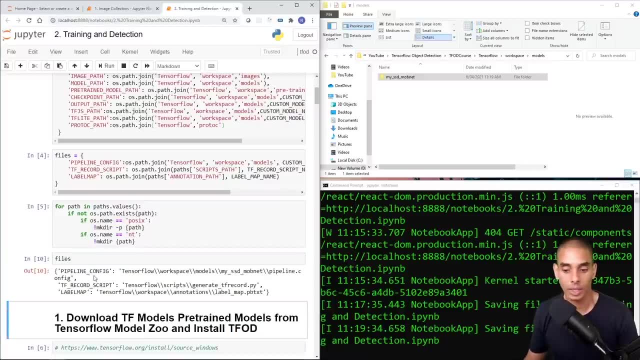 So if you want to dig into these a little bit more, you can. we've also got a couple of Variables inside of this files dictionary here. So if we type in files, You can see that we've got a file for our pipeline config which we don't have created yet. 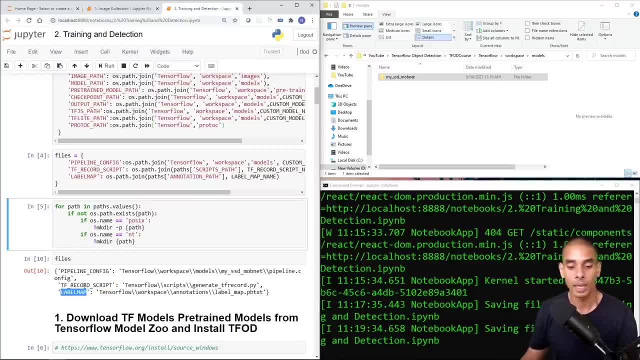 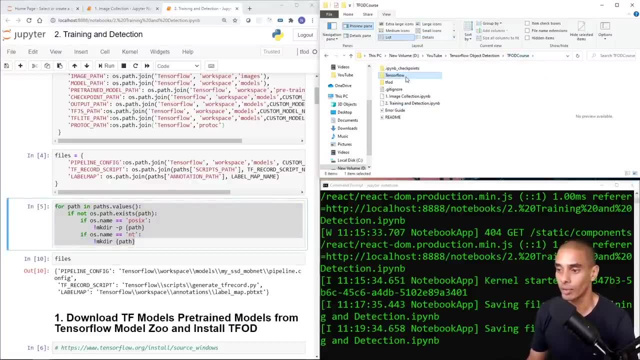 Our TF record script and our label map, But again, more on those later. This script down here is actually creating all of our directory. So you can see before that we didn't have all of these directories created right. So our script actually went and did that. 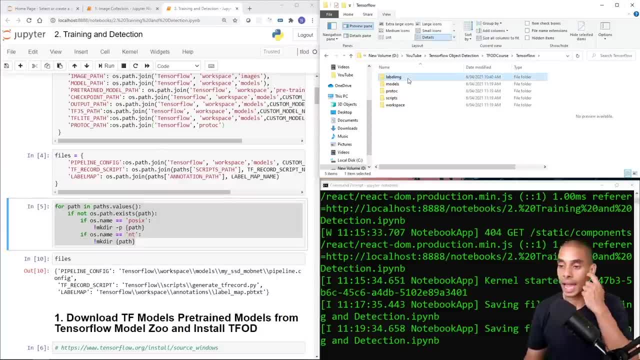 So if we actually now step in to our TensorFlow folder, we should now have five folders. So our label image folder, our models folder, Our protoc folder- Again more on that later- Our scripts folder and our workspace folder. And if you step into your workspace folder you can have a bunch more available in there as well. 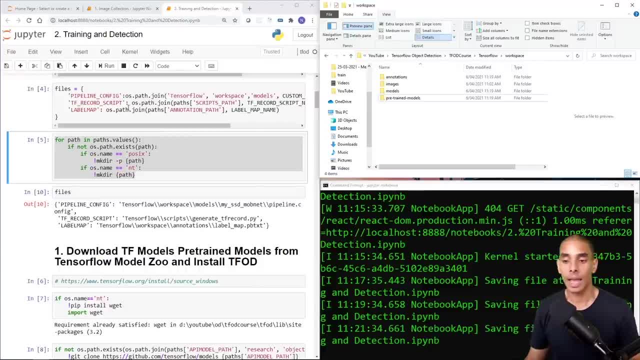 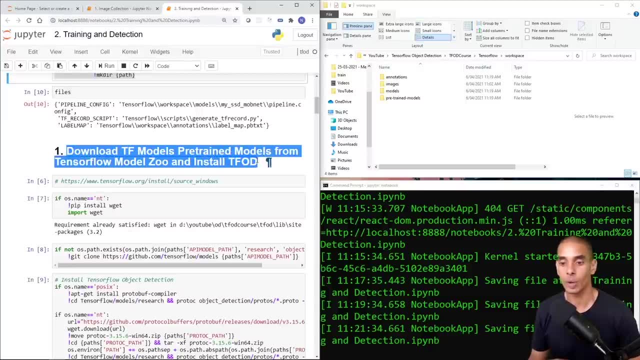 Okay, that is our folder structure now set up. Now, the next thing that we're going to go on ahead and do is actually download our TensorFlow models from our TensorFlow model zoo, And we're also going to install TensorFlow object detection. Now, this tends to be where a lot of people get stuck. 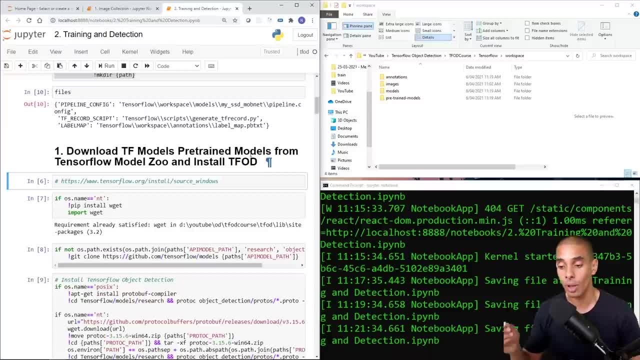 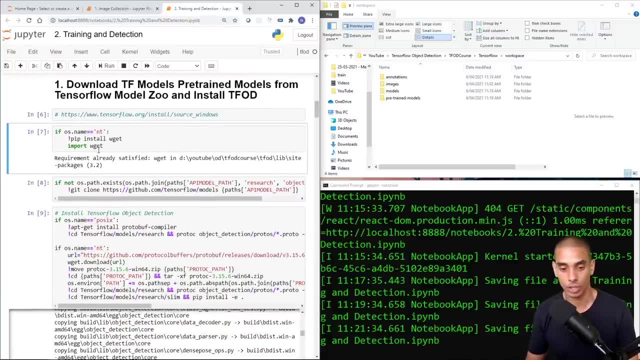 So we're actually going to take this step by step and I'm going to show you what to look for and how, How to validate that you've actually got this successfully installed. So, again, we're going to step into our first cell, which is this one over here, and we're going to hit shift enter. 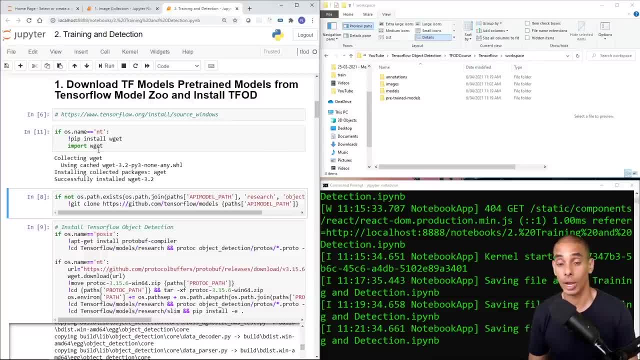 And this is going to install a package called wget. So this is just going to allow us to actually pull down our model from TensorFlow model zoo, And then what we're going to do is actually clone down the TensorFlow object detection repository. So if I copy this link here, let me actually show you that. 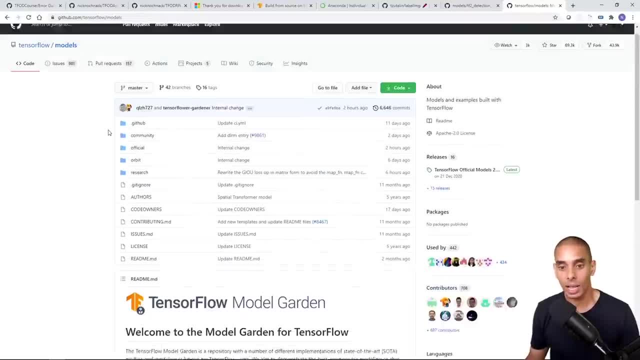 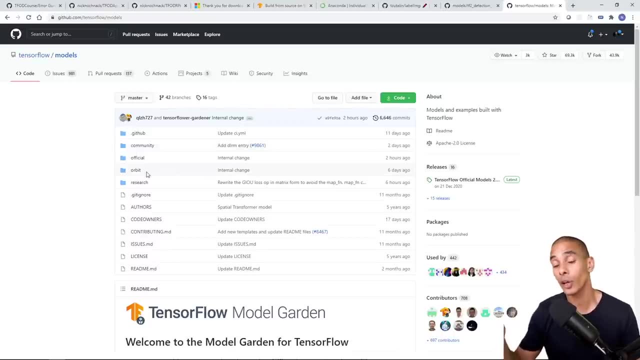 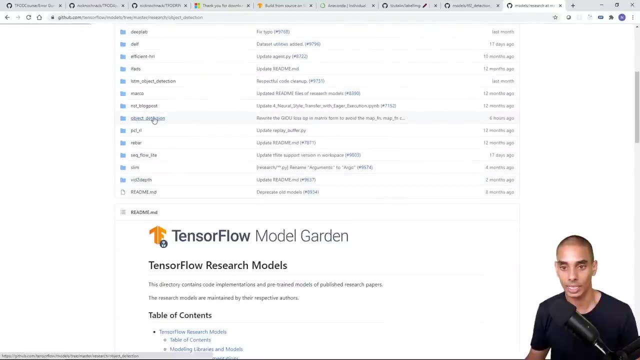 So this is The TensorFlow model garden. now, inside of here There is a bunch of stuff that is available for TensorFlow, but specifically we're interested in object detection, And when people refer to the TensorFlow object detection API, this specific section, which is in research and object detection, is what they're talking about. 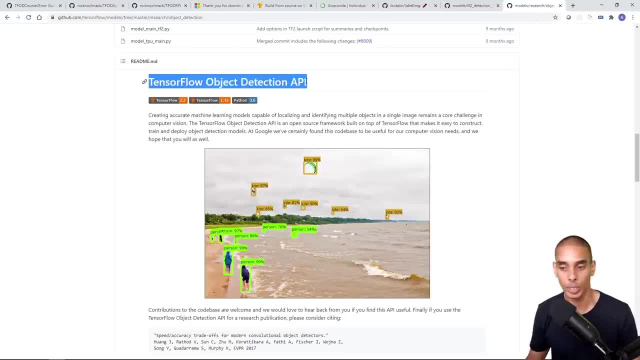 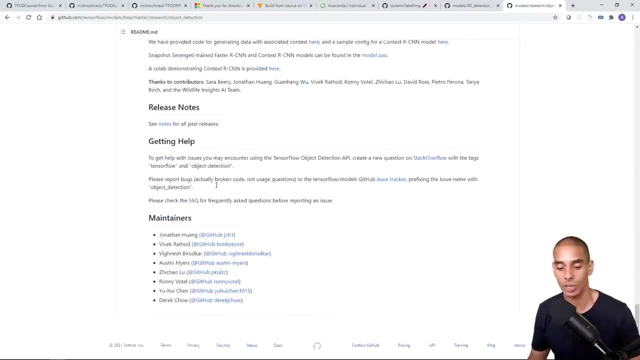 So everything that's in here is what represents the TensorFlow object detection API. Now again, you can see that there's a bunch of stuff that is available through here. There's a whole bunch of documentation on this as well. There's also a bunch of open source tutorials that are out there. 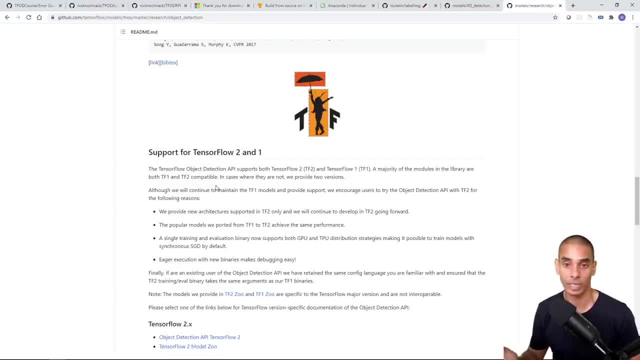 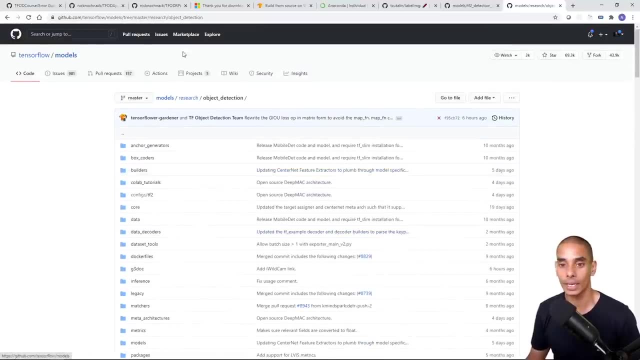 But again, I've tended to find this to be a little bit tricky to actually get through. So, again, this is why we're building up this course and why we're going to be going through it in great detail. So what we're actually going to go on ahead and do in that next line of code that we're about to run is we're actually going to clone everything that you see here. 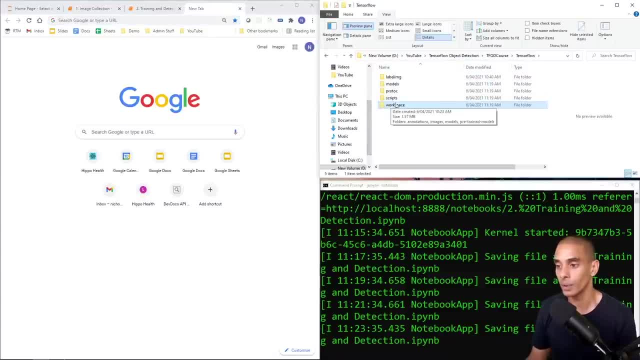 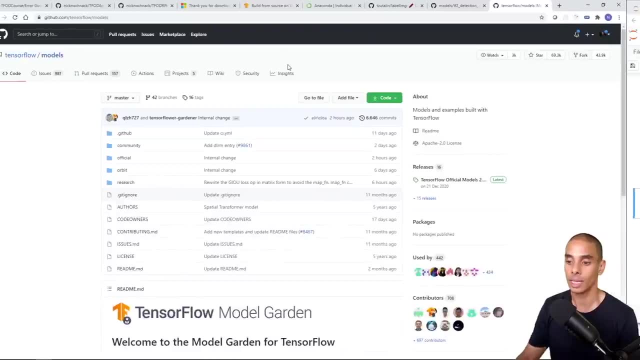 And we're going to clone it into this folder. So we're going to clone it into TensorFlow Or, if we start off inside of our root directory, so TensorFlow, object detection course, We're going to clone this model garden, which is everything you see here, into TensorFlow and then models. 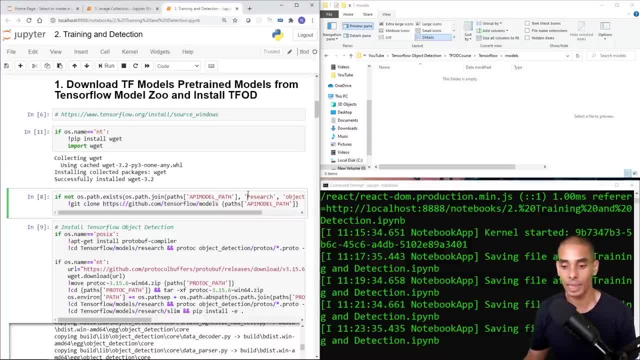 So, then, what we're actually going to do is we're going to install it from there. So if I run this cell here, it's going to do exactly that. Now, this may take a little bit of time to run, depending on the speed of your internet. 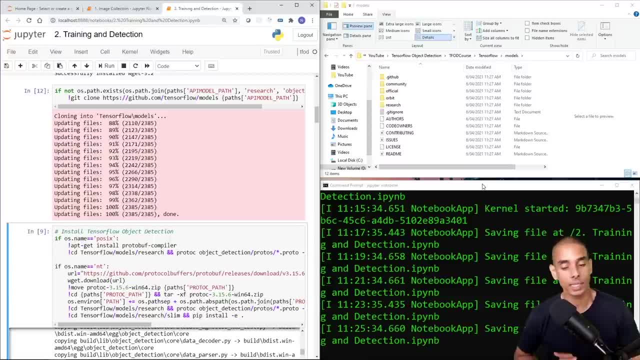 So let's go on ahead and run that. Okay, so that is our TensorFlow model garden, now cloned. So you can see in here that we've got a whole bunch of stuff. So we've got community official orbit research, so on and so forth. 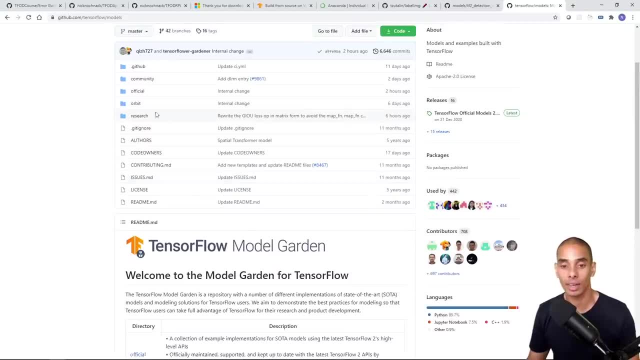 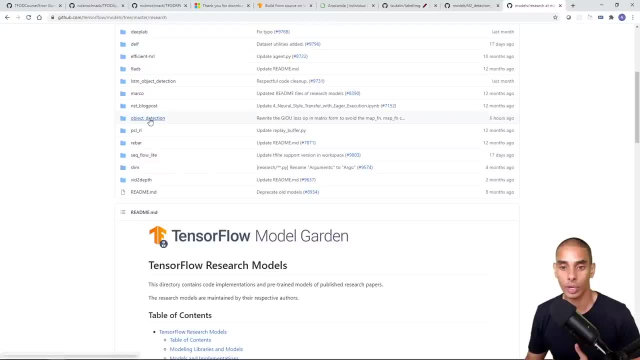 That is just mimicking this Now again, keep in mind There's a lot of stuff in here that you're not going to need for this, but we're just cloning down the entire repository. So specifically we're going to need inside of the research folder, inside of object detection: 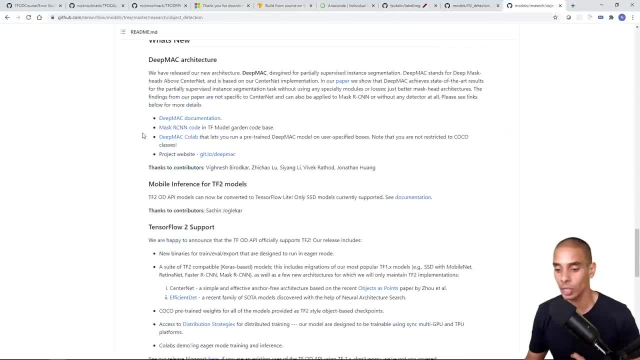 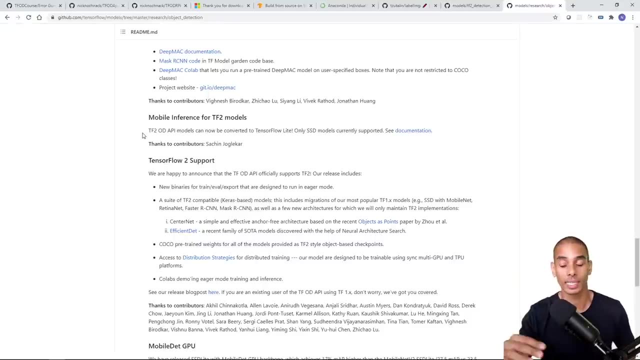 This is us right here. This is all the stuff that we're going to need to leverage the TensorFlow object detection model API or the TensorFlow object detection API. Now, keep in mind, This is TensorFlow 2.. So this is the latest version of TensorFlow, not TensorFlow 1.. 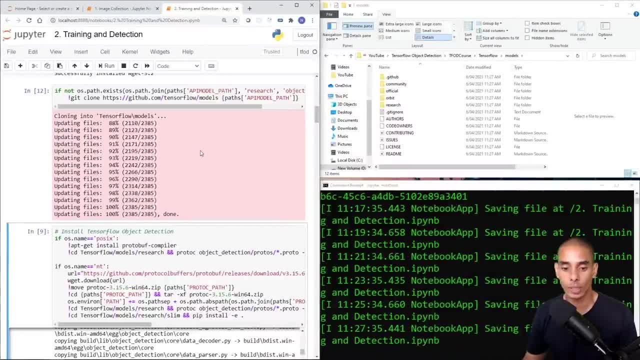 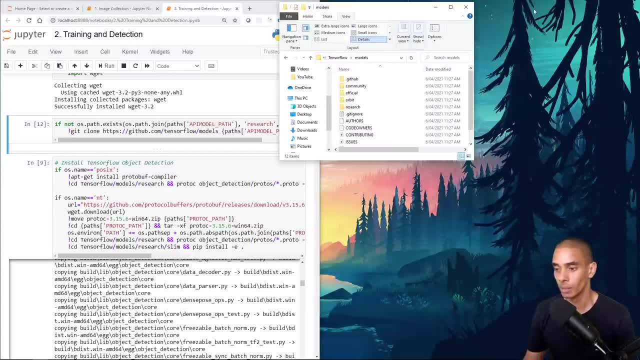 Cool, Alrighty. So what are we going to do now? So we are going to then Go on ahead and install it. So right now, we've just cloned it. So if we take a look, let's minimize this. We've just cloned it into this repository. 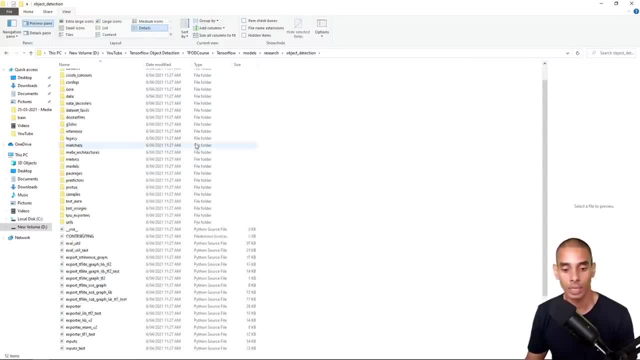 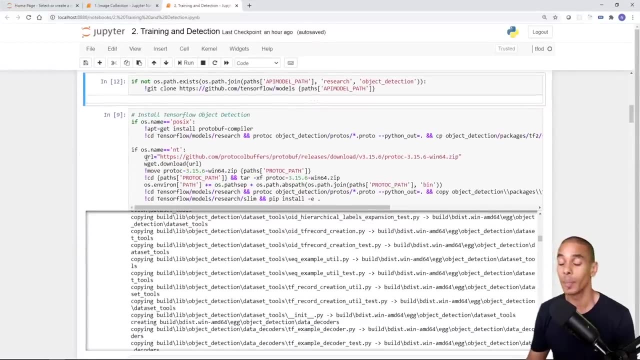 So, again, remember, inside of research, inside of object detection, This is all of the stuff that we're going to leverage Now. what we actually need to do is actually run through the install step. Now, again, there's a bunch of stuff required to actually go on ahead and install this. 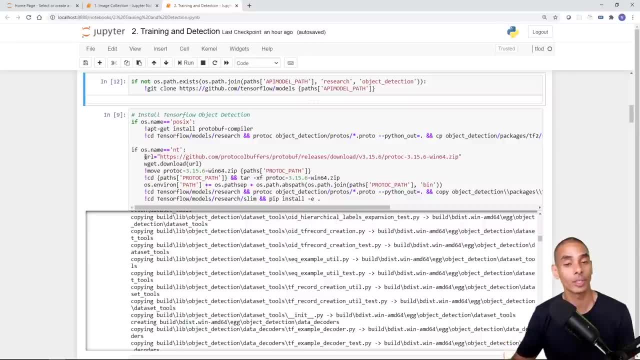 So if you do get stuck or if you do run into issues, by all means check the model guide, but I'm actually going to step you through how I actually go on ahead And install this stuff. So the next cell is actually going to again detect whether or not we're using Linux or whether or not we're installing Windows, and it's going to do three things. 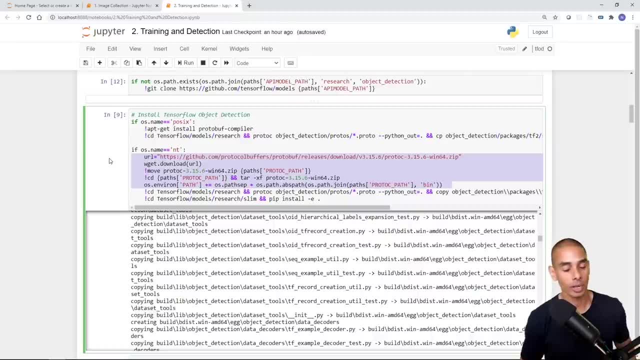 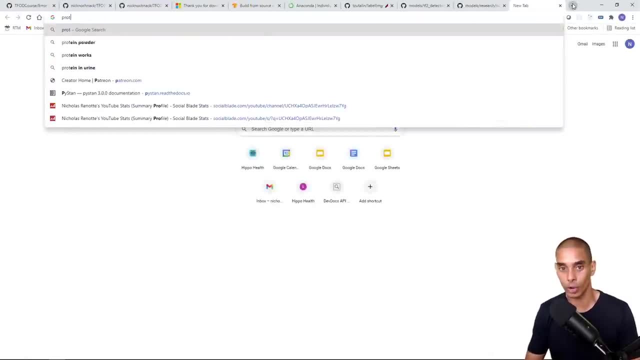 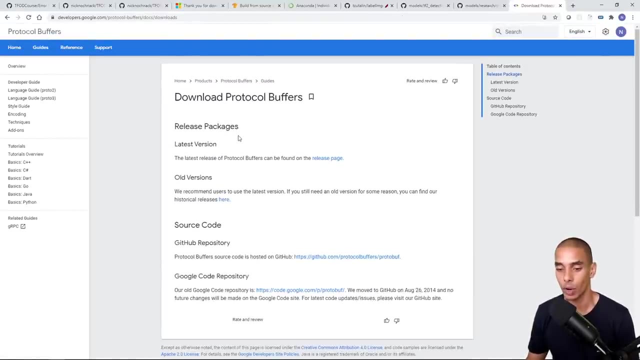 So it's at first up. It's going to install protoc. So protoc- So a lot of the TensorFlow object detection stuff using uses something called protocol buffers. So if you actually type in protoc, So what we're actually going to do is we're going to set this up for our TensorFlow object detection API. 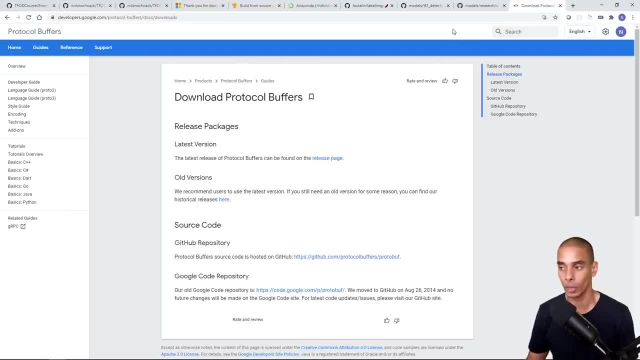 So again, you don't need to do anything But run that cell. It's going to do it for you, And normally this can be a little bit tedious. So again, it's just going to run this cell and do it for us locally. 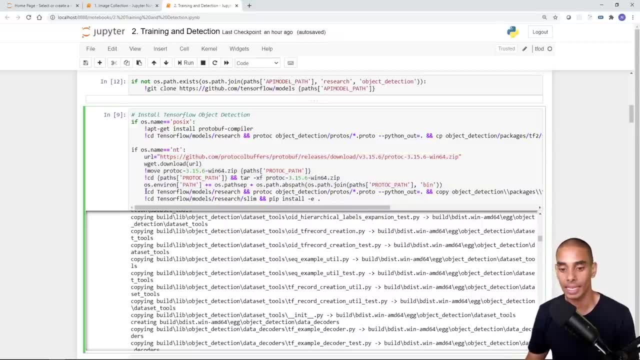 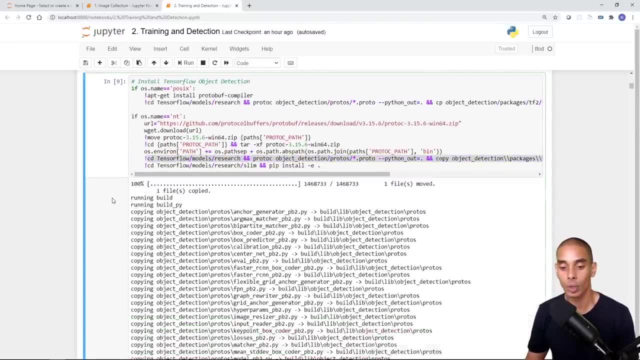 So if we run this now, it's going to install protoc And then it- this line over here is actually going to go on ahead and install the official TensorFlow object detection API, Then what we'll do is we'll actually verify our installation. 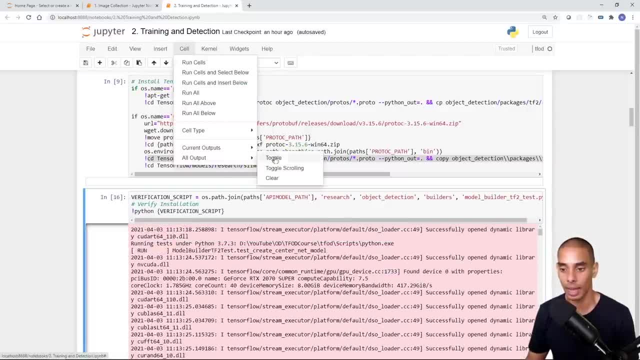 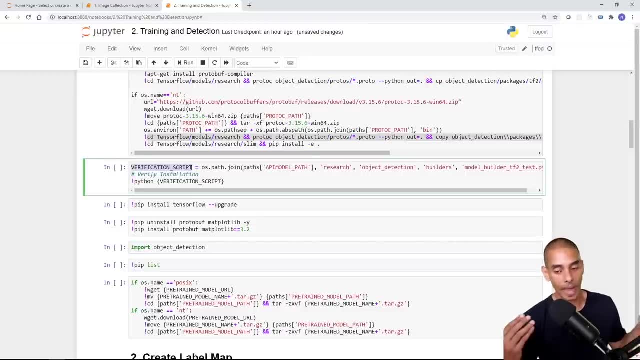 So this script down here, So let's actually clear our output so we can see that. So this cell down here is actually going to run our verification script. So this will tell us Whether or not we've actually got the TensorFlow object detection API installed successfully. 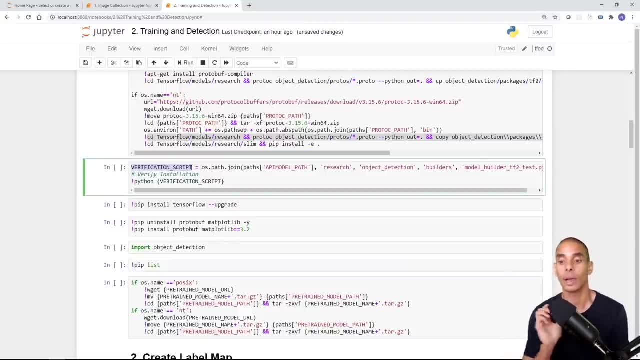 If it is installed successfully, you'll see it read as okay. So that will mean that we've successfully installed the object detection API and we can kick things off. If not, I'm going to show you how to work through it and how to get it installed appropriately. 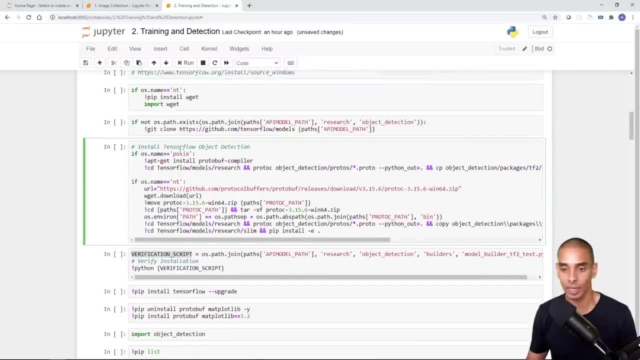 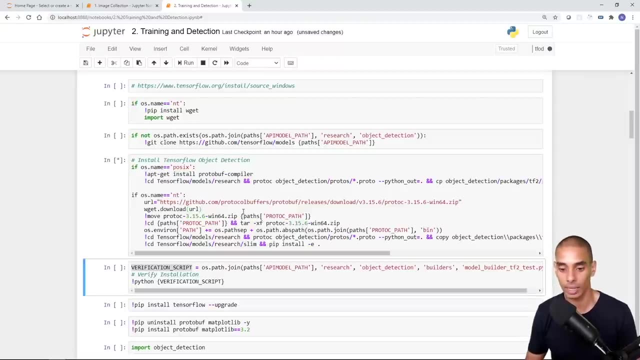 Okay, So what we're going to do now is we are going to run this cell over here, So this going to install protoc, set it up, and it's going to install the object detection API. So let's run this now. again, This is going to take a little while to run, and ideally if you're running inside of a notebook on Windows. 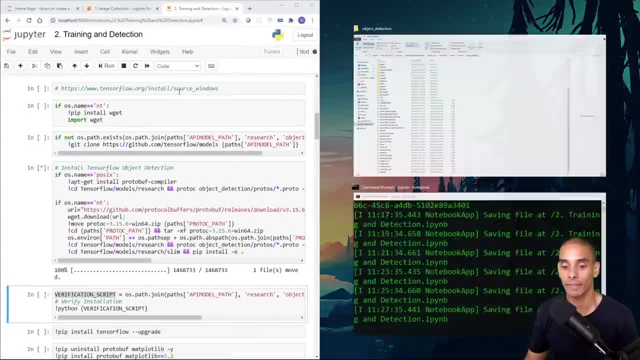 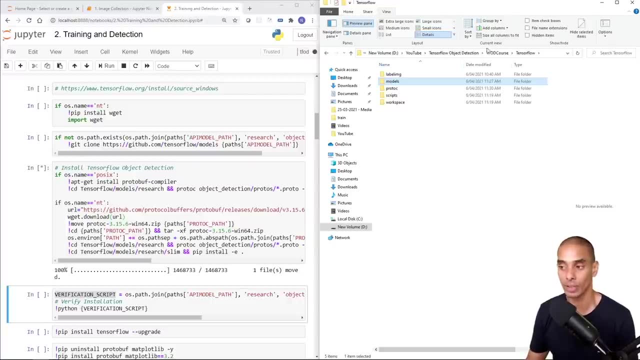 you might not get the status updates, But the way to check if it's currently running is if you go into. remember we're inside of our virtual environment here. So again, make sure that that's enabled and you're running it inside of that particular notebook, inside of that environment. 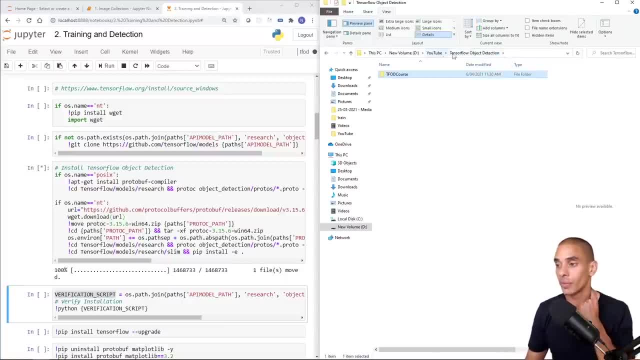 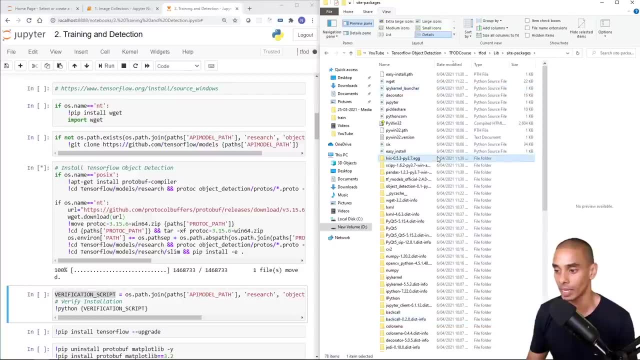 So what we're going to do is actually show. so I'll show you that. So if we go into our tfod file now in the inside of lib site packages, you'll actually see that it's installing packages. So Right now it's up to 1030 or 1130.. 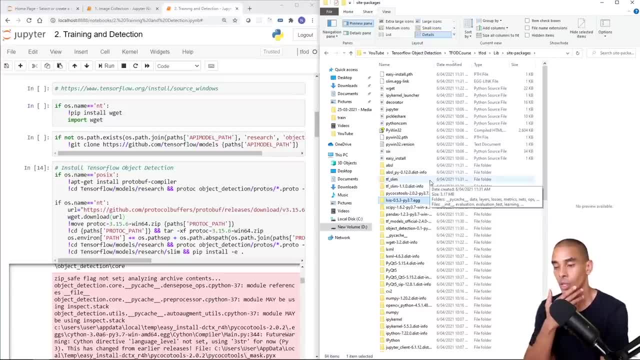 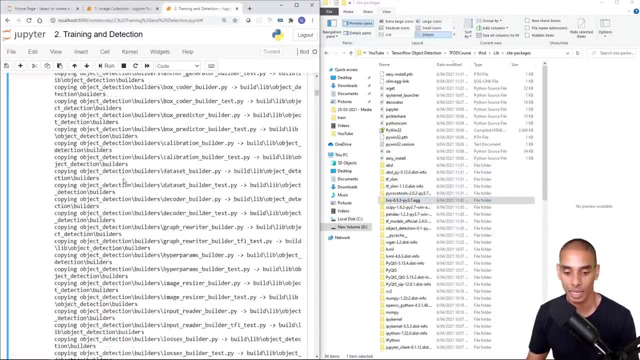 So you can see it's installing a whole bunch of different libraries. So what you should ideally see is that this is continuously installing stuff. now It may say that it's successfully completed, But ideally what you want to do is until you get an okay from that verification script. 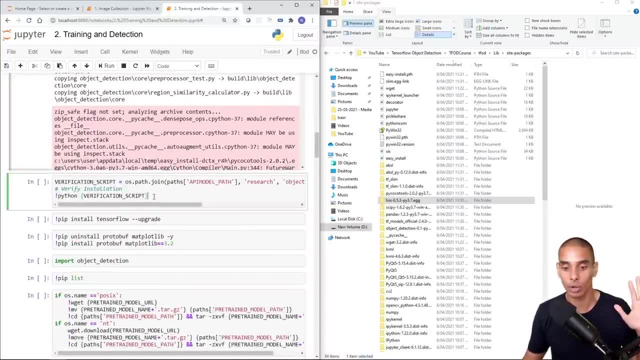 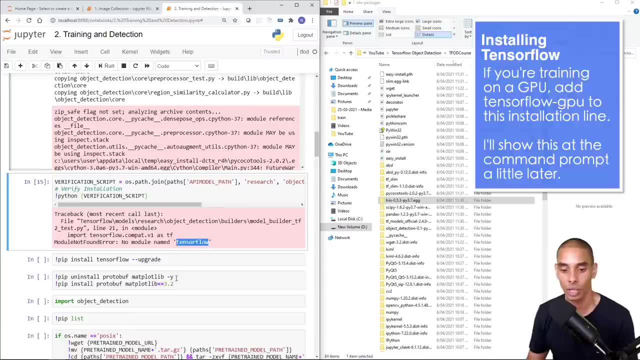 It hasn't successfully installed, right? So this is going to be your golden Bible. So let's run the verification script So you can see here that it's saying that it there's no module. So what we're going to do is run this next line down here, which actually installs TensorFlow for us. 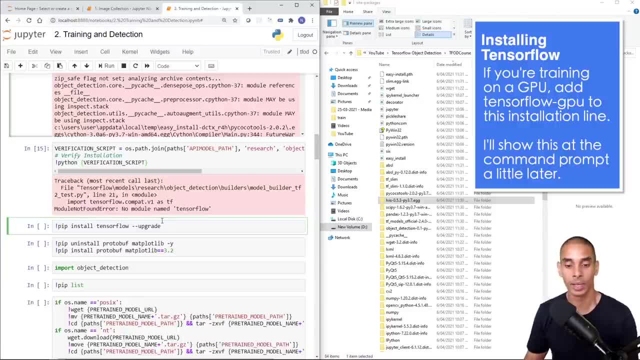 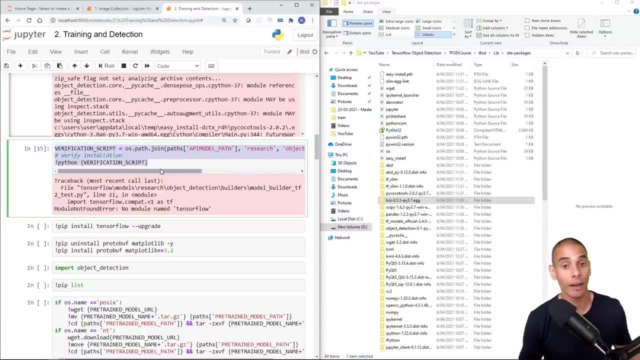 So what I did is I included some of the lines that I use to solve these errors, So by running our verification script. this is again a standard tense flow object detection script that allows us to verify our installation. So in this case it's telling us: hey, even though we've gone and run that script, it doesn't look like we've got tense flame sword. 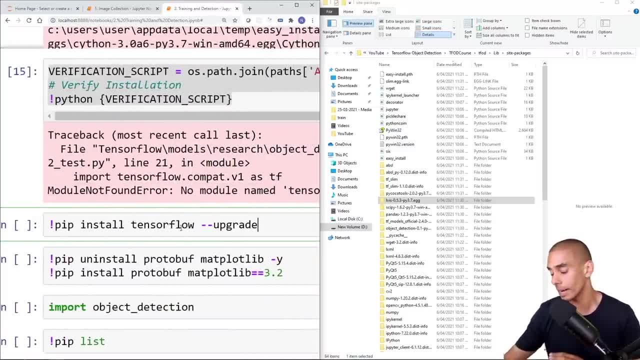 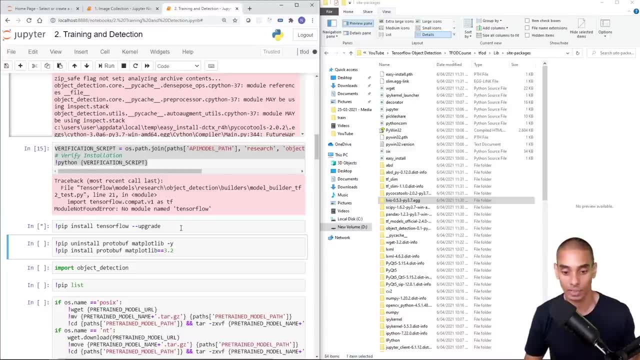 So this next line down here is: you might not need to run. it might say: okay, and I'll show you what it looks like when it's successful. Might work all perfectly. If it doesn't, then in this case we're going to install tense flow. 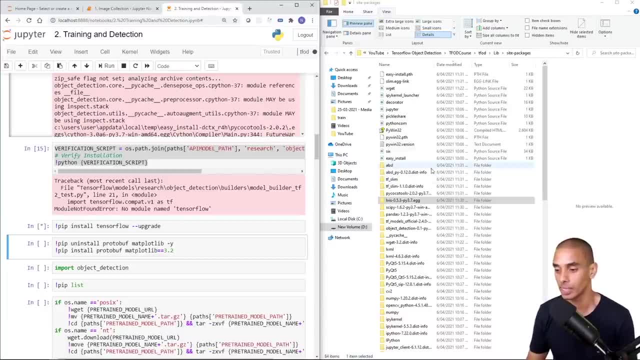 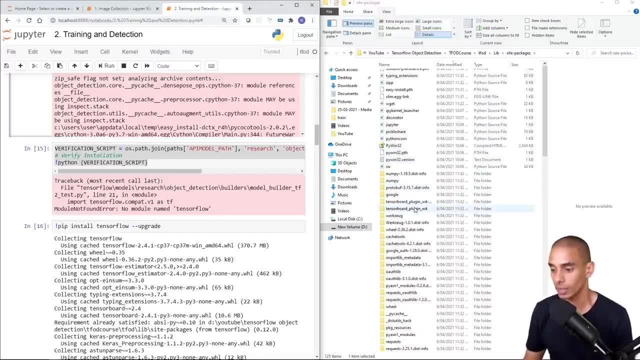 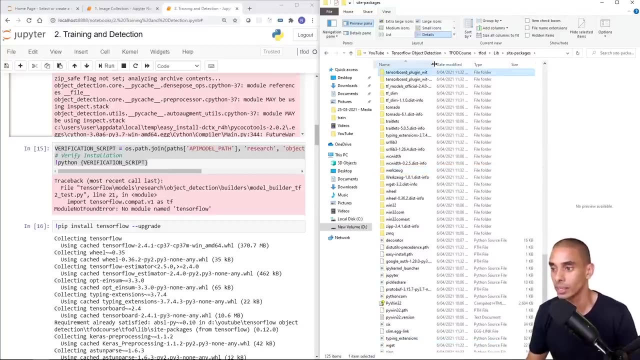 So let's do that And ideally you should start to see tense flow installing on the right hand side. Cool, So that should be tense of flow installed, even though it's a right now, keep in mind. So sometimes you can run into errors with this. 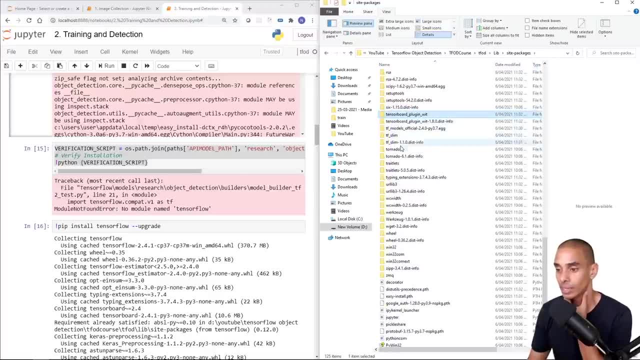 So even though we ran tense flow installed doesn't look like it's in store tense flow So I can't actually see the tense flow file or library there. So tense Board and support plug-in TF models: official TF slim. So if we go and run this again, it's still going to tell us no module installed or no module named tense place. run it again. 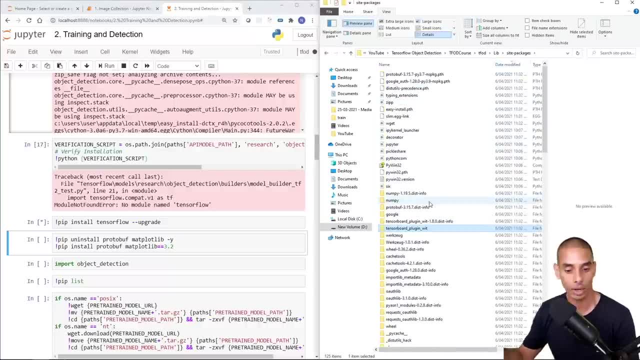 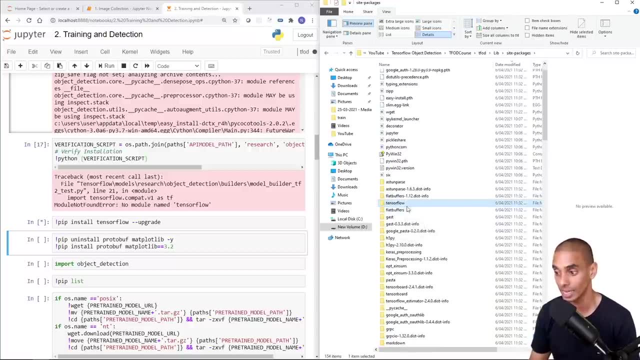 And again it should ideally install the second time around. don't ask me why. it just seems like sometimes it throws up, doesn't seem to want to run, So now it's installing a bunch of additional packages. You can see tense flow there, So ideally this is looking a little bit better this time. 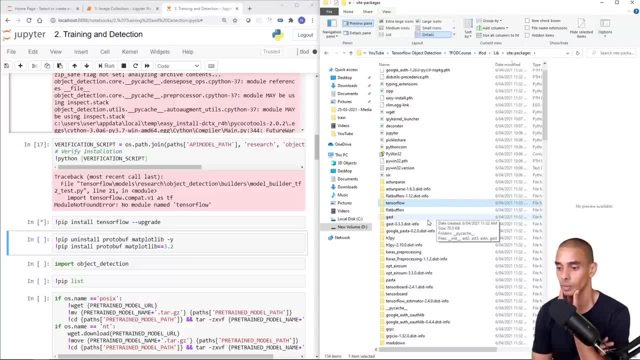 So let's wait and see. So again, that verification script is your golden Bible, right? So like if you get the okay sign, then you should be good to go. So in this case, looks like it's still installing Completed over here. 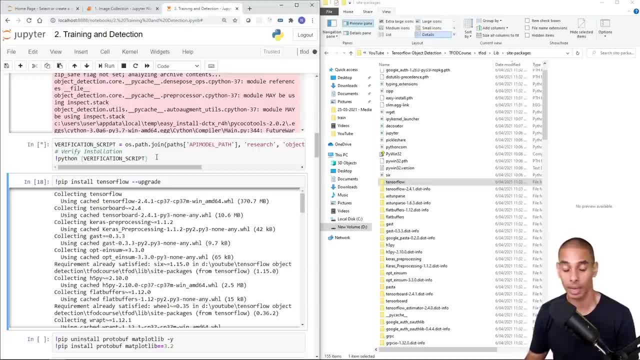 Let's run a verification script again. That's looking a lot better this time, So it didn't run really fast, So ideally it'll take a little bit of time. All right, So we've now got an error called no module named matplotlib. 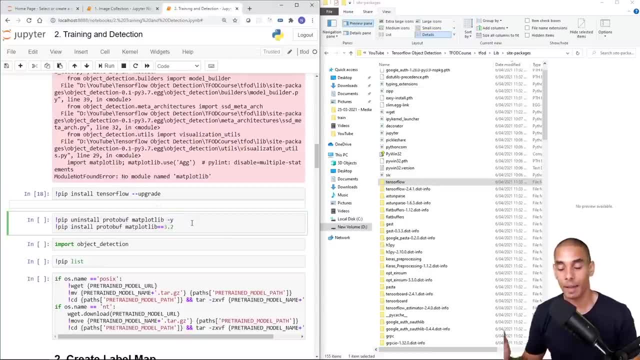 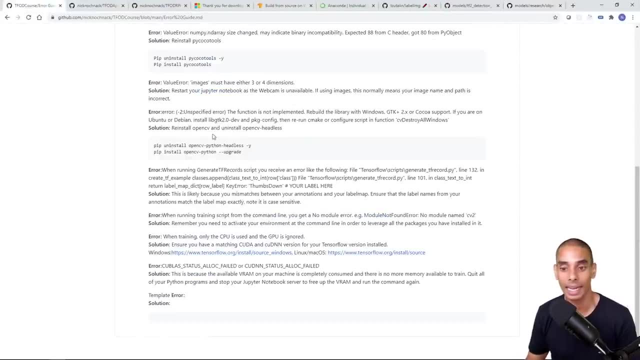 So this one, and looks like again. I've got the script to run that. now again This no module found error is pretty common, So this just means that you need to install a package. Now I've got this again inside of the error guide. 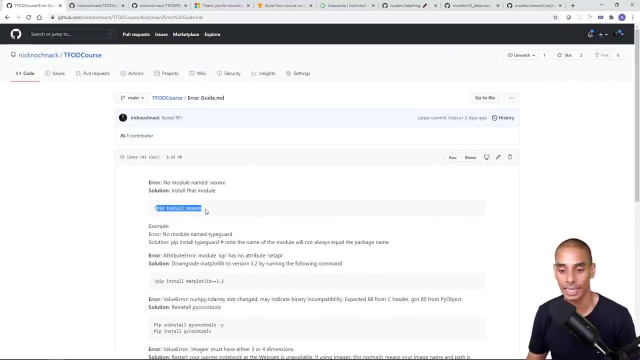 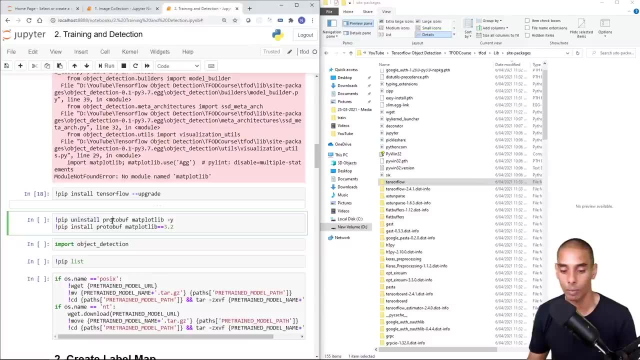 So if you get no module, named whatever, you just need to go on ahead and install it. Sometimes you need to uninstall it and then reinstall it. If you need to uninstall, it's just pip uninstall and then whatever library you need to uninstall, and then dash. 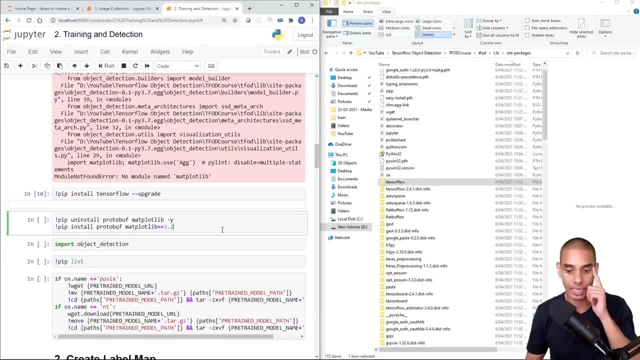 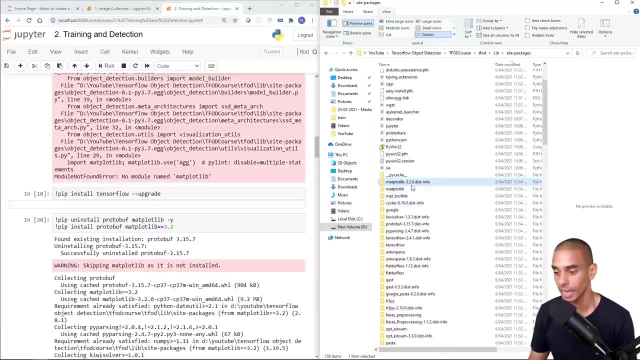 Yes, and then you install whichever one you want. So in this case, here I'm going to run this next cell, which does matplotlib and protobuf for us. Okay, that's looking good. So you can see again inside of our virtual environment. 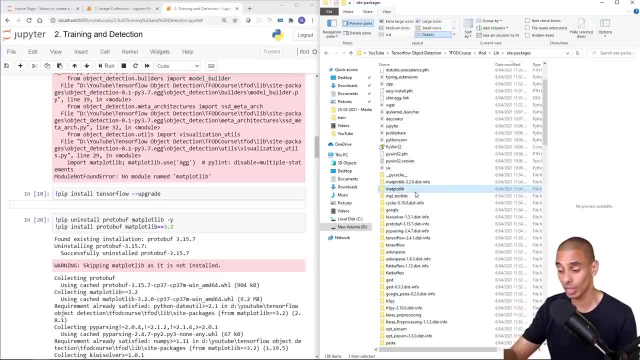 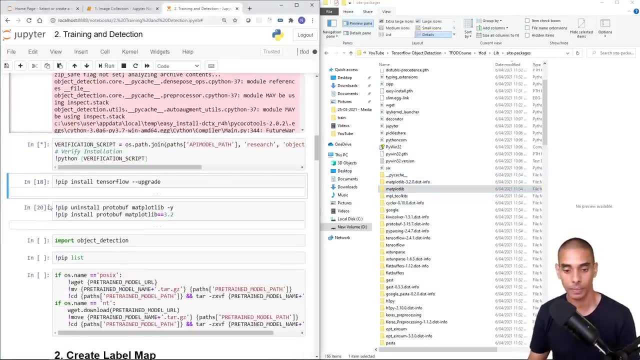 This is the advantage of having the virtual environment: You can actually see visually what libraries are installed. So that's looks like it's gone and done that it's gone. run this verification script again. All right. so no module named PIL, So let's go on ahead and install this. 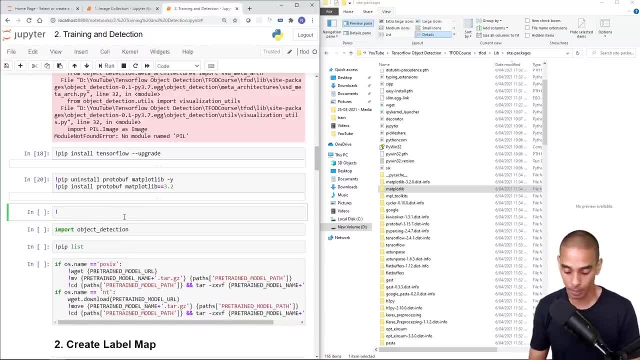 So this one is one that I didn't have pre-configured right, So we can do that. So pip install PIL. I believe PIL is pillow right, So so, again, if you get these types errors, you can just Google them. 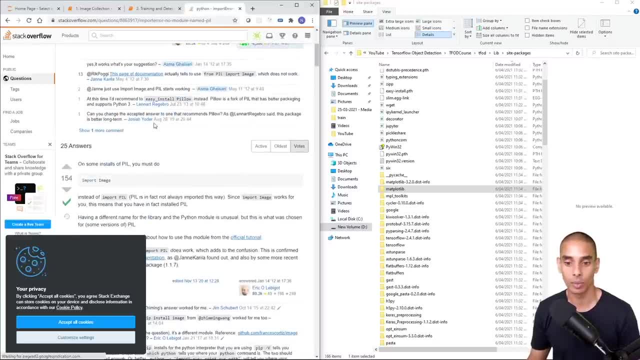 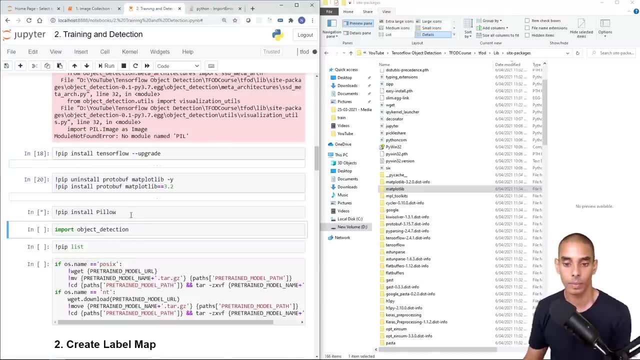 So no module named pill just means you need to install pillow. So more often than not they're not. people are going to tell you to install pillows, pip, install pillow right. So let's go on ahead and run that. Cool, That looks like it's installed. 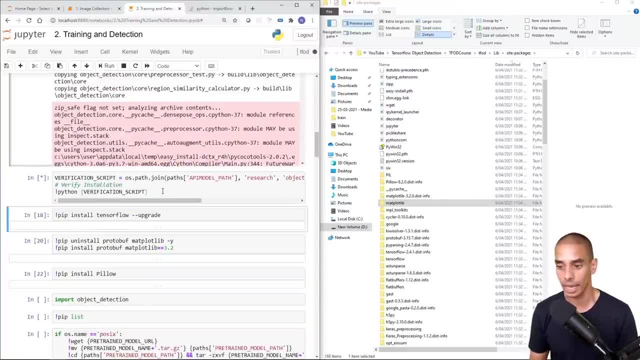 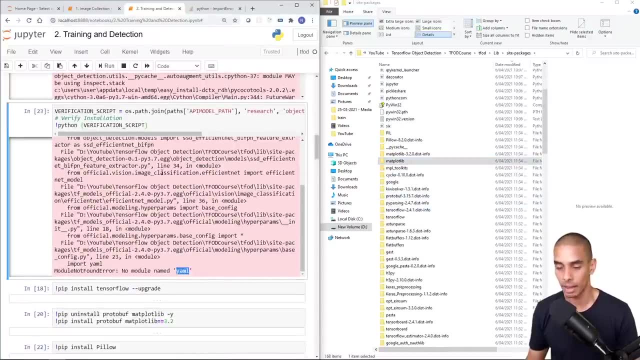 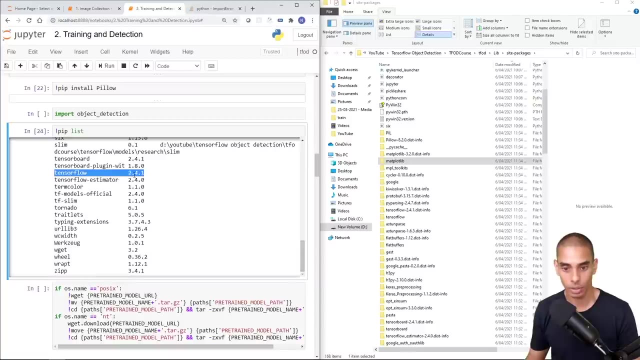 Run that now And checking our verification script. What are we getting now? No module named yaml, So this looks like it might not have. let's check out. So let's run pip list now. So have we actually installed tensorflow, got 2.4.1.. 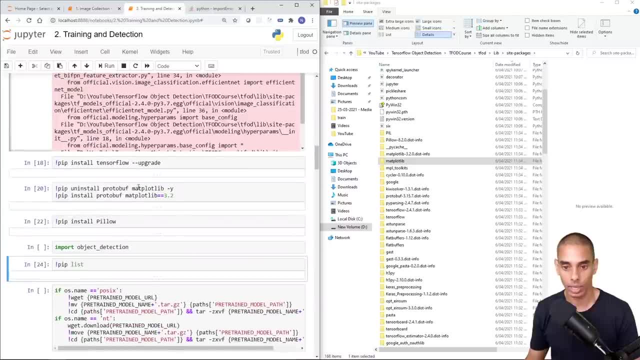 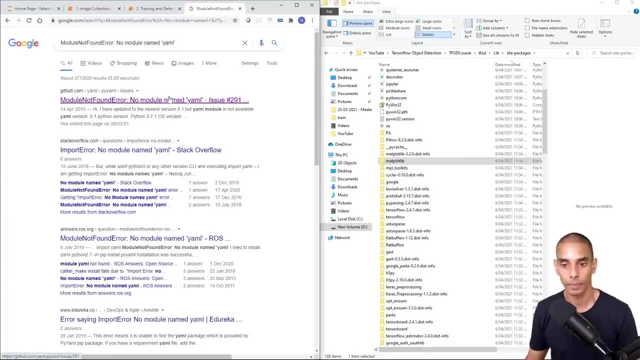 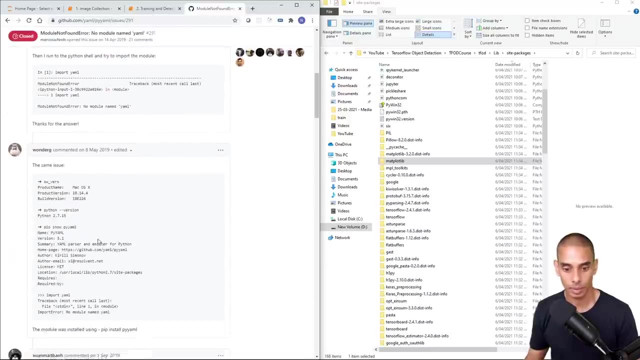 That's looking good. Okay, All right. So let's install yaml. now. No module named yaml, So let's see how we install that. To install yaml, We need to run: believe it's pi yaml. Yep, So it looks like. so, python, pip, install pi yaml. 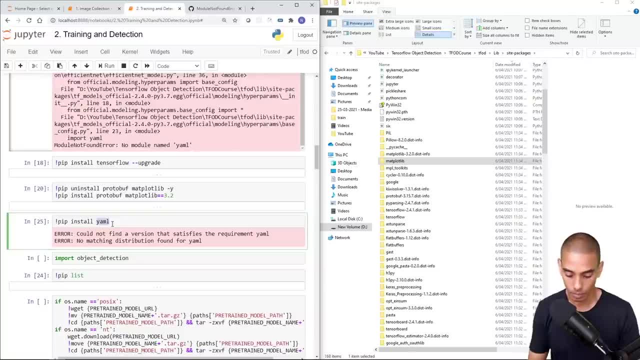 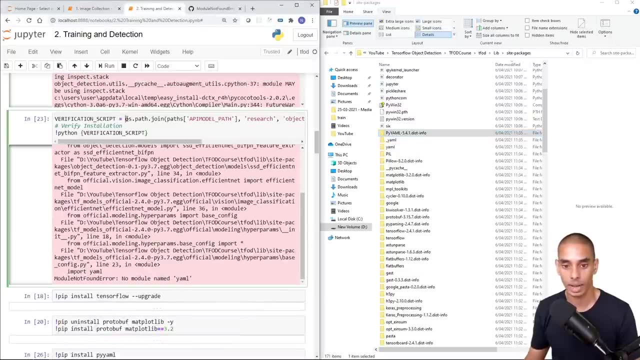 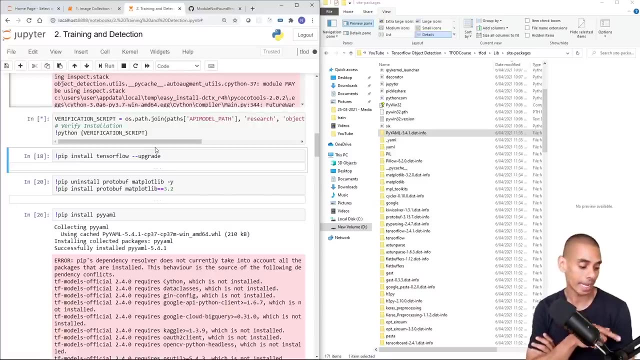 So let's do that. Okay, So that looks like it's installed. You can see pi yaml there, So let's again run our verification script. I can hear my GPU spinning up right now, So maybe that looks like a good sign. 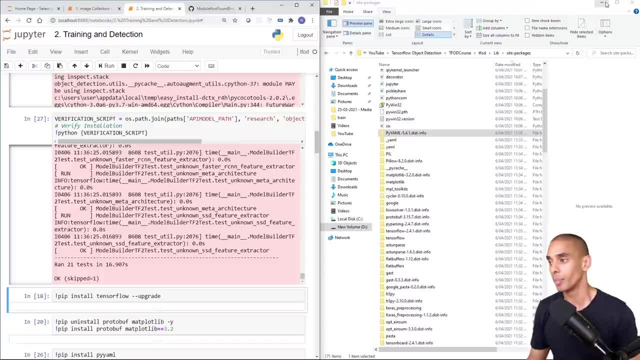 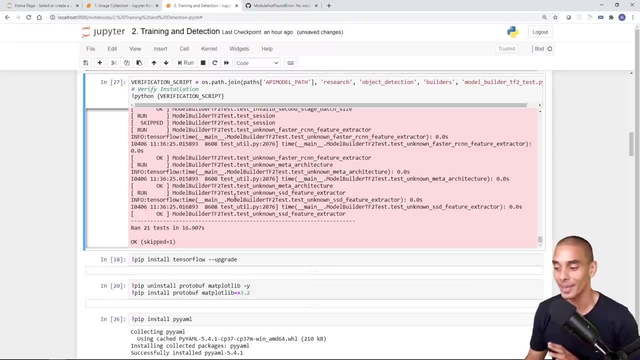 So this is looking good, even though it's in red. All right, beautiful. So we're good. now, If you get to the point where you run this successfully and right down the bottom, even though it's in red- I know it doesn't look that great- 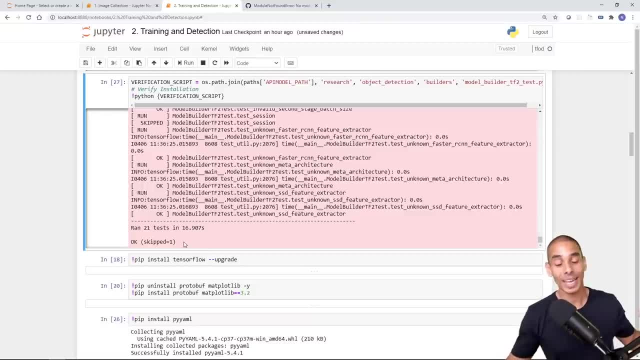 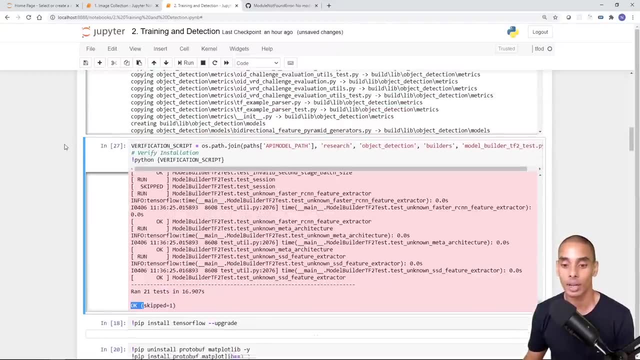 It should say okay. So if it says okay, then that means you have successfully installed the tense flow object detection library, right? So basically, this means that it's going to go and run all of its verification tests to make sure that it's actually working. 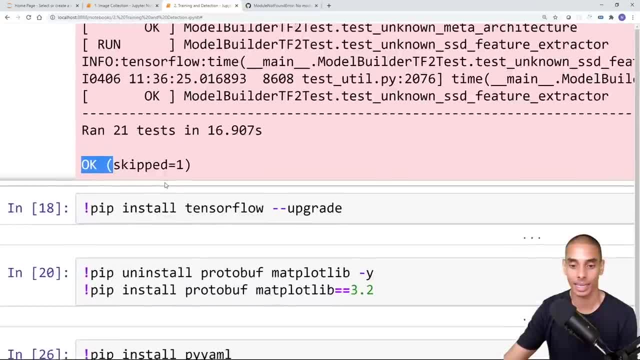 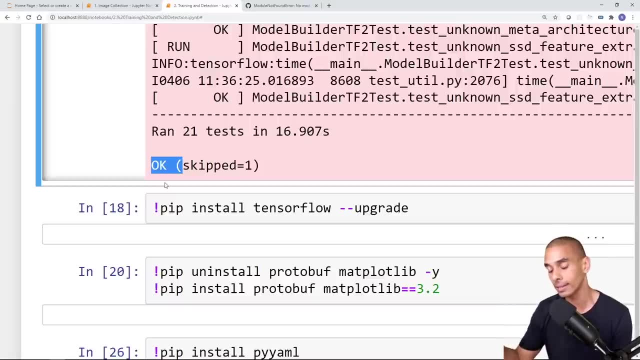 And if it's run successfully, you should get okay down the bottom. Let me zoom in on that because that if you get to that point, that's a huge win. right now You saw how I was solving those errors. So if you got no module X, just go and install that module. 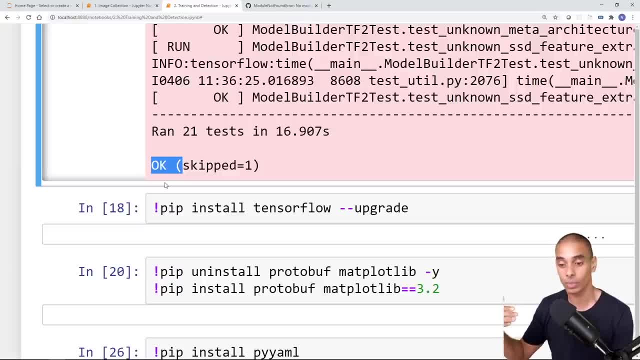 If you got no module Y, go and install that module. Sometimes you need to uninstall stuff And reinstall stuff, But again, if you get stuck, hit me up in the comments below. Join the discord server. But ideally that's going to be the same pattern, right? 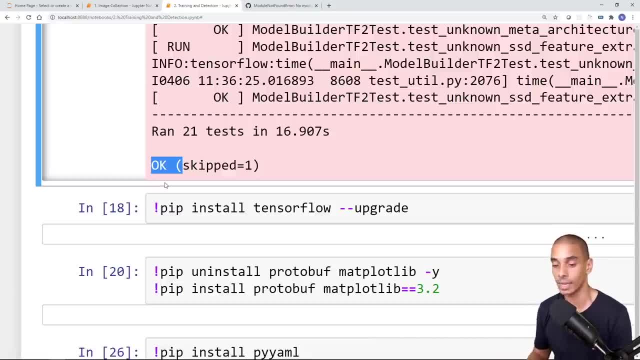 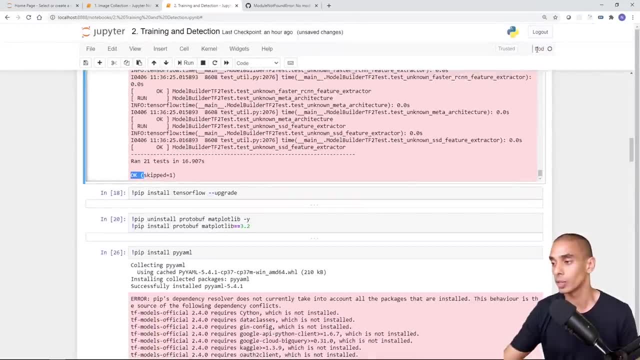 So if it says no module X, you just go and install module X And because you're inside of your virtual environment, it's going to be installing in the correct place. Now, remember our virtual environment is up here, So we're using TFOD. 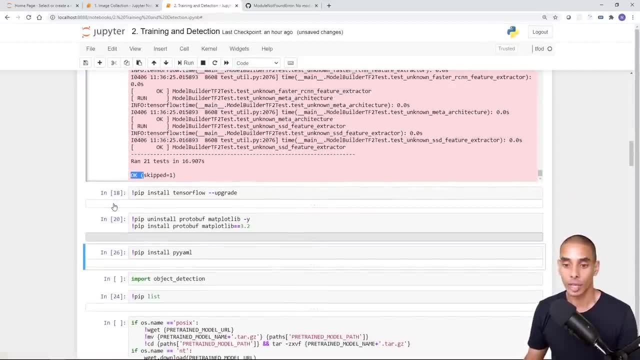 Need to make sure you're in there. So what did we have to go and do to get ours to run? So we installed tense flow again, We installed matplotlib and protobuf and we installed pillow. So remember, we're going to run it. 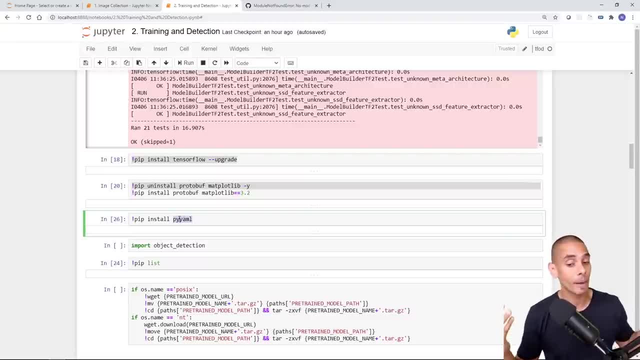 We installed pip, installed pillow and we also installed pyeml. Now again, this might be different depending on your particular environment. You might need to install more stuff, less stuff. It might just run perfectly fine. But I wanted to show you a real-life installation, because this is me installing from scratch. 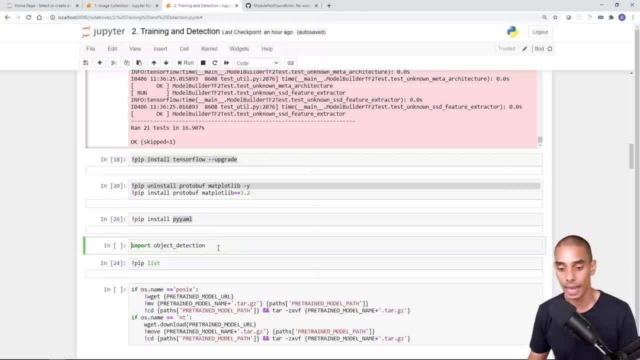 You can start to see what it actually takes to install it. Okay, so it's not all sunshine and rainbows. That's, I guess, that the core thing that I wanted to point out. So I'm not just doing it in smoke and mirrors. 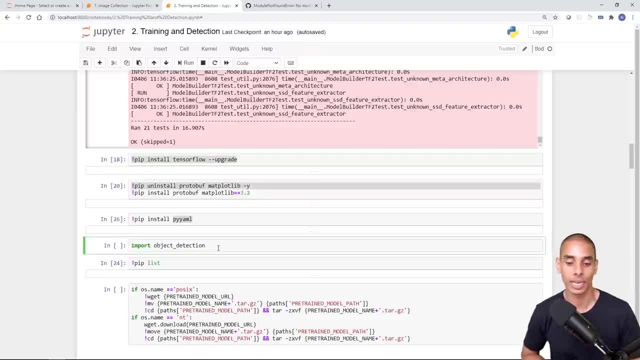 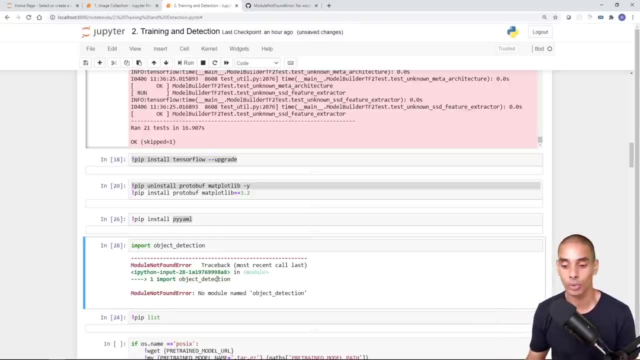 You can see that you might run into stuff, But more often than not it's just a pip install that you need to do. Now, if we run import object detection, you might still see that you get a error here where it says no module named object detection. 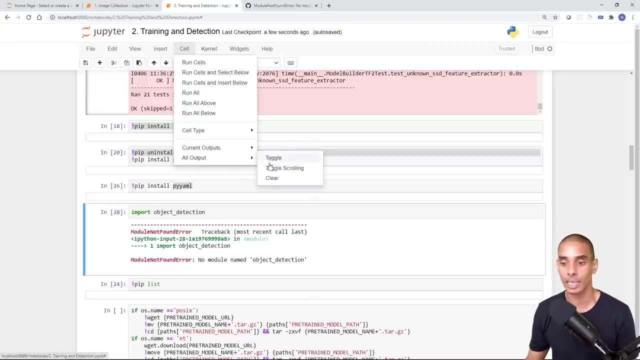 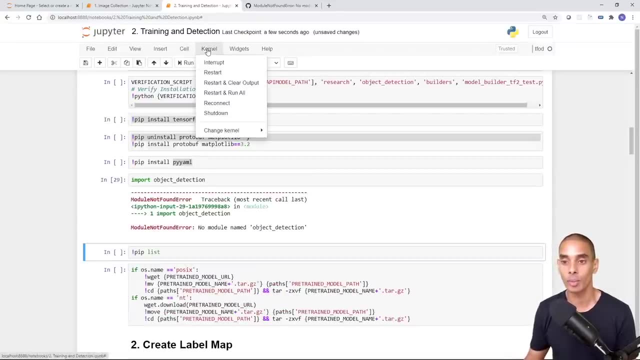 What you can do to solve this is just restart your kernel. So first up, let's clear all of our output from this. So it's a little bit clearer If I run import object detection again still saying no module. So what I normally do here is I'll restart my notebook. 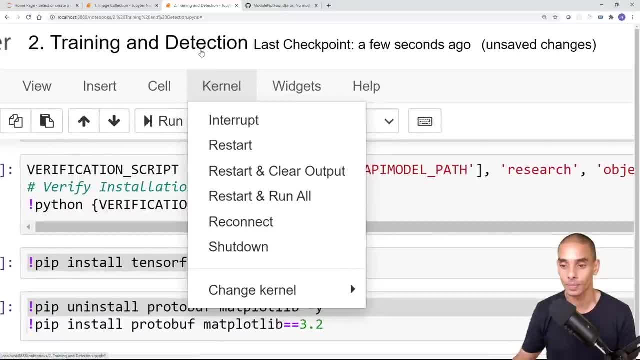 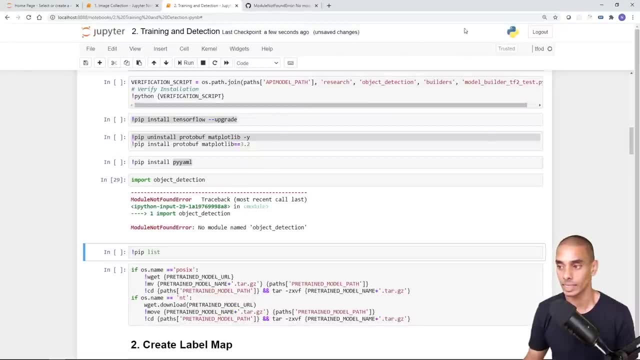 So if I hit, let me show you. So if we go to up to kernel restart and then I'll say restart, You can see it said kernel ready, Then what I'll do is I'll go up to here, zoom out, re-import these. 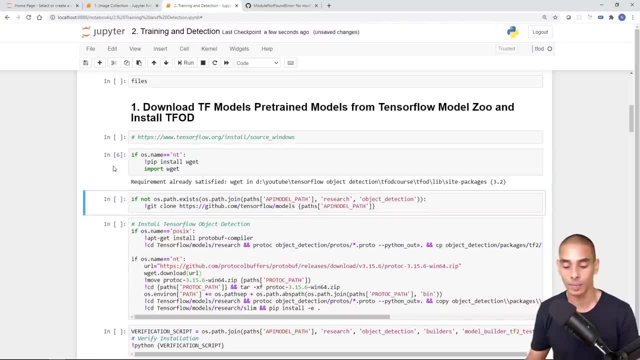 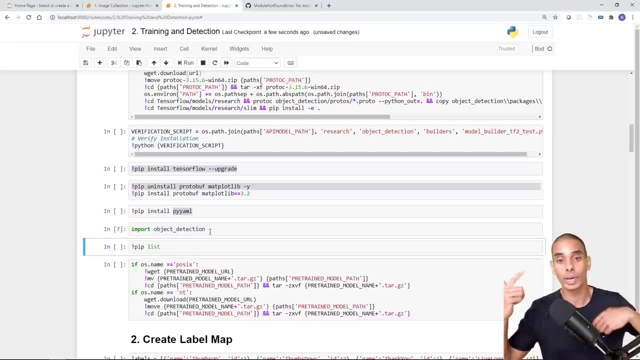 You don't need to do all of this again. So we just need to run wget And then, if we go down here, you can see that it's now installed successfully. Sometimes you just need to restart your kernel to be able to import into your notebook. 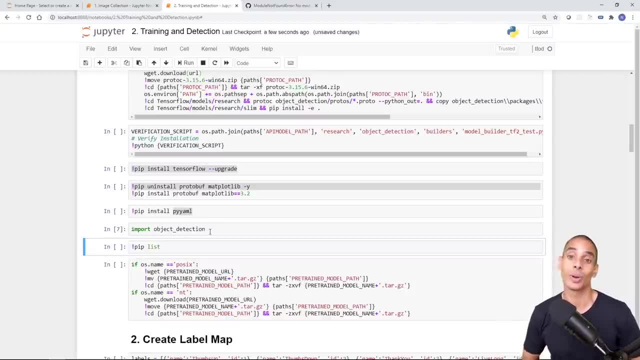 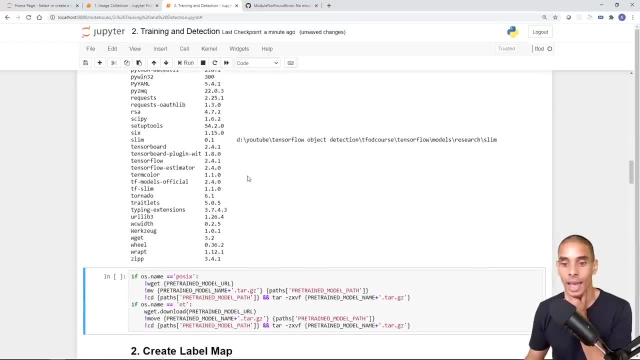 And in that case that's our object detection API now installed and available and ready for use. So we went and installed a bunch of stuff There. So if we run pip list you can see that we have a heap of additional libraries now installed. 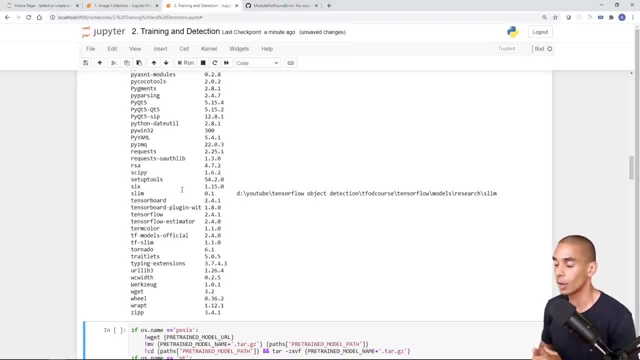 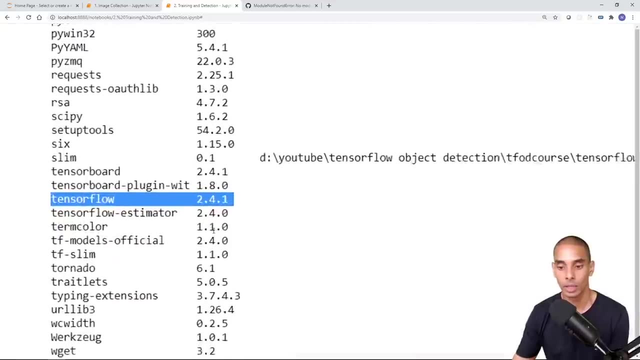 Now remember when I sort of said that if you install tense flow and you want to use your GPU, you got to install some additional stuff. Well, in this case, here we've got tense flow 2.4.1.. So this is the equivalent of 2.4, like falls into the 2.4.0. 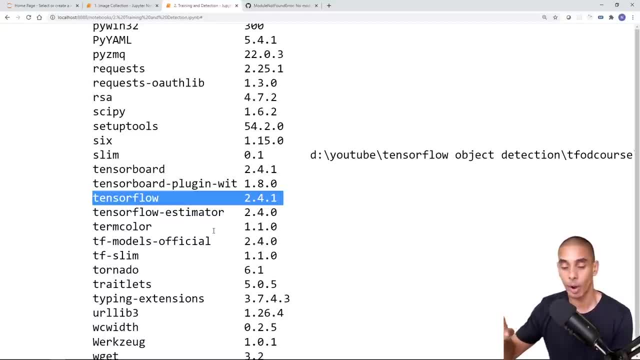 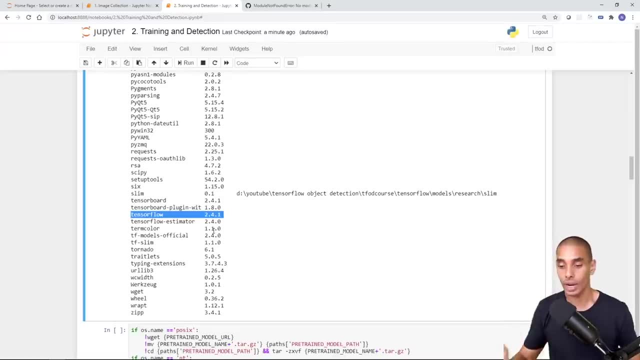 There is tense flow 2.5.0 available at the moment, So you just need to make sure that you find the appropriate CUDA and CUD And then version for that. Now, to do that, what I normally do is I'll go into Google and I'll just search for CUDA. 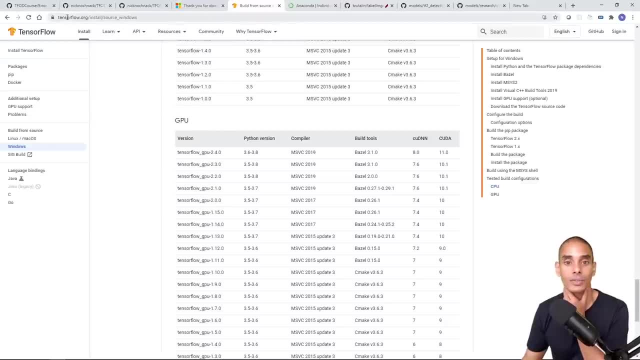 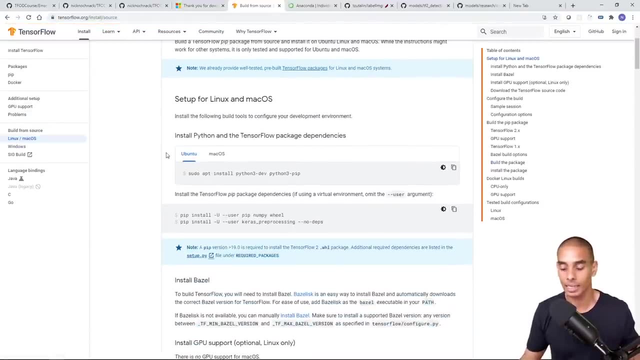 Well, let's take a look at what version we need first. So again, we go to tensefloworg forward slash install forward slash source windows. because I'm on a Windows machine. We could just as easily go back to the Linux and Mac OS page and do that. 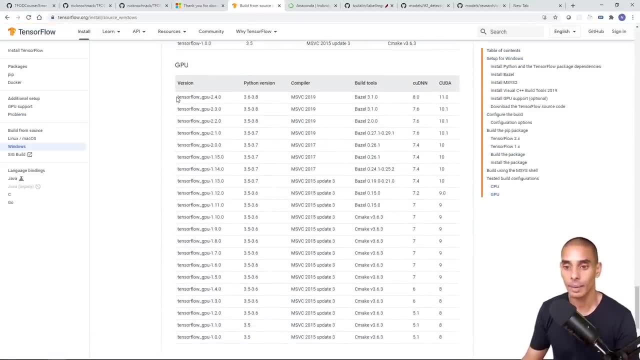 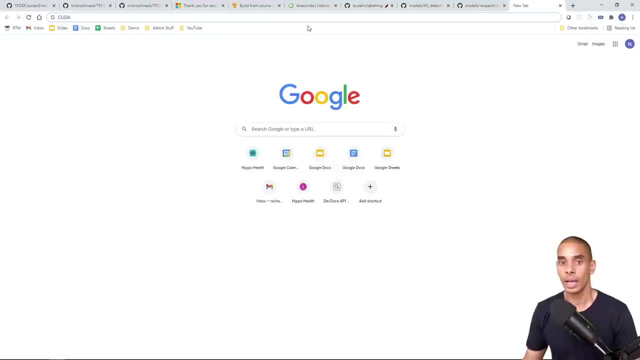 In this case, we're on Windows, So if I scroll down because I'm using 2.4.0,, I need to have CUDAN 8 or and CUDA 11 installed Now. in this case, I've already got it installed, but I want to show you where to get it from. 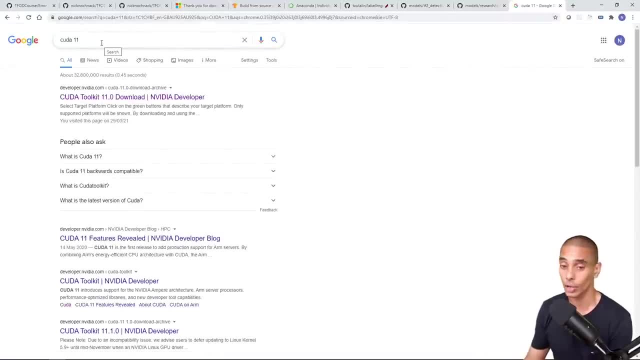 So if we go to CUDA 11, if you just go to Google and type in CUDA 11, you can see that CUDA toolkit 11.0 is available. So if I select that and then I choose my operating system, So in this case I'm on a Windows- 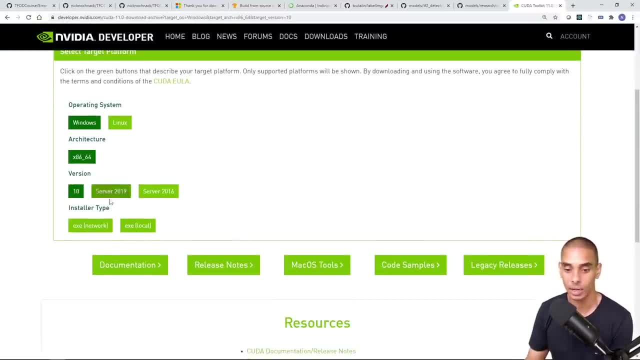 You can choose version- what version of Windows I'm on. So I'm on Windows 10, not server- And then you can choose which type of installer you want. So you can either choose the network install Or a local install which downloads everything. 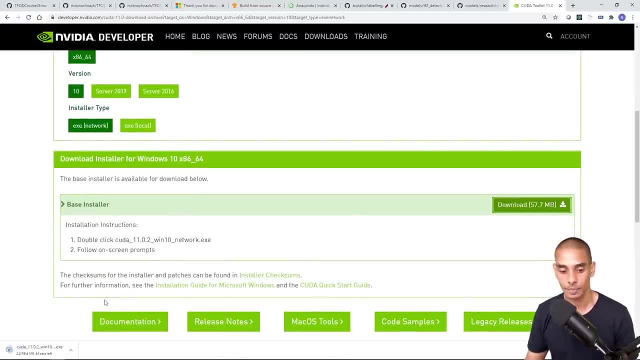 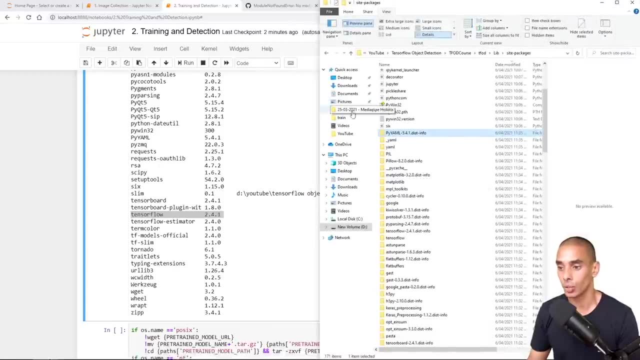 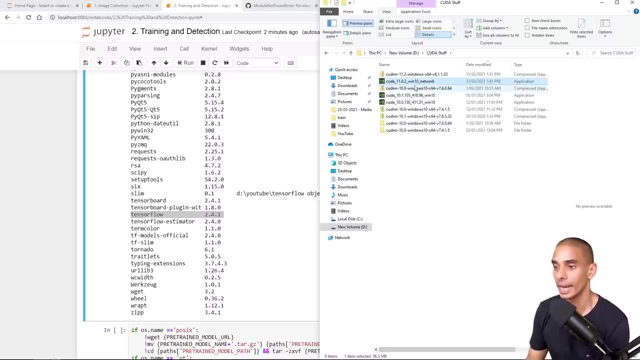 So if we choose network install and then hit download, I've already got this downloaded, So we don't need to wait there. So once you've got it downloaded, you should get a file called this: So you'll get a file. Let me make that a little bit bigger. 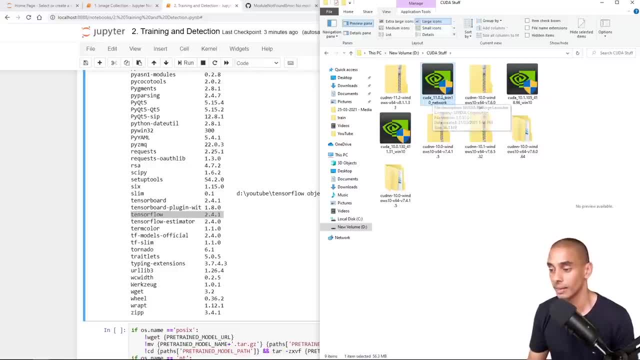 So it's called CUDA, underscore 11.02.. And then in my case it's Windows. So if you actually double-click that, it'll walk you through The package installation And in this case it's going to install into my CUDA folder here. 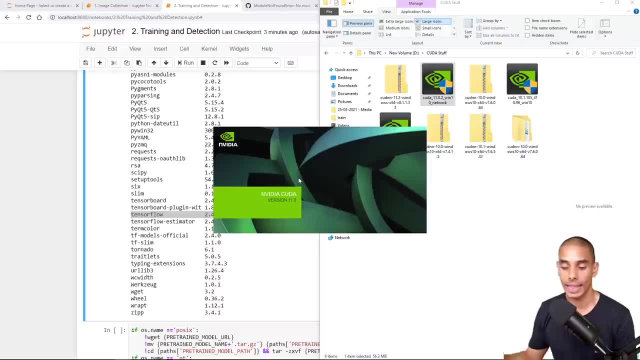 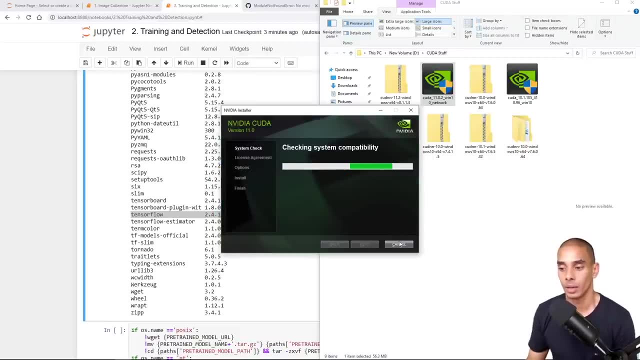 So if I hit OK, And then basically what I do is I just click, click, click and go through that CUDA installation. There's nothing too crazy there, Right? So you just hit next, next, next, no issues. So it's going to install CUDA into your machine. 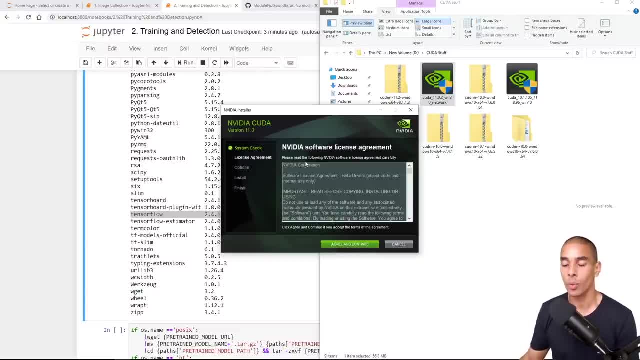 So, rather than sitting through this, I'm actually going to show you the next step. So, once you've gone through and installed CUDA, So again I've got the full install video where I show up from scratch, but basically In a double-click CUDA: install it, walk through the installation. then what you need to do. 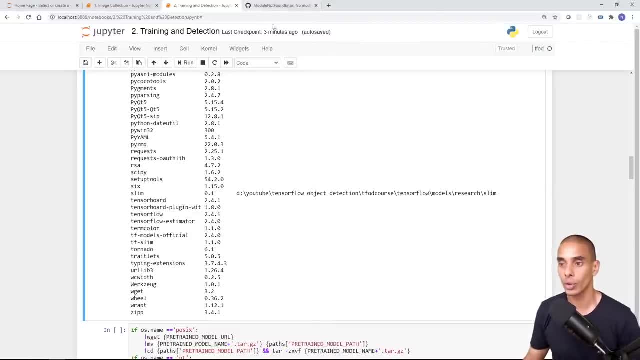 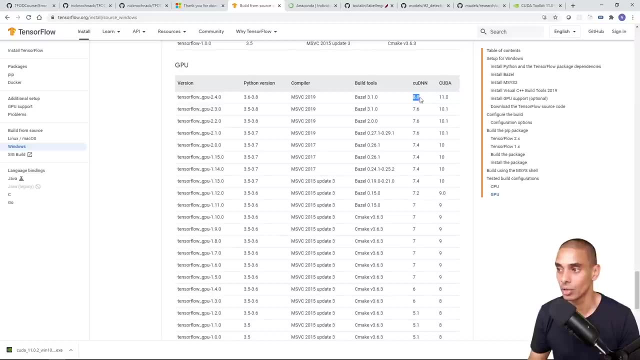 And this is the bit where it is a little bit more tricky. So once you've got CUDA, you then need to get the matching installation of C U D N N, which in this case, here is going to be C U D N N 8.0.. 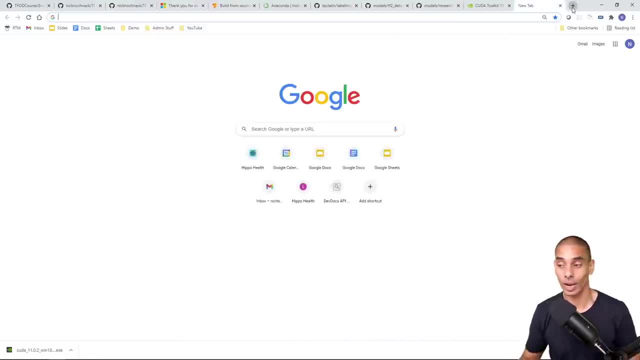 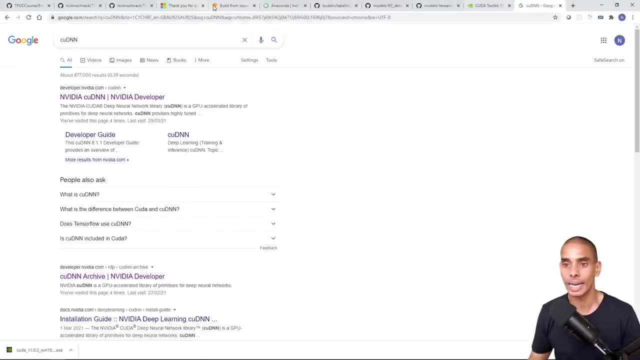 So again, to find that- and I'm showing you how to find it on Google rather than just giving you the direct links, because these are going to consistently change. So if we type in C U, D, N, N and remember we needed, what version do we need? 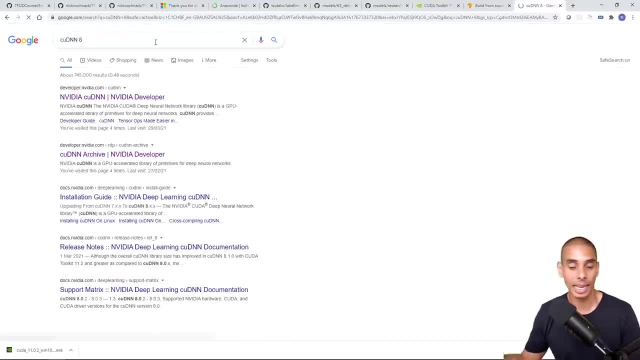 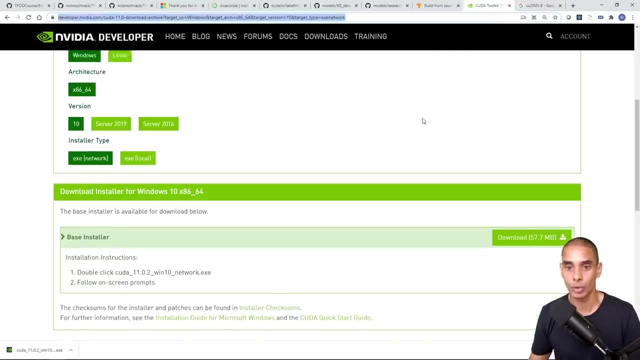 We need eight, So I'm going to Type in C U D N N eight, because, again, these consistently change, And in this case these are going to be available from the NVIDIA site, just as we got from CUDA as well. 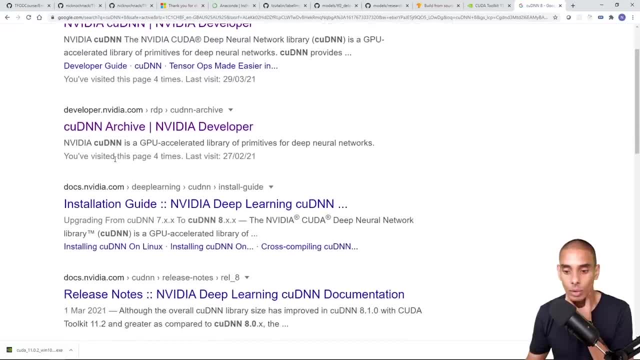 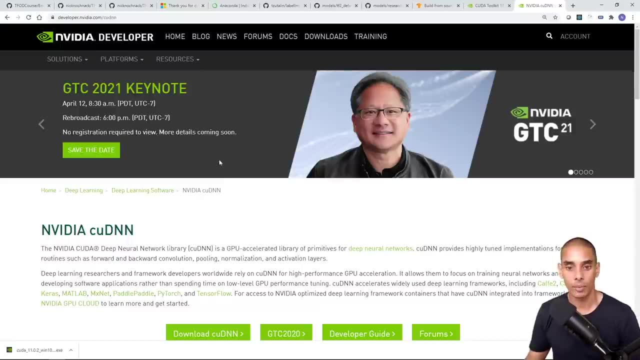 So we're going to go to NVIDIA C U D N N and we're going to look there should be C U D N eight. Let's see what's available there Right So down here we've got a link to GTC. 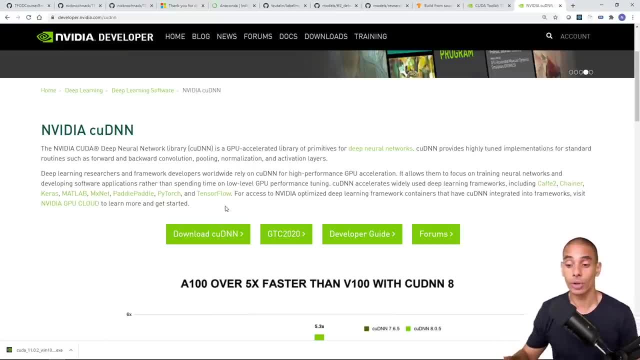 Now we want to download C U D N N Now. in order to do this, or in order to download C U D N N eight, you're going to need A NVIDIA developer account, but it's free, You just need to sign up. 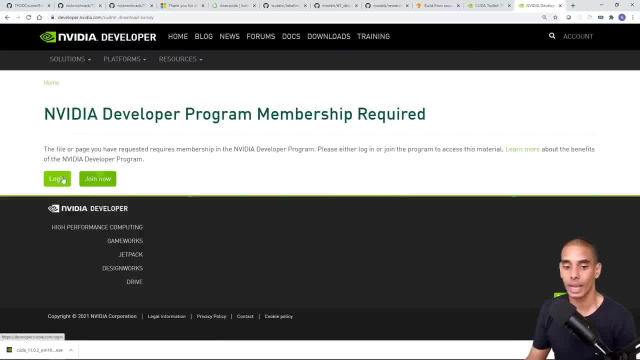 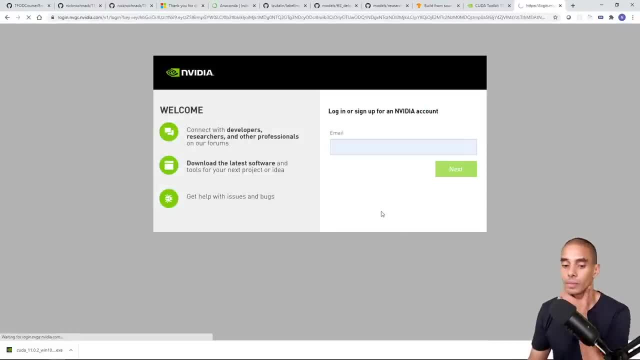 So I'm going to select download, C U D N N, and then we need to log in. So this is why you need the developer program membership. So in this case I can log in And then log in. So do the capture. 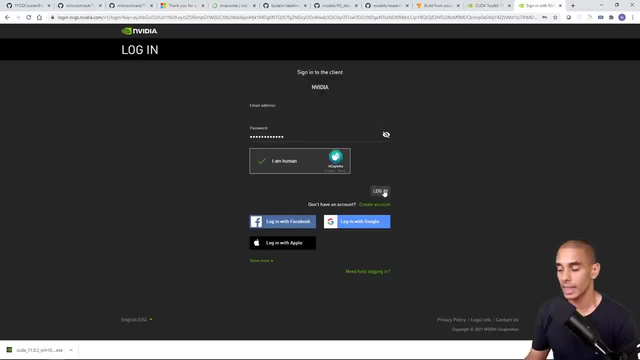 So what are we doing? trucks? And then it should allow you to actually go on ahead and download C U D N? N. Now you do need both, but only if you're training on a GPU. If you don't have a GPU on your local machine, you don't need to go on ahead and do this. 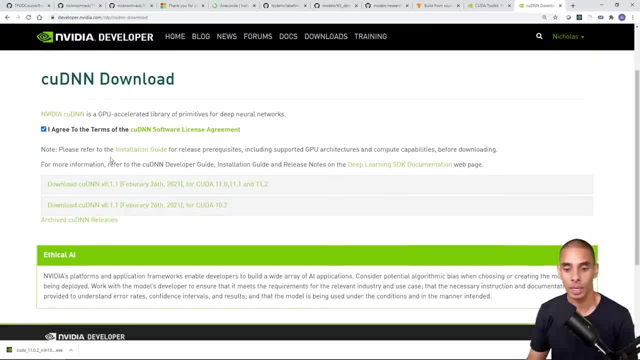 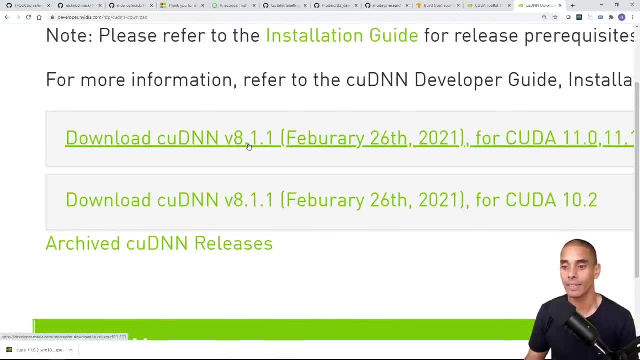 So in order to download it, you just need to hit I agree to the terms And then you're looking for the version that you need. So in this case, there's two versions available here. So there's C U D N N V eight for CUDA 11, and there's C U D N N V eight, dot one for CUDA 10, dot two. 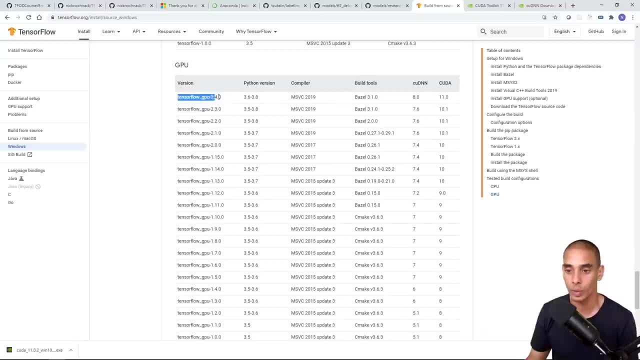 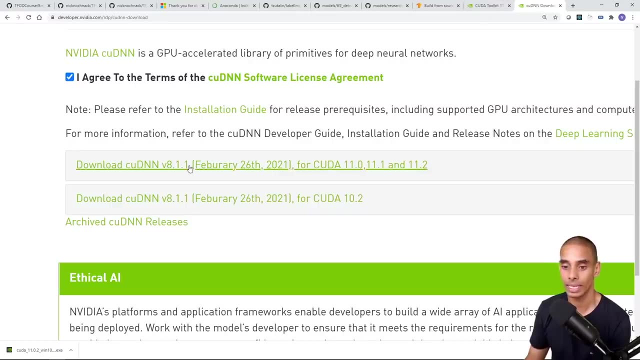 So remember that we had for our particular version of tense flow, which is two dot four dot X, We need C U D N N eight for CUDA 11.. So in this case we Are going to get C U D N N, which I believe. that's V eight, one dot one. 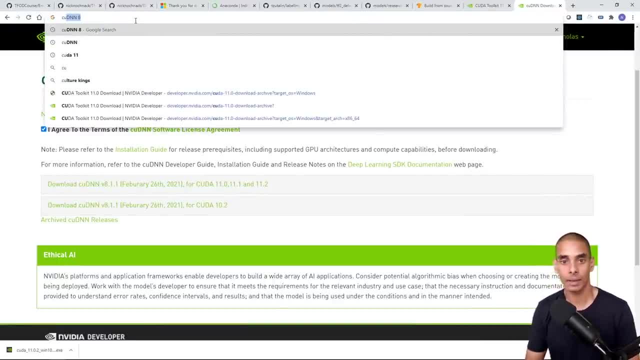 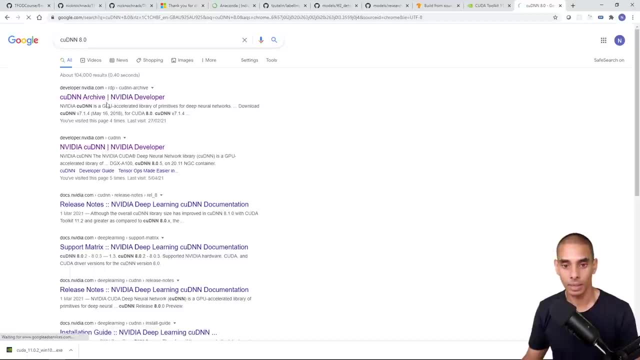 So we actually need to go find a different version, right? So it's C U D N N eight dot zero, And let's find it. So in this case we're going to go to the archive. All right, So this is looking better. 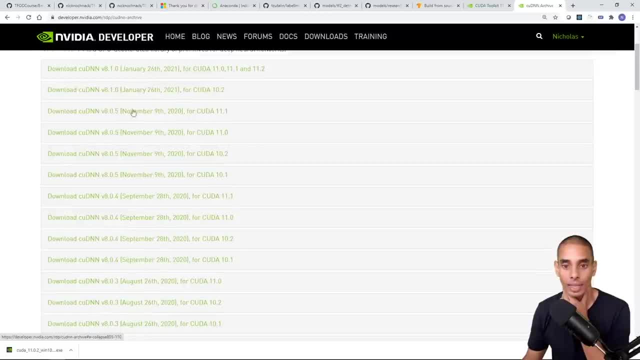 So you can see here that we've got a bunch of eight versions. So rather than having eight dot one again, these are going to consistently come out with new versions, So we need this one. So we've got CUDA 11, which is over there, and we've got C U D N N V- eight dot zero five. 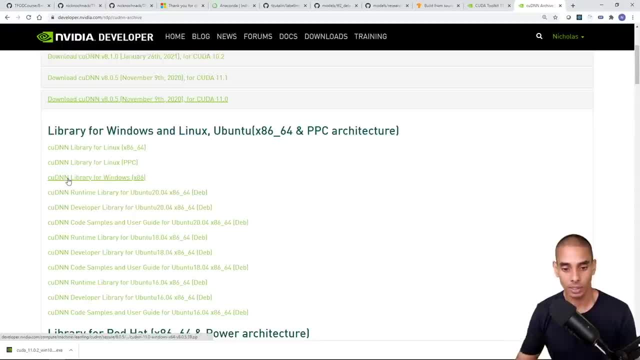 So we can download this. just find the version for your machine. In this case we've got C U D N N library for windows X 86. I can download that And that's going to download. So in this case again, I've already got this installed so we can cancel that. 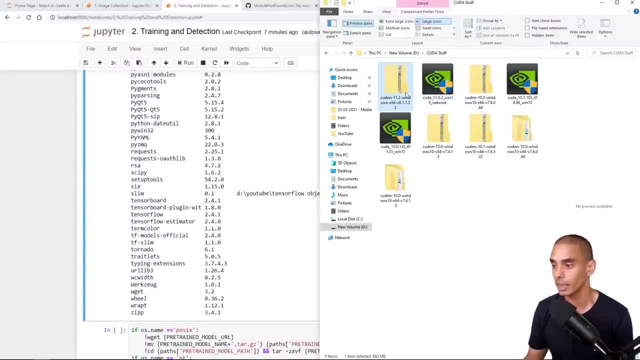 So it's going to look a little something like this. So it looks like I got 11 dot two here. but what do we need? C U D N N. Okay, I guess this one must've worked All right. So it's going to look a little bit like this. 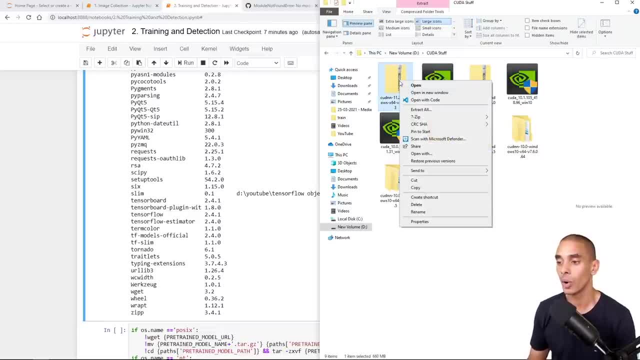 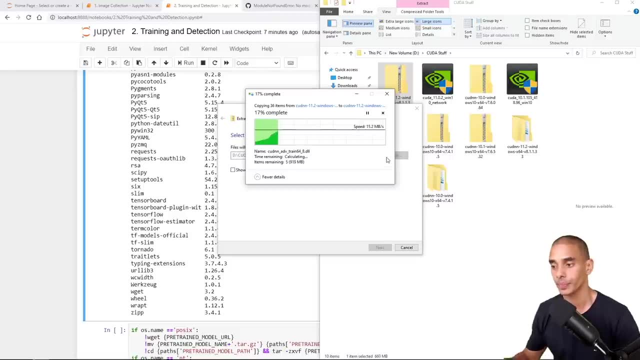 So we've got C U D N N and it's a zipped file, So what you want to do is extract it- And in this case I'm just going to extract it here- And then what we're going to do is we're going to copy the C U D N N files into their respective folders inside of that CUDA installation location. 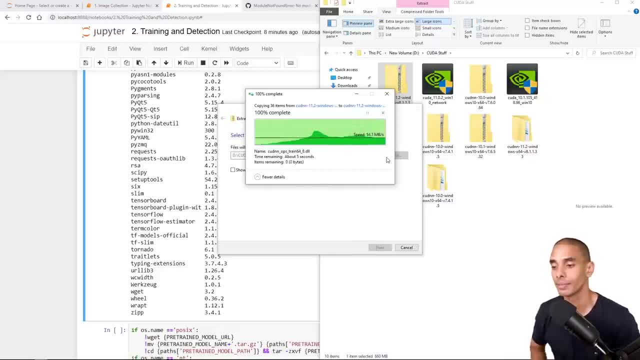 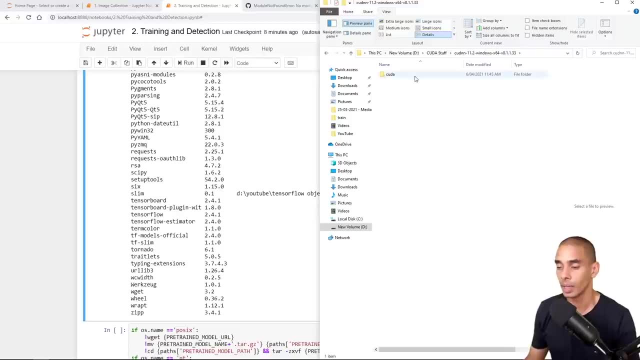 That was probably a bit of a mouthful, But basically you're just copying and pasting stuff. Okay, So we've got our stuff extracted. So which one is it? It's this one here. So if I double click into it now, you can see inside of CUDA. 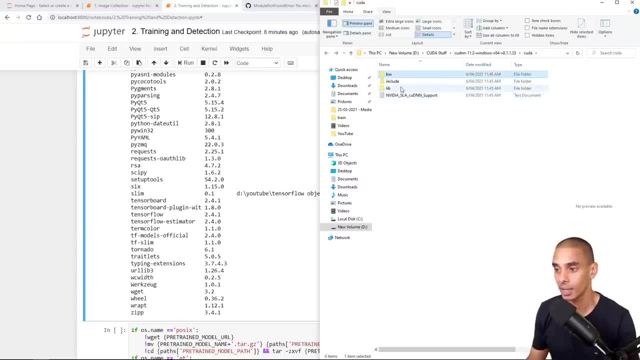 I'm going to have a bin folder which has a whole bunch of C U D N N stuff and includes folder which again has a bunch of C U D N N stuff, and a lib folder which again has a bunch of C U D N N stuff. 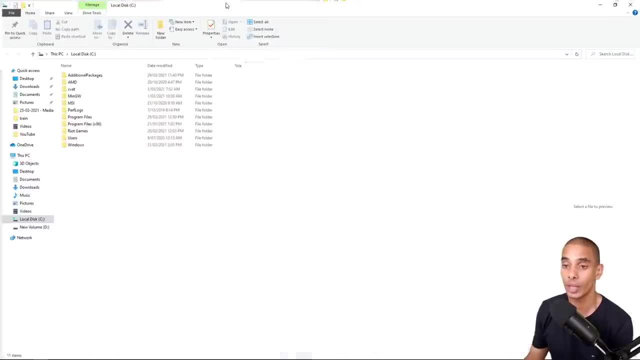 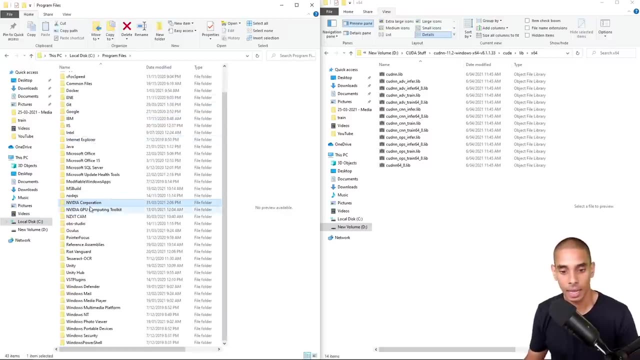 What we need to do is open this or is copy those folders into our CUDA folder. So if I actually show you what mine is, Mine looks like. so if we go and find Nvidia and I believe it's inside of this folder called Nvidia GPU computing toolkit, 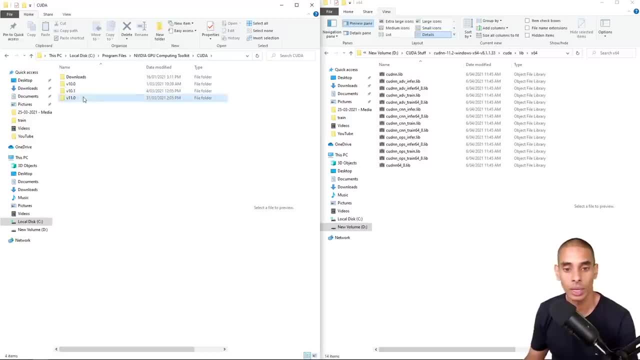 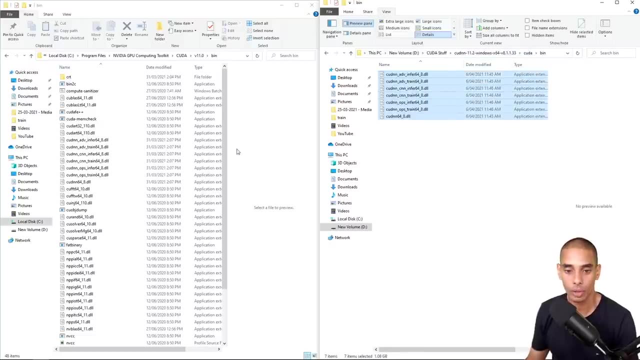 So I've got CUDA and I've got a bunch of versions pre-installed inside of my bin folder. I just copy these bin files, So I'd copy all of those over now. I've already got them done So I'm good to go, but you can see that I've already got these available here. 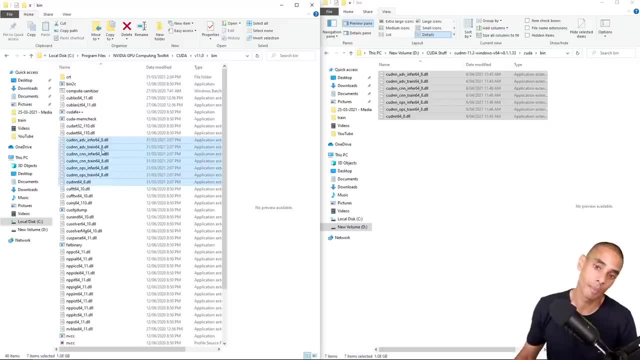 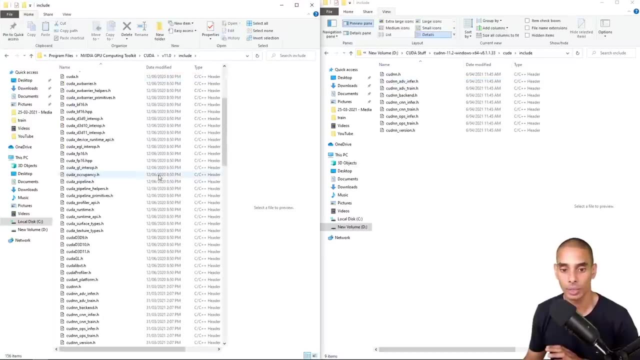 So I've copied these C U D N N files into the bin file inside of my CUDA directory. Again, if I go back I'll have to do it for my include file Again. include, do the same thing. So I've got. they should be in here. 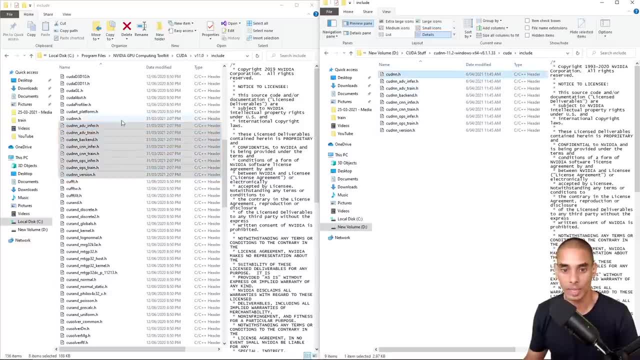 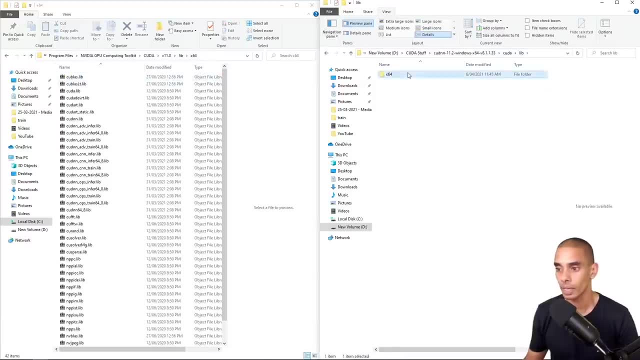 So you can see that I've got all the C U D N N files. Just copy those into here And again. likewise you got to do it for the lib x86.. Lib x86. And again, we're just doing it back into here. 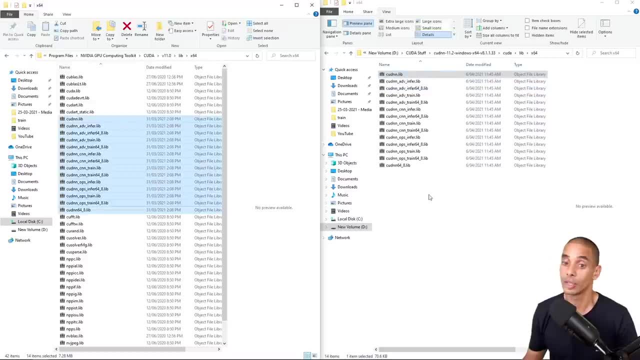 So you can see I've got all of these C U D N N files. Again, I've just copied these over into the respective CUDA folder. So once that's done on your Windows machine, You just need to do one last thing and make sure that it's added to your path. 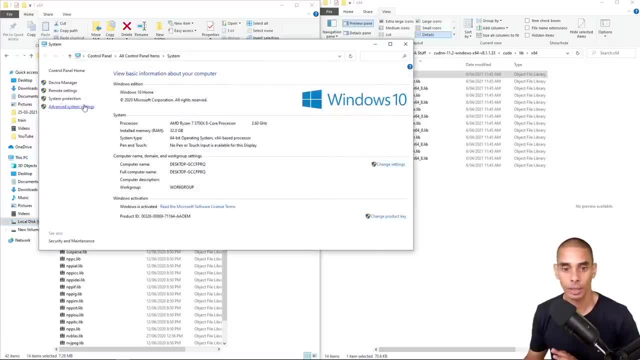 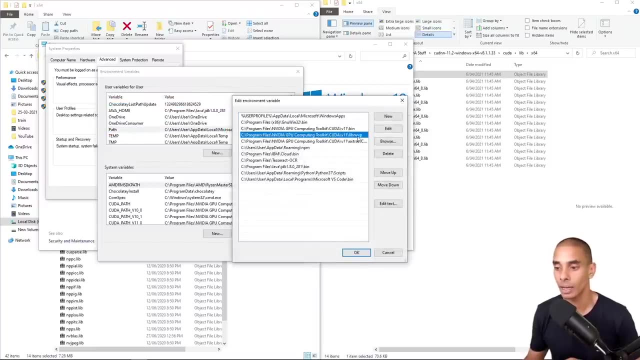 So in this case, if I open up my properties, go to advanced system settings, environment variables- and then go to my path, You can see I've got my bin folder or the path to my bin folder, the path to my lib N V V P folder and the path to my C U P T I folder. 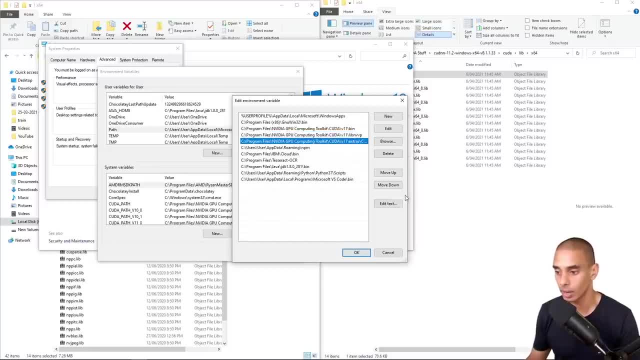 So there should be three. So this one, this one and this one. I don't know. Let's see if we can make that a bit bigger. There you go. So these three file paths are the ones that you're going to need. 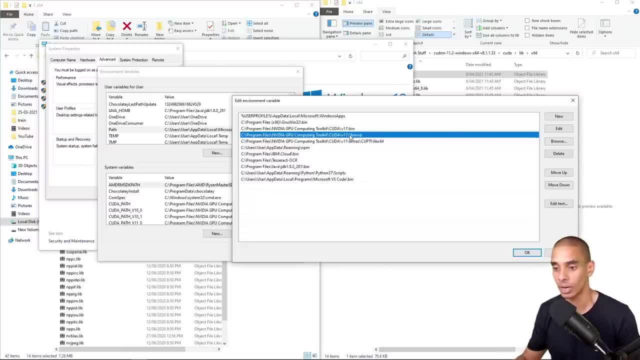 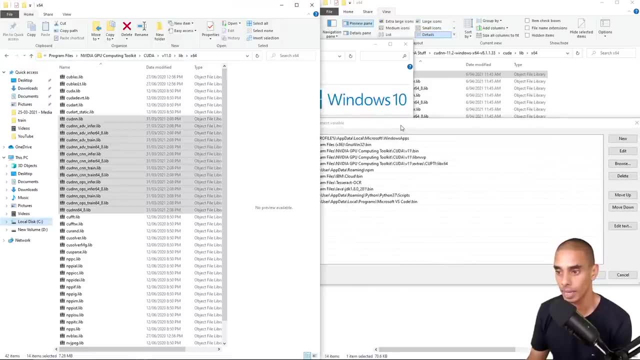 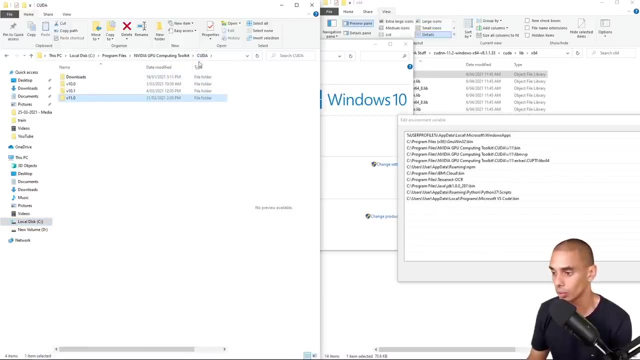 Added it to your path on a Windows machine in order to enable this to work. So, again, this is just pointing to this particular folder over here. So if I go in, let's make this a little bit easier to see. So we are pointing to our so NVIDIA GPU CUDA, CUDA, CUDA, and then see some. 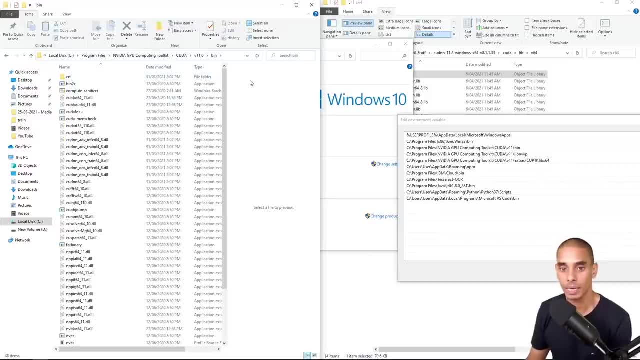 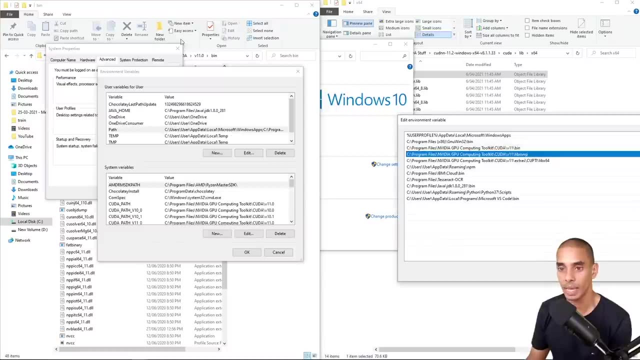 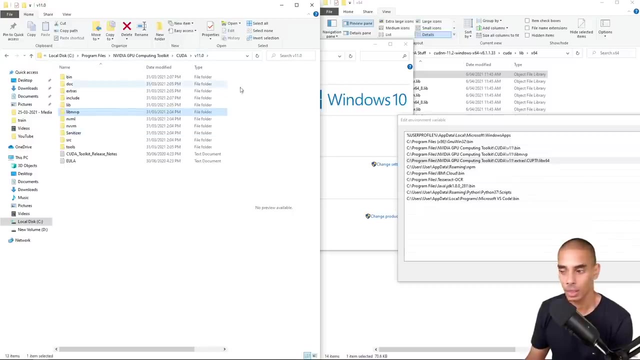 pointing at V 11 and then bin, and then you can see I'm pointing to. so my bin folder, which is this one, my V V P folder, which is this one, And then my C U P T I folder. So if I go back in, so it's under extras C U P T I, then lib XX 86, or that. 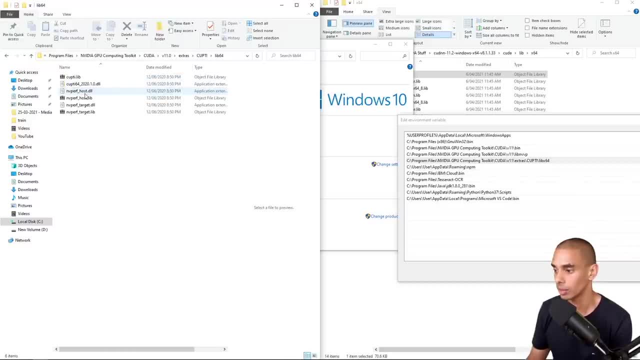 doesn't actually look like that. one's been defined right. That's a bit better. Lib 64. Cool, So that should be all good. But again I'll tell. I'll show you how to check whether or not that's. 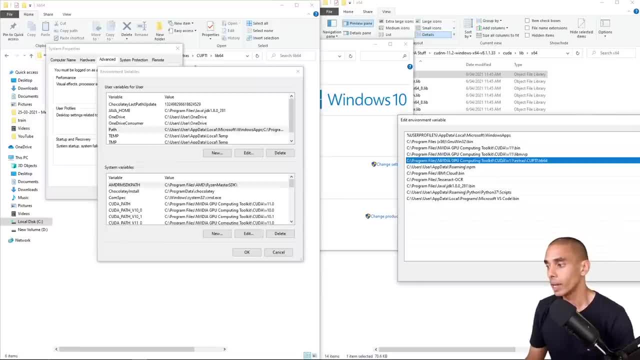 working when we actually go to train. So you'll be able to actually see whether or not it's picking up the appropriate version of CUDA. So that should be all good. But again, I'll tell you, I'll show you how to check whether or not that's. 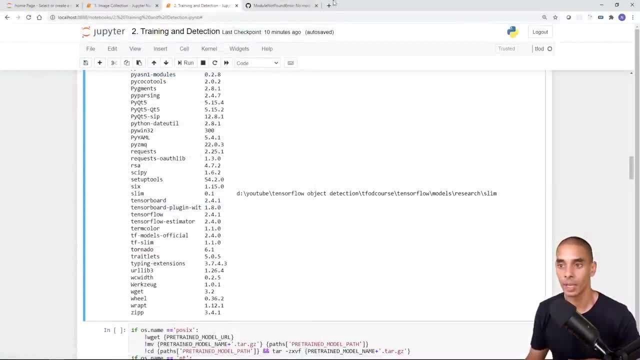 working when we actually go to train. So you'll be able to actually see whether or not it's picking up the appropriate version of CUDA. So that's sort of just an extra in-source step that you need to go through if you want to train on your GPU. 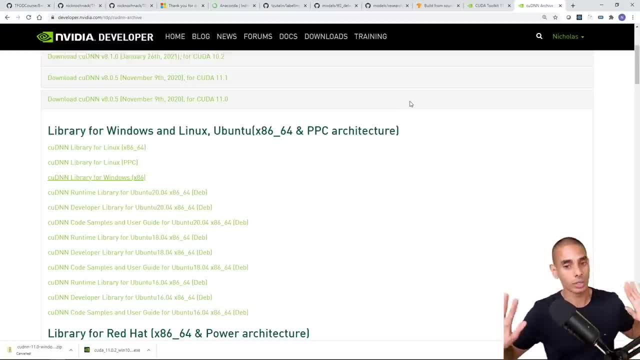 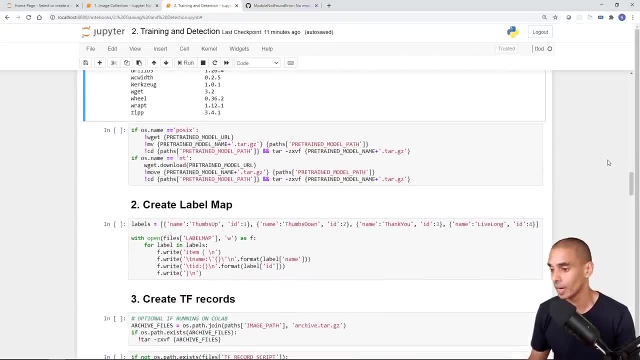 If you don't have a GPU on your machine should be good to go. Don't need to worry about that, But that is our installation done Now. more often than not, that can be a bit of a nightmare process, but you can start to see that there is a flow to it. 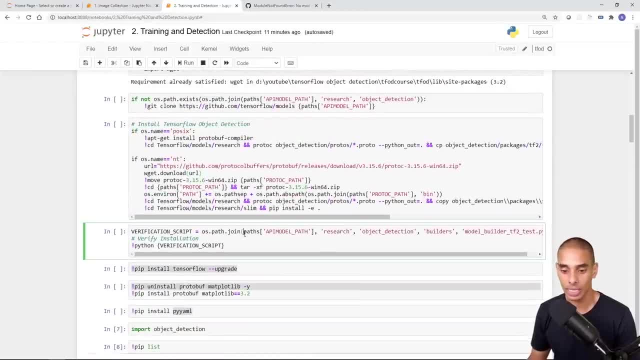 So go through, run through your install, test your verification script and then just keep running through to make sure that you effectively get that okay symbol at the end when you run your verification scripts. So again, we can actually run that. So let's run this again. 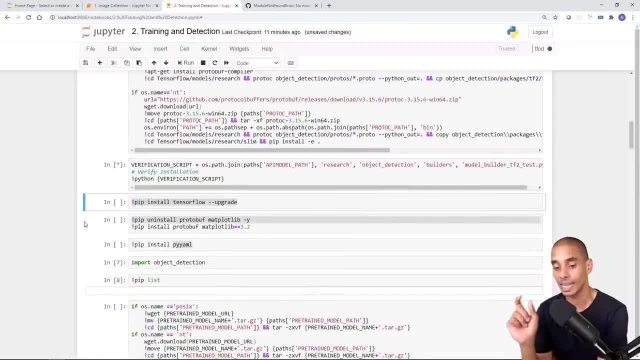 And ideally what we should get is that okay symbol or that okay status right at the end, even though it's in bright red. As long as you get the okay at the bottom, you should be good to go. So let's run this. 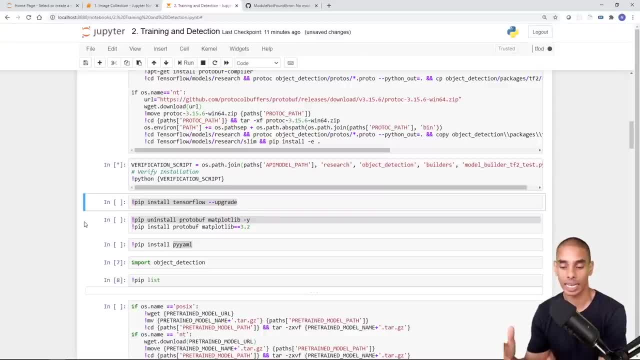 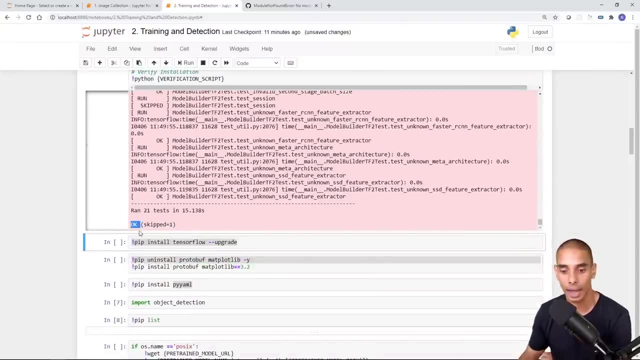 And keep in mind, we restarted our kernel So even though we restarted, we should still see that okay, pop up And again it looks like it's okay. So we're inside of our virtual environment, We've got our okay status popping up. 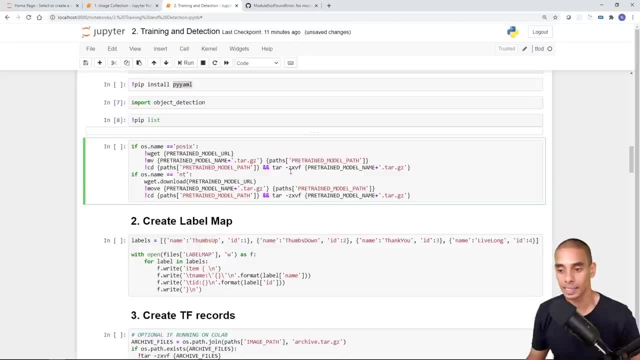 We're good to go, All right. So let's see if we can get that up to this cell down here. So this cell over here is actually going to download our model from the TensorFlow model zoo. So if we cast our minds back, our TensorFlow model zoo was this one over. 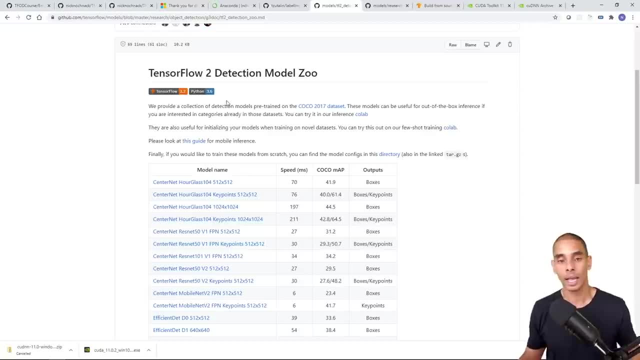 here. So, remember, we've got a whole heap of models that we can already use for our training. Now, the reason that we do this is because, one, we get a state of the art architecture that we can use And, two, we're going to be leveraging a technique called transfer learning. 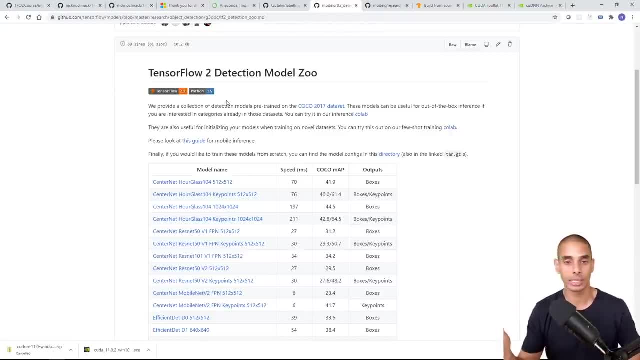 Now, out of the box, we can actually use these models to do some kind of standard object detection. so this is detecting just generic objects, so a phone, a bottle, a towel, so on and so forth. what we're going to do is we're going to leverage what that machine learning model. 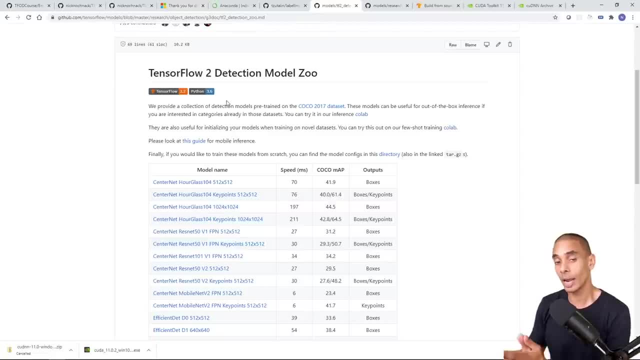 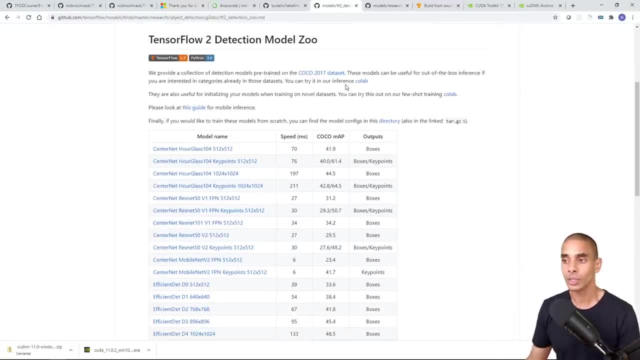 or what that deep learning model already knows, to be able to transfer that knowledge over and detect custom objects. in this case, we're going to be detecting our different hand poses right. so the reason that we're using that architecture is mainly for those two reasons. now what we're going to do is we're going to run this cell. 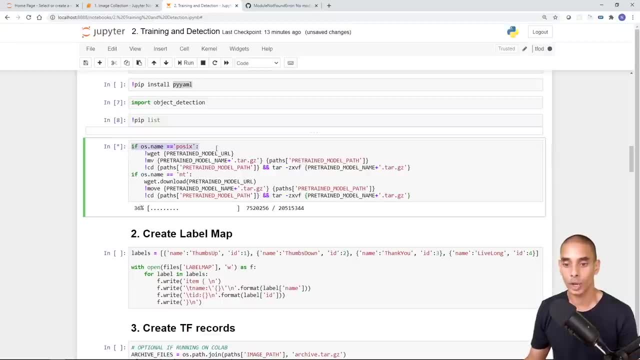 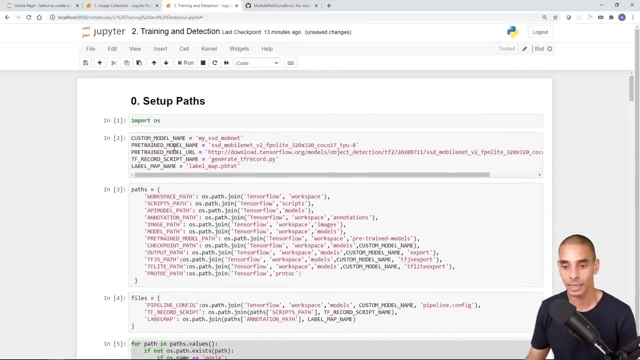 and again it's checking which operating system we're in. it's then using wget to get it from our pre-trained model url, which is what we defined up here, and i'll show you how to do a more sophisticated or a different model once we get to our performance tuning section. 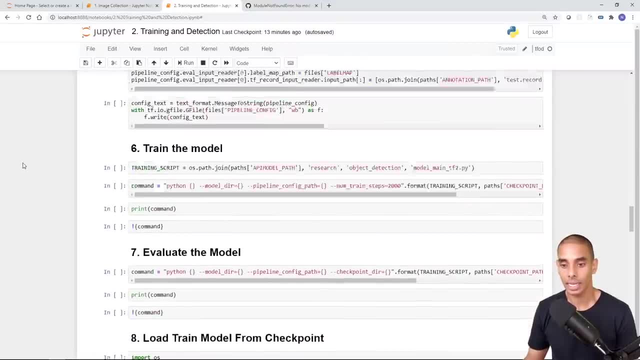 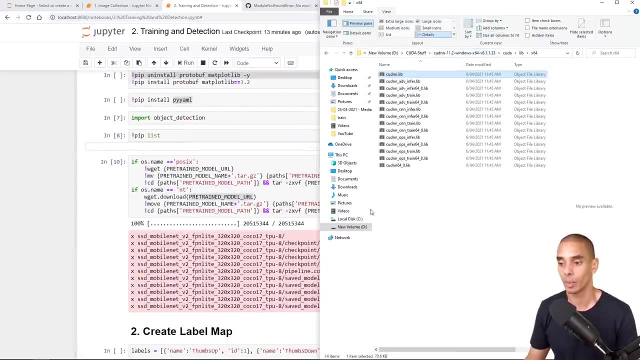 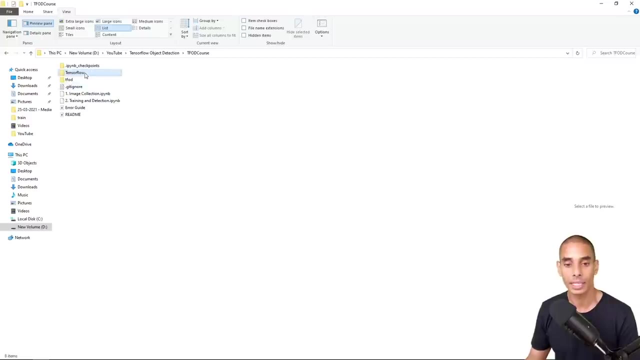 so now that that is ideally what should happen is that this particular cell over here is going to clone down that model from tenseflow, model zoo, and it's going to be able to do that and paste it or put it inside of a specific folder. so if you're going to tenseflow workspace, 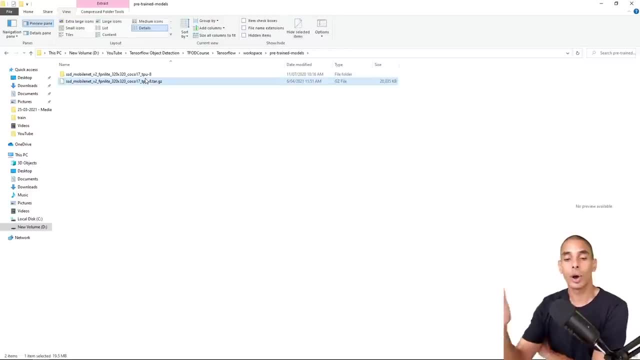 pre-trained models. you can see that it's actually gone and cloned down that model into that specific folder and this is why i defined the name of that folder earlier on, because we are actually going to be leveraging all of the stuff that it's in here. so inside of that folder, let's go back. you're going. 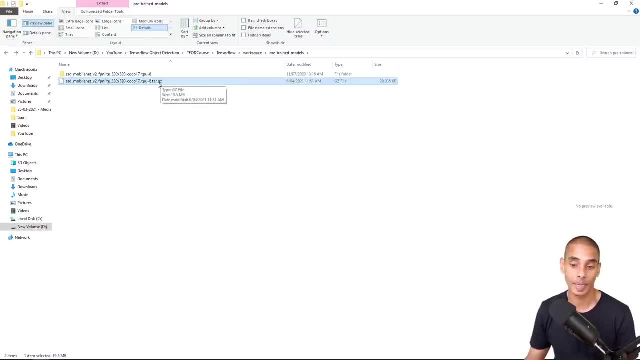 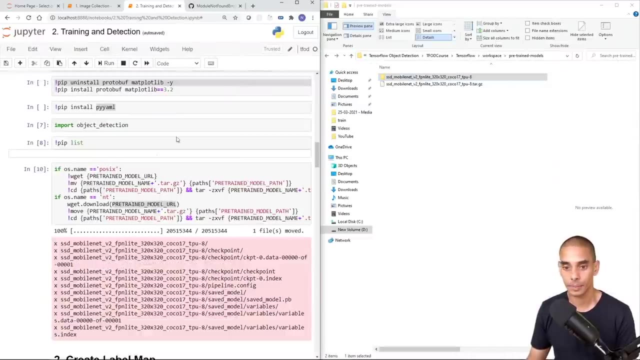 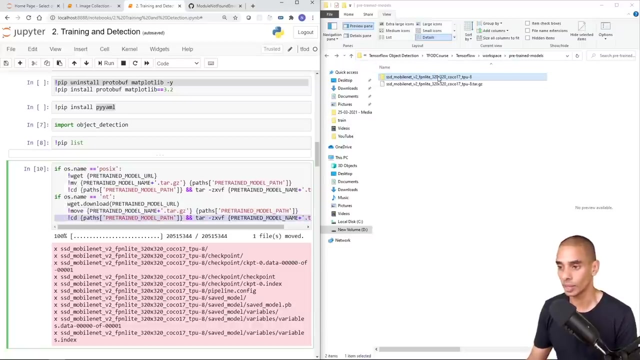 to have the cloned repository. so in this case it's just copied down the compressed file. it's then untied that file. so that is. let me just bring that over here. it's then untied it, which is over here, and it's also moved that particular file into this workspace. so now you should ideally have all. 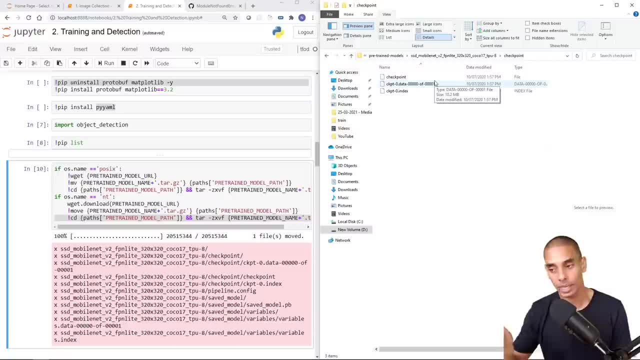 of this. so you've got a checkpoint folder which contains all of the different checkpoints for your file. think of this as the different saved components to your model or the pre-trained model. you've got a saved modelprotobuf file and a variables file. so, again, this is everything that. 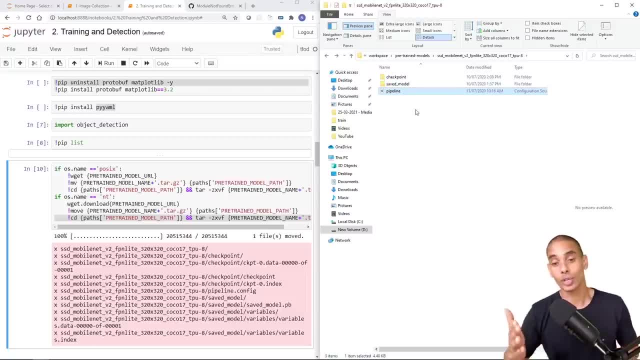 you get when you actually freeze your model- and again i'm going to show you how to do that in a bit later on- for your own custom model as well. but just think of this as your pre-trained model that you're going to be able to leverage for your custom object detection. so that's good now. now the 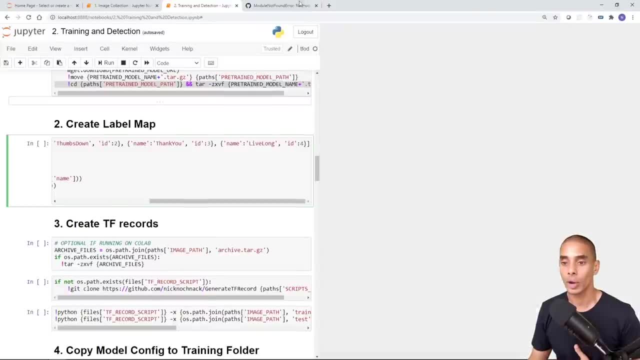 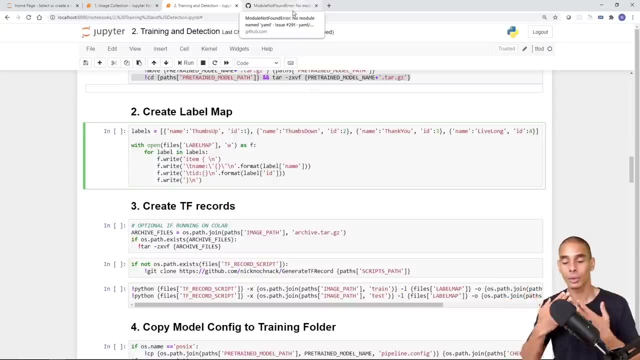 next thing that we want to do is create something called a label map. so a label map effectively represents a map of all your different labels. so remember, we had thumbs up, thumbs down. thank you and live long. now i've already got these written here, right? so i've got thumbs up, thumbs down. 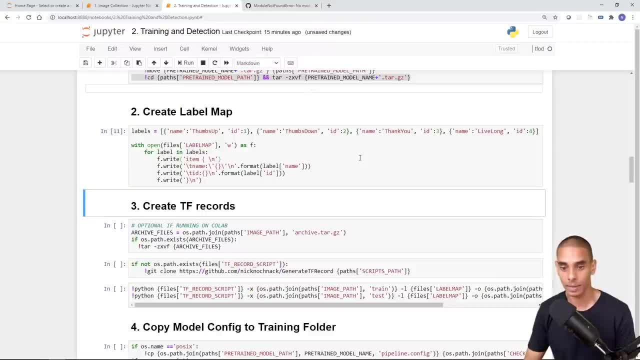 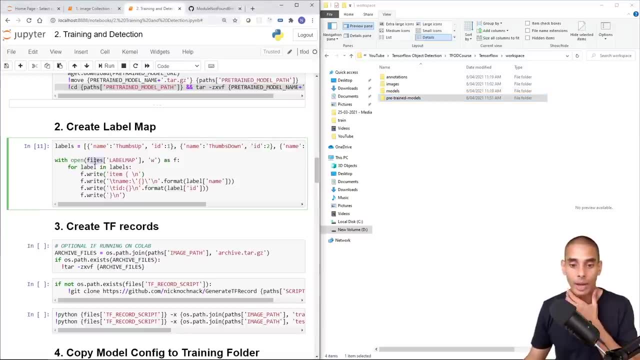 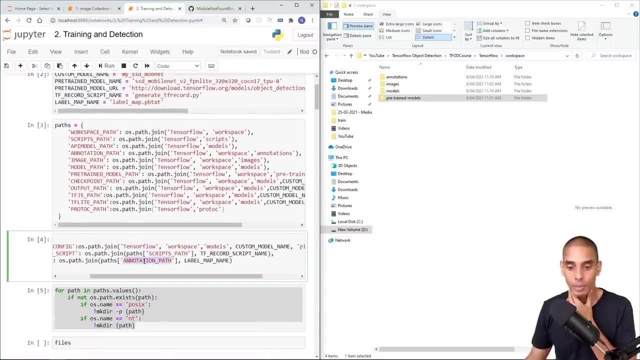 thank you and live long, so let's go ahead and run this. this should run successfully, so no errors there. so if we go into our workspace, so this is going to be written into our files- label map file, which was defined over here, so it's going to be inside of annotation path and then the label map name and our annotation. 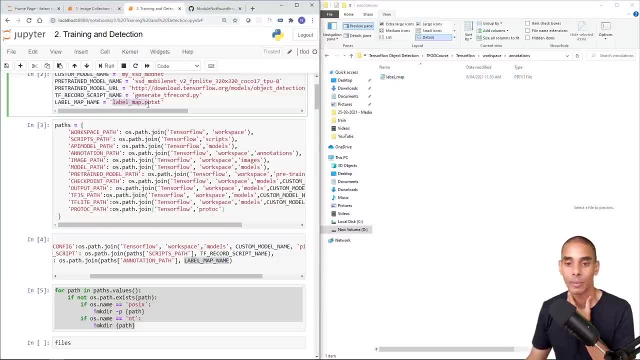 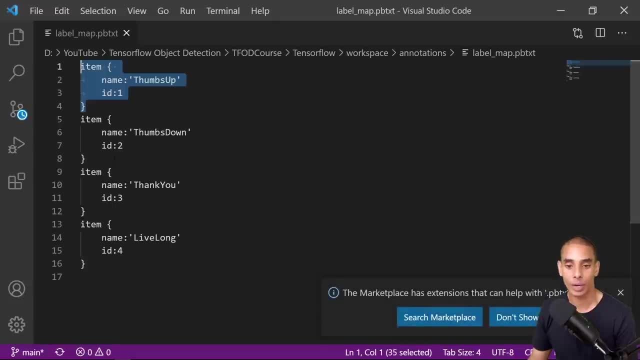 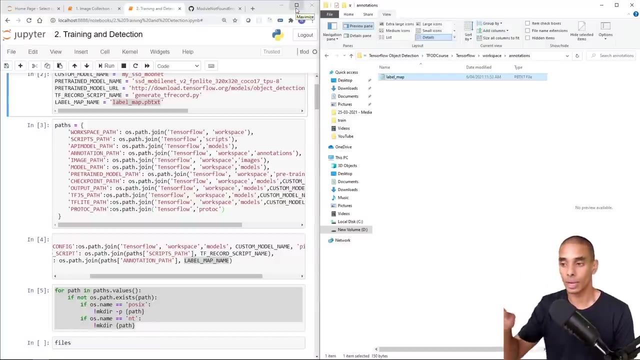 path is annotations and then our label map is named label map and or dot pb text. so if we open this up, you can see we've got a item for each one of our objects. so thumbs up, thumbs down. thank you live long now remember when i said the case was really, really important. this is why. so when we go, 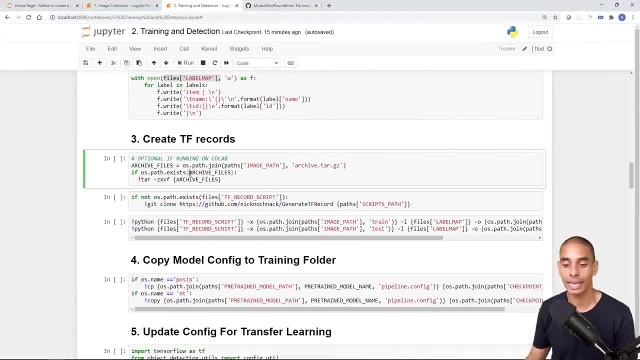 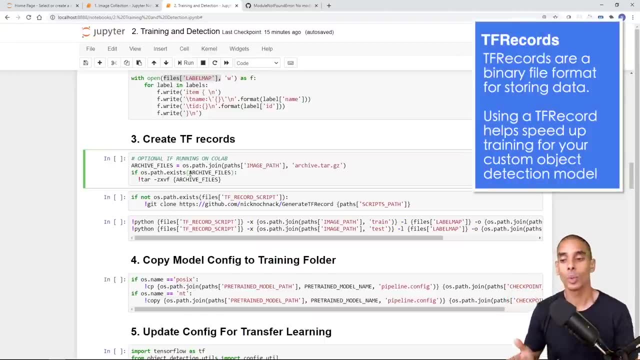 the next step that we're going to normally run through is actually creating our tf records. so what this actually does is it creates a file format, which is called a tf record, which is available to be used to actually go on ahead and train your object detection model. 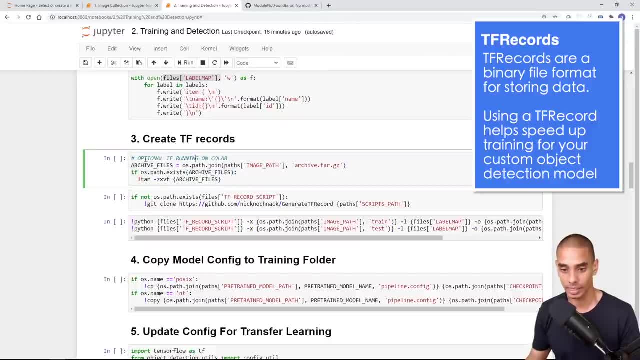 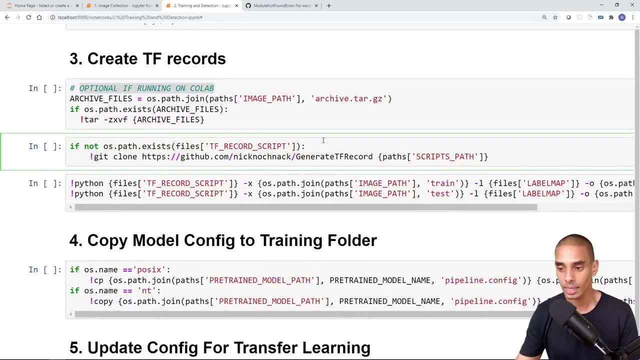 so if we go into these next two lines, so you can skip this one over here. so this is only used if you're training on colab. so if we go and run this tf record script which is there, this is going to run a or clone a file from my github which is called generate tf record. so let 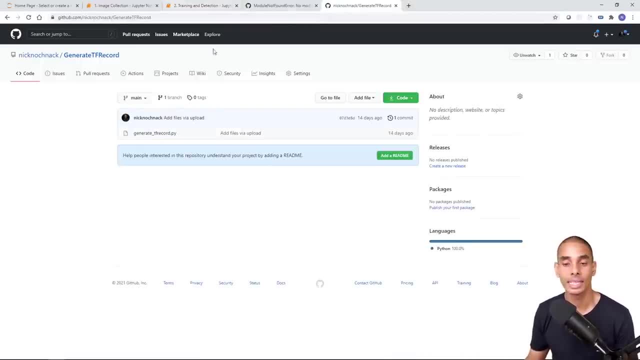 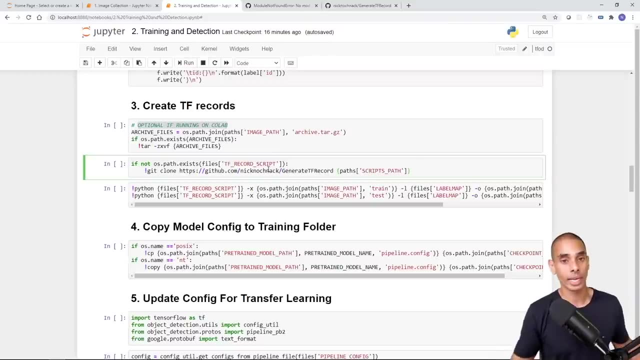 me show you that. so it's going to clone this file and this is the file that generates your tf records. again, you don't need to go into a great amount of detail for what that actually does, just know that it's converting your annotations in your images into a file format that it can use. 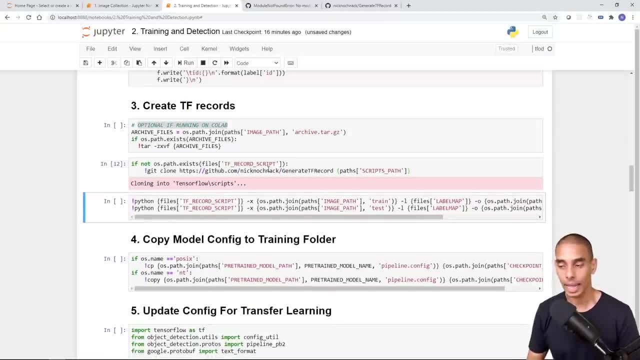 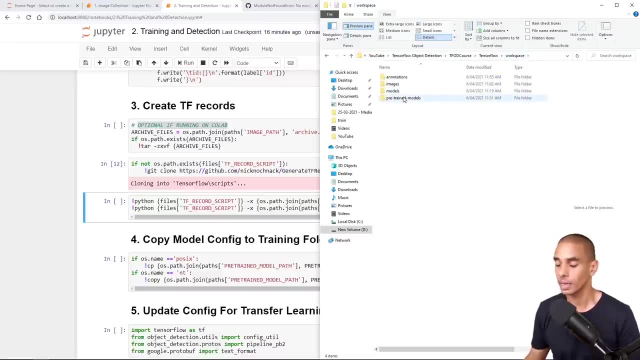 so if i run this cell, it's going to clone it down and then you should ideally have a file. so if you go into workspace and then where is this? this is intense flow. sorry, scripts should get that file. so generate tf record or generate underscore tf record. so that's now. 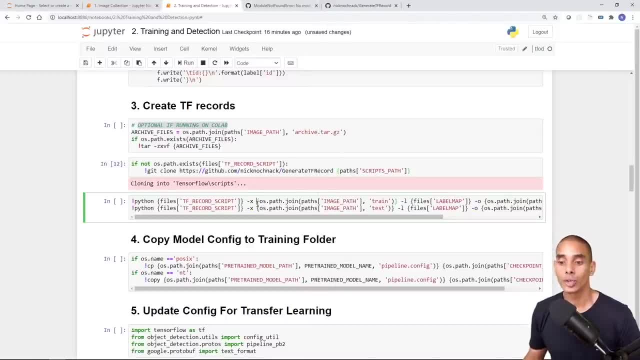 available there. now what we're going to do is run this file here, so i'm going to show you once running without errors, and then i'm going to screw up our label map to show you why the case is so important. so if i run this, oh, it looks like we've got another module error. so in 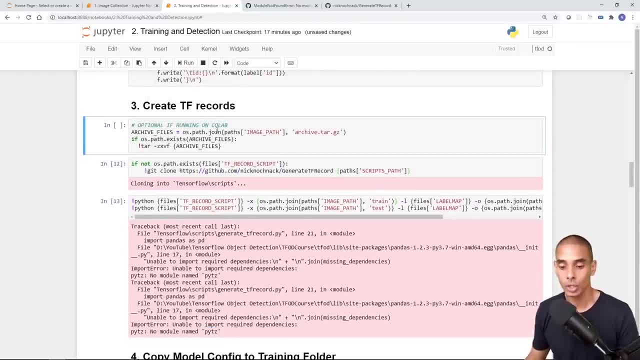 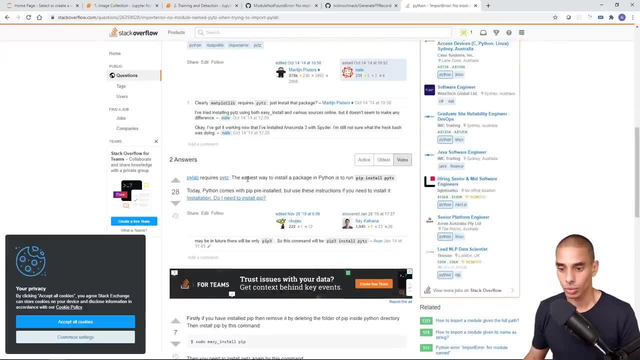 this case we've got a module error. so what do we do when we've got a module error? just go install crushed design. so again, i've done that before. let us go ahead and install that. so it looks like it's pytz. so let's check how to install that. do, do, do, so it looks like we. 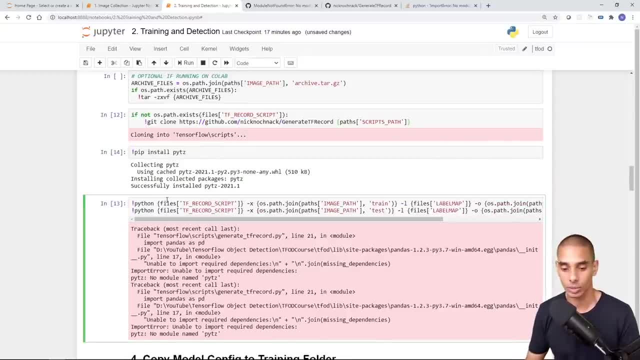 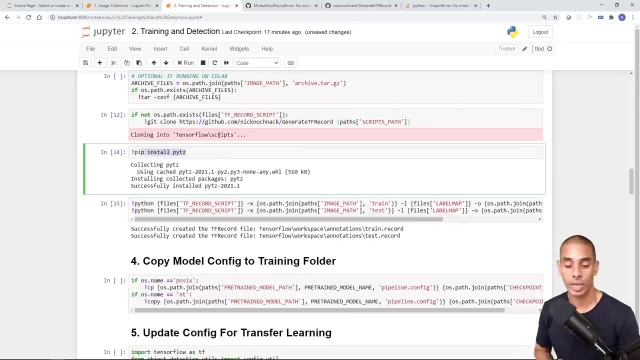 just need to pip installivel python, install pytz. so let's go ahead and do that. so again, if you get any of those no module errors, you just need to install it. see if that runs now. okay, that's looking like it's running successfully. so again, to solve that error. it was a no module error, so to solve that, we just install the module. 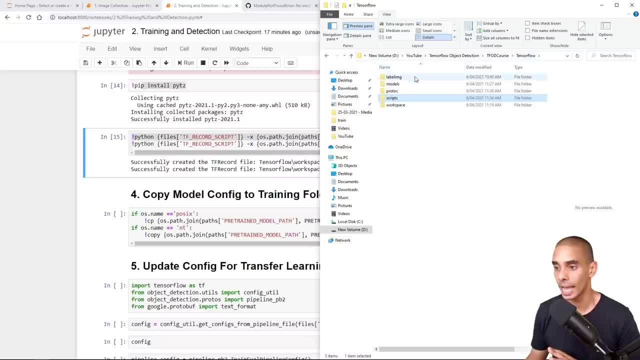 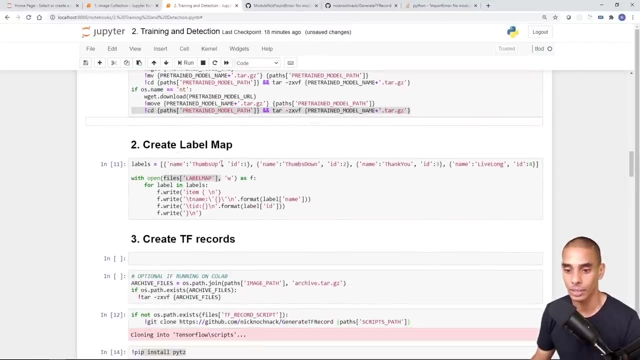 run our tf record script. what it's actually going to do is go on ahead and create. so if we go into our tense flow workspace annotations file, we've now got a train and a test record. so these are what are going to be used to actually train our model. now, if i screw up our label map right. so 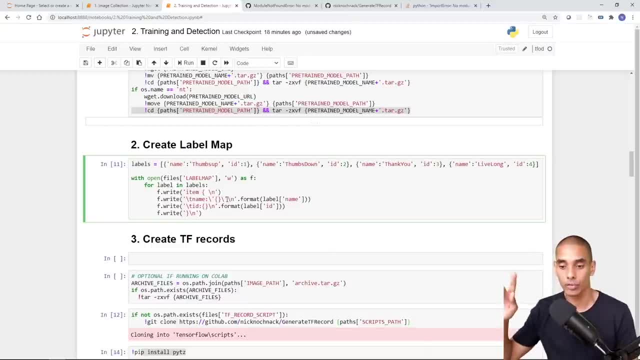 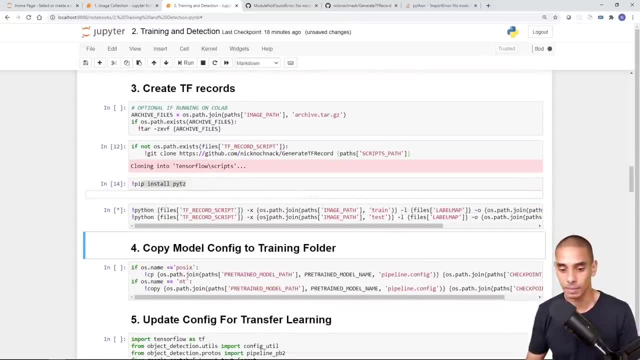 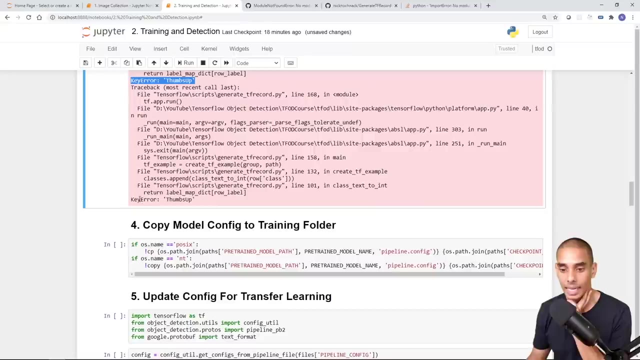 say, for example, i take off the capital u from our thumbs up label. this is going to screw up that generation. so if i go and run our generate script again, watch this so you can see that we've got this key error. so key error thumbs up and then key error thumbs up. so this is because we have 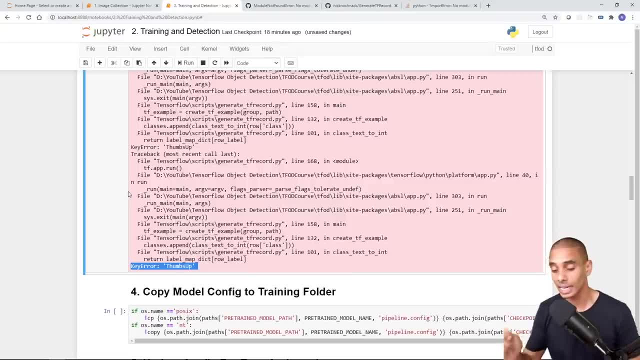 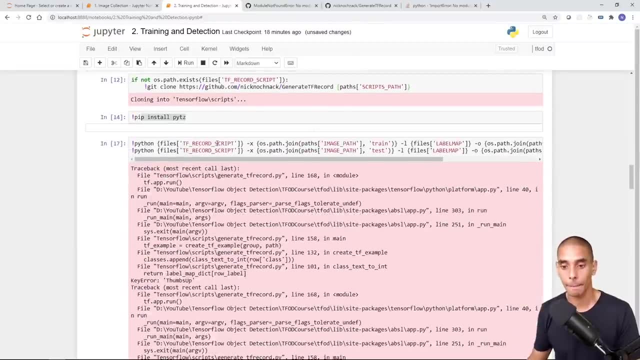 included the incorrect label. so it is case sensitive. so you need to make sure that the case is correct. so if i go and fix that up now and change our label name to thumbs up and rerun that again, so this should now run successfully and again, no issues. 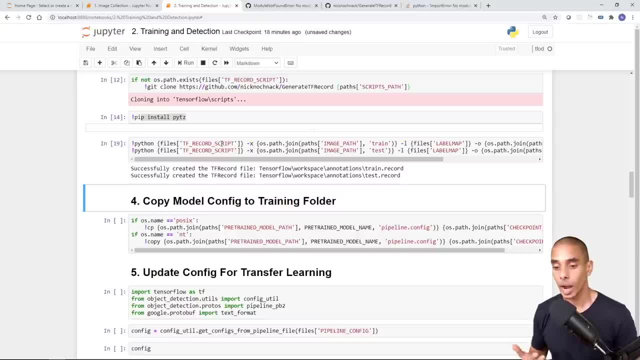 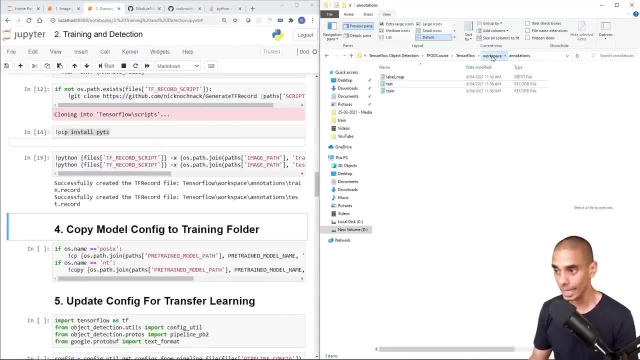 cool. now the next thing that we're going to do is pretty straightforward. so now what we're going to do is just go and copy our model config. so our model config is so. remember, there were a bunch of different types of- let's just close- this and this and this. so there are a bunch of different types. 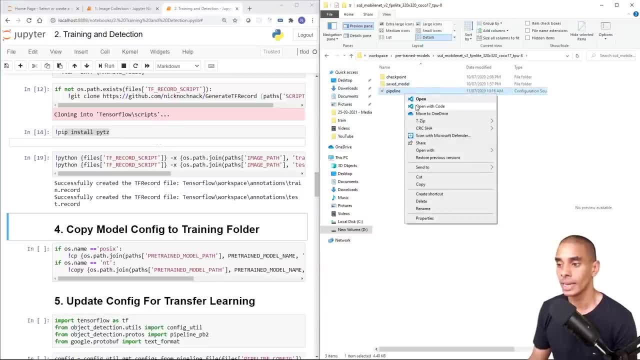 of models inside of our tensorflow model zoo. now the pipeline config is what controls what your model actually looks like. so if i go into, let's start from the start. so, tensorflow, so we're going to go into our tensorflow model zoo and we're going to go into our tensorflow. 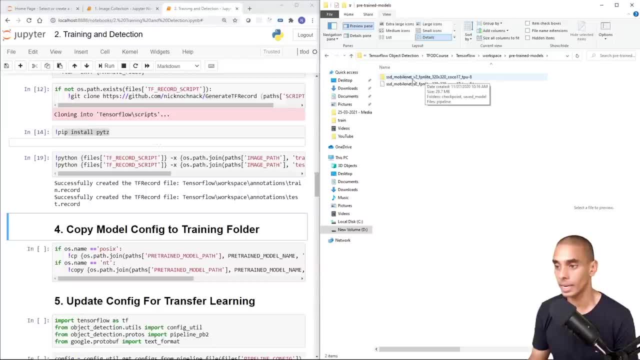 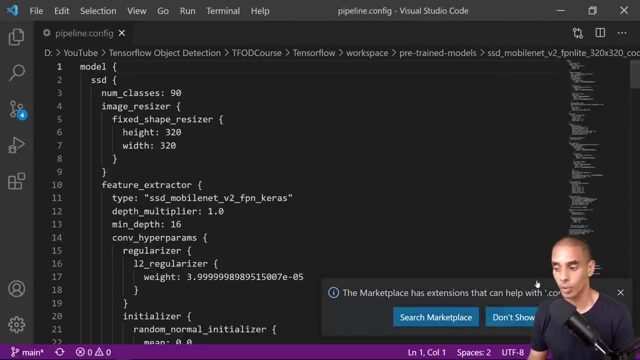 workspace pre-trained models: ssd mobile net. underscore v2. underscore fpn light. underscore 320 by 320. underscore coco 17. underscore tpu8. this pipeline file over here is what defines the architecture of your model and what it actually looks like. now what we're going to do is we're. 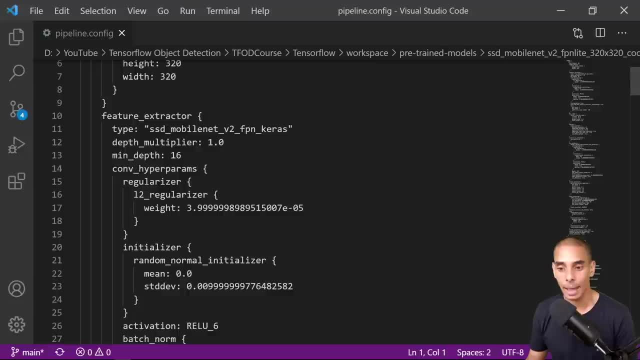 going to customize this for our specific model, but this sort of gives you a baseline. so in here you're going to have the number of classes, you're going to have that image resizer which i was talking about. so remember, that's going to be the image resizer, and then you're going to have the 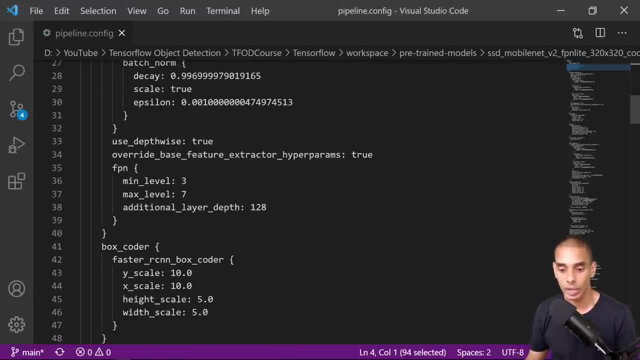 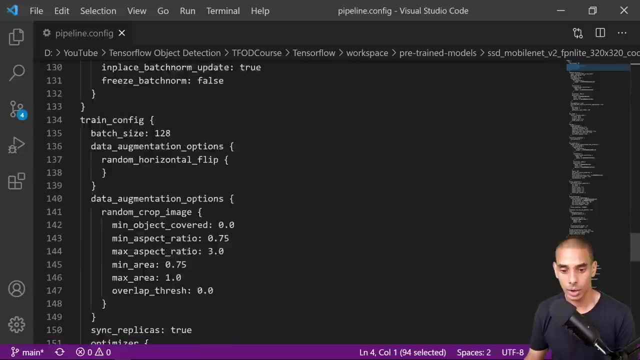 number of classes. you're going to have that image resizer and then you're going to have the remember. it resizes it 320 by 320. your feature extractor- one that i particularly like- is post-processing: no data augmentation. so you can see here that it actually does your data. 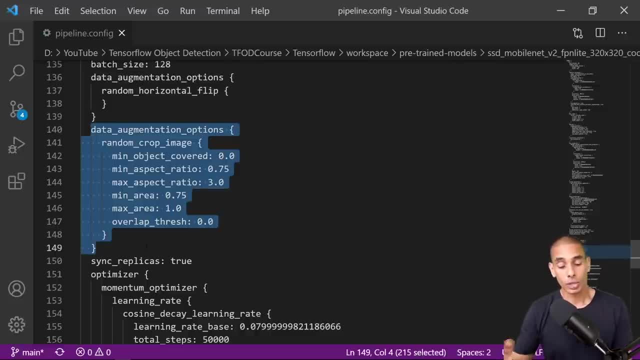 augmentation for you. this is important because i'll show you in some of the other models later on. you'll get a slightly different data augmentation architecture. this is just important to note that it gives you some pre-built data augmentation inside of your model. if you scroll down, you can see that it's got a little bit of a different architecture. so if you scroll down you 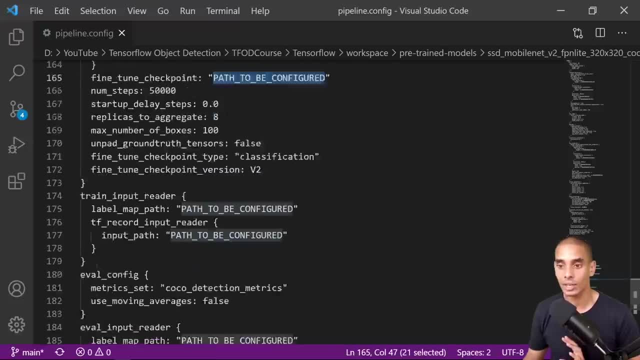 can see that you've got all of these paths to be configured components, so we actually need to update these with our components for our model. so we need to update fine-tune checkpoint. we need to update our label map path, our input path, our label map path and our input path, our. 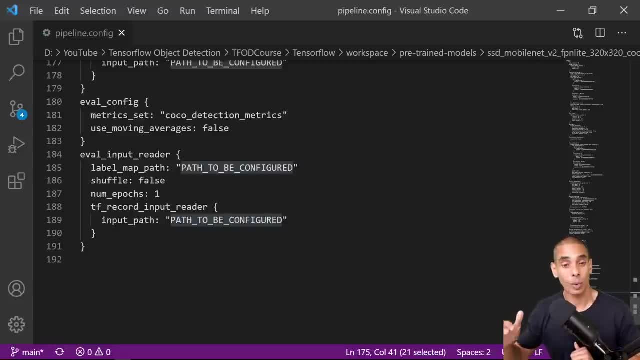 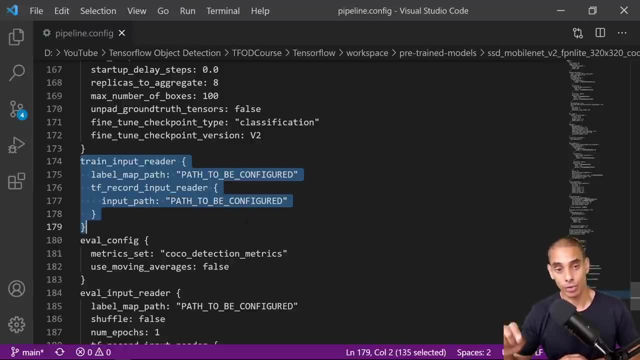 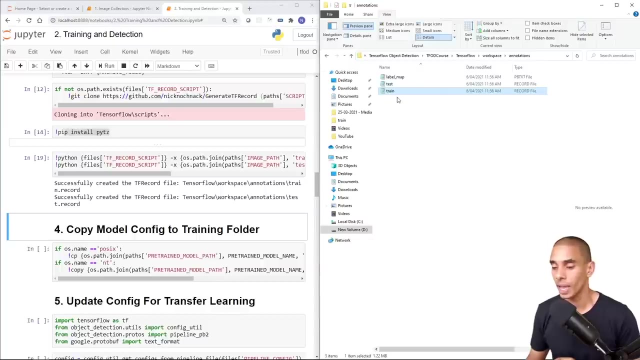 label map path is our label map dot pb text, so that's what we created, and our input path- in this case our train input reader, or our train input path- is going to be our trainrecord file, which is this file here, and our test input file, which is what's being referred to, or our eval input file. 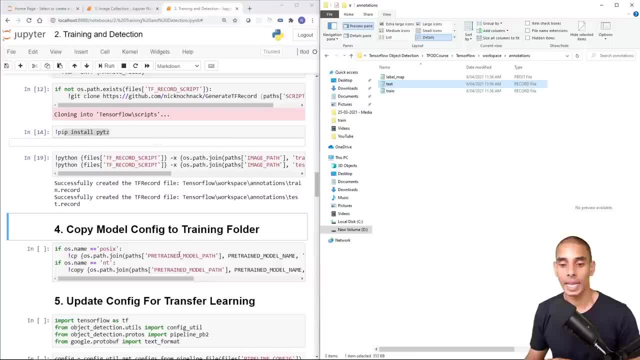 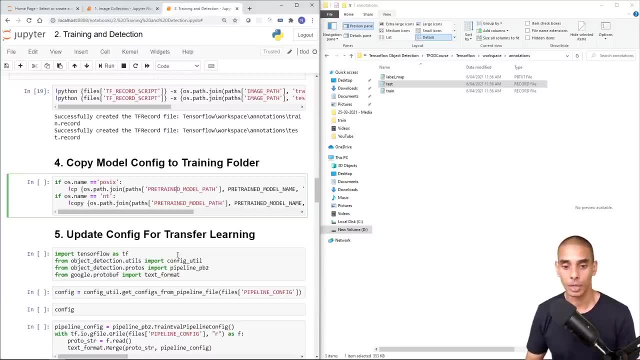 which is what's being referred to down here, is going to be our test file, but again, you don't need to worry about this. i just wanted to give you a little bit of additional background. our code is going to do that for us. so if we go and step through, so first up, what we're going to do is: 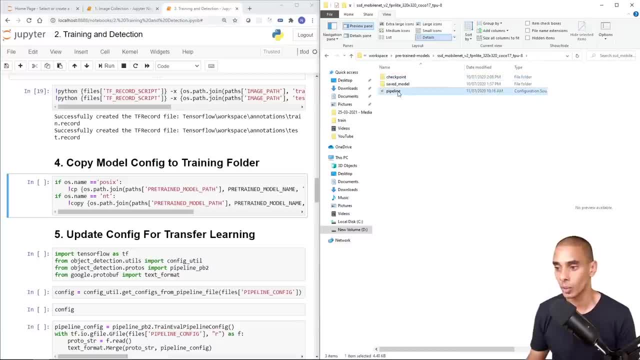 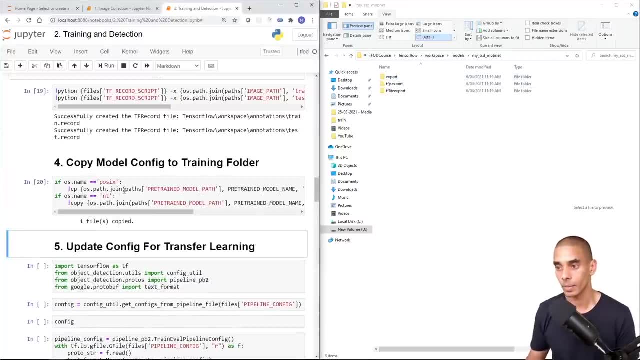 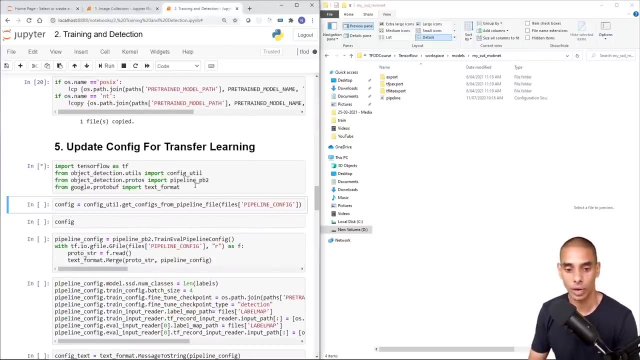 copy that pipeline file from our pre-trained models folder. so we'll copy it from here into my ssd mobnet folder. so if we run that you can see that that's now being copied and then the next sets of code are actually just going to do all of that configuration for us. so if we actually just step through all of that, 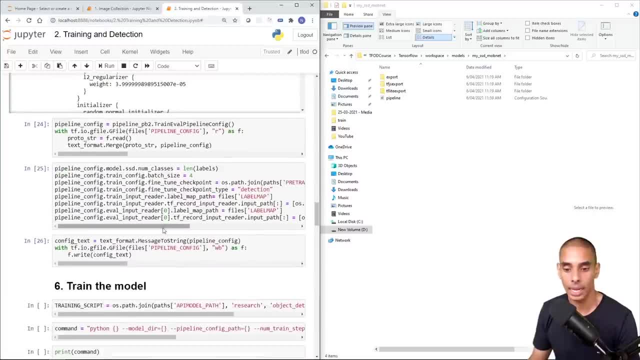 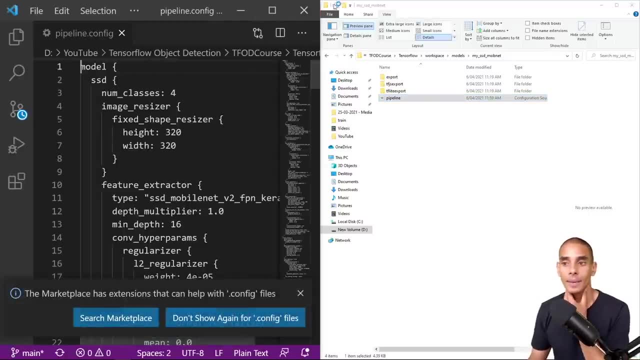 right. so it's opened up our config file. it's gone and set all of our different file paths and it's gone and saved it. so if i open up our customize one now, what you'll see is that it's going to change the number of classes. so this represents the number of different types of objects we're. 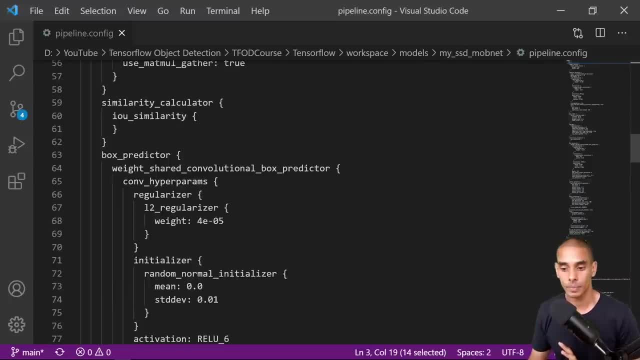 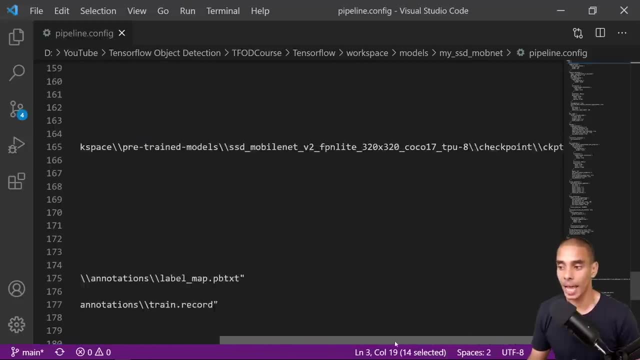 going to use and if we scroll on here, we're going to see that it's going to change the number of objects we're going to use. and if we scroll down- let's close this- you can see that we've actually also gone and set up our different. 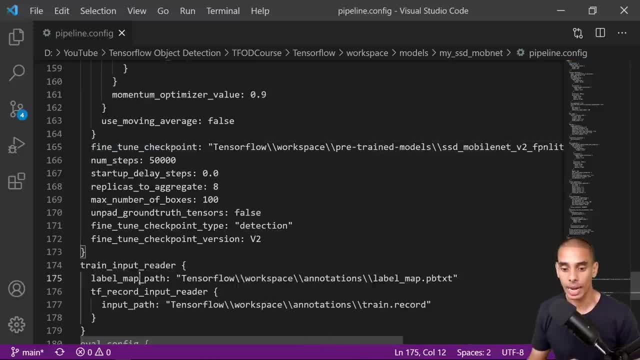 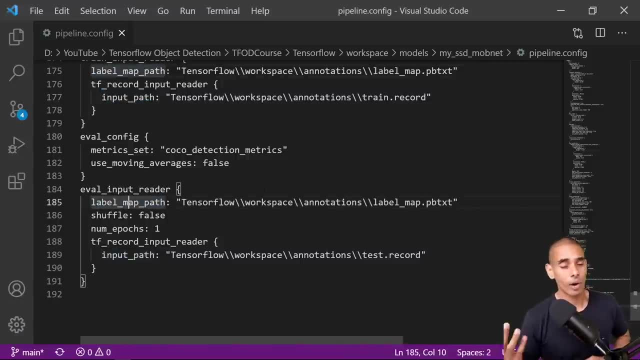 paths. so we've gone and set up our fine-tune checkpoint, our label map path, our input path, so on and so forth. so we set that up, set that up, set that up. so this is now all configured and pretty much good to go for us to kick off training. so if we close this now, 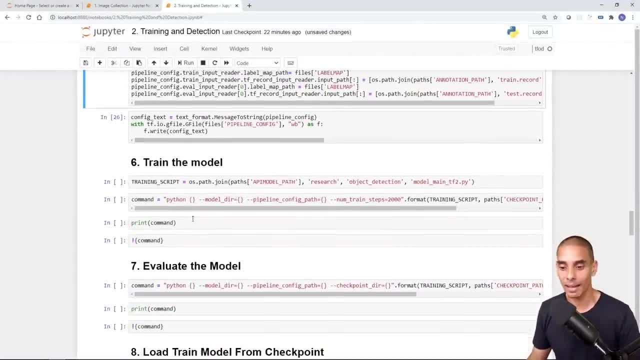 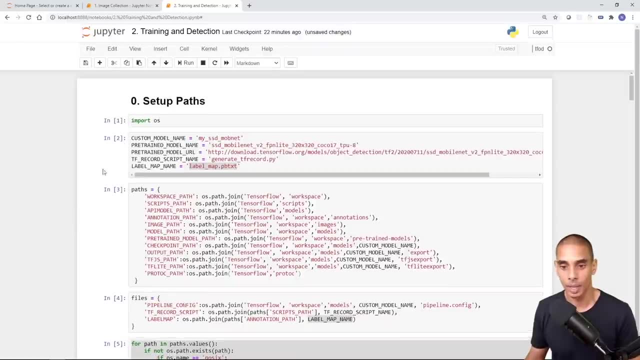 what we can actually do is actually start training our model. so we're now finally up to the good bit. so before we actually go and train our model, let's take a look at what we've done, because we have done quite a fair bit. so we set up all of our paths, we downloaded and installed the tense flow. 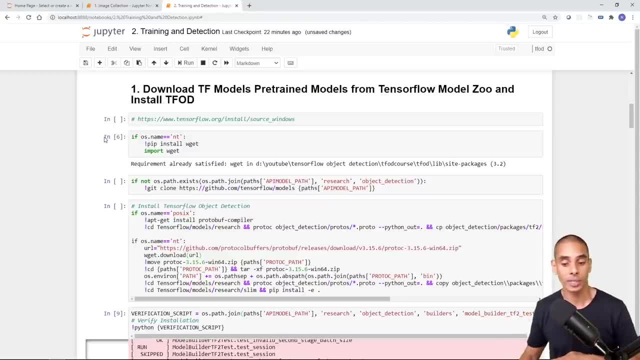 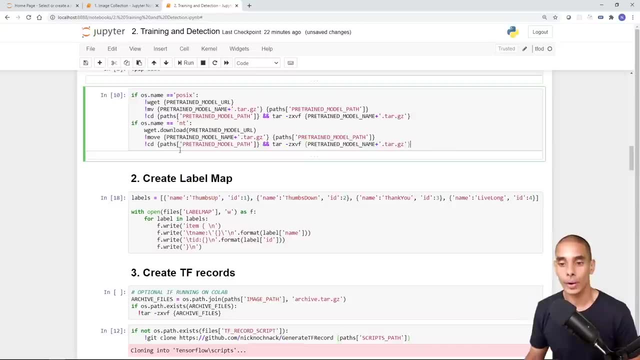 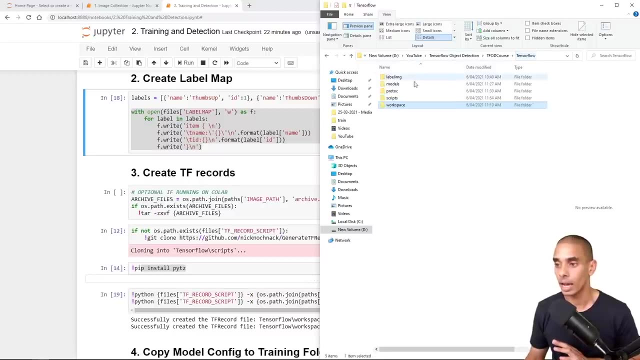 object detection api. so remember we had to go through a number of iterations, but as long as your verification script says okay, we are good to go. we then went and downloaded our pre-trained model from the tense flow model zoo. we created our label map and remember that is inside of our workspace. 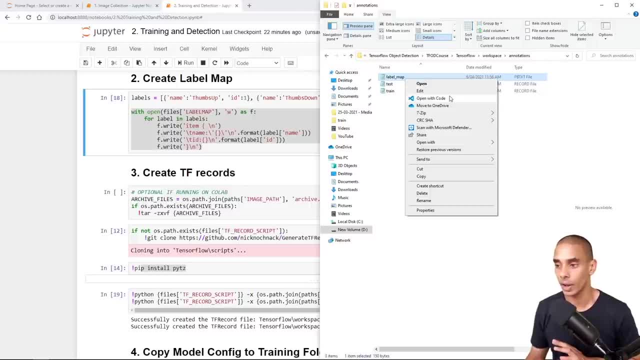 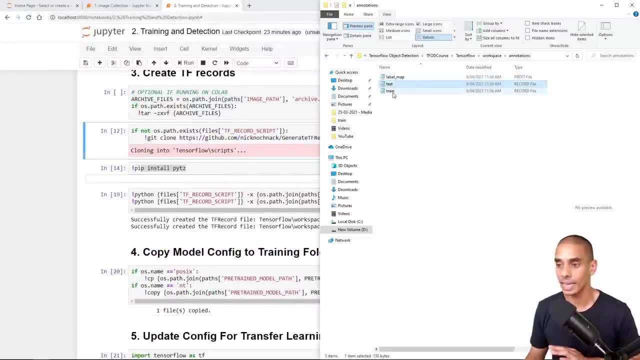 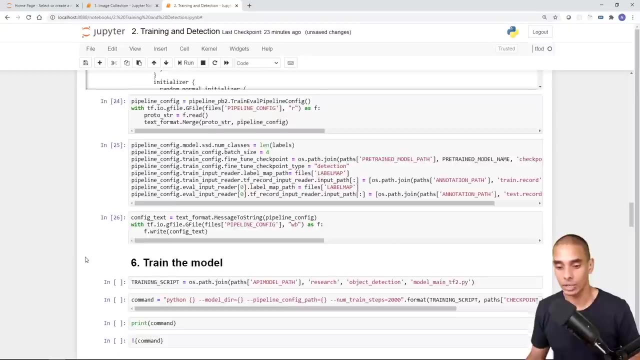 annotations and then label map dot pb text. so if i open that up, it's really just this. we then created our tf records, which again are our test and our train files. we copied our config to our training folder and then updated that. so again, that's all just code driven. you don't need to do. 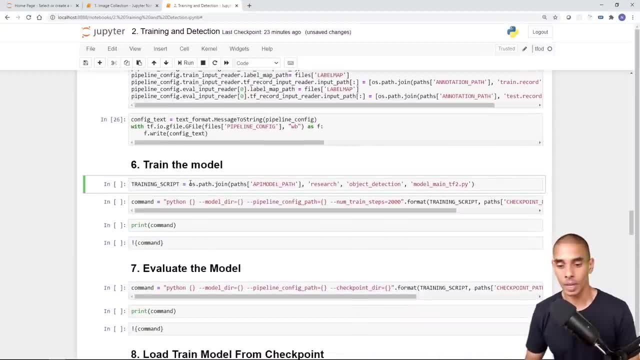 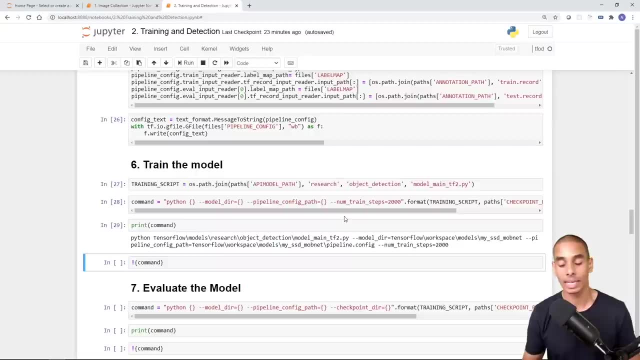 anything there. now we're up to the good bit, training our model. so in this case, what we're going to do is hit shift enter, shift enter and then print out our command. now i'm going to run this outside of a notebook, so that's going to allow us to see our progress as our model is. 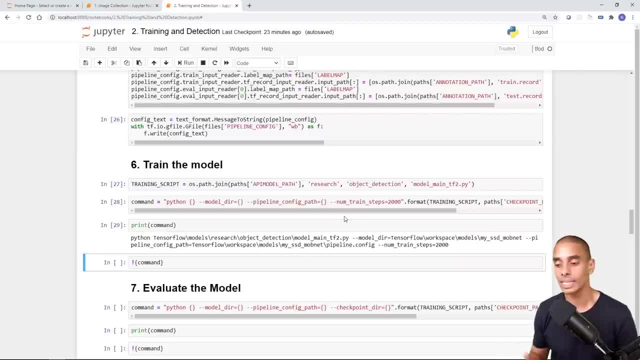 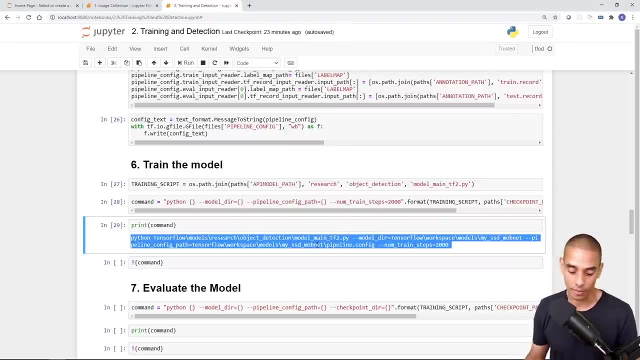 actually training. now, if you run it inside of the notebook, the only disadvantage is that, particularly on a windows machine, you're not going to see the status update in real time. so i'm going to copy this over here and then i'm going to open up a new command prompt, then navigate to where i've 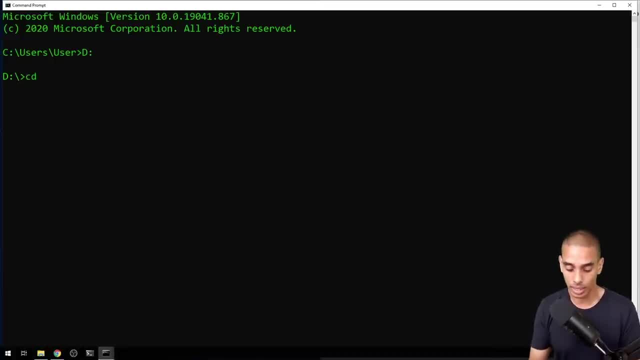 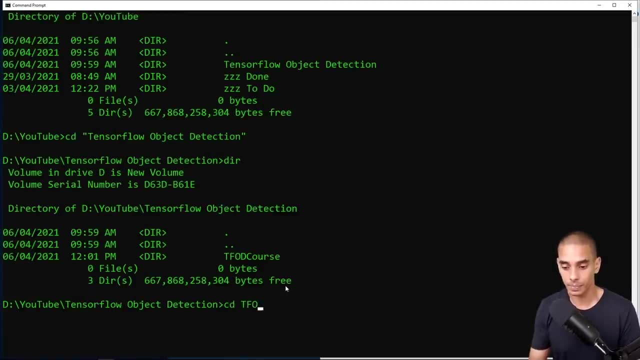 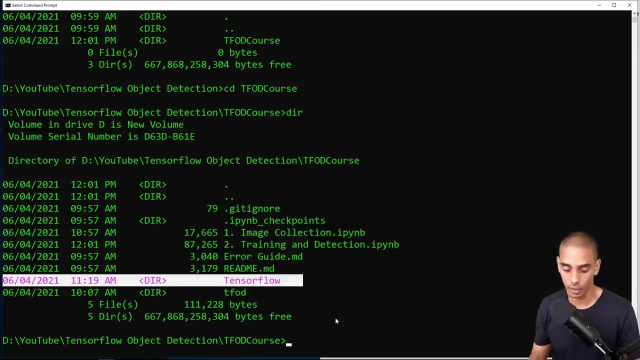 got my root tensorflow object detection course folder. so let's do that and i'm going to go into tfod course. all right, cool. so we want to be in this top level folder, so you should ideally see the tensorflow folder. so let's clear that now what we need to do again is remember we need to activate. 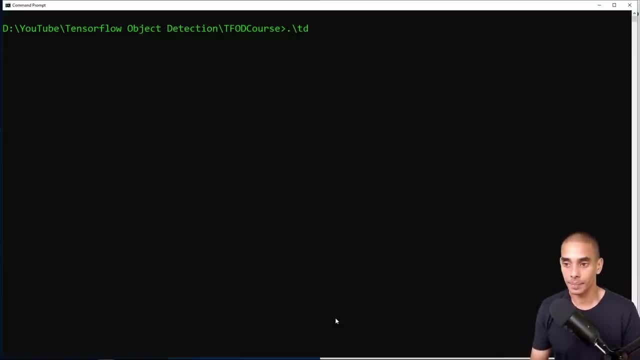 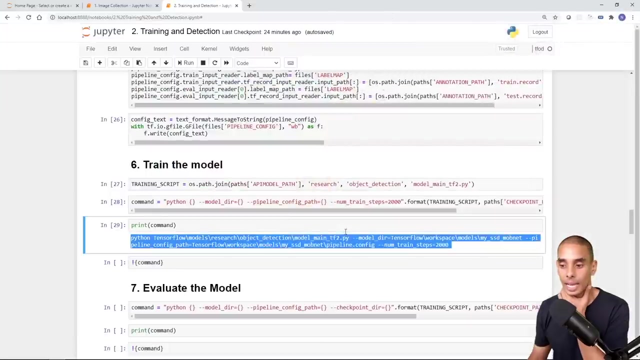 our environment. so to do that we can do backward slash, tfod, backward slash scripts, backwards activate if we type that. so again we're still inside of our tensorflow folder. now what we can do is we can actually copy that command. so let me just explain that command a little bit. so the first thing is actually running. 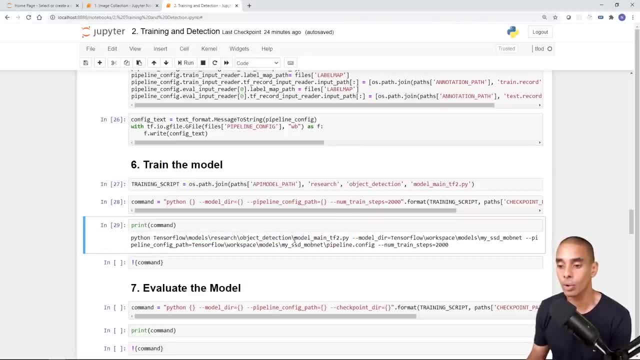 our model training script. so what it's doing is it's using the model underscore, main underscore- tf2.py script. now again, i'm going to this into a little bit more detail than i usually would, because i really want to explain to you how this actually works. so what it's actually doing is: 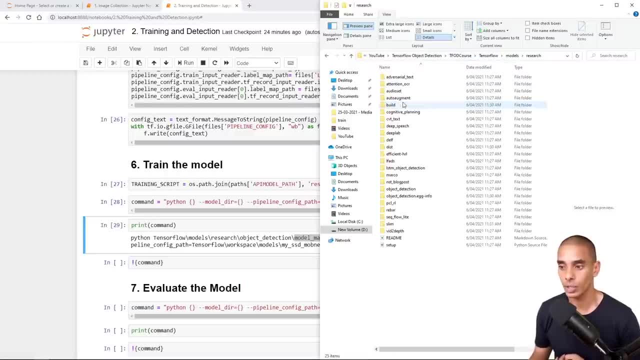 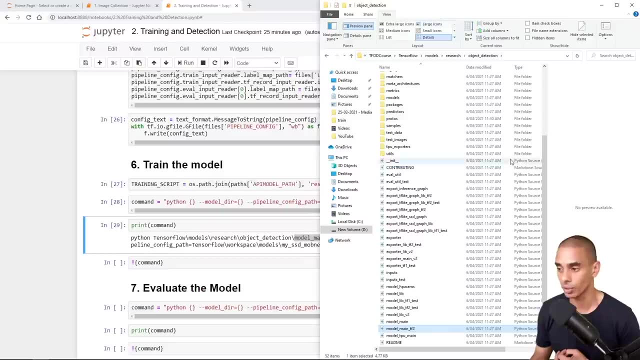 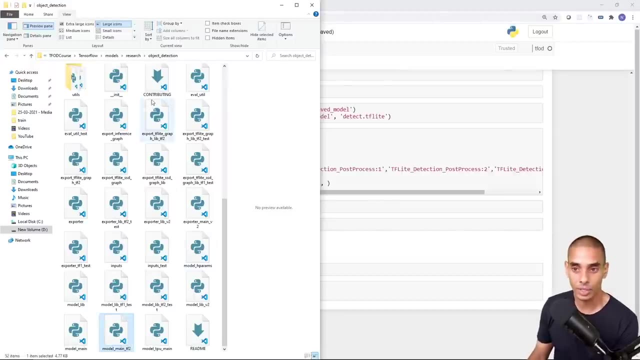 it's going into tensorflow models, research, object detection, and then it's running this script down here, model main, underscore tf2. probably a little bit small to see, so model main tf2 down there. that was probably obscured by me, so it's running, uh, that over there. so model main underscore tf2. 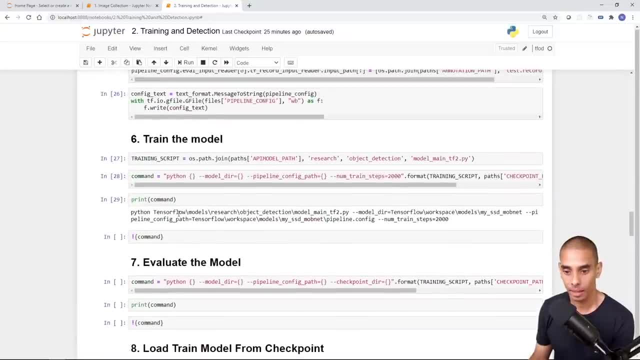 so that is this component here. so it's running that. then we're passing through a number of arguments. so first up we're passing through our model directory. so this is where our pipelineconfig file is. remember, our pipelineconfig had all of our custom paths, had a number of our labels and had 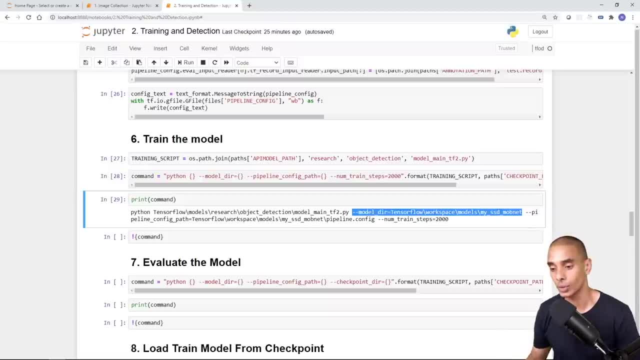 all of our different details of the specific object that we're going to use. then we are passing through our actual pipelineconfig and we're also passing through the number of training steps that we want to go ahead and run through. so in this case we should be good to go now. so we're going. 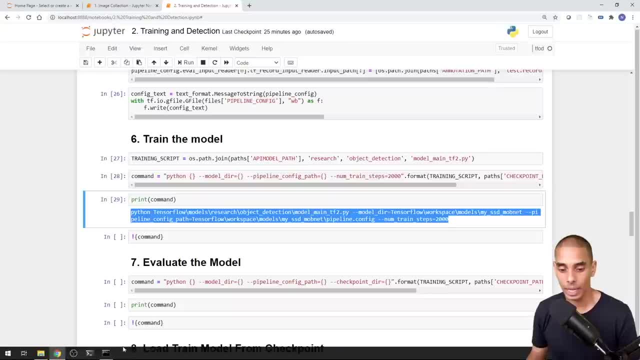 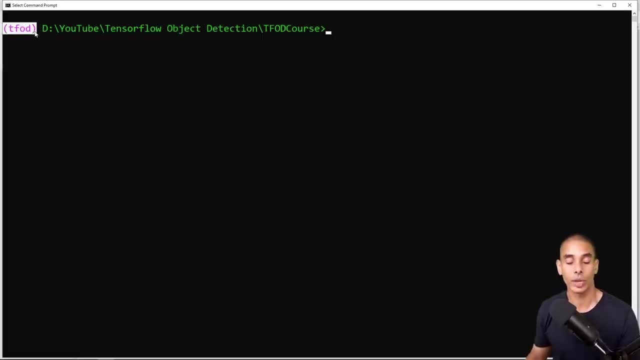 to copy this command and we are going to paste it into that new command prompt. so let's clear that and keep in mind: we've activated our virtual environment, so your virtual environment has to be activated, otherwise you're not going to be able to leverage all of that tensile object detection stuff that you've. 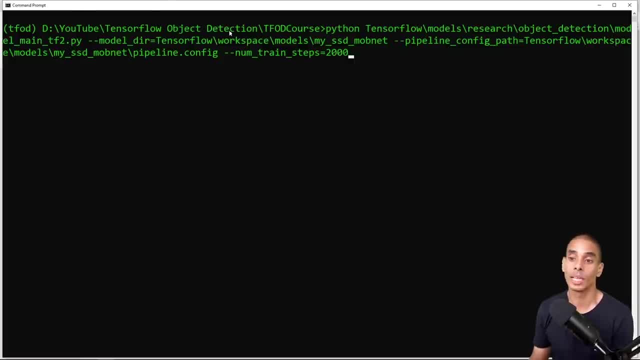 gone ahead and installed. so if we paste that command in there now, oh, the last, uh, the last parameter is the number of training steps. so you can increase this or decrease this. ideally, i normally set it to 2000 for my first prototyping step. then i'll go and clear out all my training. 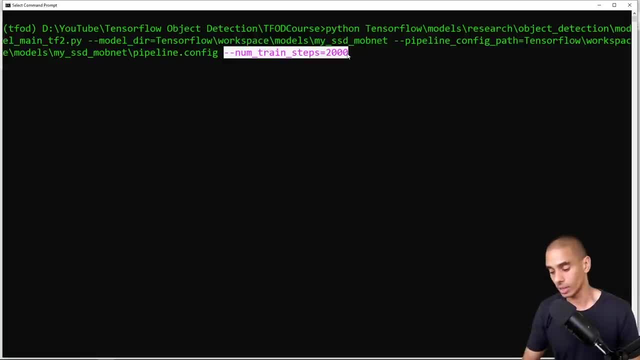 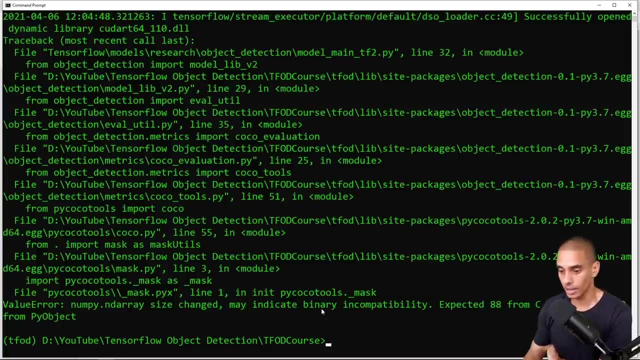 and then i'll set it to 10 000 when i come to do my actual training run. so let's go ahead and run that, and ideally so you can see that it's successfully opened and looks like we've got an error there. okay, this is. 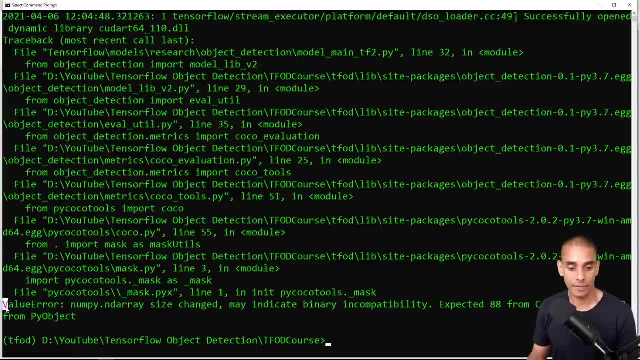 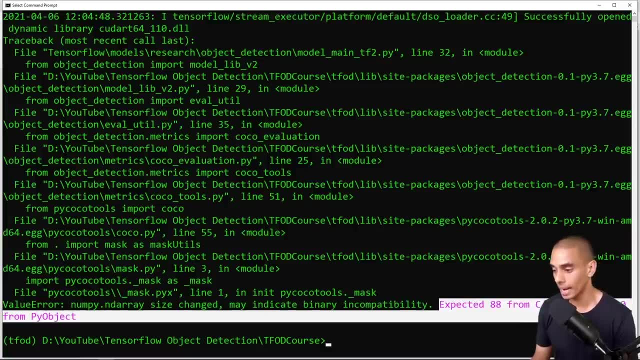 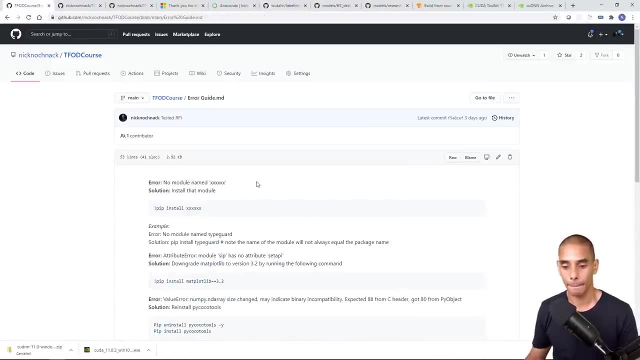 good, cool. so we've got this area here. so value error numpy nd. array size change may indicate binary incompatibility. expected 88 from c header. got 80 from pi object. so if we copy this and again go into our error guide and search for that, you can see that that. 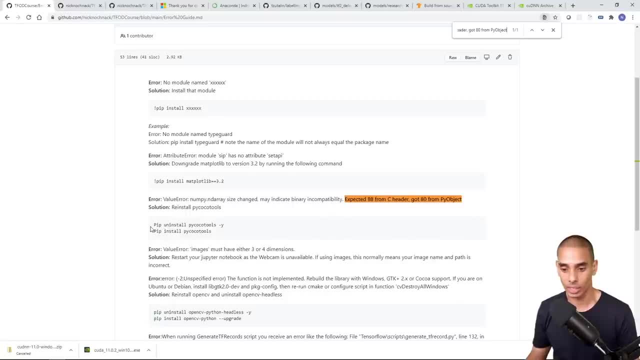 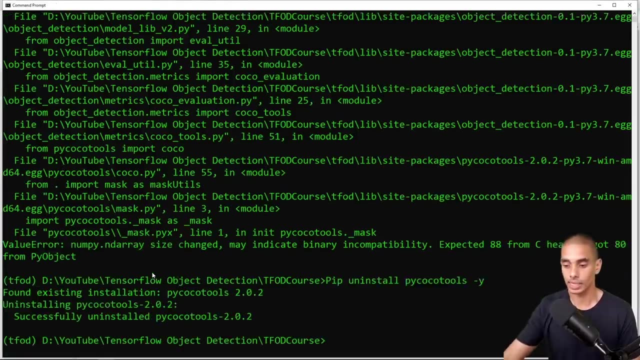 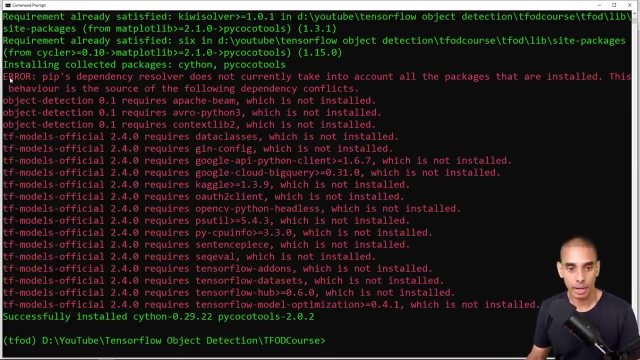 particular error is solved by reinstalling pycoco tools. so let's go on ahead and do this so we can pip: uninstall pycoco tools. so let's copy that. cool, so that's it uninstalled, and then we can reinstall it. okay, so in spite of these, that looks fine. so it says it's successfully installed pycoco tools. 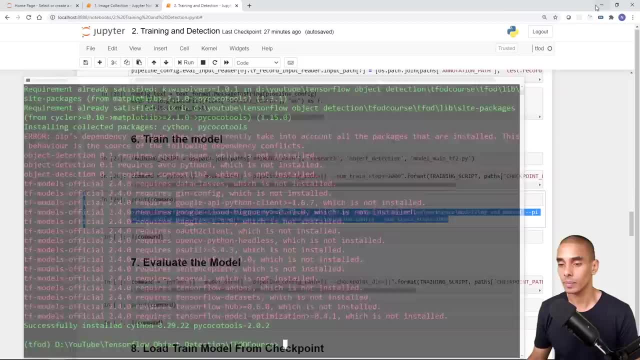 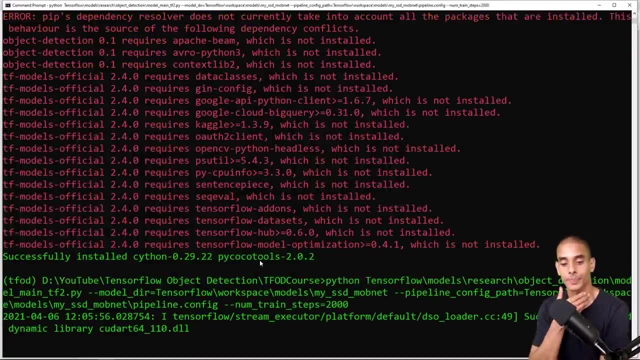 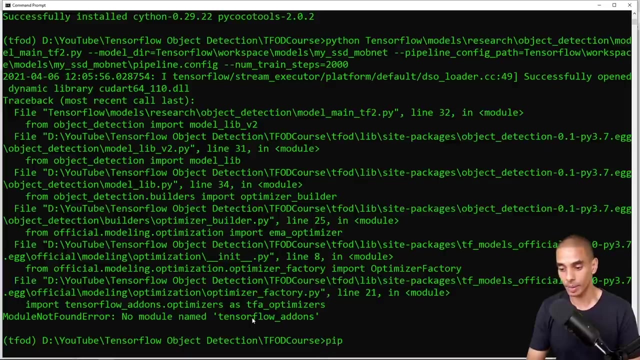 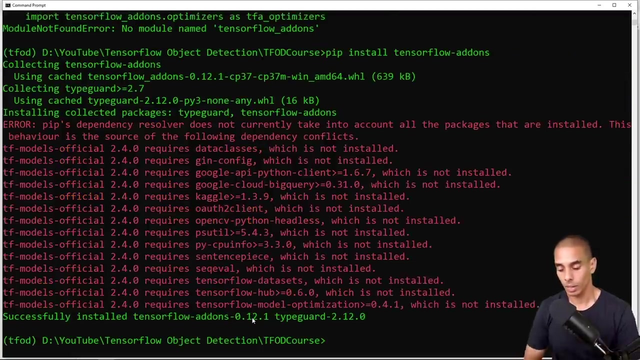 again. so let's go ahead and paste in our command again, so if we go back to our notebook we can copy this no module name: tense flow add-ons. so again, this is a no module error, so we should be able to pip install tensorflow add-ons. now let's try running our command. 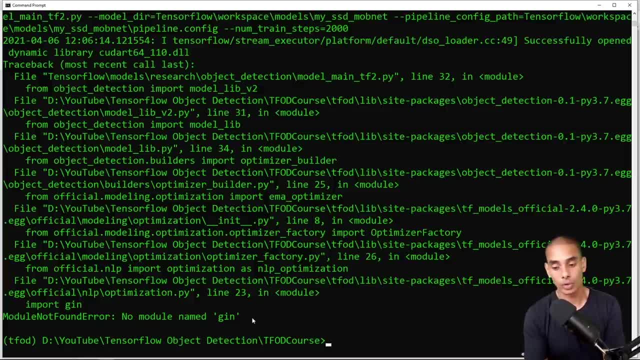 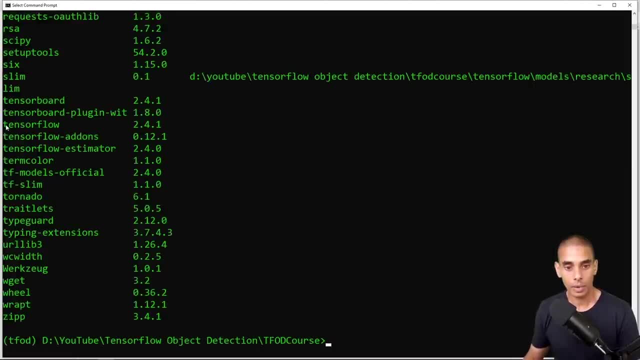 no module name: gin, all right. so this: these no module errors are specifically attached to the tense flow version. so let's just type in pip list first up. so even though we've got tensorflow 2.4.1, tensorflow estimator, so let's run, let's install gin. so pip install gin. 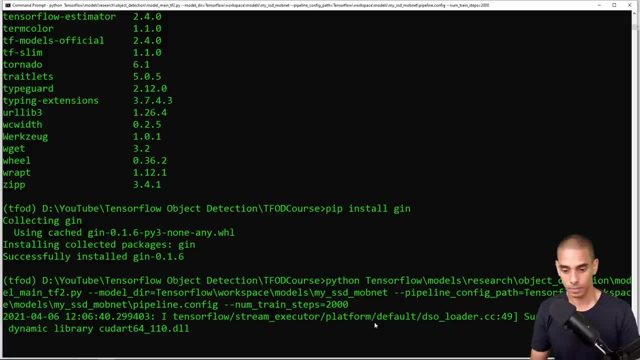 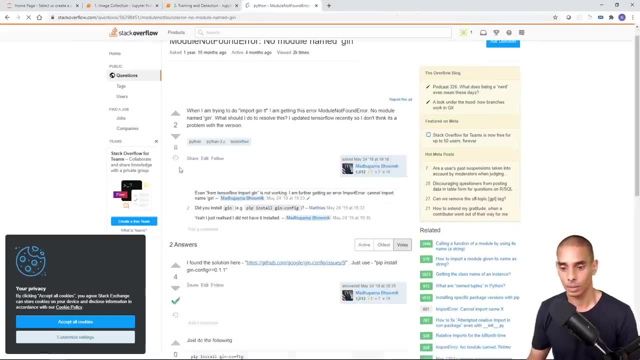 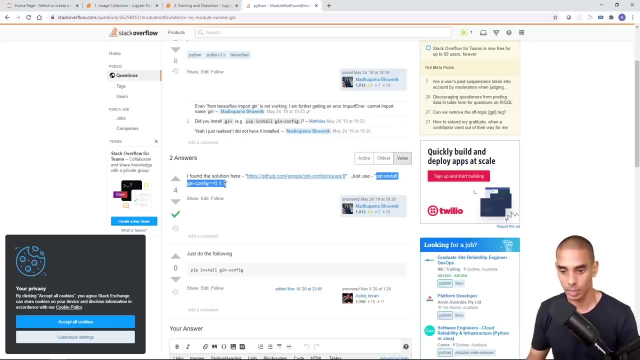 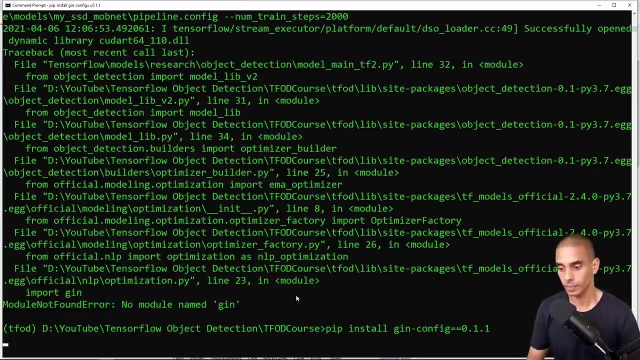 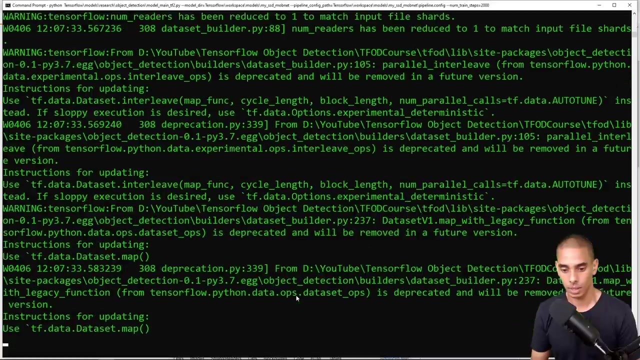 try our training command again. so let's search for that one. looks like i've encountered that one again and it looks like we need to downgrade, so let's do that. so let's pip install gin dash config: zero one dot one, dot one. So let's try that, Try this. Okay, that's looking good. So it looks like we. 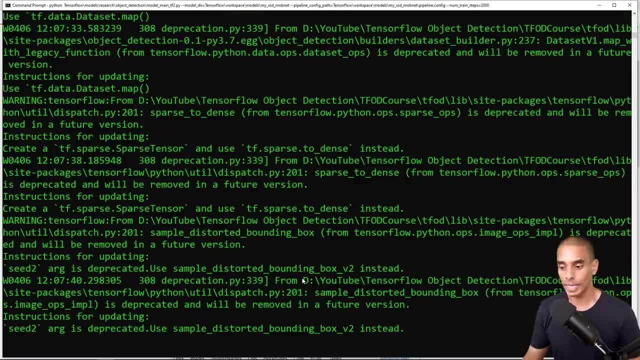 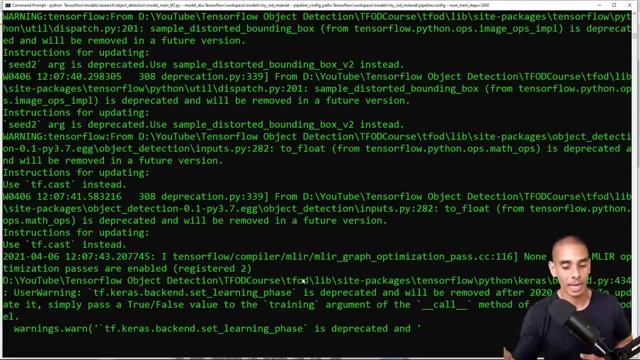 sorted through those errors And again, no more dual errors are normally just solved by installing the right library. If you can't find the right library, just take a look, Google around, see what people have done, And more often than not these are common errors. So in this case we just 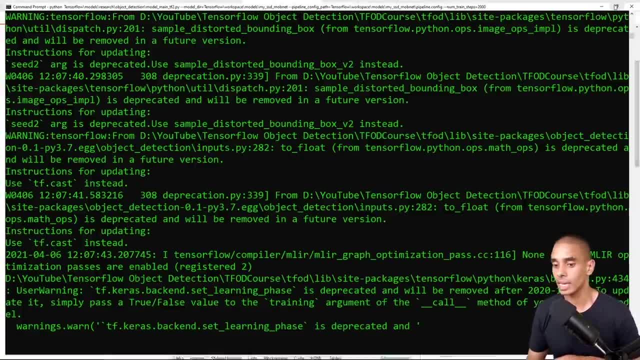 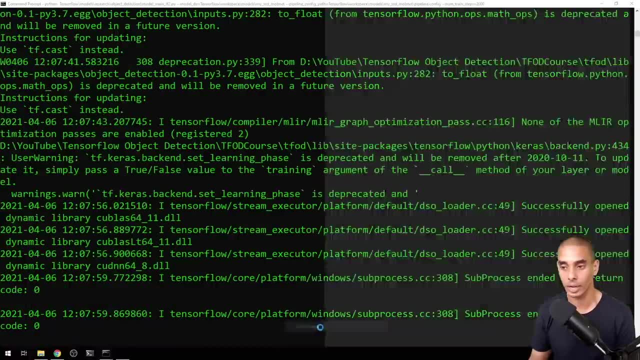 needed to install, or pip install, gin config, And now you can see that this is actually running. Oh well, I know from experience that this is actually running now. So what you're going to see is first up, if you're running on a GPU, that your GPU memory is taken up. So you can see that. 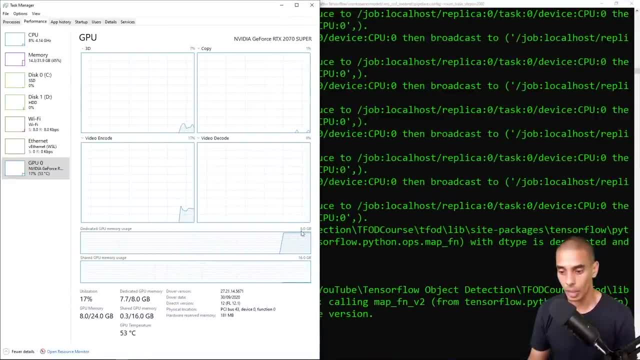 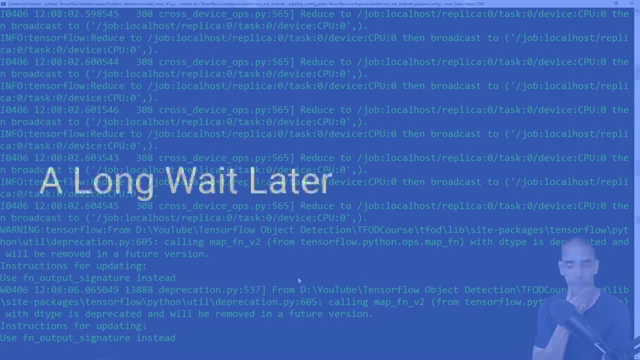 let me bring this over to this side, So you can see that I'm now using the full eight gigs on my GPU And ideally in a couple of seconds, you should start to see our loss metrics showing up. Now, one of the things I actually just 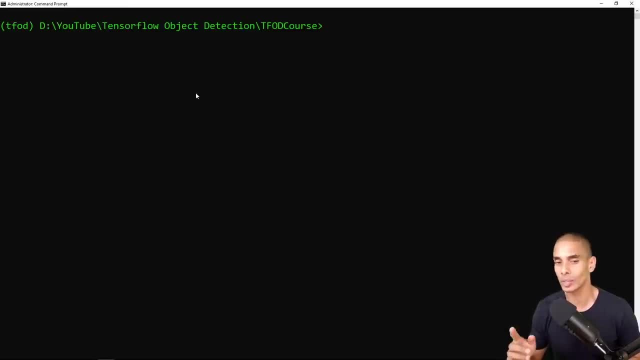 noticed is that we didn't actually have TensorFlow GPU installed, So it was taking a long time for that training to kick off, which was a little bit weird, to be honest. So normally it should take no more than 15, 10 to 15 seconds to actually kick off. So what we're going to do is we're 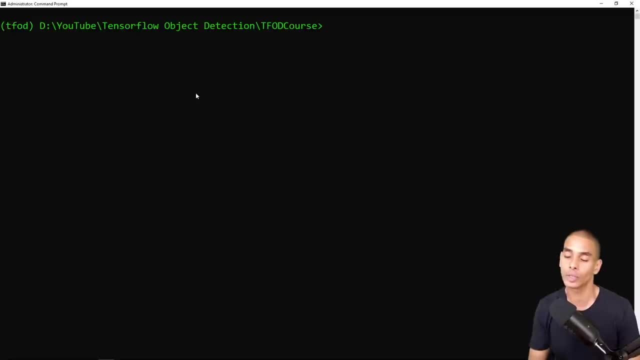 going to. so I actually just installed TensorFlow And then what we're going to do is make sure that we've got the right versions of TensorFlow and TensorFlow GP installed. So we'll install pip, install TensorFlow And we add 2.4.1.. And we're going to. 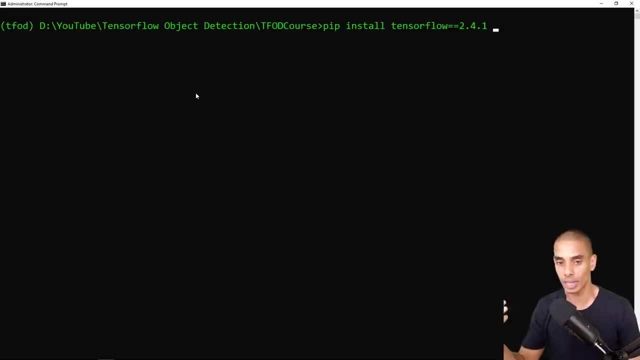 install TensorFlow GPU as well, because you need TensorFlow GPU to leverage the GPU. So run TensorFlow dash GPU equals 2.4.1.. So even though our verification script is fine, we do still need TensorFlow GPU. So before it was fine to run on CPU to leverage the GPU, we need TensorFlow dash. 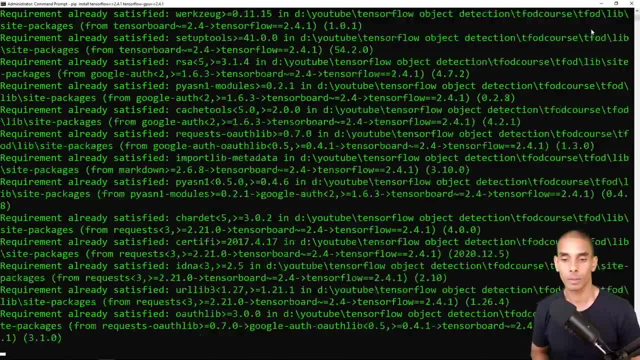 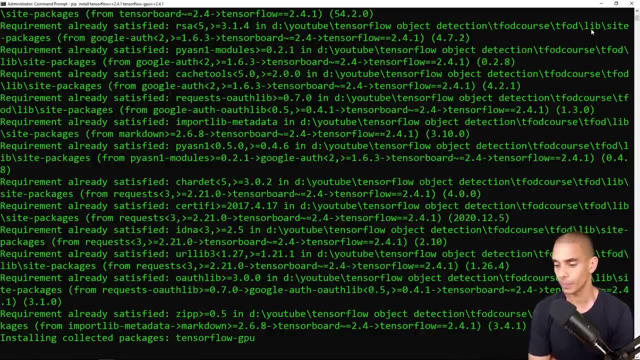 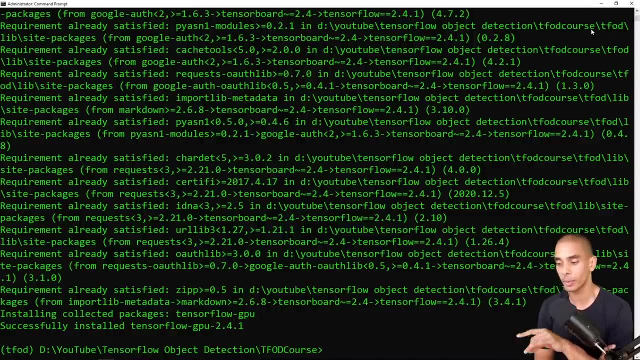 GPU. So let's go on ahead and install that And give that a couple of moments to install And ideally we should see that we've got TensorFlow GPU installed. So if you kick off your training and you do have a GPU set up- CUDA and CUDNN- the next thing to check if it's not kicking. 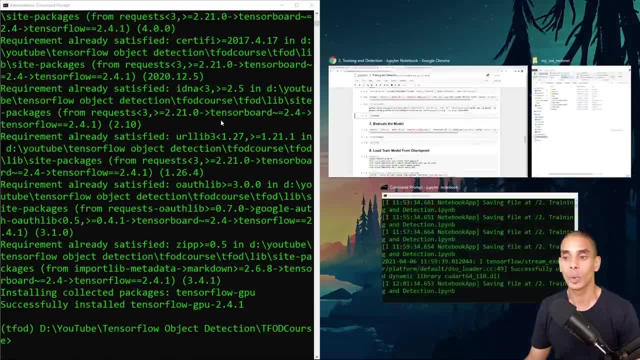 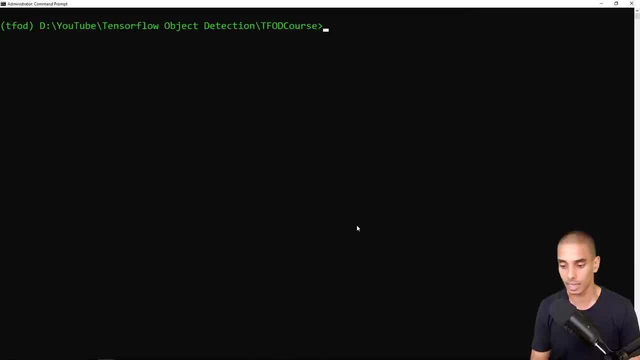 off on your GPU or not. starting to train relatively fast is whether or not you've got TensorFlow GPU installed. So then we're going to copy our command And now you should see that our training kicks off a lot faster. Let's clear this, paste that in And let's see how long this takes now. 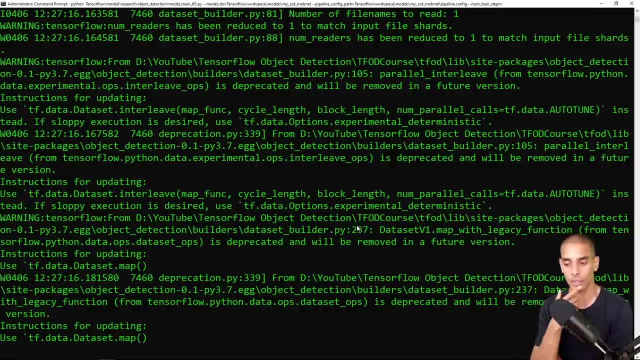 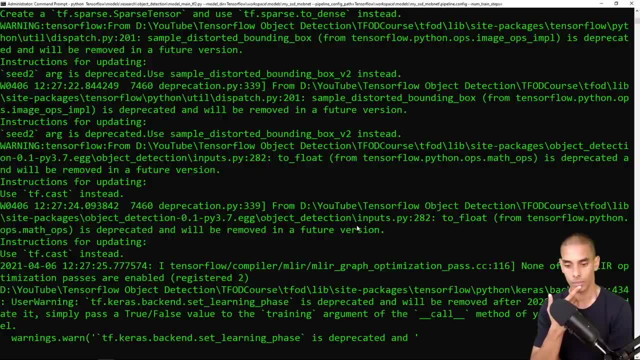 So if it takes a long time, double check that as well, So whether or not you've got TensorFlow GPU installed. So let me go ahead and paste that in And let's see how long this takes now. So let's see how long this takes. So these are all pretty normal outputs. 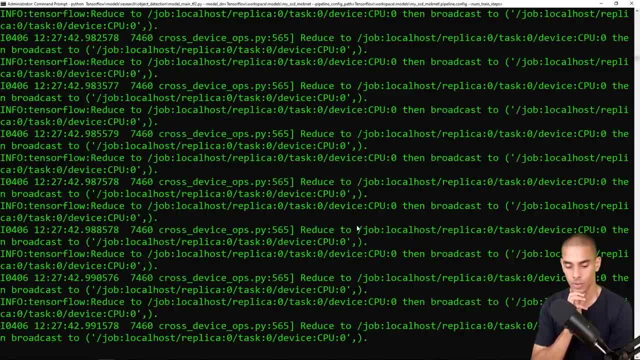 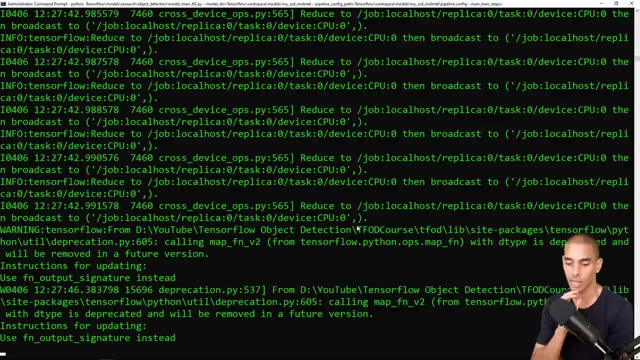 It's looking positive. So when it sort of gets to the end of the training, we're going to go ahead and install the GPU, this line- and again it might be a little bit different depending on what you're training on. so use fn, underscore output, underscore signature instead. so normally that means that it's sort of. 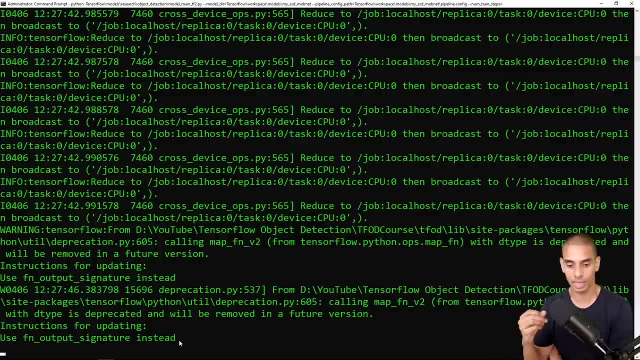 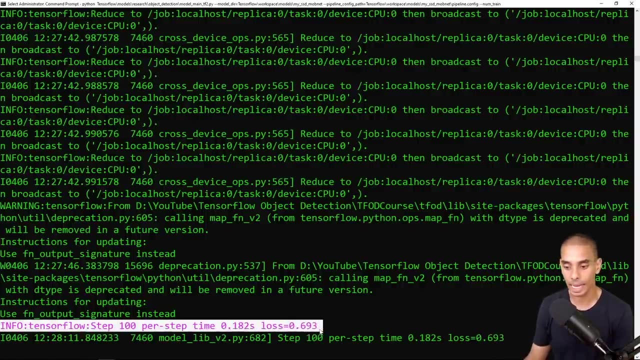 got to the next step. so ideally, what you should see is the loss metrics appear after this: let's wait and see sort of stalls, we'll restart it. no, there you go. all right, cool, so that looks like it's kicked it off, so you can see that now we're getting these metrics here. so basically after: 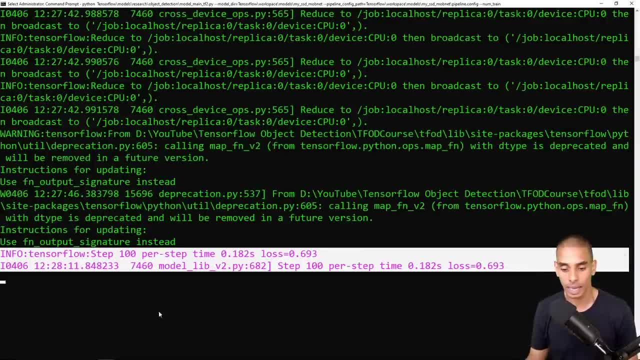 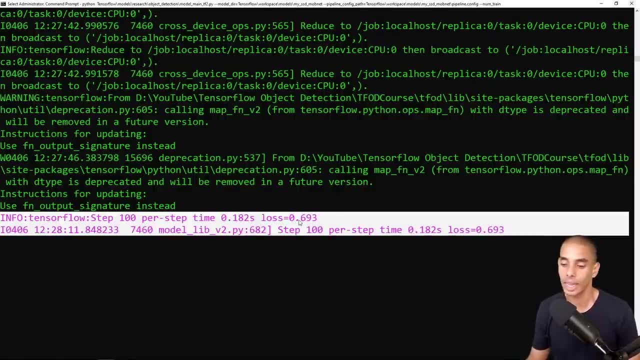 every 100 steps. this is going to be printed out. so you'll get step 100 per time. so you'll get the time per step. so in this case it's 0.82 s or seconds. we've also got the loss. so in this case, 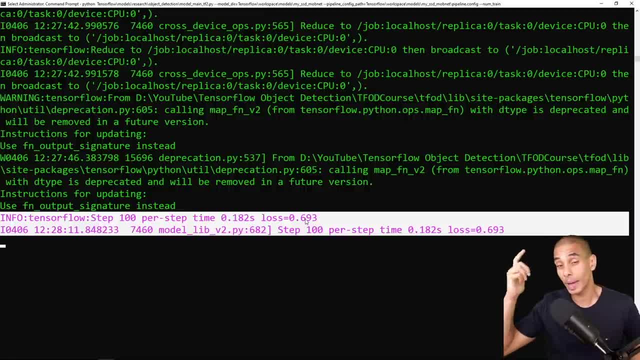 our loss is 0.693. now, if you cast your minds back to our evaluation step, what we're saying is that you want your loss to be as low as possible, your mean precision and your or your mean average precision, as well as your recall, to be as high as possible. so in this case, we're going to let this. 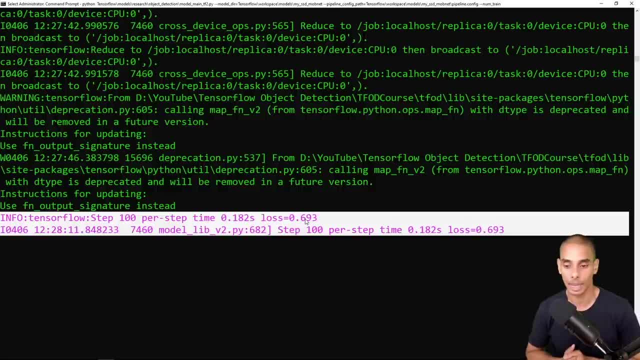 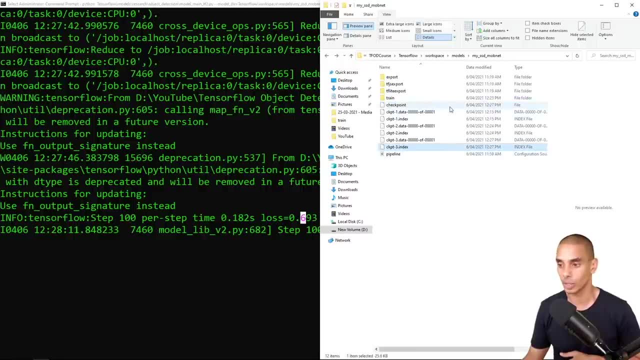 run, so ideally you're going to see this output after every hundred steps. so in this case, we've got our first 100 steps, and if we also take a look, you can see that we've got our checkpoints starting to generate here as well, so we're looking good. for now we're going to let 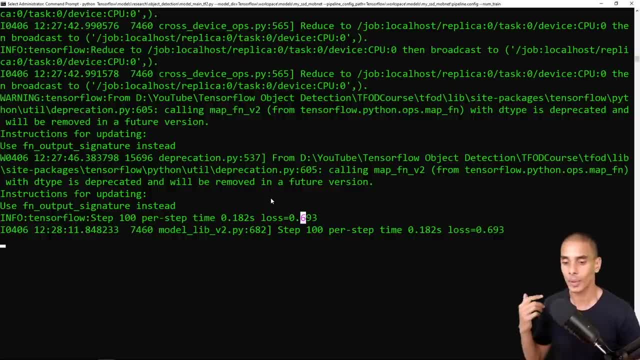 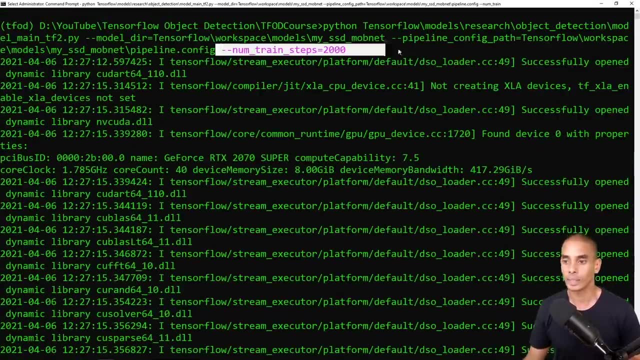 that run and we'll see how we go. so ideally, remember we- we kicked off our training for 2 000 steps in our training command, which is right up here, so we had 2 000 training steps. ideally, after 2 000 training steps, we should have our fully trained model. so 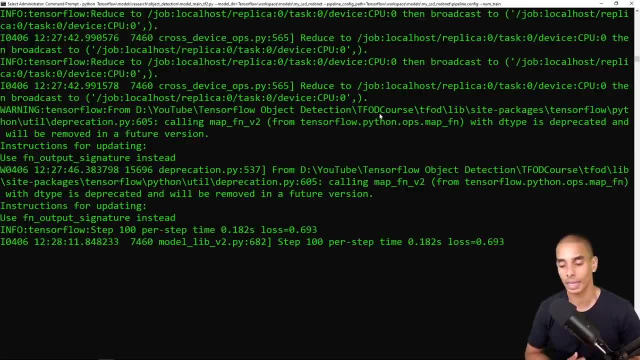 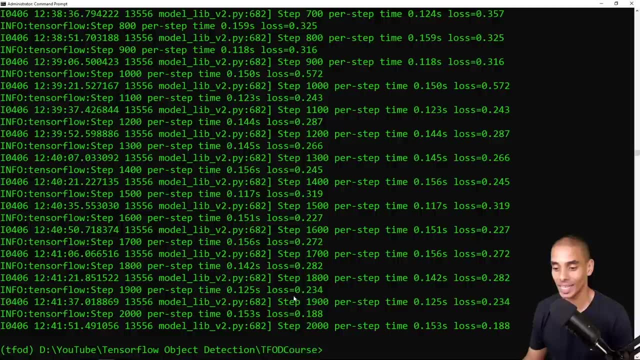 let's let that run and then we'll come back and take a look and do some detections. so that is our model, fully trained. so you can see that we got up to step 2000 and our final loss- let me bring this over to this side- and our final loss. 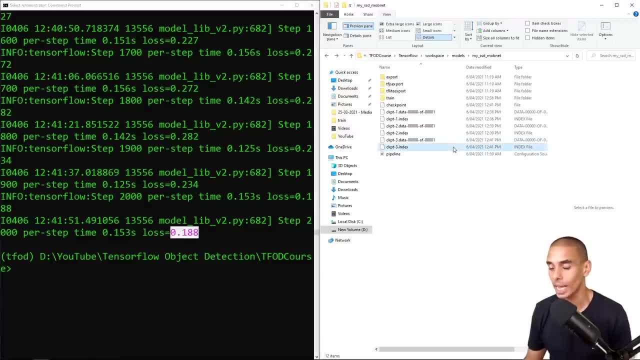 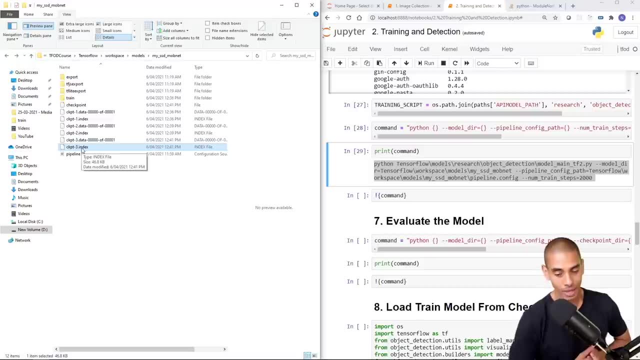 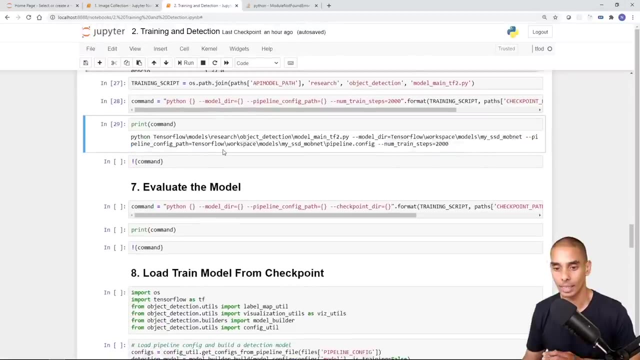 was 0.188. now if you also take a look inside of our my ssd mob net, you can also see that we've got all of our checkpoints generated. so we've now effectively gone through and trained our model. now what we can do is actually go and evaluate it. so remember how sort of saying you've got your. 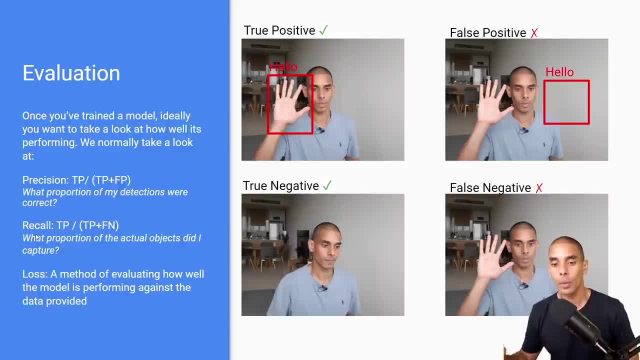 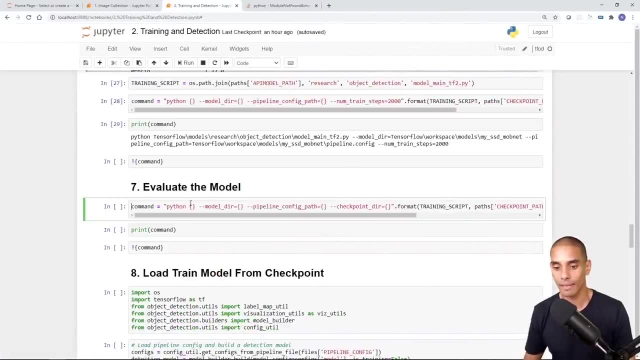 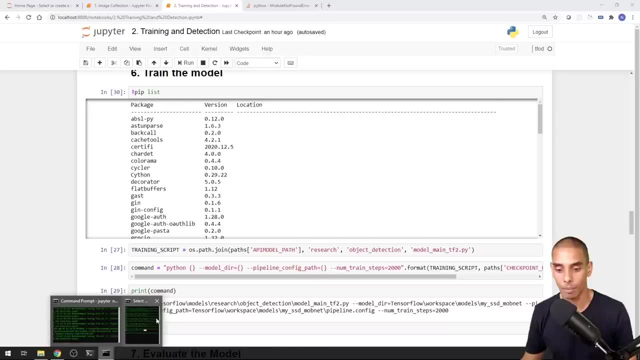 precision metrics. so you've got precision and recall. we can actually go and calculate these using the tense flow object detection library. so what we can do is run our evaluation script. so if we go and run our evaluation script model, so we've gone and done step six and again our model. 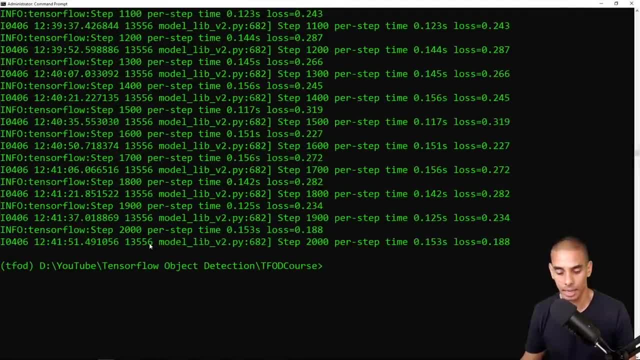 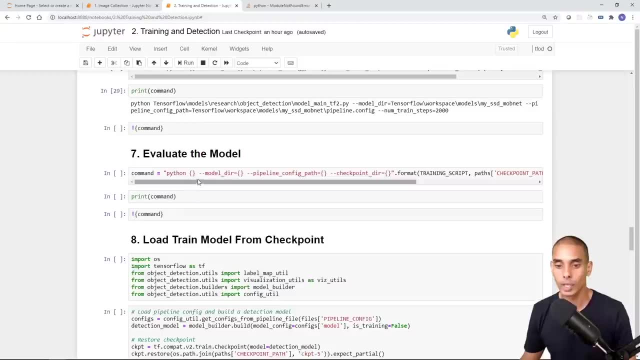 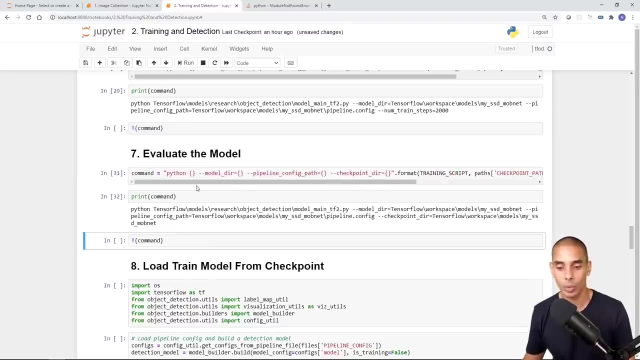 is successfully trained, so it didn't take too long. what did it take? um so 0.153 seconds per step. so again, it got pretty fast on the gpu. now what we can go on ahead and do is evaluate. it's so, if we go to step seven, hit shift, enter, print out that command. now we can actually run this one. 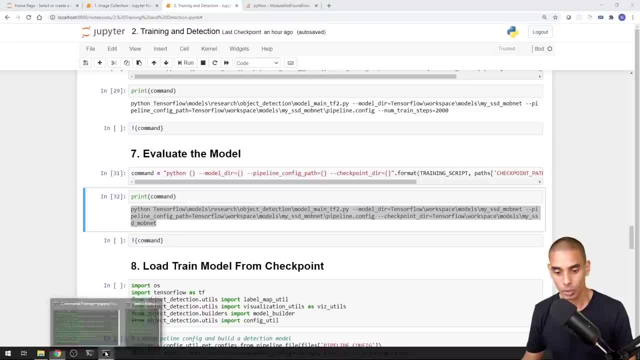 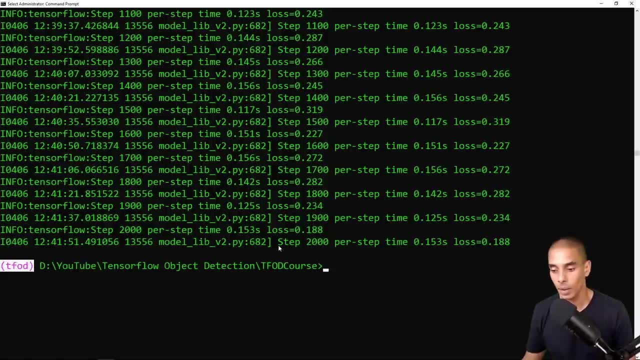 uh, we'll run it using our command prompt, so we'll copy that. so if we go and paste that command again- so we're making sure that we're inside of our virtual environment- and go and paste this, hit enter and this is actually going to go on ahead and calculate our performance metrics for the 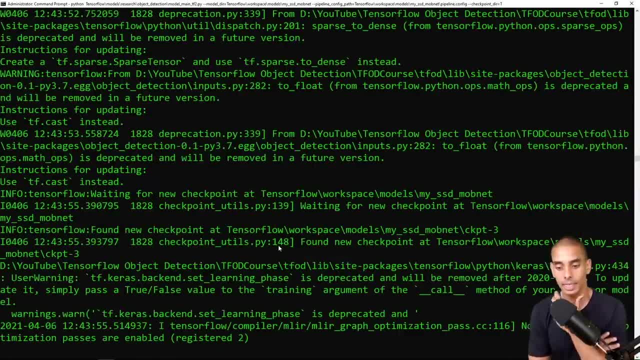 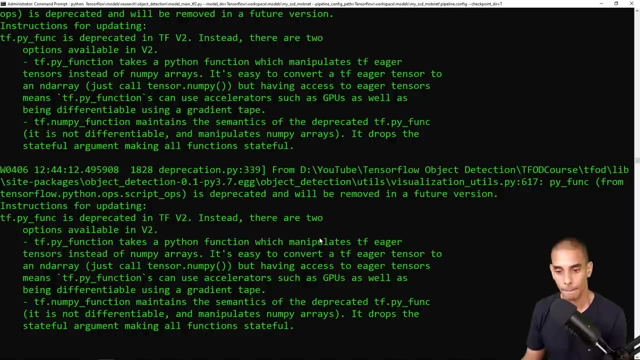 model that we've currently got in that folder. so again, it's going to go through all of these and ideally, what you should see towards the end of it is that you get this little table that gives you all of your performance metrics, and there you go, so you can see here that we're getting our 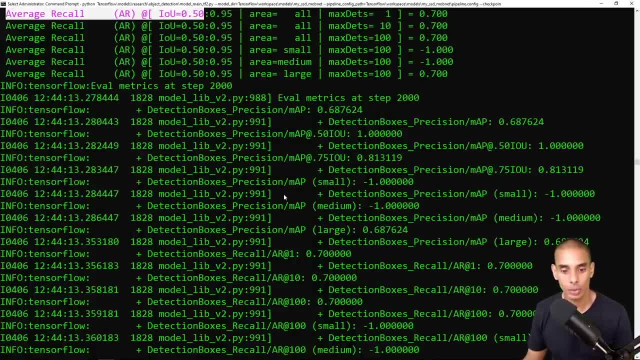 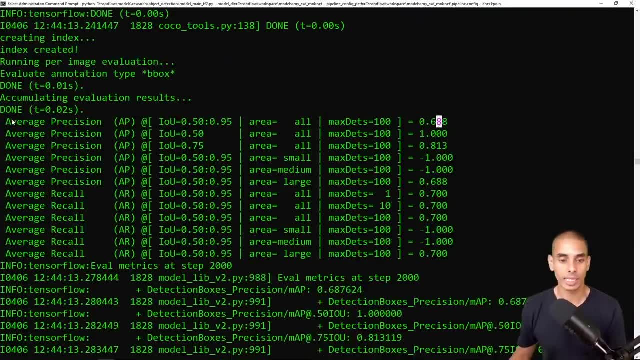 average precision, our average recall. we should get some loss metrics as well, so they're down here so you can see that we've got a bunch of loss metrics, but i'd pay most attention to these ones up here. so you can see here that our average precision at 0.5 to 0.9. 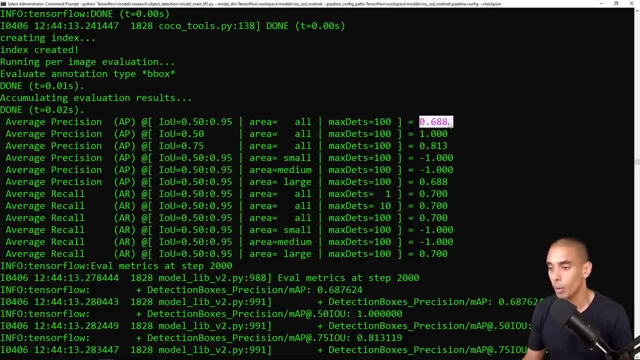 five iu. so just pay attention to this- is 0.688. so again, it's not the highest precision, but it's not too bad. our recall is about 70, so again not too bad, given the fact that we only gave it what like five or six images per class. so again, not too bad. right now, what you can also do is you can. 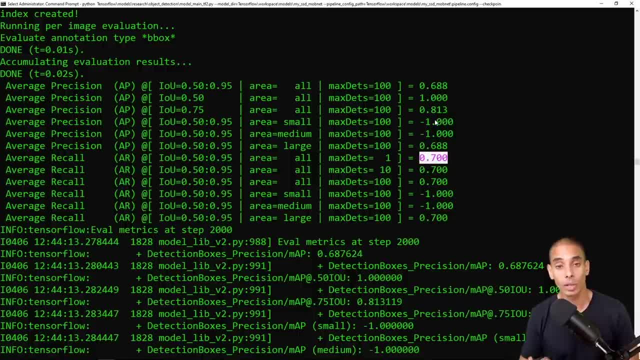 also open up these same detection metrics, as well as the loss metrics, using tensorboard. so if you haven't worked with tensorboard before, basically it's an interactive monitoring tool that comes or that is open source through tensorflow. so what we can do in order to use that, so we can just step. 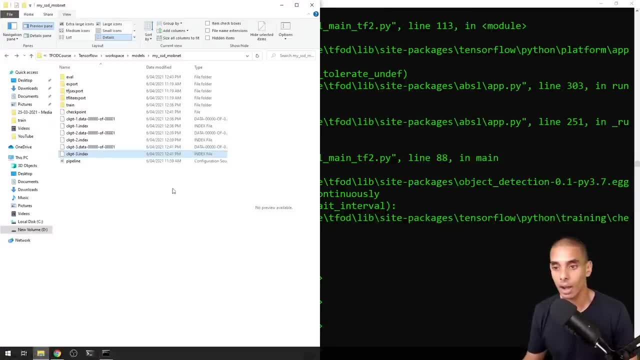 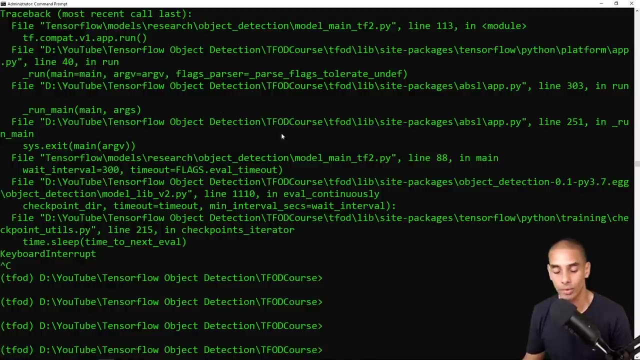 out of this by hitting ctrl. c is inside of our my ssd mob net folder. you've got two folders which i haven't really talked about yet. so you've got this train folder that's generated when you kick off your model training, and you've also got this eval folder which is generated once you go and run this. 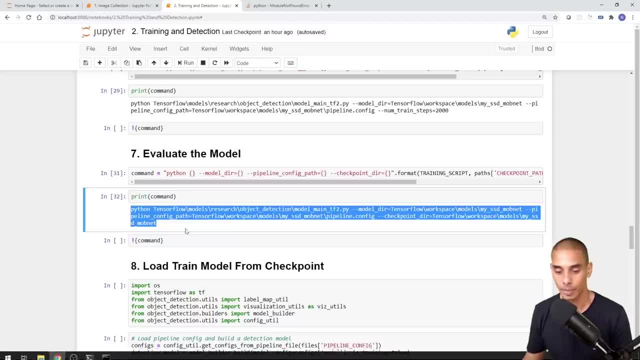 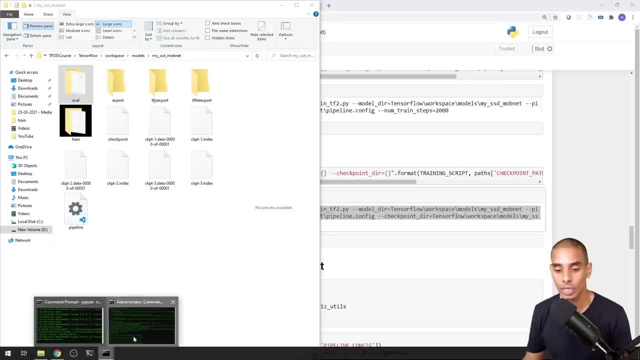 evaluation script so effectively. uh, script the script under seven: evaluate the model. so these two folders are the ones that are going to be used to evaluate the model. so these two folders are going to be generated after training and after evaluation. now what you can actually do is you. 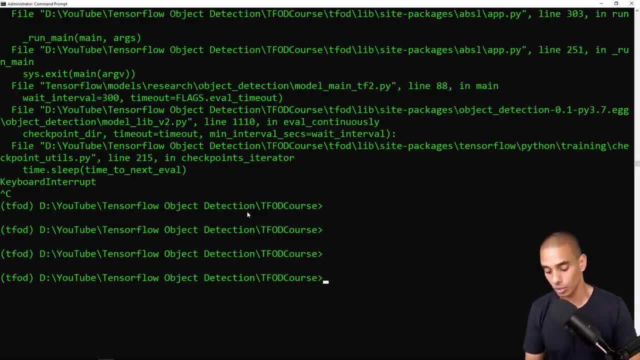 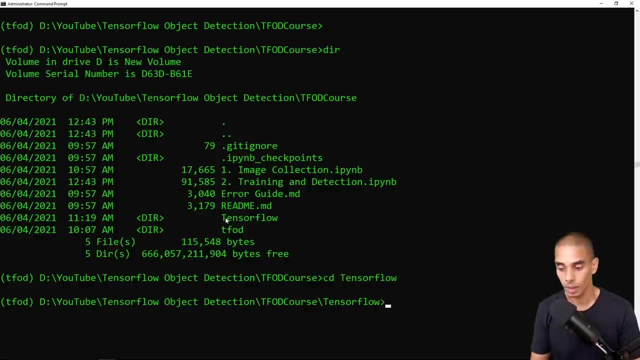 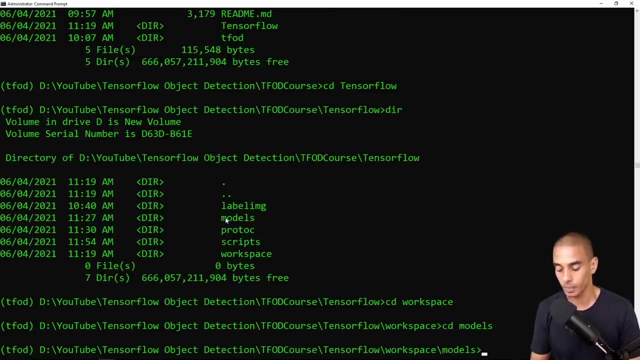 can actually step into these folders and spin up tensorboard. so let's go ahead and do this. so right now we are in our root folder so we can go into tensorflow, and then we can go into workspace and then, i believe, cd models and then we want to go into our my ssd mob net folder. 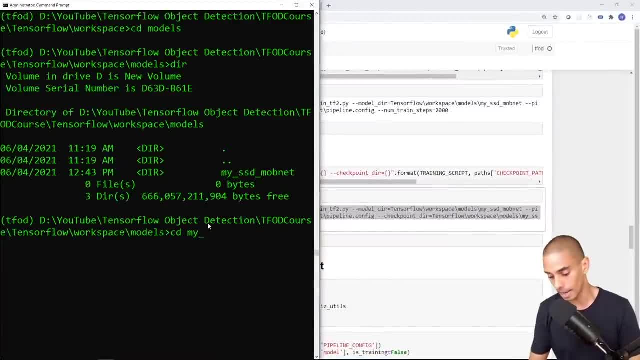 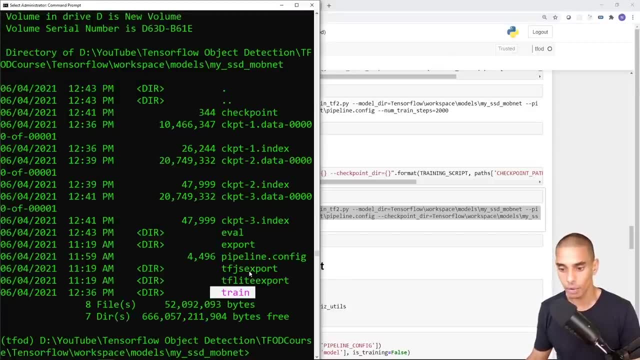 this is probably going to be right down in the corner- see my steep mob net. and now we're going to have this train folder and this eval folder. so if we go into, let's do train first because train is going to get if you open up tensorboard inside of the train folder. 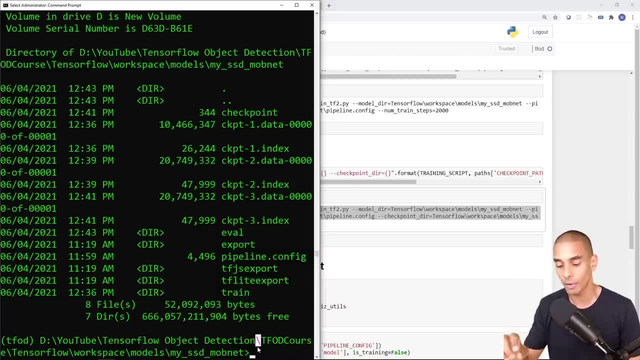 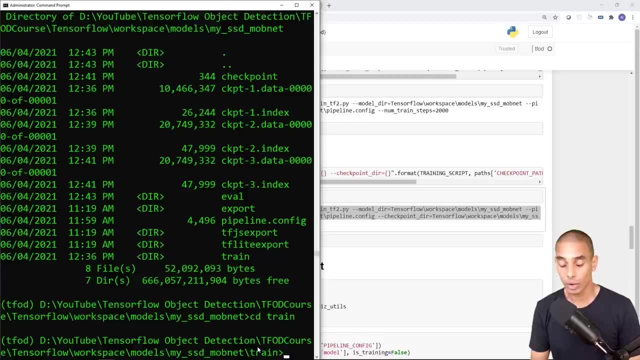 you're going to get loss metrics if you open it up inside of the eval folder. you're actually going to get your evaluation metric. so let's do our train folder, cd train, and then the command that you want to write in order to open up tense board is tensorboard. let's write that: refugees with NC2. 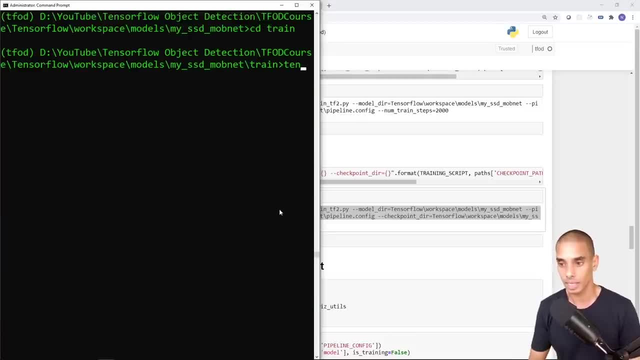 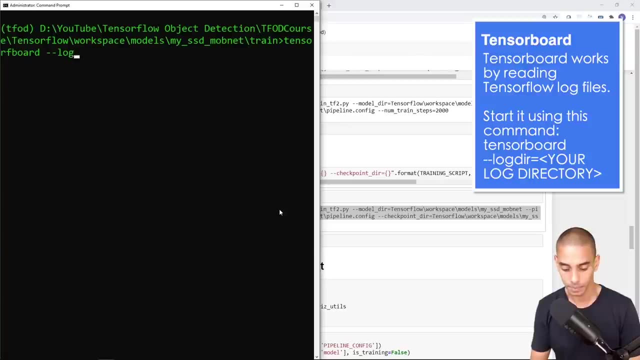 borings raining in order to open up tensport is tanks aboard. let's write a little bit of work there. of course these are barrer primary fields so you can have that in the library if you run them or call any down the bottom. let's clear this first tensorboard: dash, dash log, dear equals. 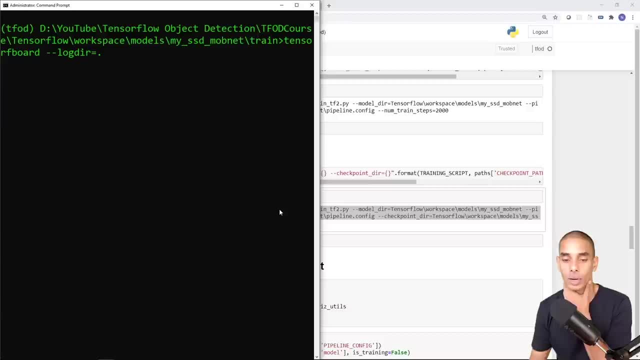 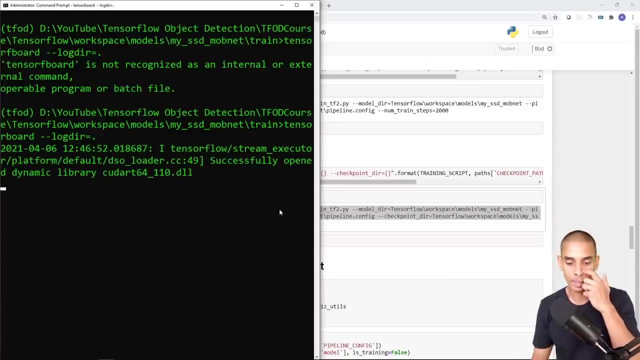 dot. so this is going to open up tensor board in the current folder. so if we do that- and I've typed in tensor board wrong- this should open up tensor board and tensor boards installed. when you install tense float, then what you can do is you can go to this URL here, so localhost 6006, and this is going to open. 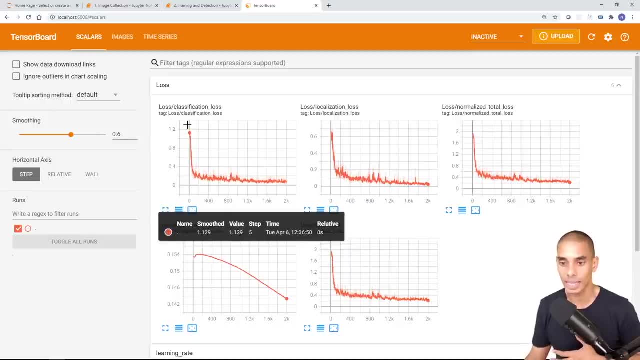 up tensor boards are through. here you can see all of your loss metrics so you can see that over time the loss is reduced. and remember, we want loss to be lower because loss, a reduced loss, indicates it's performing better on our training data. so in this case you can see our classification loss and 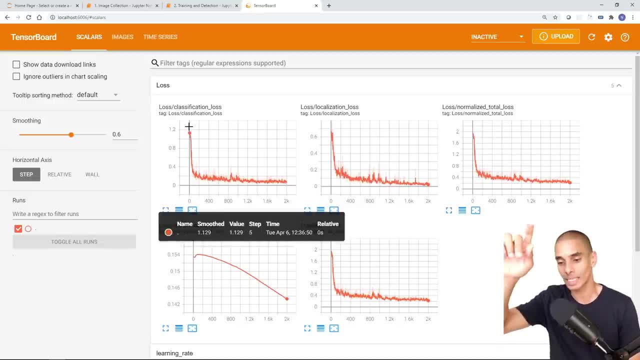 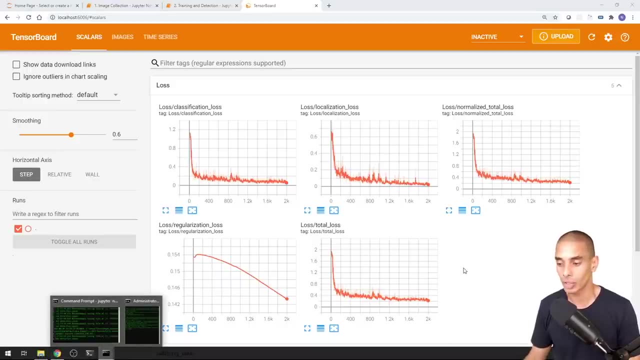 localization loss and our normalized loss. so you sort of want these to be in an inverse hockey stick trend, so starting up high and then dropping low, okay, so that's the first thing we're going to do, is we're going to go to our now. this is all well and good, but you're probably more interested on the. 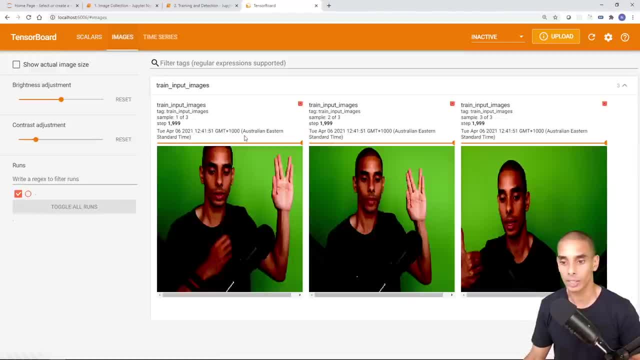 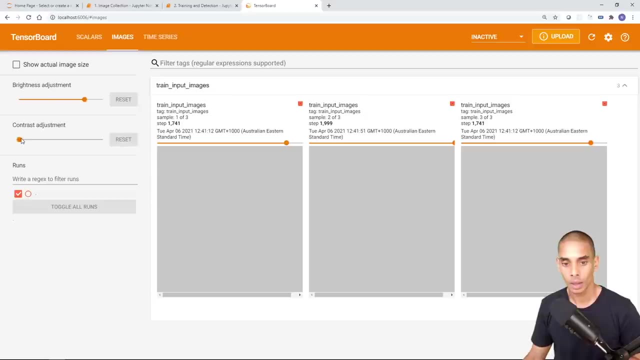 evaluation metric. so again, you can sort of navigate through this. you can also see the images that we've gone and used to our train images, and these are our different samples. can adjust your brightness, and this is just viewing them at the moment as well. right, cool, but what we actually want to do is take a 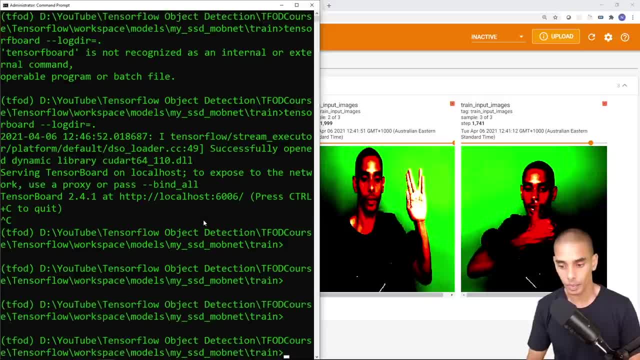 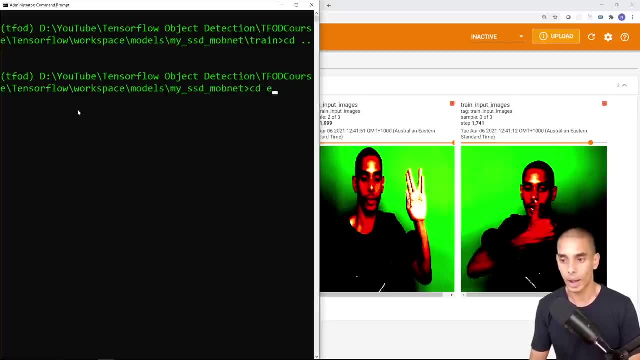 look at our evaluation metric. so if we step out of this and if we, rather than being inside of our training, we look at the make it work metric data, emergence metric, and we look back at this and if we'd like to change any of our modestly energy, this can be done. 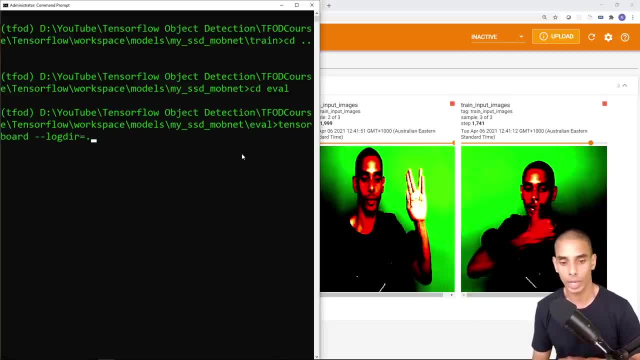 by lowerinating all of the lead. what's going to come up on the illustrations is the additional output. so obviously I can actually use this in some case. another thing I would like to do is I can use this as the main to calculate the actual lots and lots. so let's take a look at the display, gra Klima, and you can. 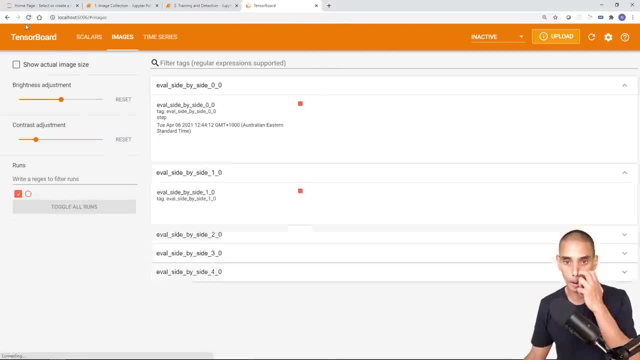 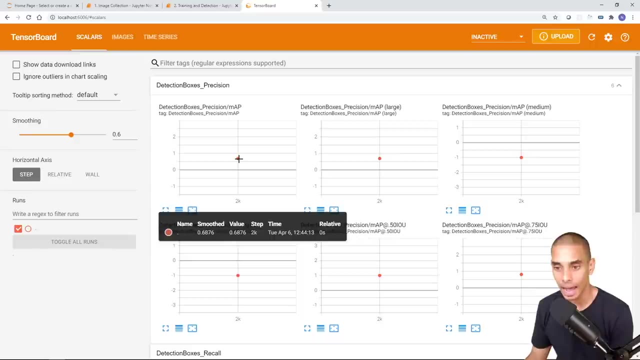 see inside of there's, as you can see here. you can see this, So we can actually just refresh this And you can see that this is giving us our evaluation metrics now, So you can see that our mean average precision is 6.876 down the bottom there. 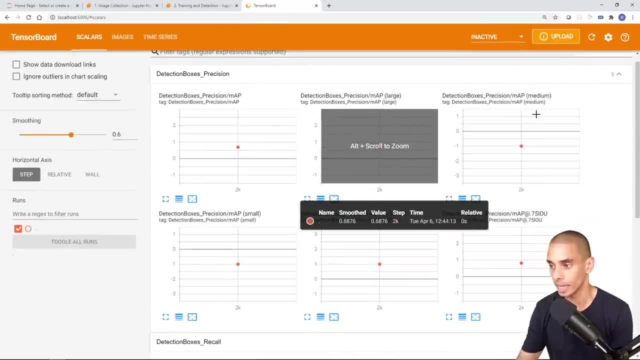 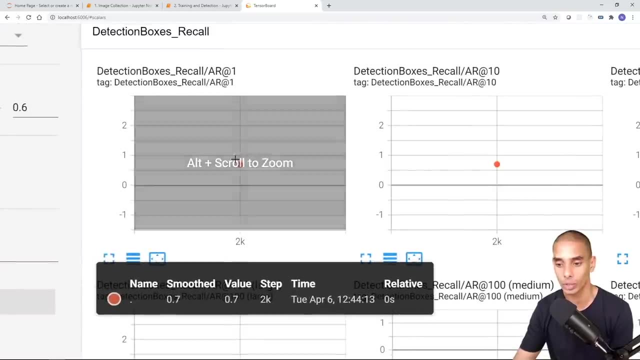 So it's a little bit hard to see. And now, what is this metric over here? This is again our precision. You can close this. We've also got our recall, which is 70%. Again, these are the same metrics that you saw when we ran our evaluation script. 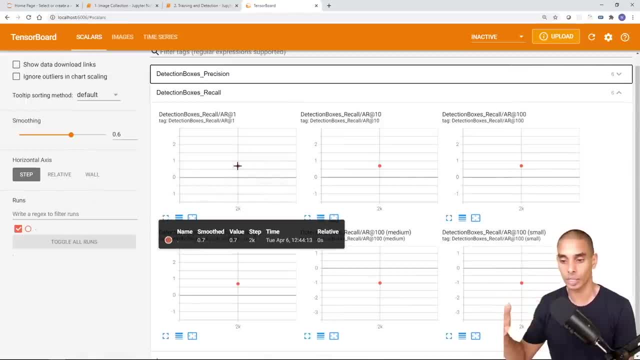 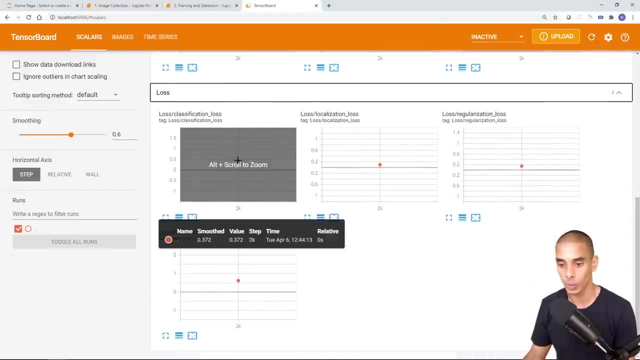 Now what we can also do is we can run this after every training run, So we'll actually be able to see what our performance looks like over time as well. So again, you've got the ability to do that. You can also view your loss as well here. 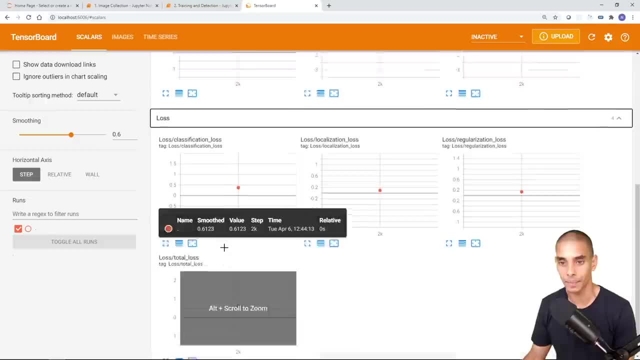 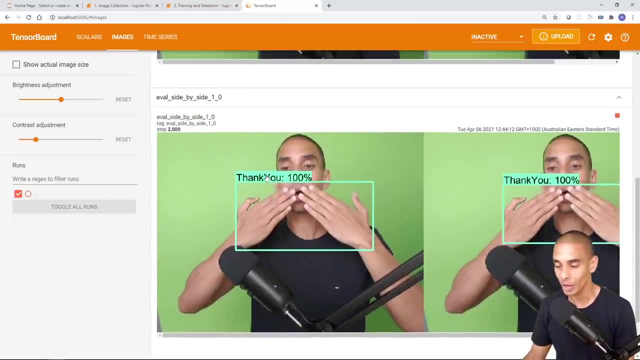 So this gives you your testing loss on these particular sets of data. You can also view your images Again. this sort of gives you an idea of our real-time performance. So again, you can see that this is what it's actually going to look like. 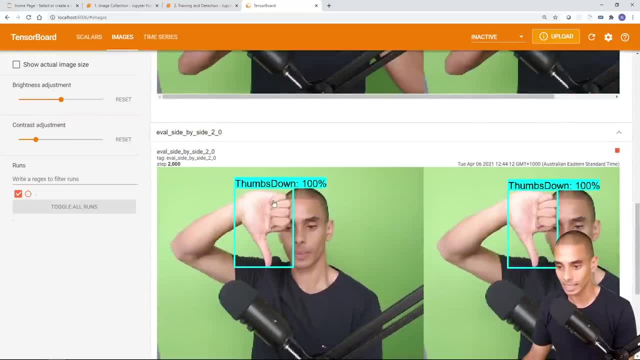 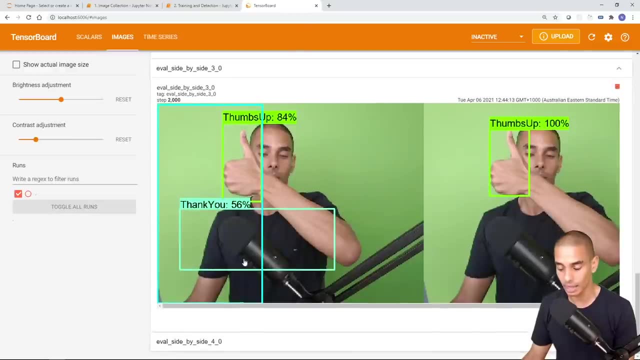 when it comes to actually go and detect our models, And it looks like it's detecting pretty accurately. So that is thumbs down. That is thank you. That is live long. This one looks like it's gone and had a little bit of an issue with thank you there. 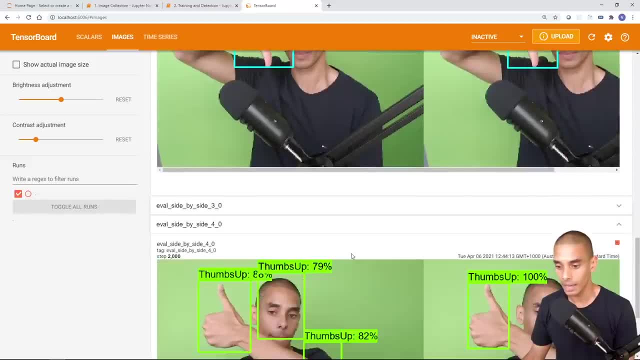 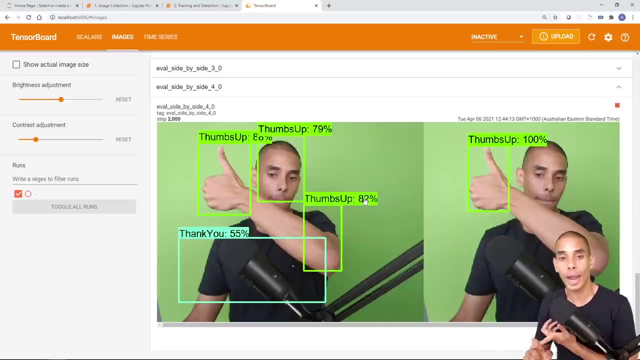 But thumbs up looks like it's performing all right, And eval side by side All right. It looks like it got a little crazy there as well. So all right. So that looks all well and good. So that gives you an idea of how to train and evaluate your model as well. 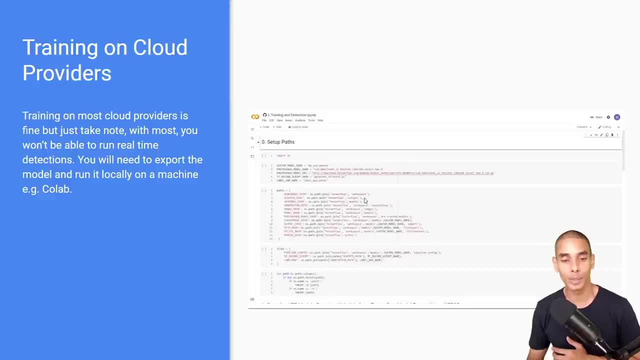 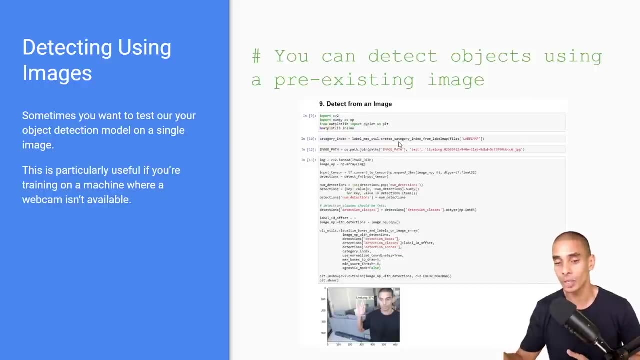 Now, on that note, we are now up to detecting objects. So, first up, what we're going to do is we're going to detect our object or detect an object with an image. So this is particularly useful if you're detecting from a cloud provider. 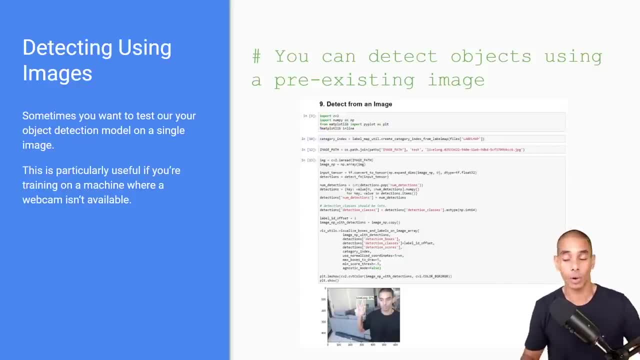 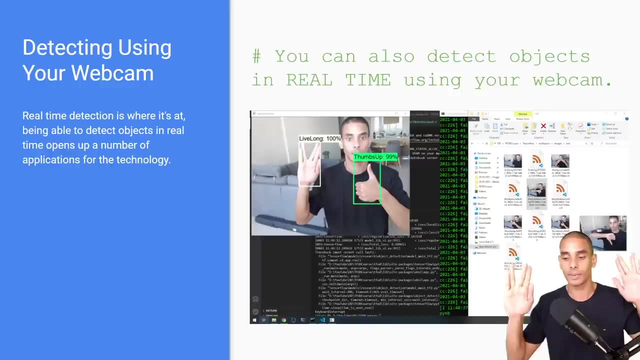 that doesn't actually have access to a sensor like a webcam or, in this case, a microscope. So we're going to detect using an image, but then we're also going to detect in real time, So we'll be able to throw up different symbols. 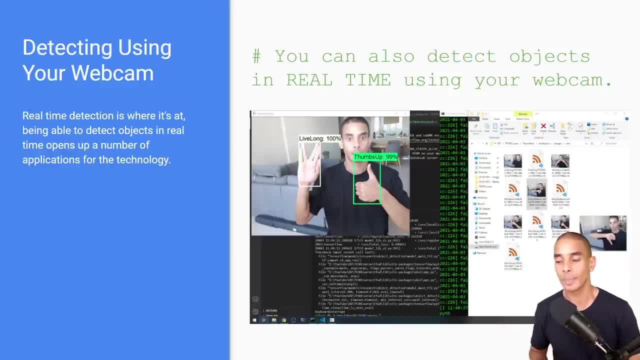 So live long thumbs up, so on and so forth, And we'll actually be able to see those detections in real time. Once that's done, the last thing that we're going to do is freeze our graph and then export. So let's go on ahead and perform our detection. 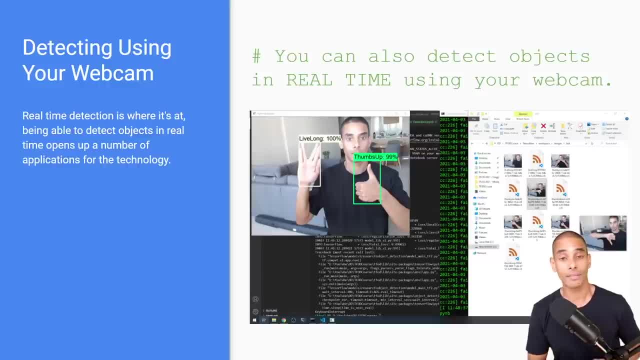 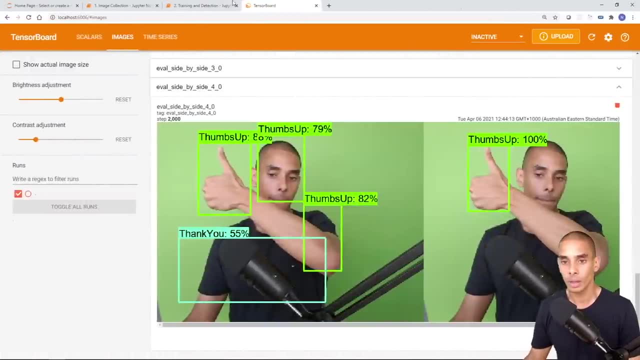 And then we'll run through our last step, which is going ahead and freezing and exporting our graph, And then we've obviously got our projects and pulling and tuning as well. So let's step back. So, again, using our same notebook, what we can do is we'll just kill off our TensorBoard. instance. 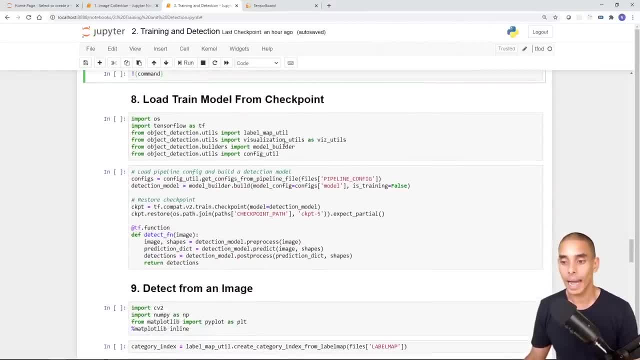 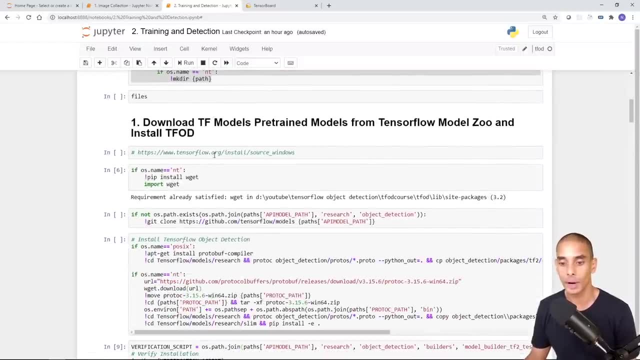 So this doesn't use up our GPU. So what we can now do is we can actually load our trained model from our checkpoint. So we've now gone through. let's quickly recap. So we've set up our paths under step zero. So we downloaded our pre-trained model and installed TensorBoard. 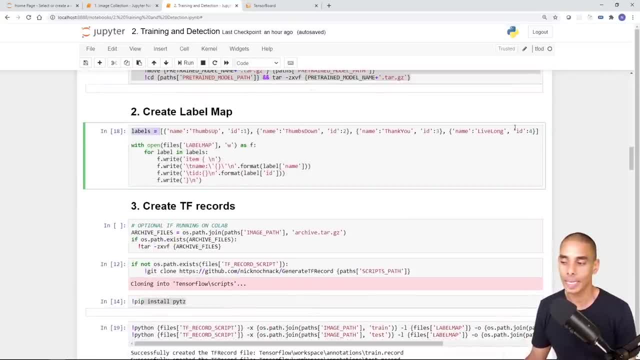 So we've set up our pre-trained model and installed TensorBoard. So we've set up our pre-trained model and installed TensorBoard. So we've set up our pre-trained model and installed TensorBoard. We created our label map And remember, this is just a set of labels that represent our different objects that we want to detect. 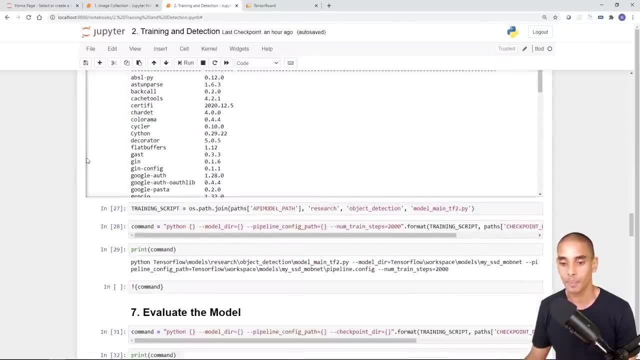 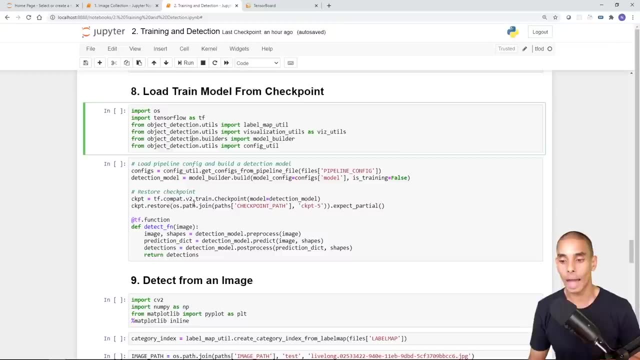 Created our TF records, copied our config and set that up. We then went and trained our model using the command prompt and evaluated as well. The next thing that we're going to do is load our model. So now, if you go into your pre-trained model folder or your trained model folder, 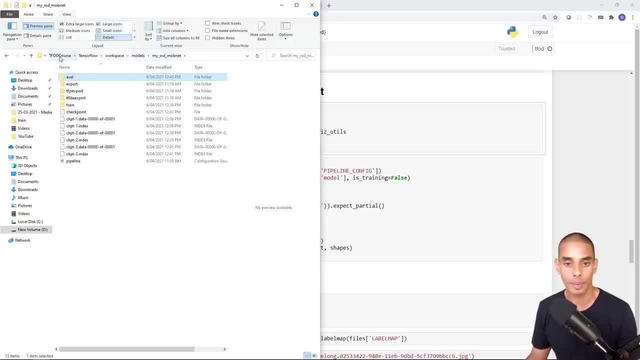 which is the MySSDMobNet folder. So remember, if we go into TFOD- TensorFlow Workspace Models- MySSDMobNet, this is your custom model, right? So everything in here represents your trained custom model. So, if you wanted to give this to someone else, 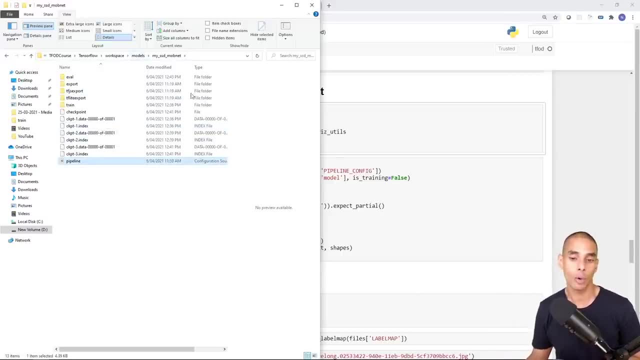 you'd be giving them this folder because it contains your pipeline and all of your checkpoints. Now, the latest checkpoint that we can see here is checkpoint three. So this is our most trained model. If you train for longer, you'd ideally get checkpoints with greater numbers as well. 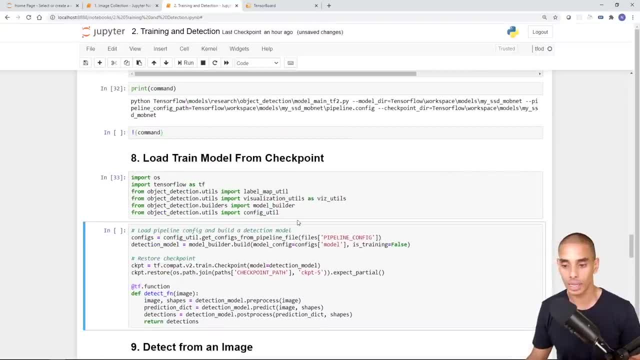 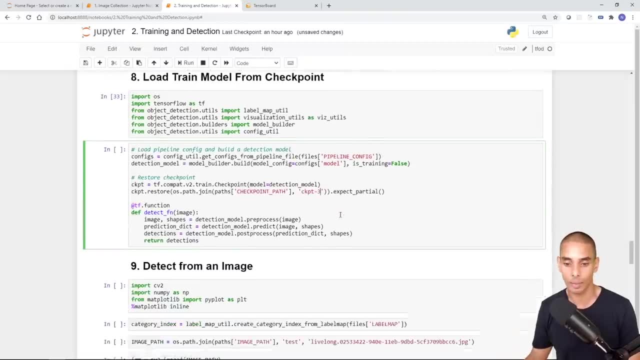 So what we're going to do is we're going to run that particular cell, So the import, And then we're going to change this line here which, you can see, says checkpoint five to checkpoint three, because that is our latest checkpoint. So we can run this and set it up. 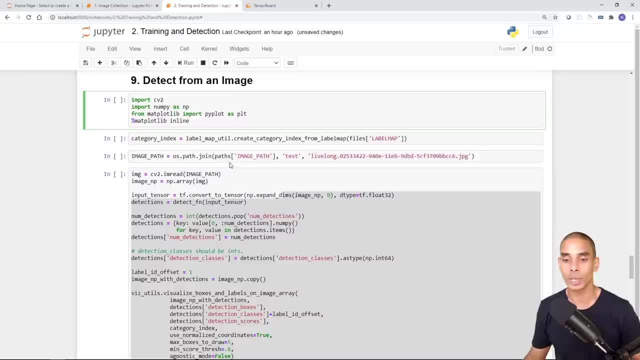 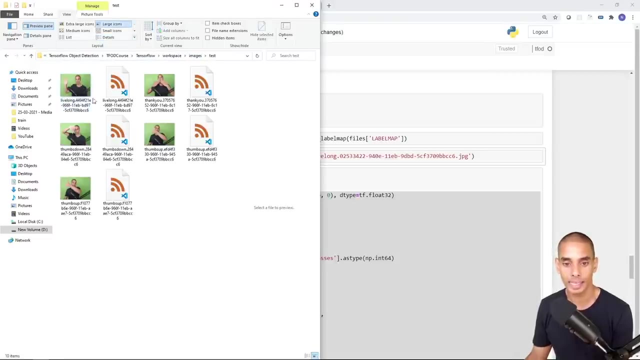 That's going to import our latest checkpoint And then what we can do is actually detect from an image. So let's go on ahead and import that dependency. under step nine, set up our category index and then we'll grab an image. So let's go into our workspace, our images, and we'll grab a test image. 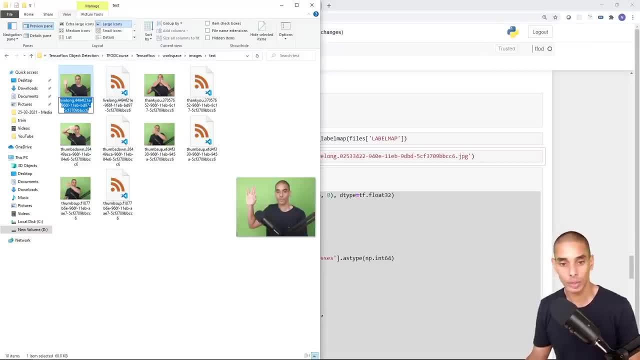 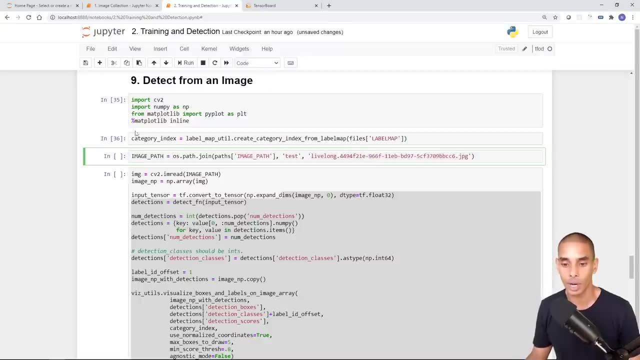 So let's grab this one over here. So I'm just going to grab the name of that image and I'm going to replace it over here, Right? So basically inside of this line here. So under step nine, we've got the third cell, which is image path equals OS dot. 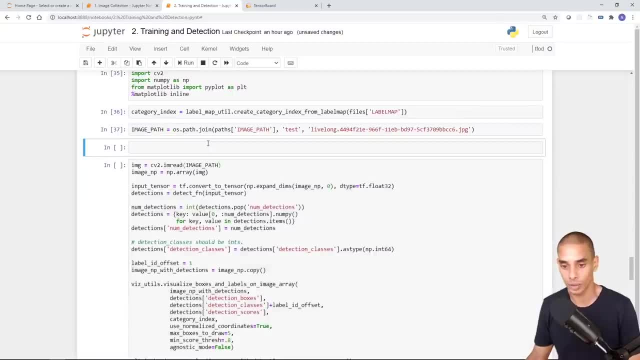 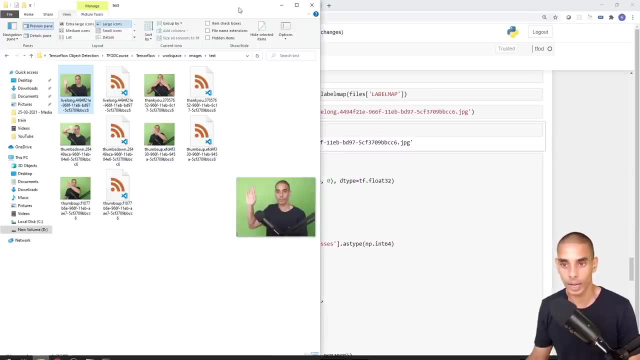 path dot join. We're basically just resetting the path to that image. So if I type out image path, now right, It's just the path to that particular test image that we had there. So if I go and take a look, so basically the full file path. 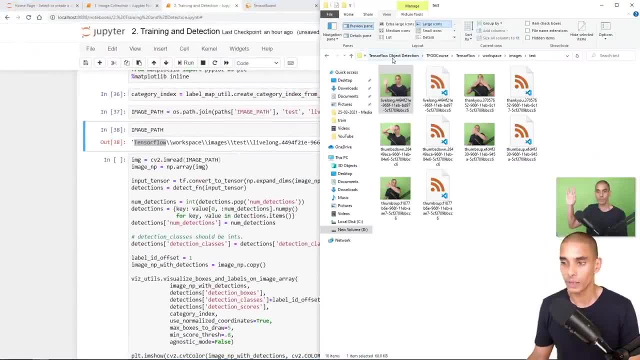 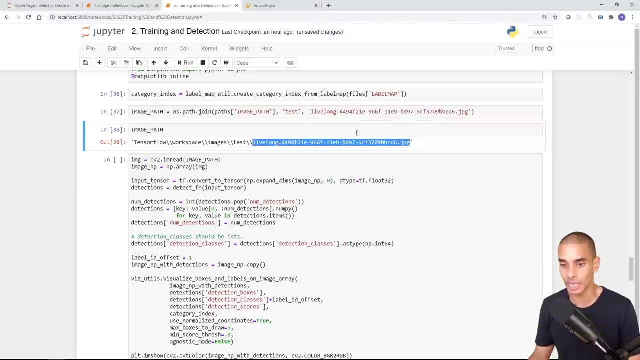 is tense flow object detection, TFOD course: tense flow workspace images tests. tense flow workspace images tests and then that particular image. So we're good to go. So now what we can do is run this cell and this is actually going to run object. 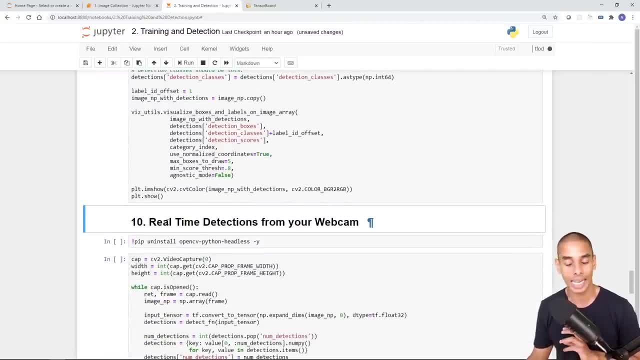 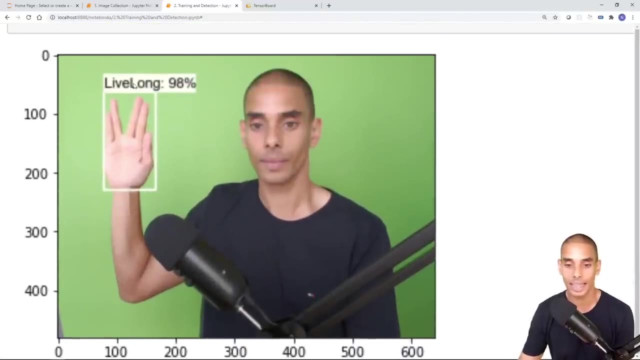 detection on that image and print out our results, which we should see here in a second. So let's give that a sec And there you go, So you can see right Down there it's gone and accurately detected that that particular symbol is live long with a 98% confidence metric. 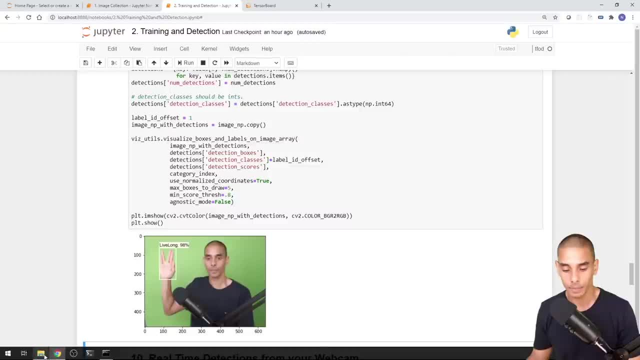 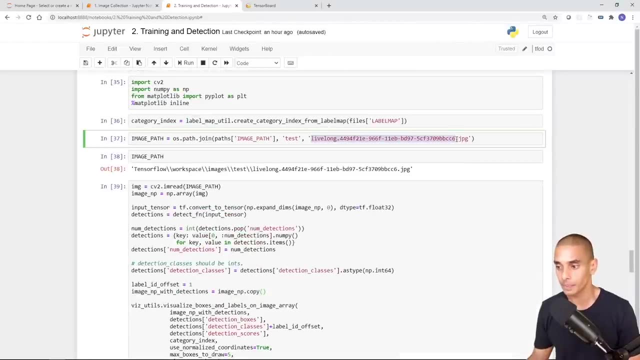 So again, we could do this on a different image if we wanted to. So let's grab another one. Let's grab, Thank you. So if we grab that label, we'll grab that image name and replace this. Run this again. 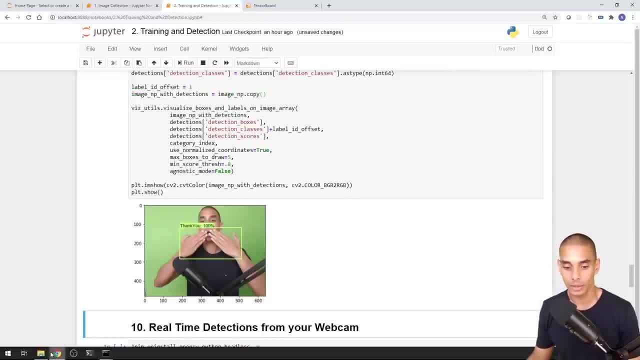 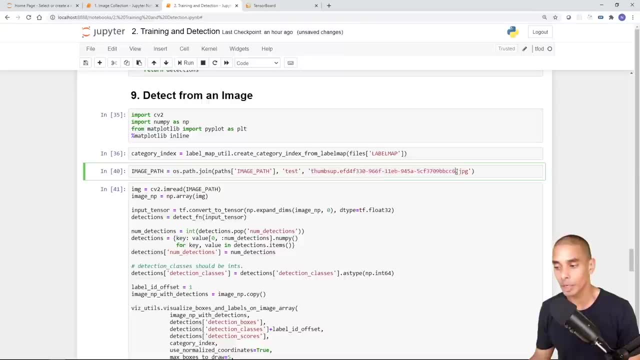 We can delete that now. So again, that's detected. Thank you successfully. Let's try another one. Thumbs up. So again, all I'm doing is I'm Changing the part to that image. You had your images somewhere else. 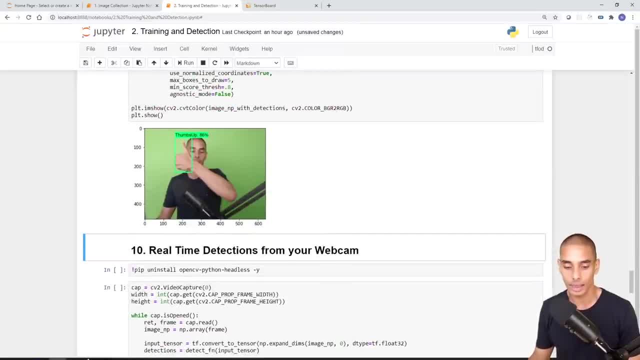 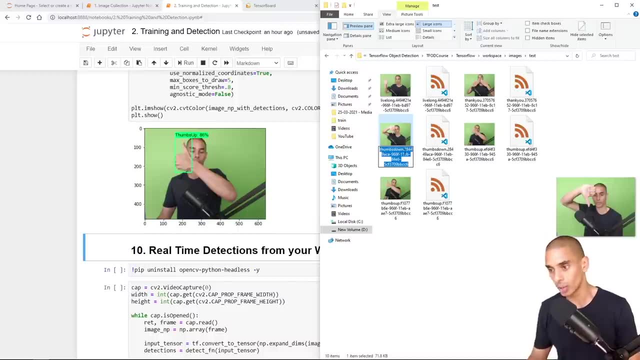 You could do that as well. So it's it accurately detected. thumbs up: 86% confidence. So not the greatest. on that one, It's thumbs up. Thumbs up was the one that we took new images of as well, Wasn't it? 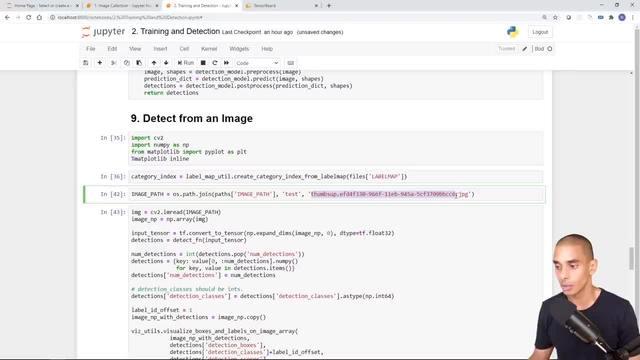 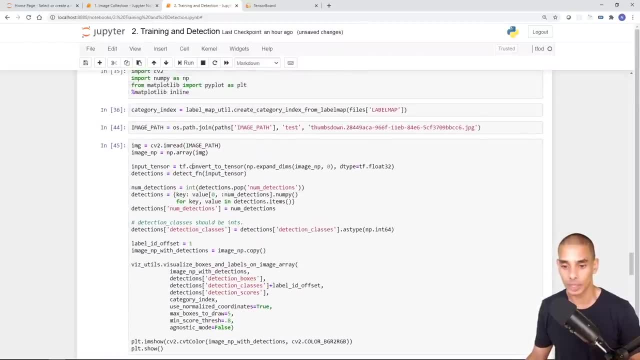 So again, we could performance stream there and let's do thumbs down. Okay, So not too bad. So a hundred percent on thumbs down. So that gives you an idea of how to do it with images. Now, basically, what we're doing here is we're loading the image into Python. 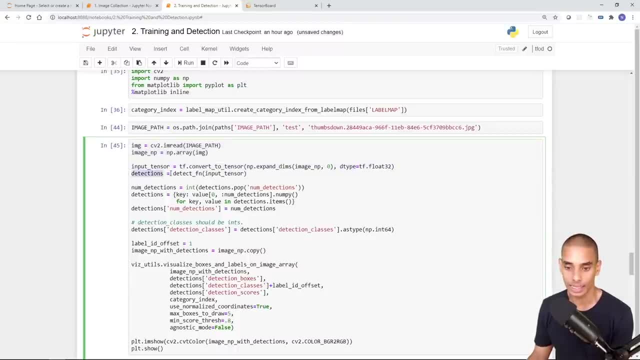 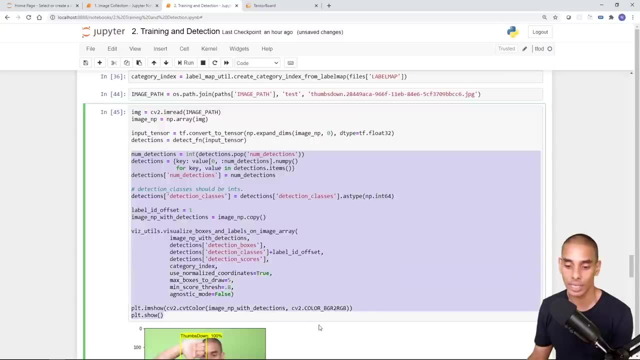 We're creating it or converting it to a tensor and running our detection. So this line over here is actually using our detection function, which we imported, And then it's going ahead making those detections and then visualizing it. So again, if you'd like to see me explain this in more detail, or maybe even code it, 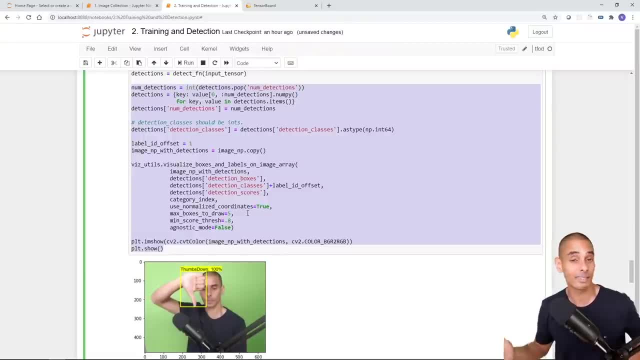 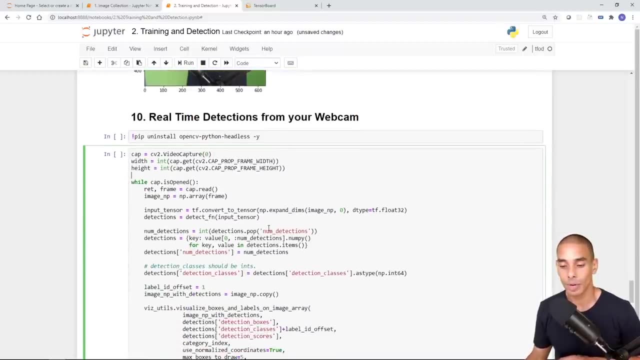 up from scratch. by all means, do leave a mention in the comments below. I'd love to hear your feedback. Okay, So those are our detection. So that's all great. Now the next thing that we actually want to do is make some real time. 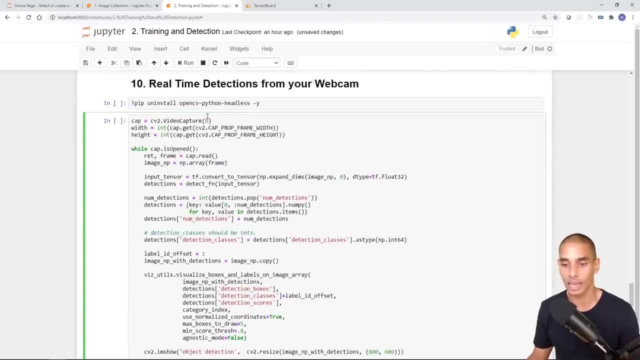 detections from our webcam. So let's go on ahead and run this cell Under step 10.. Now I'm going to not run this cell, which is pip. uninstall open CV. dash Python, dash headless, dash Y. We'll come back to that in a second. 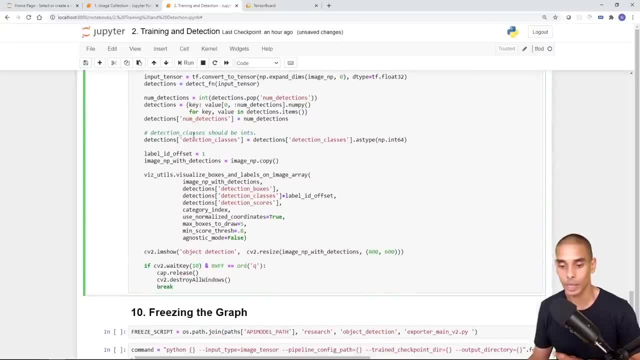 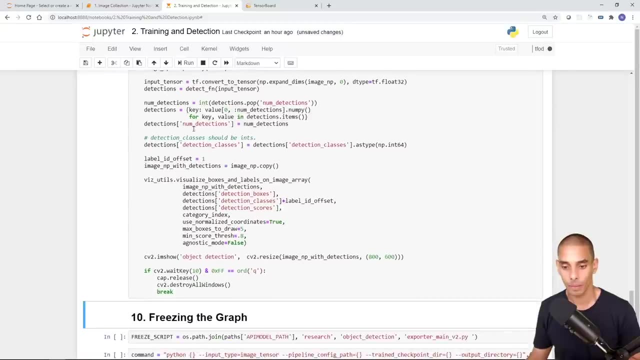 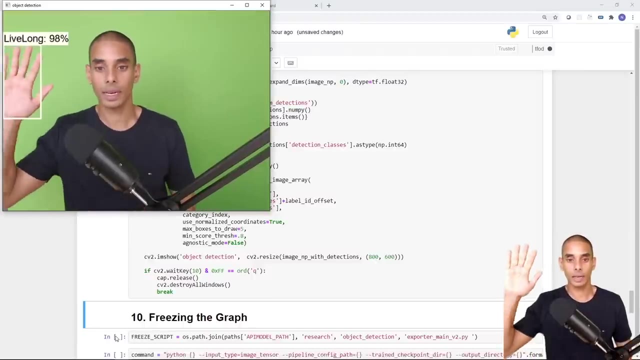 And that's normally a resolution to a pretty common error. but let's go on ahead and run our real time capture and see how we go. So it looks like it's running Okay. So it looks like it's got our feed. That's got live long. 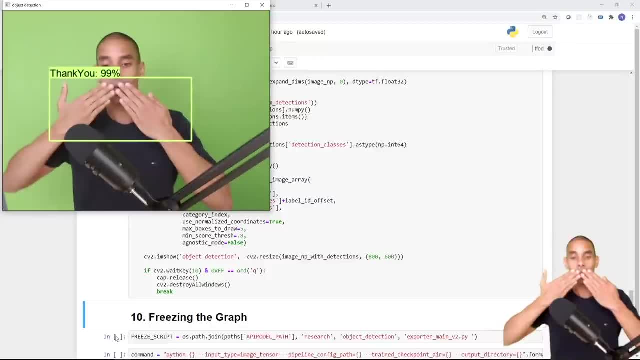 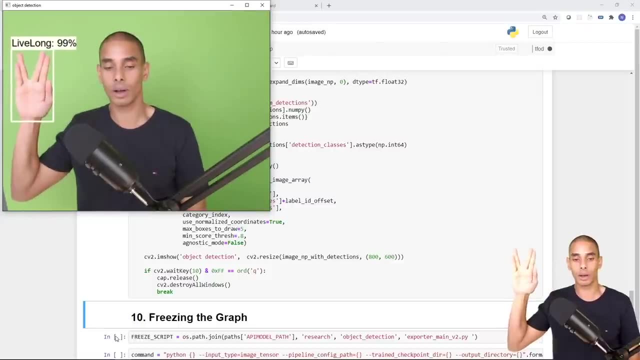 Thumbs up, thumbs down. That's actually really really good. considering we only trained for 2000 steps with not a whole heap of images. That's actually performing really well. So live long thumbs up, thumbs down. Thank you. 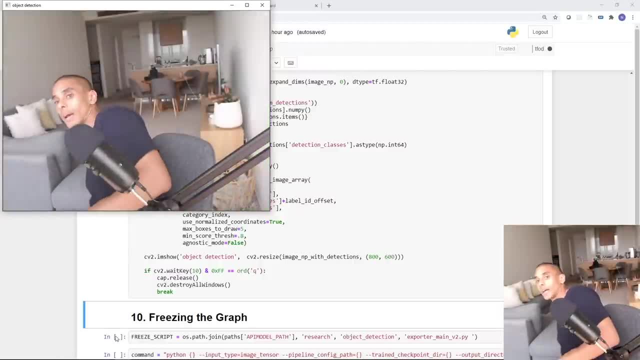 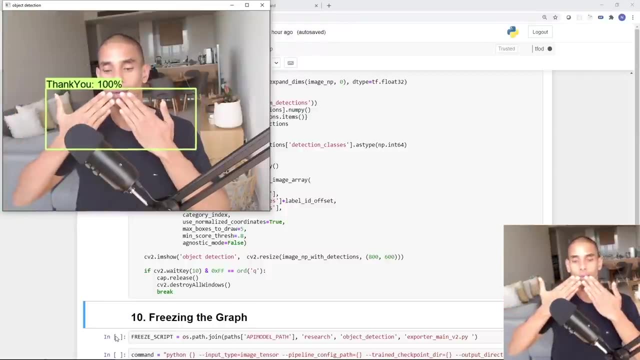 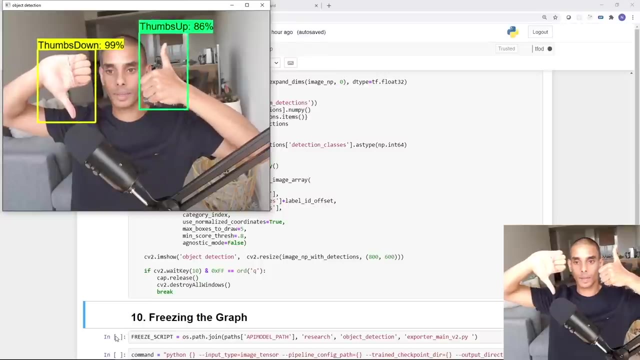 Let's see what it looks like with the green screen down Cause. remember we didn't train with this. So live long, still performing well, thumbs up, thumbs down, Thank you. What if we did a joint? Okay, So thumbs up. so thumbs up is not performing the best, but if we did, live long, you can. 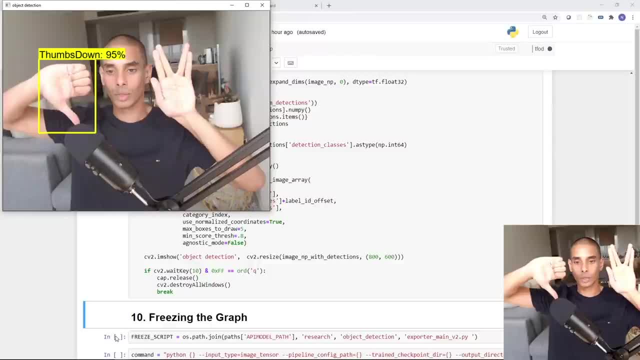 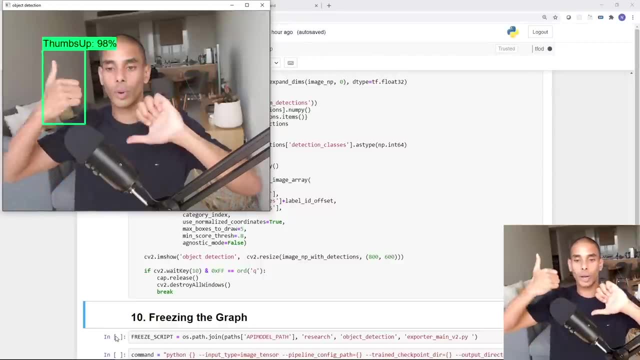 see there that because we maybe haven't done too many images trained on, So let's do thumbs up, So all right. So again, so you can see that the performance isn't so good when we try to change it or use different hands. 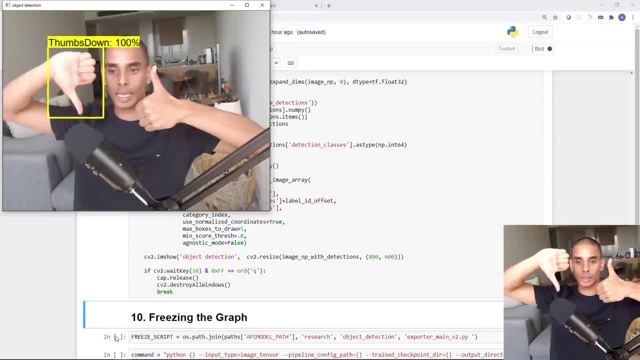 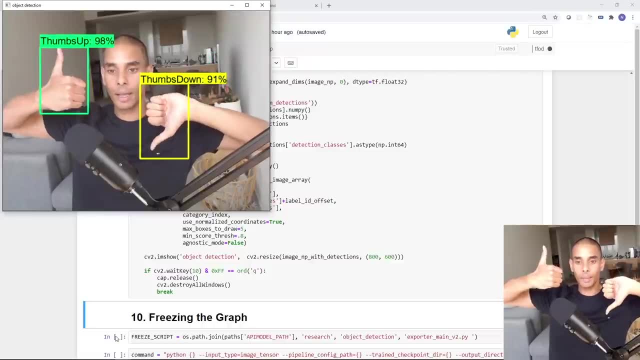 So okay that maybe that's performing not too bad. So thumbs up isn't performing well with this particular hand, So again, we might add some additional images. We might add images. Okay, We might add images of each hand. but again, that's performing reasonably well. 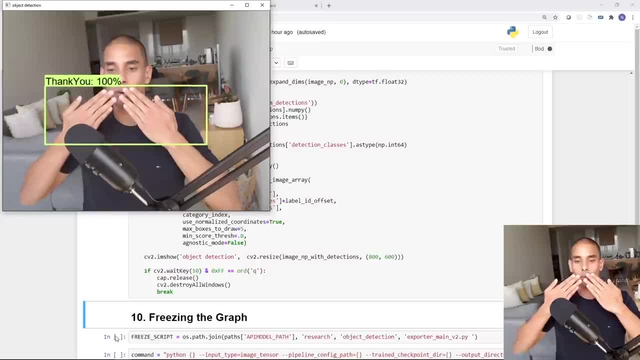 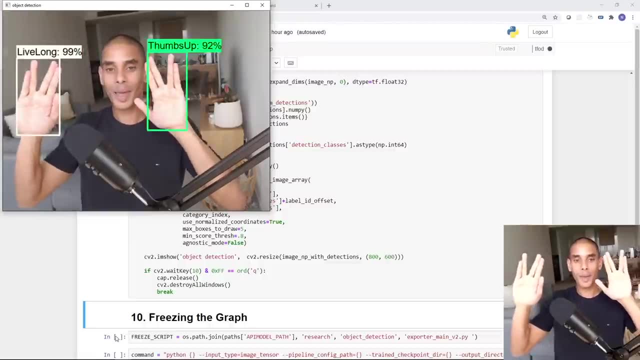 Right And like this is jewel hand right now, So it's, it's not too bad. Thank you for me. Okay, How about live long to live long on this hand? Yeah, pretty cool. That sort of gives you an idea of what's possible, right. 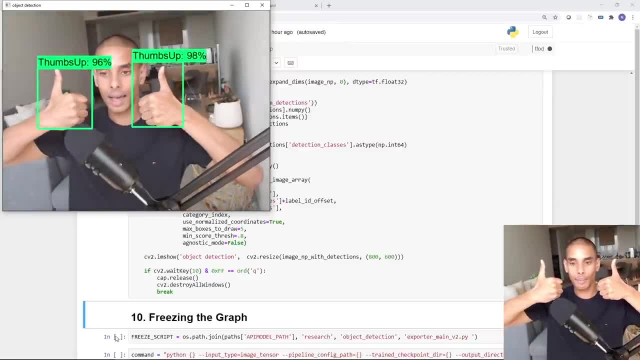 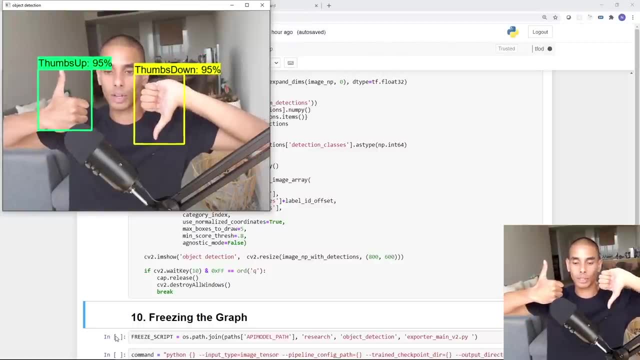 So like, really, really quickly, we've built an object detection model That's able to detect a bunch of stuff. So thumbs up is perfectly fine. What was it, The thumbs down? Okay, It's not so bad. Maybe it's needs to be a little bit closer. 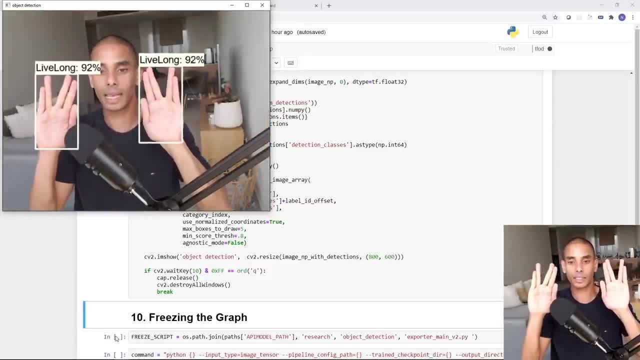 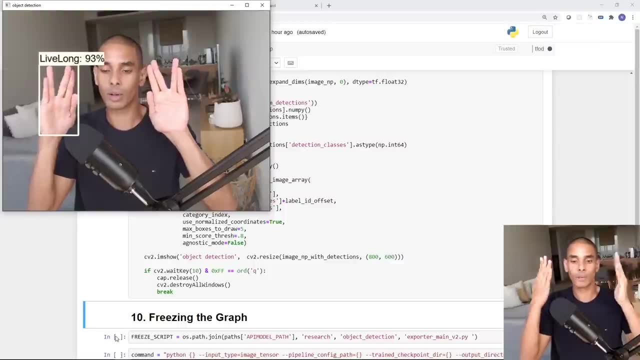 Closer to the camera. But again, these are the things that you could additionally train for So we could add more images of closer to the camera. We could add more images of this hand doing live. long Sort of gives you an idea of how you can performance, tune and update your model to be able to perform. 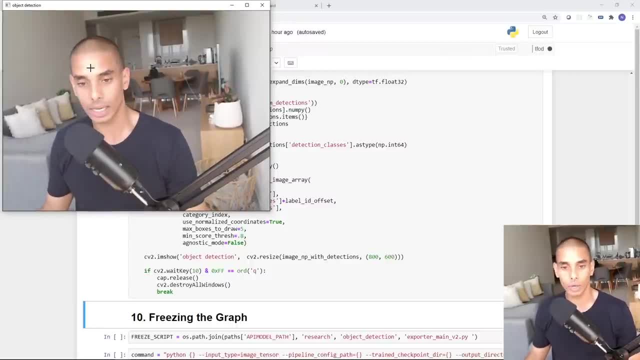 better. Now, if you want to quit out of this, all you need to do is hit Q and that's going to close it off. But again, that's what. it gives you an idea of what's possible with real time object detection. 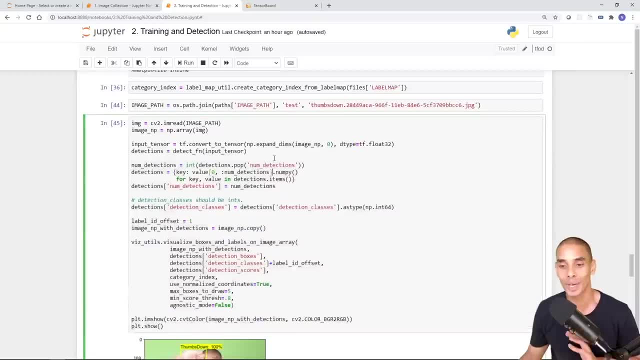 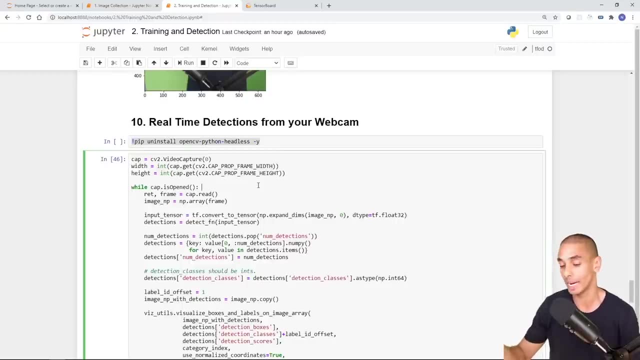 Alrighty. So we've now gone And also made detections using an image as well as using a webcam. Now you can also do this with an existing video feed or an existing video. If you'd like to see me do a video on that, by all means mention it in the comments below. 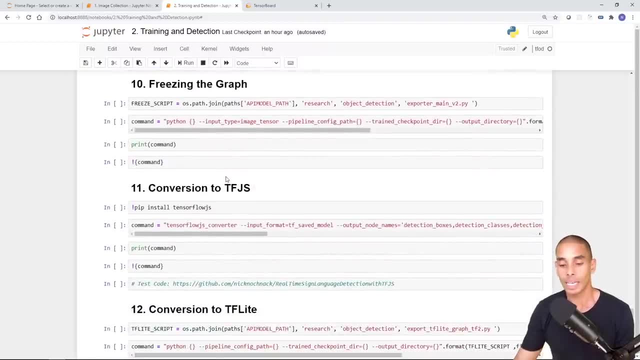 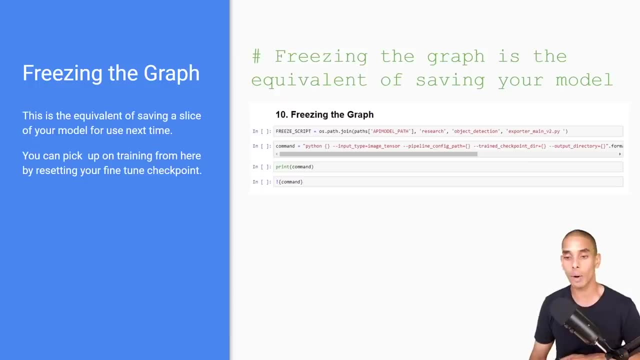 I'd love to hear your feedback. All right, So this brings us to freezing and conversion. So part five, freezing and conversion. So now what we're going to do is freeze our graph And again, as I was sort of saying, freezing your graph is the equivalent of 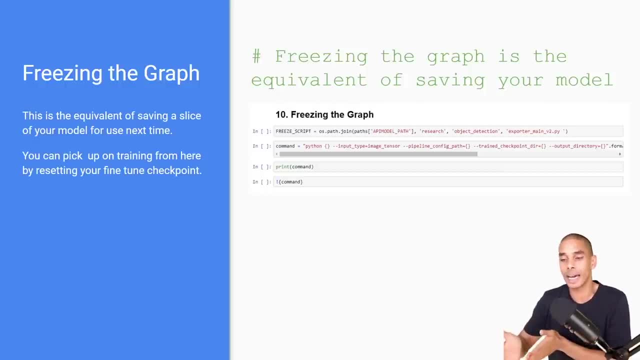 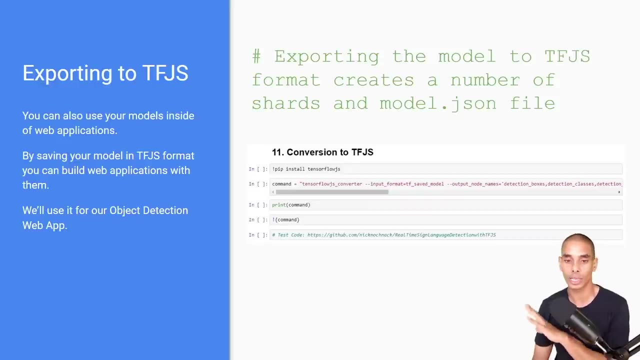 Saving- saving a slice of your model or effectively saving it down so that you can use it next time. So we're going to freeze our graph. We're also going to export it to TensorFlow JS So if we wanted to use it later, and we're also going to export it to TF flight and we'll eventually use this in our Raspberry Pi project. 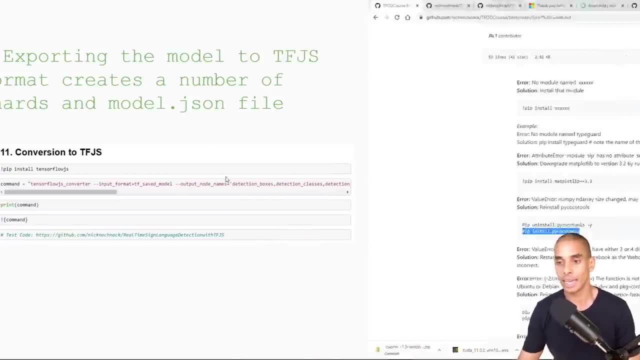 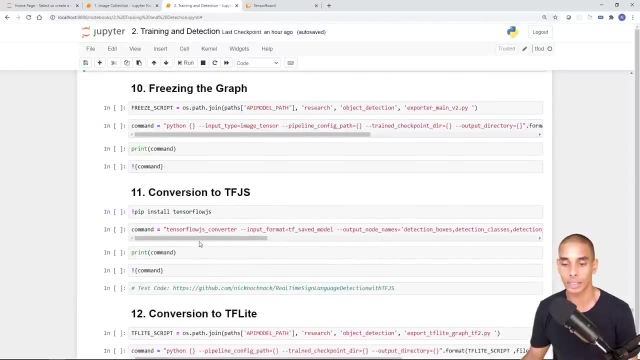 We use our TF JS export for our web app. Now, these are all reasonably straightforward, So I've just got step 10,, 11, and 12.. All you need to do is run through these and it's going to freeze your graph. 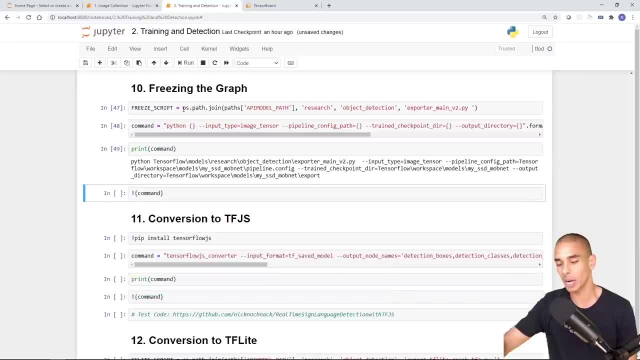 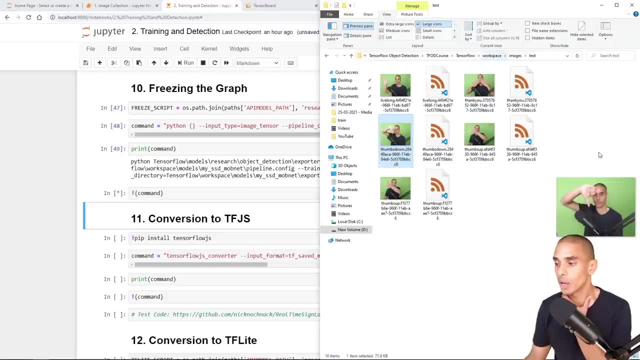 So let's go ahead and run this- And I'm not going to copy this command outside of the notebook, It's probably just easier to run it here- And once you've frozen your graph, this is going to appear. let's just make our mouse work. 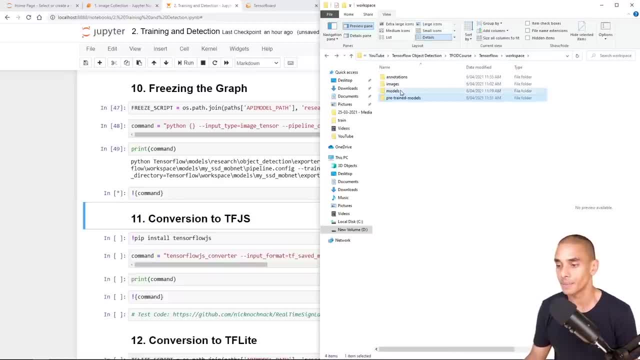 This is going to appear inside of our export folder, So ideally, what you should get is inside of. if we go back to our root, so TensorFlow workspace models, my SSD mobnet- inside of our export folder, we're going to have our frozen graph made available. 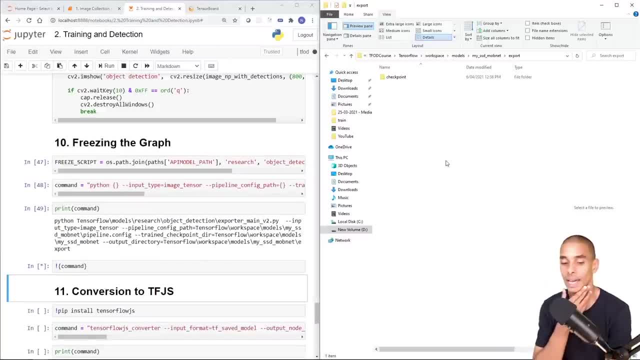 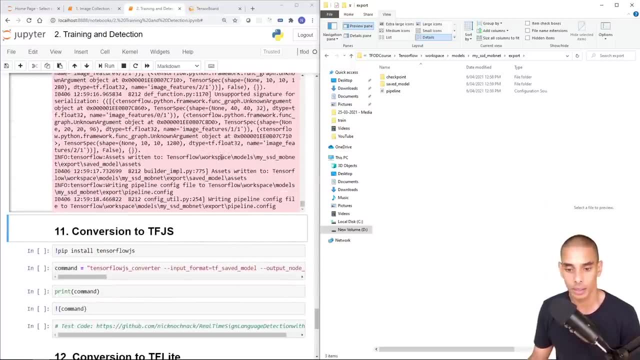 So let's give that a second. So again, this might take a little bit of time to run And so that looks like it's now complete. So let's just check. Doesn't look like any errors there And you can see that you've now got your checkpoint, your saved model assets variables and your saved model dot protobuf file. 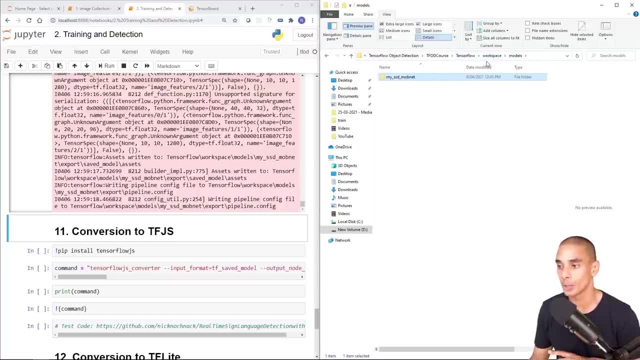 Now, if you remember correctly- you remember how I said that we were going to create a similar output to what we had for our pre-trained models. You can see that we're now doing the exact same thing, Okay, Okay. So we've now created our own slice of our own custom model, which looks almost identical to what we had from our pre-trained model. 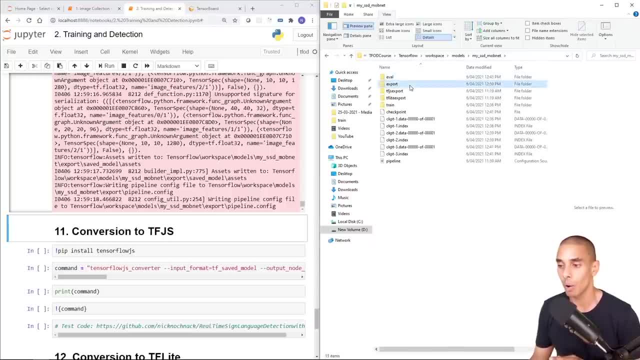 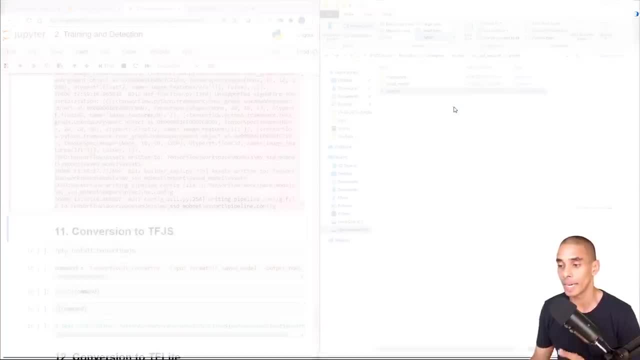 But now again, this is based on our custom model. So again, we've got all of that available inside of our export folder. So we've got our checkpoint, got our saved model and we've got our pipeline config and this will mimic exactly what we had for our custom one. 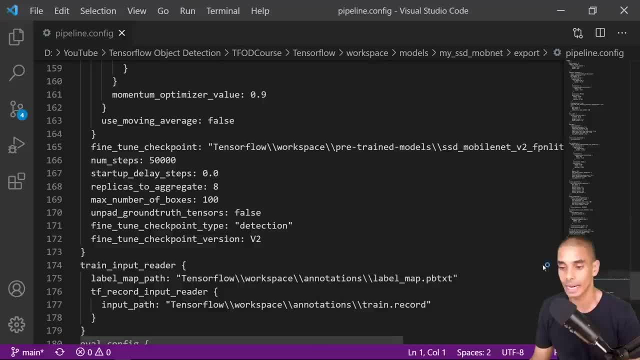 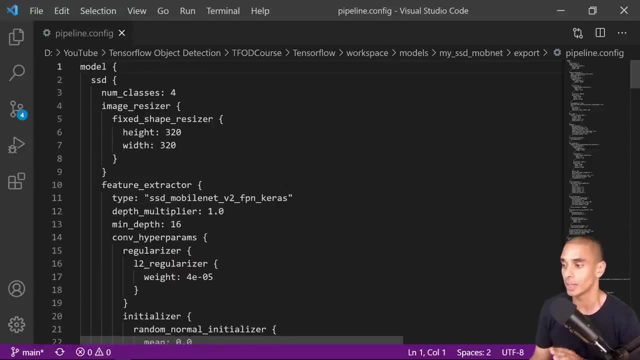 So if I scroll down again, so this is currently still pointing at our own file folders, but you can see that you've got all of the stuff that you custom built for your own model right, So this is now available to be used elsewhere. 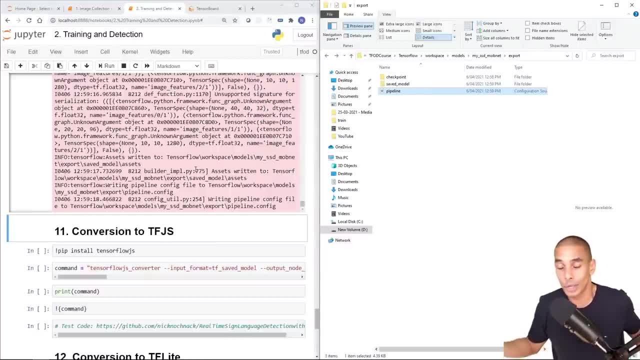 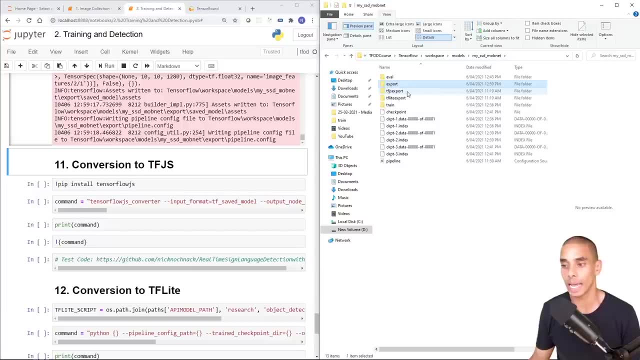 So you could actually go and convert this, which is exactly what we're going to do, Um, but again, you could pass this off to someone. they could pick this up and use it as well. Now, the next conversion that we're going to do is we're going to export this to TFJS. 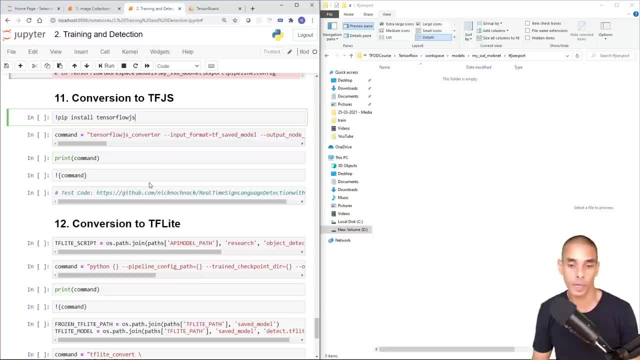 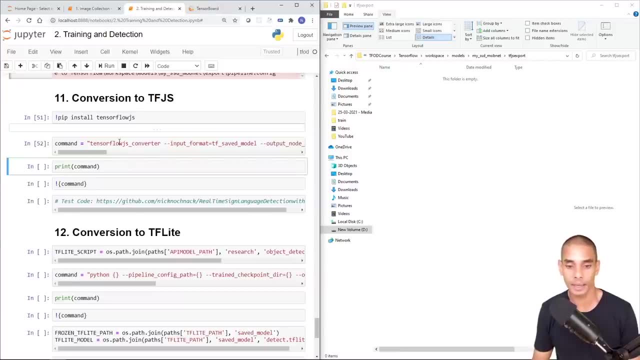 So if we go and run all the steps beneath step 11, so first up it's going to install TensorFlowjs converter or the TensorFlowjs converter, And then again it's going to create this command, print it out and then it's going to run it. 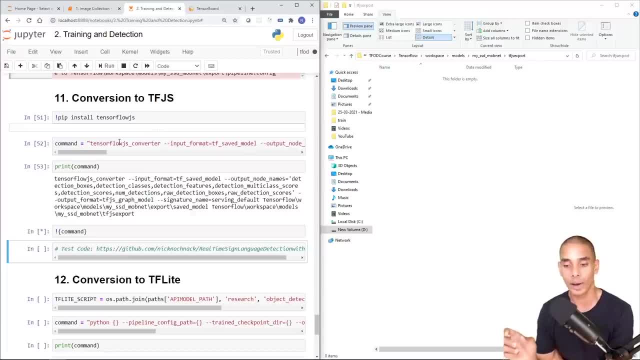 So ideally, this should create a modeljson file and a number of bin folders, And I'm going to show you how to use this inside of our projects. but for now, we're just going to convert it and we'll be able to leverage it later on. 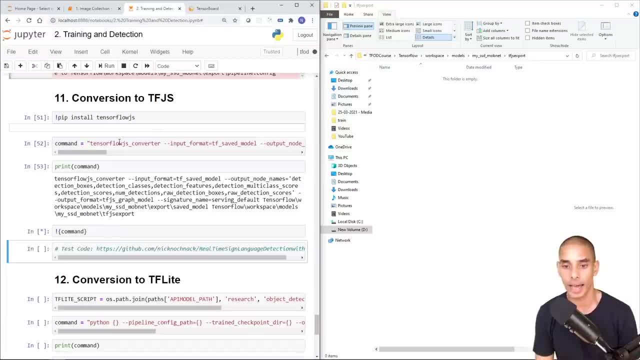 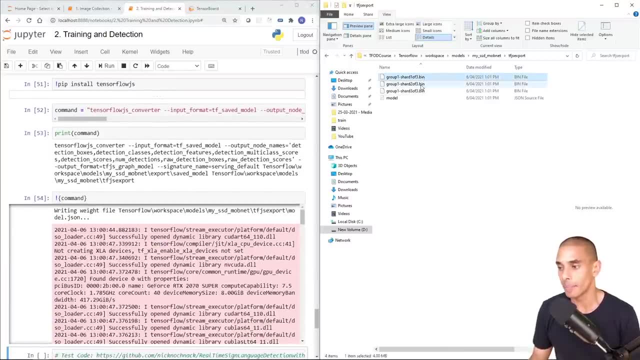 So give that a couple of minutes and you should effectively have your converted TensorFlowjs model. And there you go, So you can see that we've now got our bin files, So we've got our different shards and we've got, We've got this modeljson file, which is huge. 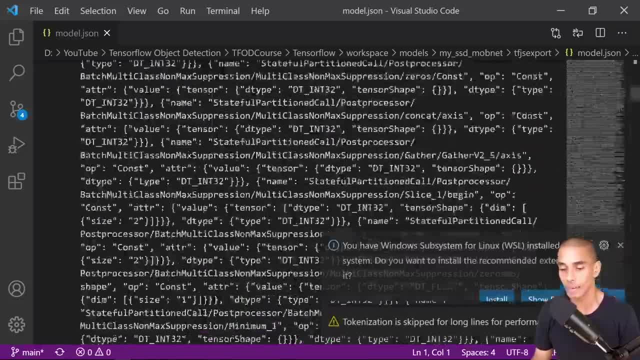 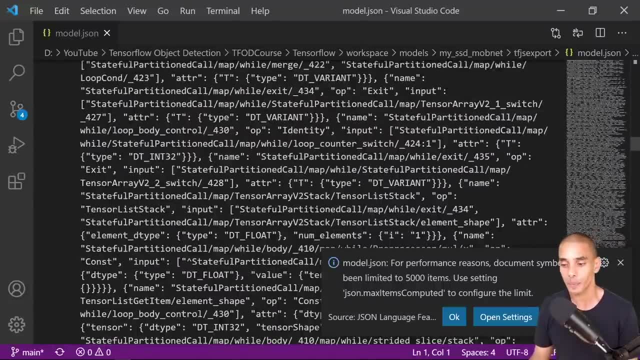 So if you actually scroll through this, this represents our entire deep learning model in JSON format. Now, when we load this into our React app or into our TensorFlowjs app, which is in JavaScript, but again, I've written all that code for you. 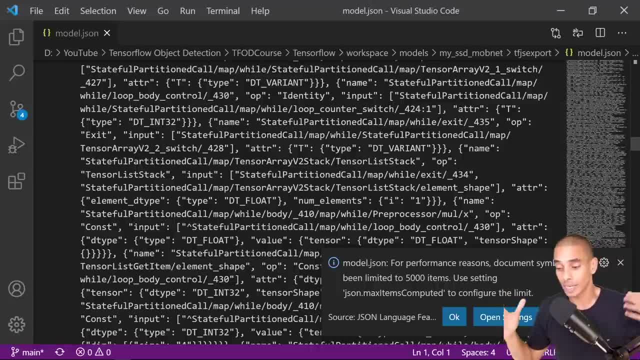 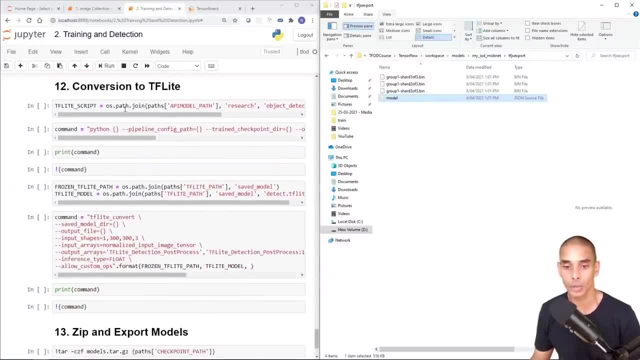 You just need to paste it in there. This effectively represents the full architecture and the weights and everything, which is actually pretty cool. Now the last conversion that we want to do is conversion to TF light. So again, same sort of deal, except this: 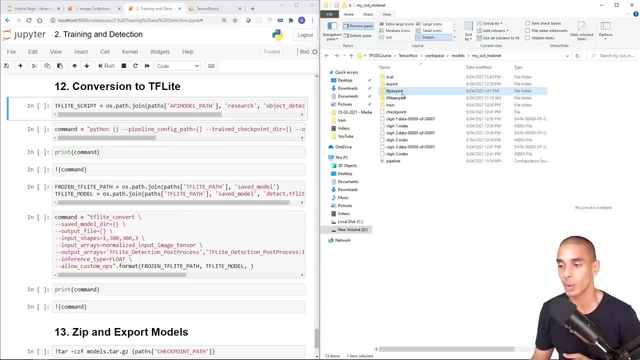 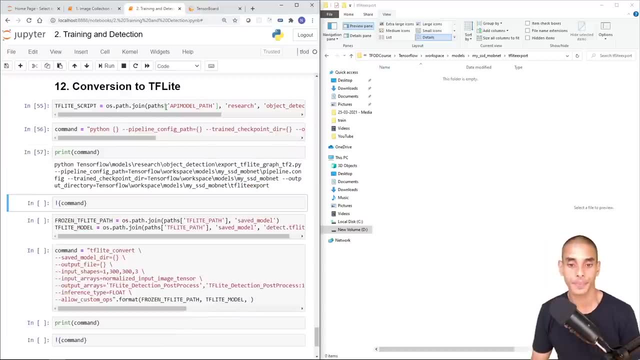 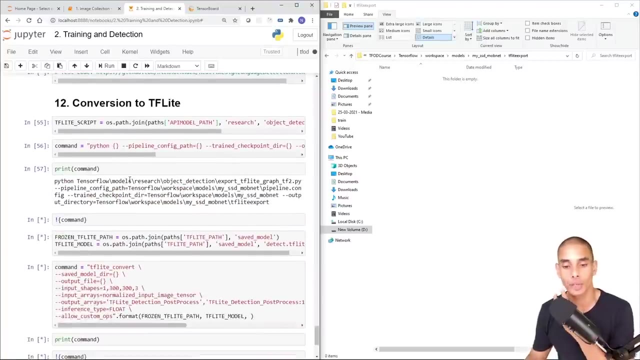 Time, rather than our exports being export or TFJS export, we're going to export into TF light export. So again, let's just go on ahead and run these commands. So the TF light conversion takes two parts. So first up, we convert it to a. what was it again? 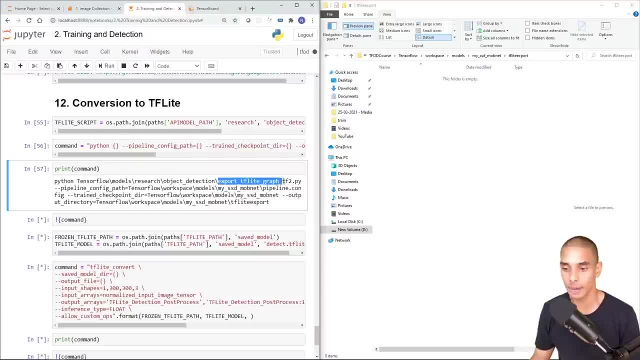 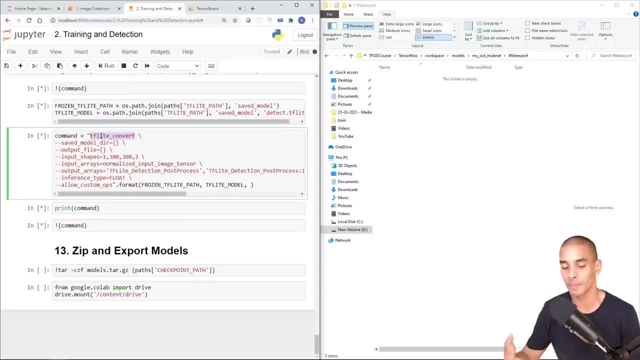 So we export it to a TF light graph And so we do it using this command and then we go and actually run it using the TF light converter. So this is again a slightly separate app, but again you don't need to worry too much about this. 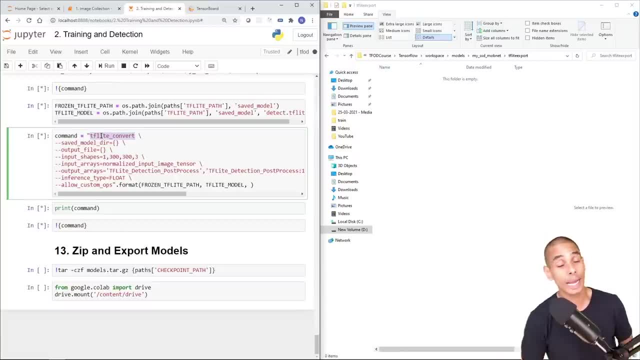 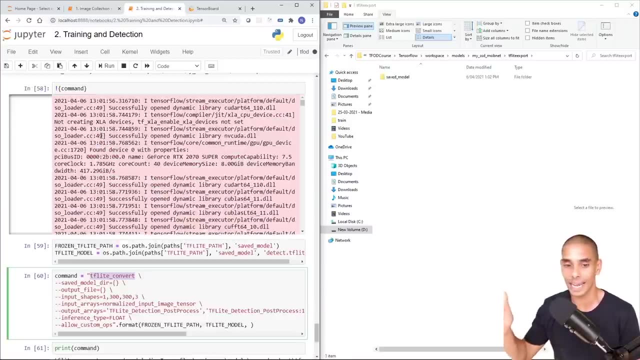 It's actually just going to convert it and output it to exactly the output that you need to be able to go and leverage that. So let's let that run. And that brings us to the end of this end to end model. So you can see it will now gone and converted and it's still running. the second part: 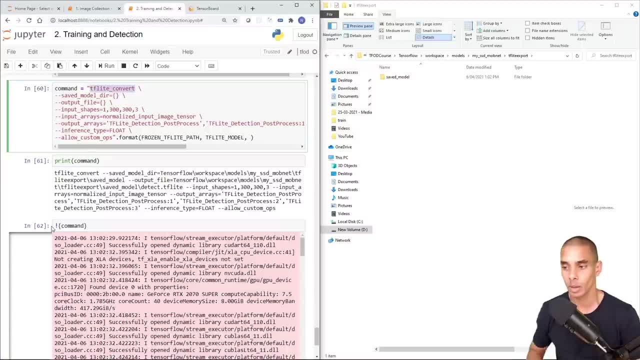 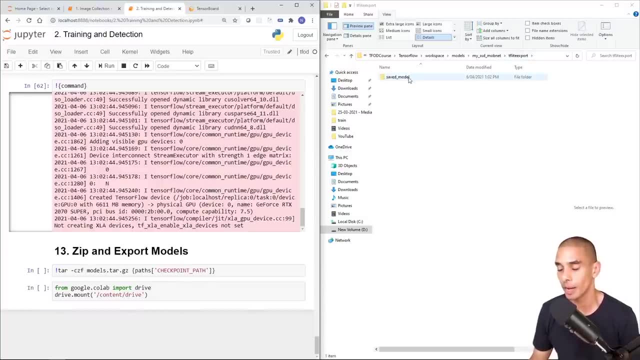 So let's give that a sec. Perfect, And that looks like it's gone and effectively finished. So now, if you go into this TF light Export folder, double-click save model, you've now got this folder called detect dot TF light and that is your TF light export. 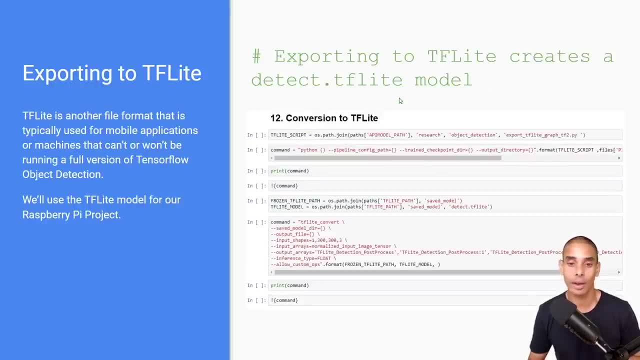 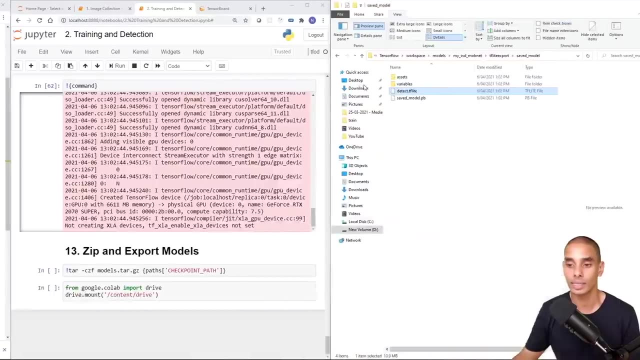 So that about brings us to the end of our conversion. So we've now gone and frozen our graph, exported it to TFJS and exported it to TF light And it also brings us to sort of the end of our full run through of actually working with tense flow object detection. 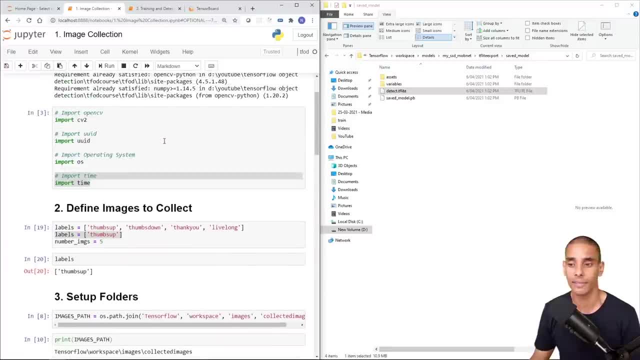 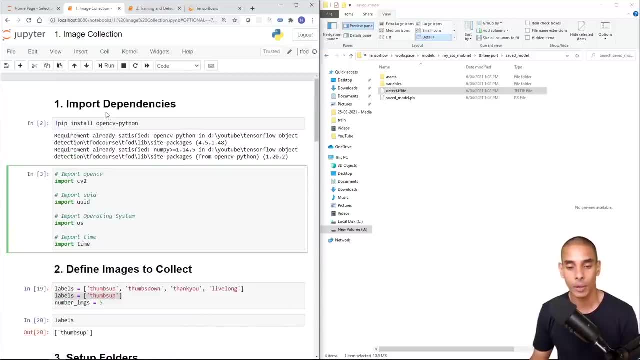 So, all up, what we did is we set up all of our stuff and installed all of our stuff, All of the tense flow object detection dependencies. We set up our virtual environment, which is called TFOD. We imported our dependencies, defined our new images to collect, set up our folders, captured our images and labeled them. 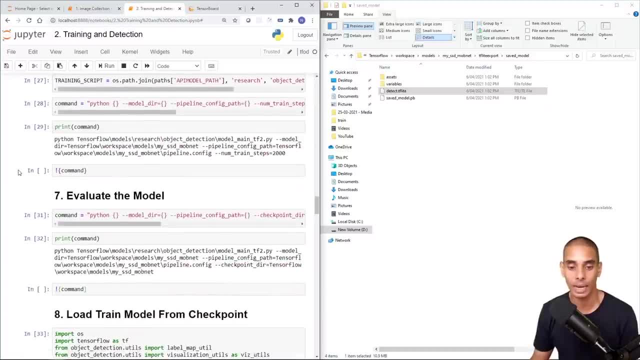 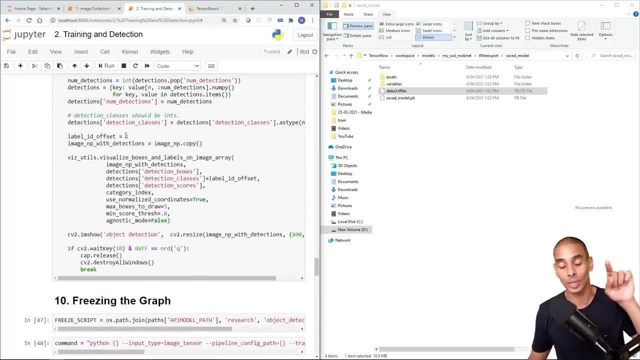 We then went and did all of our installs, We trained our model and then we evaluated it, Detected from an image which you can see here. We also detected from our webcam, which you saw using the real-time webcam feed. We then went and froze our graph and then converted it to TFJS and converted it to TF light. 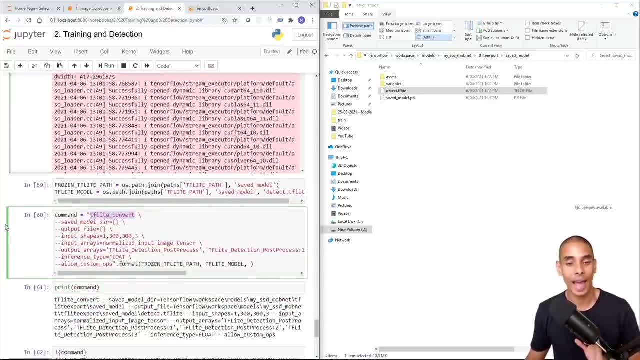 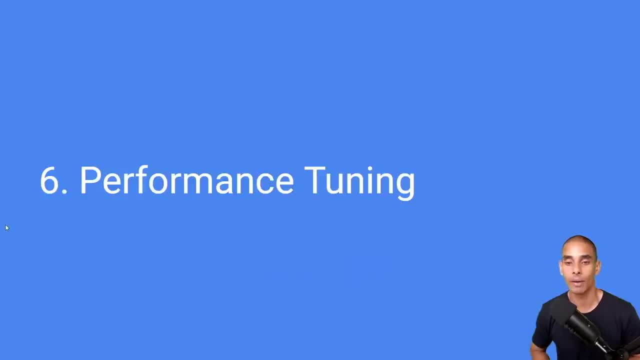 So that is a full end-to-end walkthrough of how to work with the tense flow object detection API. Now what we're going to do is get started with our performance tuning. So say, your model doesn't actually perform that well, what do you go about doing? 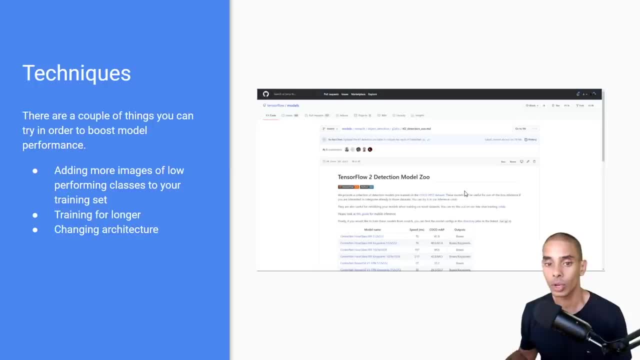 Well, this is really where performance tuning comes in. So normally there's three key things that I'll do to improve the performance of an existing model. So the first thing is adding more images of a low performing class to your training. So you saw that when we were doing thumbs up- thumbs down, live long and thank you- we were sometimes getting not the greatest detections. 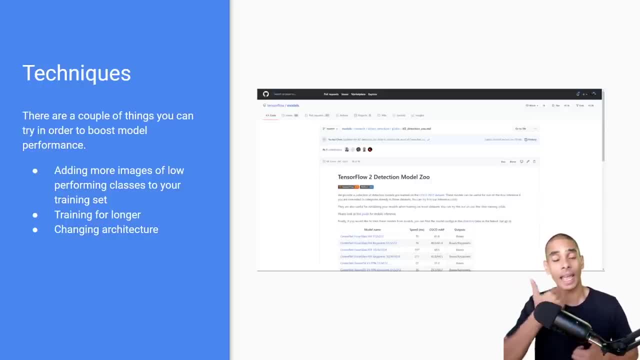 Now one of the easiest ways we can fix this is to take the green screen down and take images of both of our different positions using different hands. So this is going to give a model a better chance to generalize. So when people talk about the model generalizing, really it's being able to perform well in real world situations. 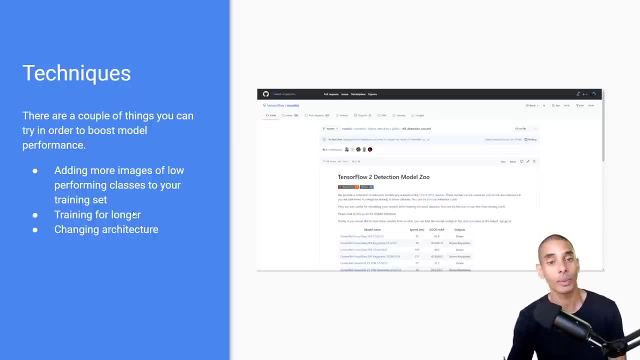 The second thing that we can do is train our model for longer. So you saw that when we generated our training command, we had 2,000 steps. Now what we can do is we can actually clear out our training folder and bump that up a little bit. 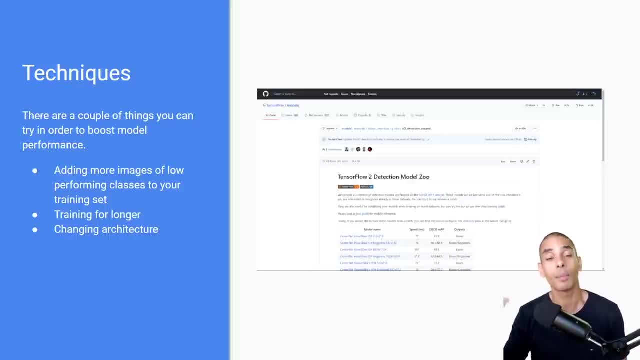 So say, for example, we trained for 3,000 steps. This gives our model a better chance at reducing its loss, generalizing and performing better overall. Now, the last thing that we can do is also change our model architecture. So we talked a little bit about the TensorFlow model zoo. 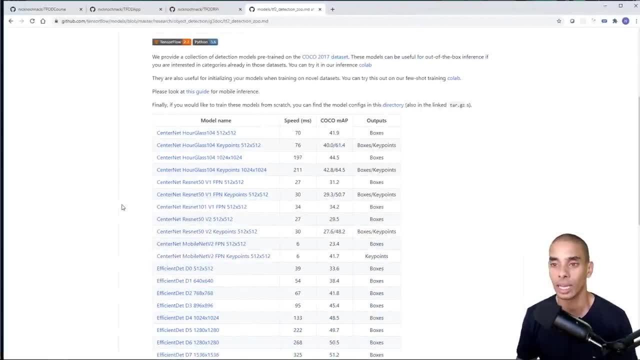 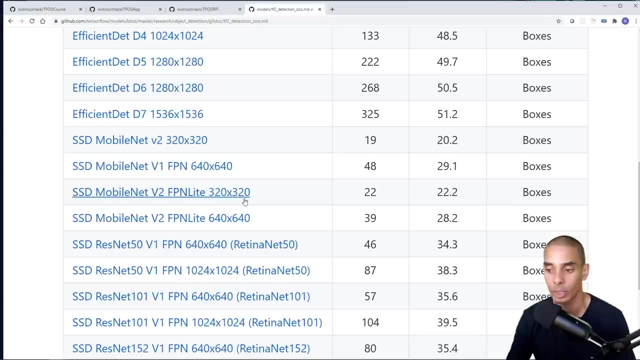 So you saw that we were using the 320 by 320 model. So if we actually take a look at that, we were using this model over here. So SSD mobile net V2FPN light 320 by 320, which had a speed of 22 milliseconds per frame and an average accuracy of 22.2.. 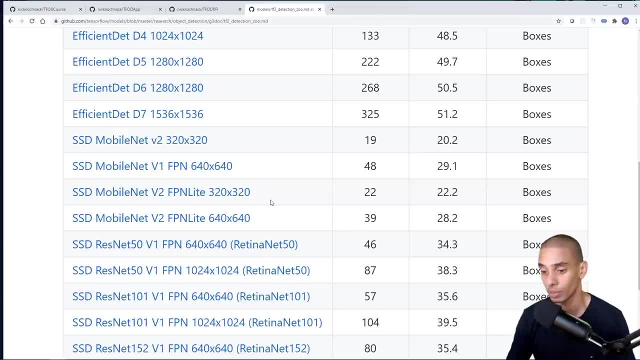 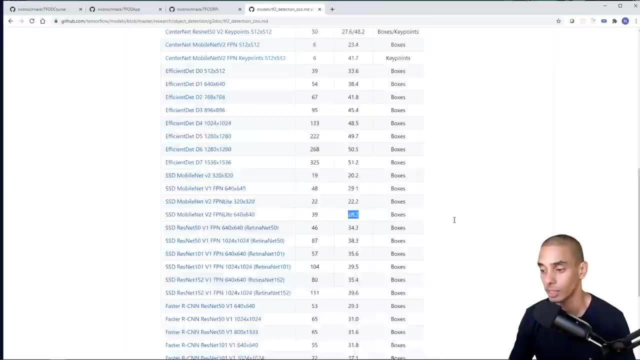 But we could also upgrade this and use a slightly more advanced model. Now again, we're going to have that performance trade off, So you might have a slower model, but again it might make better detection. So say, for example, we were to use this model here, which in this case takes 39 milliseconds per frame but also has a better accuracy metric. 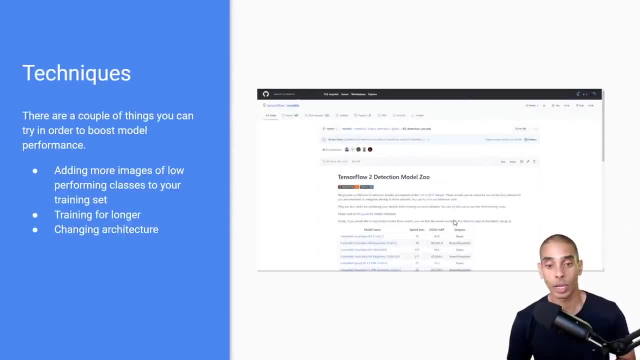 So we could do that as well. So what we're going to do is we're going to add some of these techniques to our existing model. So what we'll do is we'll add more images of our different classes. In this case, we know that our thumbs up, thumbs down detections weren't working so well. 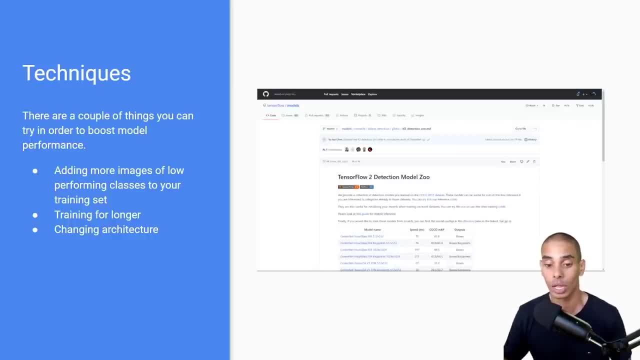 So we'll add more images of those, And then what we'll also do is we'll train our model for longer, So we'll bump this up to 3000.. And if we get time, we'll change our architecture and I'll show you what that looks like. 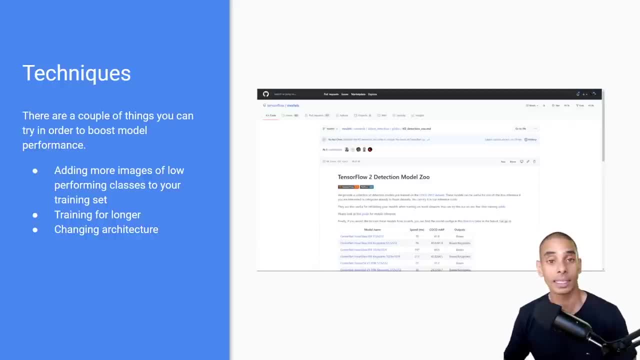 So effectively. that's really just creating an entire new model. But the nice thing about the Jupyter Notebook that I've sort of set up is that you can Plug in the new URL and this will allow you to create an entirely new model and build it using a new architecture. 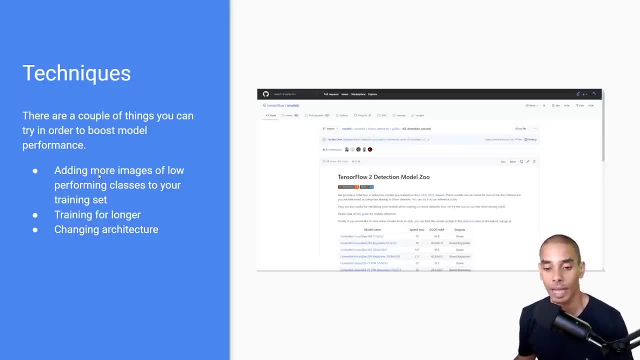 Alrighty. So first things first. So adding more images of our low performing classes to our training set. So we're just going to add more images of thumbs up, thumbs down, with our green screen down, and we will see how our performance looks like. 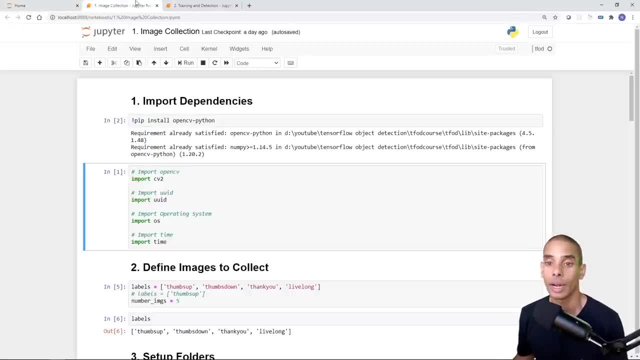 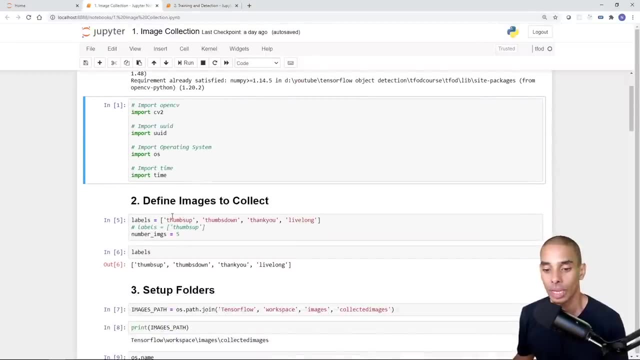 So if we go back to our notebook, So remember, we've got our image collection notebook and our training and detection notebook. Let me just check. we're zoomed in, We're good. So what we're going to do is, rather than collect images of every single class, we're just going to collect some more images of our thumbs up and thumbs down. 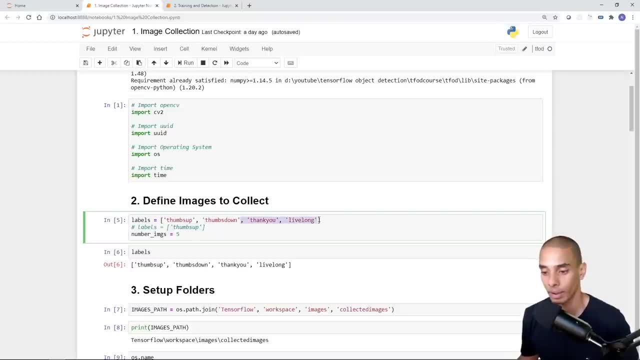 So we can get rid of thank you and live long, So that way we don't have to label a ton of stuff, Right? So these were the classes that didn't seem to perform that well, particularly when we were doing it with different hands. 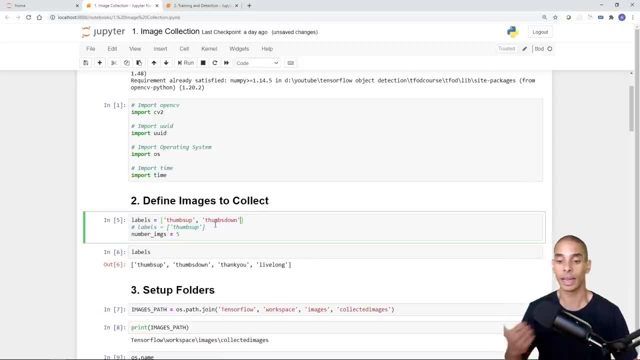 Right. So when we were switching, it wasn't actually performing that great. So what we'll do is we'll grab some more images of those and label them. Now we'll add, let's add six, So we've got an even number. 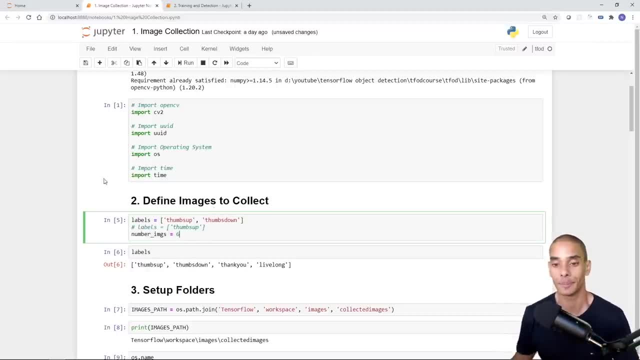 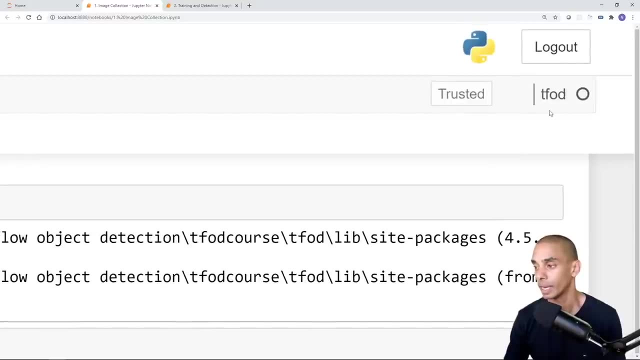 So we'll do Three of each hand in each position, Okay. So again, we're going to import this and again, make sure you're inside of your virtual environment So you can see up here that we're inside of TensorFlow object detection, which is a virtual environment that we created. 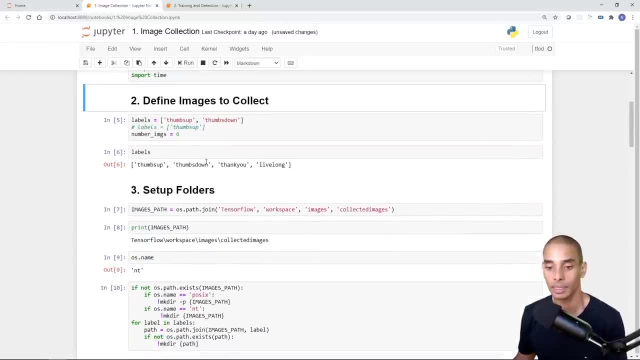 So what we'll do is we'll import, open CV or import our dependencies. Then we'll update our label map. So before, let's just have a look. So before we had a thumbs up, thumbs down, thank you and live long. We are going to just remove the stuff that we don't need. 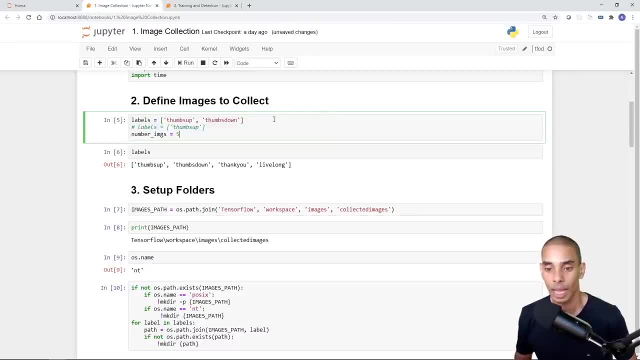 So thank you And live long so we can remove those and we'll change the number of images that we want to collect. So, rather than collecting five, we're going to collect six or three of each run that we can then take a look at our labels. 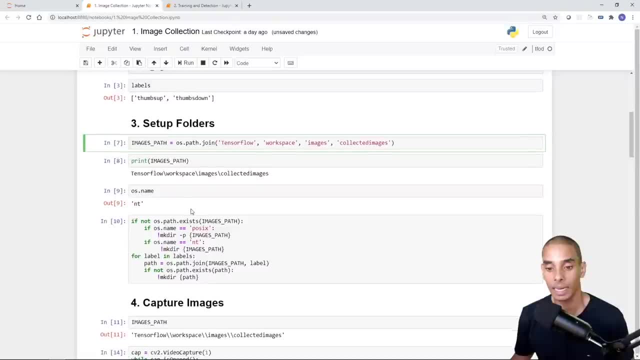 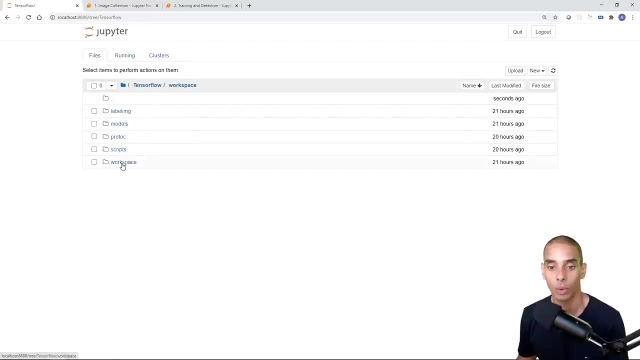 So now we're just collecting thumbs up and thumbs down And again. so when we actually output these particular images, they're going to be inside of our images part. So if I go into TensorFlow workspace images and collected images, remember they're going to appear inside of these folders again. 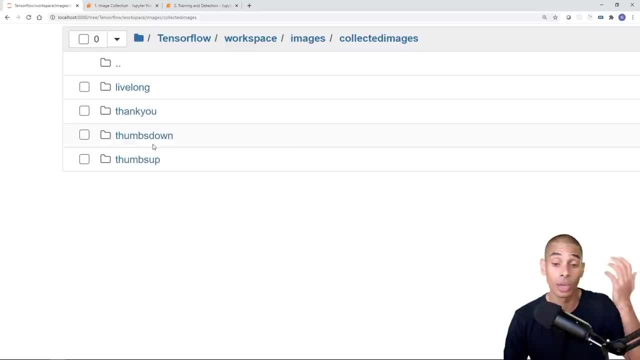 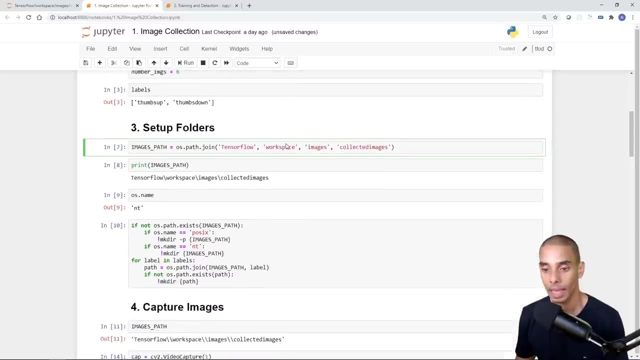 So live long. Thank you, Thumbs up, Thumbs down. Now it's not going to add additional images to live long and thank you, Just thumbs up and thumbs down. So let's go on ahead and do that. So if we set up our folders, we've already got these folders created. 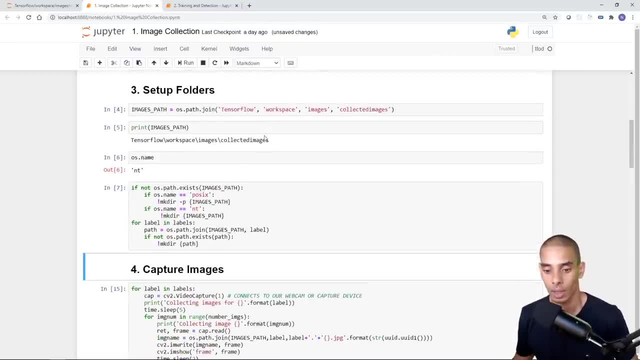 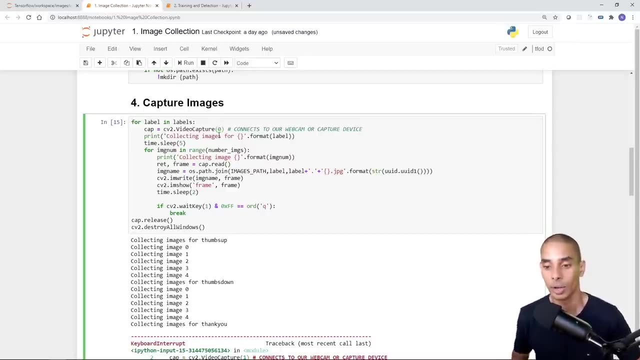 So, again, if we step through this, not going to break anything, And then what we can do is run our image capture. So now I changed this while I was doing some testing, So we're going to set that back to zero And again. so what we're going to be doing is we're going to be capturing images in our different positions. 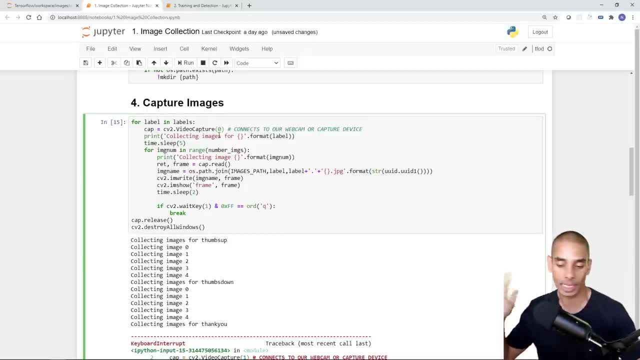 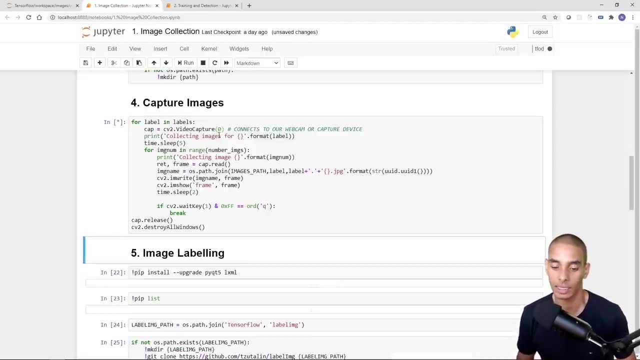 So we'll step back and we'll take a look. So if we take images, we might take the green screen down and might not. we'll just evaluate and see how it goes. So what we'll do now is we'll hit shift- enter. 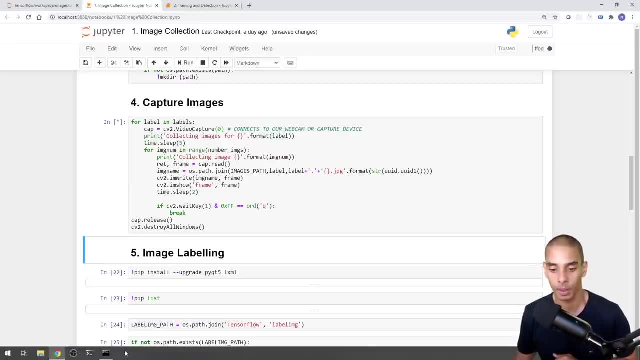 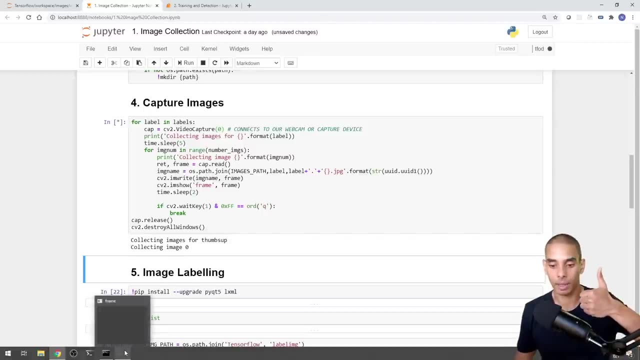 And ideally you should see the little Python pop up towards the bottom. Remember, it sleeps for a little while before it opens up. We're just going to have a thumbs up, Cool Right Now. we'll do it with the other hand. 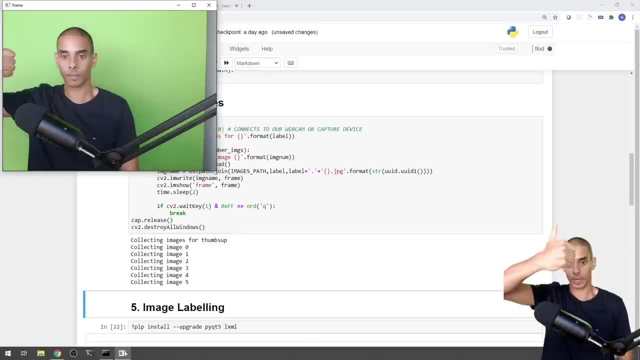 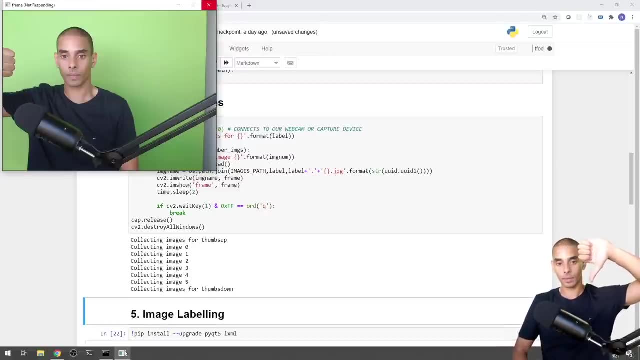 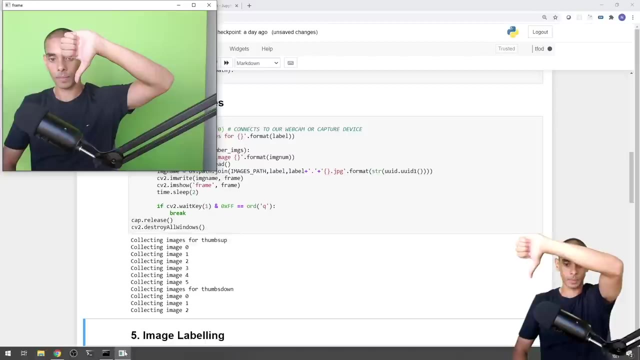 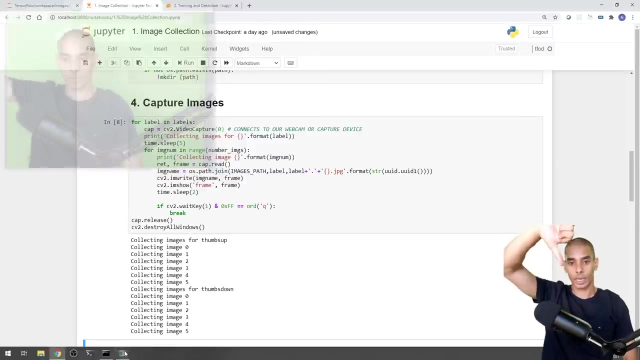 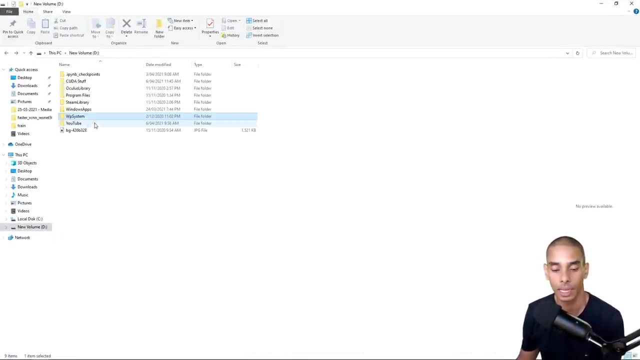 That's off the screen, then we're going to do thumbs down, So three on each. again The screen again looks like we had some sucky images there. So let's just go take a look at what we Collected, because I've got a feeling some of those were going to be off the screen. 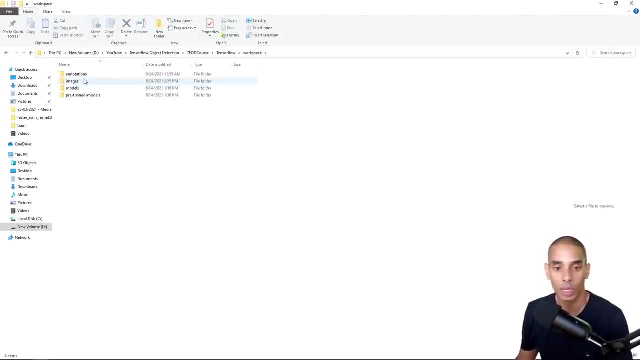 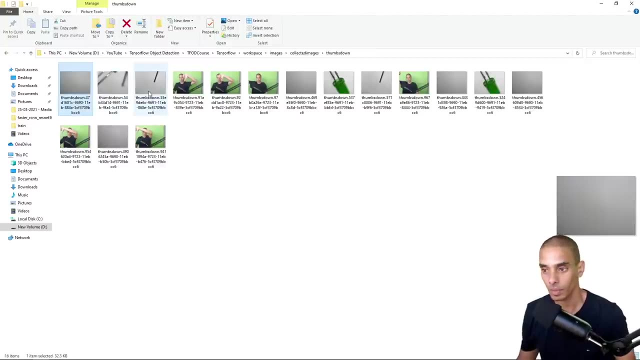 So if we go to tense flow- tense flow workspace images and then collected images- So remember we collected thumbs down and thumbs up. So if we go to, it looks like there's some images there left from my testing, So let me just delete those. 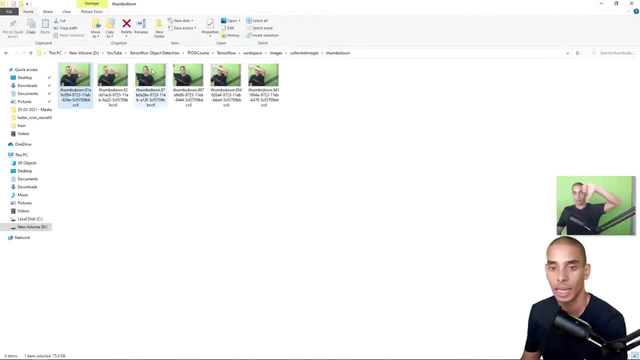 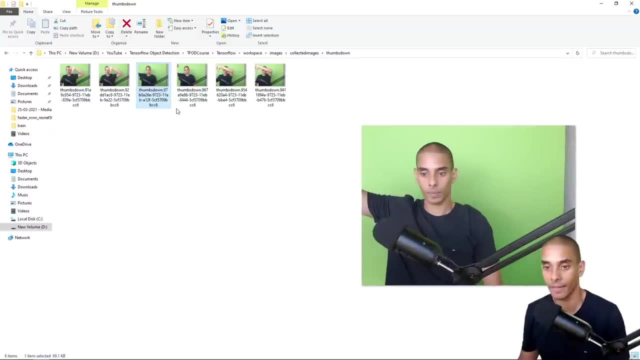 So these look okay. So that's thumbs down, thumbs down. This one doesn't look so good too. Let me just make that a little Bigger, So you can see that we don't even have an object on the screen to detect. 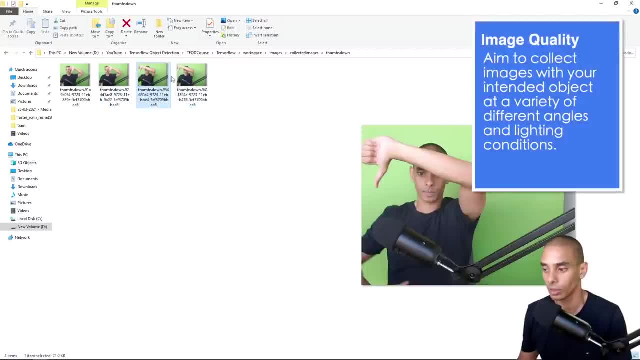 So we can delete that one and delete that one. This looks fine. This looks fine Again. ideally, we could probably get better detections, and these are all of the same side, right? So it doesn't look like we've captured the other ones. 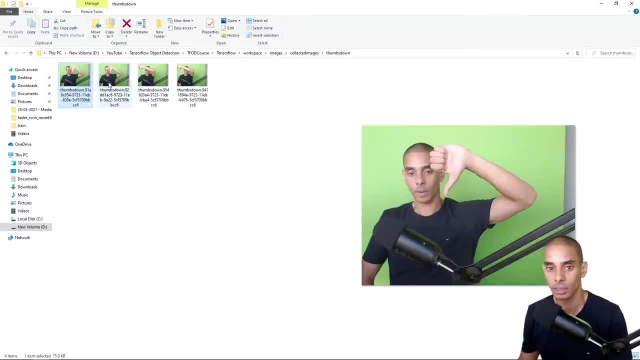 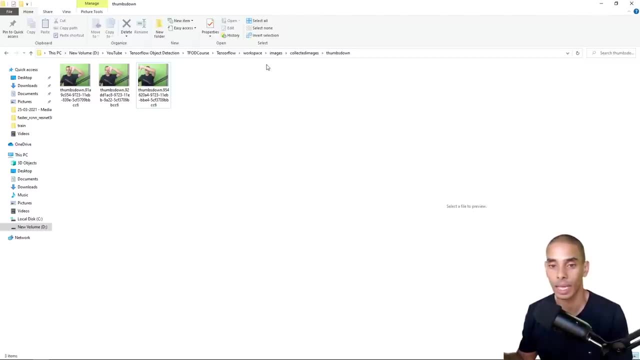 I was probably a little bit too slow, So let's just uh. so that one, I'm happy with that one. I'm happy with that one's okay, Let's delete that one, And we're going to grab some three more thumbs down, ideally, with the other hand. 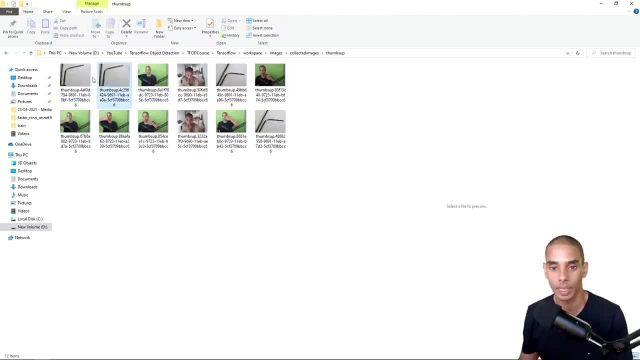 Okay, So let's go to thumbs up again more images from testing. Okay, And so again, that's poor image. There's no class there. It's all right. It's a little bit dark. That's all right, It's a little bit dark. 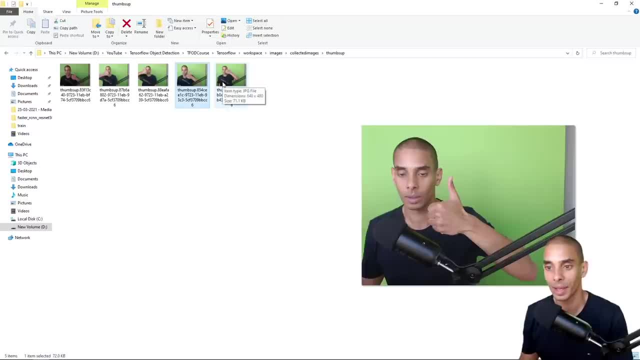 It's fine. That's fine as well, Even though I look a little sleepy there, and that's okay. So one, two, All right. So we can add in a couple more images and then we'll just sort of evaluate what we actually want to keep. 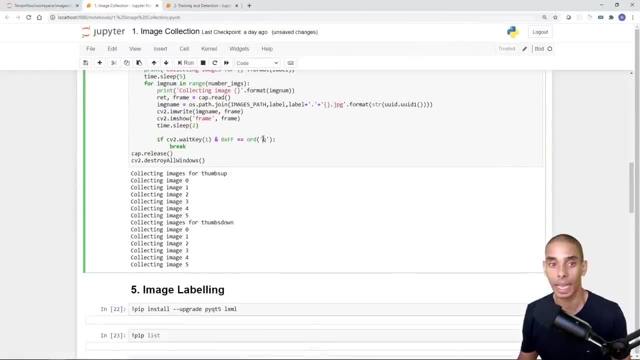 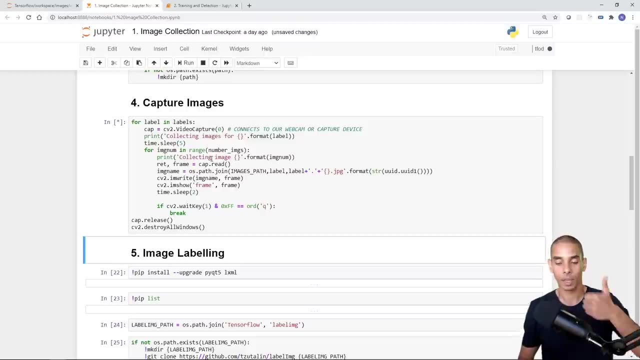 So Let's do a couple more. So again, to do it again, all we just need to do is run this cell under four capture images, and this is just going to capture our images again. So if we run this again, we'll do some more thumbs up. 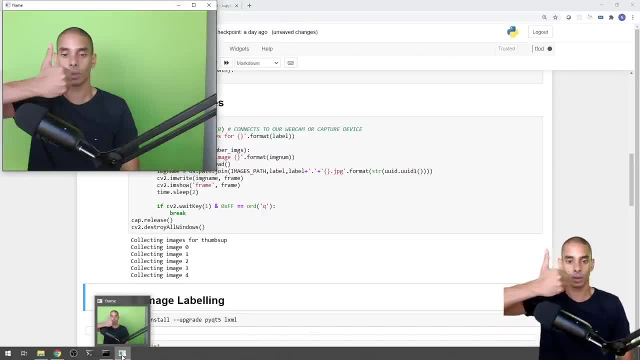 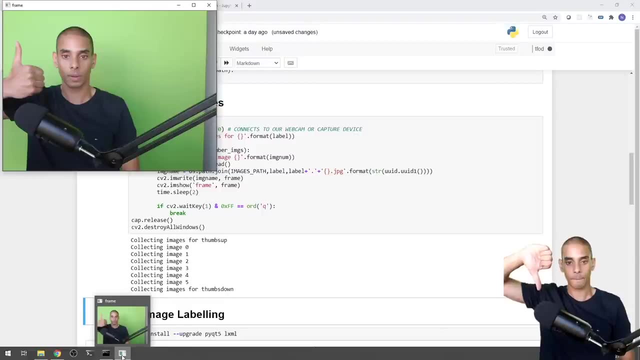 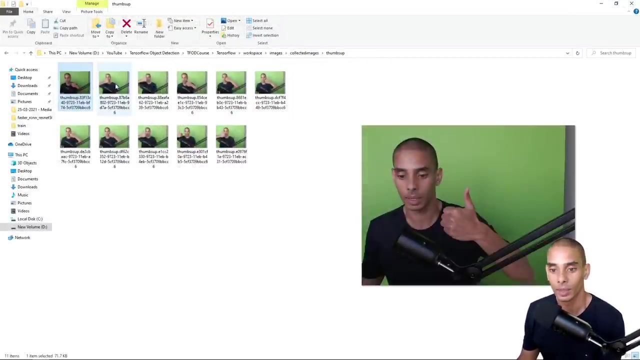 One Switch. That's going to be thumbs down. Okay, So we've got some more thumbs up. this is kind of good. So you can see that this is a little bit dark. So I mean that might be a good chance to give our model to general, might give our model some additional data to generalize. 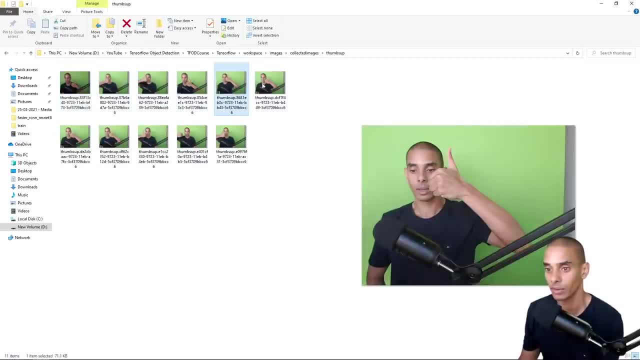 So that's fine, That's okay, That's fine, That's fine, That's fine, It's looking better. Okay, So I think we're good there. So for thumbs up, So it looks like we're going to have what is this? 11 new images. 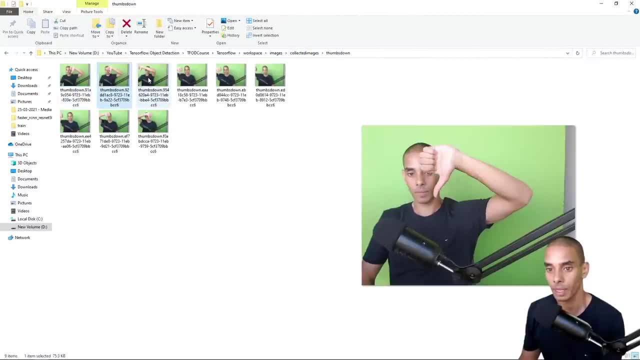 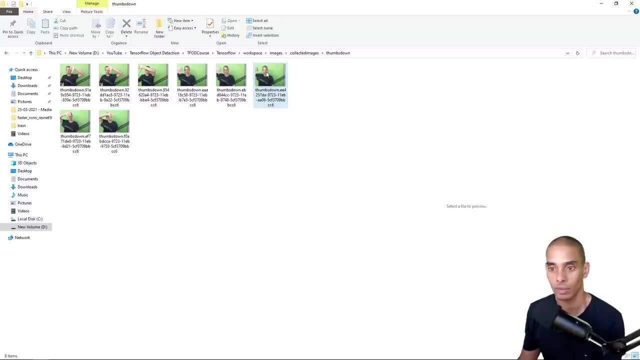 And if we go into thumbs down, let's take a look at what we've got. It's fine. Again, we're going to get rid of this one because that's off the screen, This one, because that's off the screen. 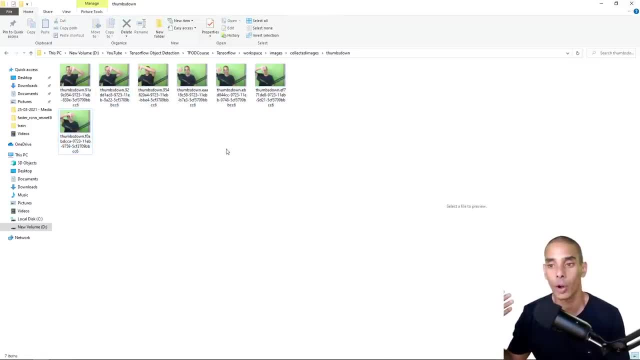 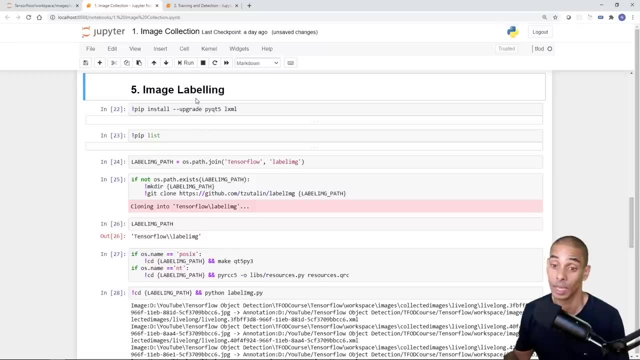 Okay, cool. So we've got a bunch of new images. Now what we're going to do is we're going to go on ahead and label These again. So remember when we went and labeled. all we need to do is go through our step five and image labeling, and this is going to open up label image to be able to label images. 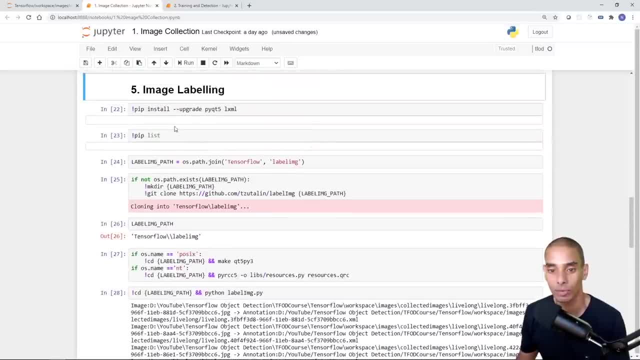 Now, because we've gone and installed all of this already, we don't actually need to run every single cell. So these ones up here, so pip install, pip list, these couple, these are just doing the installation. So everything, all of these cells which you can see here, these are really just doing the installation. 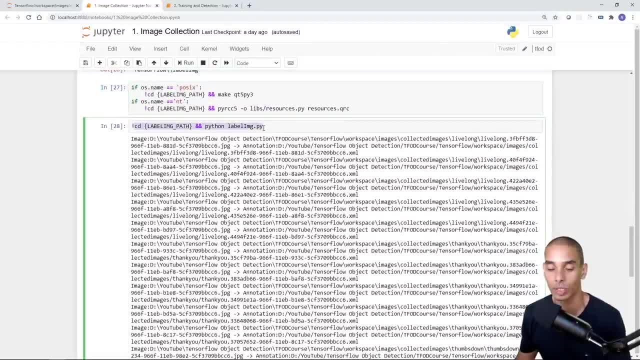 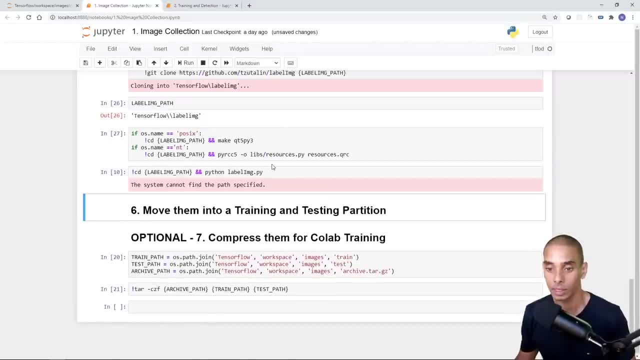 All we need to run is this one. So this is actually. We're going to open up label image. So if you've already run through the installation, you're good, You don't need to go on ahead and install it. So if we just run, this cell is: oh, we need to define our label image path. 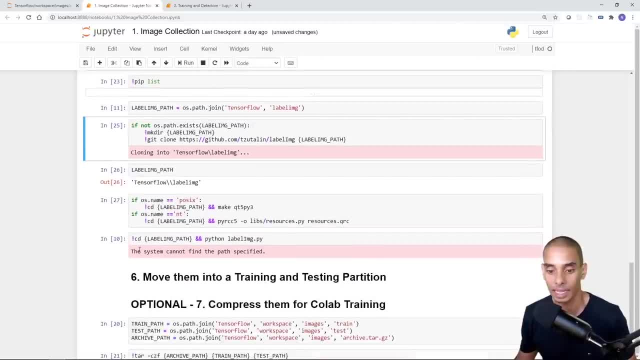 So let's run this cell So you can see here that it's saying the system cannot find the path specified, and that's because we're asking it to open up label image path over there, but we haven't defined it yet, which is this what this cell is doing? 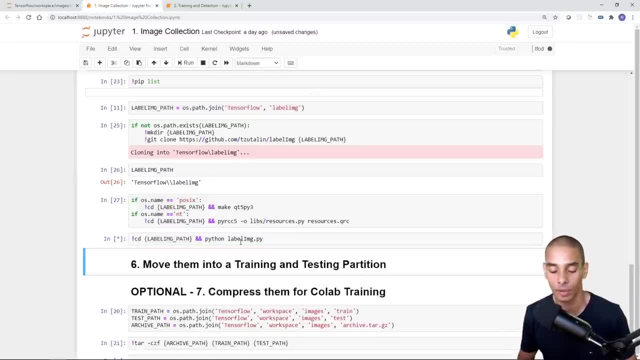 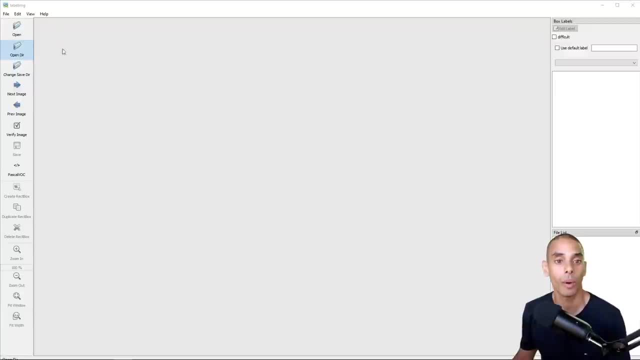 So if you run the label image path, this should allow you to open it up. So if we open this now, Hell Label image platform should open, So you can see that that's now open. Now what we're going to do is as per usual: we're just going to go on ahead and label our images. 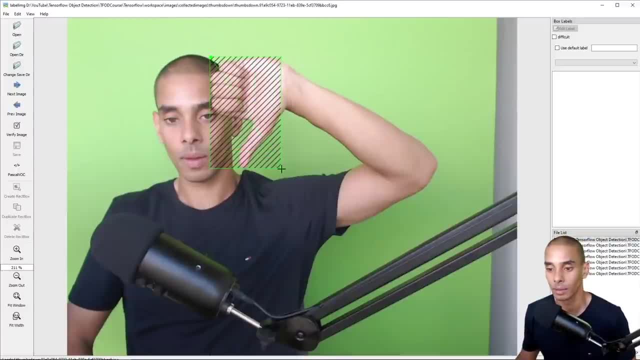 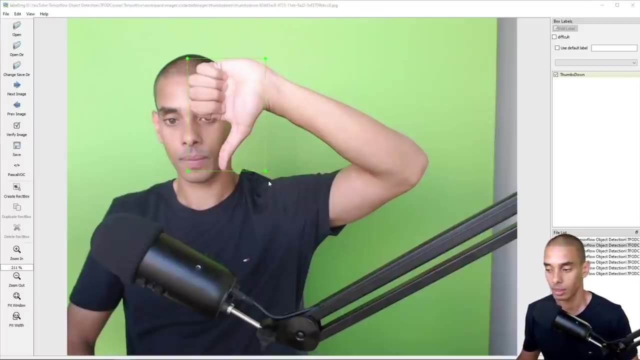 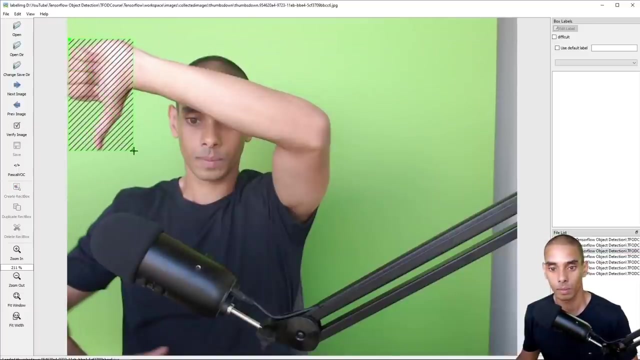 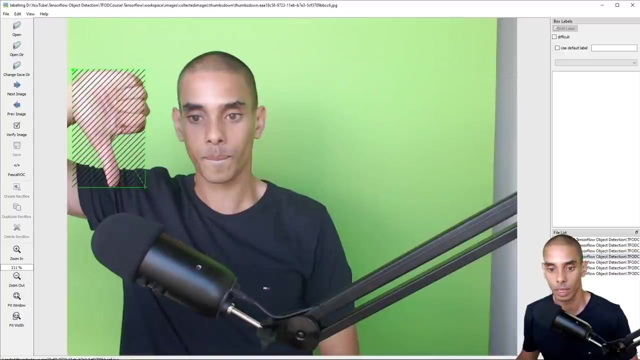 So again, w- and this is thumbs down, and remember it's case sensitive. So thumbs down, save. go to the next one. thumbs down, save. You can see that we've now got varying images right. So we've got both hands covered. so there's a better chance that the model will perform better. 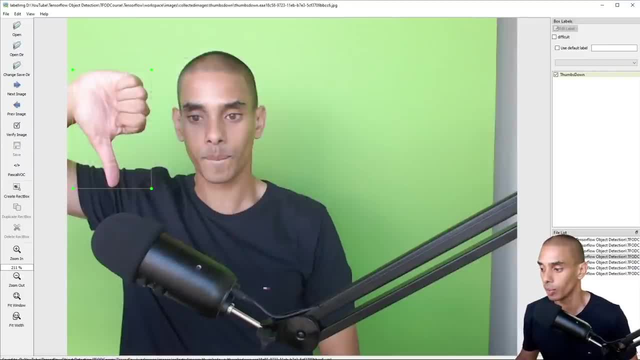 A lot of the time this is trial and error, So you've got to evaluate and see what's going to make your model perform better. But normally this is the first step, So I'll go on ahead and I'll add more images of the classes which I wasn't too happy with. 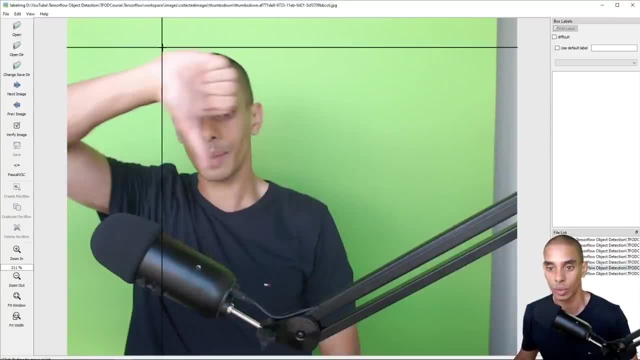 This one is a bit of a shocker, So I'm going to do it again. I'm going to hit save, Let's see what happens. this one is a bit of a shocker image, but we'll wait and see. okay, and we'll do the. 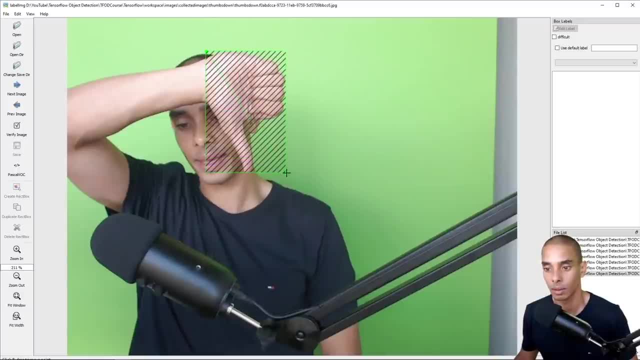 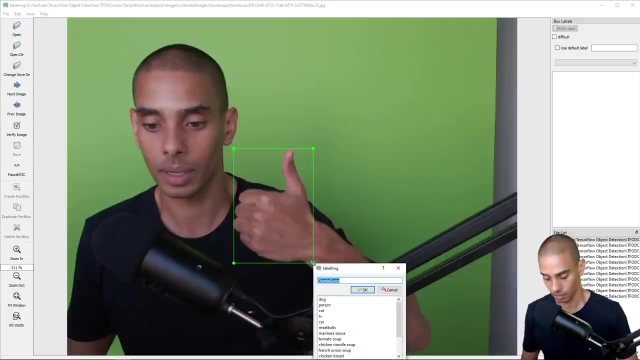 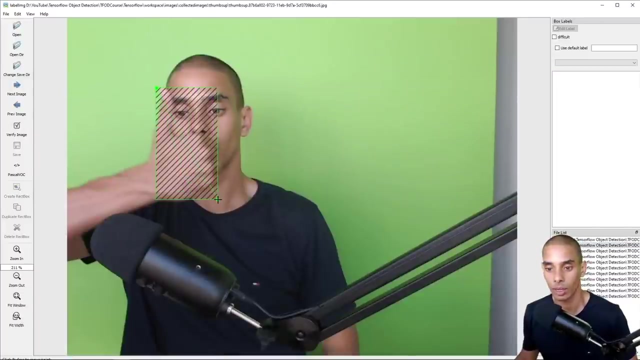 next one that this thumbs down again. cool, then we'll open our next directory, which is thumbs up, and we'll go and do these ones in the same manner. and again, we're just changing the label name, paying attention as to whether or not it's case, or paying attention when it is case-sensitive. again, we can adjust. 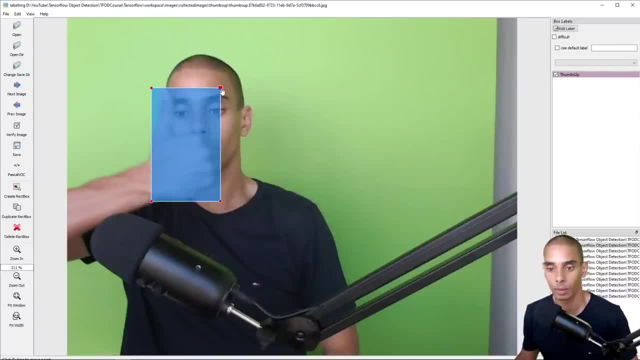 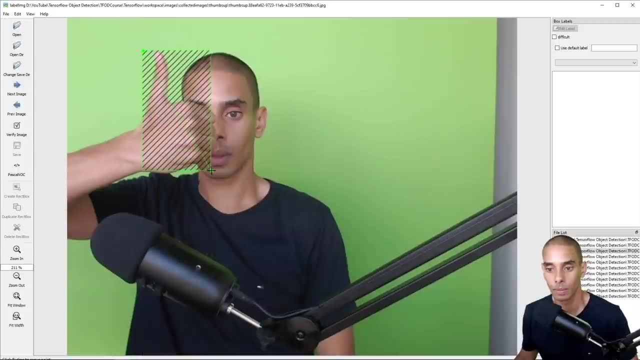 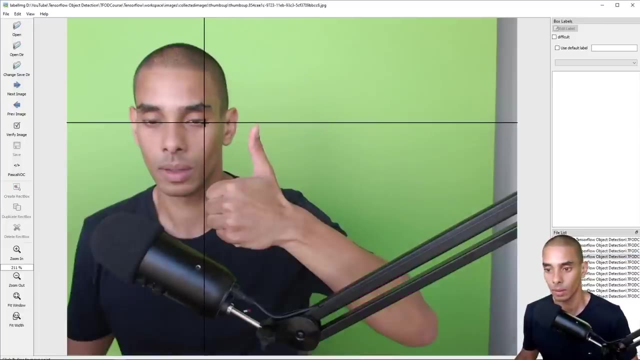 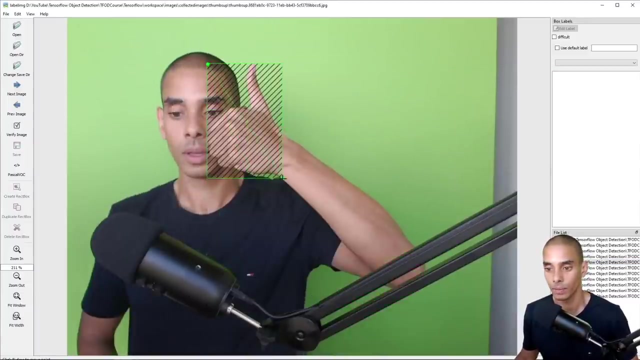 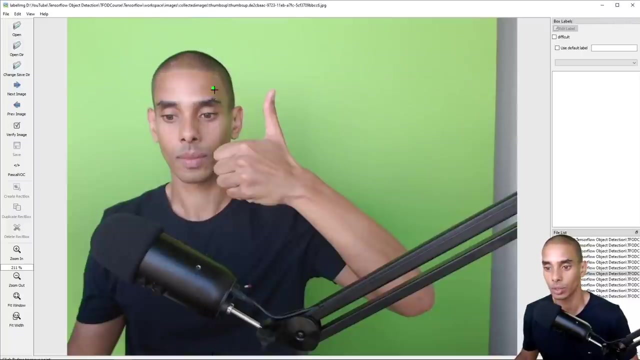 these. if we need to saving, go to the next one, save, go to the next one, save the next one and just keep going through until you've got all of your images labeled again. this is something that you could start looking at- auto labeling tools- for obviously it would improve at your efficiency. also, pay attention, pay. 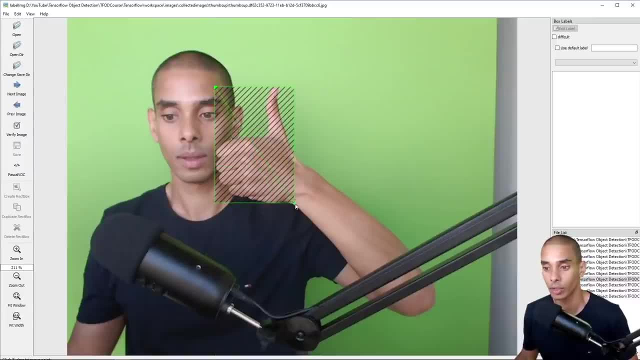 attention, if you do start using those tools, as to what the performance of those order labeled images are. Sometimes, even though you use an auto-labeling tool, you still do need to go through and do a bit of a manual review. But again, something that could potentially improve. 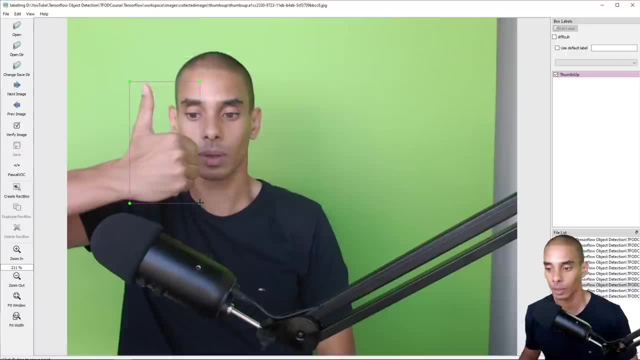 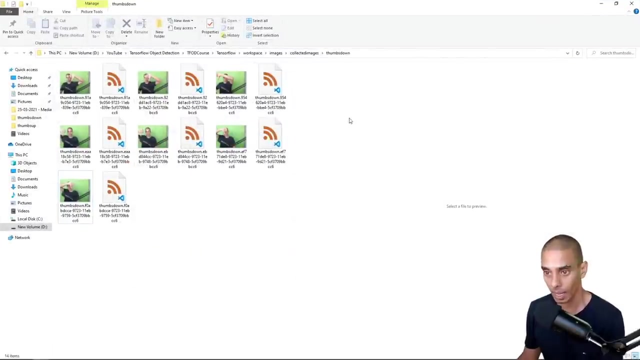 how quickly you're able to label images, So I'm just going to finish the rest of these up. Save that, Do the next one. Okay, cool, So that is now done. Now remember: whenever we are labeling new images, we need to. 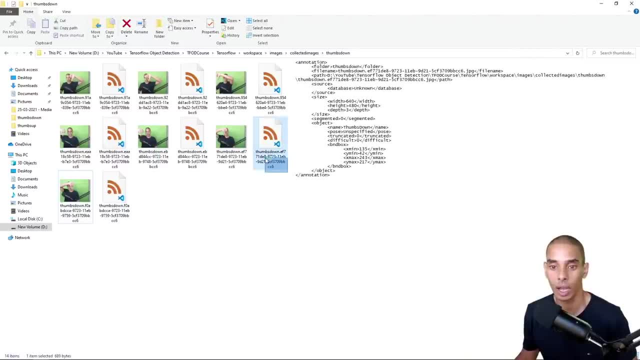 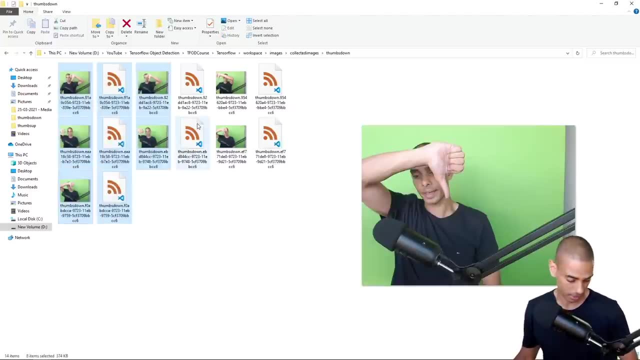 copy them into the training and test folder. So no real change there, So I'm going to copy the majority of these, So let's go. It looks like we've got a good mix there, So let's copy these. 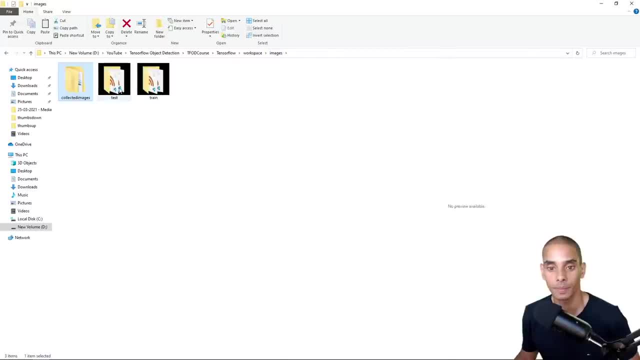 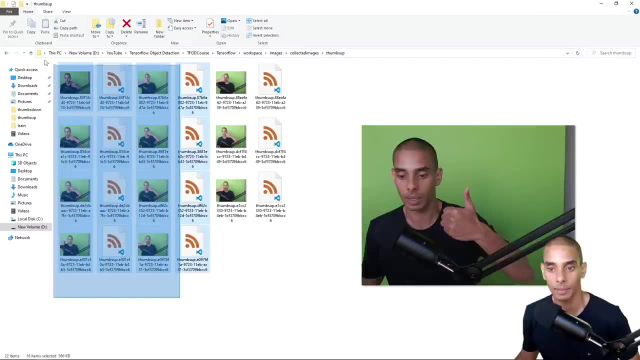 and we're going to put them into the training folder And then we're going to go back to our collected images, go to thumbs up, do the same thing And let's just Grab these And that looks okay. And remember you need to grab the annotation as well as the. 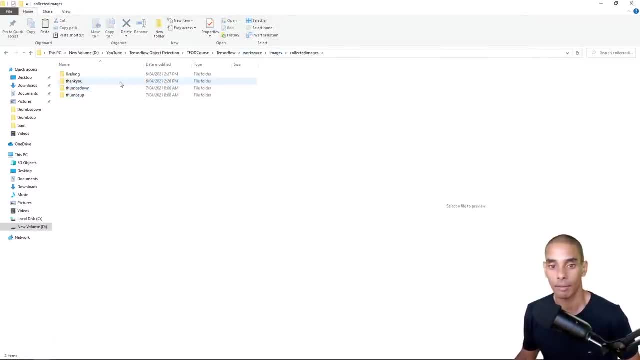 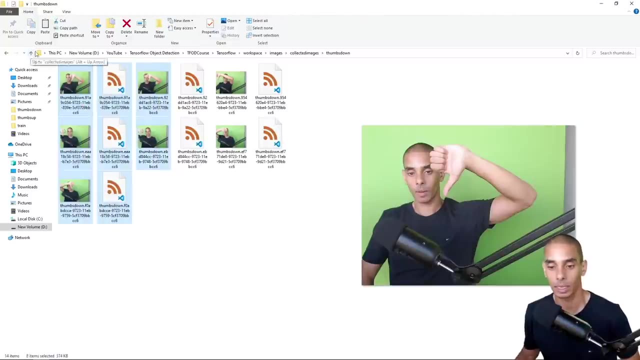 image. So if you don't have both, then you're going to have a bad time. So we are going to grab. Why do we still have a bunch of thumbs down? That's because we didn't cut, We copied. 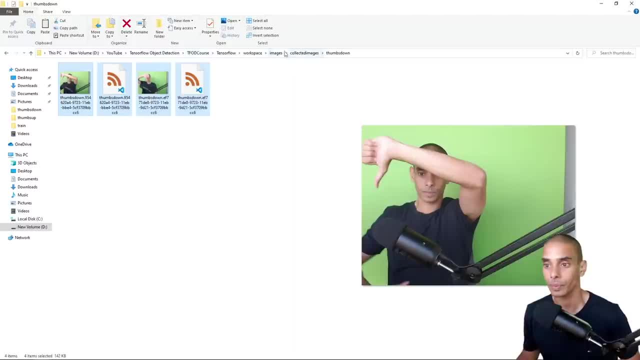 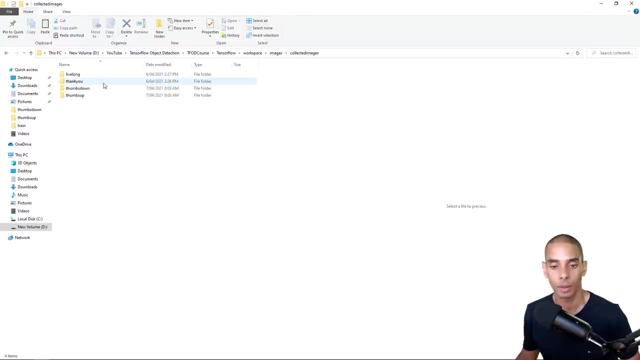 So we go to delete those, Copy those last couple, And we're going to paste the rest inside of our testing folder. And remember we did all of those, So we're going to paste the rest into our testing folder. All right, So now we've just added more images of our classes that we weren't too confident about. 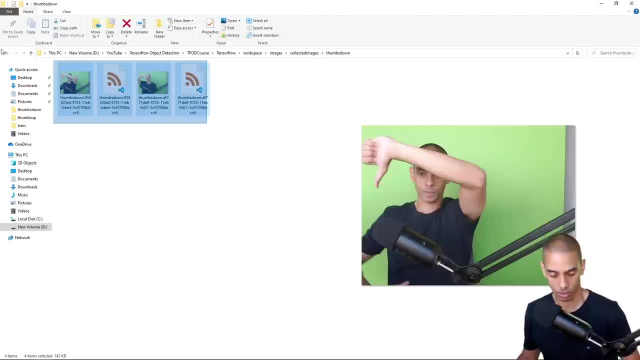 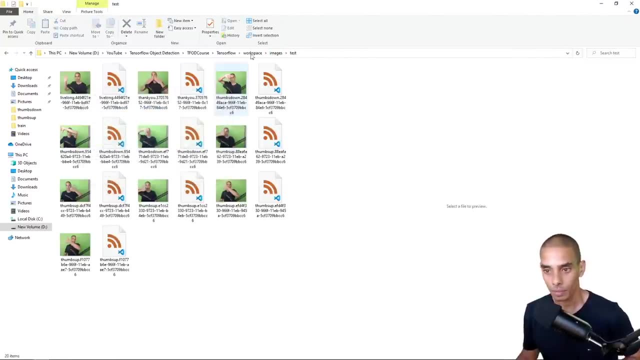 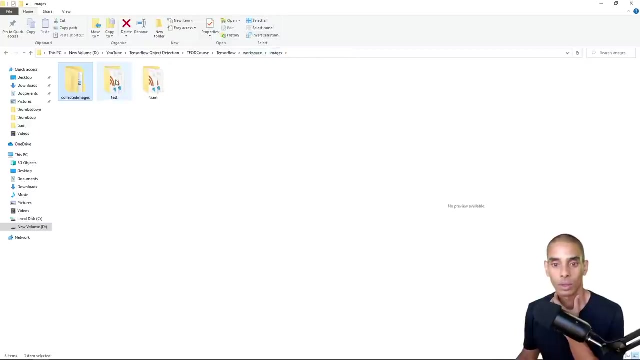 I thought we pasted those in there already, The F7. Let's just cut those. Okay, We did All right. So now, if we go into our collected images folder, thumbs down- We already did those And thumbs up: Cool, All right. So that is now all well and good. So we've now gone and added: 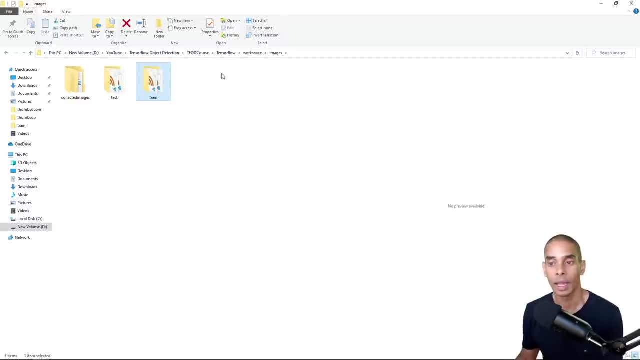 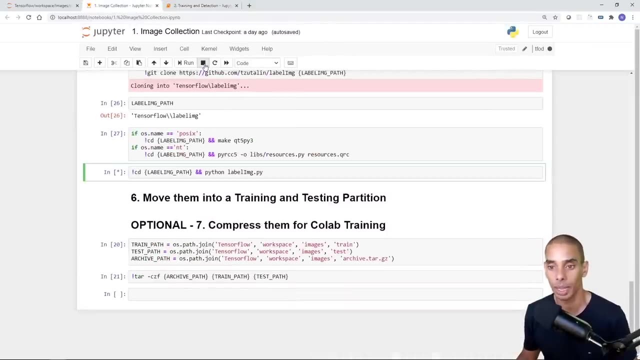 more images to our testing folder and more images to our training folder. Now, if we are going to retrain, we're effectively going to be using our training and detection notebook again. Oh, we can also stop label image. So if you just hit stop, that's going to close this off and we can close. 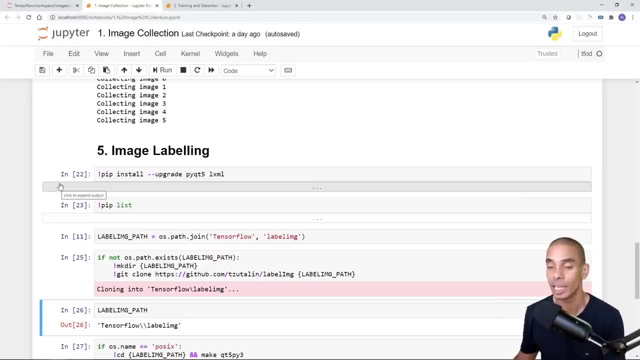 that as well. All right, So now that we've got our images collected, the next thing that we need to do is go on ahead and train our model. So we're going to go ahead and go ahead and train our model. 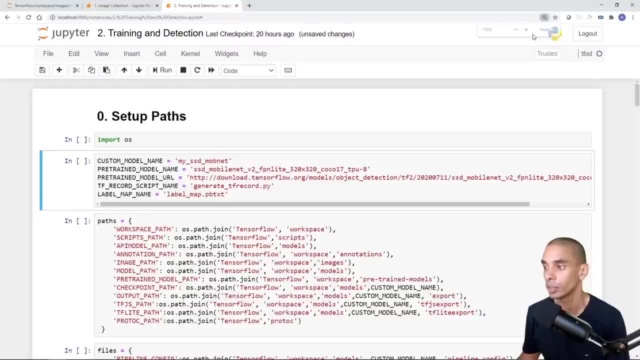 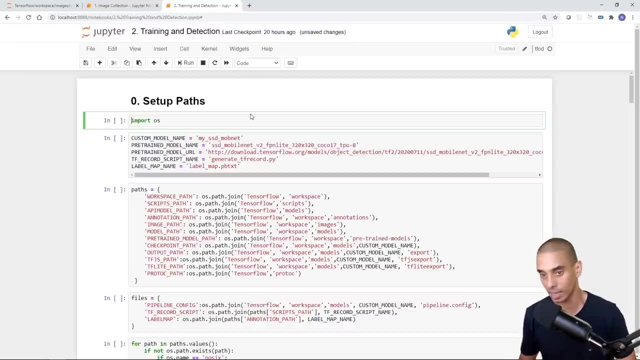 Now, in order to do this, we are zoomed in quite a fair bit there. Let's just go to 125.. So, in order to do this, we're just going to go back to our training and detection notebook and we're just really going to change one thing. So, namely, I'm going to change this custom. 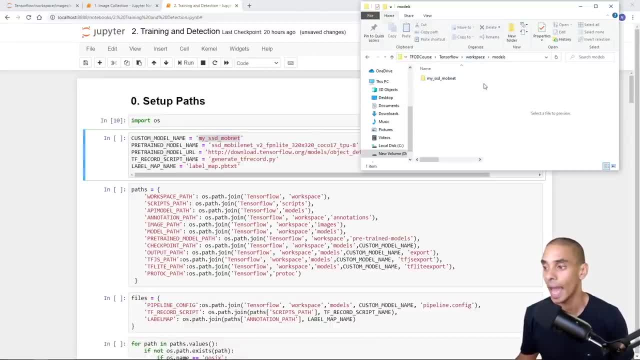 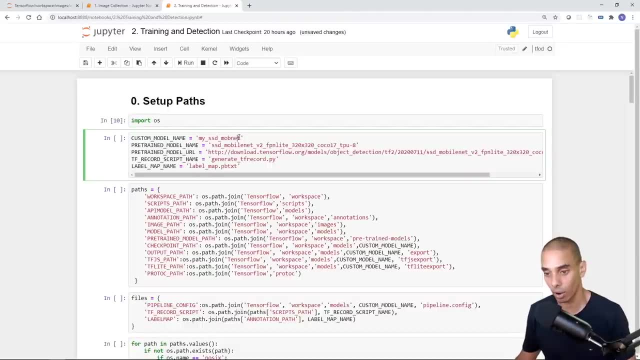 model name. So when we built our first baseline model, we actually named it Maya. underscore ssd, underscore mobnet. Now we're going to call it slightly different, So we're going to just add on underscore tuned and this is going to give us a new folder. So again, if we're going to call 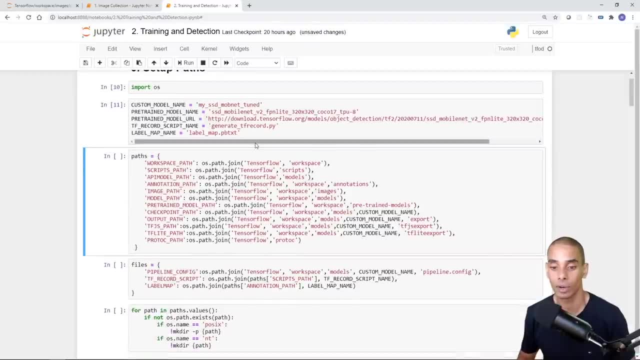 it something else. we're going to just call it something else. So we're going to just add on underscore tuned and this is going to give us a new folder. So, again, if we're going to connect our, And this is going to give us a new folder. 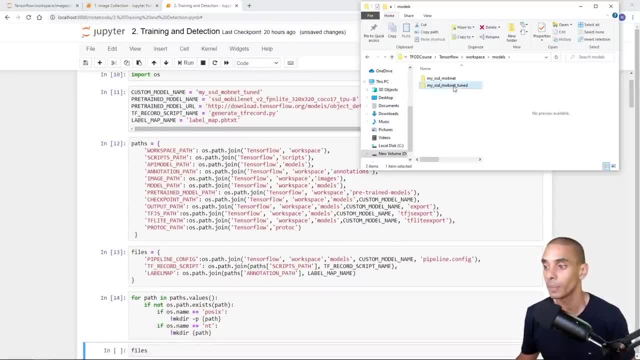 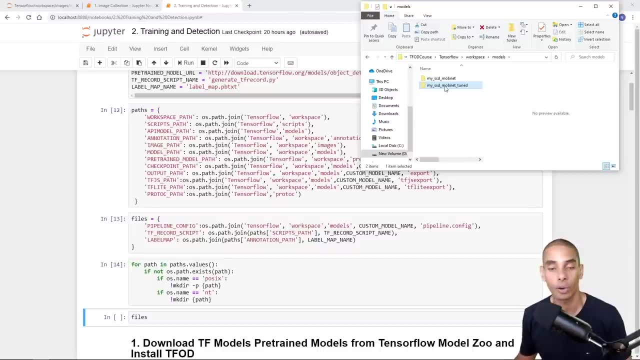 So, again, if we step through this, it's going to create a new folder which, again, you can see there. So we've now got my underscore, SSD underscore, MobNet underscore- tuned. So we've now got a separate folder that's going to contain our tuned model. 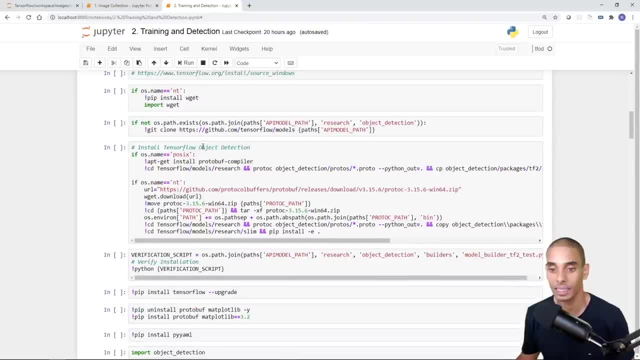 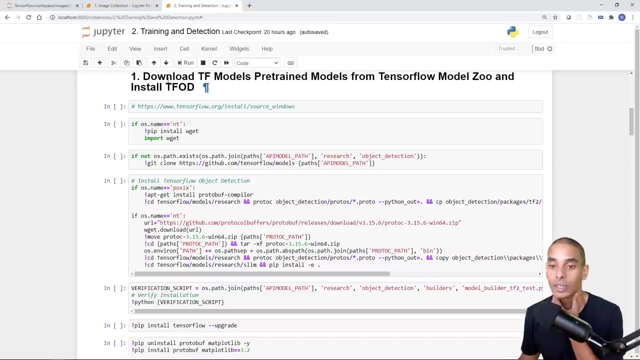 Now we can keep going through this And effectively, this is going to give us the ability to go on ahead and train a tuned model. Now we can skip this entire step entirely, So we don't need to download any new pre-trained models or reinstall TensorFlow object detection. 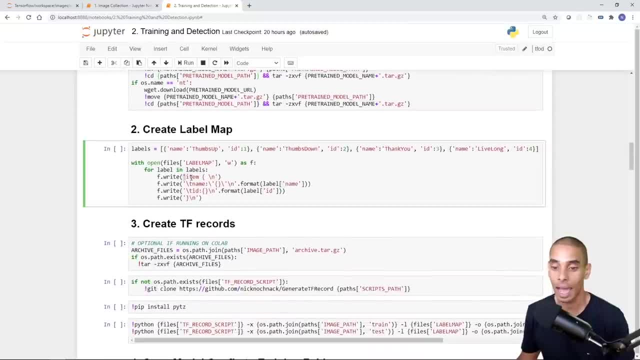 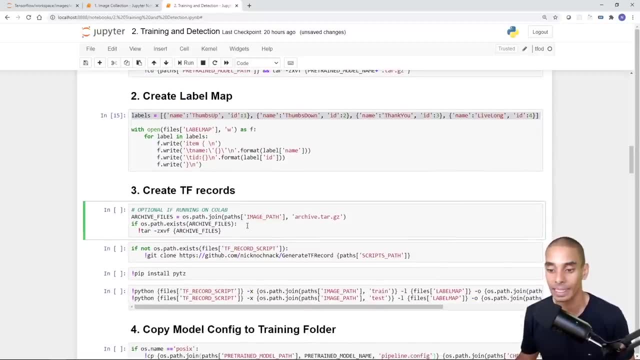 We've done that. We've gone through that pain. That's now done and dusted Our label map. we can run that again, but really we're doing this, So we've got this label line available and then we're going to create our TF records again. 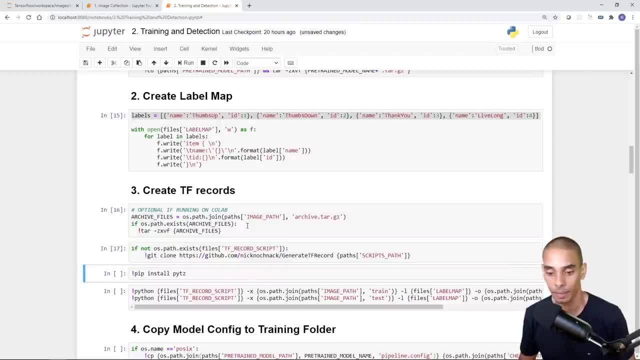 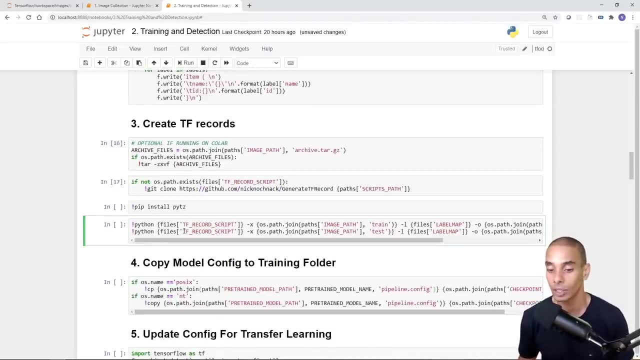 So we are going to now create new TF records And again, we don't need to install this. I'll keep installed PyTZ again. We had that installed. We are, however, going to run this generation, So remember, this is going to create our test record. 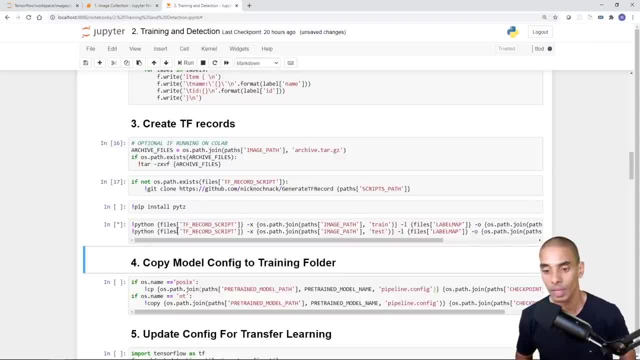 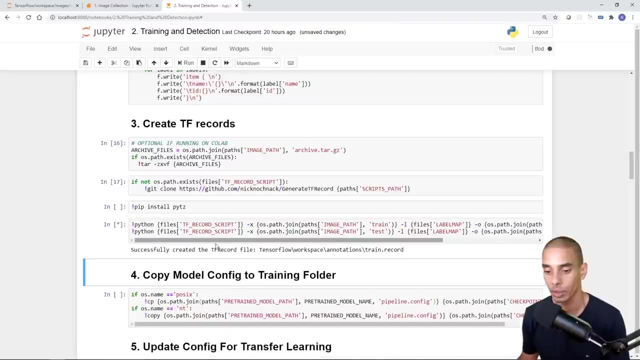 and our train record. So if we run this, hopefully fingers crossed, no issues, And this should give us our new TF records to be able to go on ahead and train with. So let's let that run And it looks like we don't have any errors there. 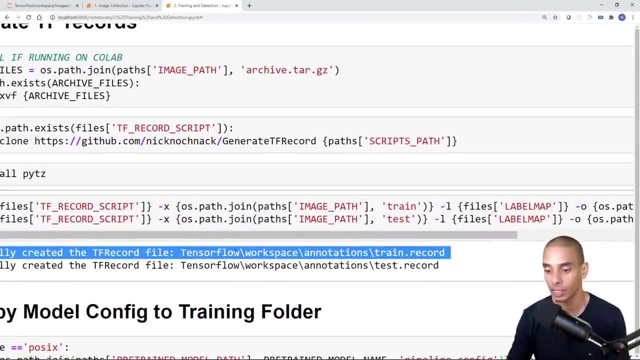 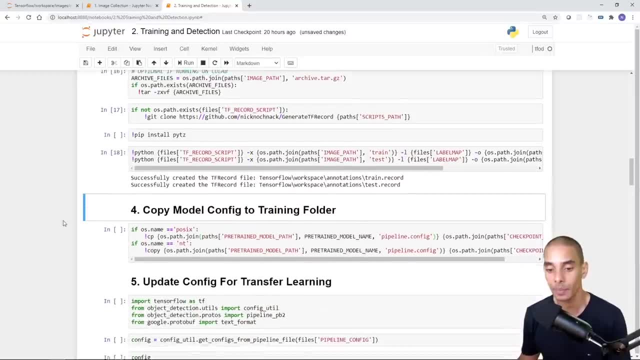 So we've successfully created our TF record file- IntenseFlowWorkspaceAnnotationsTrainRecord and IntenseFlowWorkspaceAnnotationsTestRecord, So we're good to go now. Now the next thing that we need to do is copy our pipeline config. So this is going to copy the pre-trained pipeline config. 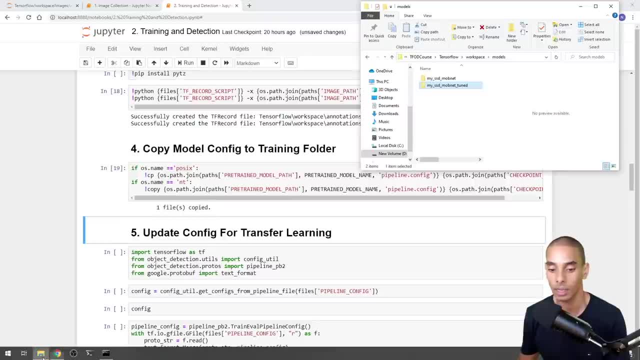 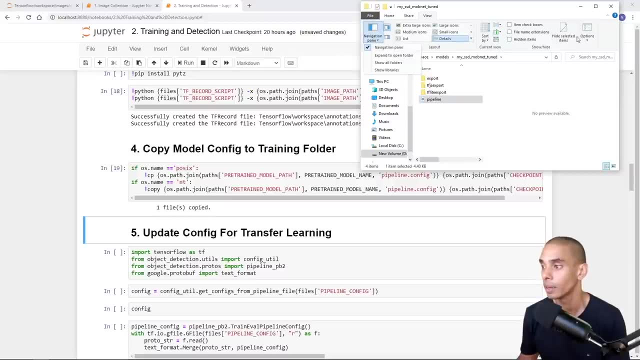 into our new tune model. So if we run that inside of our MySSDMobNetTune folder, you've now got this pipeline file. You can hide this. We don't need a preview pane. Minimize that so it's a little bit easier to see. 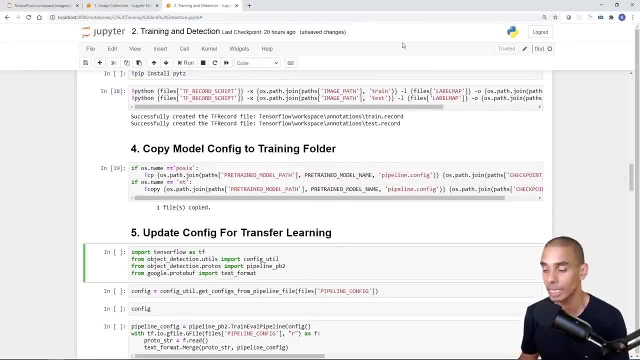 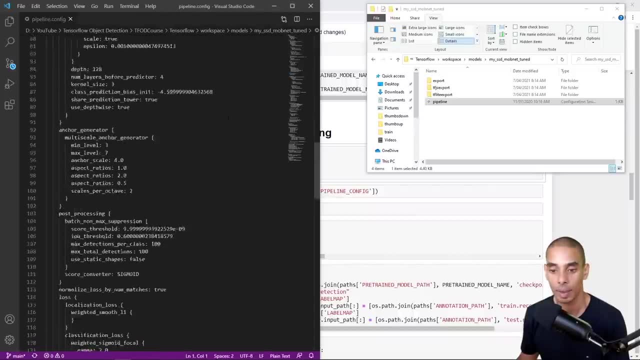 So we've got this pipeline config file And then really we just need to make our updates as per usual. So this is really just filling in what's inside of this pipeline config. so if we take a look at this, remember, right down the bottom we need to configure all of these parts, but we've got our code here that's going to do it for us. 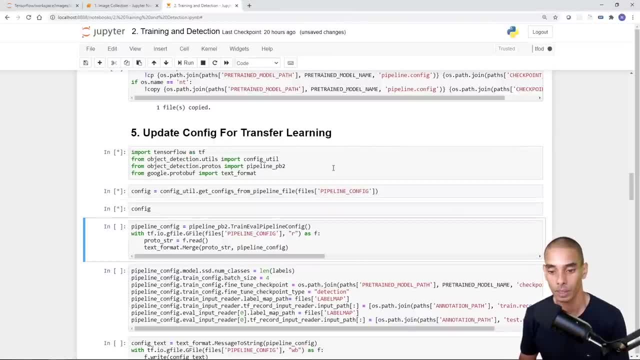 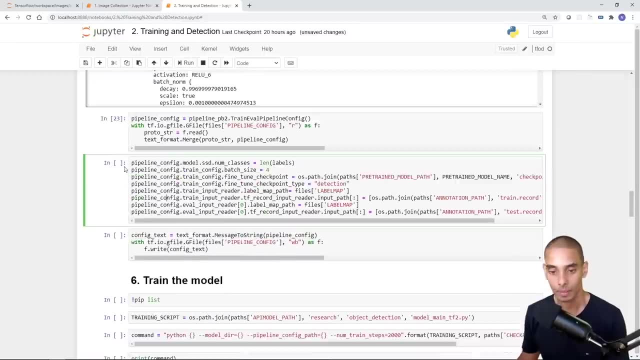 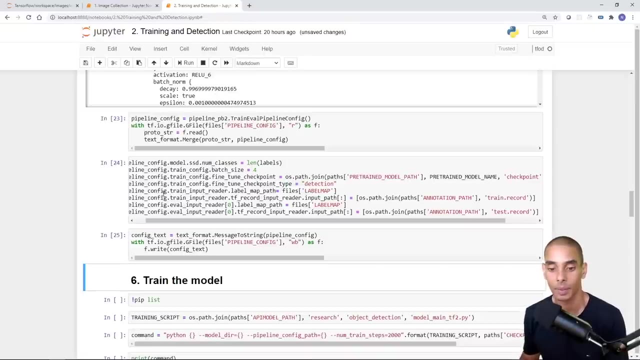 so we're just going to step through. it's going to open up our pipeline config and again, this is just the standard one we keep stepping through. so this section here is probably one of the most important. this is actually updating the pipeline config. so if we go and run that, run that again, or? 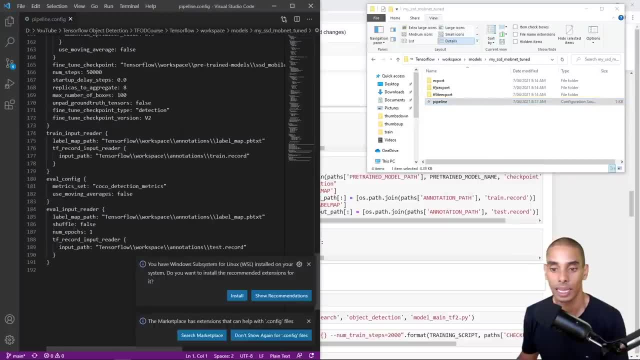 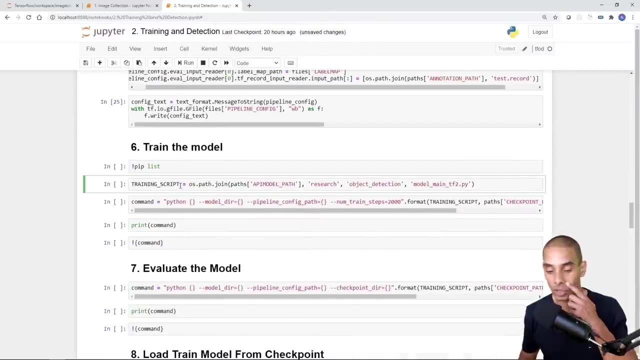 run the next cell. now, when we open up this pipeline, you can see that we're now going to have all of our label, map, paths, so on and so forth defined. so that's all well and good. now what we can do is run our training script. so, again, this is all sort of pretty modular, so you can just sort. 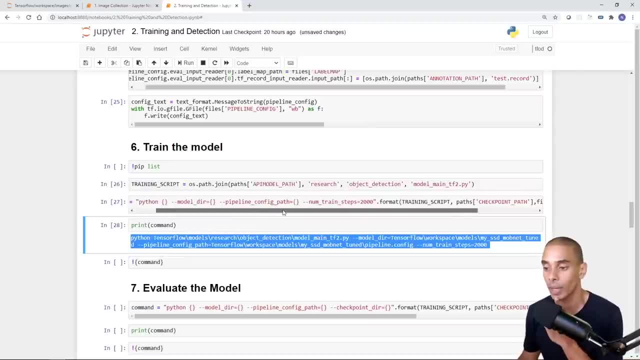 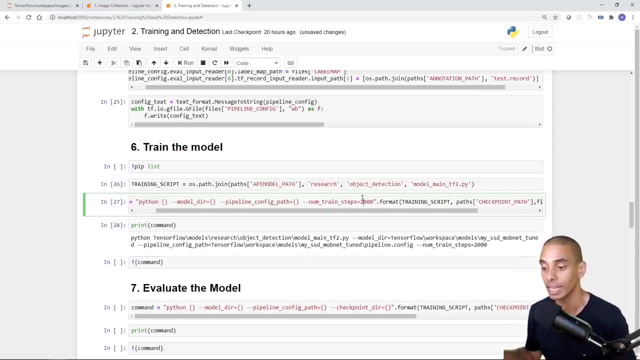 of run through it and it should ideally work now. the one thing that we are going to change is the number of training steps, because, remember i said, the things to try are adding more images and changing the length of training time, so we can bump that up and we'll increase that to. 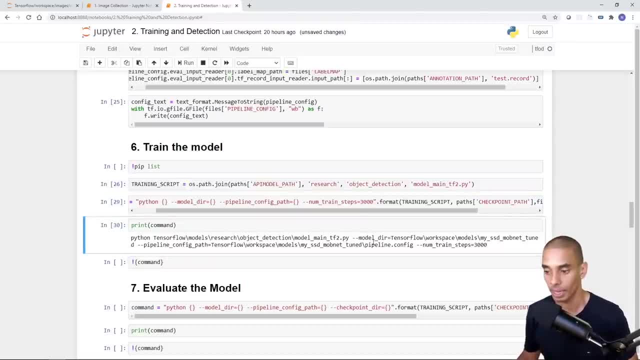 three, Does this help? 3000, and we can run that command and again try this out, so you might want to play around. you might want to train for longer, train for a shorter amount of time. the world's your oyster here. so again, a lot of it is experimental, so we're going to copy this and we're going to open up a new. 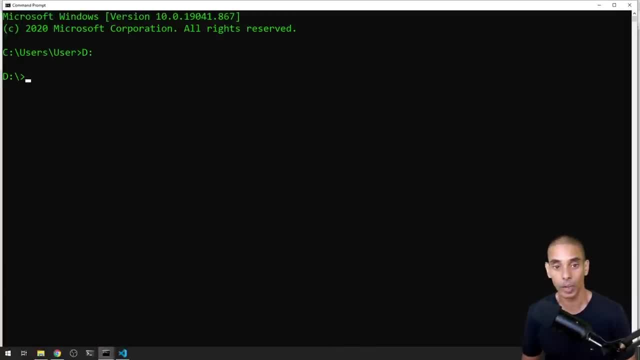 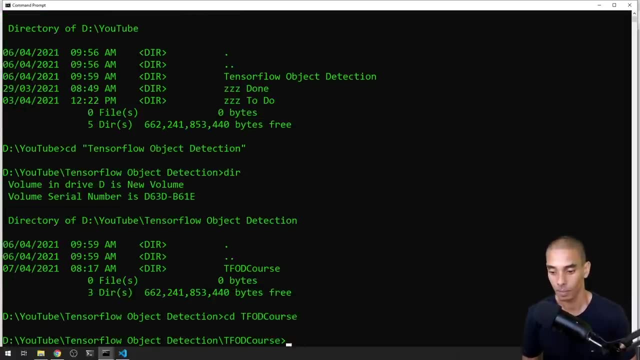 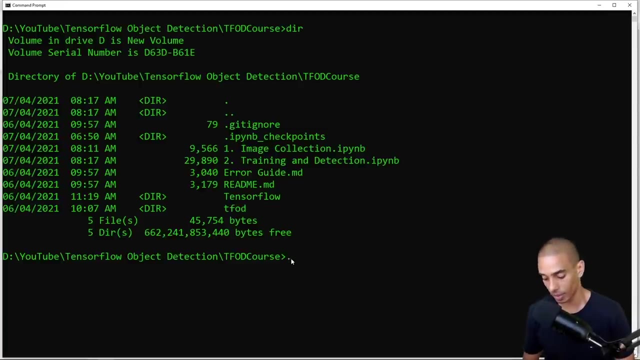 command prompt and, as per usual, we're going to go to where our virtual environment is and activate that. so let's go and do that. okay? so that's where our virtual environment is. so you can see that we've got tfod there, so we can activate that. so remember, dot backslash tfod scripts activate. 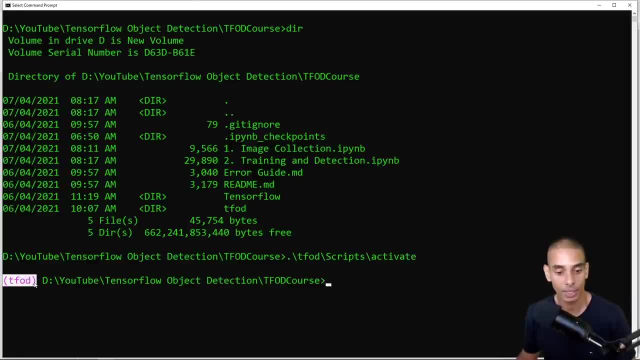 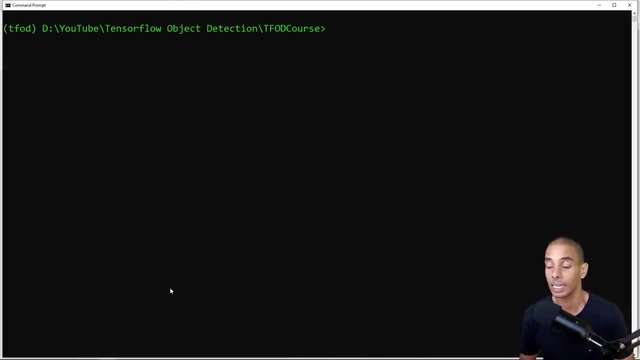 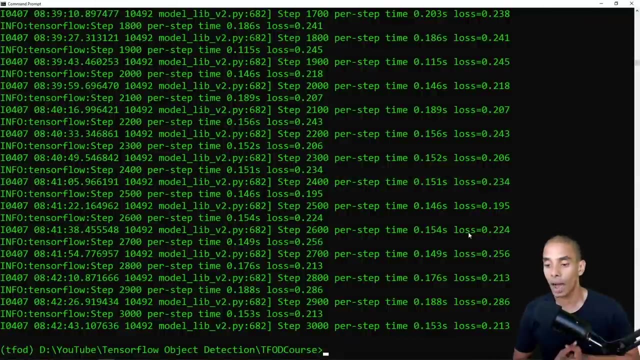 so that's our virtual environment, now activated. you can see it there, and then what we can do is paste in our training command. so let's go on ahead and run this, and ideally we should have a train model come right about after you, okay? so after 3 000 steps of training, we finally got our final trained model, which had a loss of. 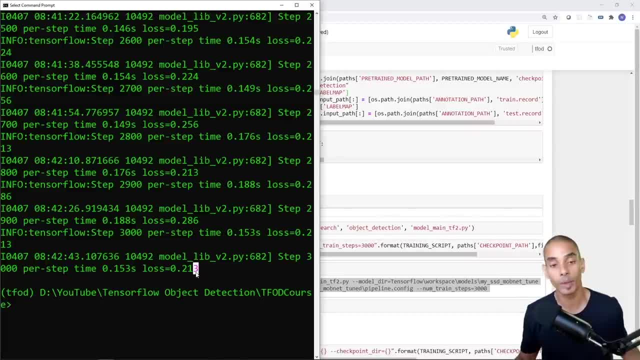 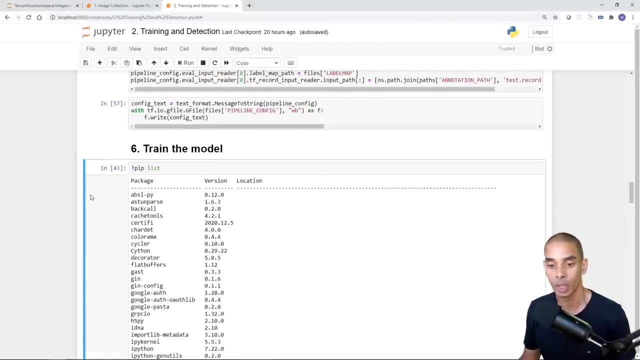 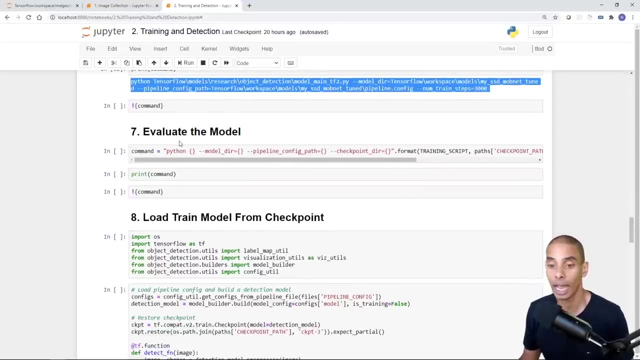 0.213. now, keep in mind we had more images. we had images at different angles, so ideally, what we want to do is run our valuation script to see how our model is actually performing. so, remember, our last model had a- i believe it was mean average precision of 0.7. so now we can see what our model 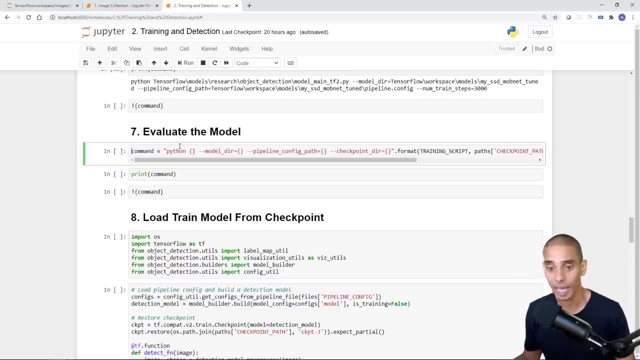 or how our model is performing. so let's go ahead and run our evaluation script and let's see what our model is actually performing. so remember, our last model had a- i believe it was mean- average is performing like this time. so to evaluate our model, remember we just go through and run the 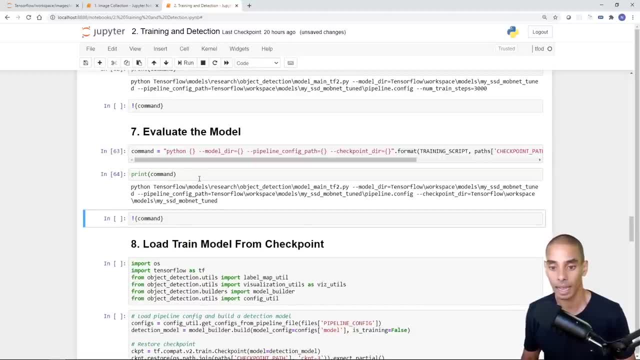 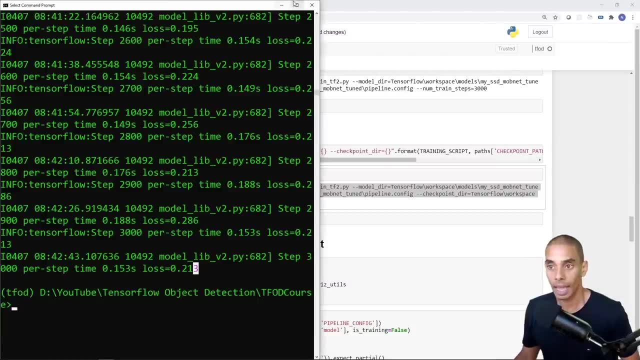 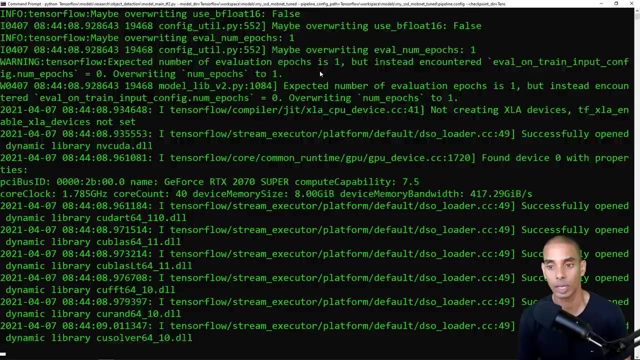 code under step seven. so if we hit that and enter that, so this is going to give us our new evaluation code, so we can copy this over and paste it into a mod or into our command prompt. so this should ideally run our evaluation pipeline. so it will take a little while and ideally we should get 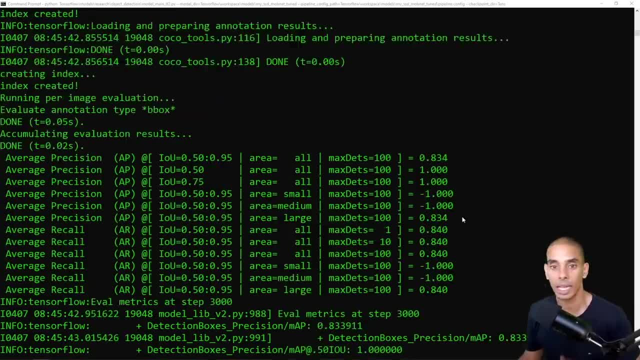 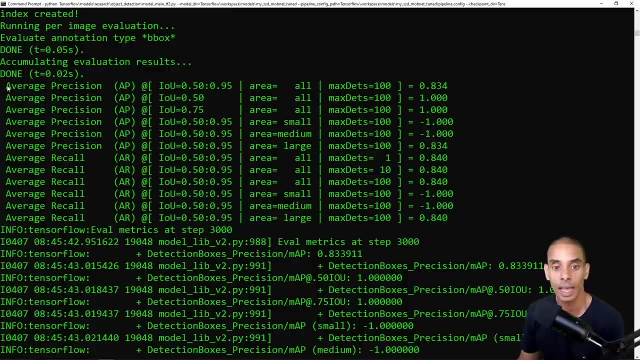 some evaluation metrics generated, okay, and you can see that we've now got our valuation metrics calculated and it looks like we have managed to improve our model. so you can see here that our average precision is now 0.834, so that's a bit of a reasonably large jump compared to what 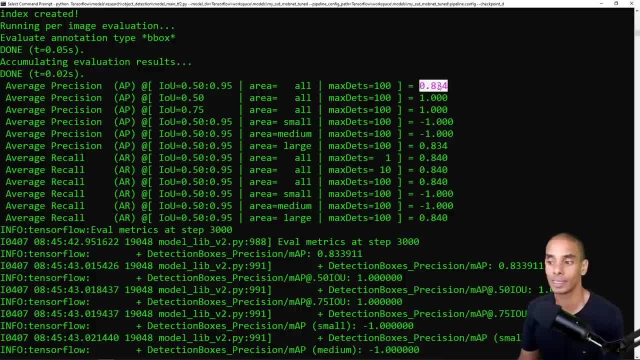 we had initially so before this was about 0.7, and i believe average recall was 0.69 or something along those lines. so again, they were way lower. they were in the sevens and sixes, not the 84 to 80- what 84 range. so so again, we have managed to improve our model and generate a better object. 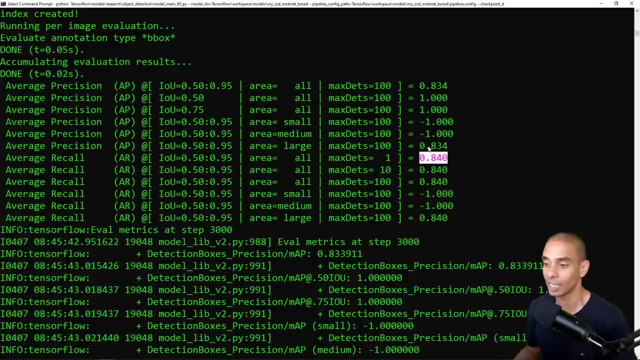 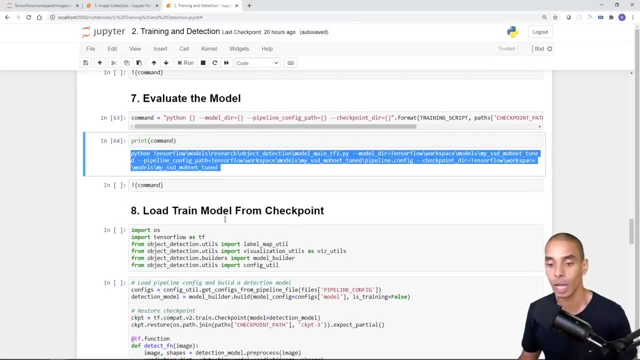 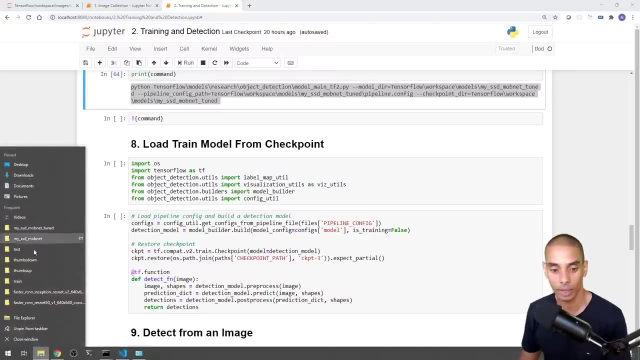 detection model. so simply by adding more images, um, adding additional labels and different positions, we've ideally produced a model which should generalize better. now, what we can actually do as well is again load this new model now, because we have trained for longer, we're going to have a new checkpoint, so if we create a- let me just show you this- so again, if we go back into our 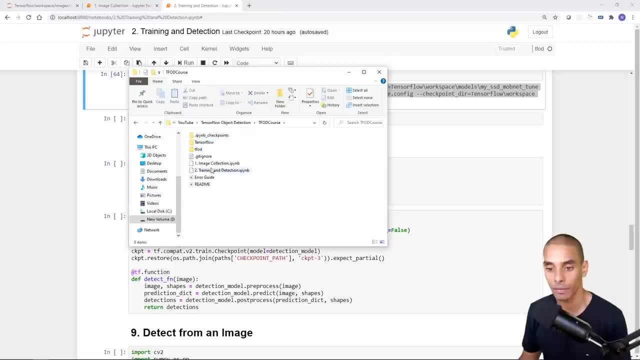 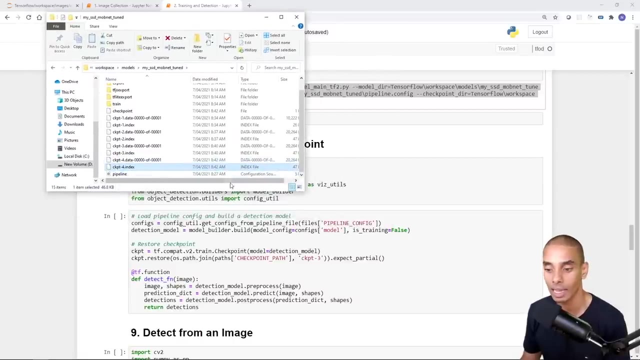 directory: youtube: tensorflow object detection- tfod course- tensorflow workspace models. and remember. so this was our baseline model that we initially trained, and then we trained our tuned model. now, if we open this up, you can see we're all the way up to checkpoint four. so this is our latest model. 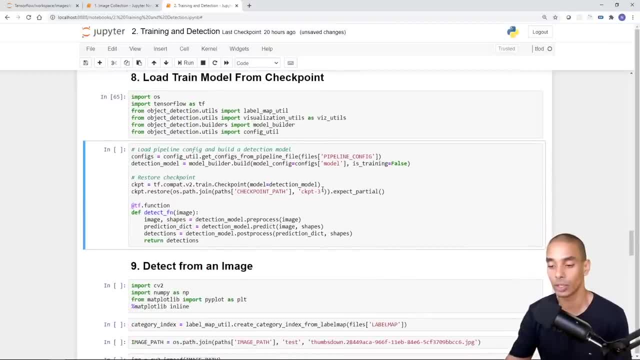 so, in order to load this, what we need to do is change the checkpoint that we're going to be loading. so, rather than loading checkpoint three, we need to load checkpoint four and then what. we can actually go and run some detection. so, rather than detecting from an image, let's just jump. 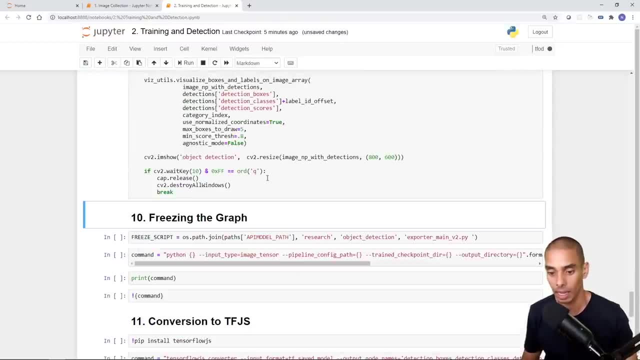 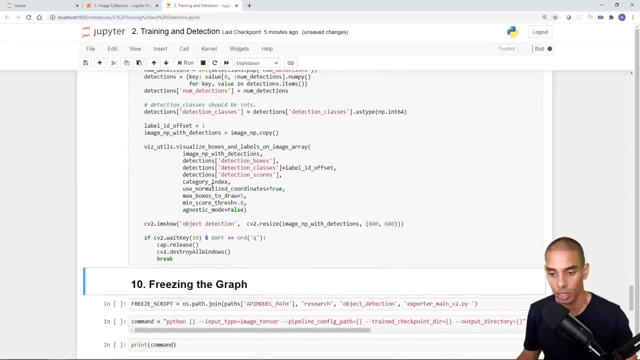 straight to real-time detection, which is effectively this cell here, and if we run that, that should effectively open up our webcam and give us the ability to make some real-time detection. so let's see how that actually performs. okay, so we've got our detection window. thumbs up, thumbs down. 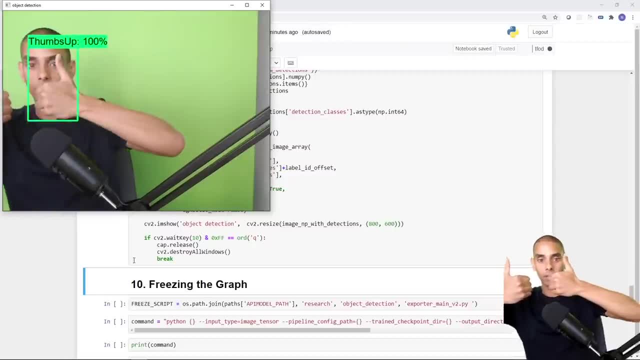 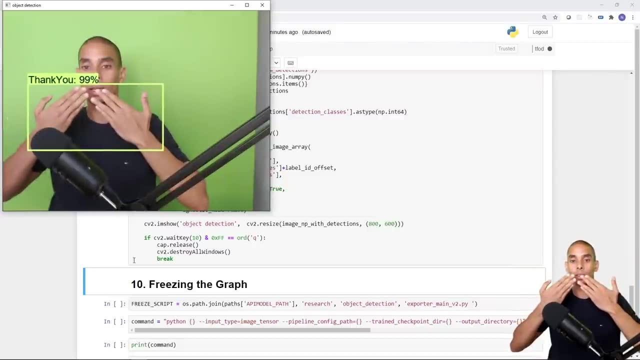 thumbs up, thumbs down. so this is detecting live long, so let's move over a little bit. there you go way better, right. so that's again forming ridiculously quickly. so we did train for longer, we trained with more images, so really fast. so right now we're really really quick. 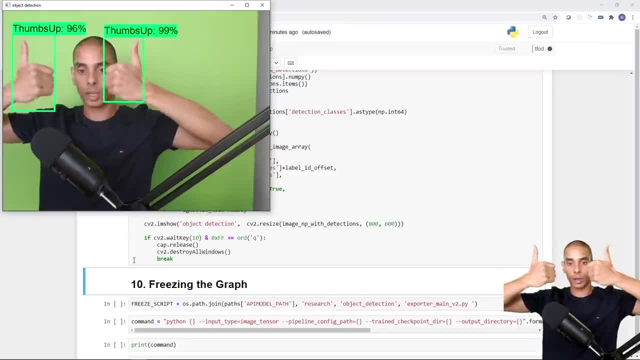 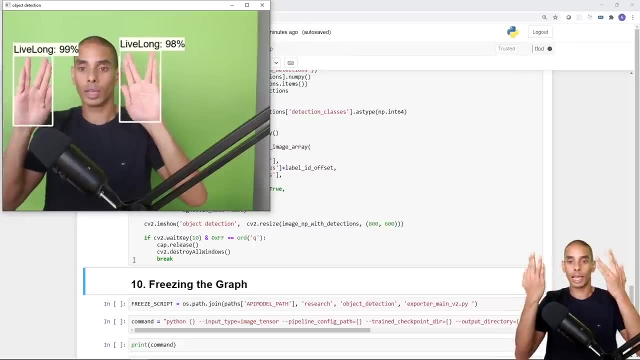 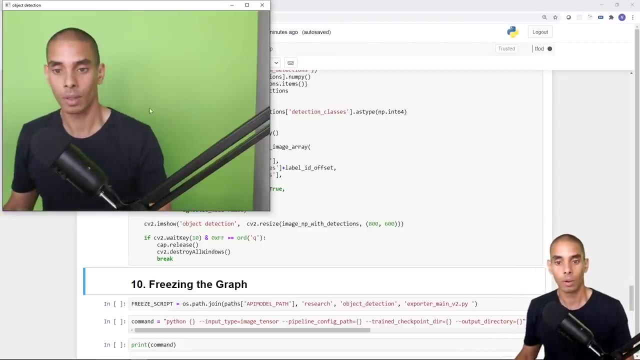 and this is switching really fast as long as my hands aren't below, and so that sort of gives you an idea as to how you can go about performance tuning. so again, you can see it's very, very quick and we're doing pretty well there. awesome, all right, cool. now the next thing that you can also do in: 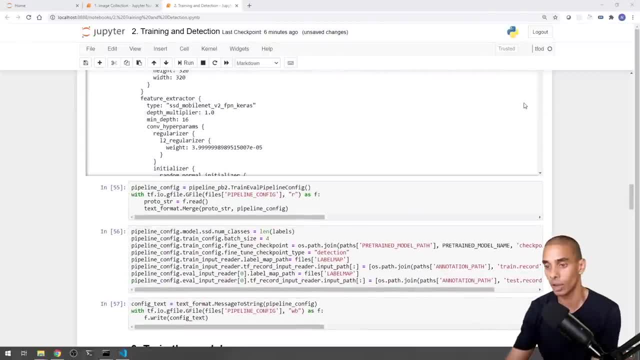 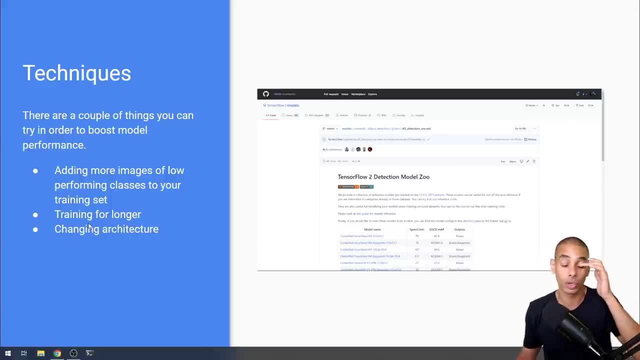 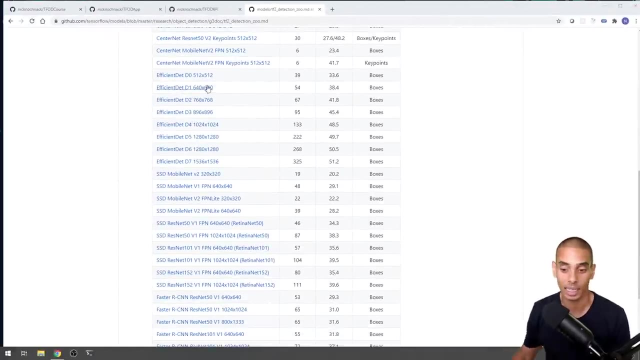 order to performance student is change the architecture. so we cast our minds back. we sort of talked a little bit about adding more images and training for longer. now the next thing that you can also do is change the architecture. now, in order to do this, you can re all you really need to do with the particular code set that i've got. 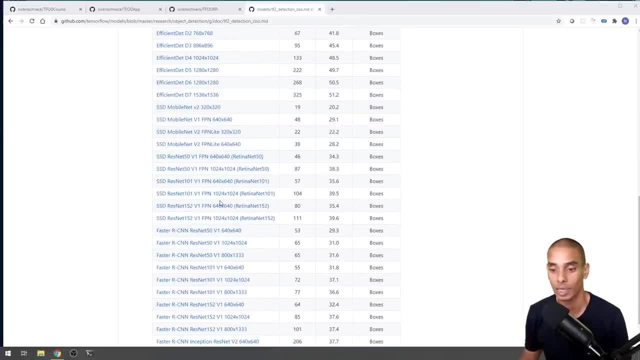 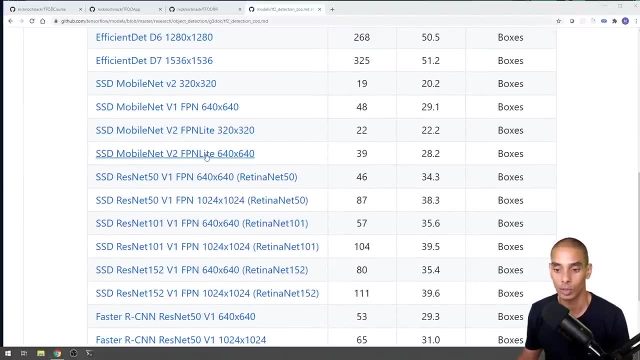 is change the link that you actually want to use. so in this case we're using- let me just zoom in- we are using this 320 by 320 model but say, for example, we wanted to use uh, this one over here. so again, there's some nuances if you want to tune them, but really all it's a matter of doing is. 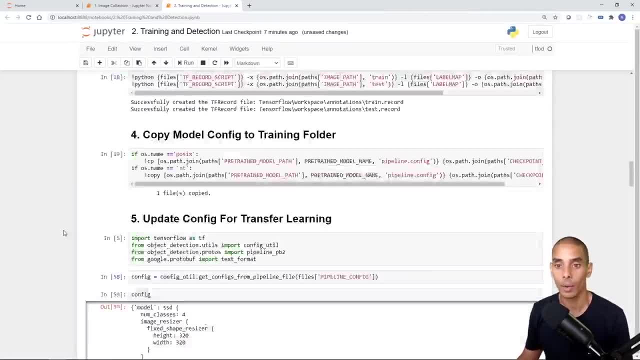 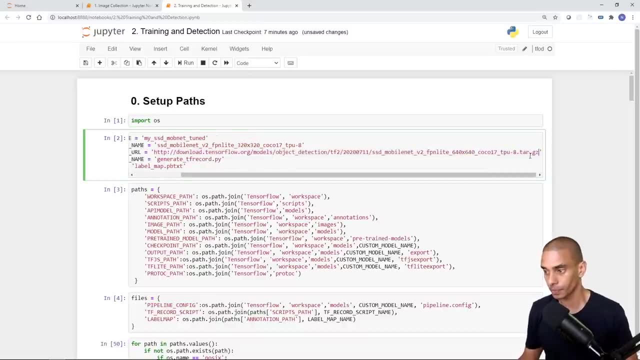 copying the link address and then going back over to our detection notebook and changing the pre-trained model url. so if i actually run this so you can see it's updated the url for that specific model and then what we need to do. so once we've got that, we just need to grab this name here. 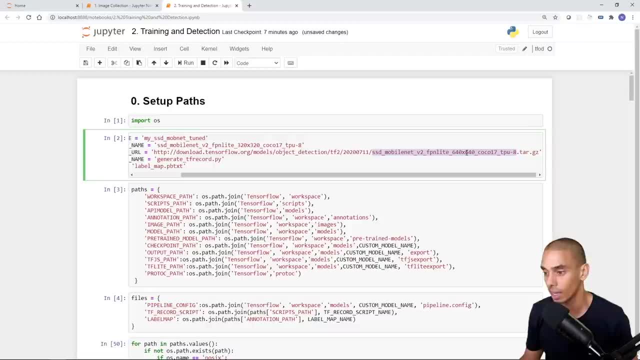 so you can see here that it's called ssd mobile net v2 fpn light 640 by 640.. goko 17 underscore tpu dash 8.. so we can copy that over and paste it here. so this is effectively going to give us. 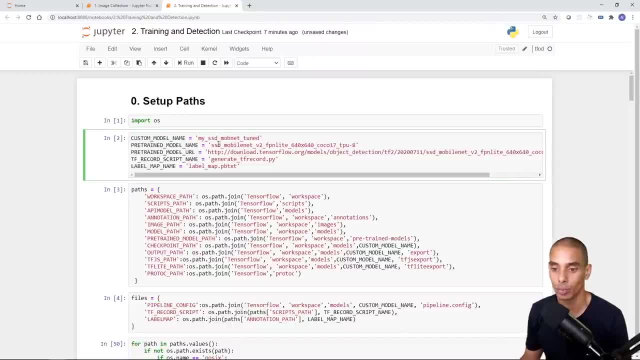 the ability to go and grab a new pre-train model. so when i run this, it's going to download a new pre-trained model and effectively walk us through the exact same steps. now i'm not going to go through this in a huge amount of detail, but if you'd like to see a more detailed video on your 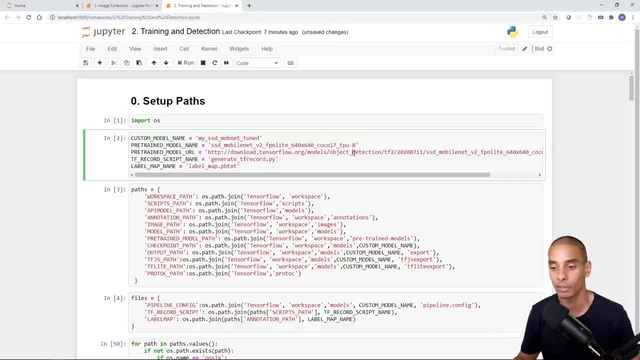 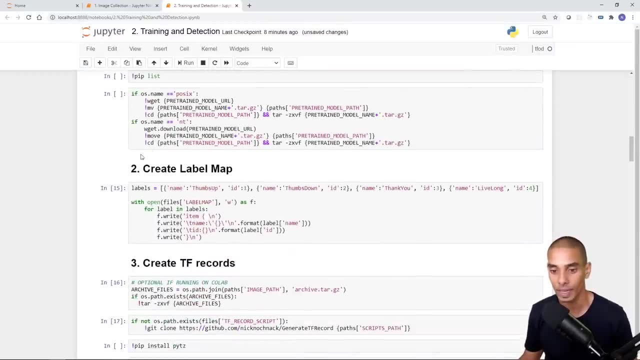 um. if you'd like to see a more detailed video on your um, if you'd like to see a more detailed video on your using different architectures, by all means do let me know. But it sort of gives you a feel for how you might go about this. So, really, you grab the new model link And then this cell over here. 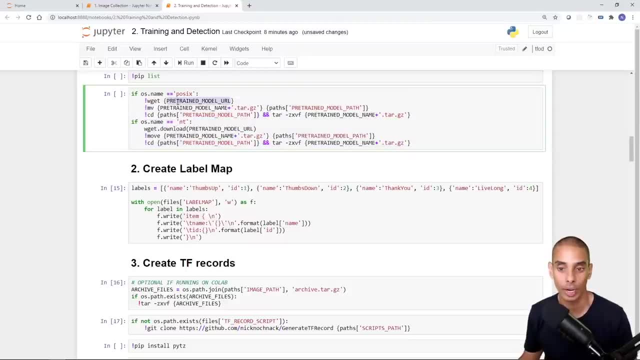 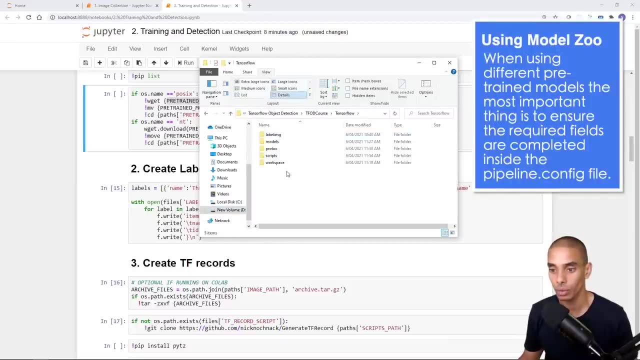 is actually going to go on ahead and download that new pre-trained model. So then what will happen is inside of your pre-trained models folder, workspace- pre-trained models, So you'll get, as you can see that I've already downloaded a bunch of different ones, So it'll just download. 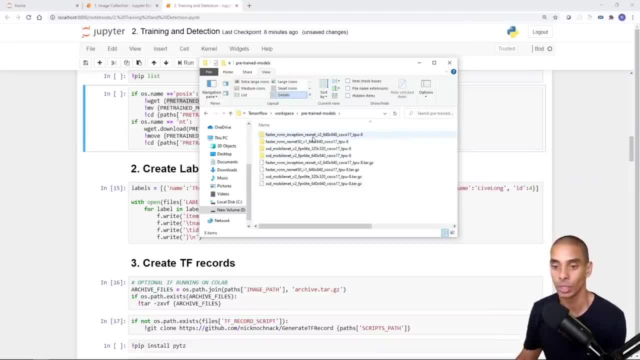 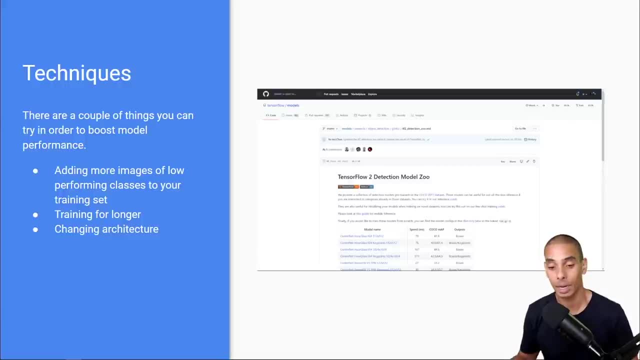 a new pre-trained model that you're able to use. So that about wraps up performance tuning. So we did a bunch of stuff there. We didn't really need to change our model architecture in order to get better performance. Really, it's about the image quality, So rubbish in is going to equal rubbish. 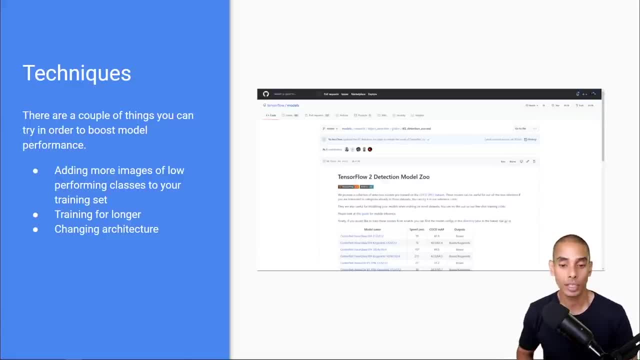 out. Quality in is going to equal quality out. So having different styles of images, different images of different qualities and different images at different angles, as well as training for longer, more often than not is going to be sufficient for producing a better model. 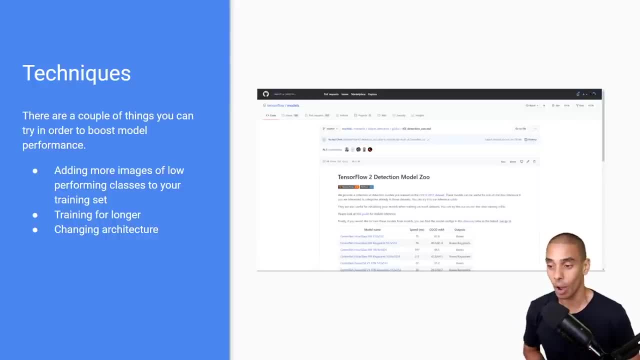 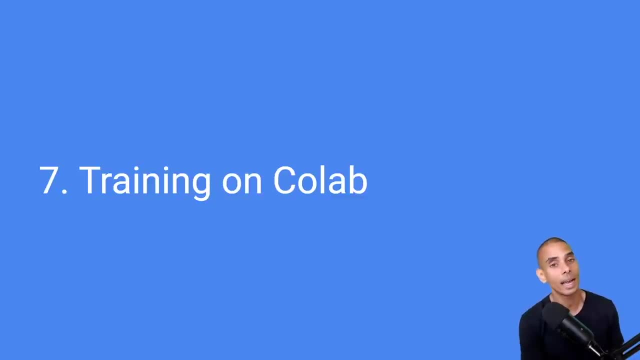 So this brings us to our next part: training on Colab. So, in order to train on Colab, you can go through pretty much the same steps. The core difference is that you need to have collected your images already in order to be able to do this. So let's go on ahead and jump onto Colab. 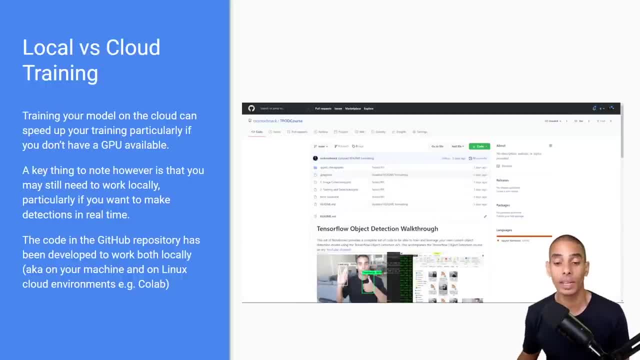 and we'll start doing that. So again, the core thing that I was saying is that, in order to train on Colab, you do need to have your images pre-collected. It just makes your life pre-collected and pre-annotated. It's just going to make your life a bunch easier. 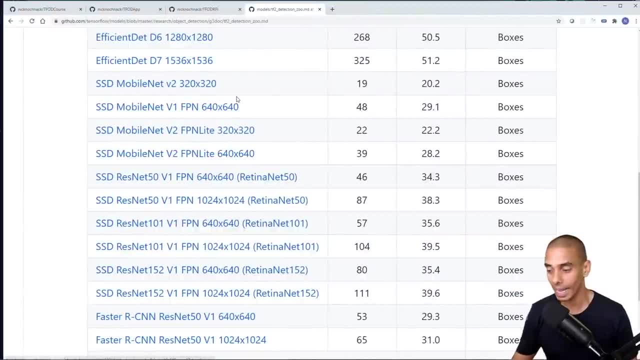 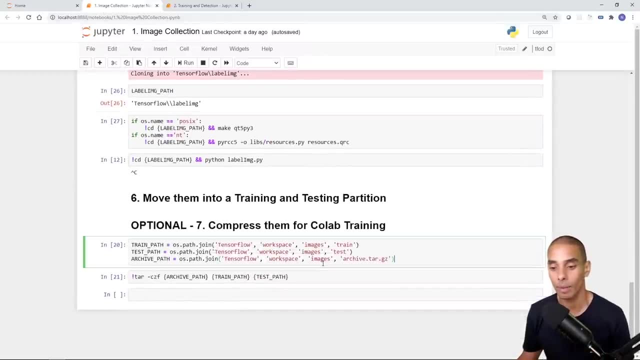 So let's go on ahead and do this Now. the easiest way to get your images onto Colab is inside of our image collection notebook. Right down the bottom, I had this code cell which allows you to compress your images and archive them. So if we actually run that cell, 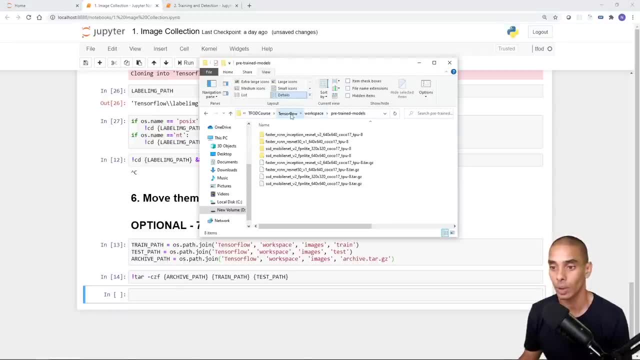 this is going to compress the images that we've got. So if we go into our images folder now- workspace images- you now you're now going to have this file called archivetargz. So this is all of our images from our training and testing folder and now compressed and 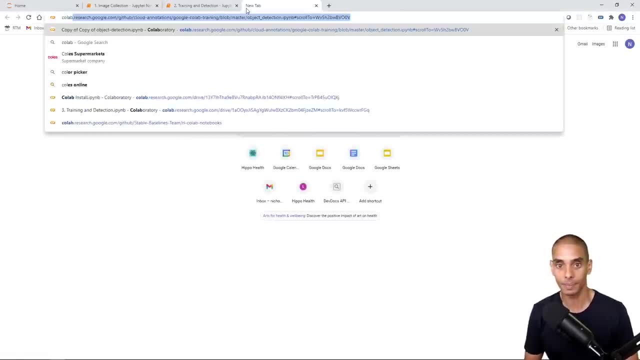 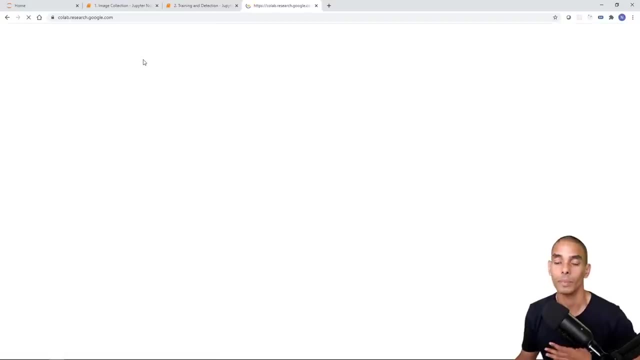 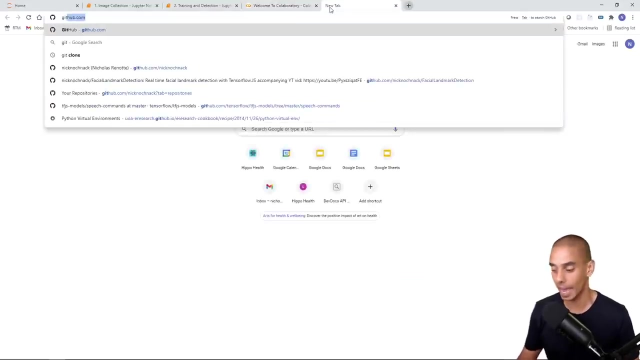 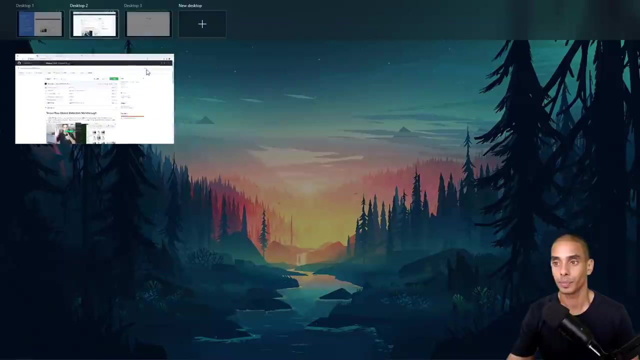 archived. So what we can actually do is jump on over to Colab. So in this case I've just gone to colabresearchgooglecom And then I can actually bring in a GitHub file. So what we'll do is we'll grab in our main GitHub repository, which was: where are we So? tfodcoursecom. 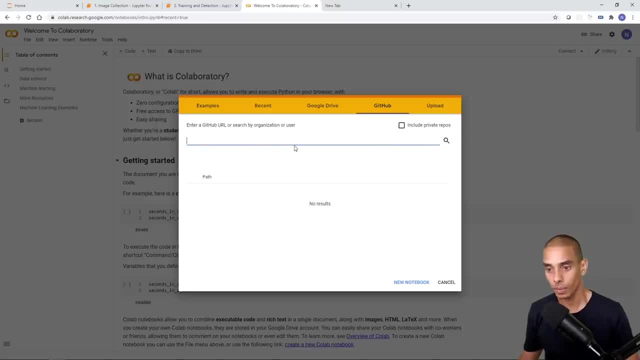 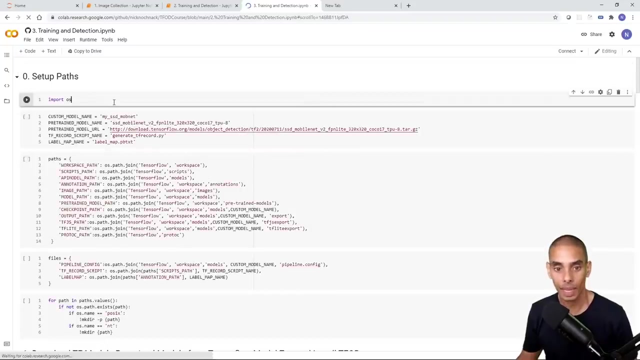 We can paste that link in, And then we're really interested in our training and detection notebook. So let's grab that. And then the nice thing about this notebook that I've set up is that you can sort of just walk through this notebook Now if you don't want to have to deal with all of the installation. 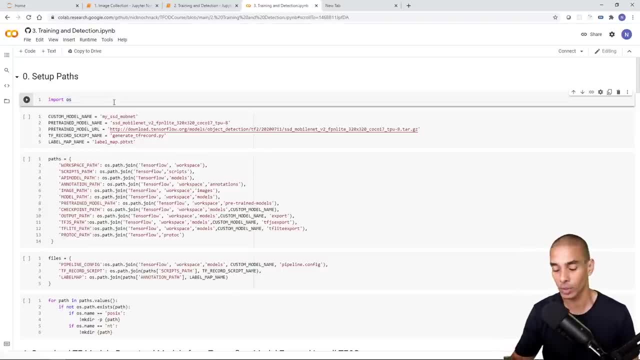 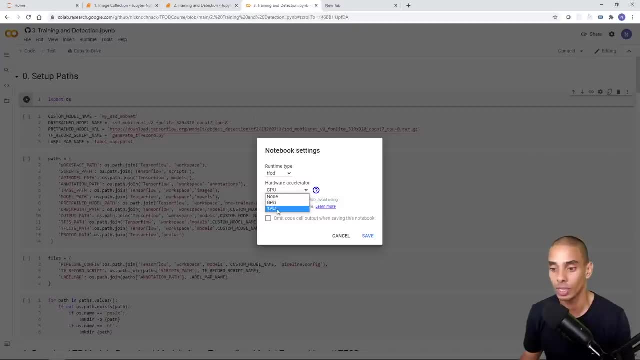 steps and all of that stuff that we had to do to get us up and running. Colab sort of gives you a nice alternative to that. The core thing you need to do is go to your runtime and change your runtime type to GPU. In this case, it looks like it's already selected, So we can hit GPU and hit save. And then what? 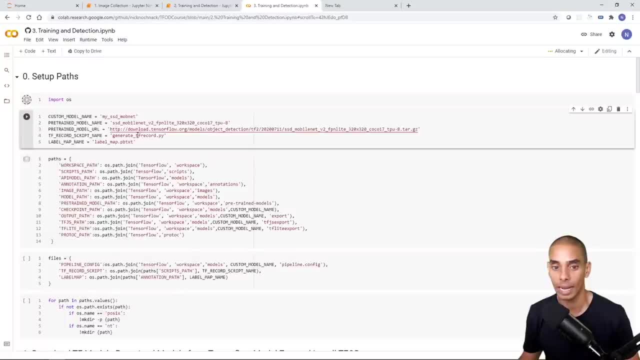 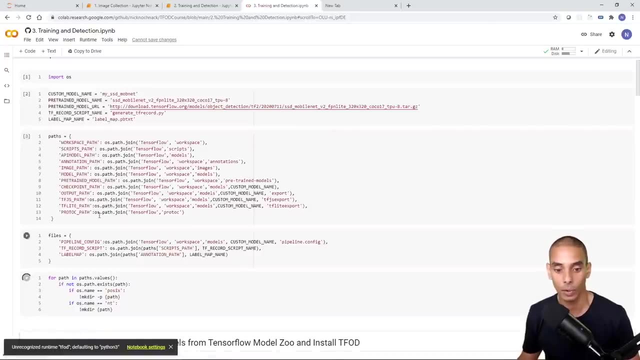 we're going to do is step through our notebook, So we're going to hit shift, enter and run anyway, And this is going to start importing and creating our folder structures. So again, by running the first four cells, we should have our folder structure created. You can. 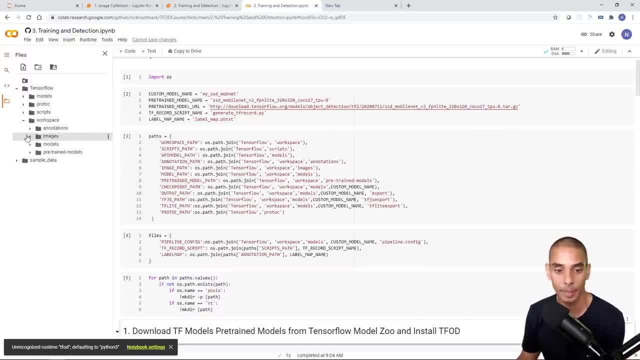 see, we do So. TensorFlow workspace annotations images. Now the one thing that you will need to do is upload your files, so specifically your images. So if we select our images folder, what we're going to do is upload the images. 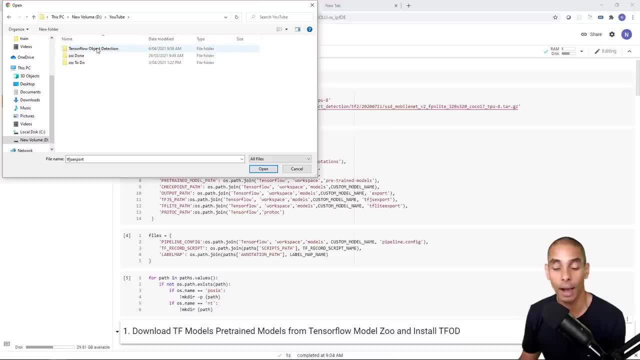 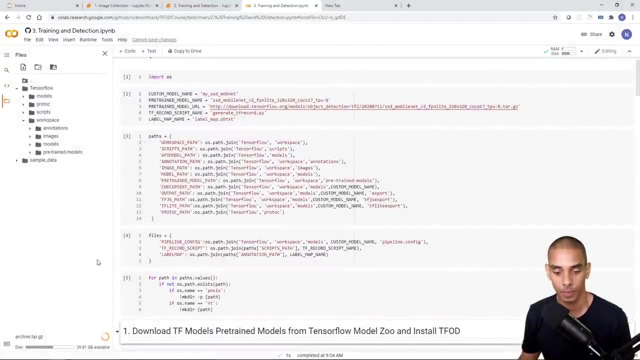 that we just compressed. So we're going to go into where our archive is. So TensorFlow object detection- TFOD course. TensorFlow workspace images. And then remember we had this archive, So let's upload that. So we've now got our archivetargz file there. What we'll do is we'll copy that into our 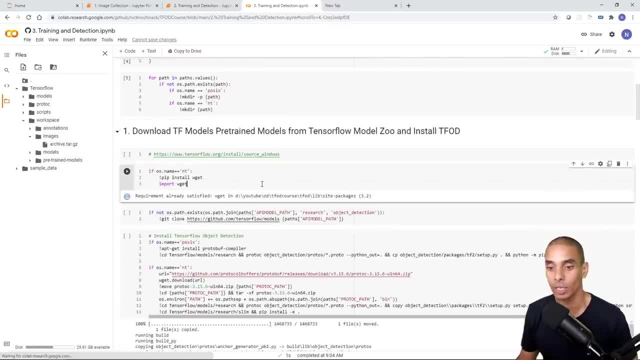 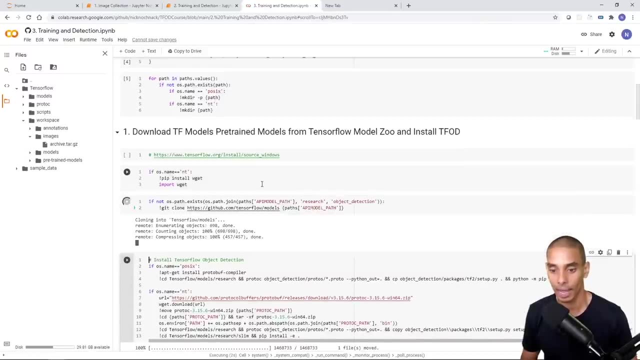 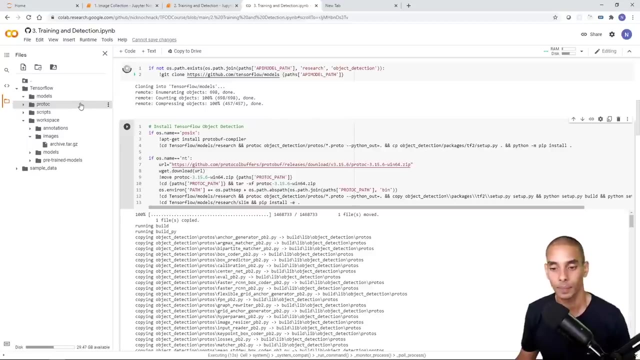 images folder, And then when we actually go through the rest of this notebook, so let's just hit shift enter. So if we keep going through, so this is going to clone our TensorFlow models repo, which should give us our files in here once that's done. And then if we go, 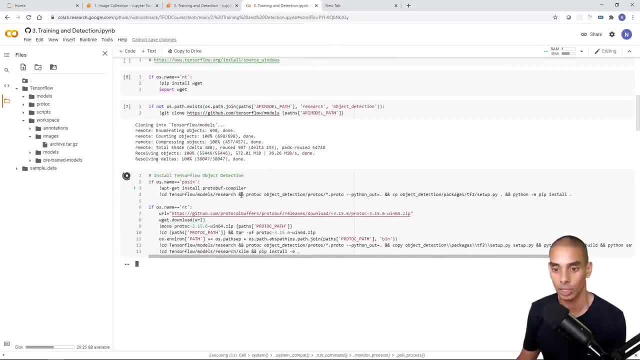 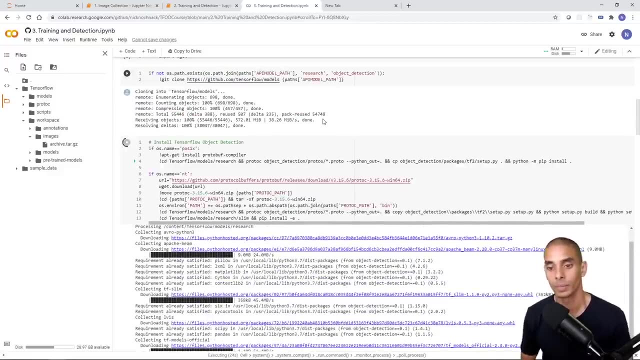 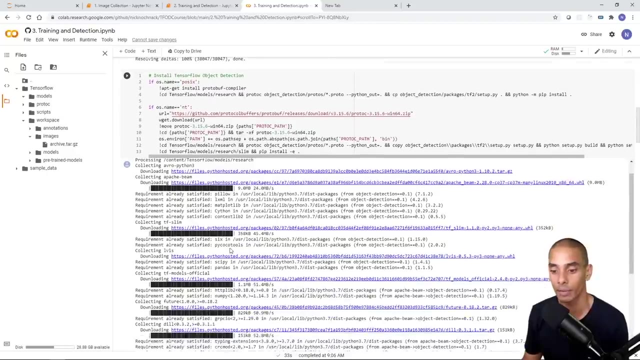 to our next cell. so now we're installing TensorFlowar object detection, So this will take a little while, And so keep in mind, this is installing all of our dependencies to be able to leverage TensorFlow object detection. So that's looking promising. at the moment, looks like it's all. 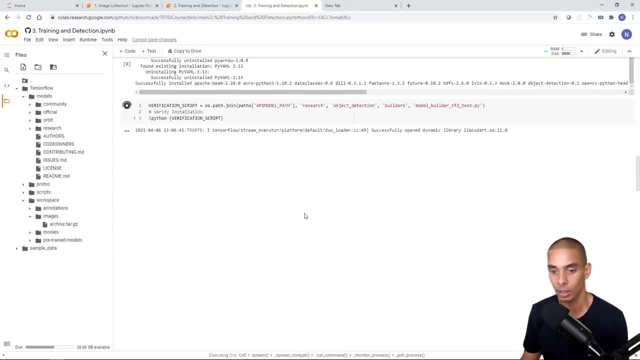 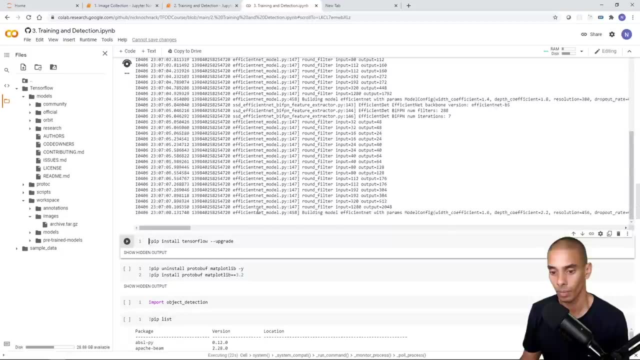 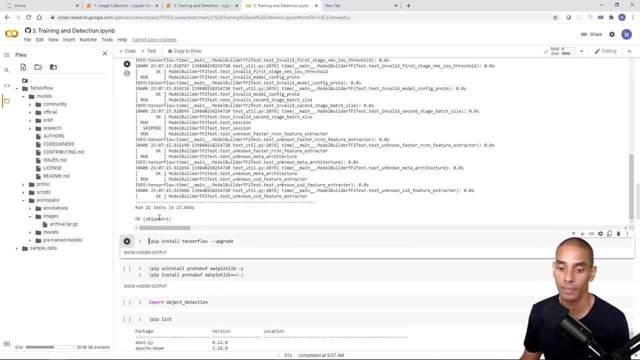 installed, we can run our verification script, see if that's all good. So this is looking promising. at the moment doesn't look like we've got any errors And again, whenever you're running the verification script got a check that it says okay. so 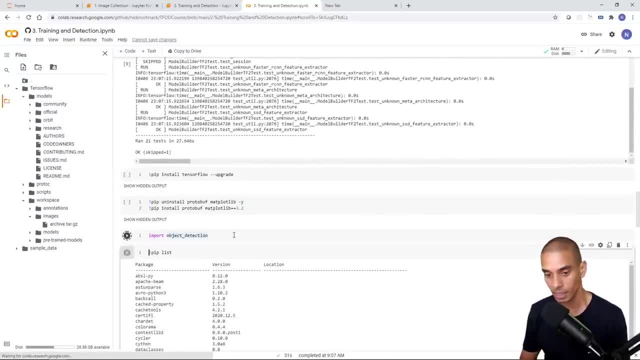 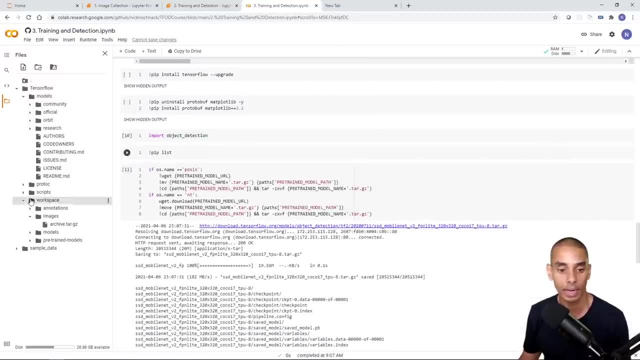 in this case we've got the all clear. so that's looking fine. Test importing, object detection: no issues there, So we're good to go right. So what we can now do is bring in our pre trained model. So again, pretty standard. So this is going to give us a pre. 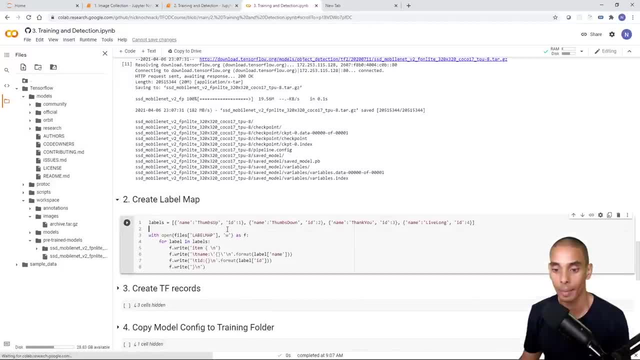 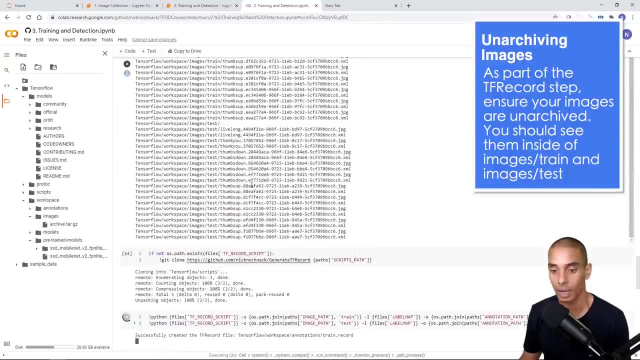 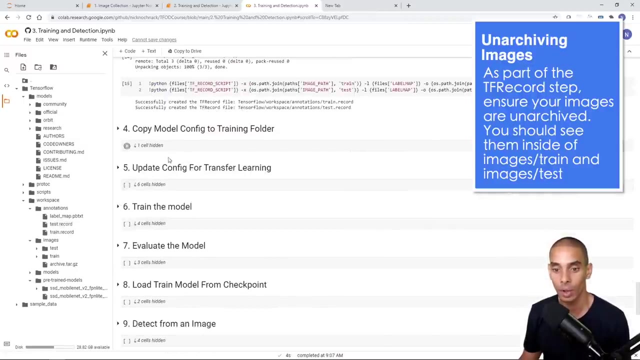 trained model over here. We can then create our label map, Create our TF records, Create our TF records. so again, this is going to create our tf record. so if we go into our annotations, we've now got our test record and our train record created. we can then go into our. so what? 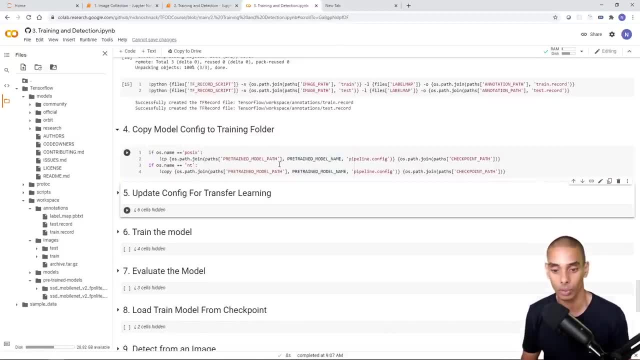 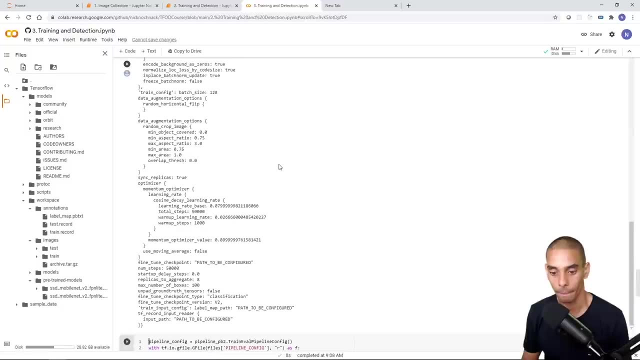 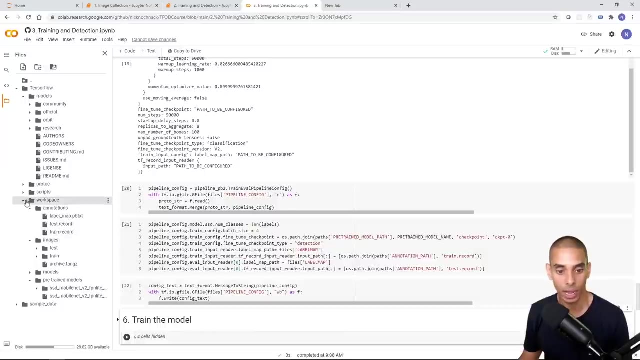 we'll do is we'll copy our pipeline config through. so we're just stepping through this notebook so it doesn't look like we've got any errors so far. update our config. so this should give us our custom config inside of our models. my steam mob net folder you can see. 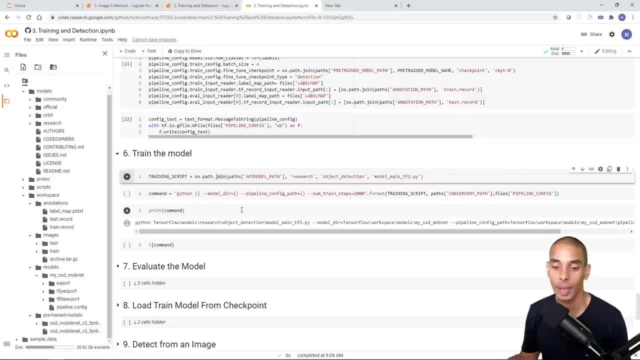 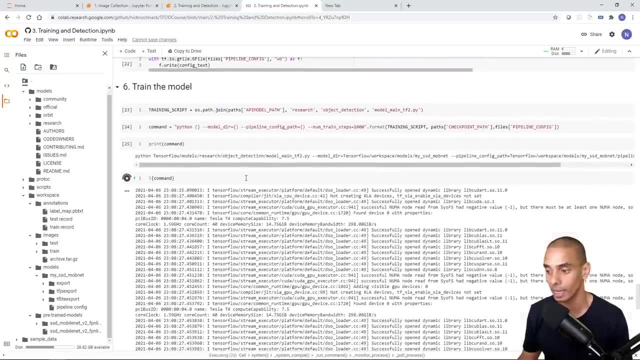 it there and then we can train the model. now the nice thing about training in colab is that we can just run through and execute that command in the cell. so you can see that now i'm running that command and all things holding equal without errors. we should get our model. 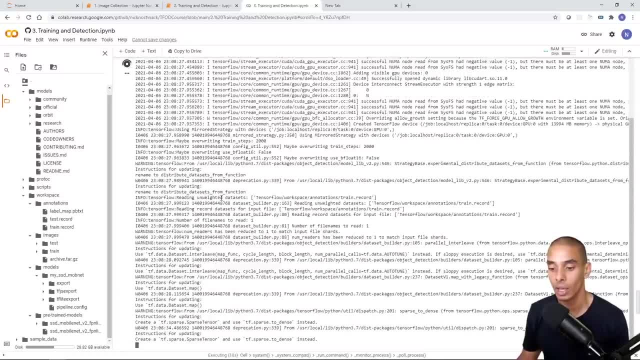 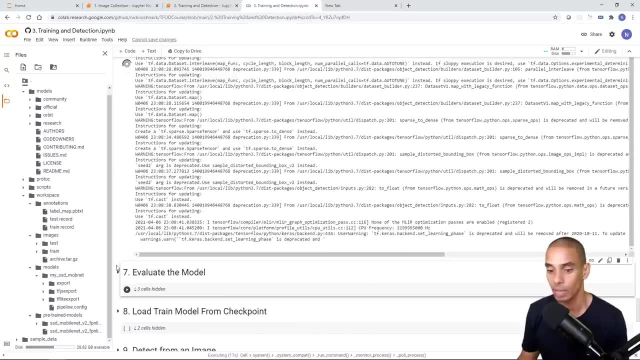 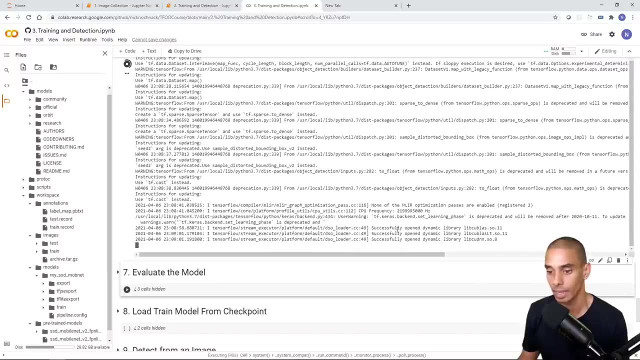 training kick off now again. the key thing in here is that you won't be able to perform real-time object detection using your webcam. you can still do it using the image, so we'll test that out. we'll see what that looks like. so that's looking like it's running there without issues. 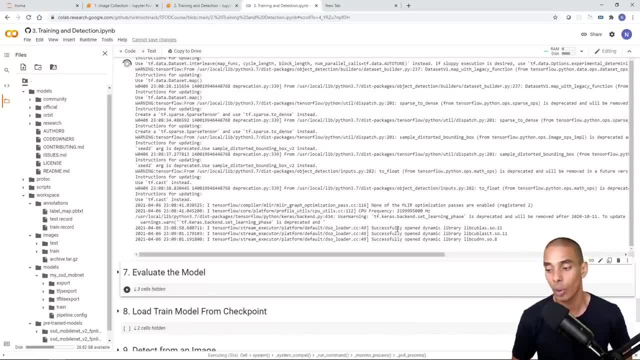 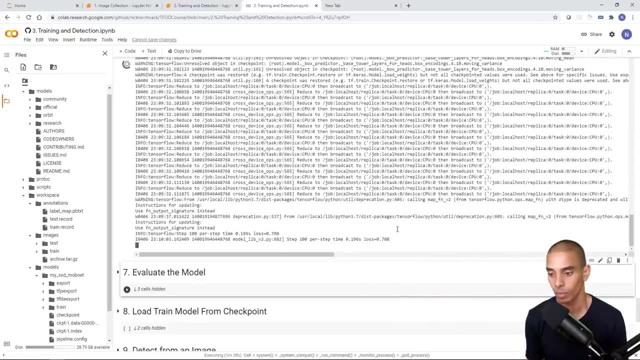 and then again we just need to wait for our loss metrics to show up, so that gives us a good indication that it's running successfully, no issues. okay, and then we can go ahead and run our training and we'll see what happens. okay, and then we can go ahead and run our training and we'll see what happens. 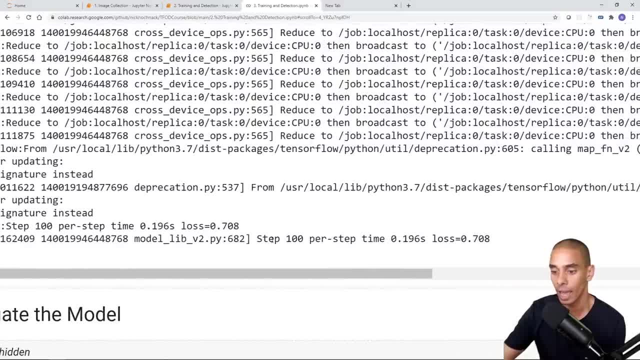 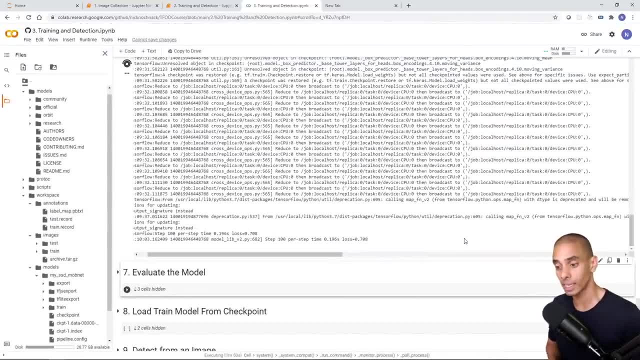 and that's our first loss metric appearing. so you can see there that we've got our step- 100 per step- and we've got our loss metrics appearing. so that's a good indication that all is successful and it's running in colab. so we can let that run and we'll 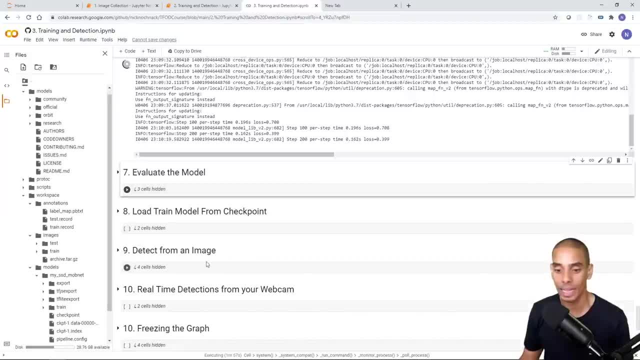 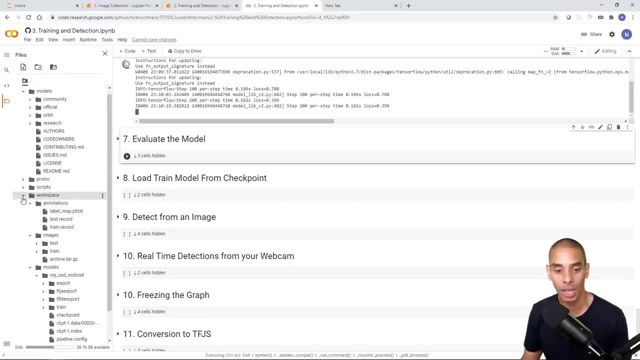 come back, evaluate that model, load it from a checkpoint and then run our detection from an image. but again, from here you can sort of keep stepping through if you wanted to. once you get to the freezing and conversion step, you can grab so you can actually zip up. 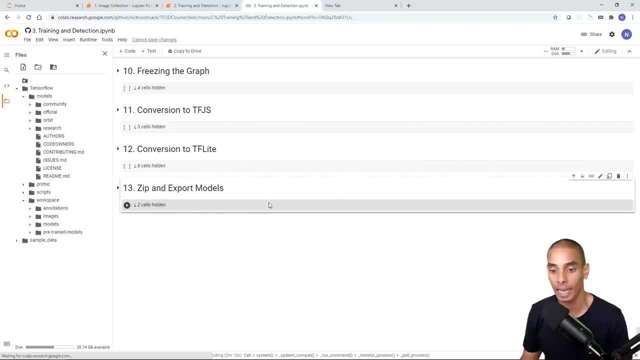 and export everything inside of this workspace folder. so i wrote the code down here so you can. if you actually wanted to grab everything, you could zip up your entire myssd mob net folder, bring it back down to your desktop and run it from there as well. but again, this looks like it's all. 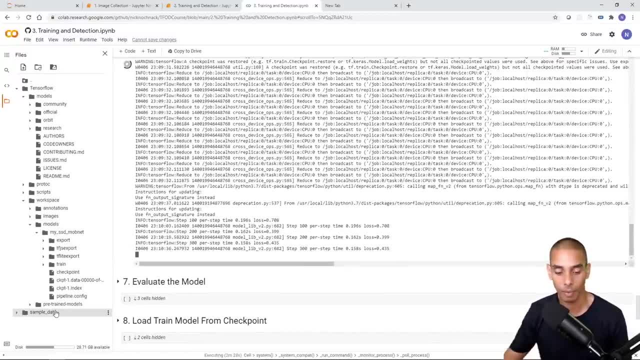 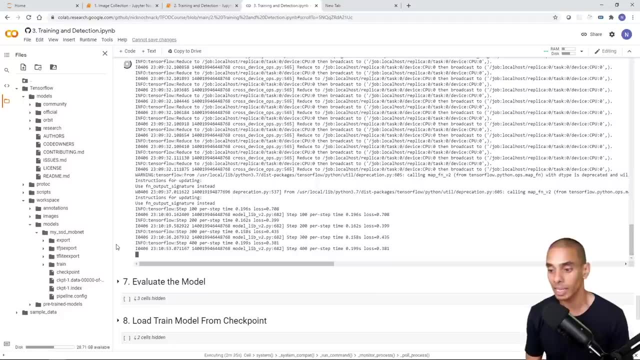 running pretty successfully. if we check out mysd mob net folder, you can see that we've got our checkpoint appearing there. so we've got checkpoint one. cool, let's let that run and we'll be right back. okay, so we're done with our step 1 SOFTWARE and now we're ready to go. have a go. now we're going. 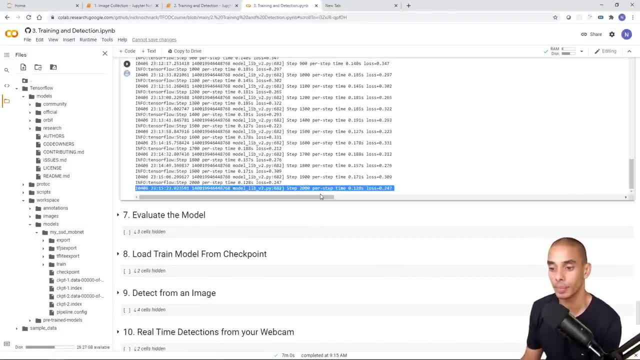 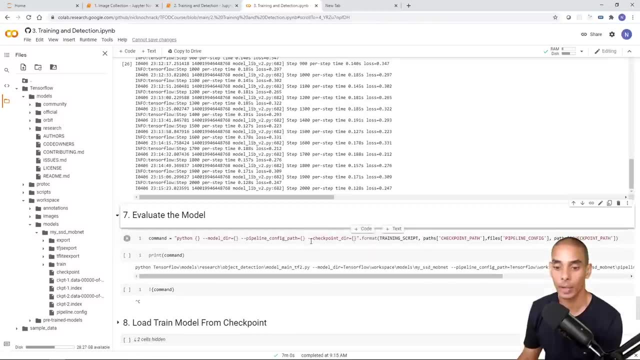 So that's our model: finish training. So you can see we got up to step 2000 right down here, with a final loss of 0.247.. Now what we can do is we can evaluate our model as well. So again, we can run it in cell. 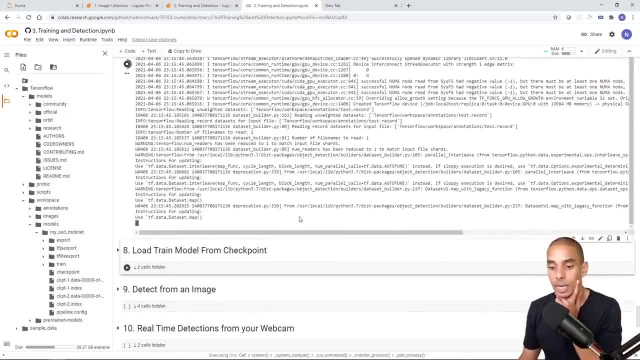 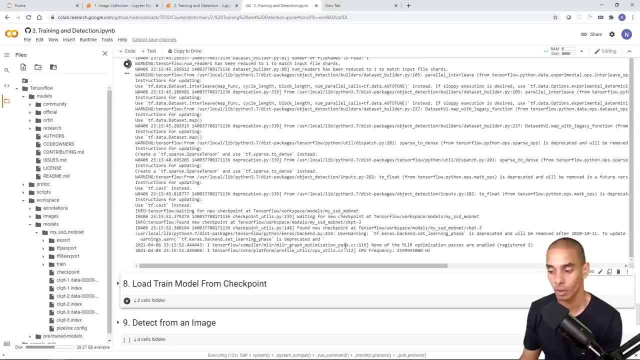 And ideally what we should see is our mean average precision and our mean or average recall as well. So ideally this will pop up once we've got that calculated And all we're really doing here is running the code under step 7 to evaluate the model. 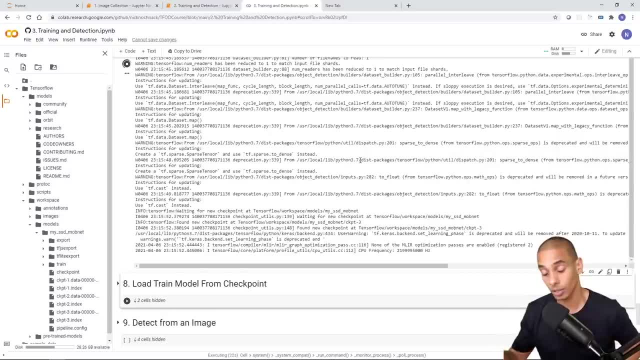 So this will appear as soon as we've got those accuracy and evaluation metrics calculated. So again, similar to what we did inside of our command prompt, but now you're doing it inside of the cell, inside of Colab. So that's looking promising. 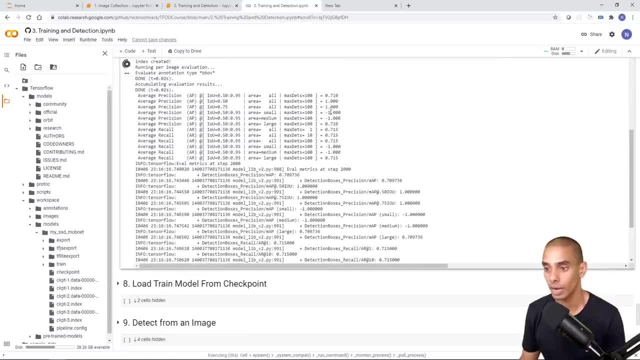 It's found, our checkpoint 3. And in a second it looks like we've got our detection metrics. So again, this is our model And this is our model. This is our non-tuned model, right? So remember, we trained our tuned model for longer. 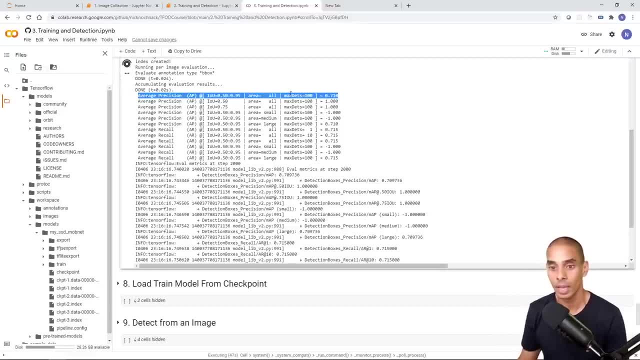 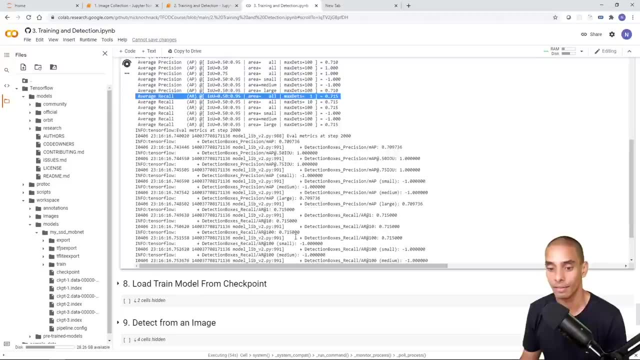 We ran that for 3000 steps. This was only 2000 steps, So you can see our average precision in this case is 0.71 and our average recall is 0.715.. Now what we can do is we can also detect our model using an image. 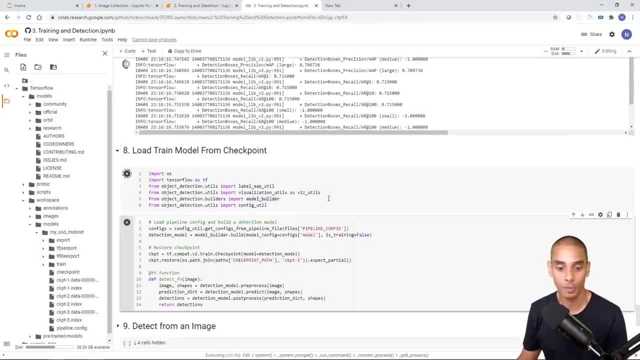 So we can run through our cells to load up our model. In this case, our latest checkpoint is checkpoint 3.. So all we need to do is change our checkpoint to checkpoint 3. In this line here which is checkpointrestore. So this is going to load up checkpoint 3 into our notebook so we can actually leave reject. 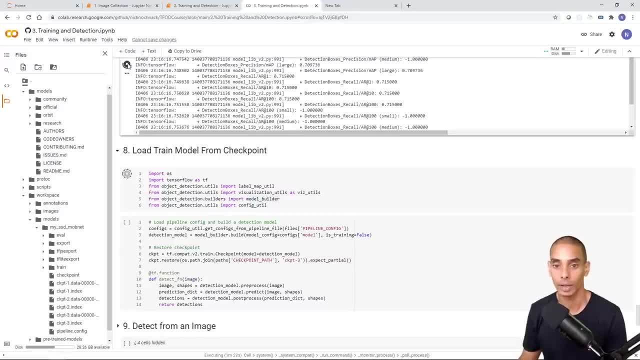 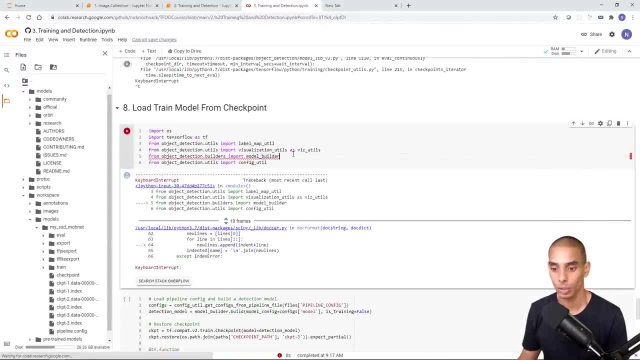 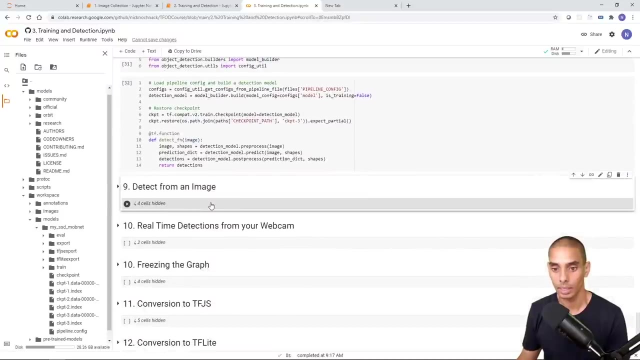 So if we run that cell well, we actually need to stop our evaluation first, And then we should be able to continue onwards and detect from an image. So in this case, we're going to be detecting from an image. So what happened? 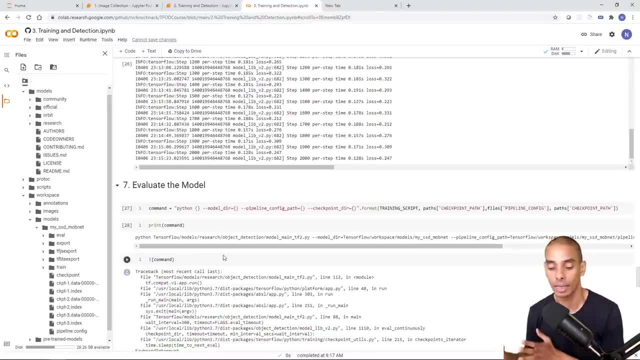 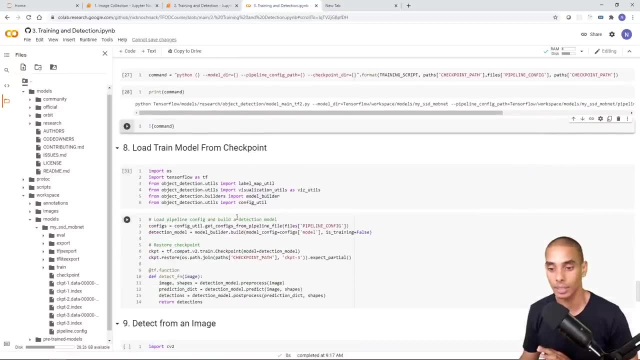 As we, our evaluation script is going to keep running and keep looking for a new checkpoint. So we actually need to force stop that in order to continue on with our cells. So in this case, I just hit stop to get that to stop. 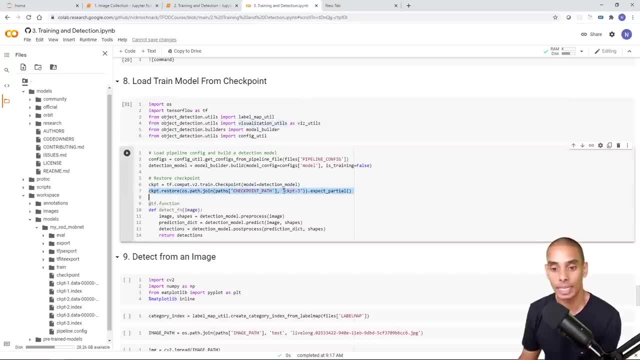 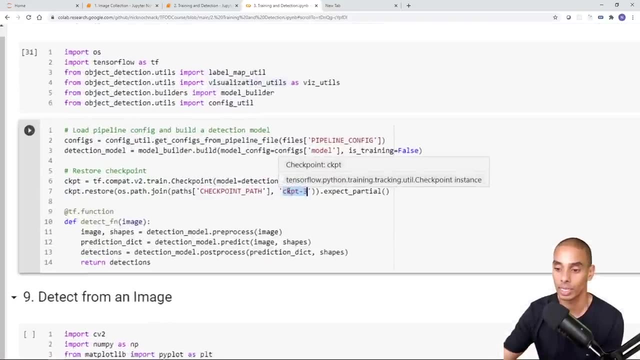 Now what we can do is we can load from our checkpoint. So what we really just did there is: we changed our checkpointrestore file and we made sure that we're pointing through to the latest checkpoint. So in this case it's going to be checkpoint 3, which is what we've got over there. 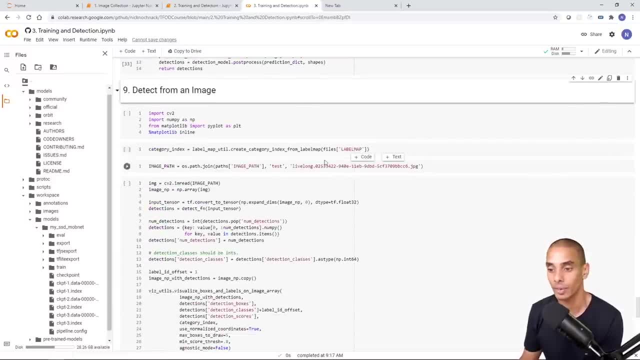 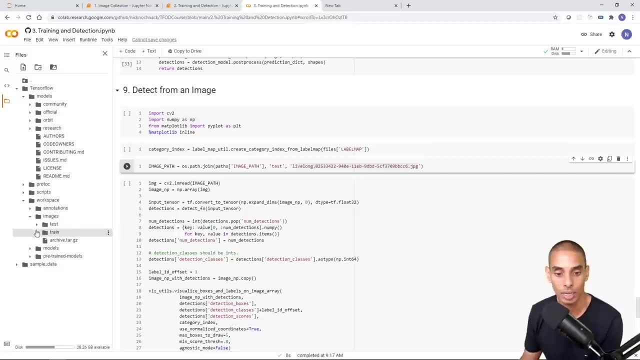 So if we run that that's all looking good And then we can detect from an image, So remember our image name- it needs to be a valid image inside of our images folder. So if we open up images and then test, you can see that we've got. let's make sure that we've actually got this file. 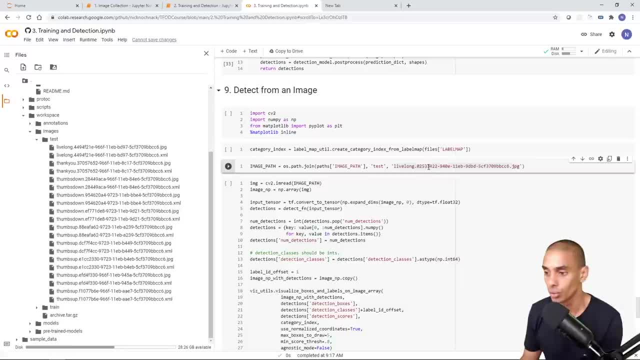 So we have a live long: 0,, 2,, 5,, 3,, 4,, 2,, 2.. So let's take a look to see whether or not we've got that. Well, easy, Yeah, We can just copy the name of this file. 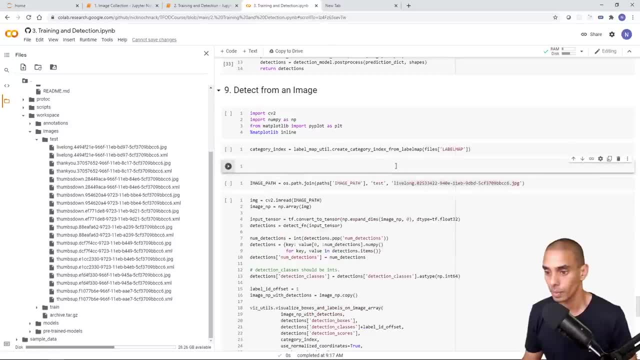 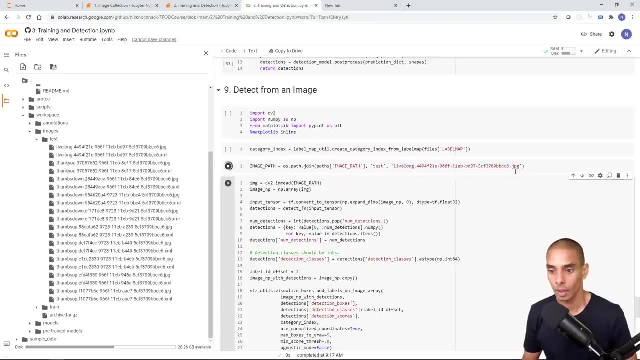 So let's grab this one and we don't need a new code cell, So let's just paste the name of the file there And then we should need to run these two cells to bring it. So this is going to bring in our dependencies. 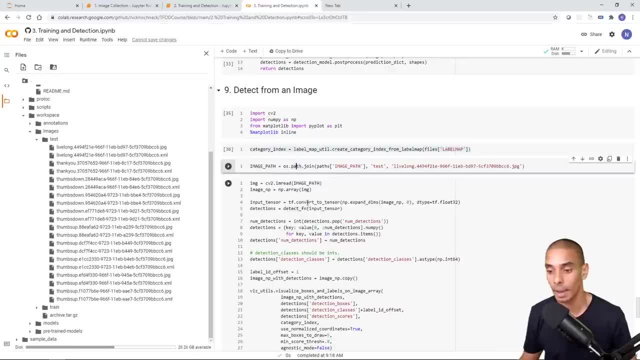 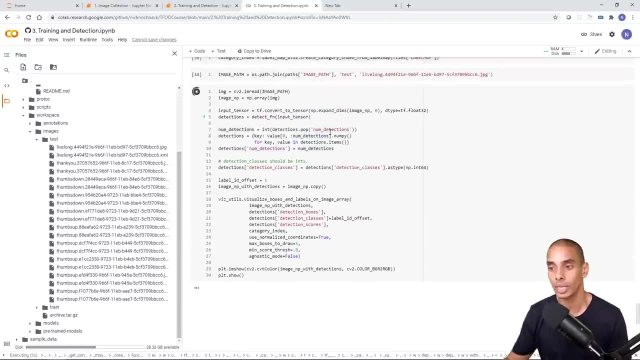 It's going to load up our category index- again same as what we did in our baseline notebook- And then, if we run this cell, ideally we should be able to see our detection. So this is going to run using our object detection model and try to make a detection using that particular image. 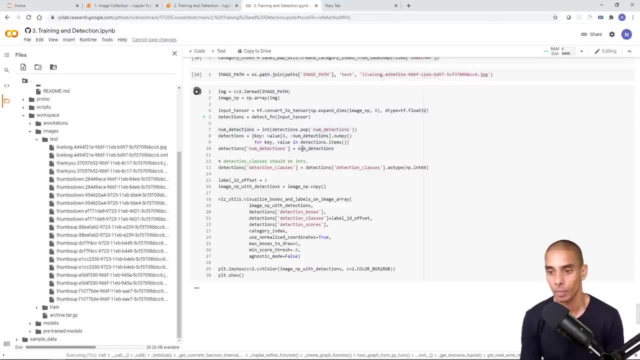 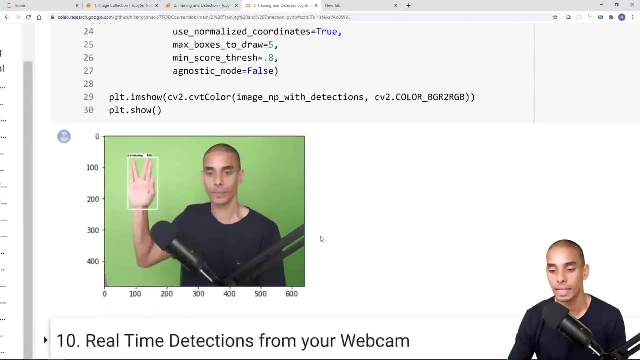 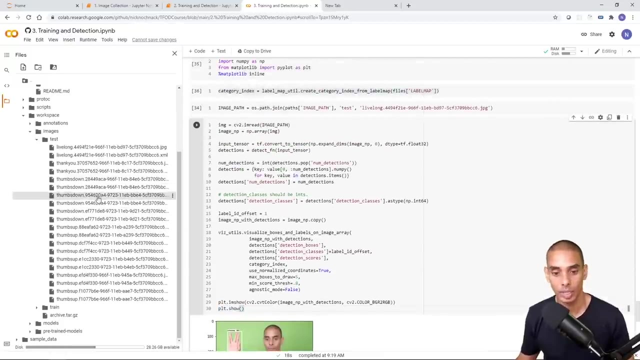 That way We've got over there. Perfect, And you can see it has in fact detected live long, So you can see that there again, you can make this image a little bit bigger if you wanted to. We could try a different image. 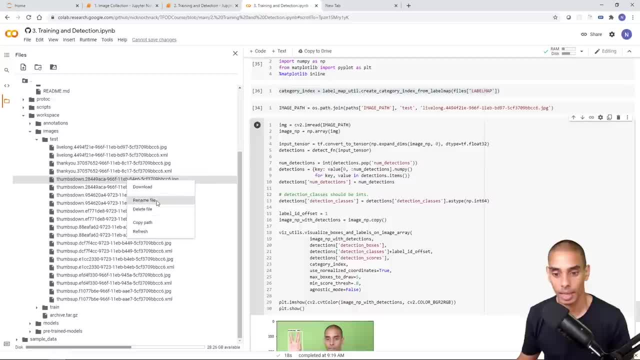 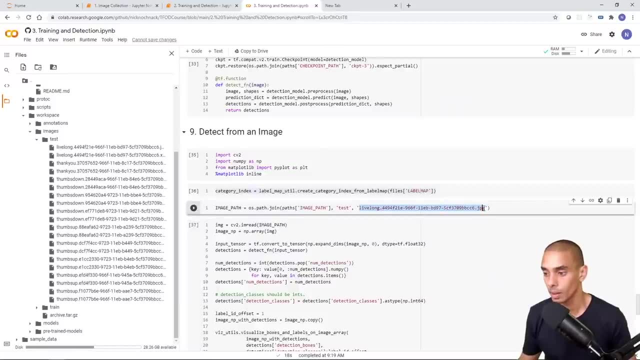 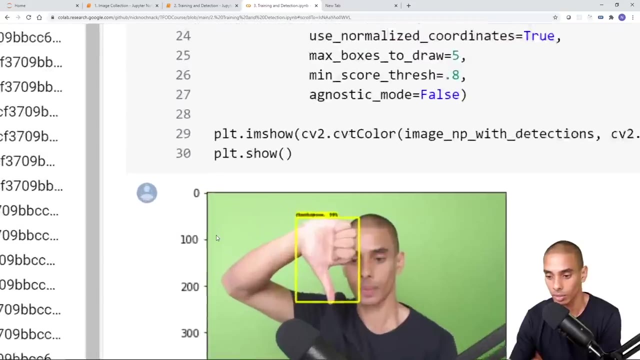 So let's try a thumbs down. So if we copy that file name and we pasted that over here again, we can make another detection- And this should be thumbs down- which in fact it has detected by the looks of it. So you could see it's a little bit sketchy there or a little bit small, but you can see that it has in fact detected our object. 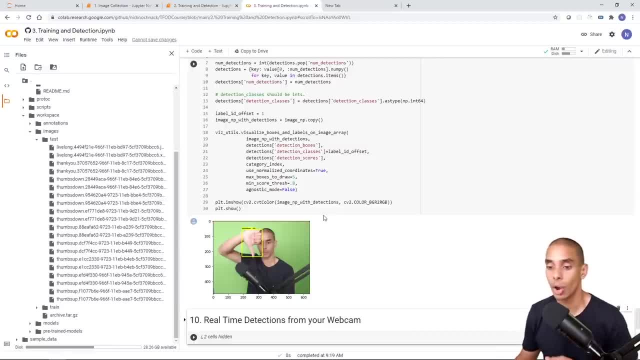 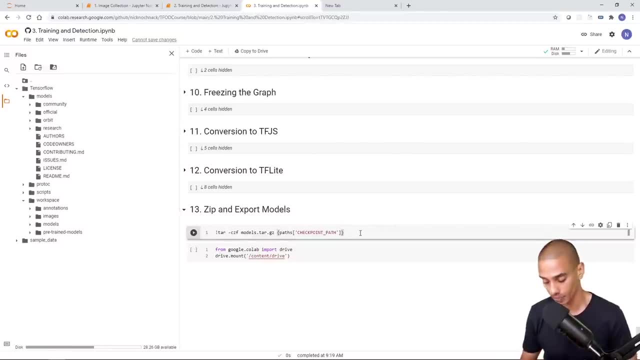 So that gives you an idea of how to train on Colab. Now again, if you wanted to convert or export all of this, I've actually got the code to export it down here. So what we can do is run this cell and it will zip up and export your files. 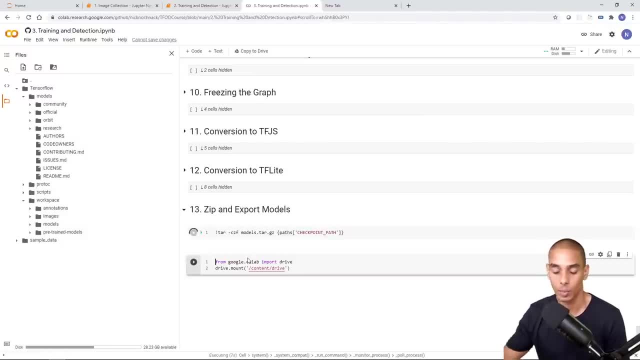 And if you wanted to, you could load that into Google drive as well And export it, bring it back down locally and run it locally if you wanted to. but keep in mind, if you want to run it locally you do need to install the object detection API to have that available locally. 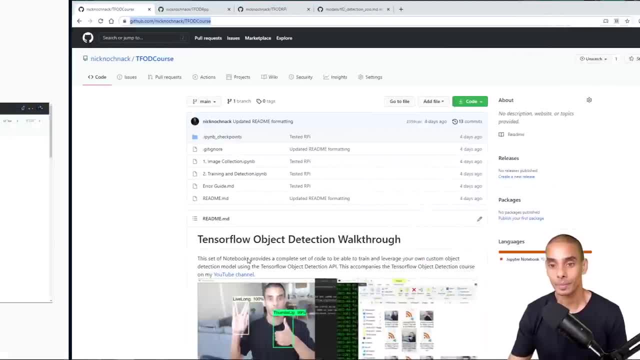 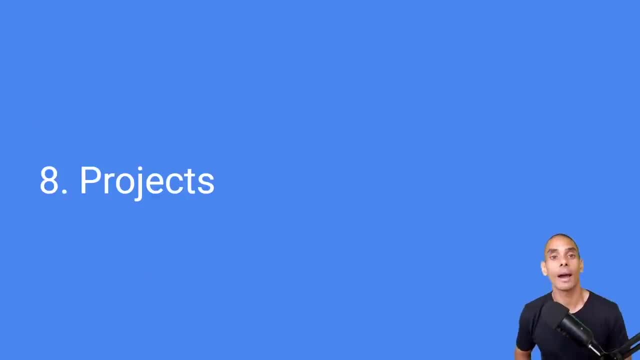 So that about wraps up the training on Colab and really wraps up our part seven of this course. The next part that we're going to be going through are our projects. Now there's specifically three projects that we're going to go through reasonably quickly. 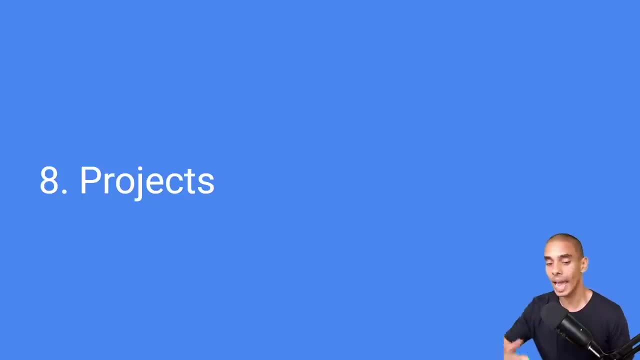 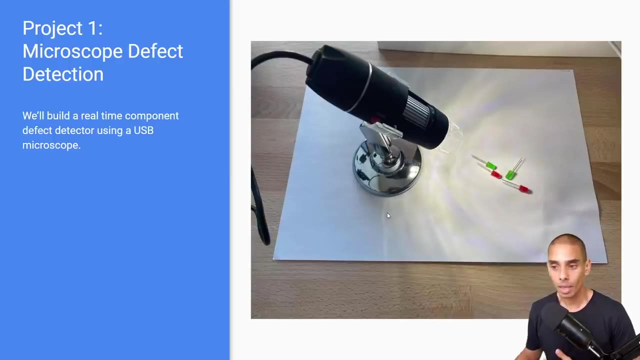 So this just sort of gives you an idea As to where you can potentially take This object detection technology further. I might give you some ideas as to where you can apply it in your real life. So the first project that we're going to take a look at is how we can use different types of sensors. 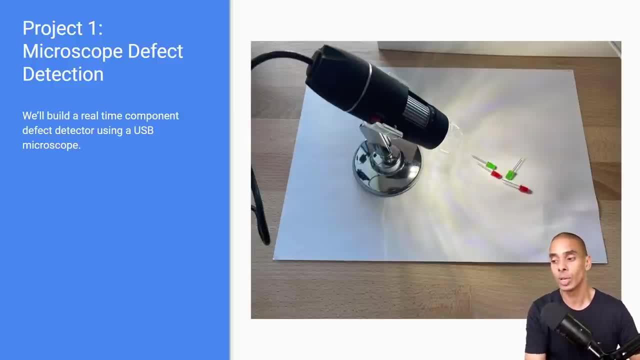 So specifically a microscope to be able to use or perform object detection. So we'll give that a try. Um, I have noticed that it does get very, very close to the object. So we'll wait and see and take a look at performance there. 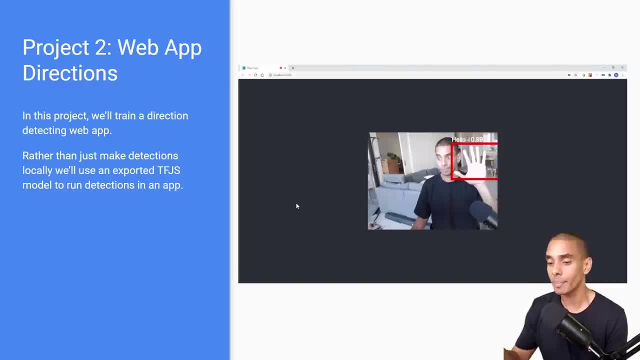 Then we'll take a look at building a web app. So, again, we're able to leverage the existing code base. We're able to, We're just able to repurpose it to be able to build up a tense flow JS app, and I'll show you where to get the code for that. 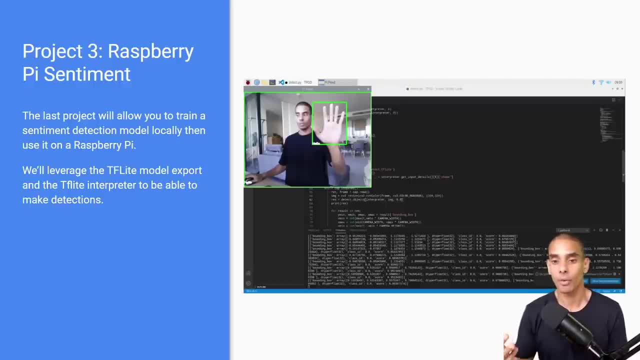 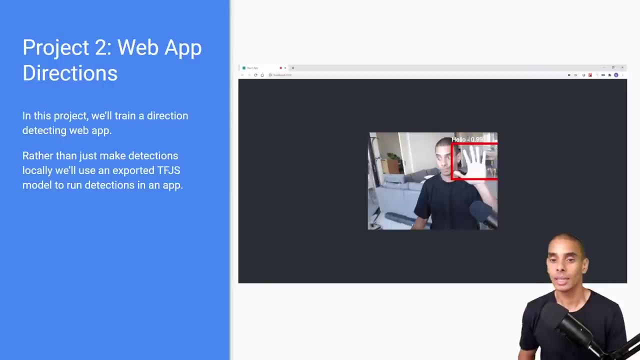 And then, last but not least, we'll export our model and be able to perform, uh, some raspberry PI sentiment. So we'll just be trying to detect one class there. So, whether or not I'm happy or not, So in this case we're going to be going through each of these three projects, but starting off with microscope defect detection, then web app directions and then, last but not least, our raspberry PI sentiment. 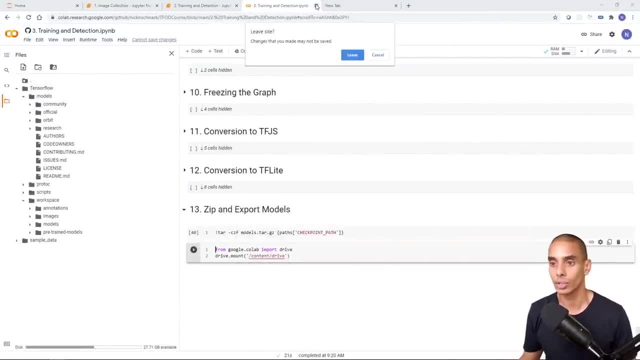 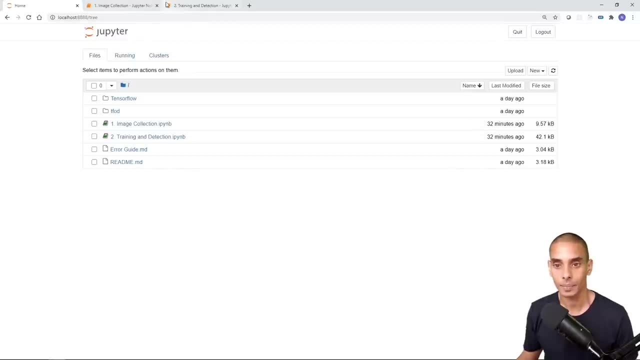 Okay, So we're going to jump Back into our notebooks. We can close Colab for now and close that, And again let's just restart our notebook. So we're going to shut these down and again all things start. So say, for example, we're starting off with our microscope defect detection. 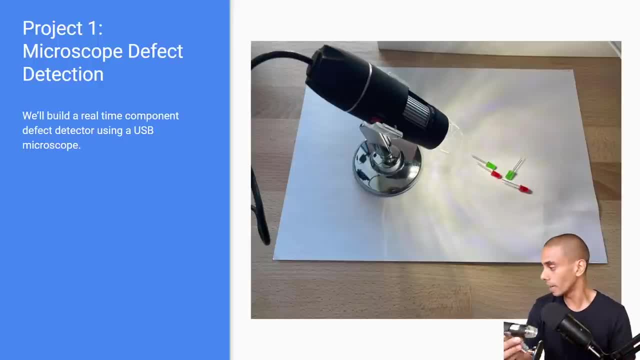 Now, this particular microscope that I'm actually working with is a USB microscope, So you can see it there, right, Um? and I'll link to this in the description below if you want to test this out or take a look at it yourself. 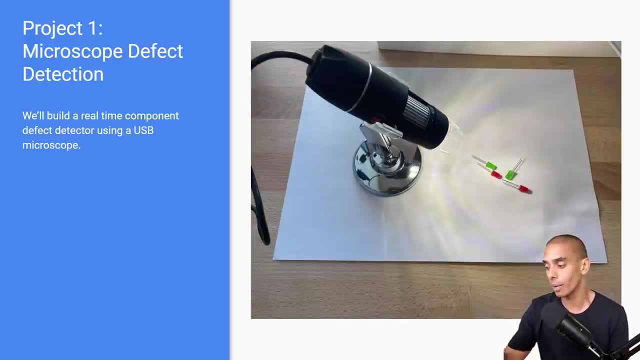 So think of this as just another camera. So right now We're- I'm using a webcam to be able to perform object detection, but we could just as easily use a different sensor. Say, for example, you had a um, a better or high resolution webcam, or a slightly different webcam. 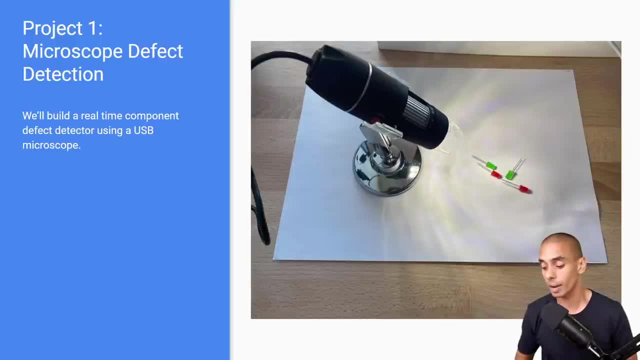 You could definitely use that as well. Now we're specifically going to be trying to train a model to detect defects in these little LEDs here. They're really really small, So it might be a little bit difficult for you to see, but, um, so you can see that this is a green led and it's got a bent pin. 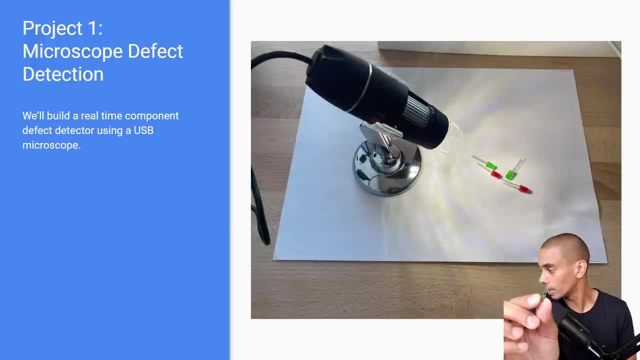 This one is still A green led, but this one doesn't have a bent pin. got a red one as well, And again, you could do this on other stuff. So if you had like a printed circuit board, you could try that out as well. 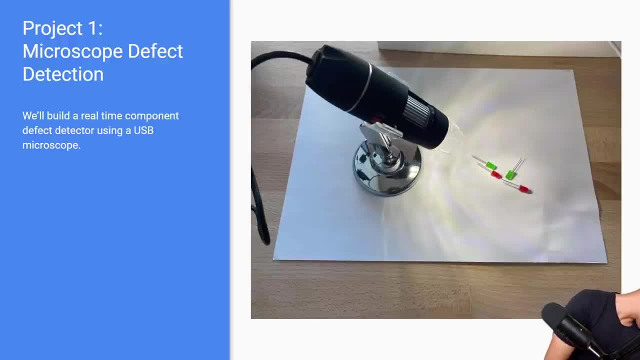 So let's, I'm going to plug in this USB microscope and take a look at what this looks like, So you need to get it into focus a little bit. So we're going to write some code to be able to see the output of this webcam first, before we commit to actually collect the images. 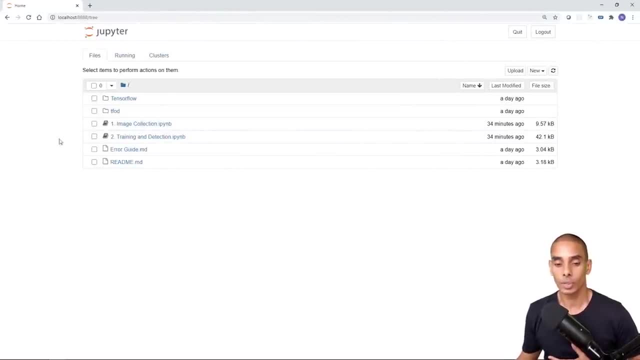 So what we're going to do now is, again, we're going to close down Our notebooks and we're sort of going to start from scratch. So we're still going to be working within our environment that we've already created because we've gone to so much effort to set this up. 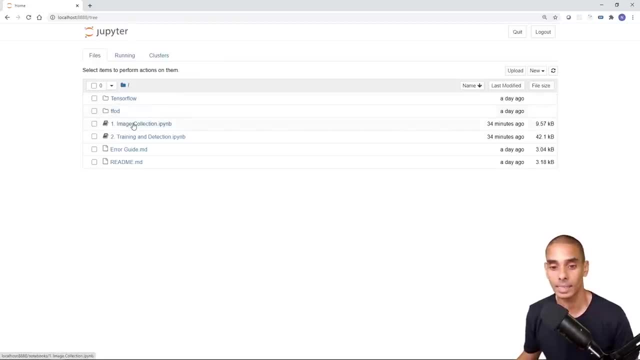 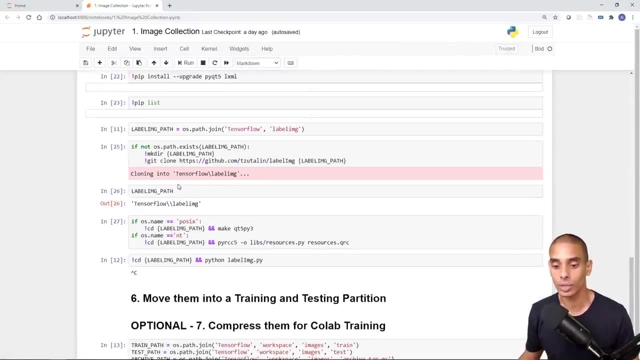 We've got our virtual environment, We've got all of our dependencies in sword. Well, first I'm going to start out by opening up our image collection notebook and we're just going to create a new section Just before capture images, and we'll call this- uh, I don't know- four dot X. 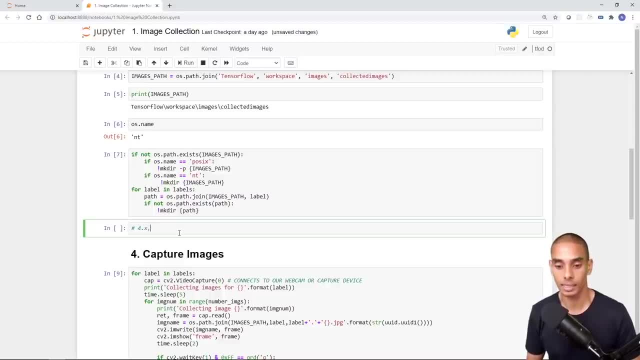 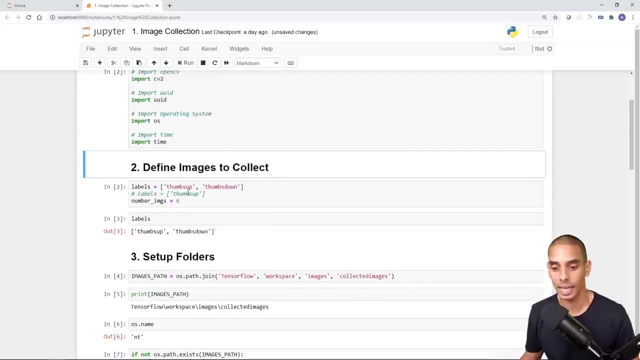 So I'm just going to create a new markdown section and I'm going to say: this is Uh, testing microscope position, Ning cool. And then we'll convert this to a markdown cell and then we're going to import open CV as our dependency and sort of just leave it at that for now. 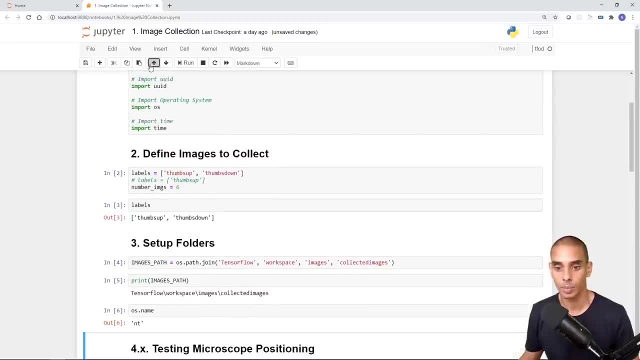 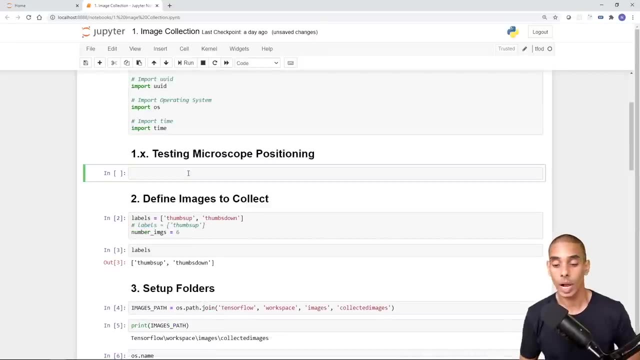 So what we'll do? actually we should probably put this up. Let's put it up here, So we'll make it a one dot X. So what we're going to try to do is we're going to try to read from our USB microscope. 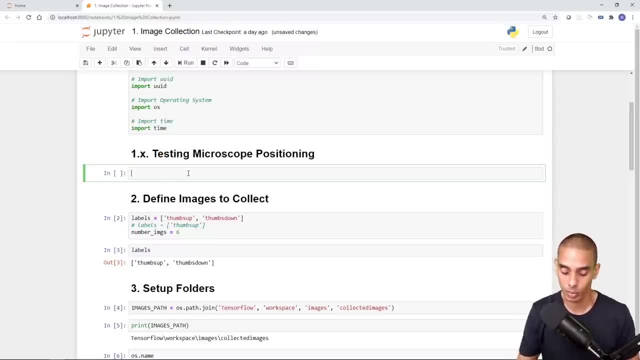 To be able to at least get a feed and then we'll position it, try to get some zooms appropriately and then see what this looks like. I've never tested this before, So I wanted to see whether or not it's possible, what our results look like and what it looks like to do object detection with different types of sensors. 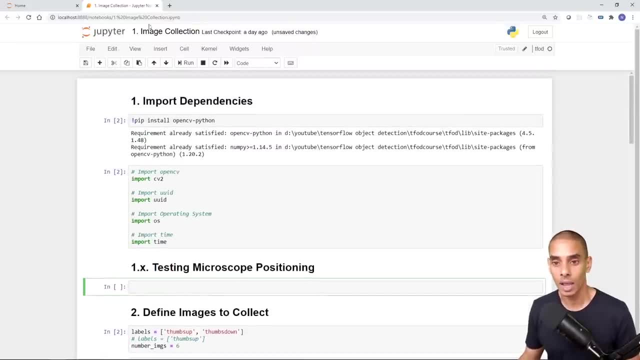 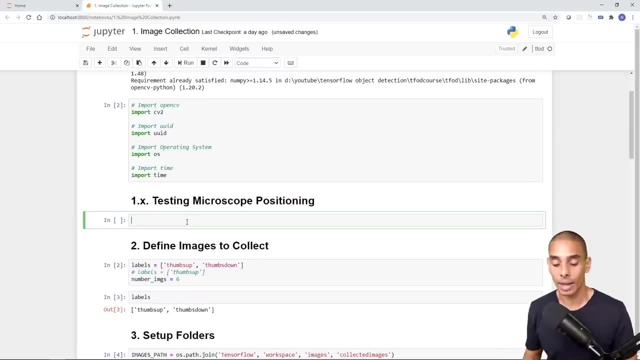 Okay, So the first thing that we're going to do is we've imported our dependencies from an image collection notebook. Now we're going to try to read in a feed from this particular microscope. So in order to do that, we first up need to get a feed. 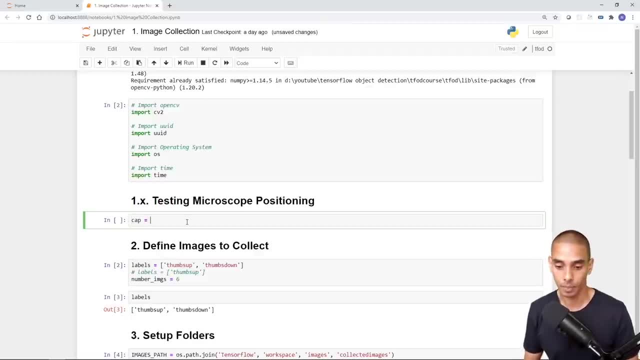 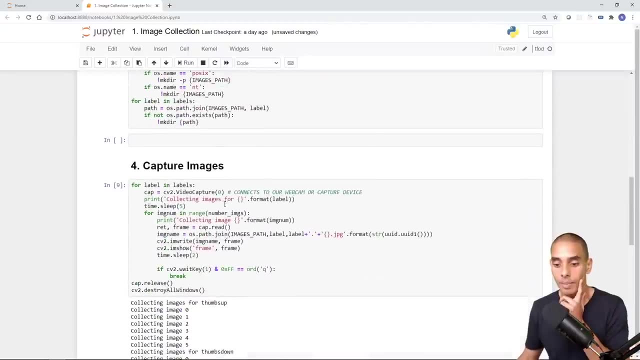 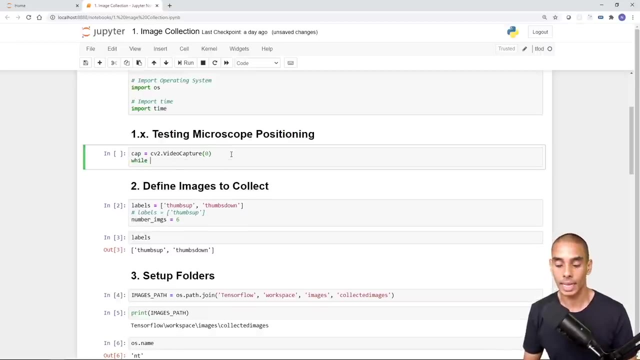 So we're going to call or create a new variable called cap equals CV- two dot video capture and we're going to try out sensor zero first. So remember, this is no different to this line down here. So we're just grabbing a video capture from our capture device and we're going to include a while loop. 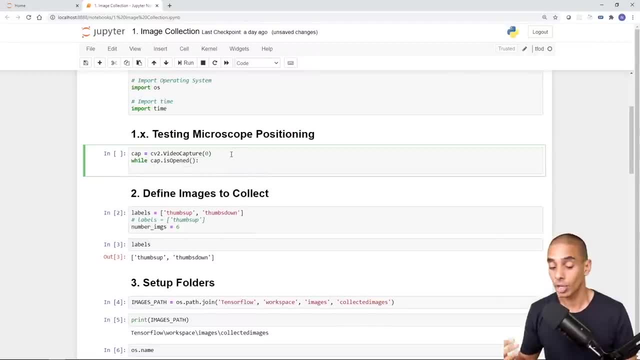 So while cap is opened- so this is checking that our capture device feed is still available. So when you actually set up this capture right, you can type in cap dot read and this is going to read the feed from your microscope. So what we can then do is 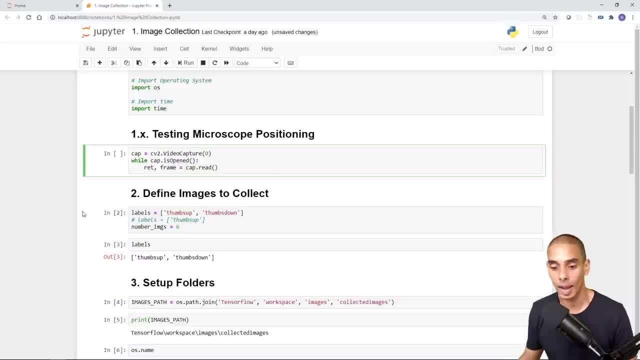 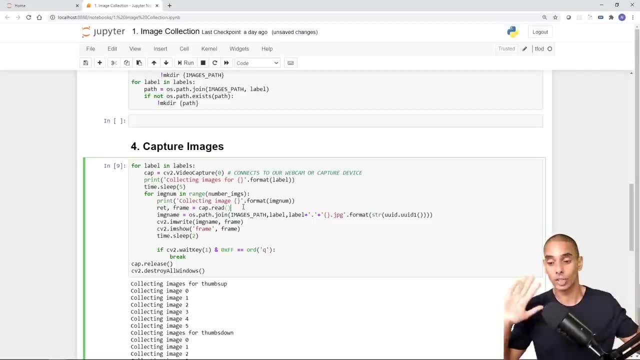 Extract the two variables that we get from that So we can type in ret, comma, frame, which again is no different to what we're doing when we're capturing the images from our webcam, which we did for our different gestures. So in this case we're going to be trying to detect two different classes. 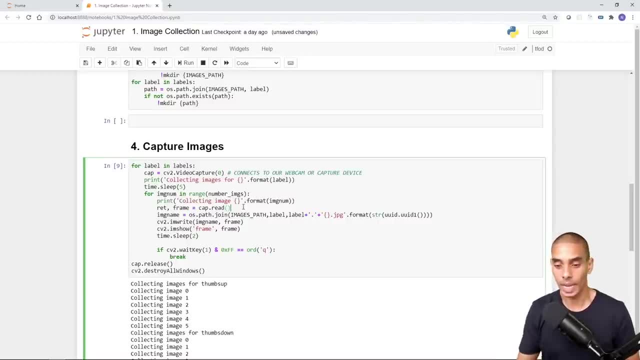 So either a bent pin or not a bent pin, but we ideally want to position our microscope appropriately first, Cause I played around with it yesterday and it is a little bit temperamental in terms of focusing, So let's position it first and get it in the right spot. 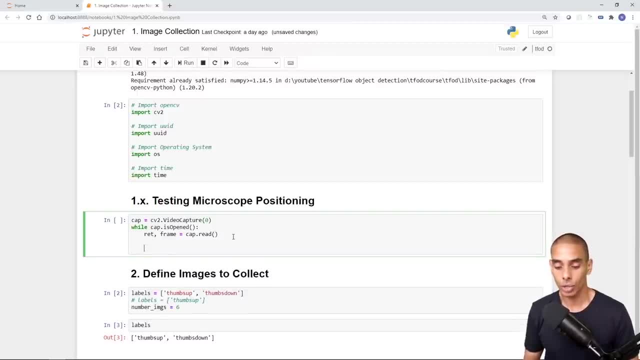 So we're going to write ret, comma, frame, cap, dot, read, and then we need to show our feed. So to do that we can type in a CV: two dot, I am show. and then we named the name of our frame. So we're going to call this microscope feed and then we are going to display our frame. 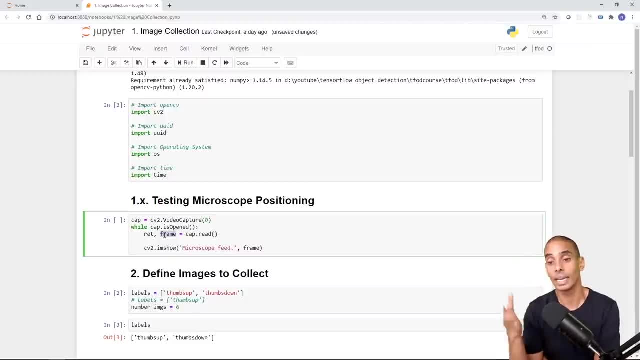 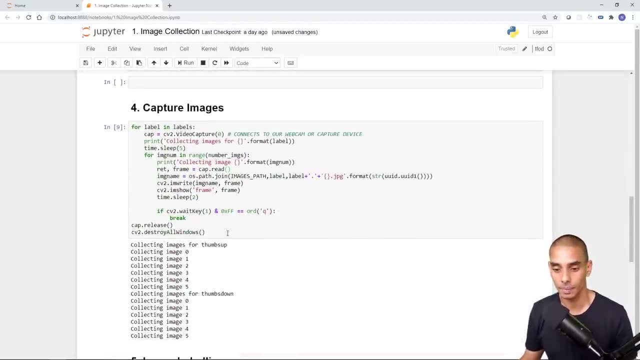 So our frame that we actually get back from here is actually just an image, right? It's an image from our microscope, So that should give us our feed. Then we can copy this little bit over here. So this is um, these four lines of code. 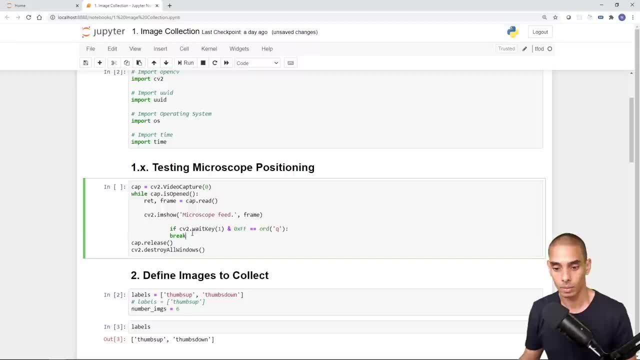 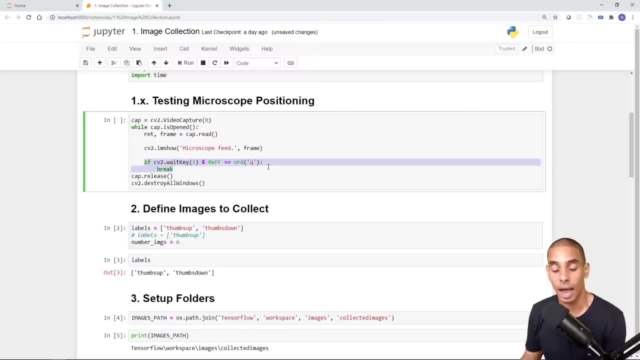 Let me actually explain that in a sec, Right. So these four lines of code, So this basically, is what gives us our ability to sort of quit out of feed and close that little Python window And then cap dot release is just best practice. 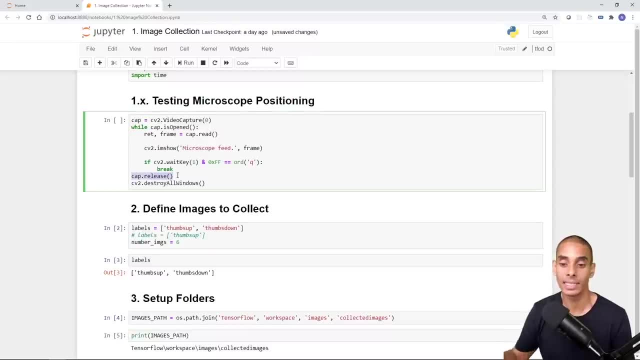 So this allows us to release our capture device and destroy any of our open CV windows. Ideally, you want to run this after you close any CV two Web capture And sometimes you might get your sensor hung up, So say, for example, it won't detect images anymore. 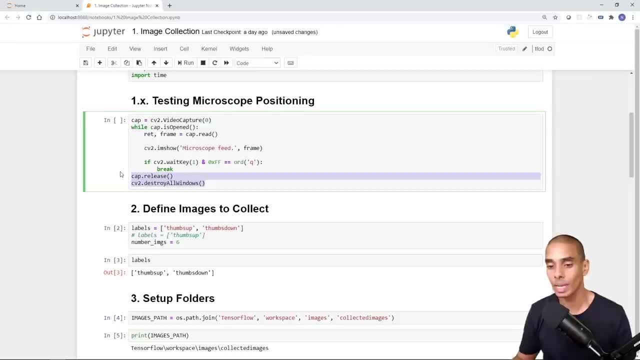 It might sort of freeze up. um, running those two lines normally resolves a bunch of those problems, So let's go on ahead and test this out. So in this case we let's just double check. So we've written, so we're getting our capture. 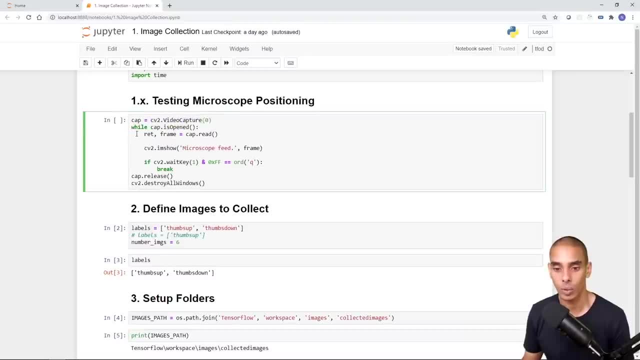 So cap equals CV, two dot video capture and we're testing out device one and we're looping through. So while the capture is opened and grab or read the frame, show back to us and then, And if we try to break out of it, then break out of it. 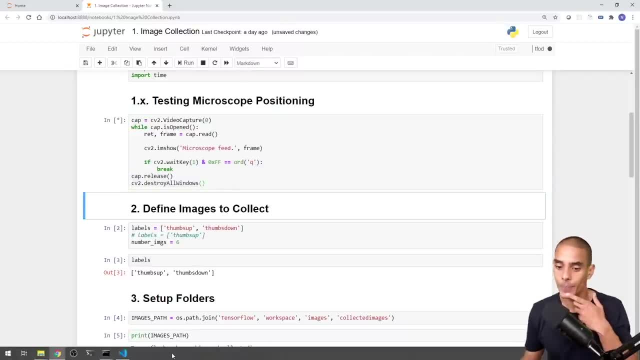 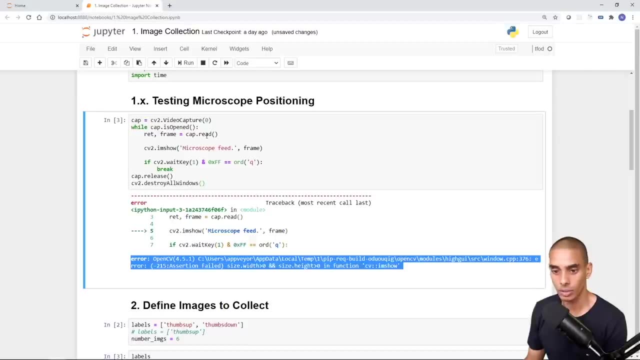 So let's run this and see what happens. Okay, So what are we getting there? So, uh, so CV, two dot I'm show, So let's try another capture device. Okay, That's looking more positive now, All right. 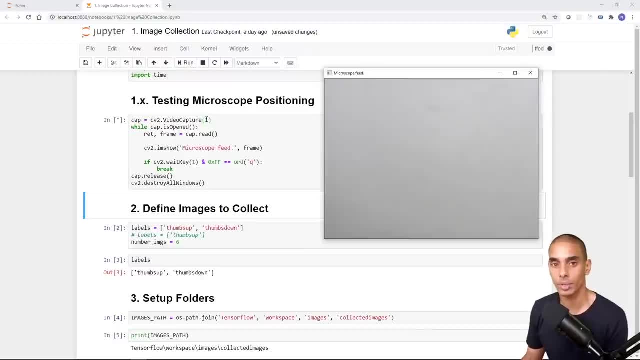 So this looks good. So I had to change the video capture devices. Capture device zero is probably my current webcam that I'm actually streaming on, So we might need to change that now. right now This Looks kind of weird, So we're not actually seeing anything from our microscope feed, but that's because I'm just got it currently. 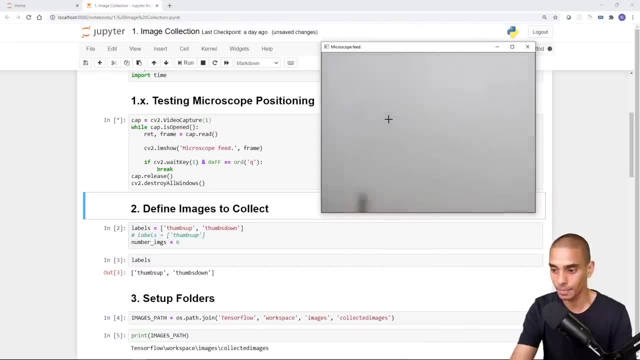 pointed to a piece of paper. So if I move this around right, let's move it there So you can currently see like one of the LEDs. So if we bring that into focus a little bit more, nope the other way. 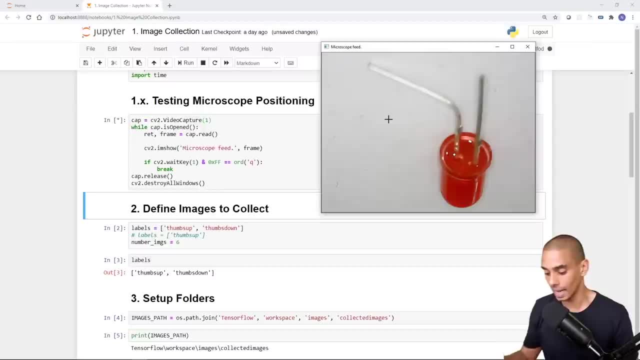 All right, cool. So we've now got one of the LEDs actually appearing So I can move this around and you can currently see That We've got that actually appearing. So we've got a bent pin there, So you can see that it's definitely broken or it's obviously not going to work. 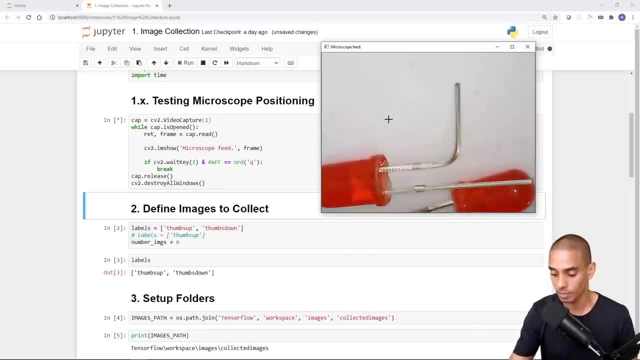 If we try to plug it in, we're going to try putting in a another LED. Then this case, we've got one that actually is working All right. Now you can sort of see that we're sort of going down the same path, right. 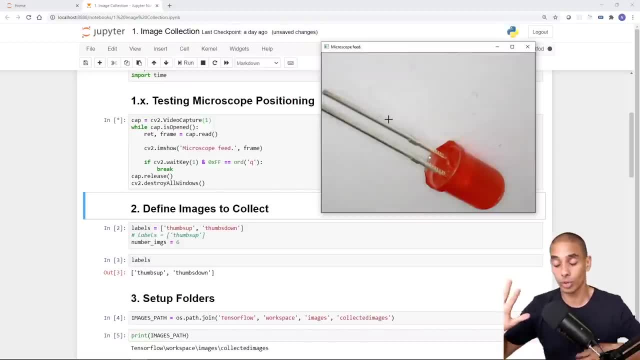 So, rather than having um a particular or doing gesture based detection, this time we're actually just going to be using a slightly different feed, but we're still Grabbing pictures from a camera, So in this case we're sort of good. 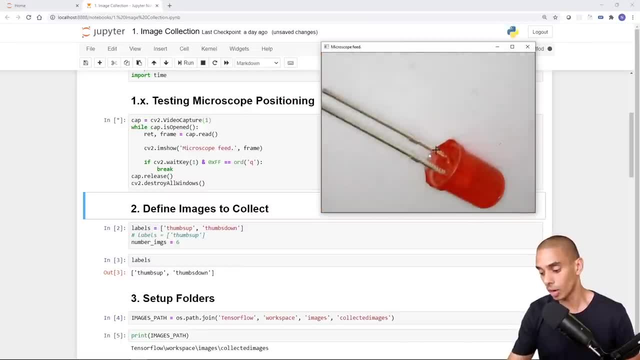 So I've got a got the position based on my sheet of paper, So I'm doing it on a white background to ideally allow us to see this a little bit better. So we actually want to collect some images of our- uh, the different pins and whether or not they're broken or not. 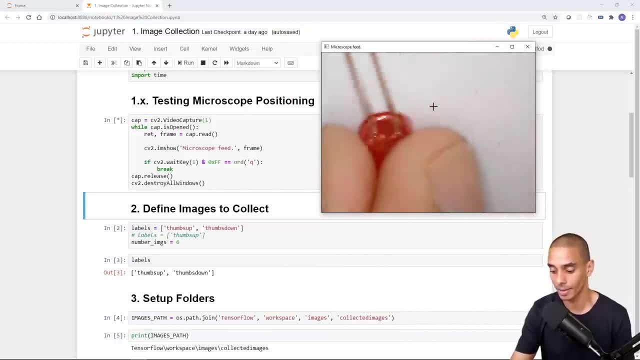 So I'm just going to put it back into position and it's rolling away from me. There we go. Yeah, Let's bring that a little bit closer. There you go. It still wants to roll. Okay, So I'm going to hold it there. 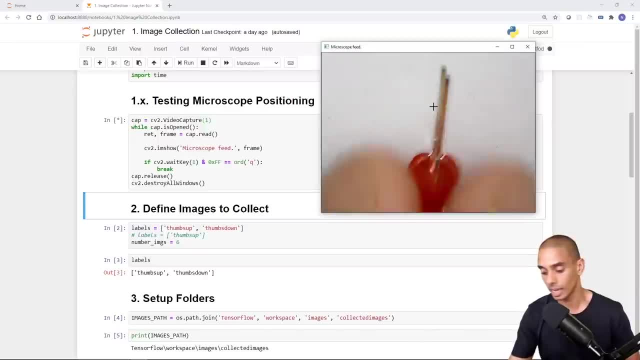 Stay Okay. So what we need to do now is actually collect a bunch of images of our particular um led. So if I bring that back into frame, I should have kept it in position, but so right now this is pins. 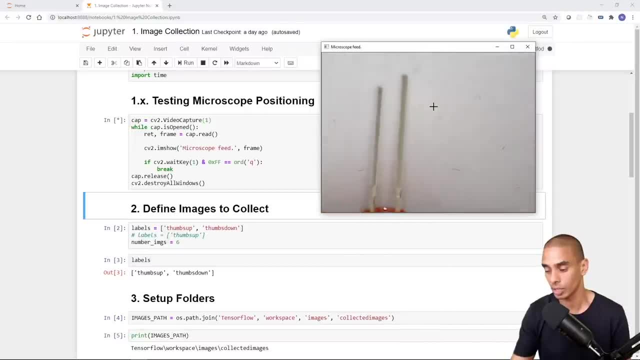 The pins are fine. We need to collect a bunch of images of different styles of pins, So, again, this is probably going to be a little bit finicky. We need to obviously get these right into position in order to get the photos appropriate. 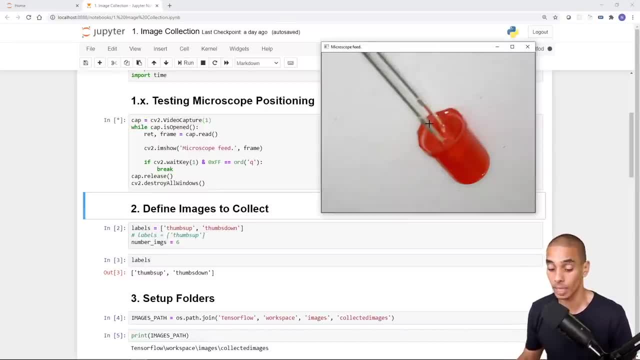 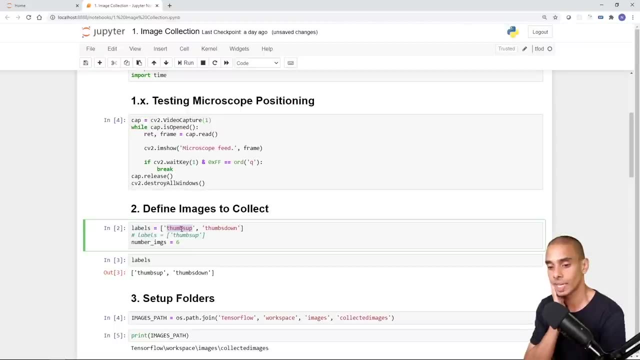 We'll test this out. Okay, So we've got our webcam position appropriate. Oh, Uh, microscope position appropriately, So we can quit out of that using queue And what we probably need to do for this particular project is collect images for two particular classes. 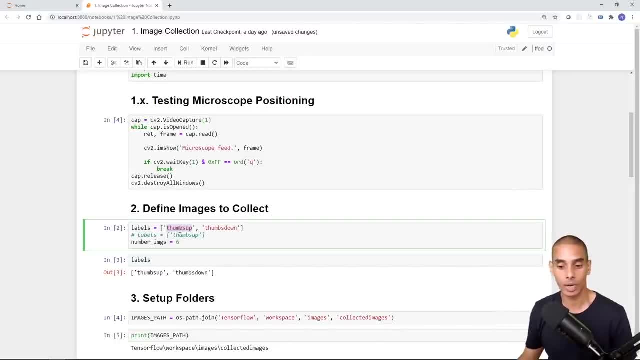 So really a bent pin and a non bent pin. So we're going to create two different image types. So bent pin and I don't know what should we call the other one, Okay, Pin. Actually we'll call it defective and non defective effective. 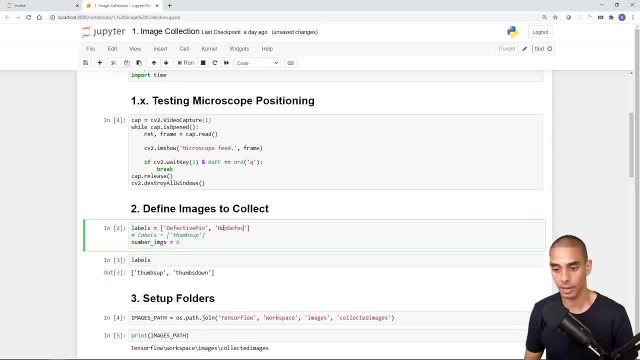 In non. so we're going to only collect two different classes this time. So defective pin and non defective pin, and we'll try with I don't know five images again and we'll give that a crap. So this is going to create two new sets of images. 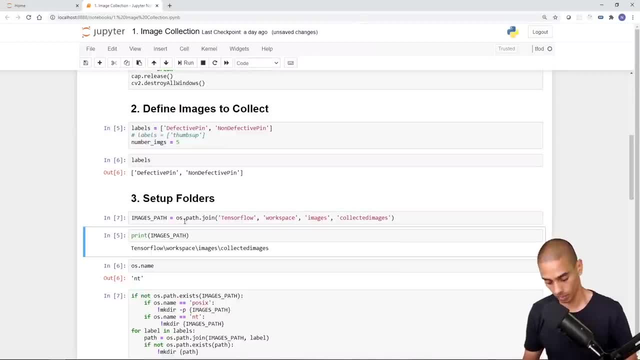 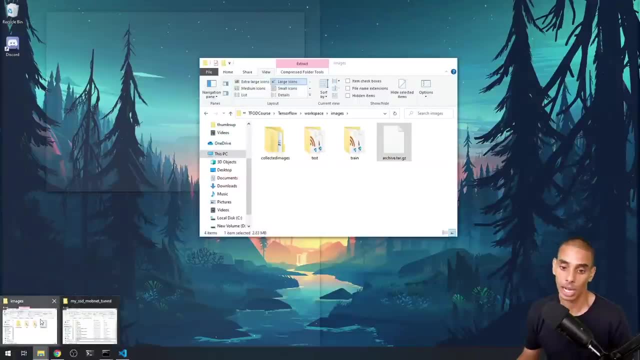 And again when we go through and run our setup folders so we can delete this that's left over. So this is going to create new folders for our new image classes. So if we go into our images, we've now got a folder for defective pin and non defective pin. 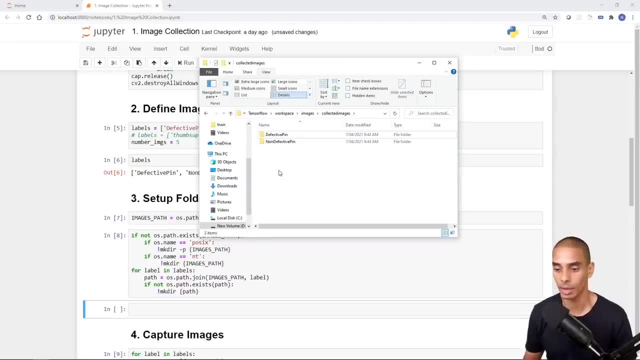 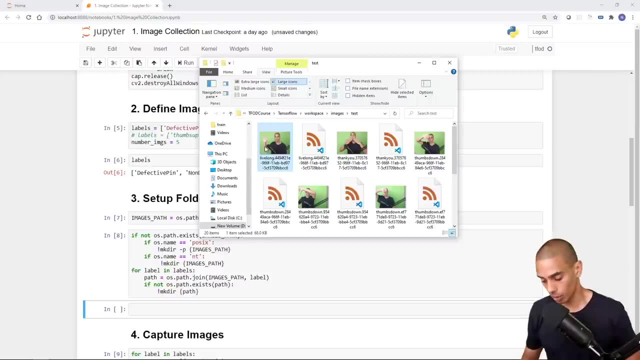 We can actually delete these old ones. So live long, Thank you. Thumbs up, thumbs down. We don't need those anymore, So those are now all cleaned up. Now, what we also probably need to do is clean up what's inside of our test folder. 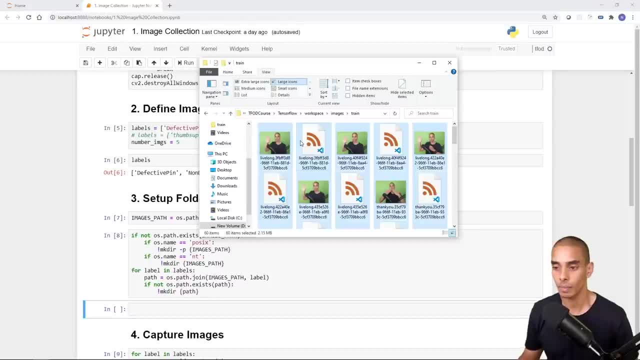 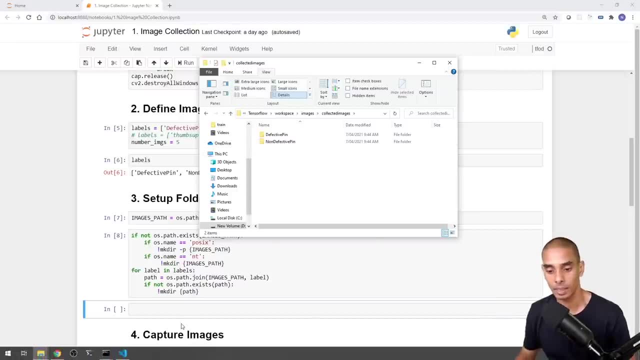 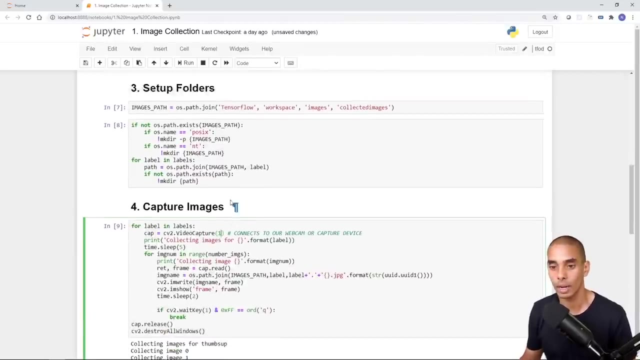 Cause we don't need those anymore. We're doing a new project and we are now going to collect our images for our defective pins and our non defective pins. So we've got the folders created, We can now go to our capture and we're going to test out video capture device one, because that's the device that we had to grab up here to be able to grab the images of our pins. 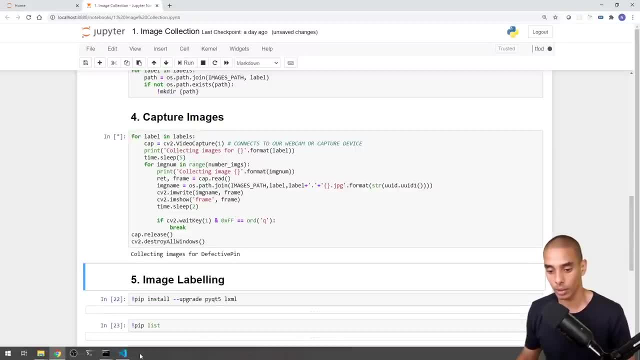 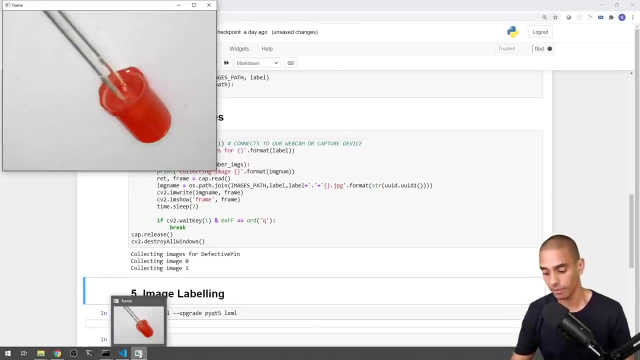 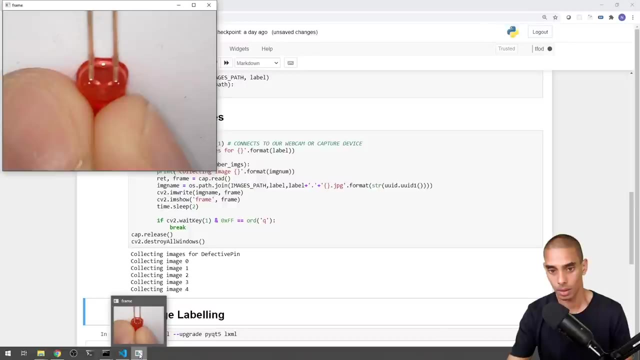 So let's run this and see how we go. Okay, We're getting our frame Back. Okay, so I've got it. We probably need to run this again. So right now I've got a. we had a picture of a non defective pin. 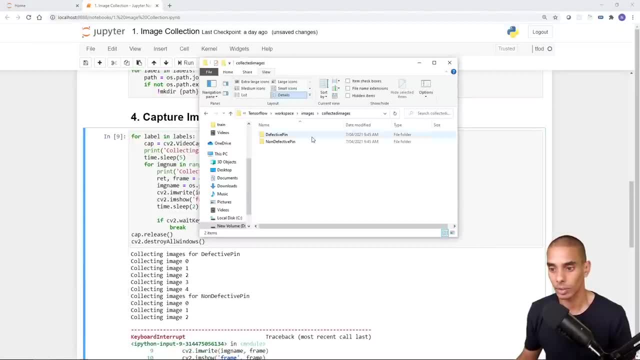 So let's stop this and go back into our collected images. So these are the okay pins, So we want to delete those because those are fine They are. they are effectively non defective. but we had those images in defective, So we're going to put the images of our defect. 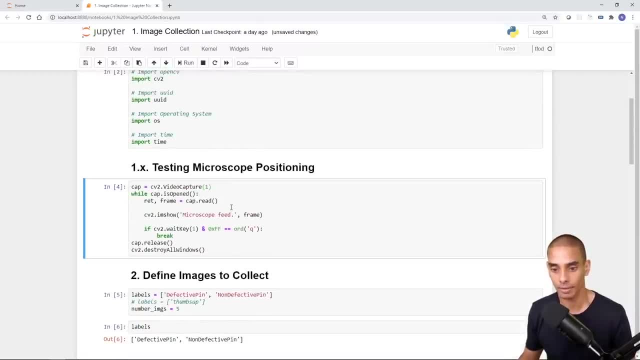 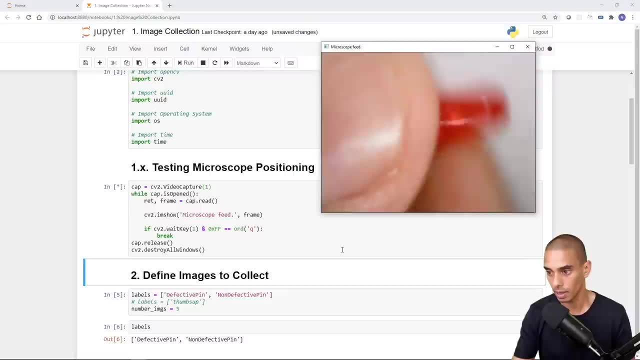 In their first up. let's just double check. We've got the feed right, Okay, So that's looking fine. Actually, position it this way, Right, So that looks okay, Just making sure we can get it in the frame appropriately. 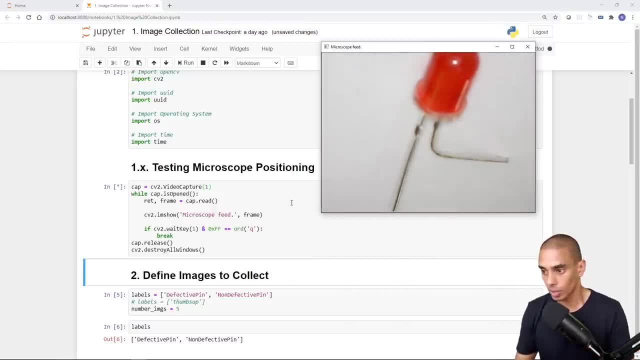 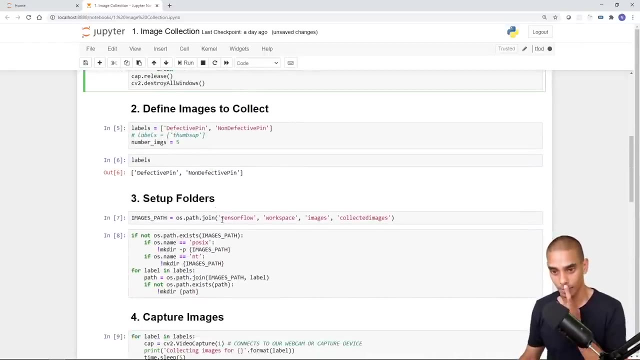 Okay, That's looking good, So let's just try to bring it in a little bit more. that looks good as the tricks, I move the paper, not the actual pin. Okay, Mastery at last. Okay, So what we're going to do now is collect images of that defective pin. 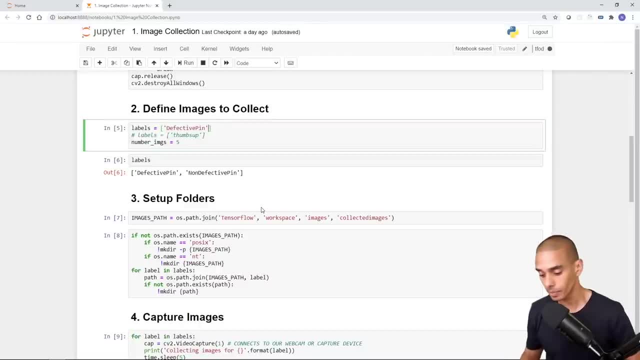 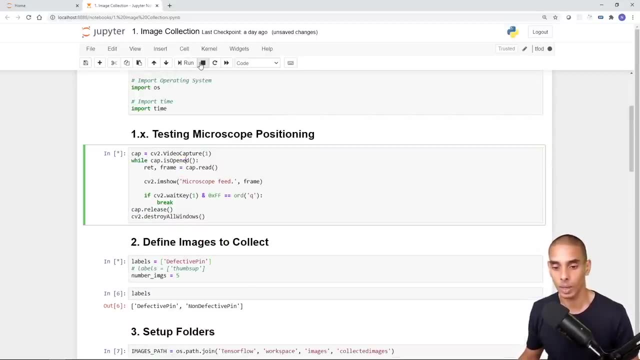 Let's just do one at a time so that we can actually pause, and I'm just going to do it for a red one. We won't bother with the green ones for now. Let's do a defective pin. Oh, we need to stop this cell as well. 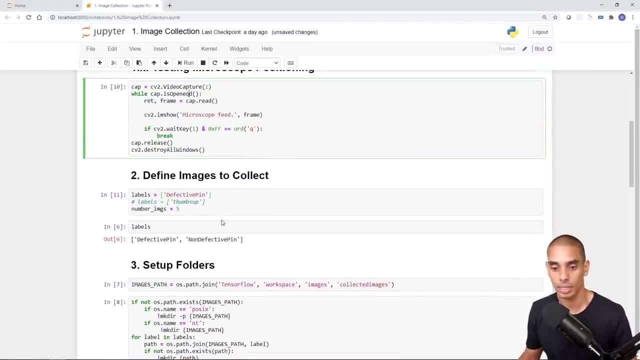 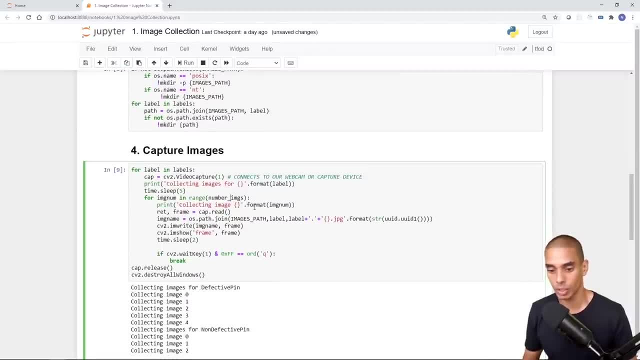 Okay, Okay, Okay. So what we're going to do is collect images of this defective pin and I'm just going to move it around slightly and we can probably increase the time that we want to sleep between frames. So let's give us a little bit more time. 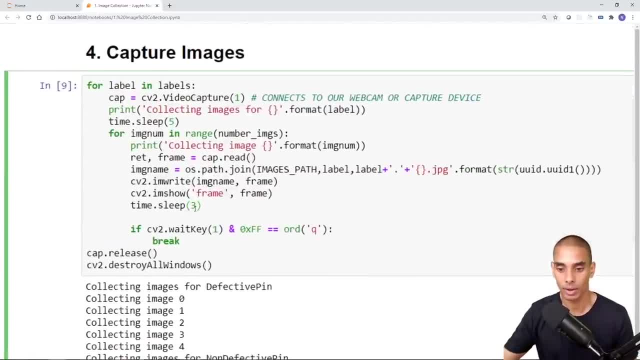 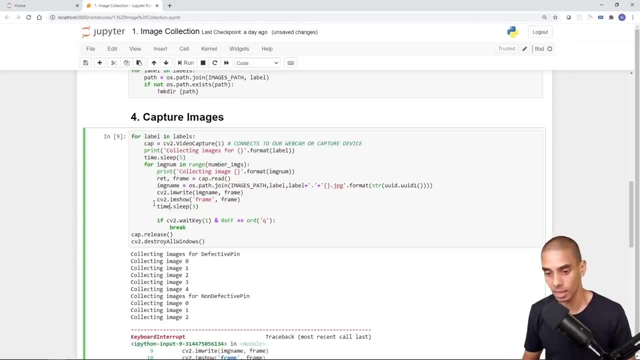 So three seconds. So this line here, which you can see, that reads: time dot, sleep. This is how long we actually sleep between each image capture. So right now it's set to three seconds. So if we run this, let's wait for our frame to pop up. 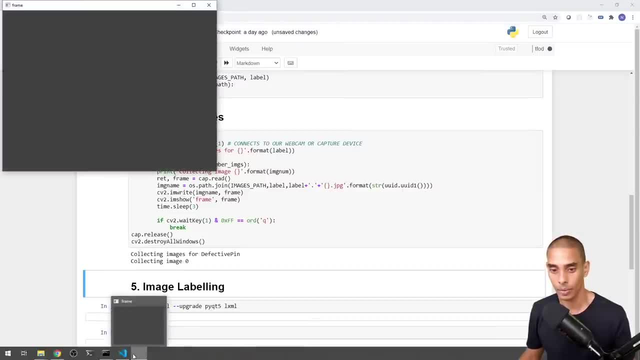 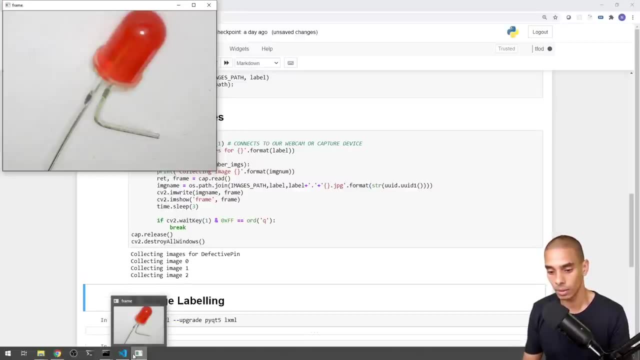 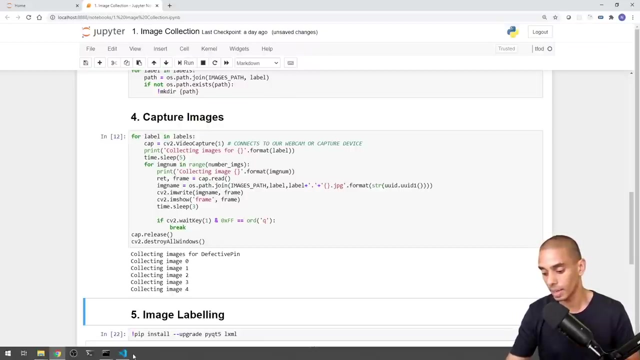 Okay, right now it's position, so ideally we should be getting appropriate images already. cool, all right, so we can move it slightly. okay, so that's done. so we've got our images for our defective pin. let's do our non-defective pin and remember we're not collecting a whole bunch of images here. so this will be interesting to. 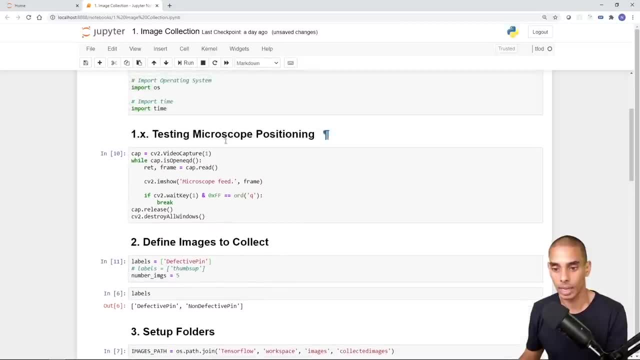 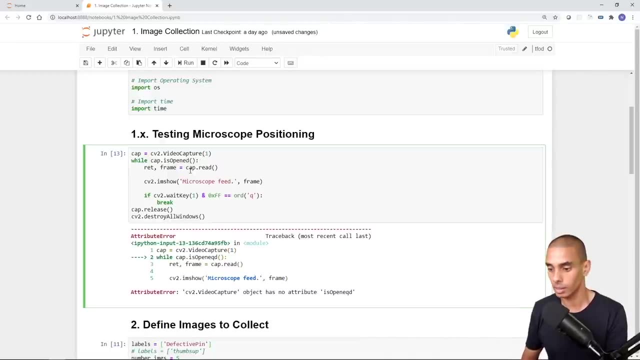 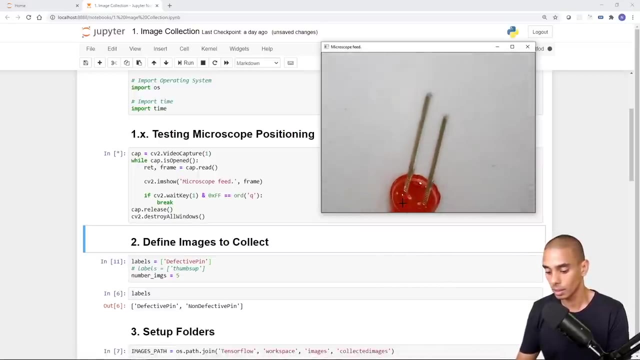 see what performance looks like. let's just position it again. so we'll run this cell up here and we've added a new cell there, so that looks like a typo, so let's just run that again, okay. so we want to position it down, okay. so that's looking okay, all right, so let's try that. 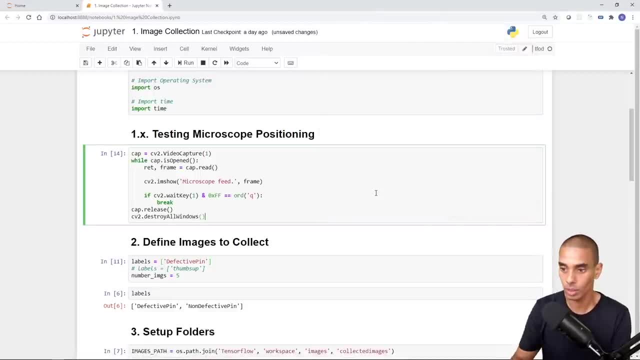 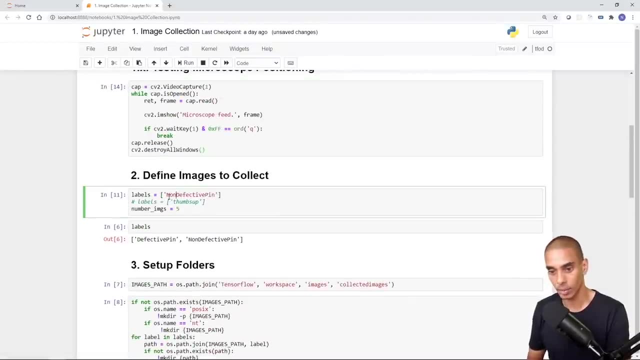 okay, and then we can quit. okay, and then we can quit okay, and then we can quit that by hitting q, just holding the sheet of paper as we're collecting, and what we need to do now is type in: this is going to be a non-defective pin that we're collecting. 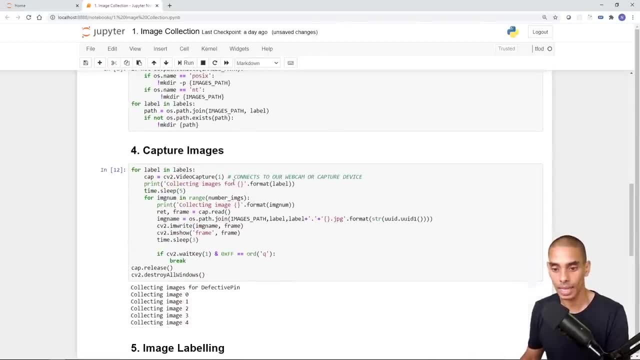 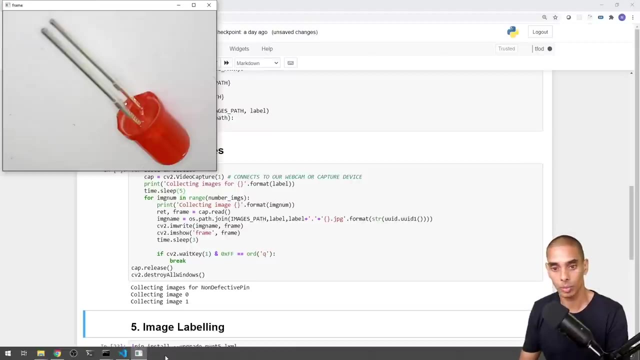 so we can set that label and then we can run this. so this is going to collect images of our non-defective pin or non-defective led, but again, you could do this on a whole bunch of different use cases, right? so i'm doing it on leds and specific components and we're just going to 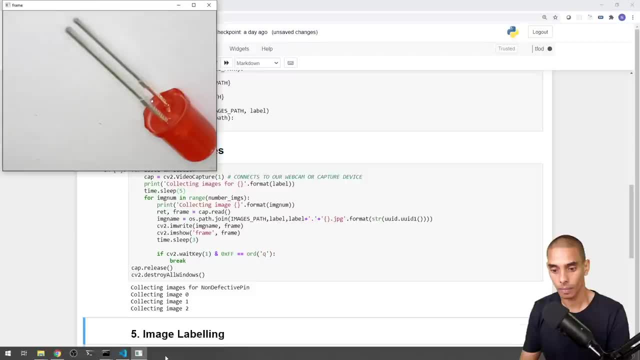 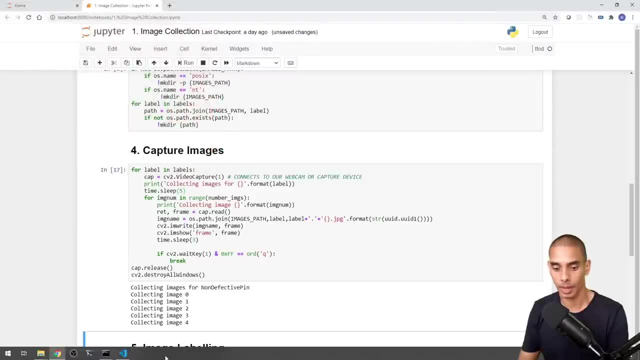 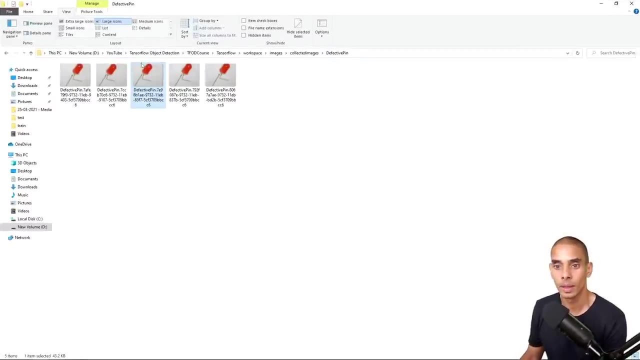 move it slightly each time. okay, so we've got our non-defective pin and we're going to hit q. okay, cool, so let's take a look at our images. all right, so we've got some defective pins here. let's show our preview pane. so we've got defective pins. 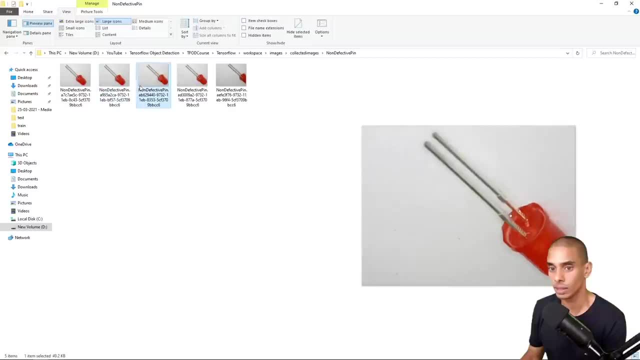 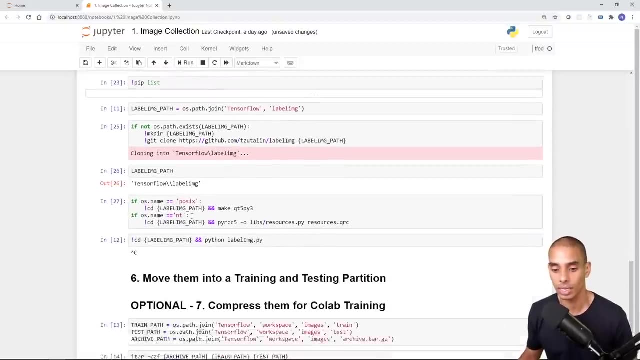 and if we go into our non-defective pins, looks like we've got non-defective pins, cool. so again now, what we're going to do is go through our same process. so we're going to label our images. so we've got all of this installed, we are going to go into our non-defective pins. 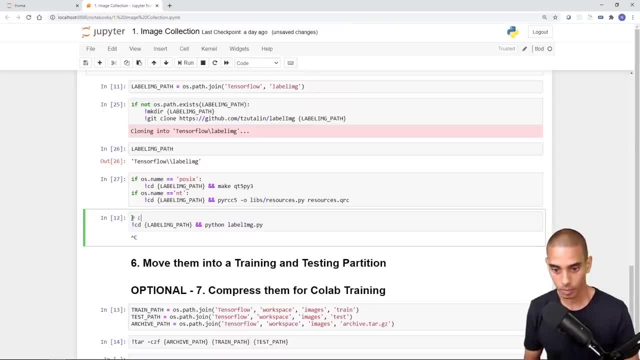 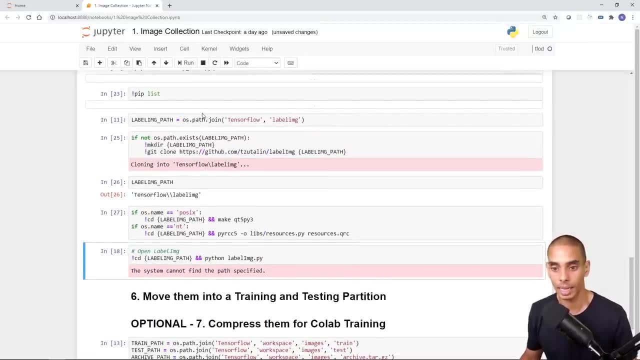 we're going to run our labeling line, which is this one down here. so this will open up label image. so let's run that. and again, we need to set up our label image path, which is this really, we should bring this down here. i mean again, if you've got any feedback for 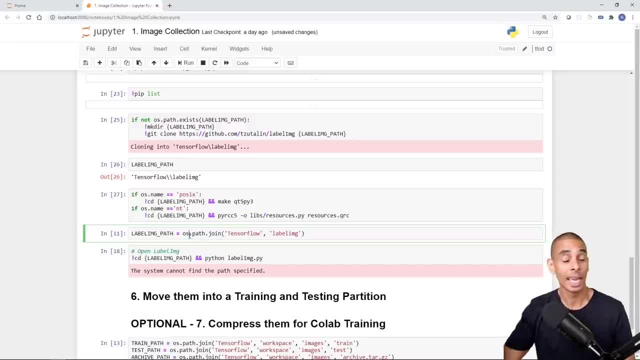 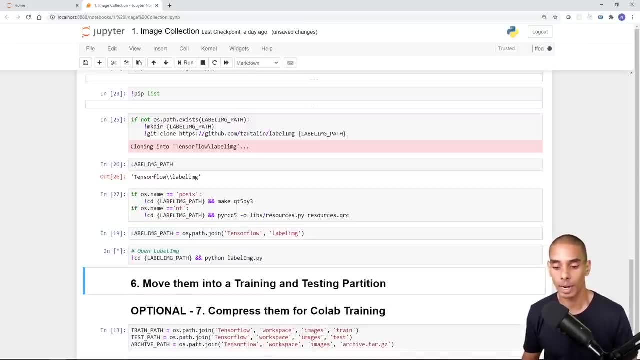 the code or the notebooks, or, if you want any clarification, hit me up in the comments below. join the discord server. more than happy to have a chat, so let's open up. i'll set our label image path. open up label image and get to our image path. so let's run that. and again, we need to set up our 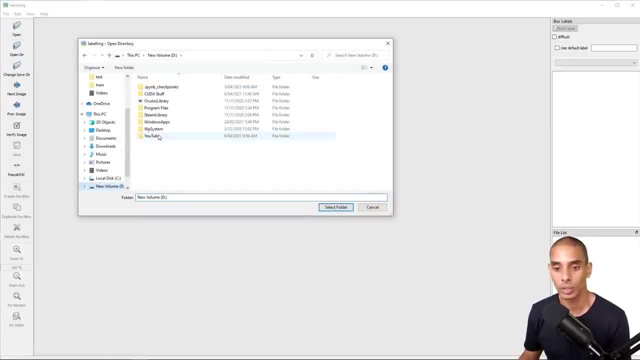 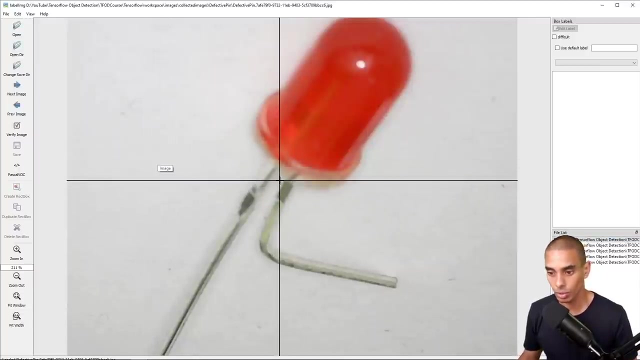 labeling. so we're going to open our directory, we're going to go into where our images are. so in this case it's again in our workspace images folder, collected images and defective pin. so we're going to hit w and we'll just do. let's just do this bit. 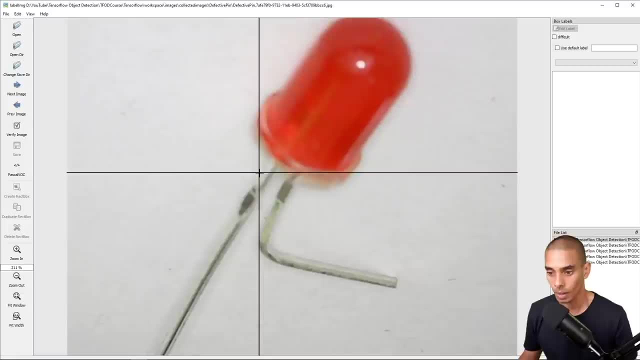 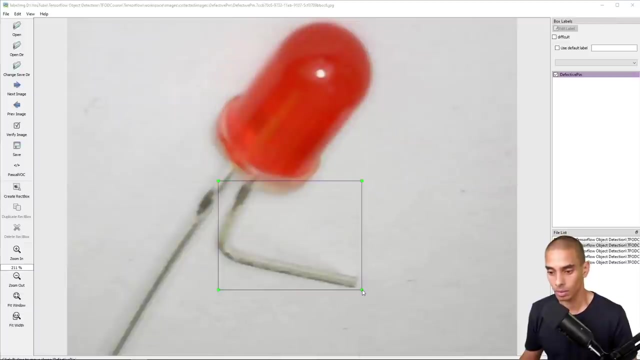 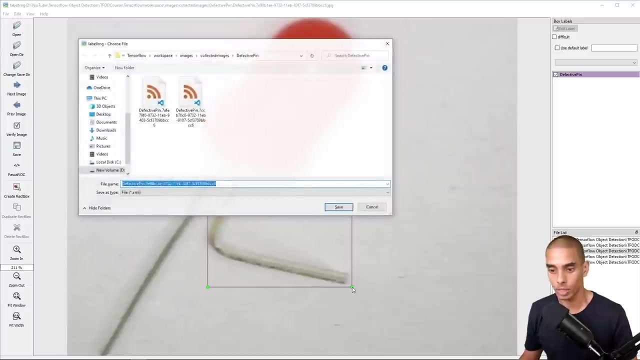 this bit. yeah, let's do that. so we're going to say this is a defective pin, right, and then we're going to save, save again. i'm hitting w and i'm just labeling each one of these. now, if it wasn't so finicky, i probably would have done a bunch of different positions, but the microscope is super sensitive, so 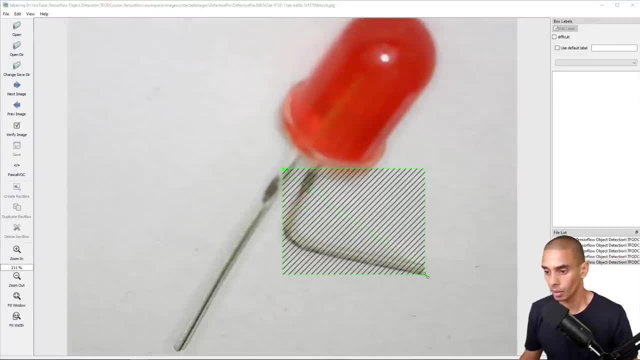 you know we'll wait and see what performance looks like. on this, i'm just going to label it- it's safe, all right, and then we're going to open up our other directory. so again same process, we're just using a different sensor, and this is going to be pretty consistent. 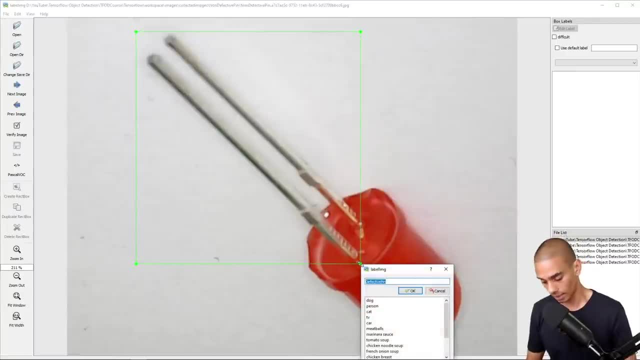 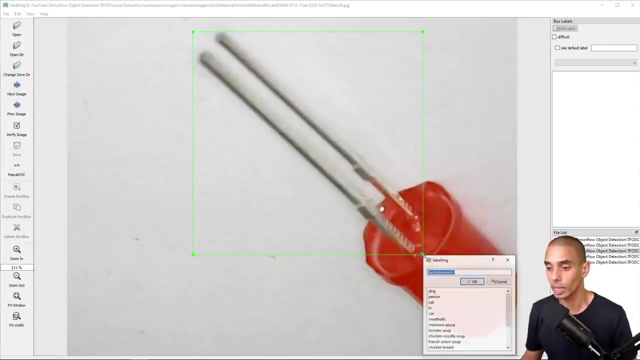 with most of the projects. so, then, we're going to label these non-defective pin save and pay attention to your labels as per usual, because it is important and i've got a feeling our model will won't be generalized as much as possible, because right now, 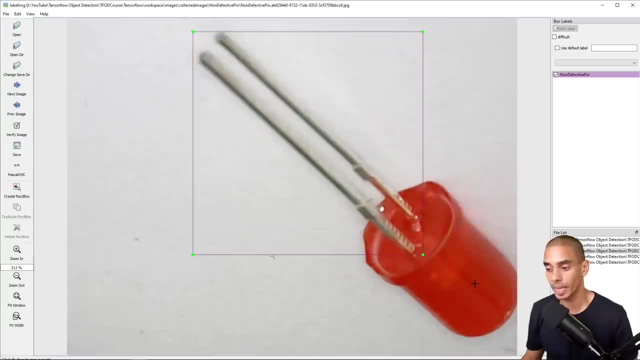 we've only got our pins in one direction, so we'll see what that looks like. but again, you can always go through the performance tuning steps to get this to perform better, and we sort of went through that. so you add in images of different angles at different positions under different lighting. 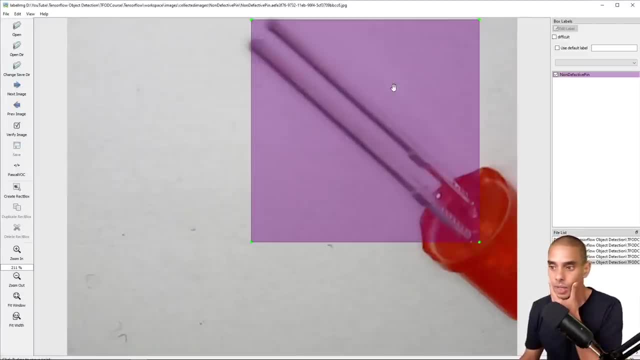 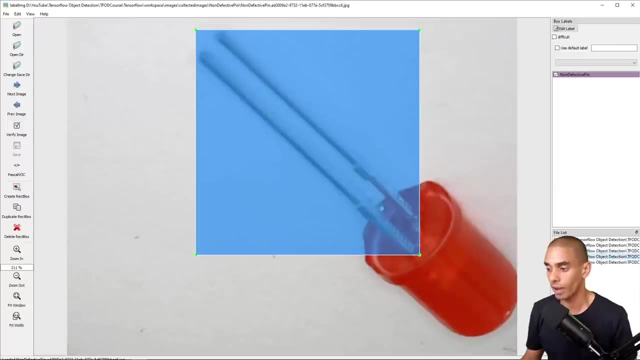 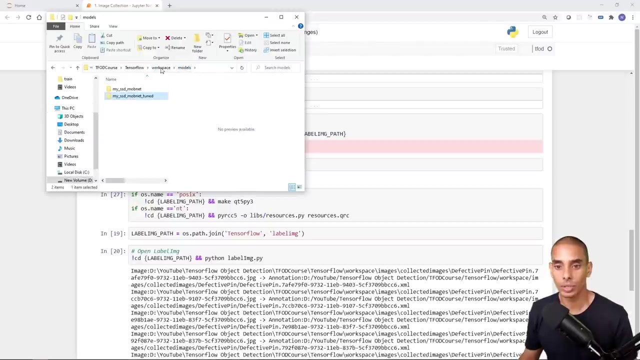 positions. that should help out. okay, so those are our images labeled, so if we go through, so you can see that they're they've all saved and we've got five of each class, so we're good to go there now. as per usual, we're going to copy our images into our training and testing folders, so we're going to. 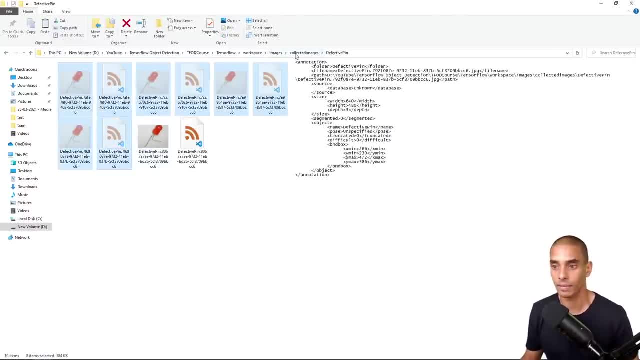 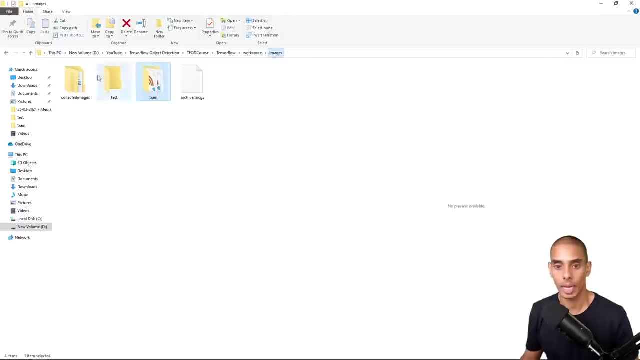 grab the majority. so we'll only leave one for testing for each class and we're going to paste these into our training folder. let's go back into our images: collected images- non-defective pin. we'll leave one and again back into there and then the last. 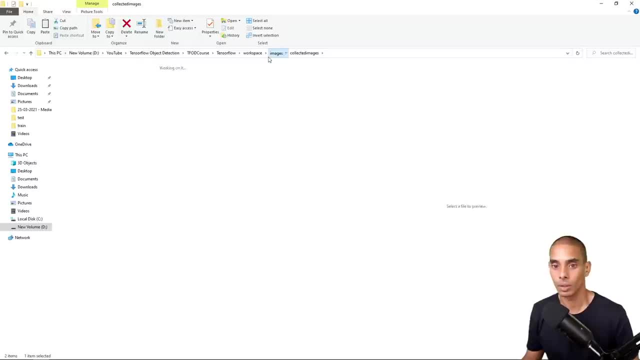 one. we're going to put that into our testing folder. So cool. All right, so we are all set up now. So we've got our training images, or testing images, and our training images. Uh, so we should be able to now go through again our training. 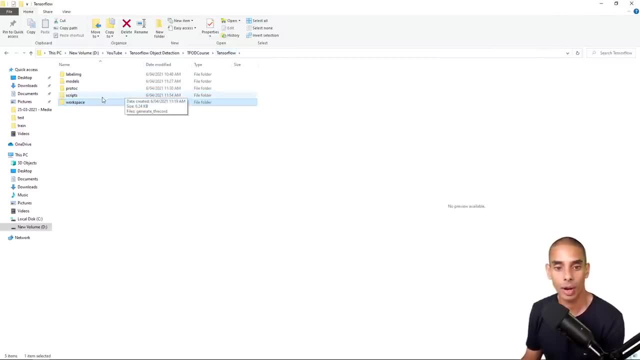 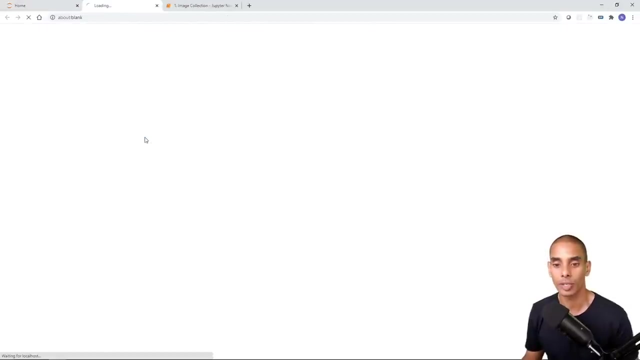 pipeline. What we will do, however, is we're going to probably create a a new folder for our custom object detection model, in this case for our project, So we'll call it uh pin detection or something along those lines, and we will do that by opening up our training and detection Jupyter Notebook and. 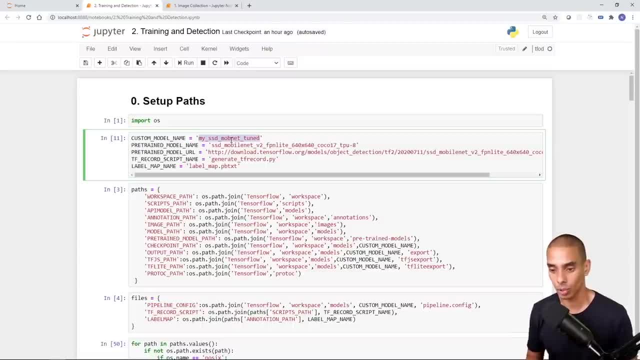 so our last model that we had was my SSD MobNet tuned This case, we're going to call it microscope and we are going to leave everything pretty much the same. We want to revert this back to our, our other model. So this right now is our custom model. We 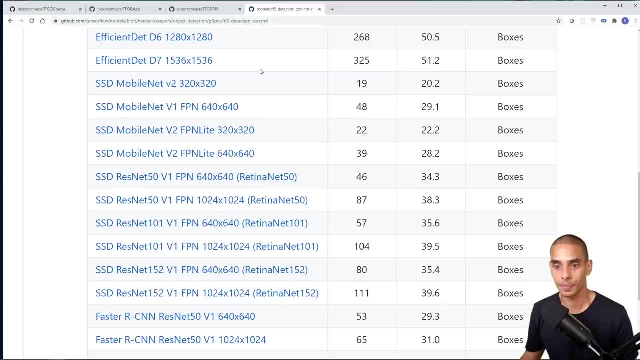 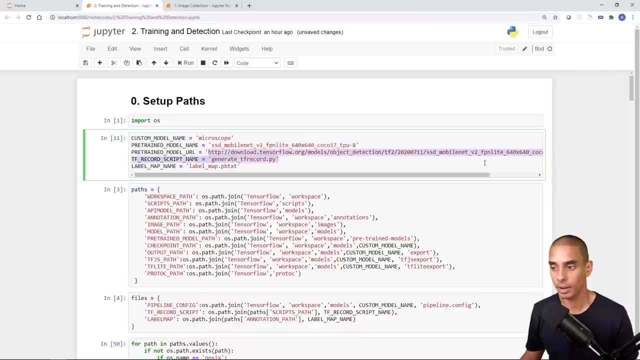 don't want to use that, So let's grab the link to our existing one, which is going to be this one here, Copy link address and I'm going to paste that there. Really, this is sort of just making sure that we're resetting back to usual, So 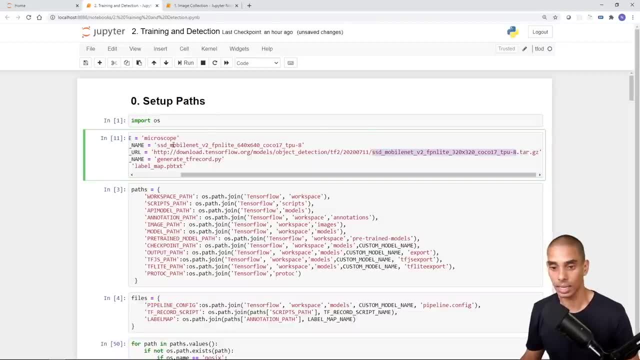 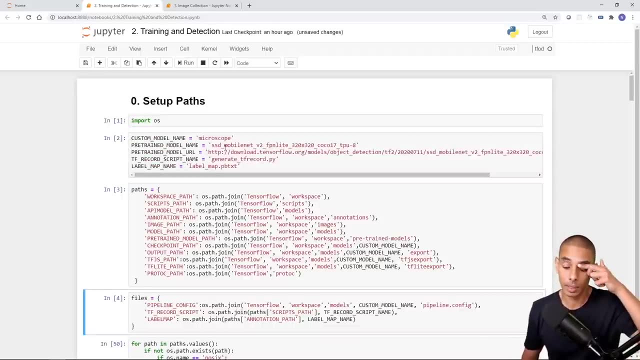 uh, we've already got this model downloaded, so we don't need to download it again. Uh, but we could if we wanted to. Alright, so we're going to import our operating system, set this up, create our file paths and create those actual directories. 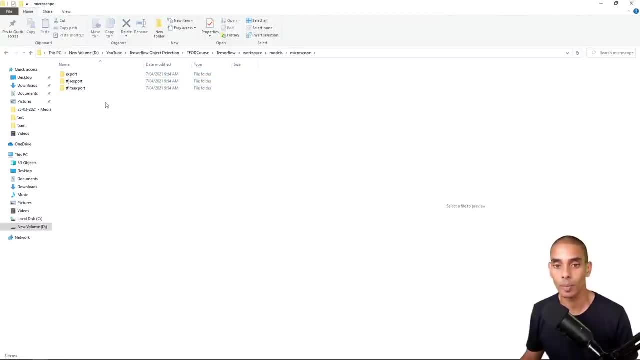 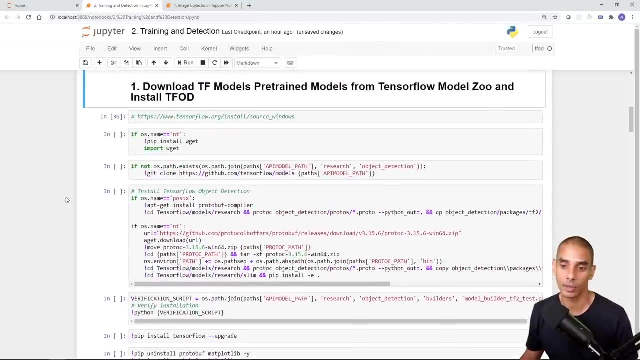 So now if we go in, you can see we've got a folder for our microscope model and then we're going to go through the rest. So again, we can skip step one. we don't need to do that because we've already set up tense flow object detection and we've 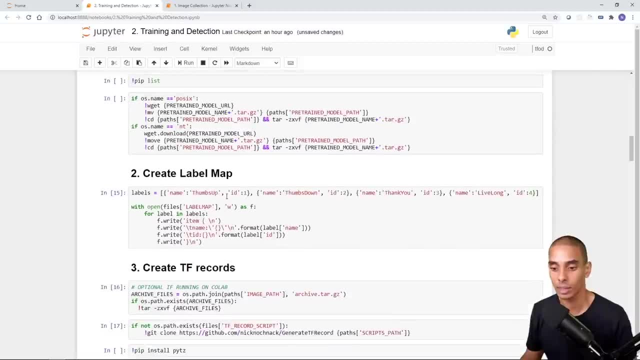 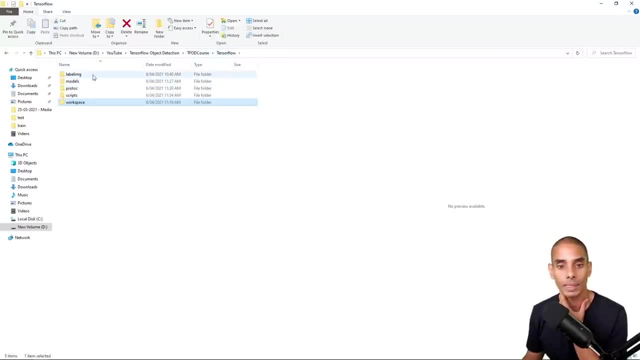 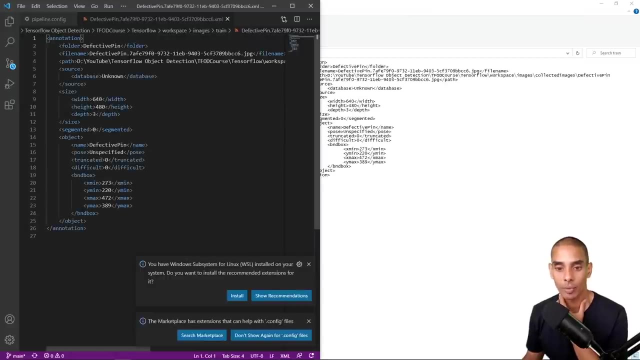 already cloned our pre-trained model, which is what this cell does. What we do need to do, however, is update our label map. So if you cast your minds back when we set up our images, so if we go into Workspace images, train, so we need to make sure we get the appropriate label, so it's going to be defective. 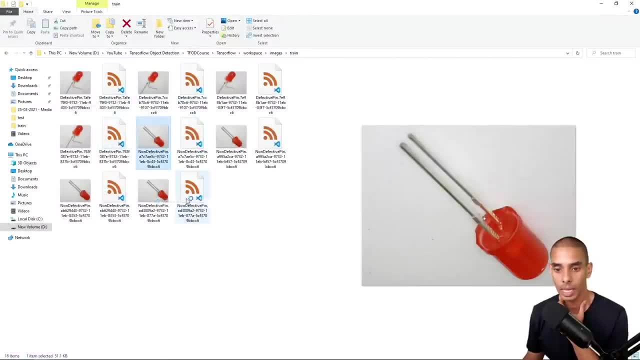 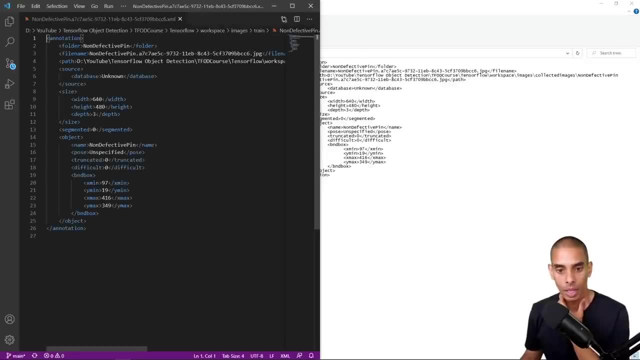 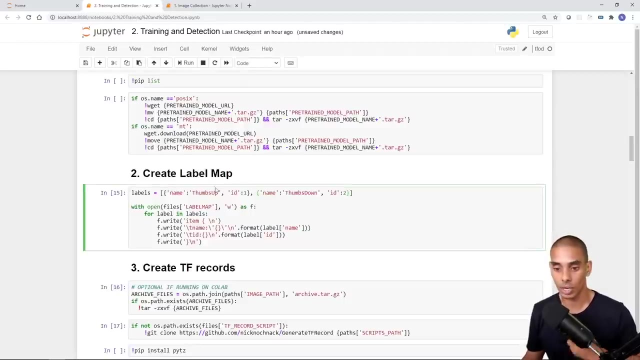 pin and it will be. what was the name of that? sorry, i've got to open up the actual annotation and non-defective pin, so we're going to update these labels here. so again, this, this whole code base, is really really general purpose, so you could do a bunch of stuff with it. so we're just 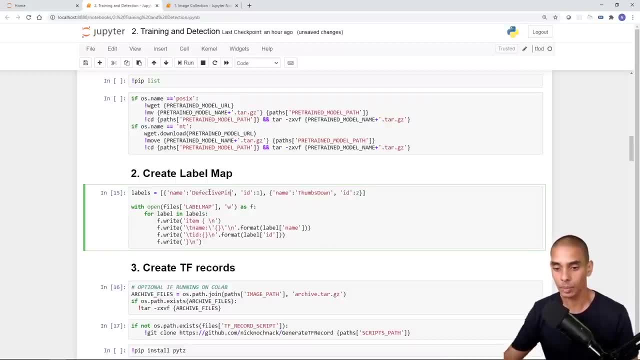 going to rename our labels, so defective pin, and i'm doing this under step two, label map. so this first line here again, we probably talked about it a while ago, but this first line is what sets up our labels. then this is what creates our label map, which is what tense flow object detection api. 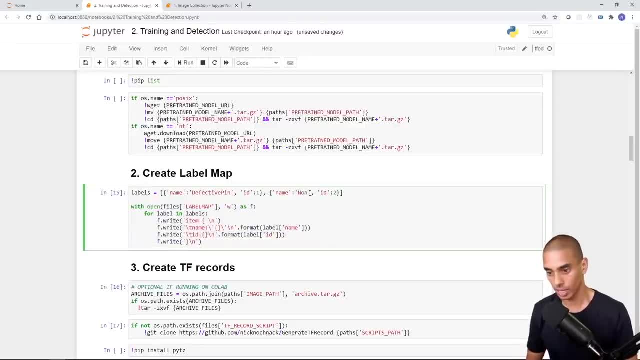 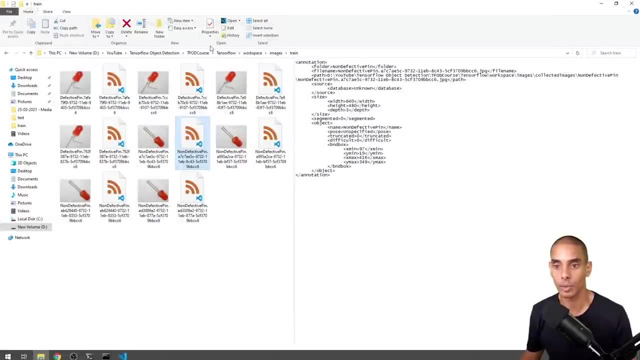 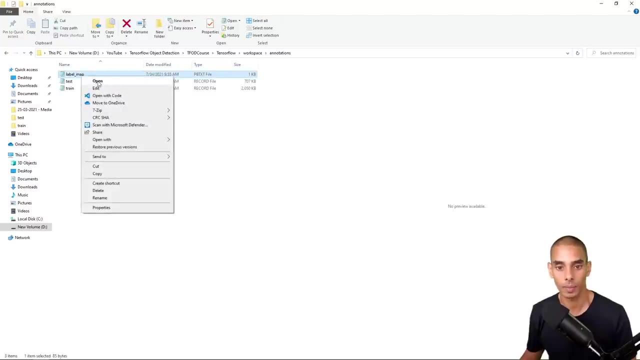 needs to actually to actually train, then we're going to set up our next label, non-defective pin. so we'll do that. and now, if we go and open up that actual label map, which will be inside of tensorflow workspace annotations, let's open this. you can see, we've now got one class for defective pin and one class for non-defective pin, so we're. 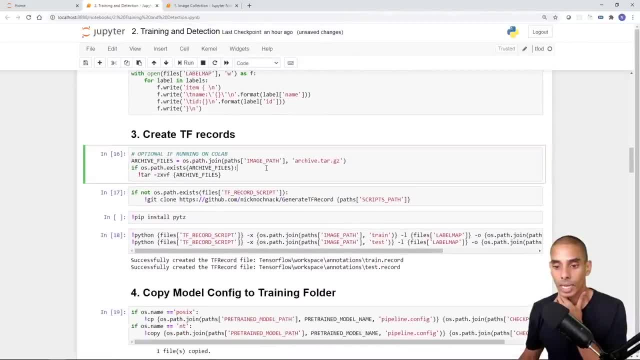 good to go there. now what we want to do is, again, we are going to create our tf records, so we don't need to run this cell here. this is what unarchives our images inside of colab. because we're not running on colab, we're good to go. don't need to run that. this cell actually clones our generate. 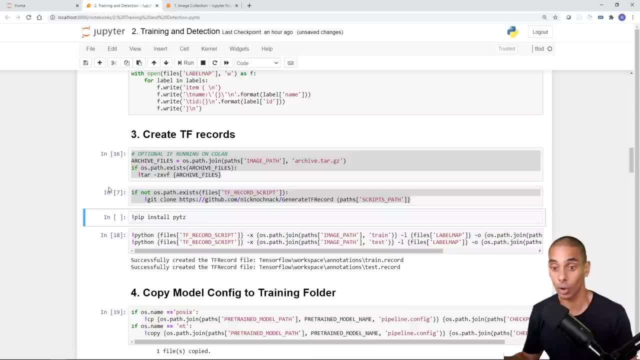 tf record script so we can run that and then we're going to create our tf record script and bring that in. it's not really good because it already is there. it's not going to clone it again, so we've got a conditional statement there that's going to prevent that happening. what we do need to 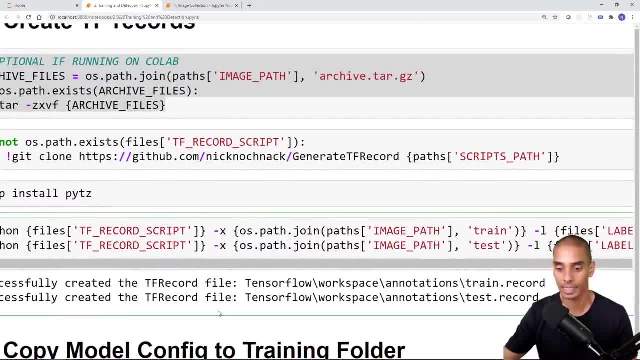 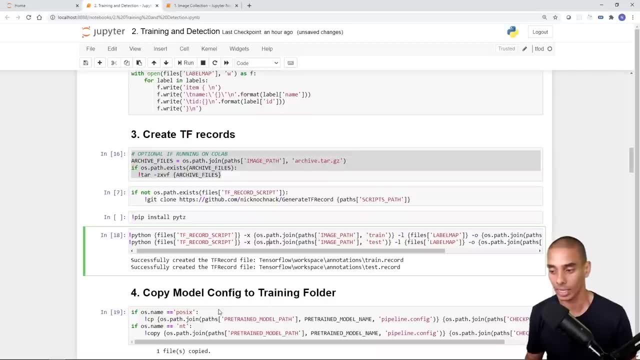 run, is this cell here? so this cell here is what creates our tf records and remember. our tf records are what allow us to actually train our model. it's what our tense flow object detection, api, uses. so if we run that fingers crossed, we effectively create our tf records. so it looks like no issues. 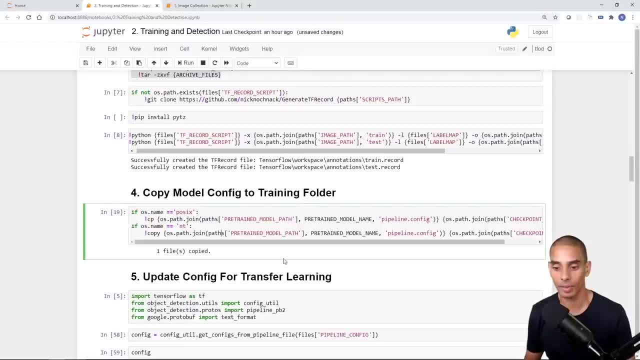 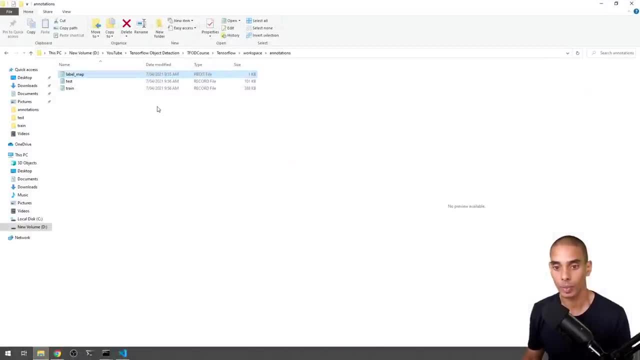 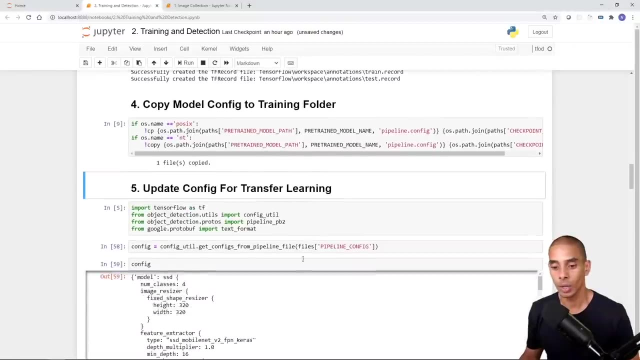 there and then again we're going to copy our model config to our training folder. so remember we created a new training folder called microscope. so if we run that, we should be able to go into our microscope folder, which is in models- microscope- and you can see that we've got our pipeline there. we just need to update our config. 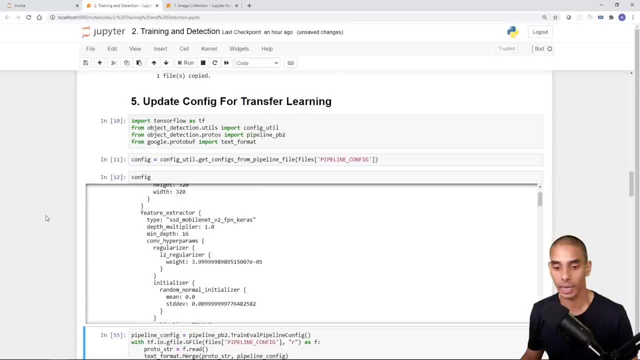 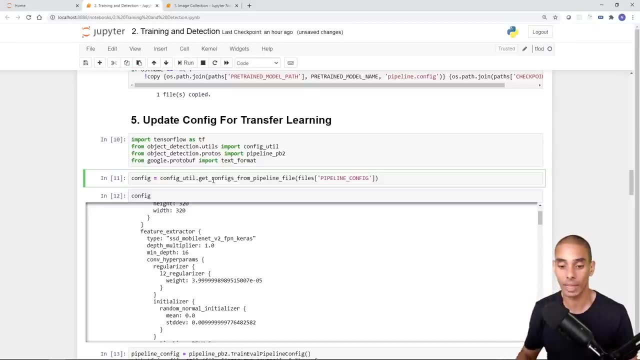 so again, so that's our baseline. we make our updates if we reload it. this is a cool thing, right? so you can actually reload that config by running this cell here. so config- underscore- utils dot. get configs from underscore pipeline file, and then we're specifically going to load that up. 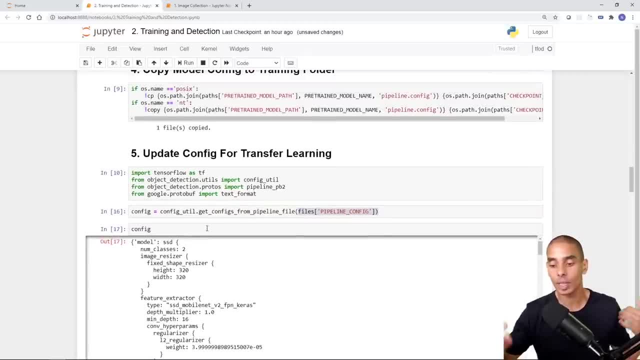 another thing that i had a thought about is if you'd like to actually see me write this code from scratch, please do let me know. i think it'll be a huge tutorial, but if you think it'd be useful to be able to learn how to actually do this, i'd love to hear your thoughts on this as well, maybe. 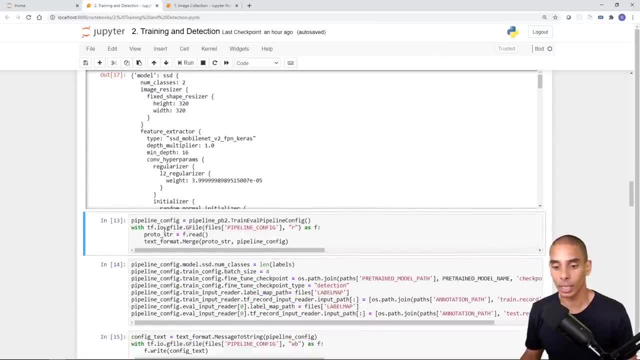 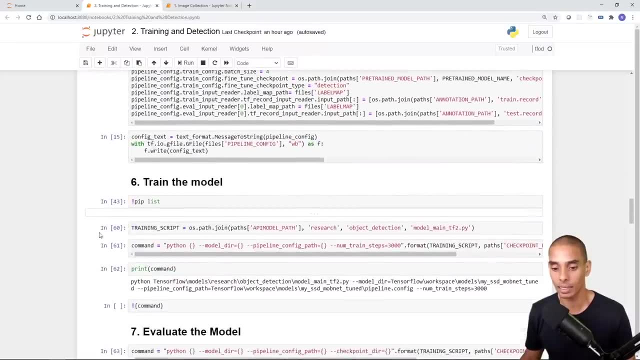 we'll do a live stream. so in this case, that's looking good. so we've reset our classes and if we scroll down, we'll reset our label map and where our testrecord file is, and we'll be able to see where our testrecord file is. let's go on ahead and train our model. so, again, we're going to. 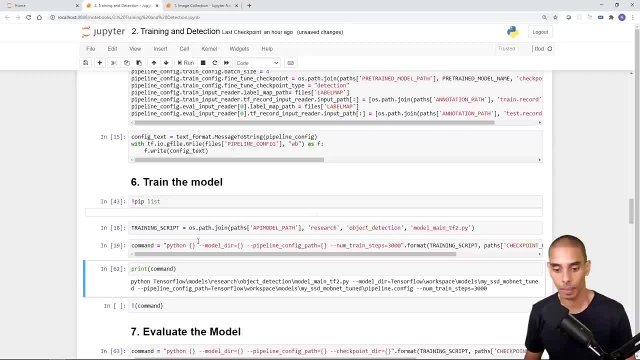 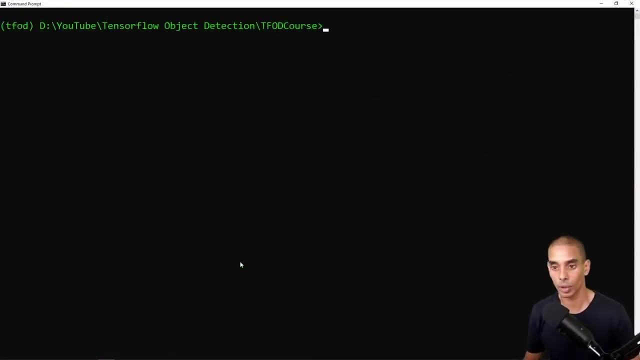 generate our training script under step six, which gives us this here and we probably don't need to train for 3 000 steps, let's do our regular 2 000. so then we'll copy this into a new command prompt and again same folder, so we can stick inside of this folder here. so 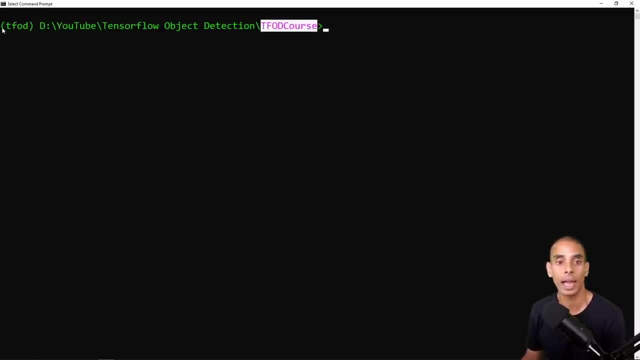 the youtube tense flow object detection- tfod course folder and we've got our environment activated. we should be able to see that we've got our environment activated and we've got our training. we should be able to paste this in and kick off our training. so we'll kick this off and 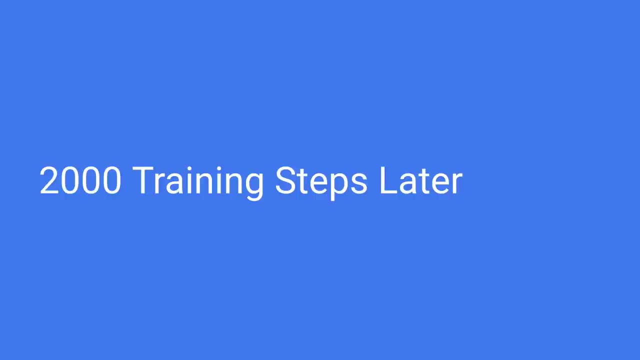 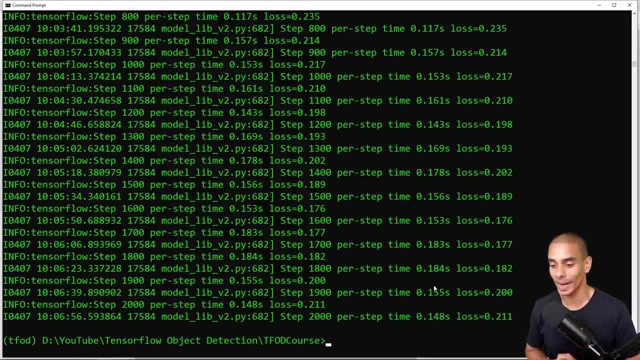 we'll be right back as soon as that's done. all righty, so our microscope object detection model has now finished training, so ideally the end goal for this is, when we load this up, we should be able to detect a bent pin and effectively, or a defective pin and a non-defective pin. so i'm interested to 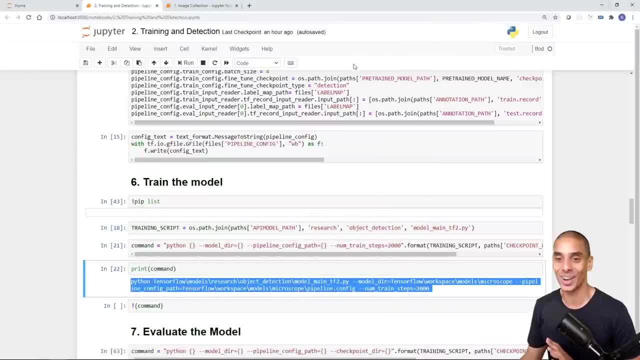 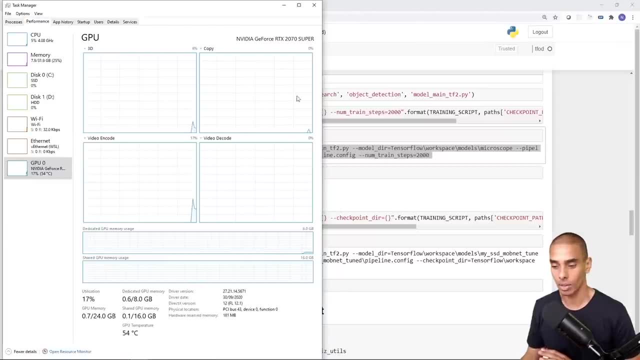 see how this goes, because i've never tried this, so this would be really, really interesting. so let's go on ahead and do this now, so we'll just make sure our gpu is fully released, because sometimes it can throw up a whole bunch of issues if it's not now inside of our microscope folder. 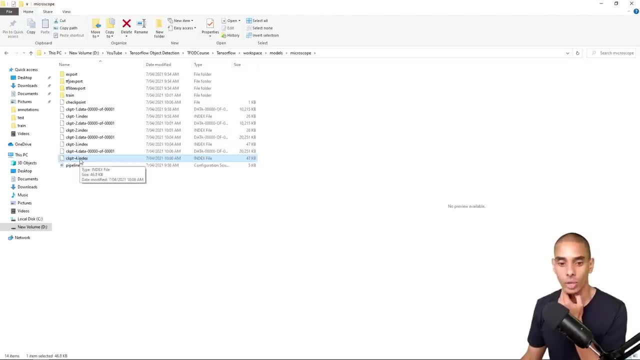 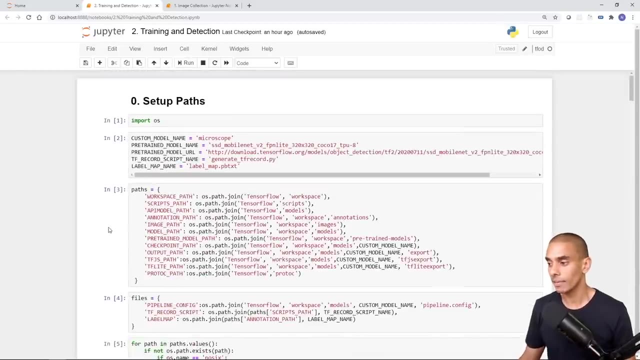 you can see, we're up to checkpoint four, so this is a little bit further than usual. so what we'll do is we will load in checkpoint four. so that's looking good, and so let me just quickly give a recap on this notebook. so step zero sets up your path. step one, or ideally point one, is: what's going. 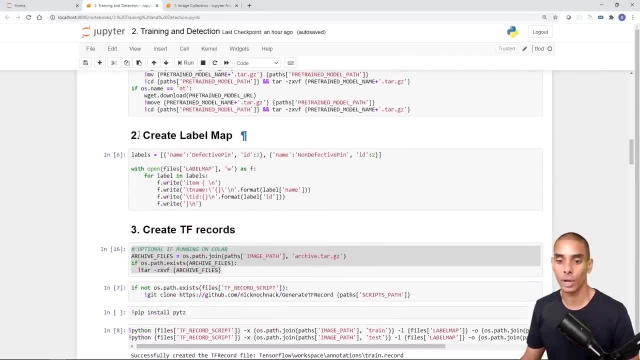 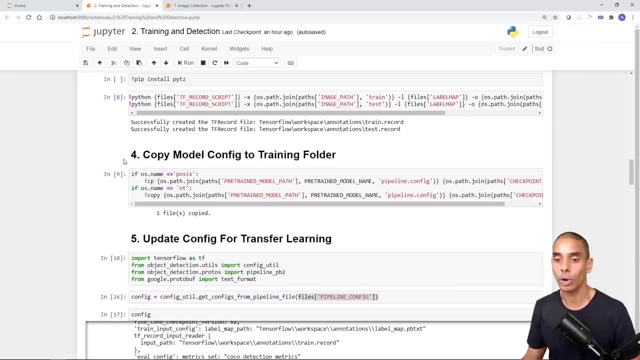 download your pre-trained models from tenseflow models and install tensorflow. step two is where we create our label map, so our different labels. step three creates our tenseflow records. four copies our pre-trained model config into our custom model config folder or into our custom model folder. step fives updates that config. and then step six trains, which is where we copy our. 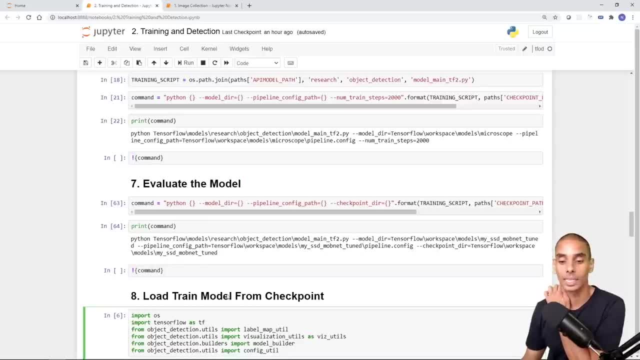 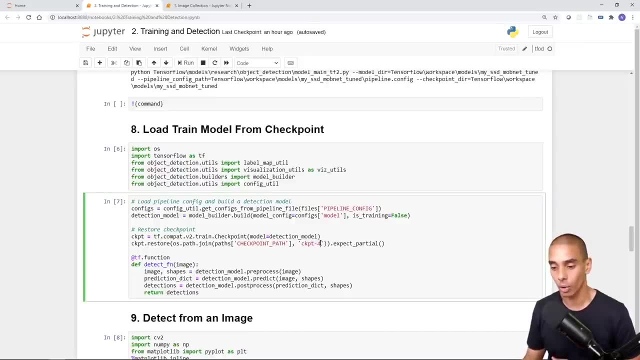 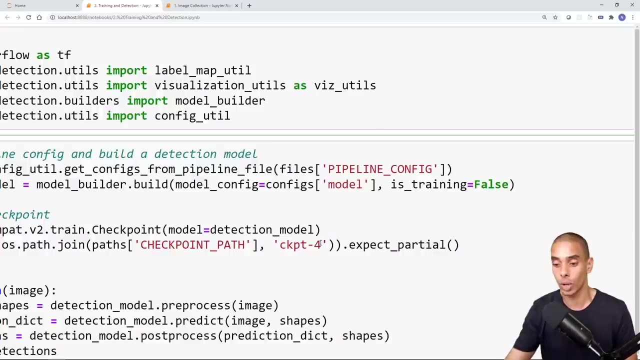 command. step seven goes and evaluates that model. so this is purely optional. step seven, eight is where we actually initially load our checkpoint. so if you get more checkpoints than checkpoint four, which is what i wanted to call this out, you can change this number to detect or use an older model or use a newer model. you sort of world your eyes to that. so, and then step nine. 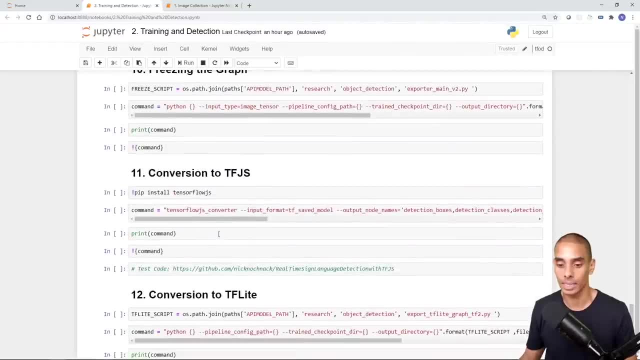 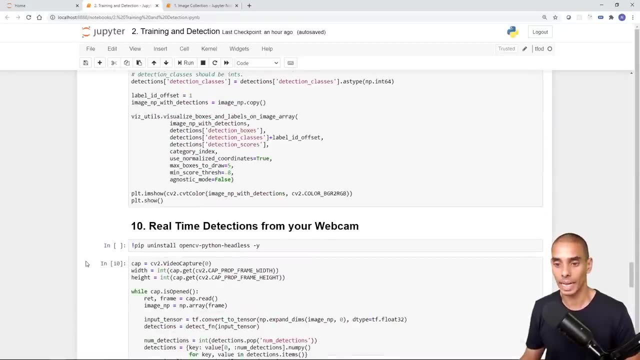 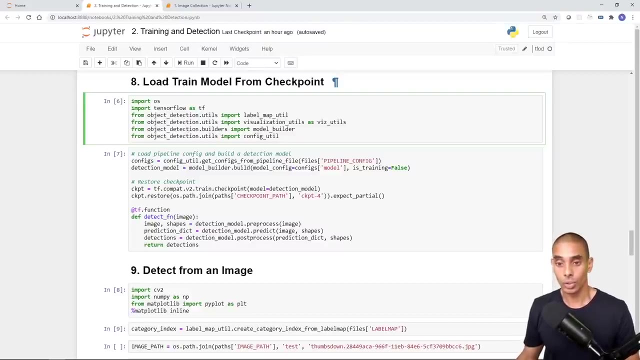 is detecting from an image. step 10, detect from your webcam. and then step 10, 11, 12 are going to be your exporting and freezing. step 13 is your zip and export. so again, i sort of wanted to drive through that step, so to run through step eight. what we're going to do is run this import cell. 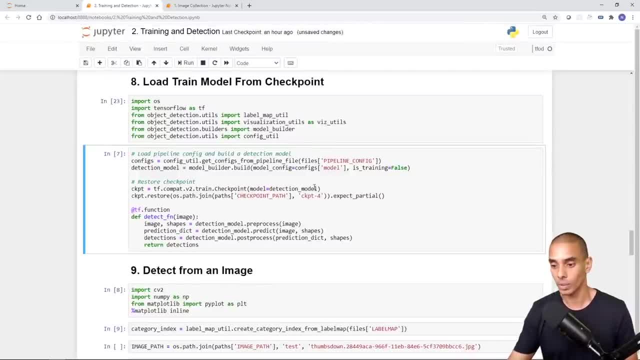 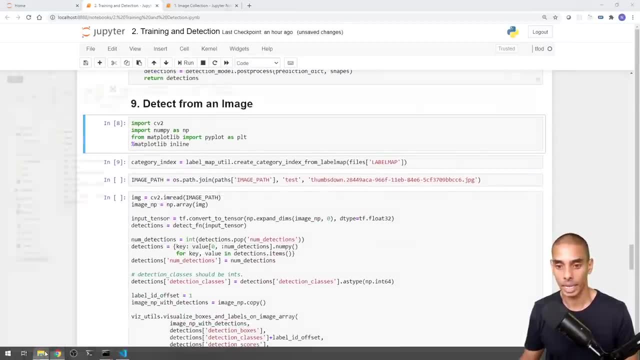 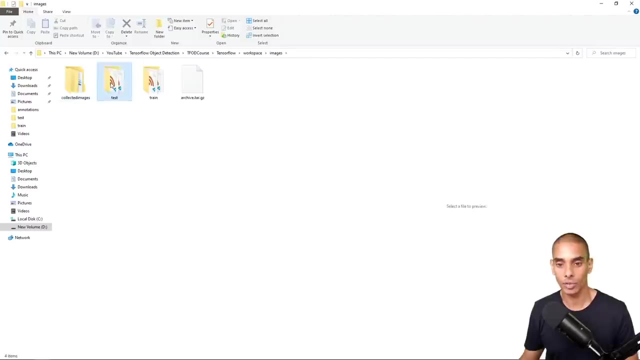 which you can see here, and then we'll load our checkpoint. so we've set it to checkpoint four and then we can detect from an image. so let's try detecting from an image first before we mess around with actual, the actual microscope. so we're going to grab the name of an image from our 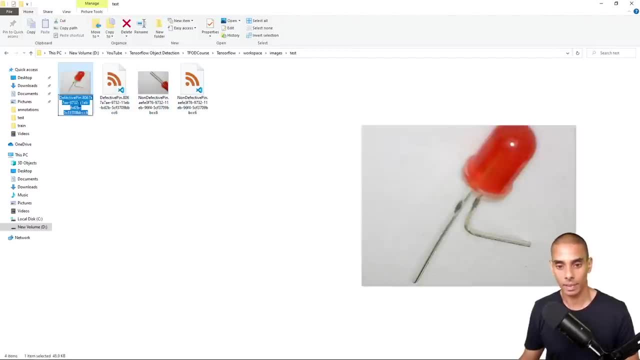 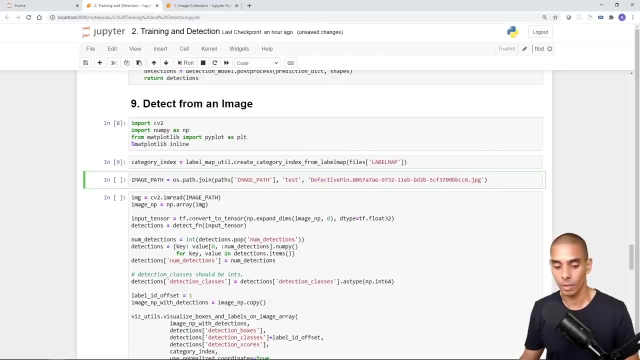 test folder. so we'll grab this defective pin and we're just going to grab the name of that image and then paste it in here, right? so all i did was i grabbed this particular image, i grabbed the name of that particular file and then i've overridden what's in this cell here. so this: 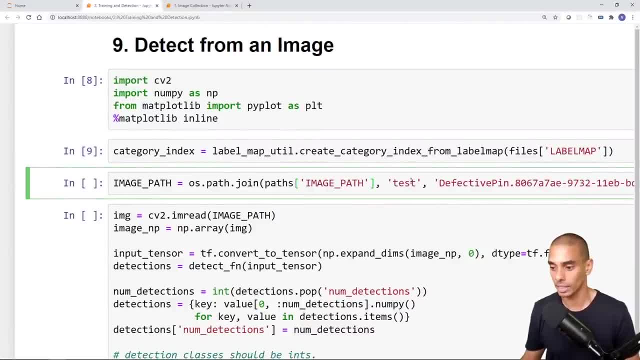 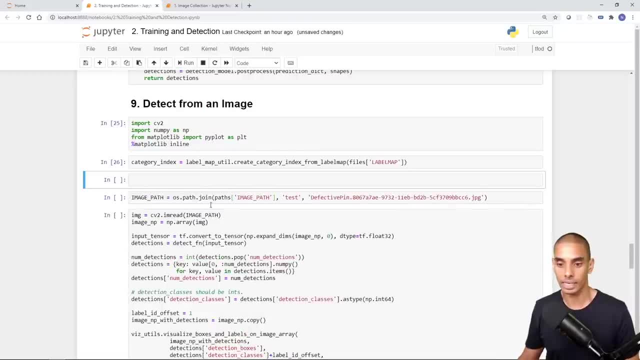 is basically pointing to where our image actually is. so i'm just updating that and what we can do is run that import, which we just did, then set up our category index and if you take a look at this category index, probably haven't talked about it much and this is just another representation. 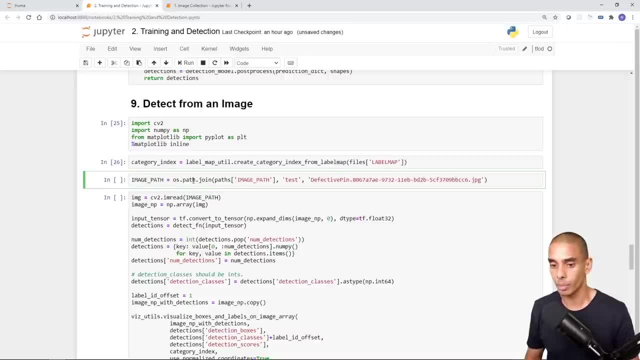 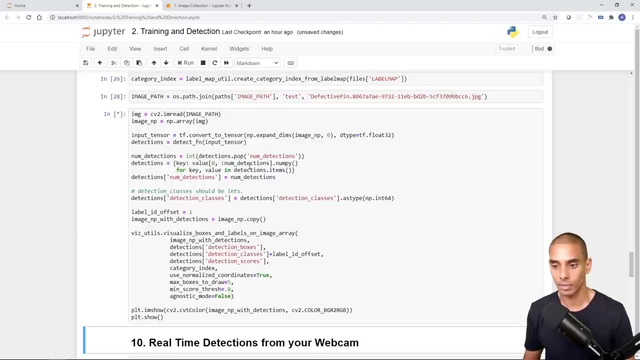 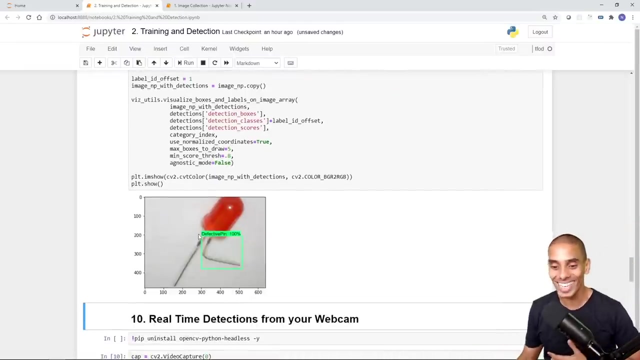 of a label map so we can close that again, bring in our image and then, ideally- fingers crossed- this should be able to detect whether or not it's defective or not defective. so now we're actually running the cell to detect. oh my god, it actually detected it. how cool is that. 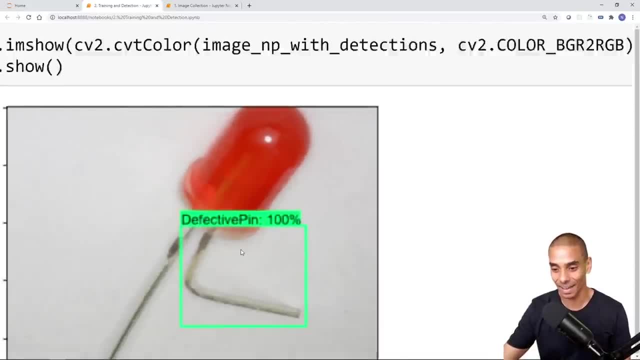 so you can see that it's actually detected the fact that it's a defective pin. now, this is probably a defective pin. so you can see that it's actually detected the fact that it's a defective pin. now, this is probably a gimme, because i mean, they're sort of in the same position, but that is is really really cool. what's? 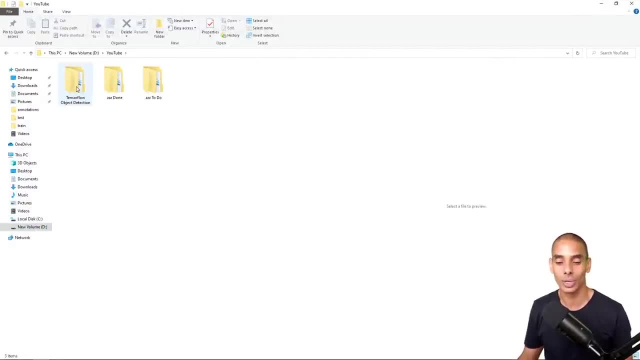 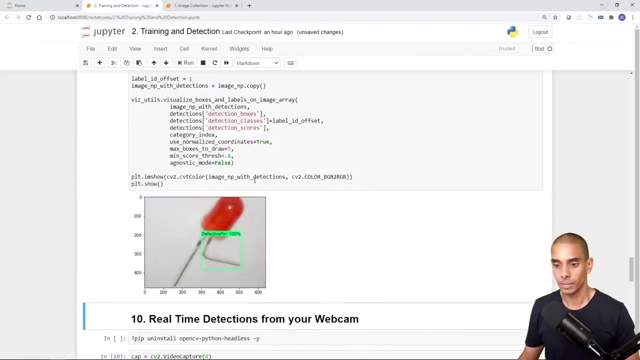 possible there. um, because this opens up a whole wide range of opportunity. right, like you can now use different types of sensors, you can scan over different types of things. let's grab another image. so, um, so what was the other one inside a test? so non-defective pin. so let's see if that works. so we're just going to update the name of the image. 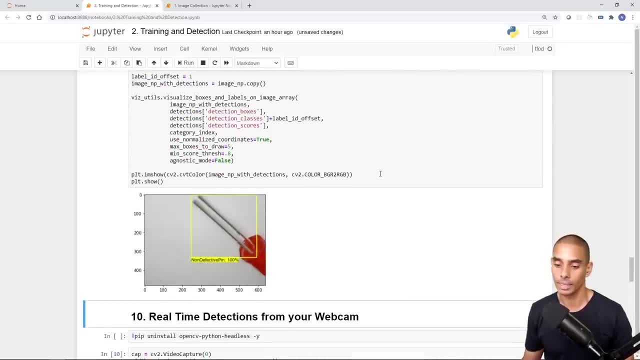 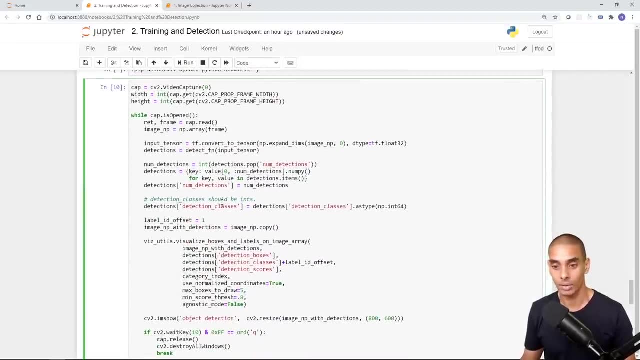 to non-defective pin. run it again. oh and it's detected, non-defective pin. we're going to run this pin with super confidence. the bigger test, however, is if we detect. try doing this on real time and see how it actually performs. so video capture zero. i think we actually need to go to video. 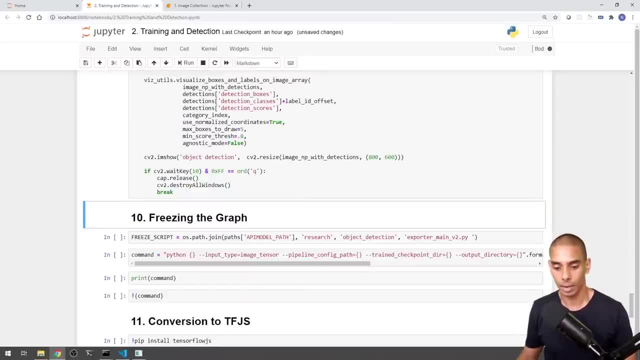 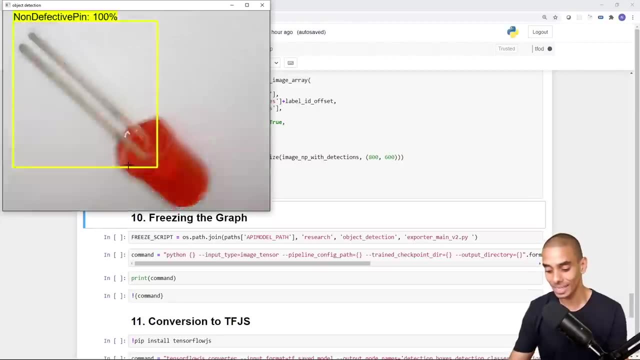 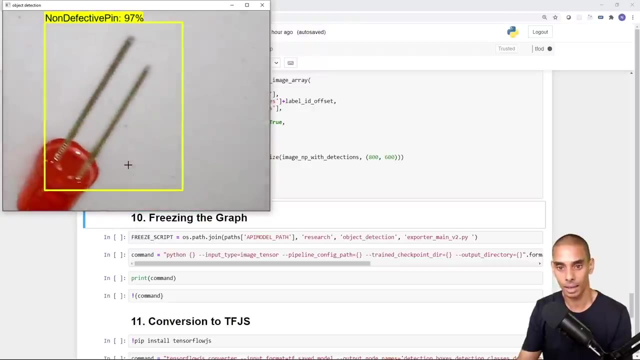 capture one, so let's test that and see if that opens up. that's looking like it's working pretty cool. so that's detecting a non-defective pin. even if i switch it the other way, it's still going pretty okay, sweet right. and this is all coming through that little microscope that i 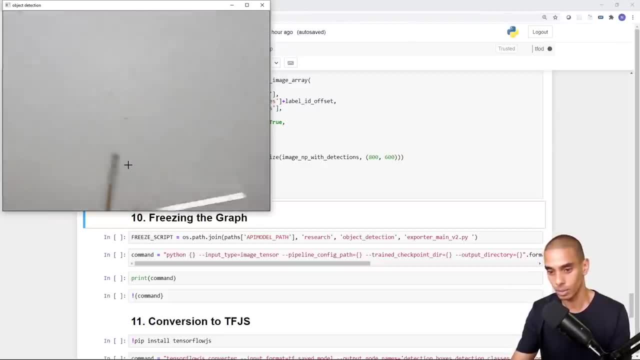 showed you what if we did a defective one? let's bring it into frame. look at that. uh, where are we? so this is sort of the concern that i had with having the defective pin in a particular position. so you can see that it's it's definitely not performing as well with the defective pin, but 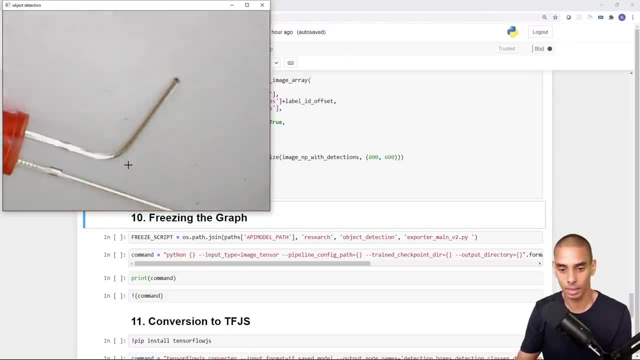 you sort of get the idea right. what's possible there? nope, is it going to pick it up? so it doesn't like the defective pin, at least from the images. okay, so it's actually picking. wait, it's picking that up as non-defective. what if we did a different? 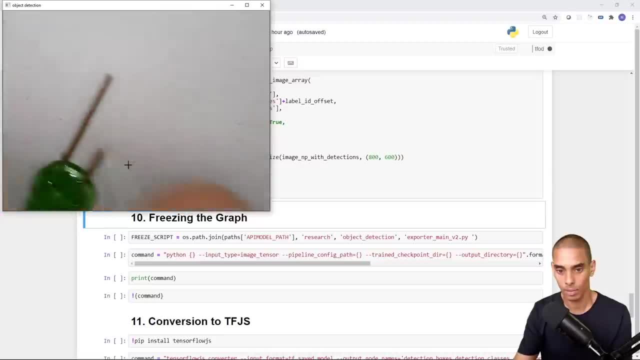 color. i wonder if it's the lighting as well. oh, this is me just just with defective pins and stuff. okay, just trying to get this into the center. there we go. okay, so it had a little. so what we can actually do here, this is actually a good point. time to. 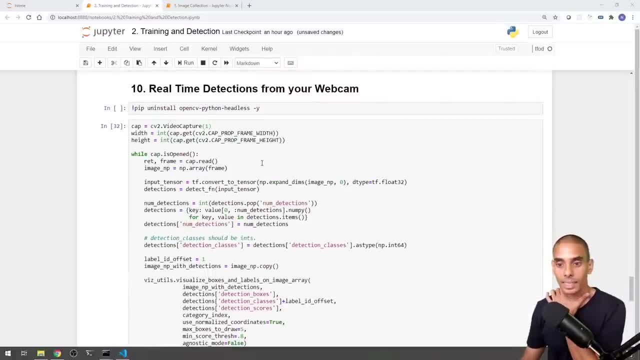 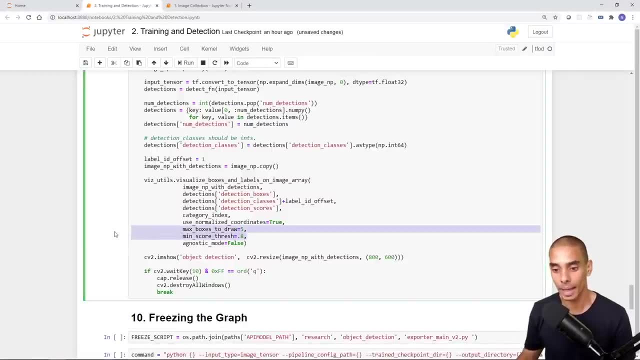 actually show you something. so if i quit out of this, this detection frame here actually has a bunch of parameters that you can choose to tune. now, the two that i'm going to get you to pay pay most attention to are the two that i'm going to get you to pay most attention to are the two: 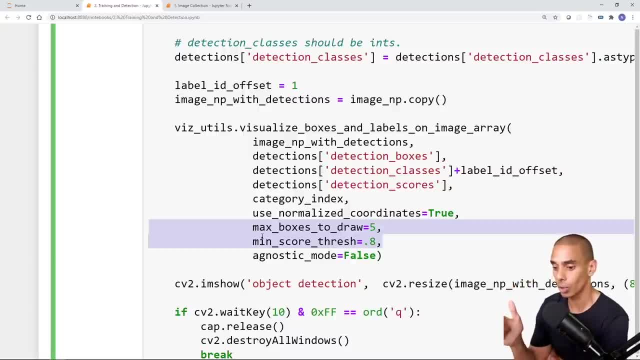 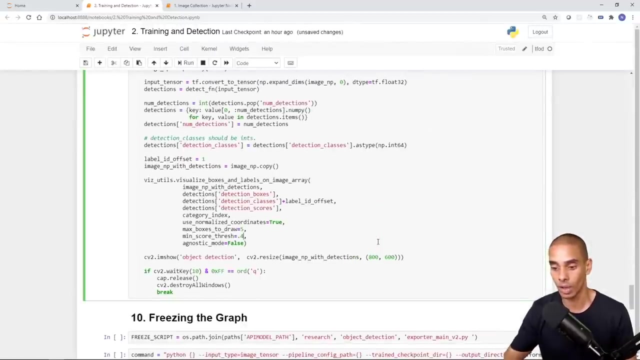 are these down here? so these two lines- max boxes to draw and minimum score threshold- define what level of quality detections you're actually going to show. so right now i've got it set to reasonably high, right. so i'm not going to show anything that has a detection accuracy of less than 80. but in this case we're not be we're not able to pick up the defective pin. so what we might do is we might relax this constraint a little bit and drop it to 40, for example. so if we run that again, okay, so now you can see that it's. 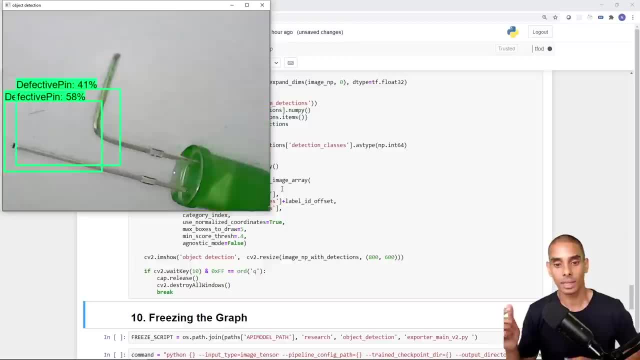 we're obviously getting a whole bunch of detections, so this is sort of what happens, right. so there's a bit of a trade-off as to whether or not you're going to be able to, or want to, show everything versus not show everything. so in this case, you can see that it's we're getting 60, so what we might do. 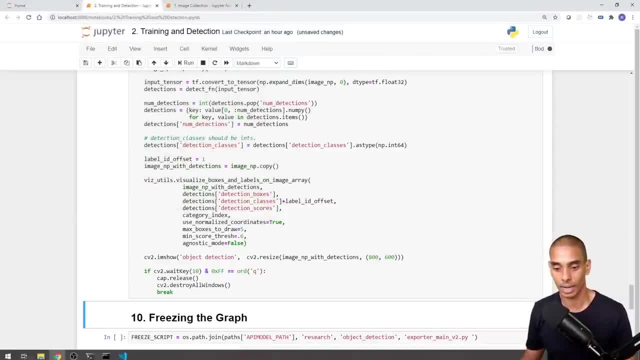 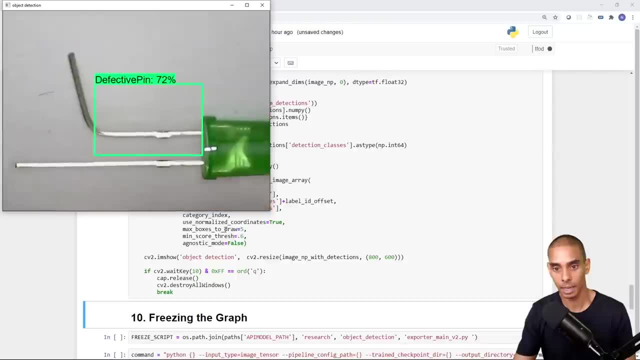 is not drop it down so much to four. let's drop it to 60 and try that again. okay, so we're now not getting anything. all right, so you can see there that it's detecting defective pin reasonably well. it's interesting that it's not actually doing the bend. 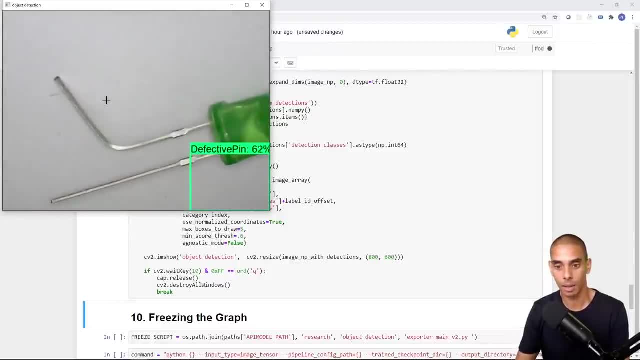 it's still detecting that it's a defective pin, but it's not doing the bend interesting. so this is the green one. let's try the red one and keep in mind we didn't train on a green image on a green pin. the led is rolling away, so that's a non-defective pin. 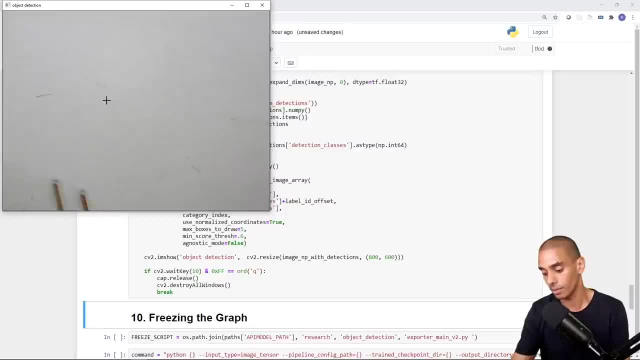 try another green one which is a non-defective, and keep in mind when we trained, we trained. it's still detecting that it's a defective pin, right. so this is going to be obviously skewed. so when i put it at an angle, for whatever reason, it thinks that that's a non-defective pin straight away. but if we change it the other way, 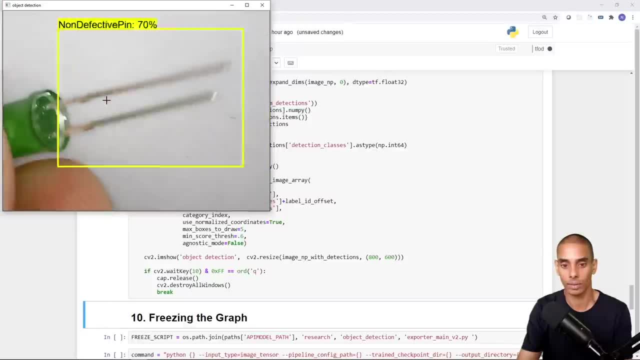 you can see that we're getting some lower accuracy detections for whatever it's detecting my thumb as a defective pin. they're pretty cool, right like so you can start to see what's possible with this. so if i bring that into frame again, it's detecting my fingers is non-defective. 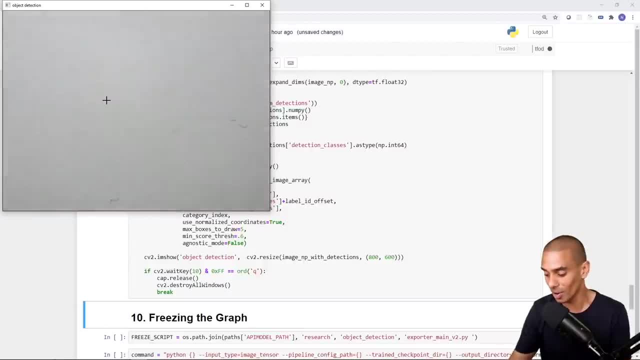 pretty cool. so let's throw in a bunch of them defective, and these are all sort of overlapping, right. so let me move, spread them out a little. so we're getting non-defective on that red one, which is appropriate. what about if we went to this green one saying that's defective? so that might be an indication. 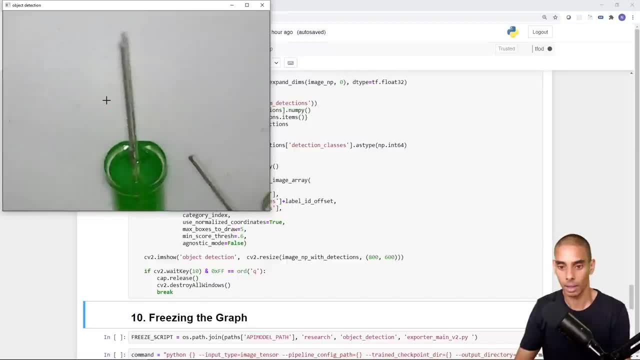 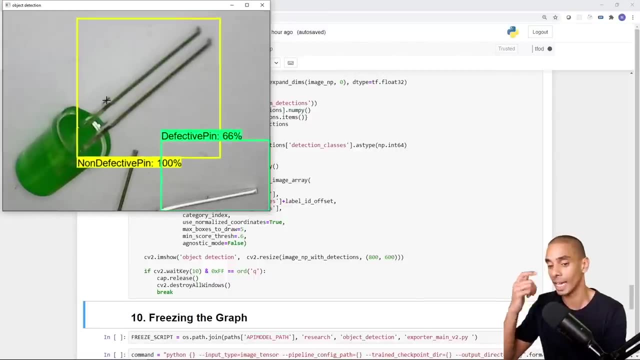 that we need to train a little bit more on that red one. so let's throw in a bunch of them right, spin this around, okay, so you can see at that angle it's detecting that it's non-defective. so that might be an indication again that we need to give it a couple of different angles. 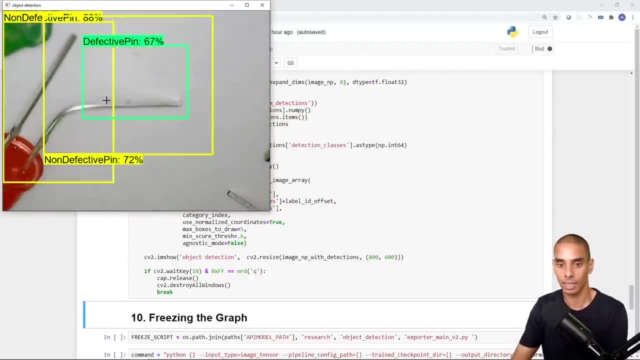 let's try it. that's saying it's a non-defective when really it should be defective, and you can reduce the number of boxes that you're also going to draw as well. so in this case, i'm drawing a bunch. you can change that parameter again. 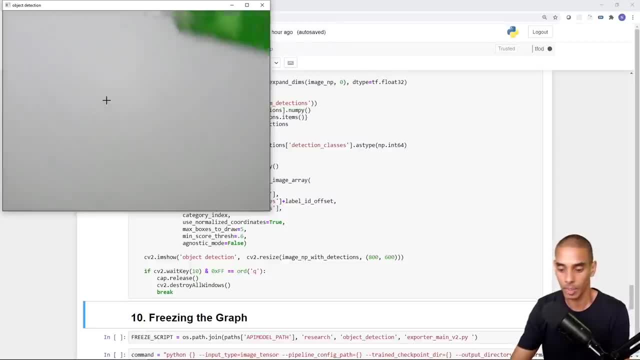 hopefully losing that pins, let's move it around. pretty cool, right? so that shows you what's possible with a bunch of other different types of sensors. so again, you could train this, you could performance tune, you could get it better. so that sort of summarizes project number one: being able to use different types of. 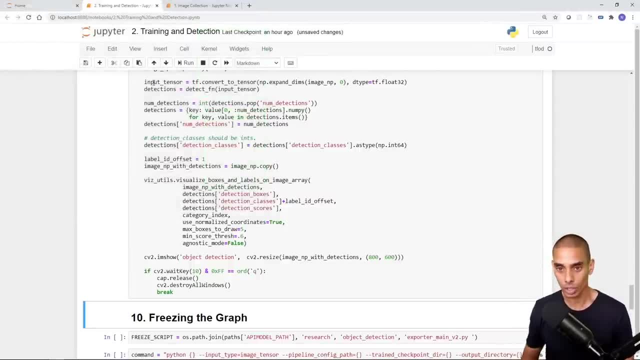 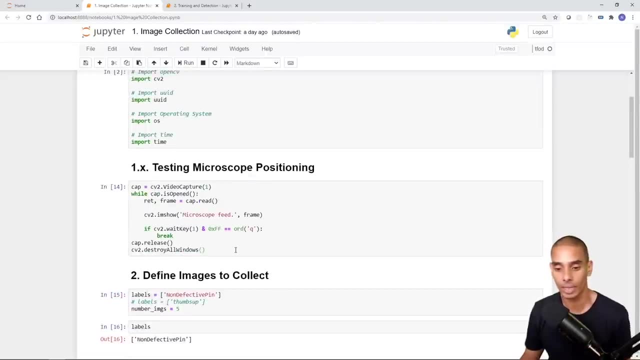 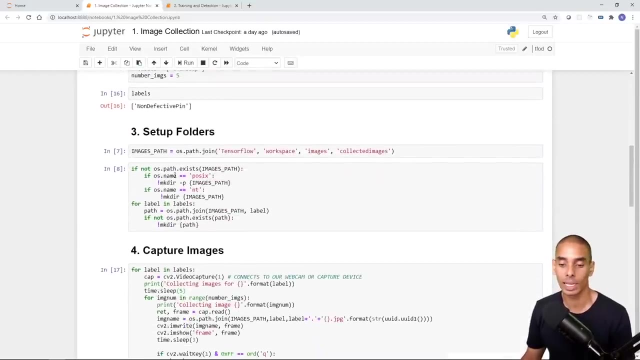 sensors for our object detection. so just to quickly summarize what we did: we went through our image collection notebook. we repositioned our microscope, so we wrote this custom code here to be able to make sure that we get our microscope positioned appropriately. we then defined our images that we wanted to collect, set up our new folders, captured our images. 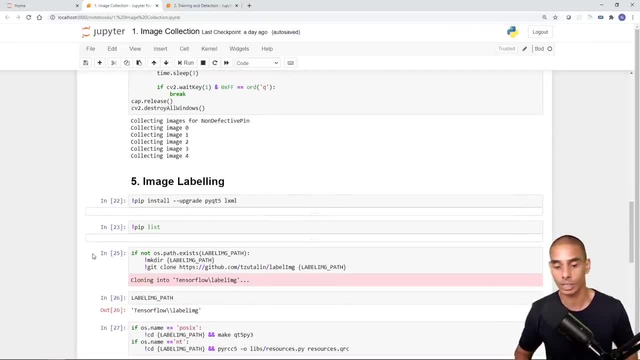 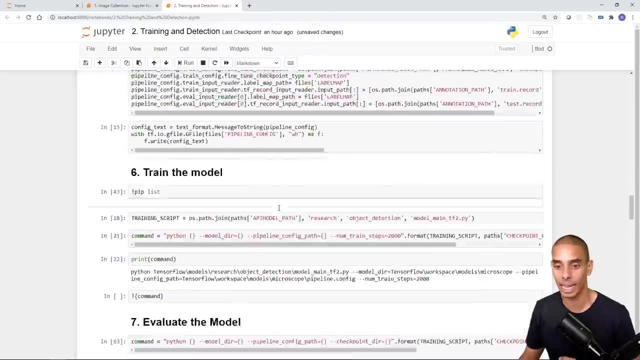 and then we labeled using label image again. so again pretty standard process. so you're always going to capture your images, label your objects, then train. now we're in our training. we sort of went pretty standard here. we didn't do anything too crazy, we just created a new folder called. 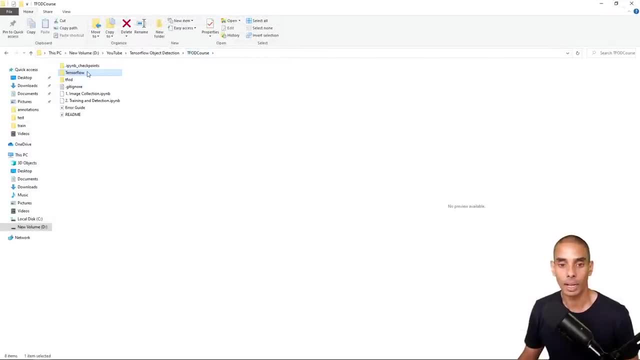 microscope. that means that all of our microscope stuff is going to be stored inside of a folder called microscope. now again, for our new projects, we're going to just create a new folder, or for our next couple of projects, we're just going to create another folder and build up from that. 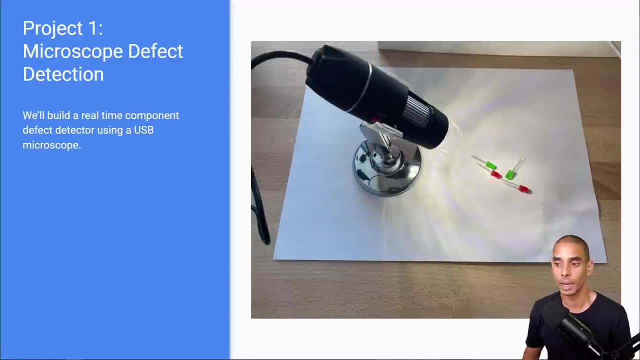 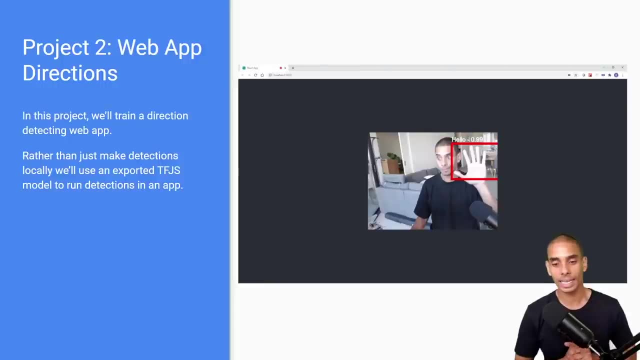 that brings us to project number two. so in this case, our next model is going to be a web app for direction. so what we're ideally going to try to do is build a object detection model that allows us to detect up down left and right. then what we'll do is we'll use a little. 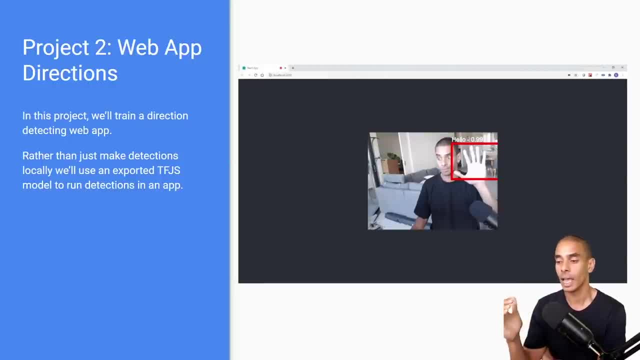 bit more of the conversion code to export this out to tenseflowjs and i'm going to show you how to actually create a web app like what you can see on the screen, so that's actually running in a browser at the moment. so let's go back to our jupyter notebook and again we're going to start. 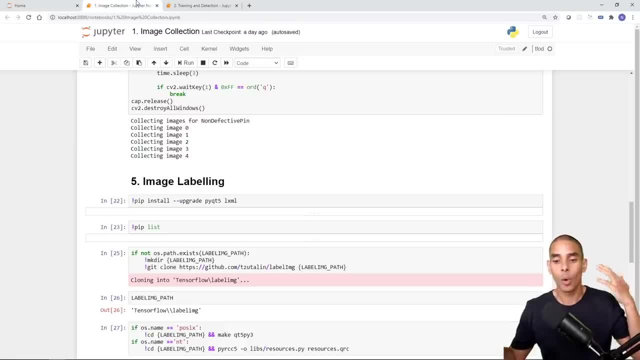 as per usual, sort of this is sort of what i wanted to drive home. so, whenever you're, regardless of what you're building, you're sort of begun. you're sort of going to be going through the same process. so you're going to collect your images, you're going to label, then you're going to do whatever. 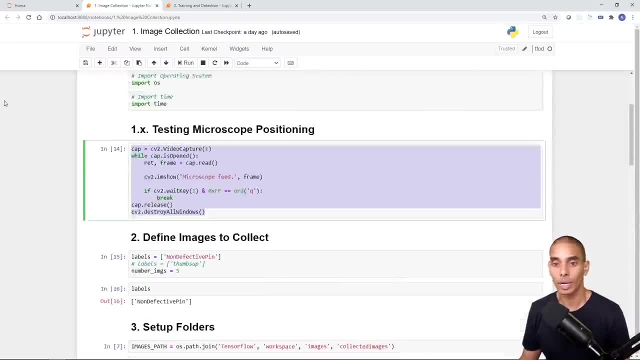 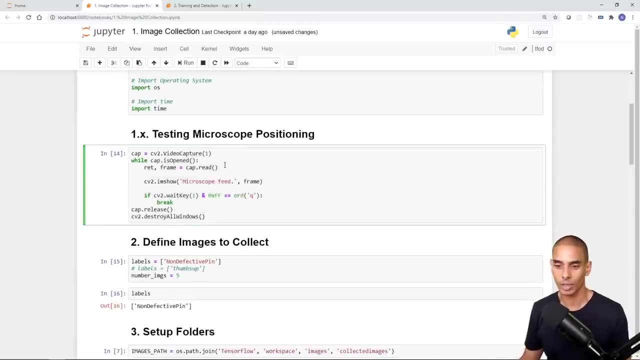 exporting you want or you're going to run real-time detection. so here we're going to go back into our image collection. code imports done, we don't need to retest, or actually we should probably retest to see, because i've gone and unplugged the microscope now and i've plugged in a webcam, so let's see. 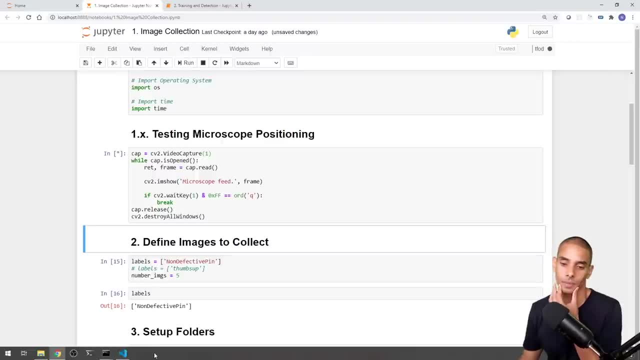 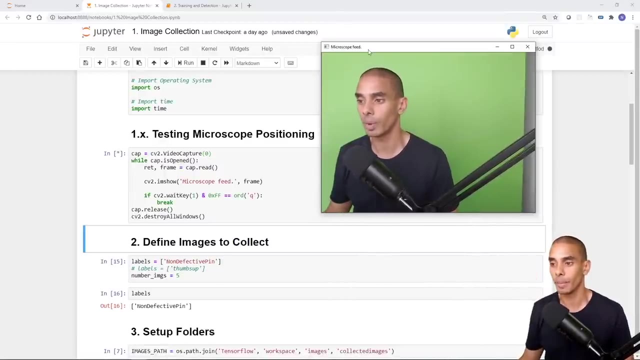 if that's working. okay. that doesn't look like it's happy, let's try video capture device one. plugged it in, looks like it's okay. all right, cool, so that's our webcam. so i just had to change the video capture device. so we're back to video capture device one. so if i'd move this way, 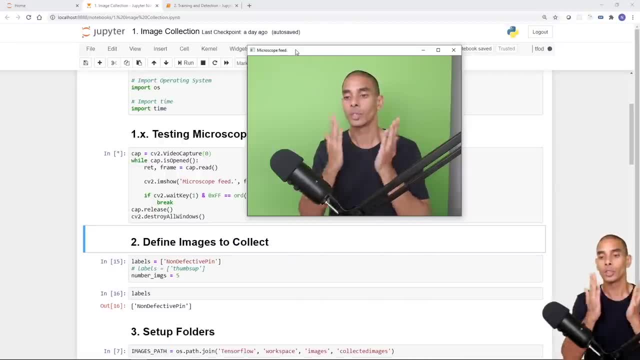 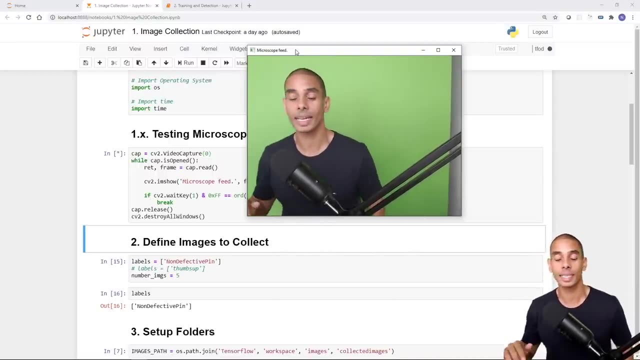 it's fine if i move this way, so it looks like i'm in front of the camera. so what we're going to do for this particular model is we're going to be detecting- let's get back in front of the mic- is we're going to be detecting up, down, left, right? so ideally, we should be able to detect those. 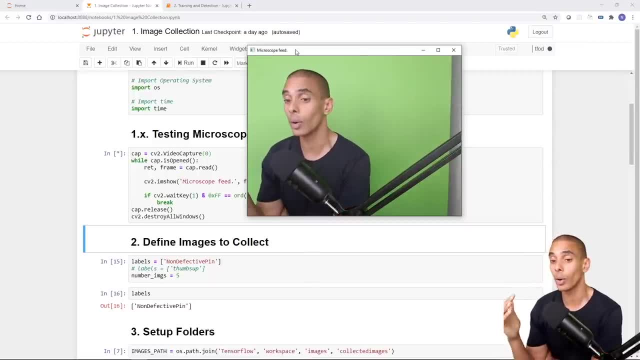 inside of our web app. now the beauty of doing this web app is that you could go and deploy this as your own website later on and have users be able to actually use that. so now this is going to take a little bit of javascript skill, but it's not a whole heap, and we're also going to need to upload. 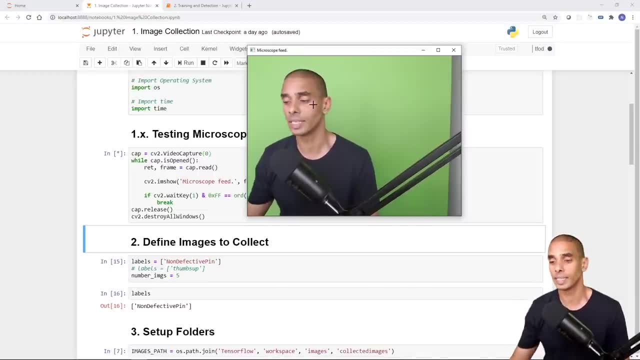 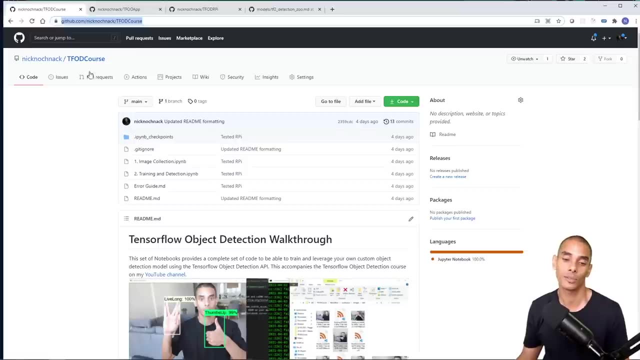 some files, but again, i'm going to walk you through this- and all the code for this is actually available inside of the github repository. so now what we're going to be doing is we'll be combining the code from our tense flow object detection course and the code from our tense flow object. 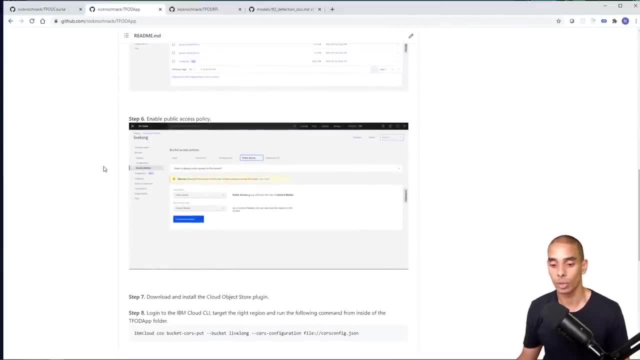 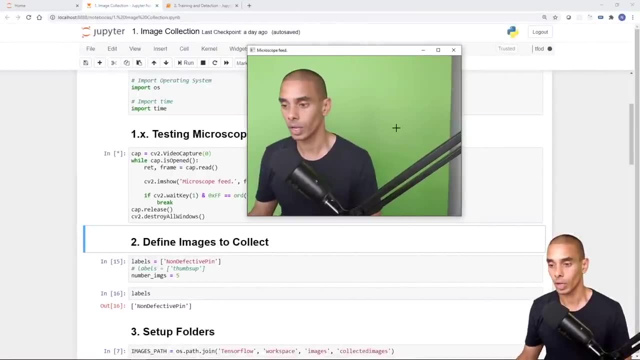 detection app github repository to be able to load this up. so let's go ahead and do this. so i'm going to quit out of this. so we've got the right feed and we're just going to change our video capture device back to zero down here to. 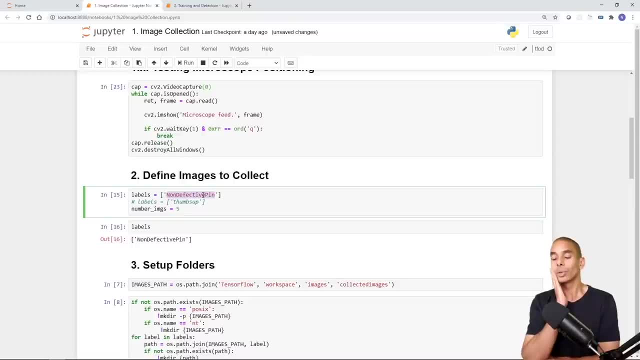 make sure we've got the right camera, and then what we need to do is collect images of left right up and down. so we're going to set, reset our label, so left right, up and down. okay, so now we're, rather than collecting thumbs up or thumbs down, or 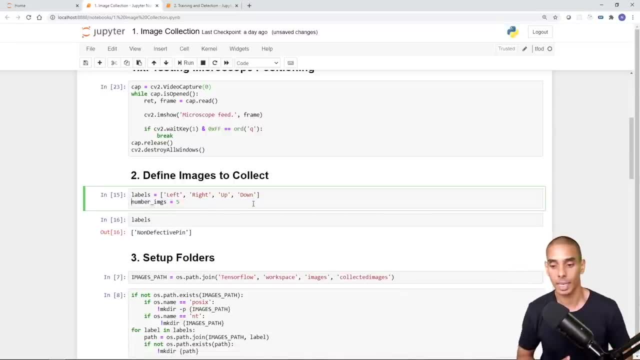 live long or whatever, or even the defective and non-defective pins. we're going to be just defining directions, so left right, up and down, and we'll try with different hands and whatnot. so what we can now do is run this particular cell and we can test our labels. i don't know. 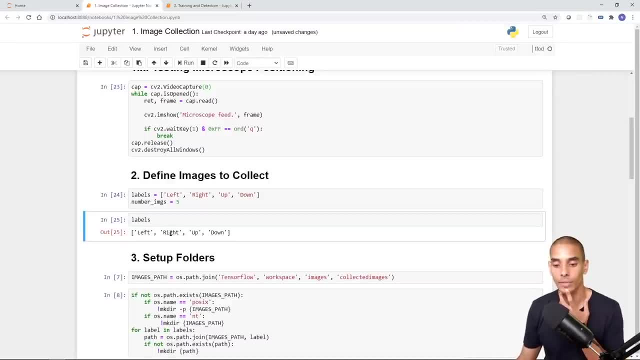 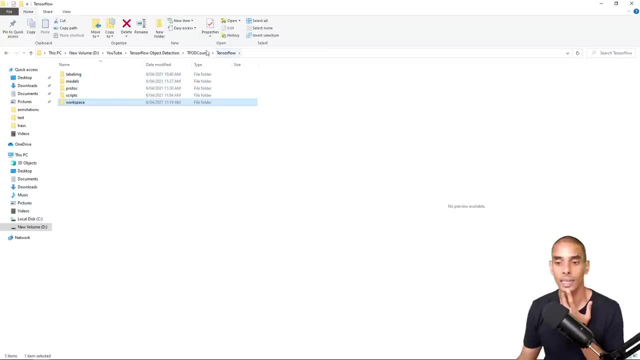 why i deleted that and you can see that we've got our correct labels. so left right, up and down again we're going to set up our folder. so if we go into our images, we again can delete everything that's in there. so if we go into tense flow workspace images, 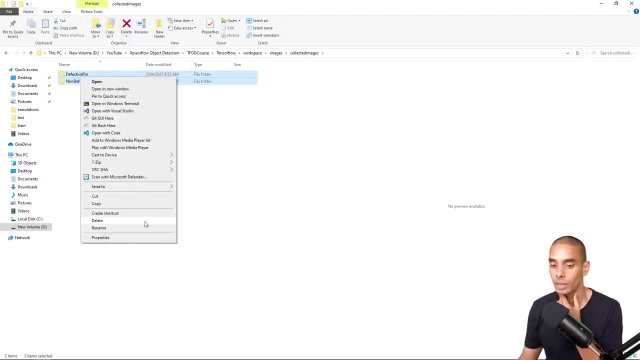 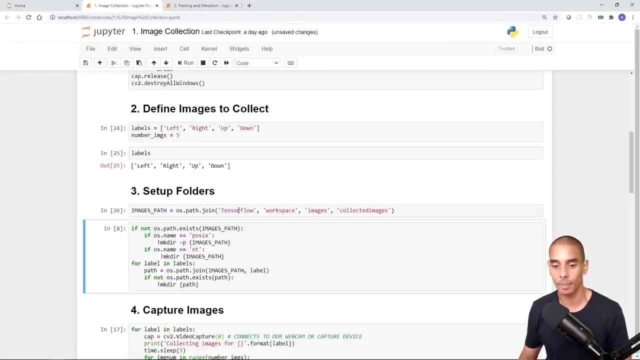 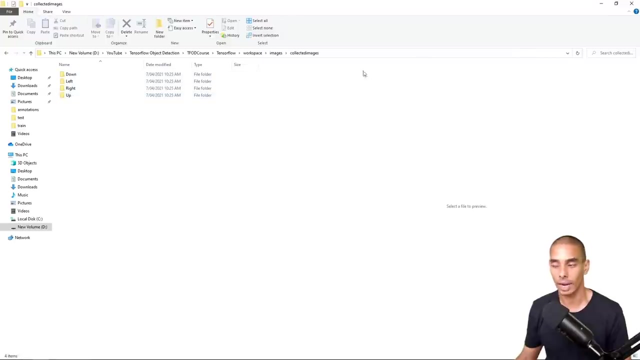 and collected images. so we've got defective and non-defective pin so we can get rid of those. we don't need to do that, need them anymore, and what we're going to do now is create our folders for left right, up and down. so if we do that and run through the steps under step three, this should create our down, left, right up and 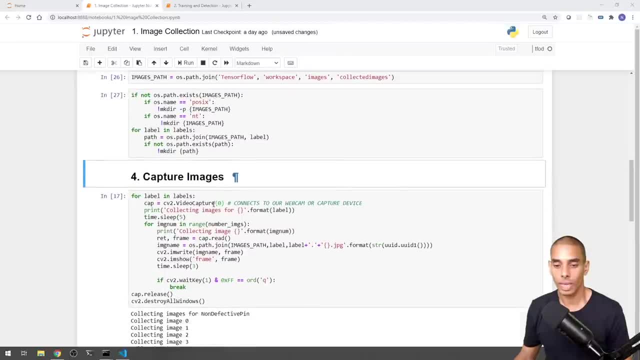 down folders and then what we can do is capture our images as per usual. so again, we probably don't need three seconds break, so we can change that. so again, we're just gonna point in our different directions, capture our different images and labels. so let's go ahead and kick things off, so we should. 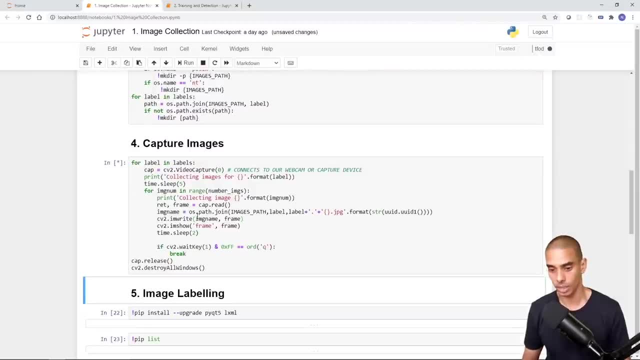 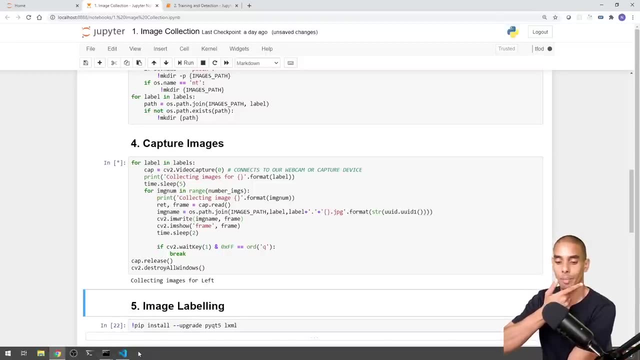 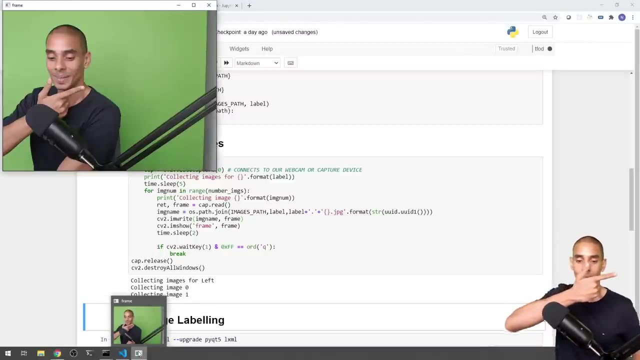 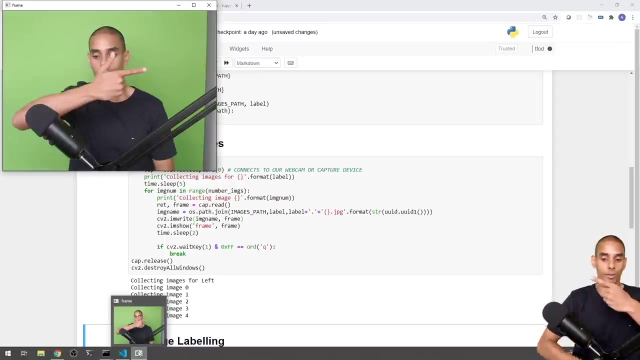 be going left, right, up and down. so let's do it again. we should get our little pop-up. so we're going to be going left first. i have to use my mouse with my left, right or left hand. okay, so left and right again, move your hand around. i probably should have collected different images. 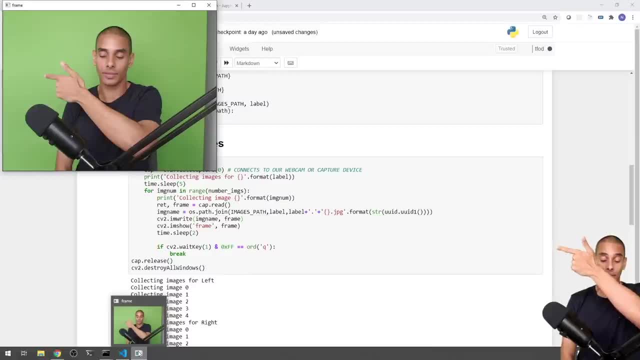 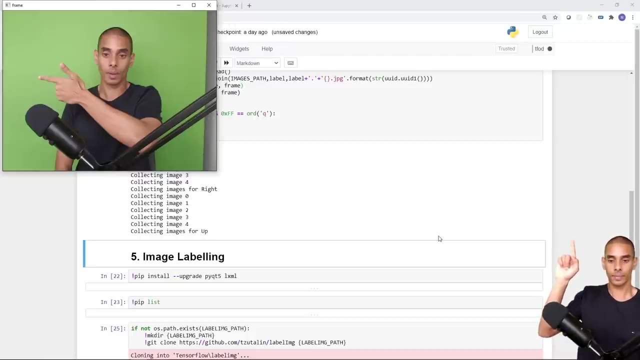 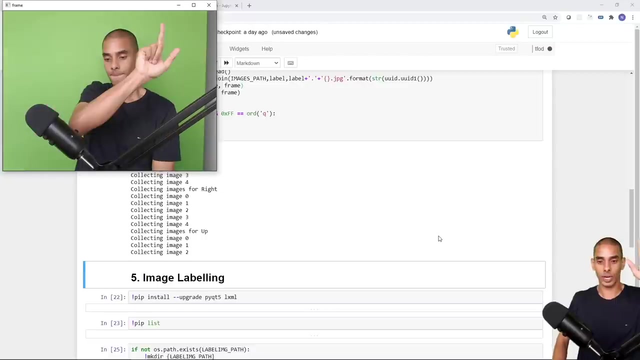 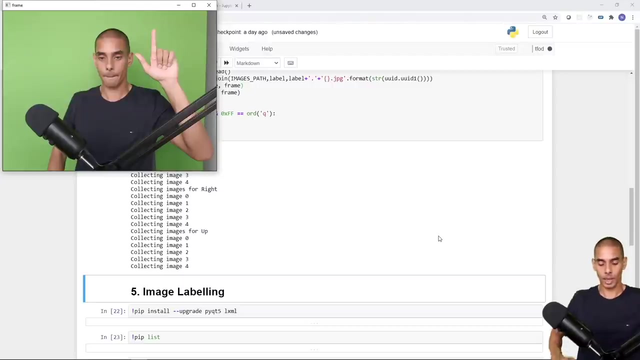 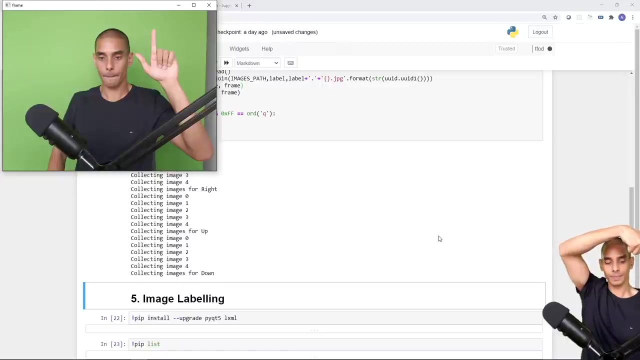 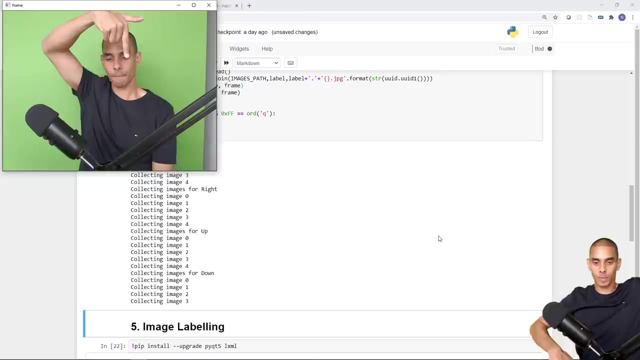 when i collected left right now it's covered all my faces behind it, so i'm just going to move my hand around, and it should be. we should be up to up right. so up and down probably do both hands to help generalize, and then down again. we'll try to use a different hand. 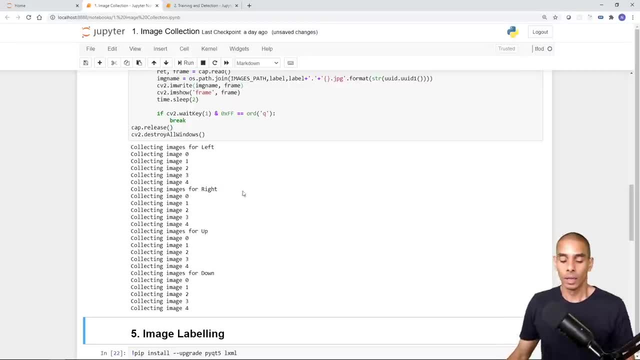 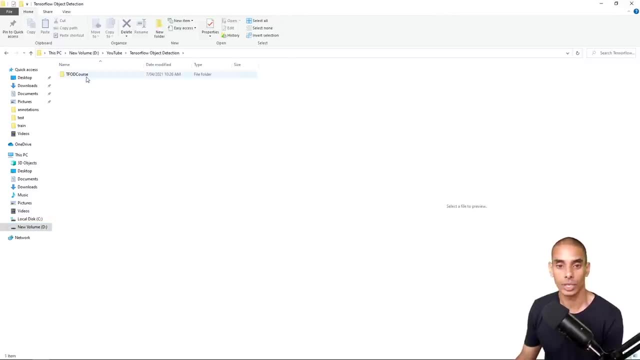 oh, that's a jewel hand, cool. all right, so those are our images collected so we can go and check those out. so if we go into youtube- tense flow object detection, tfo, d course tense flow workspace images, collected images. so we've now got images inside of down, left, right and up. so that's looking. 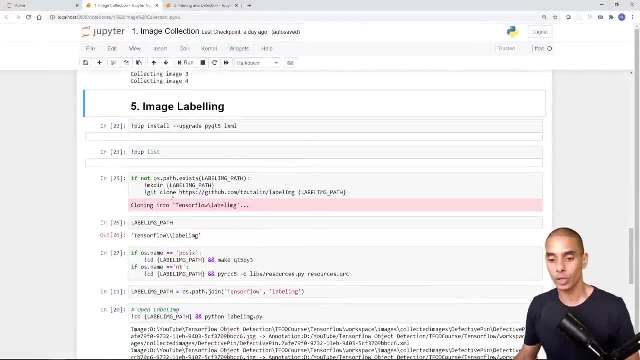 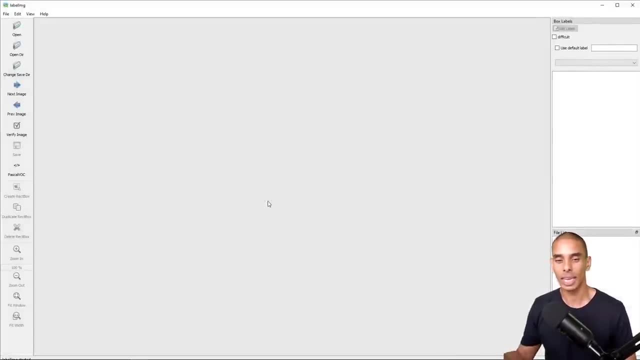 good, okay, now what we need to do is label, as per usual. so, again, we need to define our label image path, which we need to define our label image path, which we need to define our label image path, which we had already. and we need to open up label image because, keep in mind, we've already got it. 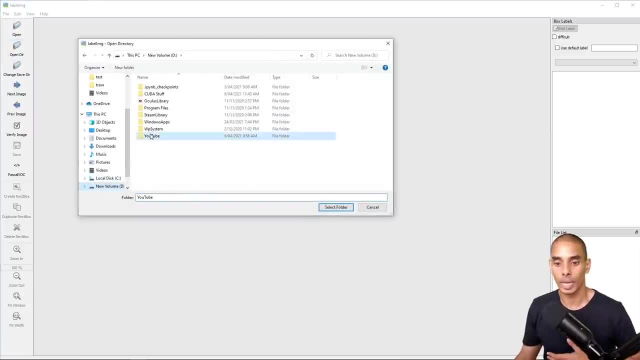 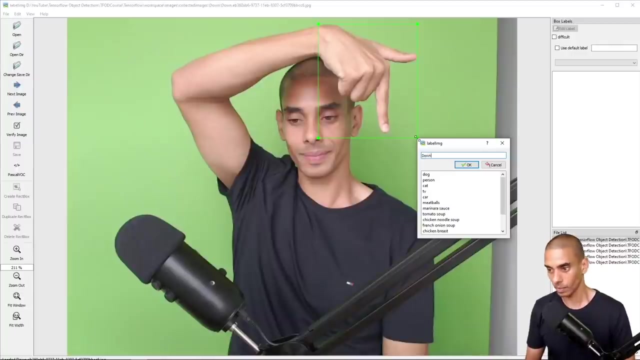 installed so we're just going to open it up. so i'm going to go into my image path or image path, and we're going to start labeling. so we're going to go into collected images and down and then open those up. so that's down and again paying attention to the case on our images. 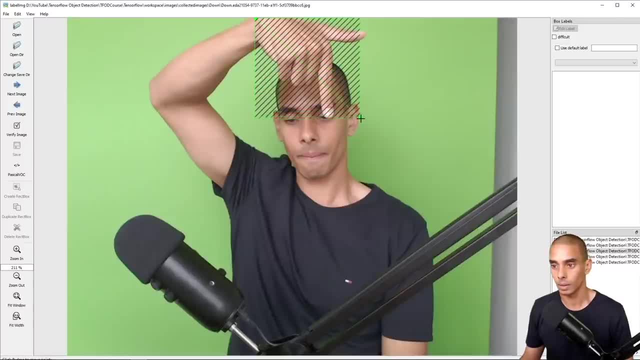 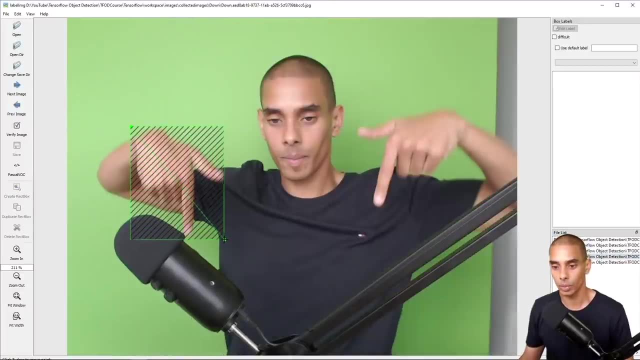 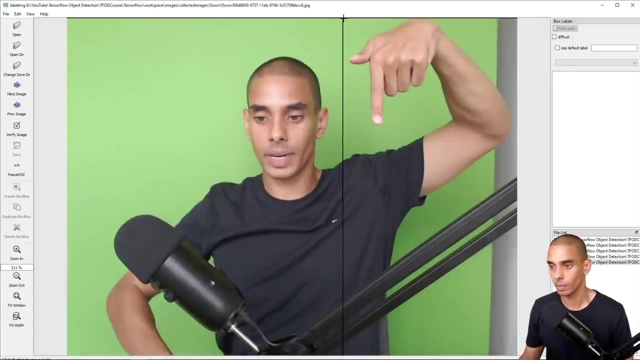 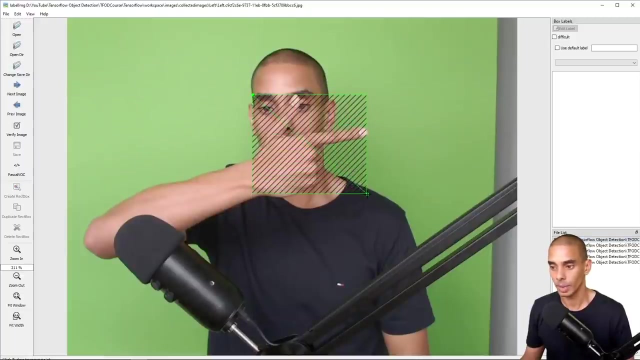 beautiful. do the next one now. again, if we get lackluster performance, we can always come back and performance tune as well. so we're going to do down on that one beautiful, all right. so that's down done. let's grab the next one. so left probably needs to be flipped, but that's fine. 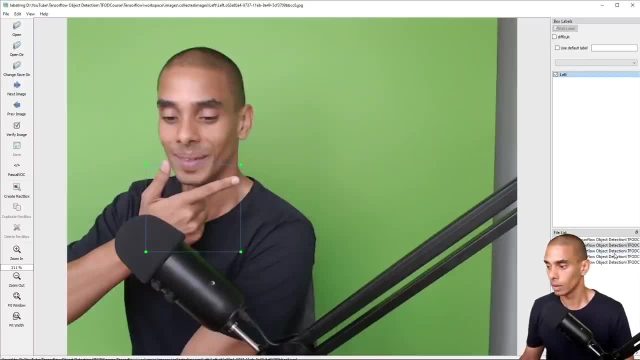 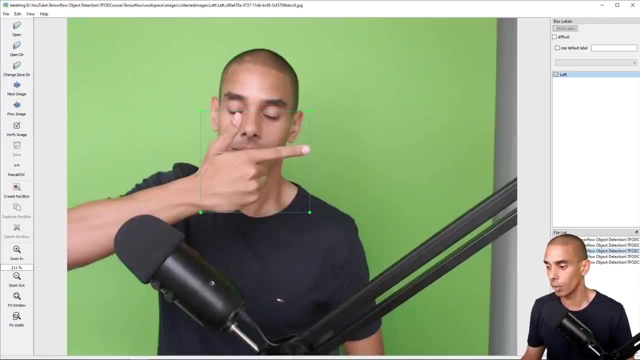 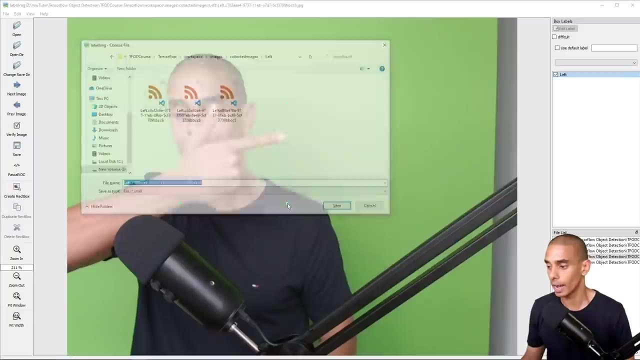 behind the mic. yeah, that'll be an interesting one and we'll keep on going. so left. so down had okay images left. i'm a little concerned because they're all kind of in front of my face. so again, we might not get the best performance on here, but again, it's all about testing and training and trying it out. so left, then we'll go left again. 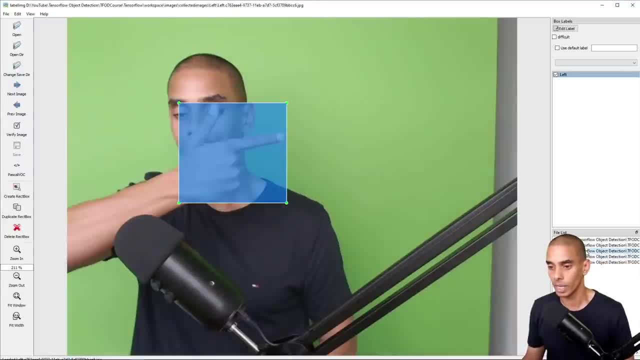 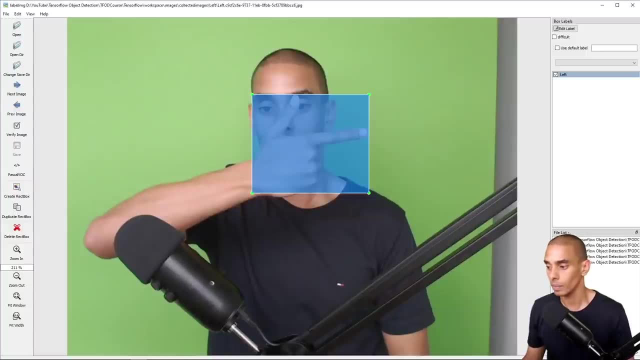 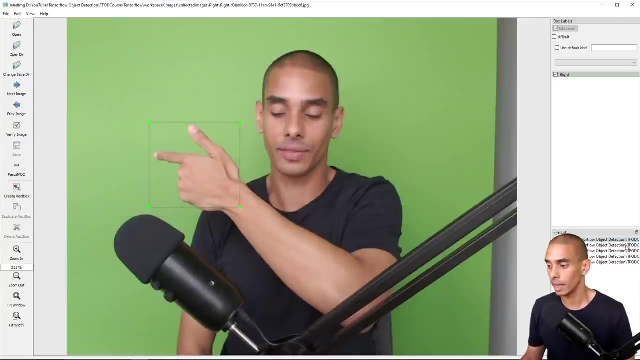 out cool so that, all of them done, we can check our labels. all right, so we're good there. then we'll go into right, let's do that Verdict. we're going to change our label again. save right, save the next one, all right, so that's something that can happen. 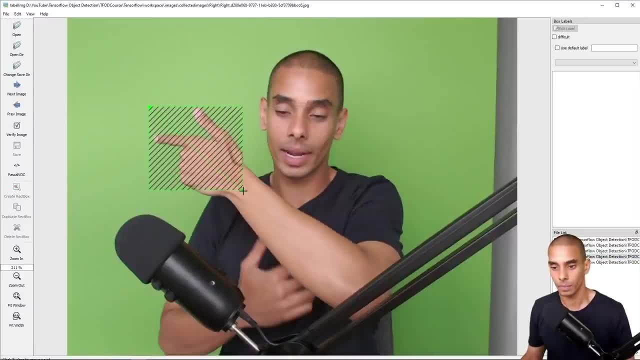 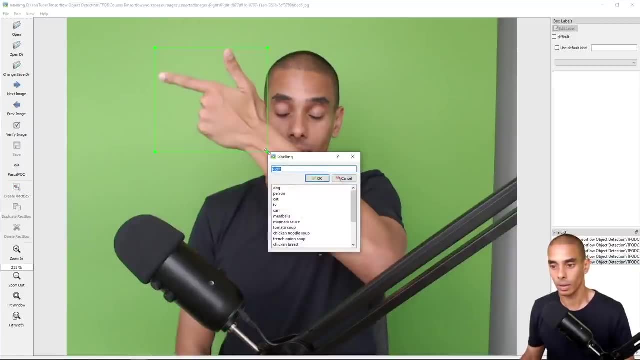 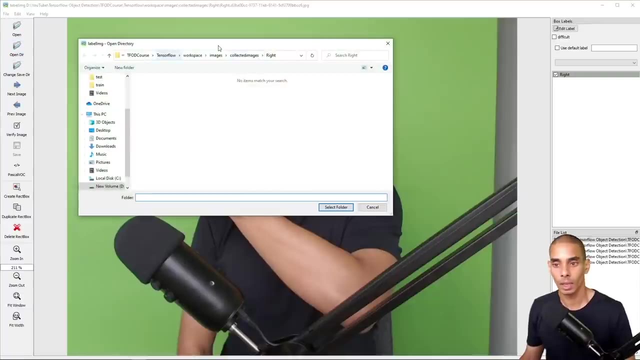 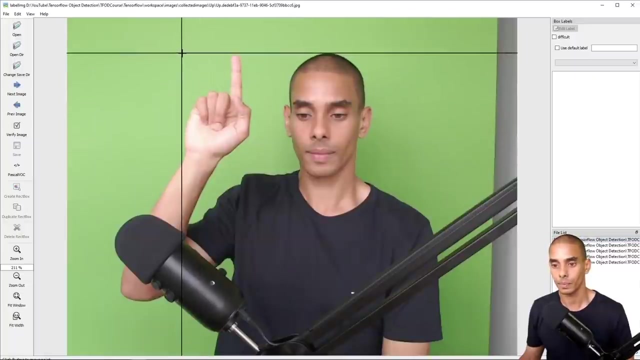 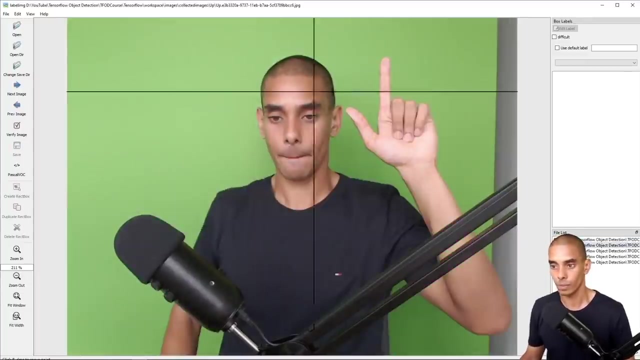 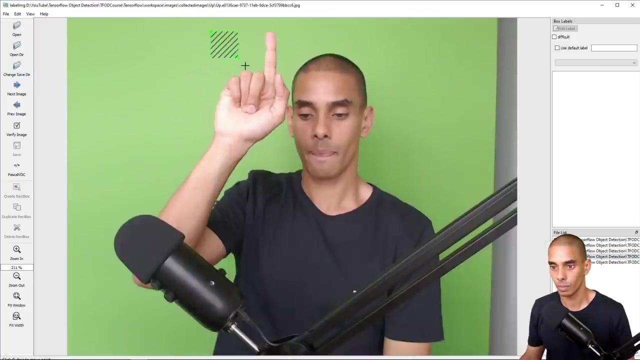 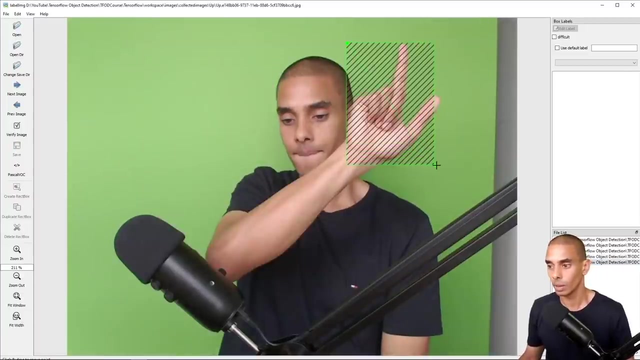 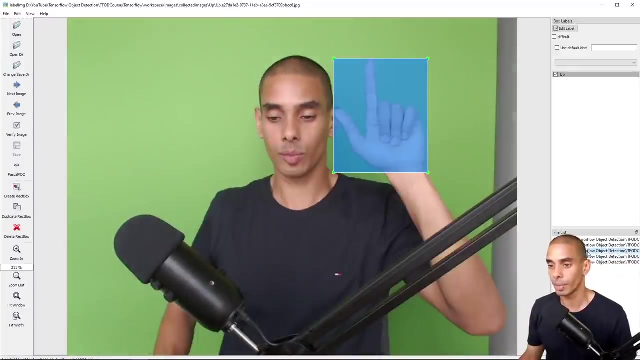 Save that, save that. and then last one over here. okay, check our labels, beautiful, alrighty. last one up and let's do it, okay. and then last one, and keep in mind we're only doing five images per object or per class at the moment. 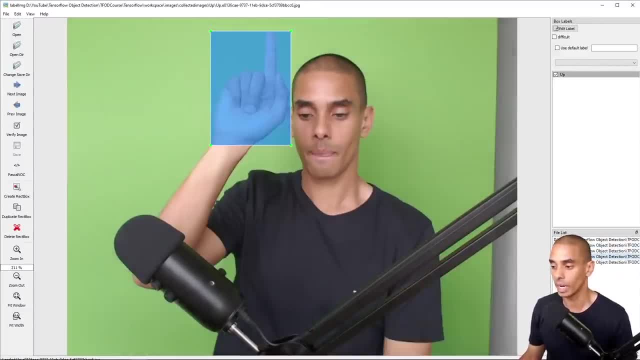 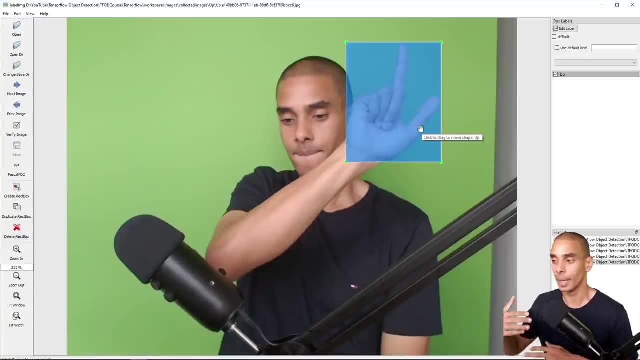 but you could definitely do more. I normally do five, ten, twenty when I'm just prototyping and obviously if I'm labeling twenty images in this tutorial, it's going to take quite a while. so five is fine, but play around, add more images, add less images and remember you can collect. 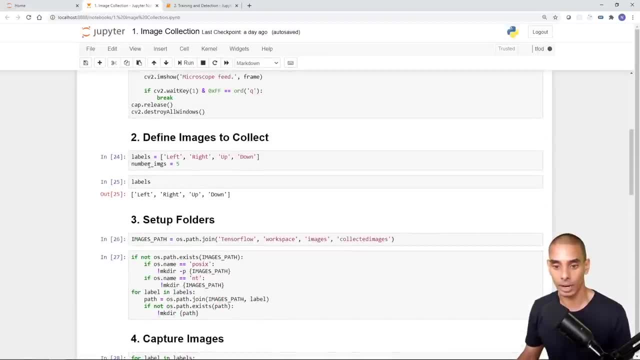 a varying number of images just by changing this line over here. so number underscore images. so right now I've got it set to five. we could set it to ten, twenty, thirty, forty, fifty, hundred if you really wanted to. 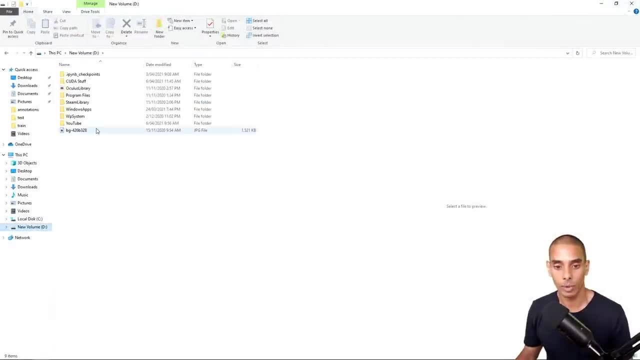 okay. so on that note, we have now gone and labeled our images. so if we go into our images folder again and again, it's probably getting repetitive now, but it sort of gives you an idea of again the process is going to be the same. so we've got our images in down. 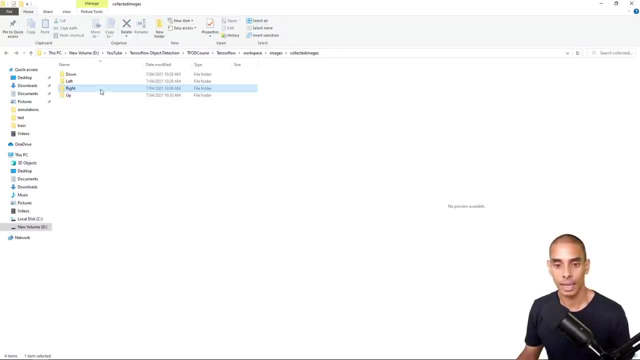 and our annotations for down and left, right and then up. and so what we'll do is we'll clear out our test folder of our pin stuff. and now what we'll do is we'll go to our collected images and again we're going to do the same thing. 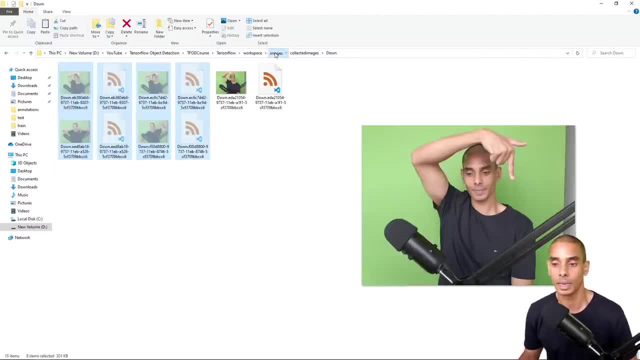 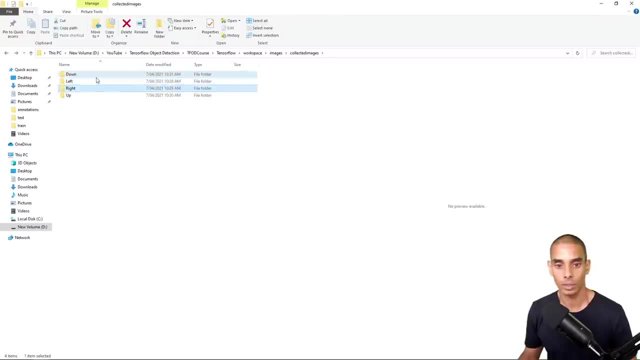 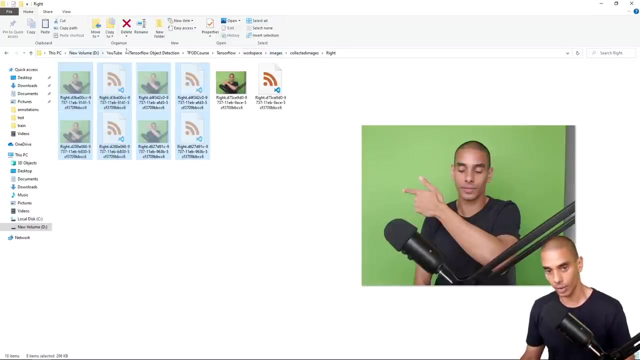 so we're going to cut them out and paste them into a training and testing split. so we've done down, let's do left. we're going to paste them into a training and testing split. so at the moment I'm pasting four of the available images inside of the training folder. 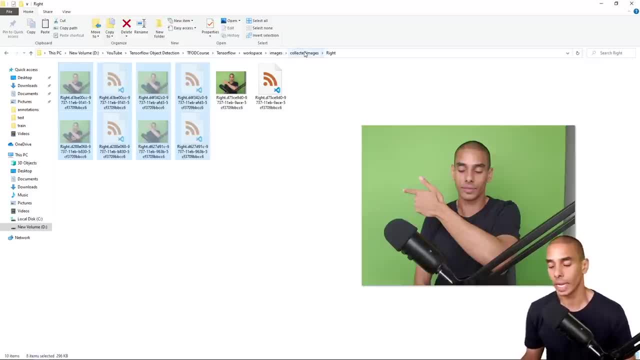 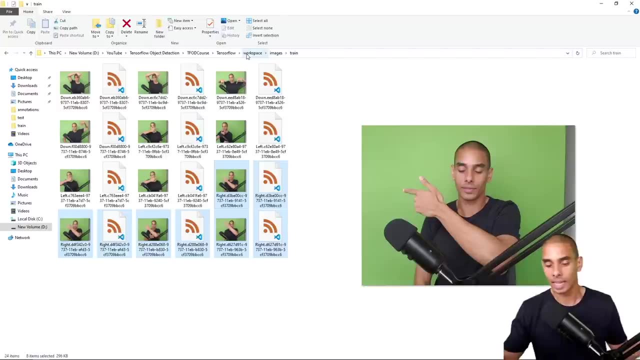 so what would that be? an 80-20 split and play around if you want to include more or less again sort of trial and error a little bit here and data science, and specifically this being deep learning and data science. it is an iterative process so you can go through. 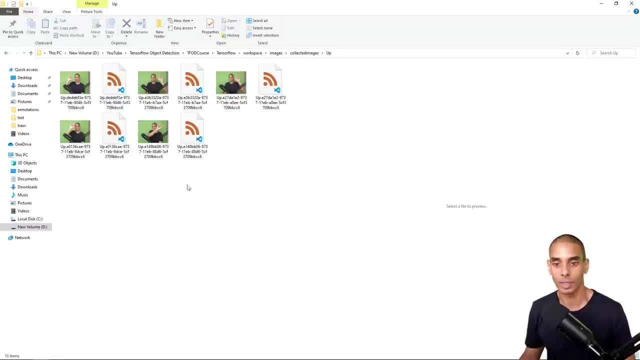 an experiment. you don't need to get it perfectly right the first time. it's more than okay if you play around and try different things out. Okay, so we've got our images there. what we want to do now is go and grab the rest. 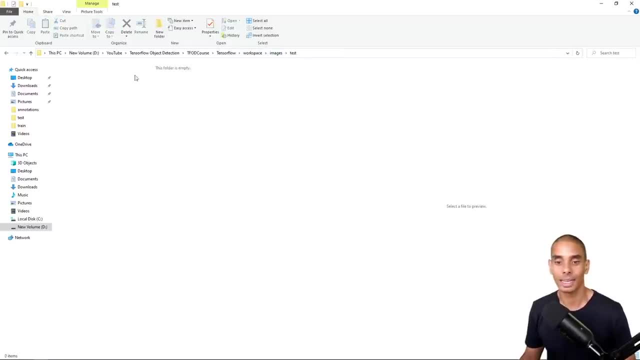 and throw it inside of test. so we're going to have one image per class in our test folder. I'm just going to keep doing this and again, this is just copying and pasting, right, so you could potentially automate this if you use the OS library and just randomly choose. 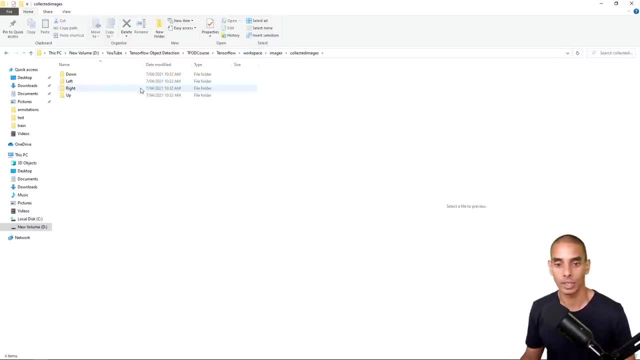 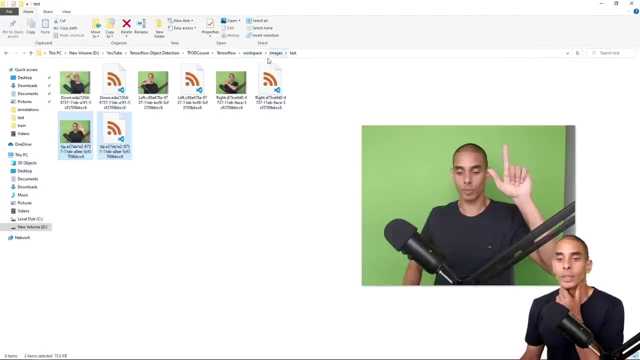 which files to place into train and test. but in this case I just find it easier to do it manually, because then I've got a little bit more control over it. Okay, so where are we? so we've now got our images inside of test. so we've got. 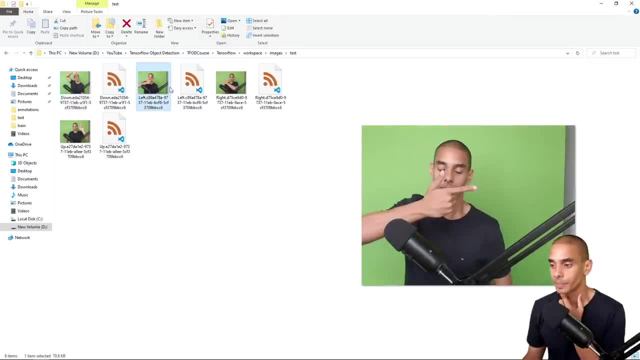 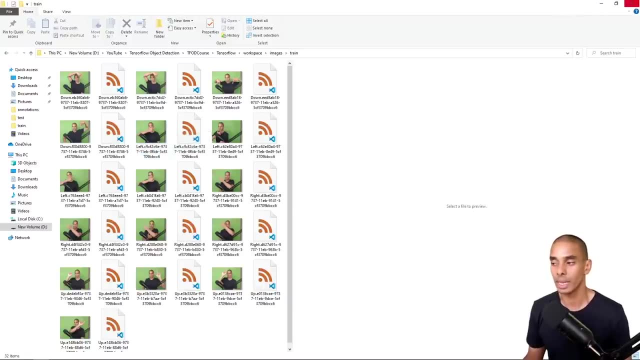 four images, so left, so down. what is that? left, right and up and again inside of train. we've got a whole heap more. we're going to go through our standard process now. so we're going to go through back into our training folder and again we are going to. 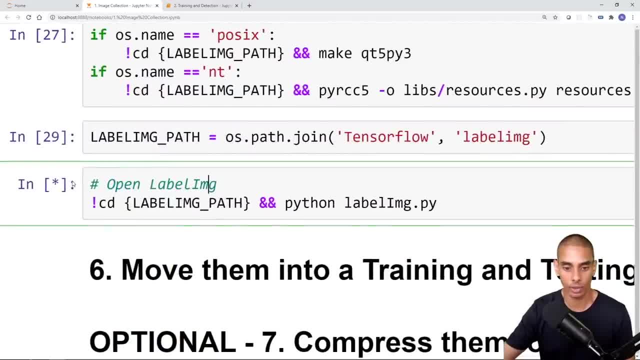 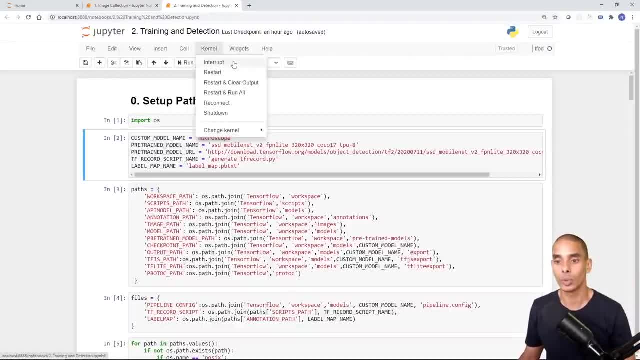 stop label image, because you can see it's still running up there and we've got our little star, so we can stop that, Jump into our training and detection folder and what we'll do is we'll just re. we can actually. 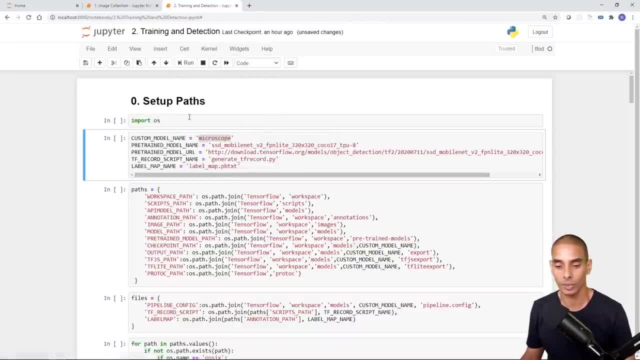 just clear all of our stuff here so we can make sure that we are importing. so we're going to import our operating system. we're going to change our folder name, so we're going to call this one directions and then so this will effectively. so remember we had our my ssd mobnet folder. 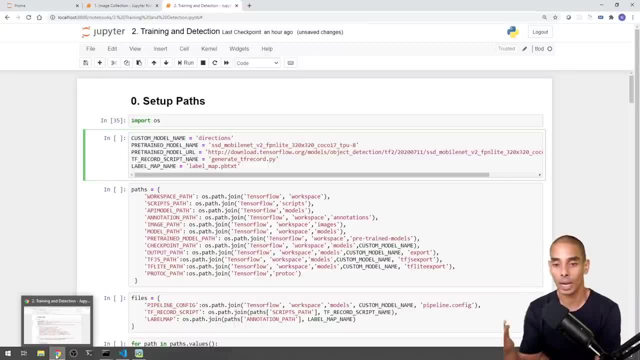 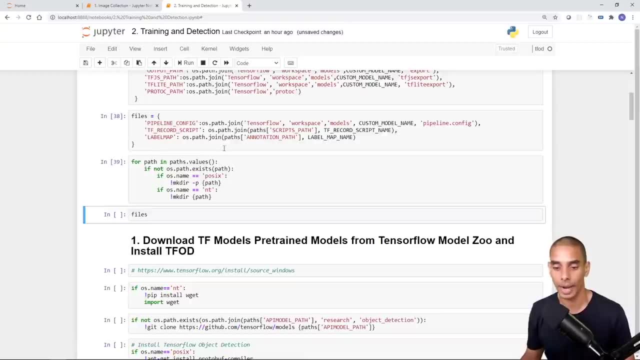 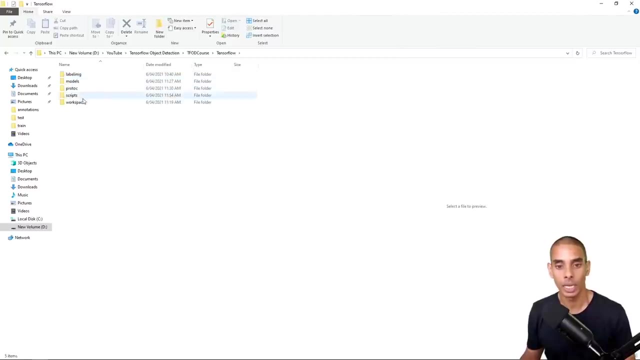 my, my ssd mobnet tune folder. we also had our microscope folder. now we're going to have one called directions. so if we run this and run this and this and this, this should create our new file paths. go into youtube. tense flow object detection- tfod- tense flow workspace where i have models. 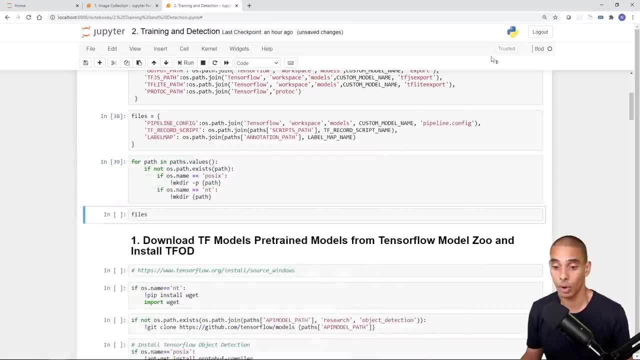 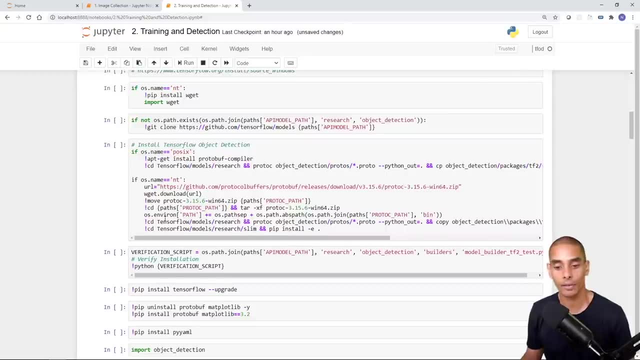 you can see, we've now got a folder called directions, and this is going to be the current model that we build, and then again we can skip step one because we've already set up our environment. we are in our virtual environment already, so we don't need to do anything. 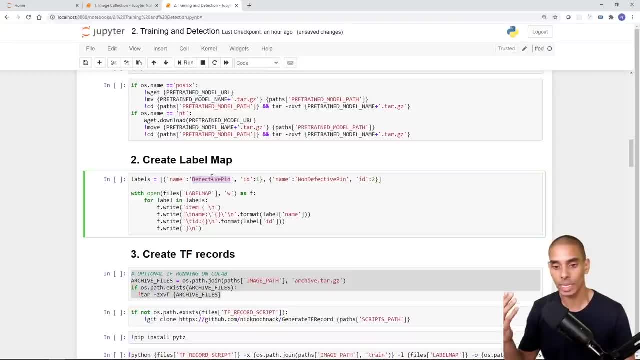 magic there. what we do need to do, as per usual, is update our environment. so we're going to do update our label map. so remember, we had left right, up and down and they were all capitalized. so we're going to create those new labels, so left right, and then we'll create two new items. 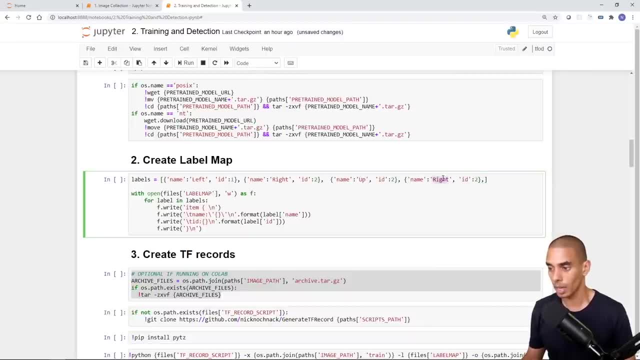 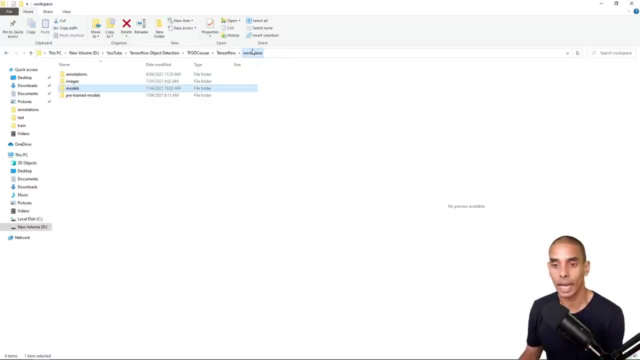 up and down and again, just double check. you need to make sure these unique, these ids, are unique as well. so this should be three and four- another good thing to know. so let me just quickly show you. so, again, we want to check out images, so make sure that we've got the right case. 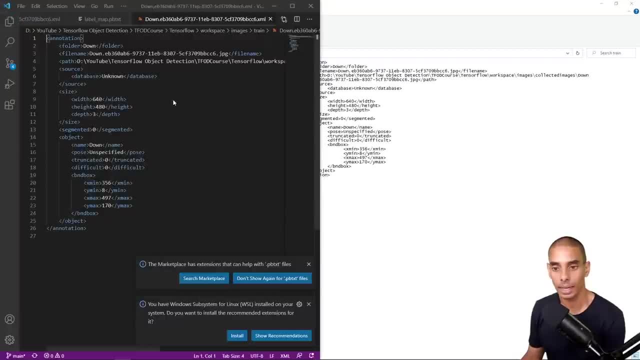 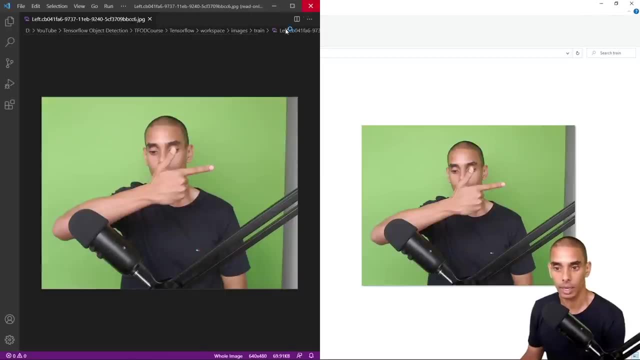 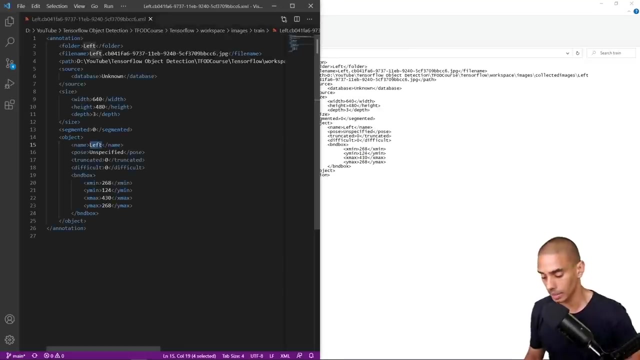 so if we go into train, let's take a look at down again, that's capitalized. let's look at left again. that's the actual image. again, left is capitalized here, so you can see that let's do right. so i'm just double checking. 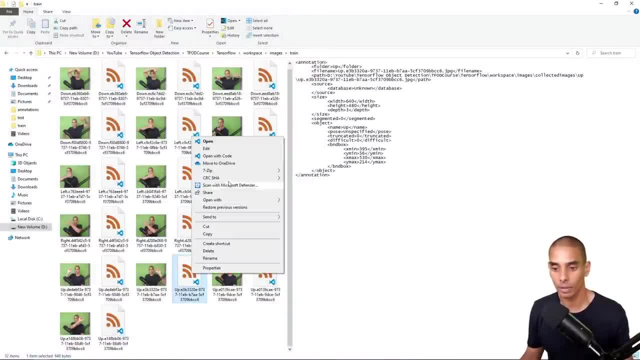 because obviously checking up front is going to save you a lot of time down the track when you're trying to debug errors if they do come up, and up is capitalized as well. so we're good, there we are good. 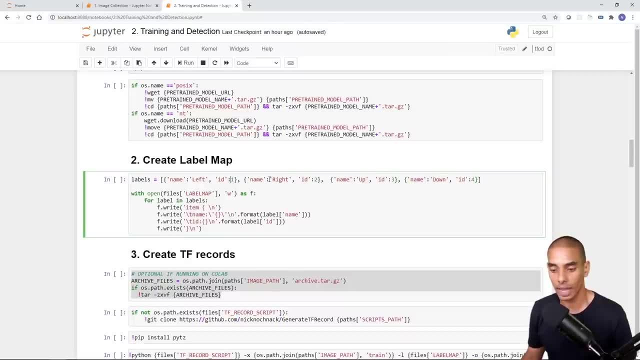 so we've got left right, up and down. we've got unique identifiers for each one of them. so one, two, three and four. i think we're good to go. so let's go and run this annotation. 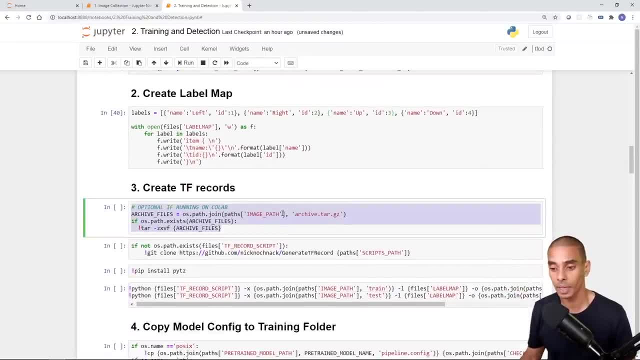 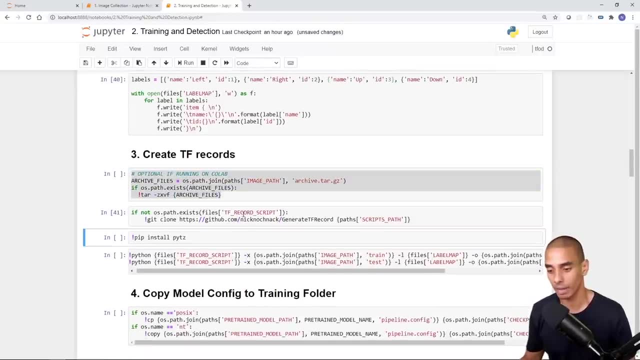 which is fine. so that's going to update our label map, create our tf records. so again we can skip this cell because it's only for colab, so we can import our new generate tf record script again. we've got it already, so it's going to skip it. we already had pyTZ installed. 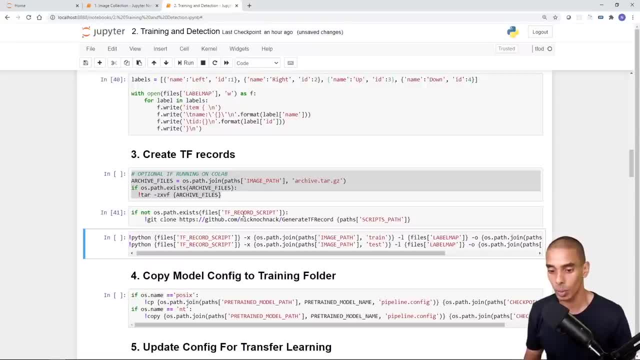 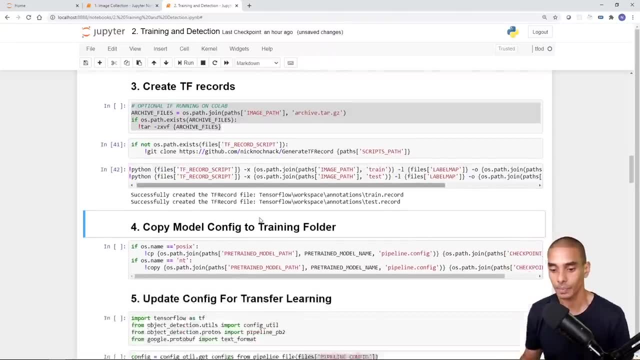 so we can actually delete that cell. we don't need that anymore and then we can run our tf record generations again. ideally this should successfully create our train record and our test record. we're going to copy our model config to our custom folder again, which will go into our 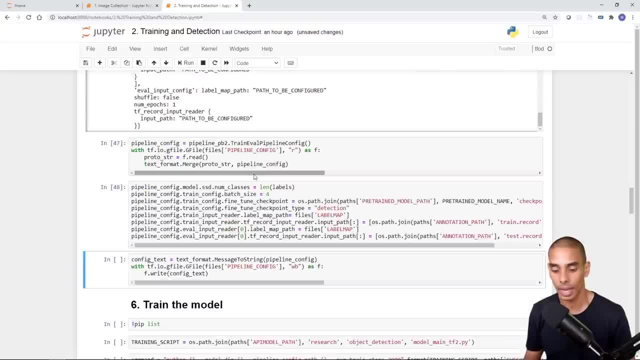 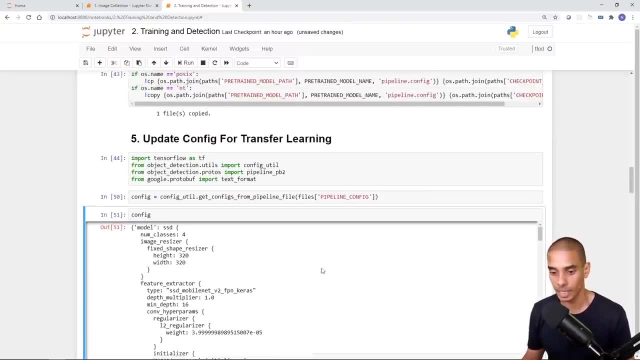 directions folder and then we're going to go on ahead and update our config. so if we re-import it in this cell, you can see that in fact we've gone and updated. it looks like we've got. the number of classes equals to four. 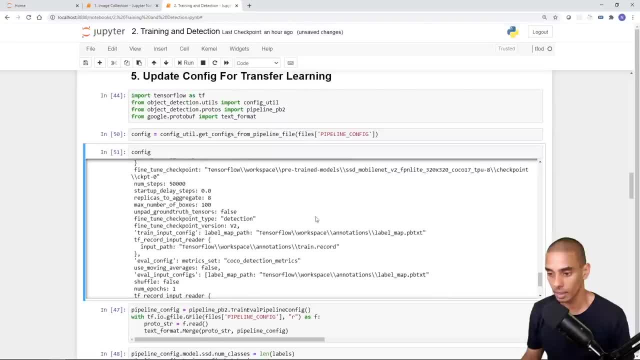 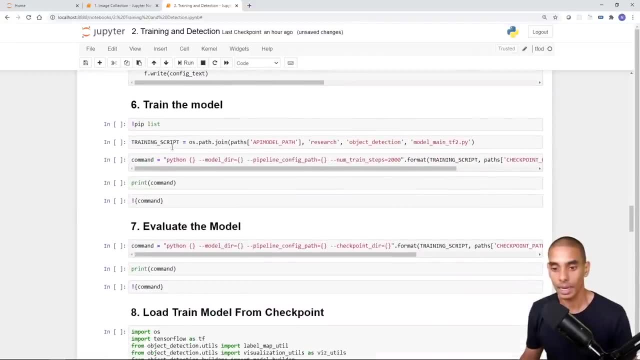 so again, this is updated. if we scroll on down, again we are picking up our correct folders. this is all looking good. okay, so again now, what we're going to do is train our model. so we're going to run our command to generate our training script. again, print it out. we're going 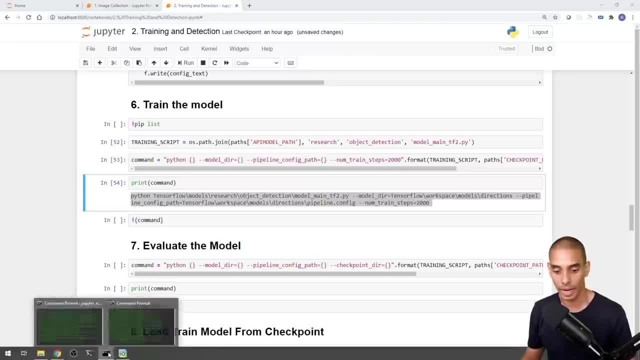 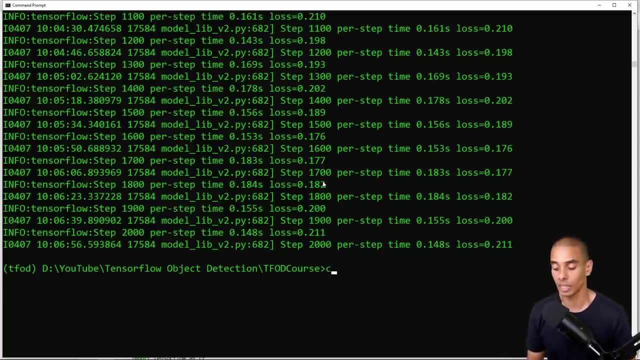 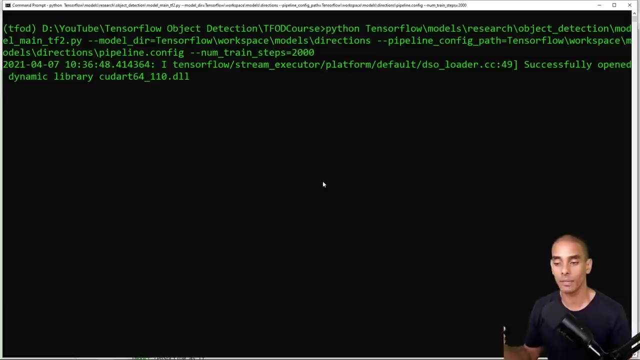 to copy this. we are going to create a new command prompt and again, we've already got this one, or is this from the defective, non-defective pin example or project and we're going to run our training code. so if we paste that in this should kick things off and it should kick off our. 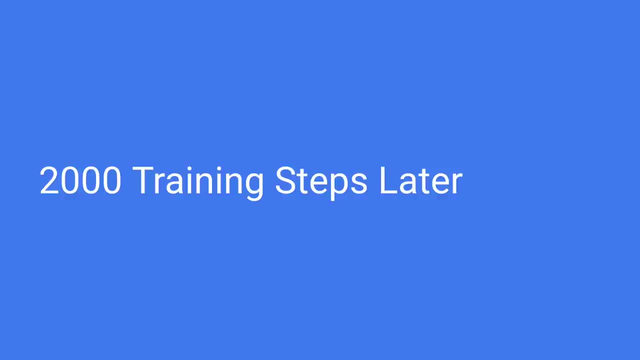 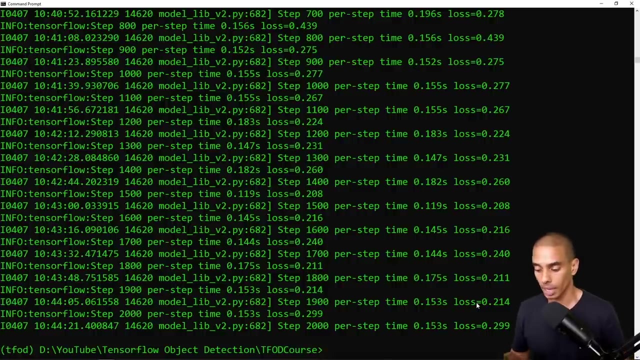 training. so, again, we'll be right back as soon as this is done. okay, so that is our model train. so this is our directions model and eventually what we're going to be plugging into our web app. so you can see, we went all the way up to step 2000,. and ended up with a loss of 0.299,. 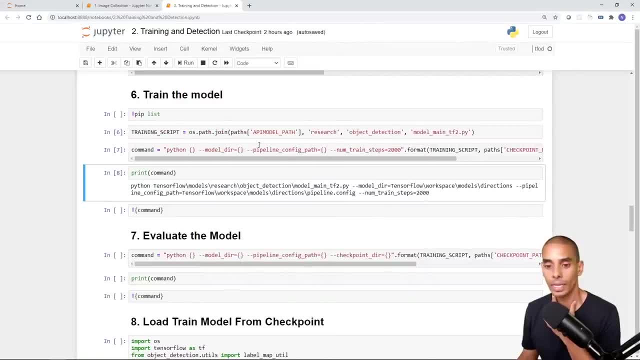 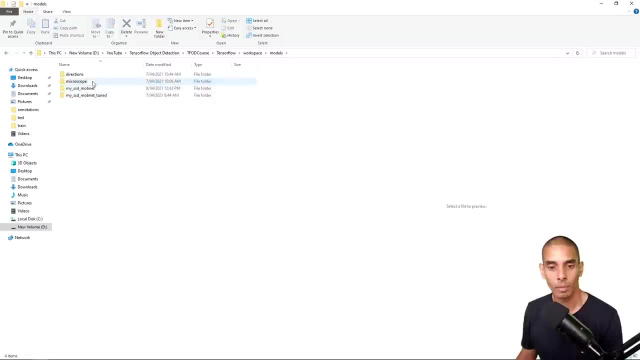 now what we'll do is we'll test this out inside of our Jupyter notebook, as per usual. so again, let's take a look at our checkpoint. so if we go into our workspace models and then directions, so you can see we're now up to checkpoint three. this is a key thing to take a look at, guys. so if 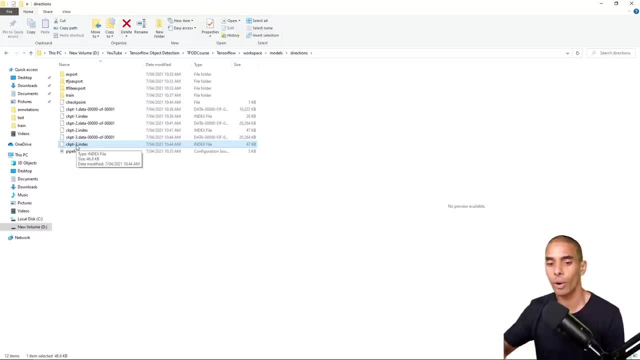 you're training your model, don't always assume you're going to be at checkpoint four after 2000 steps or checkpoint three. it could vary, so you always want to make sure you pull down the one that's going to be checkpoint three. so there's checkpoint one, two and three. so we want 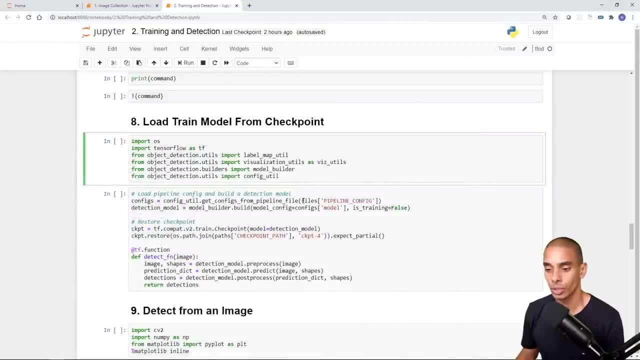 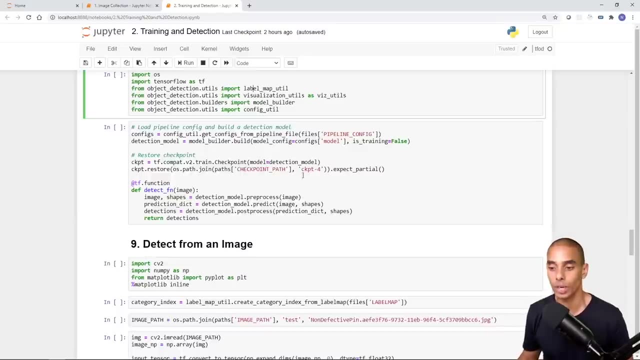 checkpoint three in this case. that's exactly what we're going to do. so remember for our what was it? our pin or defective pin detection, what we had, the latest model that we had was checkpoint four, so we updated it to that there, but what we're going to do is we're going to do. 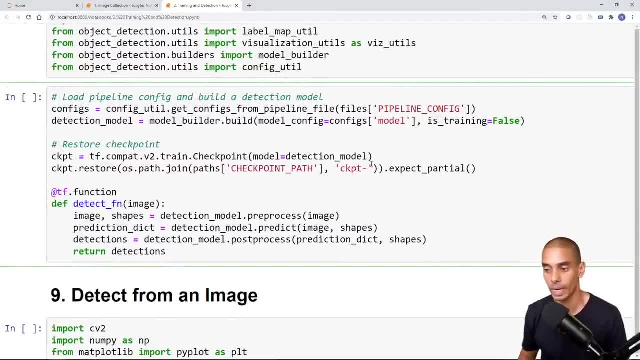 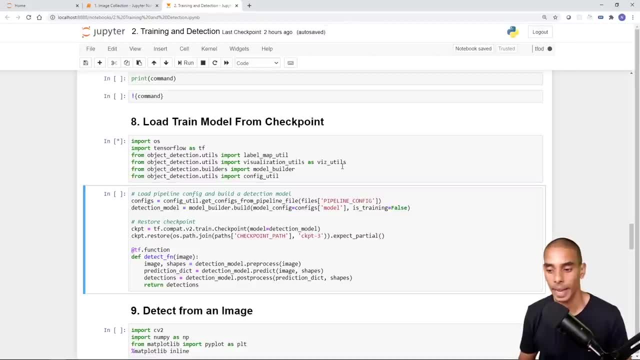 checkpointrestore and we're going to specifically pass through checkpoint three in this case, then what we'll do is we'll import this as per usual, so all of our dependencies for step eight, load up checkpoint three and again we're going to skip right through to real-time detections. 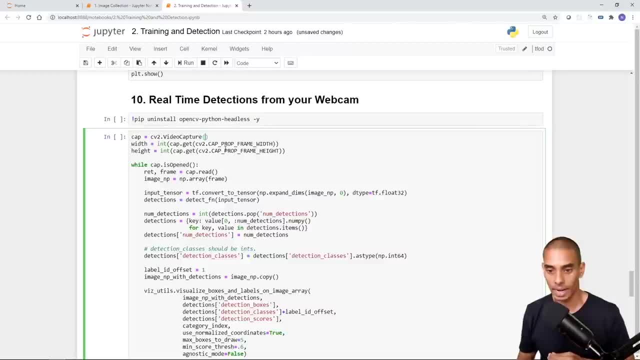 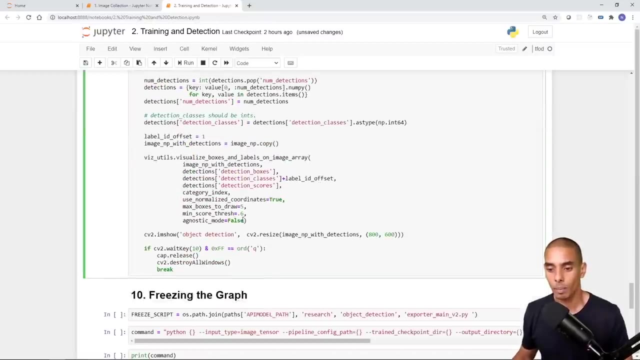 because that's my favorite. we're going to make sure that we set our video capture device back to zero because, remember, video capture device one was for our microscope, number zero was for our webcam, so let's try this out. so, in this case, I'm just going to hit run and we'll bump up our 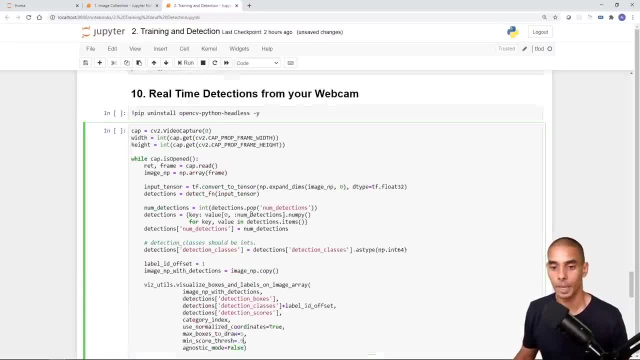 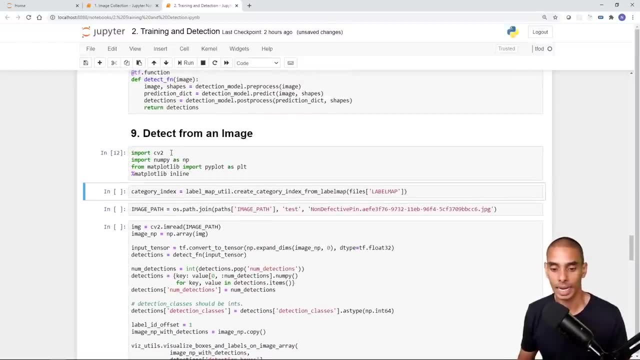 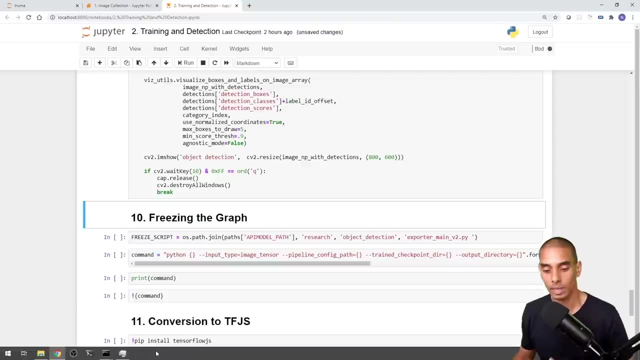 minimum score threshold back up to, let's say, 90% and give that a run. so let's run that. and we need to import CV2, which is part of this cell, and we're probably going to need our category index and we don't need that image path. so let's do that, let's see. hopefully we should get a. 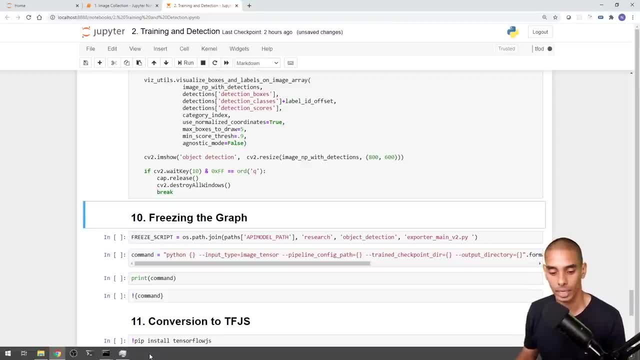 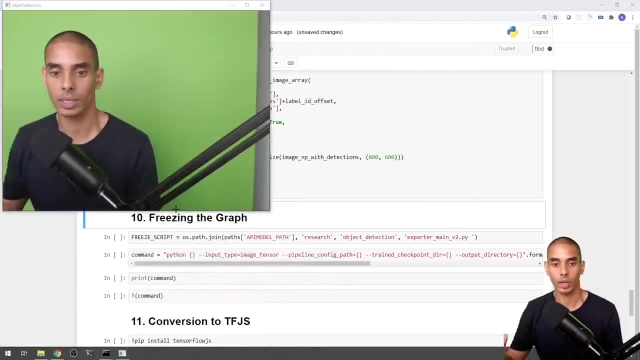 little pop-up and all things holding equal. we should get some real-time detections so I can see my webcam's just activated. so sometimes it takes a little bit of time to start and close task manager. okay, so that's open. 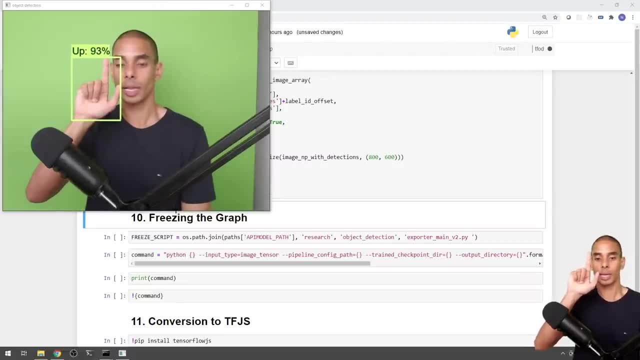 so up looks like it's detecting appropriately. down- looks like it only wanted: oh no, that's fine. so down. left: oh, that should be right. okay, so we've got an issue with left and right. 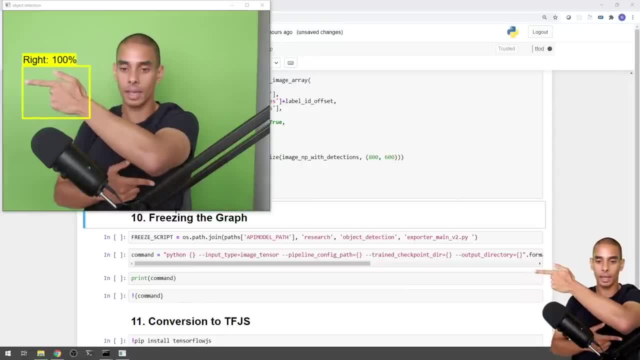 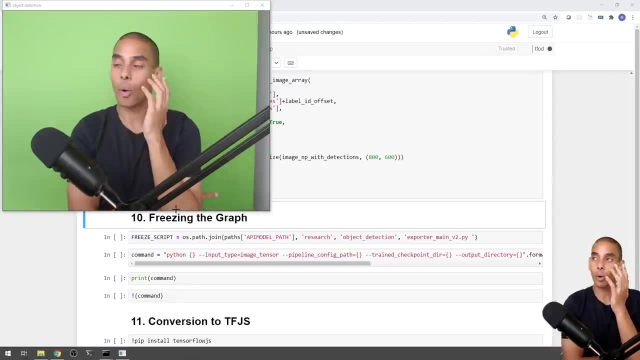 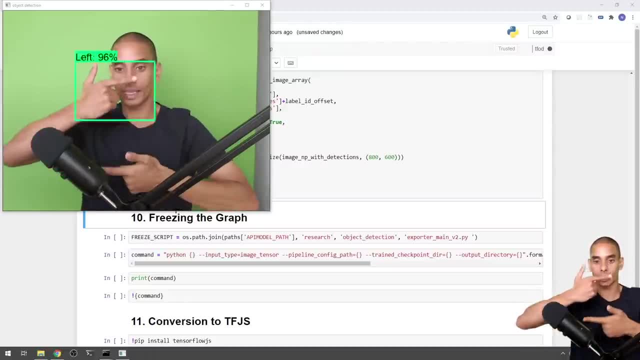 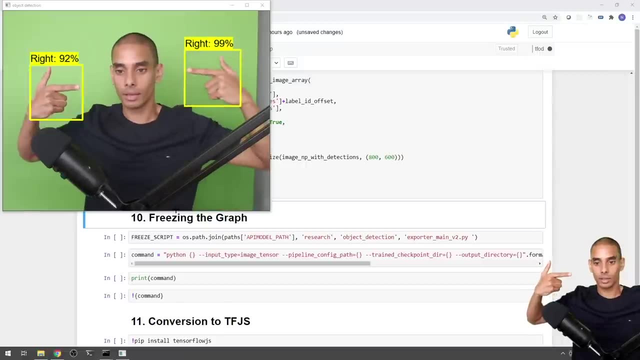 because right now it's saying that both left and right over my face is left, but if I put right over here in the green it's okay. so it's saying right as long as it's not on my face is going to be right now left over my face, okay, all right. so we might want to do a little. 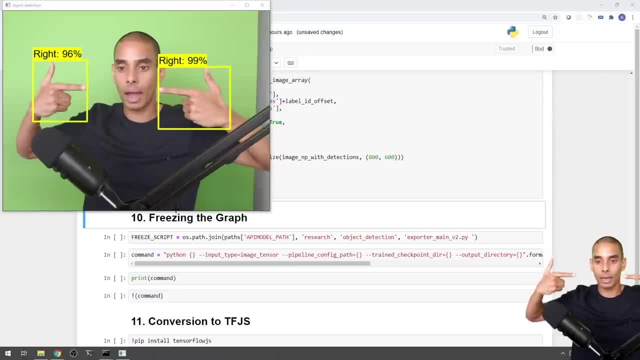 bit more performance tuning on there, but you can sort of see how you might go about building your detection model. so what I'd actually do in order to solve this is I'm going to do a little bit of this- is I'd include more images of me purely pointing what's this? this is left so in this. 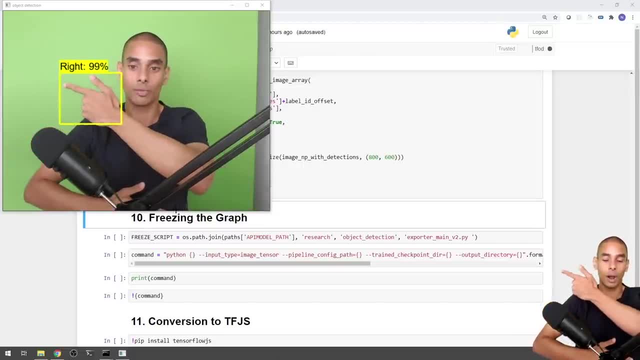 case that left is fine. left is okay. if I do it over my face and if I always did right over my shoulder, then I'd be okay. but in this case, if I did it like this, you can see it's maybe not. 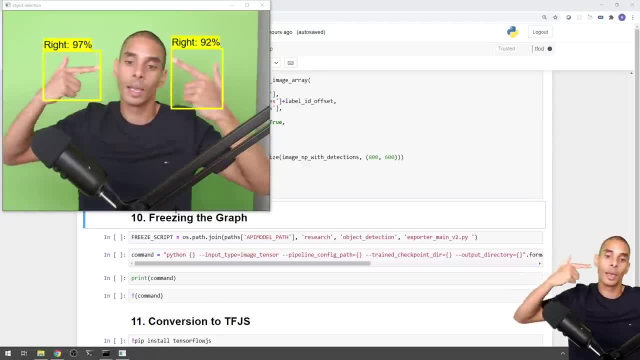 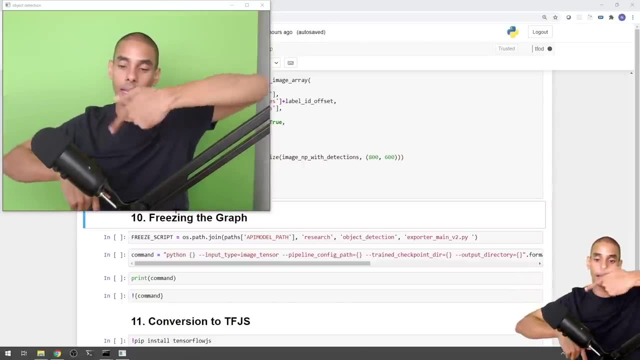 performing as well. but you sort of get the idea right so you can go and performance tune this, make it better, improve that model accuracy. so we've got up working fine, down working fine. we can do it that other hand okay. so other hand we might need to add in a little bit more. 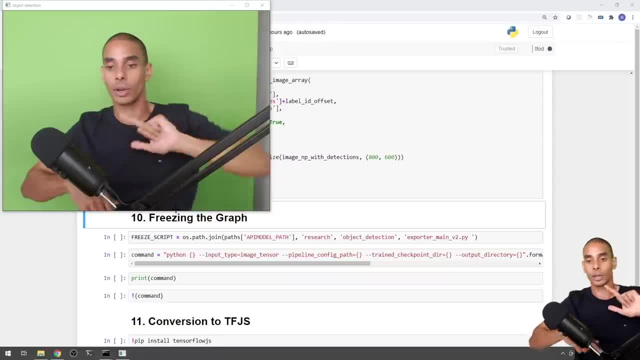 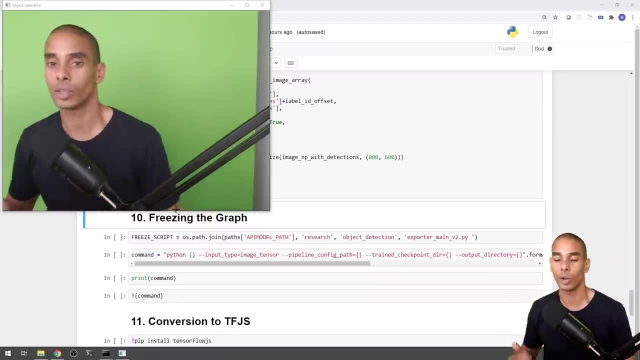 tuning there. so up is okay, down with that hand is not okay, but you can start to see. this is how you might evaluate your model, and you'd add in additional images of the particular classes that aren't performing so well. so that's sort of how you go about that performance tuning. 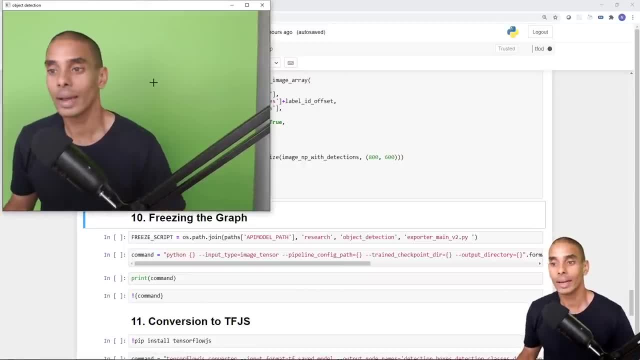 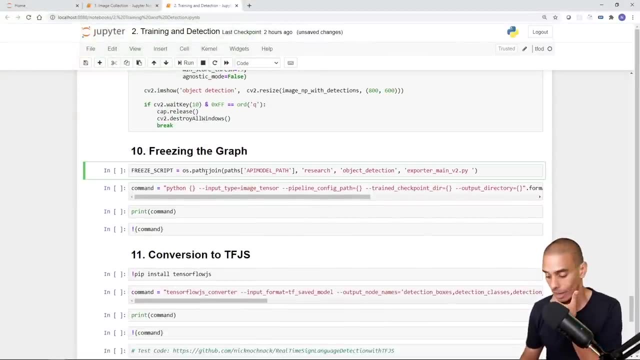 but it doesn't stop there for this particular model. we are going to take this one step further. so I'm going to quit out of this particular detection and we are going to freeze our graph this time. so we're going to run through step 10, and freeze our graph. 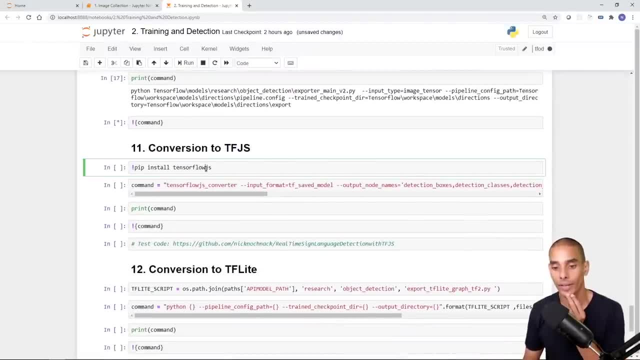 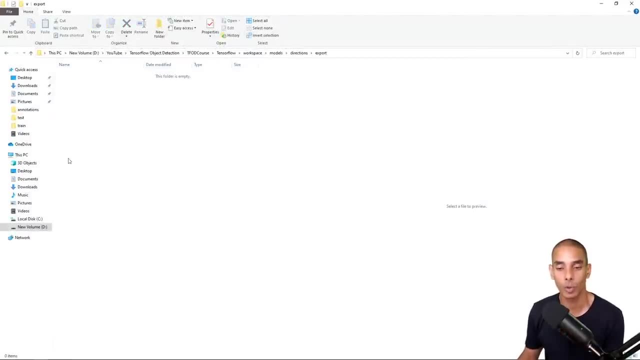 and so we'll go ahead and run through step 10, and we're going to run through step 10,, run that, and we're also going to run through everything in step 11, and convert to TensorFlowjs as well. so this should do two things. so inside of our export, once our frozen graph is done, 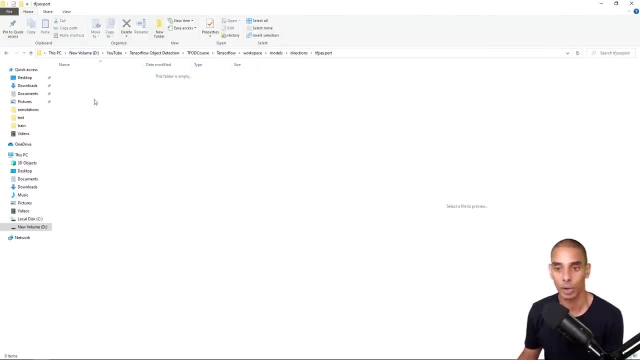 we'll get an export here, and then we'll also get a TensorFlowjs export, and then what we're going to do is we're actually going to build up this app. so to do that, we've got to do a couple of. 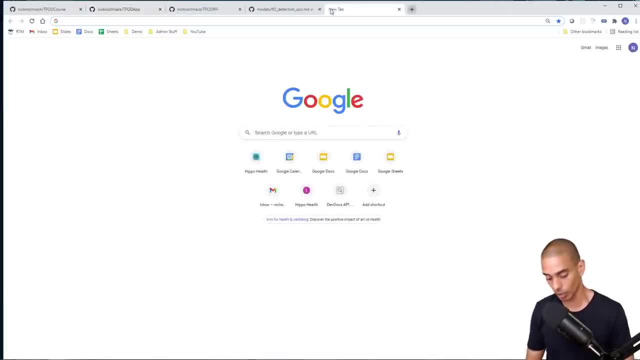 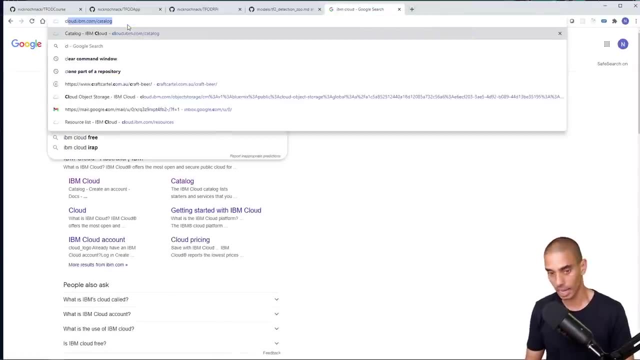 key things. so, namely, what we need to do is go to IBM Cloud. in this case, we're using IBM Cloud to host our model and we specifically want to go to cloudibmcom forward slash catalog. what we need is cloud object store. 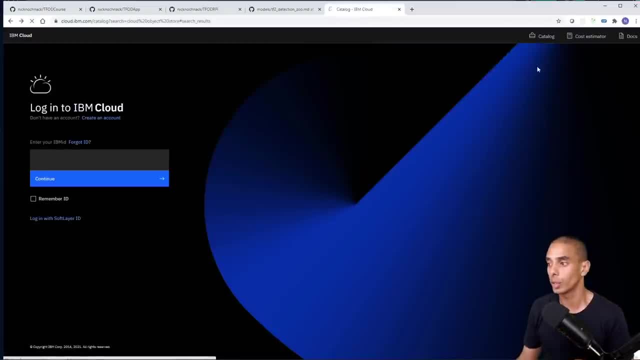 and so I'm just going to log in. so what you'll need to do is, if you're doing this for the first time, you'll either need to log in or sign up. so sign up if you haven't signed up before. 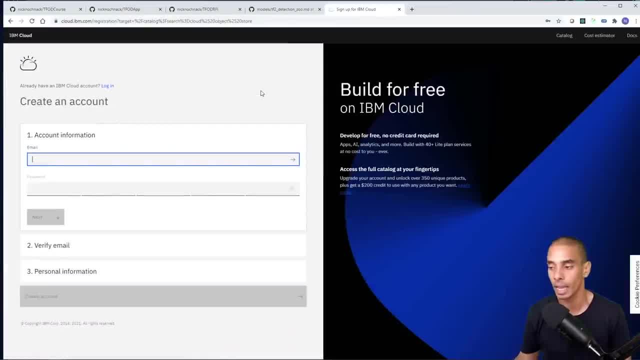 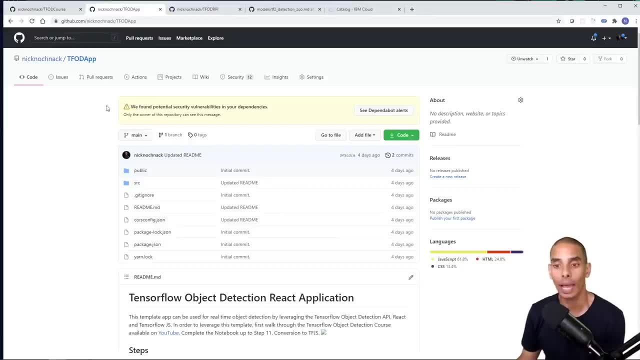 and you can just plug in your details and, again, this is all free, so you can run this for free at the moment, based on your model. so what I'm going to do is I'm going to log in and, if you actually take a look at the steps inside of the GitHub repository, so githubcom. 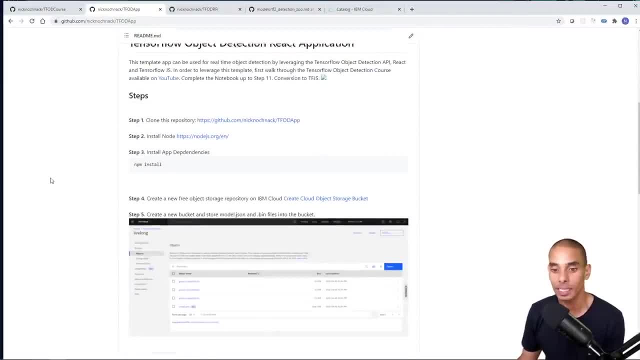 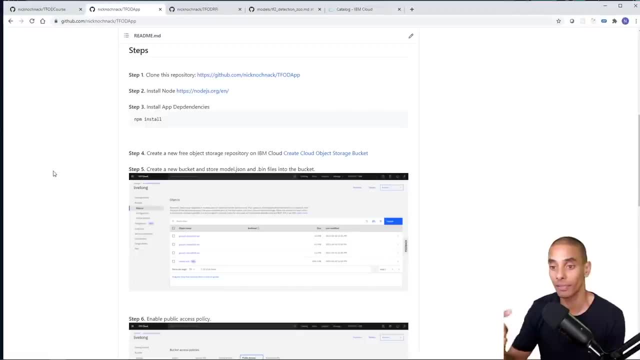 forward slash nickknockknack. forward slash tfodapp. this is actually going to walk you through each of these steps, so if you maybe get a little bit lost as to where I'm going through, then by all means do check that out. but effectively, we're going to be following the steps that you can see. 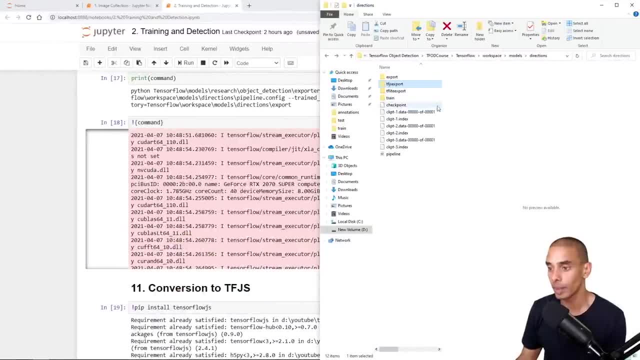 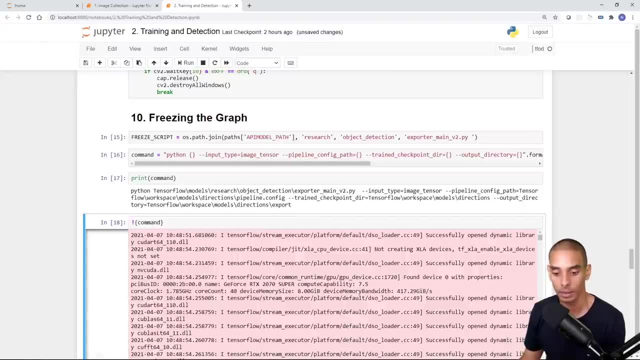 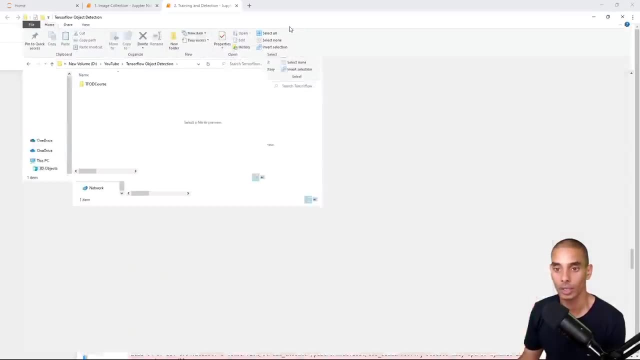 there, Okay. so let's actually do this one step at a time. so let's make sure that our exports work. so it looks like our frozen graph has been generated. so let's take a look at that. so if we go to YouTube, TensorFlow object detection- tfod course- TensorFlow workspace. 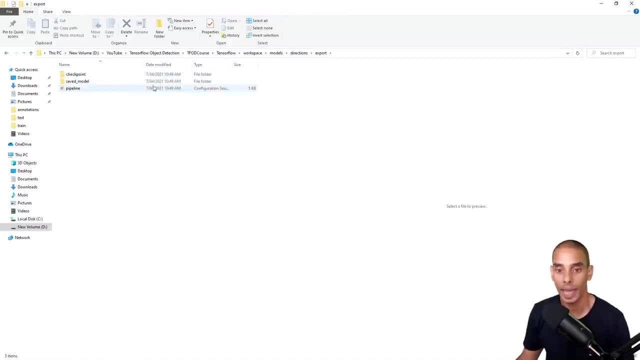 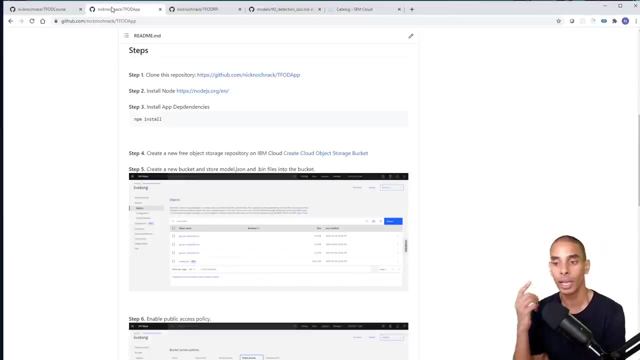 models and we look at directions. inside of export, we've now got our frozen graph and if we take a look at tfjs export, we've got that done as well, so we are in good shape. Now let's go back to our TensorFlow object detection app component and see what we need to do. 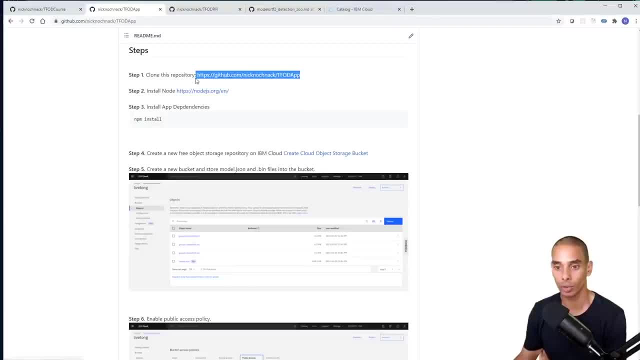 so, first up, what it's saying is: we need to clone this repository, so let's go on ahead and do that, and so if we copy this link here and again, the link to this, all of this stuff, is going to be. 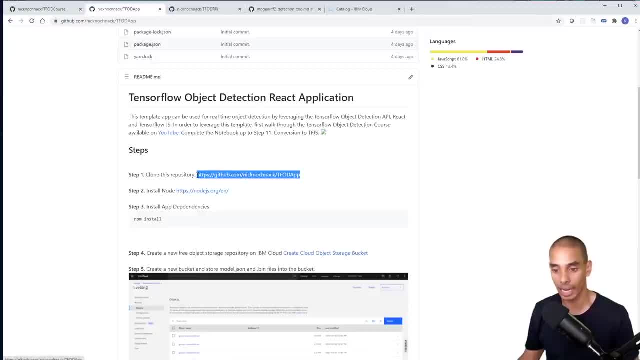 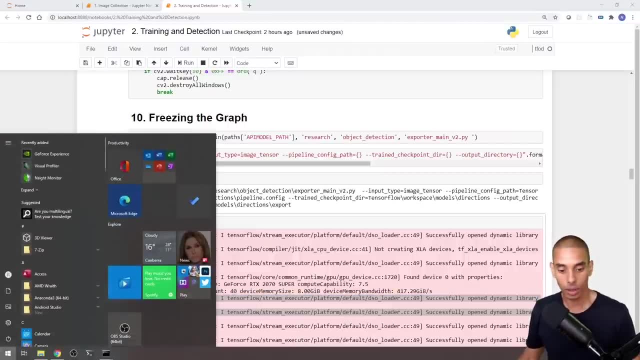 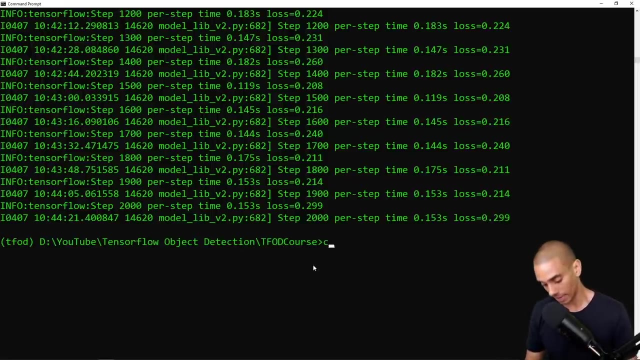 available in the description below. so by all means, do check it out there, and if you need anything else, by all means hit me up in the comments. so we are going to open up our new command prompt, and what I'm going to do now is I'm going to cd out of my tfod, course. 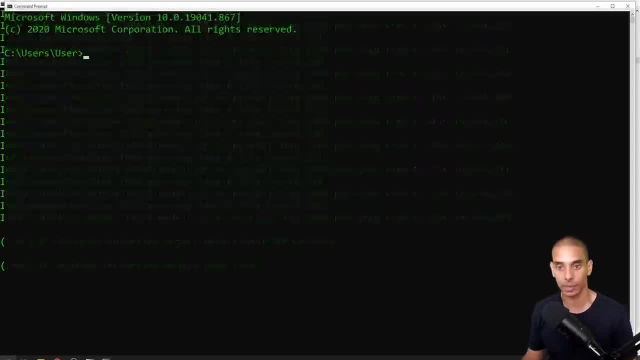 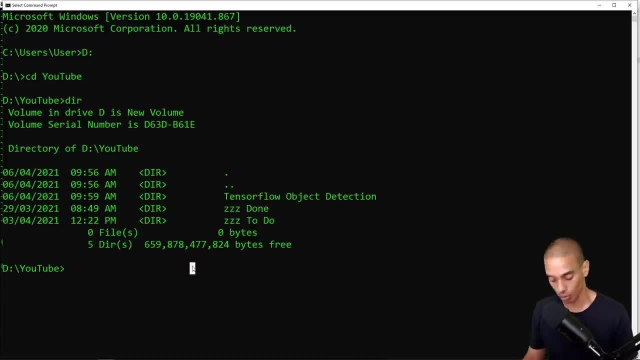 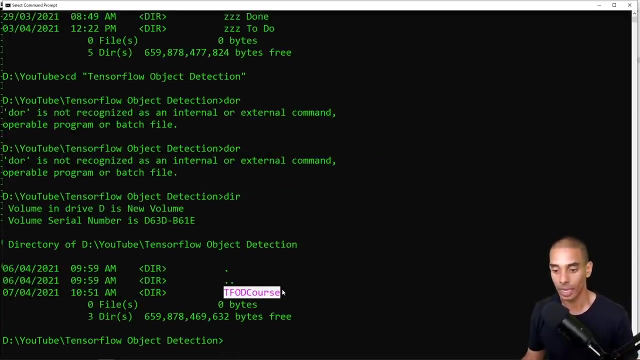 actually we should just probably create a new command prompt for this. so we're going to go into d drive, cd, YouTube, go into our TensorFlow object detection repository. typing is a bit of a shocker. all right, so we're in. so inside of that folder we've got TensorFlow. 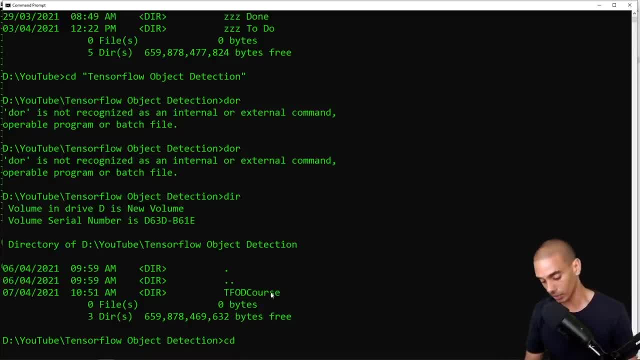 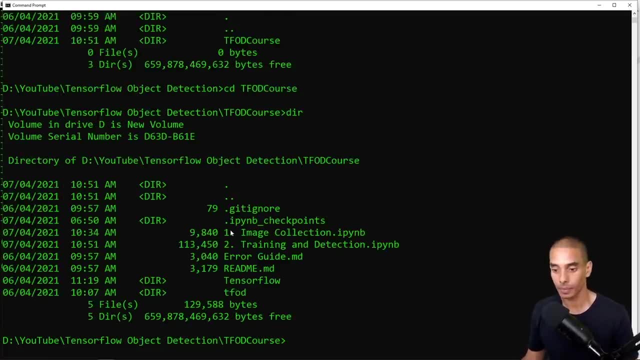 object detection course and then if we go into that TensorFlow object detection course, that's our root repository for where we've been doing everything so far. so you can see if I type in deer. if you're working on a Linux, I'm typing in deer, it's going to be ls if you're on a Linux. 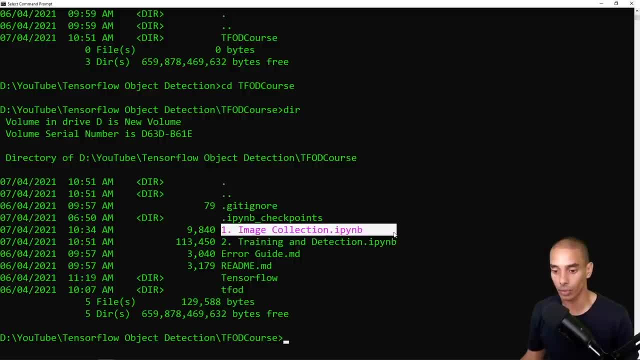 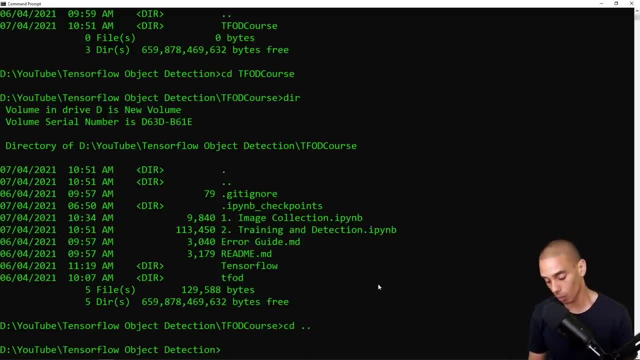 machine. so that's all of our baseline root dependency. so image collection and our training and detection Jupyter notebook is in there. so we're going to jump back out of that and what we're going to do is we're going to clone that repository that we were just looking at. so 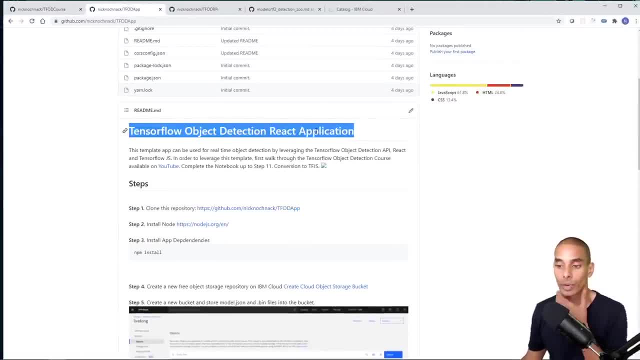 this one over here which is the TensorFlow object detection react app. so this is using a JavaScript web development library called react, or web development architecture called react, and it's just a really good, pretty sort of stable library. it looks really similar to HTML. so if 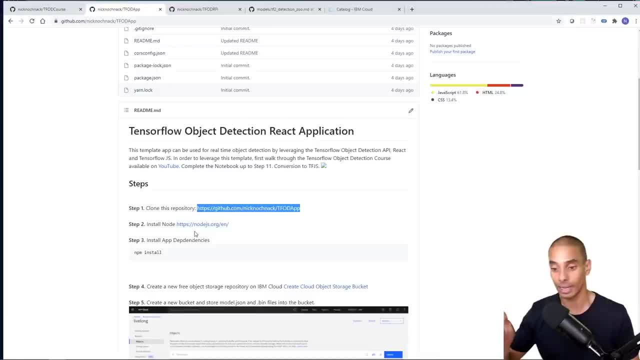 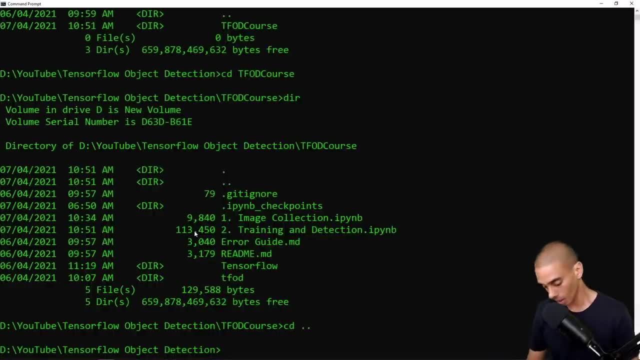 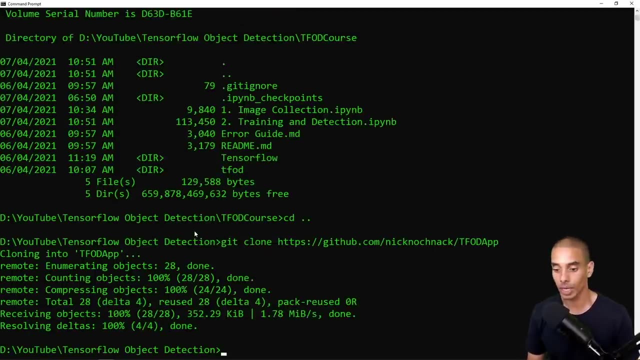 you've ever done any HTML, but you don't actually need to write anything. that's the beauty of this. so I've pre-written it all. you should be able to pick it up and go. so I'm going to clone this repository. what we'll do is type in git clone, clone that. and then what I'm going to do is I'm. 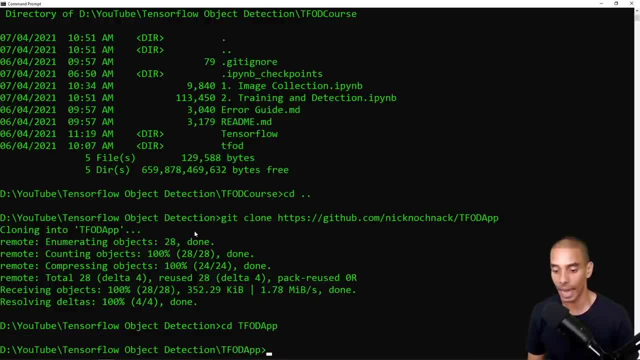 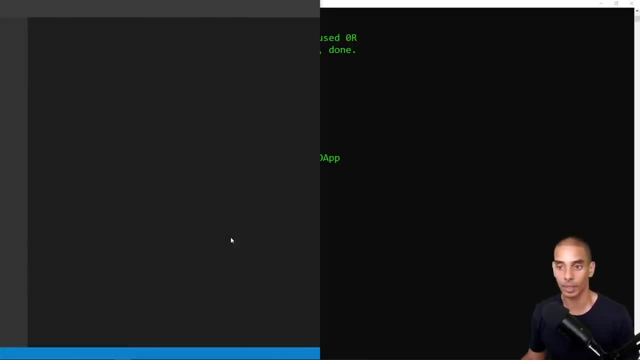 going to go into that folder, so cd, and it's going to be called tfod app and then let's take a look at that. so we've got all of our stuff there, and then what we'll do is we'll open this up inside of a code editor. so I'm going to open it up in. 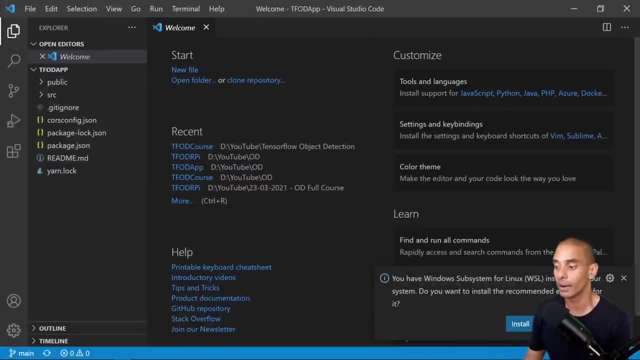 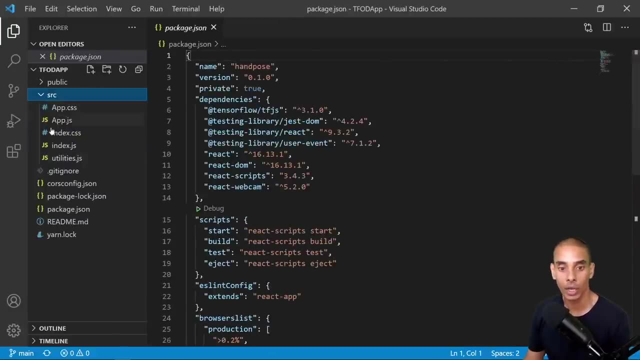 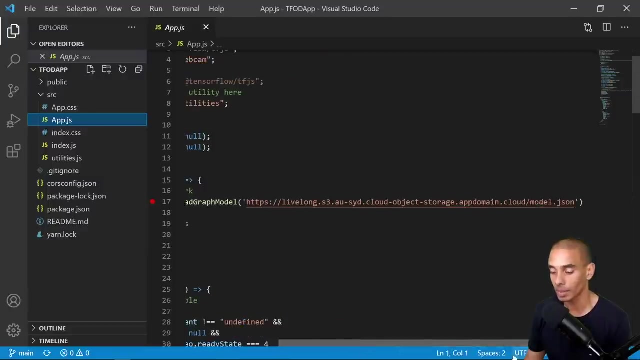 VS code. so inside of here there is a bunch of stuff that you can take a look at. so there's cause config. more on that later packagejson. you don't really need to worry about too much of this apart from this line here inside of the appjs file. but I will come to that and sort of. 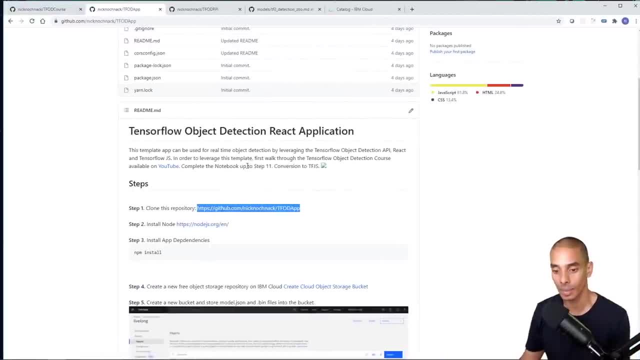 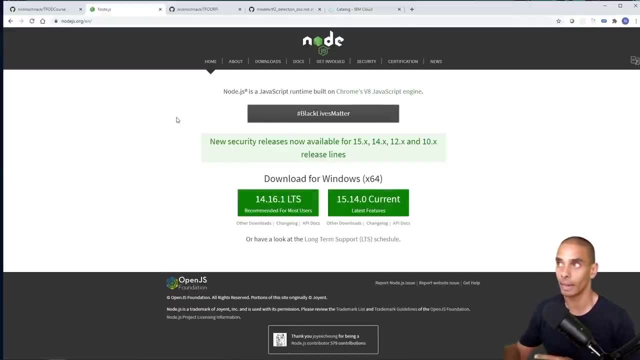 explain what we need to do. so let's go back to our walkthrough steps and do that. the next thing that we need to do is install node, so nodejs. so we're going to go back to our walkthrough steps and we're going to install nodejs. so if you haven't got this installed, just go to nodejsorg. 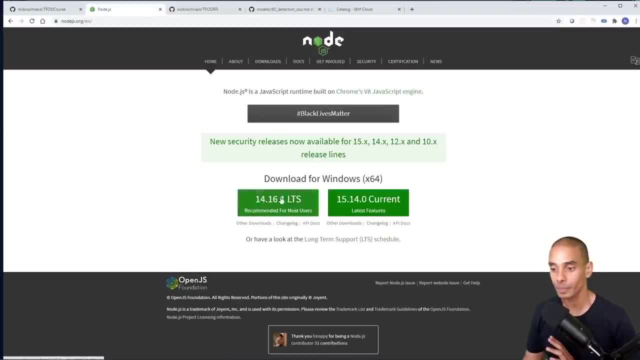 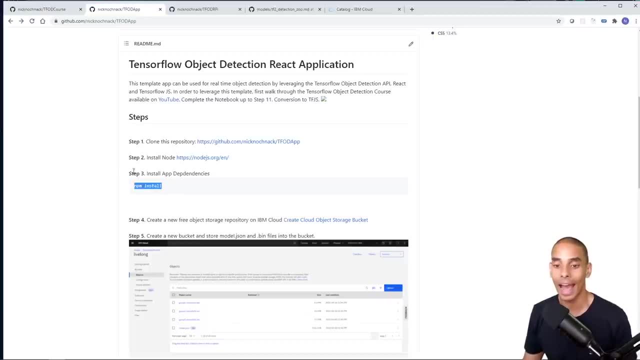 and again, the link is available inside of the GitHub repo. download it and install it, and you should be good to go. then the next thing that we want to do is install our app dependency. so under step three, we're going to go on ahead and do that. so if we go back, what I'm going to 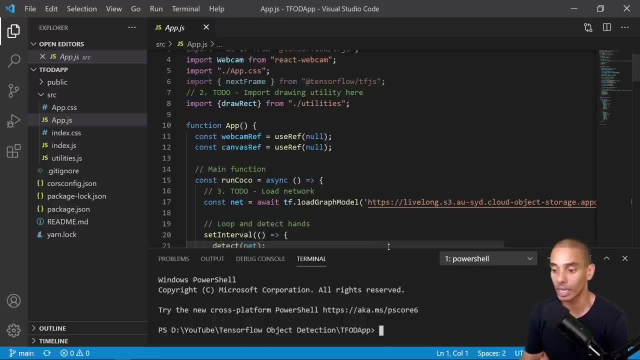 do is install nodejs, and then we're going to go ahead and do that. so if we go back, what I'm I'm just going to open up a new terminal inside of VS code, and what we're going to do here is we: 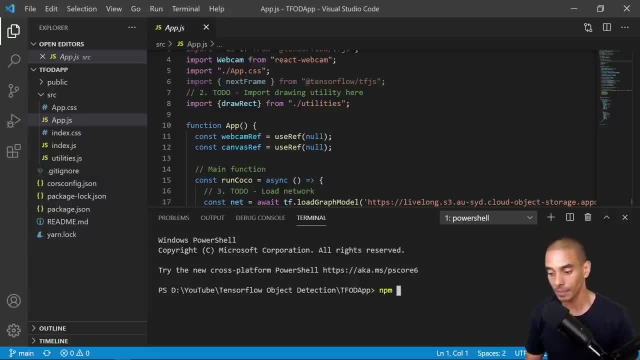 are going to type in the following command: so npm install. so think of npm as the package manager or the equivalent of pip, but for javascript in this case there's a bunch of others or resource managers, but in this case we're going to be using npm. so an npm comes when you install node, so keep that. 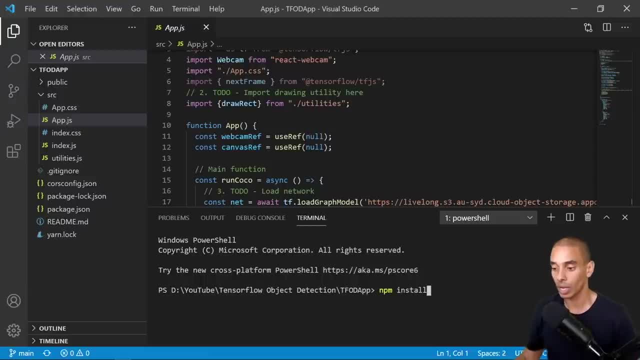 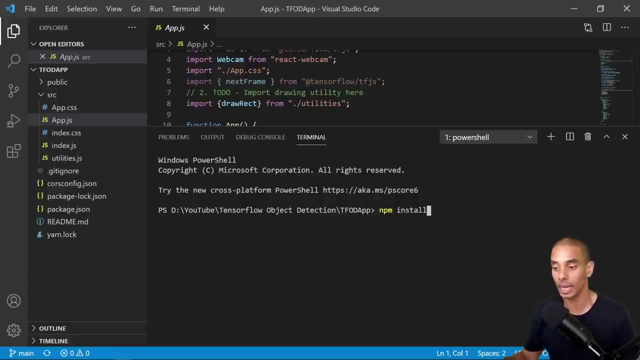 in mind. you need to have node installed in order for this to work. so we're going to type in npm install- and I'm just going to bring that up just to make sure my head isn't covering it- and hit enter. so this is going to install all of the dependencies for our react app that we're. 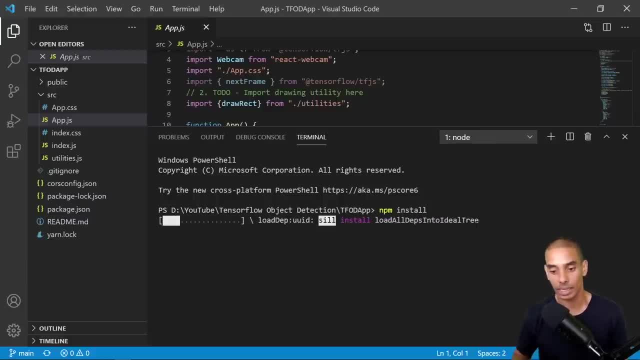 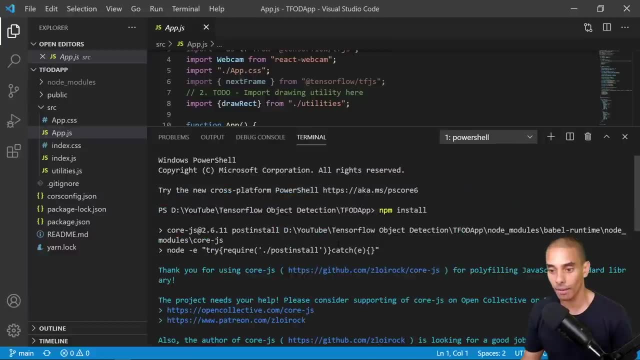 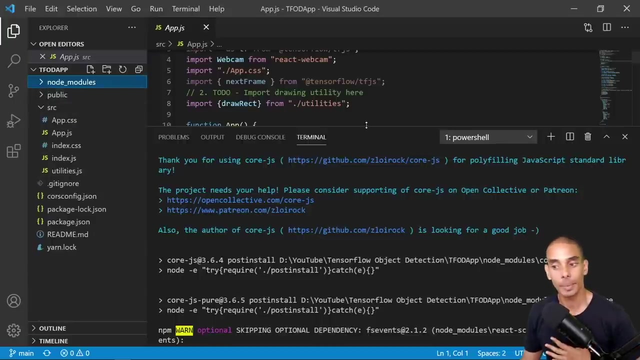 going to need, and this might take a little while. so let's let that run and then we'll be right back. okay, so those look like all of our dependencies are now installed and you can tell based on the fact that we've now got this node modules file. now this is going to be using tensorflowjs in. 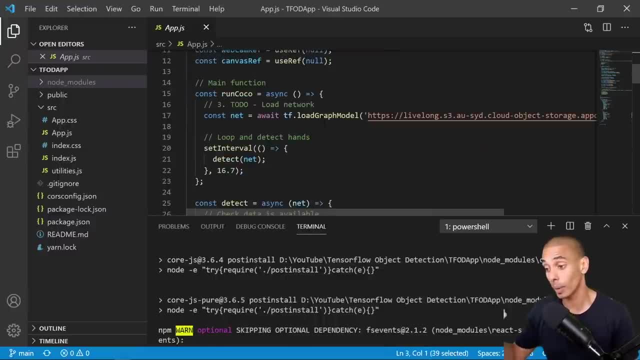 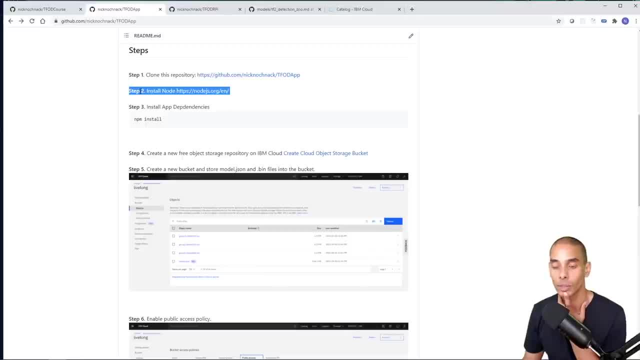 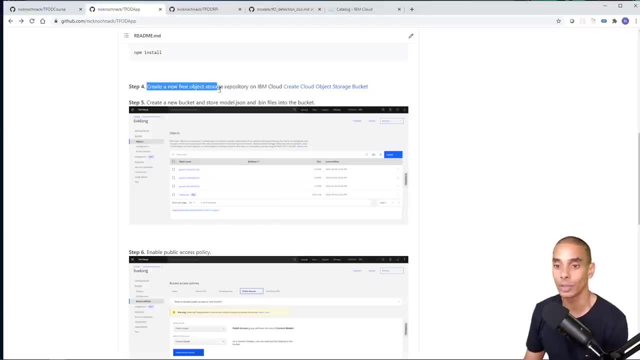 so in this case we've done steps one. we've cloned the repo, we've installed node. I've already got it installed, but again, I'm showing you sort of where to go to do that. the next thing that we need to do is actually create a new free object storage repository on ibm cloud. so to do that we're 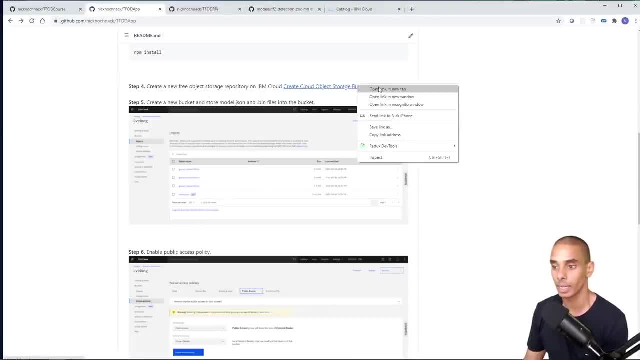 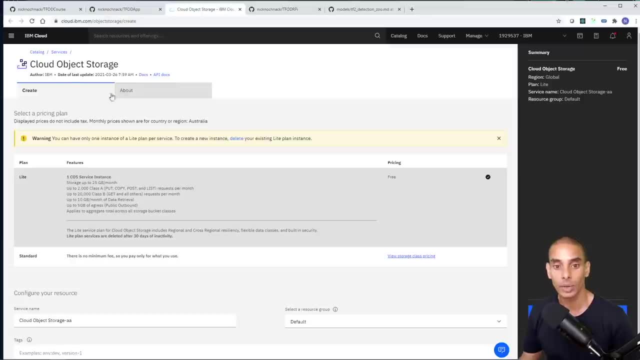 going to hit this link. we should do this in a separate link, so we'll open a new tab and again, this is that, that place that I was sort of referring you to. so in this case, we can create a new cloud object storage and just hit light and then hit. 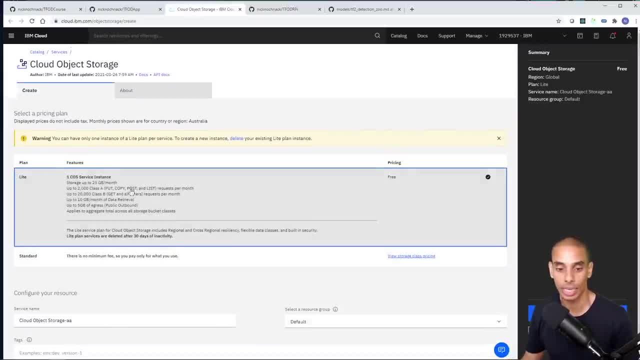 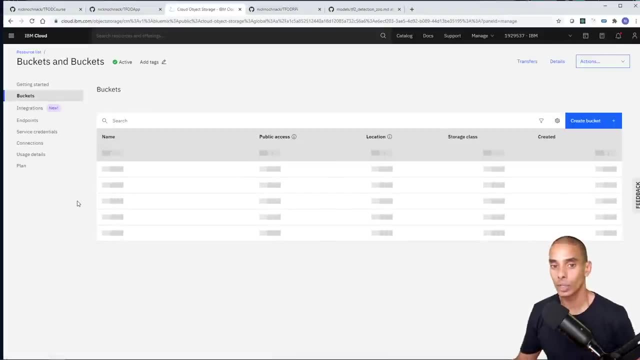 create. in this case, I've already got one created, so all you need to do is hit light and then hit create down here, and then what you can do is you can go and ahead and open it up. so if I go and open up my instance, I'll show you what it looks like. so once you've got your cloud object storage, 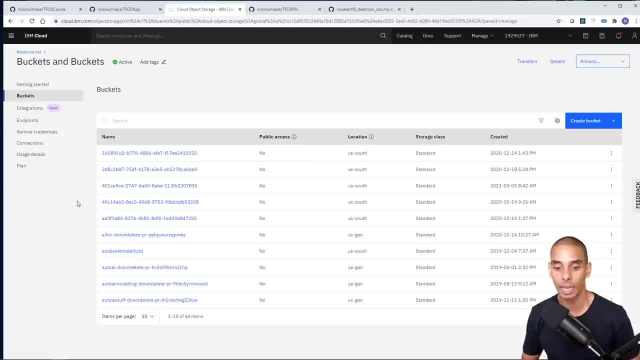 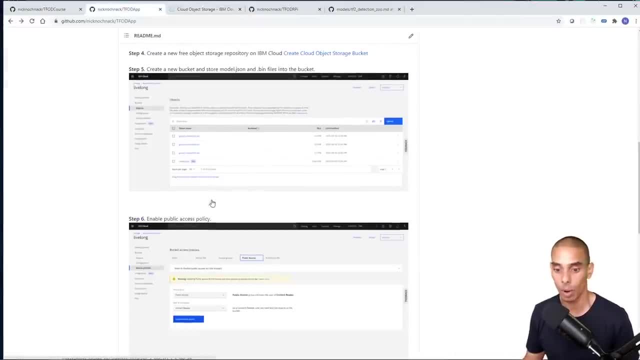 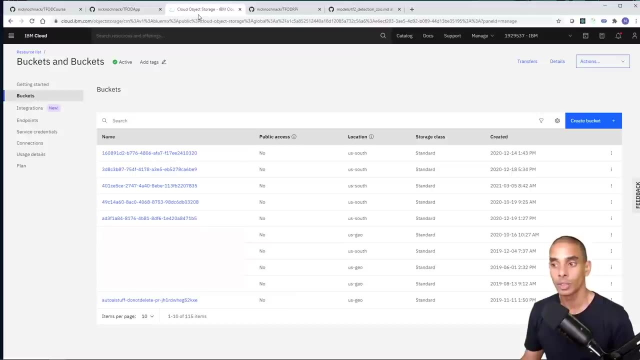 repository made available. it's going to look a little bit like this: now, what you want to do- is you want to do from here- is create a bucket, so to do that, which is effectively what we are doing in step five. so assume we've already gone and created that cloud object storage bucket, so what? 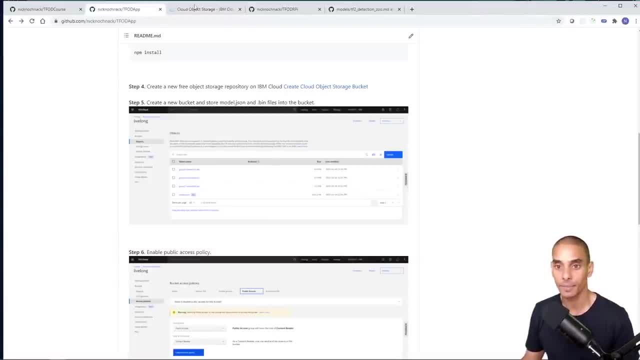 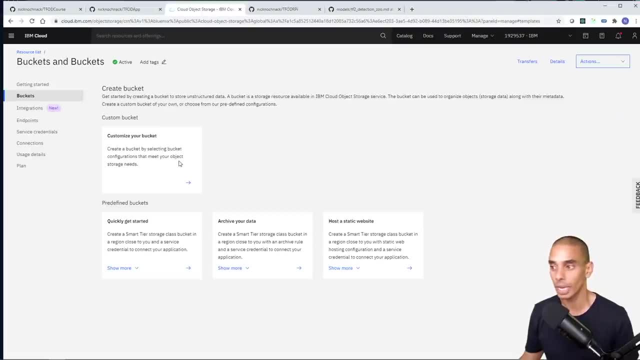 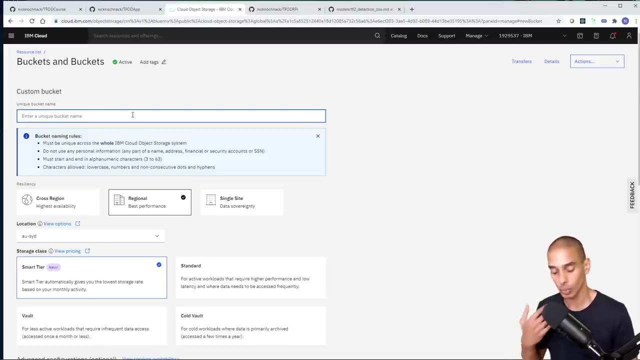 we'll do is we'll create a bucket now, which is step five. so we'll hit create a bucket or create bucket, and then what we're going to do is just hit. I think we're going to hit customize your bucket and we'll name our bucket. so what we're going to do is we're going to 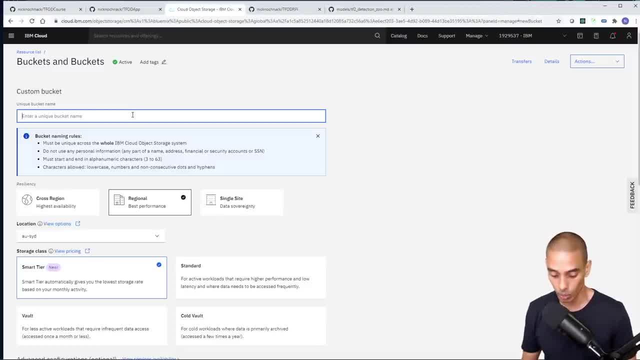 name this. pay attention to this name because you'll need it later on, so we're going to call it directions tfod. that sounds good. again, you can name it whatever you want. you just make sure you keep note of that particular name, and then we are going to select our location, so I'm going to choose. 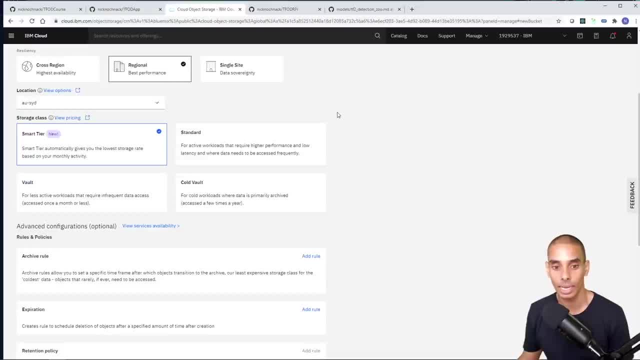 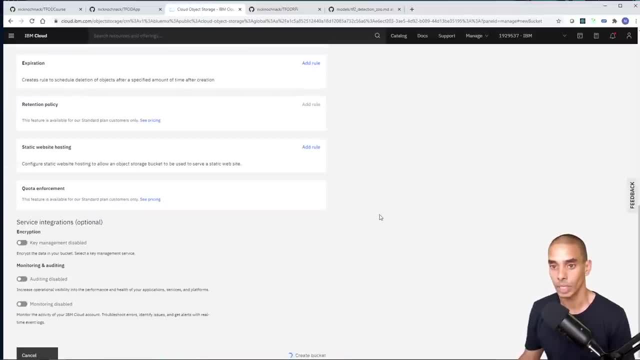 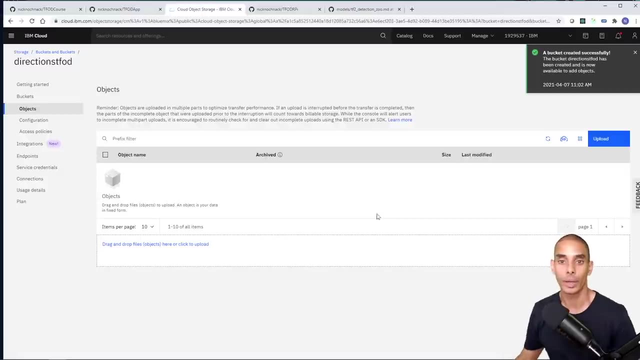 a usid, but you could choose a bunch of different regions to host this in and then that's about it. then we can skip all the way down to the bottom and hit create bucket, and so this will spin for a little while and we should be good. okay. so that is step five now, or it's half done, so we've created the bucket. 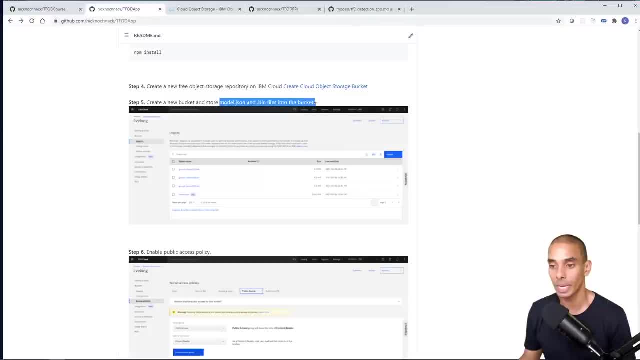 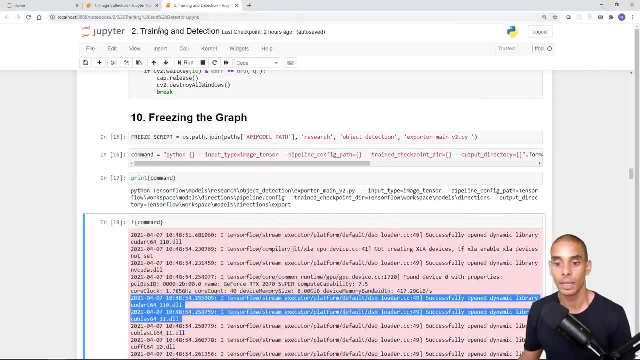 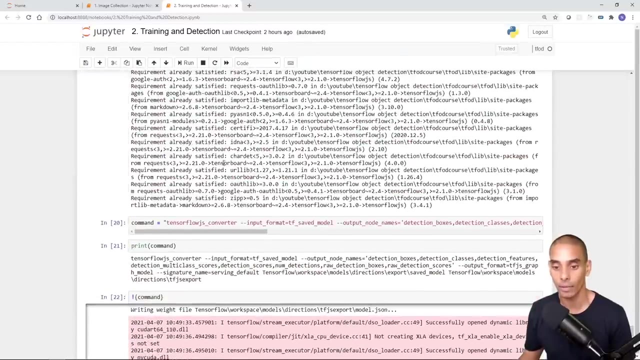 we need to store the modeljson file and the dot bin files in the bucket. so these were the files that we created. let me minimize this and this and this. so these were the files that we that were created when we went and ran our TensorFlowjs export. so this line over here is what 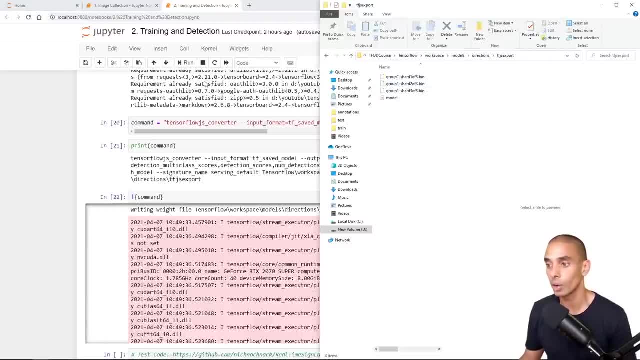 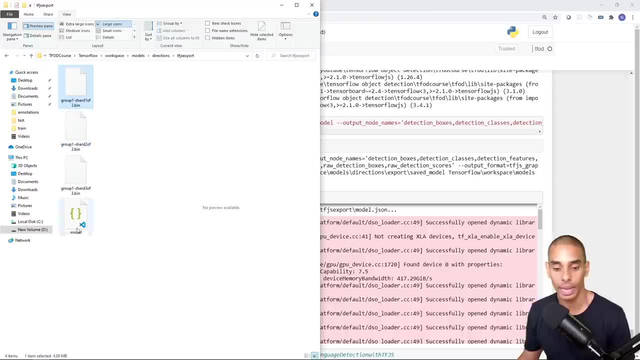 created those particular files. now, if you go into the folder called tfjs export, all of the files that you're going to need to upload are in there. so group one, dash shard, one of three, all of these. so you need to upload all of these into your bucket to do this. we just go back to our bucket. 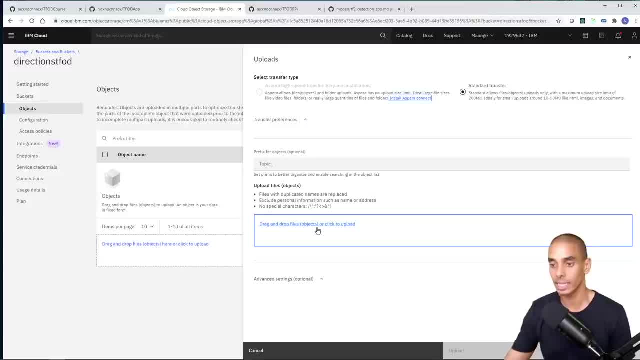 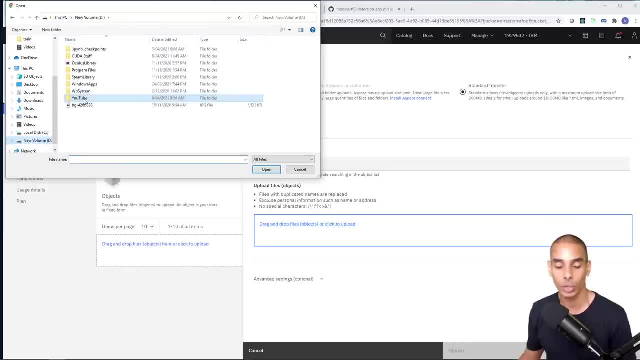 hit upload and then we can select this little region over here to actually upload our file. so we're going to click into that, go into our repository. so youtube, TensorFlow object detection, tfod course, tensorflow workspace, and then where our models, and then we're going to go into our 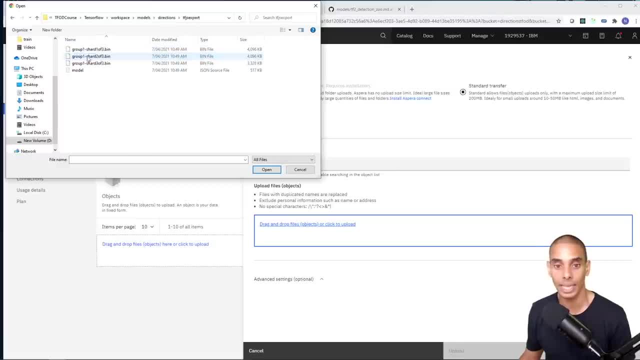 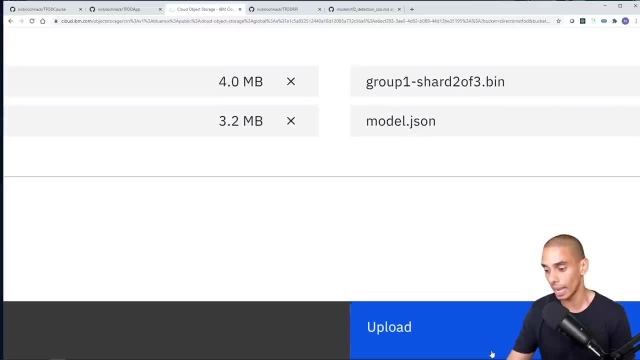 directions folder and then we want our tfjs export and we're just going to select all of that and hit open and that's going to upload our folders. then what we need to do to actually go on ahead and upload. i've got a feeling my head is going to be blocking that. i'll move out of the way. 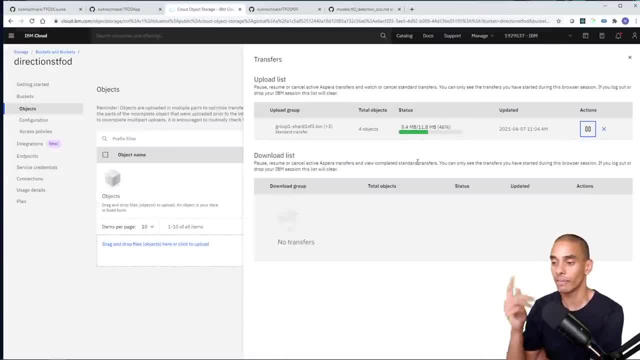 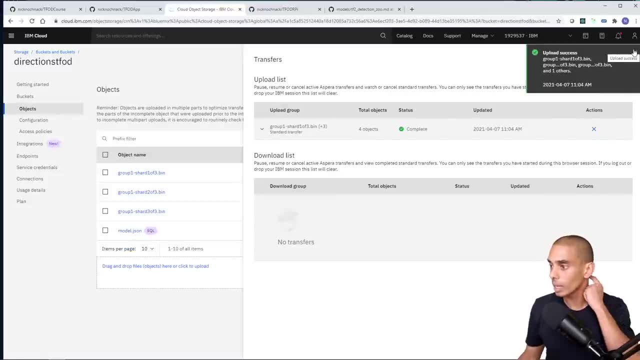 we just need to hit upload and that will upload our files into there, and then there's two things that we need to do in order to get this all good and running okay. so that's looking like it is working fine, so we can go on ahead, and 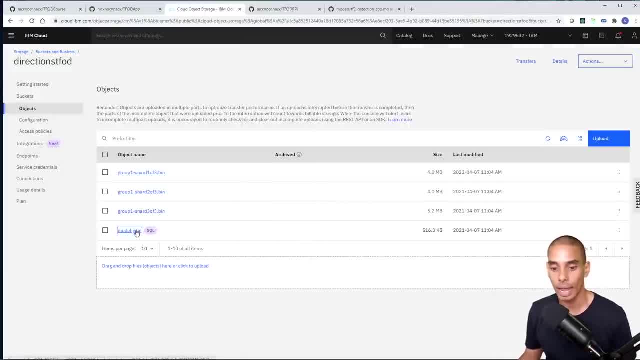 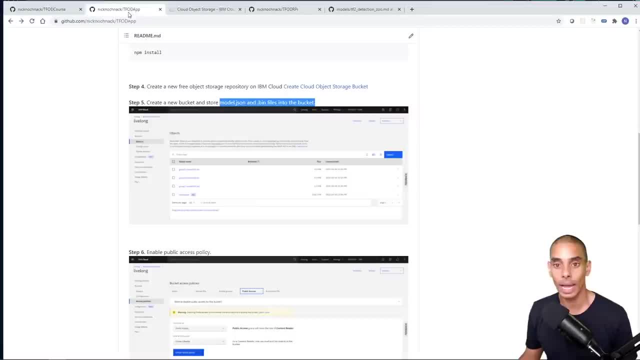 close that, then what i want you to do is grab. i'll select this modeljson file. oh, it hasn't been generated yet, so we'll come back to that. so we're then going to go on to our next step, which is enable a public access policy. so this is step six, over here. 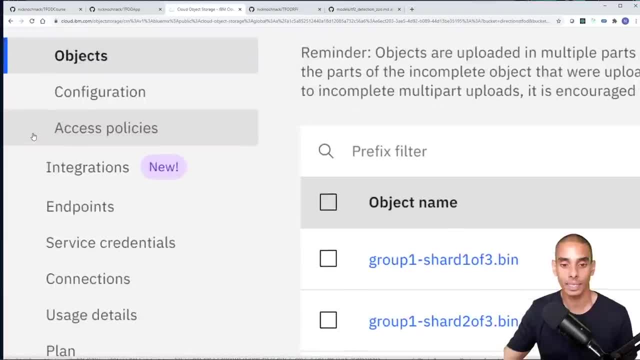 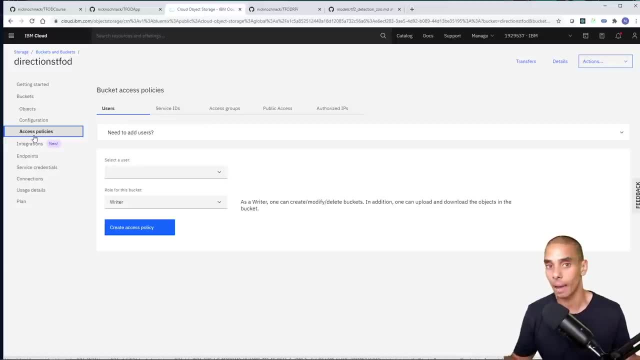 so, to do that, we can close this and on the left hand side you're going to see this button over access policies, so we can select that, and what we're effectively doing is we're hosting our model here. so this is going to allow us to actually host our model and leverage it from. 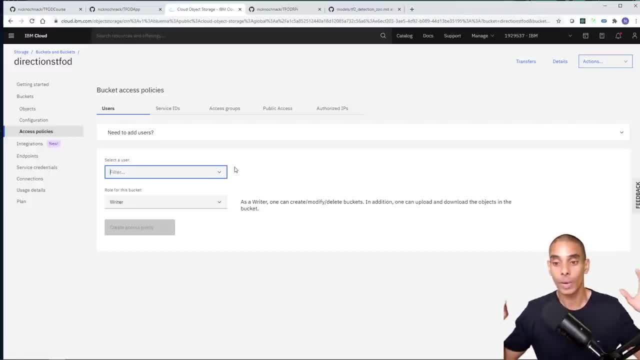 pretty much anywhere in the world. so we need to do two specific things: we need to put our model in a bucket and then we need to make it available to the world wide web so we can reach it from our app. so right now we've got it in our bucket, but right now we can't actually access it from our 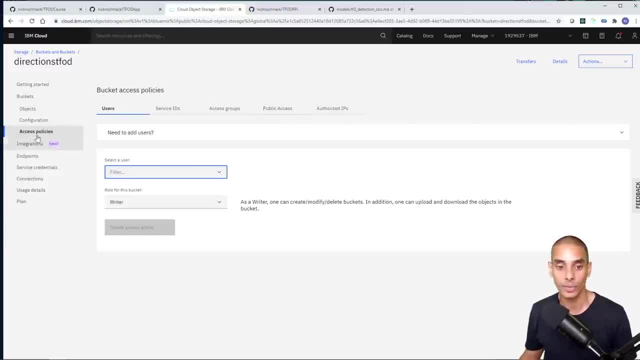 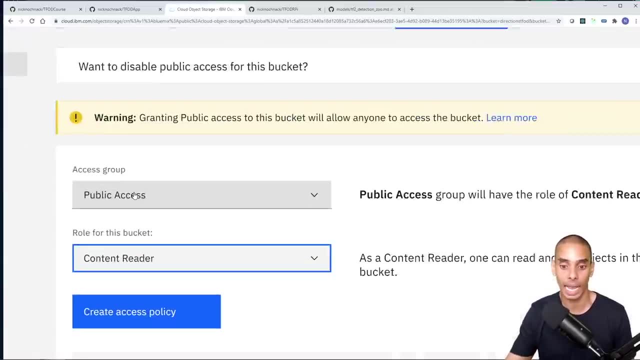 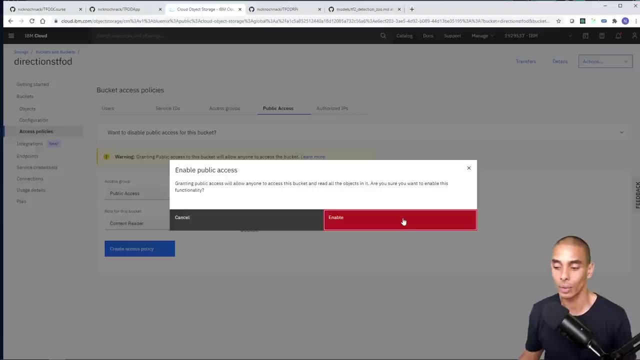 app. so we're going to enable public access. so once you've hit access policies, go on over to public access and then choose uh, so leave the leave it as access group public access and then leave the role as content reader and just hit create access policy and then it's going to give you a warning. 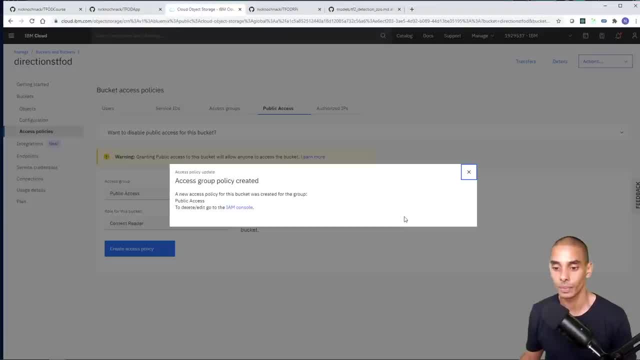 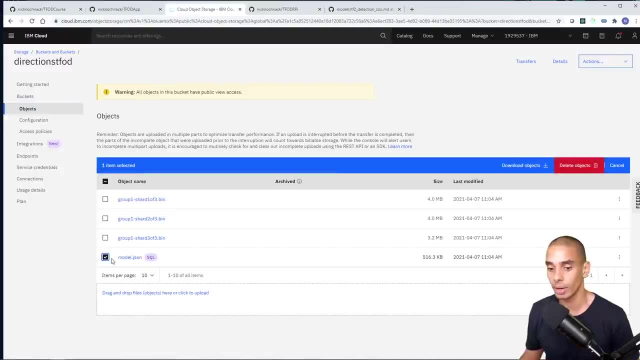 because now it's going to be publicly available. hit enable, and that is our access group policy created. so then what we want to do is actually go back and grab the url to this particular modeljson file. so now that you've created the public or enabled public access, you should be able to grab. 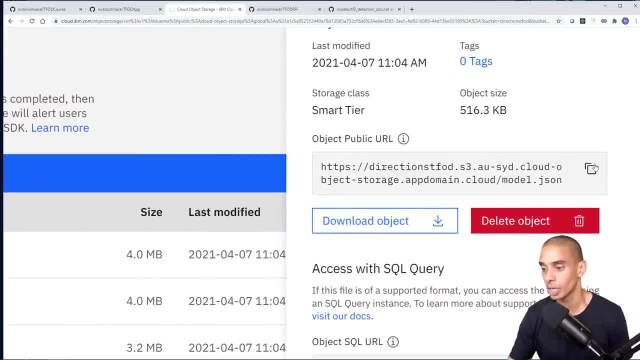 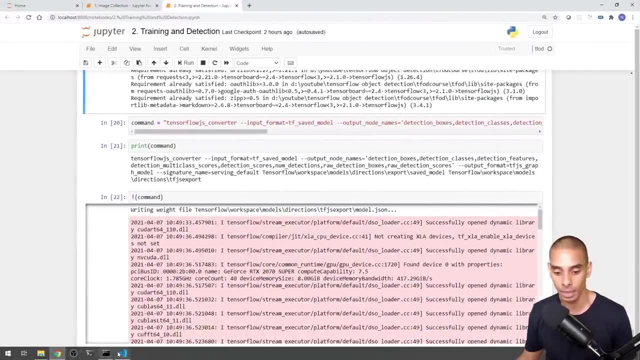 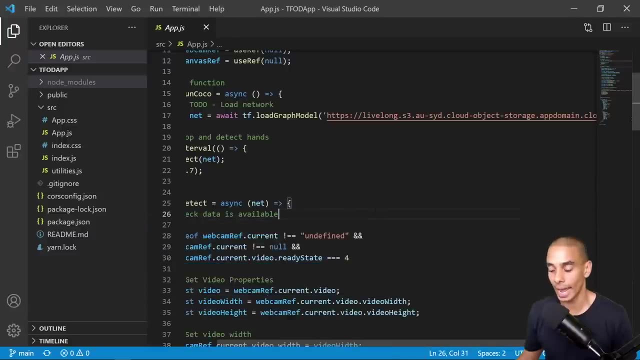 this object public url over here. so i'm just going to copy that and what we'll do is we'll go over into our app that we created, which is this over here. so what we clone down and in order to use that particular line that i just got you to create, you just need to go inside of so say: this is your. 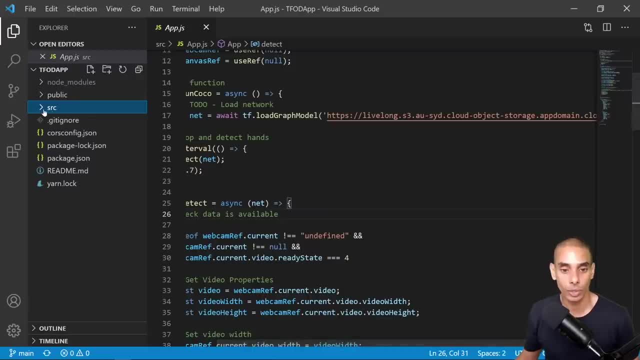 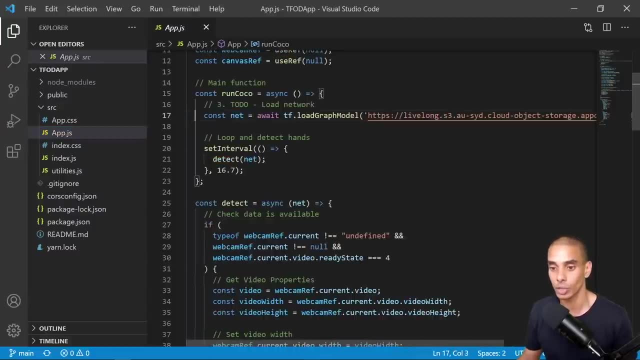 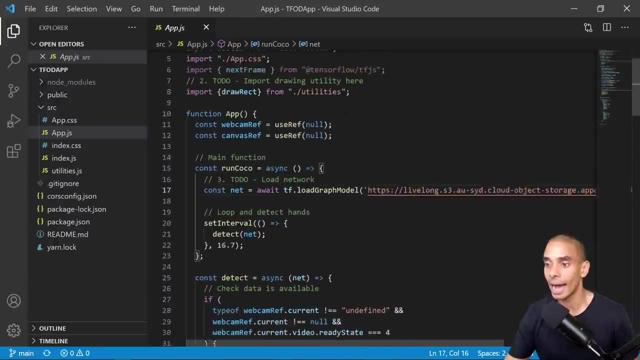 main app folder. what you're going to need to do is go into source, appjs, and if you go to line 17, but if you just search for the line that says const net equals, await tf load graph model. so this is actually going to load our react or a load our tense flow js model into our web app. 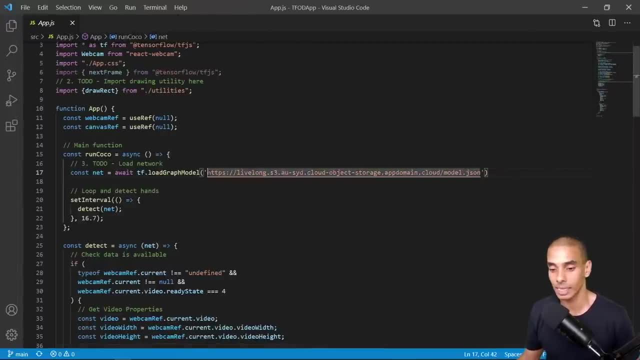 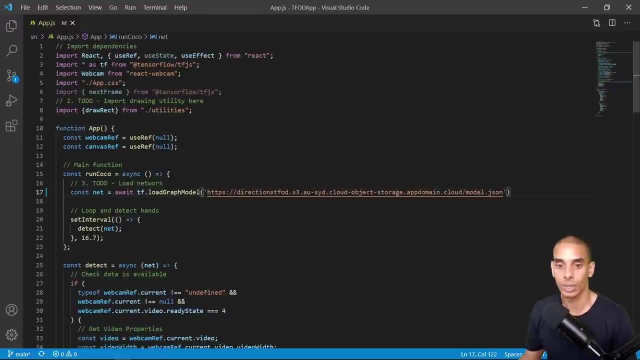 if i minimize this, it looks like that at the moment that's an existing one. i tested, so we're just going to paste our new link over there and hit save. so we're good for now. so there's going to be a few other things that we need to update to get this to run now. namely, we need to enable 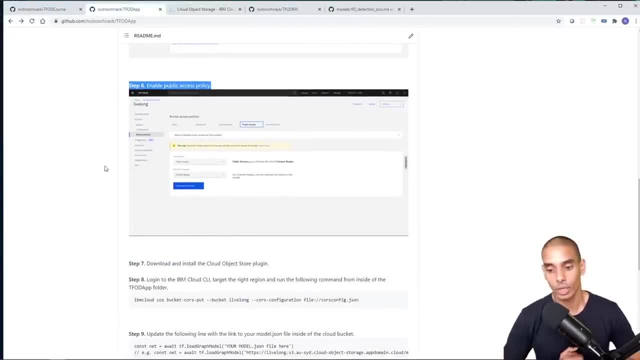 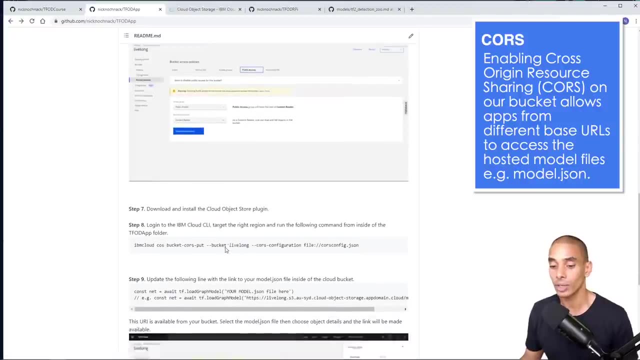 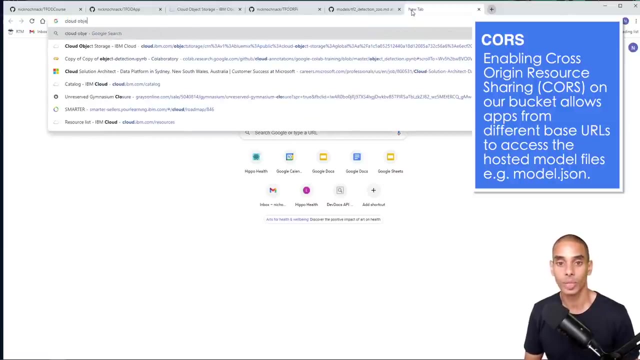 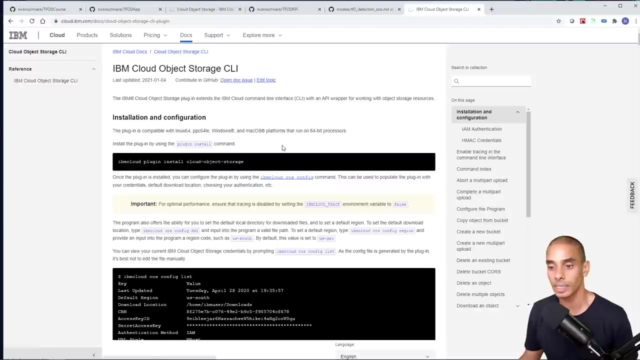 something called cross origin resource sharing. so in order to do this, we need to run through a couple of key commands and in order to actually do that, we need to have the ibm cloud object store cli installed. so to do that, you can type in cloud object storage cli installation and this installation over here. 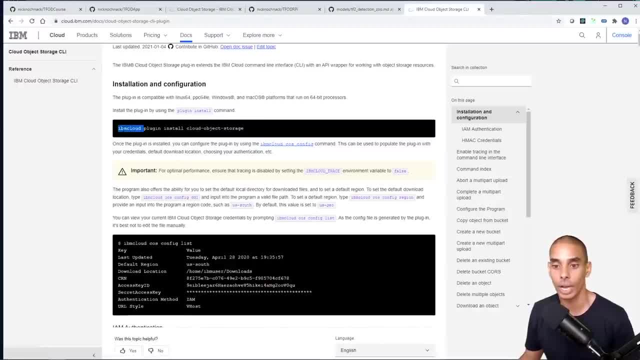 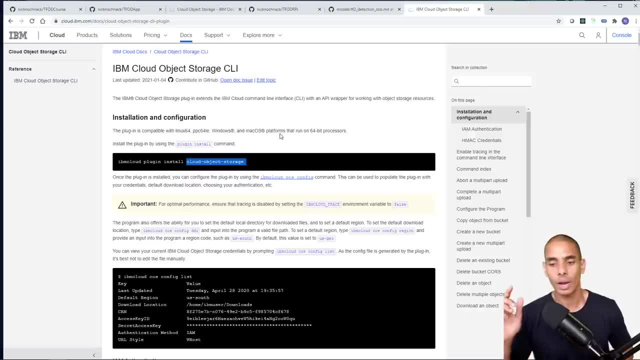 is going to walk you through how to actually get up and running. so you're going to need to install the ibm cloud cli first and then the cloud object storage cli. so again, i've got a full-blown tutorial on how to install this. but if you run through the installation steps on here, it's going to walk you through. 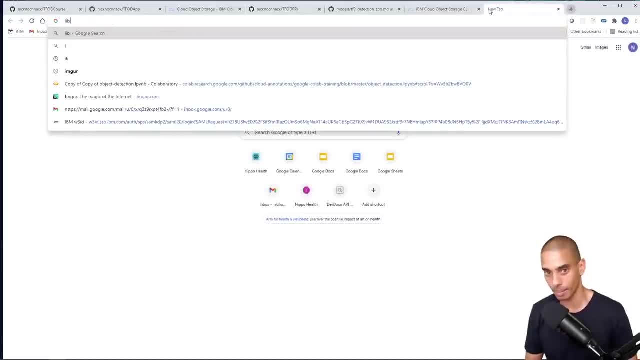 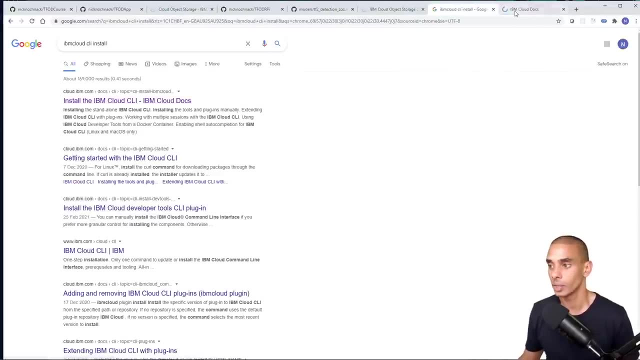 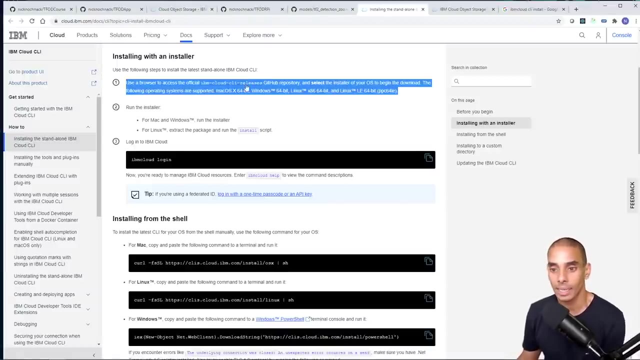 how to do this. now if we go through, let's actually take a look. so if we go to ibm cloud cli install, so this is the first one, so we've got to do the ibm cloud cli install first up. so to do this we can use a browser to access the official ibm cloud cli. 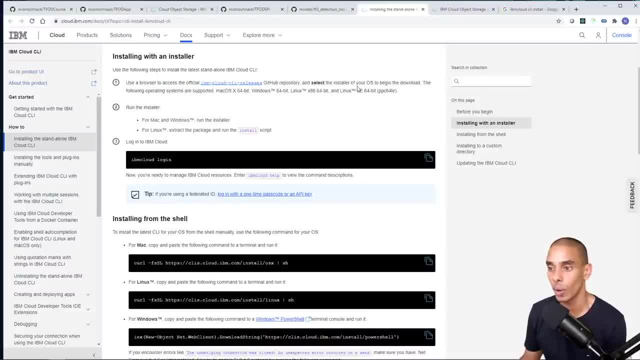 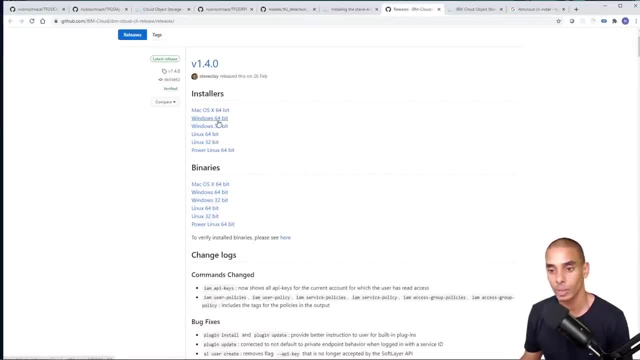 cli, release github repository and select the installer of your os to begin the download. so let's select this and you can see there's a bunch of different installers. so you can use mac os, windows 64-bit, windows 32-bit, so we'll do windows 64 and you can see it's downloaded. 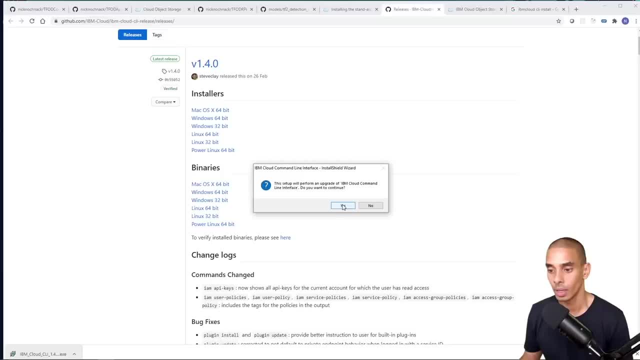 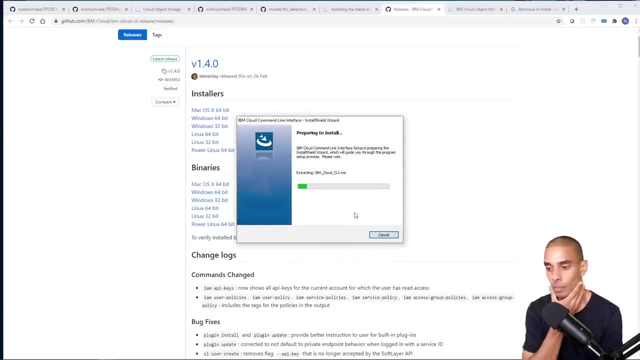 let's run this, hit yes, so it's going to perform an upgrade. so i've already got it installed, so it's just going to upgrade. so let's let it install. and so you need this for the next step. so this is actually going to be what allows us to 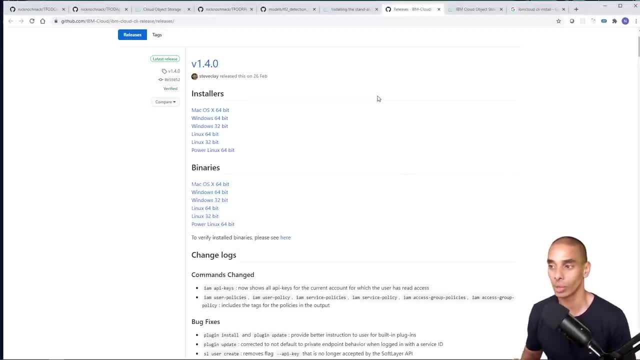 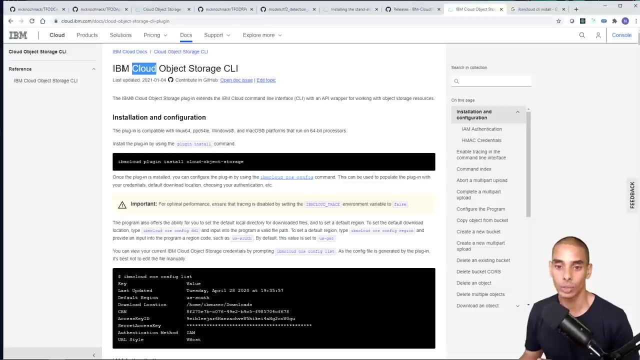 this is going to allow us to enable something called cross origin resource sharing, but i'll explain this a little bit more in a second. and then what we want to do is install the ibm cloud object storage, cli, so i'm going to show you how to do this, so you actually do this through the 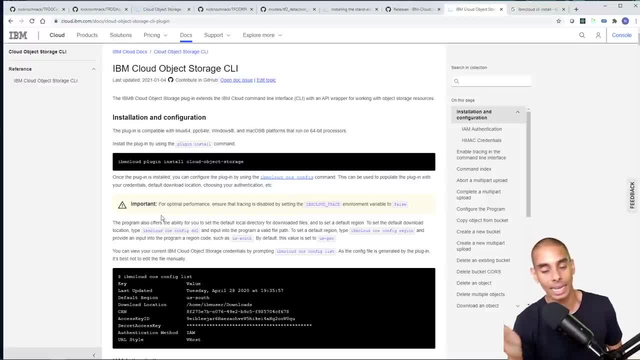 ibm cloud, cli, and cli just stands for command line interface, so it's basically, it allows you to run it through a command line, right? so to do this next step, what we need to do is run this command here, so i'm going to show you how to do this. so, first up, what you need to do is log into ibm cloud. 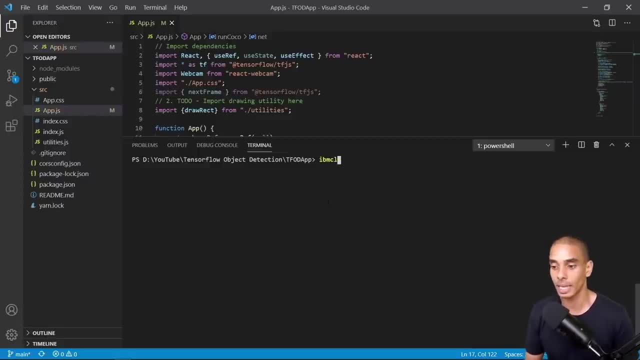 so i'm just going to clear this. so, to do that, you can just type in ibm cloud log in and, by default, as soon as you hit login, it's going to ask you to pass through your email and your password, and these are going to be the same details that you passed through when you went and created your. 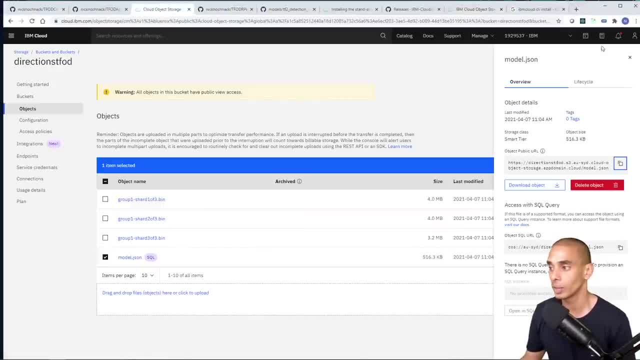 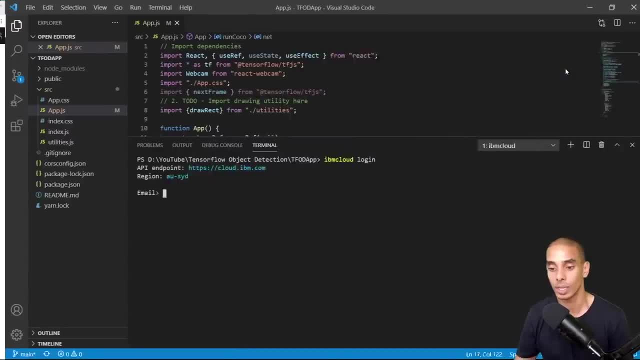 bucket. so when you created your bucket- uh, right up here- i was sort of saying that you would have had to either hit log in or sign up. when you hit sign up, you would pass through your email and pass through your password. so the details that you put here are going to be the same. 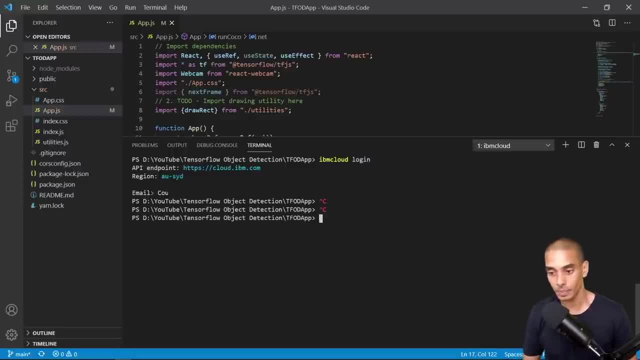 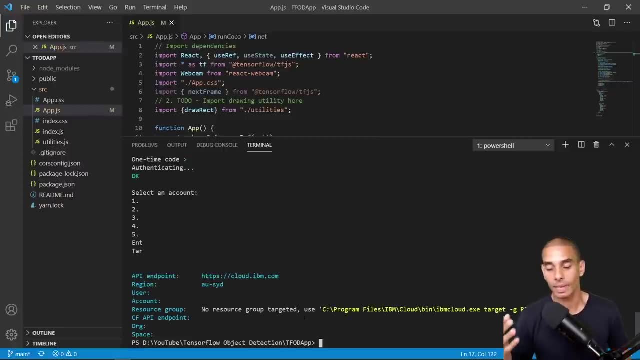 details in this particular case. so you pass through your email and your password. so i'm going to go ahead and log in. okay, so i've now gone ahead and logged in. so i just passed through my email and my password. i did it slightly different because i've got a different. 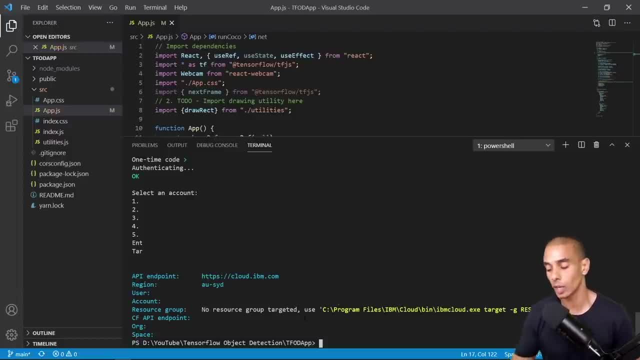 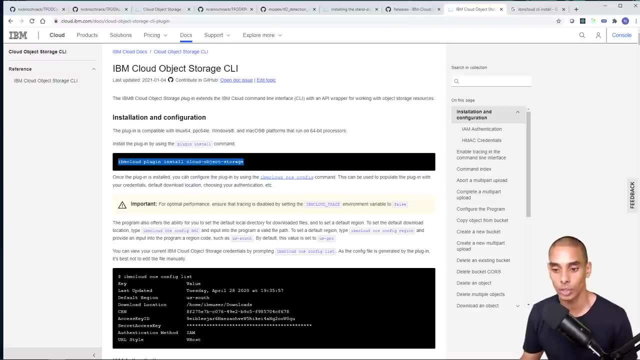 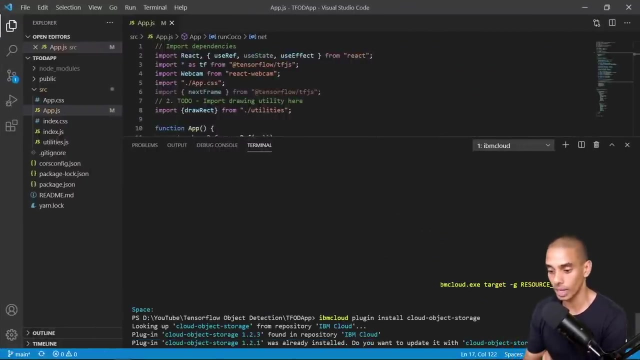 account. but that's fine. you just pass through your email and your password and you'd be able to log in. now what we need to do is install the ibm cloud storage cli. so to do this, we just copy this command here and paste it, and so this is going to go on ahead and install that cli so we can. 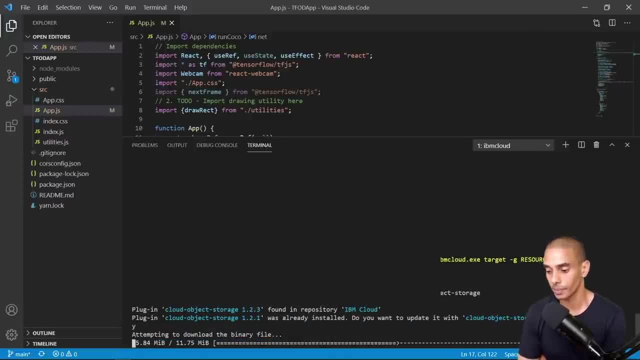 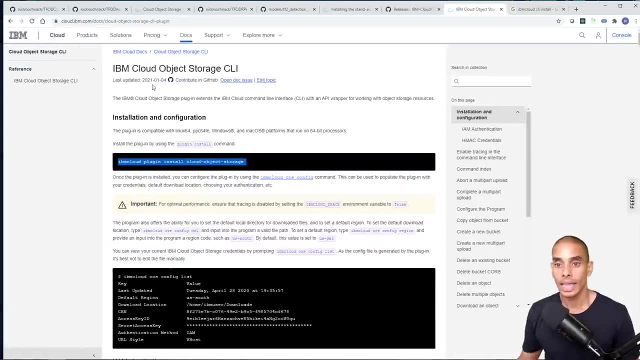 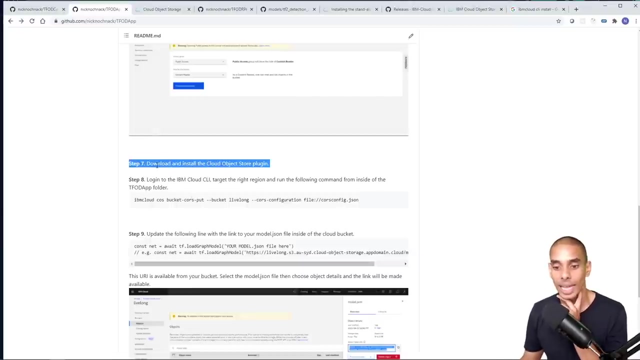 just hit yes and we should be good to go cool, so that's now done, so we can clear this to give us a little bit more space. and then if we go back to our tense flow object detection uh repository or tensplode object detection app repository, that is now step seven done, so we installed the ibm cloud. 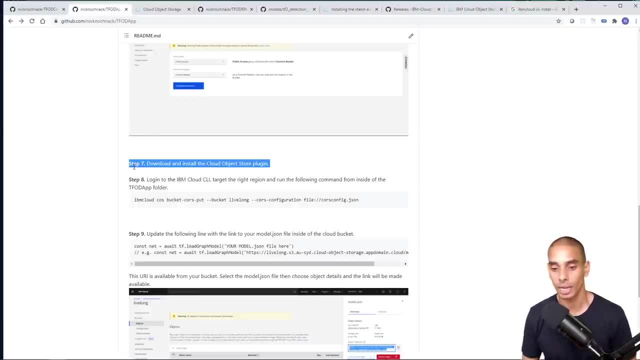 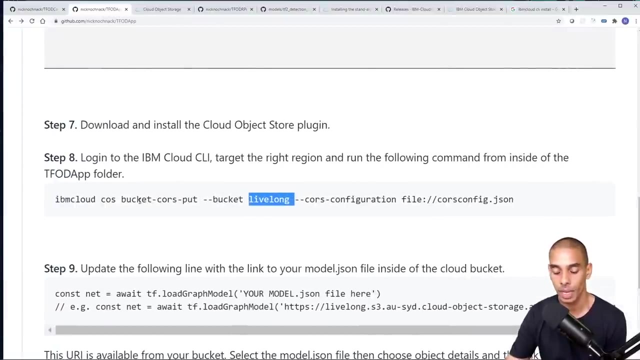 cli and we installed the cloud object storage plugin. now what we can do is we can just run this command here. so what you need to do is change one single thing, and that is the name of the bucket. so the full command is going to be- let me just zoom out a little- it's going to be ibm cloud. 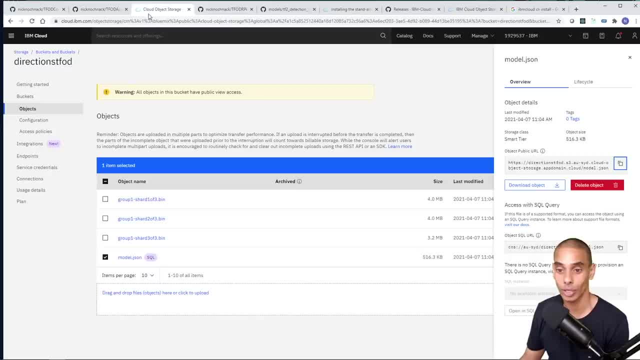 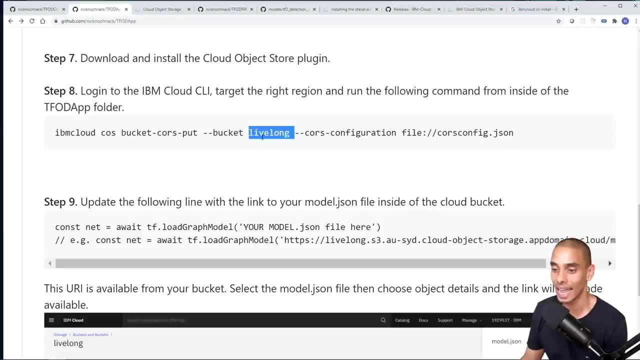 cos, so cloud object store, that's the cloud object storage service which you saw over here. bucket dash cause. dash put dash dash bucket. so this is the name in this case, the. my old bucket name was called live long because i was doing a live long uh detection, then dash dash cause. 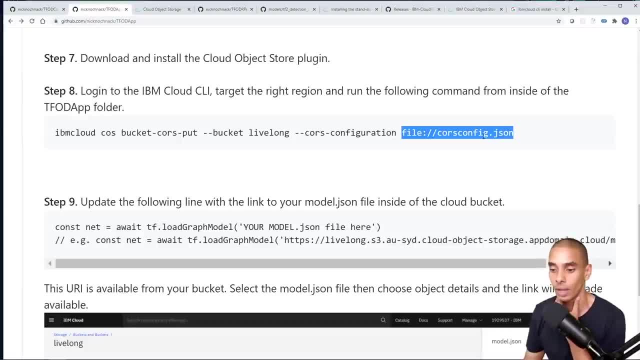 dash configuration and then we pass through the name of the configuration file. but i've already got that available for you, so you should be able to work with that reasonably easily- not reasonably easily you. you won't need to make any updates to that or write your own configuration, so i'm going. 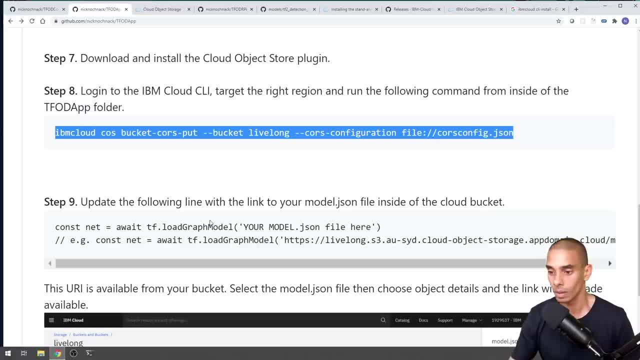 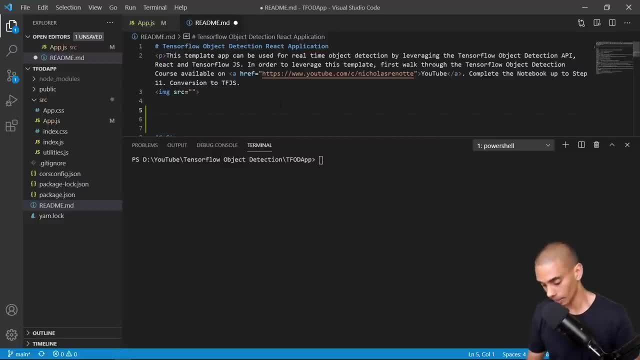 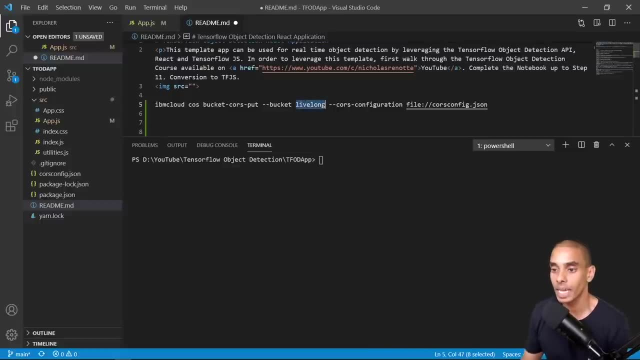 to copy this and we're going to update this. i'll show you how to update it. so let's bring jump back into our app. so, over here, just jump into the readme for now, and i'm just going to paste this command. let's just paste it in here. so what we need to do is, namely, replace this bucket name with the name. 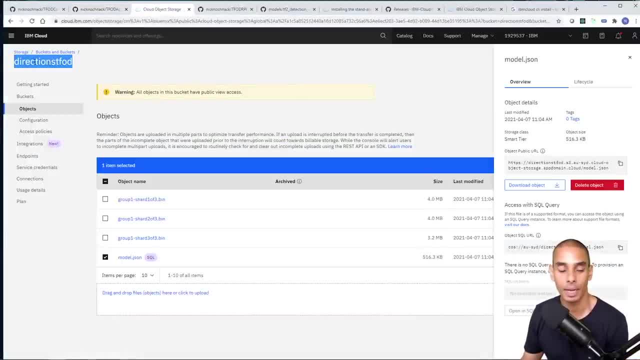 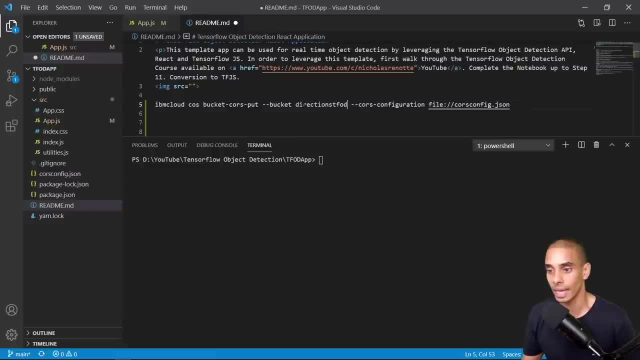 of our bucket name. so if we go back, remember we created the name of our bucket. in this case it was called directions, tfod, so we can copy this and then just replace that there and then in the next step we're going to run this command line. so you obviously need to be logged into the 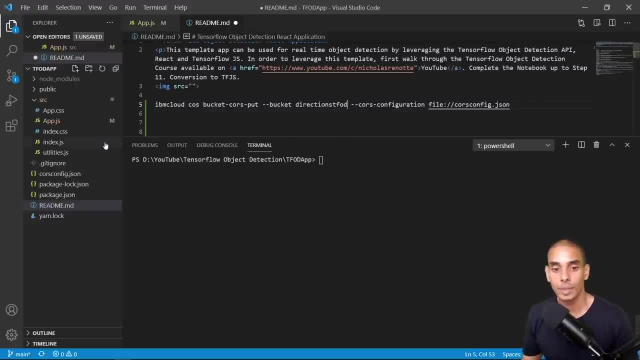 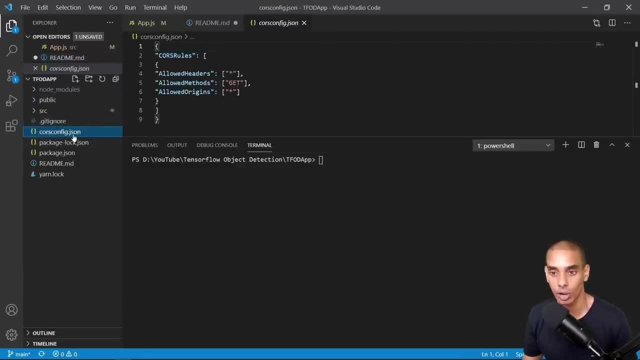 ibm cloud cli, which is what we just did. you need to be in the top level repository or the top level folder of our tfod app. so in this case, we've actually got this file called cause config. this is going to do what we need it, or this is effectively what's going to enable cause for us. 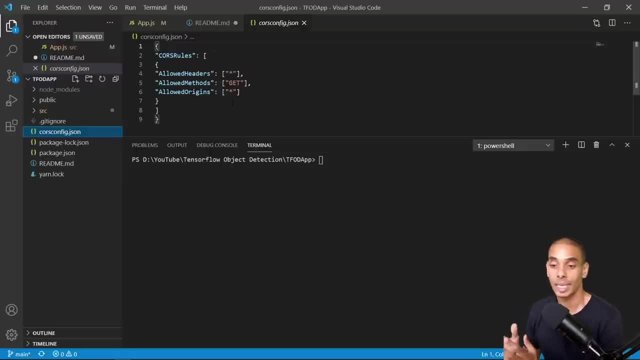 now cause stands for cross origin resource sharing, so it basically means that our web app can access a url from somewhere else. so, namely, you don't have this enabled because you don't want your web app to be accessing a whole bunch of stuff, and namely, we're locking down the buckets because we don't. 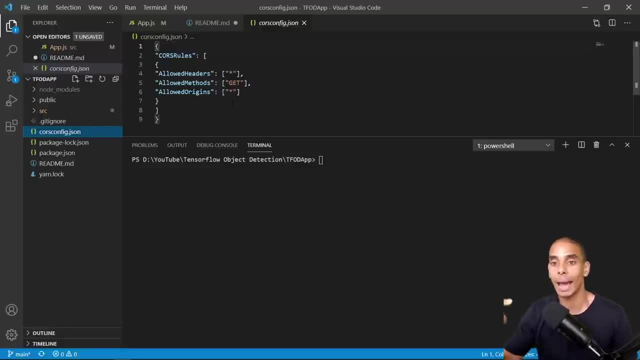 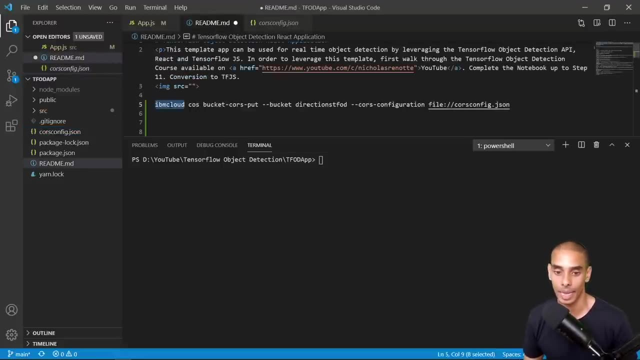 want them to be accessible from anywhere, but in this case we do, because we want our app to be able to get to it. so we're going to enable it, right, and then, in order to do that, we're going to be running this command. so this is going to be going to our cloud object storage service. 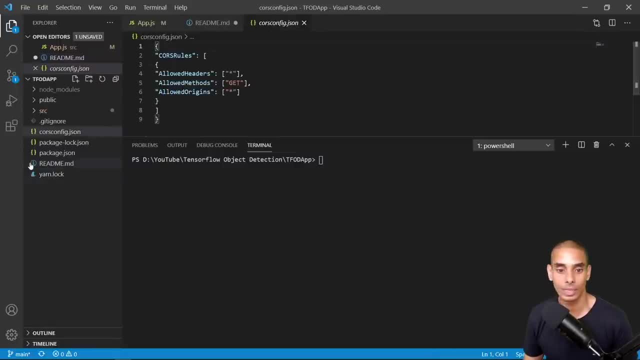 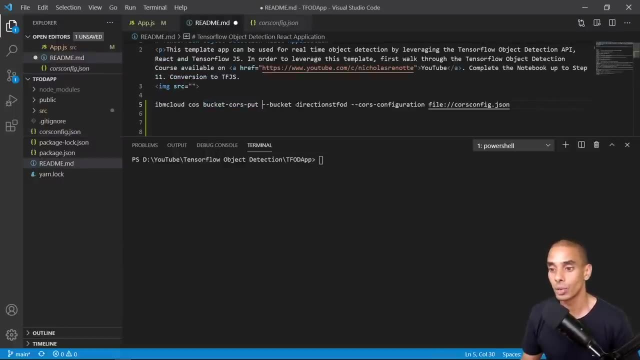 it's going to put our cause policy, which is what we've got in this cause config file, and this is part of the clone repository, so you don't need to create anything from here. so what you really need to do is log into ibm cloud and then just change, or whatever- the name of the. 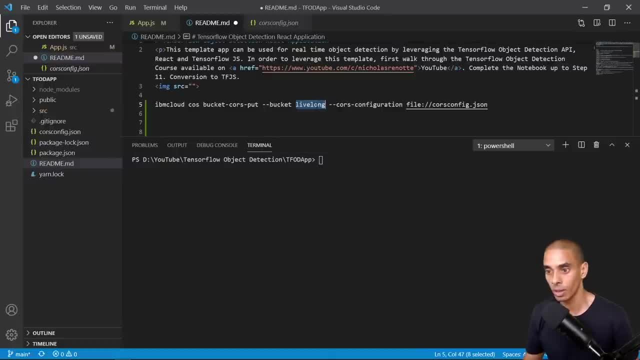 bucket that you created was you need to replace that here. so in this case it was live long before. we're going to paste in the name of our bucket, which is directions tfod, so paste that there and then what we're going to do is we're going to run this inside of our 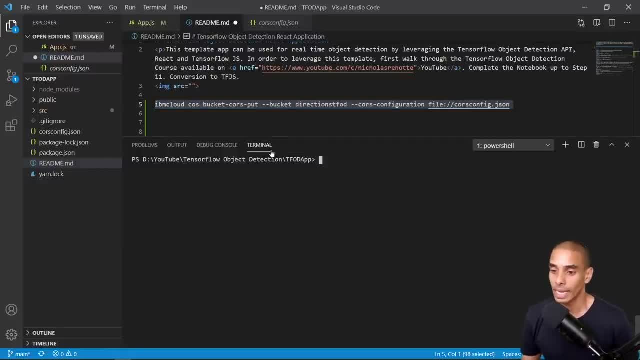 command line or terminal. so in this case i'm running inside of windows, so it's brought up a powershell terminal. but if you're doing this on a mac you might be doing it inside of a terminal. it's just called terminal or bash terminal, so we're going to run that command. so let's just make sure we've got that. cause config file. we do. 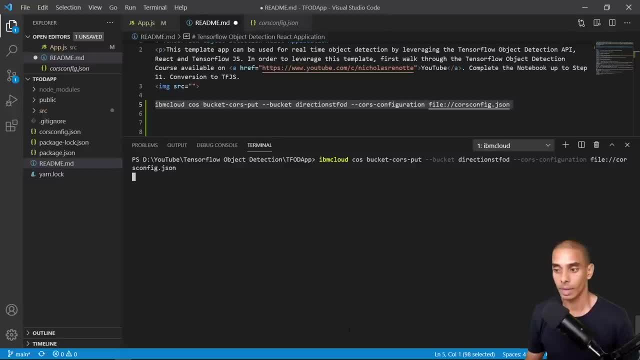 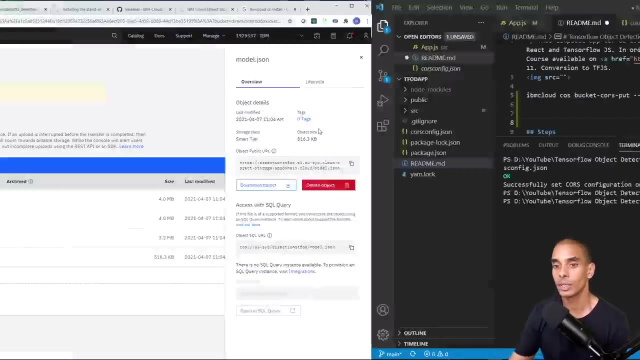 so we should be good to go. so let's clear this. run that command and it looks like no issues there. so it said: okay, successfully set cause configuration on bucket directions, tfod. so we are looking good now. now what we need to do is go through the rest of our steps. so step nine is update the following: 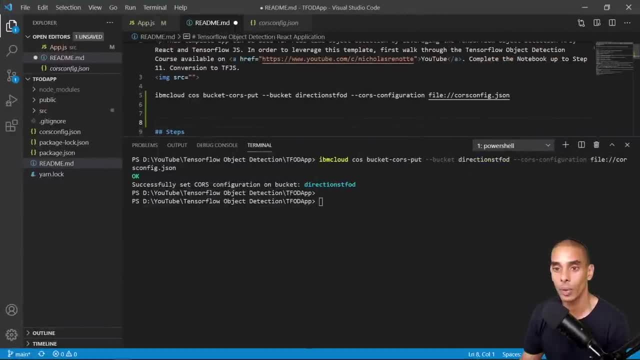 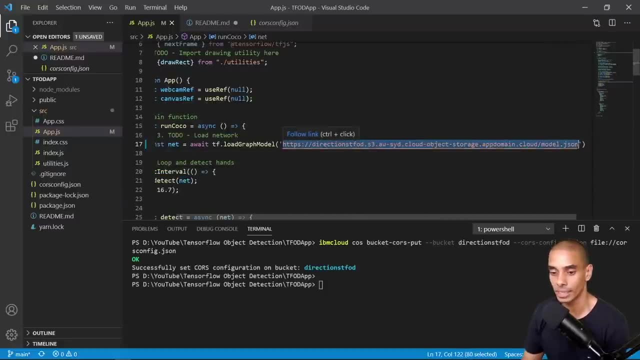 line with the link to your model url. so we've actually already done this right. so, remember, we went into appjs and we actually already pasted the name to our custom modeljson file and this is what we uploaded into our bucket over here. so this modeljson file is our tenseflowjs model and 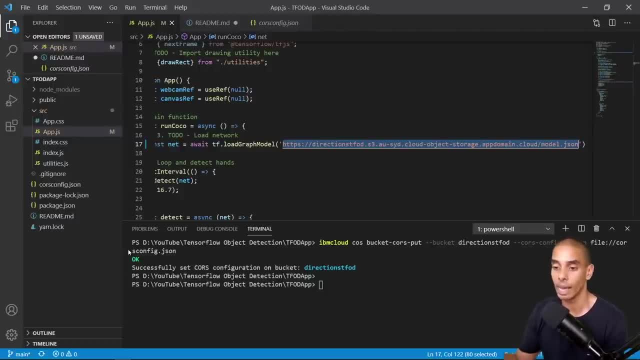 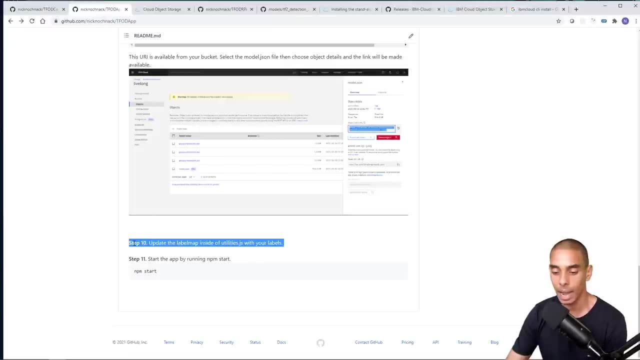 it's going to be what allows us to run our web app using our model, so that step 9 is now done. step 10 is update the label map inside of your app. so if you update the label mapl relay and edit your layer library, go that step nine is now done. step 10 is update the label map inside of your login query. 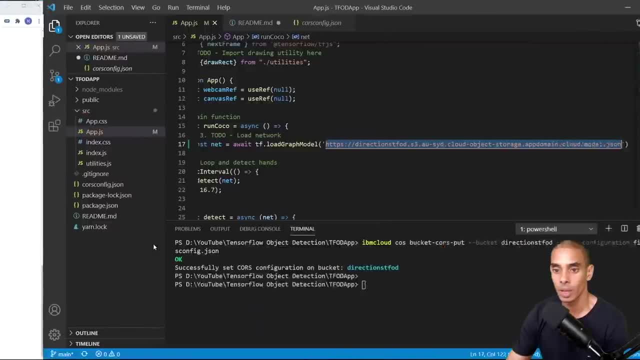 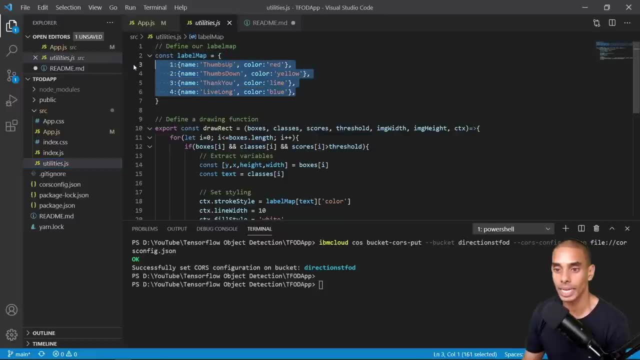 so a great portion of the steps have been done. so first of all, we need to show theонline printer to this side of utilitiesjs with your labels. so what we can do is we can go into utilitiesjs over here and all we really need to do is update this label map up there. so we need to update it. for what? 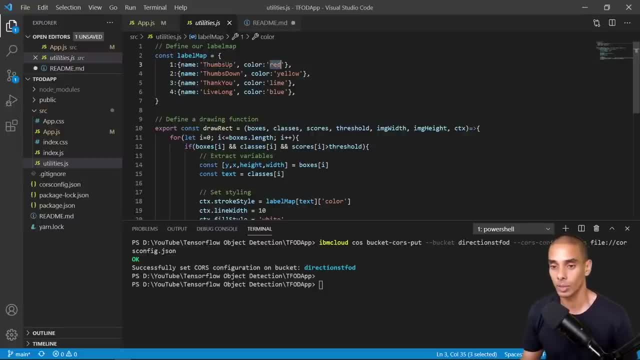 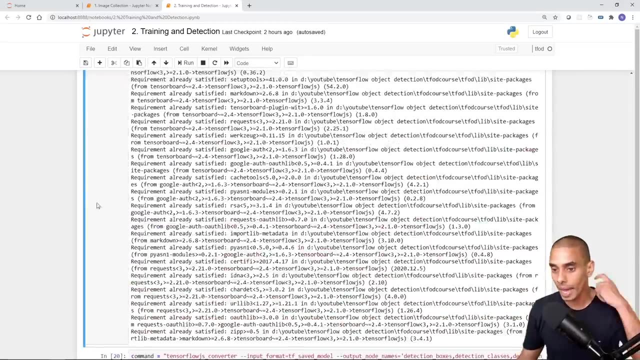 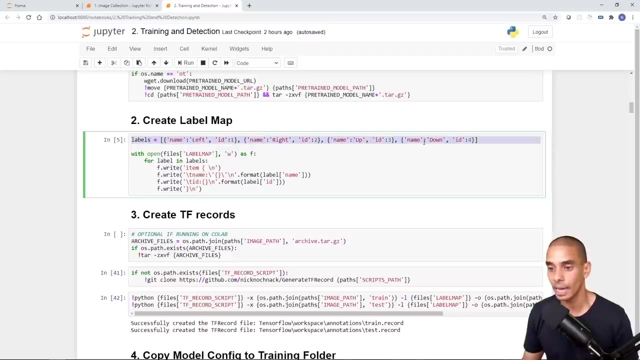 names or what our labels actually are and the colors that we want them to represent. so in this case, we're going to go back to our jupyter notebook and remember our labels were right up here. so remember we set up these labels so left right up down. so we're just going to do the exact same thing here. so if we go back into our app, 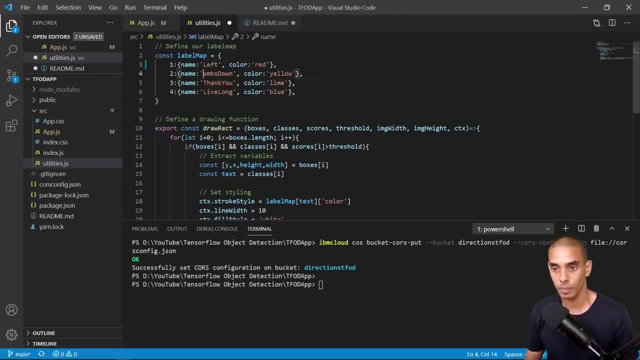 so left right up down, and save that so you can add in more if you wanted to. so you can add in additional labels, you can add in additional colors and you can update this based on your specific app. in this case, we're just updating it for our different labels, so we're just going to go back into our jupyter. 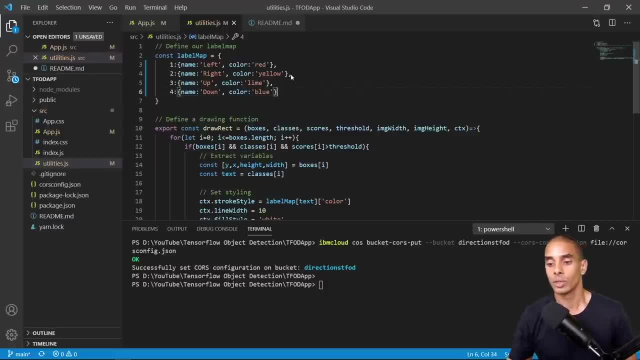 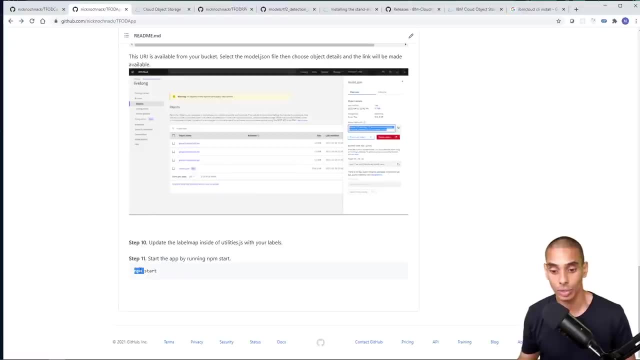 different directional models and then make sure you hit save. so that should be it in terms of all the stuff that we need to do. so we've now gone and done step 10. now step 11 is just starting the app. so to do that we'll run npm start. let's try this out. so again, make sure you're in the root directory. 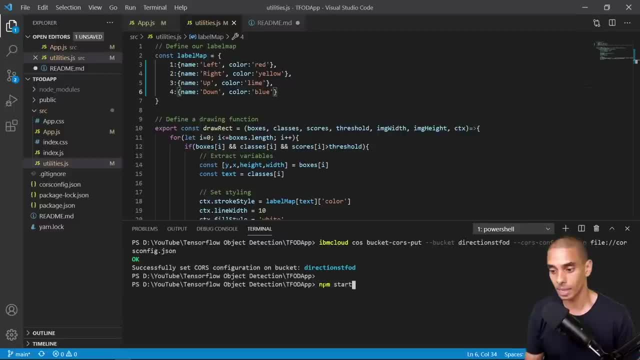 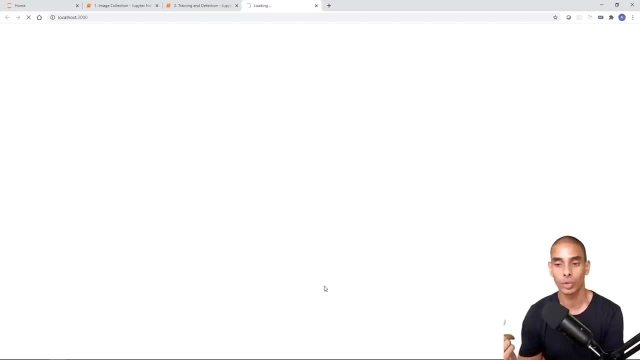 so tfod app, and then what we can do is type in npm, start and all things holding equal. this should work. so let's wait and see. so this will automatically open up your browser to the link that's actually running and it should access your webcam. now, it'll take a little while to start up. 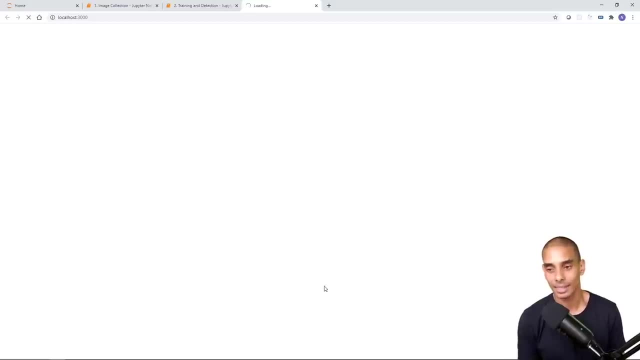 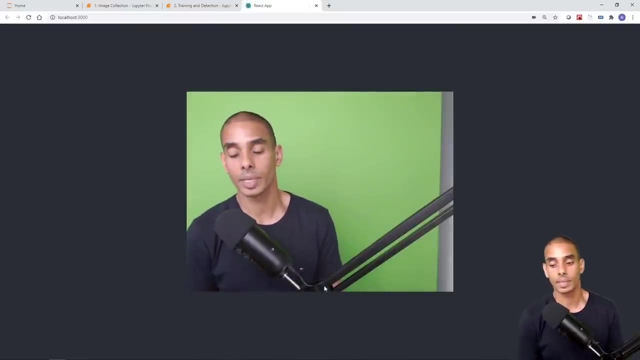 and compile, but then you should be able to test it out, so let's give that a second and then we'll take a look at our results. okay, so it looks like our react app has started and you can see that we've got our camera available. so if we take a look, it doesn't look like it is detecting. now, if 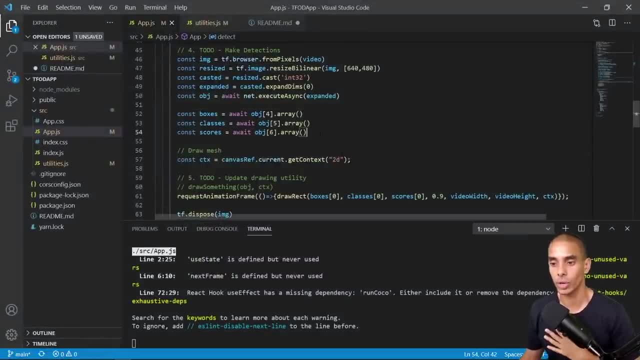 you get errors like this and you're not actually getting detections. i want to show you how to actually debug this. so in this particular app, from like the start of this video, i'm going to show you how to actually debug this. so in this particular app, from like the start of this video, i'm going to 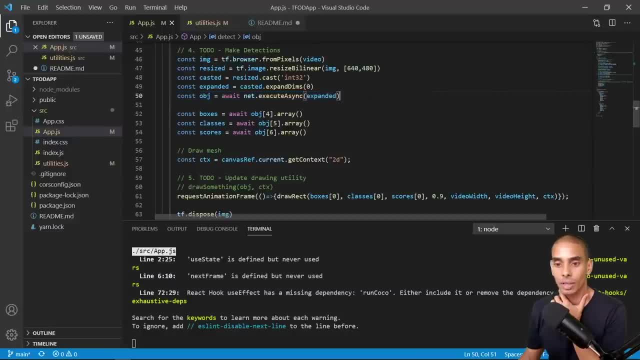 line 50 onwards, you're actually getting your detection. so this line here. so line 50. so const obj equals await netexecute async expanded. and you can see how i actually built this up. if you want to see the full tutorial for how i actually wrote this, again, i've got the code available and i can. 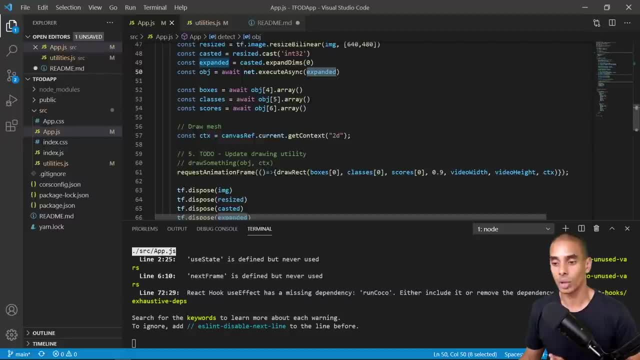 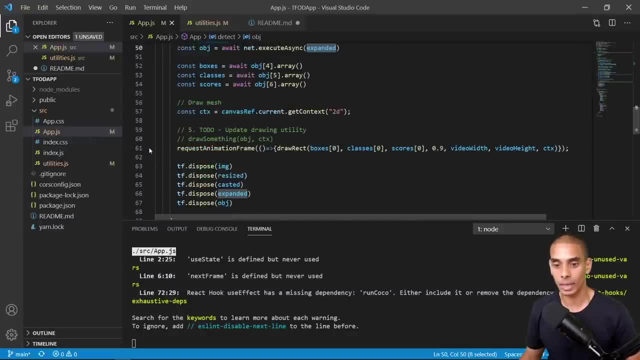 more than happy to share that with you if you're getting errors and it's not working. so this is the way that i sort of normally process through this. first up, what i'll do is i'll change the confidence metric and in this case we've got our confidence metric available through this line here on line 61. 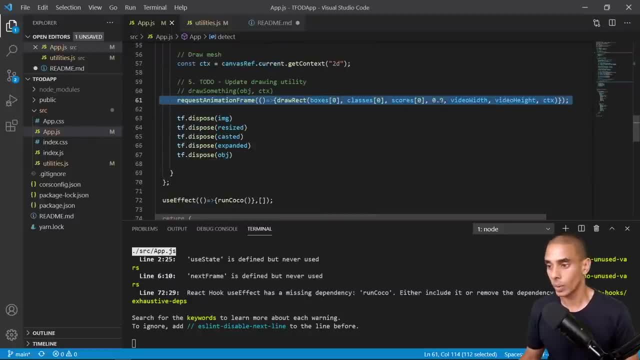 so let me just check. yep should be line 61, so we can change this number here. so right now it's set to 90. let's just jump out of that. so it's set to 90, so we can change that and drop it down. so let's. 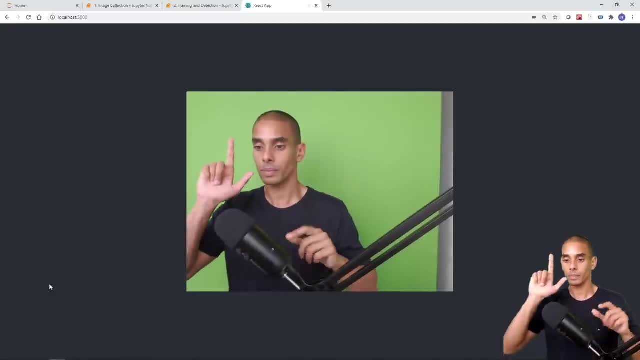 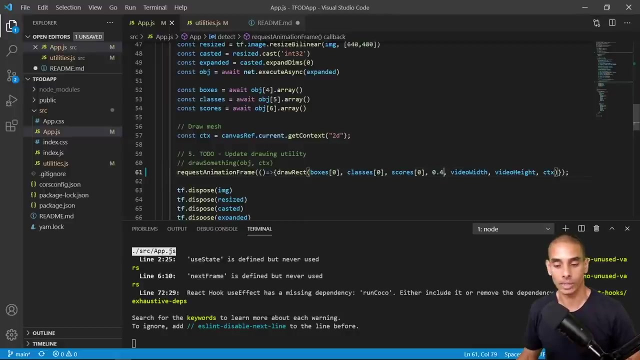 drop it to 40 and see if we get any detections. nope, okay, this is just me pointing at myself. then the next thing to check is sometimes tensorflow. js will change the order of objects from the converted model to the converted model, so let's just check that out and see if we get any. 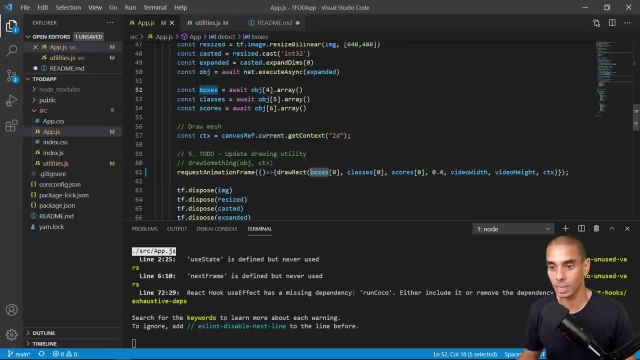 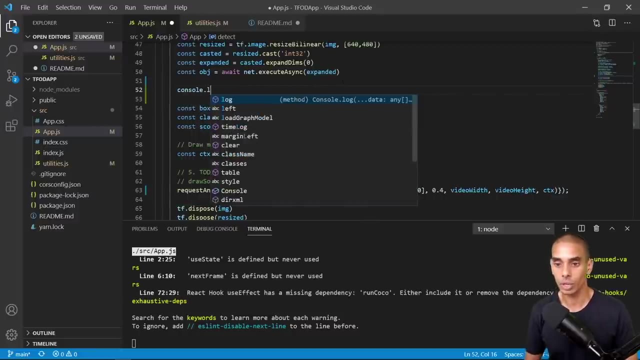 model. so in this case what we actually do is we expect the boxes to be the fourth item in the detection result array, we expect the classes to be the fifth item and we expect the scores to be the sixth item. but it's not always the case. so if we actually type in console dot log, this is the. 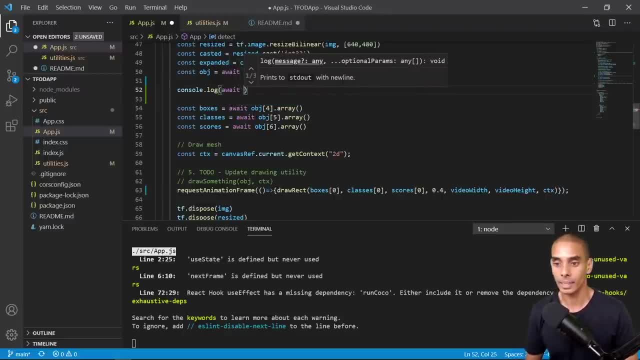 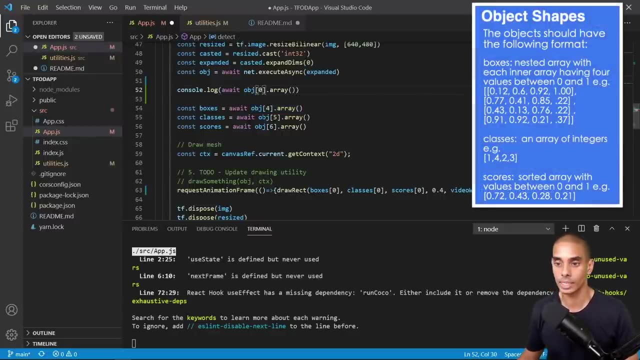 equivalent of print in python. and if we type in a weight, and then if we go through each one of these objects in the object array, we can actually determine what is what. so if we type in object zero, this is the object zero, and then if we go through each one of these objects in the object array, we 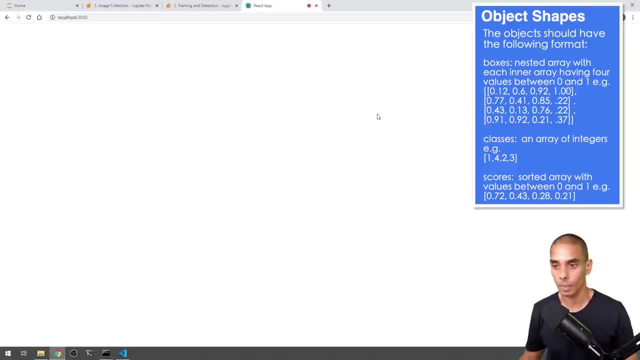 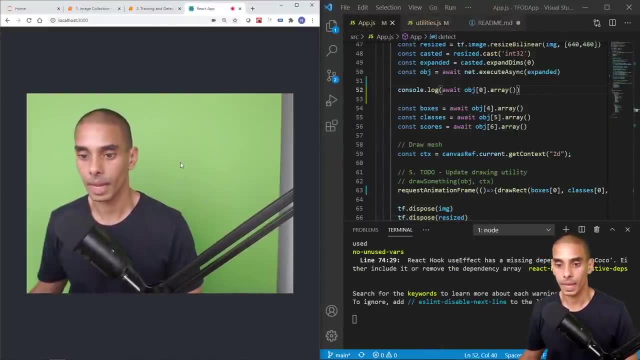 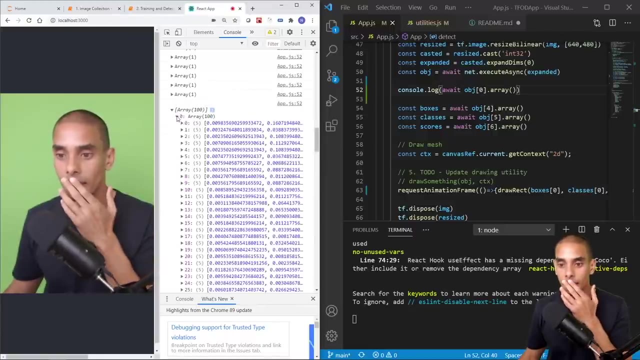 this is going to print out the first object. so if we take a look at that and let's just bring this side by side and hit inspect, so this is going to allow us to see what object is what. so you can see here that we've definitely got something in there and it looks like it's an array and each array has. 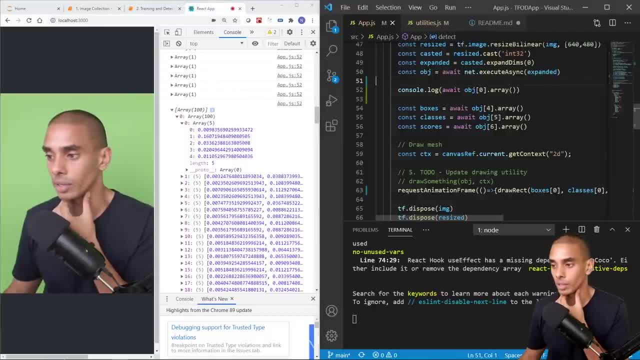 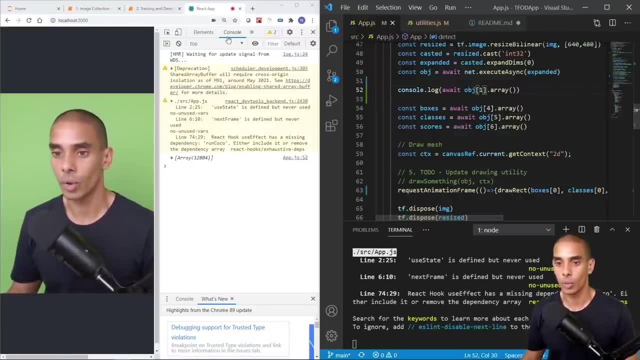 five values. so that is not our boxes, so let's try object one. and so this is sort of how to work out where your objects actually are when you go to deploy this object. so let's try object one. so what you're looking for and this is a slightly different one, so it's not that one. oh, actually it. 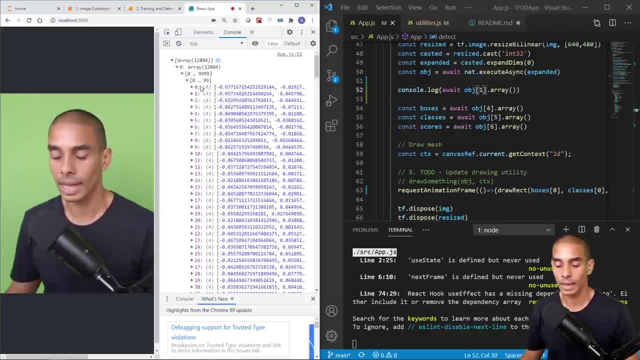 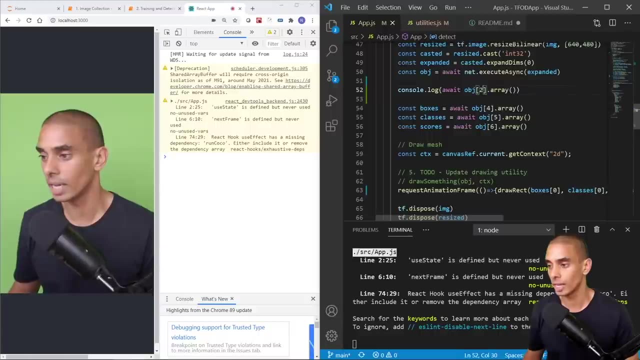 might be so this looks like. so this is the non-normalized result. so right now you can see that we're getting add boxes, but they've got negatives in them. you don't want that one, so let's try object two, and all i'm doing is i'm changing the number over here so you can see i'm. 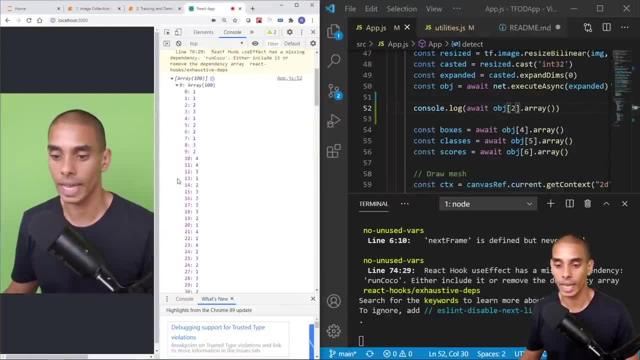 changing that. so let's take a look at this. so this is okay. so this is our classes, so this is what we do need. so you can see here that we've got one, two, three, four. so this represents the different classes that are available for our particular app. so what i'm going to do is i'm 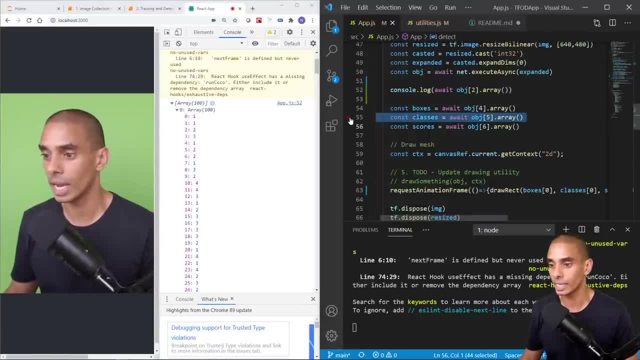 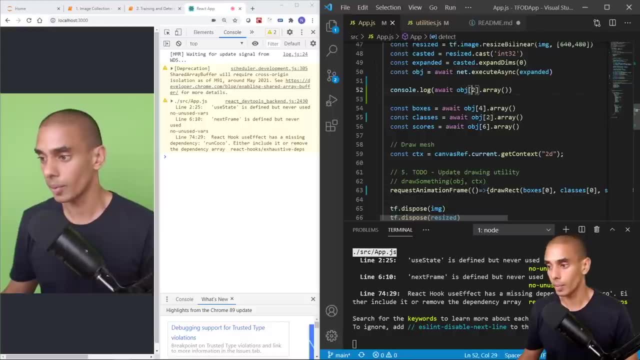 going to change this line here. so line 55, which has our classes, we're going to change that to object two hit save. so now we've at least got our classes placed appropriately and then we're going to go through our next value. so we want to check what's in object three or position three in our 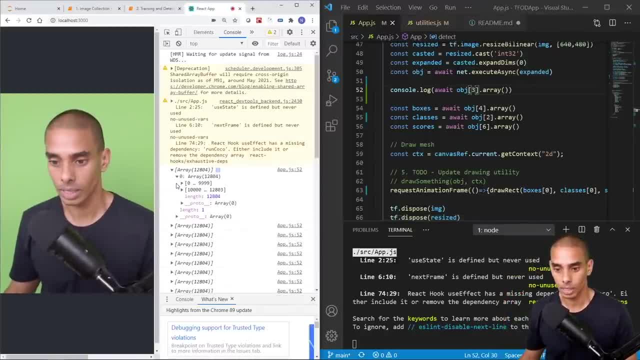 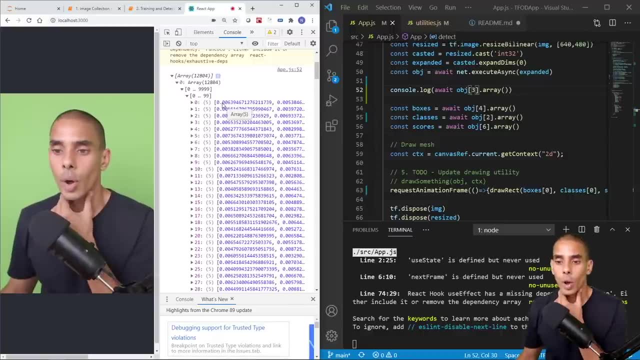 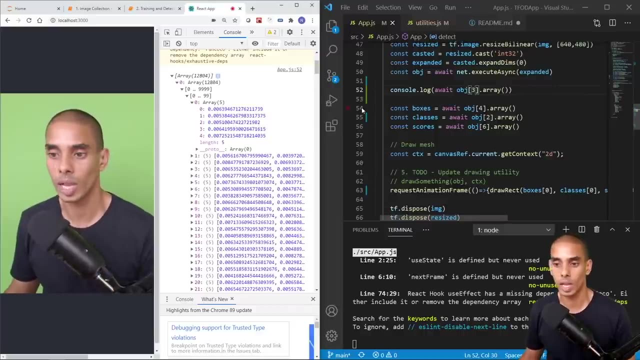 or our results array and what's this. so this looks like some, this looks like non-post process box classes. so you can see here that these are very low numbers. so if we actually try to use these for our boxes, well, i'll actually give you an example, right? so this is object three. so if we set this to our boxes, let's take a look. 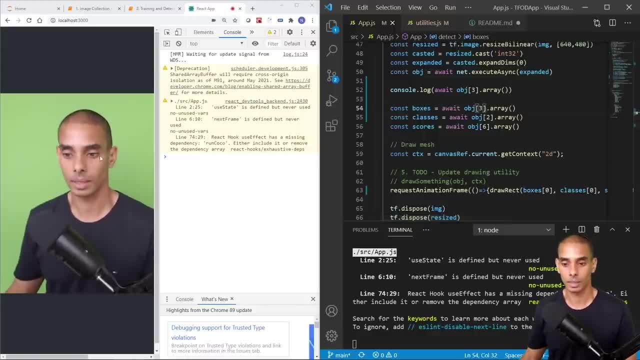 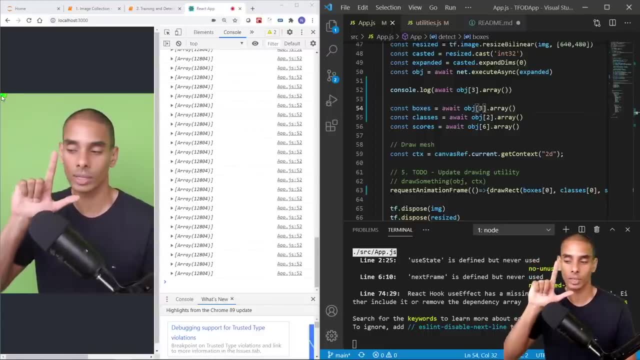 so it's getting detections, but let's wait for it to run. but you can see that it's detecting all the classes in the top corner, so it's really really small. so if you set that value to your boxes it's not really going to work. so let's try. object four: see what that is. 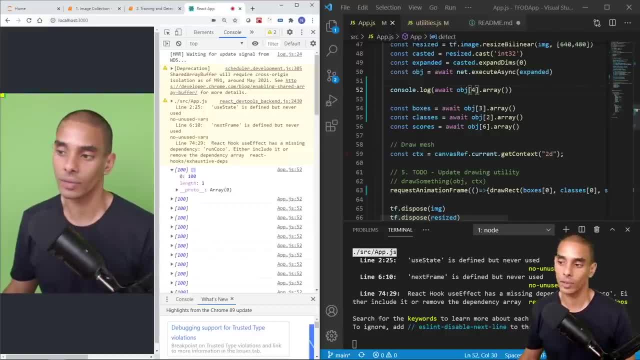 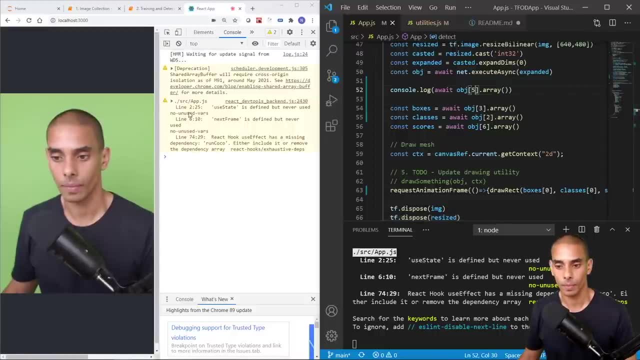 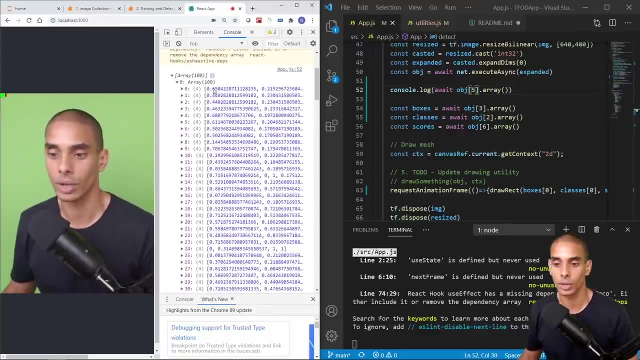 and so it looks like we've got a hundred. that's just the count of objects that have been detected. let's try object five. this is looking promising. array 100: okay, so this might actually. yeah, so this one is Korean, or this particular set of arrays is our boxes, so it should look something like this there. 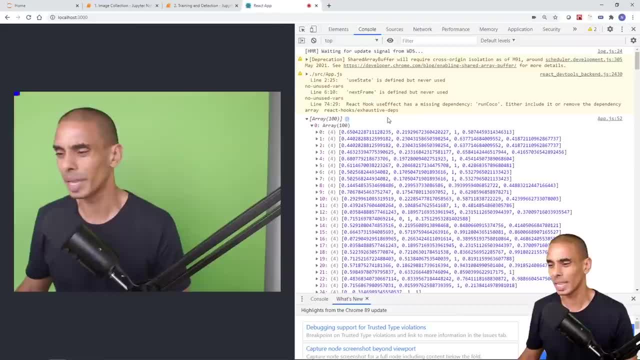 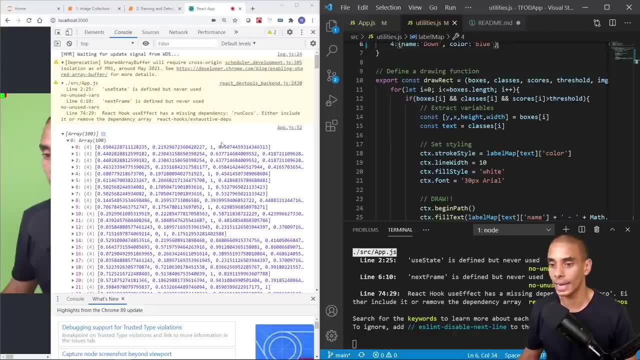 should be a number between zero and, ideally, one. so i believe it's x. i can actually tell you correctly. so these values represent your y value, your x value, your height and your width. so in this case you've got all of your box values. so this is what you'd expect your box value to. 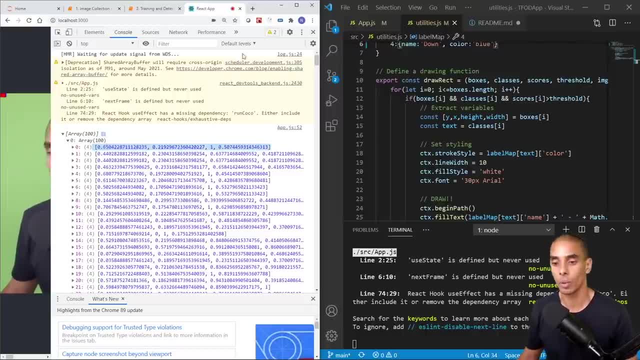 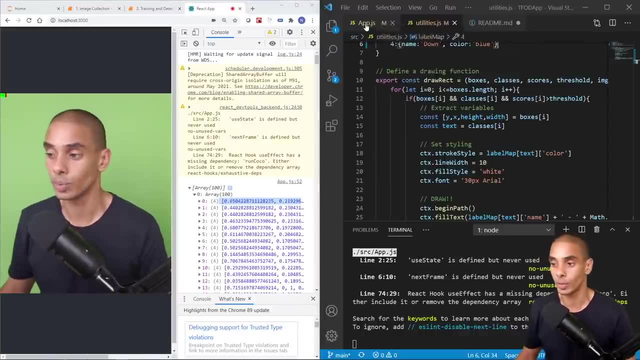 look like. so it's a bunch of numbers between zero and one, so there shouldn't be any negative values in there. if it is, it's the- i believe it's the non pre or pre на box value specifically, and you can pre or non post process value. so you don't actually want those. so what we're going to do? 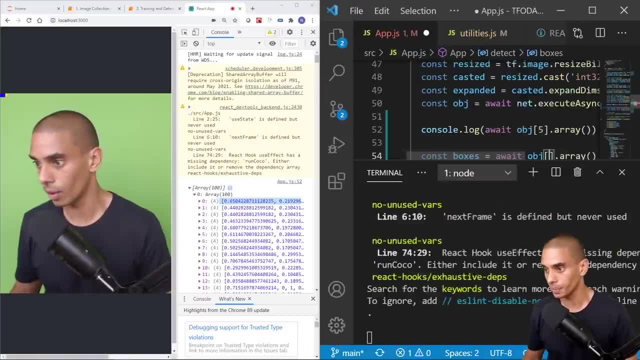 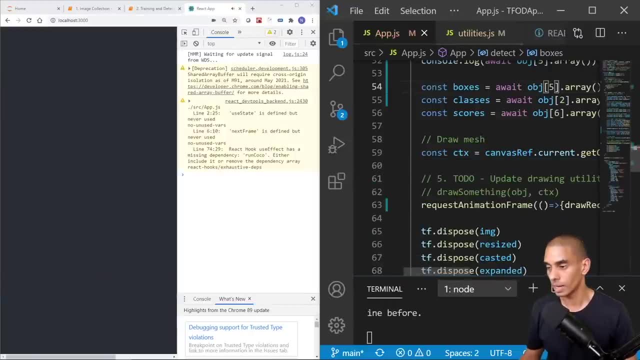 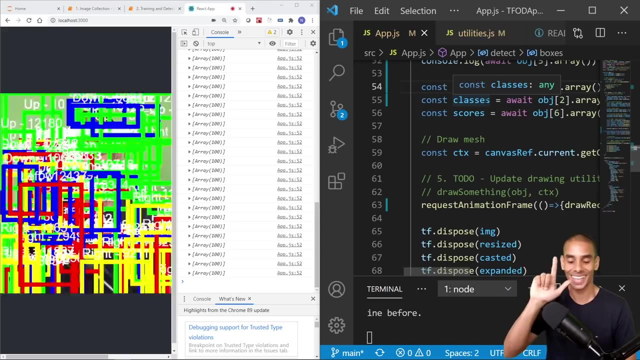 is we're going to set the value of the boxes array, so line 54 equal to five, so let's just minimize this right. so now we should be drawing our boxes correctly. oh, and we've remember we've set our confidence metric really, really low, so let's bump that up. 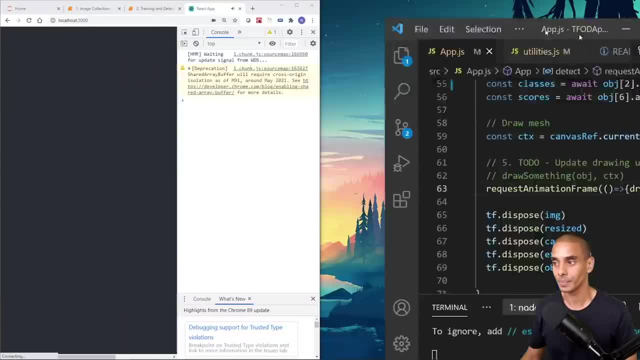 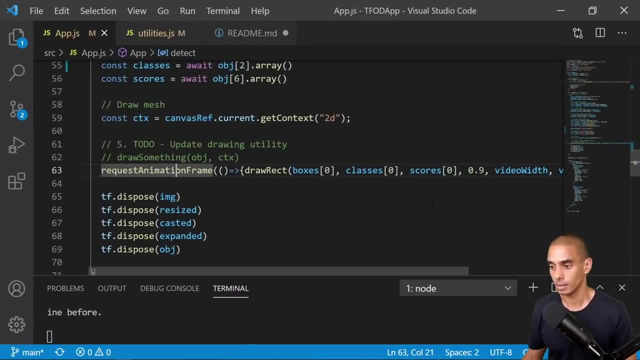 because right now it's losing the plot. so we're going to set that back to up to 90, so we're at least getting detect detections now. have we saved that? oh, we haven't changed our scores, so we've got to find where our scores are first as well. 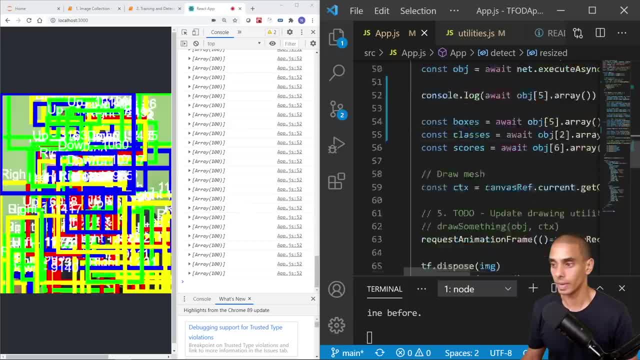 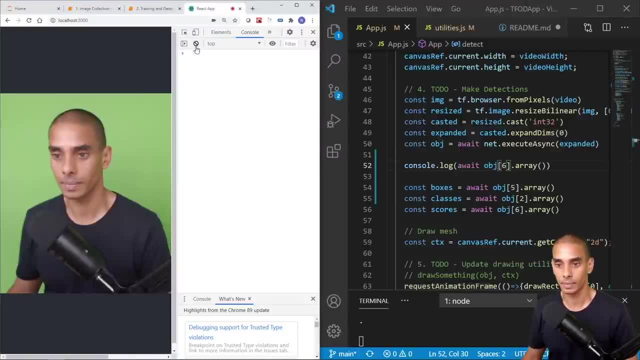 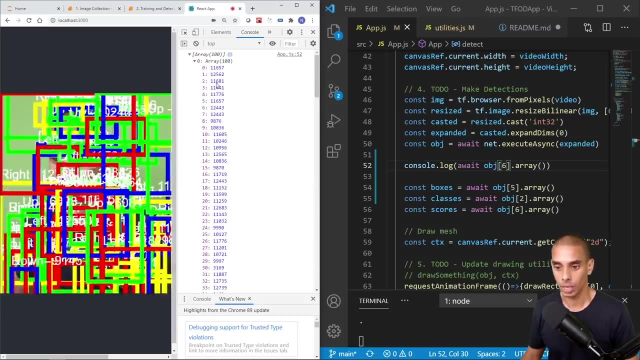 so let's go and change that for now. so let's zoom out a little bit there. right now it's going a little crazy, so let's see what object six is. this looks like it's just going to be a little bit crazy, so let's see what object six is. 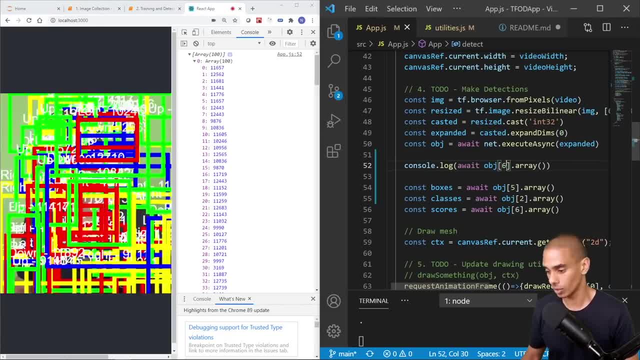 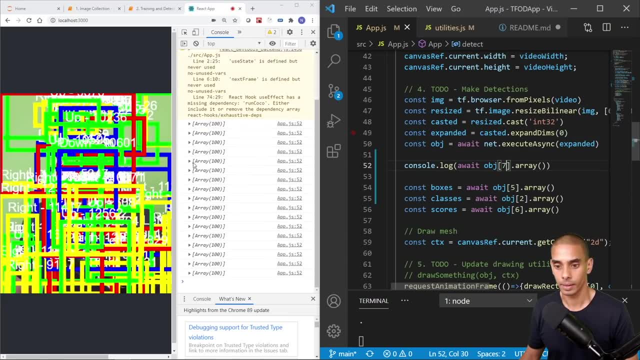 just going to be a little bit crazy. so let's see what object six is. all right, so it's not that. so this, i believe, is an index value, so we don't want that. try object seven. let's see what these values are. okay, these are our confidence scores, so they should be a value. 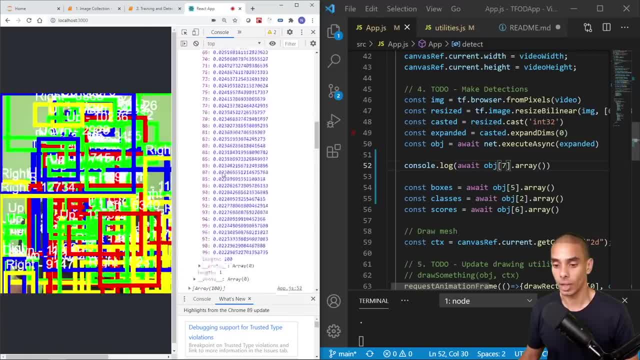 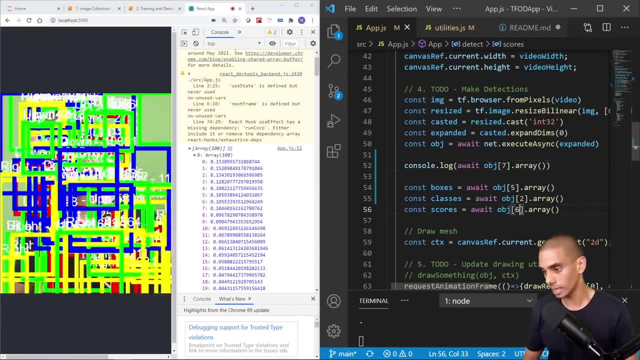 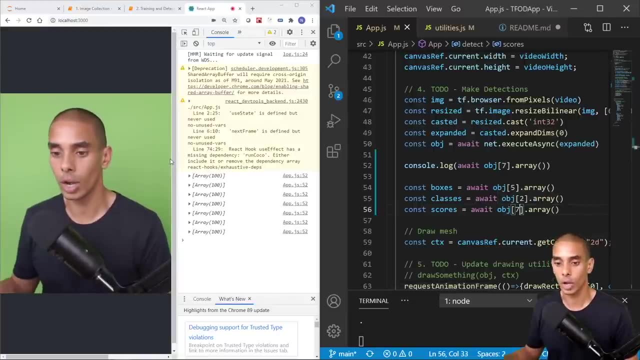 between zero and one. so i believe they're already sorted as well. so the highest confidence is going to be the top value. so what we need to do is just set this number equal to seven. let's do that, and we should have resolved it now. so again, you just got to work through it and all right. so if we take a look, 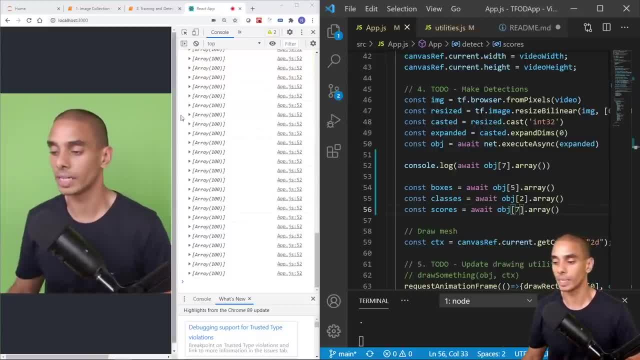 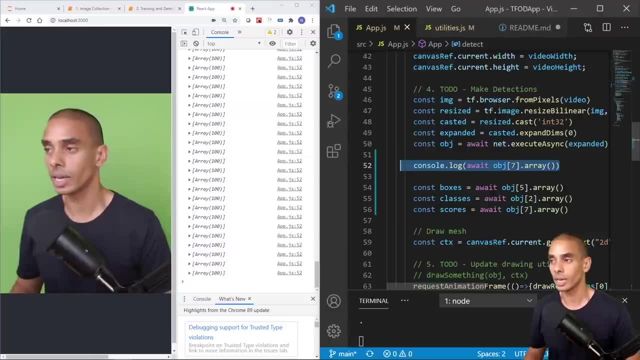 beautiful. so now we're working. so you might need to change this around, depending on what the results of your object array come out as. so again, but that sort of shows you how to sort it through. so your boxes are going to be a value. it should. you should have a number of arrays and each one 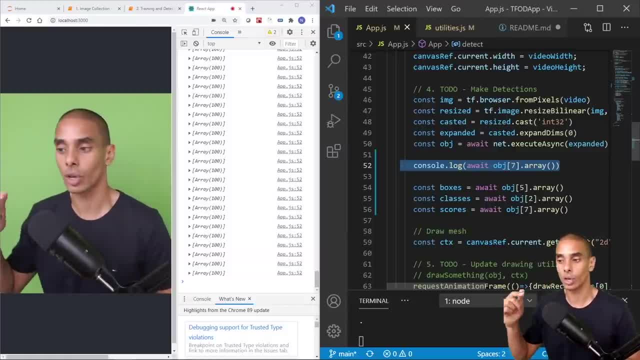 of those arrays are going to have four values, between zero and one. so those represent your coordinates. your classes are just going to be standard integers, so it's going to be one, two, three and four, or the number of the values that you're going to be sorting through. so that's. 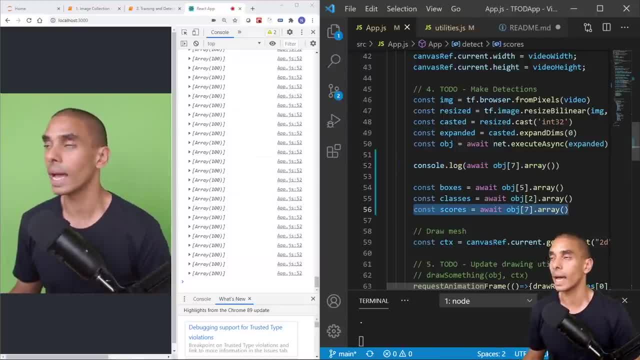 different objects that you've got in your model, and your scores are going to be the sorted array with the highest confidence value at the top. now let's go ahead and test this out. right? so we've actually gone and done quite a fair bit here, so we can minimize this, expand it out and, if we take a 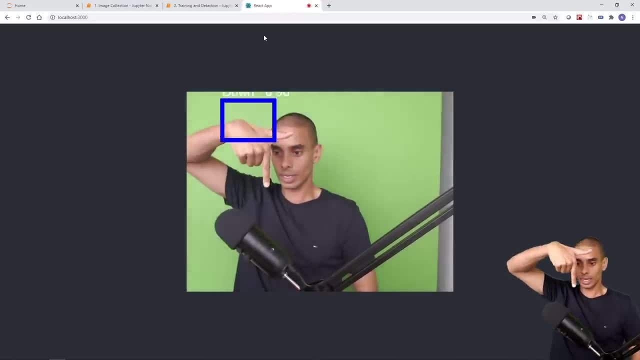 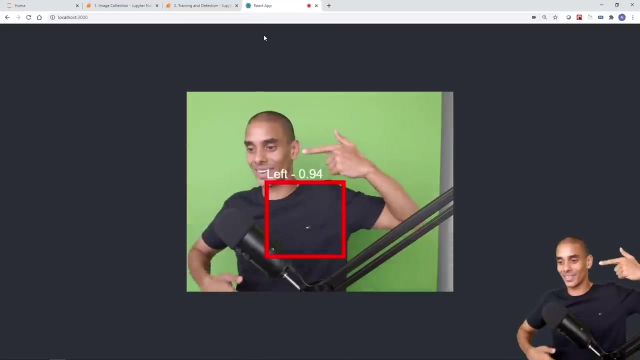 look, we're accurately detecting up. we go down. we're getting down. it looks like it's okay, the coordinates might be a little bit off, that's a bit better. and then left right and left, so left over my face, but anywhere else it's, it's detecting right. so and then we're getting right. 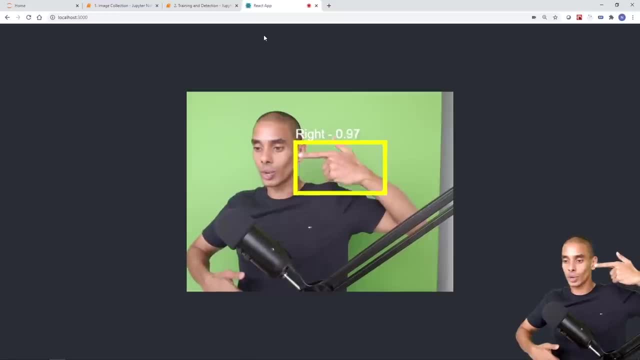 over here and again, reasonable confidence metrics, but that sort of shows you what's possible, right, like you could do so much with this. you could build apps, you could build directional apps. um, you could do sentiment analysis via the web. again, there's a whole bunch of ideas. so if you 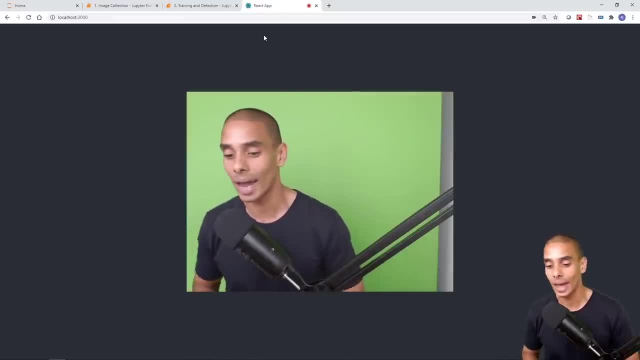 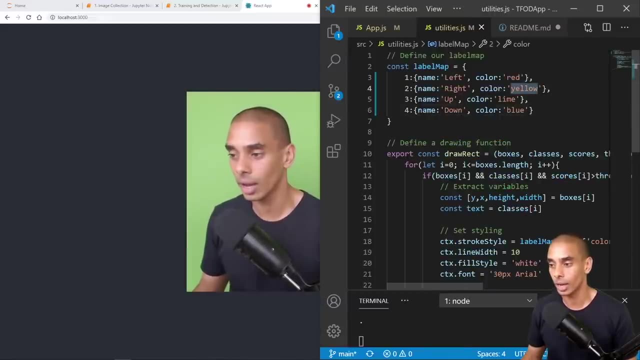 think of anything awesome, let me know. i'd love to hear your ideas. now you can also change the colors of the different um labels. so in this case you can just change it by changing the color attached to each different class, and then you can also change the colors of the different. 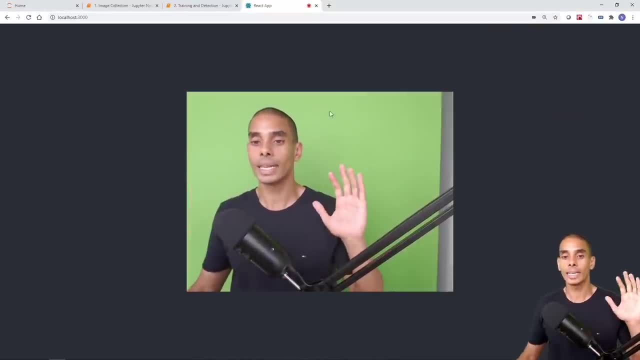 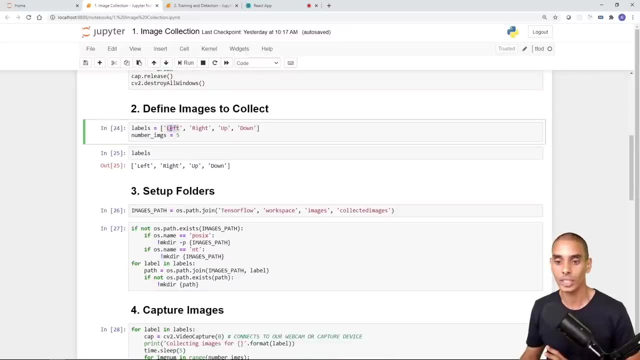 class. but on that note, that is project two wrapped up. so we've now gone and taken a raw object detection model. we collected our images again using our image collection script. we change it from left right up and down and again the performance on left and right wasn't the 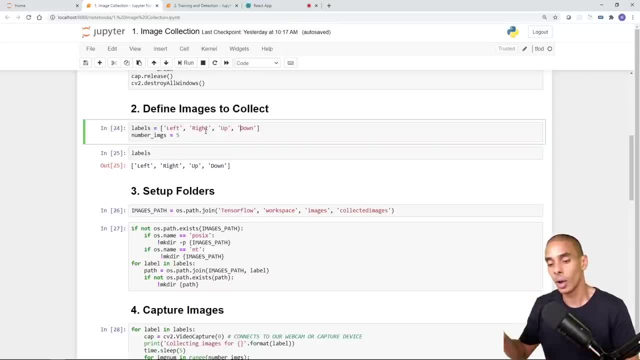 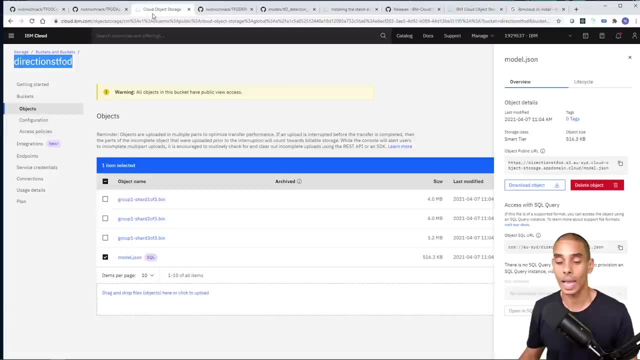 greatest, but remember, we took images right over our face, which isn't always that cool. we then went and trained our model using our regular training script. we then went and did a bunch of stuff as well, right, so we uploaded our model into ibm cloud to be able to host it. we then set 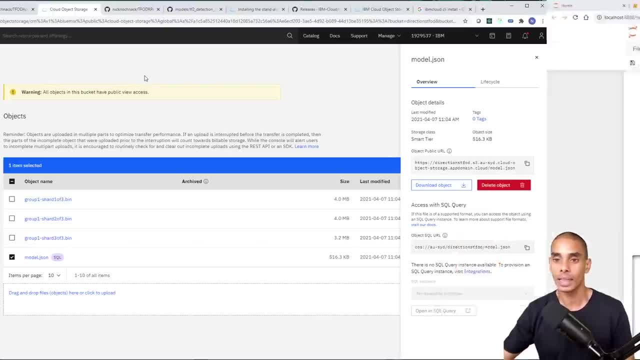 our image collection script. and then we went and did a bunch of stuff as well, right, so we updated our cause value so we're able to access it from our app. and then, last but not least, we actually went and updated all of our app details. remember, when you're updating in here a couple of 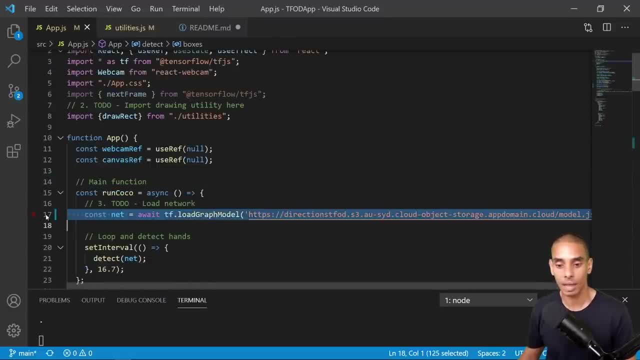 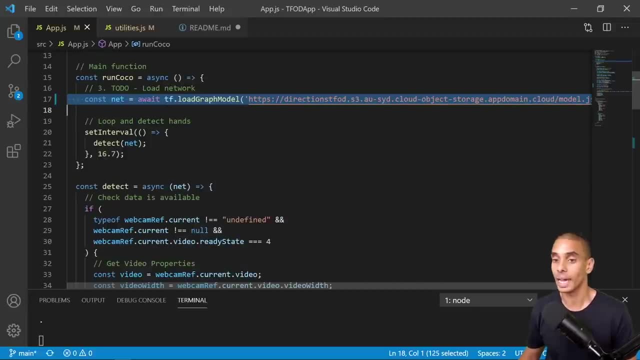 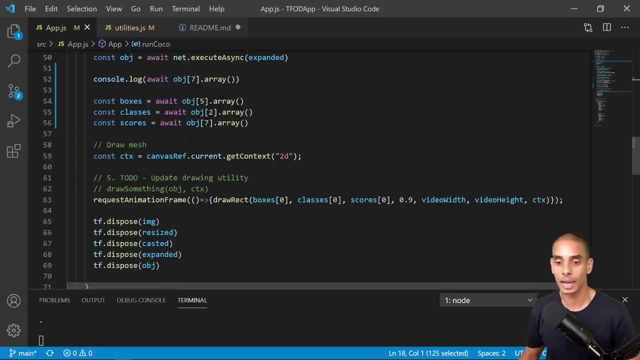 key things to do. so you need to go into your appjs file, update line 17- in this case it's line 17, but just look for the line that says tfload graph model. so you update that with your hosted model. update your labels inside of the utilitiesjs file, and then you might need to play around. 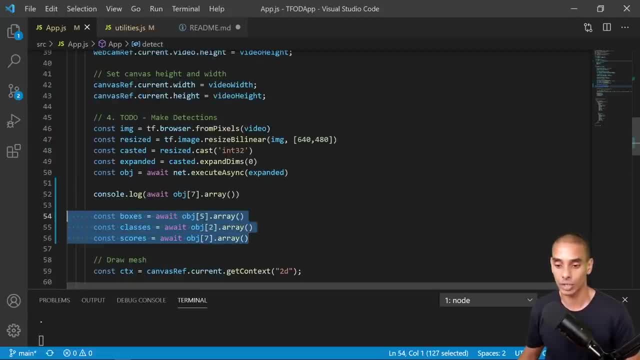 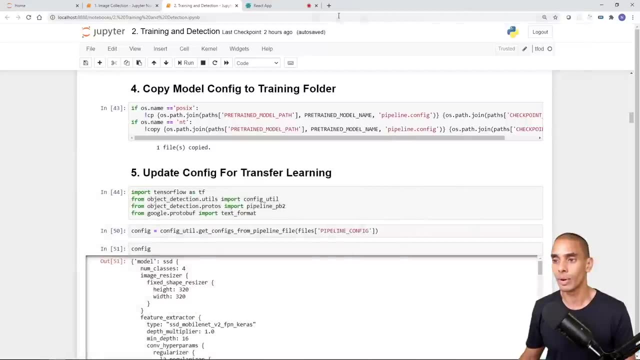 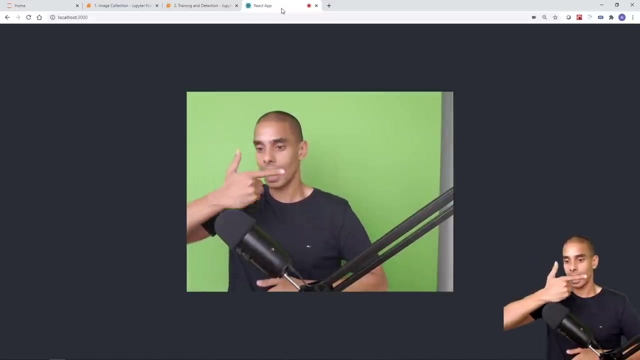 with your object detection array, so you might need to change these values, but in this case we are pretty much done so for project number two. so we've now got our real-time app up and running. it's able to detect up down left and right- pretty cool, right- and so what we'll do is, if you want to stop that app, you can. 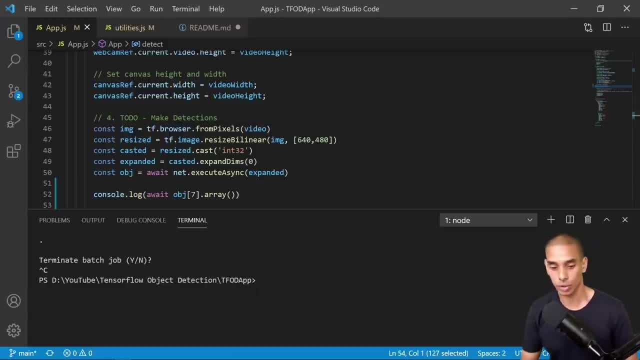 just jump in to vs code and just hit ctrl c or it'll be command c on a windows machine or on a mac machine. so we're going to go ahead and do that, and we're going to go ahead and do that, and we're going to go ahead and do that. so that is our app done. so you could do that with a whole bunch of 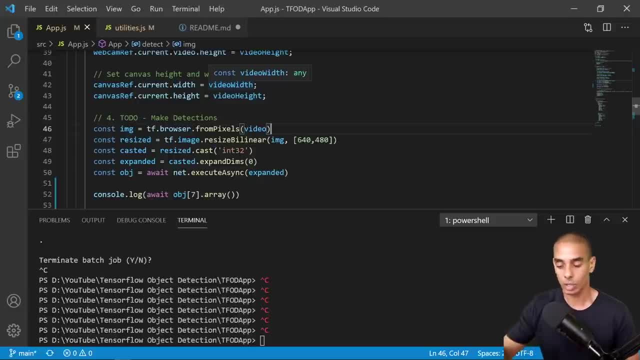 different models, so it doesn't just need to be your directions model. we did it for the sign language video. so, again, if you want to take a look at that video, by all means i will link to that in the description below so you can take a look at that. but now we are up to project number three. 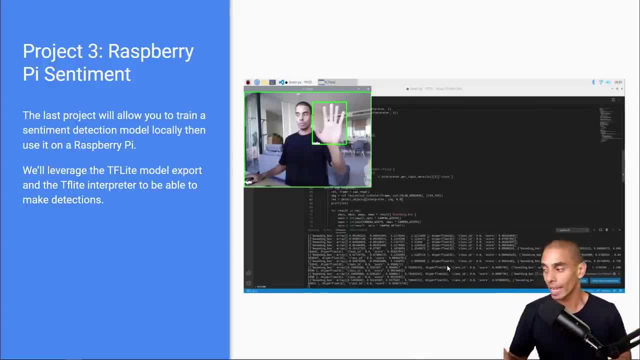 so raspberry pi sentiments. so we're going to keep this one relatively simple. so we might try one or two classes, so maybe happy and then like sad or something like that. so we'll um. so, obviously, running object detection models on a raspberry pi uh does have certain things that you sort of need. 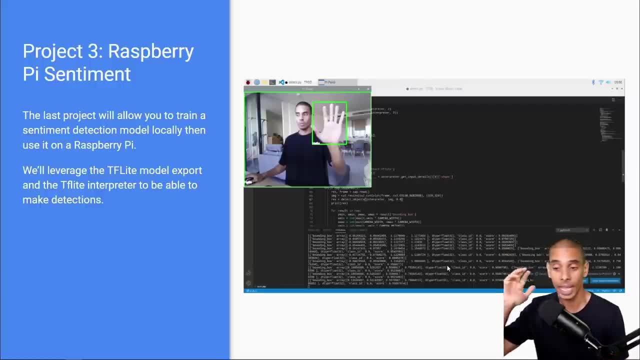 to cater for. obviously i don't have a gpu on this particular one, it's just a raspberry pi. there's nothing fancy happening there, just a raspberry pi. now you can get a gpu extender like, for example, coral um. you can also get like jets and nanos or sort of linux style devices like that to be able. 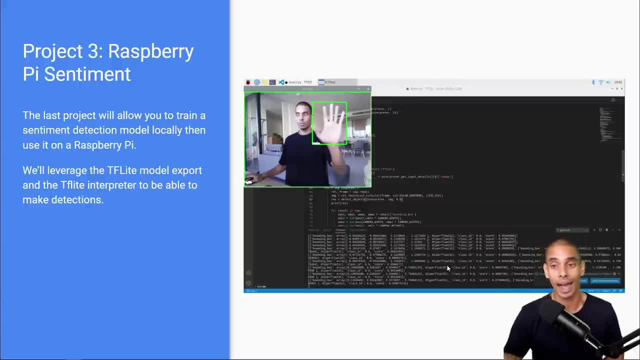 to run it, but we're going to use a standard raspberry pi box and test this out. now i've got it sitting right next to my webcam, so we're actually going to remote desktop into our raspberry pi to be able to work with it and we should be able to run similar detections to what 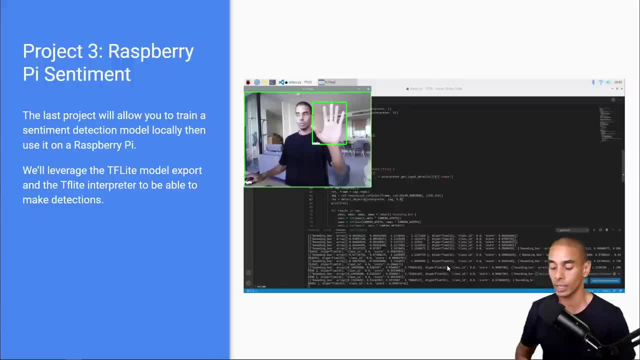 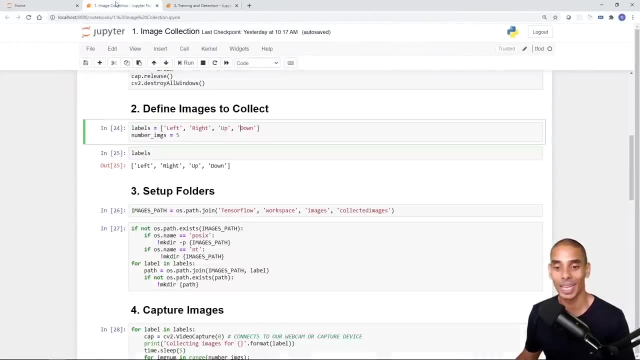 we've done already. in this case, we're just going to be doing it from scratch. cool, all right. so what we're going to do is kick this off and again, as we've done before, we're going to be doing it very much in the same manner. so we're going to be collecting our images, training our model, the. 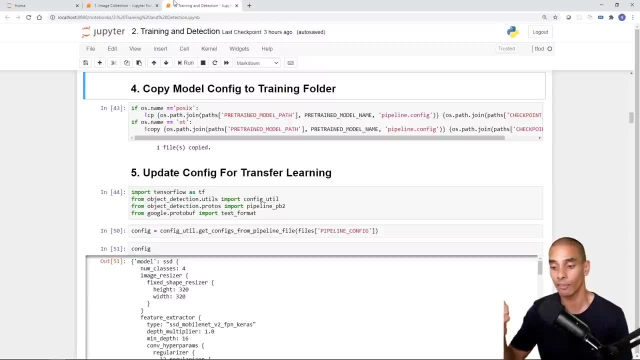 key difference between this particular project and the last two is in the first one we just used a straight up um. we used a microscope to be able to make those detections. so for our tfjs app we converted to tfjs to be able to run it. now for our raspberry pi model. 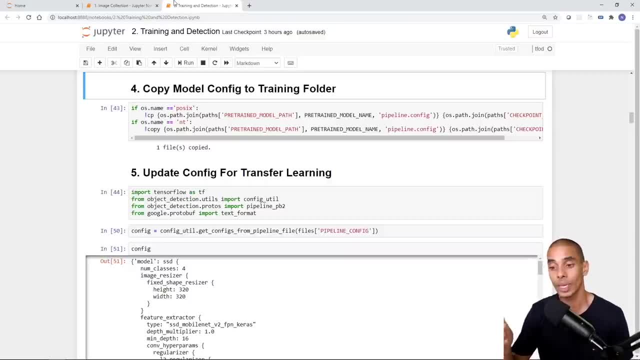 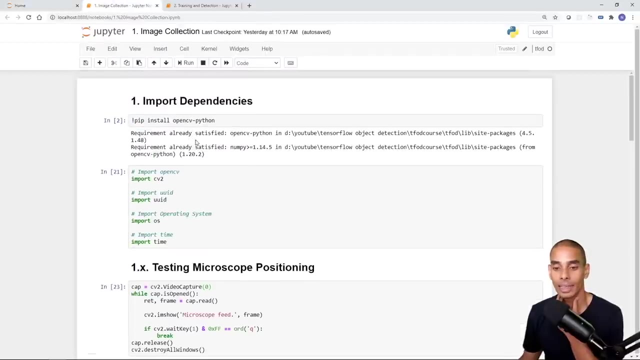 we're actually going to be focused on converting this to tf light, and we're going to be using our specific model in a tf light format. so let's go on ahead and do this now. what we'll do is we'll first up, open up our image collection notebooks. again, nothing crazy there, and this time rather. 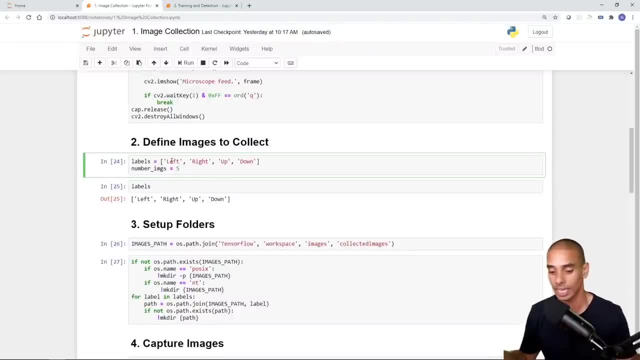 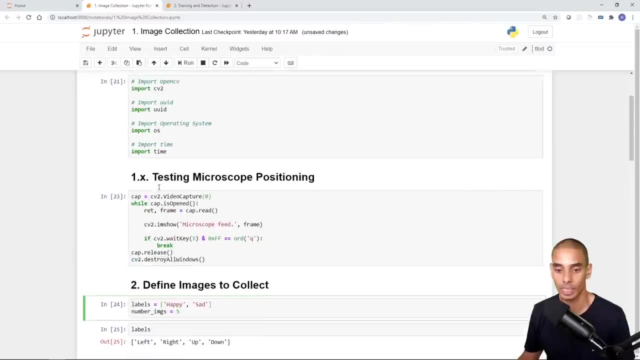 than having so for our directions model, specifically our tfjs app, we had left right up here. we're going to have- let's just try- happy and sad, so we're going to update those. so we're really just going to have two objects now. you could even try one object, depending on performance. 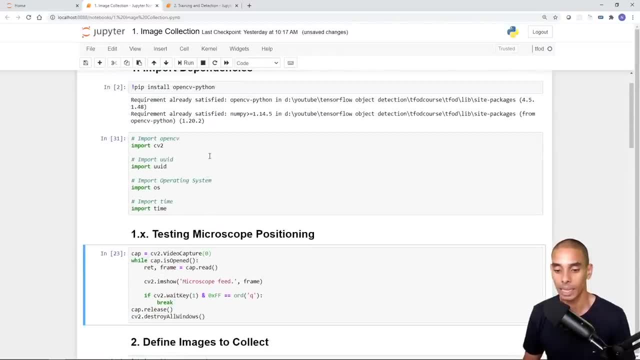 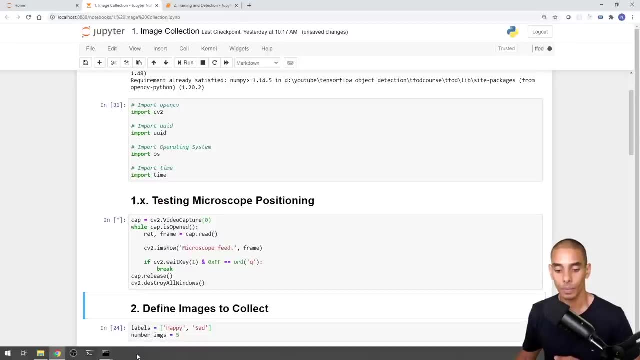 and see what that looks like. so again, we're going to import our dependencies. there's a no need. let's actually test our webcam to make sure it's pointing at me appropriately. let's wait for that to open up. cool, that's all good. so we'll move over to here to collect our images and maybe we'll do. 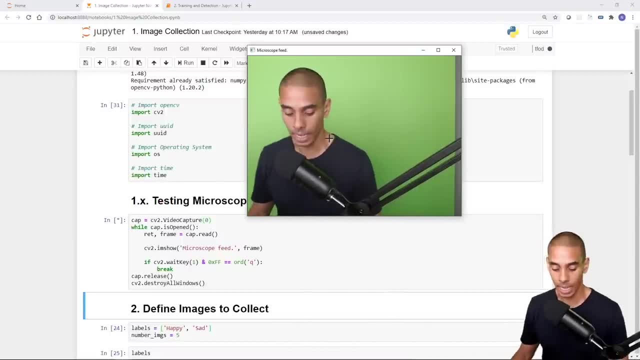 our face covered. so we've got really clear and defined objects, because, again, the camera that I've got on the raspberry pi is not as good as the webcam that I'm using on my PC as well- another thing to keep in mind. so let's go on ahead and do this. so we've got our labels and we're just going. 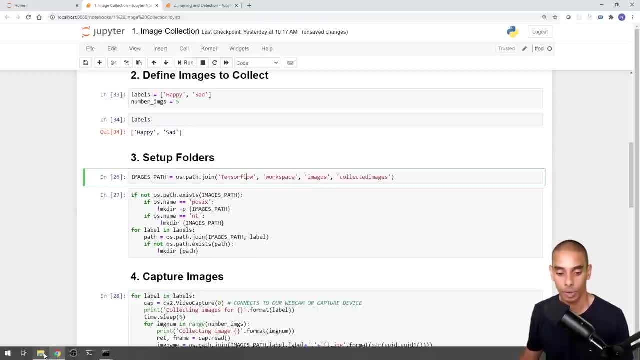 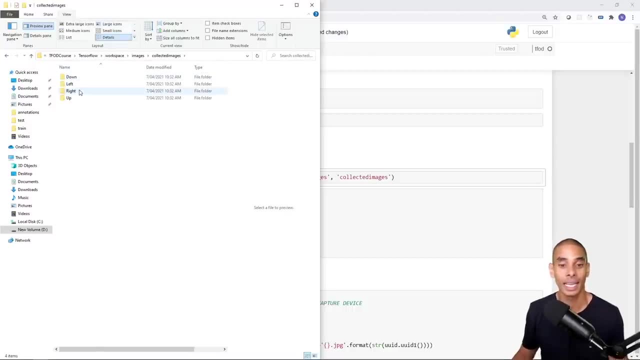 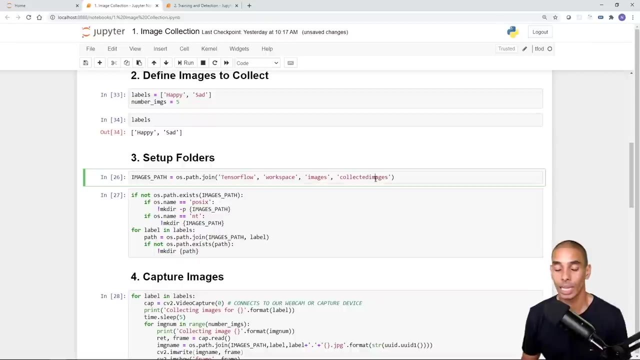 to collect images of happy and sad. we should probably clear out our existing images. so if we go into tensorflow workspace images and then collected images, remember we had the down left up images so we can delete those. we don't need them anymore. now what we're going to do is collect our 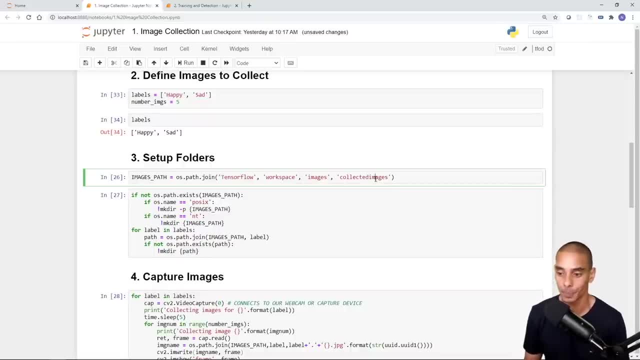 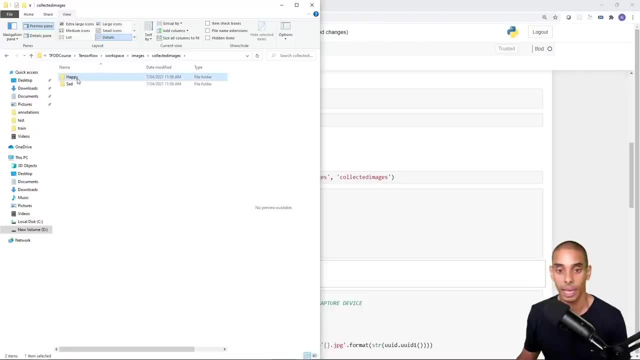 images for our sentiment detector, so happy or sad. so, first up, we need to create the paths, and this is what step three does. so that should have created our path. so you can see we've got happy and sad and what we're going to do is collect our images. so, again, we're going to collect five images, but 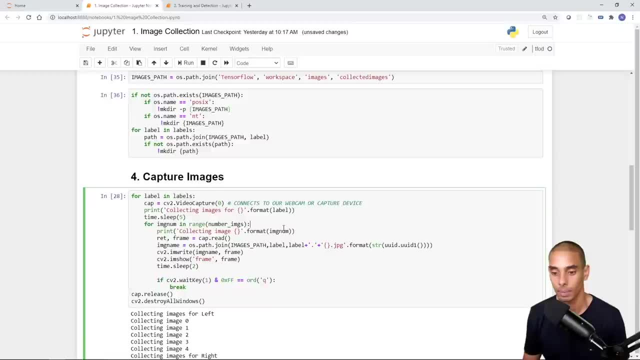 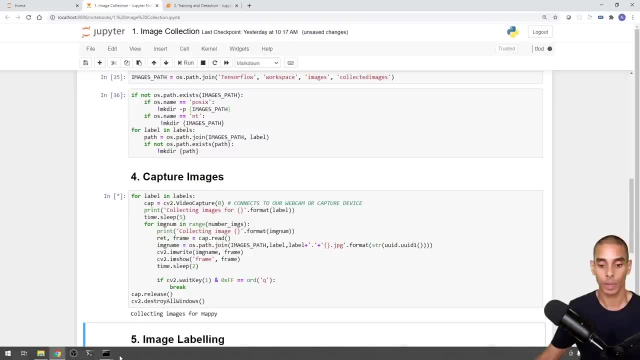 you could change this if you wanted to. so I'm going to get into position and collect them. so let's run this and we'll wait for our little pop-up. sorry, I'm a little away from the mic. oh no, it's running. that's not happy. 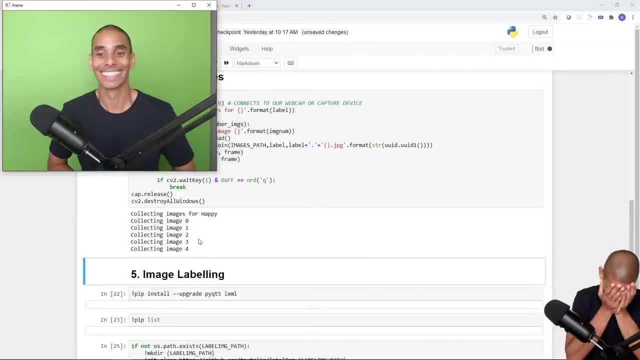 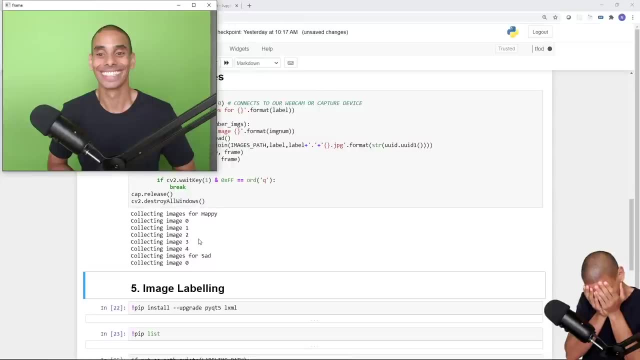 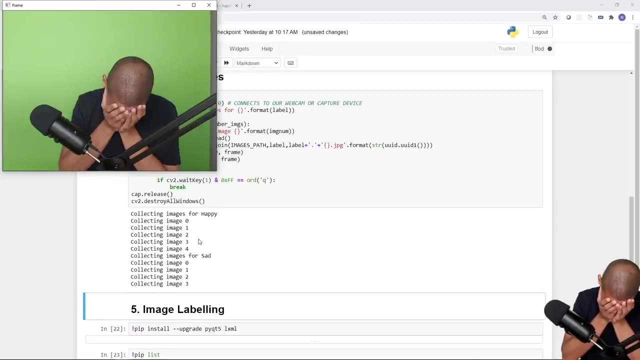 right, and then I think we're up to sad, so the sad will be covering our face. sorry, you probably can't hear me. I'm trying to see through my fingers. all right, cool, all right. that should be all of our images collected, so let's go and take a look at what. 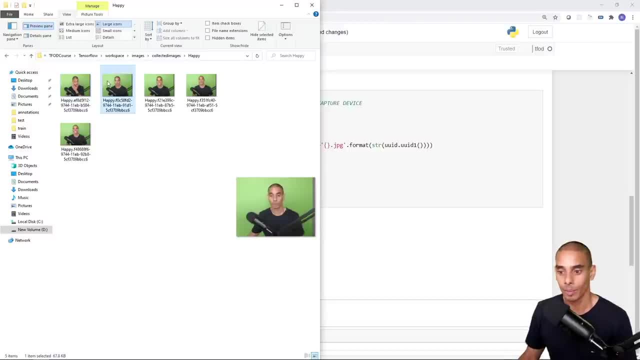 we've got so insider happy. we probably should. I love this phone. this is great. this is me just dumbstruck. okay, so we're gonna delete that one and we're gonna delete that one. this is okay. this is now. we want me smiling in them? all right, cool, this is fine. 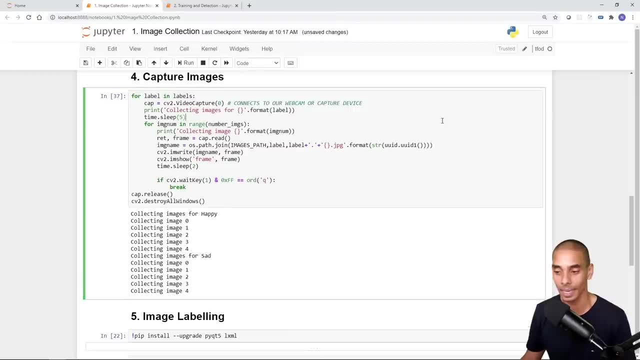 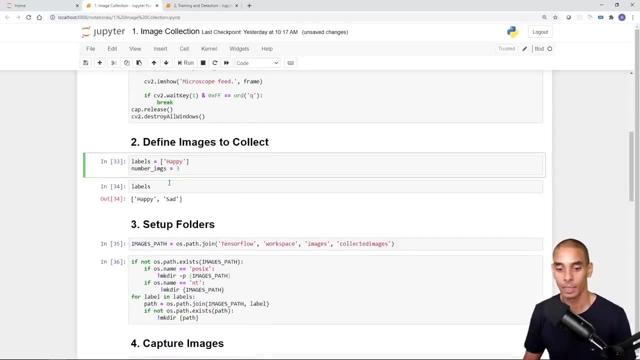 for sad. so sad is us covering our face. so we're going to do happy and let's collect some more images of happy. so remember, we can just isolate what we want to do. so we want three more images of happy, so let's do that. so all i've done is i've just removed sad from our labels, array or labels. 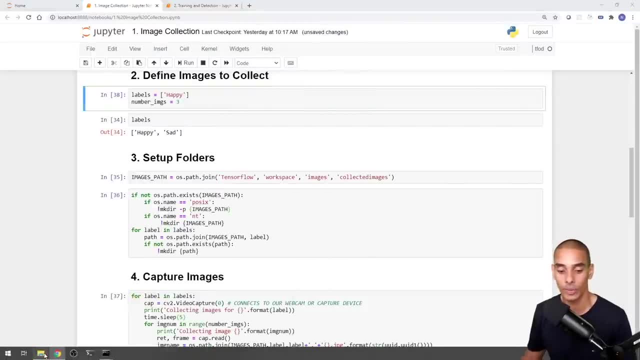 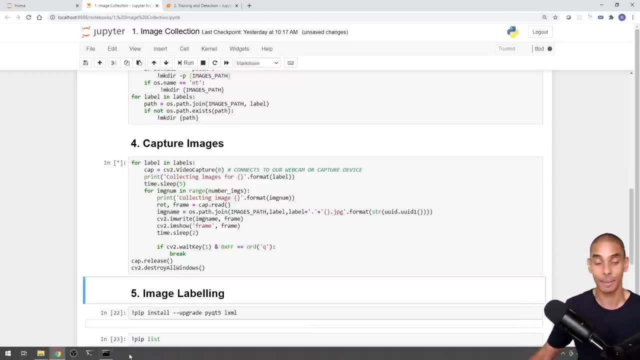 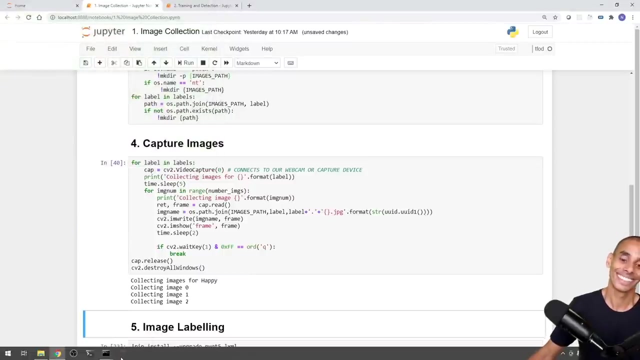 list if it's python, and then we want three more images. so we've got an even number of happy and sad images. so let's run this and then run our capture again, and i'm going to try to be happy this time. i'm just wait. okay, cool. so let's go and take a look at our images again. 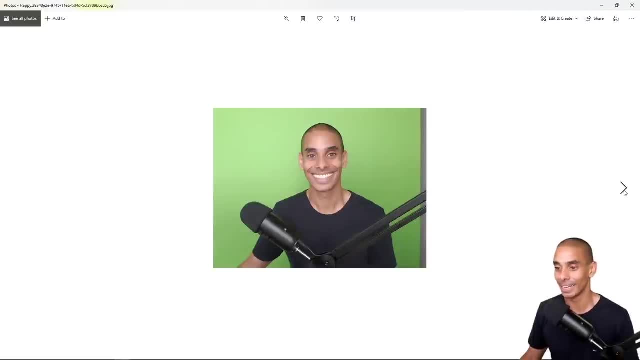 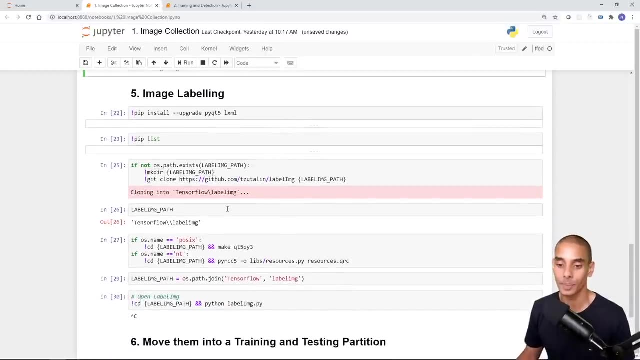 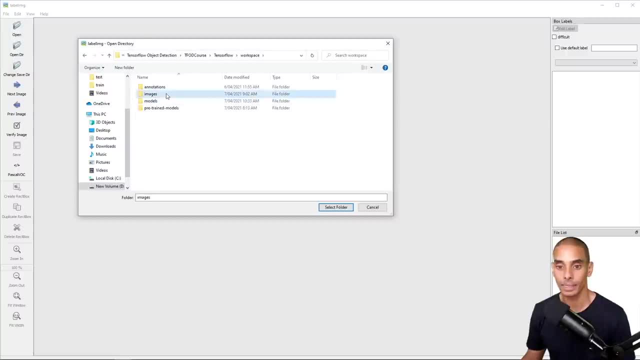 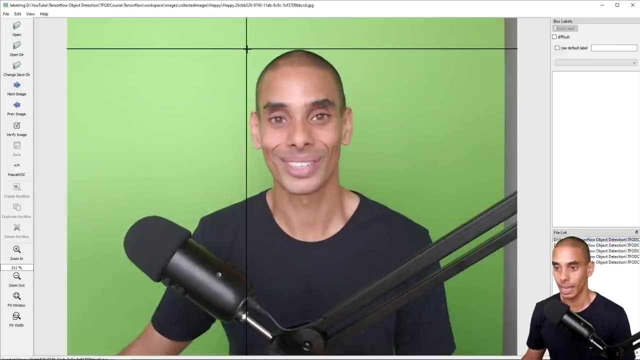 it. so we're going to go back into our images, so workspace images, and then collected images, happy, and do our labeling. so we're going to say that this is me happy, save that, save that and again i'm doing happy post, happy capitalization is super important. 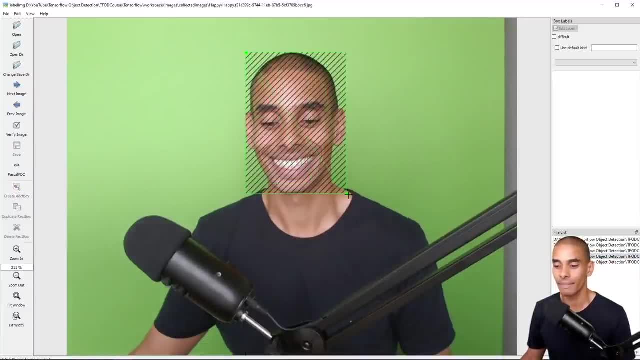 or case is super important for this. now again, for the most majority of this course, i've been doing it with a green background, but you could obviously do it without a green background or a green screen. i have just been taking the photos with the green screen, but that's okay, it will still work without. 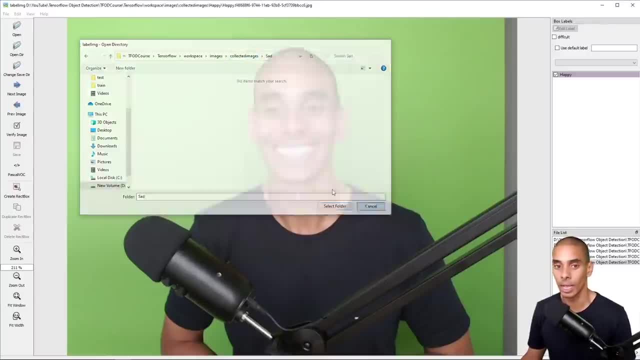 it. um, because you saw that we took it down and we tested it without the green screen. now, what we're going to do is switch into our sad folder and do the same thing. we're going to do: a s signing, okay, to get the bottom view through and a not chaser view. that's the bottom view, and so then, 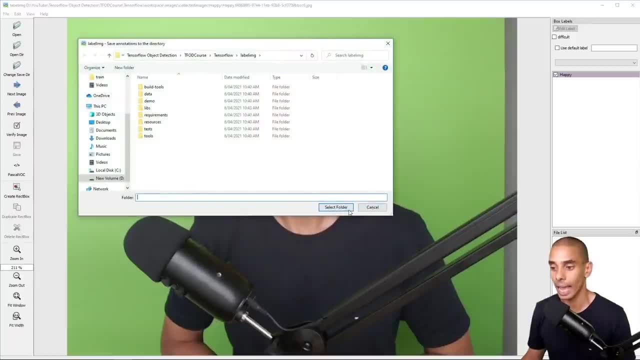 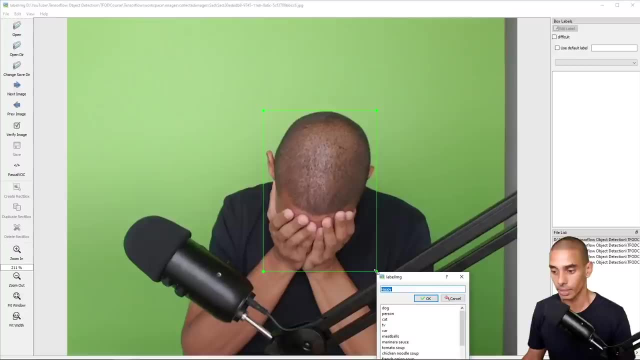 we're going to go into any of this and then we'll try and find out stars. completely, any of us are not adding any, just a maximum success. so cheese andilah, chaser monitoring building to philip and do the same. so that's our already done. happy let's do sad. so let's capture everything to there. 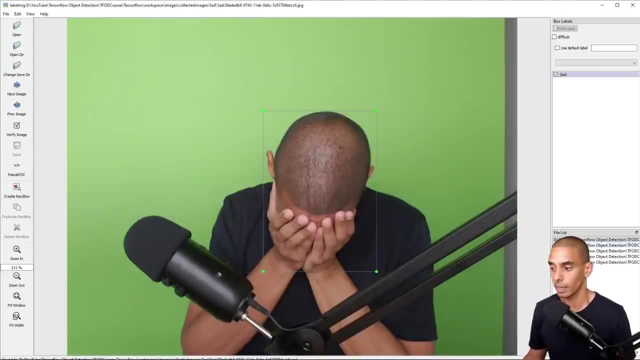 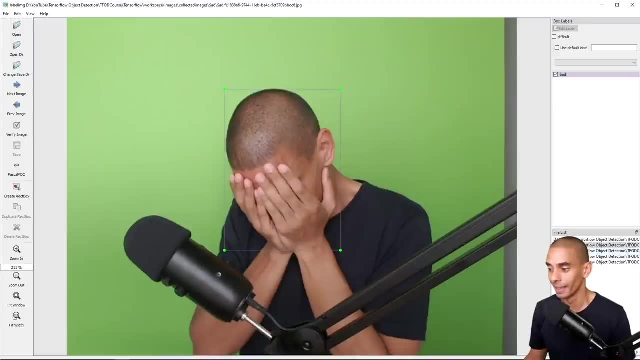 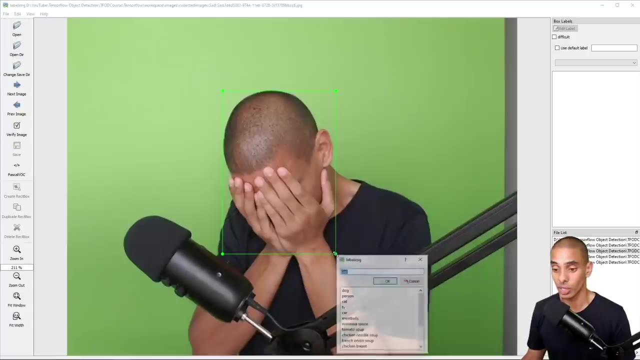 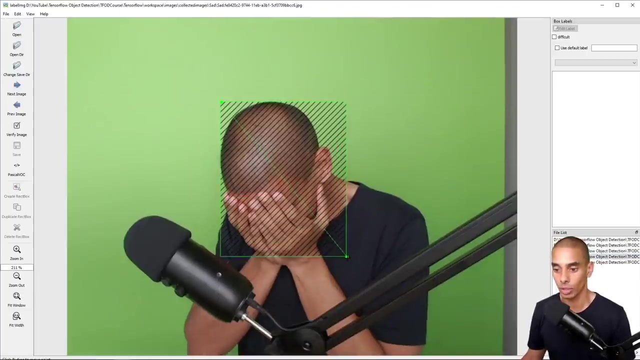 so sad, sad nick. all right, then we're going to do the next one and we're good, and again i'm just keeping going through, i'm making sure my detections or my labels are really as close as possible to correct sad, and i'm saving each object again. so this makes sure. 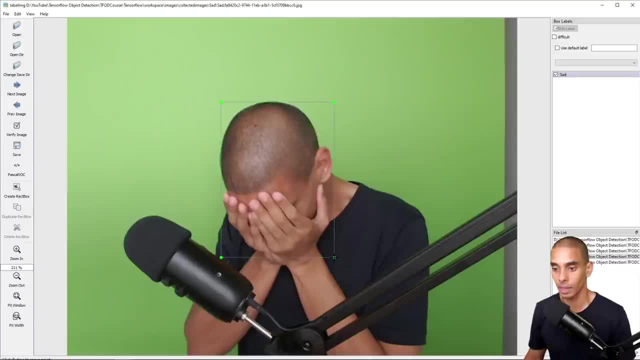 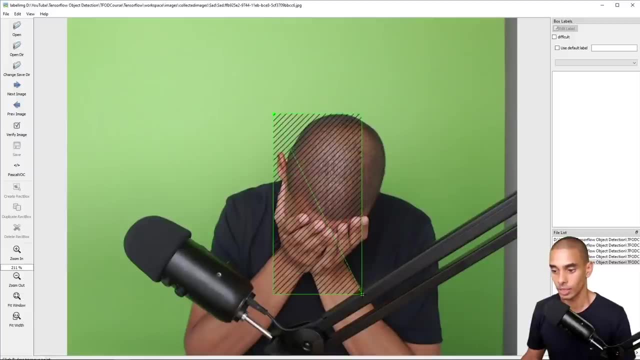 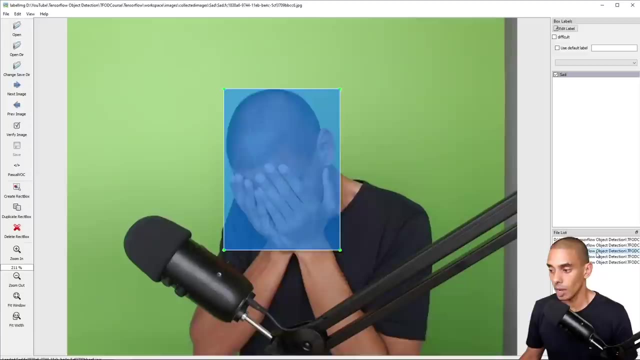 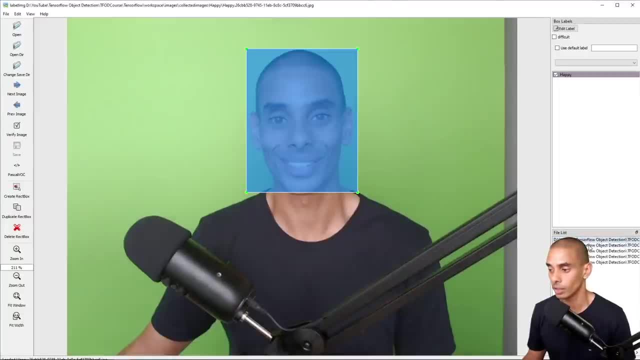 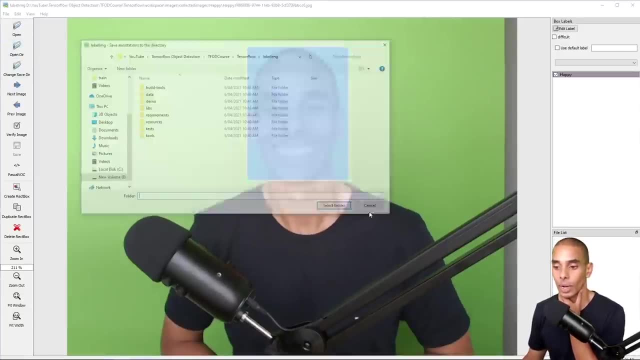 our happy directory because i wasn't sure if we saved all of those fine fine, fine. this is also another thing to note right, so you can go back and open up the directory of images if you wanted to go and update a label, for example. so say, for example, we wanted to do microphones, we could go. 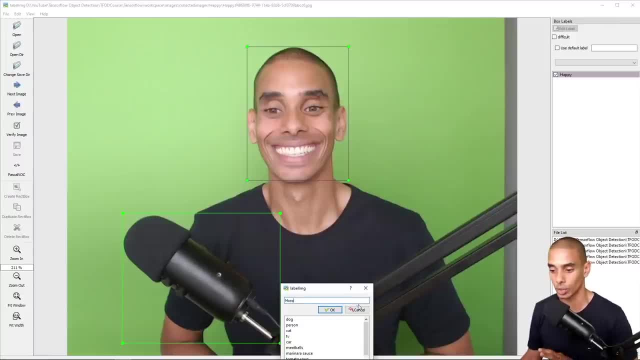 and label the microphone and type in microphone. i don't want to do it because it's going to screw up, um. but in this case we- and we only want happy and sad for this- but say, for example, we wanted to edit it, like i didn't capture my full chin, we can go and make that update and hit save to be. 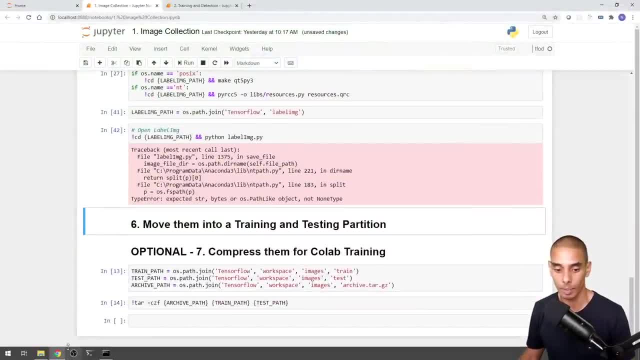 able to go and overwrite. oh, it looks like i've just gone and killed that off. let's go and make sure that we've still got that. uh, yep, so we're all still good, but you sort of get the idea. so you can open up a folder, you can. 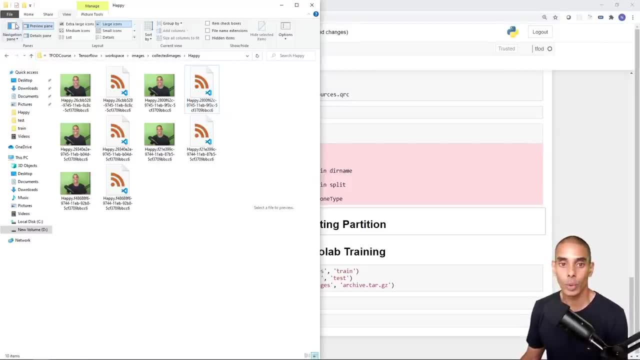 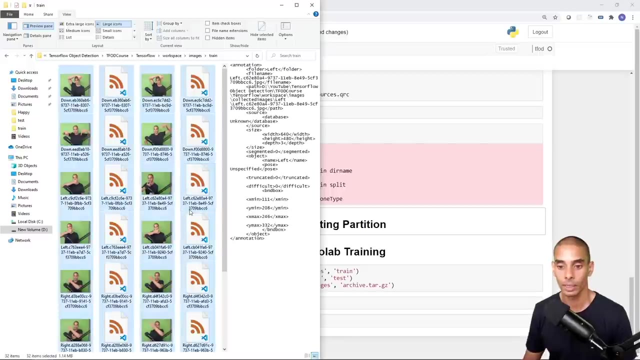 make those updates. all righty, now, as per usual, we are going to go on ahead and save our and move our annotations into our training and test folder. so i'm going to go back into our images folder. i'm going to delete everything from our test folder and our train folder that these were all. 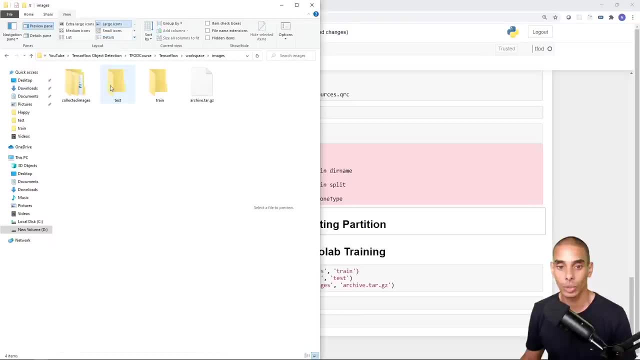 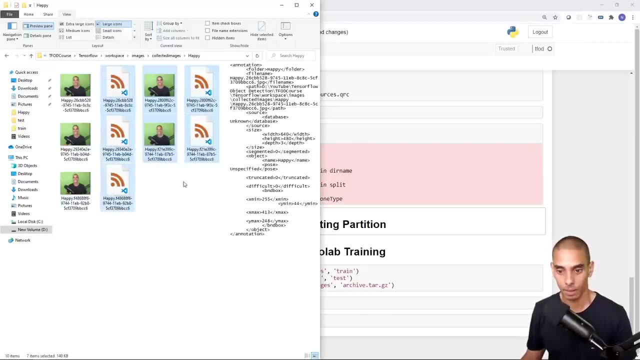 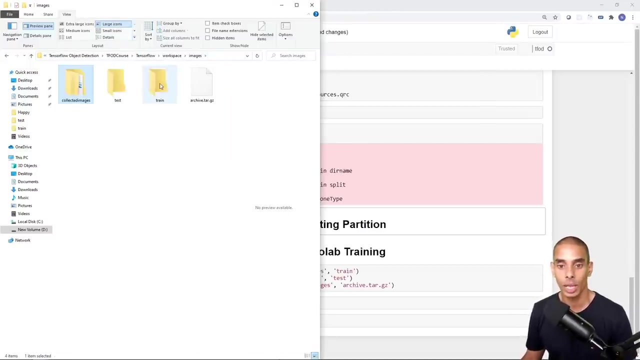 about directions and we are going to go and grab our collected images. so happy so we'll grab four and four. nope, yep, so those. so again, remember, you've got to grab the annotation and the image. we're going to paste those into train. so this will be a what. now it'll be a 80 split again. so again. 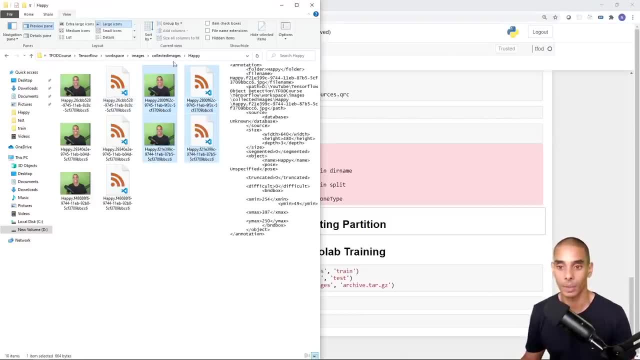 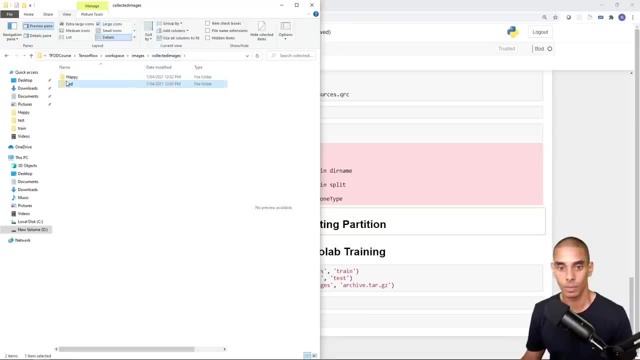 we've got one image left inside of our test folder and then we'll do the same thing with sad and we're going to copy one of these images. we're gonna copy the first one here. let's copy this as well. sorry if there's a little whining on the microphone. i've got the raspberry pi running already, so 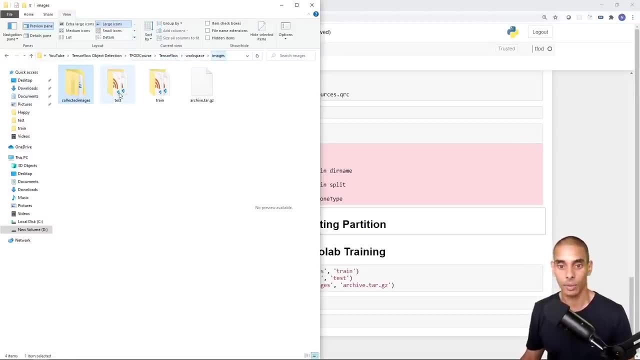 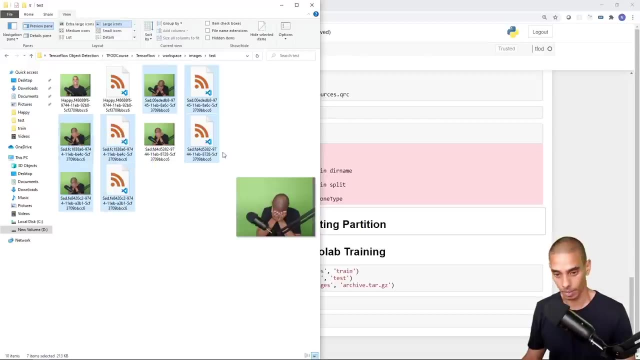 it is a little loud and we're going to copy this and then we're going to do our test images. oh, that's not right. so these test images should actually be inside of train, so let's cut those. place it into train, cool, so eight images in train and we should have two images in test. so we got to go get that other one. 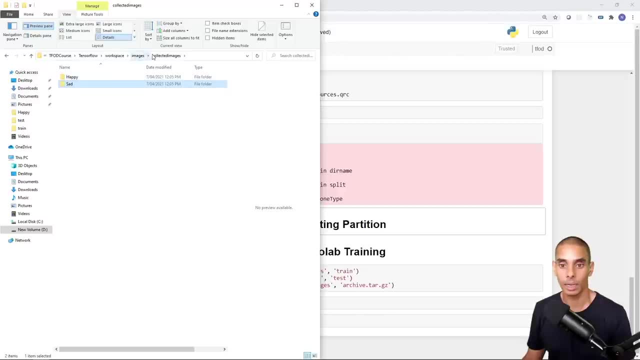 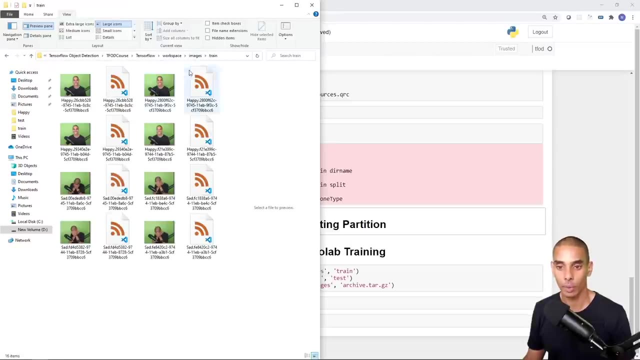 so let's grab this sad one and let's paste that in. okay, cool, we're good. so if we go into our test folder, we've got two images, and if we go into our train folder, we've got eight images. pretty cool that you can build a like object detection. 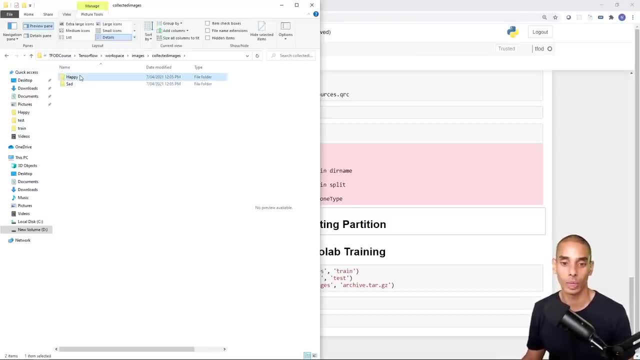 model of just eight images, right. so again, this is super powerful what we're doing here, so happy. i'm pretty sure we've already moved that so we can actually go and delete our folders inside of collected images. we don't need those anymore. okay, now the next thing that we need to do is 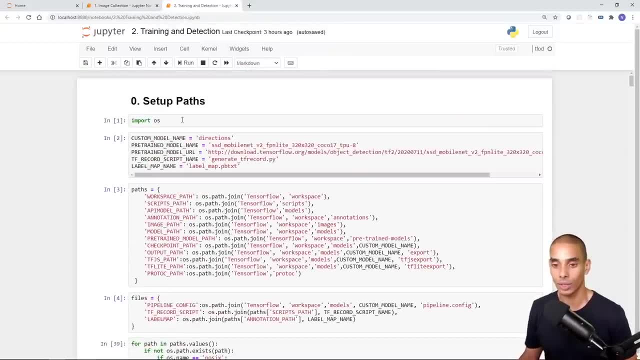 go back into our training model. so we're going to go on ahead and train a new model. so this time we're going to call our model sentiment. and again it's not a full-blown sentiment model, it's just a high-level object detection model. but 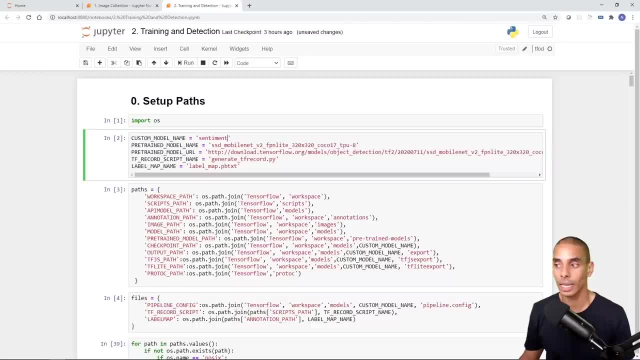 you could obviously extend this out and we are running and again, make sure you're in your virtual environment, you're in your virtual environment, you're in your virtual environment, you're in your environment. so we're going to hit, go through all of our path steps, so we'll import our operating. 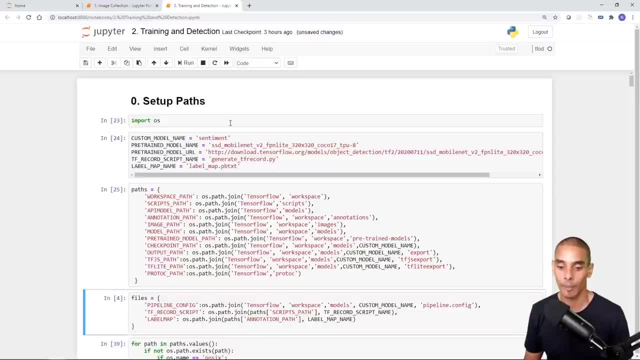 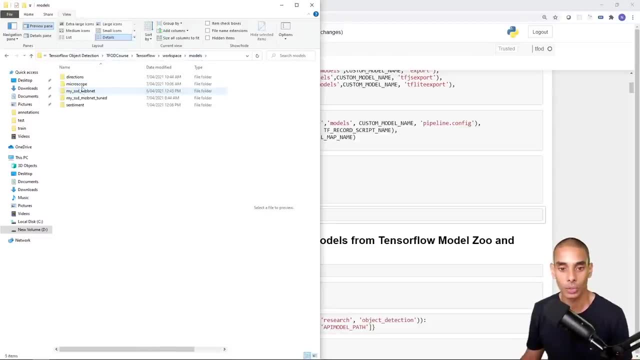 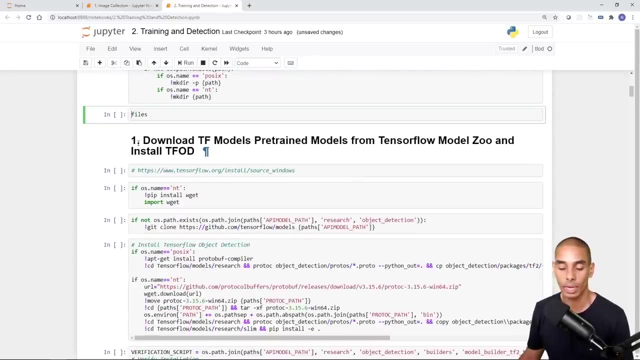 system. set up our new custom model name, set up our paths files. we'll actually create the paths. so now, if we go in to our workspace models, you can see that we've got our sentiment folder already set up. now again, we don't need to do step number one, because we did that right at the start. we set 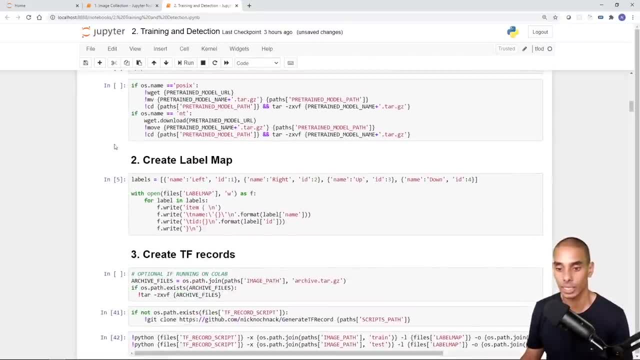 up our tense flow models, our model zoo, and we installed tense flow object detection. now all we need to do is we're going to go back to our training model and we're going to go ahead and do is update this label map. so, under step two. so we're going to say: what was it? happy and sad. 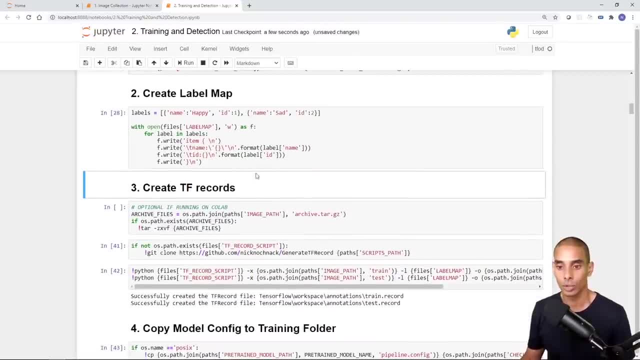 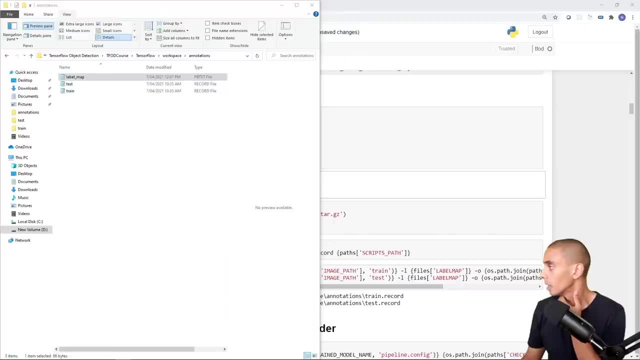 save that and then we're going to hit shift, enter to create our label map. so if we go and check that label map, if we go into workspace annotations, let's open it up inside of vs code. that's looking good. so we've got happy and sad. 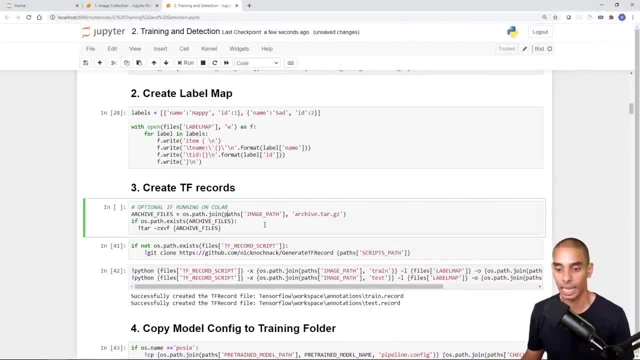 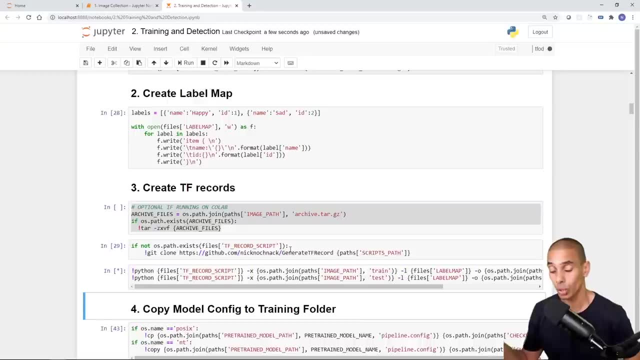 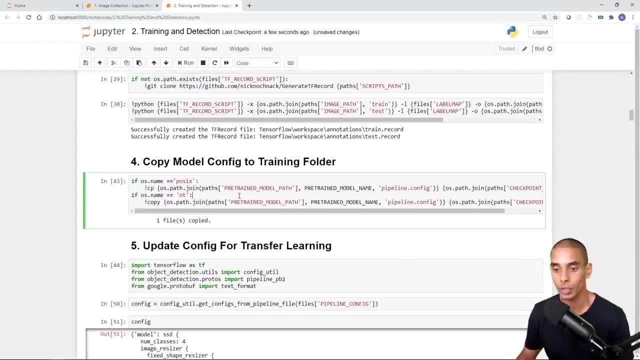 we're good to go there and then we can create our tf records. and again, this step over here we can skip that- that's the collab step- and run this and this cell- and this is going to- should ideally create our tf records without issue. cool, so that's gone and created them, as per usual. 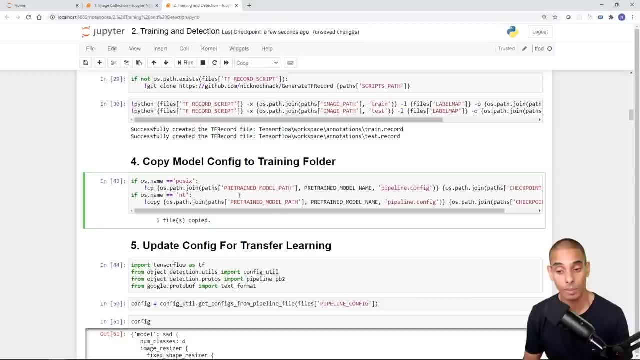 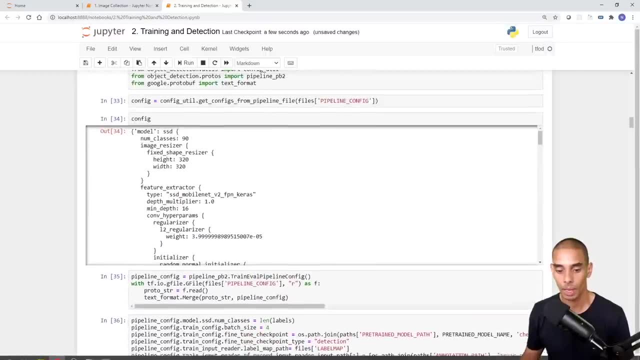 we're going to copy our pre-trained model config to our custom model folder, so let's do that. then we're going to update it using these steps. we can go and double check that it's gone updated. so if we go into our sentiment folder and open up, 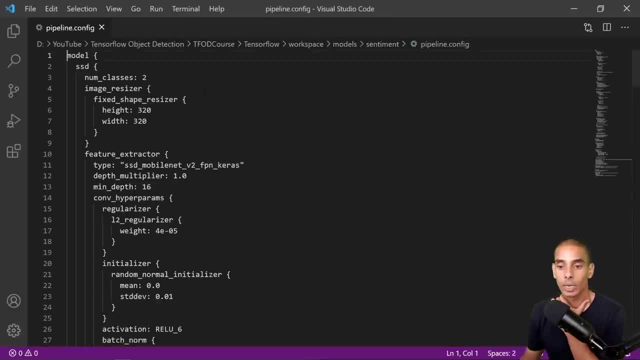 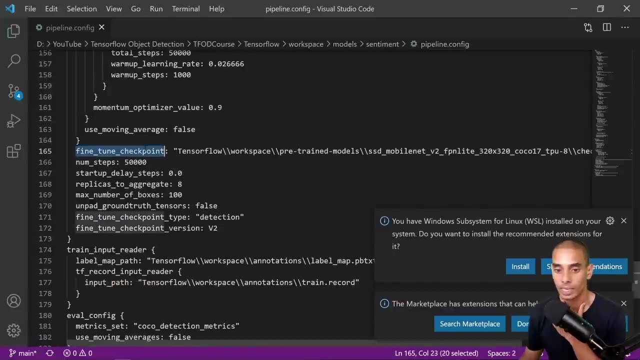 this pipeline. as per usual, let's open up one of vs code got the correct number of classes and if we scroll all the way at the bottom, most importantly we've gone and reset the fine tune checkpoint, the label, map, path, input path, so on and so forth. so we're good to go. 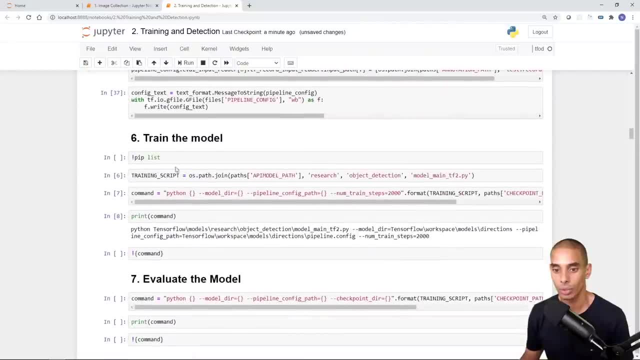 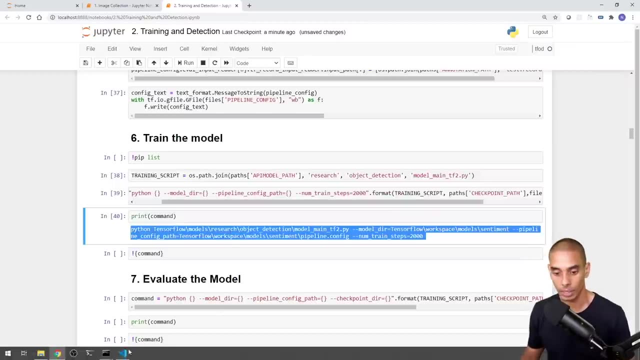 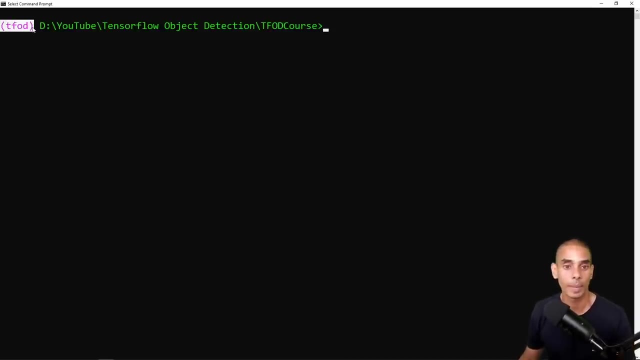 cool. now the next thing that we need to do is, as per usual, train our model. so we're going to generate our command and then we are going to go on ahead and paste this into a command prompt. so, again, as per usual, we need to make sure we have the virtual environment enabled and we need to 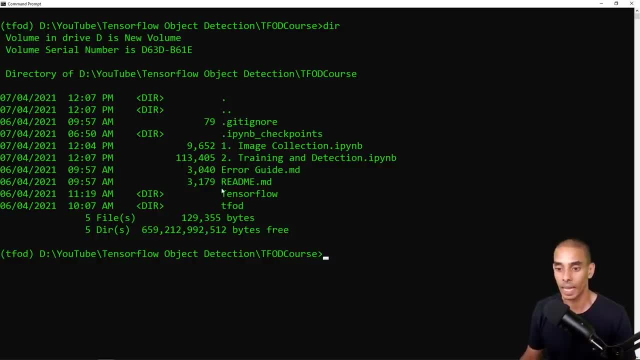 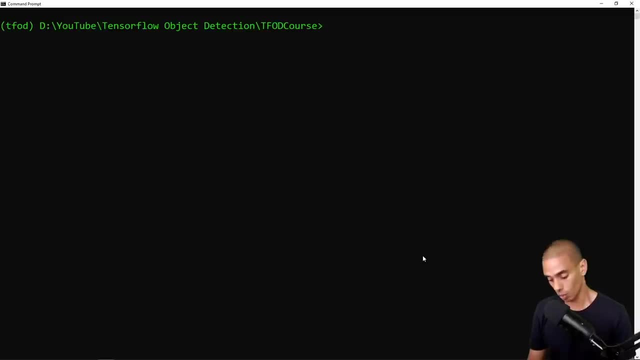 make sure we're in the top level directory. so again, from here you should be able to see tensorflow and tfod. and then we're going to go in a head, paste our training command and then we'll let that run and we'll be right back. so i'm going to paste it in and we'll be right back. it's cool, so it's. 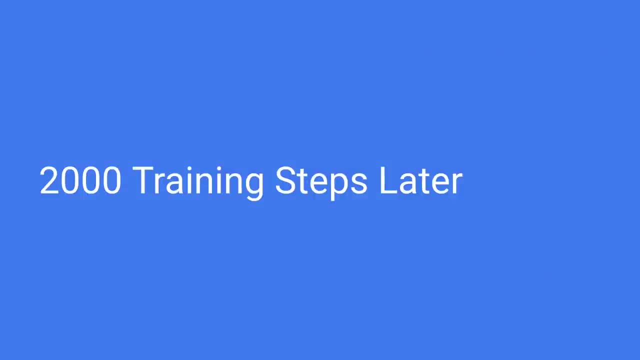 kicking off, we'll be right back, let's hit it up. so that's the little tip. very useful to see, alrighty. so that is our sentiment: modeled finished training. that was how you generate, or مث, compromise, anything that is going to be gaining visitors in this environment. trying to get the data, or maybe simply 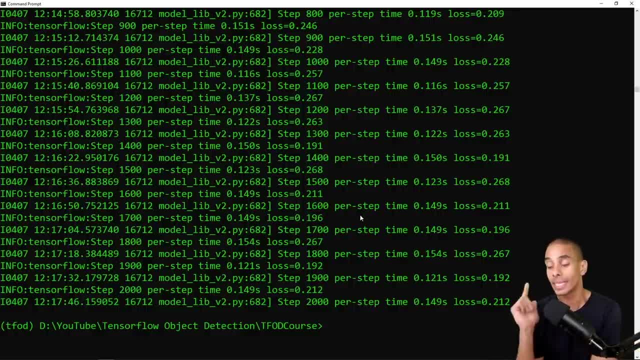 get like bothness and tradition out of. it's kind of an application that you input across yourória page, but that's how you engage it: having those performance images. so again, as per usual, we need to make sure we have the virtual environment training Now, full transparency. I did run into an error when I kicked off this training run Now it. 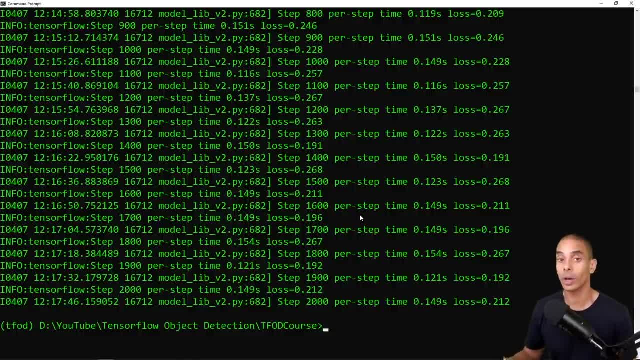 wasn't anything that we wrote in terms of code. it was because all of the VRAM available on my particular PC was taken up. Now, in order to solve that particular error, all I had to do was stop my Jupyter notebook, which was consuming all of the VRAM. So if I take a look, I want to actually show. 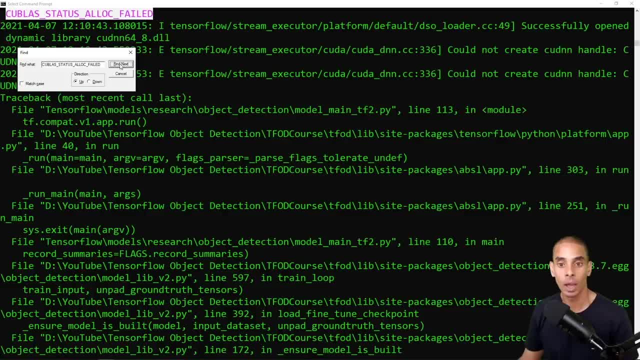 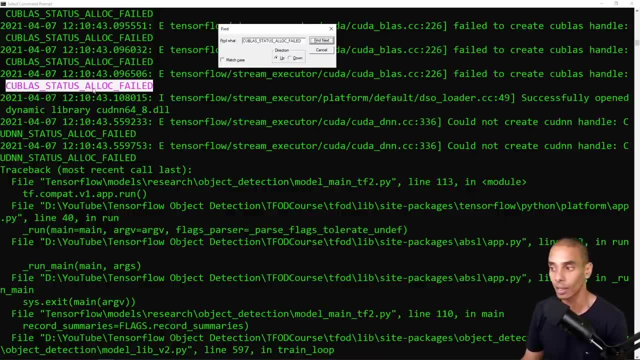 you this error, because it is pretty common, particularly if you're working on a GPU machine. If you see this error anywhere, so kubelast, underscore status, underscore alloc, underscore failed or anything along those lines. that normally means or you can see there's a similar one down. 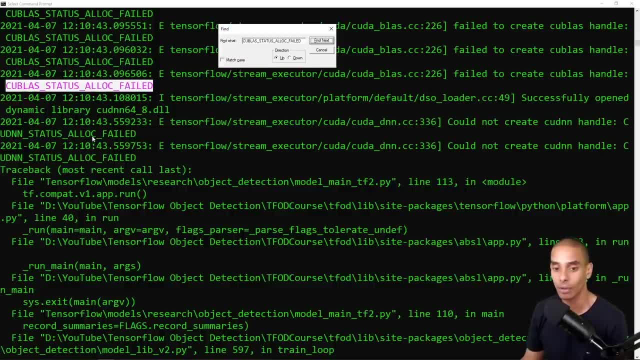 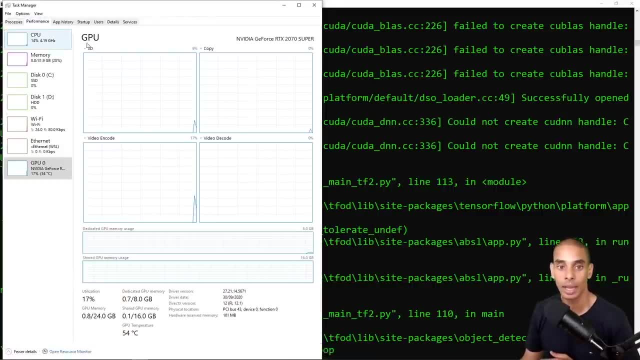 the bottom. so cudnn, underscore status, underscore alloc failed. So again, that normally means that your GPU is completely consumed. So if you go and take a look inside of your task manager and your GPU memory is completely consumed and you try to run the training run you're going to. 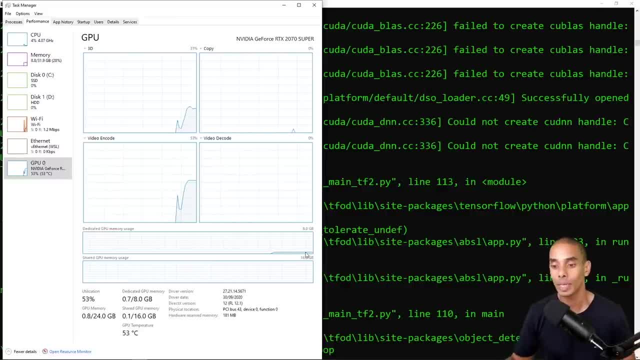 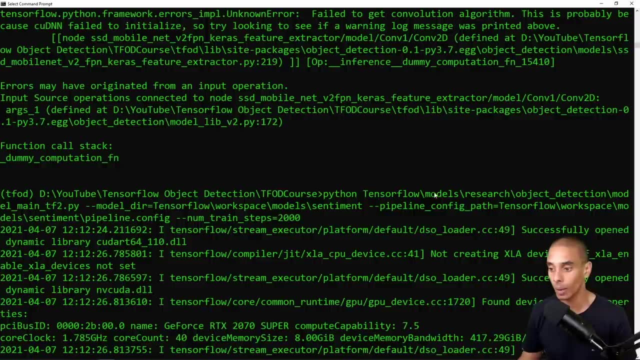 have a bad time. So, ideally, what you want to do is stop anything which might be using the GPU at any point in time and then kick off your training again Now. in this case, once I did that, so I went and ran the training command again, so 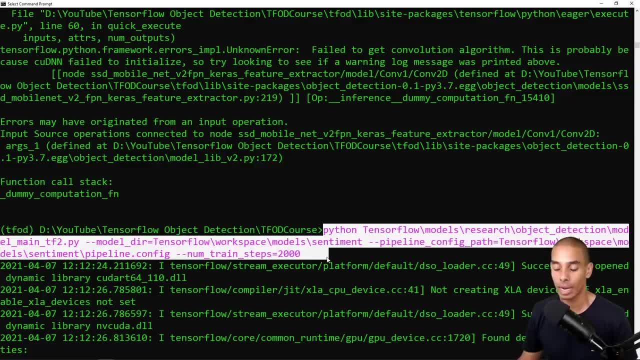 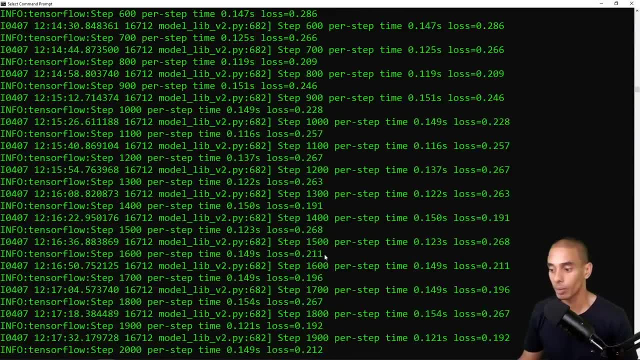 you can see it sort of errored out and it stopped there, Went and ran the training run again and it ran successfully. So right down the bottom again there's lots of lines. So right down the bottom you can see that we've got our loss metrics appearing. So step 2000 and our final loss was: 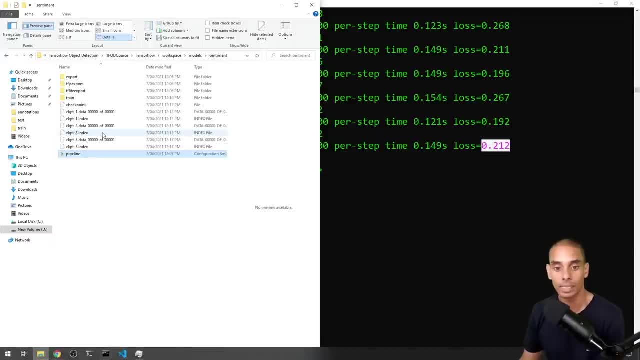 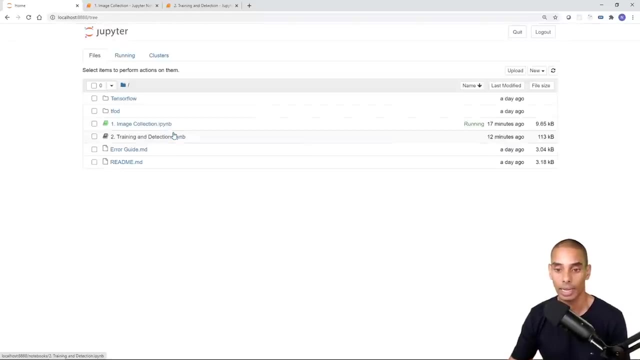 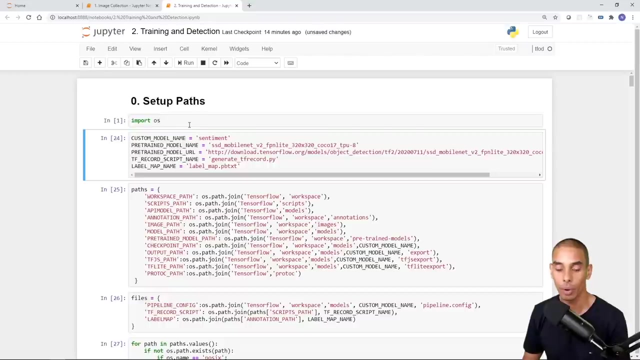 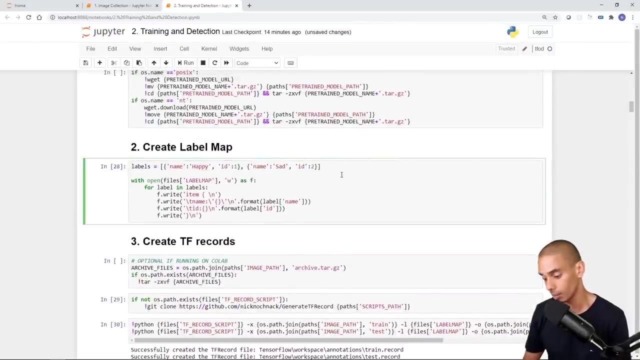 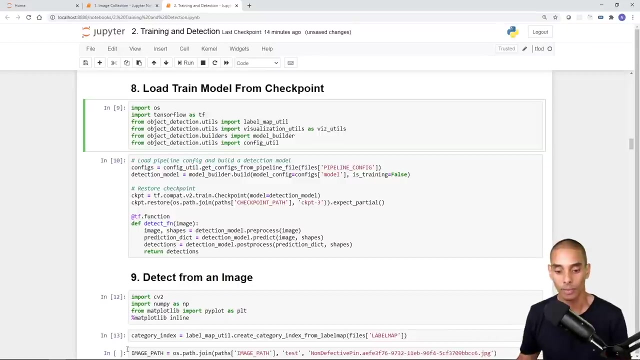 0.212.. And again, if we take a look inside of our training command, we can see that we've got, we've got our final losss of And then, if we go all the way down to step eight, you should be able to reload all of. 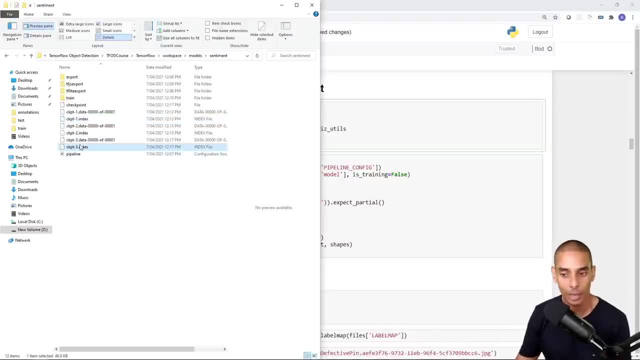 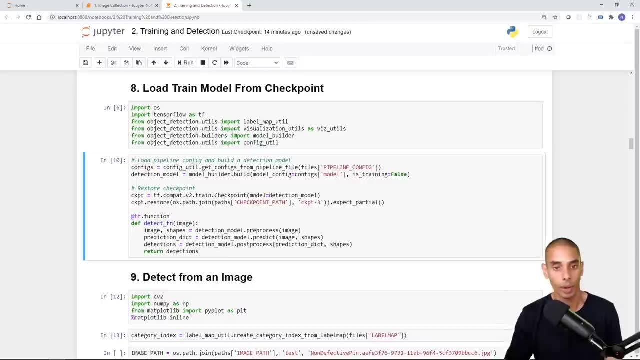 your stuff. Now again, double check what your latest checkpoint is. In this case it's checkpoint three. So we're fine with checkpoint three there. So under step eight we can import our model. So we're going to test it out before we go and push it out to our Raspberry Pi. 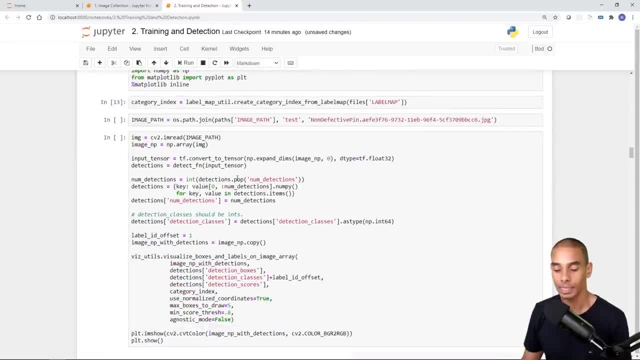 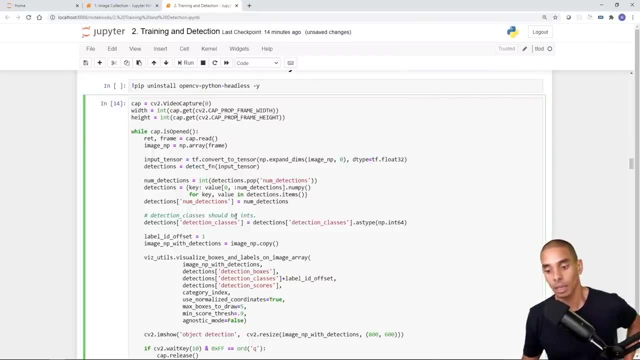 So let's import that model And again, I'm going to skip doing the image, but we could if you wanted to. We're going to jump straight through to real time to see what our sentiment looks like. So let's run this. and CV2 is not defined. 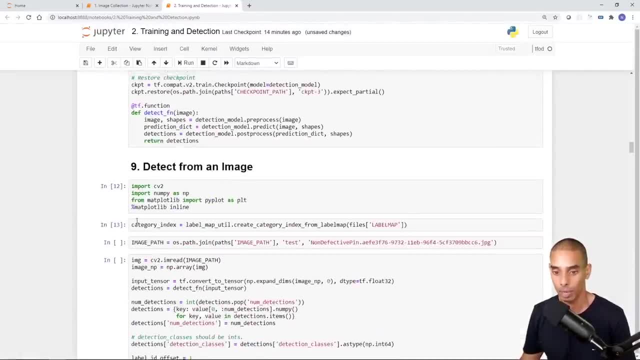 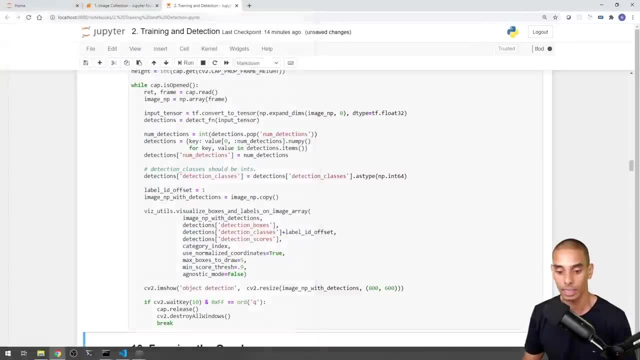 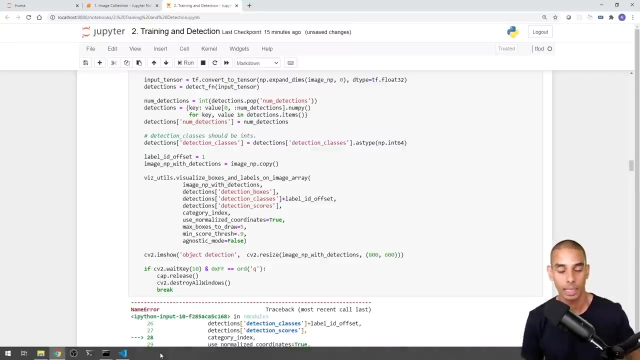 So that's our error there And that's just because we skipped importing CV2 up here. So if we rerun this, ideally, we should get some detection So we can close. our task manager Don't need that. So I've just seen my webcam start up so I can see the little light on it. 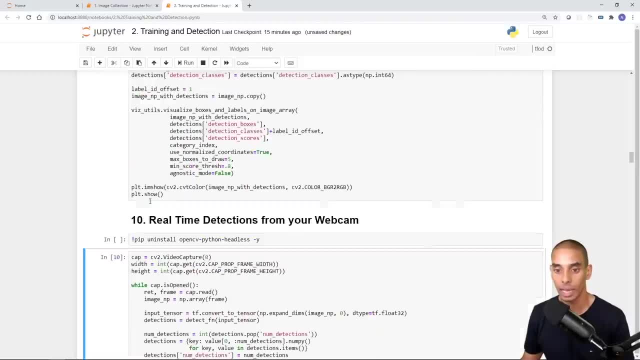 It's like we've got an error here, So category index is not defined. So that's an easy fix. We just need to re-import this. So whenever you restart your notebook, there's going to be a few things that you've obviously got to import. 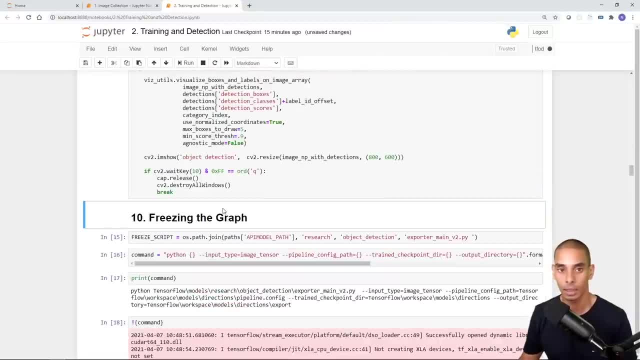 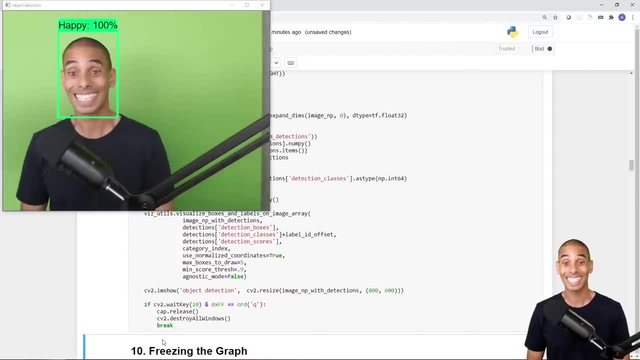 So if we import our category index, try this again, And this might actually error now because I didn't release my capture. but we'll wait and see. Oh nope, we're good, All right. So it's saying happy, sad. 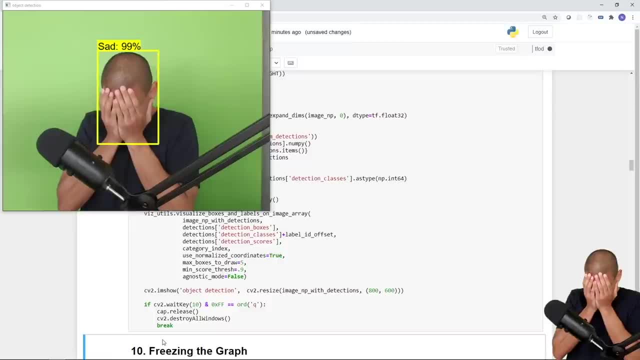 How's it looking? Sad, happy, Pretty, cool, right? So like that's a lightweight sentiment model. So it's chasing my head around. I put my head down, So what's it actually take for it to go to sad? So if I bring my hands up, so it's starting to get closer to sad. 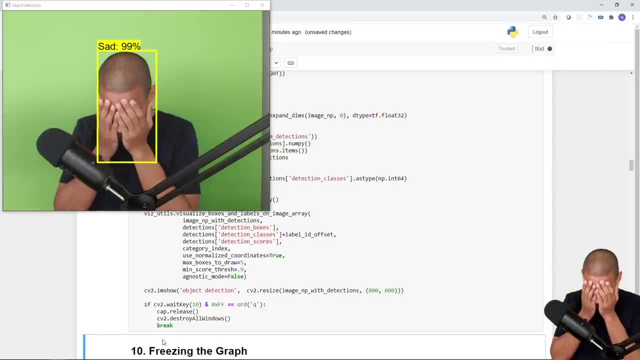 If I go all the way. so if I cover my face, it's sad. If I unhide my face, it's happy. So again, you can sort of see that it's. with these models you can pretty much build whatever you'd like. 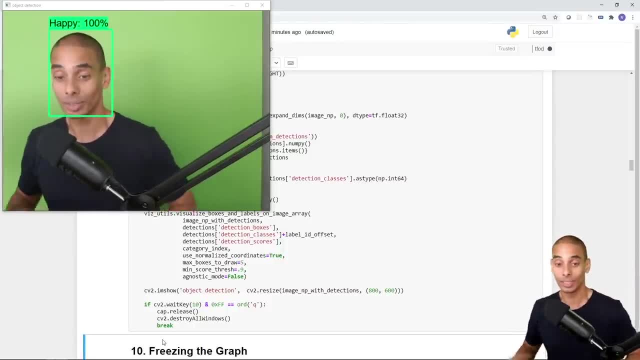 This is why I kind of love TensorFlow Object Detection, or love the TensorFlow Object Detection API. It's really reasonably quick to do once you've got it set up. You don't need to go and set up all the stuff all the time. What's it looking like? 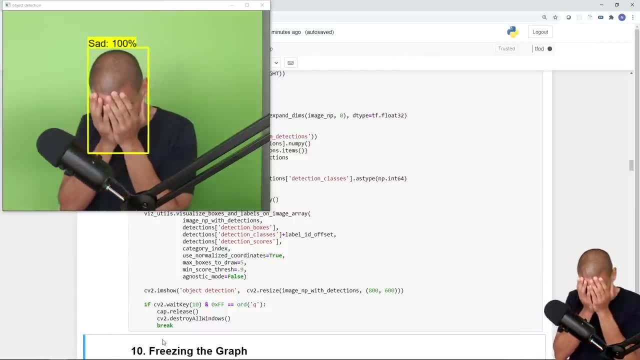 So it's still there. It's still saying that's happy We get in position. So that's saying sad. So again, you can play around with this, but I love that it's chasing my head around So cool, All right. 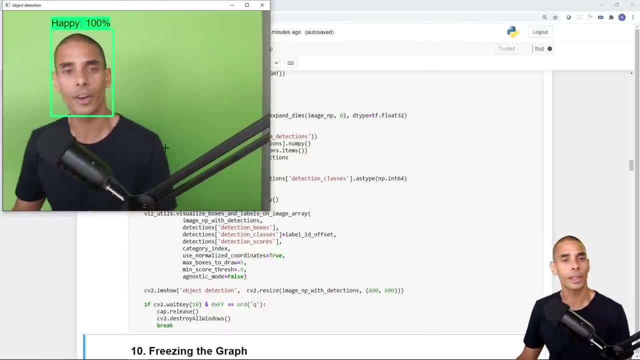 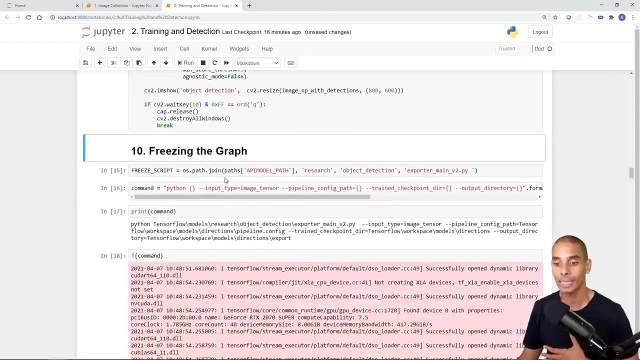 So in this case, so we're happy now, but we want to take it a little bit further and actually push this out to our Raspberry Pi. So we're going to quit out of this by hitting Q on our keyboard. We're then going to freeze our graph. 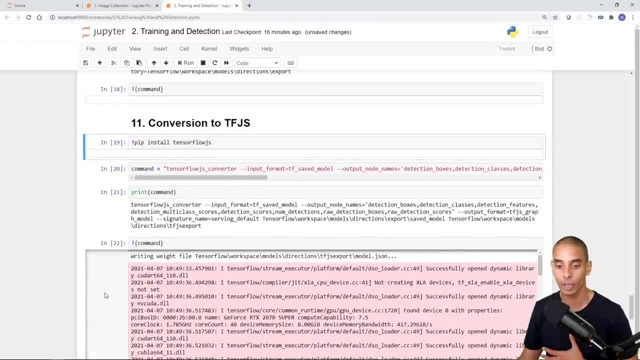 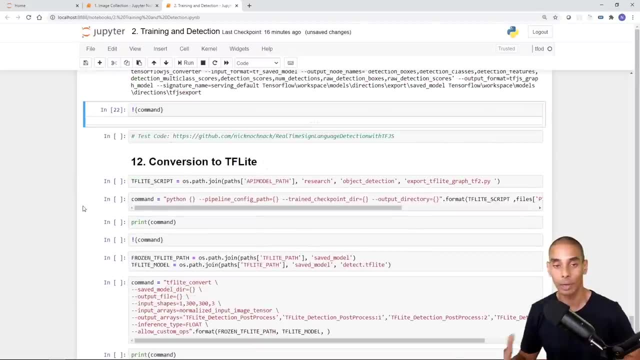 So we're going to go through step 10.. We don't need to go through the conversion to TFJS because we're not doing that this time. So we need to do everything under step 10.. And everything under step 12, in order to get this to work. 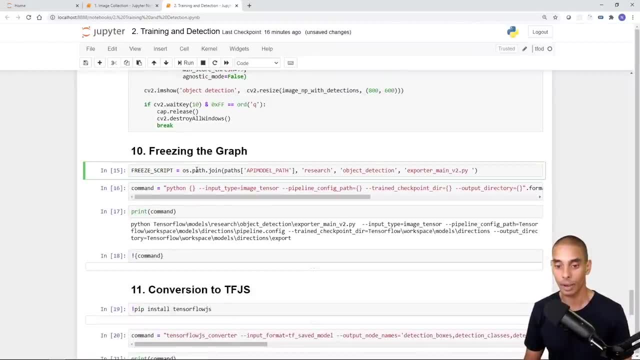 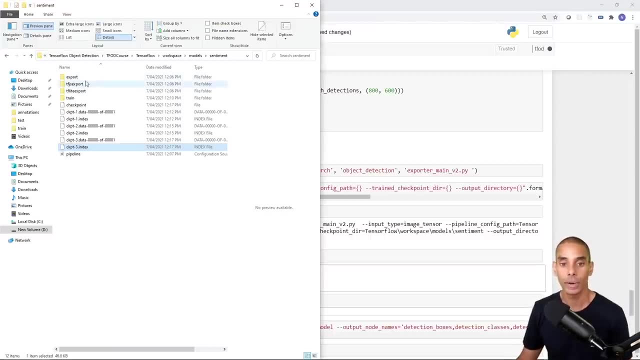 So what we're going to do is we're going to run through step 10 and freeze our graph. So if I run all of those steps, including the command, we'll run this one from the command or from our notebook. This should generate our export file, which is over here. which is over here. 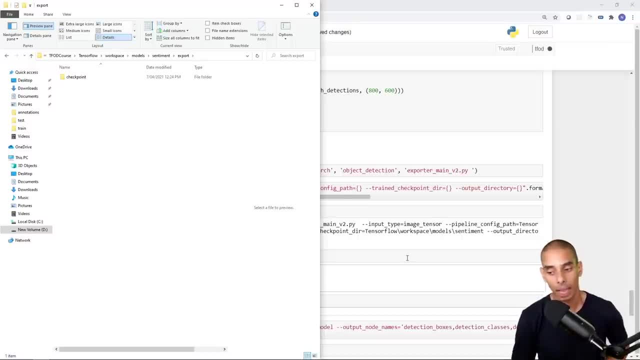 And then, once that's generated, we'll be able to run the TF Lite conversion. So again, a lot of these scripts are sort of Pre-configured. you can sort of pick them up and leverage them. Let's give that a sec. 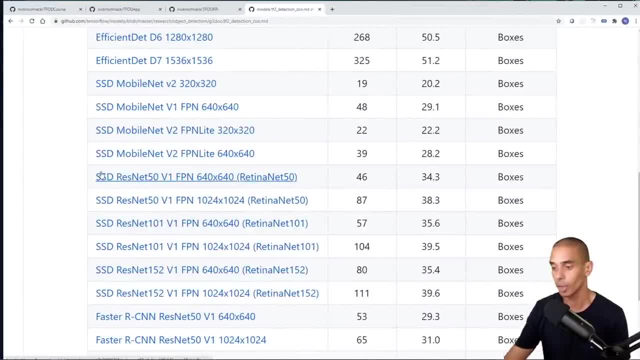 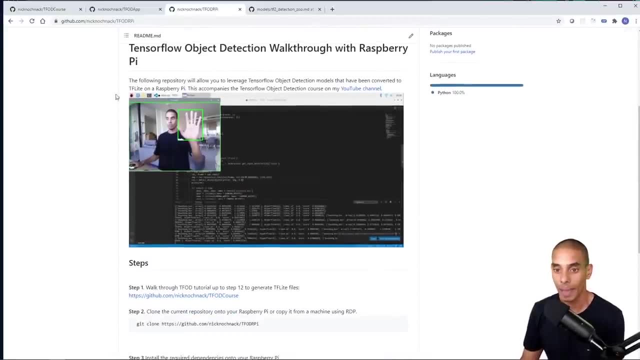 Now, while that's happening, let's take a look at the steps that we need to go through in order to build our Raspberry Pi detection. So again, the third and final GitHub repository that I've sort of made available and written up is the TensorFlow Object Detection Walkthrough with Raspberry Pi. 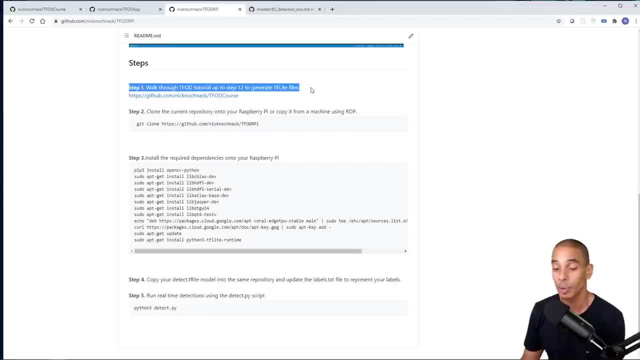 So, again, all of the steps that you need to go through to get this up and running are in here. So, first up, we're going to Start by going through our TensorFlow Object Detection course to create our TF Lite files. then we'll clone this to our Raspberry Pi, so we can either clone it from our Raspberry Pi or download it to our PC and then copy it over from our remote desktop connection. 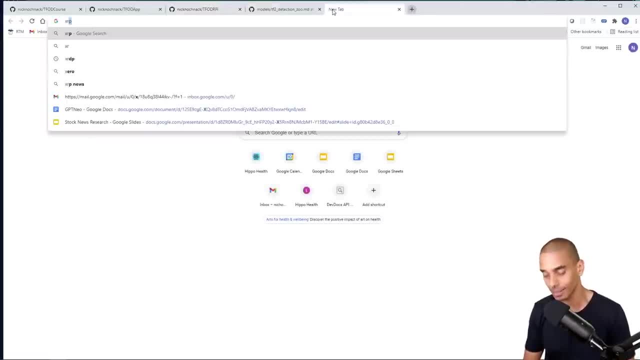 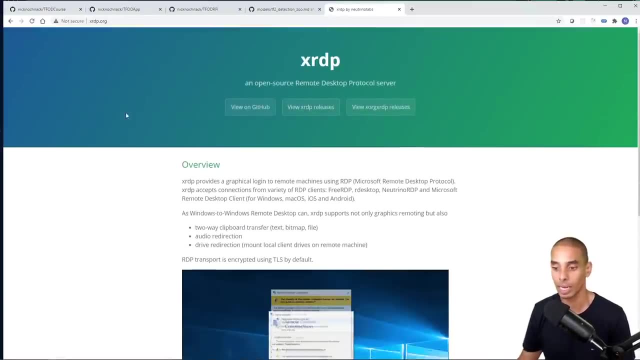 So, in terms of this remote desktop connection, I'm actually using something called XRDP, which allows you to remote desktop or remote into your Raspberry Pi, So it's actually pretty cool. So it makes life a whole lot easier. I can code. 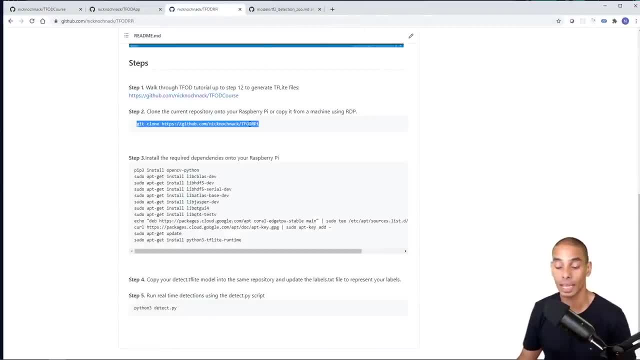 On my Raspberry Pi from my local PC without having to actually go into the Raspberry Pi, But all the code is actually still executing from the Raspberry Pi. So once we've done that, we've just got to install a bunch of dependencies, copy our converted model over and then run it. 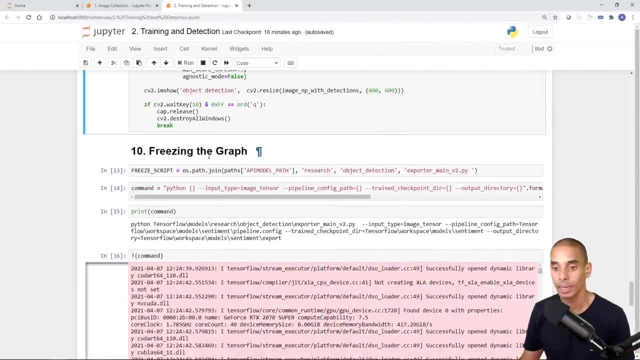 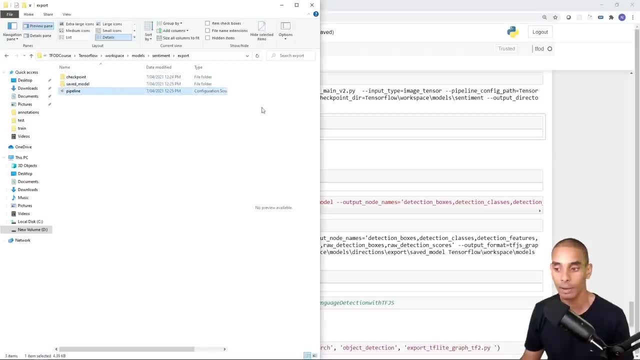 So let's go on ahead and do this. Okay, so we've now gone through and frozen our graph so we can see that in here. So we've got our checkpoint, our saved model and our pipeline file. Good to go there. Now what we need to do is convert it to TF Lite. 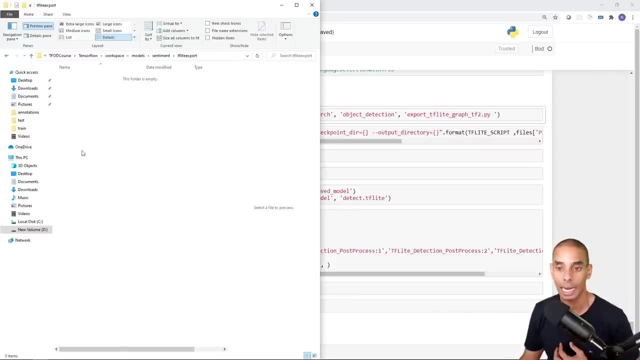 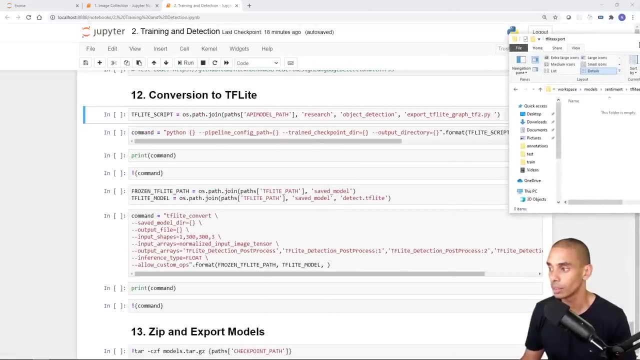 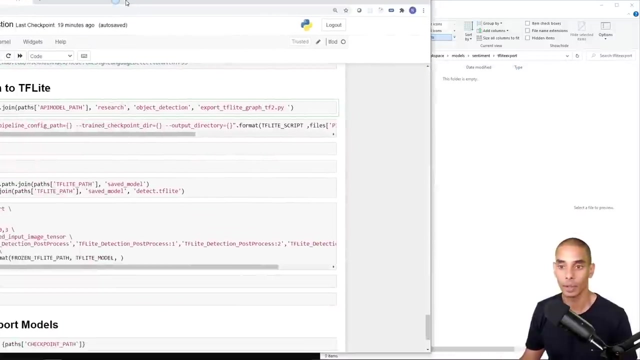 So this is all going to happen inside of the TF Lite export folder. So let's go on ahead and run this and we should see all of our results pop up. Let's just bring this over to the side here. So if we run everything under step 12, I don't know why I've focused on putting that to the side- 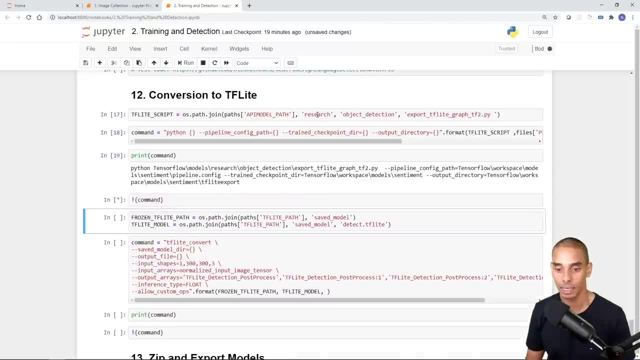 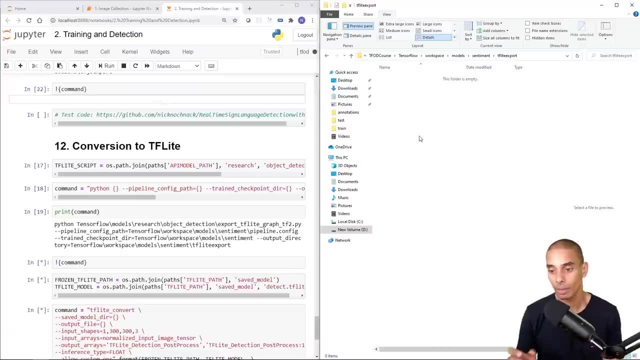 All right, so we're going to run everything under step 12.. So, TF Lite script: this, this, this, this, this, this and this, And ideally this should generate our TF Lite export. So what you're looking for is a file called detecttflite. 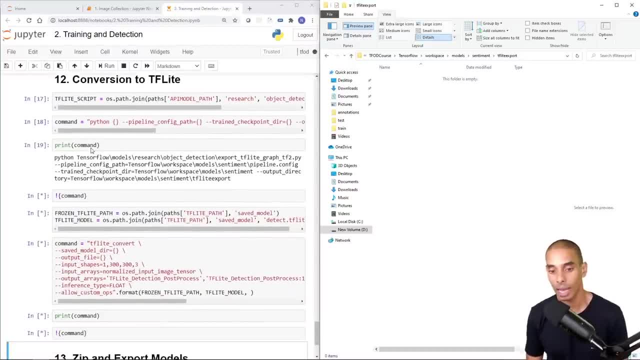 That's the core file that you're going to be able to leverage inside of our Raspberry Pi. Now I've already got our Raspberry Pi remote desktop into, so I'm already remoted into it, or hooked into it, if you want to say that. 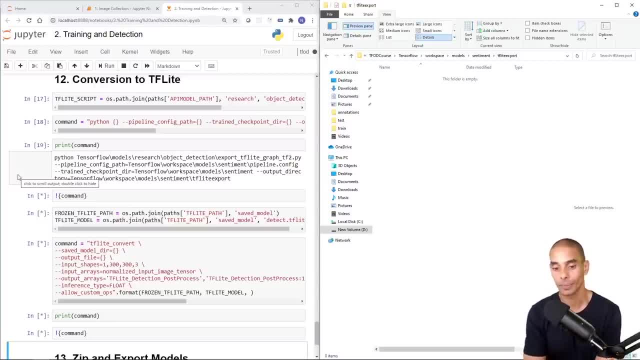 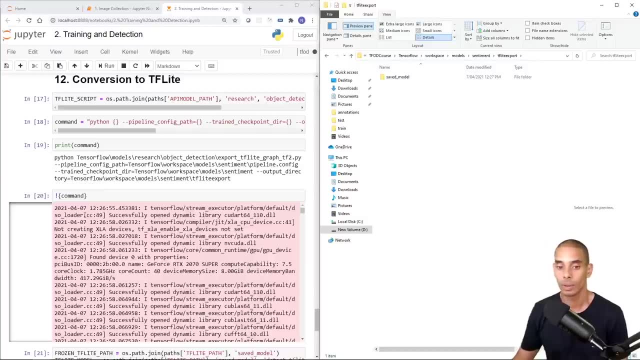 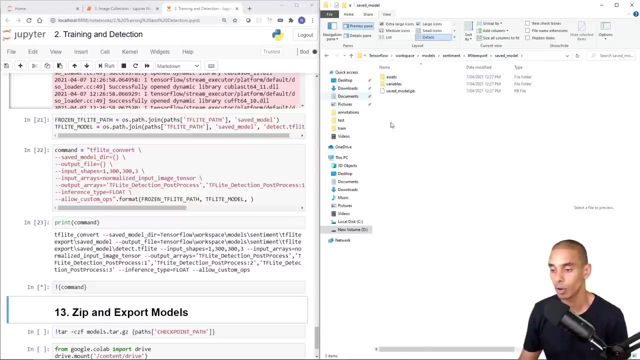 And so we'll be able to jump into that and take a look at that as well. So let's give that a sec and then we should be able to kick things off. Okay, so that's it. That's the first part of it done. in a second you'll see. so you can see inside a TF Lite export. we've got this saved. model folder. 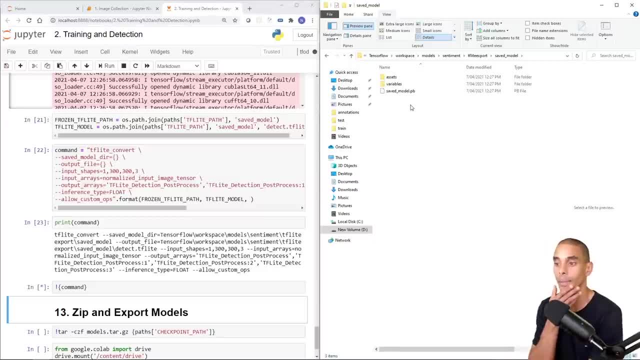 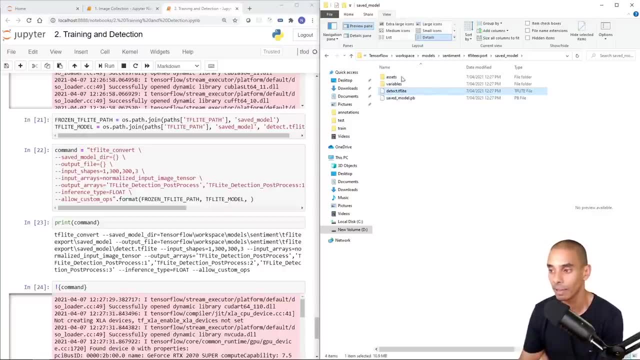 And once the second command runs, you'll have detecttflite made available So you'll be able to pick that up and leverage it. Cool, So you can see we've now got detecttflite. it's a little bit smaller. you can make it a bit bigger. it's that file over there. 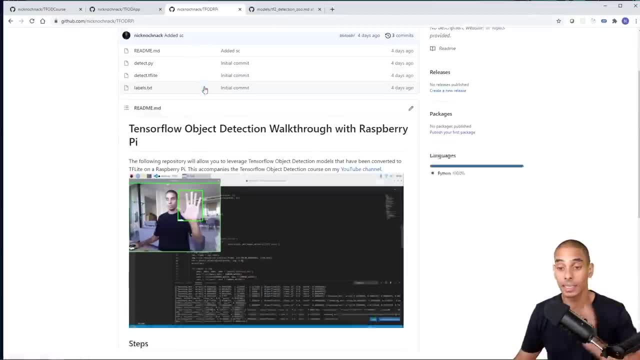 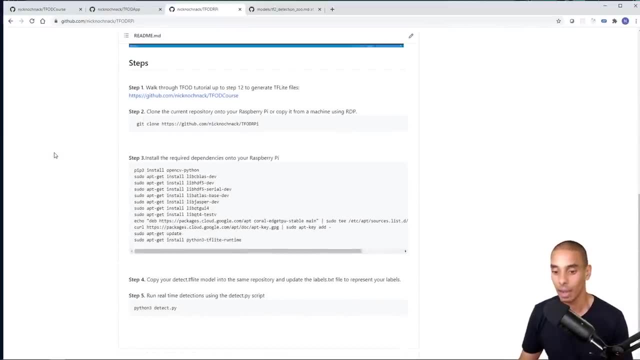 So, if we take a look at our steps, what we've now done- and this is this: these are the steps for the TFOD RPi repository, So the Raspberry Pi code in this particular case. now, what we're going to do is clone this repository. 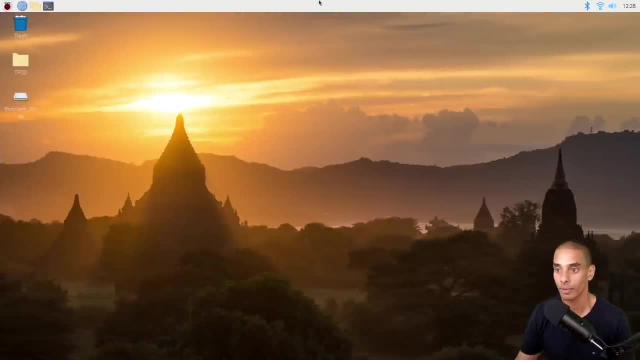 So I'm going to jump into my Raspberry Pi now And right up here you can see that I'm just remote desktop into it And I'm going to create a new file, or new folder actually, and we're going to call this sentiment. 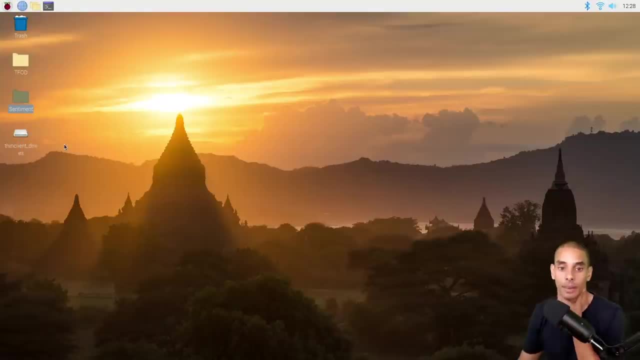 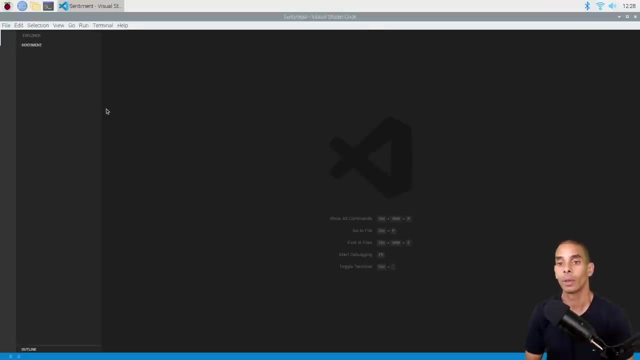 And we're going to jump into that. So we're actually going to open this up inside of VS code. So I've got VS code installed on this Raspberry Pi- Cool- nothing in there yet. So we're going to open up a terminal- and this is a bash terminal- and we're going to type in git clone and then paste that link. 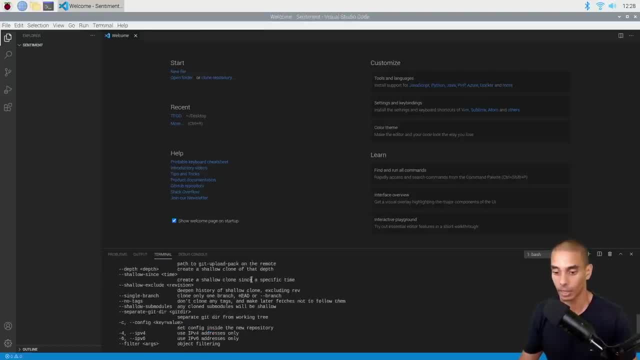 Did we have? what link do we have there? Oh, we already had a git clone, so we don't need to type in git clone. let's clear this. Let's make this a bit bigger as well, so we can see what we're doing. 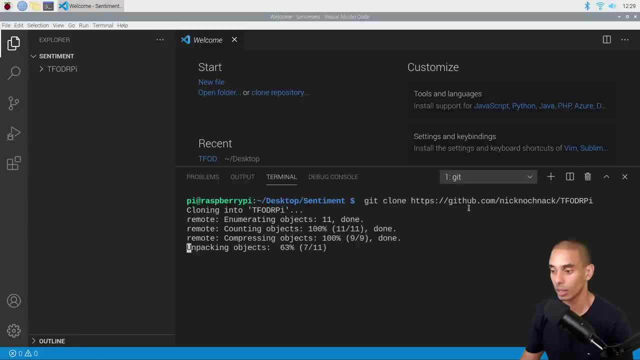 Right, so we're going to paste that command into here. So git clone, and then the TensorFlow object in here, Cool, And then we're going to run our detection repository. So you can see that we've now got that, or it's starting to come through. 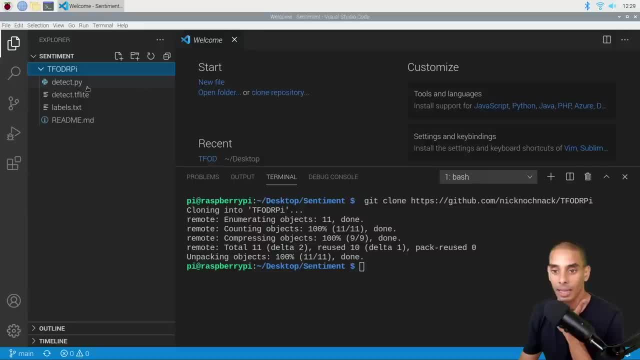 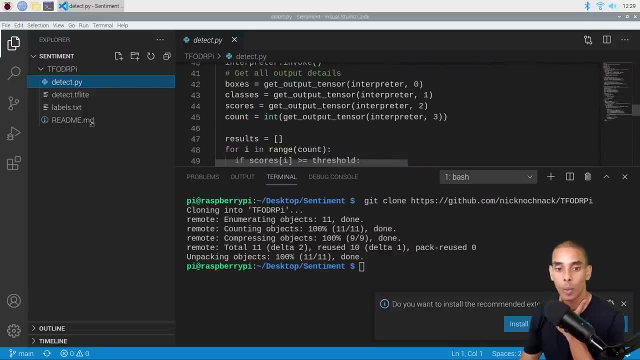 So in there we've got a couple of things. So we've got the detectpy file, And this is the main file that we're actually going to use to run our detection. So all of our good stuff is actually in here. Then we've got an existing detecttflite model. 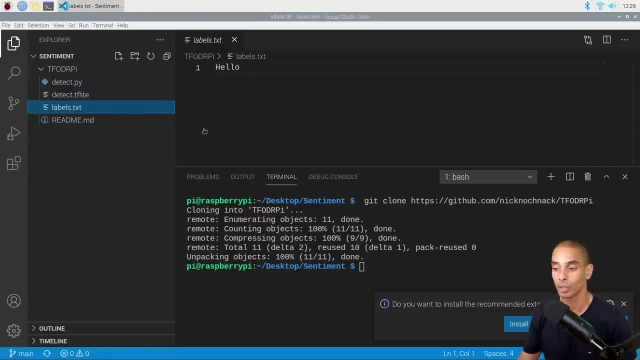 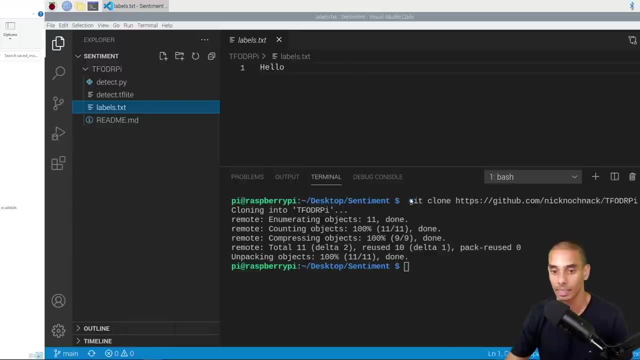 So we can actually run this off the bat without actually having to do anything else. So, in this case, it's just a simple basic hello model. Now, before we actually do that, though, there's a couple of key dependencies that we need to install. 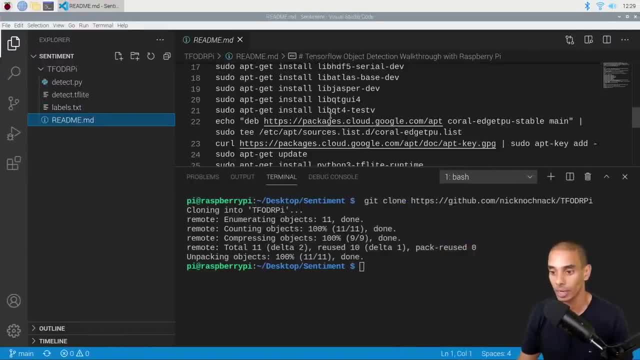 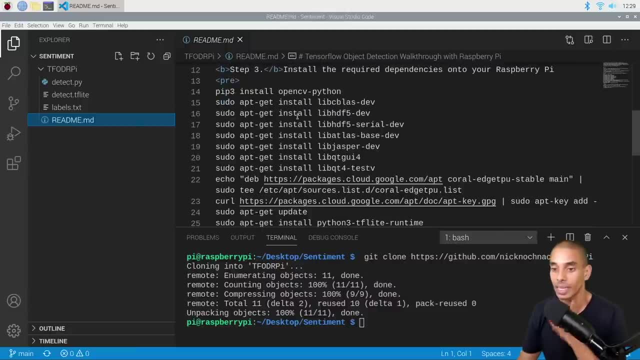 Now they're all listed in this readme here. So if we actually bring these up, you can see that we've got a bunch of files that we actually need to install. So, specifically, these are all required to be able to work with OpenCV. 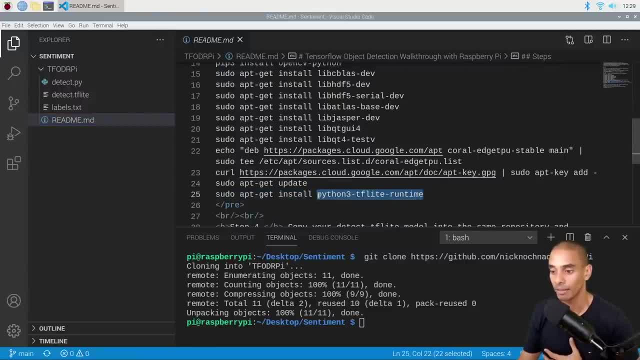 So, and then the last one is actually installing this Python tflite runtime. So this is really, really important to have these dependencies available, because it's going to mean the difference between your model running and not running. So what we'll do is we'll go through each one of these. 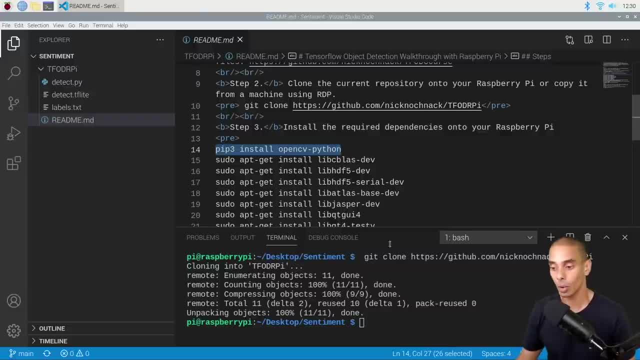 And we'll install them. So I've already got this configured. but it's all good, Let's go on ahead and do it. So we're just going to paste the first command. So let's copy this. So that's going to install OpenCV Python. 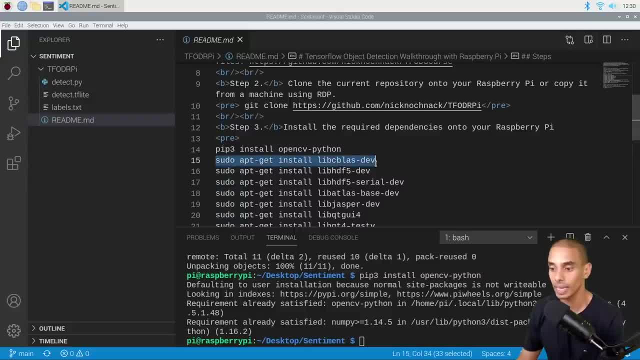 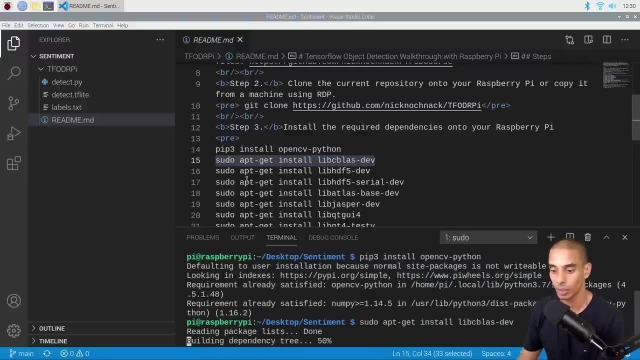 Looks like it's already installed, then we'll install this. So all of these are dependencies for OpenCV. So, specifically, we need to install OpenCV, So we need to install these as well in order for this to work. So I'm just going to copy these and install them. 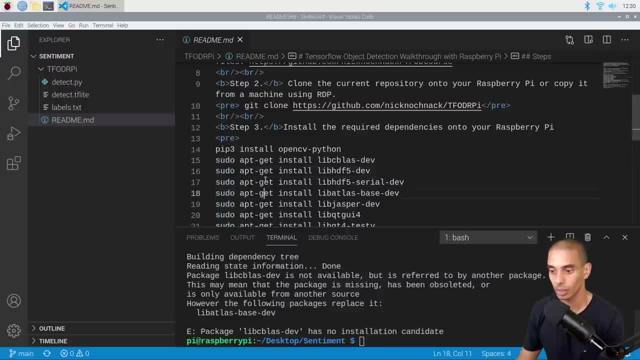 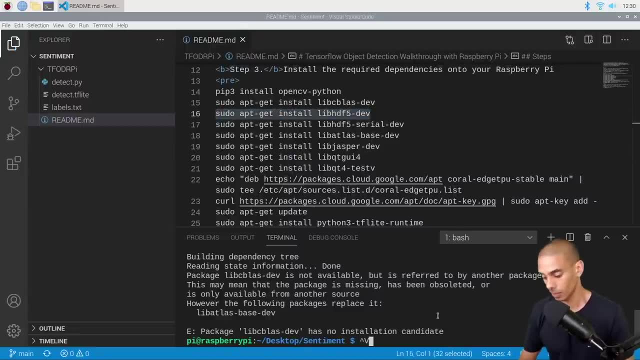 So it looks like package to do all right. so we've got to go through all of the rest of these as well, So let's go on ahead and install these Like copy and paste doesn't seem to want to work, So we're gonna have to do this manually. 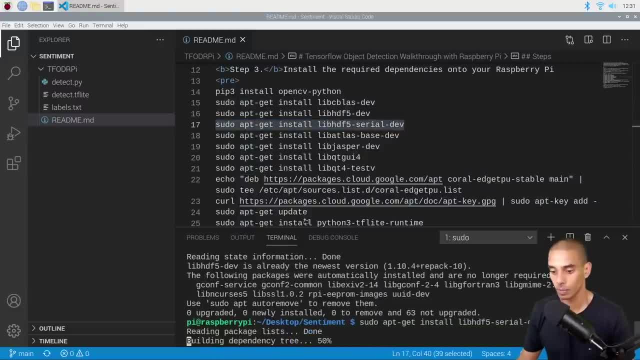 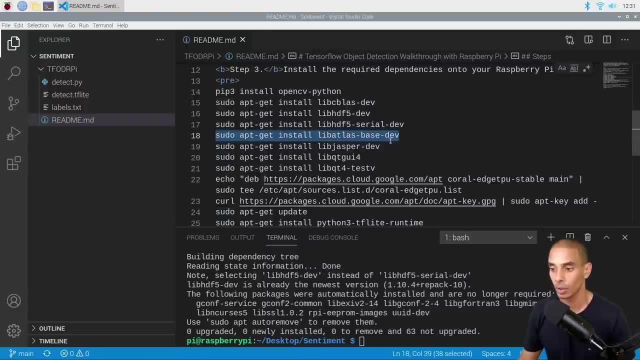 Cool. So that's the next one done. And again, I'm just going through it, Each one of these packages that we need to install, and I'm going through and installing them. So we'll just copy and paste, And I sort of wanted to show it to you from scratch because that at least you can sort of see how to actually get this up and running. 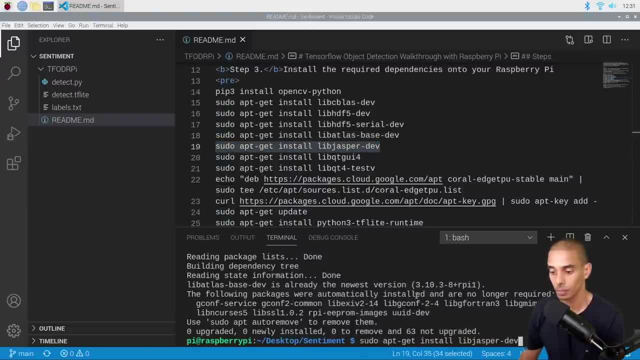 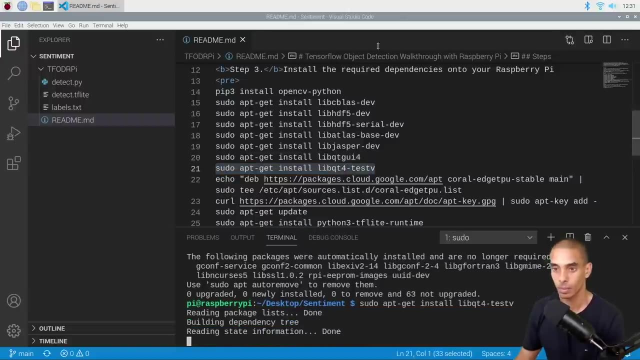 It's next one done, And it looks like a lot of these are already installed, So it's going through them reasonably quickly. It's not actually installing it. Cool, That's that Okay. so those are all of these packages installed. 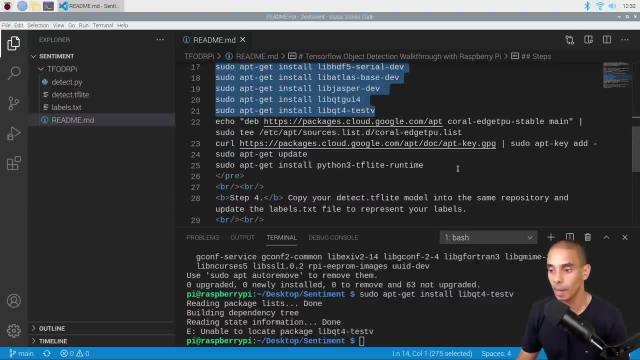 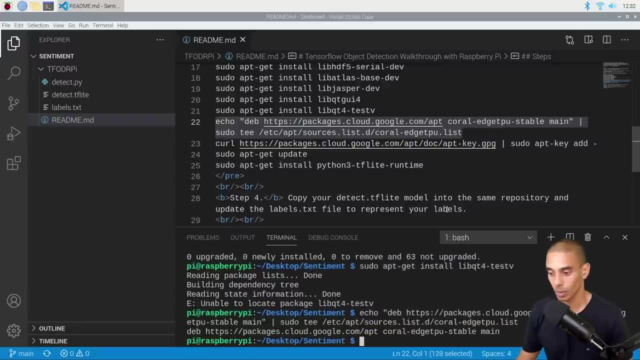 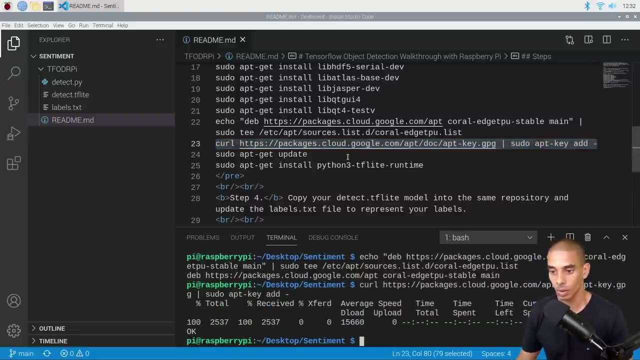 So we've now done all of these right, but we've got these couple of packages left to do, So let's go on ahead and do this one Cool, And then this one Awesome. then you should normally do a generic update. 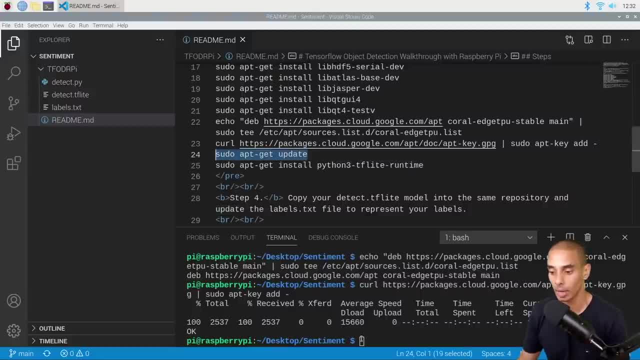 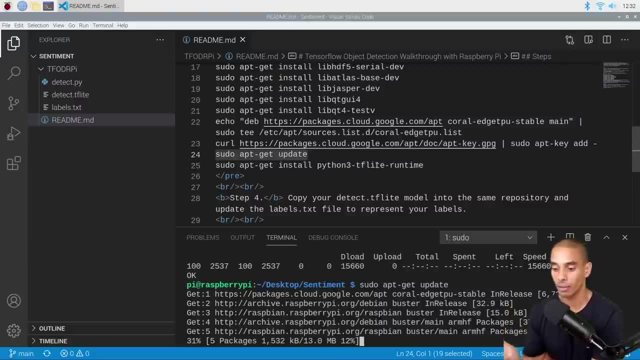 So we'll do the update and we'll install our TF Lite runtime. So this Last one is the most important one, this one over here. So this is actually what's going to allow you to leverage the TF Lite runtime without explicitly having to go and install the full tense flow object detection API. 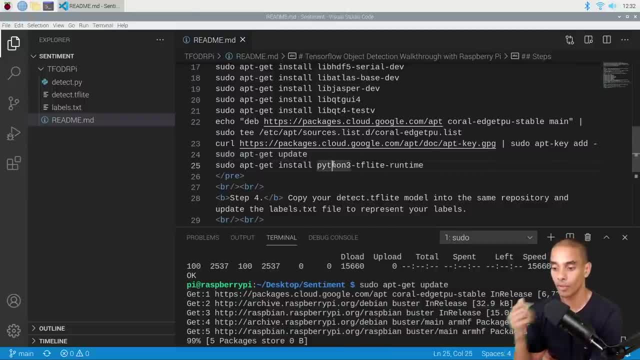 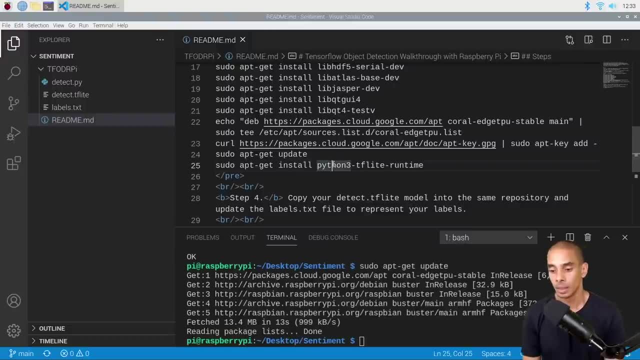 So once we've got this line done, we're pretty much home free. So let's let this run for a sec, And then we should be good to go once our update is done. Cool, that's done. Now we'll do the last one. 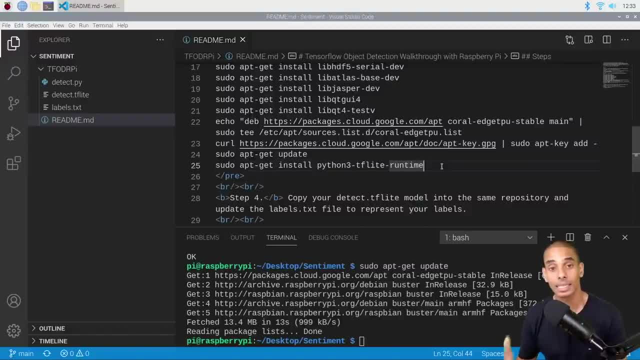 So this is going to install our TF Lite runtime. So, as I was saying, this is the main package Which allows you to leverage a TF Lite model and, specifically, our object detection model, within our Raspberry Pi. So we're going to copy this. 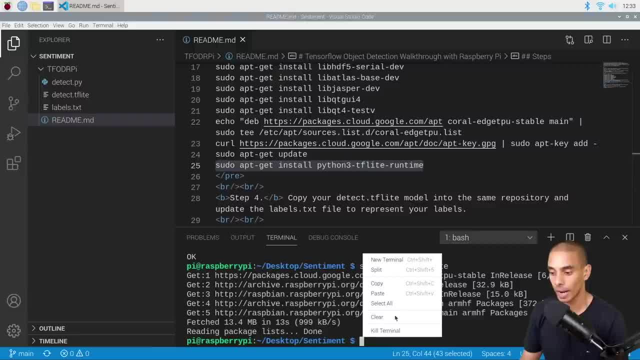 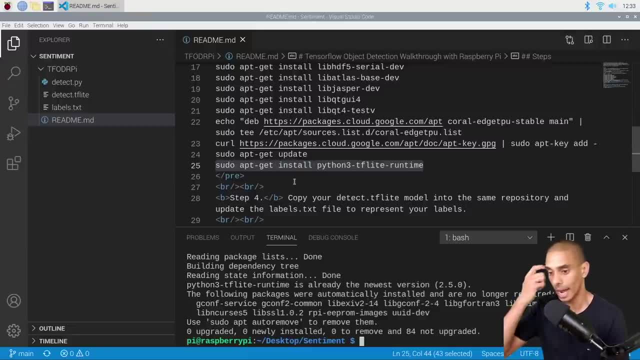 And again, these are all available through the readme, So don't fret. if you haven't picked up exactly what the command is, That's fine, All going to be available through there, Cool, So that's already installed now. Now, rather than running our custom model first up, I want to show you how to leverage the model that's already in there. 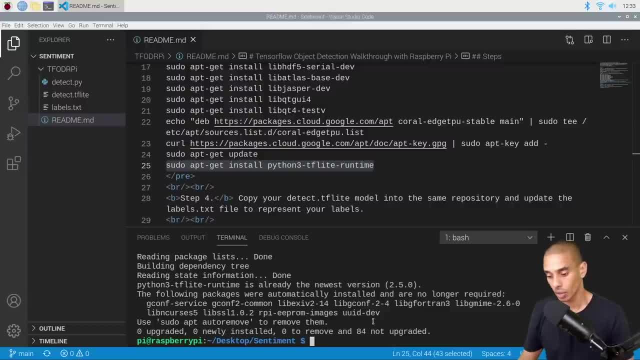 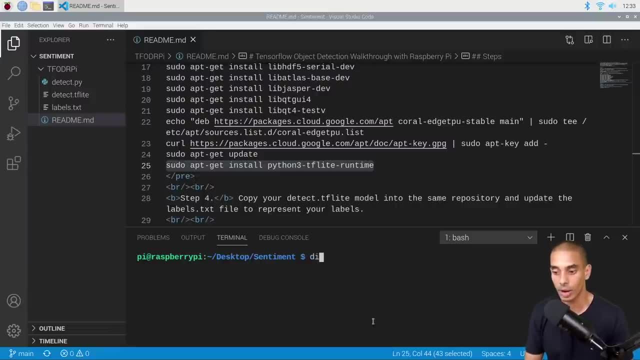 So you can sort of get a feel for what this is going to look like. So To run this, let's just clear these commands. We just need to cd into that particular directory, Because right now let's just type in ls. 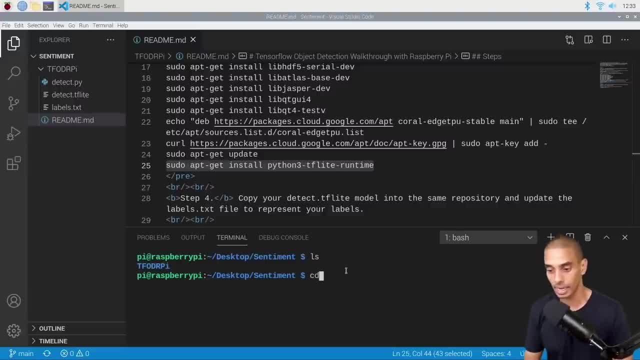 Right now we've got this sub folder right, So tfod, rpi. So we're going to cd into that And then if we type in ls now, so we've got our main folder. So to run this, all we need to do is run python3 detectpy. 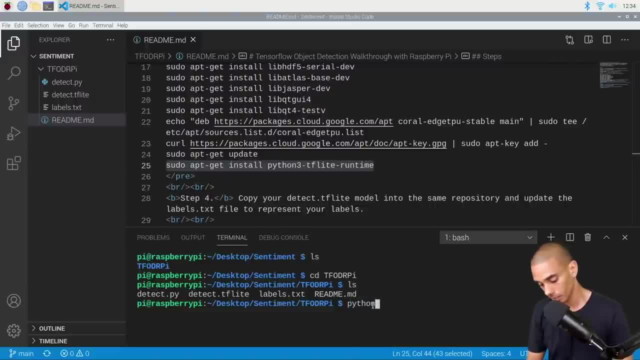 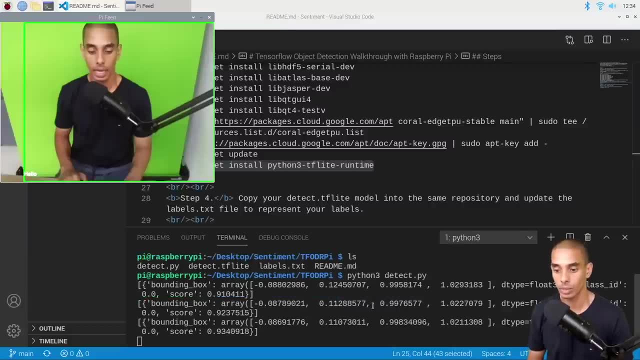 So let's go on ahead and run that. So python3, detectpy And all things holding equal, we should, okay. so we've got our object, our detection box, opening up and this is just a straight up hello model. So you can see it's a little bit slow. 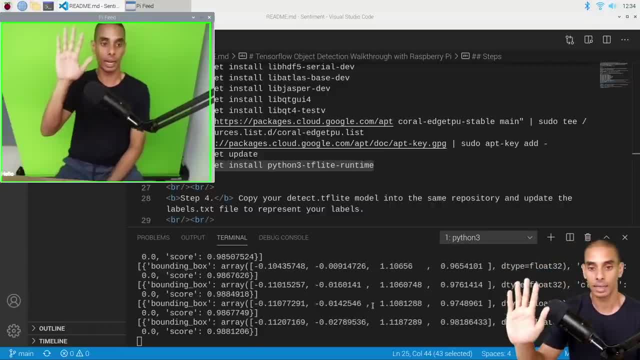 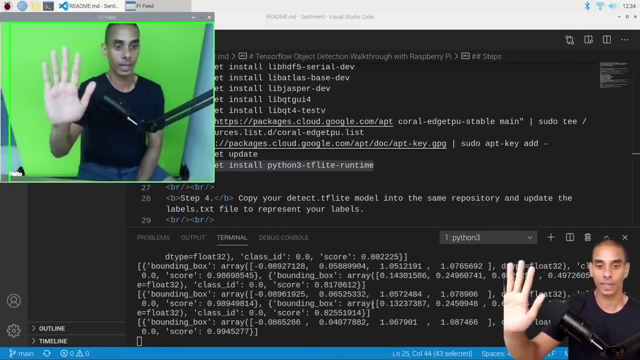 And again, it's running on a Raspberry Pi, so it's not crazy fast, But you can sort of see that it's detecting hello, it's detecting my face And again it's not the most accurate model, but you sort of get a feel for what's possible here. 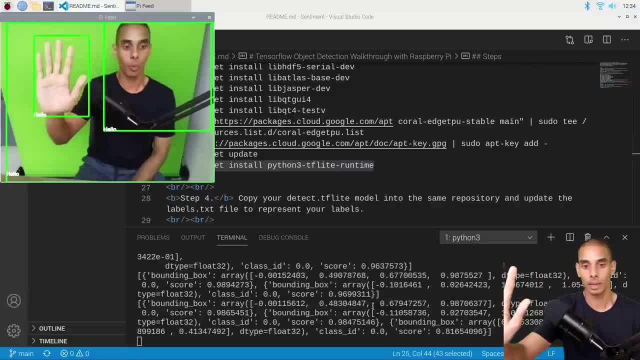 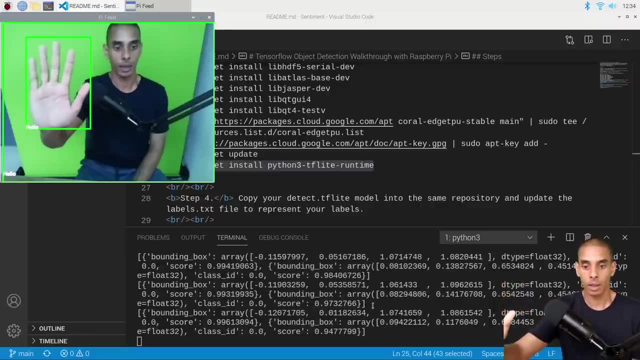 Right If I bring my hand a little bit closer And start to see that's making detection. So I'm going to go ahead and do that. We need to make a couple of additions on our Raspberry Pi, Alright, Okay, so if we hit Q, we can close that as per usual. 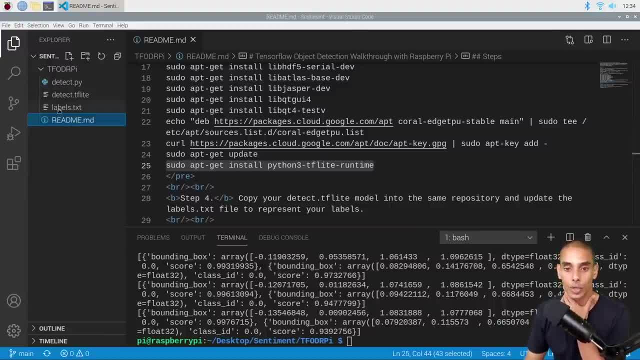 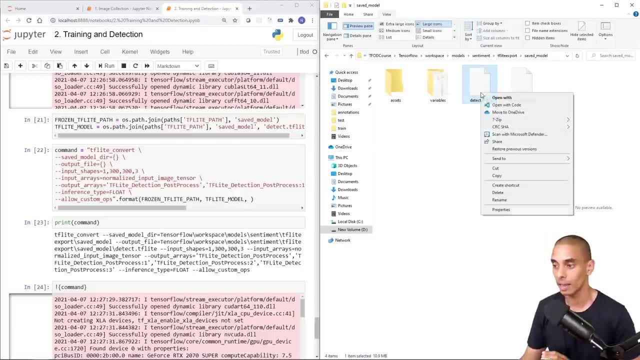 Now what we want to do is we actually want to do this without custom model. So in order to do that, we just need to go back into our, where we actually saved our detecttf lite file, copy this and paste it into this repository. 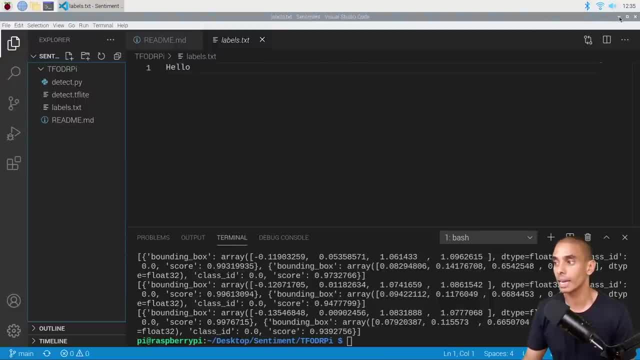 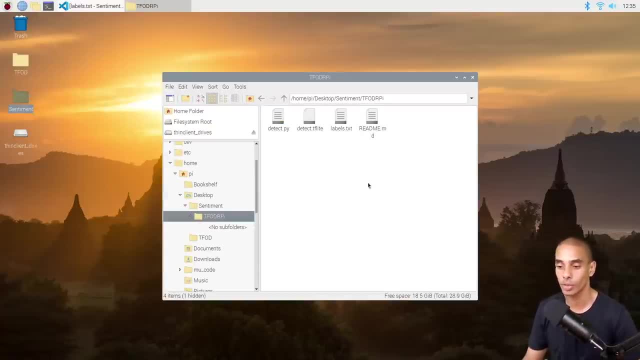 So what I'm going to do is I'm just going to paste it down And again, if you're doing this without IDPing into it, you could do that at any time. So let's do that. definitely transfer it like, save it up into google drive or box folder and bring that over. 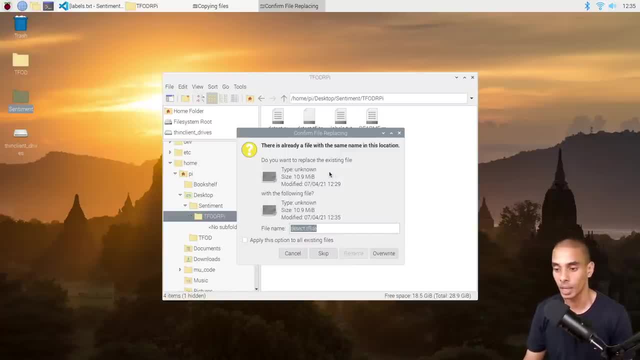 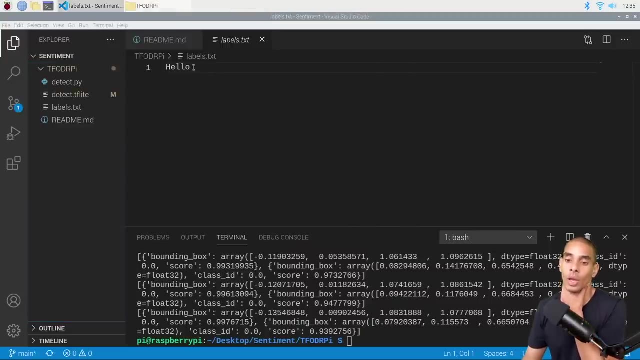 in this case, having idp available makes it a lot faster. so we're going to copy and then replace it, so we'll overwrite, cool. so that's good. and then what we need to do. the last thing that we need to do specifically is we need to update this labelstxt file. so really all we need to do here. 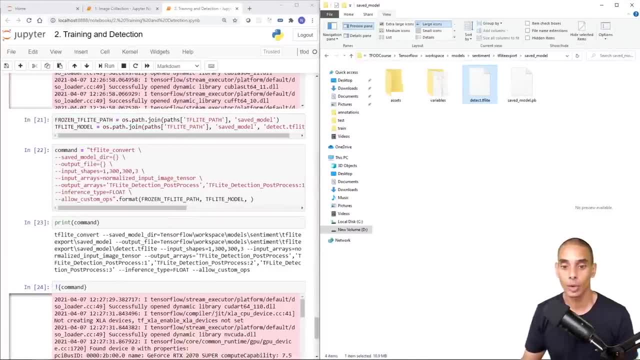 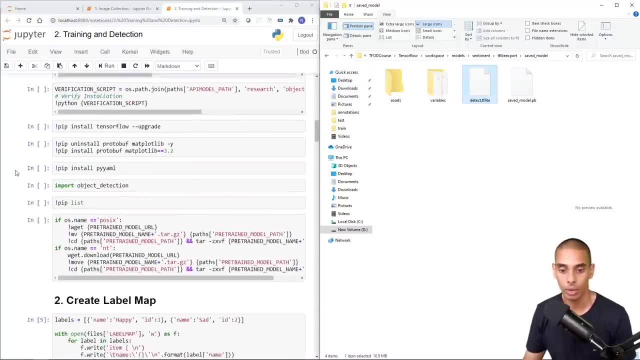 is update it for our custom labels. and remember, if you remember correctly, we had two custom labels that were just happy and sad. i'm just double checking the order that we had them in, so remember we had happy as id1 and sad as id2. so let's go on ahead and do that. so we're just going. 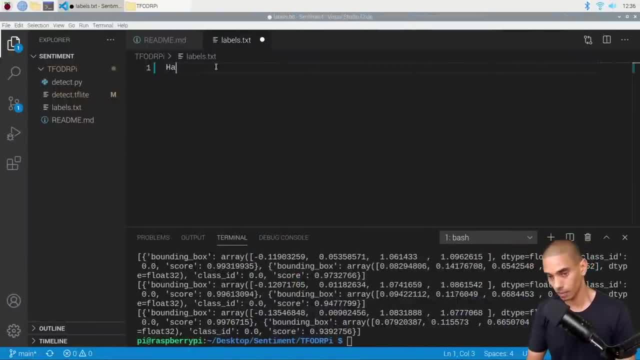 to make happy the first object and then sad the second object. so we'll hit save. now, all things holding equal. if we run detectpy again, you so python3 detectpy- we should effectively be running our custom model now. so let's clear this, let's try that. so, in order to run this, we're just going to run python3 detectpy. 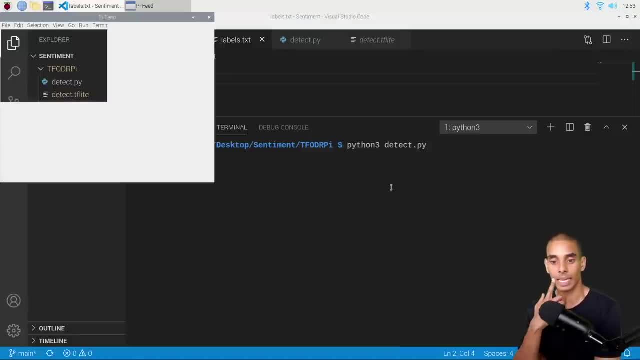 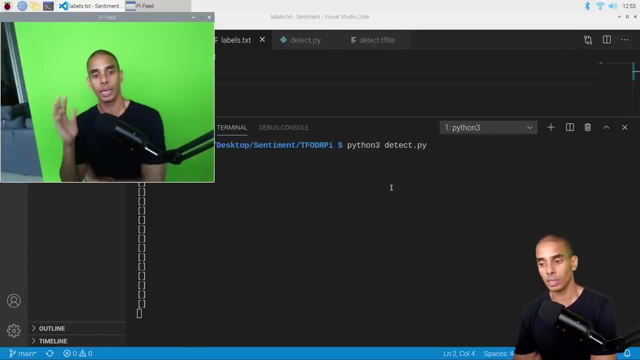 and again we'll see if we get any detection. so again, we haven't trained for that long, so at the moment it's a little bit slower. and again, we're going through idp, so doesn't look like we're getting any detections and that's indicated based on what you're seeing down here. so it looks like. 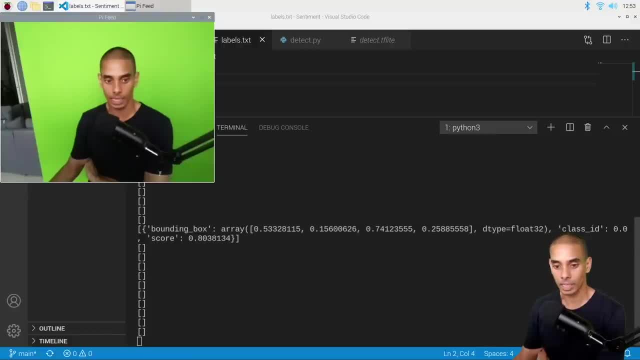 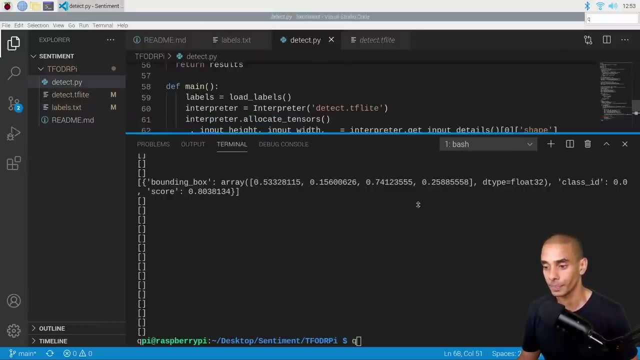 we've got a random one. looks like they're real reasonably low quality, so what we might want to do is drop our detection threshold. so if you're going to detectpy, you can actually change this up. so actually in this line here, so on line 68, if you. 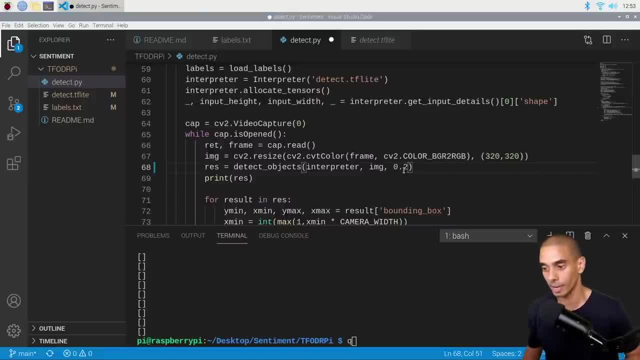 change this. so let's try dropping it to i don't know, 20 for now. so we're changing that, and then what we can do is rerun this. so rerun our command. so we're going to run python3 detectpy again. so let's see if we get some detections now. so let's try that again. so we're going to run python3 detectpy. 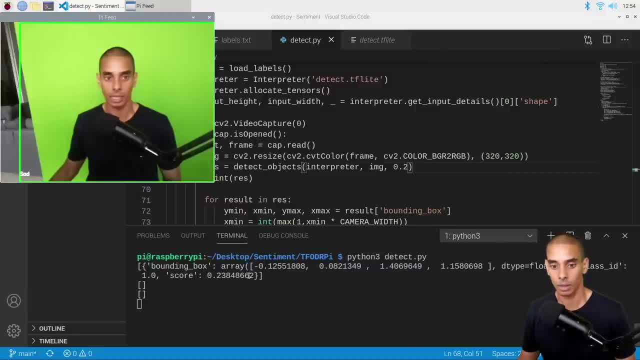 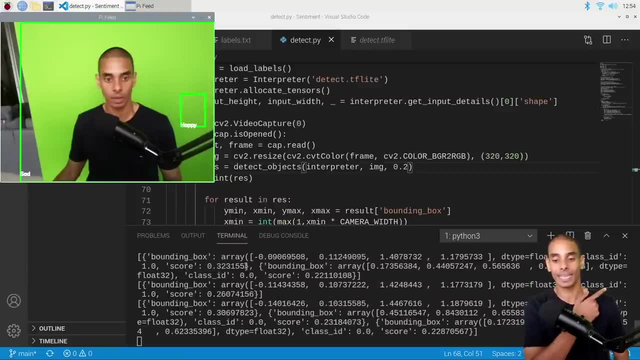 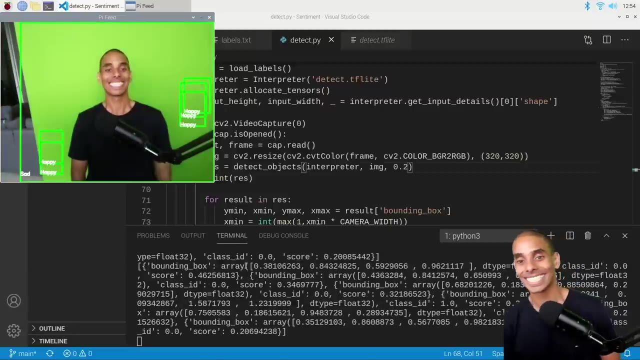 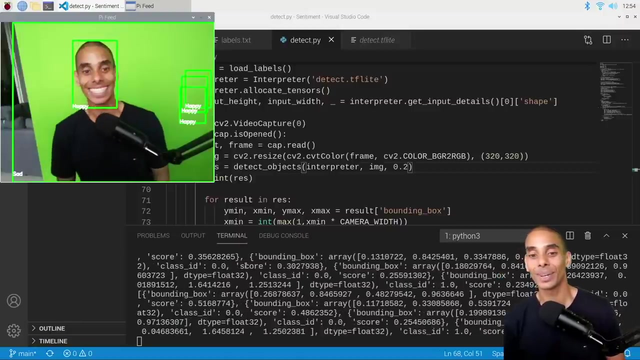 it's looking like we're getting detections already. okay, so we're getting one big sad, we're getting happy. it's looking like there's a fake detection over there. so there we go. it's detecting me- happy and sad at the same time, but you sort of get the idea right. 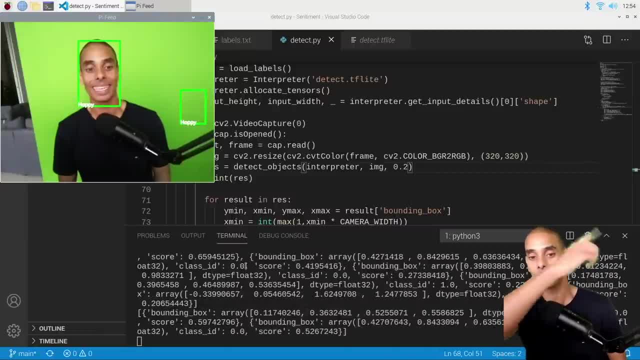 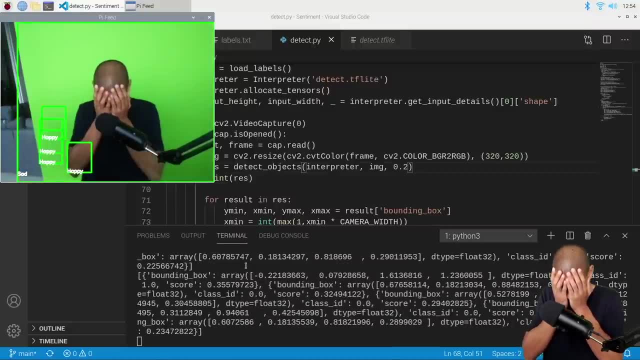 so you could definitely train this for a lot longer. you're getting these false detections over here, which isn't that great. so let's try that again. so let's try that again. so we're getting. it was a detecting sad. let's have a look. so it doesn't look like it's that great at detecting sad. 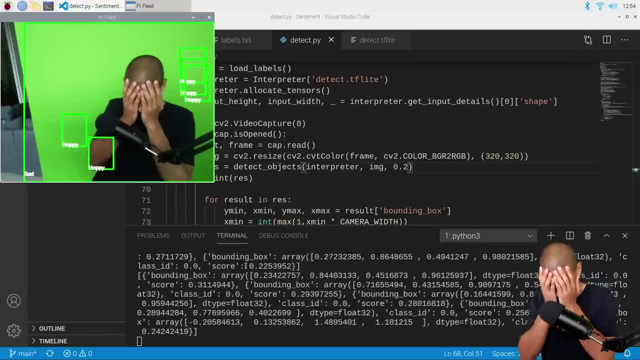 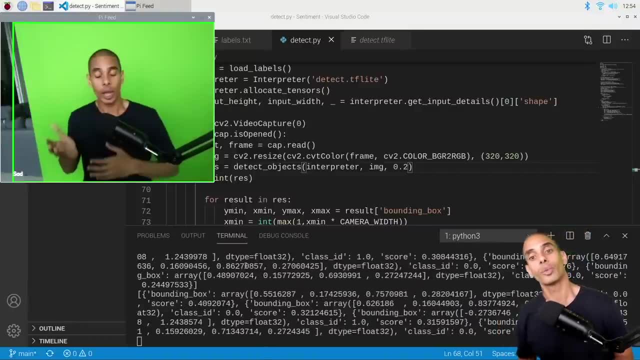 you sort of get the idea. so you can obviously train this for a lot longer performance tested. we only trained it on eight images as well, so obviously this camera on the raspberry pi is going to be different to what we trained on, so you're going to get different. 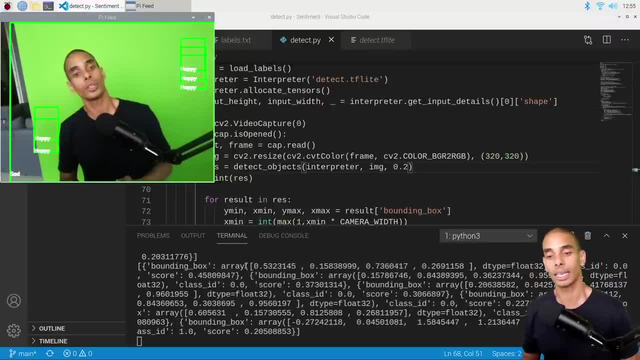 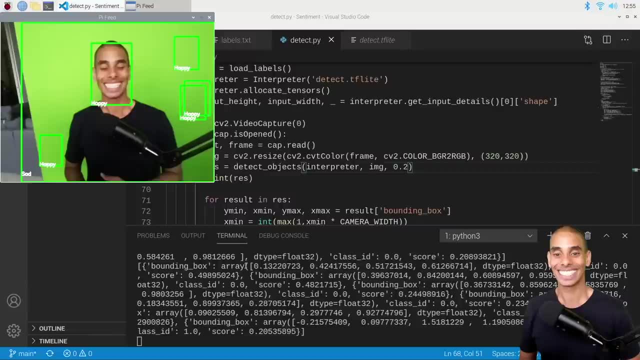 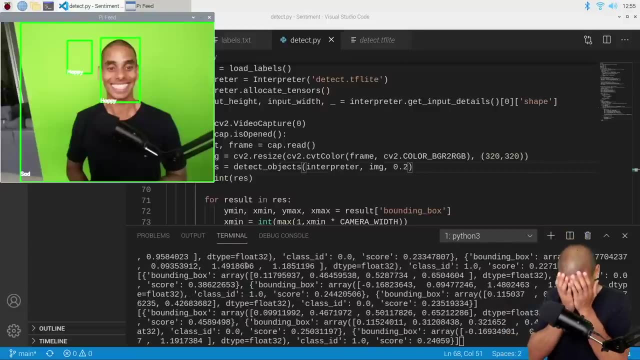 performance when you do crossover. so that's another thing to keep in mind. but if we go happy, you can see that it's definitely picking us up. there is a little bit of lag when going through idp, so if we go to sad, let's see if we can at least get one sad detection. 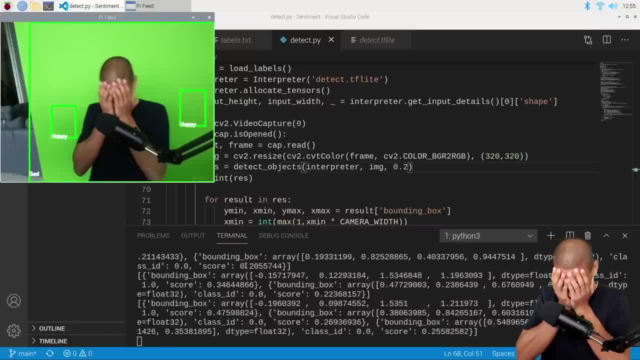 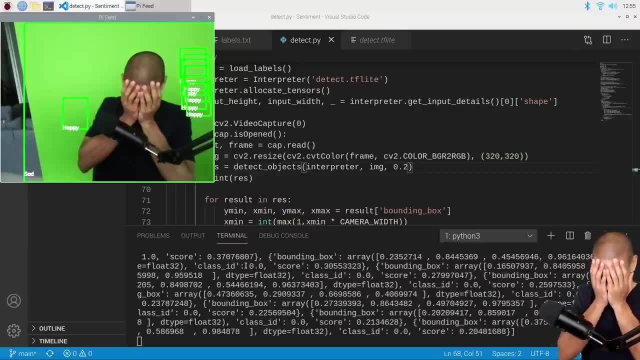 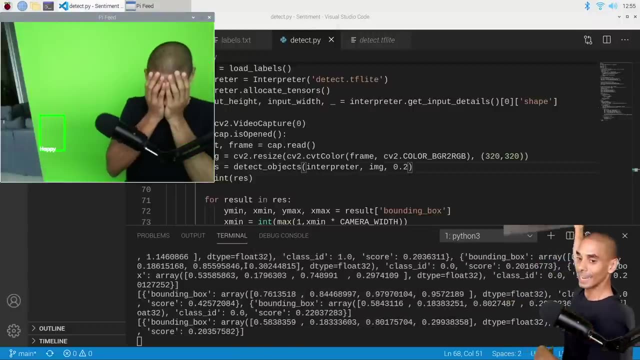 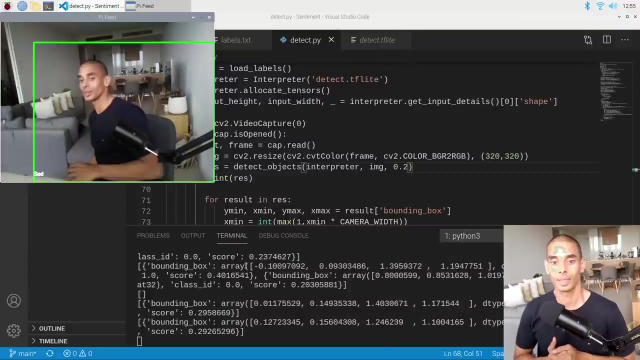 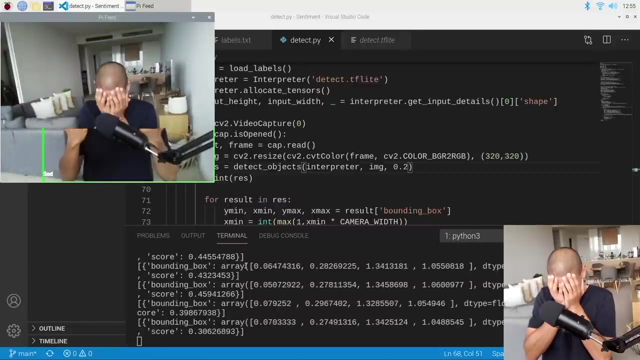 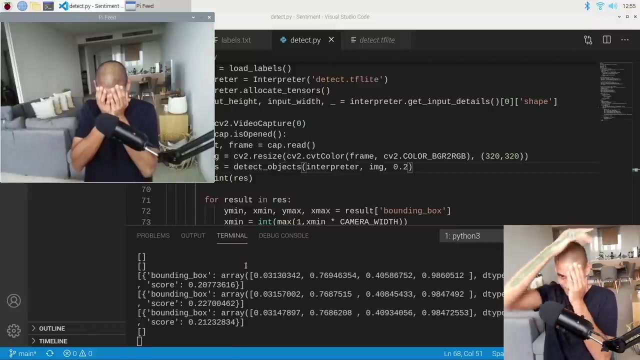 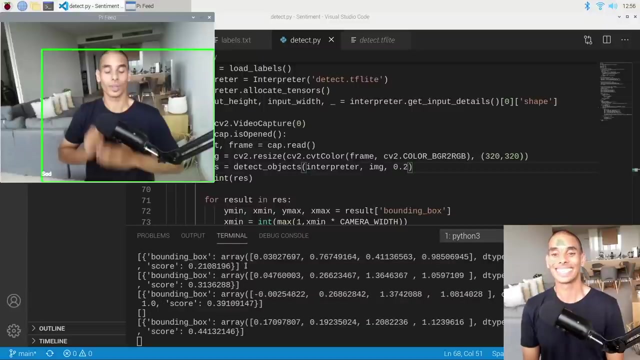 move over a little a little. Lots of happy, weirdly enough, Let's try dropping green screen. It's got one big sad but it's detecting sad, but it's somewhere up here, so it's not the best result. Oh, it's drawing a big box around me as being sad. 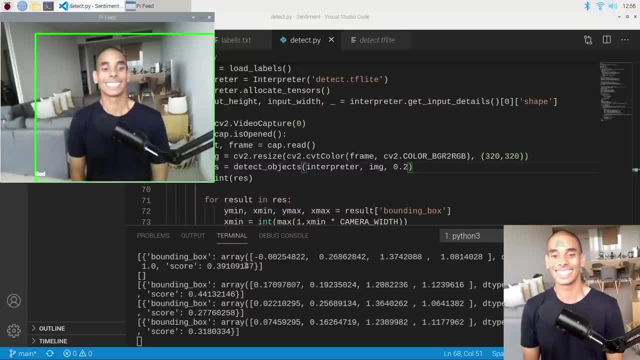 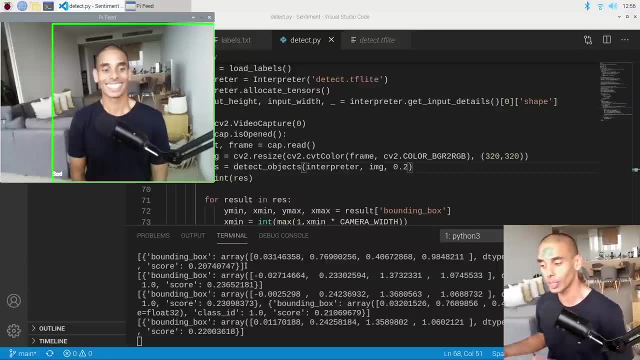 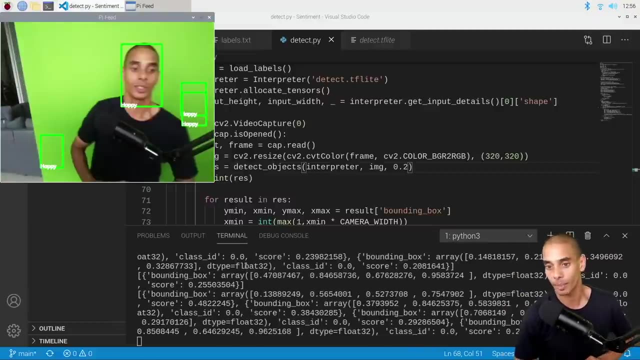 Help me smile Again. so it's not the best generalized model, but it sort of shows you what's possible, right? So that gives you an idea of how you can go about making your detections on Raspberry Pi. So again, looks like it's pretty happy. 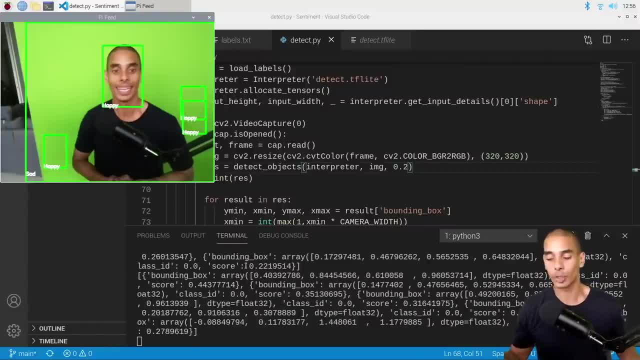 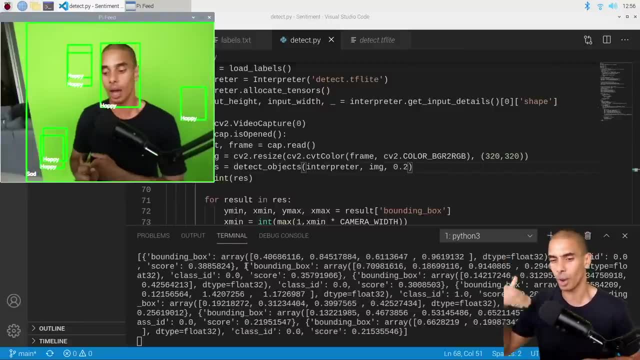 Detecting me is happy, maybe sad, not so much. So if we wanted to performance tune this, we could add in more images Of me being sad in that particular case, under different lighting conditions. I'd probably drop the lighting because the feed from the Raspberry Pi isn't as bright as the webcam. 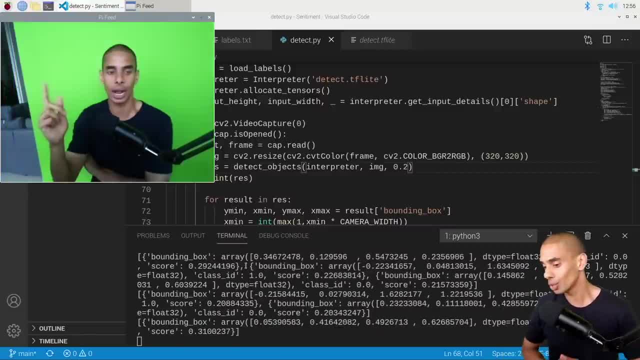 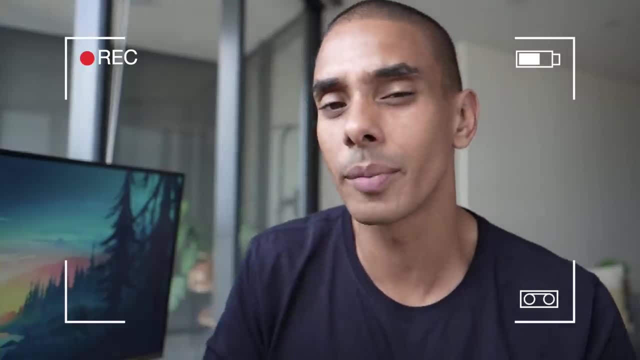 I've got on my computer, But you can sort of see that there are ways to tune this and there's ways to go and deploy your model and a whole bunch of projects that you can sort of take away to go and build yourself. Now, performance for the sentiment model was okay, but during editing I couldn't help. 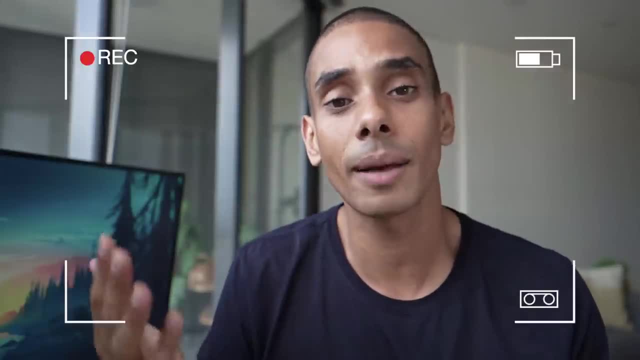 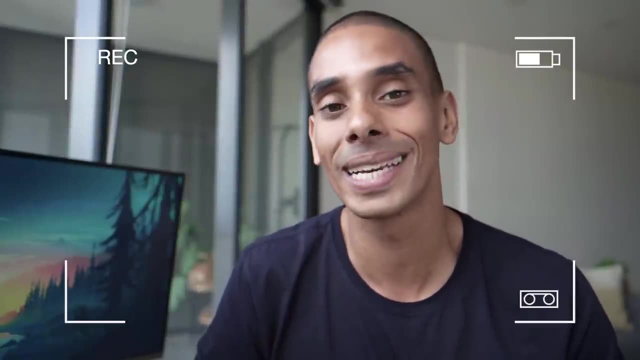 thinking that this could be so much better. So what I ended up doing is performing some additional performance tuning to To ideally eke out a little bit of additional performance out of this model. My OCD was in overdrive, so I decided to let it run free and try to get this performing. 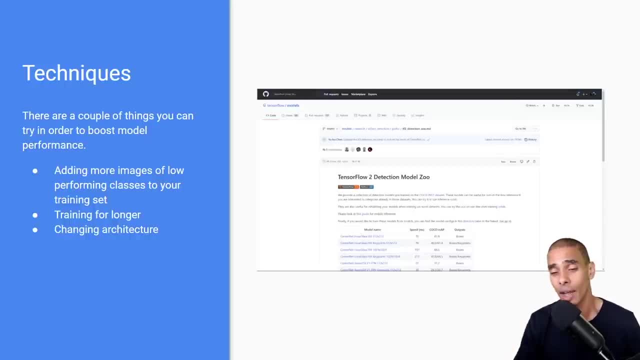 a little bit better. This is what happened. So during editing, I couldn't help thinking that I really wanted to get better performance out of that sentiment model. So again, as we went through in step six or part six of this course, I went through our 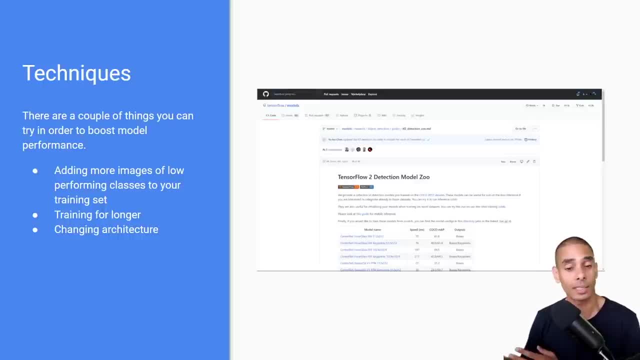 performance tuning step, So I added more images of the performing classes that weren't performing so well. In this case, I added more of both our sad sentiment and our happy sentiment, And I ended up training our model for longer. I didn't really need to change the architecture, but if I hadn't had a performance boost, that 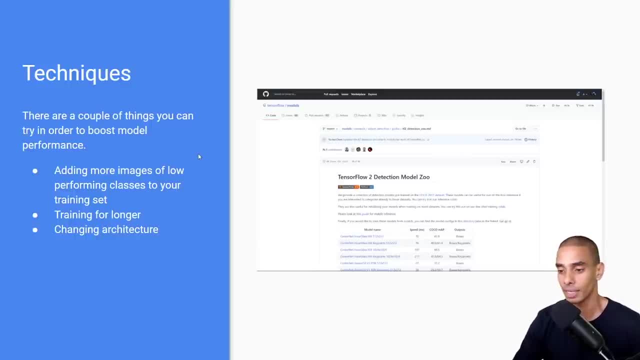 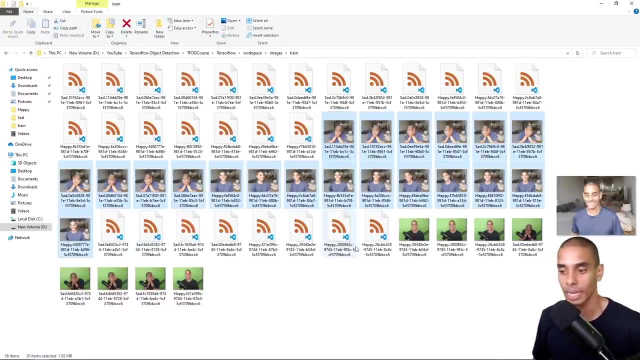 would have been my next step. So let's take a look at what it is that I actually did. So first up, I added a number of additional images. So all up you can see that I added about 20 additional images And if we actually open these up, you can see I've got images at a number of different 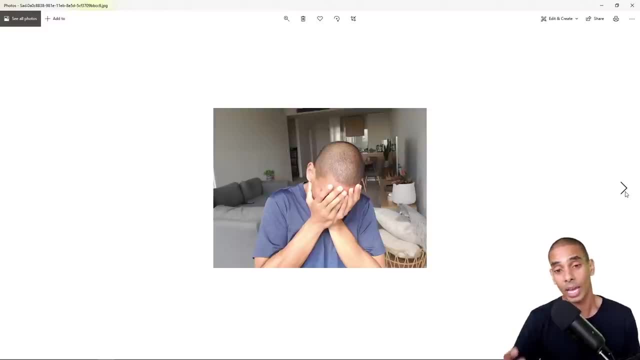 angles. So this gives or this boosts our chances of having a model that generalizes well, And I also took down the green screen, So ideally see if that had any impact on whether or not our performance was going to boost or not boost. 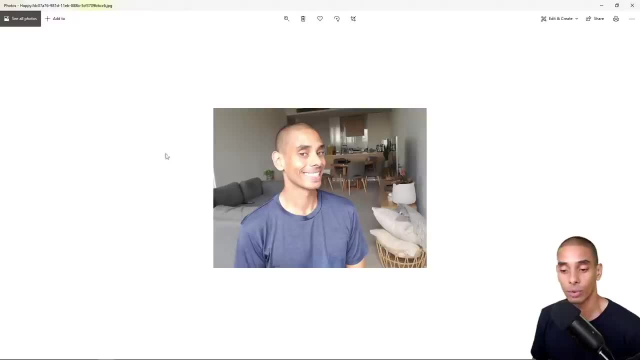 So if we keep taking a look, you can see I've got images at a whole bunch of different angles And I also had some images of me looking happy as well, And you can see I'm moving my head around, And this gives our model a better chance of actually being able to detect our head with 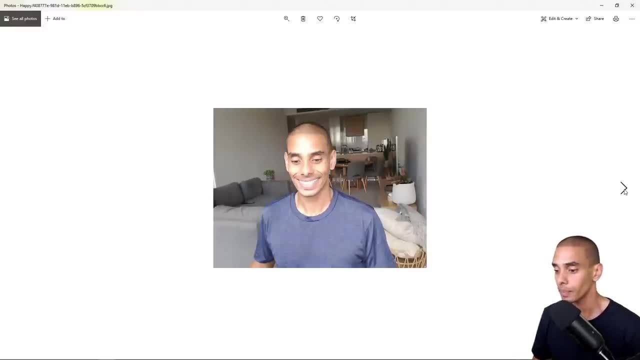 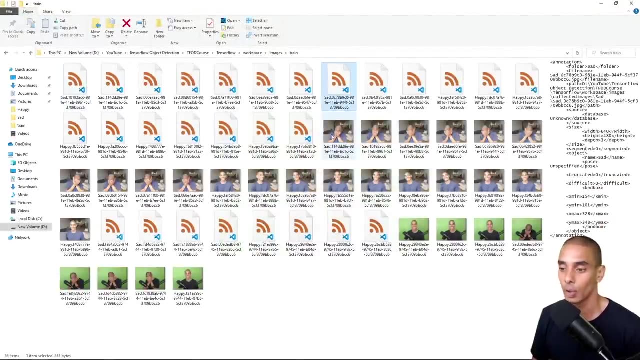 the green screen up, but also with the green screen down, So you can see a bunch of different angles. And again I went about the same labeling step. So all I did was I created. I created new images, went and labeled them again. 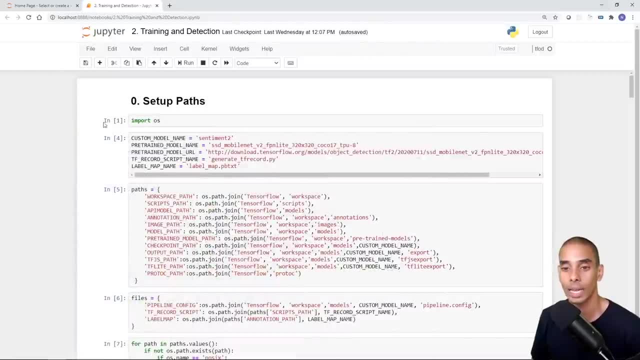 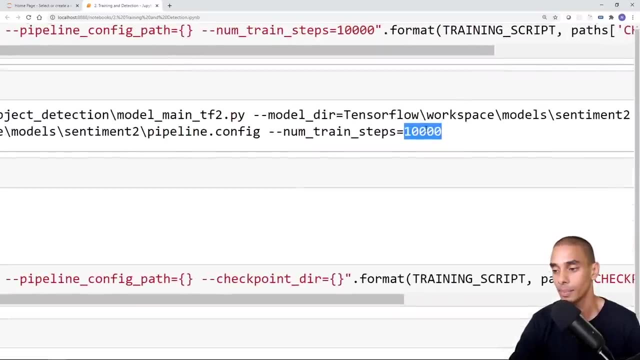 That was the first thing that I did. The second thing that I did is I went and trained our model for longer. So if I actually show you I ended up training, I kicked off the training for 10,000 steps, So you can see 10,000 there. 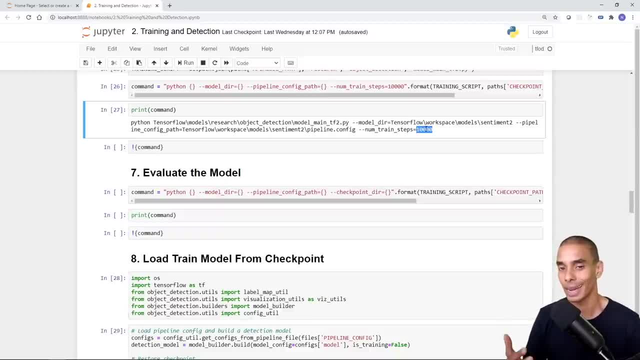 But I actually stopped this at about 5600 steps. I was kind of getting impatient and wanted to just test it out, So I trained for an additional 5600 steps. Now what that gave me is a brand new model, So I didn't retrain the existing model. 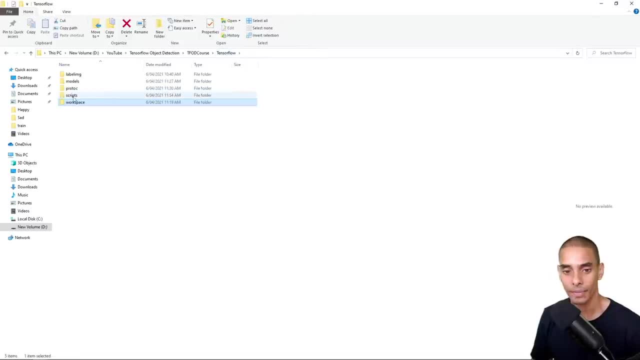 I actually went and trained it. I went and performance tuned and created a new model. So if you actually take a look, exactly is what we did during the performance tuning step. So I went into workspace models. You can see here that I've got a model called sentiment two and my checkpoint went all the 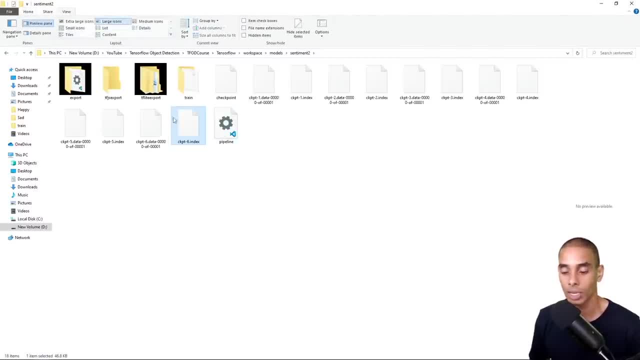 way up to checkpoint six. So you can see that there, because I trained for longer, I had a checkpoint with a greater index. Again, I went through the same steps. I went and converted it to a frozen TF light graph. I then went and converted it to a TF light model. 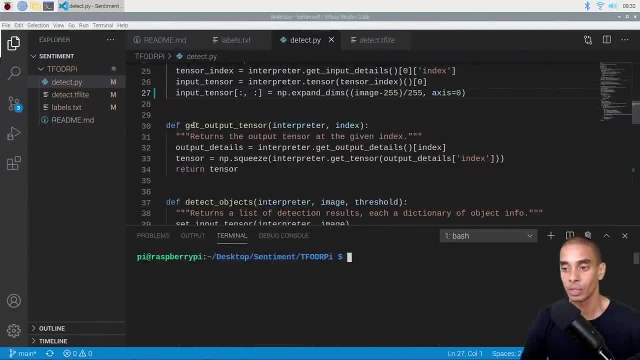 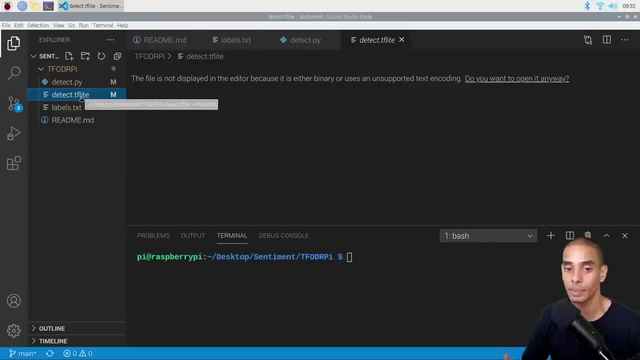 Okay, I brought this into my raspberry pipe. So now this particular detecttf light model that we had here is the model that's been trained for 5600 steps and it's been trained on 20 additional images. Those were the core changes that I made here. 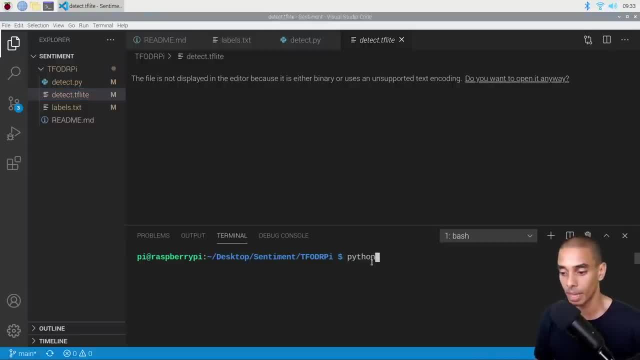 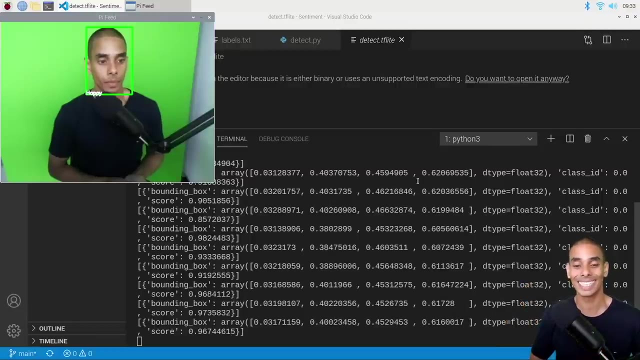 Now if we try running this model again, let's take a look at performance. So if I type in Python three- let's bring that up a little bit- Detectpy, You can see that we're detecting happy. We're not getting all of those false detections. 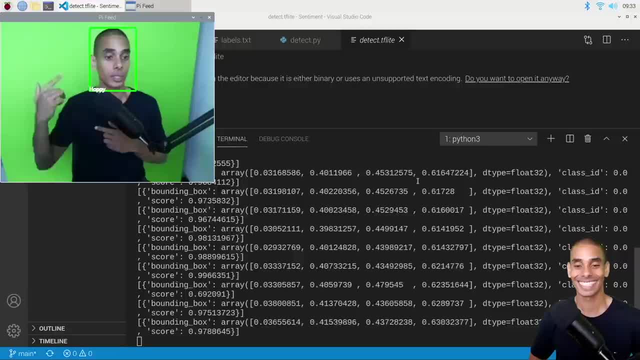 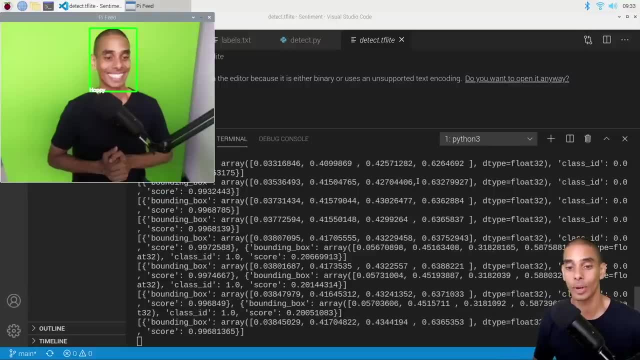 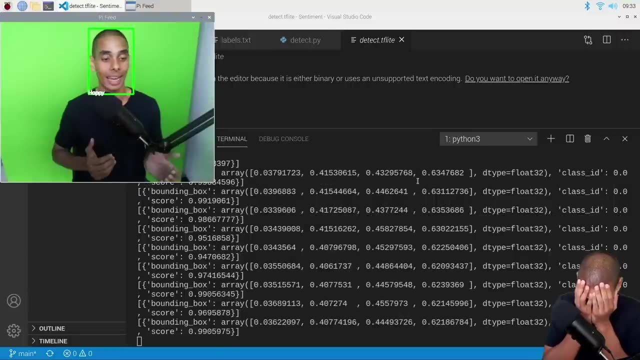 So if I smile, we're good. Now let's test out sad, because remember, sad wasn't working right. So that was the key thing that we wanted to test out. So if I put my hands over my face now, you can see that we are detecting the fact that 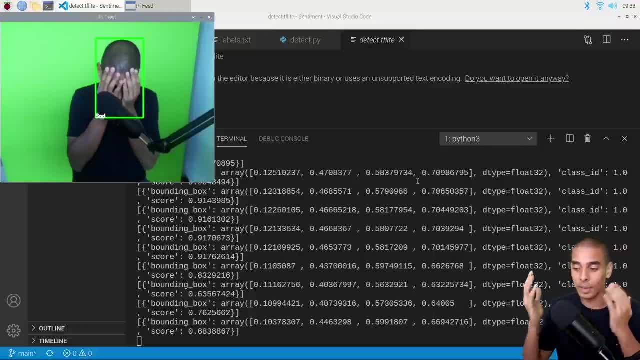 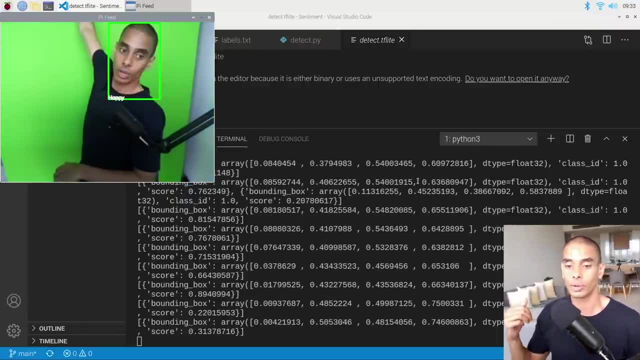 I'm sad. So again, it's a much better performing model. Okay, So if we take the green screen down, let's take a look at performance there as well. So right now it's performing well with the green screen up, But what about if we took the green screen down? 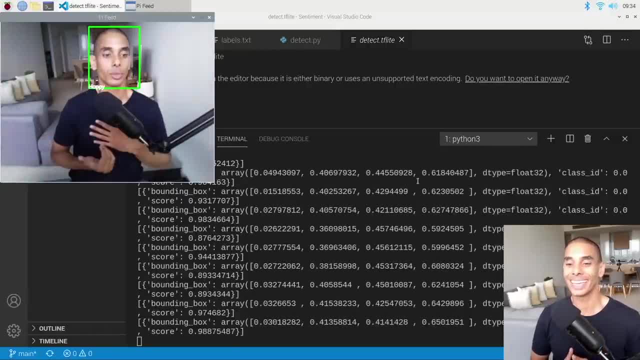 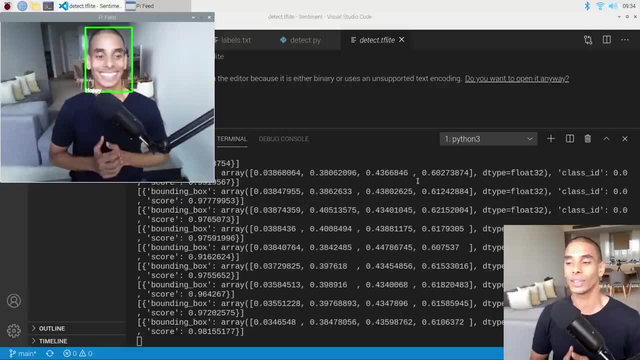 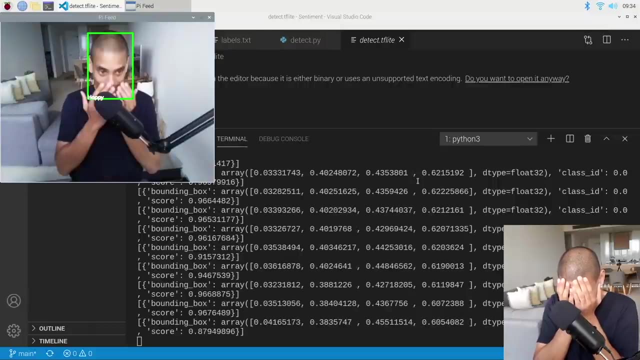 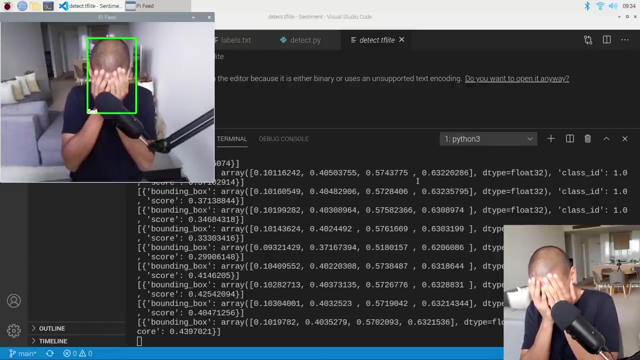 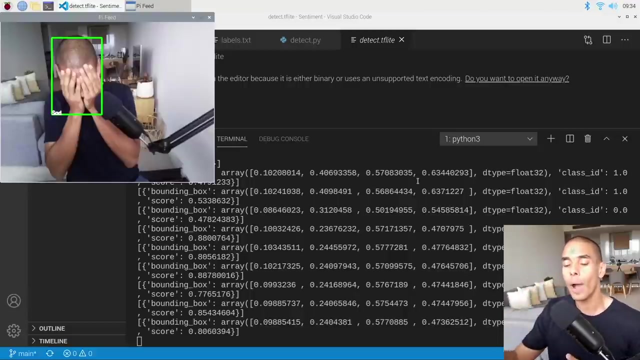 So again still detecting that we're happy And, if we try out, sad again. so if I put my hands over my face, You can see that we're getting significantly better performance now- So you can see the little label in the bottom corner- but again performing way better. 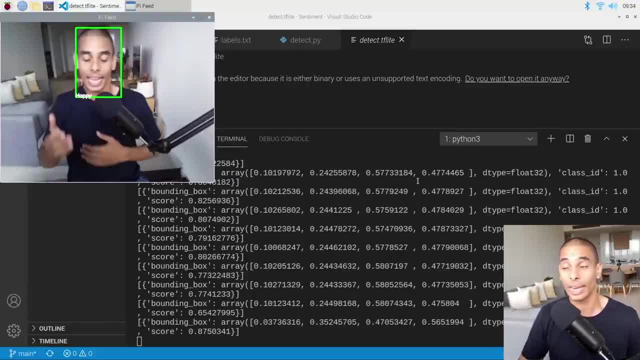 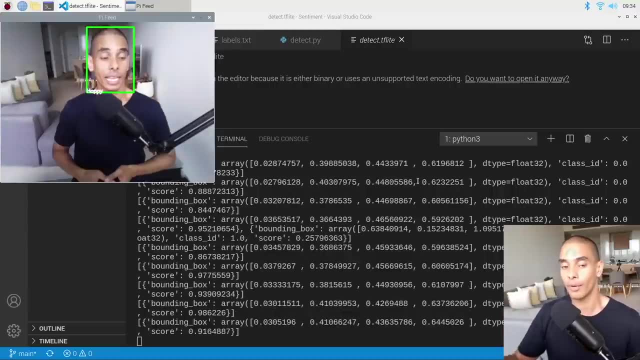 And all I really did was I added those additional images and I trained for 5600 steps. So you can see the power of performance tuning. And again, just because you get not the best performance first time around doesn't mean that you can't go and improve performance after that to be able to generate better results. 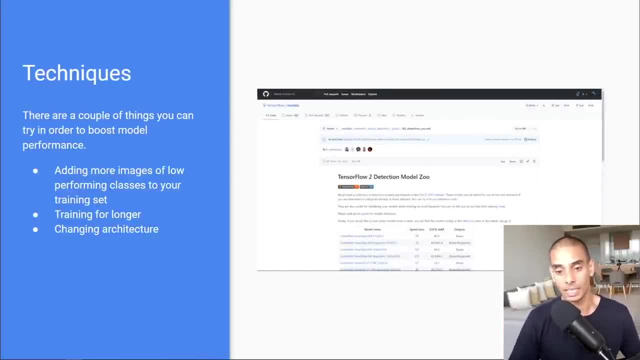 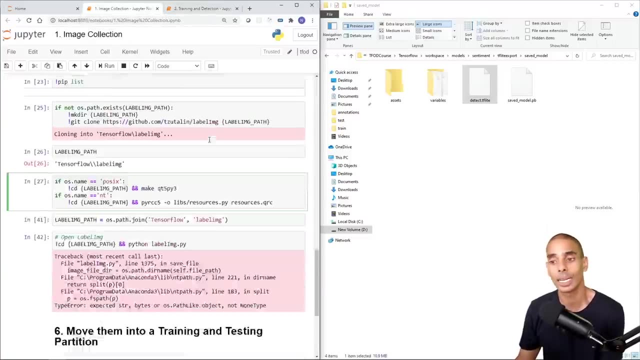 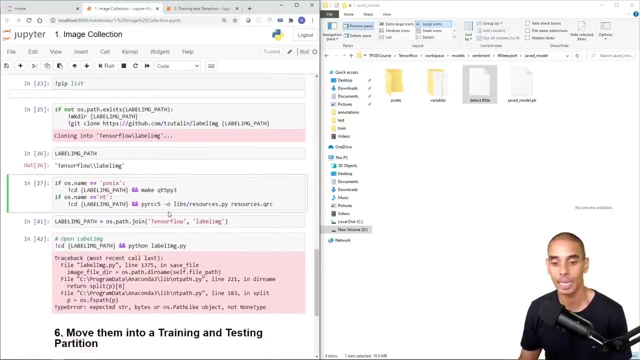 Okay, Okay. So that's the power of performance tuning, in this particular case, Editing Nick out. Now, on that note, let's do a quick recap. So the last and final project that we did was sentiment analysis. So we went and collected our images using our standard image collection capability. 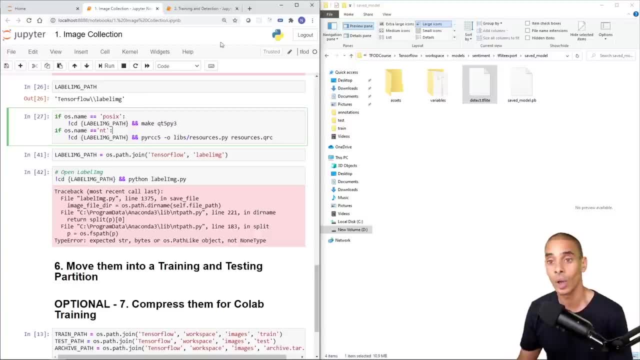 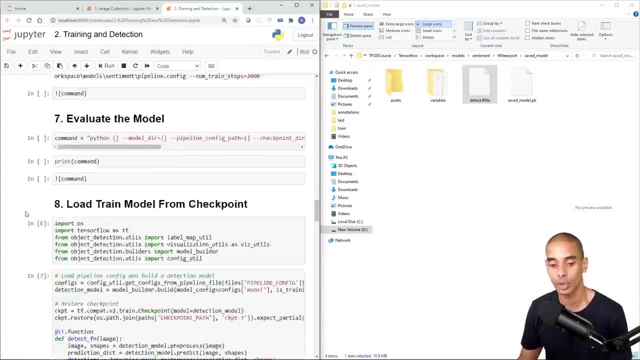 We went and labeled our happy and sad detections. We then also went and created our updated label map and trained our model. But the core difference between this and the previous two projects is we obviously went and converted it to tier Flight so that we had that capability there.